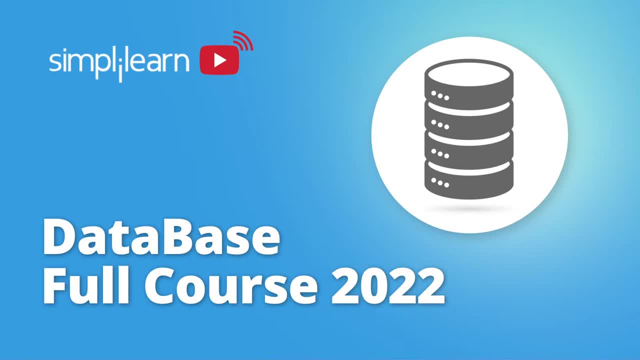 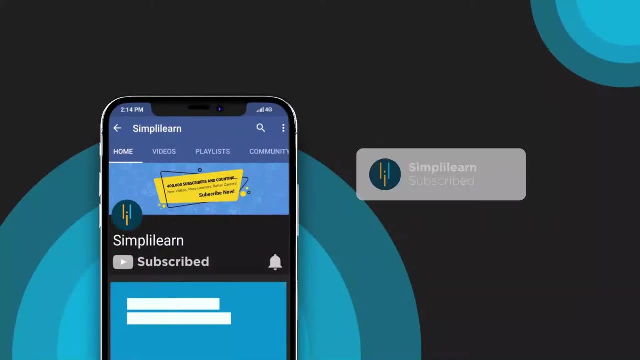 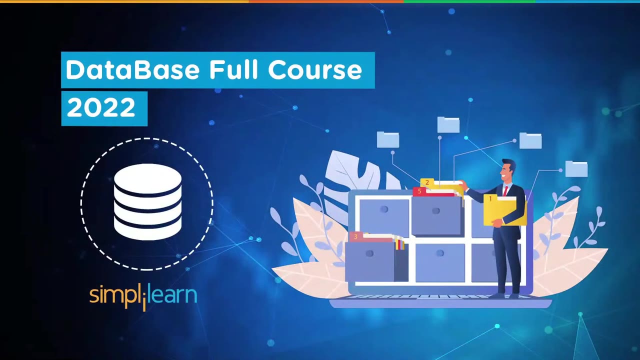 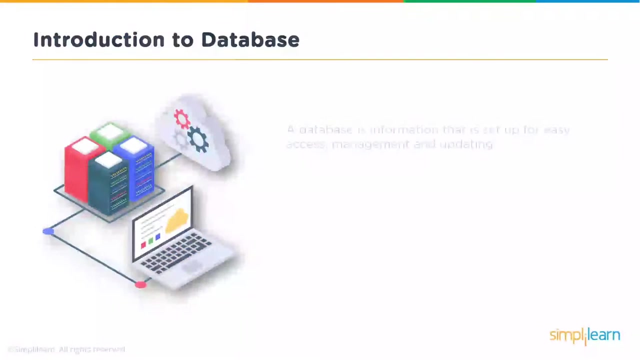 Hey guys, welcome back to another video by Simply Learn. In today's video we're going to be learning all about the two most commonly used databases, that is, MongoDB and SQL. But before we begin, let's look at a quick introduction to database. Now, a database is information. 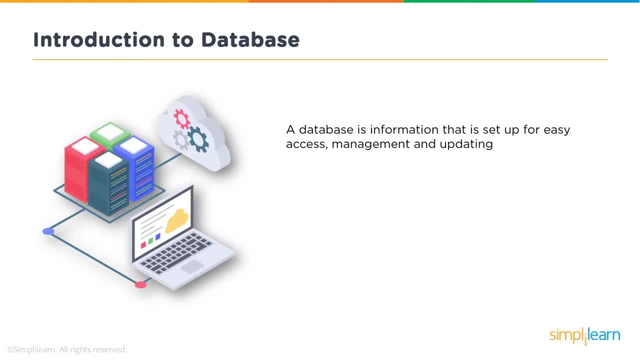 that is set up for easy access, management and updation. Computer databases typically store aggregations of data records or files that contain information such as sales transactions, customer data, finances and product information. Databases are used for storing, maintaining and accessing any sort of data. They collect information on people, places or 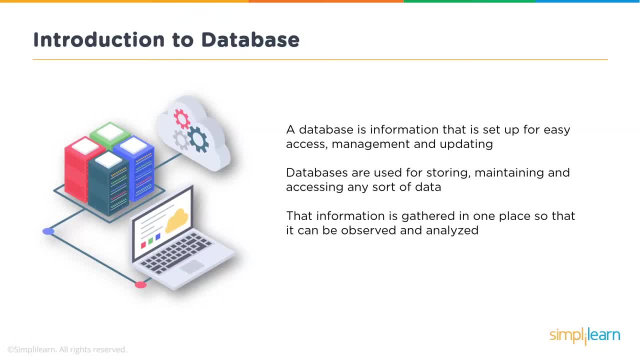 things: That information is gathered in one place so that it can be observed and analyzed. Now, in short, databases can be thought of as an organized collection of information. Some of the main features of using database includes improving business processes, keeping track of customers, secure personal health information and storage of personal data. 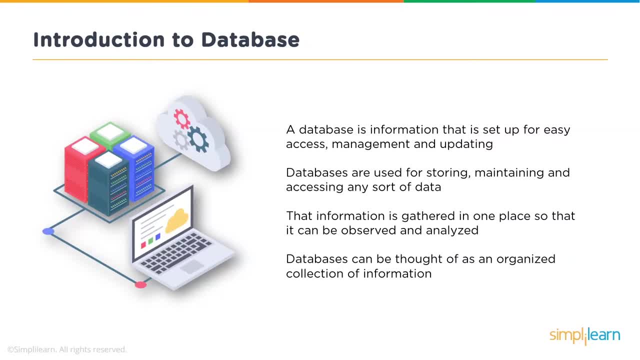 Now there are several different types of databases available. There's relational databases, no SQL databases, object-oriented databases, distributed databases and so on. In this video, we will learn about two commonly used databases, that is, SQL, which is a relational database, and MongoDB, which is a no SQL database. But before we begin, if you haven't subscribed, 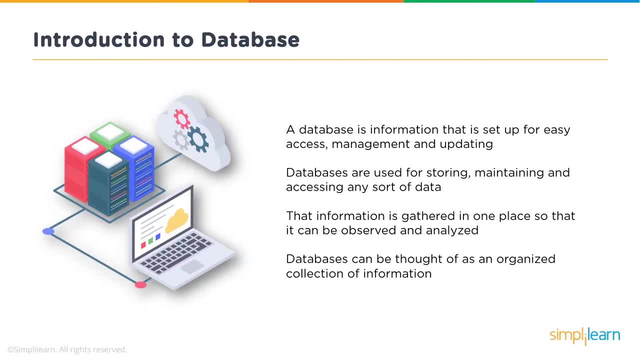 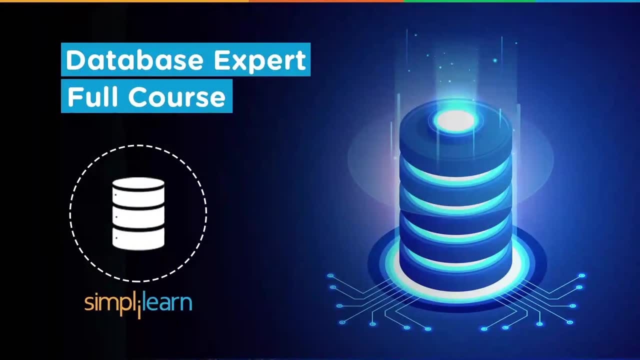 to our channel already. make sure to hit the subscribe button and the bell icon to never miss an update. Now, without further ado, let's begin. First, let's look at what's in store for you with respect to SQL. First, let's look at what's in store for you with respect to SQL. 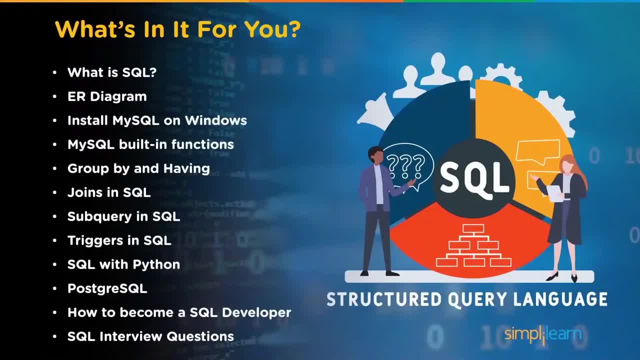 This session will help you write SQL commands using MySQL, PostgreSQL as well as SQL Server. Our highly experienced trainers will take you through this course, So here's what's in store for you. First, we'll start by learning the basics of SQL, along with understanding entity relationship. 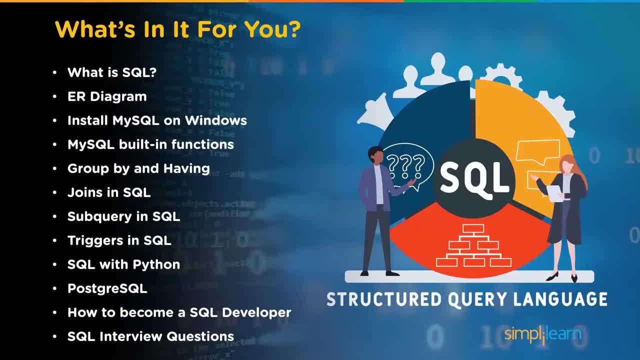 diagrams. Then you will learn how to install MySQL Workbench on Windows. We'll then look at the popular SQL commands to select, insert, update, delete records and perform other tasks. First let's talk about the basic code setup you need to use to run SQL. 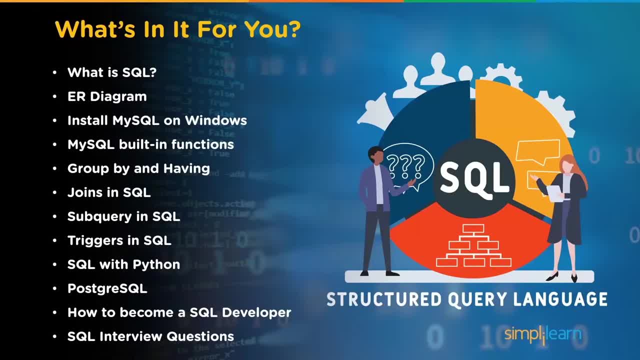 First we'll look at the basic code setup you need to use to run SQL. Then we'll look at the basic code setup you need to use to run SQL. So by using the list of more than 16 hasn in the list, you'll understand what's in. 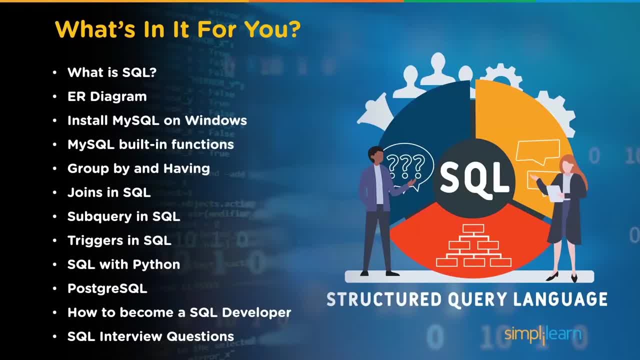 store for you. You'll then see how to apply these and some of the other operations on database tables. You will also see how to use the top numerical and text functions in SQL. Next, we'll cover how to use group by and having clauses in SQL followed by joins. You'll learn the different types of join statements, as well as sub queries in SQL And, moving further, we'll understand triggers, stored procedures and window functions in MySQL. You will get an idea about another important topic that we will attend on, so until that, we'll leave you withигnt for now. 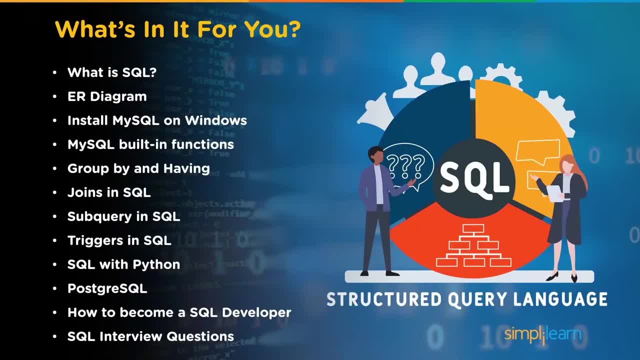 topic, that is, to write SQL queries with Python on the Jupyter Notebook. Then we'll look at another free and open-source relational database management system. that is post hands-on demonstration. Finally, you'll learn how to become an SQL developer and see the top SQL interview questions. 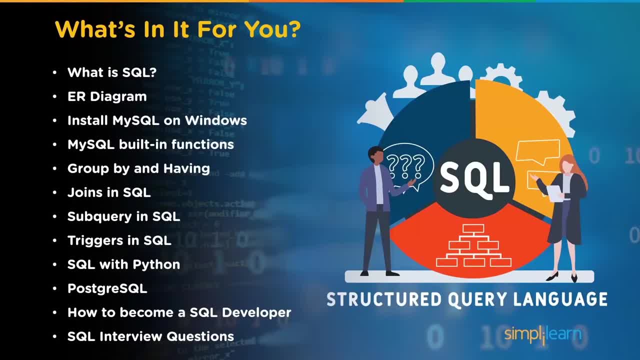 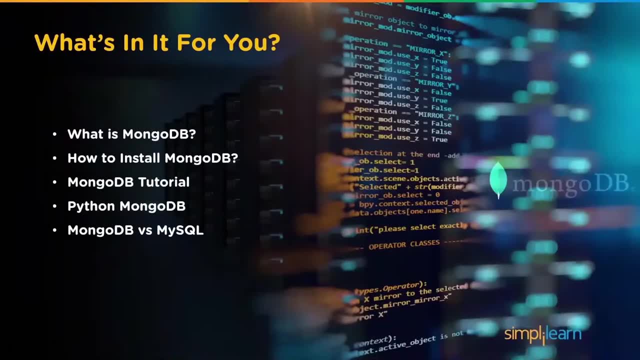 that are frequently asked in the interviews. So these are the topics covered in SQL. Moving ahead with respect to MongoDB, first you'll learn what exactly MongoDB is. Then you'll look at a simple demonstration to install MongoDB on your Windows system. Then we'll look at a detailed MongoDB tutorial that explains how to insert, create, update. 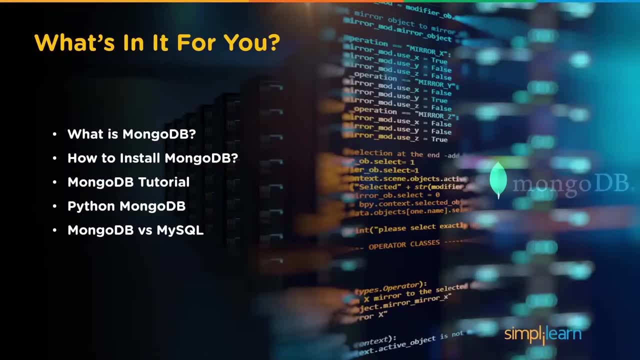 and delete data. Then we'll look at how to connect MongoDB with different applications, and in this case we'll be connecting MongoDB to Python. And lastly, we'll draw a comparison between MongoDB systems. But before we begin, if you haven't subscribed to our channel already, make sure to hit the. 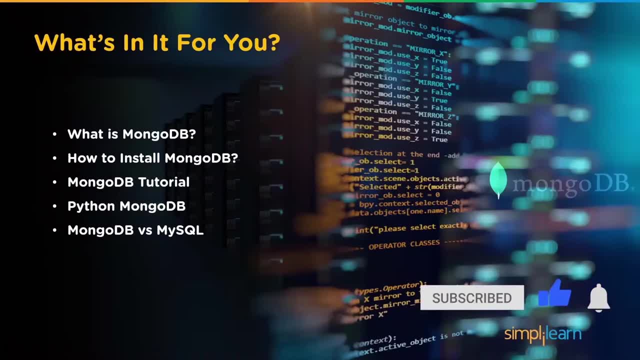 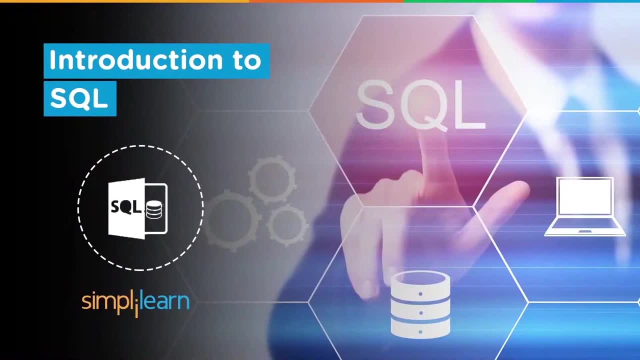 subscribe button and the bell icon to never miss an update. So now let's dive right in. In this session, we are going to learn about databases, how data is stored in relational databases, and we'll also look at some of the popular databases. 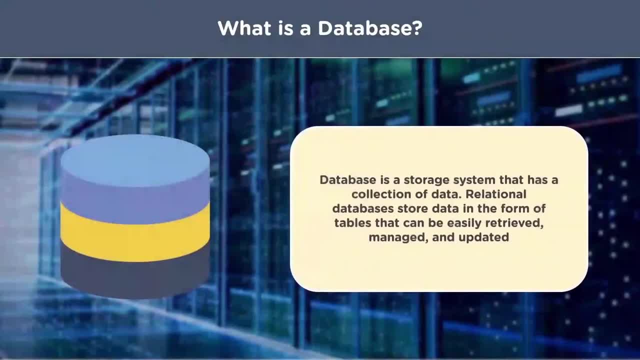 Finally, we'll understand some of the most popular databases. So, according to Oracle, a database is an organization typically stored electronically in a computer system. A database is usually controlled by a database management system or DBMS, So it is a storage system that has a collection of data. 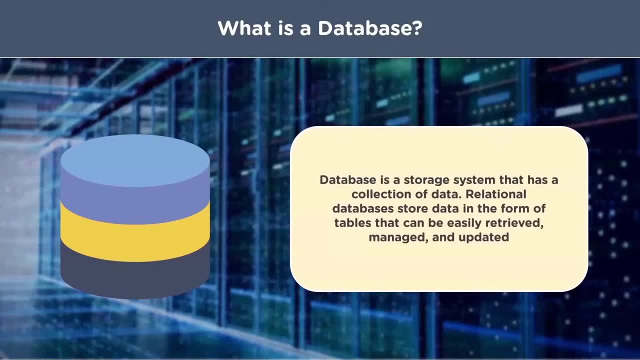 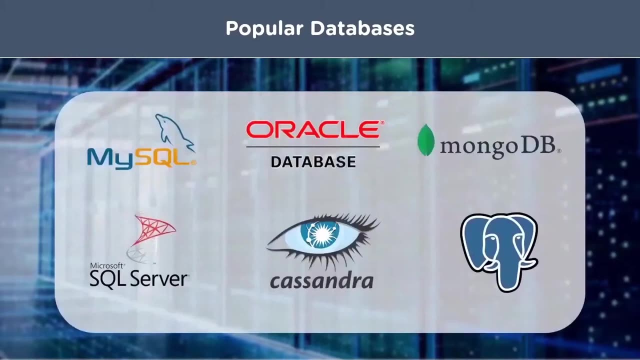 Local databases store data in the form of tables that can be easily retrieved, managed and updated. You can organize data into tables, rows, columns and index it to make it easier to find relevant information. Now talking about some of the popular databases. We have MySQL database. 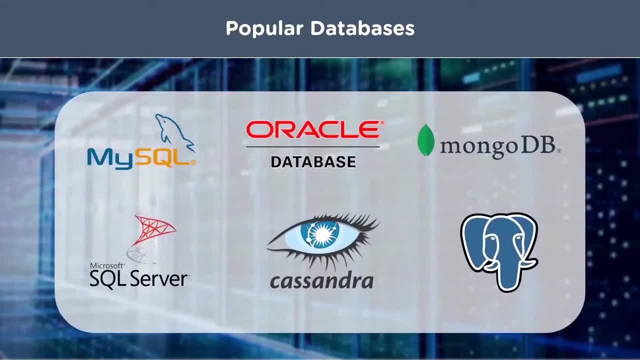 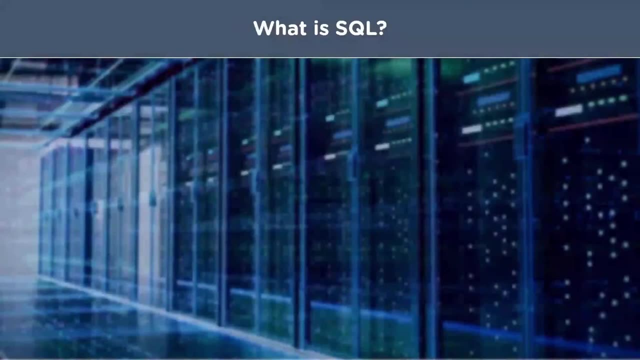 We also have Oracle database. Then we have MongoDB, which is a NoSQL database. Next we have Microsoft SQL Server. Next we have Apache. Cassandra is a free and open source NoSQL database and finally we have PostgreSQL. now let's learn what is SQL. so SQL is a domain, specific language to communicate with. 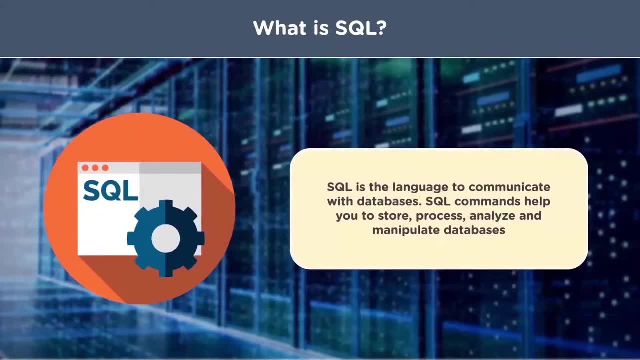 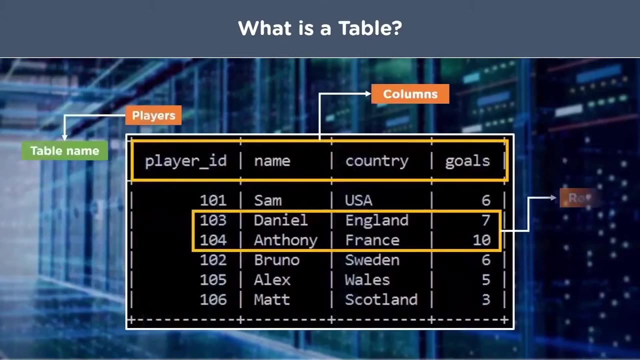 databases. SQL was initially developed by IBM. most databases use structured query language or SQL for writing and querying data. SQL commands help you to store, process, analyze and manipulate databases. with this, let's look at what a table is. table in a database looks like, so here you can see the name of the table is. 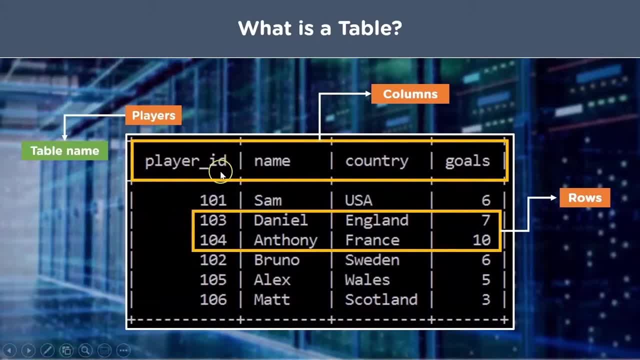 players. on the top you can see the column names. so we have the player ID, the PTO, and we also have the goals scored by each of the players. so these are also known as fields in a database. here each row represents a record or a tuple. so you have the player ID, which is 103 here. the name of the player is it. 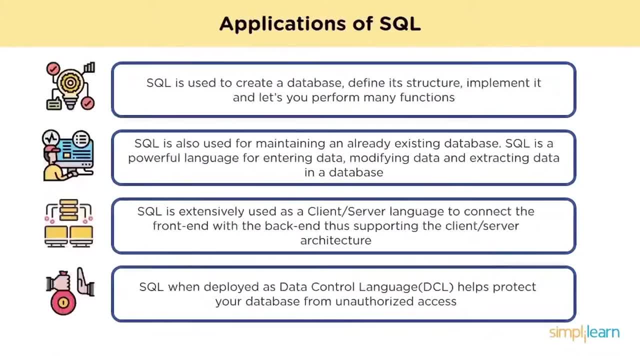 doesn't require much coding to manage databases. now we will see applications of SQL. SQL is used to create a database, define its structure, implement it and let's you perform many functions. SQL is also used for maintaining an already existing database. SQL is a powerful language for entering data, modifying data and extracting data. 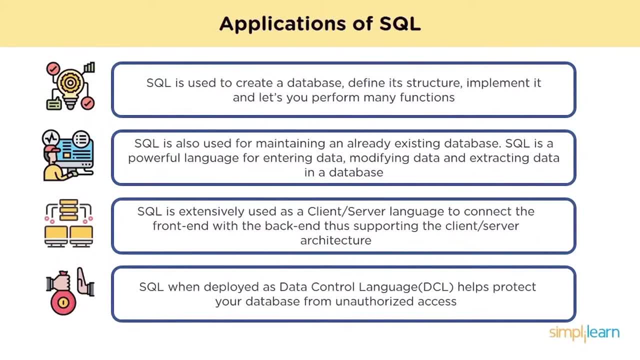 in a database. SQL is extensively used as a client server language to connect the front-end with the backend, thus supporting the client-server architecture. SQL, when deployed as data control language, DCL, helps protect your database from unauthorized access. In this session, we will learn who is a SQL developer and what are the responsibilities in a 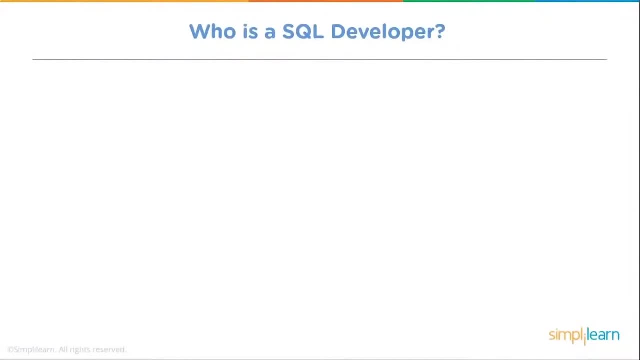 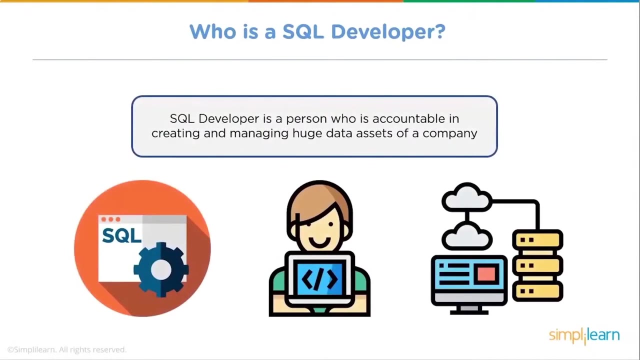 company. First, we will understand who is a SQL developer. SQL developer is a person who is accountable in creating and managing huge data assets of a company. In other terms, SQL developer is a person who can develop SQL databases as well as write and test code. Let's understand this with the help of an 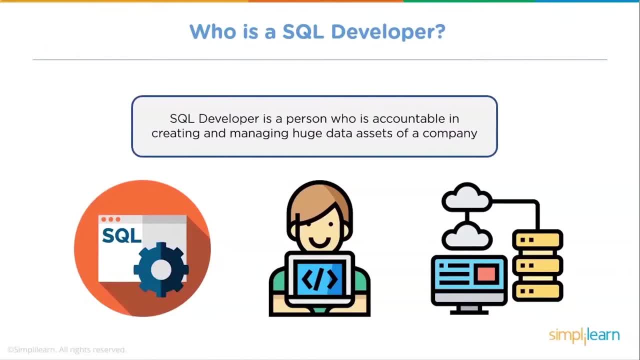 example, Let's say we want to search a particular product on Amazon website and Amazon has stored all its data about products in a database. Now we will write the product name in the search bar and when we click on the search button it will run a SQL query that fetches all the information about the 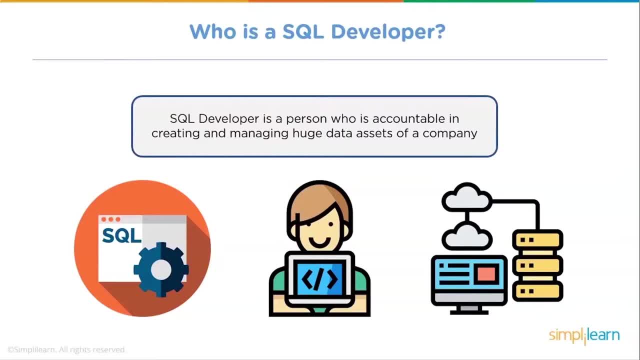 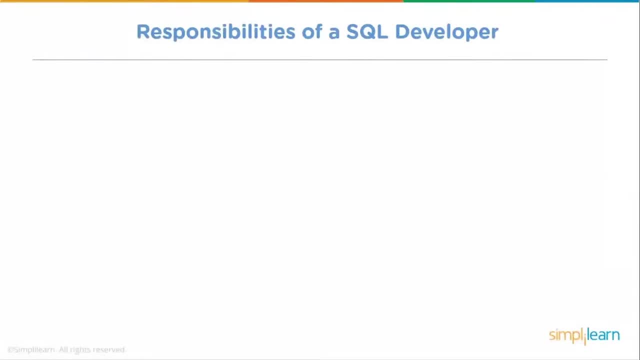 product and is stored in the database. Let's start the SQL query and we will product and displays us on the website. So this is the basic task done by a SQL developer. Now we will understand the responsibilities of a SQL developer. All databases have a structure and logic behind how data is stored and retrieved. 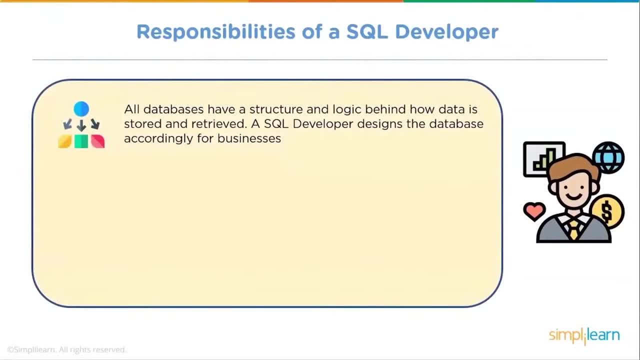 A SQL developer designs the database accordingly. for businesses that is called database modeling. After the database is created and deployed, it's the SQL developer who is responsible for fixing the general issues of the database. SQL developer should be well-versed with structured query language to create optimized SQL queries. 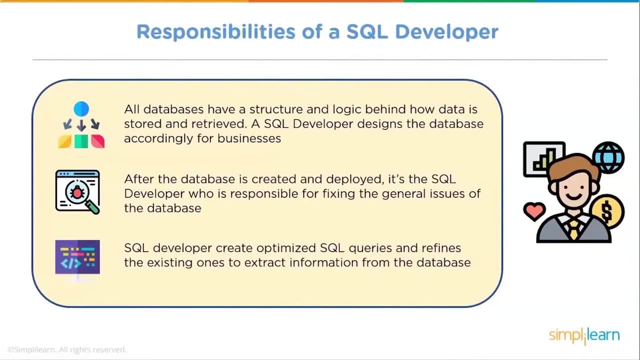 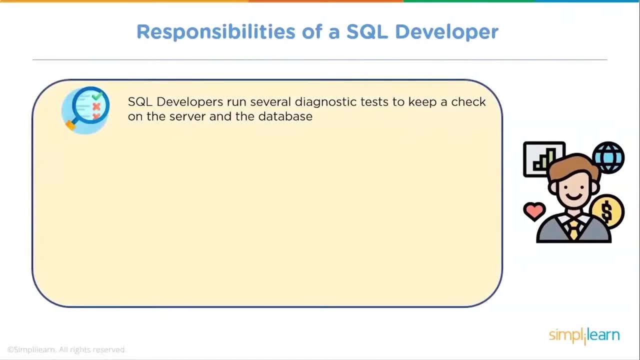 and refines the existing ones to extract information from the database. SQL developers run several diagnostic tests to keep a check on the server and the database. In order to understand how to organize company's data, SQL developers must communicate with tactical and non-technical persons from the back. 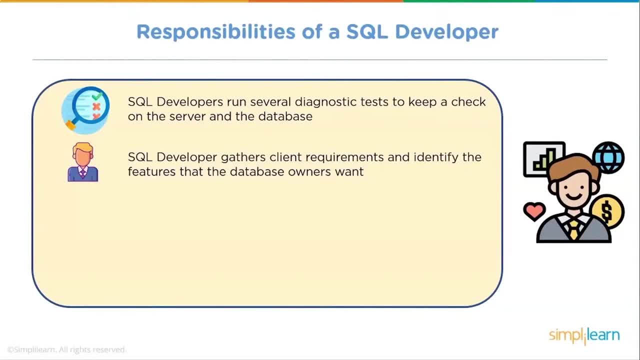 SQL developers also gather client requirements and identify the features that the database owners want, As data is an asset to a company. SQL developers backup and restore data for their clients. They also perform tasks like data management and data migration. That is, if a company has stored all its data on a local storage and now it wants its data. 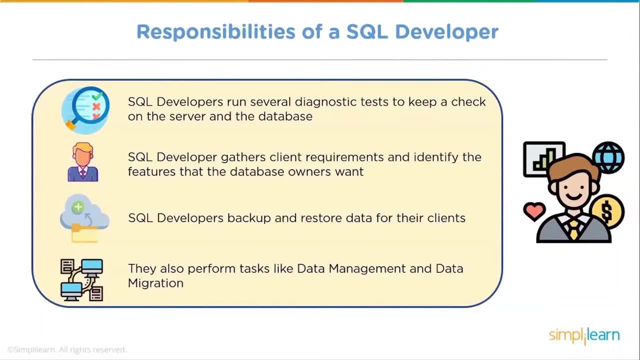 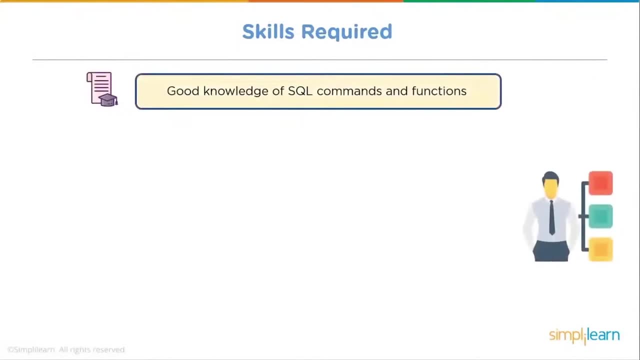 to be stored in a cloud storage, so the safe transmission of the data from local storage to cloud storage is important. After knowing the responsibilities, now we should look for skill set required to be a good SQL developer. One should have a good knowledge of SQL commands, functions, joins and procedures. 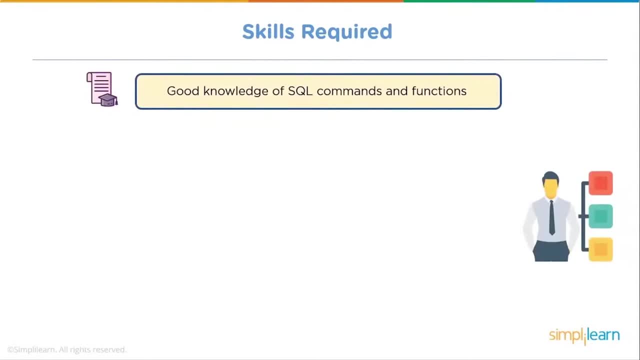 Let's have a look at few commands such as create, drop, alter and truncate. These commands come under data definition language. We also have insert, update and delete commands. These commands come under data manipulation language. We have grant and revoke commands. 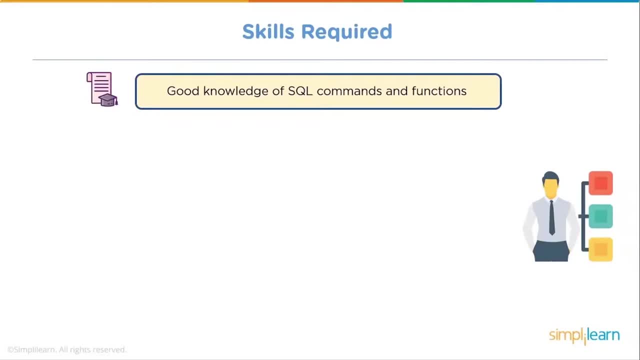 These commands come under data control language. We also have commit, rollback and save point commands. These come under transaction control language. These are the basic commands a SQL developer should be familiar with, And a SQL developer may have a little command on any one programming language. 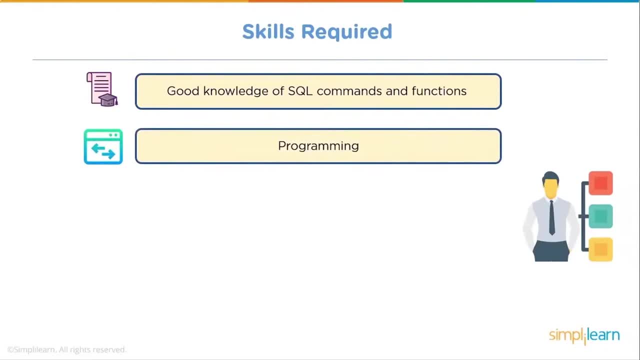 You don't have to be expert in programming. All you need is how to interface between application and your database. For example, You are using MySQL And your web application is based on PHP, Then you should know how to connect your application to the database and how to issue queries. 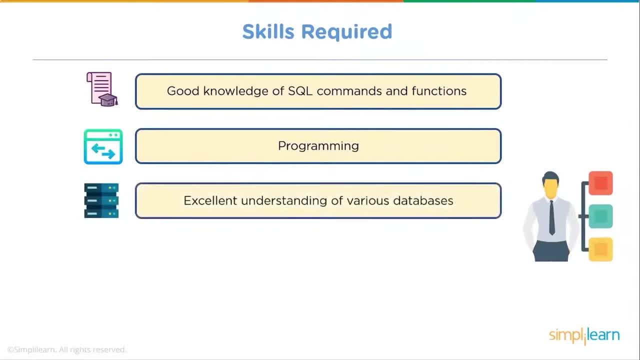 How to fetch results and then how to display it to the users. One should have a good understanding of various database management systems, Such as MySQL, Microsoft Access, Oracle, PostgreSQL Dbase, FoxPro, SQLite, IBM DB2, LibreOfficeBase. 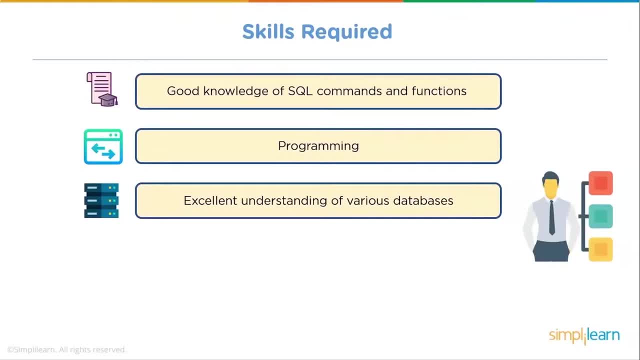 etc. One should know integration of databases with data visualization software such as PowerBI and Tableau, which helps businesses to make better decisions and give you an add-on as a SQL developer. One should develop critical thinking and problem-solving skills to create optimized queries. 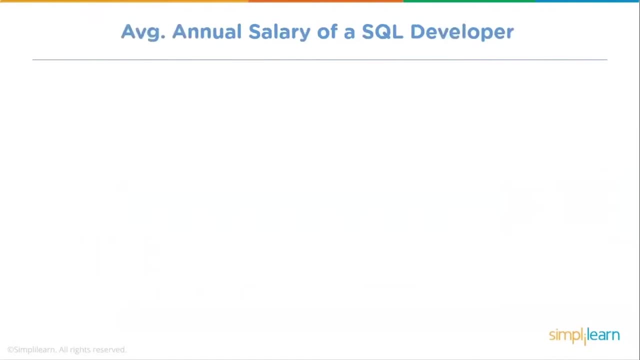 Now we will see how a SQL developer is compensated in both United States and India. In the United States, there is a single SQL developer. In the United States, there is a single SQL developer. In the United States, there is a single SQL developer. 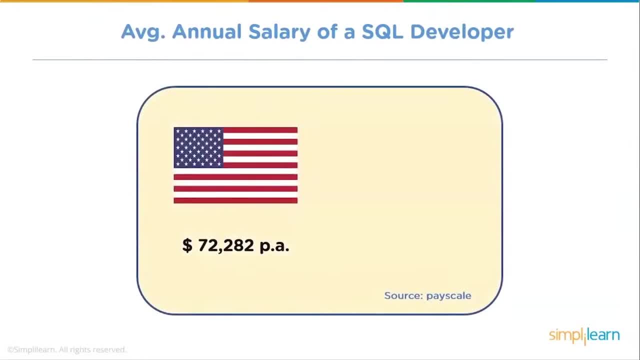 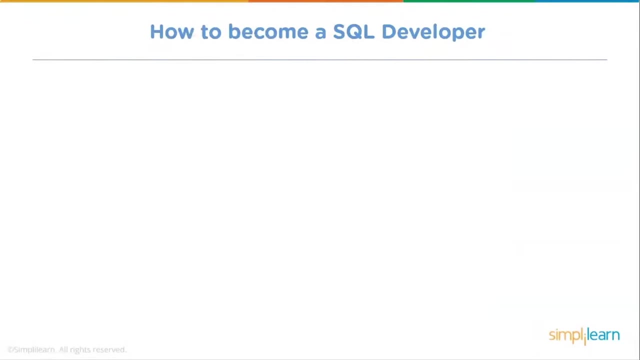 In the United States, SQL developers draw an average salary of $72,282 per annum. In India, the average salary of a SQL developer is Rs 4,49,532.. Now we will see how a person can become a good SQL developer. 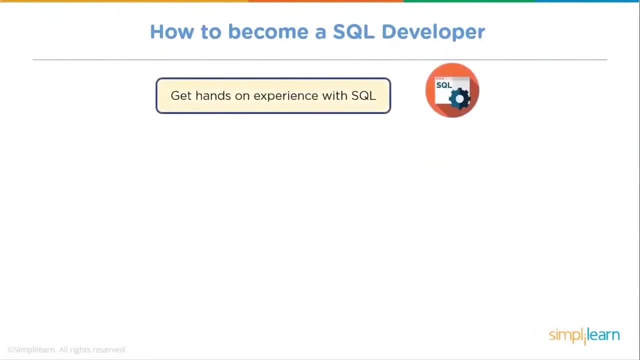 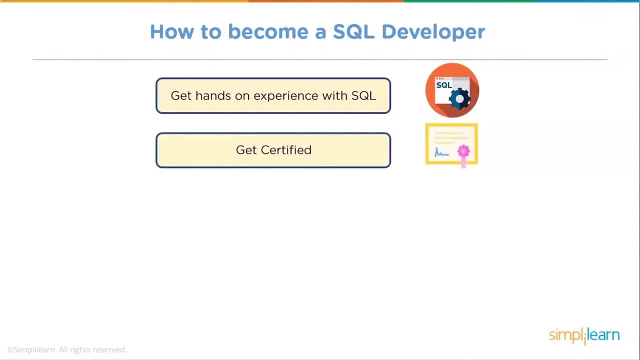 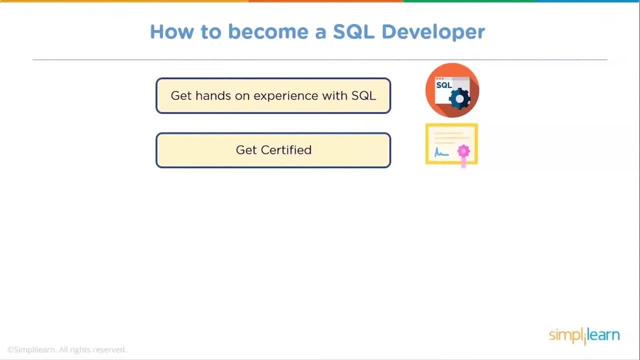 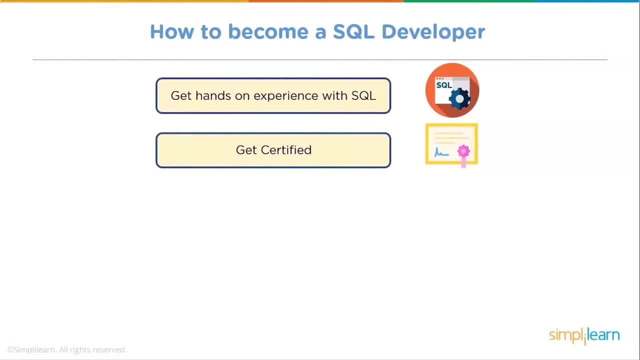 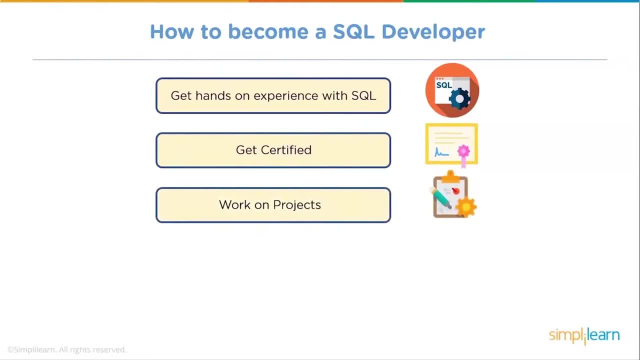 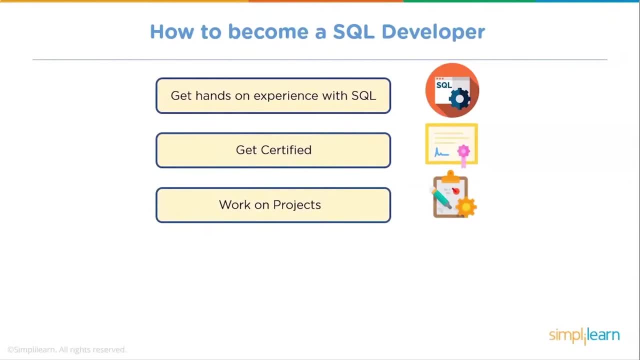 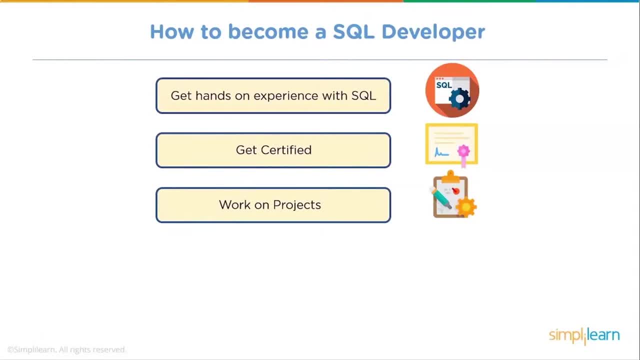 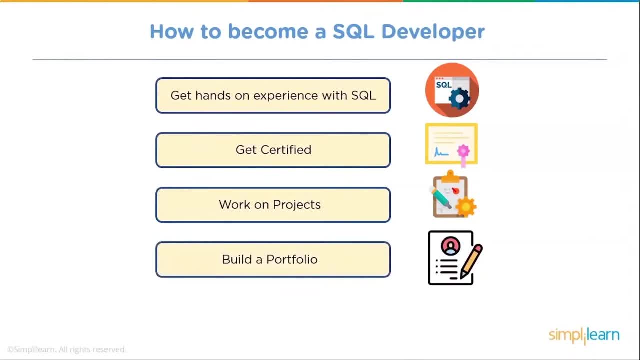 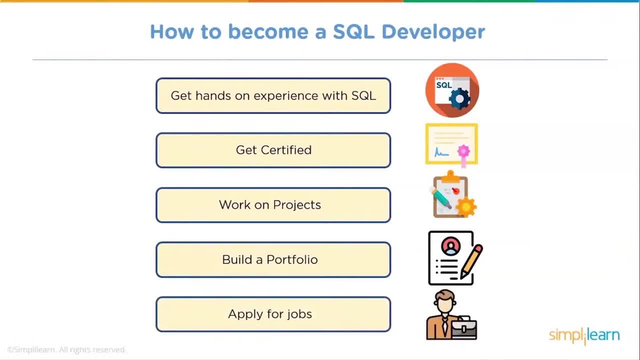 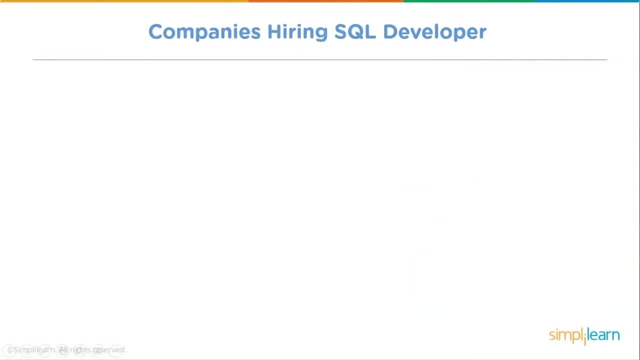 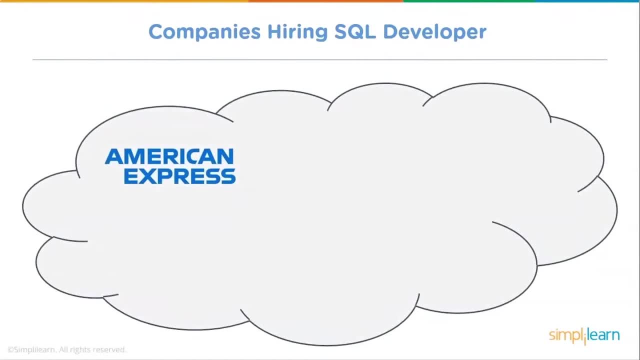 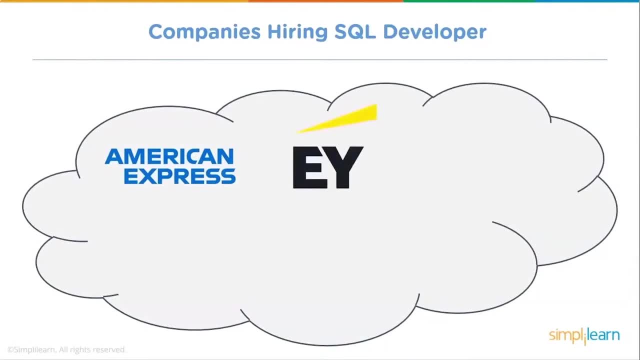 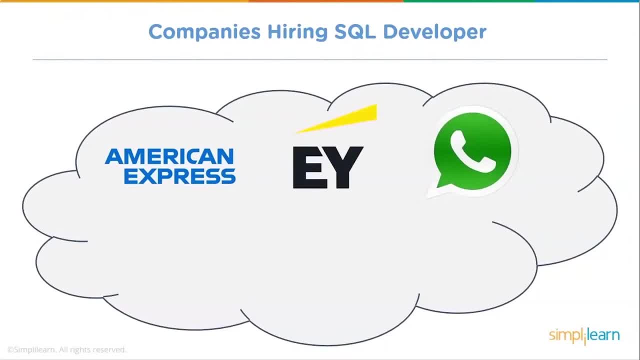 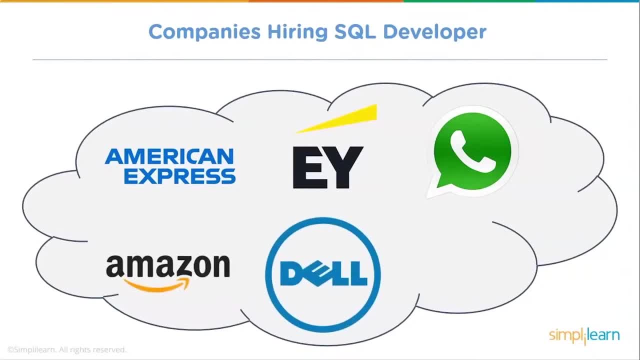 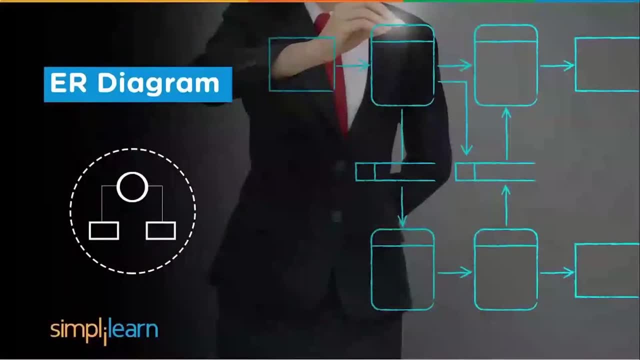 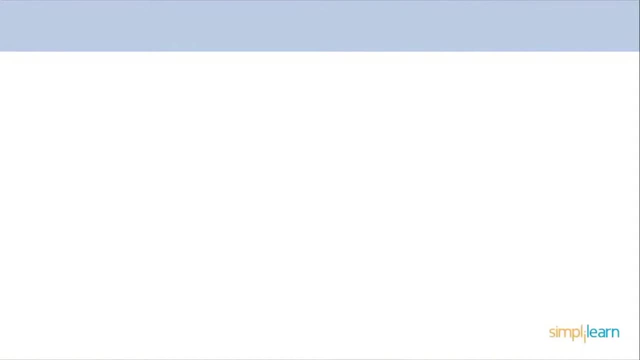 For that one should have a good command on structured query language and can issue queries to get the desired result. In this session we will learn about ER Diagram. Have you ever wondered how these big e-commerce companies manage their tons of data that keeps updating every second? 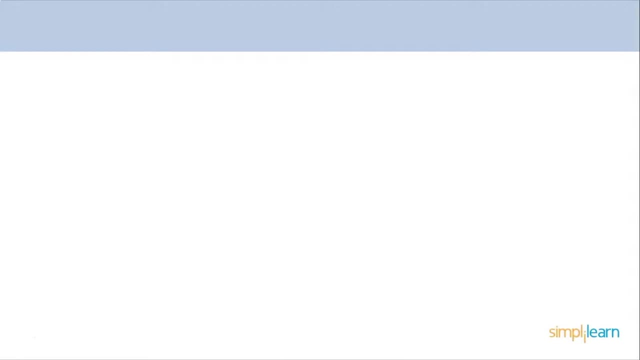 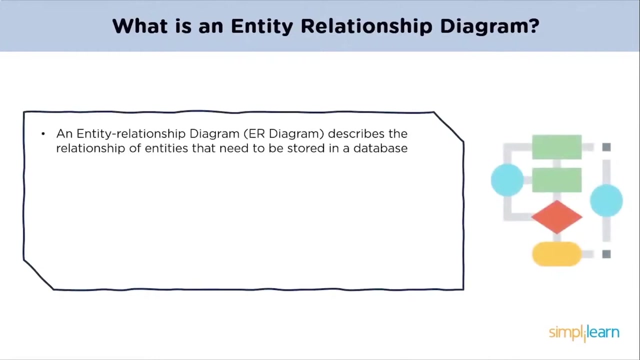 And these data sets keep on updating in their databases. To perform operations on these data, they should have a conceptual understanding of these databases, And this is done by understanding ER Diagram of the databases. So let's understand what an ER diagram is: An entity. 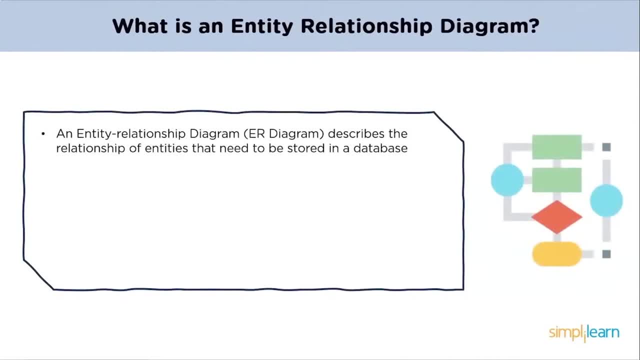 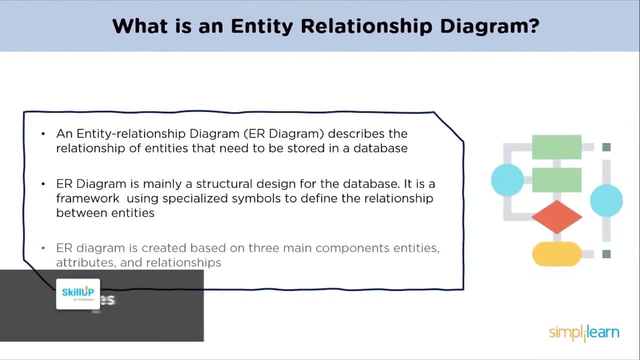 relationship diagram describes the relationship of entities that needs to be stored in a database. ER diagram is mainly a structural design for the database. It is a framework made using specialized symbols to define the relationship between entities. ER diagrams are created based on the three main components: entities, attributes and relationships. Let's understand. 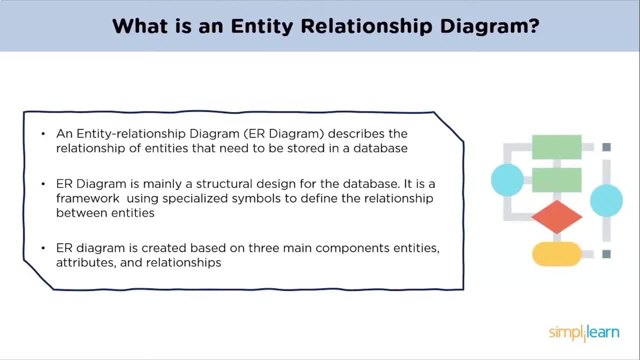 the use of ER diagram with the help of a real-world example Here. a school needs all its student records to be stored digitally, So they approach an IT company to do so. A person from the company will meet the school authorities. note all. 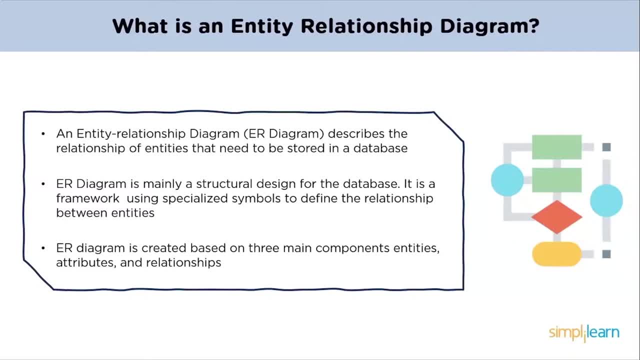 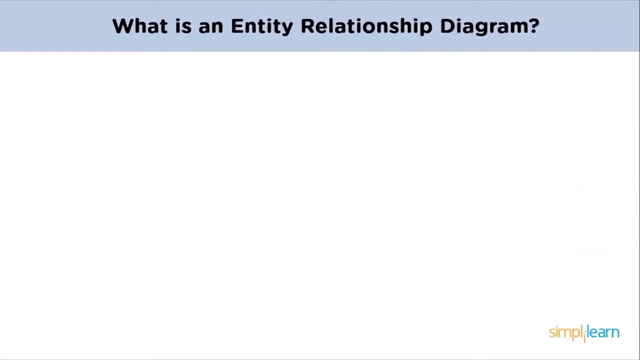 their requirements, describe them in the form of ER diagram and get it cross-checked by the school authorities. As the school authorities approve the ER diagram, the database engineers would carry further implementation. Let's have a view of an ER diagram. The following diagram showcases two. 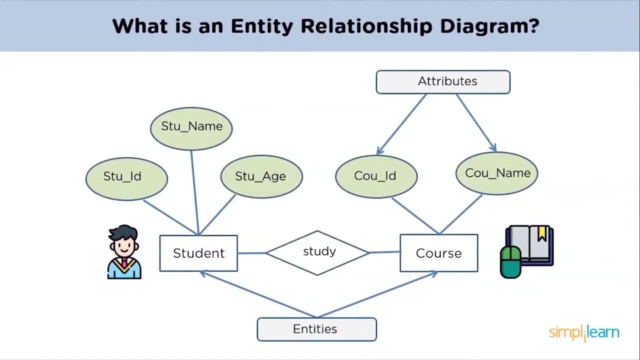 entities and their relationship. The relationship described between student and course is many to many, as a course can be opted by several students and a student can opt for more than one course. Here a student is the entity and it possesses the attributes And 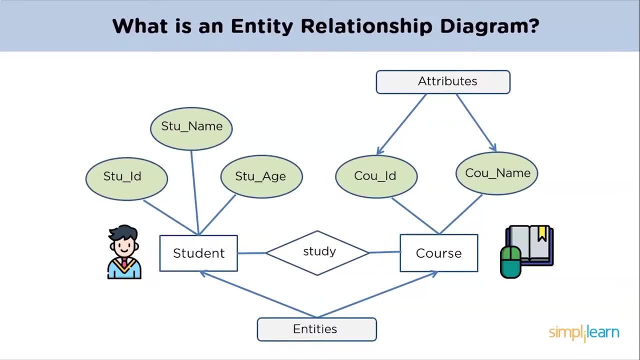 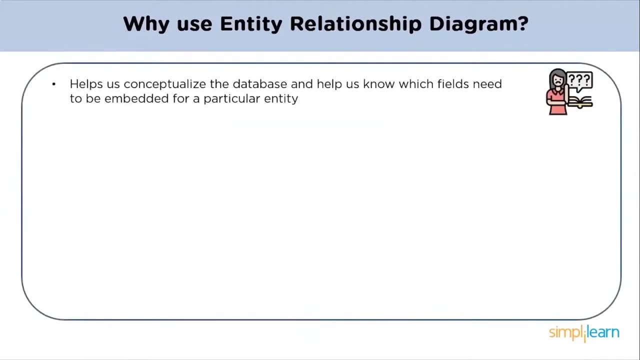 has attributes such as course ID and course name. Now we have an understanding of year diagram. let us see why it has been so popular. The logical structure of the database provided by year diagram communicates the landscape of business to different teams in the company, which is eventually needed to support the 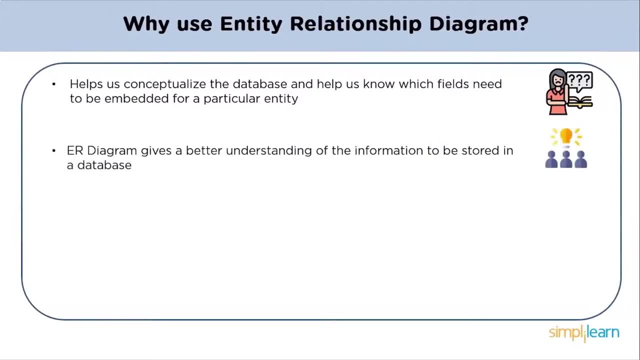 business. Year diagram is a GUI representation of the logical structure of a database which gives a better understanding of the information to be stored in a database. Database designers can use year diagrams as a blueprint, which reduces complexity and helps them save time to build databases quickly. 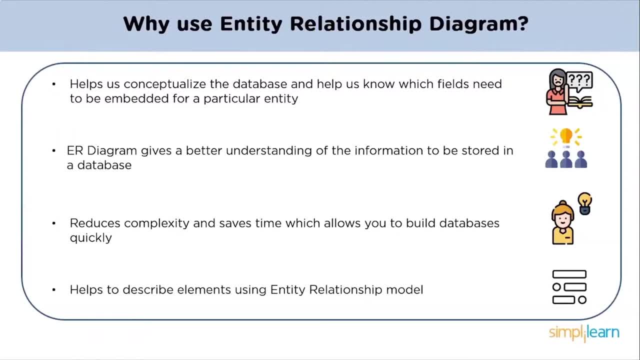 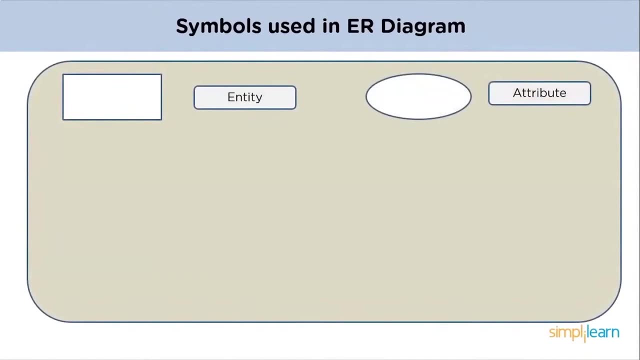 Year diagrams helps you identify the entities that exist in a system and the relationships between those entities. After knowing its uses, now we should get familiar with the symbols used in year diagram. The rectangle symbol represents the entities. oval symbol represents attributes. a rectangle embedded in a rectangle represents a weak entity. a dashed oval represents a. 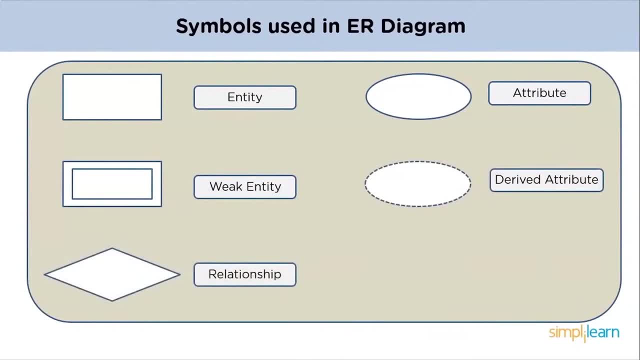 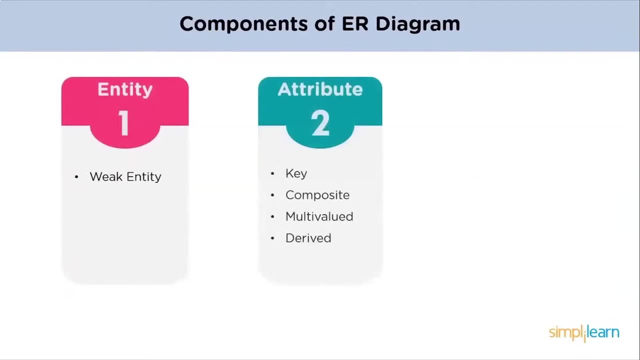 derived attribute. a diamond symbol represents a relationship among entities. double-oval symbol represents multi-valued attributes. Now we should dive in and learn about the components of year diagram. There are three main components of year diagram: entity, attribute and relationship. Entities have 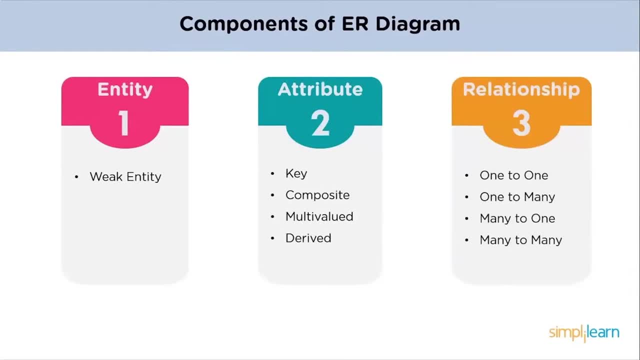 weak entity. attributes are further classified into key attribute, composed attribute, multi-valued attribute and derived attribute. Relationships are also classified into one-to-one relationships, one-to-many relationships, many-to-one relationships and many-to-many relationships. Let's understand these. 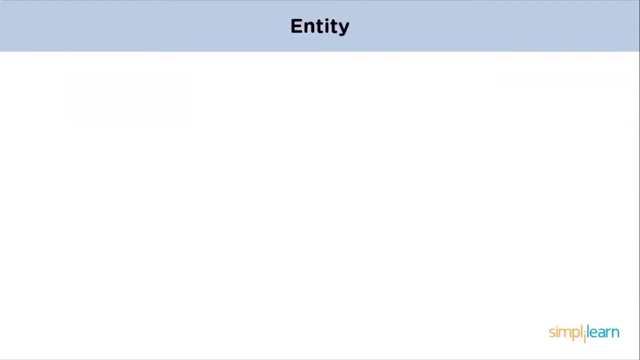 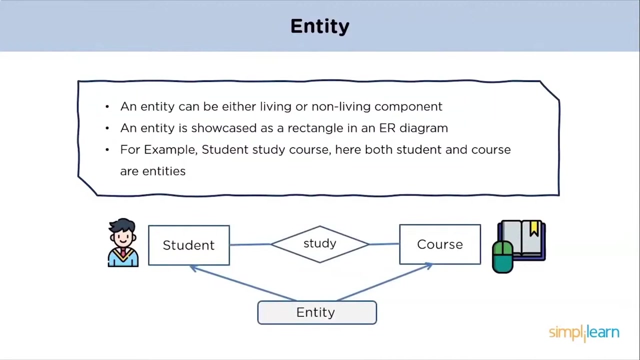 components of year diagram, starting with entities. An entity can be either a living or a non-living component. An entity is showcased as a rectangle in an year diagram. Let's understand this with the help of an year diagram. Here, both student and course are in rectangular shape and are called entities. 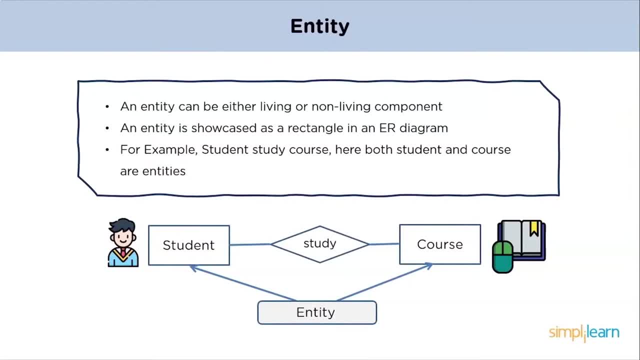 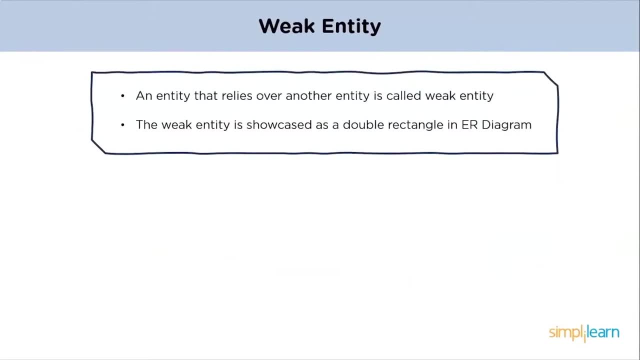 and they represent the relationship study in a diamond shape. Let's transition to weak entity. An entity that makes reliance over another entity is called a weak entity. The weak entity is showcased as a double rectangle in year diagram. In the example below, the school is a strong entity because it has a 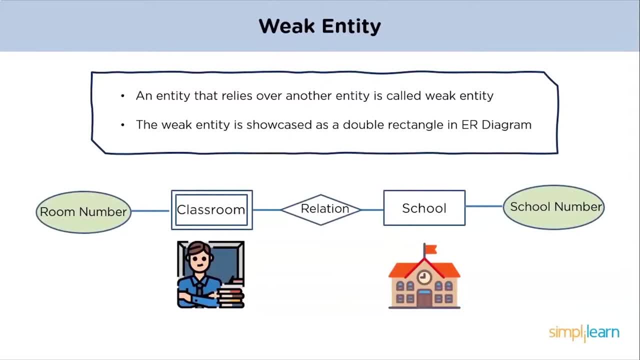 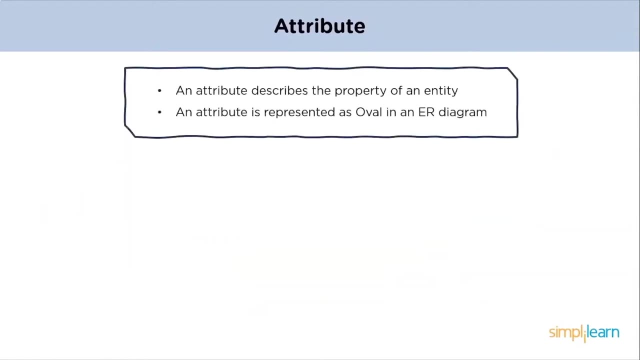 primary key attribute: school number. Unlike the school, the classroom is a weak entity because it does not have any primary key and the room number attribute here acts only as a discriminator and not a primary key. Now let us know about attributes. Attribute: An attribute exhibits the properties of an entity. An attribute is illustrated. 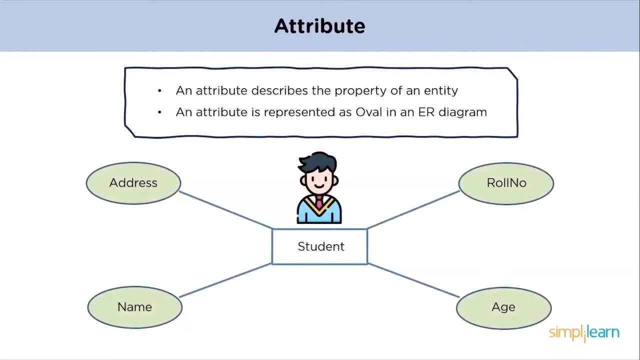 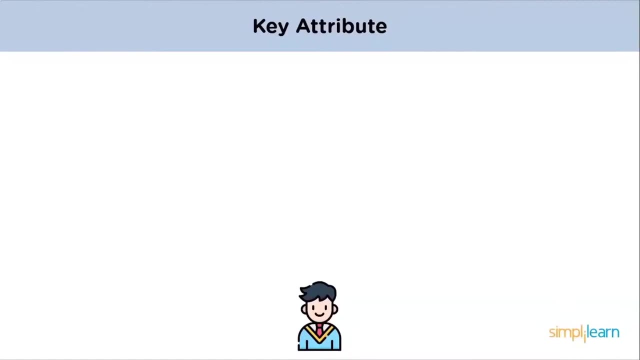 with an oval shape in an year diagram. In the example below, student is an entity and the properties of student, such as address, age and roll number, are called its attributes. Let's see a first classification under attribute. that is key attribute. The key attribute uniquely identifies an entity from an entity set The 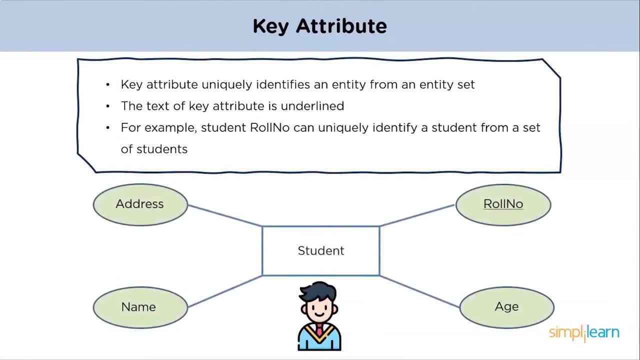 text of a key attribute is underlined In the example below. we have a student entity and it has attributes- name, address, roll number and age. but here roll number can uniquely identify a student from a set of students. That's why it is termed as a key attribute. Now we'll 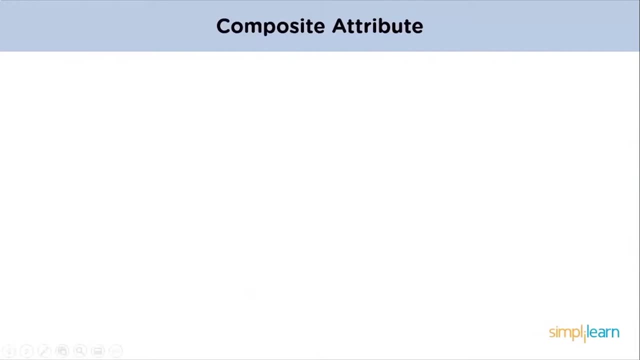 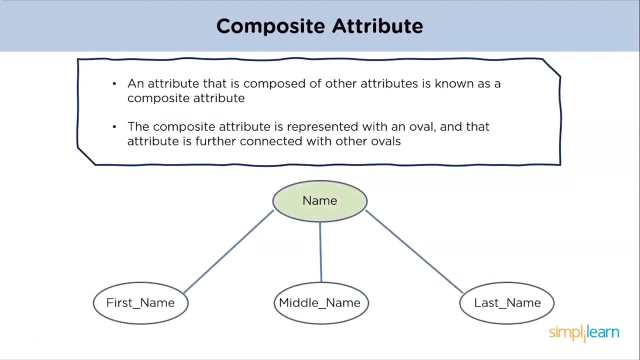 see composite attribute. An attribute that is composed of several other attributes is known as a composite attribute. an oval showcases the composite attribute and the composite attribute oval is further connected with other ovals. In the example below we can see an attribute name which can have further surpass parts. 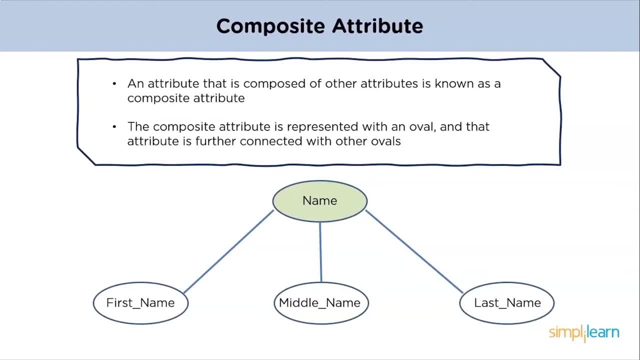 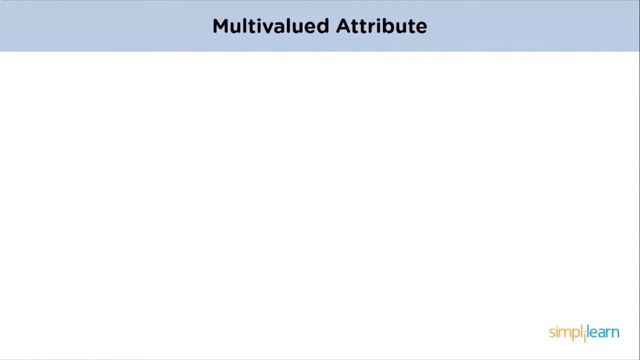 such as first, last kingdom, etc. etc. name, middle name and last name. these attributes with further classification is known as composite attribute. now let's have a look at multi-valued attribute. an attribute that can possess more than one value are called multi-valued attributes. these are represented as double old shape. 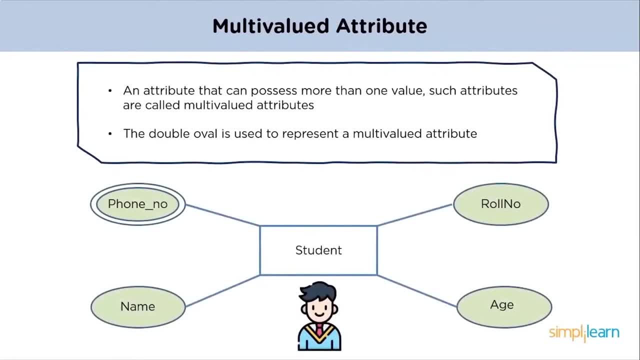 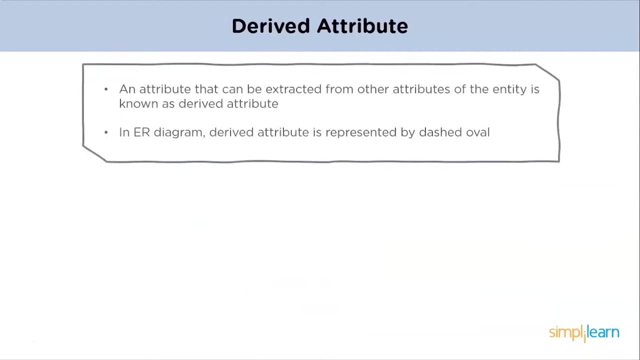 in the example below, the student entity has attributes: phone number, row number, name and age. out of these attributes, phone number can have more than one entry and the attribute with more than one value is called multi-valued attribute. let's see derived attribute. an attribute that can be derived from other attributes of the entity is known as a derived attribute in the 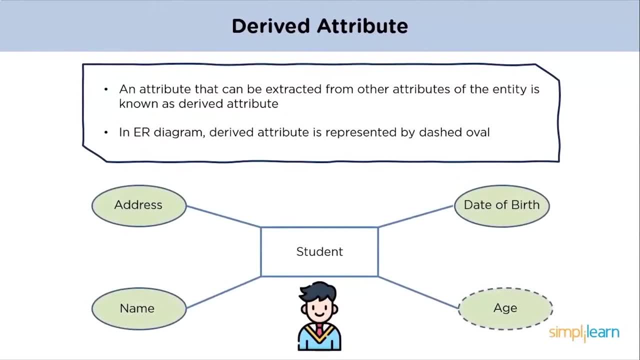 ear diagram the derived attribute is represented by dashed over and in the example below, student entity has both date of birth and age as attributes. here. age is a derived attribute as it can be derived by subtracting current date from the student date of birth. now, after knowing 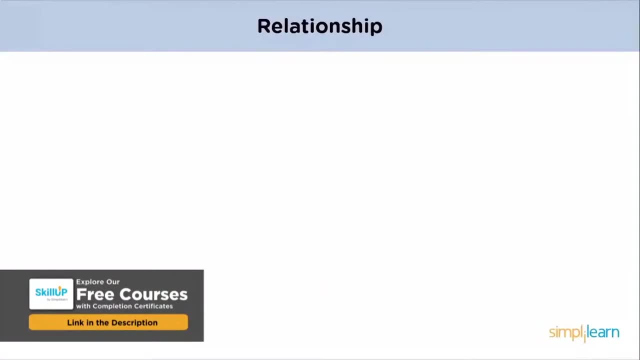 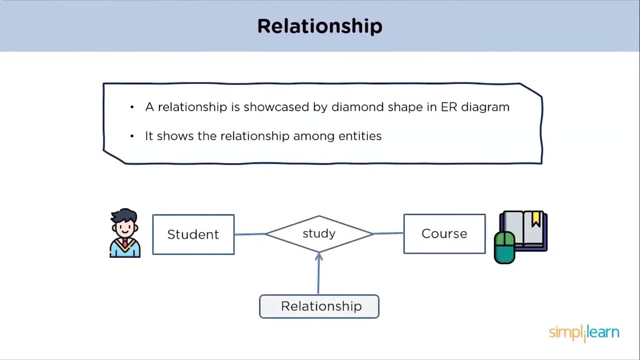 attributes. let's understand relationship in ear diagram. a relationship is showcased by the diamond shape in the ear diagram. it depicts the relationship between two entities in the below example: student, study course. here both student and course are entities and studies the relationship between them. now let's go through the type of relationship. 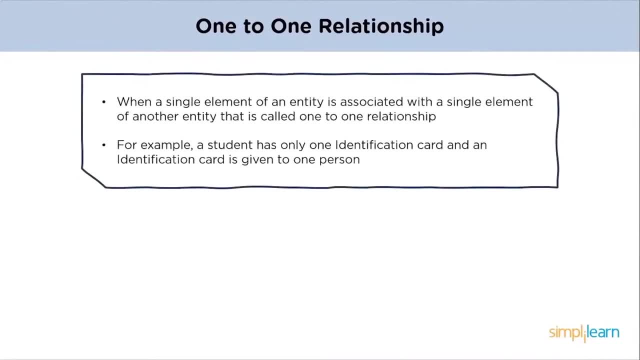 first is one-to-one relationship. when a single element of an entity is associated with a single element of another entity, this is called one-to-one relationship. in the example below we have student and identification card as entities. we can see a student has only one identification card and an identification card is given to one student. it represents a one-to-one relationship. 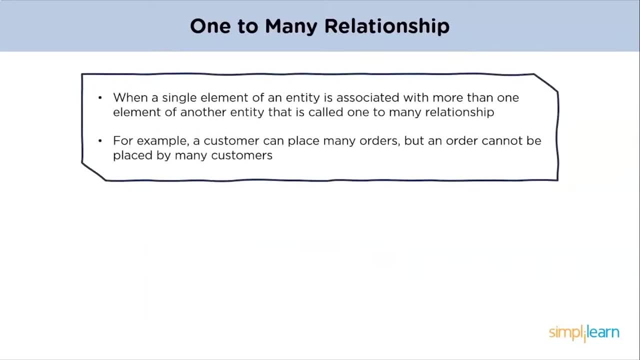 let's see the second one. one-to-one relationship, when a single element of an entity is associated with more than one element of another entity, is called one-to-many relationship. in the below example, a customer can place many orders, but a particular order cannot be placed by many customers. 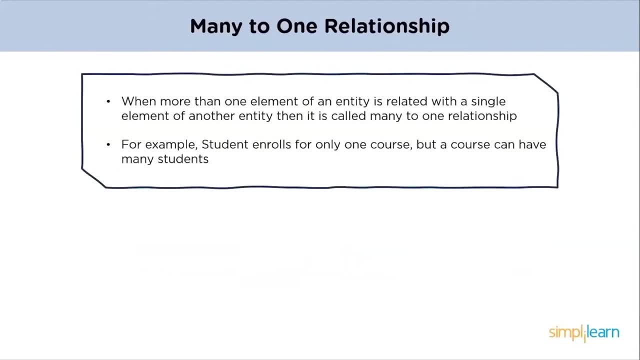 now we will have a look at many-to-one relationship. when more than one element of an entity is related to a single element of another entity, it is called many-to-one relationship. for example, students have to opt for a single course, but a course can be opted by number of students. 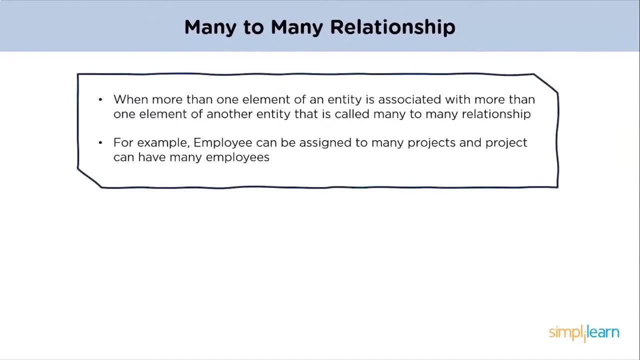 let's see many-to-many relationship. when more than one element of an entity is associated with more than one element of another entity is called many-to-many relationship. for example, an employee can be assigned to many projects and many employees can be assigned to a particular project. now, after having an understanding of vr diagram, let us know about the relationship between two entities. 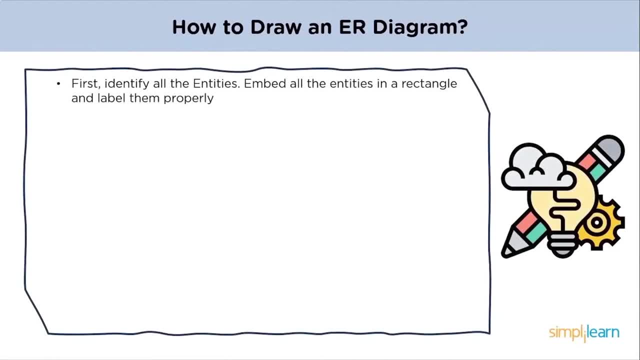 the points to keep in mind while creating the year diagram. First, identify all the entities in the system. embed all the entities in a rectangular shape and label them appropriately. This could be a customer, a manager, an order, an invoice, a schedule, etc. 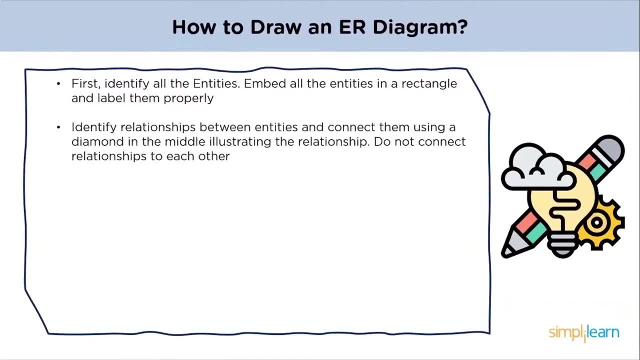 Identify relationships between entities and connect them using a diamond in the middle illustrating the relationship. Do not connect relationships. Connect attributes with entities and label them appropriately, and the attributes should be in oval shape. Assure that each entity only appears a single time and eradicate any redundant entities. 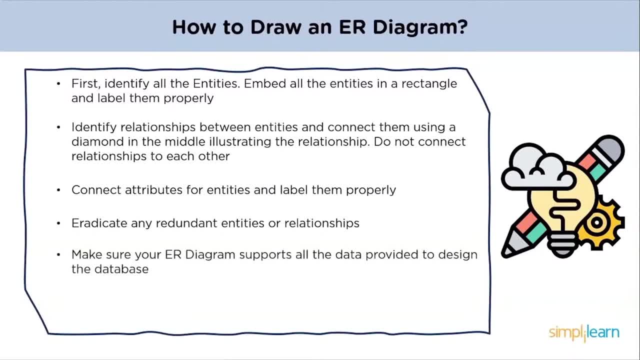 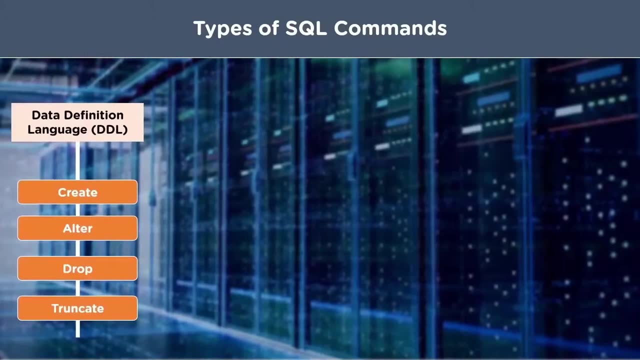 or relationships in the year diagram. Make sure your year diagram supports all the data provided to design the database. Make effective use of colors to highlight key areas in your diagrams. There are mainly four types of SQL commands. So first we have Data Definition Language, or DDL. 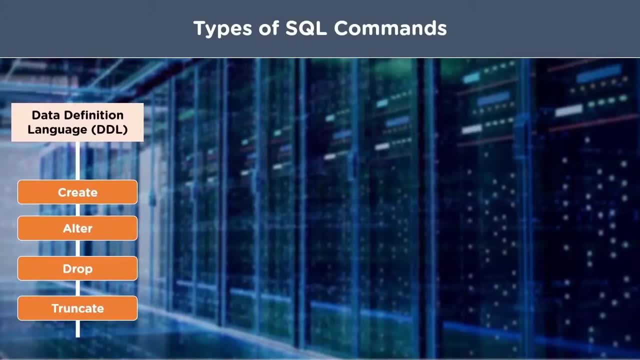 So DDL commands change the structure of the table, Like creating a table, Deleting a table or altering a table. All the commands of DDL are auto committed, which means it permanently save all the changes in the database We have: Create, Alter, Drop and Truncate as DDL commands. 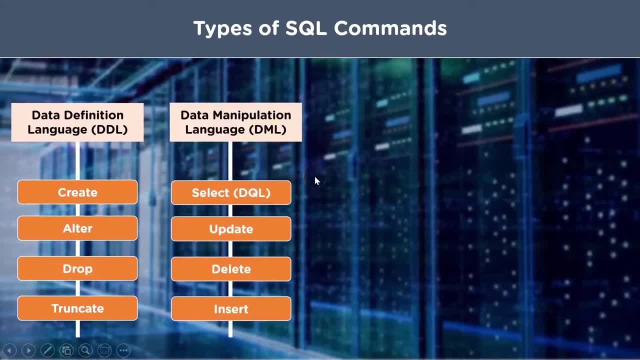 Next we have Data Manipulation Language, or DML. So DML commands are used to modify a database. It is responsible for all forms of changes in the database. DML commands are not auto committed, which means it can't permanently save all the changes. 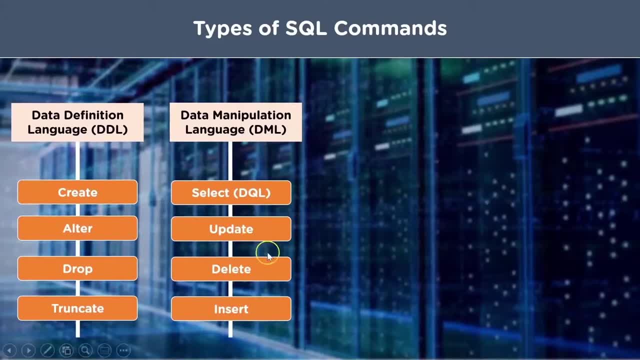 in the database. We have Select, Update, Delete and Insert as DML commands. Now Select command is also referred to as DQL or Data Query Language. Third, we have Data Control Language, or DCL. So DCL commands allow you to control access to data within the database. 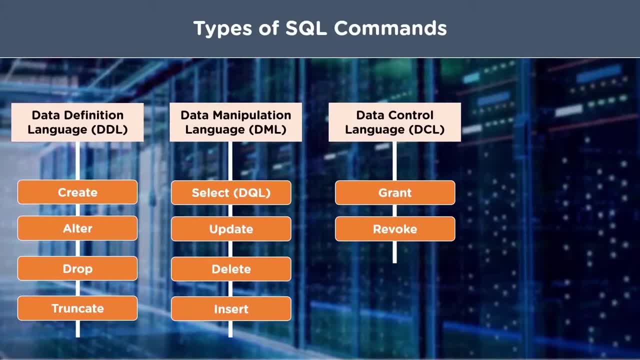 These DCL commands are normally used to create objects related to user access and also control the distribution of privileges among users. So we have Grant and Revoke, which are the examples of Data Control Language. Finally, we have something called as Transaction Control Language, or TCL. 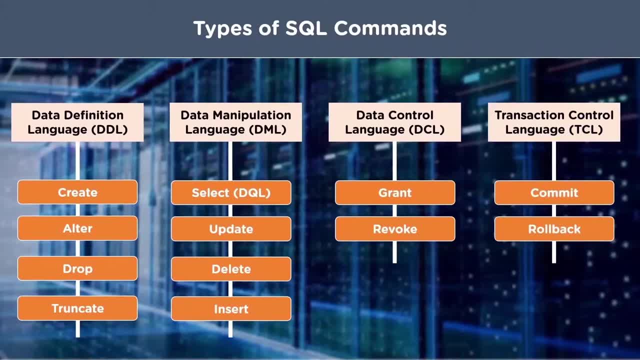 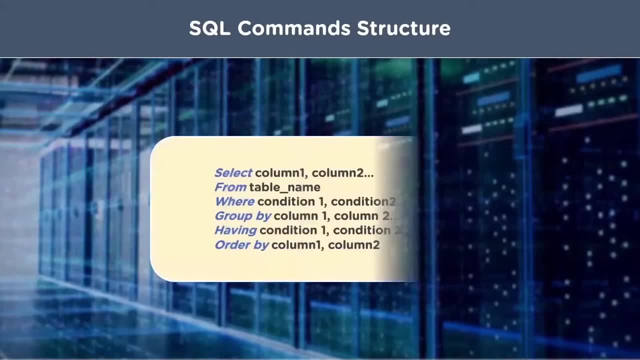 So TCL commands allow the user to manage database transactions. Commit and Rollback are examples of TCL. Now let's see the basic SQL command structure. So first we have the SELECT statement. So here you specify the various column names that you want to fetch from the table. 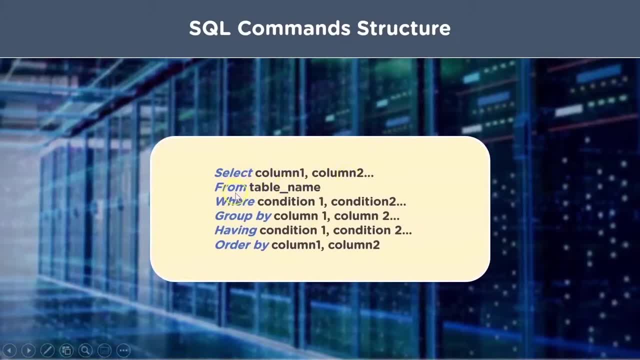 We write the table name using the FROM statement. Next We have the WHERE clause to filter out a table based on some conditions. So you can see here WHERE- condition 1,, condition 2 and so on. Then we have the GROUP BY clause that takes various column names. 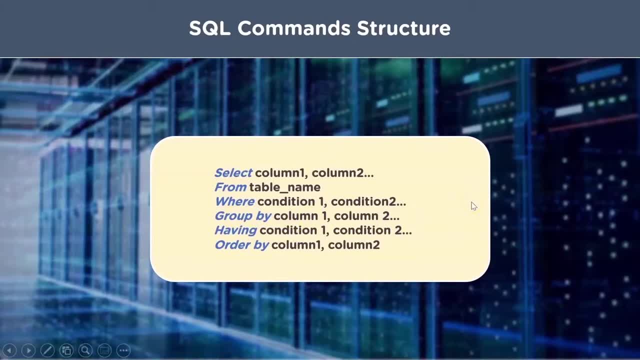 So you can write GROUP BY column 1, column 2 and so on. Next, we have the HAVING clause to filter out tables based on groups. Finally, we have the ORDER BY clause to filter out the result in ascending or descending order. Now talking about the various data types in SQL. 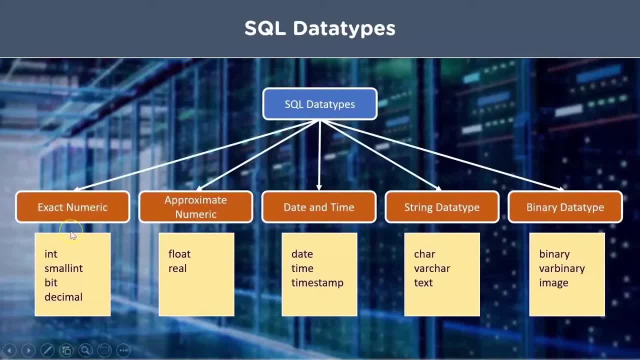 So we have the ORDER BY clause. We have the ORDER BY clause to filter out the result in ascending or descending order. Then we have EXACT NUMERIC which has INTEGER, SMALLINT, BIT and DECIMAL. Then we have APPROXIMATE NUMERIC which are FLOAT and REAL. 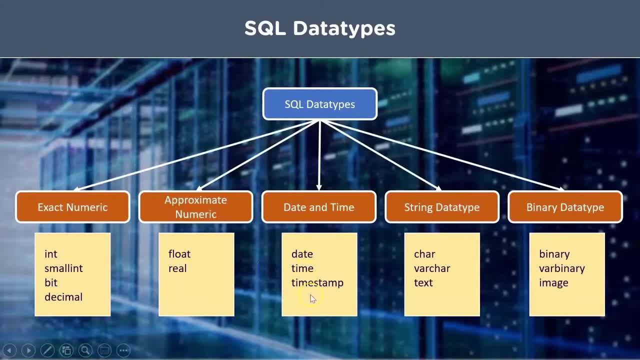 Then we have some DATE and TIME data types, such as DATE, TIME, TIMESTAMP and others. Then we have STRING data type, which includes CAR, VARCAR and TEXT. Finally, we have BINARY data types and BINARY data types have BINARY, VARBINARY and IMAGE. 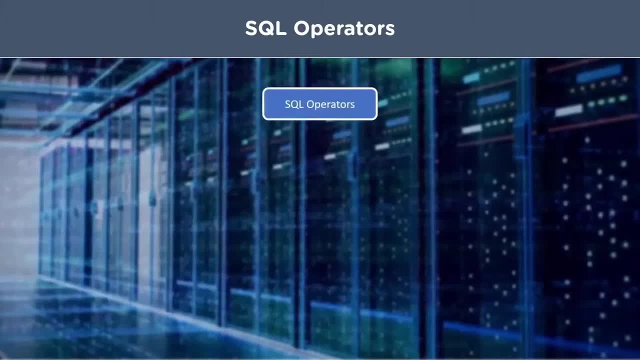 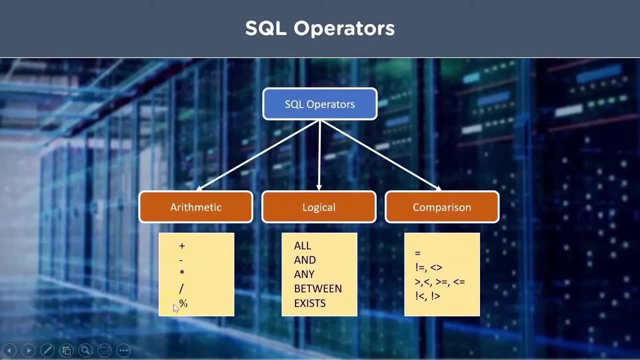 Now let's see some of these data types. Let's see some of the various operators that are present in SQL. So first we have our basic arithmetic operators. So you have ADDITION, SUBSTRACTION, MULTIPLICATION, DIVISION and MODULARS. 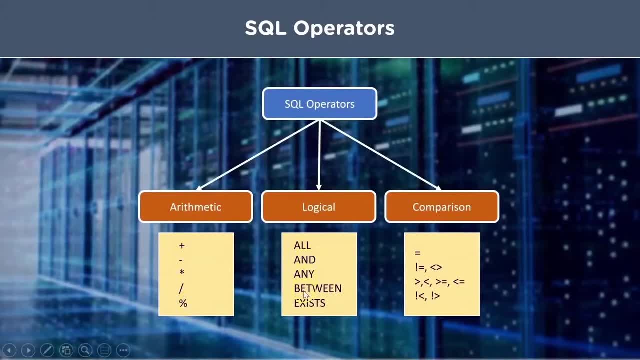 Then we have some logical operators like ALL AND ANY, OR BETWEEN EXISTS, and so on. Finally, we have some comparison operators such as EQUAL TO NOT EQUAL TO, THUS GREATER THAN LESS THAN, GREATER THAN EQUAL TO, or LESS THAN EQUAL TO, NOT LESS THAN or NOT GREATER. 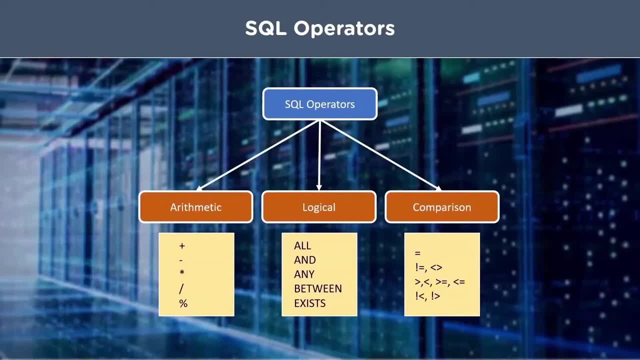 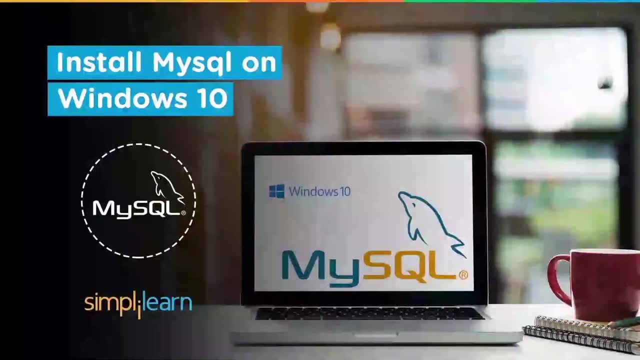 THAN. Now let me take you to my MySQL workbench. Well, we will learn to write some of the important SQL commands, use different statements, functions, data types and operators that we just learned. In this session. we will learn how to install MySQL workbench and then we will run some. 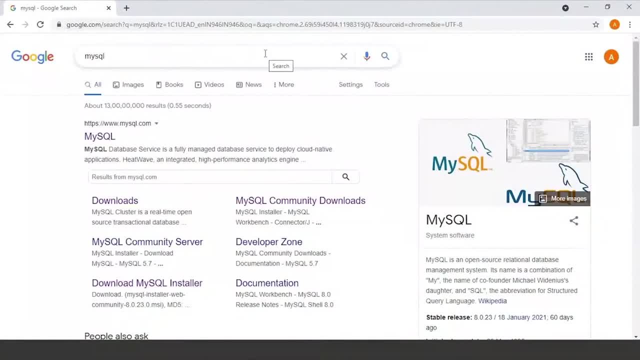 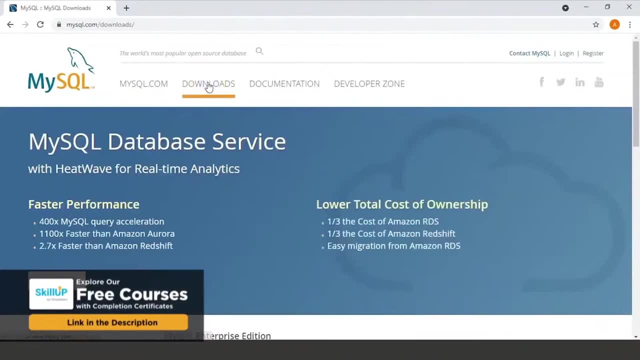 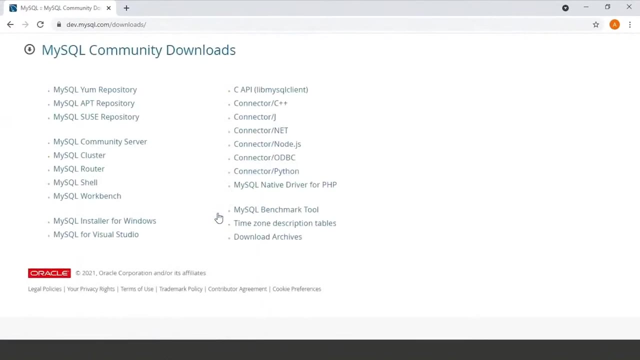 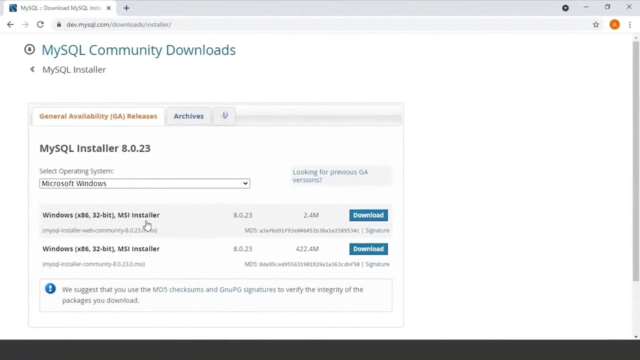 commands. Firstly, we will visit the official Oracle website, that is, mysqlcom, and now we will move to the downloads page. Now scroll down and click on MySQL GPL Downloads. Now, under Community Downloads, click on MySQL Installer for Windows. The current versions are available to download. 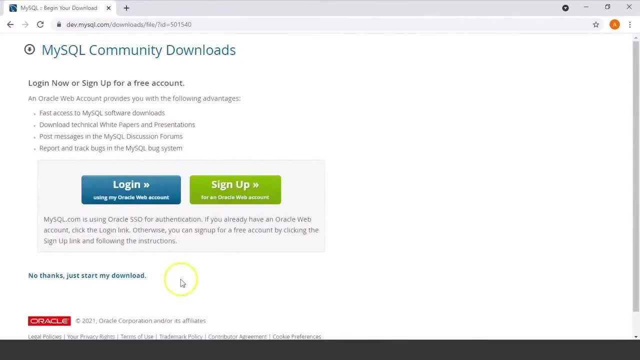 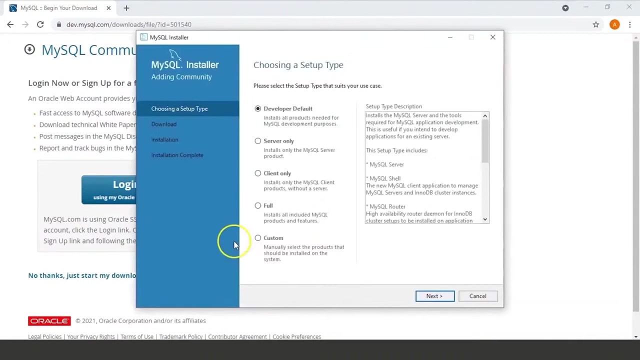 I will choose this installer and click the download button Now here. just click on No. Thanks, just start my download. Once the installer has downloaded, open it. You may be prompted for permission. Click Yes. This opens the installer. You will be asked to choose the setup type. 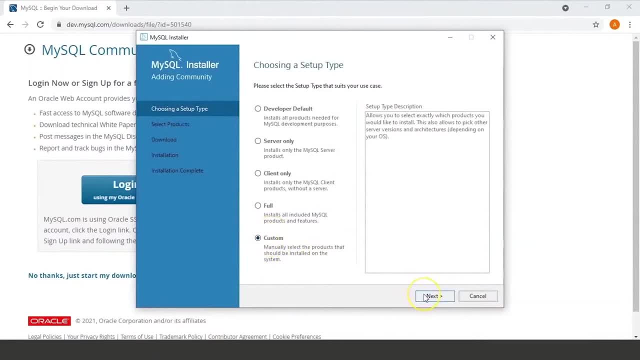 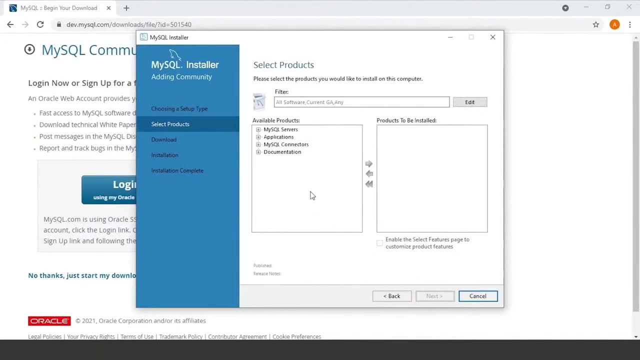 We will go with Custom. Click Next. Now you have to select the products you want to install. We will install only the MySQL Server, MySQL Shell and the MySQL Workbench. Expand MySQL Servers by double clicking on it and choose the version you want to install. 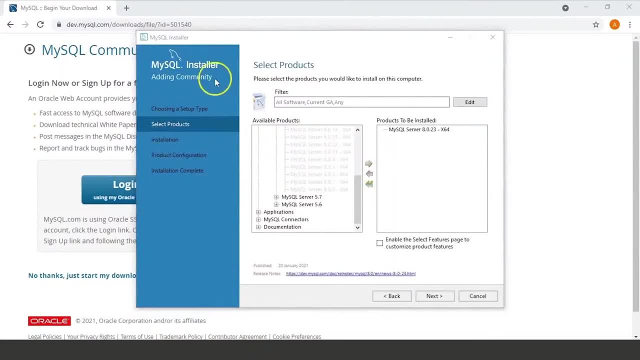 Click on this arrow. Now we have to do the same thing for applications: Expand Applications and choose the MySQL Workbench version you want to install. Click on the arrow. We will do the same thing for MySQL Shell and choose the latest version. Click on the arrow. 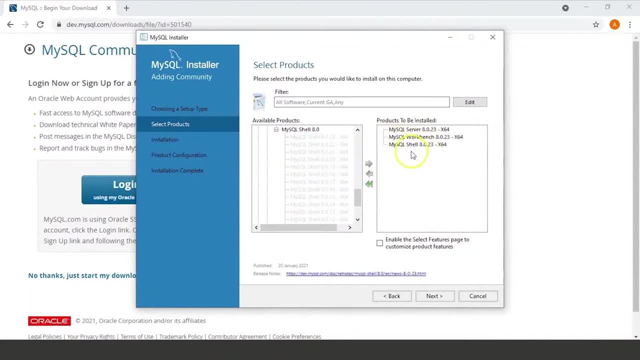 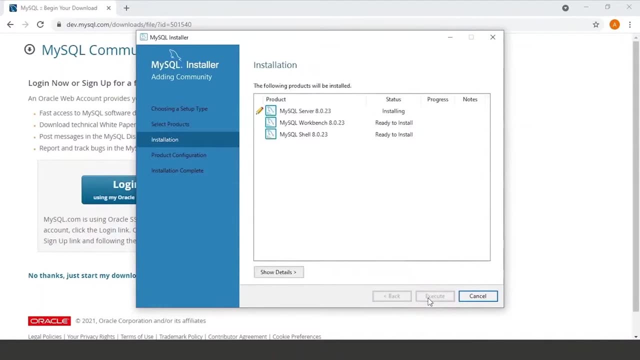 These are the products that have to be installed in a system. Now we will click Next. Now click Execute to download and install the server. This may take a while, depending on your internet speed. As the download is completed, click Next. Now you will see the product configuration. 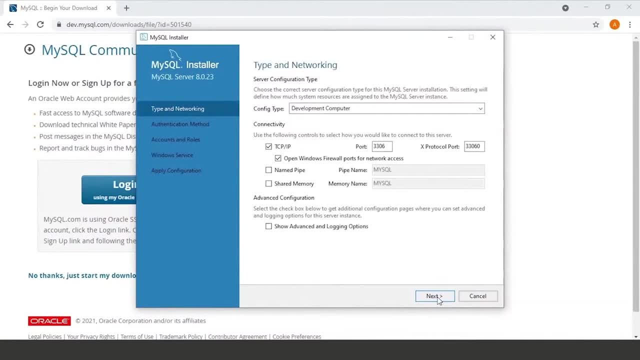 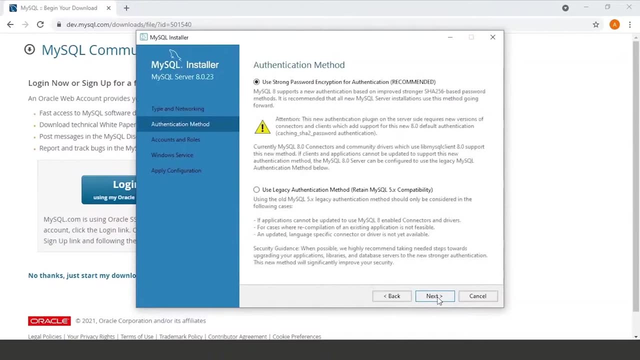 Click Next. Now we will configure our SQL Server Instance. Here we will go with the database. Click Next. Here we will go with the default settings and click Next. And under authentication, select Use strong password encryption for authentication, which is recommended, and click on Next. 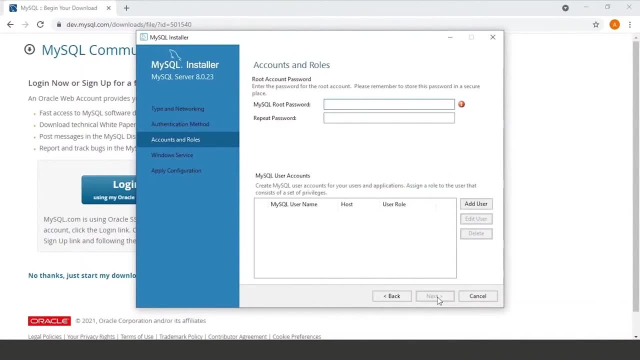 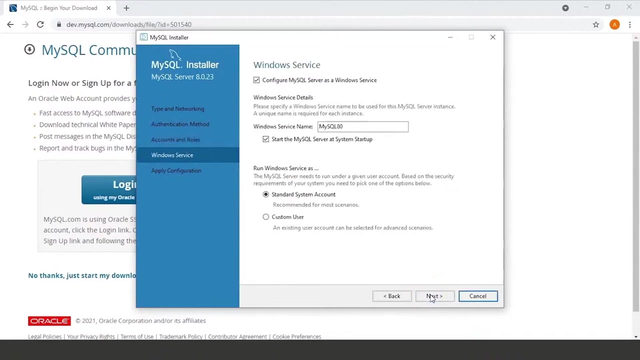 Now here, set the password for your root user. By the way, root is the default user. This user will have access to everything. Now I will set my password, Click Next. Now I will click on Next And here also we will keep the default settings. 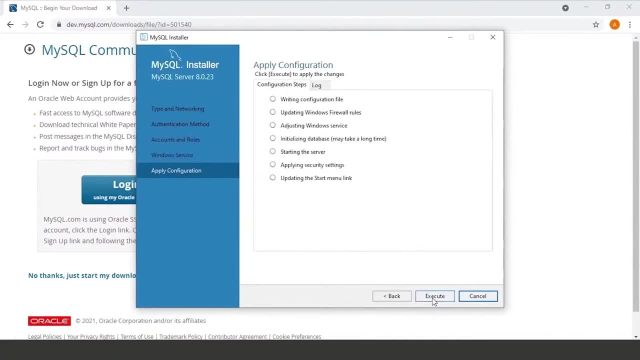 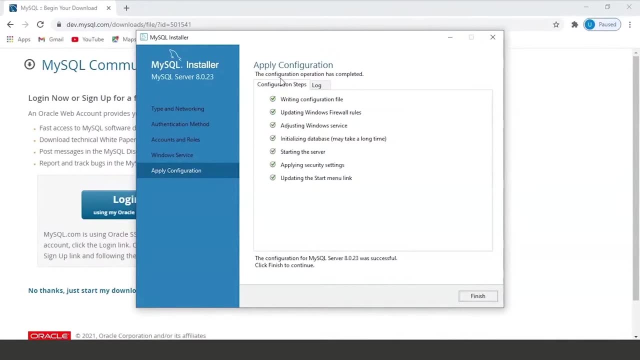 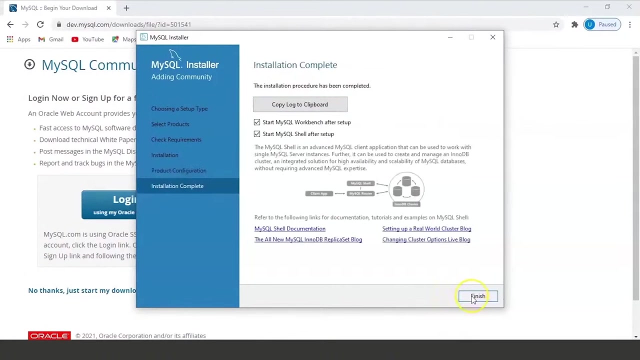 And click on Next Now to apply the configuration. we will execute the process. Once all the configuration steps are complete, click Finish. Click Next Now. you will see the installation is complete. It will launch MySQL Workbench and MySQL Shell after clicking on Finish. 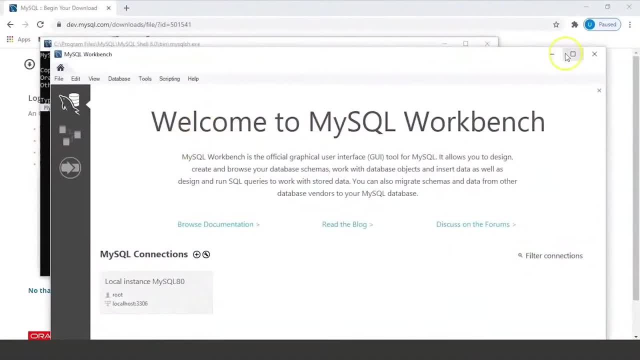 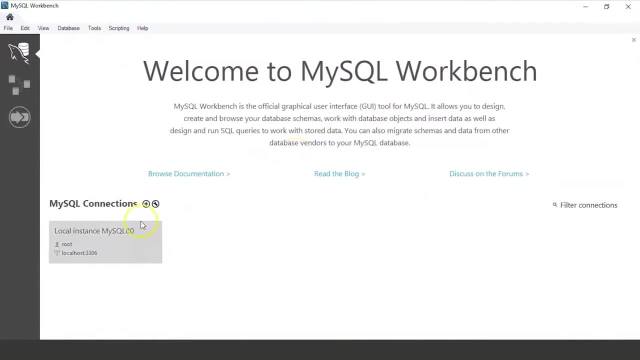 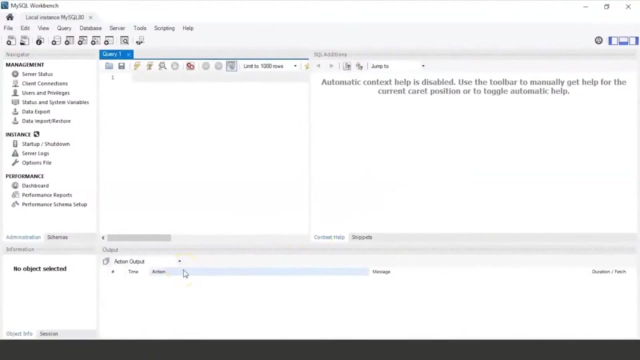 Now the Shell and Workbench has started. Now we will connect by clicking on the root user. It will ask for a password. Enter the password and it will connect successfully. Click Next Now the Workbench has started. Now we will just connect to server. 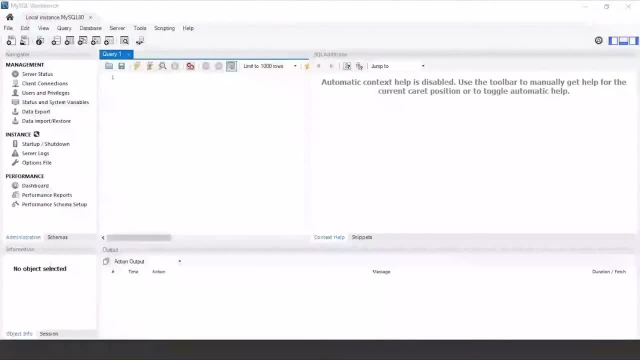 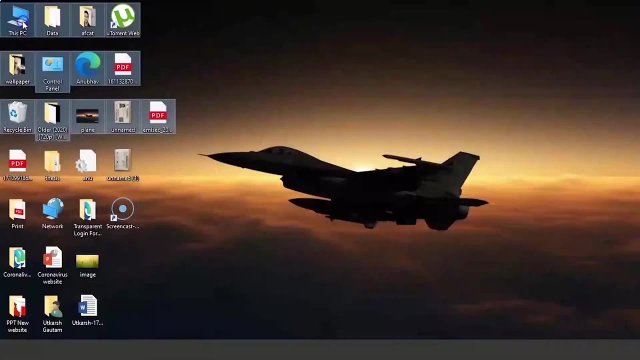 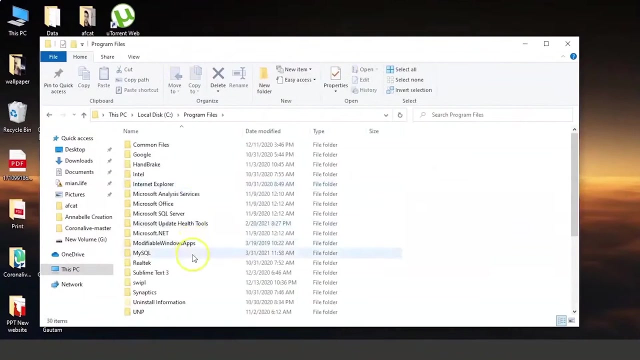 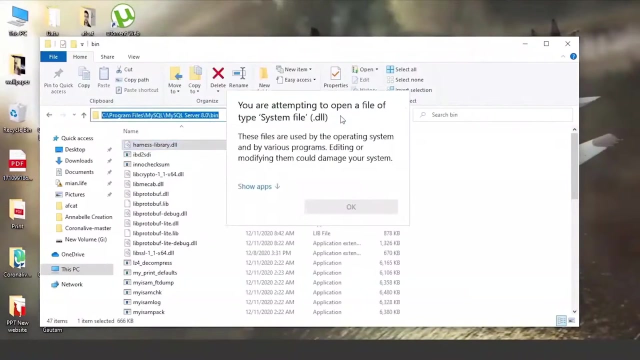 So first we will open Command Prompt, Now we will reach the path where MySQL files are present. We will go to this PC, Localhost 3. Program Files: MySQL MySQL Server 8.0. Bin. And now we will copy this path. 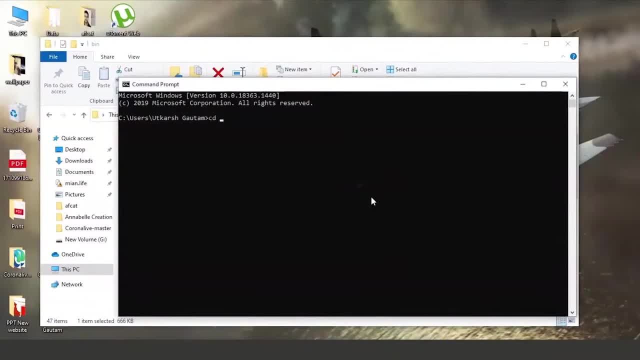 Now we will open the Command Prompt And write a command- cd space and paste the link And press Enter. Now we will write another command. Type it with MySQL Minus u, Space, Root Minus p And press Enter. 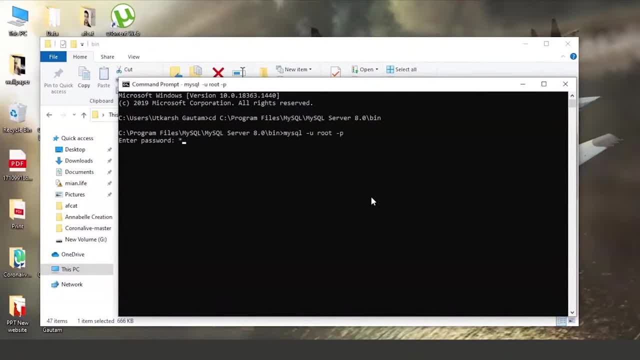 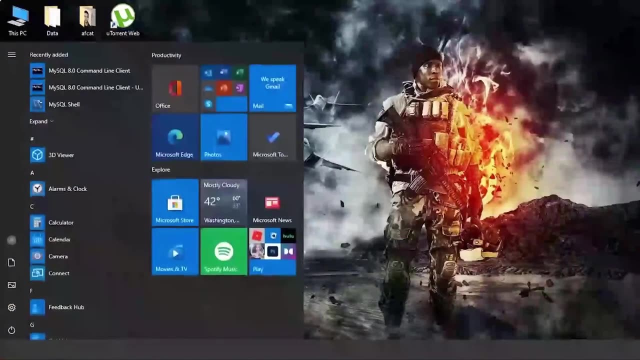 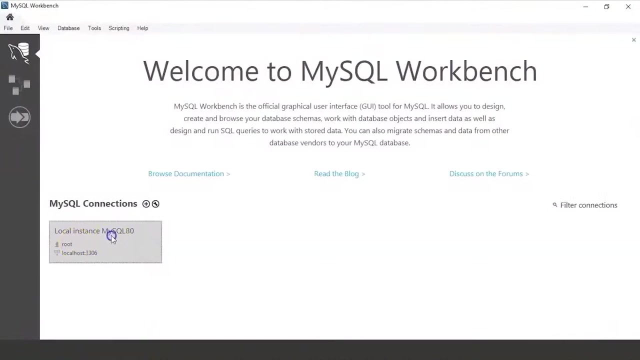 Now it will ask for your password. Just enter the password And press Enter. Now the server has started And now we will see some commands in MySQL Workbench. First we will open MySQL Workbench. Now we will click on the local instance, mysql80.. 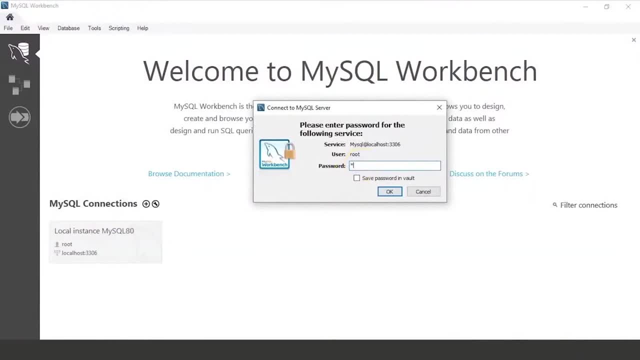 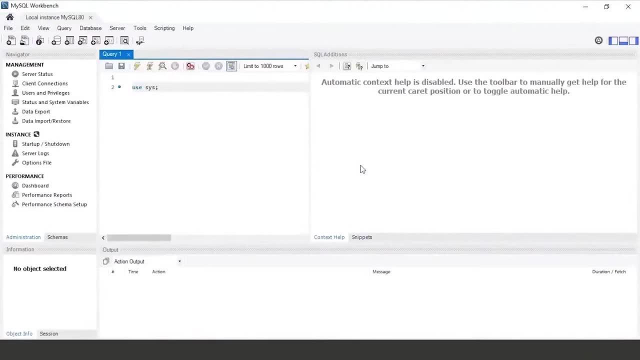 And enter the password to connect to the localhost. Now the MySQL Workbench has started. Now we will see some commands. The first command we will see is show databases- Show databases- semicolon. And now we will select the whole command And click on this execute button. 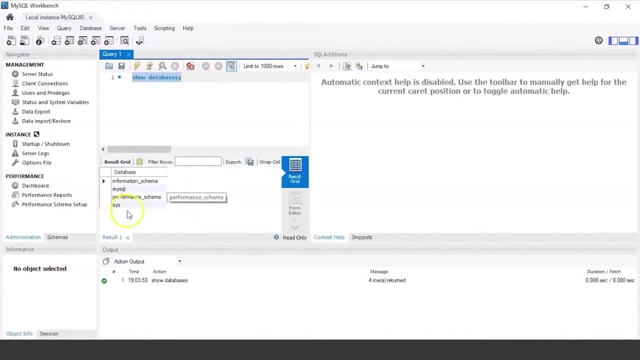 And here we will see the result In the result grid. These are the databases that are stored already in the database. Now there are four databases, That is, Information Schema, MySQL, Performance Schema and SYS. Now we will select one of the databases. 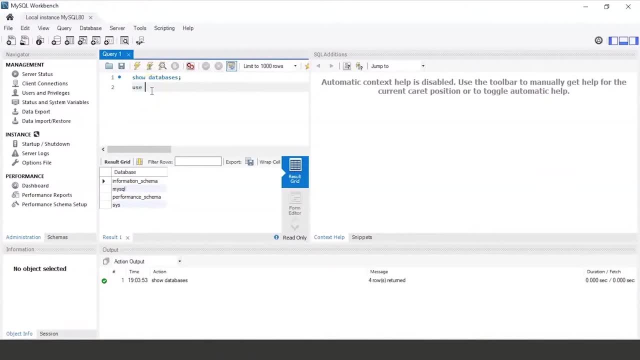 We will use MySQL. Now we have selected the MySQL database And now in this database we will see which tables are stored in this MySQL database. To see that we will run a command Show tables, We will select the command And click on the execute button. 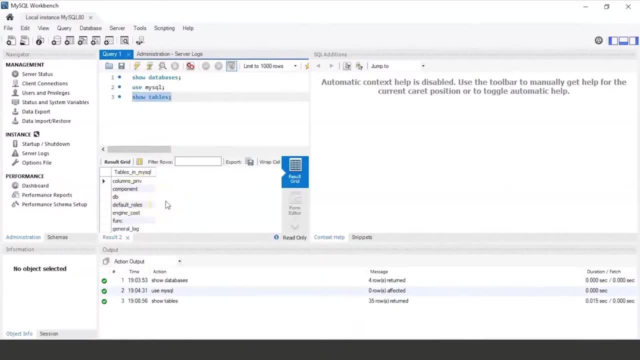 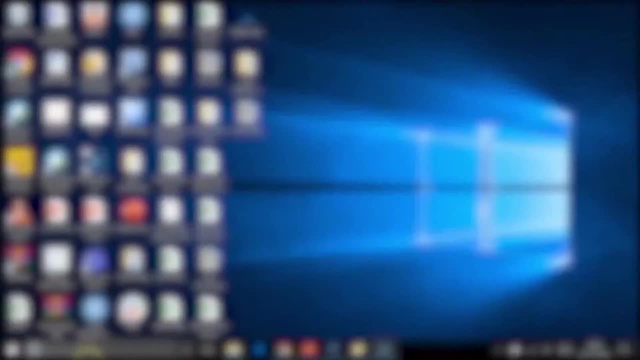 These are the tables that are stored in this MySQL database, That is, columns, underscore, prime, component db and much more Now. let me now go ahead and open my MySQL Workbench. So in the search bar I will search for MySQL Workbench. 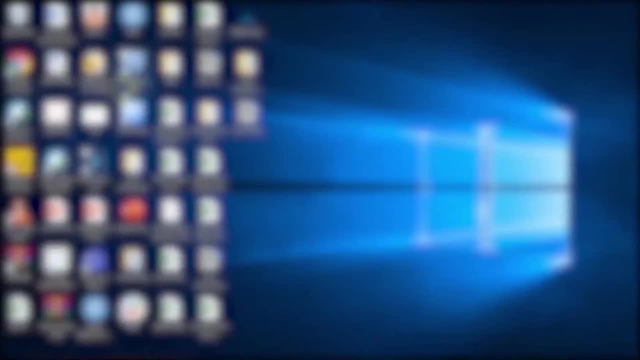 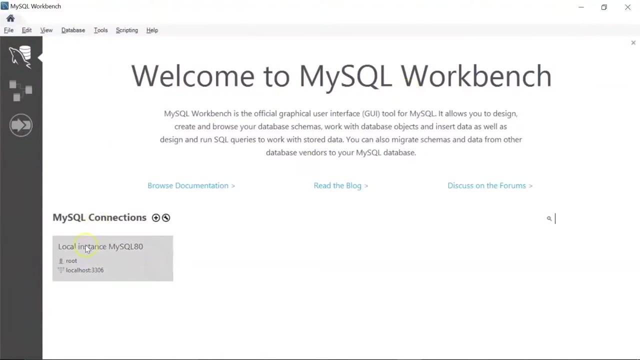 You can see I am using the 8.0 version. I will click on it And here it says: welcome to MySQL Workbench. And below, under connections, you can see I have already created a connection which says local instance. Then you have the root, the local host and the port number. 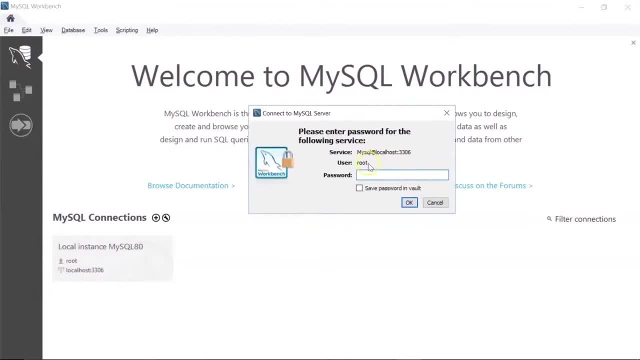 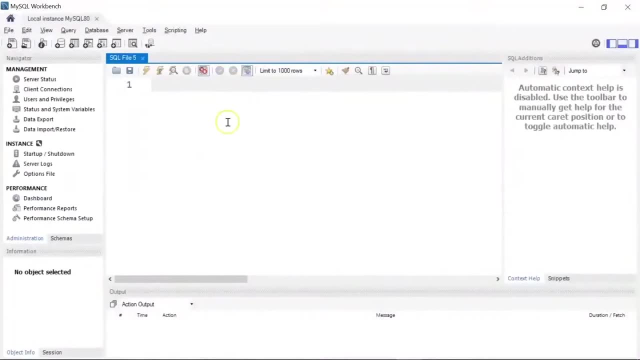 Let me click on it. You can see the service. The username is root And I will enter my password And hit OK. Now this will open the SQL editor. So this is how the MySQL Workbench looks like. Here We learn. 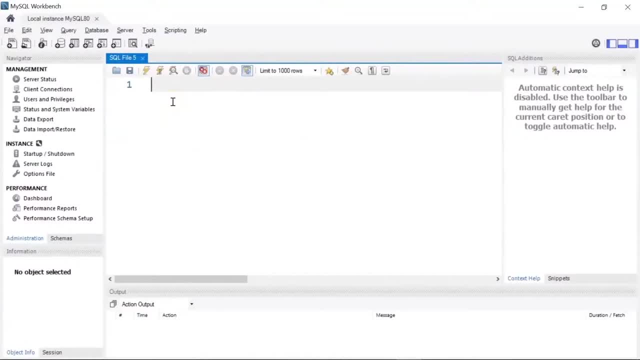 Some of the basic SQL commands. So first let me show you the databases that are already present. So the command is show databases. You can hit tab to autocomplete. I will use a semicolon, I will select this And here on the top you can see the execute button. 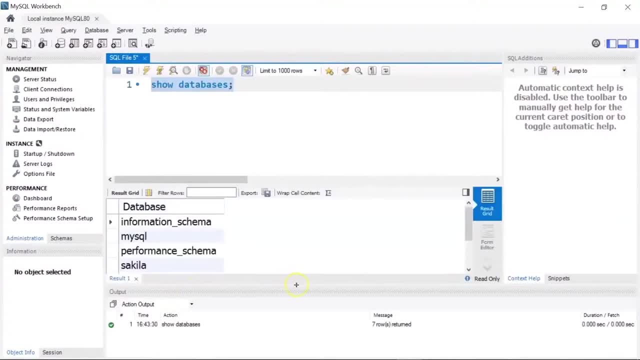 So if I run this Below, you can see the output. It says: show databases. Seven rows are returned, Which means Currently there are seven Databases. You can see the names. Alright, Now Let's say I want to. 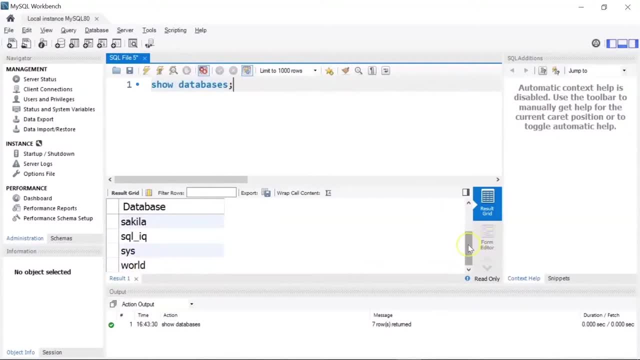 See the tables that are present inside this database called world. So I will use the command use World, Which is the database name. Now let me run it. So currently I am using the world database, So to display the tables that are present in the world database. 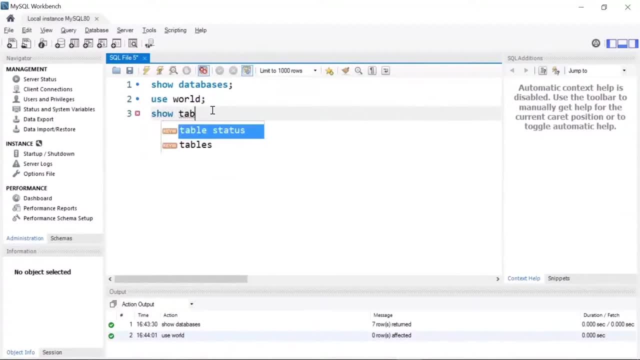 I can use the show command And write Show tables. Give a semicolon And I will hit Control enter this time to run it Alright, So you can see the tables that are present inside this World database. So we have three tables in total. 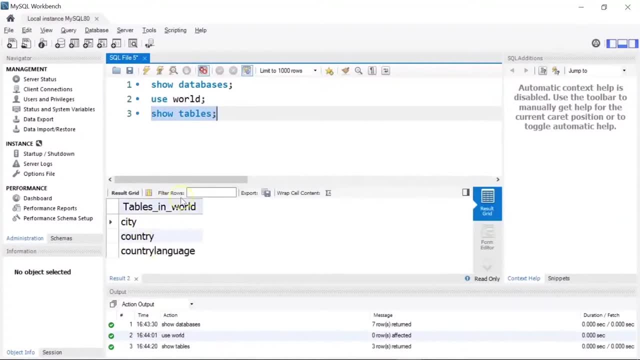 City, Country And country language. Now, If you are to see The rows that are present in one of the tables, You can use the select command. So I will write Select Star, Which basically means I want to display all the columns. 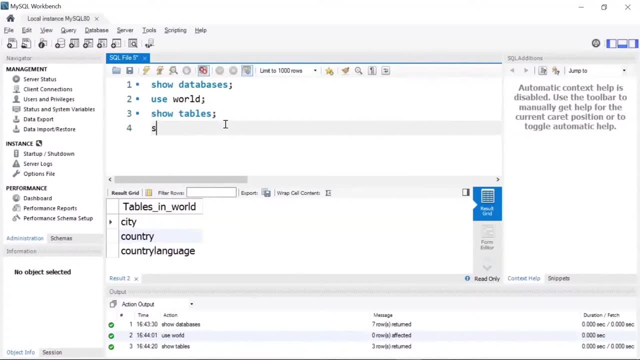 So I will write Select Star, Which basically means I want to display all the columns. So I will write Select Star, Which basically means I want to display all the columns. So star here means To display all the columns. 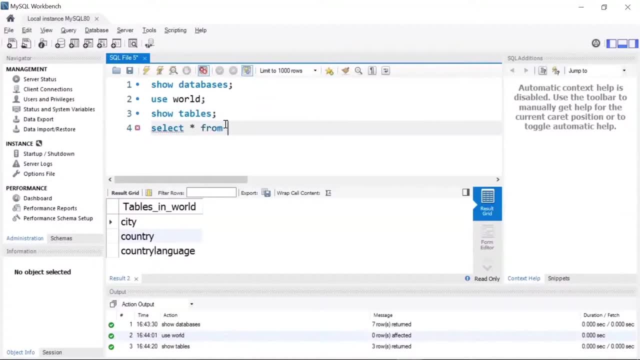 Then I will write My From The table name That is City. So this command Is going to display me All the rows That are present Inside the City table. So if I hit Control, enter, Alright. 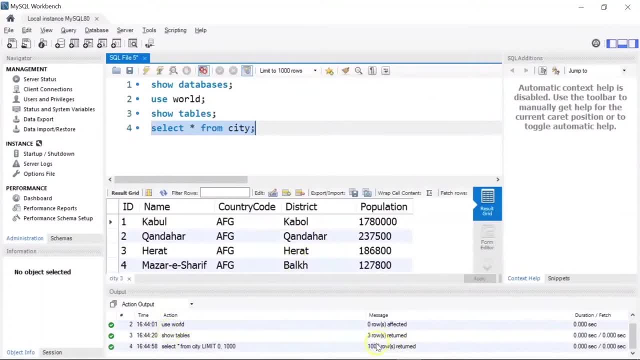 You can see the Message here. It says Thousand rows were returned, Which means There were total Thousand records Present inside the City table. So here You can see One ID column, A name column, This country code. 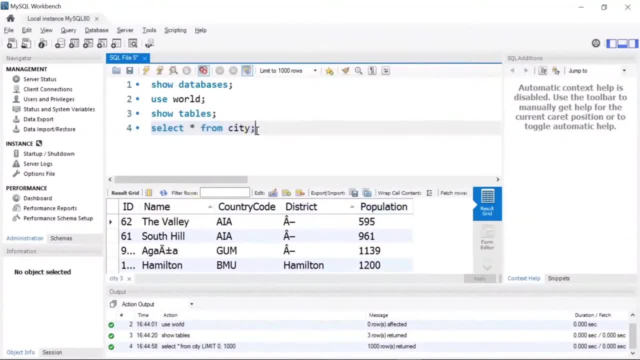 District And population. Alright, Similarly, You can Check the structure of the table By using the Describe command. So I will write Describe And then I will give the Table name. That is City. Now let's just. 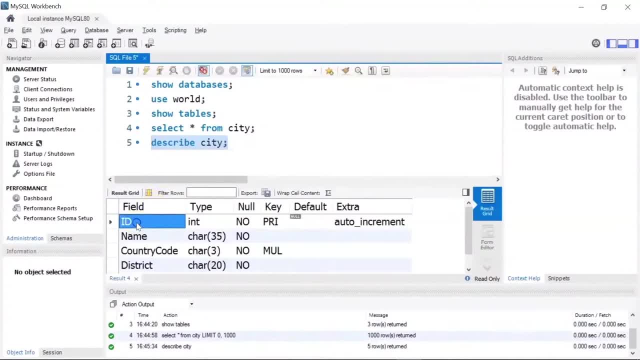 Run it, There you go. The field Shows The column name. So we have ID Name, Country code, District. So district Is character 20.. ID Is an integer. Population Is also integer Null. 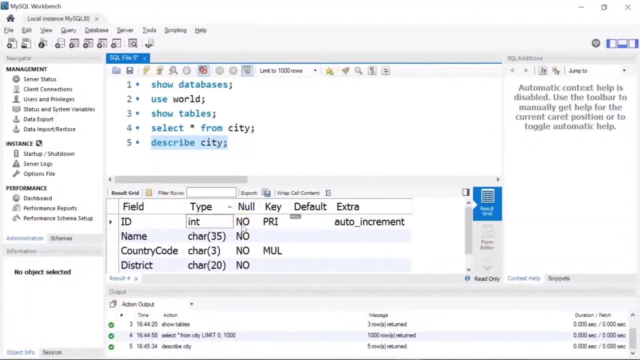 Says Yes or no, Which means If no, Then there are no null values. If it's yes, Which means There are null values In your table. Key here Represents Whether you have Any primary key Or foreign key. 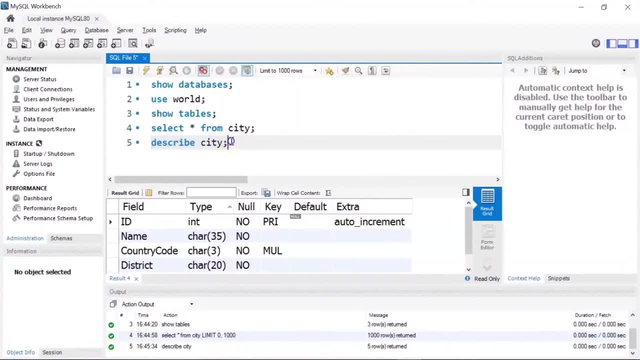 And these are Some extra information. Now let's learn How to create A table In MySQL, So I'll use the Create Database. Let me create A database And I'll name it as SQL Intro. 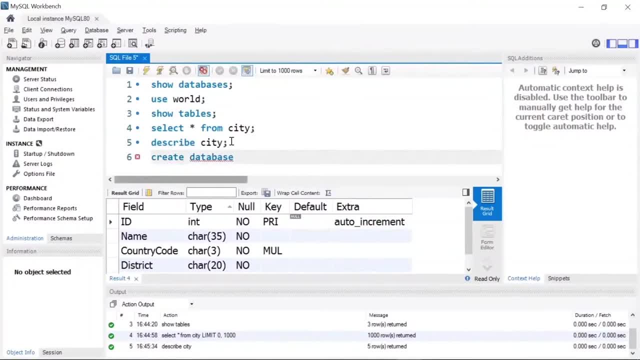 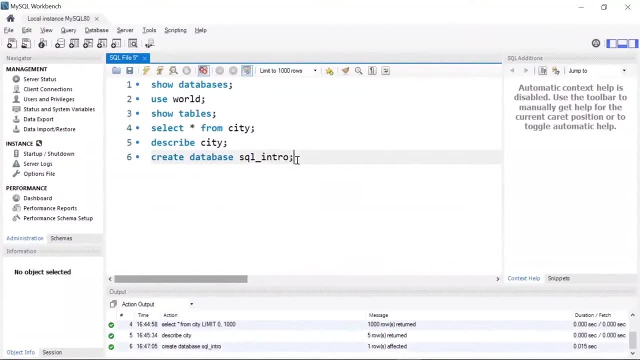 So the command is Create Database And I'll give My database name, That is SQL Underscore Intro. Give a Semicolon And hit Control Enter. You can see I have created. 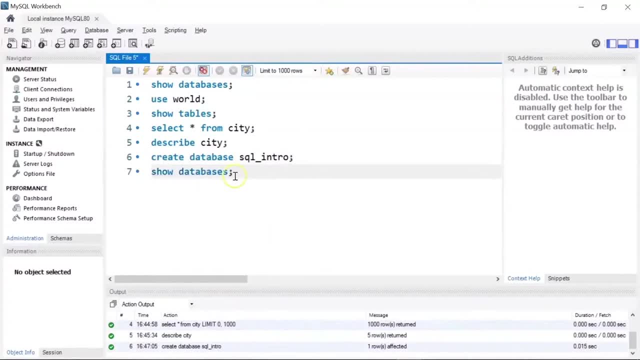 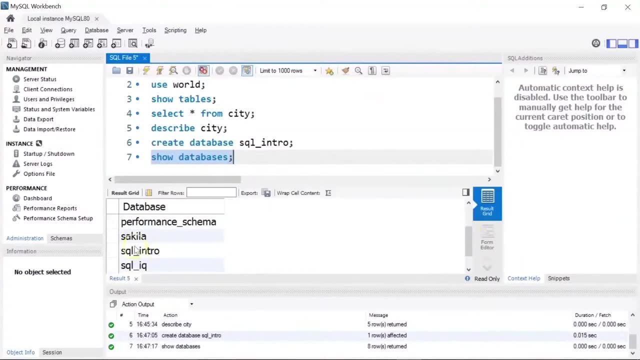 A New Database. Now, If I run This command, That is SQL Intro. If I scroll down, There you go, You can see The name Here: SQL Intro. Okay, Now, Within this: 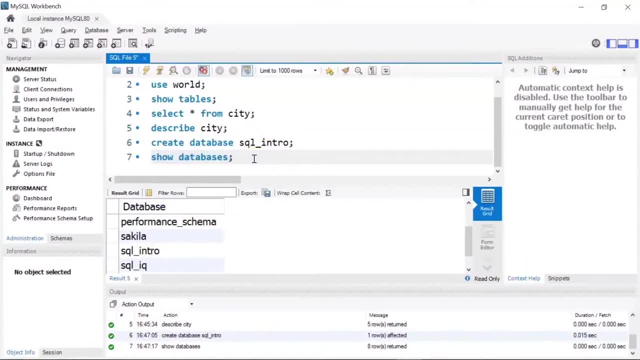 Database. We'll create A table Called Employee Details. Now This Will Have The Details Of Some Employees, So Let Start With The Name That Is Going. 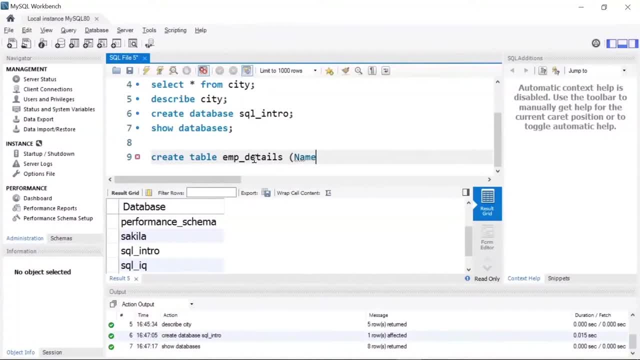 To Be Employee. Underscore Details. Next, The Syntax Is To Give The Column Names. So My First Column Would Be The Name Okay, Next I 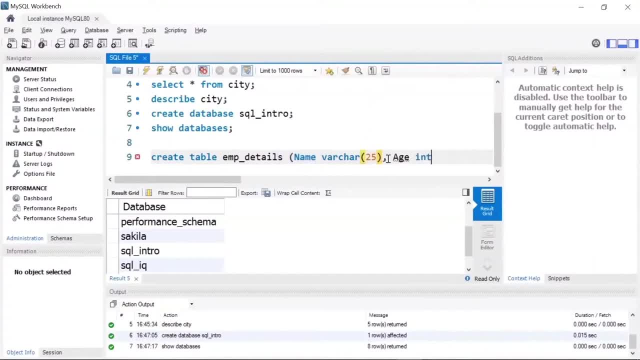 Also Want The Age Of The Employee. Now, Age Is Always An Integer, So I'll Give Int. Okay, Then We Can Have The Gender Of. 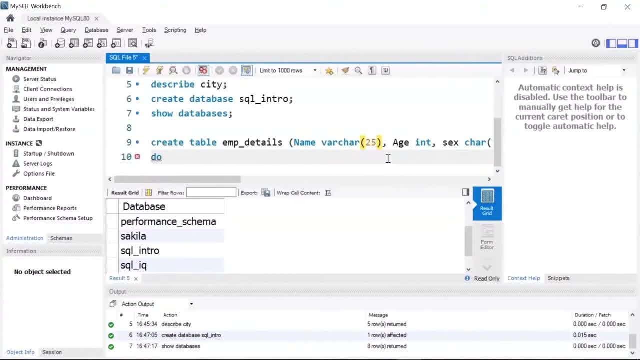 The Date Of Join Or Doj, And This Is Going To Be Of Data Type Date. All Right. Next We'll Have The City Name. That 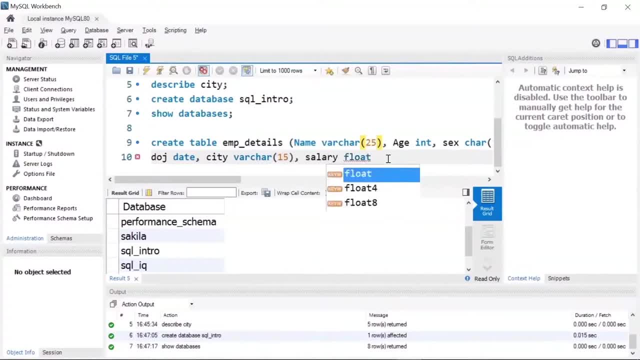 Is The City To Which. Decimal Numbers As Well. Now I'll Give A Semicolon, All Right, So Let Me Just Quickly Run Through It. 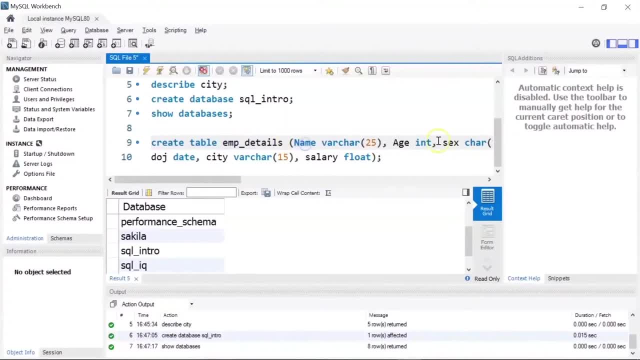 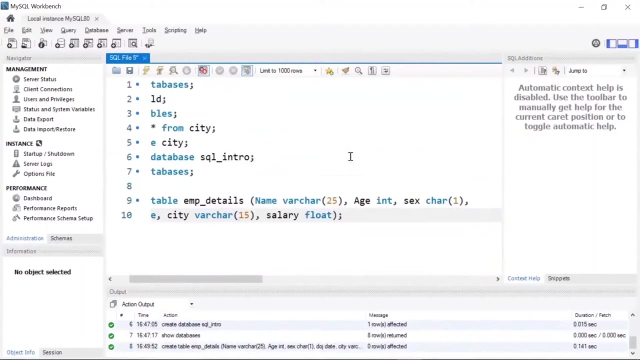 So First I Wrote My Create Command, Then The Table. For Each Of The Columns We Also Give The Data Type. All Right, So Let 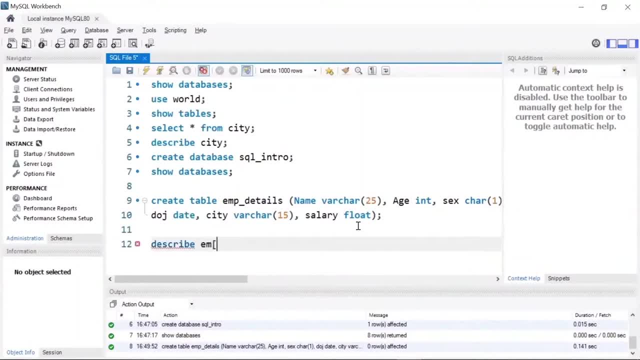 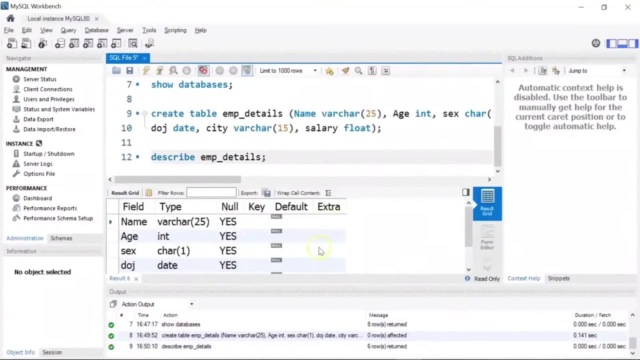 Me Just Run It Okay. So Here You Can See. We Have Successfully Created The Data Types. Null Represents If The Table Can Accept Null Values. 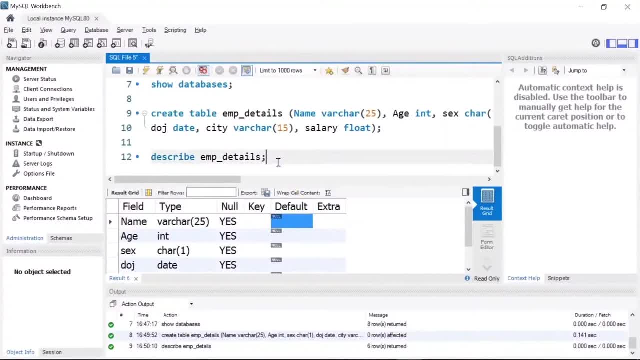 Or Not, And These Are Basically Empty And We Haven't Set Any Default Constraint. All Right, Moving, All Right. So If You See This, So 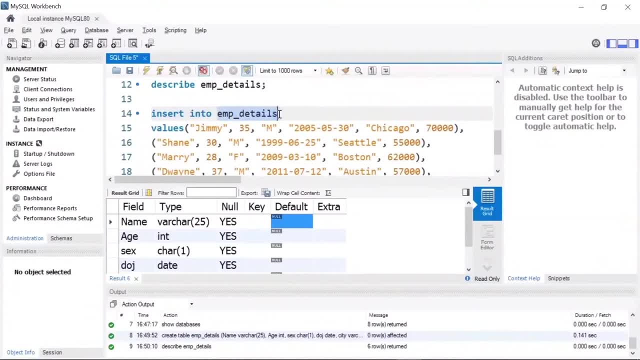 We Have Used An Insert Into Statement Or A Command Followed By The Table Name, That Is, EMP Details, Then This Line. Next We Have 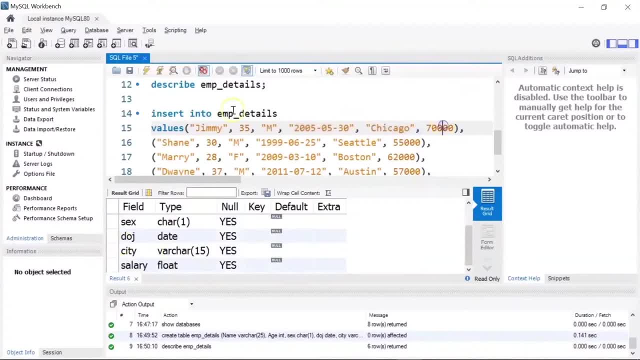 The City To Which The Employee Belongs To, And Finally We Have The Salary Of The Employee. So This Particular Information Represents One Record Or 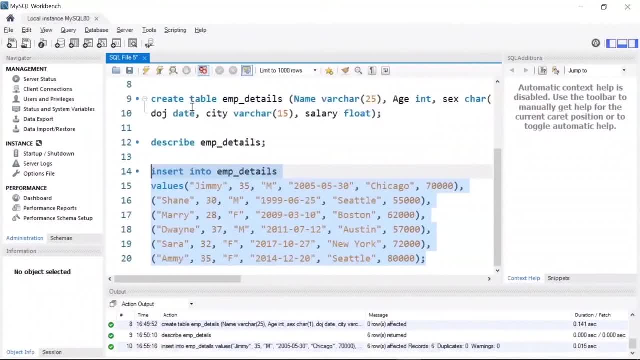 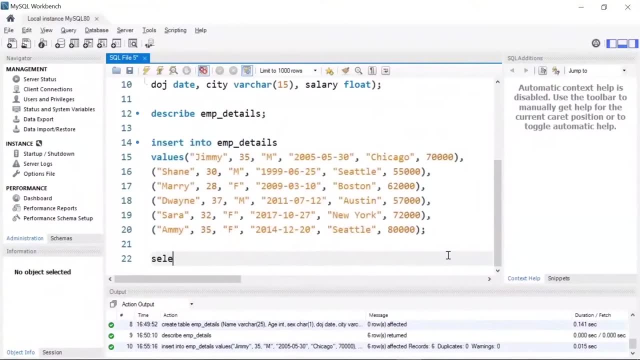 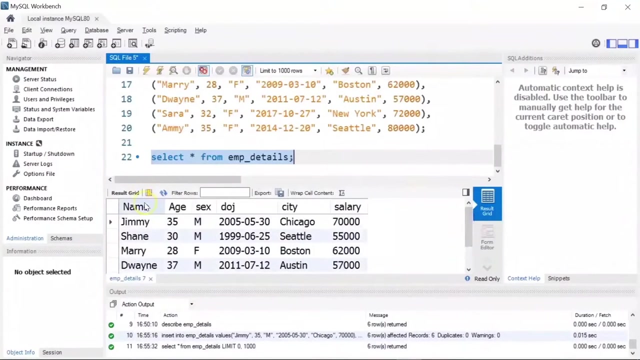 A, The Table That You Have Created. You Can See We Have Successfully Inserted Six Records. Now To Display The Records, Let Me Use The 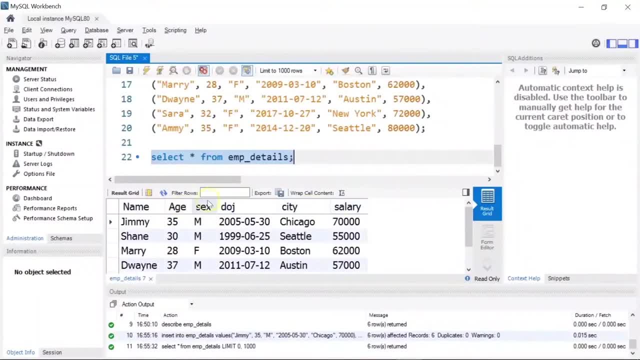 Select Statement. So I'm Using, And These Are The Values That You Can See Here. Moving Ahead Now, Let's Say You Want To See The. 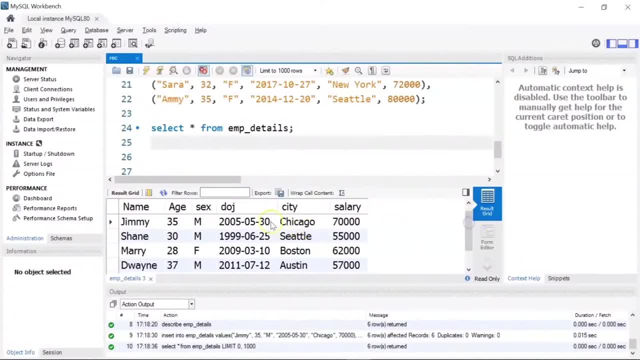 Unique City Names Present In The Table. So In The Table I Will Repeat It Again. So I Only Want To Print The Unique Values. So 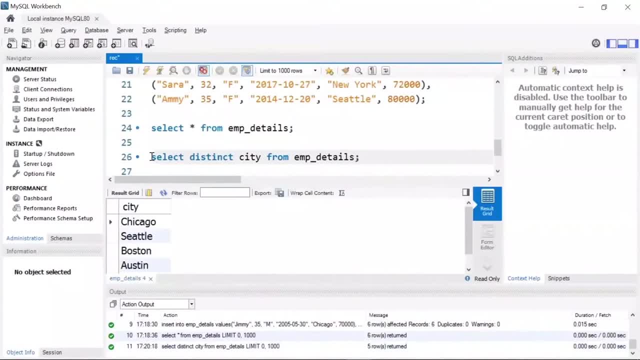 For That I Can Write My Select Statement As Select Distinct. Then I Will See How You Can See It Works. Now Let's See How. 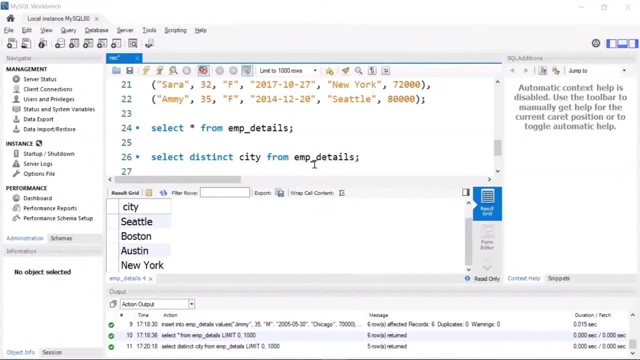 You Can Use In Build Aggregate Functions In SQL. So Suppose You Want To Count The Total Number Of Employees, I'm Going To Use Their. 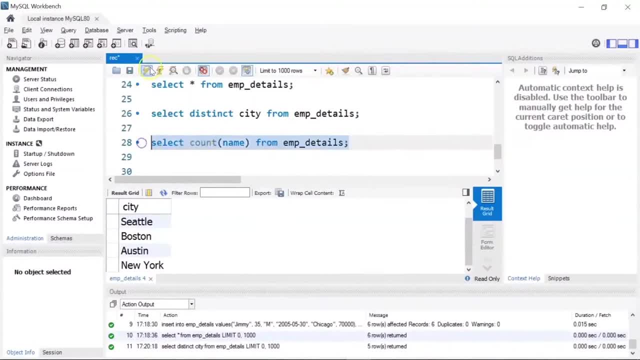 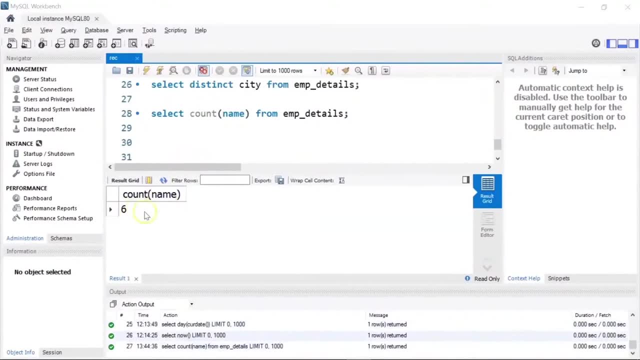 Name Inside The Brackets From Employee Underscore Details. Now, If I Run This, This Will Return The Total Number Of Employees, So You Can. 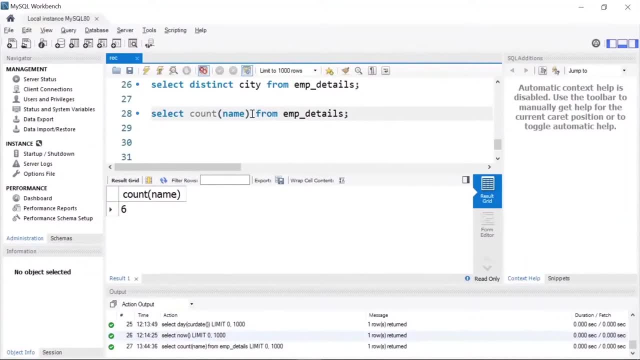 Give An Alias To The Resultant Output. So Here I Can Write, Select Count Of Name And Use An Alias As As I Can Give. 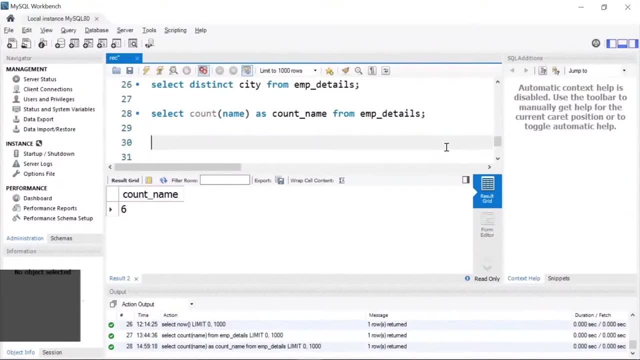 The Total Sum Of Salaries. You Can Use Another Aggregate Function, Called Sum, So I'll Write My Select Statement, And This Time Instead Of Count. 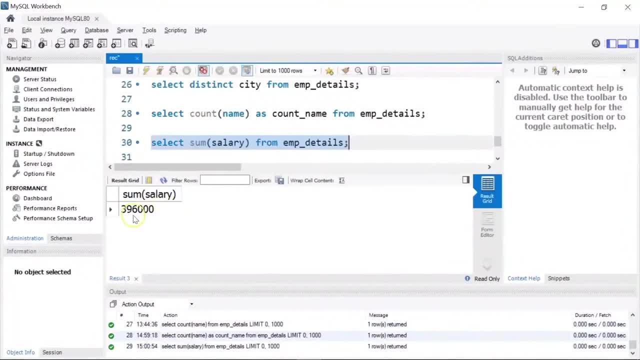 I'm Going To Write. So, Basically It Adds Up All The Salaries That Were Present In The Salary Column. Now Let's Say You Want. 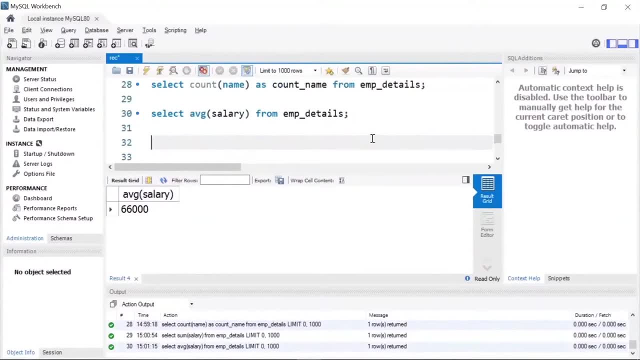 To Find The Average Salary. So Instead Of Selecting All The Columns For Example, Like You Saw Here, The Star Represents That We Want To. 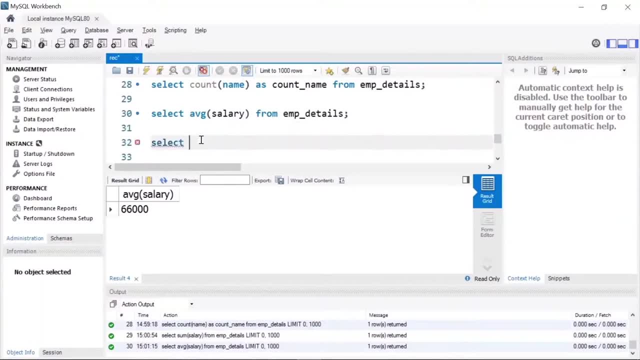 See All The Columns From The Employee Details Table. Now, Suppose You Find The Employee Details, So This Will Result In Displaying Only The Name. 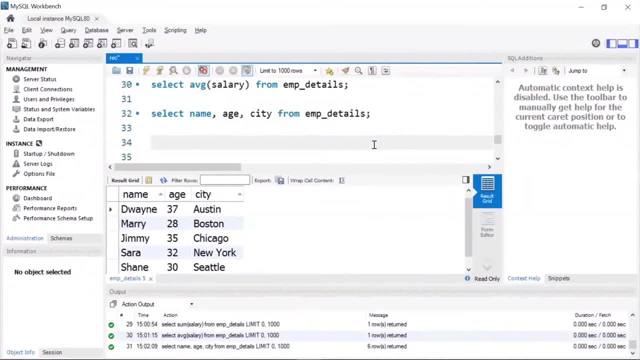 Agents City Column From The Table. If I Run It, There You Go. It Has Given To Find The Employees With Age Greater Than 30.. 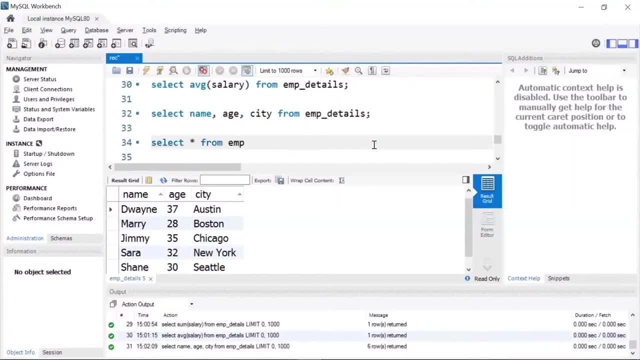 In This Case, You Can Use A Wear Clause. So Let Me Show You How To Do It. I'll Write. It Will Give Me The. 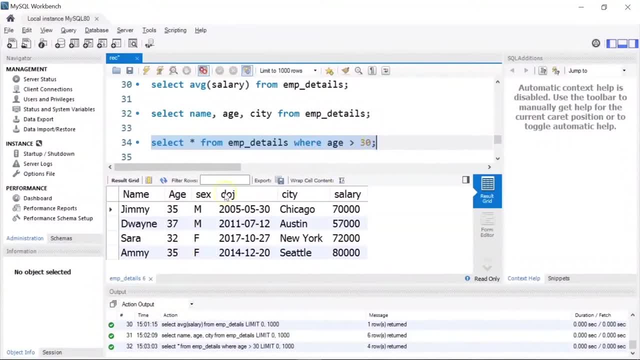 Output Where The Age Is Only Greater Than 30. So It Excluded Everything That Is Less Than 30. So We Have Four Employees. Whose? 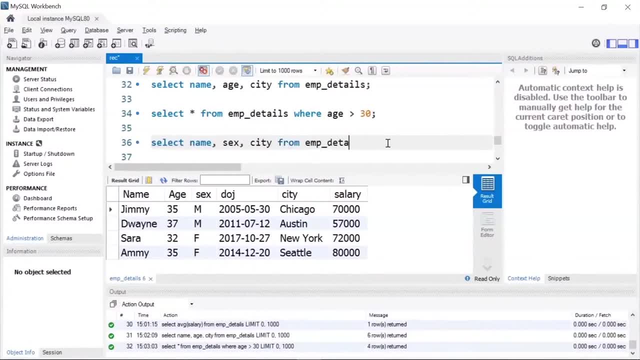 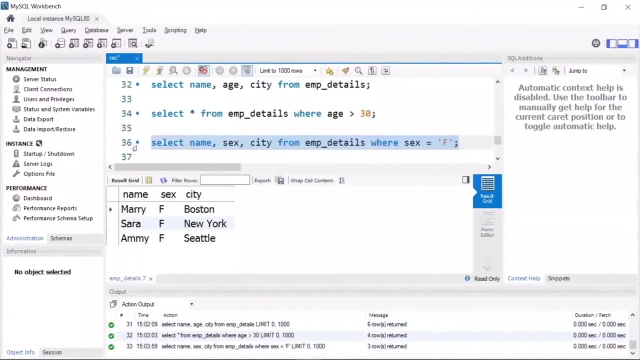 City From My Table. That Is Employee Details Where I'll Give My Column Name. That Is Sex Is Equal To, Since I Want Only The. 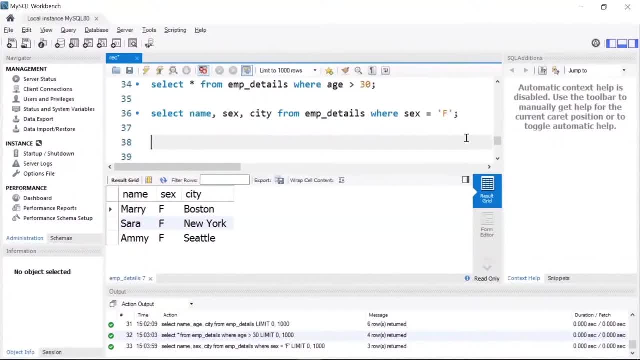 Female Employees, I'll Give My Name To The Employee. In This Case, You Can Use The Or Operator. Now The Or Operator In SQL Displays. 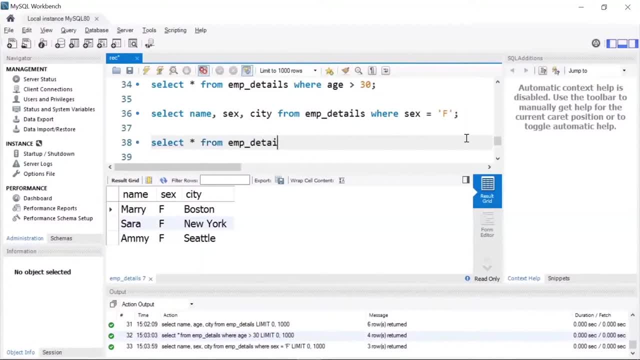 A Record. If Any Of The Condition Separated City Equal To, I'll Give My City Name As Chicago, And Then I'm Going To Use. 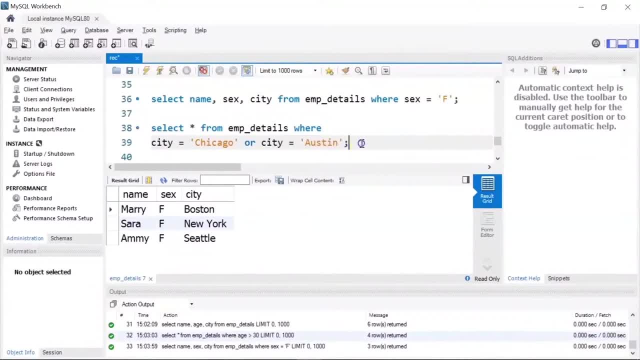 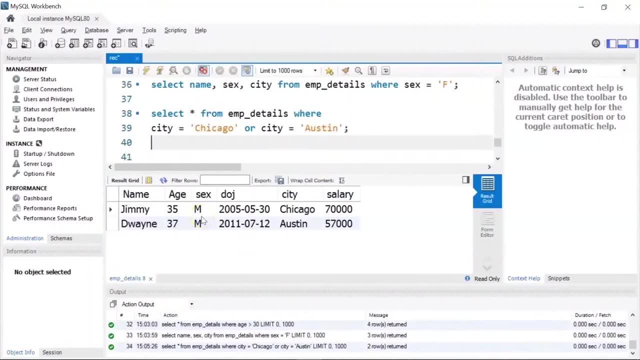 The Or Operator Or City Equal To. I'll Write Austin. I'll Give A Question. Now There Is Another Way To Write The Same SQL Query. 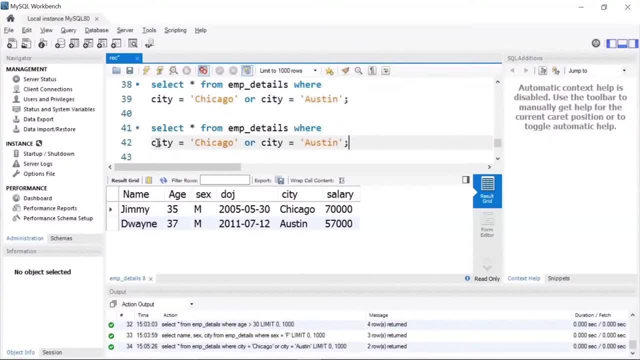 So You Can Use An In Operator To Specify Multiple Conditions. So Let Me Just Copy This. I'll Give My City Names As Chicago And. 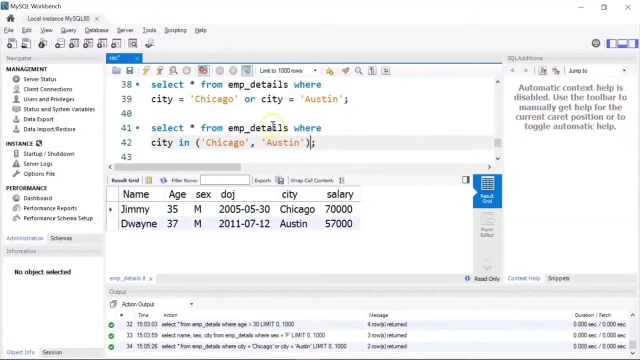 I Want Austin. So I'll Give A Comma And Write My Next City Name. That Is Austin. So This Query Is An Range: The Values. 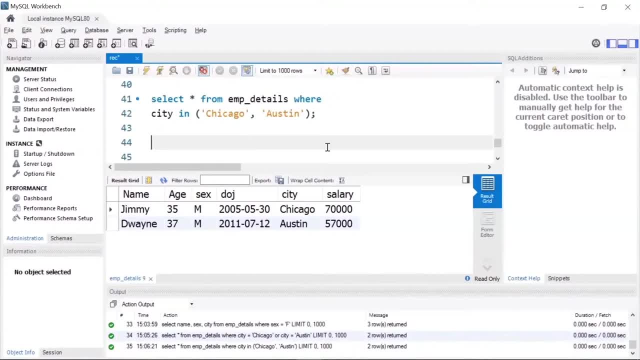 Can Be Numbers, Text Or Dates. Suppose You Want To Find The Employees Whose Date Of Join Was Between 1st Of December 2010.. 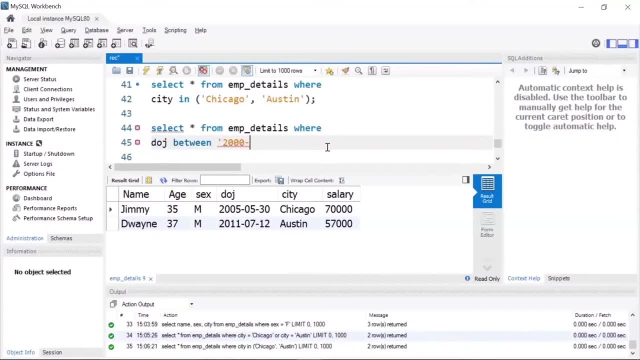 So Let Me Give Two Date Values. That Is 1st Of Jan 2000.. And I'll Give My Second Value, The Date Value That 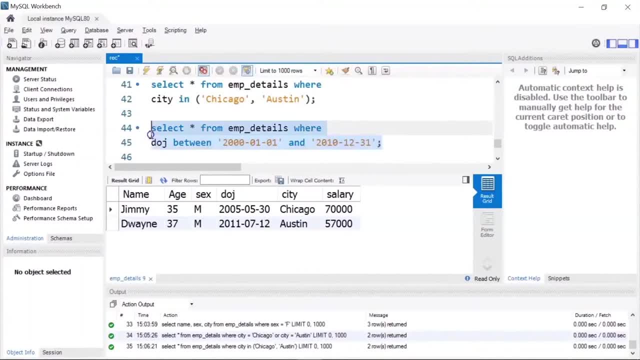 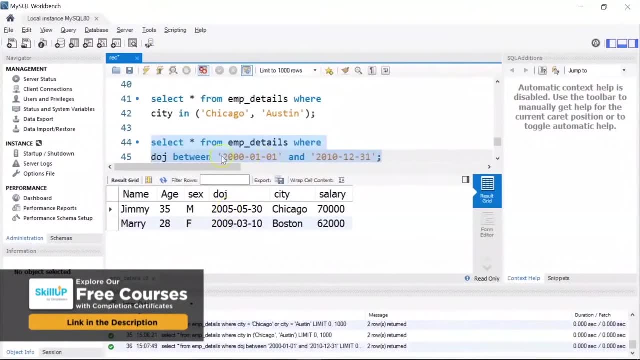 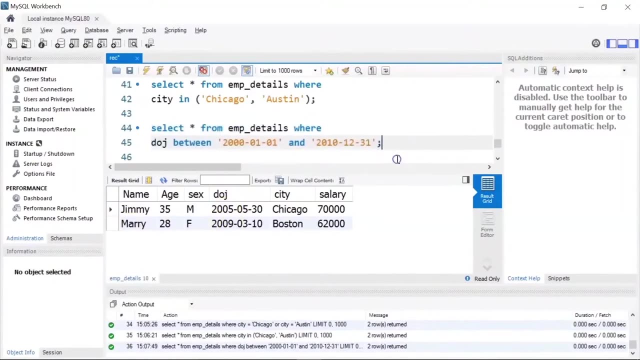 Is 31st Of December 2010.. So Every Employee Who Is Who Had Joined Between 2000. And 2010.. So We Have Jimmy And 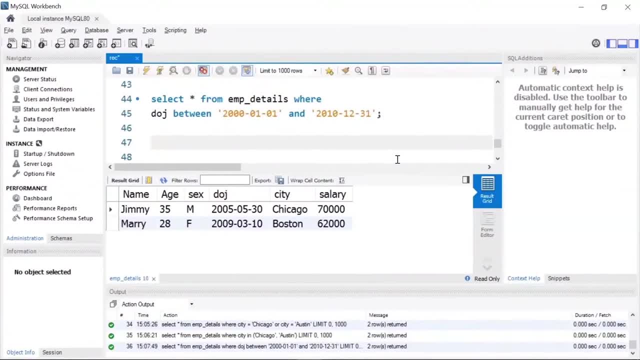 Mary Here, Who Had Joined In 2005.. And 2009.. Respectively, All Right Now In Where Clause Employee Details Table, Where I Want The. 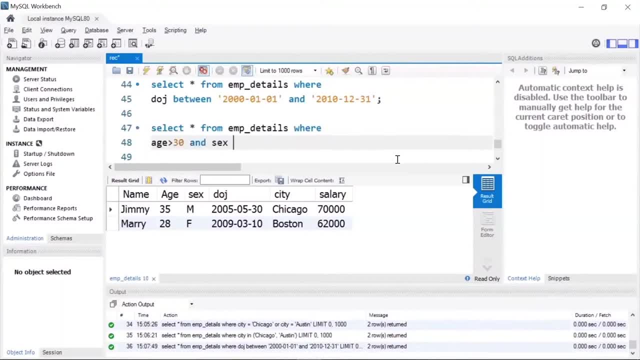 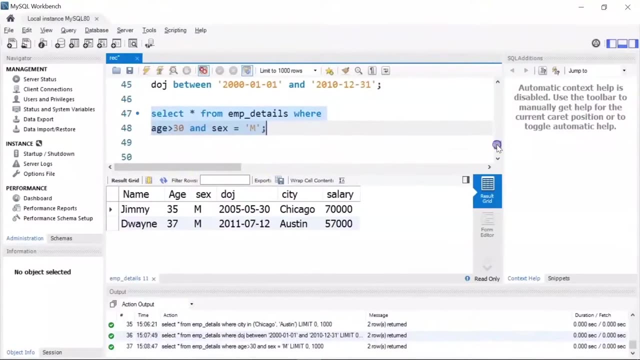 Age To Be Greater Than 30. And I Want Sex To Be Male. All Right, So Here You Can See: I Have 30. Now Let's. 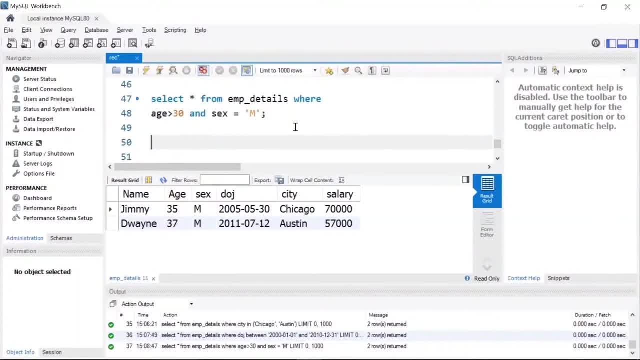 Talk About The Group By Statement In SQL. So The Group By Statement Groups Rows That Have The Same Values Into Summary Rows, Like For Example. 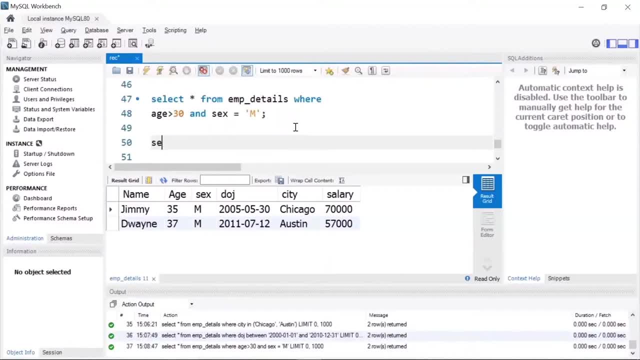 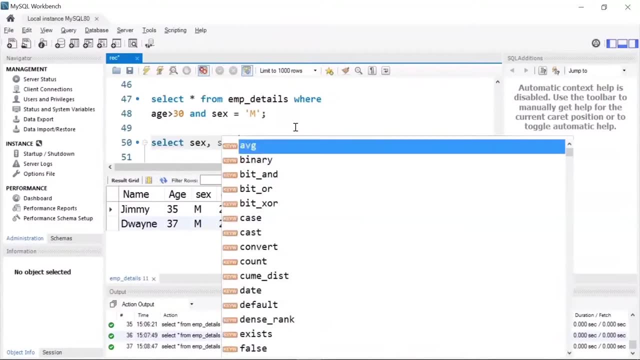 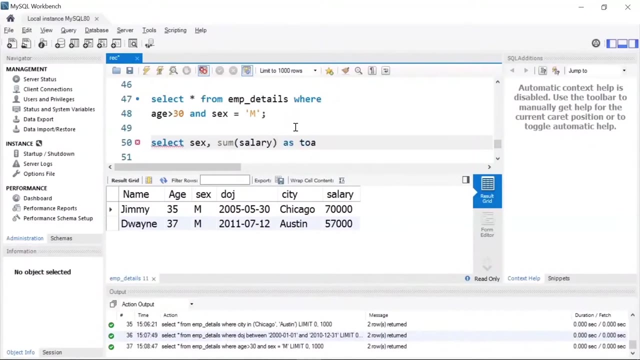 Gender. So In This Case You Can Use The Group By Clause. So I'll Write: Select, Let's Say Sex Comma I Want To Find. 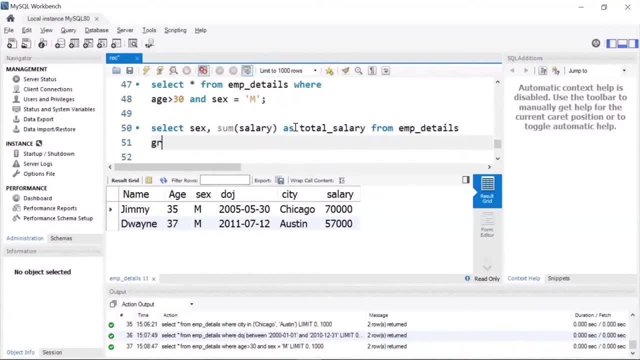 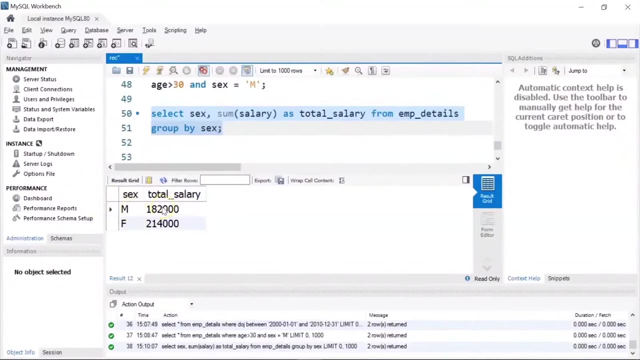 The Total Sum Of Salary. As Okay, Let Me Run It. There You Go. So We Have Two Genders, Male And Female, And Here You 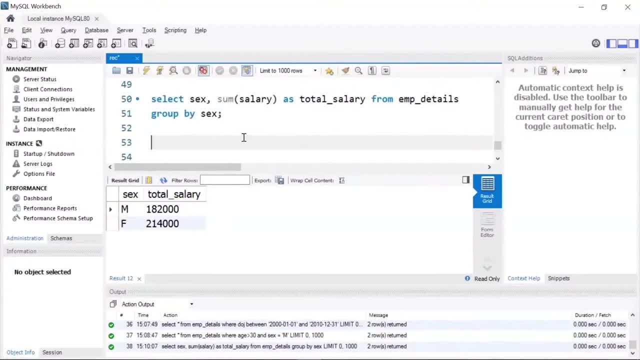 Can See The Total Salary. So What This Is. Assigning Order By Default. To Sort The Records In Descending Order, You Can Use The Desc. 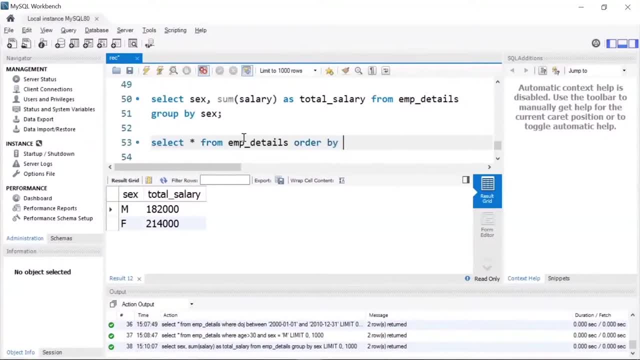 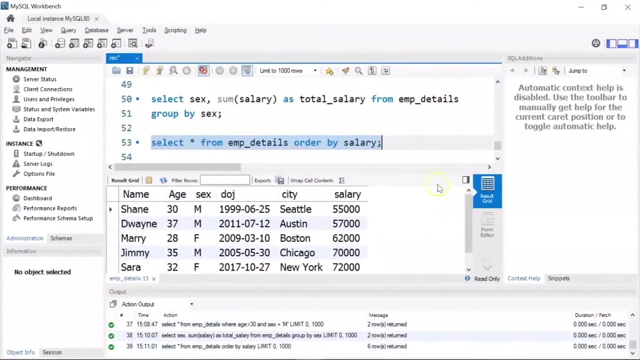 Keyword. So Let's Say I Want To Sort My Employee Details Table Of Their Salary, Which Is By Default. You Can See The Salary Column. 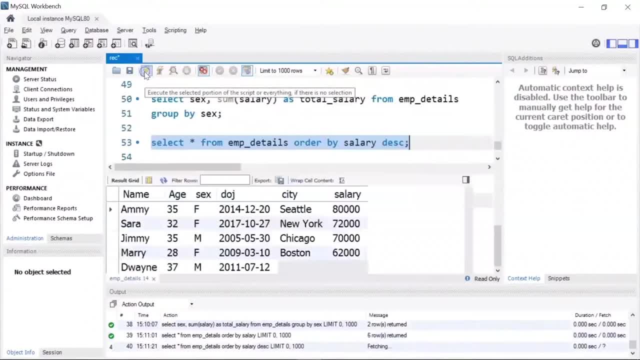 Is Sorted In Ascending Order. Now Suppose You Want To Sort The Salary Column And Display Of Your Employee And Do An Addition Operation. Let's. 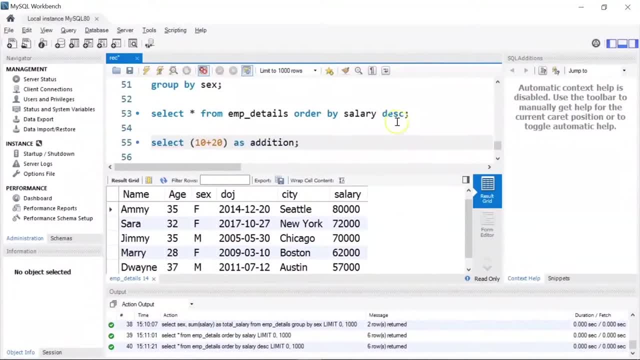 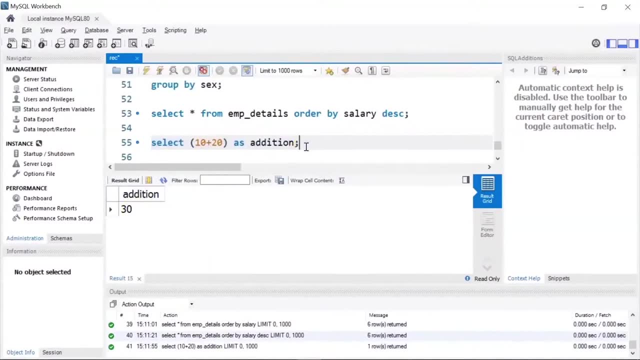 Say Ten Plus Twenty, And I'll Given Alias Name As Addition. If I Run This, It Will Give Me The Sum. Let's Run It, You. 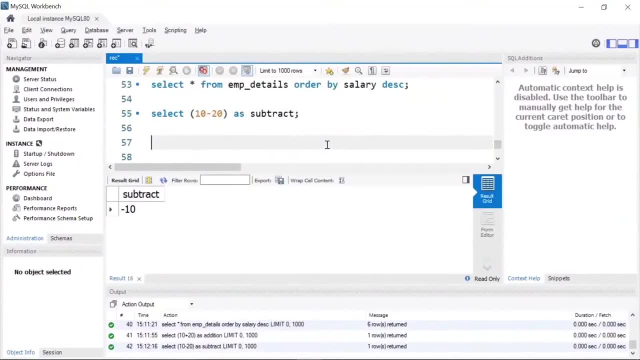 Get Minus Ten. Now There Are Some Basic In Build Functions. There Are A Lot Of In Build Functions In SQL, But Here I'll Show. 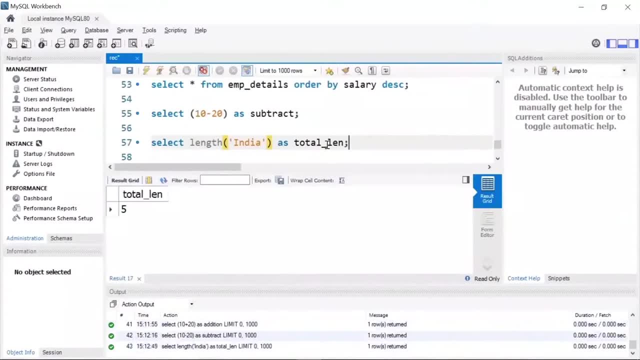 You The Total Length. If I Run It, You See Here, It Returns Five, Because There Are Five Letters. In India There's Another Function Called 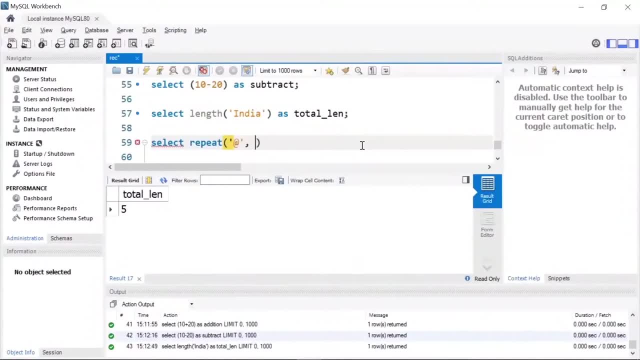 Repeat. So Let Me Repeat This Character For Ten Times: Close The Bracket And Let's Run It. You Can See Here In The Output It: 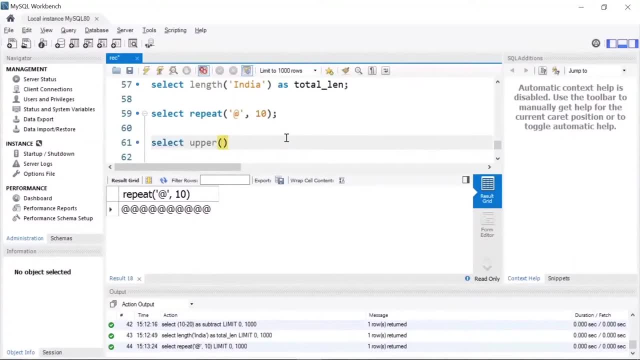 Has Printed At The Rate Ten Times. You See, It Returns To The Alias Name. If I Run This, See, My Input Was Capital, I And. 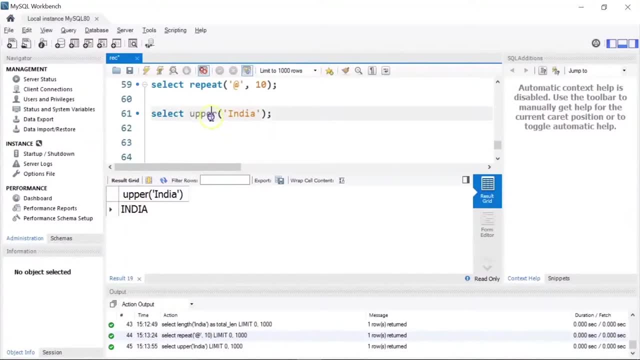 Everything Else Was In Small Letter In The Output. You Can See. This Time Everything Is In Upper Case. If I Run It, It Converts India. 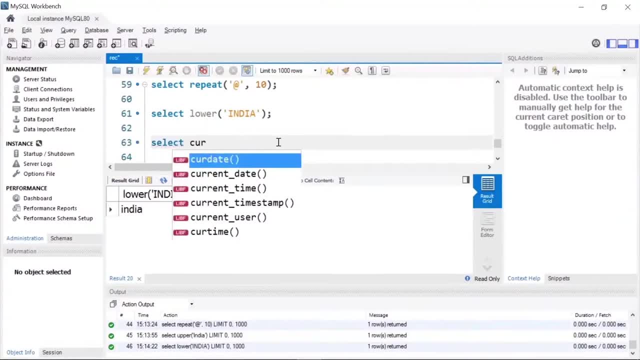 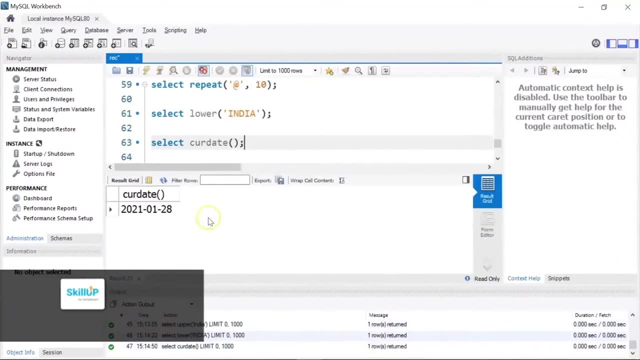 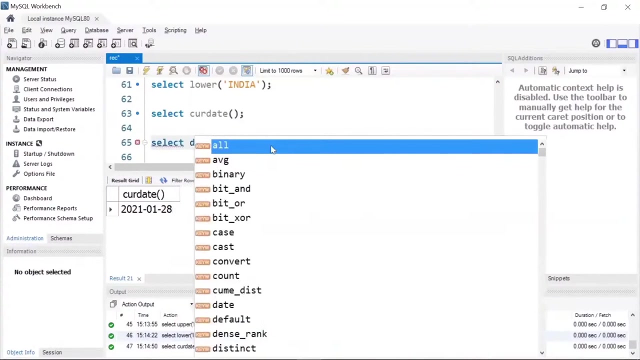 To Lower Case. Now Let's Explore A Few Date And Time Functions. Let's Say You Want To Extract The Day From A Date Value, So 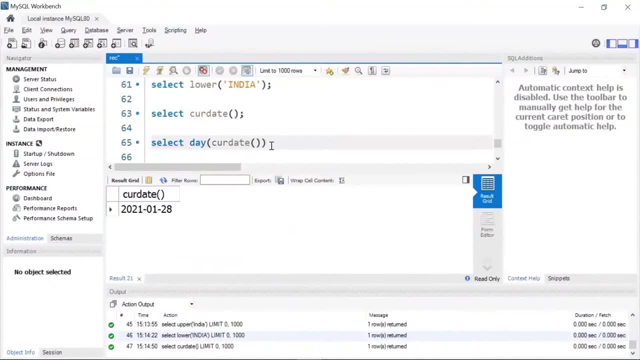 You Can Use The Day Function. Let's Say Use Day And I Want To Find The Day From My Current Date And Time You Can. 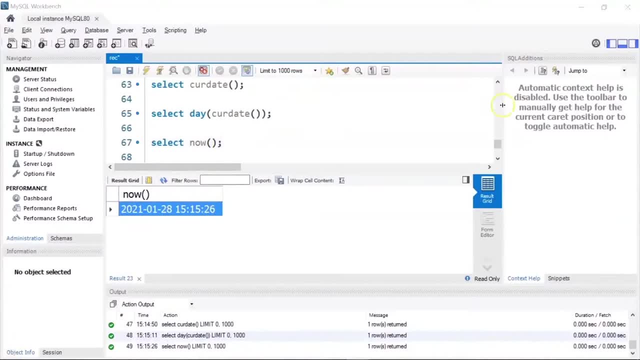 See, This Is The Date Value, And Then We Have The Current Time, All Right, And This Brings Us To The End Of Our Data. 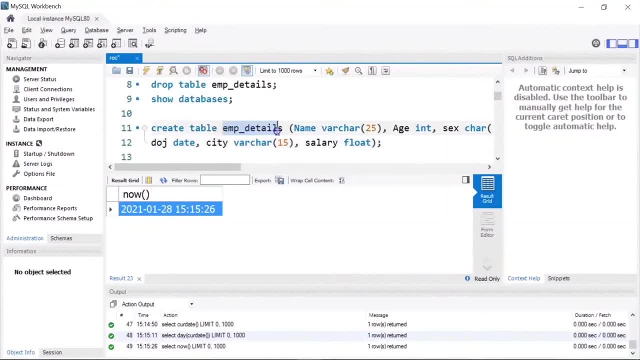 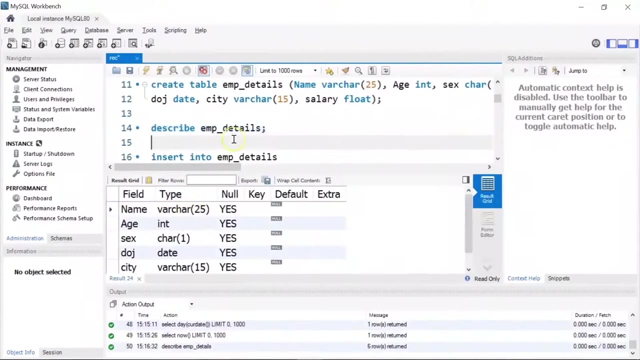 So Let's Use That Database. And Then We Created This Table Called Employee Details, With Column Names Like Name Integer: The Sex Date Of Joint. 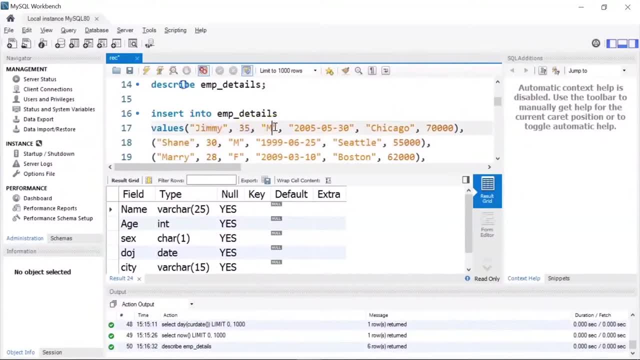 City And By Name, The Age, The Gender, The Date Of Joint The City To Which The Employee Belongs To And The Salary Of The 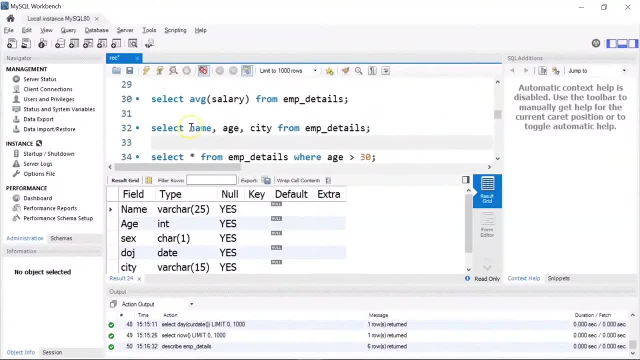 Employee. Then We Saw How You Learned How To Use Where Clause. Then We Used An Or Operator. We Learned About In Operator, The Between Operator. 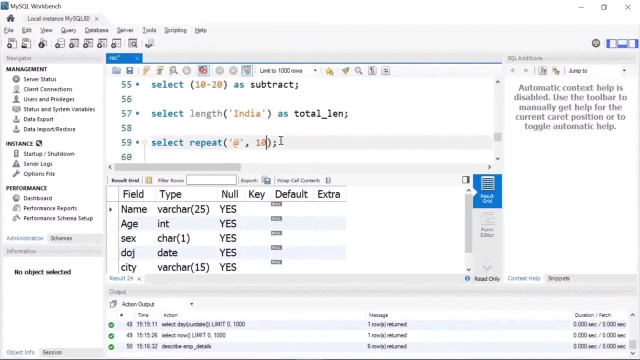 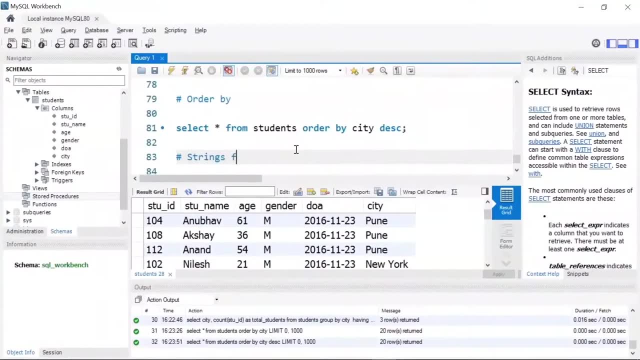 Then We Used An And Operator To Select Multiple Conditions. So I Have Given A Comment String Functions. First, Let's Say You Want To Convert. 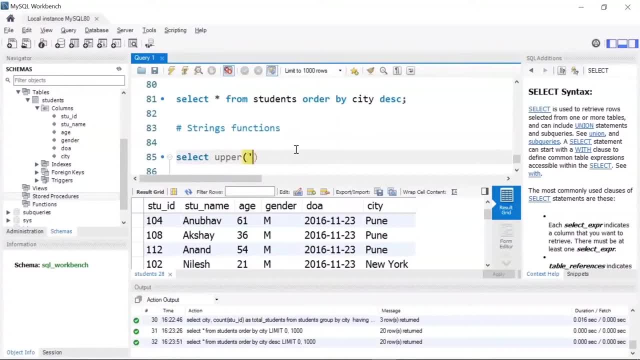 A Certain String Into Uppercase So I Can Write: Select The Function I Use. I Will Give A Semicolon And Let's Run It. 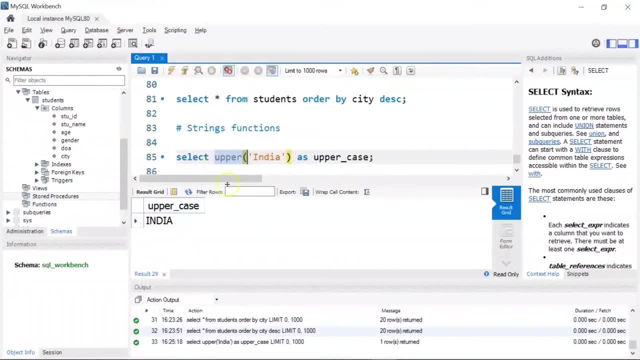 There You Go. So My Input Was In Sentence Case And, Using The Upper Function, We Have Converted Everything Into Lower Case. Now, Of Course, I 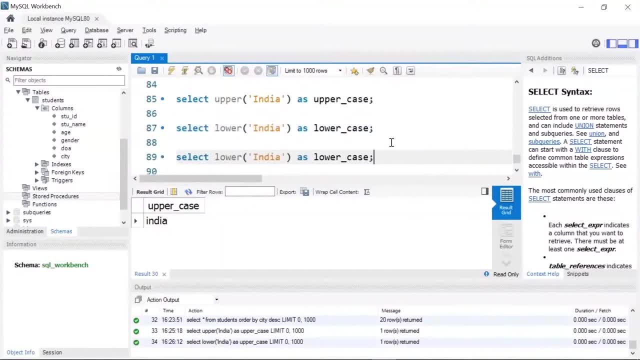 Need To Change The Alias Name To Lower Case. Now, Instead Of Using Lower As The Function, There Is Another Function That My Now Moving On. 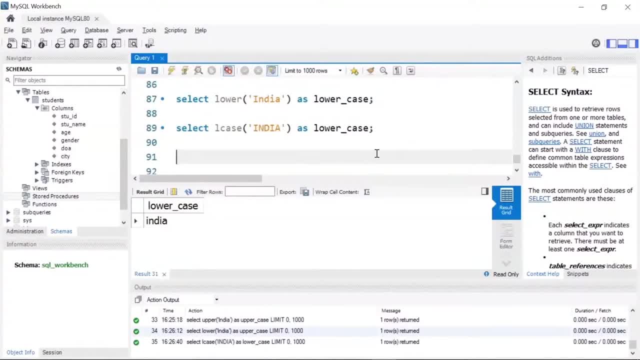 Let's Say You Want To Find The Length Of A String. You Can Use The Character Length Function. I'll Write Select. Use The Function Character. 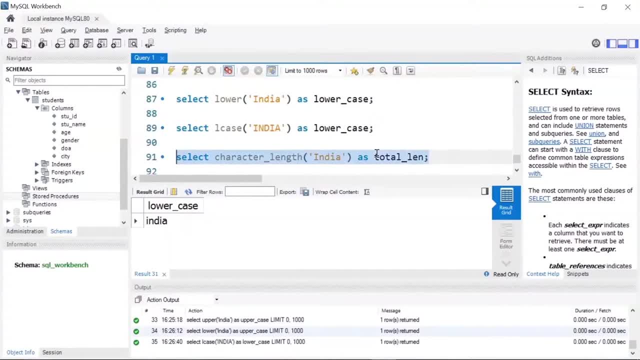 Length. This Time I'm Going To Hit Control Enter To Run My Sql Command. There You Go. It Has Given Us The Right Result, Which. 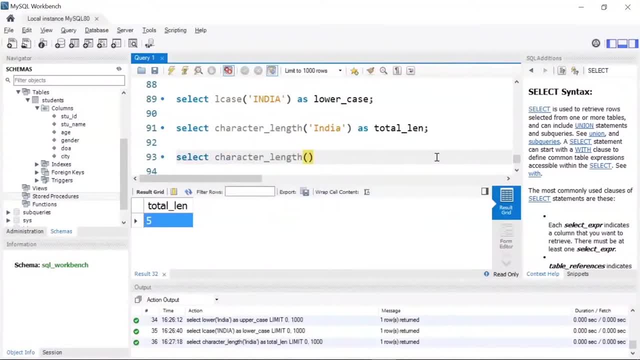 Is 5. Because India Has As To Underscore Name And You Can Give The Same Alias Name, Let's Say Total Length, And Then You 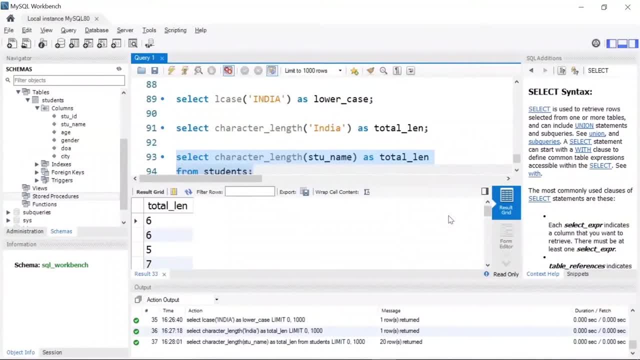 Can Write From Table Name, That Is Students. If I Run Student Names So That We Can Compare Their Length, All Right, I'll Run This. 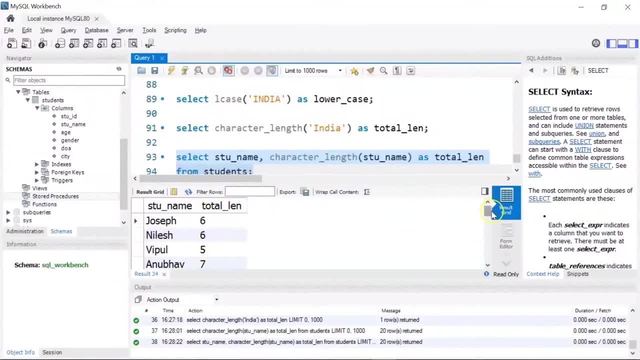 Again, And Now You Can See The Result. So Joseph Has 6. Characters Niles Has Now. Instead Of Using This Character, Length, You Can Also. 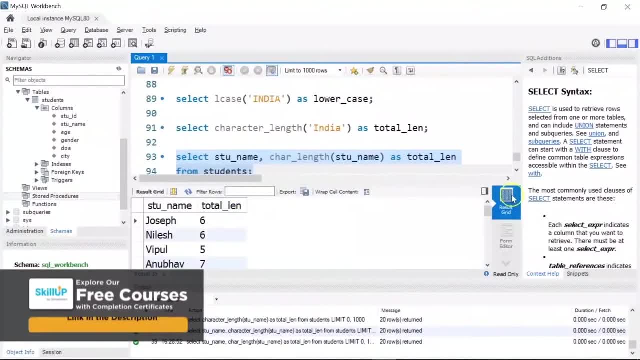 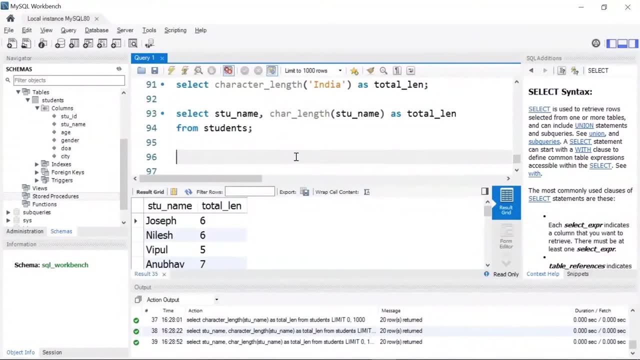 Use The Function Car Length, It Will Work The Same Way. Let's See The Result. There You Go. It Has The Function Con Cat In. 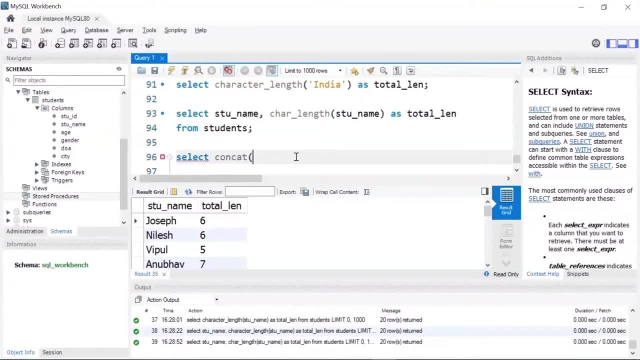 It. The Function Is Actually Con Cat And I'm Going To Pass In My String Values. Let's Say India Is In Asia. Let's Run. 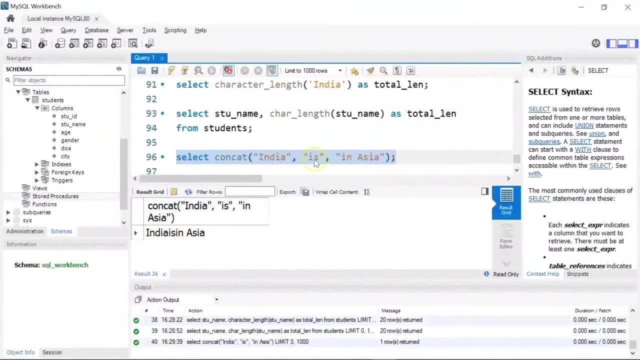 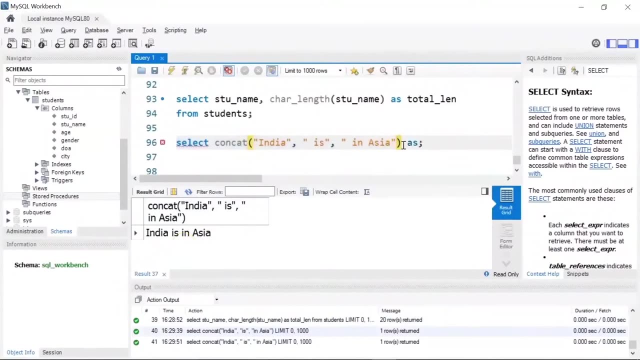 This Can See Here. It Has Concatenated Everything. Let Us Make It More Readable. I'll Give A Space In Between So That You Can. 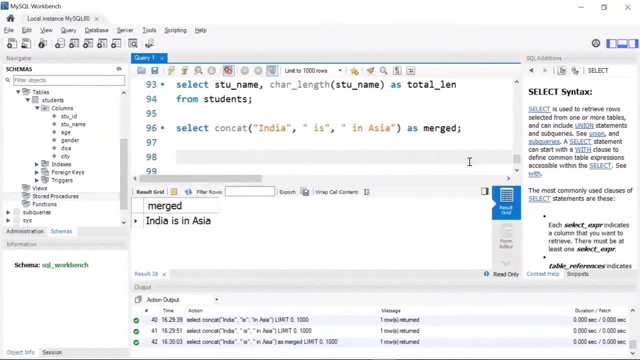 Read It Clearly. Now, This Is A Student Table. Let's Say I Want To Return The Student ID Followed By The Student Name, And Then 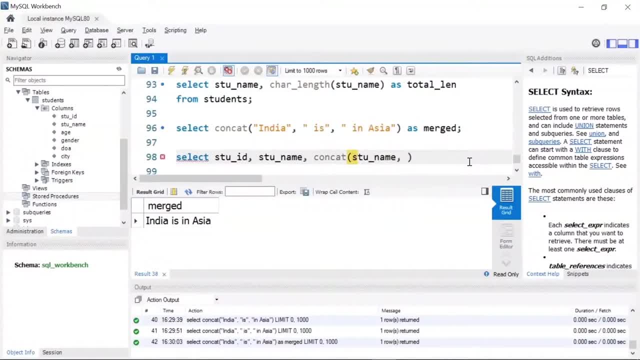 I'm Going To Merge The Student Name Followed By A Student From My Table, That Is Students. Let's See How This Works, Okay, You. 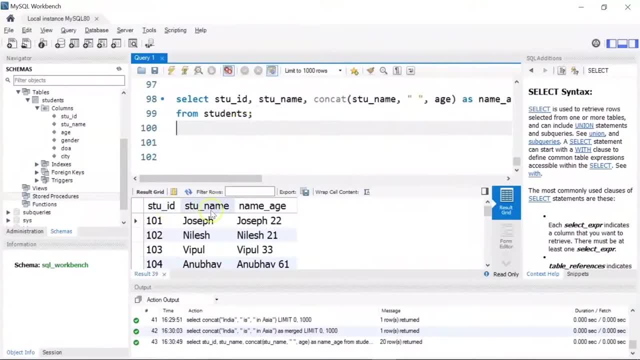 See Here The Result Is Very Clear. We Have The Student ID, The Student Name And The Student And The Result. Cool, Now Moving Ahead, Let's. 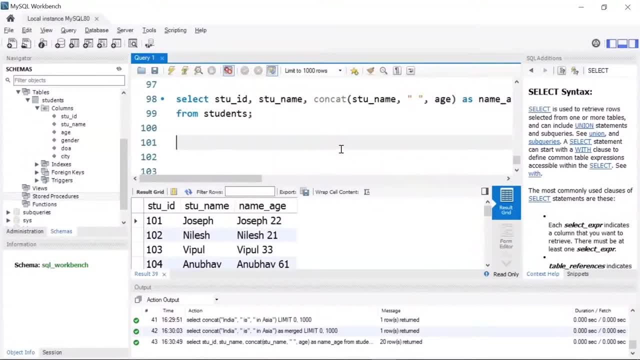 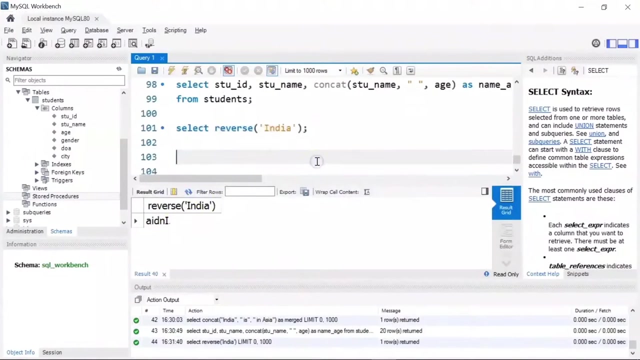 See How The Reverse Function Works In My SQL. So The My SQL Reverse Function Returns A String With The Student Name And The Student Name. 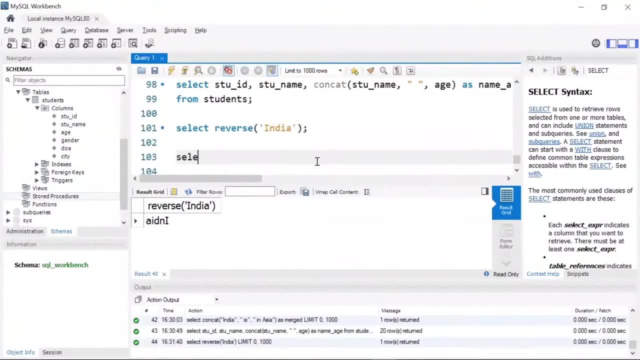 And The Student Name Returns To The Student And The Student Name From My Table That Is: Students, Let's Run. It Gives You Okay Now. 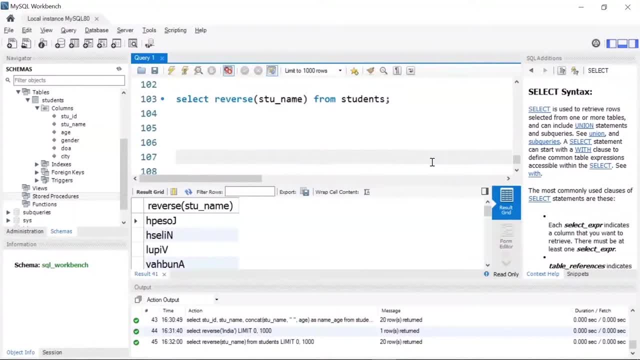 Let's See What The Replace Function Does. So The Replace Function Replaces All Accurances Of A Sub String Within A String Within A New. 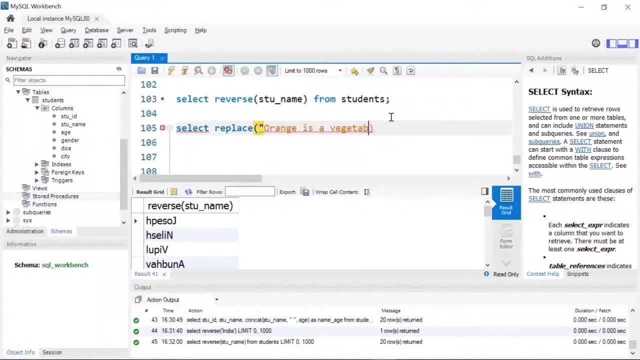 Sub String, Which Is Ideally Incorrect. I Am Purposely Writing This So That I Can Replace The Word Vegetable With Fruit. Okay, So What This? 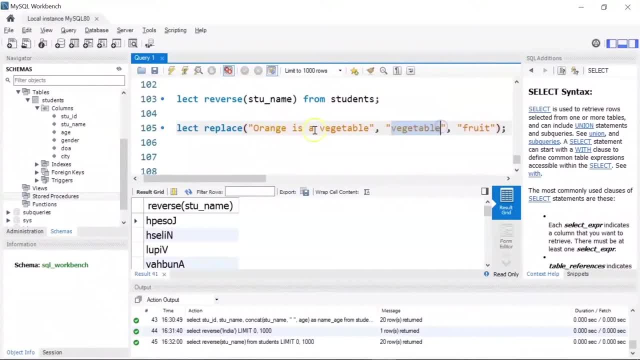 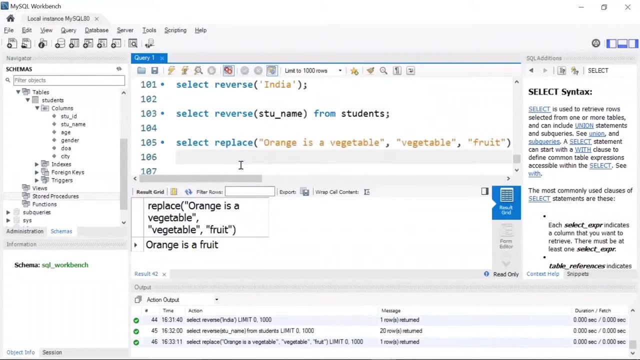 Replace Function Does, Is It String? And It Is Going To Replace My Word Vegetable With Fruit. Let's Run It And See The Output There. 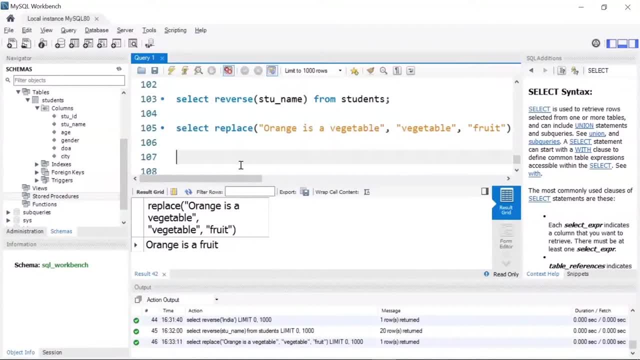 You Go. Now, This Is Correct. Which Is Orange Is Red, It Is Red. So Let's See What This Is Going To Replace The Fruit. 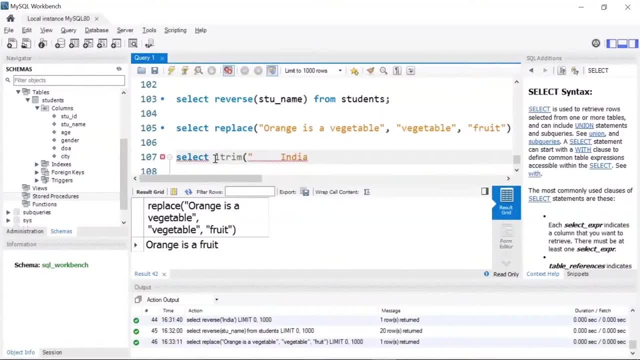 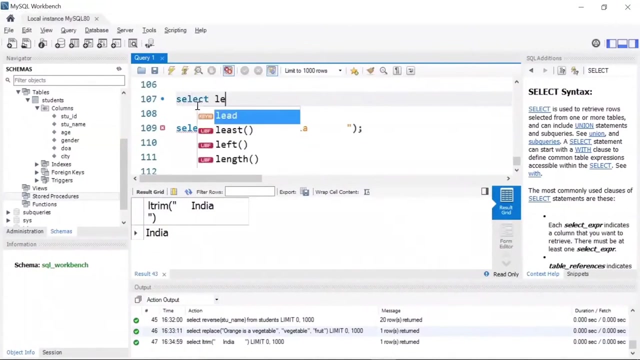 Vegetable With Fruit. It Is Correct. This Is Correct. Now Let's See How The We Run This. It Gives Me India, Which Is Fair Enough. 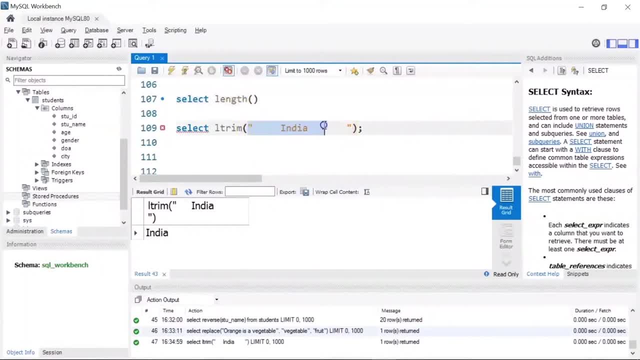 But Before That, Let's First Find The Length Of My String. So I'll Use My Length Function Here. Okay, So The Entire String Is 17.. 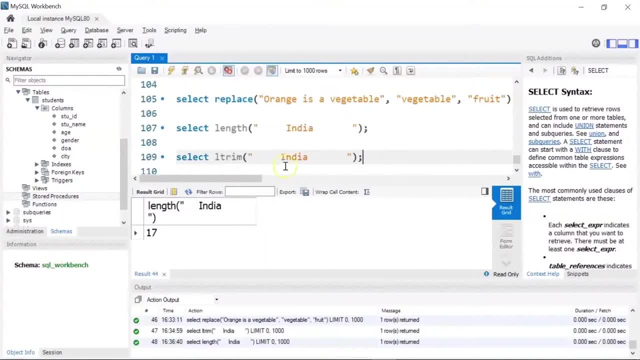 Characters Long, Or The Length Of The String Is 17.. Now Say I Use L Trim On My Same String What It Can See Here. 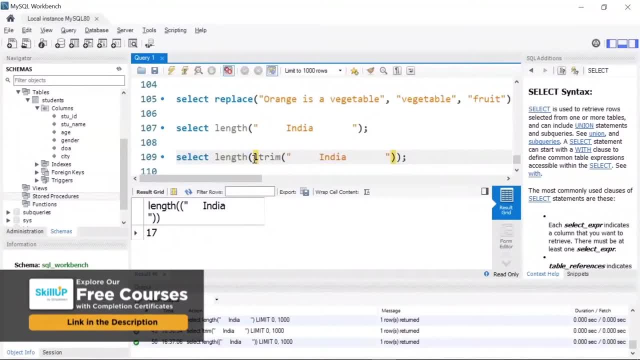 Now It Says 17. And I'm Going To Use L Trim. Let's See The Difference It Gives Me 12. The Reason Being It Has: 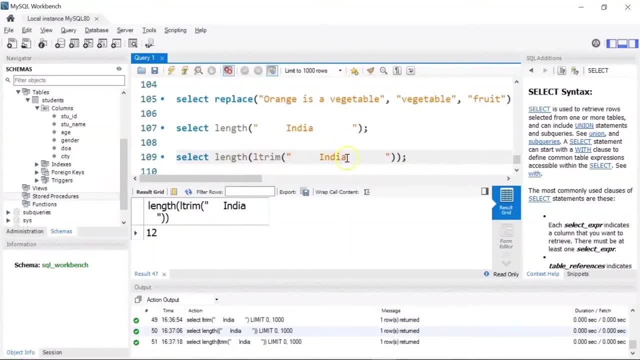 Deleted. 5. Trailing Spaces From A String Trailing Spaces Are These Spaces? When You Use Left Rim, It Deletes The Leading Spaces, Which Is 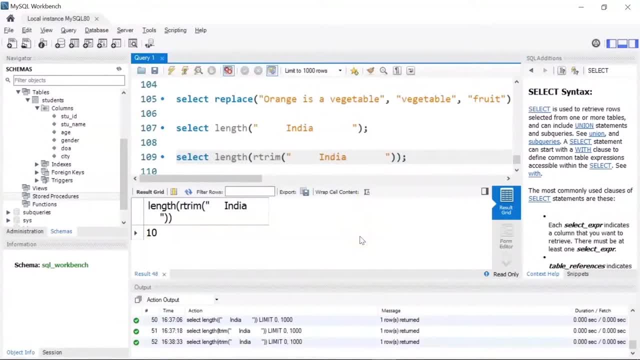 This. Now Let Me Just Replace L, 4., 5., 6. And 7.. Cool, You Can Also Use The Trim Function, Which Will Delete Both. 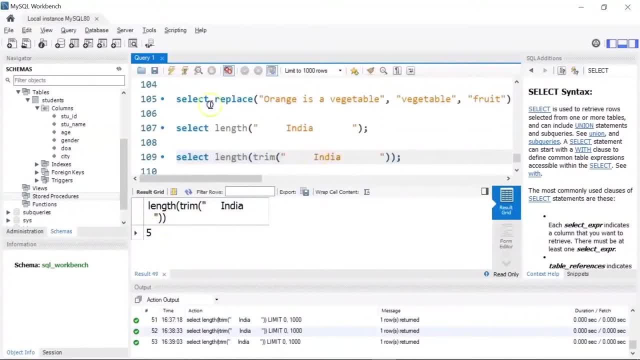 The Leading And The Trailing Spaces. So Here, If I Just Write Position In My Sql, The Position Function Returns The Position Of The First. 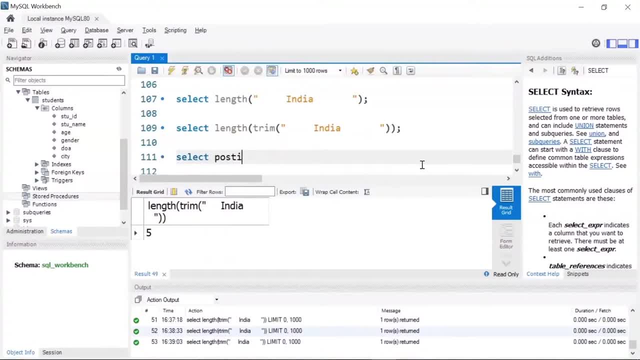 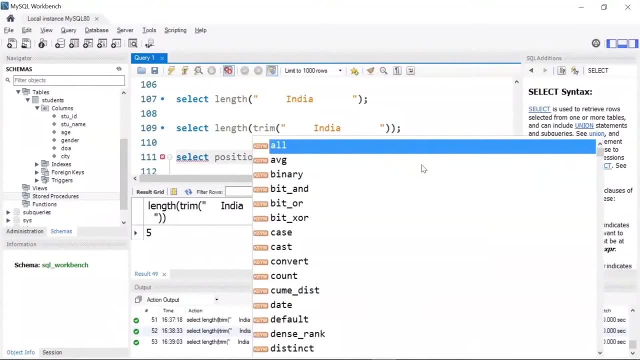 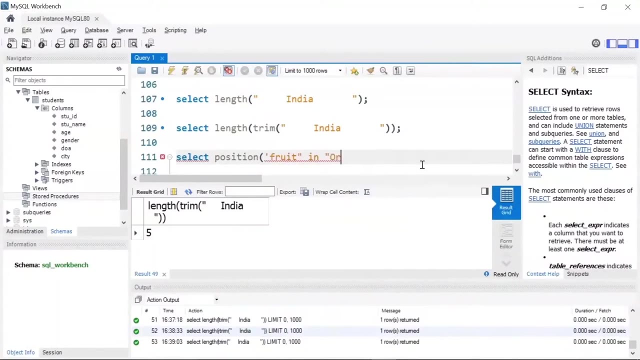 Occurrence Of A Sub String In A String. So If The Sub String Is Not Found, That Is. Orange Is A Fruit I Will Give. 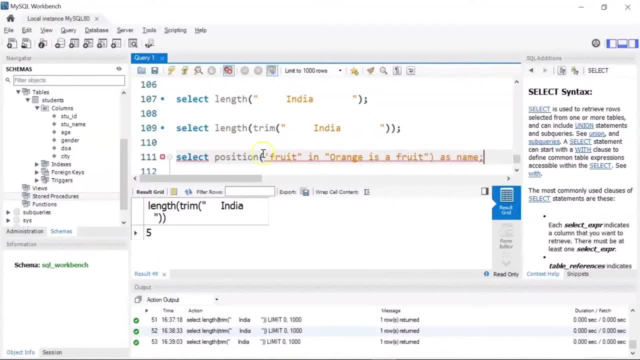 An Alias As Name The Sum Error Here. This Should Be Within Double Quotes. Now Let's Run It And See The Final Function We Are. 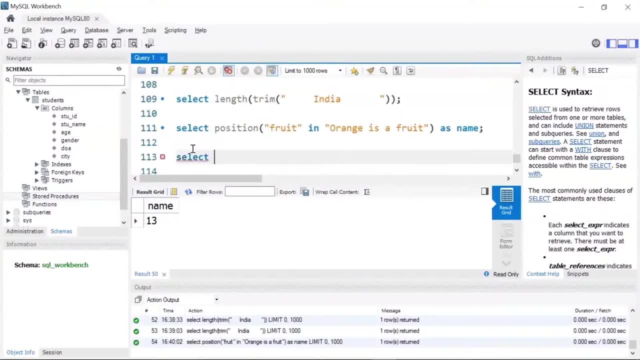 Going To See Is Called Ascii. So The Ascii Function Returns The Ascii Value For A Specific Character. Let's Say I Write Select Ascii. 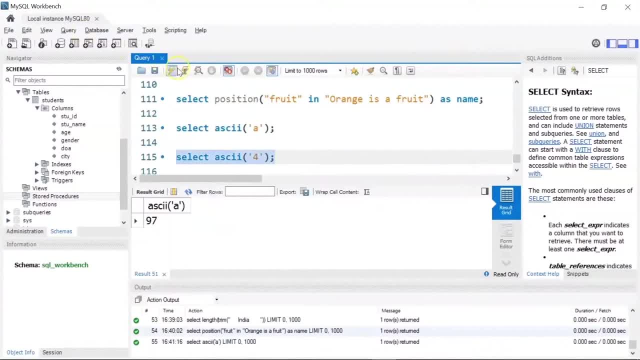 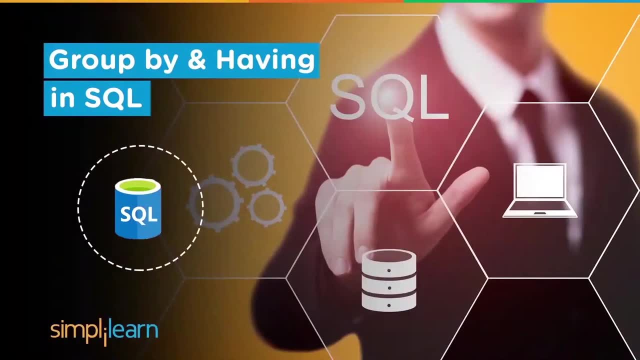 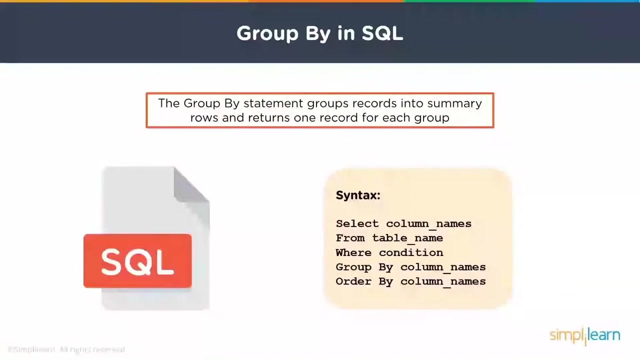 Of. Let's See The Result. It Gives Me 52. All Right, In This Session We Are Going To Learn Two Important SQL Statements Or Clauses. 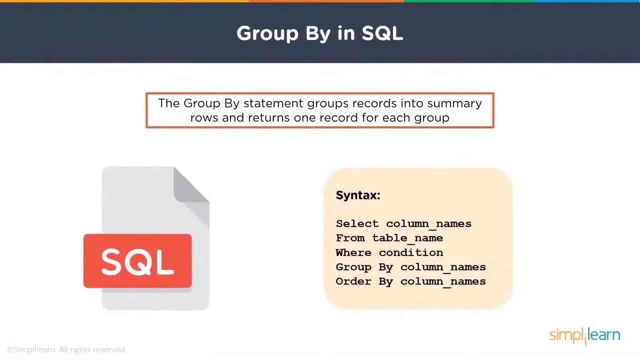 That Are Widely Used. That Groups Records Into Summary Rows And Returns One Record For Each Group. It Groups The Rows With The Same Group. 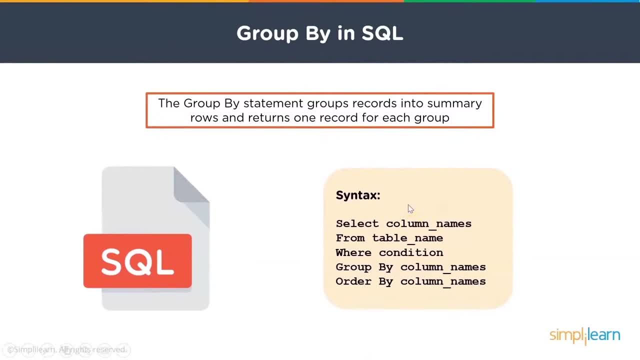 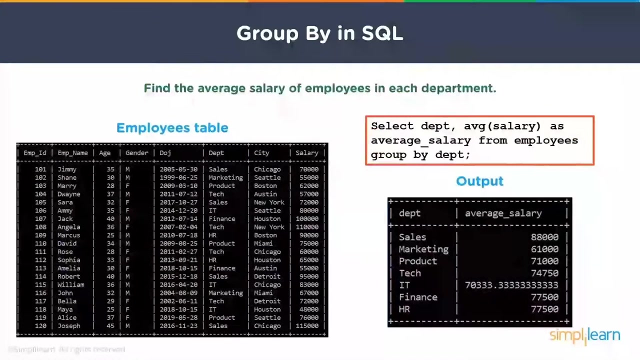 By Item Expressions And Computes. Aggregate Functions For The Group By Clause. We Have The Table Name, Followed By The Where, Condition And Next We. 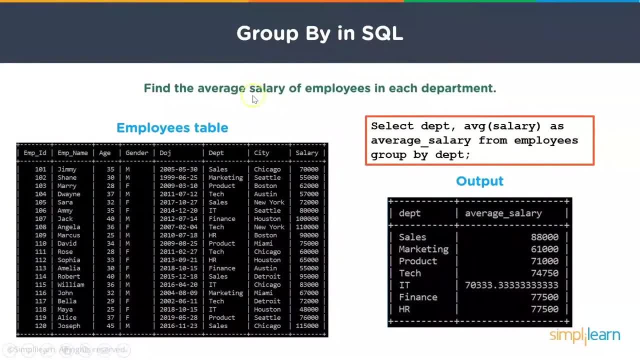 Have The Group By Clause, And Here We Include The Column Names. Finally, We Have The Age Of The Employee, We Have The Gender, The Date. 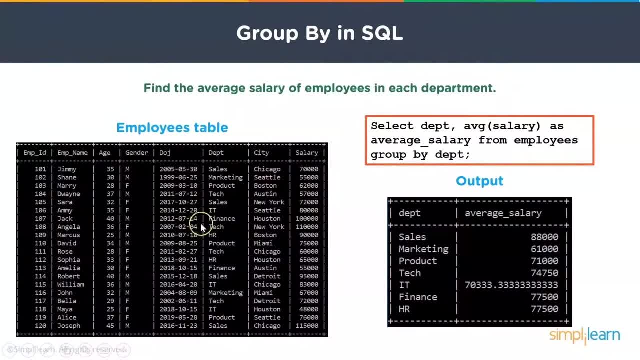 On Which The Employee Had Joined The Company. Then We Have The Department To Which Each Acted Department, And Then We Are Using An Aggregate. 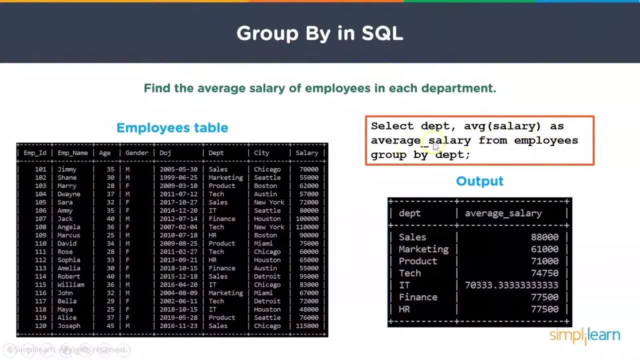 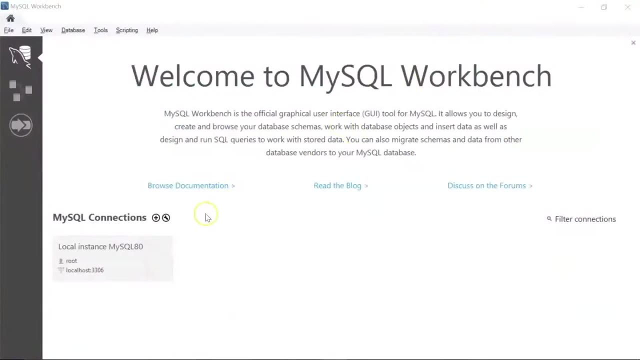 Function, That Is Avg, Which Is Average, And We Have Chosen The Salary Column And Here We Have Given An Group By And Solved Specific. 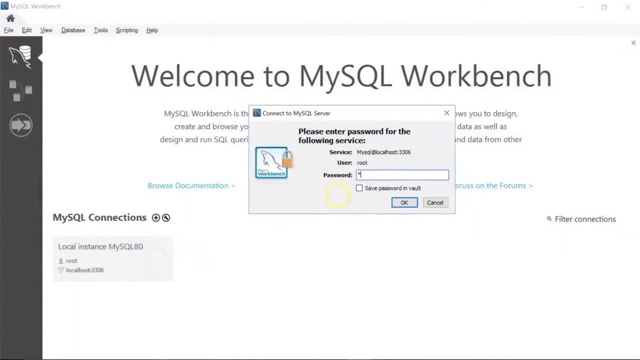 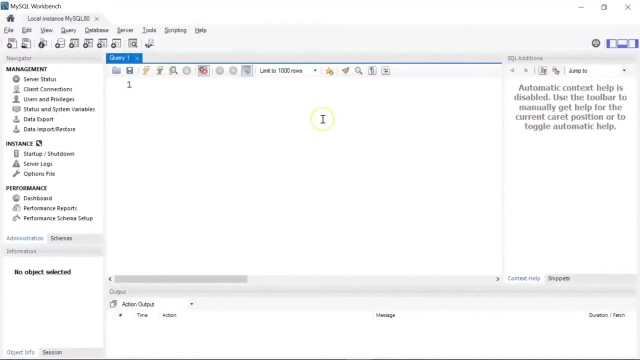 Problems. Okay, So I Am On My My SQL Workbench, So Let Me Make My Connection. First, I'll Enter The Password, So This Will Open. 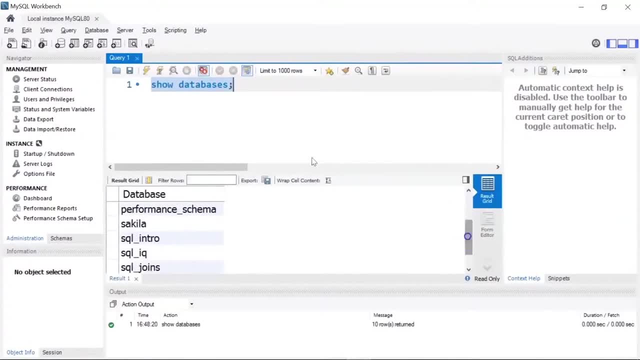 Okay, You Can See We Have A List Of Databases Here. I'm Going To Use My SQL Intro Database, So I'll Write: Use SQL. 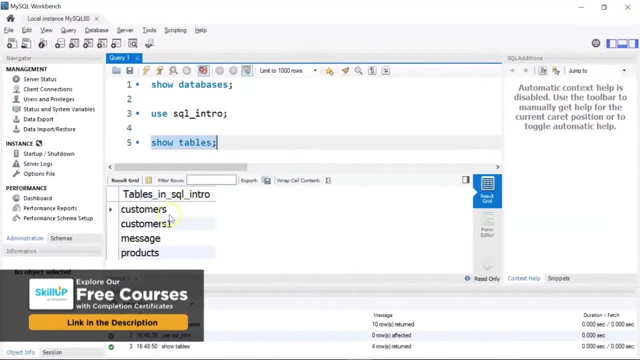 Intro, So This Will Take The Tables That Are Already Present In This Database To Do Our Demo And Understand Group By, As Well As Having 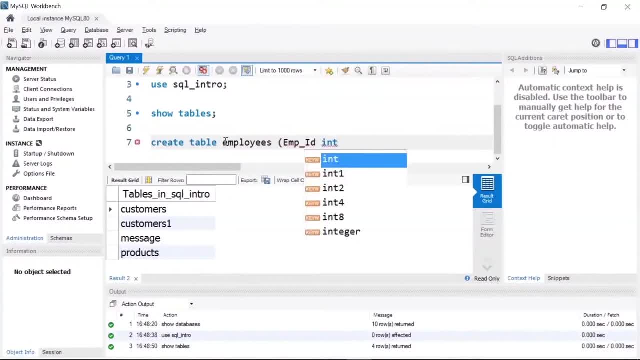 Let Me First Create An Employee Table, So My Primary Key. Next, I'll Give Employee Underscore Name And My Data Type Would Be Bar. 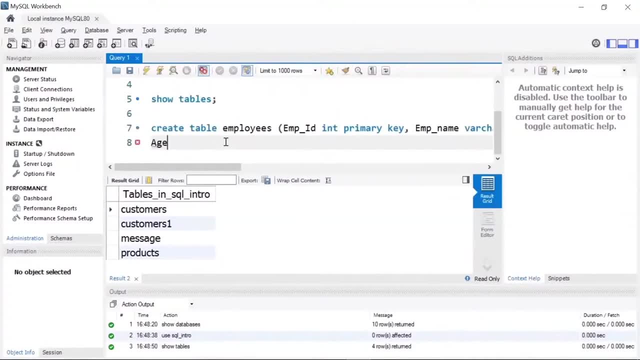 Car. I'll Give The Size As 25.. My Third Column Would Be The Date. I'll Use Character Data Type And Assign A Value Of. 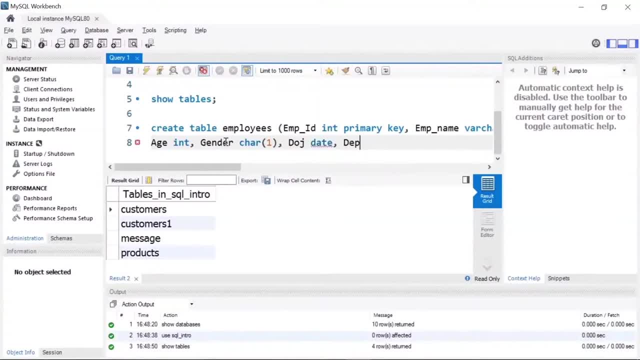 One Or Size Of One. Next, We Have The Date Of Join And The Data Type Will Be The City, Which Is Actually The City To 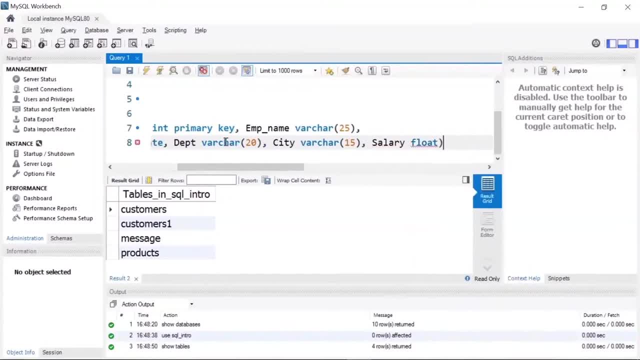 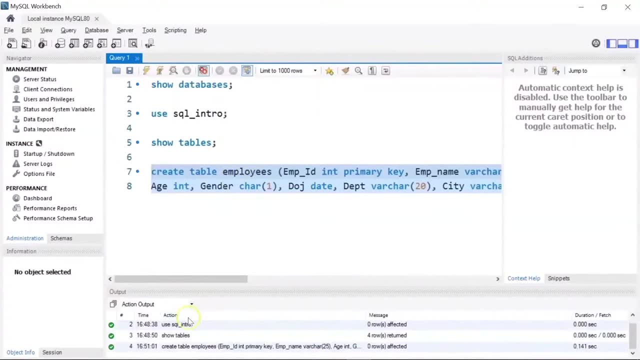 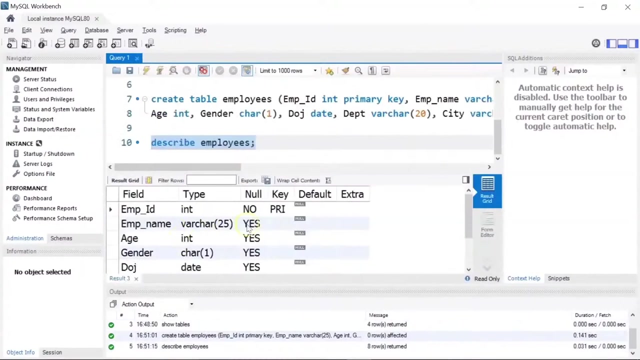 Which The Employee Belongs To. And Finally We Have The Salary Column, Which Will Have The Salary For All The Employees. Okay, You Can See. 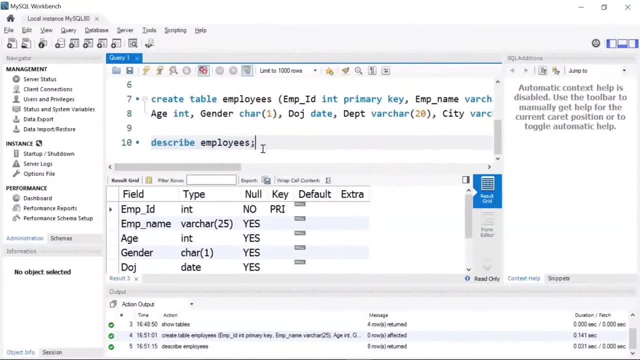 The Structure Of The Table So Far. All Right. Now It's Time For Us To Insert A Few Records Into This Employees Table, So I'll 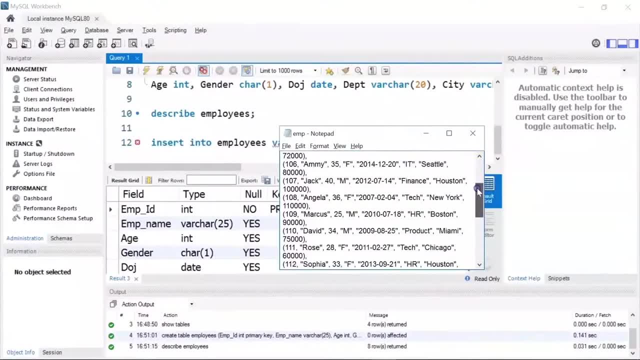 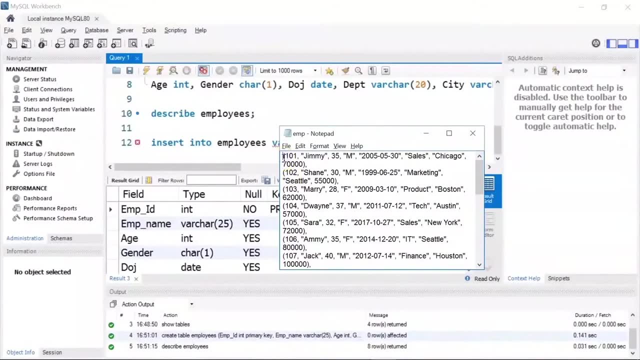 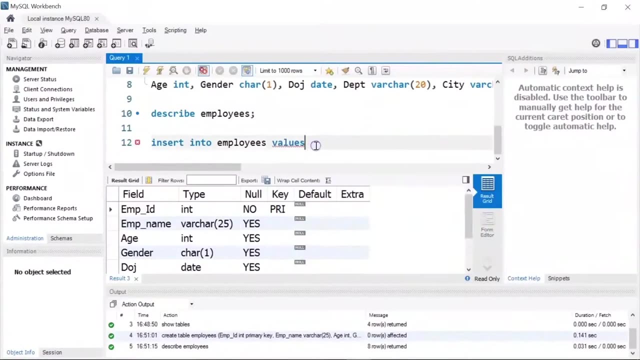 Write Insert Query To All The Employees. So Let Me Just Copy This And We'll Paste It Here. All Right, Let Me Go To The 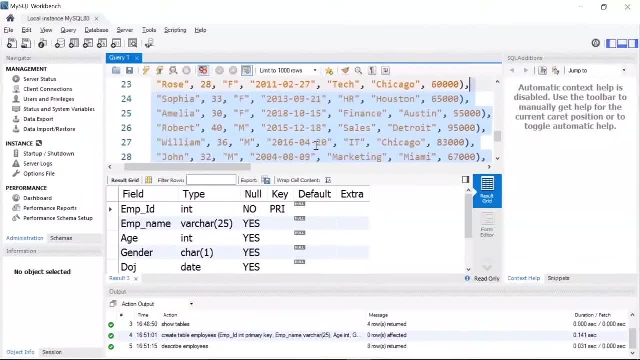 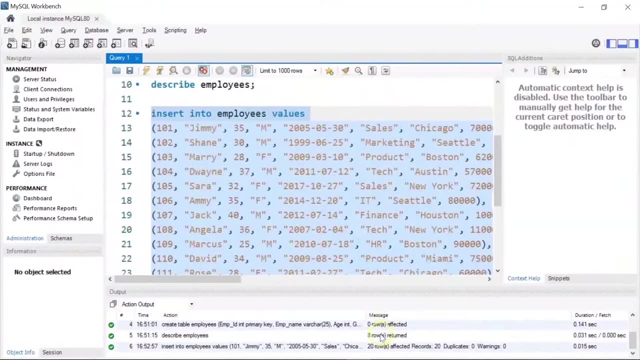 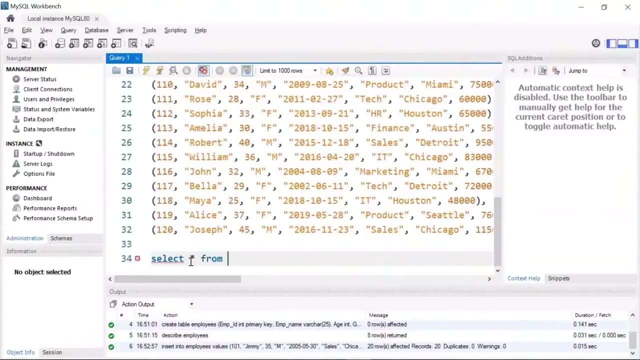 Top And Verify, All The Records Are Inserted. Okay, So You Can See, Here We Have Inserted 20. Rows Of Information. And Now Let's. 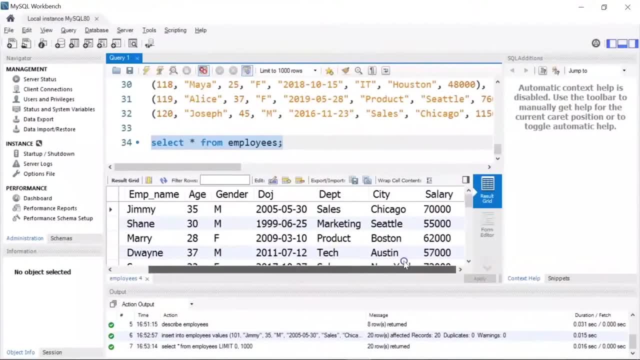 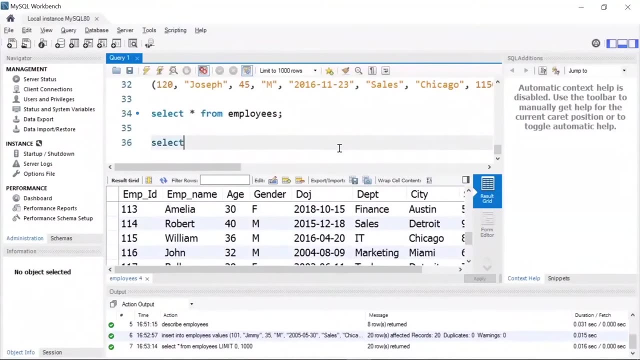 Check The Table Information Or The Records That Are Present In Our Table. Now Let Me Run A Few Sql Commands To Check How The Structure 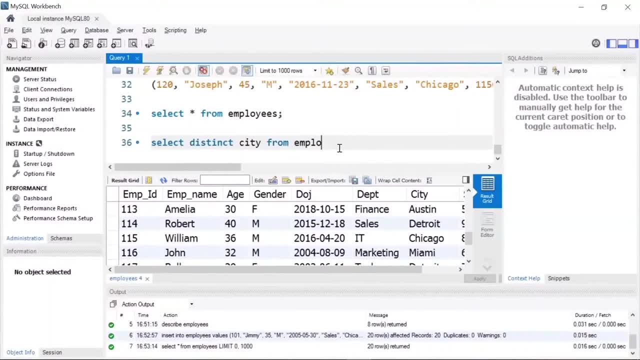 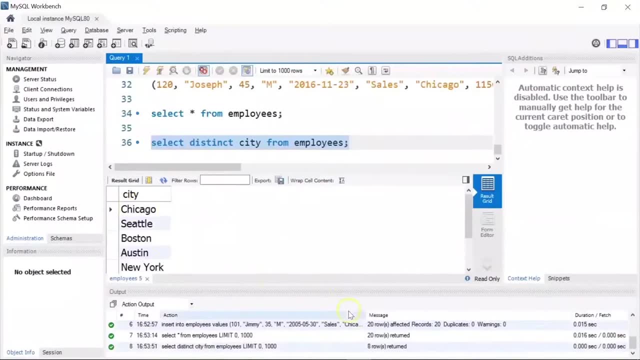 Of Our Table. Let's Say: I Want To See The Distant Cities That Are Present: Chicago, The Seattle, Boston. We Have New York, Miami And 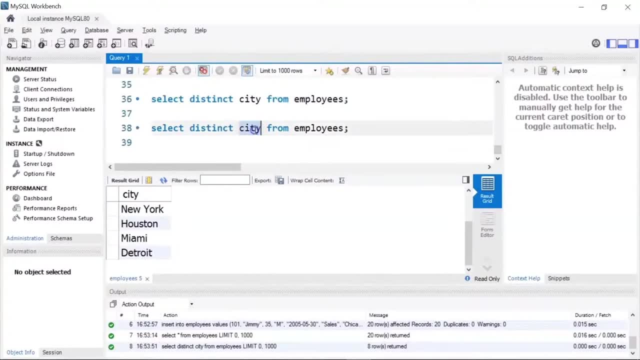 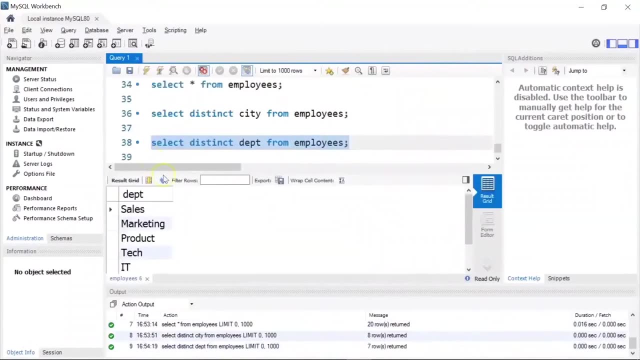 Detroit As Well. Now Let's Say You Want To Know The Total Number Of Departments That Are Present. So It Finance And HR, All Right. 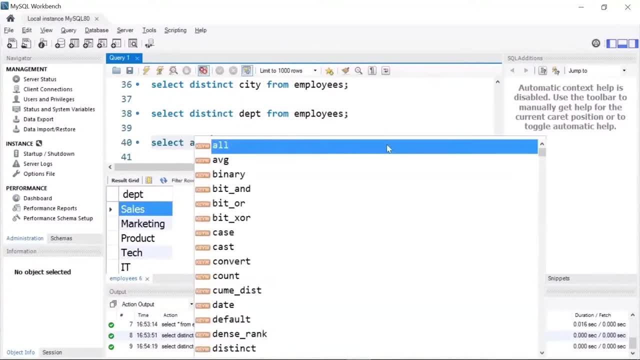 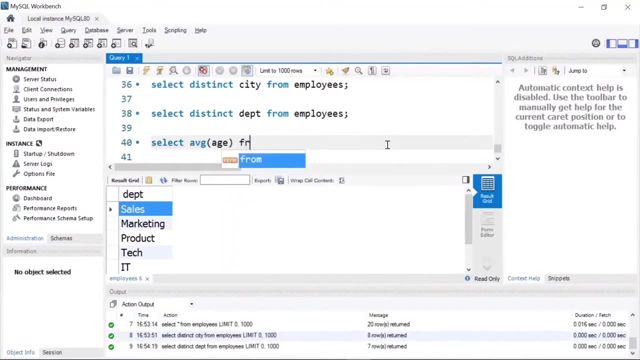 Now Let Me Show You Another Sql Command. Now This Is To Use An Aggregate Function, So I Want To Find The Average Age From Employees. 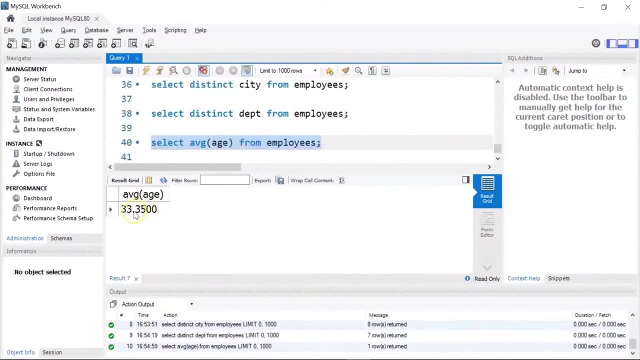 If I Run This. So The Average Age Of All The Employees In Our Table Is 33.35.. Now Say You Want To Find The 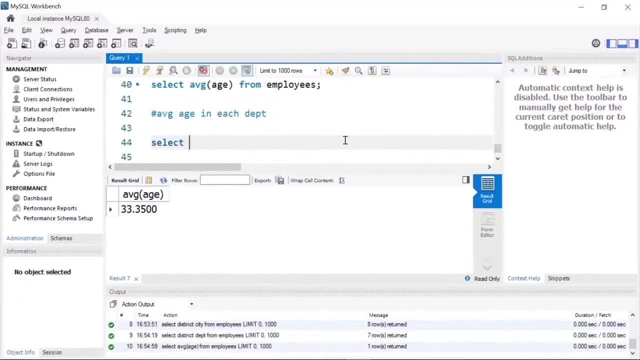 Average Age. In Our Table I Will Write Select Department Comma. I Will Write Average Of Age From Employees Group By Department. Now, If I 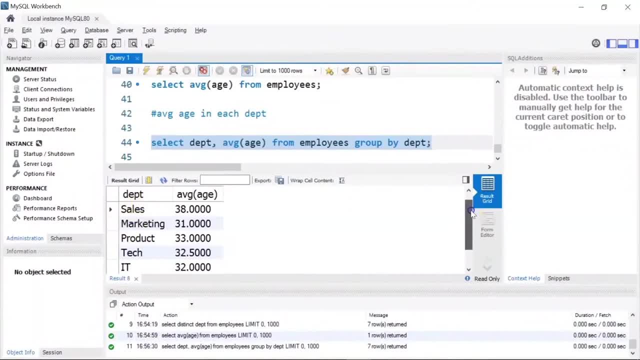 Run This. You Can See On The Left And On The Right. You Can See The Average Age Of Employees In Each Of These Departments. Now 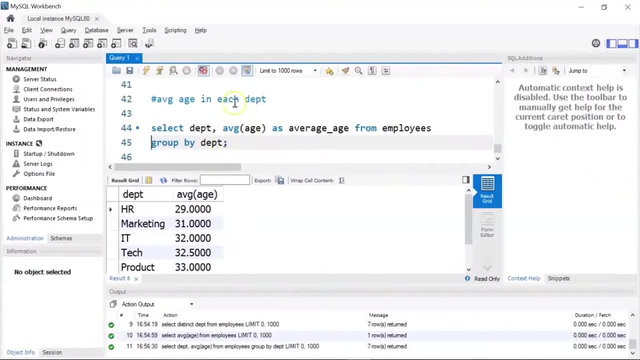 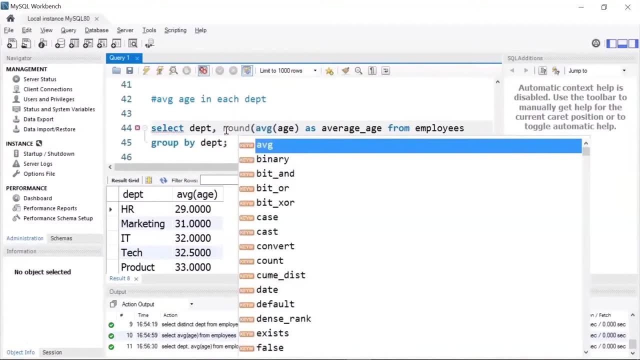 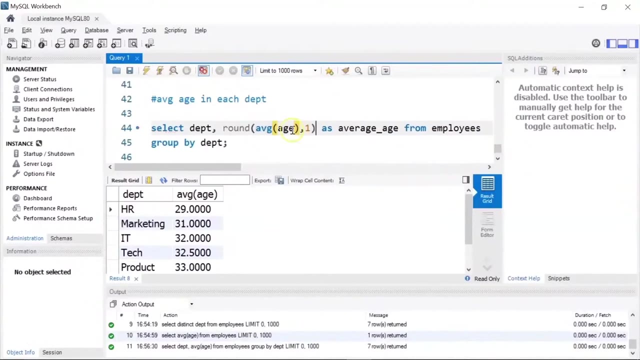 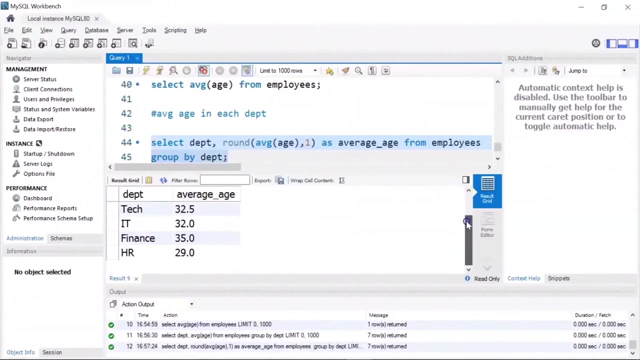 You Can See Here In The Output It. So I Will Use A Round Function Before The Average Function, And The Round Function Takes Two Parameters. 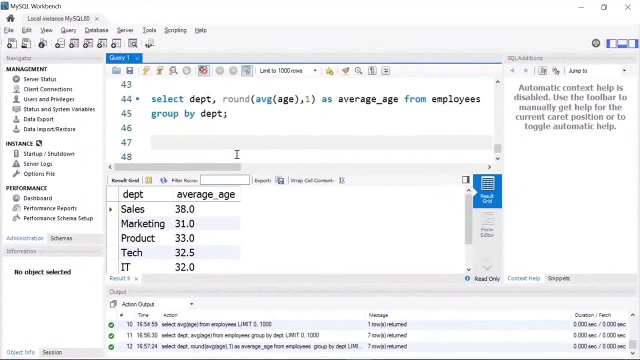 One Is The Variable And The Decimal Place You Want To Write Select Department Comma. Now I Want The Total Salary, So I Will Use: 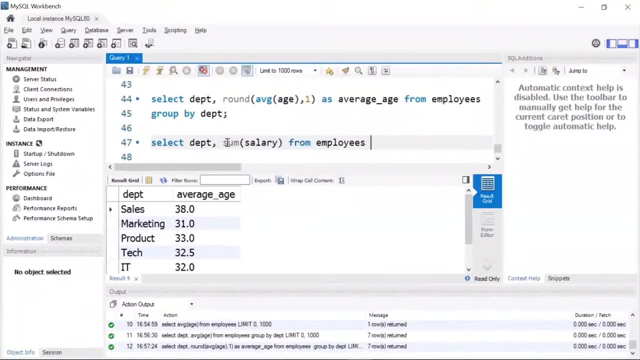 The Sum Function And I Will Pass My Column As Salary From Employees Group By Department. See Here In The Output We Have The Different Departments. 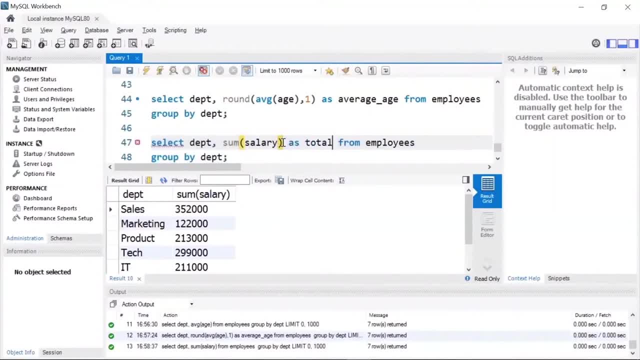 And On The Right You Can See The Total Salary Of All The Employees In Each Of These Departments. You Can Also Use The Order By: 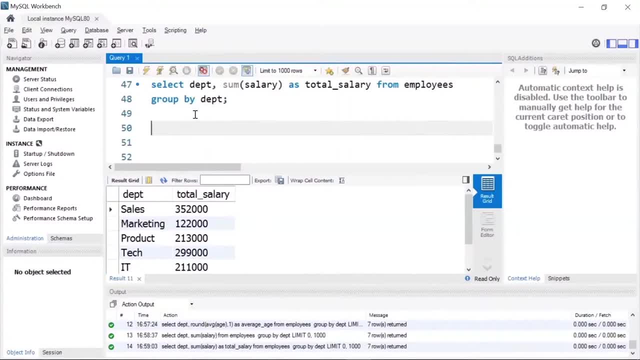 Clause Along With The Group By Clause, Let's See. You Want To Find The Total Number Of Employees In Each City And Group By City. 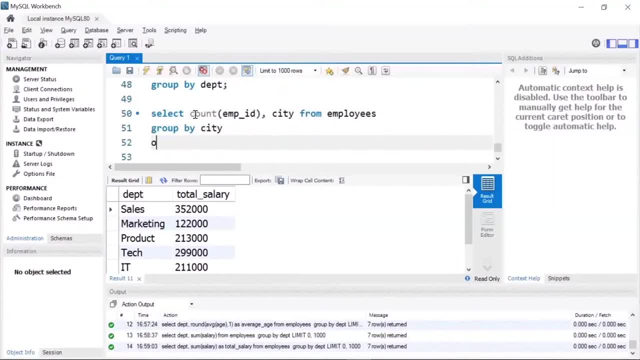 And Next You Can Use The Order By Clause. I'll Write Order By Count Of Employee Id And I'll Write Desc Which Stands For: 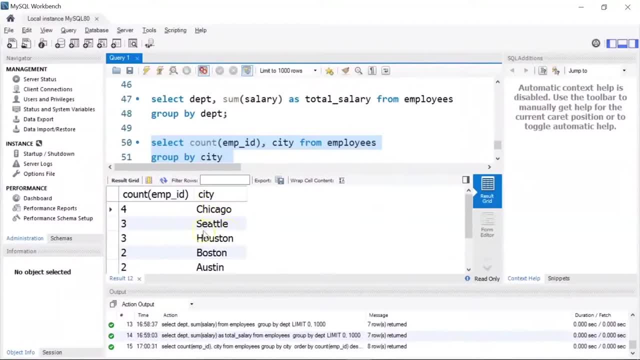 Descending, If I Have The City Names. So In Chicago We Had The Highest Number Of Employees Working. That Was Four. Then We Had Seattle. 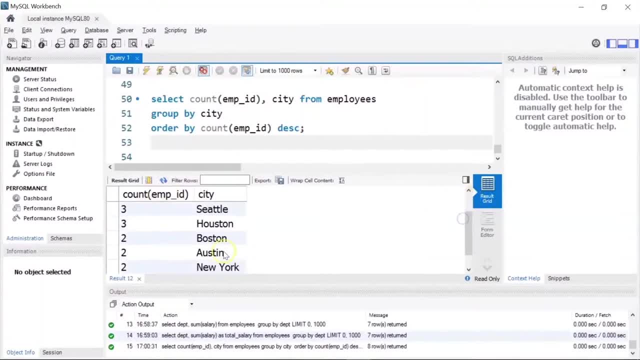 Houston, Boston, Austin And The Remaining. Also Another Example Suppose: We Want To Find The Number Of Employees That Joined The Company Each Year. We Can. 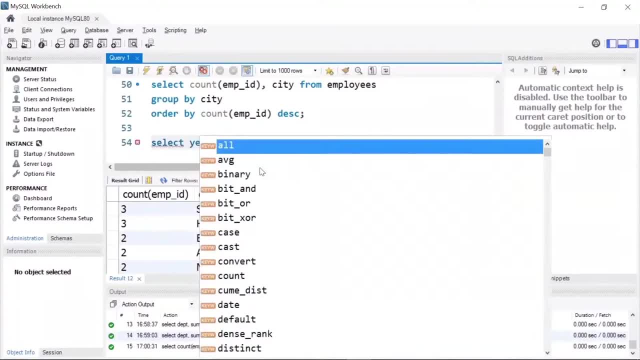 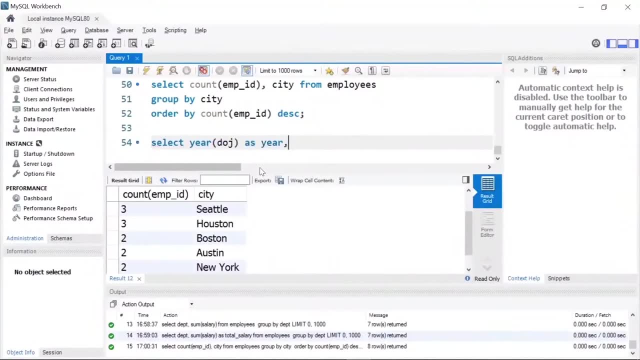 Use The Year Function On The Date Of Joining Column. Next I'll Count The Employee ID From My Table Name. That Is Employees And I'm 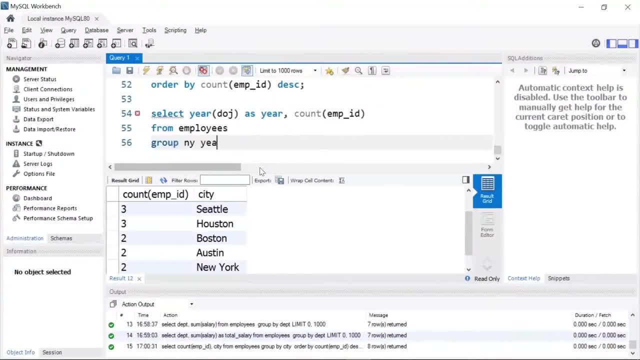 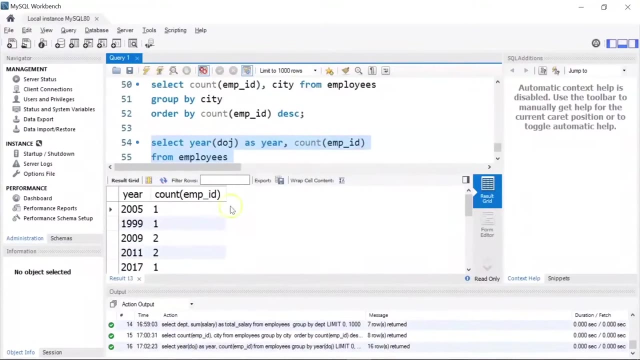 Going To Group It By Year Date Of Join. I Give A Semicolon, All Right, So Let's Run This Great. You See Here In. 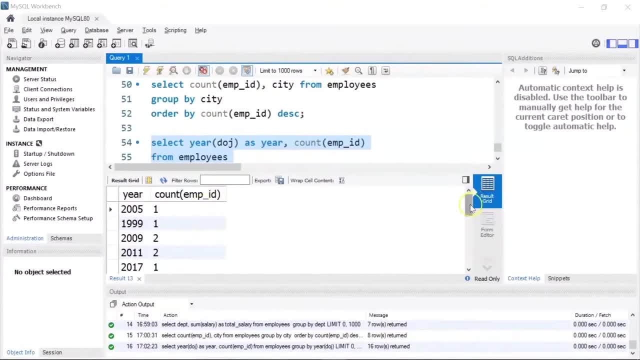 The Result We Have, The Year That We Have Extracted From The Date Of Join Column And On The Right Order. This As Well Based. 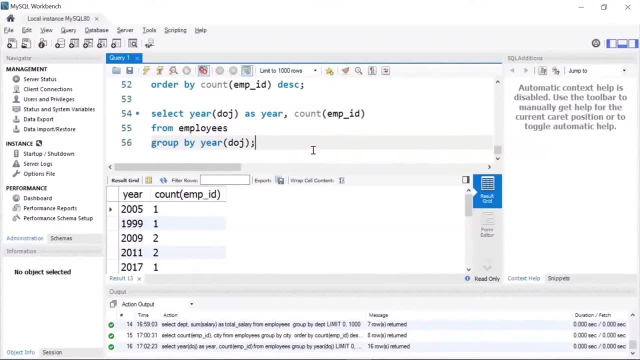 On Year Or Count. Okay, Now You Can Also Use The Group By To Join Two Or More Tables Together, So To Show You Then We. 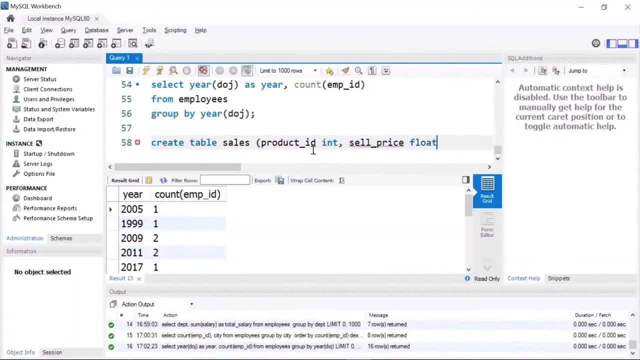 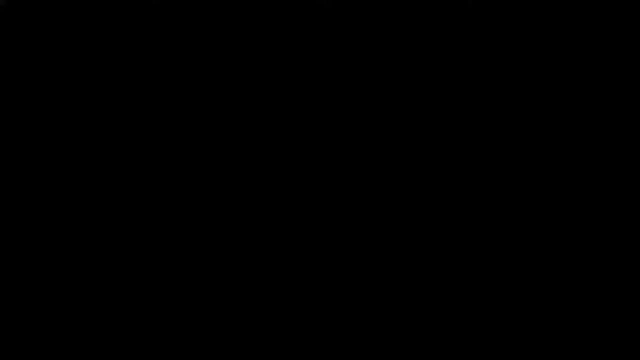 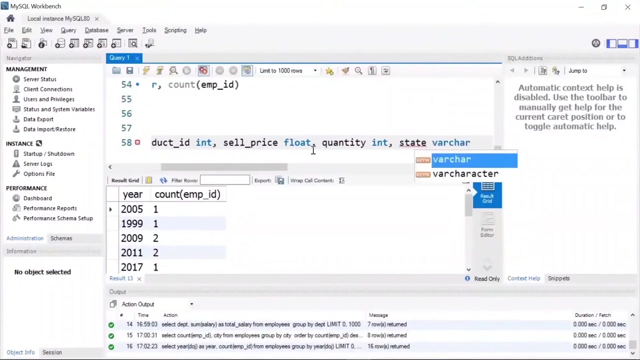 Have The Selling Price Of The Product. Now This Will Be A Float Value. Then We Have The Quantity Sold For Each Of The Products. So 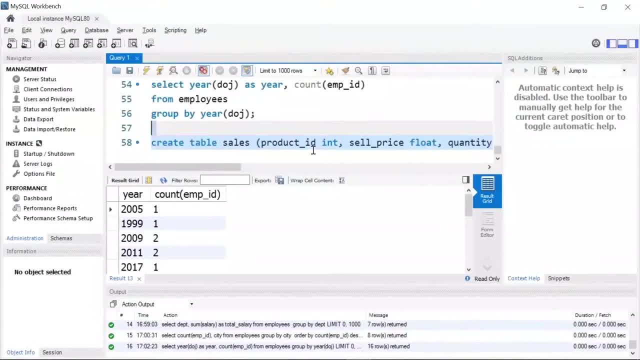 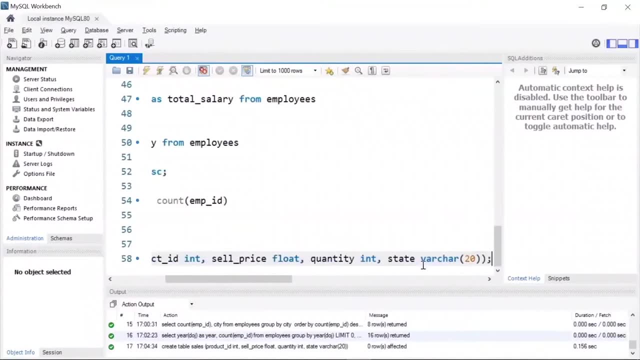 I'll Write 20.. Let's Run This, So That Will Create Our Sales Table. All Right, So We Have Successfully Created Our Sales Table Next. 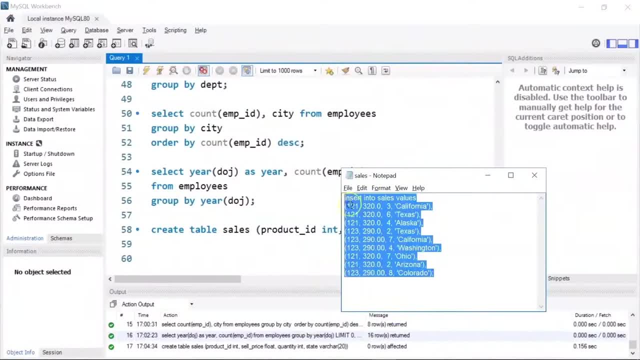 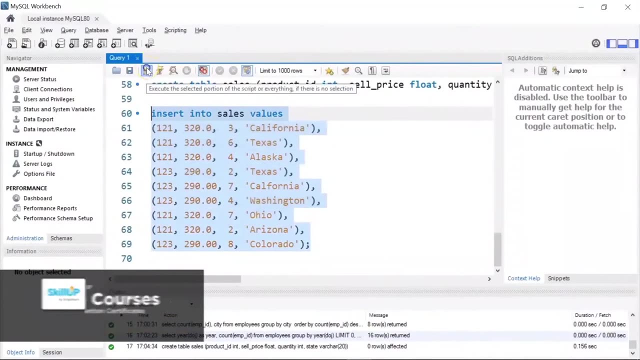 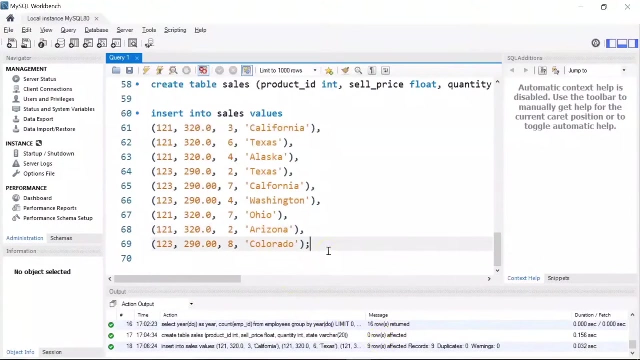 We Need To Insert A Few Values To Create Our Sales And To Create Our Sales. So Let Me Go Ahead And Run This Insert Command. 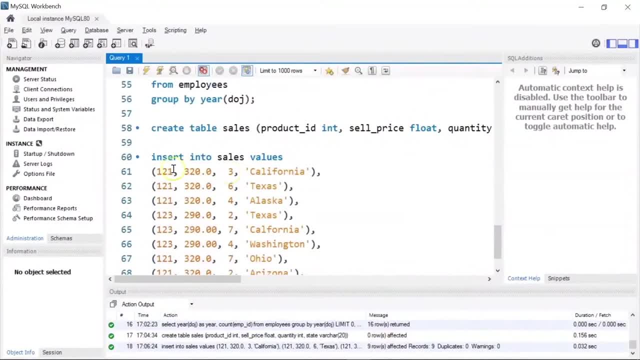 All Right, So You Can See Here We Have Successfully Inserted Sales. Then We Have The Quantity That Was Sold And In Which State It. 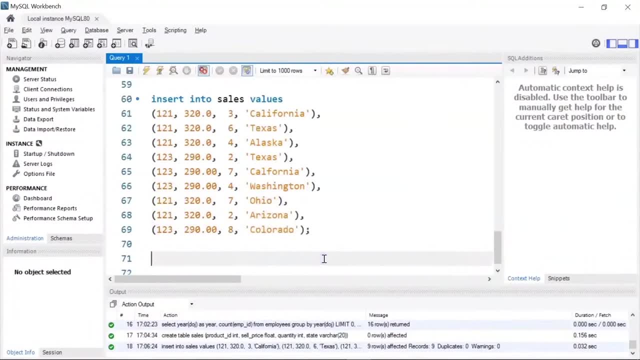 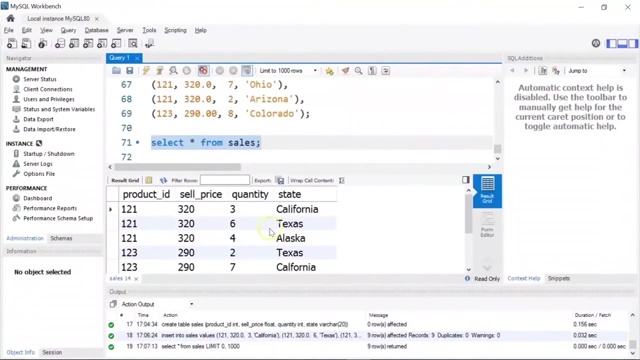 Was Sold. So We Have California, Texas, Alaska. Then We Have Another Product Id, Which Is Our Sales. We Have Successfully Created Our Table. Okay, Now 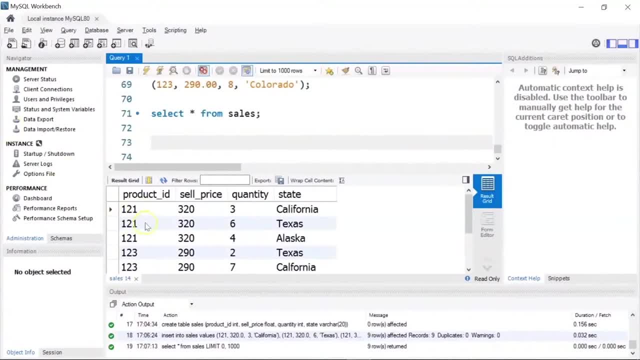 Suppose You Want To Find The Revenue For Both The Product Ids One To One And Let's Say One To Calculate The Revenue. So Revenue. 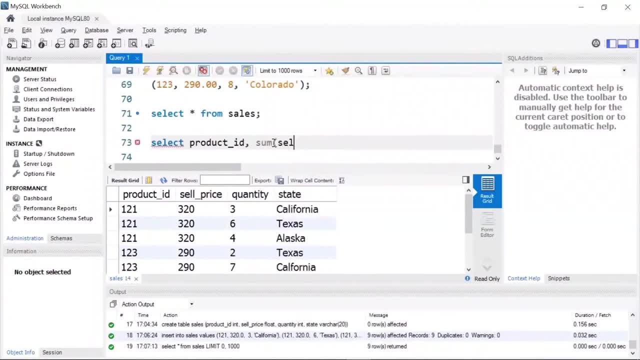 Is Nothing But Selling Price Multiplied By The Quantity. So I'll Use The Sum Function To Find The Total Revenue And Inside The My Table. 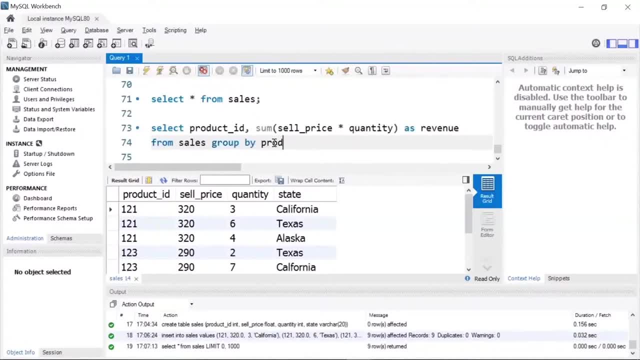 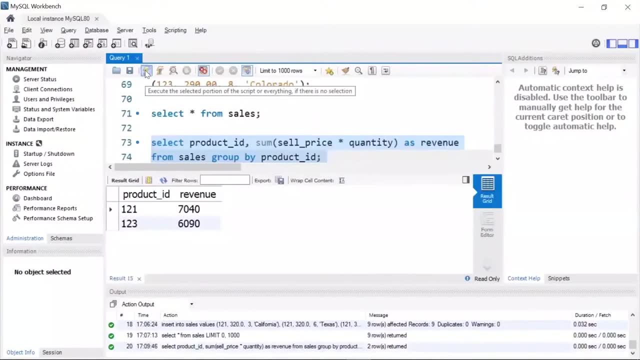 Name, That Is Sales. Finally, I'll Group It By Product Id. Let's Run It. There You Go. So Here You Can See, We Have The. 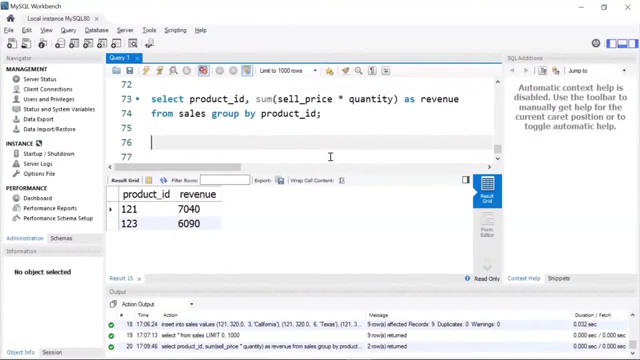 Two Product. We Have To Find The Total Profit That Was Made From Both The Products: One Two One And One Two Three. So For That, 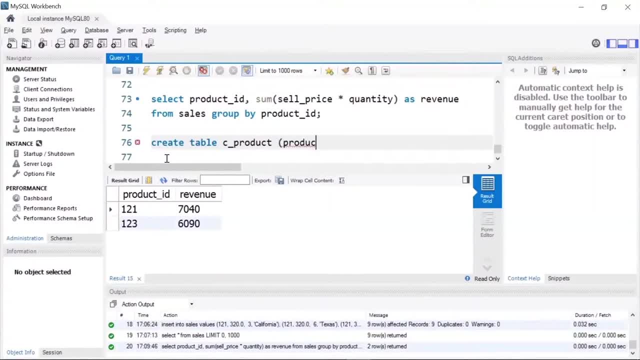 I'll Create Another Table Now. I'll Have My Product Id. This Will Be An Integer, And I'll Have My Second Column As Cost Price. 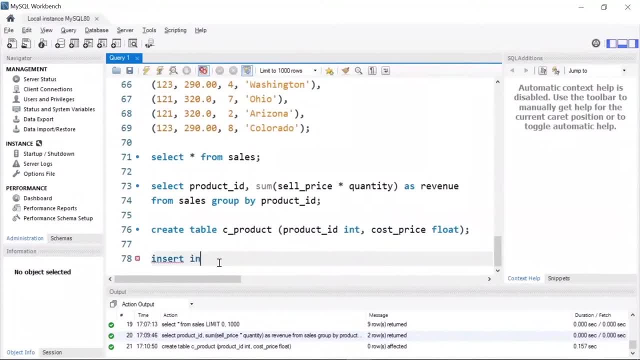 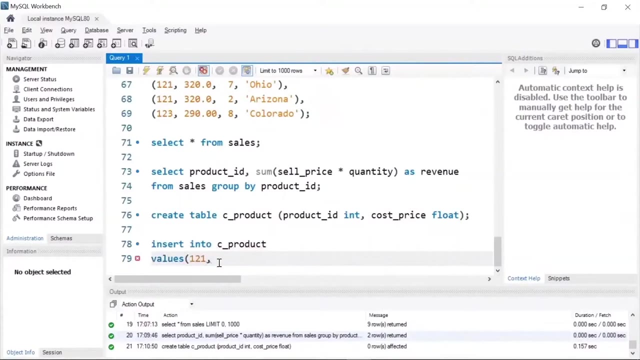 Cost Price Will Have Floating Type Values. Let's Run This So I'll Give My Values For One To One. Let's See The Cost Price. 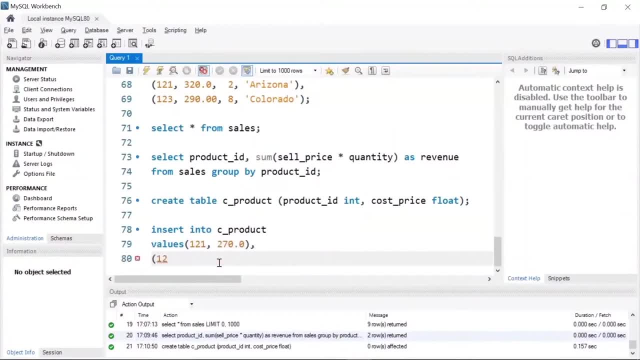 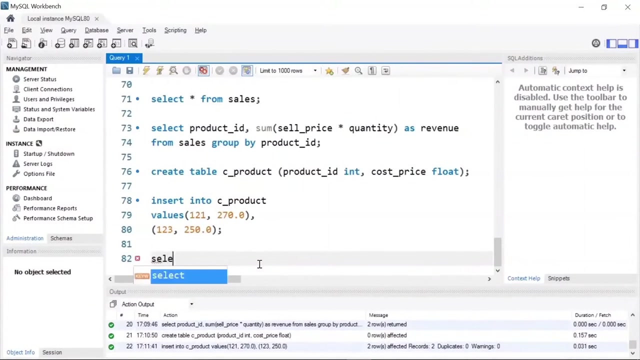 Was Two Hundred And Seventy Dollars For Each, And Next We Have My Product As One. Two Values. Okay, Next We'll Join Our Sales Table. 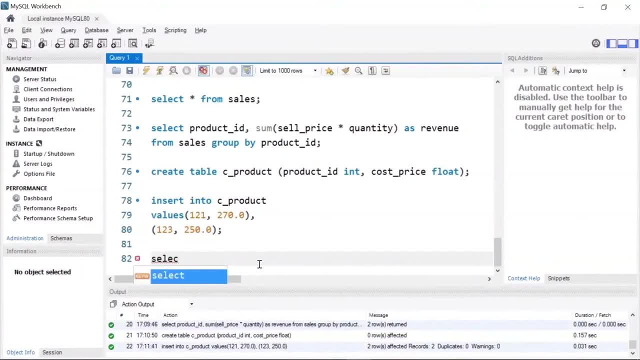 And The Product Cost Table. So This Will Give Us The Profit That Was Generated For Each Of The Products. So If I Subtract My Cost, 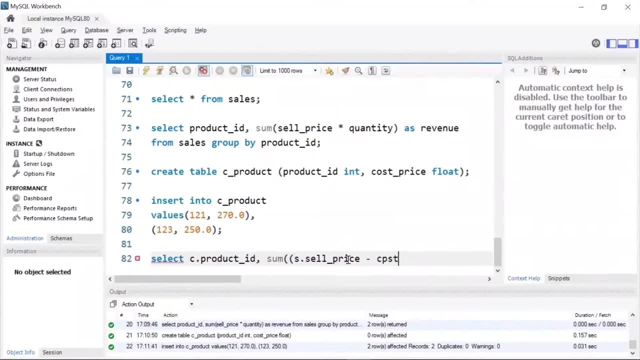 Price From The Selling Price. That Will Return The Profit That Was Generated. I'll Multiply This With S Quantity. Close The Bracket. I'll Give The 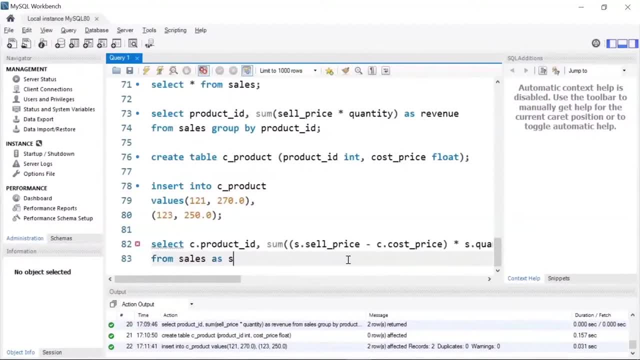 Profit From Sales As S. So Here S Stands For The Sales Table. I'm Going To Use Inner Join C Underscore Product Table As 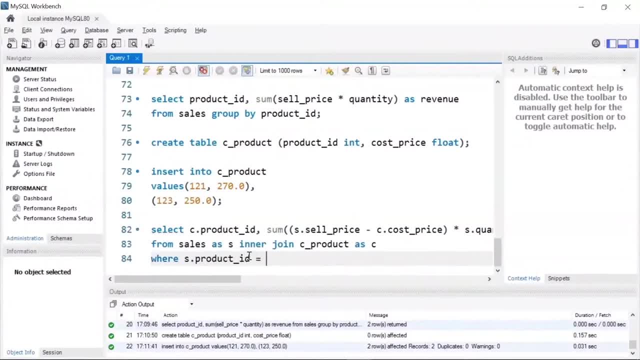 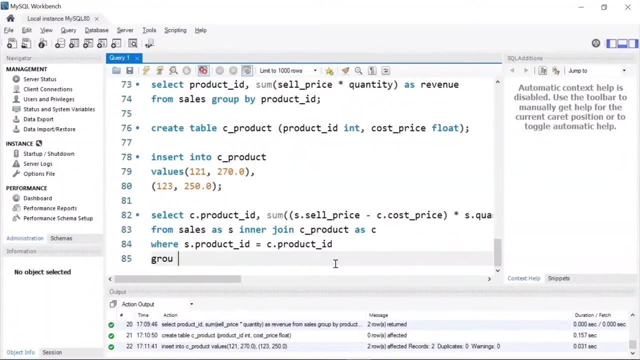 The Alias Name Should Be C Dot. Product Underscore ID. We're Using Product Underscore ID Because This Column Is The Common Column To. 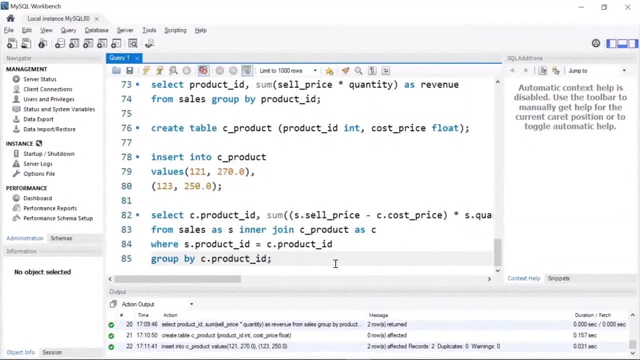 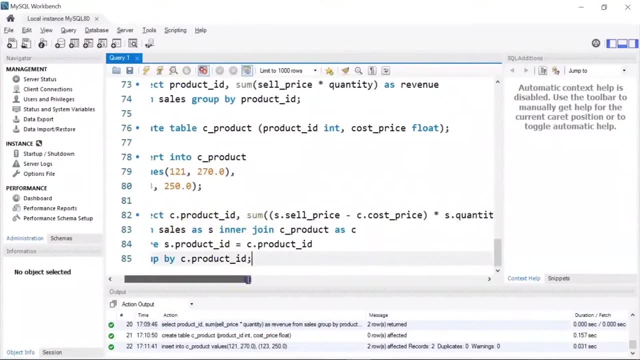 Both The Tables. And Finally, I'm Going To Group It By: I'm Calculating The Profit By Subtracting The Cost Price From The Selling Price. 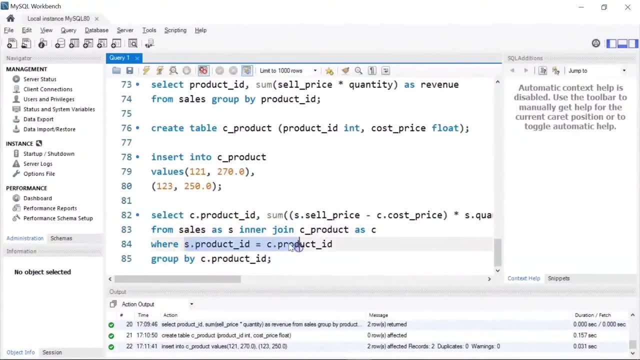 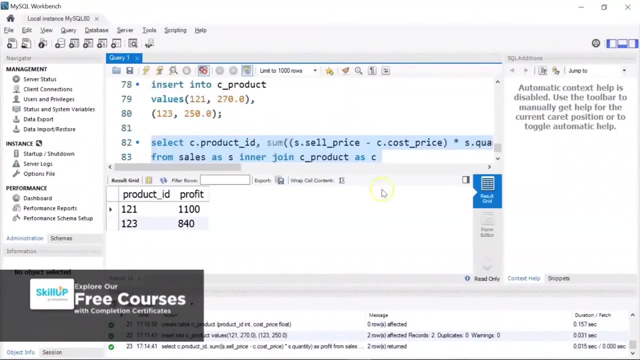 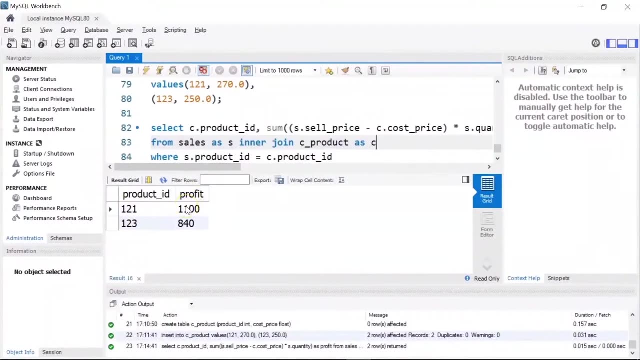 And I Have Multiplied The Quantity Column. I'm Using An Inner Join To Connect My Sales Of 1100. Dollars And For Product ID 123.. 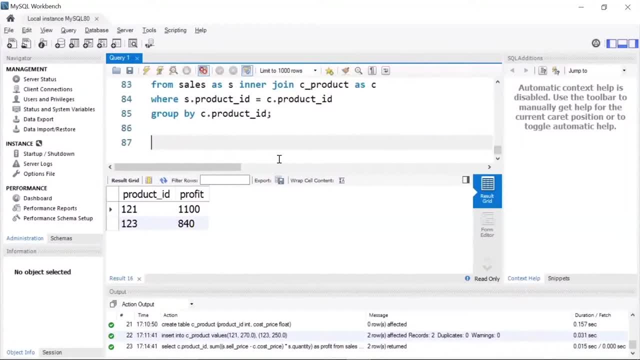 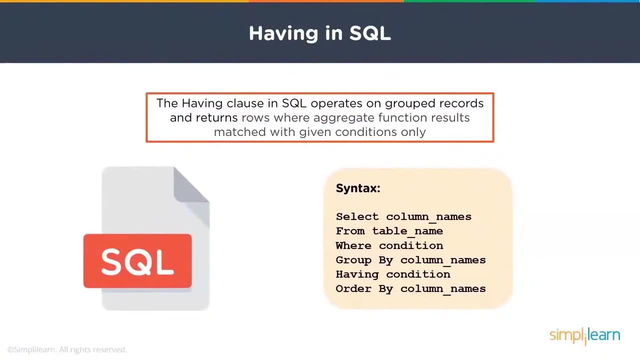 Made A Profit Of 840. Dollars. So Now That We Have Learned Group By In Detail, Let's Learn About The Having Here You Can See. 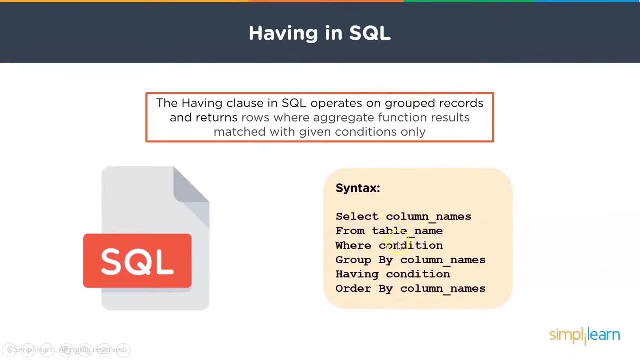 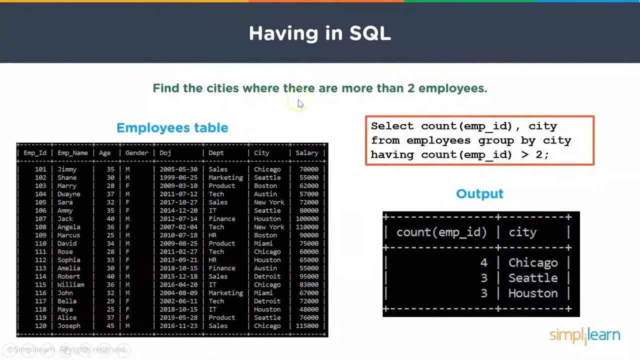 The Syntax Of Having Clause. You Have The Select Statement Followed By The Column Names From The Table Name. Then We Have The Where Conditions. 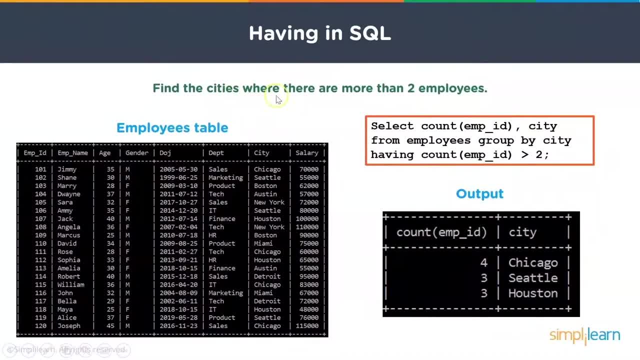 Group By Clause As Well. So If You Were To Find The Cities Where There Are More Than Two Employees, So This Is How Your SQL. 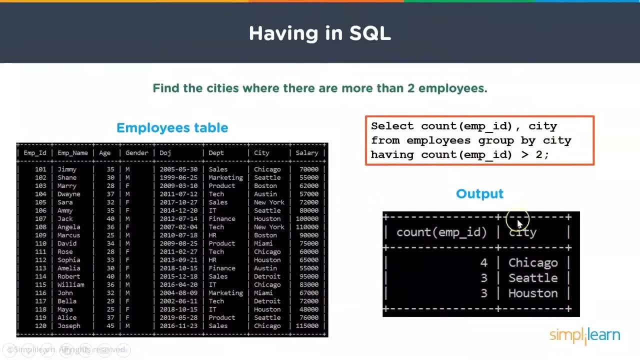 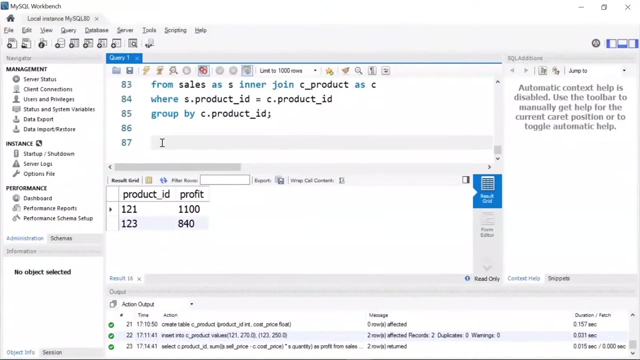 Queries Should Look. So, If You See The Output, We Have The Different City Names And These Were The Cities Where The Count Of Employees Was. 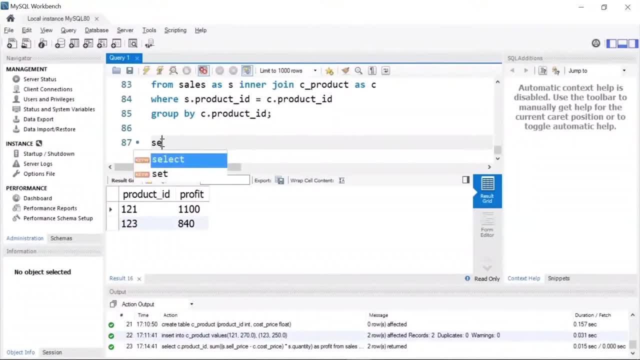 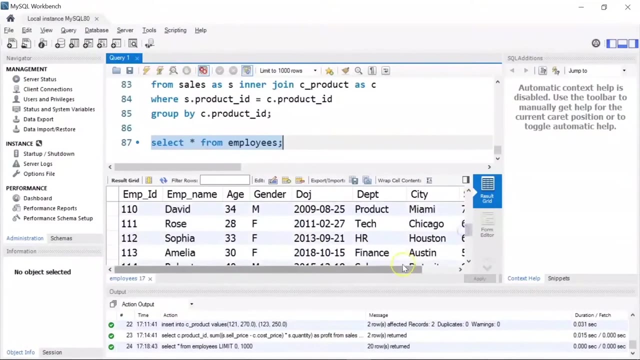 Greater Than Two. All Right. So If You Have The Cities, Where Are More In The Cities Where You Have The Count Of Employees, If I? 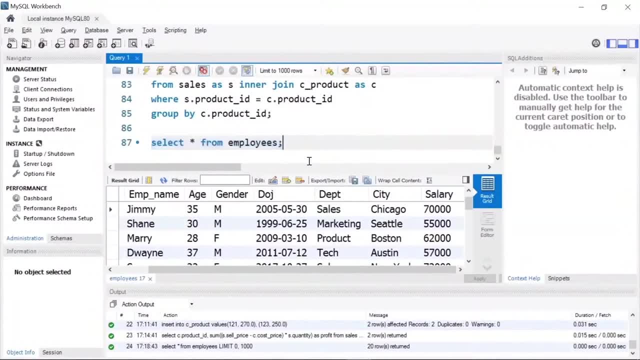 Run This. You Can See We Are Inserted 20.. Comma: I Will Use The Aggregate Function, That Is Average Salary. I Will Give An. 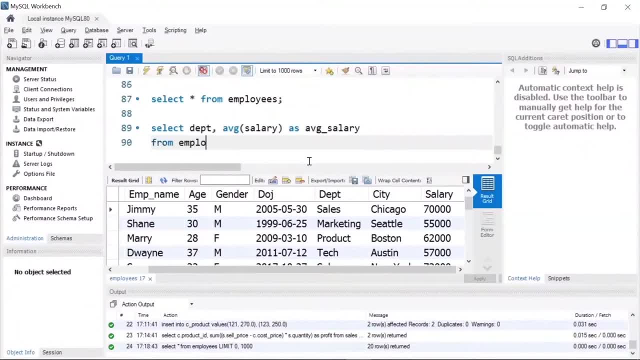 Alias Name As Avg Underscore Salary From Employees. Next Will Use The Group By Clause. Then I Am Going To Write My Having Clause So. 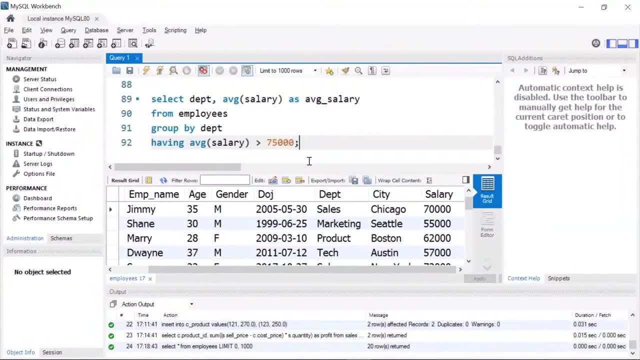 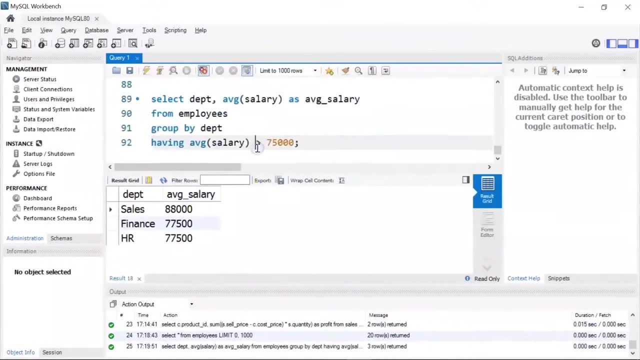 In Having Clause, I Use My Condition, That Is, Having Average Of Salary Greater Than $75,000.. Let's Run It And Find The Cities, Okay. 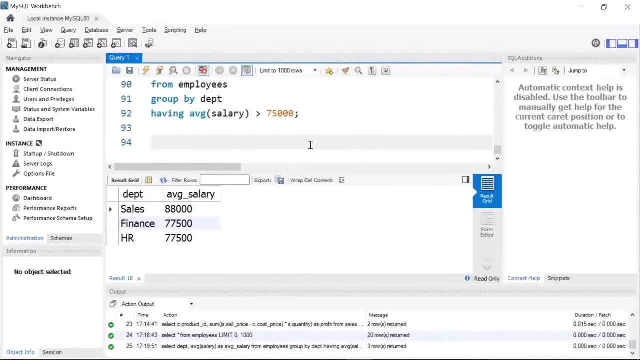 Next, Let's Say You Want To Find The Cities Where The Total Salary Is Greater Than $200,000.. So This Will Again Be A Simple. 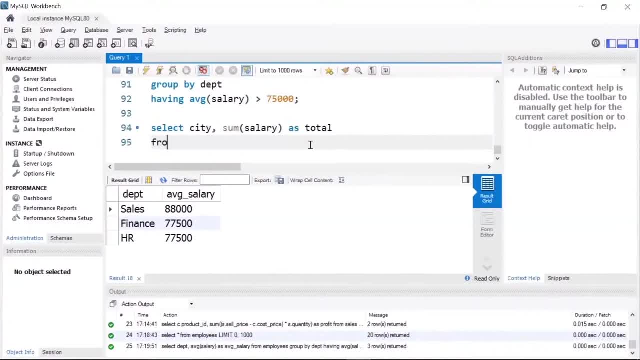 SQL Query Alias Name As Total From Employees Group By City. And Then I Am Going To Use My Having Clause. I Pass In My Condition. As Having Some Of Salary In Cities Are Chicago, Seattle And Houston, Where The Total Salary Was Greater Than $200,000.. Now Suppose You Want. 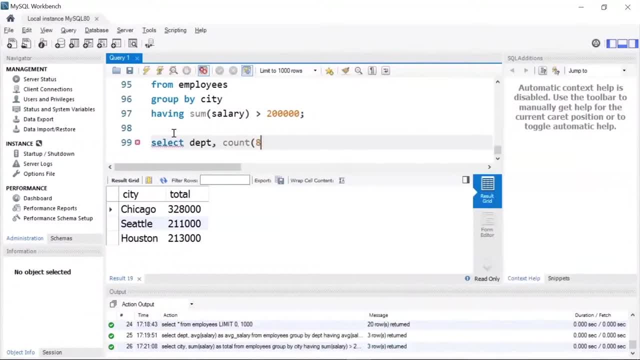 To Find The Departments That Have More Than Two Employees, Or Emp Underscore Count, Which Is My Alias Name From Employees Next I'll Group. 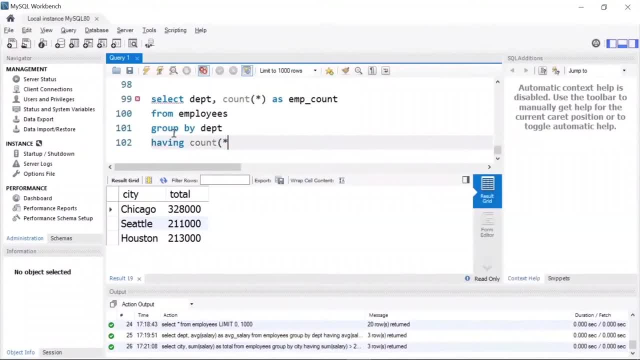 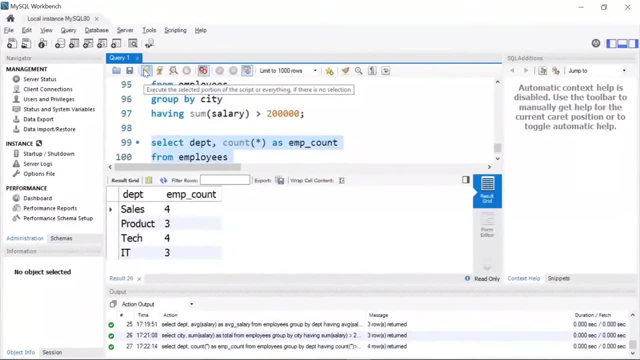 It By Department Having. I'll Give My Condition: Count Star Greater Than Two. Let's Run. This Is A City Where There Are More Than Two. 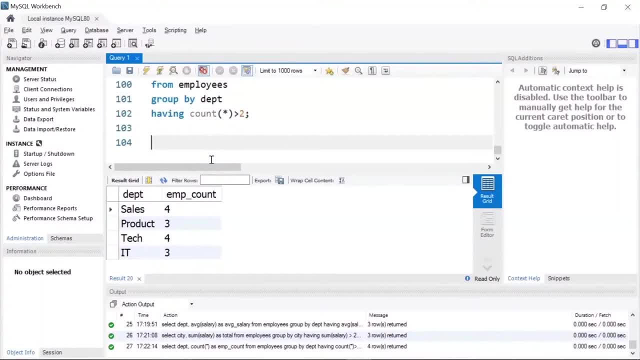 Employees. Okay, Now You Can Also Use A Wear Clause Along With The Having Clause In An SQL Statement. Suppose E M P Count From Employees. 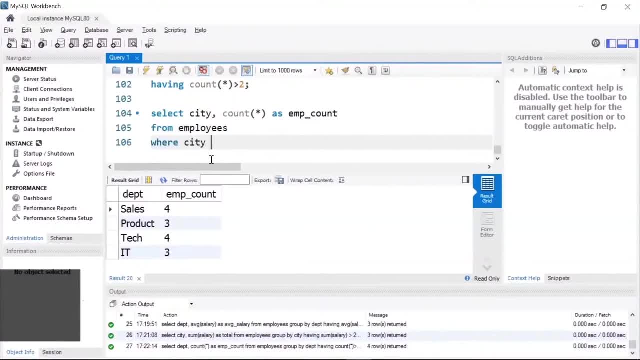 Where I'll Give My Condition City Not Equal To Houston. I'll Put It In Double Quotes, Since I Keep It By City Having Count Of. 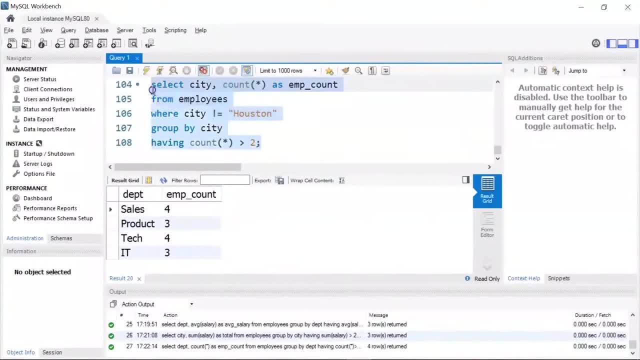 Employees Greater Than Two. If I Run This Query, You See We Have Information For Chicago And Seattle Only And I Want To Find The Total. 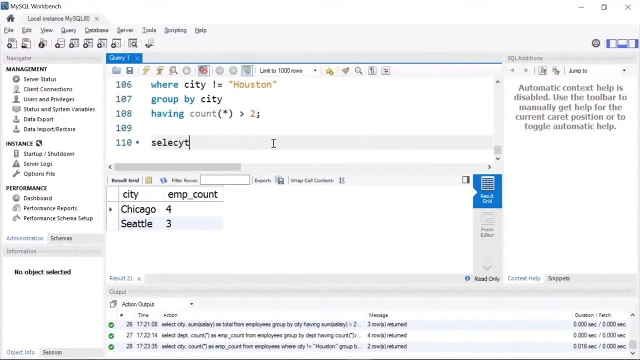 Number Of Employees For Each Department That Have An Average Salary Greater Than $75,000.. I Can Write It Something Like This: Select Department Employees. 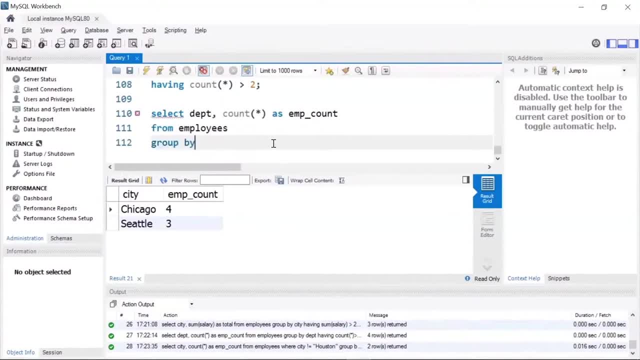 Group, By Department And In The Having Clause. I Am Going To Provide The Column Name. That Is Not Present In The Having Clause. Let's 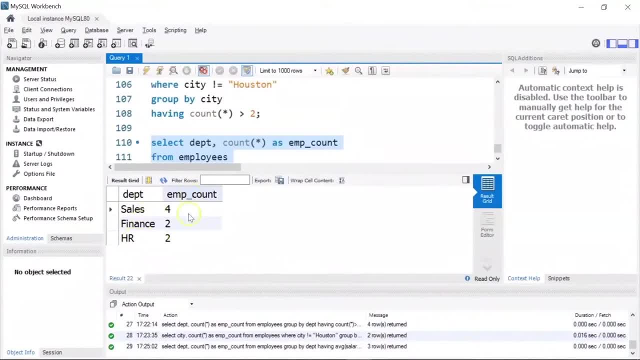 Run This All Right. You Can See We Have Department Sales, Finance And HR And You Can See The Employee Count Where The Average Salary We 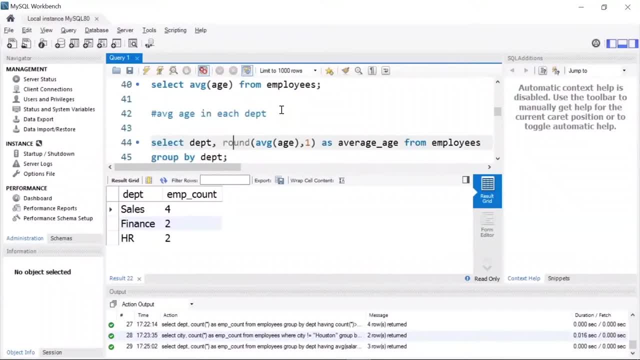 Explode. A few SQL Commands Like Distinct, Then We Used Average And Finally We Started With Our Group By Clause, Followed By Looking At How. 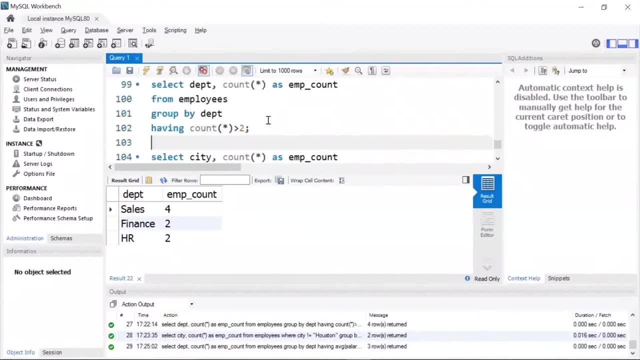 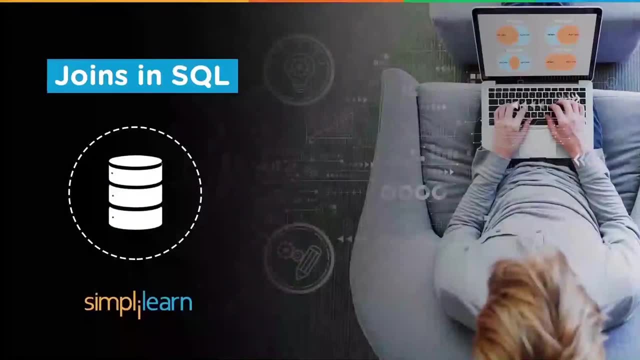 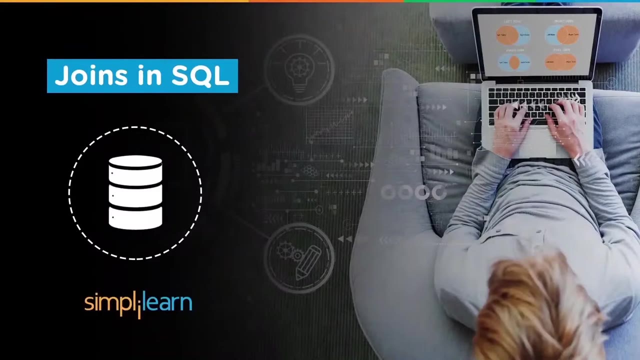 Group By Can Be In SQL. In This Session We Will Learn About Joins In SQL. Joins Are Really Important When You Have To Deal. 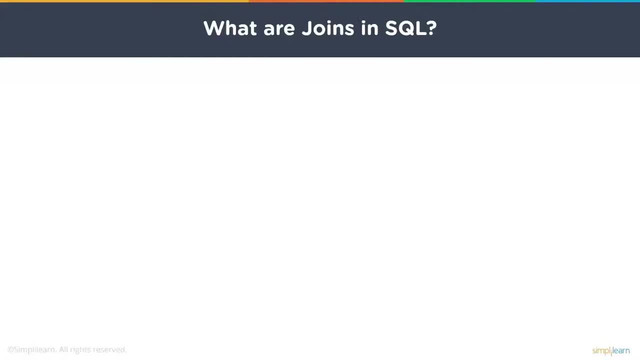 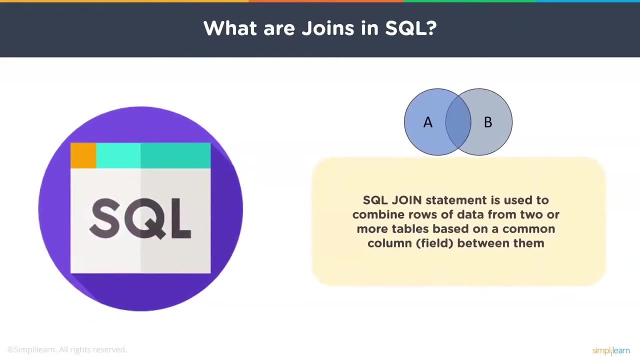 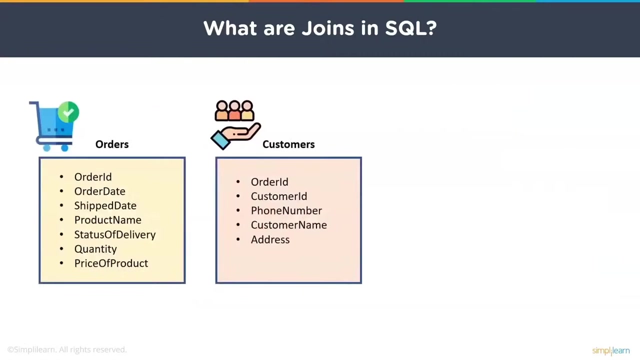 With Data That Is Present On Multiple Tables. SQL Joins Are Used To Combine Rows Of Data From Two Or More Tables Based On A. 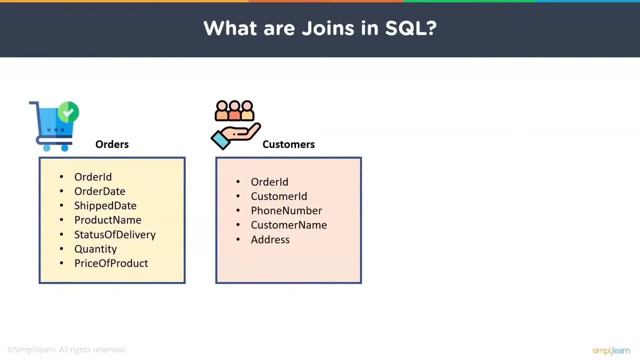 Common Field Or Column Between Them. Now Consider This Example, Where We Have The Date On Which The Order Was Shipped. Then We Have The 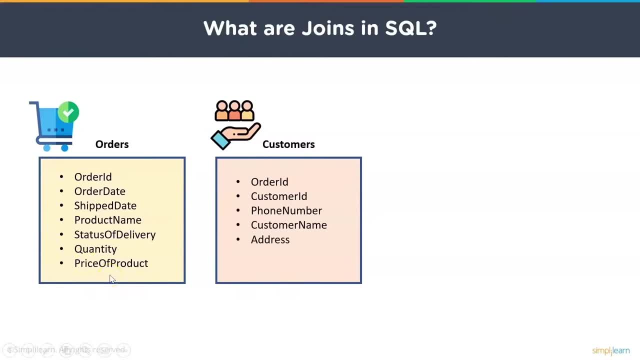 Product Name, Which Basically Is The Names Of Different Products. We Have The Status Of Delivery, Then We Have The Customer ID, Which Is The Primary. 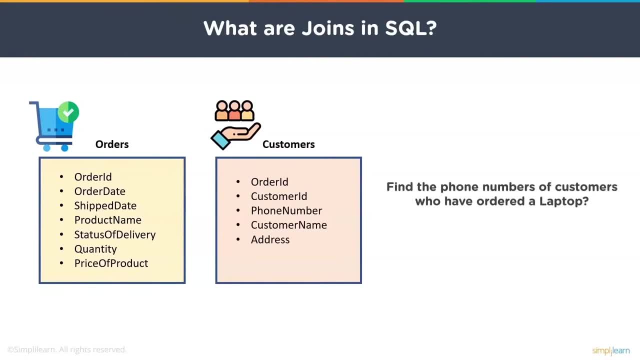 Key For This Table. We Also Have The Phone Number, Customer Name And Address Of The Customers. Now, Suppose You Have Order Table Which You Can 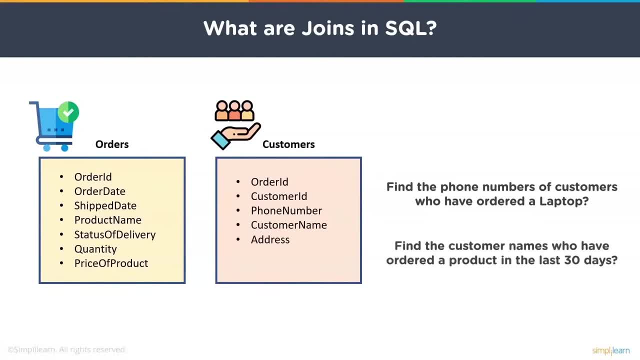 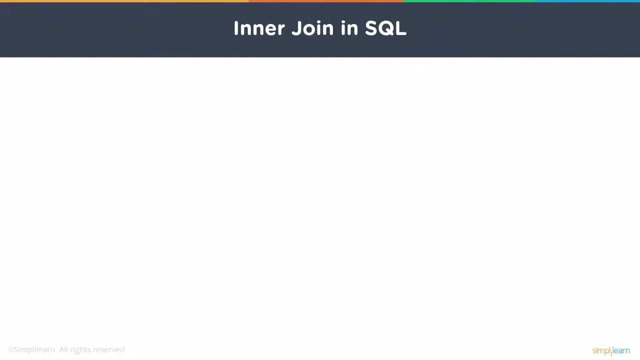 See It Here. So, Using A Joint Statement, You Can Find The Phone Numbers Of Customers Who Have Ordered A Laptop. Now We Have Different Types. 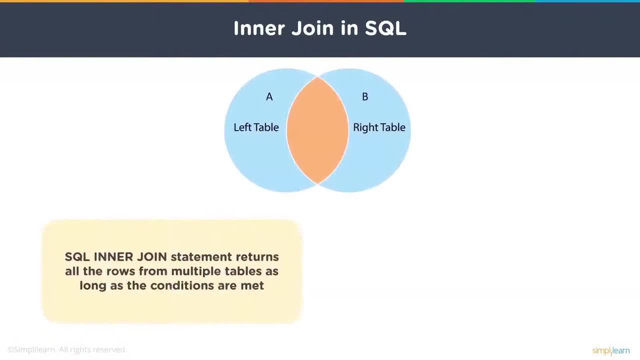 Of Joints One By One. So First We Have An Inner Joint, So The SQL Inner Joint Statement Returns All The Rows From Multiple Tables. 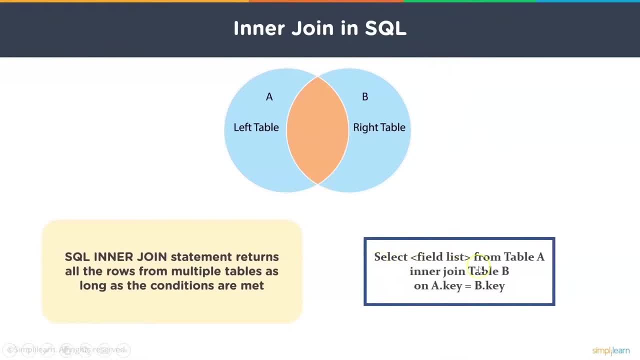 Now You Can See The Syntax Here. So We Have The Select Command And Then We Give The List Of Columns From Table A Which You 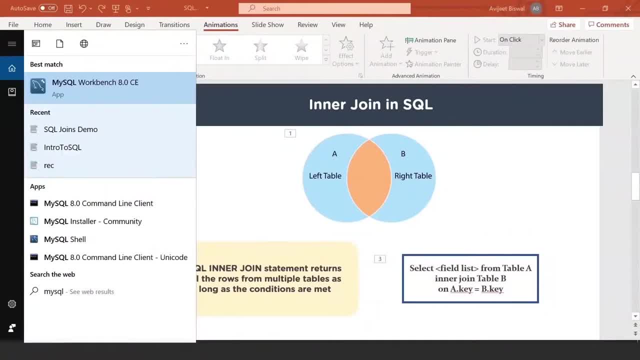 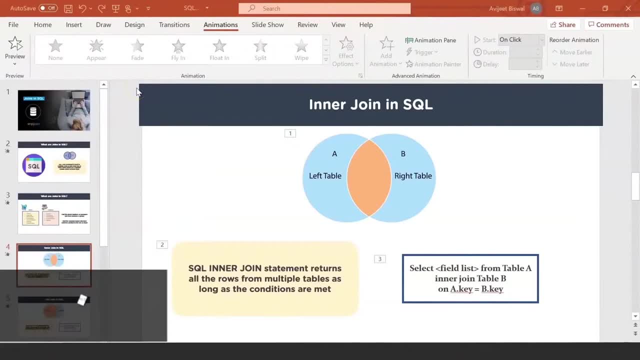 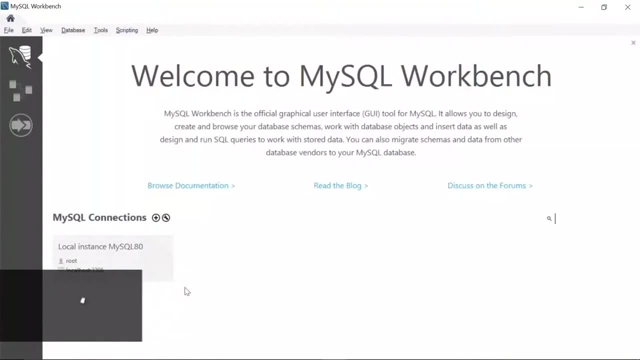 Can See Here SQL. You Can See I Have Got My SQL Workbench 8. Version Installed. I Click On. It Will Take Some Time To. 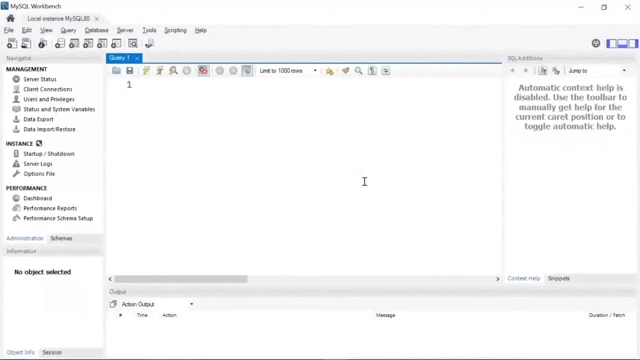 Open. Okay, I Click On This Local Instance. So First Of All, Let Me Go Ahead And Create A New Database. So I Write: Create Database. 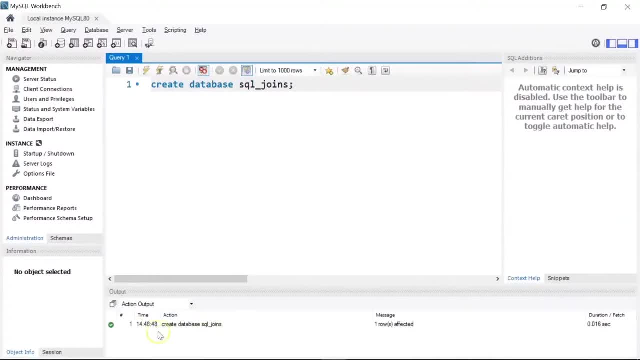 This Is Going To Be My Command, Followed By The Name Not Using Show Databases Command. If I Run It Here, You Can See I. 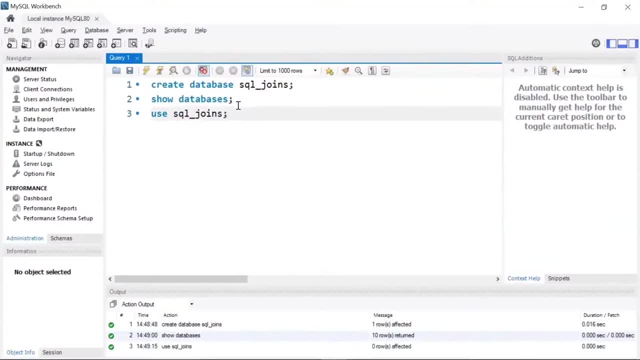 Have SQL Joins Database Created. Now I Use This Database So I Write, Use SQL Authors. So Let's Create Two Tables: Cricket And Football. So 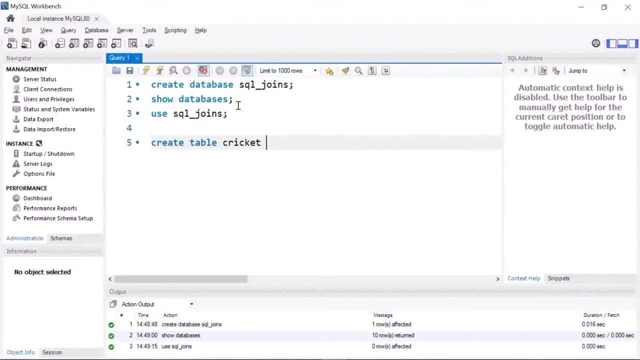 I Write Create Table And My Table Name Is Going To Be Cricket. Next I Am Going To Create Two Tables, So I Use The Auto. 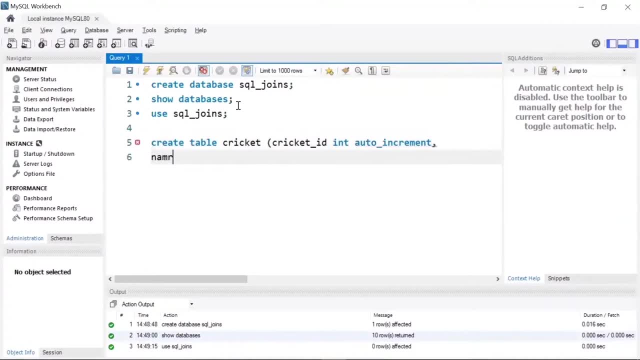 Increment Operator. I'm Using Auto Increment Because My Cricket Id Is Going To Be My Primary Key. Then I'm Going To Give The Cricket Underscore. 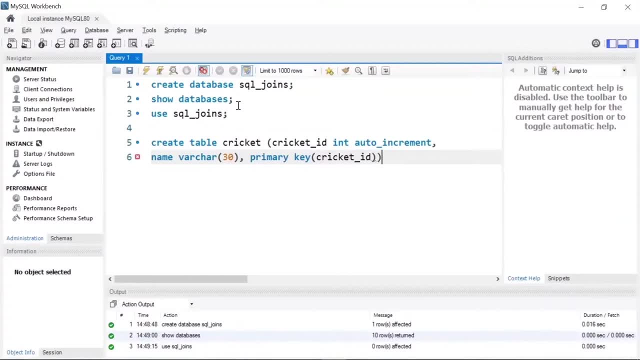 Id. Cricket Id Is Nothing But A Unique Identifier For Each Of The Players. Like You, Have Role Numbers In College. Okay, Let Me Just Run. 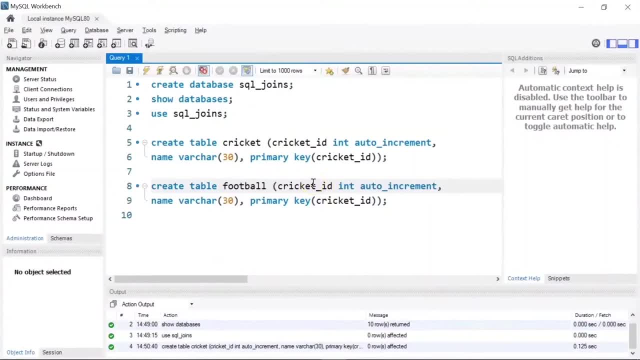 It The Information Of All The Students Who Are Part Of The Football Team And, Instead Of Cricket, I'm Going To Give This As Football. 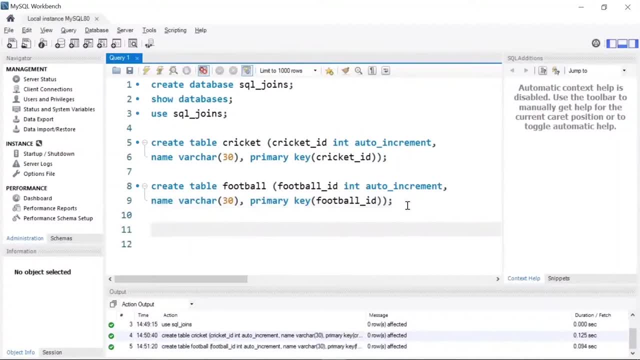 Id All Right And The Table. The Next Step Is To Insert A Few Player Names Into Both The Tables, So I'll Write My Insert. 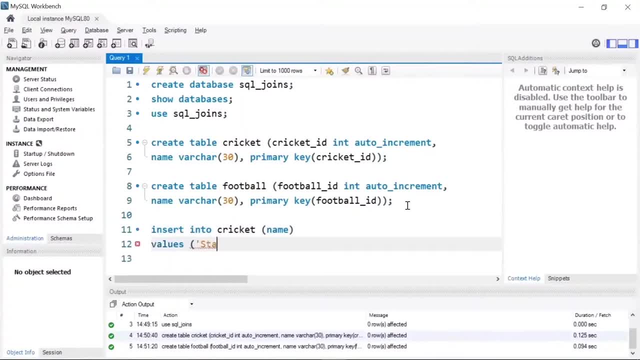 Into Command. First, Let's Load Some Data To Our. The Next Player I'll Choose Is, Let's Say, Michael. Similarly, I'll Add A Few More. 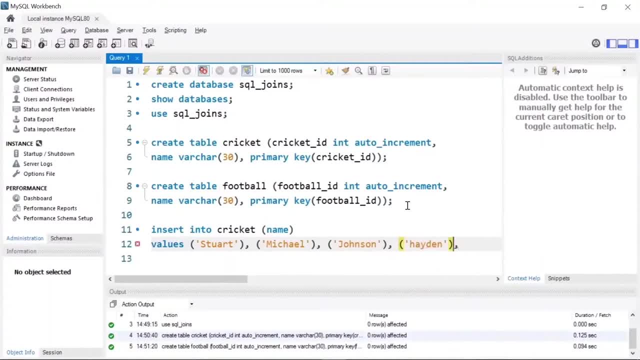 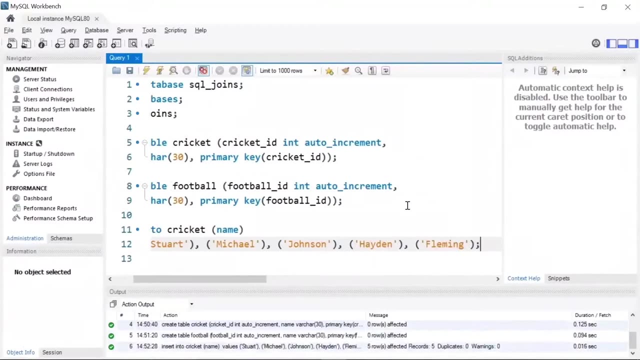 Let's Say We Have Johnson. The Fourth Player I'll Take Is, Let's Say, Hidden, And I'll Give A Semicolon And Run This Okay. 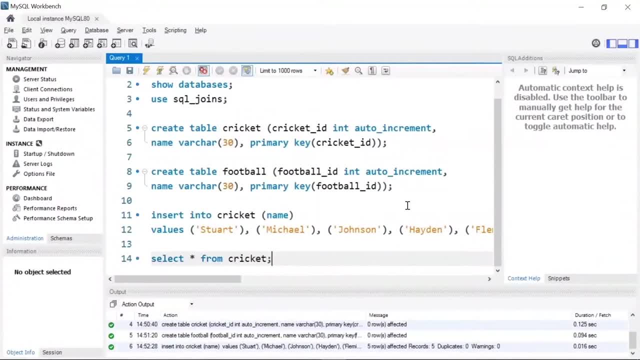 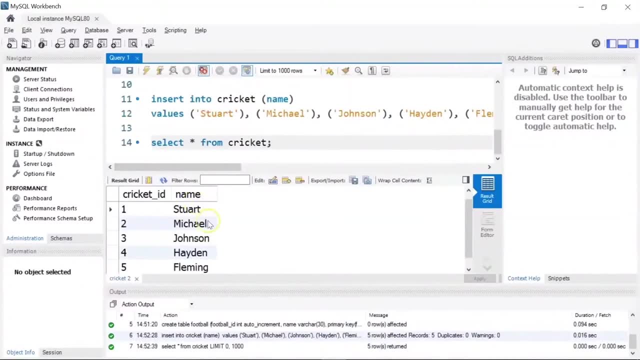 So Let Me Just Check If All The Values Were Inserted Properly For This. I'll Use Select Star From Table That For Our Football. 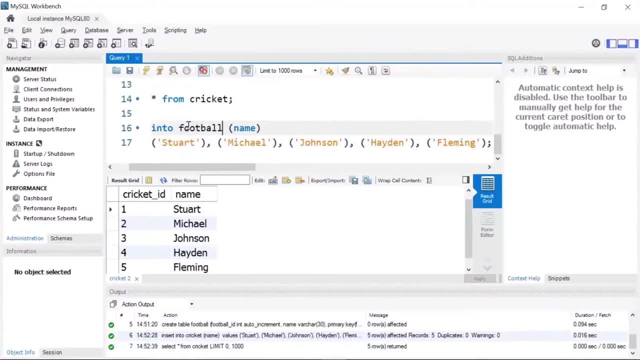 Table, So I'll Change This To Football And Obviously There Would Be Students Will Be Part Of Both Cricket And Football Team, So I'll Keep. 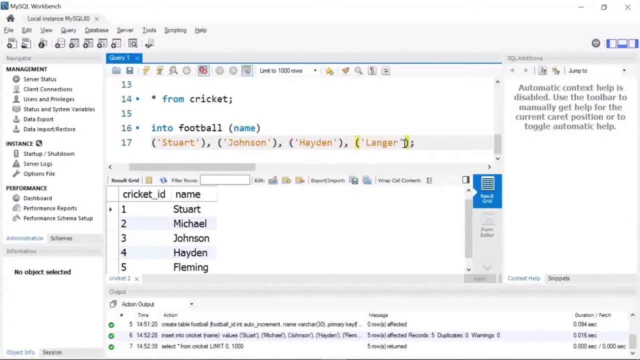 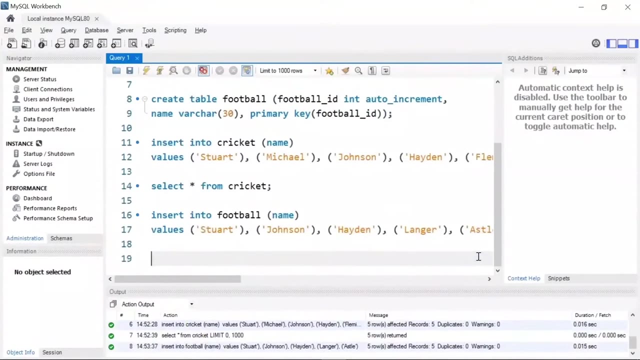 A Langer. And Let's Say We Have Another Player In The Football Team, That Is Aston. I'll Just Run It. Okay, You Can See. 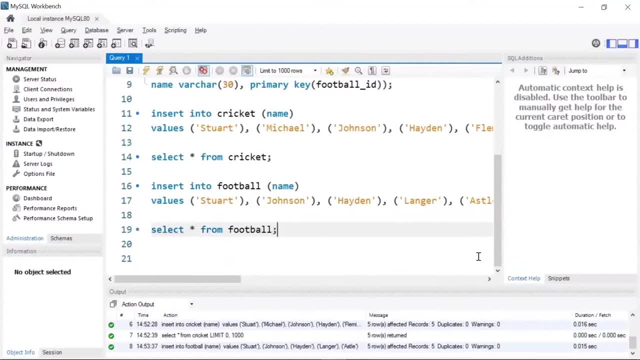 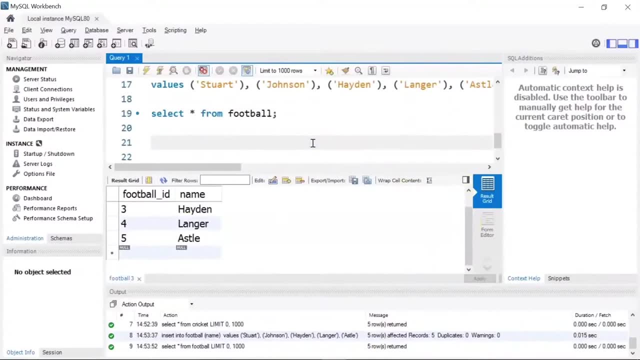 There Are No Errors, So We Have Five Players In The Football Team As Well. Okay, Now The Question Is Suppose You Want To Find The 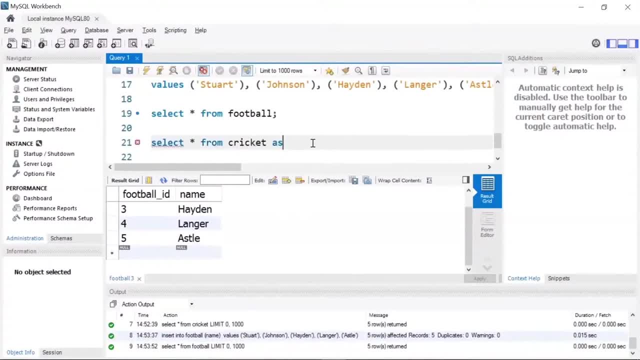 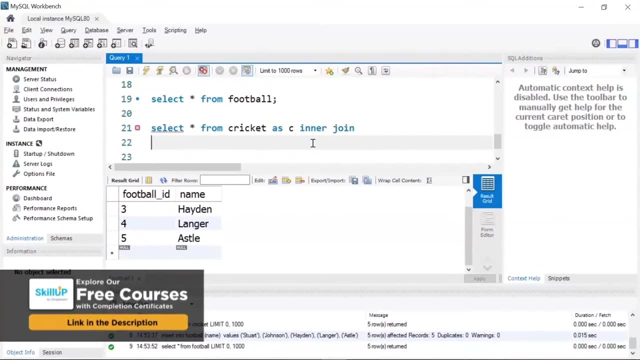 Students That Are Part Of Both The Cricket And Football. My Next Table Is Going To Be Football As F, Which Is An Alias Name For 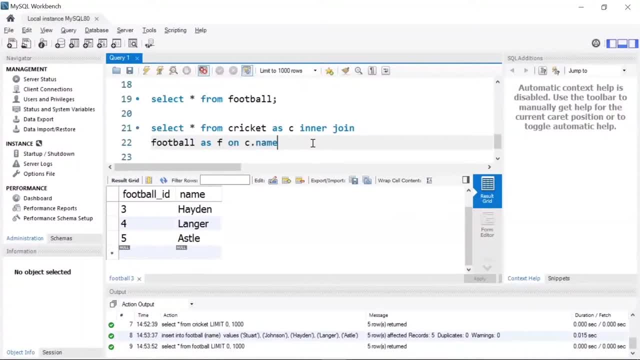 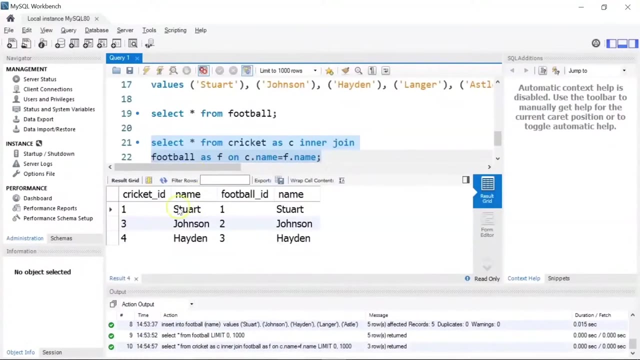 The Football Table, Then I'm Going To Use The On Command Or Operator, So Let's Just Run It. There You Go. So, Stuart Johnson And. 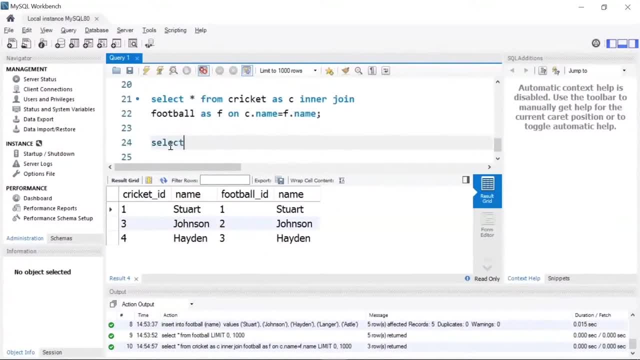 Hayden Are The Only Three Students Who Are Part Of Both The Teams. All Right, Now You Get The Football As F On F Name From: 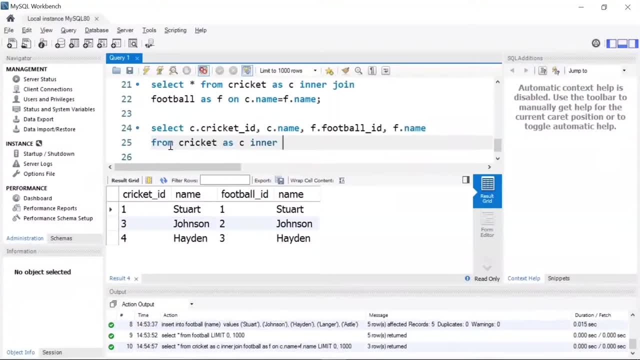 I'll Write Cricket As C Inner Join Football As F On. C Name Is Equal To F Name. Now, If You Are A Student, You. 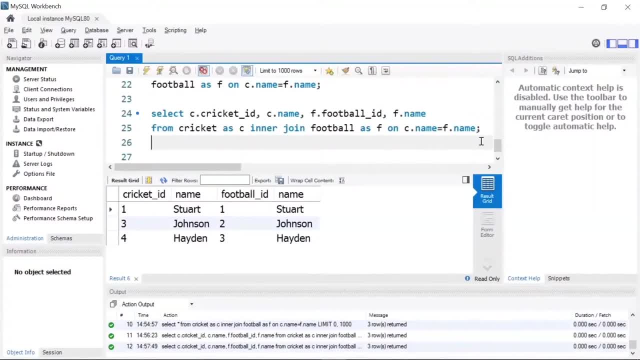 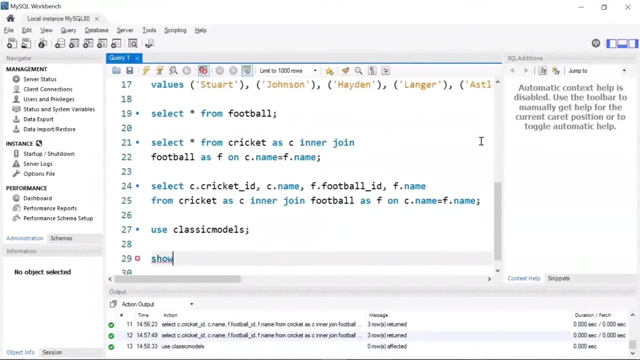 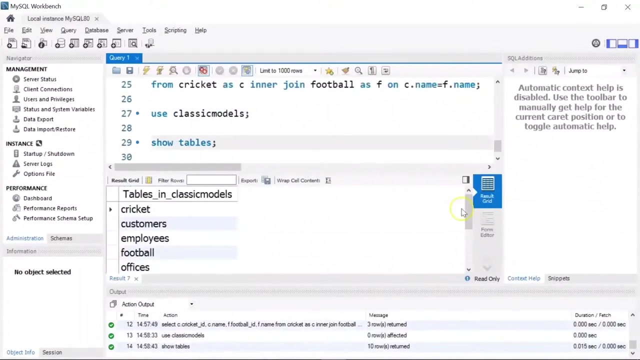 Are A Student. Now Let's Explore Another Example To Learn More About Inner Joins. So We Have A Database Called Classic Models. Let Me See. 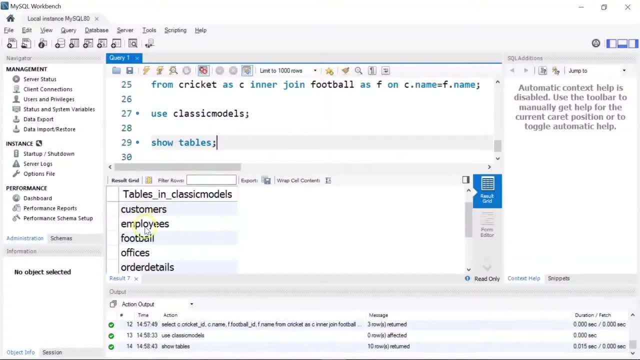 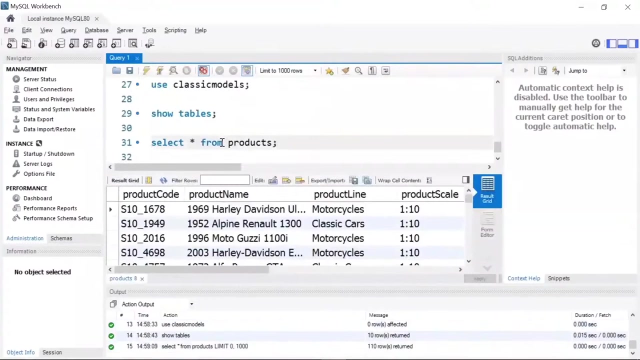 All Right. So Here You Can See, There Are Tables Like Customers, There's Employees Office, There's Office Details, Orders, Payments, Products And Product Lines As 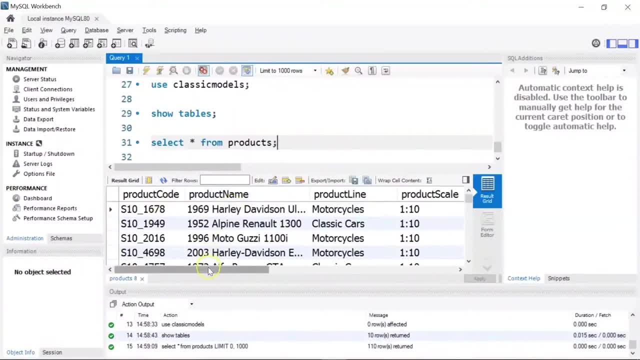 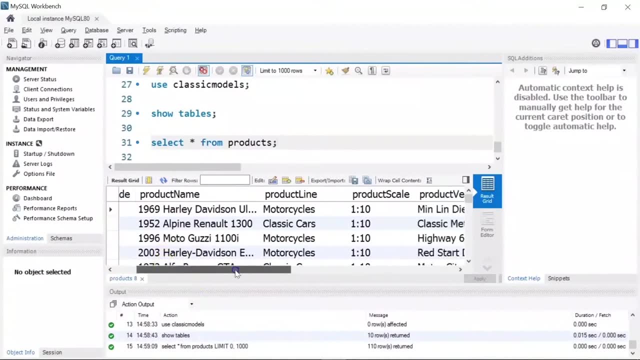 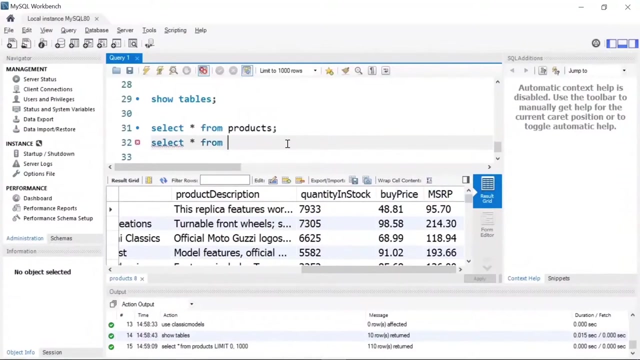 Well, All Right. Information About Different Product Names. You Have The Product Code Now This Product Code Is Unique. Here We Also Have The Product Vendor. 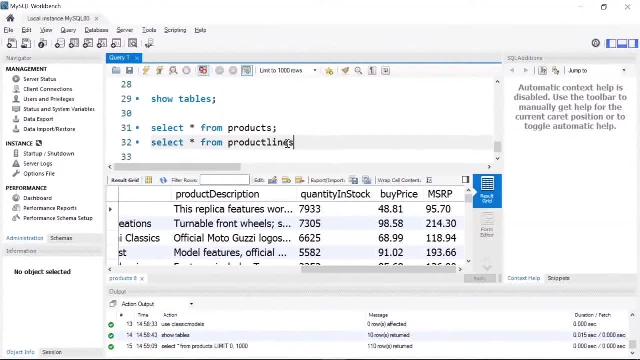 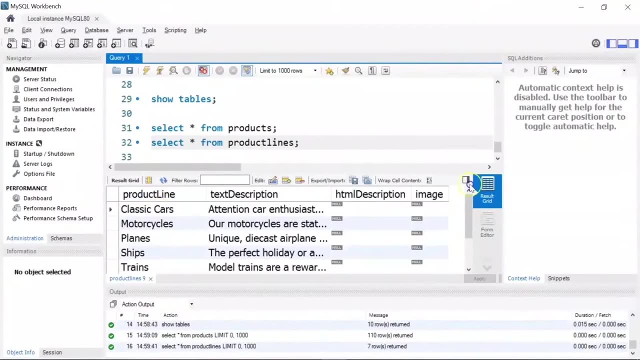 Little Description About The Product. Then We Have The Product Line, Which Is The Primary Key For This Table. Then We Have The Textual Description. 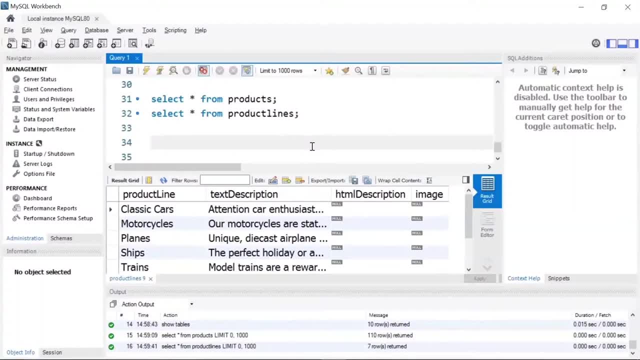 For Each Of The Products. This Is Basically Some Sort Of Columns, So We Choose My Columns As Product Code. Then We Have Product Name And 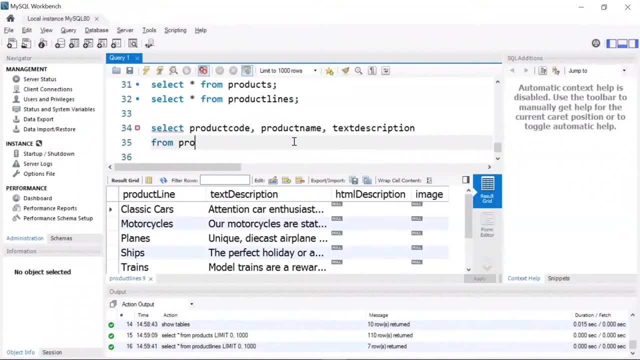 Let's Say, I Want The Text Description, So I'll Write This Column Name. Okay, Then I Can Use Using The Common Key Column, That Is: 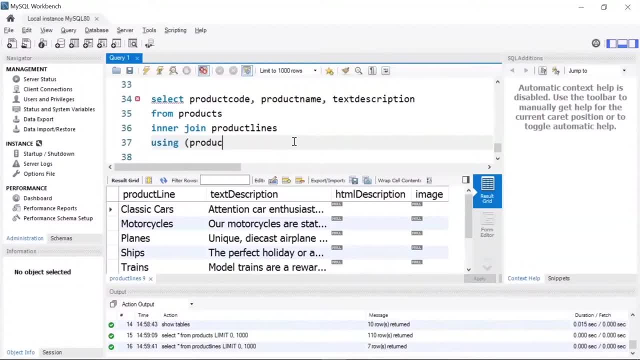 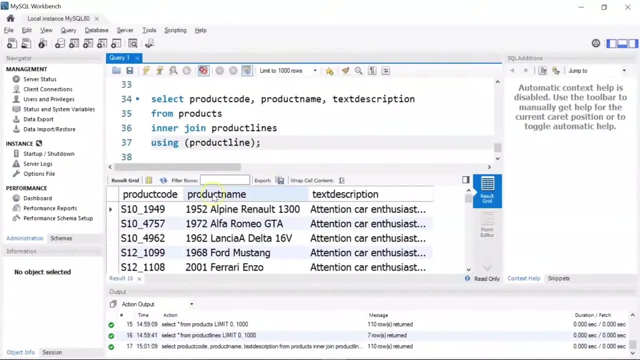 Product Line. Close The Bracket, I'll Give A Semicolon And If I Run It, There You Go. So You Can Do This By Joining. 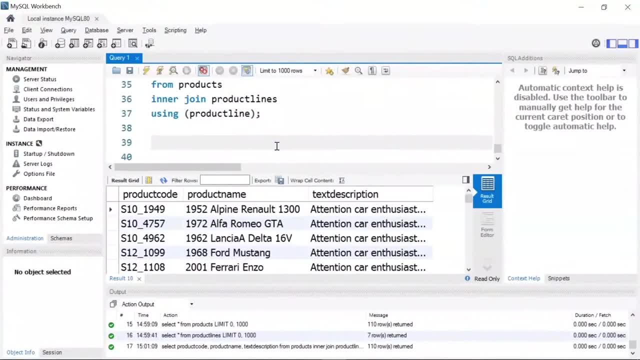 The Products Table And The Product Lines Table. All Right Now, Suppose You Want To Find The Revenue Generated From Each Product Order And The Order. 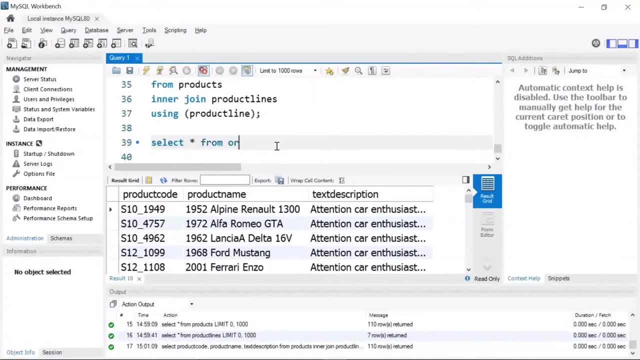 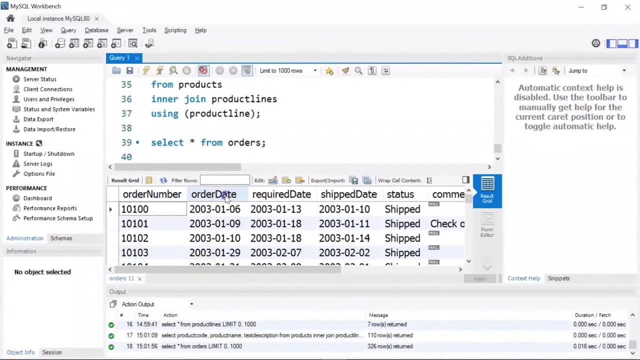 Details Table. So I'll Write Select Star From Orders By Run It You Can See It Has Information About The Order Number, The Date On. 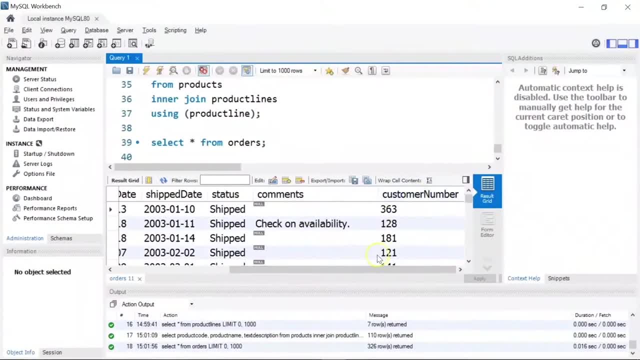 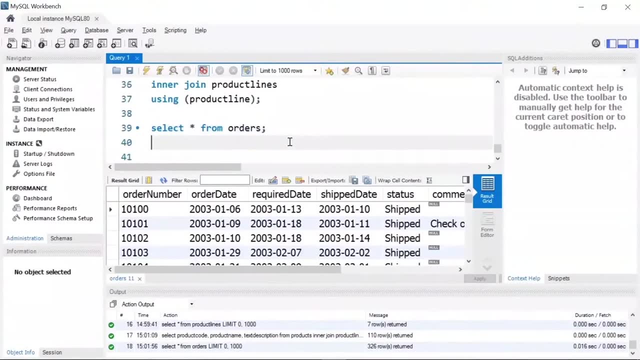 Which The Order Number? Who Order This Particular Product? Similarly, Let's Check What We Have Under Order Details. So I'll Write. Select Star From. 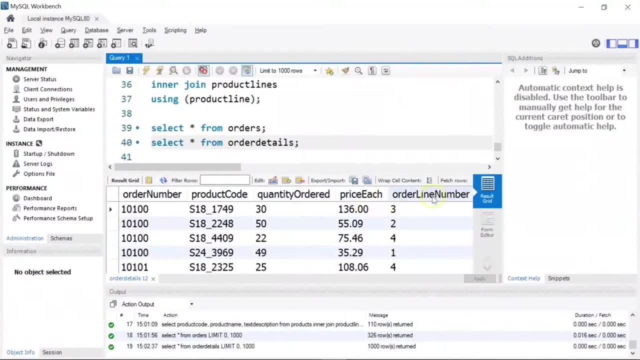 Order Details. If I Run It, You Can See An Order Details. Let's Perform An Inner Join, So I'll Write. Select O Order Number, Comma. 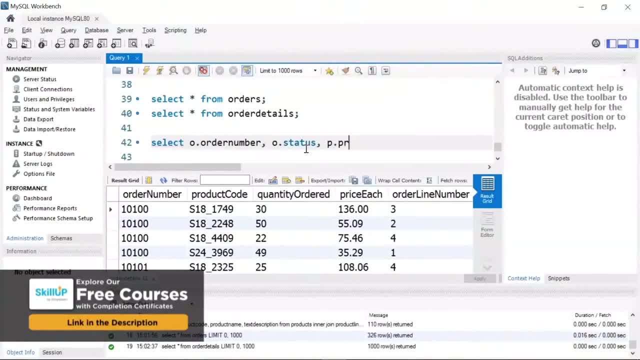 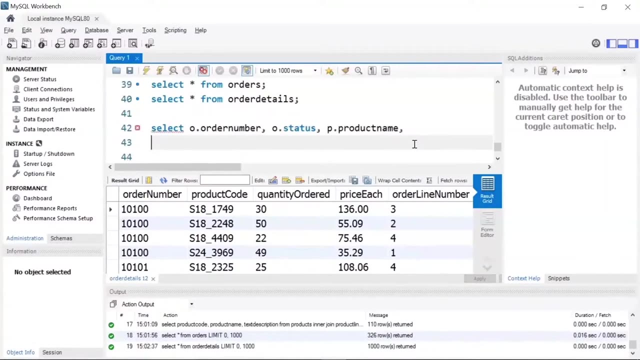 O Status: Comma. I Need The Product Name, Which I'll Take From The Products, And I'll Use O D For Order Details. Comma Since. 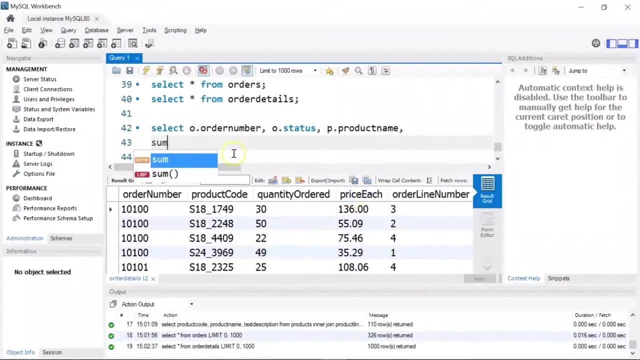 You Want To Find The Revenue. We Actually Need To Find The Product Of Quantity Ordered Into Price. I'll Use An Alias As Revenue Then. 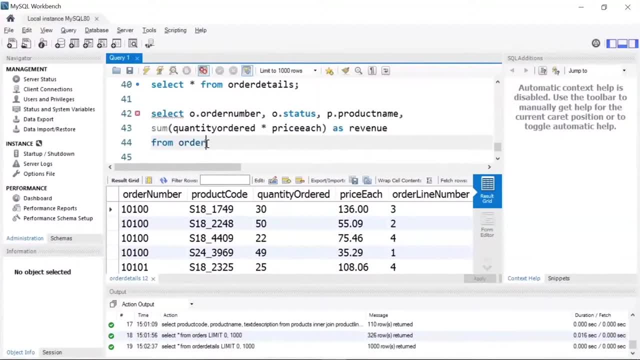 I'll Use My From Clause From Orders As O Inner Join Order Details, As I'll Use An Alias Name As O D On Order Number. 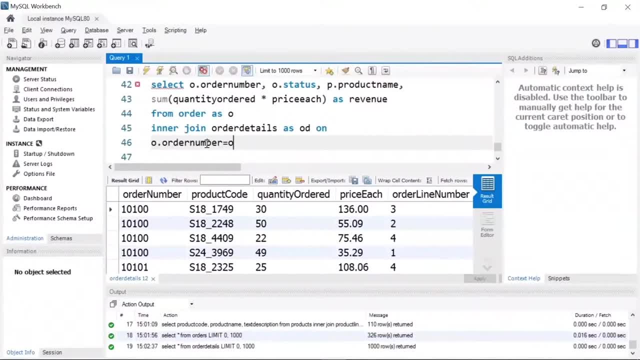 Is Equal To O D Dot Order Number. I'll Use Another Inner Join And This Time Will Join The Products Table, So I'll Use My. 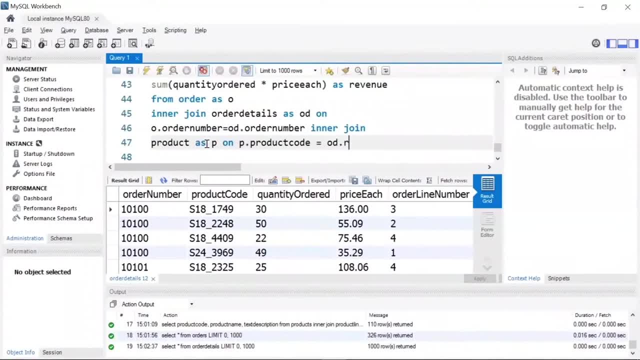 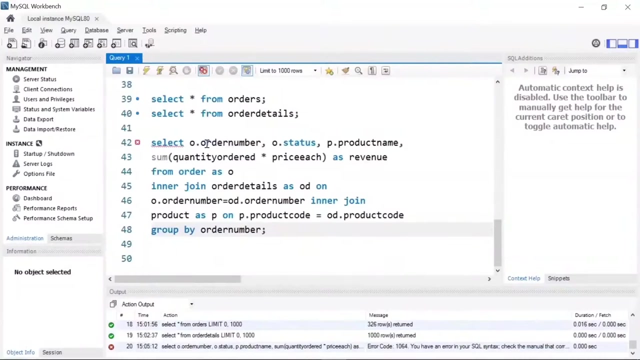 Order Name As O D Product Code And Finally, I'll Use The Group By Clause And Group It By Order Number. All Right, Let Me. 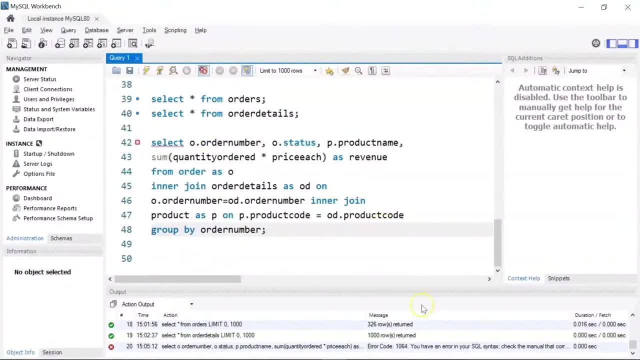 Run This. It Says You Have An Error In Your Sql Syntax. Check The Manual. All Right, Okay, I Think The Name Of The Tables Is. 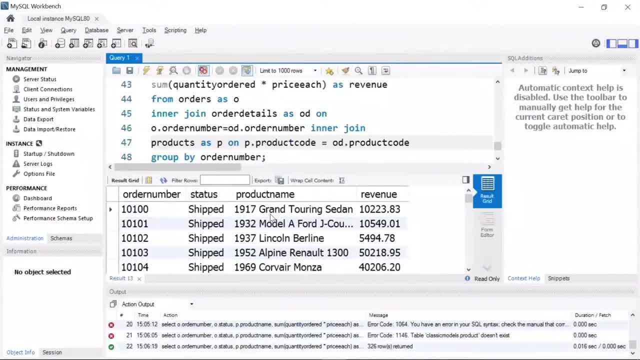 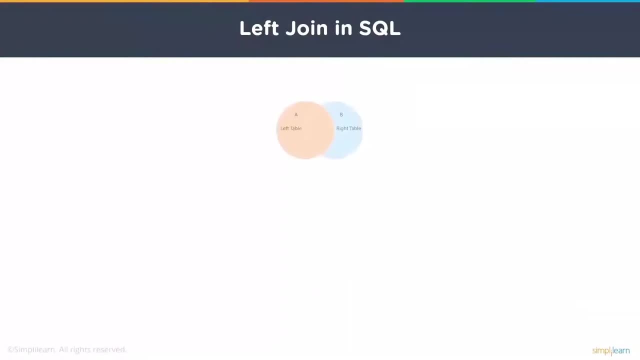 Actually Orders Are Not Order. We Have The Order Number, The Status, The Product Name And The Revenue. This We Got It Using Inner Join From. 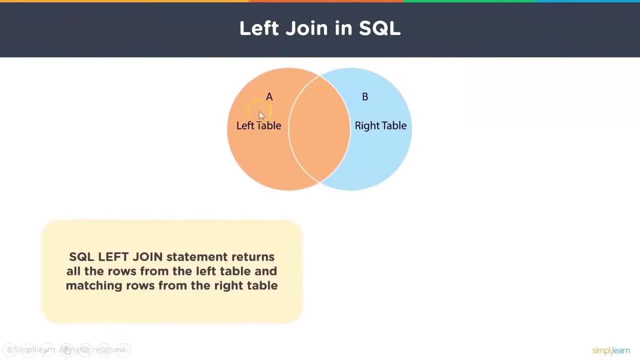 Three Different Tables Now Talking About Left Joins Is B, So You Can See This Overlapped Region And The Syntax For Sql: Left Join. 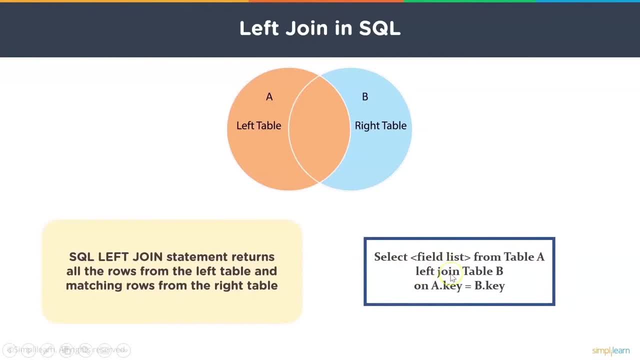 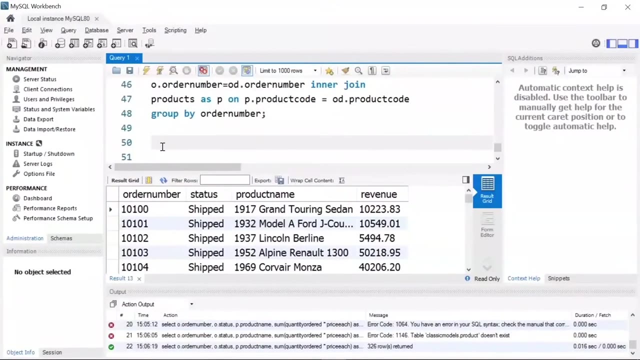 Is Something Like This: So You Have The Select Statement And Then You Can Find The Customers And Order. So If You Want To Find The 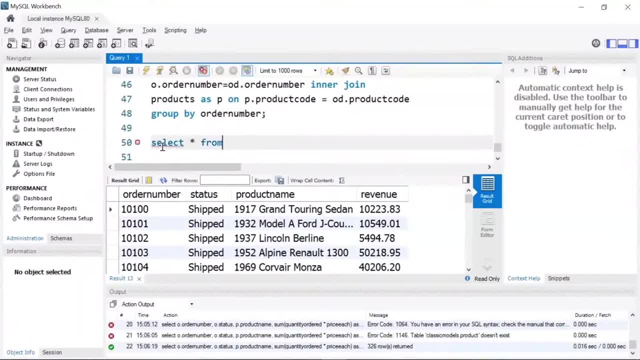 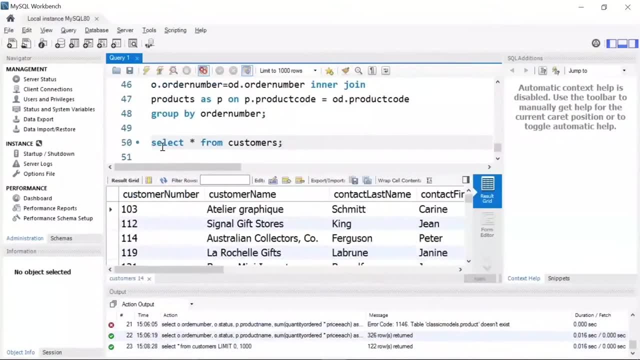 Customer Name And Their Order Id. You Can Use These Two Tables. So First Let Me Contact Last Name, The Contact First Name. We Have The. 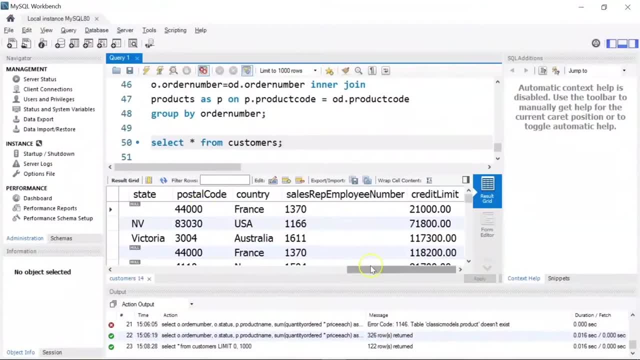 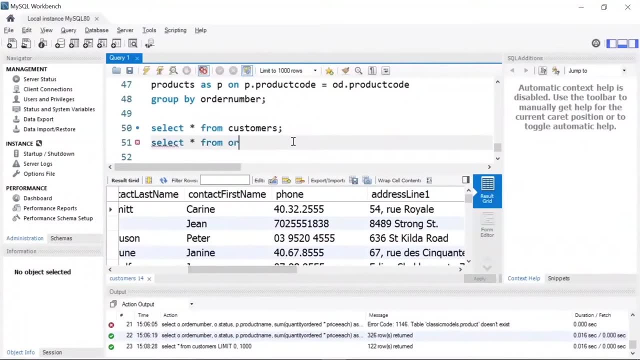 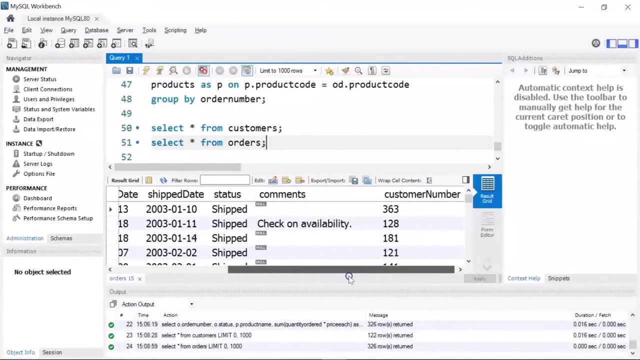 Phone Number. Then There's An Address Column. There Are Two Address Columns Actually. We Have The City Name, The Order Table. Okay, So Let's Perform. 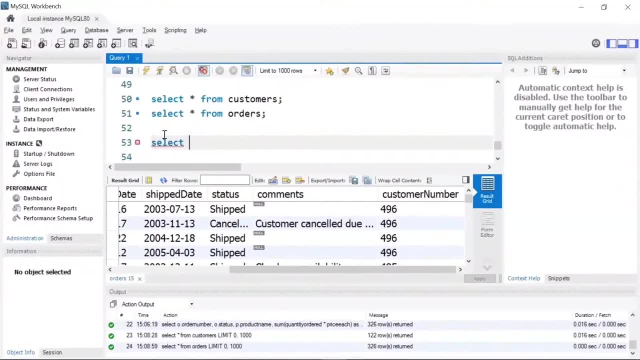 A Left Join. We Want To Find The Customer Name And Their Order Ids, So I'll Write Select C Customer Name. Or Let's Say: 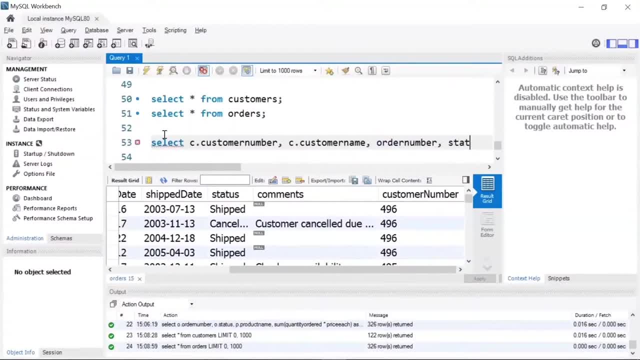 Number Column Which Is Present In The Orders Table And Let's Say, Also Want To See The Status, Then I'll Give My Left Table That. 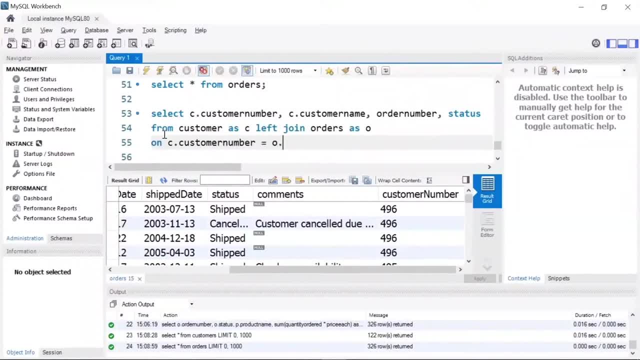 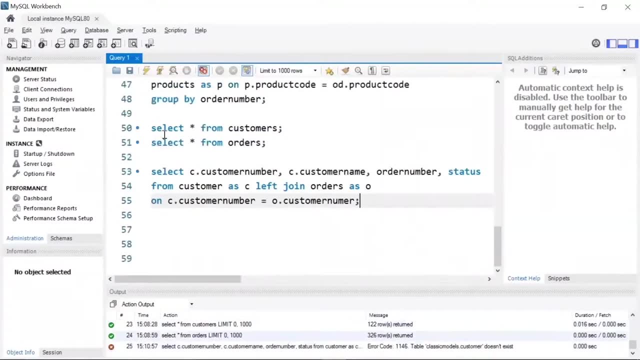 Is Customers As C O Dot Customer Number. Let's Run It Okay Again. There Is Some Problem. All Right, So The Table Name Is Customers. 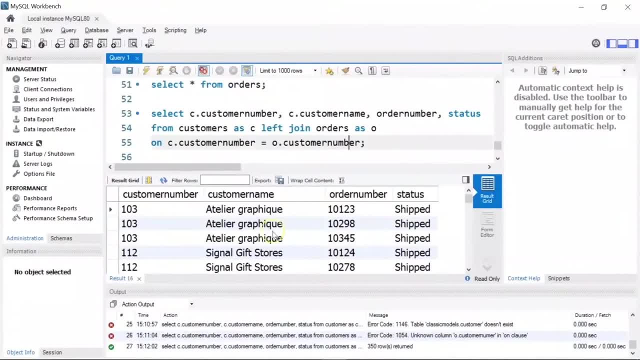 Let's Run It So There's Another Mistake Here. Then The Respective Customer Names. We Have The Order Number And The Status Of The Shipment. 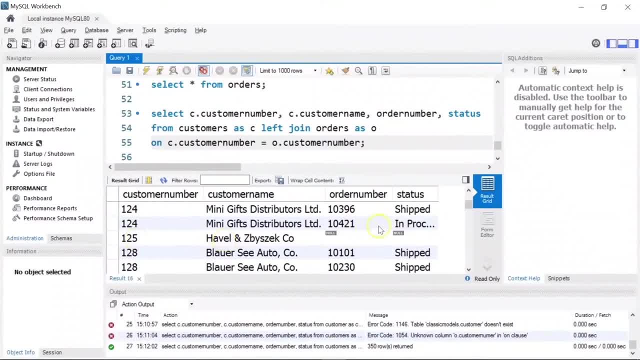 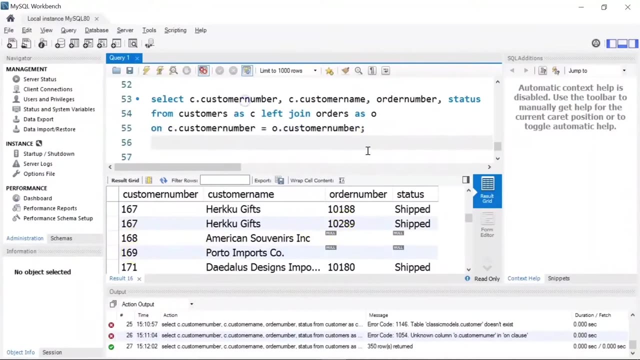 So If I Scroll Down, You'll Notice One Thing: There Are A Few Customer Number: 168. And 169.. There Were No Orders Available All. 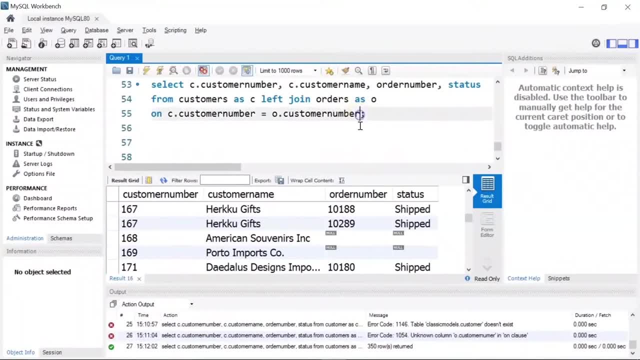 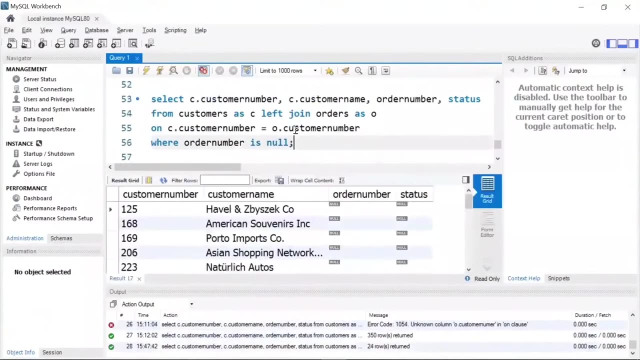 Right Now, To Check Those Customers Who Haven't Placed Any Orders, You Can Use The Null Operator. So Okay, So Here You Can See There. 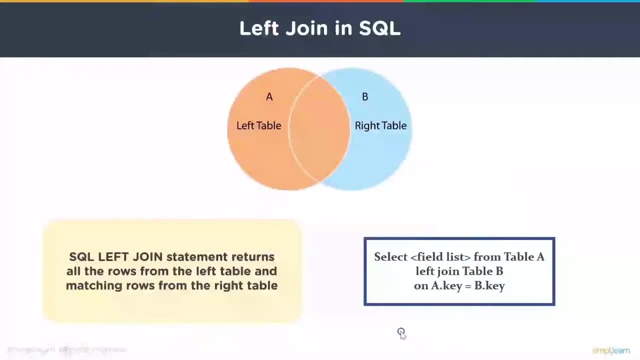 Are 24. Customers From The Table That Don't Have Any Orders In Their Names. Okay, Now Talking About Right Joins, So SQL Table And 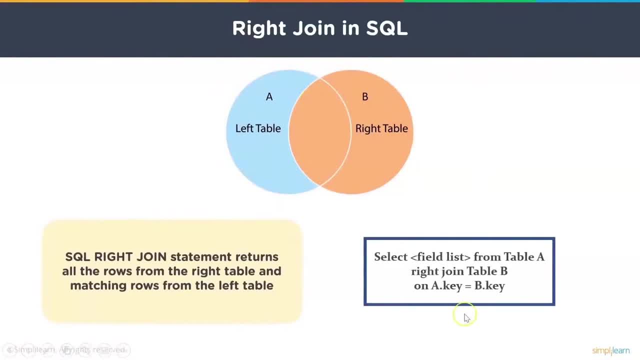 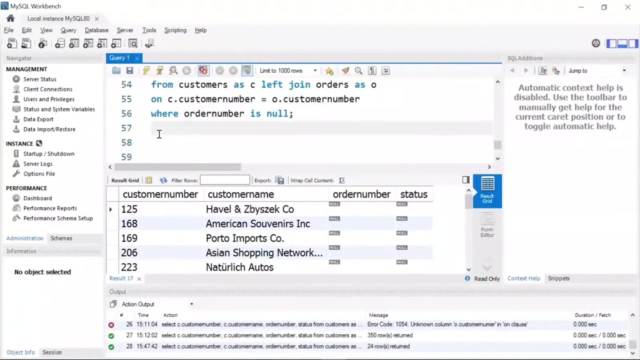 Only The Matching Rows From The Left Table. Now Talking About The Syntax. So Here You Can See. We Have The Select Statement, Followed By. 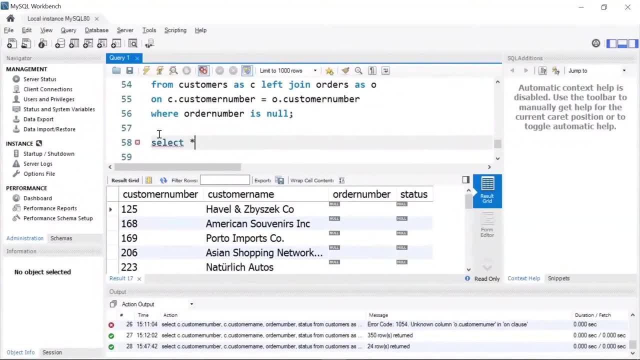 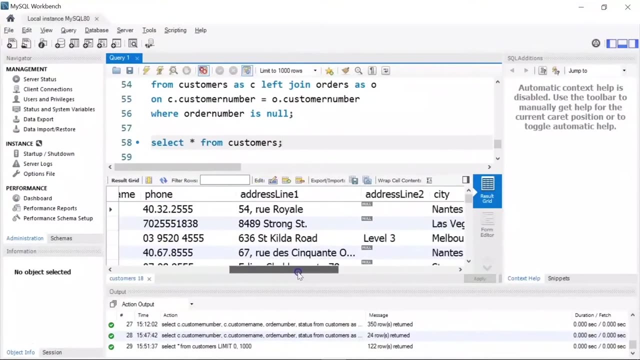 The Select The Rows Of Data That Are Present In The Customer Table First. So I'll Write Select Star From Customers. Let's Run It So. 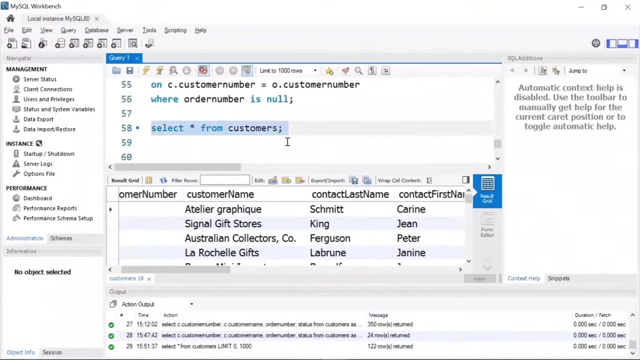 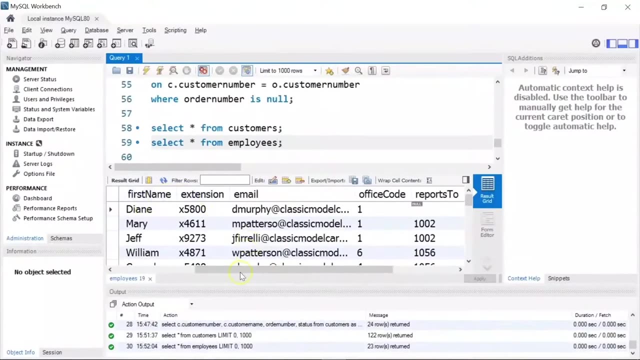 Here You Have The Customer Number. Here I'll Change Customers To Employees. Let's Run It Okay. So We Have The Employee Number, The Last Name. 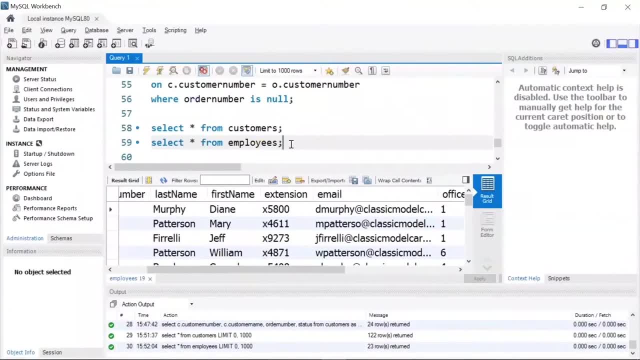 The First Name. We Have The Extension, The Email Id, The Name, The Customer And Employees. So Let Me Show You The Command, So I'll. 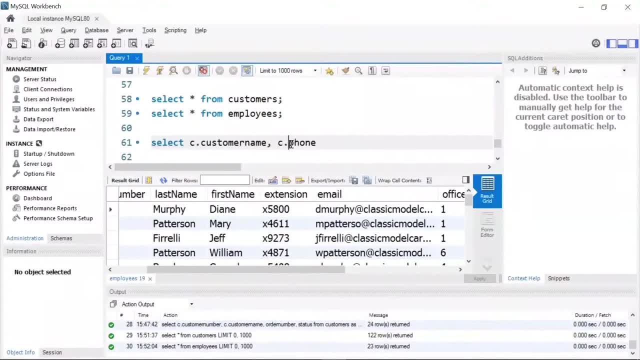 Write Select C Customer Name Comma. Then We Have C Dot Phone. I'll Give A Comma E Dot Email From Customers As C Right. 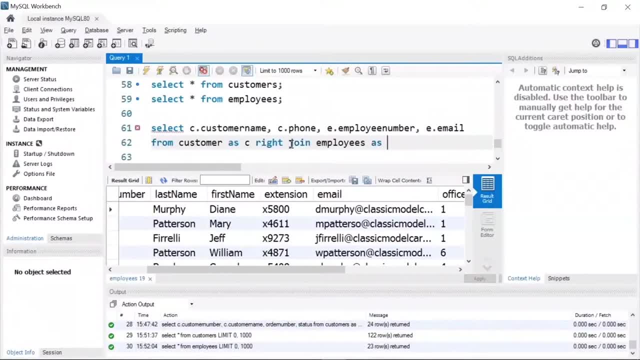 Join Employees As E On E Dot, My Common Key Column Is Employee Number Here, So I'll Write Sales Representatives- Employee Number, And I'm Also. 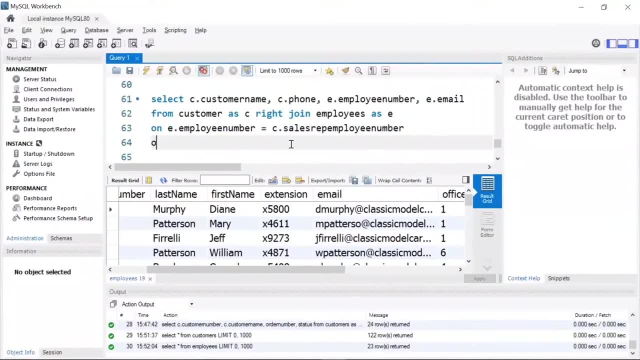 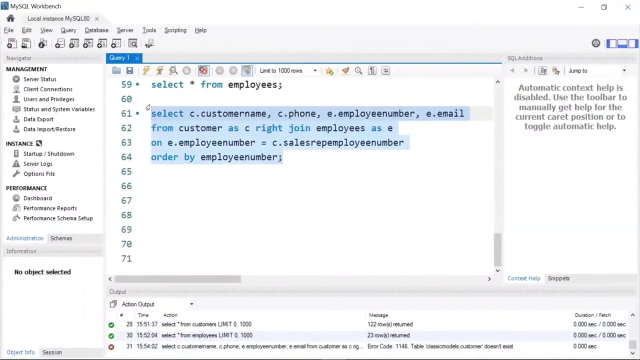 Going To Order It By The Employee Number Column. Okay, So You Can See. I Have My Customer Name Selected From Customers, So Let Me Run. 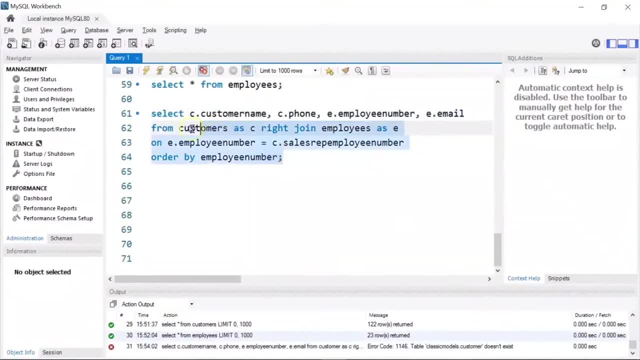 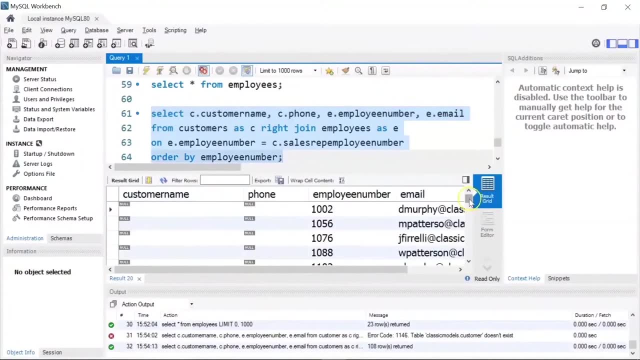 It. Okay, There's Some Problem? All Right, So The Table Name Is Customers. Actually, Let's Run It Once Again. There You Go, So You Have. 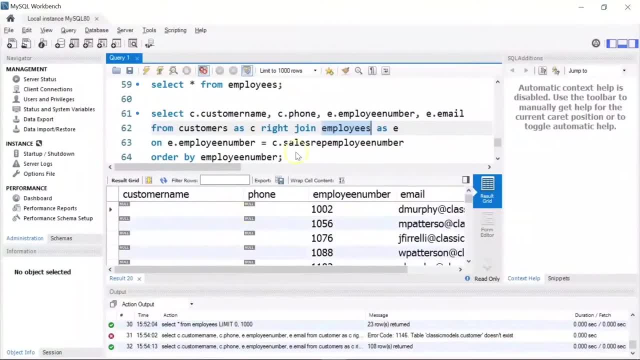 Customer Name And Phone Numbers Of The Customers From The Customer Table, Which Is Actually Your Left Table. So You Have A Few Employee Number Such 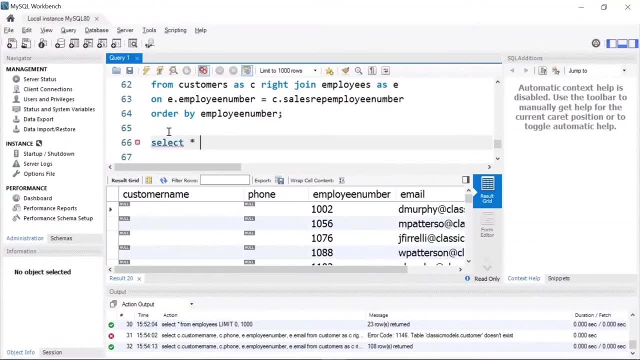 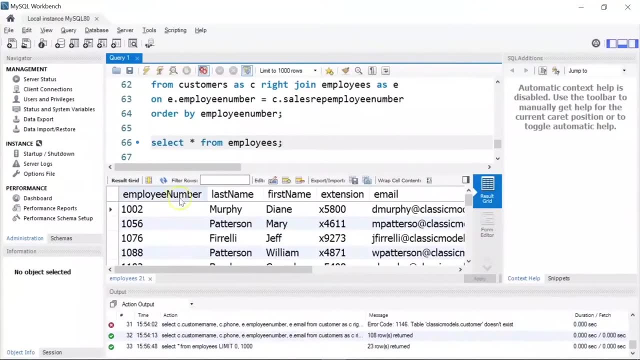 As 1002.. Table Called Employees. Let Me Show You The Table First. All Right, So Here You Can See We Have The Employee Number, The. 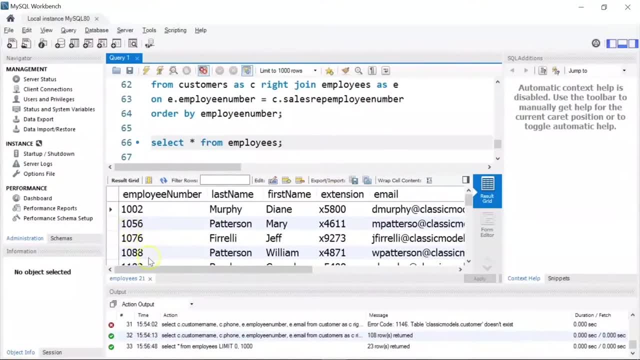 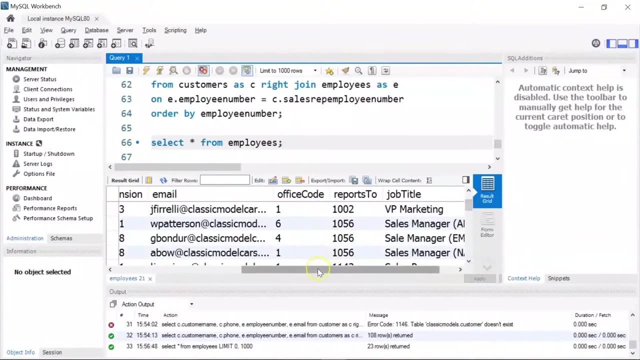 Last Name, The First Name Of Employee Number Is 1002.. So If You Check For 1002.. We Have Dane Murphy Then, If I Scroll. 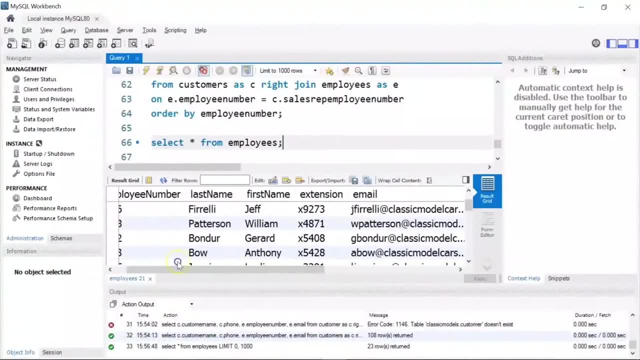 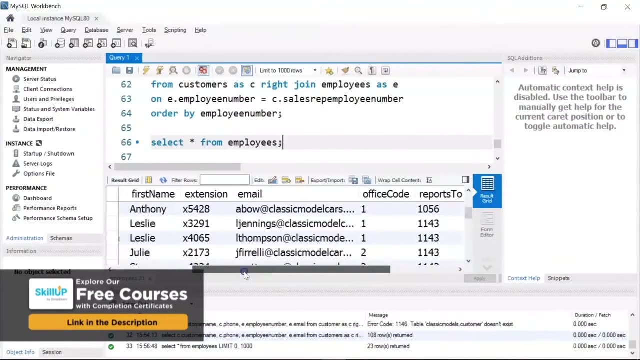 Down, Let's See For Employee Number 1102.. Yeah, For Employee Number 1102.. Scroll Down, Let's See For Employee Number 1188.. We Have. 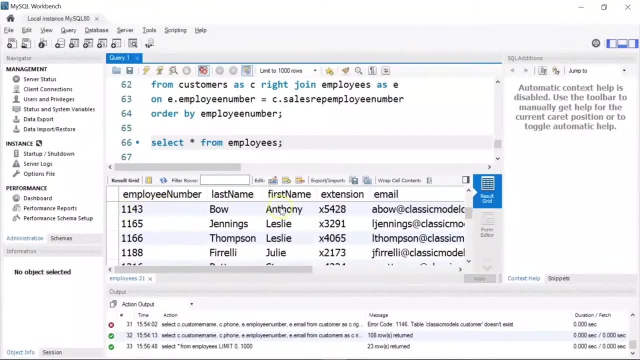 The Manager As 1143.. Now, If I Check The Table, At 1143.. We Have Anthony Bow, So So The So Let Me Show You. 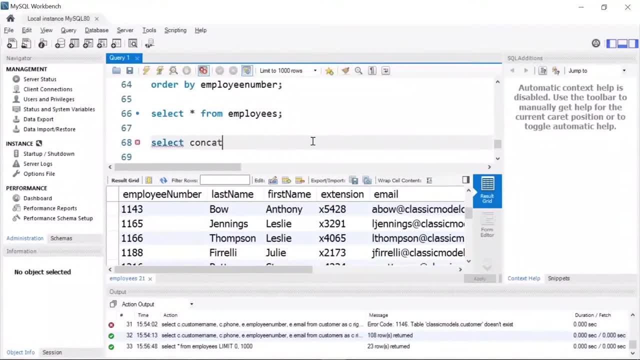 How To Join This Employees Table. I'll Write Select And Then I'm Going To Use A Function Called Concat Within Brackets. I'll Start With. 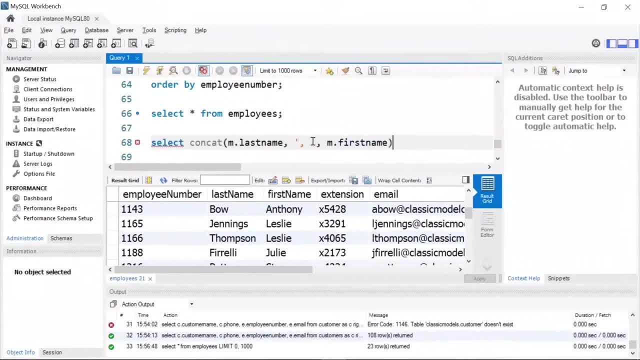 This Bracket. I'll Close This Bracket, And Then I'm Going To Give My Alias Name, Let's Say Manager Comma. Next I'm Going To 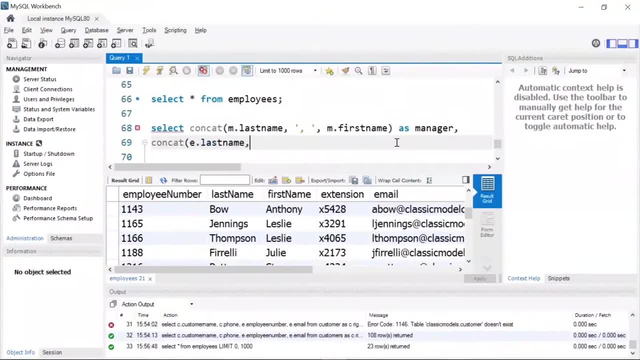 Concat, The Same Last Name And Single Quotes. I'll Give My Comma And Then I'll Write E Dot, First Name. I Close This Bracket. 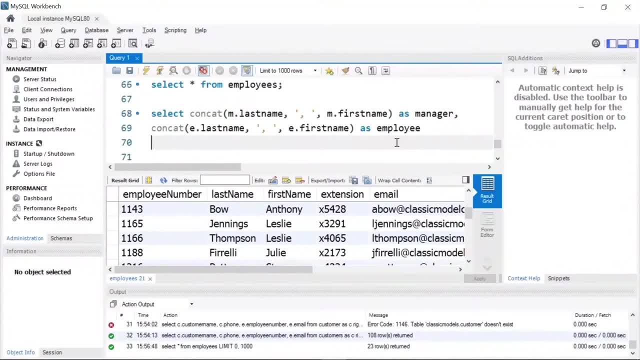 I'll Give An Alias As, Let's Say Employee From. I'll Write Employees Inner, Join Employees As M On, M Dot, I'll Use My Common. 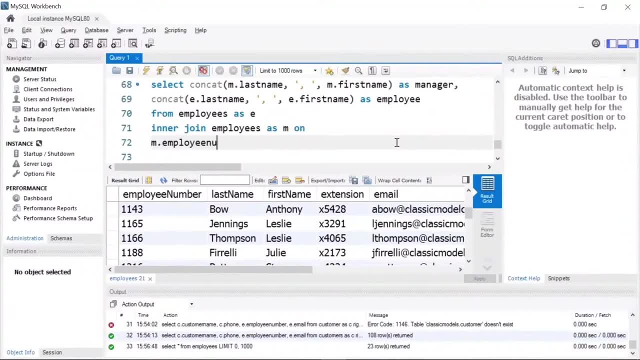 Key Column As Employee Number. So I'll Write M Dot Employee Column And Then I'll Order It By, Let's Say, Manager. Okay, Now Let's. 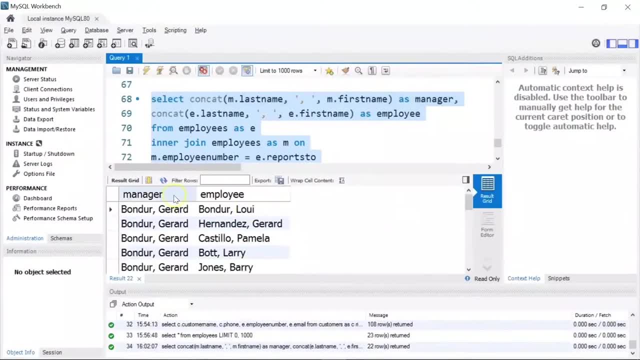 Run This, There You Go. So You Have Your Two Columns As Manager And Employee, So Employees Reporting To This Particular Manager. Similarly, We Have 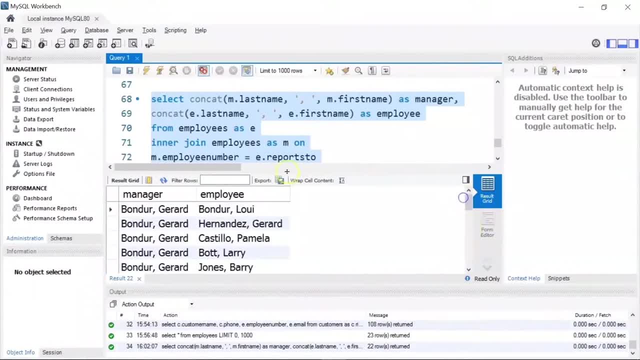 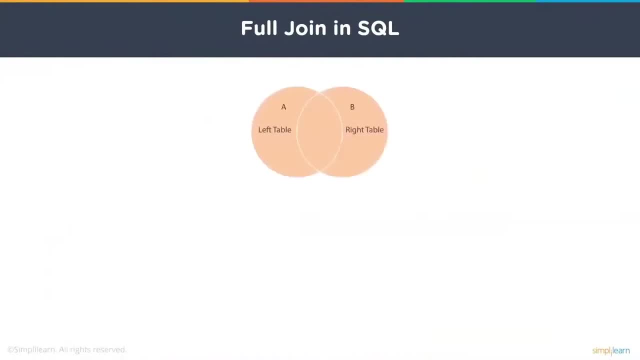 Our Manager As Anthony Bow, And We Have Different Employees Who Are Reporting To This Particular Manager, And So On. The By Default, So By. 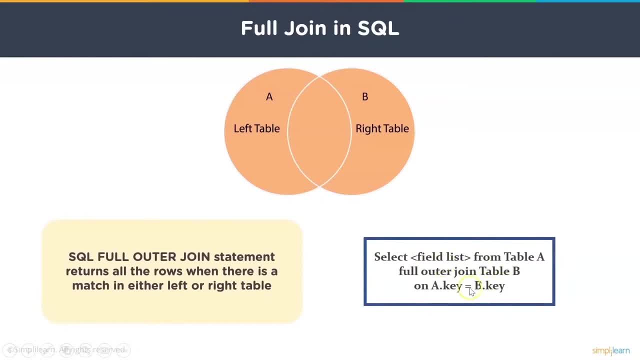 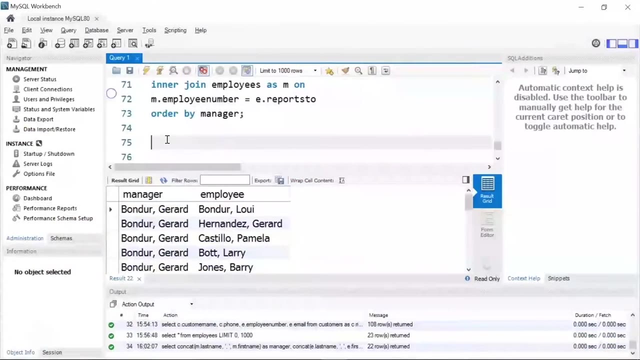 Default. This Is How The Syntax Of Full Outer Join Looks Like Now. This Statement Will Work On Other SQL Databases Like Microsoft SQL Server. 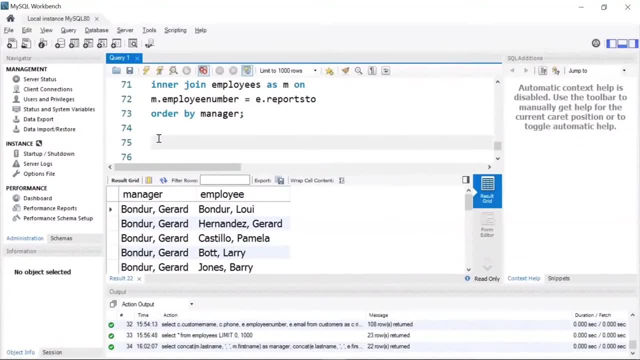 finally, we'll use a union operator. so the union operator is used to combine the result set of two or more select statements. so first of all let me write c dot customer name. so for this example i'm using the customer table and the order table, comma o dot order number. so i just want to know the 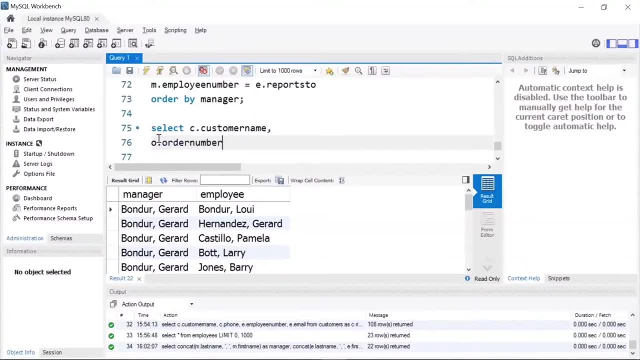 customer name and the order number related to the customer from. i have customers as C left join. I will write orders as who on C dot customer number equal to O dot customer number. let me just copy this and after this I am going to use my union operator. so union operator is used to merge results from: 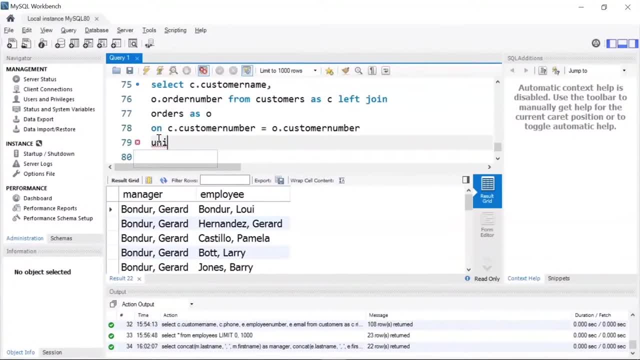 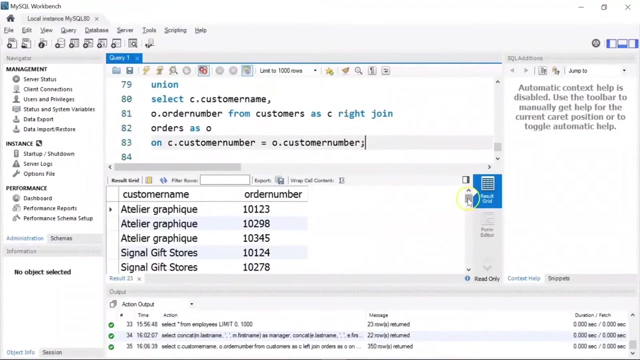 two or more tables. so basically this performs a vertical join, and next I am going to use my right join operation. so here, instead of left join, I will write right rest. all looks fine, let me just run it. there you go. so we have successfully run our full outer join operation. you can see we have the different customer names. 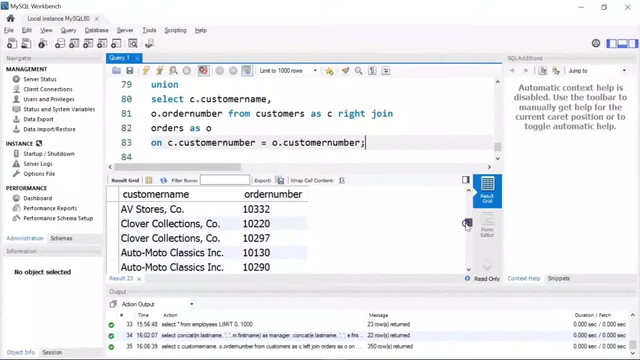 and the order that each customer had placed. all right, so that brings us to the end of the video of our demo session. so let me just run through whatever we did in this session. so first we created a database called SQL joins. then we created two tables. 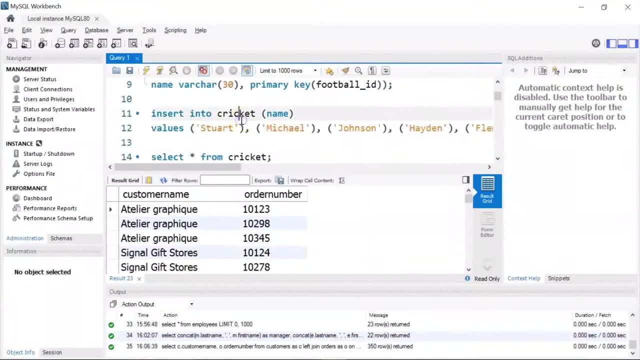 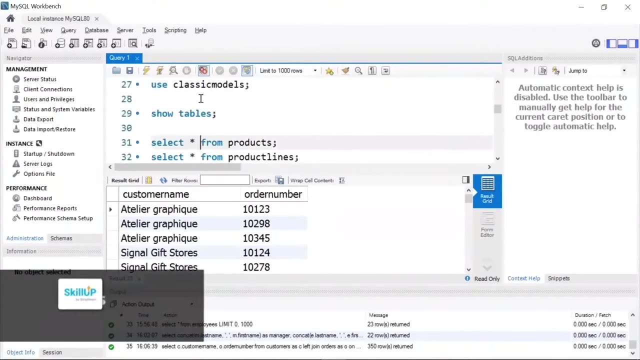 like cricket and football. then we had inserted a few rows to each of these tables. then we used this table to learn about inner join. next, we used a database called classic models. it had multiple tables. so we explored all of these tables. like products, there was product lines, orders, customers and 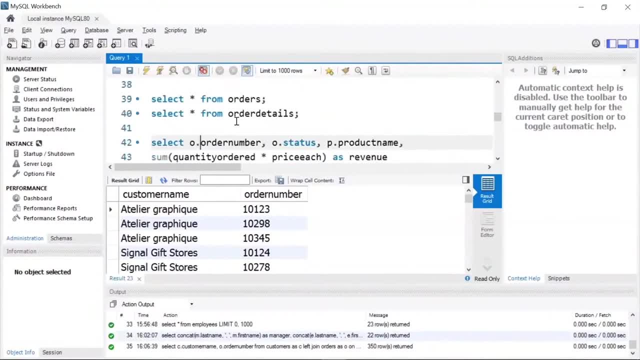 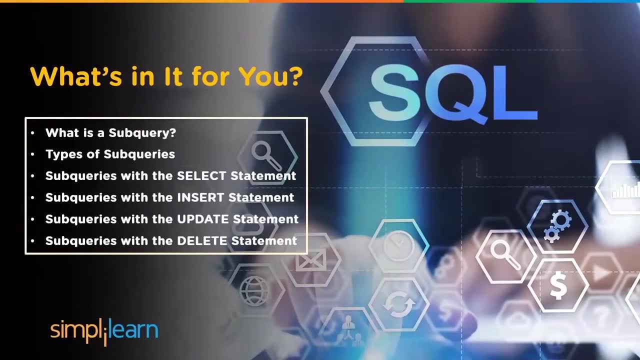 employees and learned how to use inner join, left join, self join, right join, as well as full outer join. in this video, we will learn what is a sub query and look at the different types of sub queries. then we learn sub queries with select statement, followed by sub queries with insert. 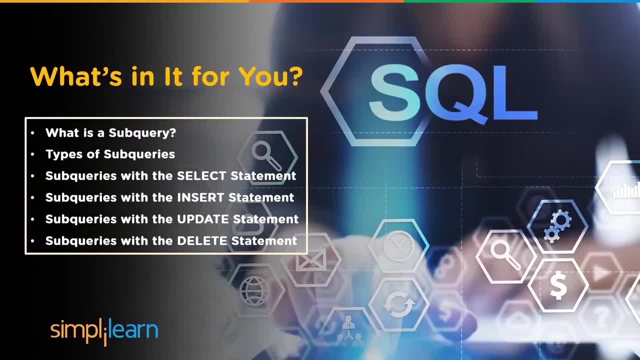 statement. moving further, we will learn sub queries with the update statement and finally we look at sub queries with delete statement. all this we will be doing on our mysql workbench. so before i begin, make sure to subscribe to the simply learn channel and hit the bell icon to never miss an update. so let's start with what is a sub query. 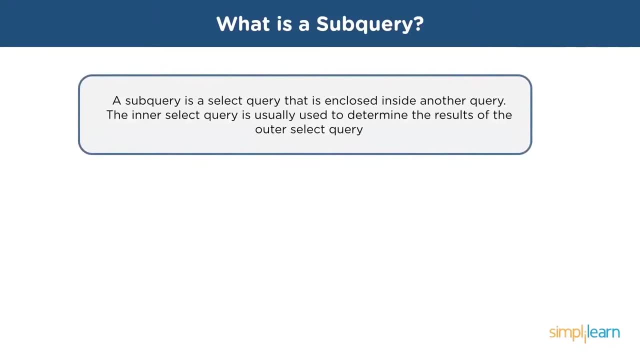 so a sub query is a select query that is enclosed inside another query. so if i show you, this is how the basic structure of a sub query looks like. so here, whatever is present inside the brackets is called as the inner query and whatever is present outside is called the outer query. 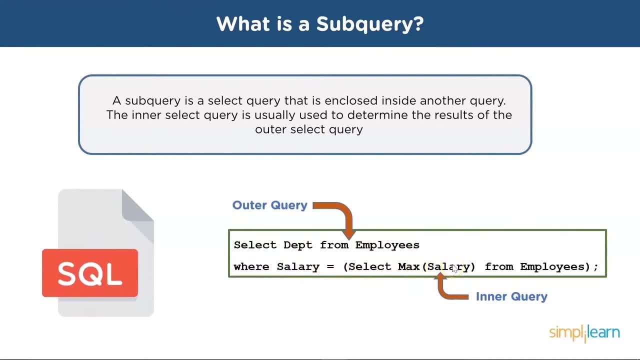 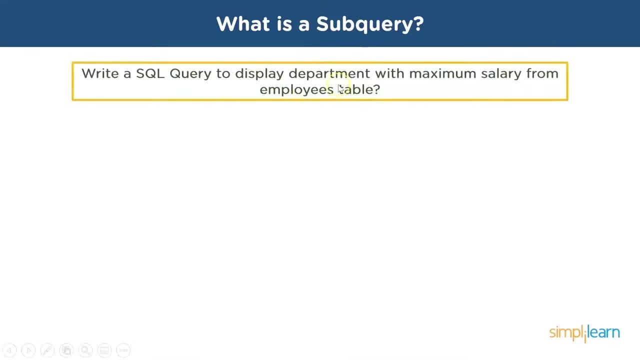 so first the inner query gets executed and the result is returned to the outer query, and then the outer query operation is performed. all right, now let's see an example. so we have a question at hand, which is to write a sql query to display department with maximum salary from. 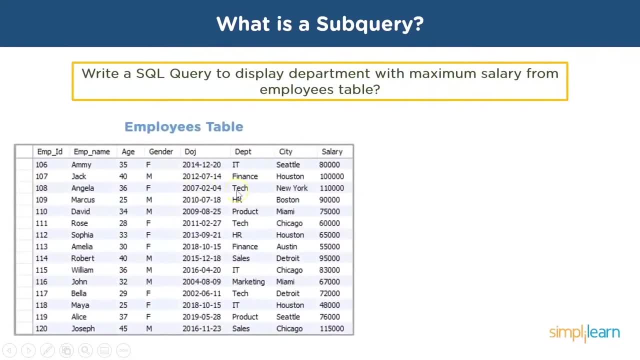 employees table. so this is how our employees table looks like. it has the employee id, the employee name, age, gender. we have the date of join department, city and salary. now to solve this query, my sub query would look like this. so i'll first select the department from my table, that is, employees. 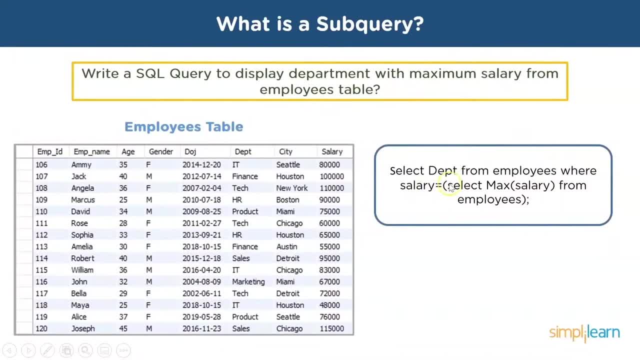 where i'll use the condition salary equal to and then i'll pass in my inner query, which is select max of salary from employees. so what this does is it will first return the maximum salary of the employees in the table, then our outer query will be the salary that is required for the table. 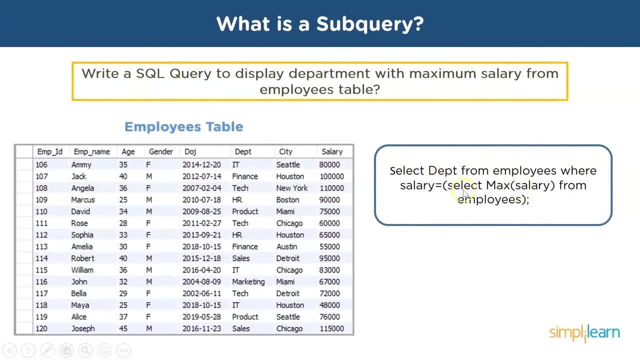 will get executed based on the salary returned from the inner query. so here the output is: department sales has the maximum salary. so one of the employees from the sales department earns the highest or the maximum salary. if you see, in our table the employee is joseph, who earns. 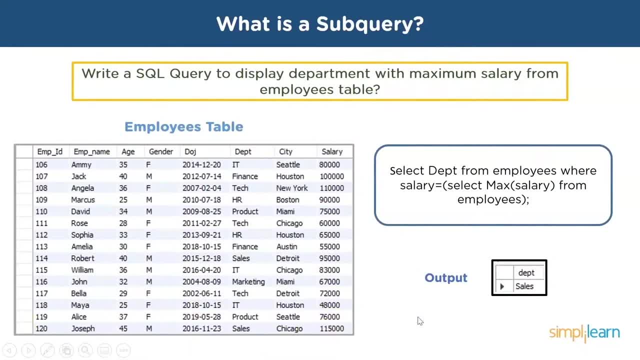 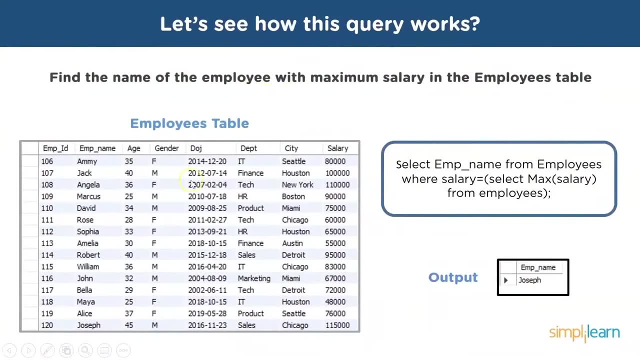 hundred and fifteen thousand dollars. all right, and joseph is from the sales department. now let's see how this query works. so here we have another question, which is to find the name of the employee with maximum salary in the employees table. so this is our previous employees. 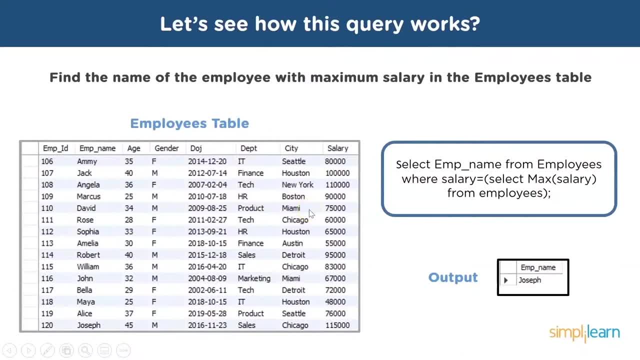 table that we saw and to find the employee who has the maximum salary. my sub query would look something like this: so i'm selecting the employee name from my table, that is, employees, where the employee name is from the employees table, and i'm selecting the employee name from the. 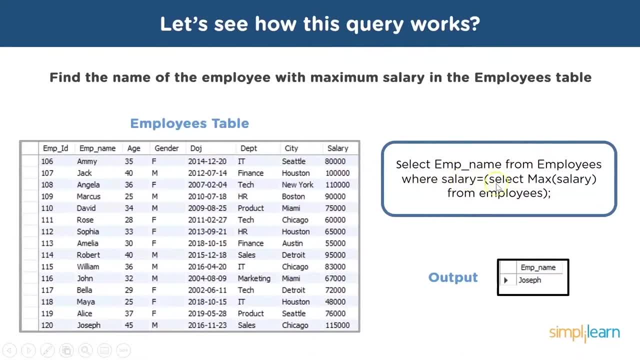 employee. i'm using the condition salary equal to and then i'm passing in my sub query or the inner query. so first i'm selecting the maximum salary. this will return a particular value, that is, the highest salary from the table. and if you see our table, the highest salary is hundred and 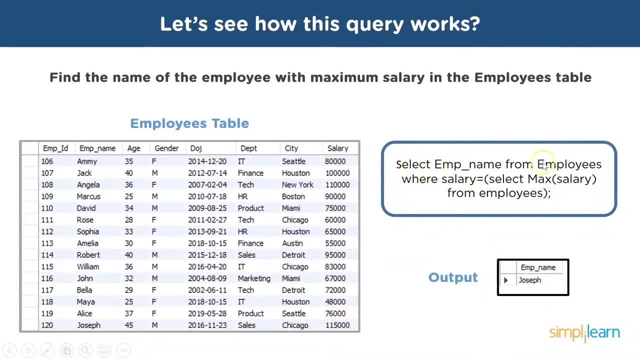 fifteen thousand dollars. so our query becomes: select employee name from employees where salary equal to hundred and fifteen thousand dollars. so the employee name is joseph here, and that's the output. now, if you want to break it down, you can do that by selecting the employee name from the 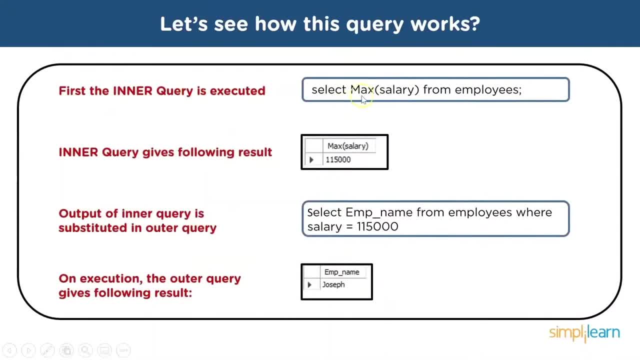 table. here you can see: first the inner query gets executed. so our sql query will first execute the inner query that is present inside brackets. select maximum salary from employees. the result is hundred and fifteen thousand dollars and then, based on the return result, our outer query gets executed. 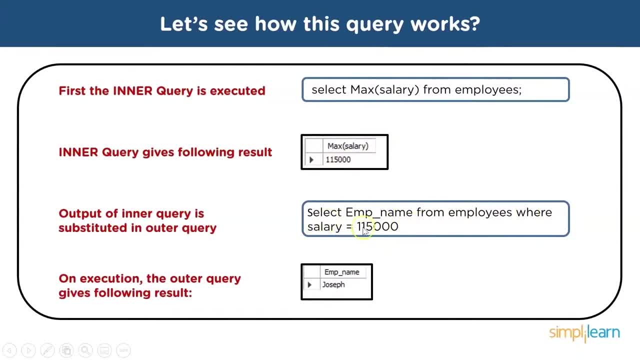 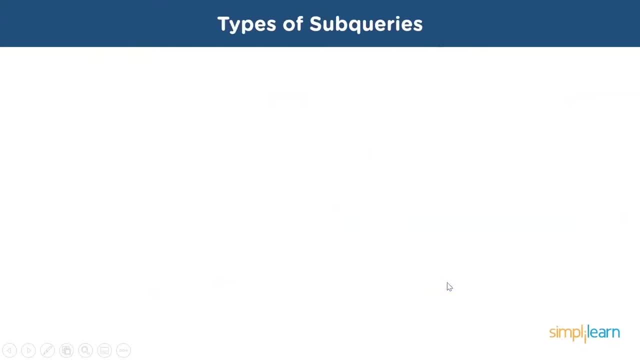 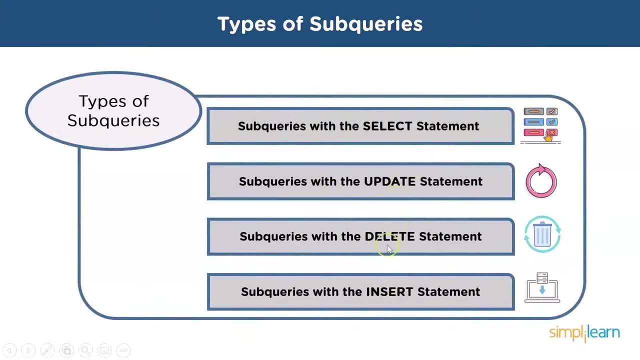 so the query becomes select employee name from employees where salary equal to hundred and fifteen thousand dollars and that employee is joseph. all right, now we'll learn the different sub queries so you can write sub queries using select statement, update statement, delete and insert statement. we'll explore each of this with the help of example on my mysql workbench. 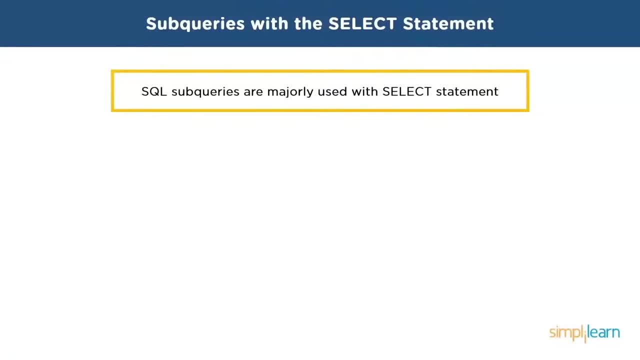 so let's learn sub queries with the select statement. so sub queries are majorly used with the select statement. and this is how the syntax looks like: you select the column name from the table name, then you have the where condition, followed by the columns that you want to pass the 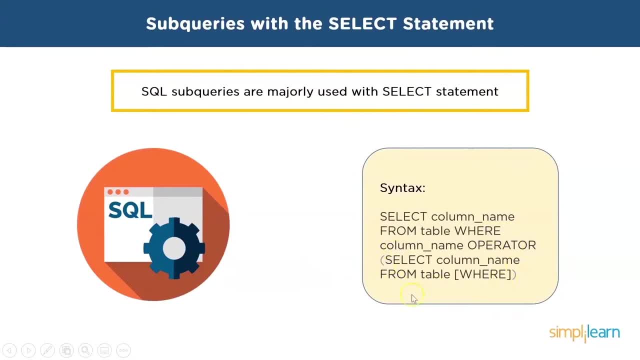 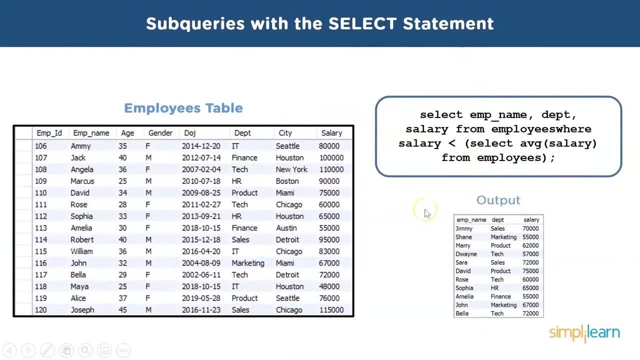 operator and inside that you have this sub query. so here is an example that we will perform on our mysql workbench. so in this example, we want to select all the employees who have a salary less than average salary for all the employees. this is the output. so let's do this on my mysql. 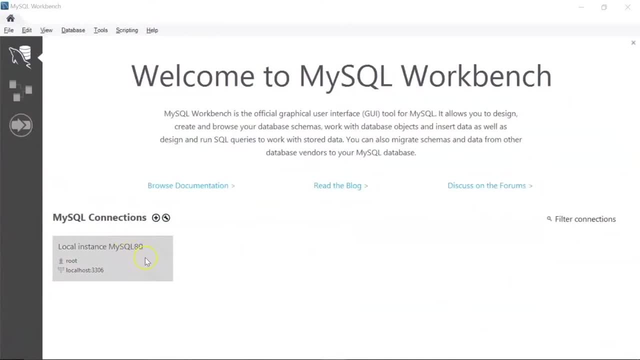 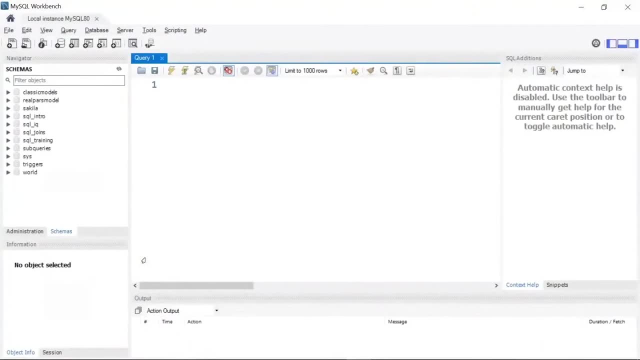 workbench. all right, so let me log into my local instance. i'll give my password. okay, so you can see i'm on my mysql workbench. so let's start by writing our sub query using the select statement. okay, so for this demo session we'll be using a database that is, sub queries. you. 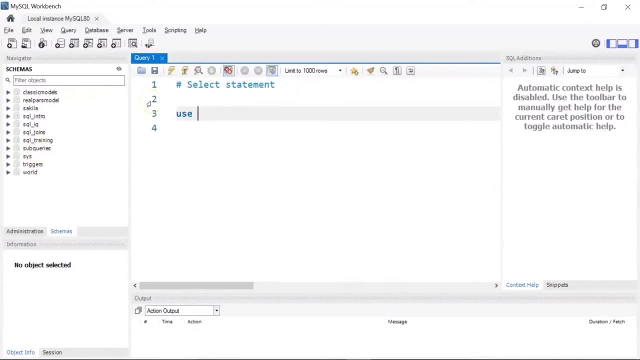 can see it here. i have a database called sub queries, so i'll use this sub queries database and we'll create a few tables as well. okay, if i run it now we are inside the sub queries database, so let me just show you the tables that are present inside this database. i'll write show tables if i run it. okay, there are two tables. 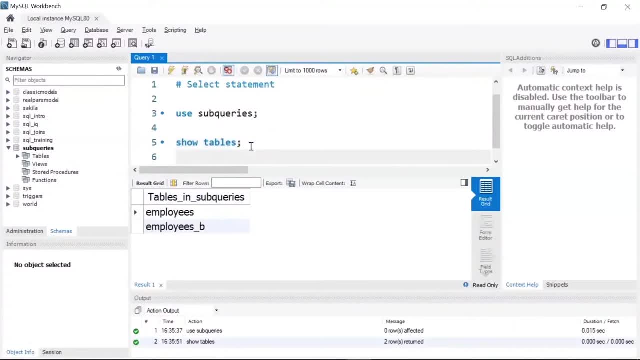 employees and employees underscore b. we'll use this table throughout our demo session. all right now for our select sub query. we want to fetch the employee name, the department and the salary whose salary is less than the average salary. so we will be using the employees table. so let me first show you. 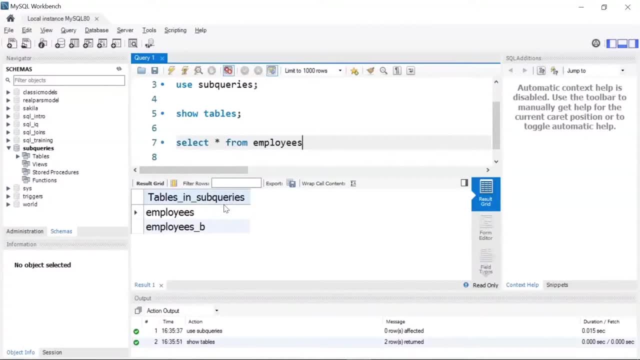 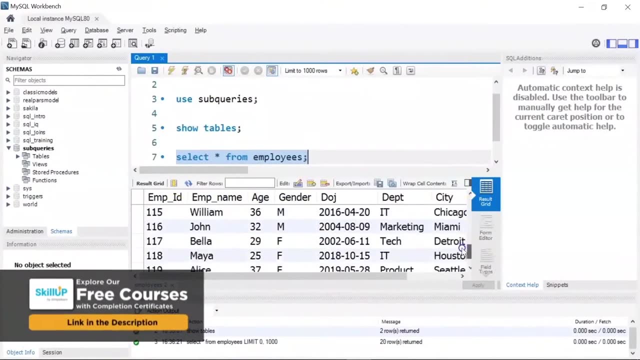 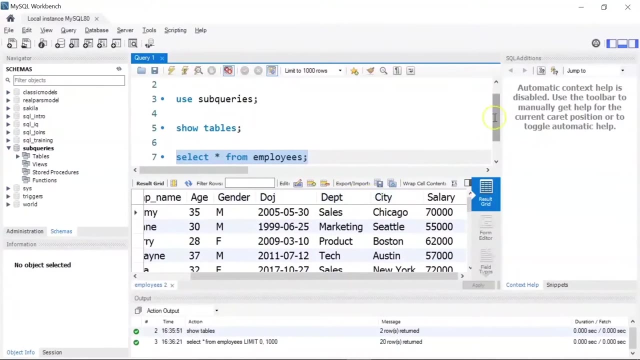 the records and the columns we have in the employees table. so i'll write select star from employees and run it. okay, you can see here we have 20 rows of information. we have the employee name, the employee id, age, gender, date of join, department, city and salary. so this is the same table that we saw in our slides. 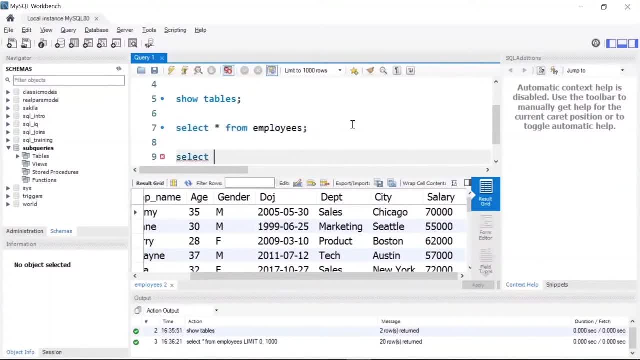 okay, now for our sub query. i'll write select. i want to choose the employee name, the department and the salary. there should be a comma here instead of a period. next i'll give my table name, that is, employees where my salary is less than, and after this i'll start my inner query or the sub query. i'll write select. 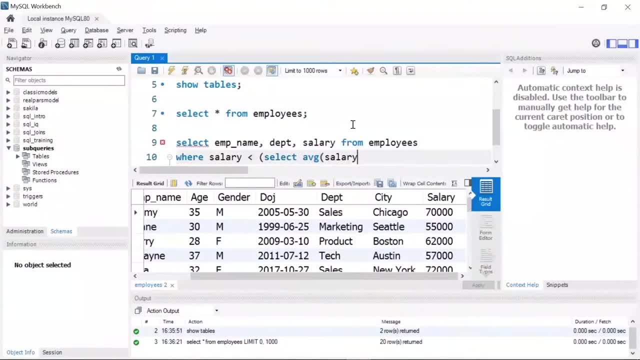 average salary. so i'm using the avg function to find the average salary of all the employees from my table, that is, employees. if i give a semicolon and run this, you'll see the output. so we have total 12 employees in the table whose salary is less than the average salary. 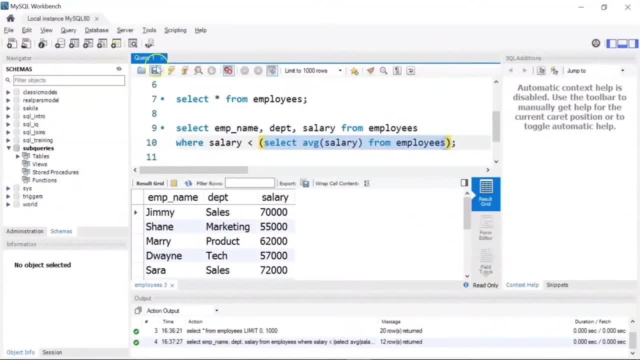 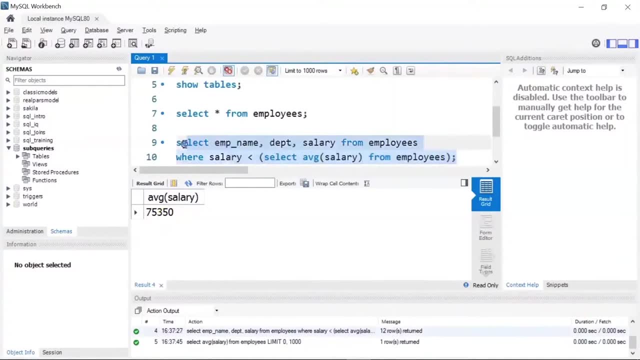 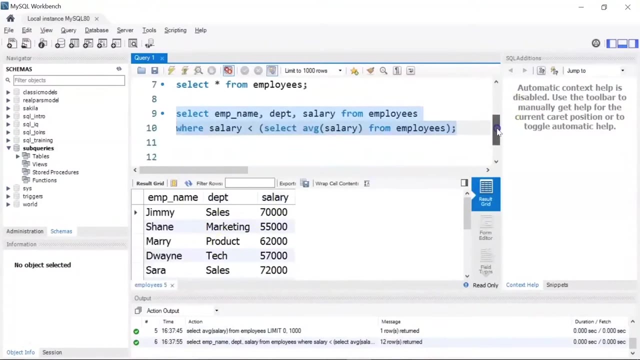 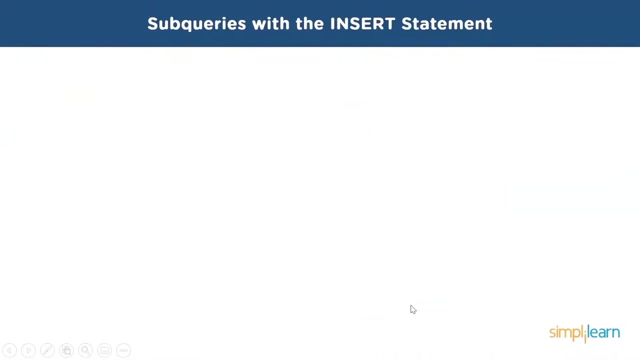 now, if you want, you can check the average salary. so the average salary is 75 350 dollars. now the employees who have a salary less than the average salary. so these are the people all. right now, moving back to our slides. okay, let's see if you can use this, depending on which keyboard your laptop takes. 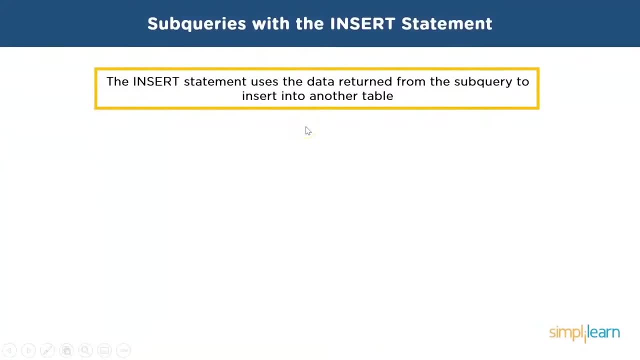 now let's see how you can use sub queries with the insert statement. now the insert statement uses the data written from the subquery to insert into another table. so this is how the syntax looks like. so you write insert into table name, followed by select individual column. so start from the table, use the where clause and then you give the operator. 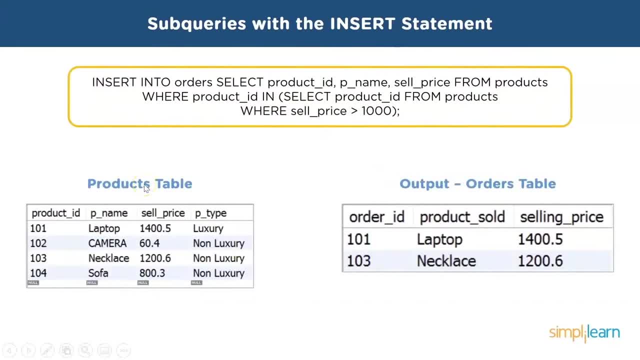 followed by the inner query or the subquery. so here we will explore a table called products table. are going to fetch few records from the products table, based on a condition, that is, the selling price of the product should be greater than hundred dollars. so only those records will fetch. 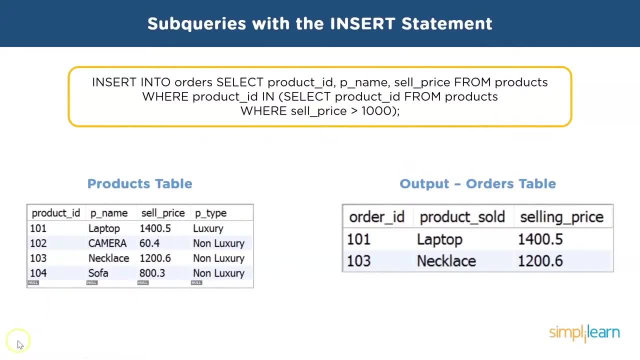 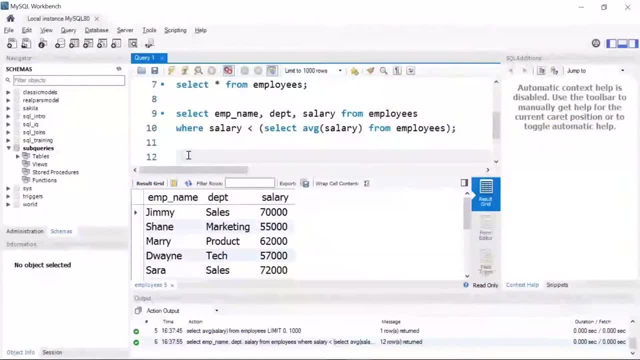 and put it in our orders table. all right, so we are going to write this query on my mysql workbench, so let's do it. i'll give my comment as update subquery, all right. so first of all let's create our table. that is products. so i'll write create table- products. then we'll give our column names. 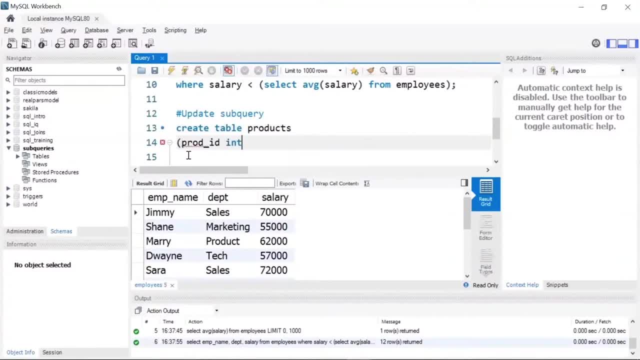 the first column would be the product id of type integer. then we have the column as item or the product which is of type varchar 30. next we have the selling price of the product. the selling price will be of type float and finally we have another column which is called the product type. 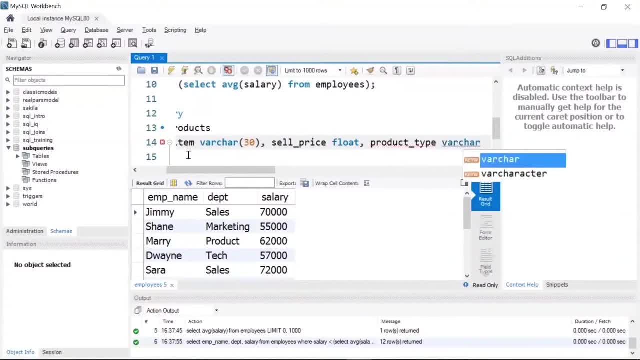 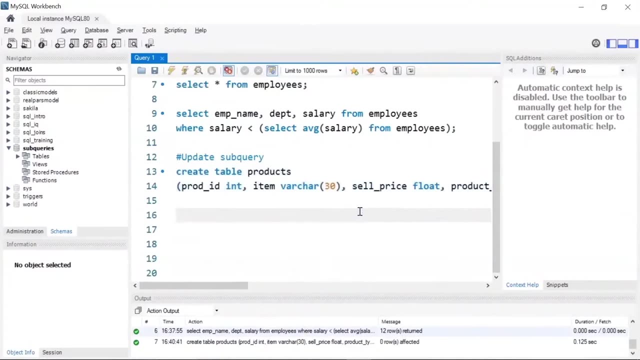 and again, product type is of the data type varchar. i'll give the size as 30, close the bracket and give a semicolon. now let's just um run it. it's like: uh okay, so we have successfully created our products table all the year, that positive. now let's insert a few records to our products table. so i'll write. 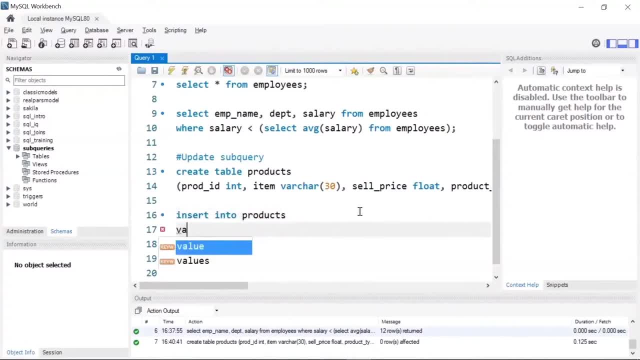 click here to watch similar. if you'd like to watch similar videos to nerd up and get certified, click here. i'll give four records. the first product id is 101, the product is, let's say, julia. then the selling price is, let's say, 800, and the product type is: it's a luxury product. 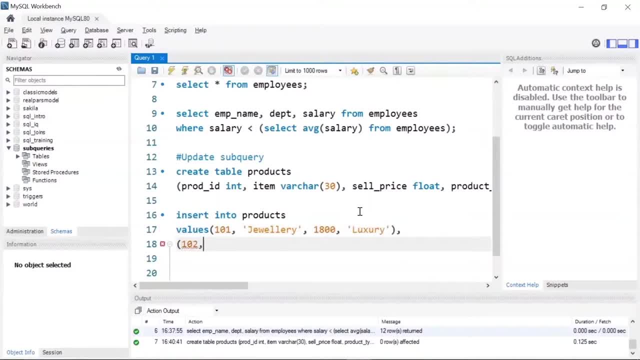 next, let's insert one more product detail. the product id is 102, the product is, let's say, t-shirt, the price is, let's say, hundred dollars and the product type is non-luxury. next i'll just copy this: to reduce our task, we'll edit this. the third products id is 103. 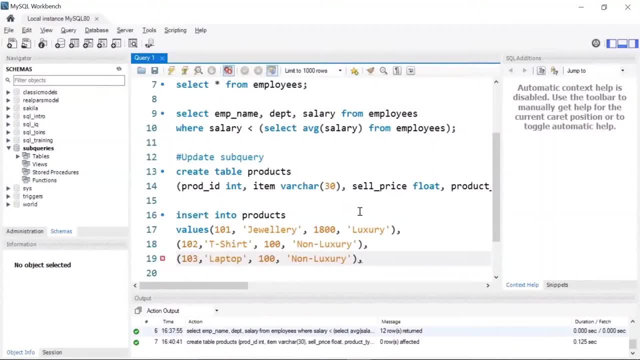 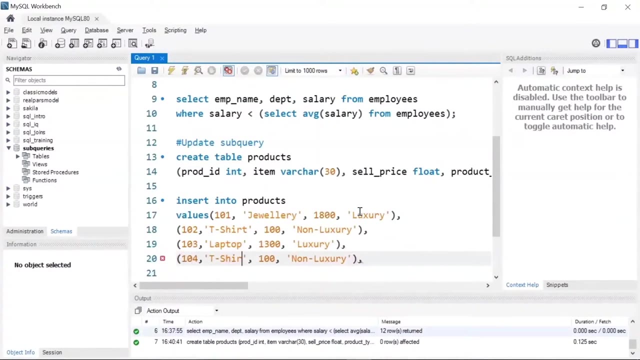 the product is laptop and, let's say, the price is 1300 dollars and it's a luxury product. i'll paste, paste again. and finally, I'll enter my fourth product, which is, let's say, table, and the price is $400 and it's a non-luxury product. I'll give a 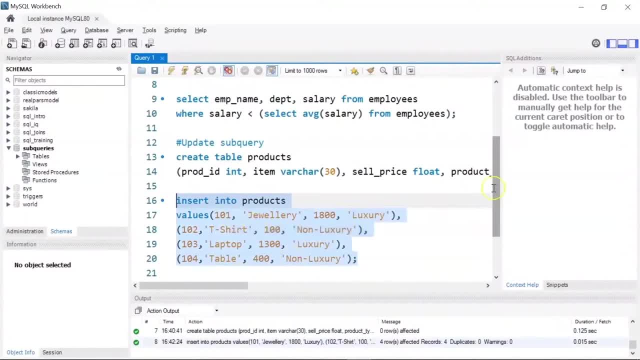 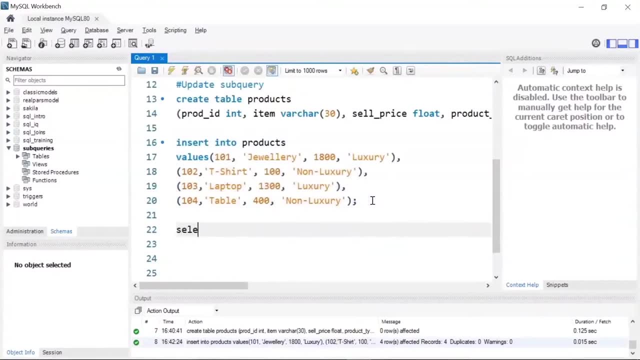 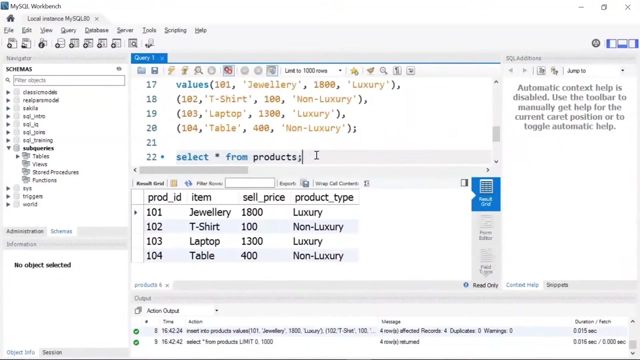 semicolon and we'll insert these four records to our products table. you can see we have inserted four records. let's just print it now so I'll write select star from products. if I run it, you can see we have our four products ready. now there's a real need. 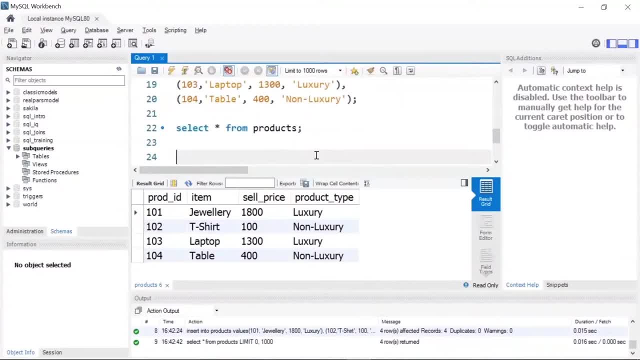 for innovation in cell therapy manufacturing. we see a tremendous benefit to bring parties together to collaborate. in this case, we bring together the academic excellence that exists in UCSF and Thermo Fisher's teas and cell and gene therapies. Compared to other therapy, cell therapy are curative. 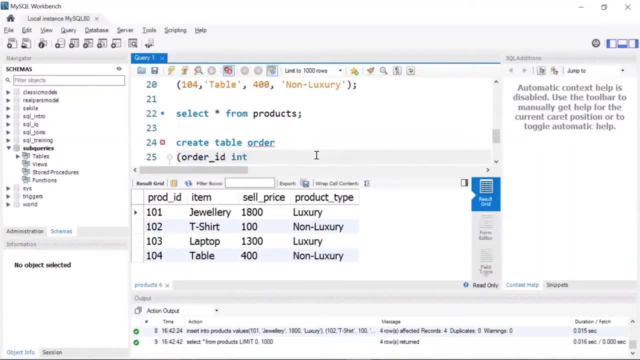 instead of the other therapy, like small molecules or antibody, they treat the symptom. I believe it's the next big revolution in medicine where we're going to move from drugs in vials to engineered cells that pinpoint disease and reduction in the number of side effects that people with devastating 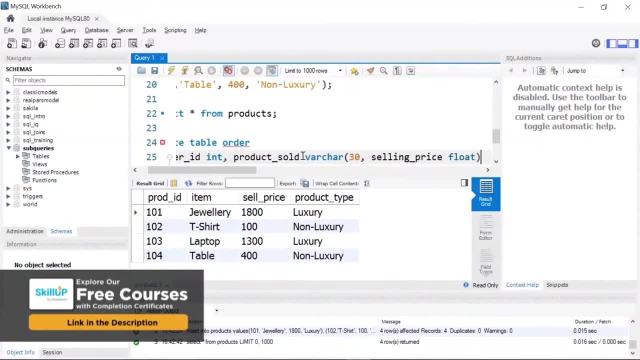 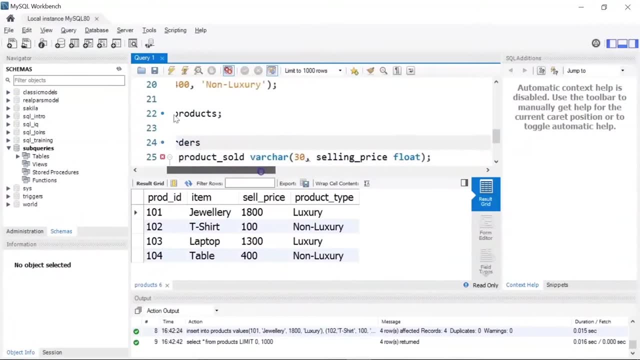 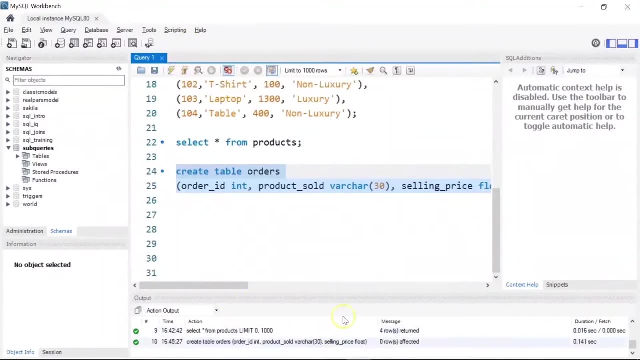 diseases have. Cell therapy is mostly used, what we call for liquid tumor, but the next frontier is really getting into solid tumors. Scientists at UCSF have developed very exciting therapies that may be effective against solid tumors, and so we're excited about potential of these new therapies. This is not a 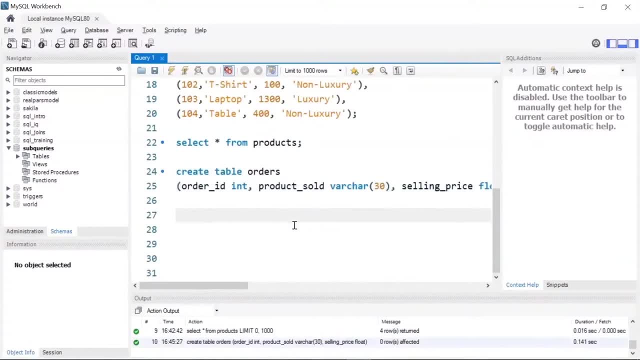 problem that can be addressed by one person or one company. it's something that needs to be done together. Here at UCSF, we're one of the leading health research universities in the country. while we are extraordinarily skilled at discovering new technologies, New targets for therapeutic intervention and indeed, actually discovering drugs. 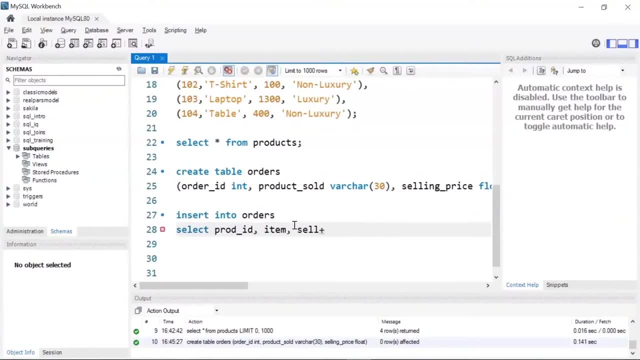 We are ill-prepared to actually develop those, let alone commercialize them. We knew we needed a partner. Thermo Fisher can work with our partners to help translate all of this exciting work done in the collaboration center into commercially available therapies. The ability of those cell engineers to talk directly with Thermo. 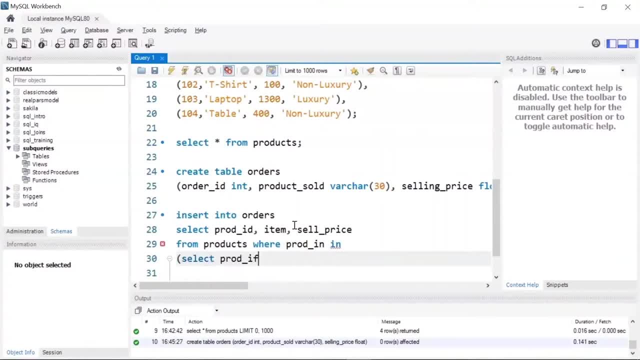 Fisher, technicians and scientists who have the skills of taking those discoveries and manufacturing cells for human use. that close proximity can't be overstated. I think it's going to be a unique collaboration, unlike virtually anything that I'm aware of that will push this field further and faster. 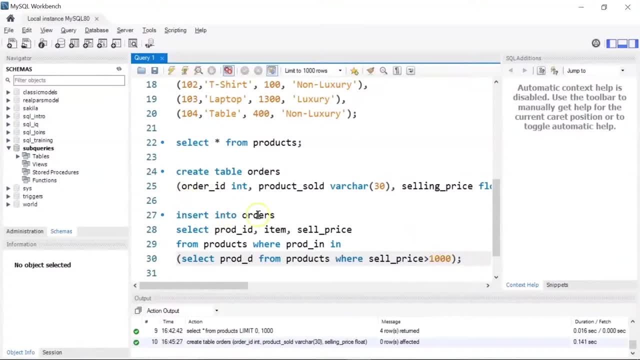 So today a lot of the cell therapy products are coming from patients. We get the blood drawn, they're sent to a manufacturing facility, we produce the drug, we engineer the T-cells and we put them back in injects. So you can imagine the logistic context. 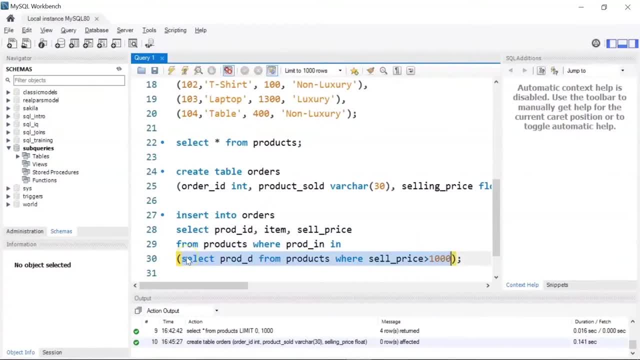 So the ability to work closely with the people who are involved in the process. So the ability to work closely with the people who are involved in the process, So the ability to work closely with the, So the ability to work closely with the three earners are- we are fully. 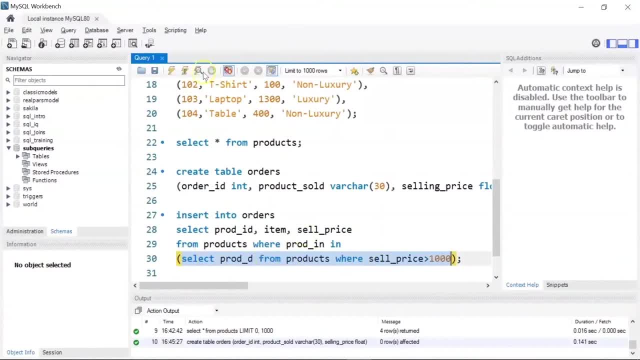 working closely with Thermo Fisher, to take our inventions, optimize how they're manufactured and then dose them into patients literally across the street at our Precision Cancer Hospital. That is truly unique. This will be a resource for patients literally around the world because 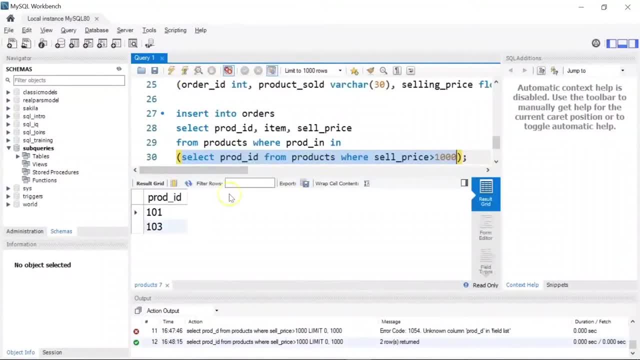 we'll be doing first-in-kind human trials, which seem extremelyOh we get the decrease in coverage to commercial. it takes many, many years. Thermo Fisher is focused on addressing this challenge by working with our partners to more standardized approaches, with the ultimate goal of shortening therapeutic development. 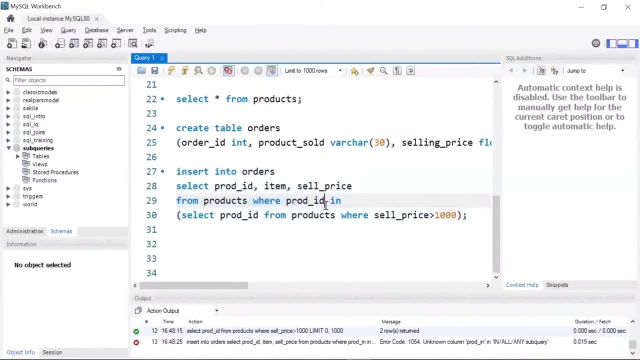 timelines, driving down costs for customers and helping to avoid failures on the path toward commercialization. there's no better partner for us in this space than thermoficial scientific. i'm just incredibly excited to begin work on what i think is the next big revolution in medicine. 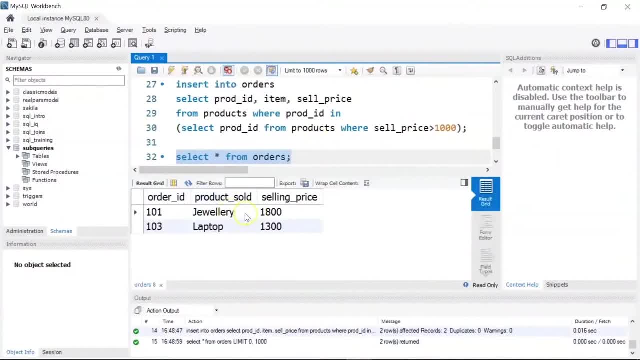 if i run it, there you go. so there were two products from our product table that were jewelry and laptop, which have a selling price greater than one thousand dollars. so the selling price for jewelry was eighteen hundred dollars and for laptop it was thirteen hundred dollars. so this is how you can use a sub query, using the insert statement. all right, now going back to our 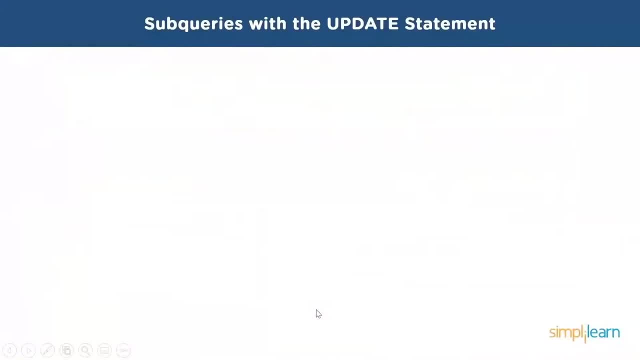 slides again. all right, now let's see how you can use sub queries with the update statement. now the sub queries can be used in conjunction with the update statement, so either single or multiple sub queries can be used in conjunction with the update statement, so either single or 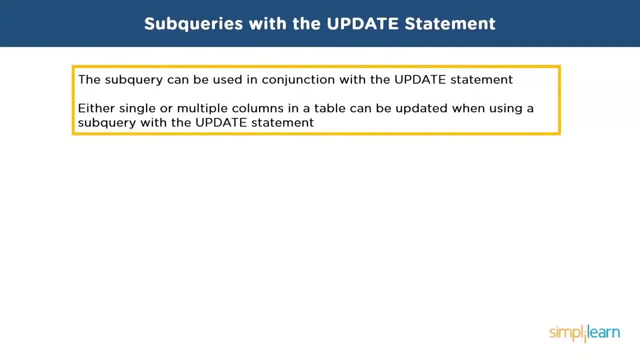 multiple columns in a table can be updated when using a sub query with the update statement. so this is how the basic syntax of an update sub query looks like. so you write update table, followed by the table name. you set the column name. you give the where operator. 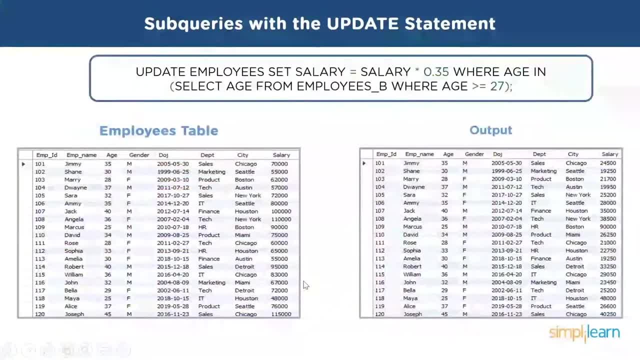 and then you write your inner sub query. so we are going to see an example where we will use this employees table and using this employees table, we will update the records of the salaries of the employees by multiplying it with a factor of 0.35, only for those employees which have age greater than 27. so we are going to use a new table called 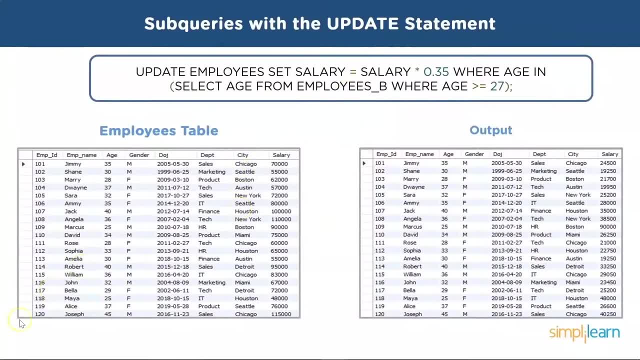 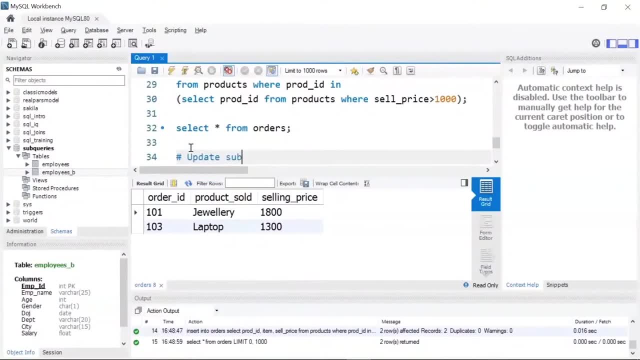 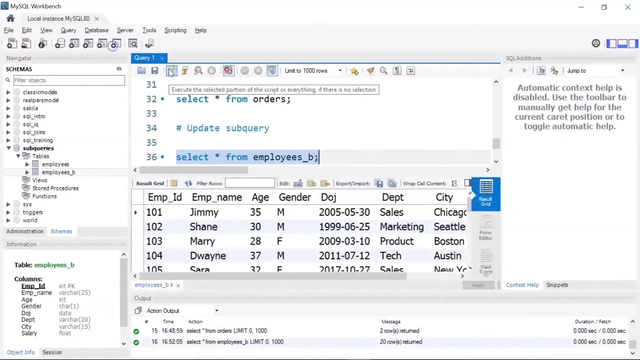 employees underscore b for this as well. so let's see how to do it. so i'll give my comment as update sub query. before we see the sub query, let's see what we have in the table: employees underscore b. this is basically a replica of the employees table. there you go. it has the same records that our. 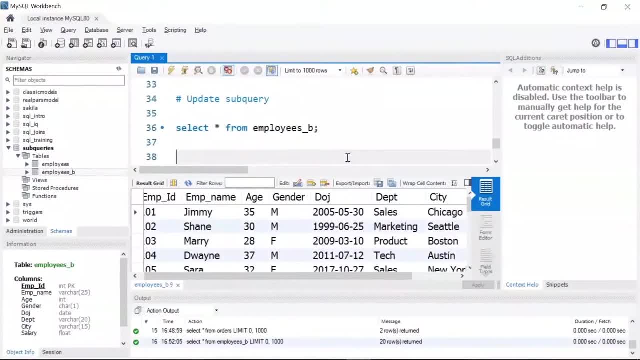 employees table has. we are going to use both the employees table and the employees underscore b table to update our records. so i'll write: update employees. set salary equal to- let me this. to the next line I'll write: set salary equal to salary multiplied by 0.35. 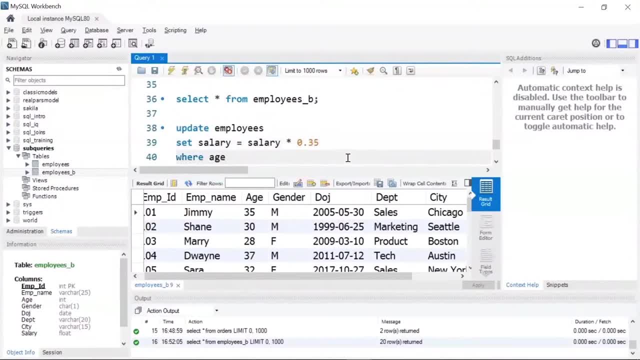 where age in. then I'll write select age from my other table, that is, employees, underscore B, where age is greater than equal to, let's say, 27. all right, so let me run through this query and tell you what we are going to do. so I'm going to 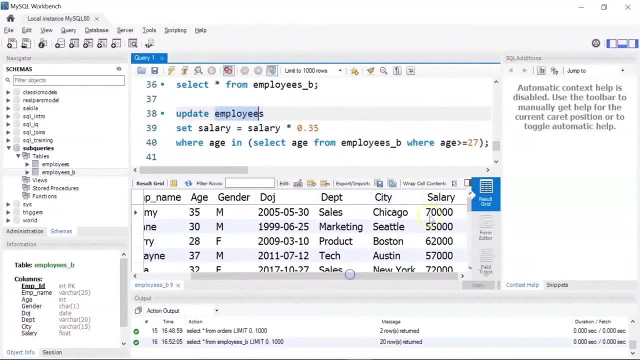 update the records of the employees table specifically for the salary column. so I'm checking. if the age is greater than 27, then we'll multiply the salaries of the employees with a factor of 0.35 in the employees table. let me just run this, then we'll see our output. okay, so 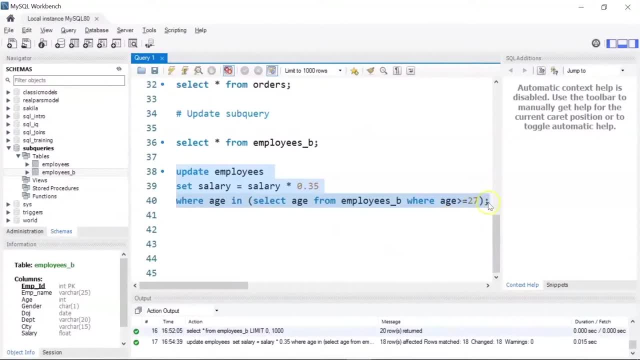 it says 18 rows affected, which means there are total 18 employees in the table out of the 20 employees whose age is greater than 27. now, if you see, I'll write select star from employees. you can see the difference in the salaries, if I 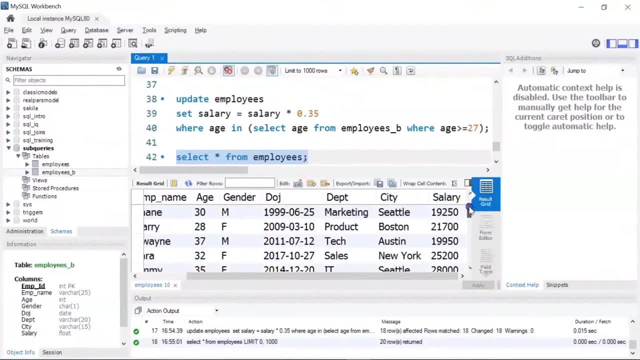 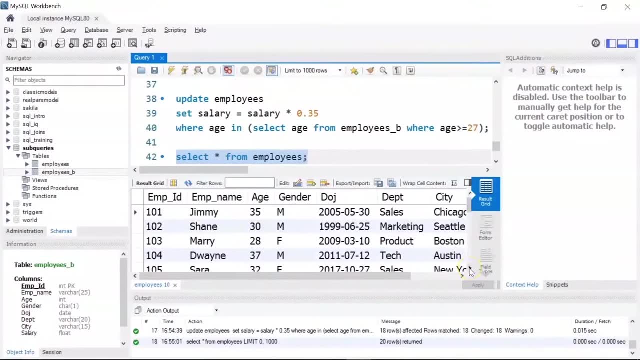 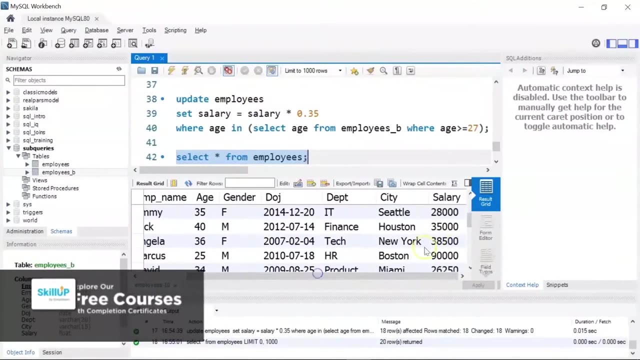 scroll to the right, you can see. these are the updated salaries. okay, now if you check for employees who have an age less than or equal to 27- for example, Marcus, whose age is 25- his salary is the same. we haven't updated his salary. then, if you see, if we 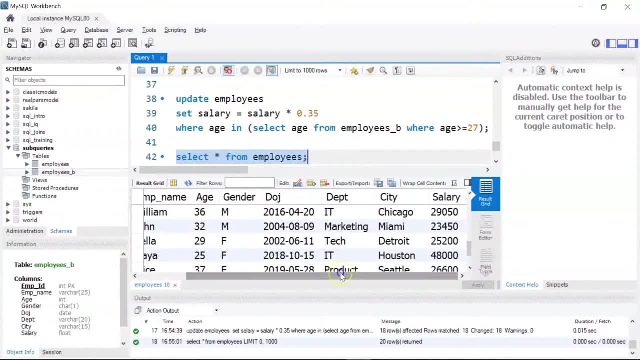 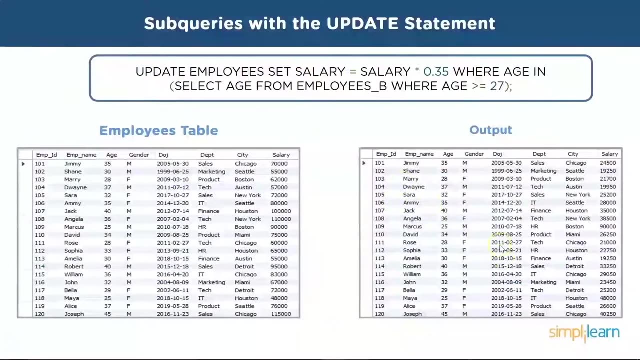 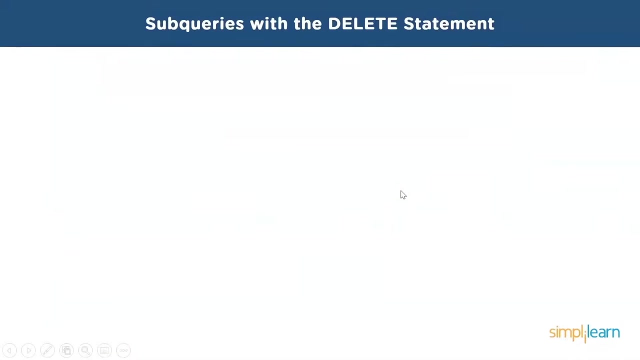 have. okay, there is one more employee, Maya. we haven't updated the salary of Maya because the age is less than 27.. 27, all right. now let's go back to our slides again. as you can see, we got the same output on our my sequel workbench. now let's explore how you can write. 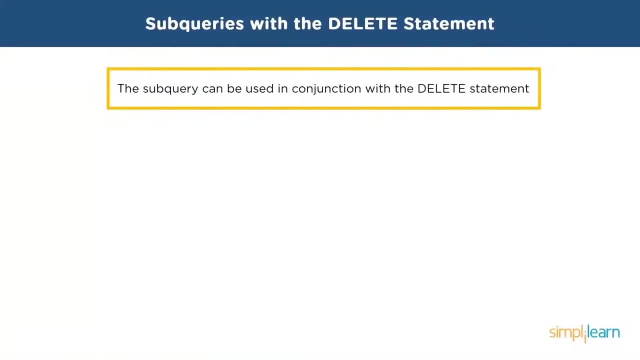 sub queries for the delete statement. now sub queries can again be used in conjunction with the delete statement. so this is how the basic syntax of a delete query using sub query would look like you write: delete from the table name of sub query, from where clause the operator value, followed by the inner query and. 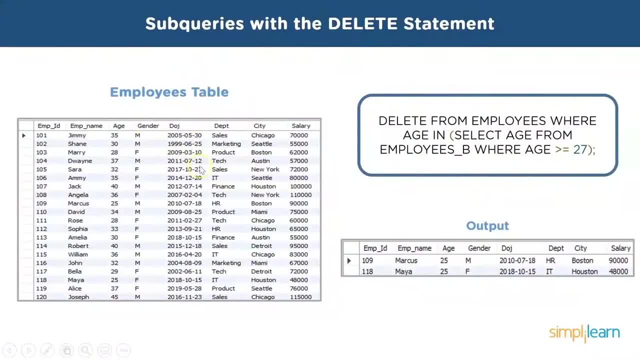 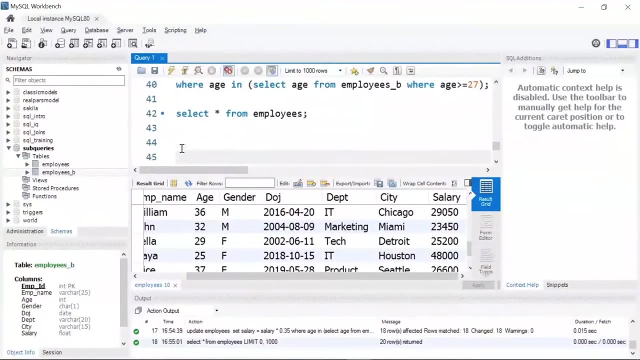 within brackets. so here we are going to use the employees table and what we are going to do is we'll delete the employees whose ages greater than equal to 27. so let's see how you can do it. all right, so I'll give my comment as: delete sub query. 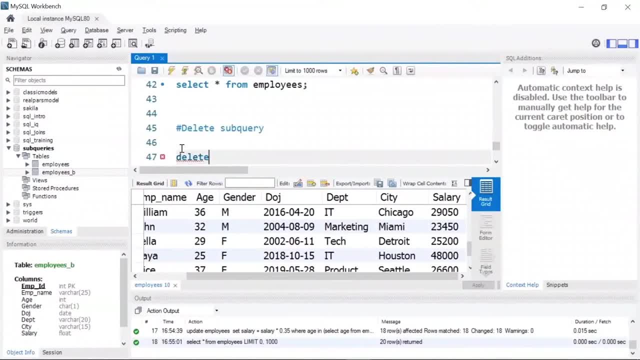 so we'll follow the syntax that we saw. I'll write delete from my table name. that is employees. I'll write where age in and then I'll start my inner query or the sub query. I'll write select age from employees, underscore B where ages, let's say. 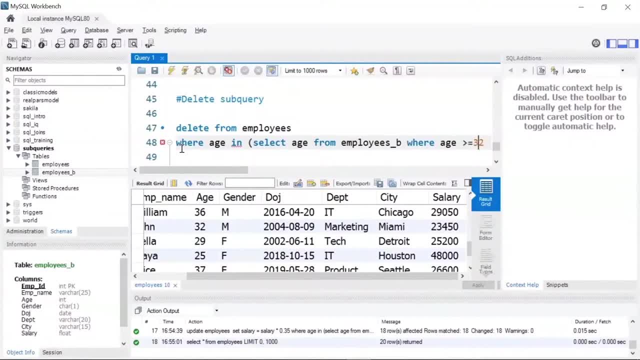 greater than equal to 32, or let's say the age is less than equal to 32. close the bracket and I'll give my semicolon. let me first run the inner query for you, so that you get an idea of the employees who are less than 32 years of age. so 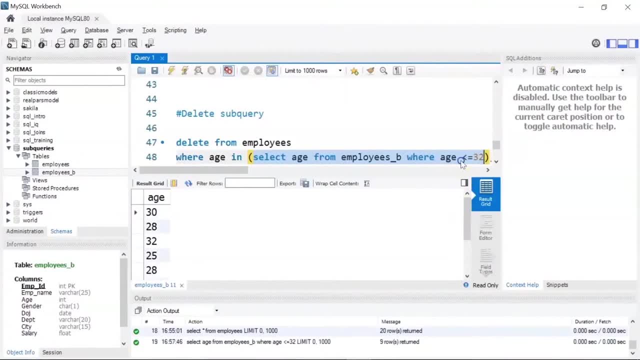 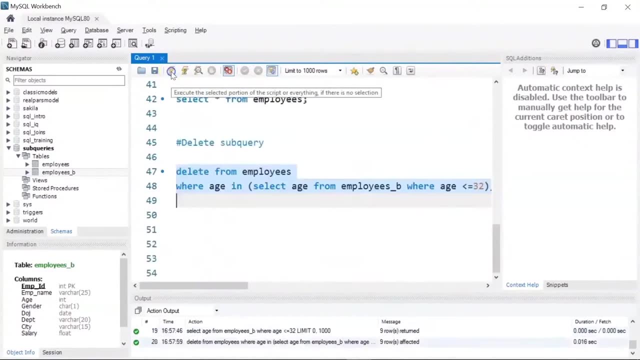 there are nine employees in the table who have an age less than equal to 32, so we are going to delete the records. if I run this, okay, it says nine records deleted. now let's print or display what we have in the employees table. if I run this, there you go. so if you see the age table, we 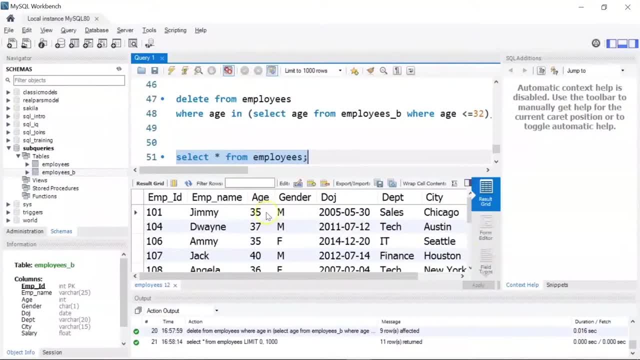 have total 11 employees now and all their ages are greater than 32, because we have deleted all those employees who had an age less than equal to 32. okay, so let me show you from the beginning what we did. so first we used our sub queries database, then we used our employees table. 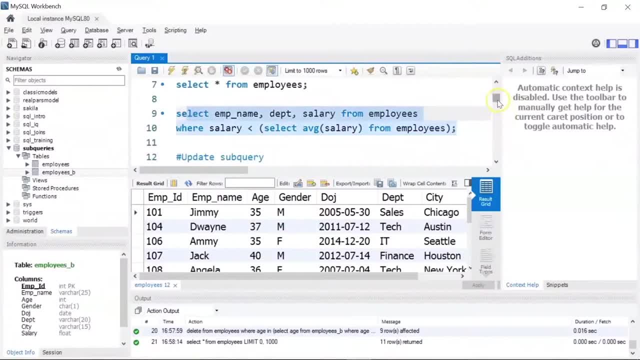 so we started by looking at how you can use the sub query with a select statement. this should be insert instead of update. so we learnt how to write an insert sub query. we used two tables: products and our orders table. moving ahead, we saw how to write sub queries using the update command, so we 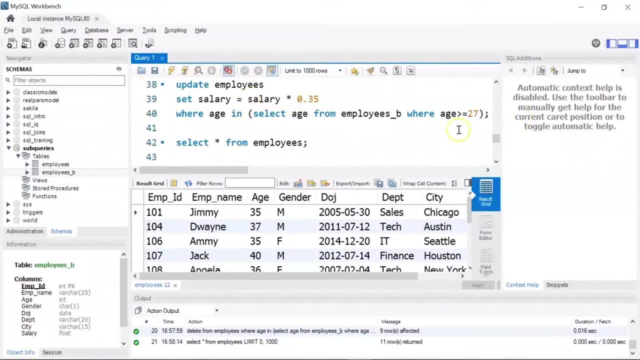 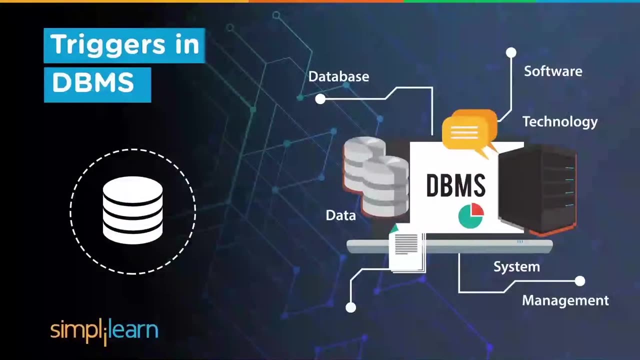 updated the salaries of the employee by a factor of 0.35 for those who had an age greater than equal to 27 and finally, we saw how to use the sub query using the delete statement. so we deleted all those records for the employees whose age was less than equal to 32 in this video. 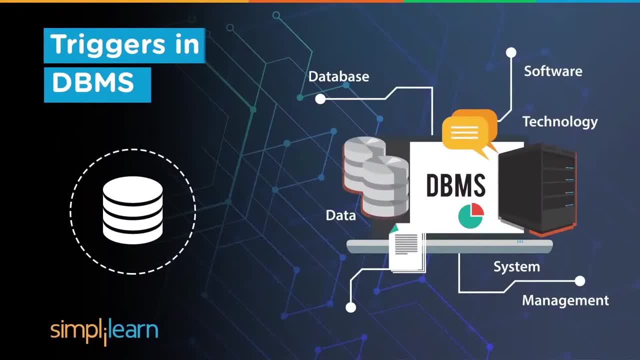 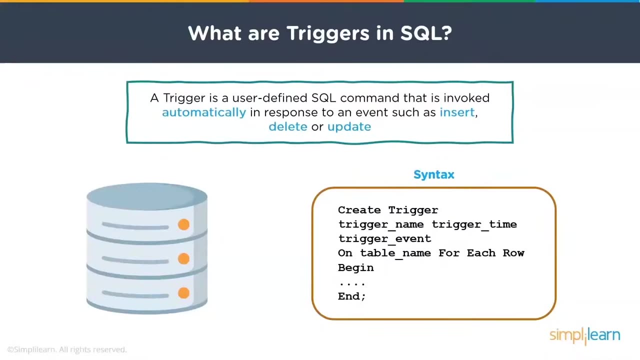 we will discuss an advanced SQL concept called triggers. we will learn what triggers are and how they can be used to solve problems. will look at how trigger queries are written on my sequel bug bench. so let's get started first. what are triggers in SQL? so a trigger is a user-defined SQL command that is invoked. 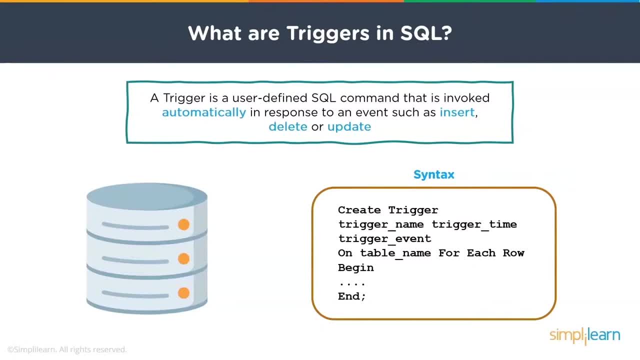 automatically when an event occurs. an event can be related to inserting, updating or deleting records in a table. in mySQL, triggers be executed automatically by the oracle server. below is how the syntax of writing a trigger is. so you write create trigger, followed by the trigger name. now the trigger name should be a. 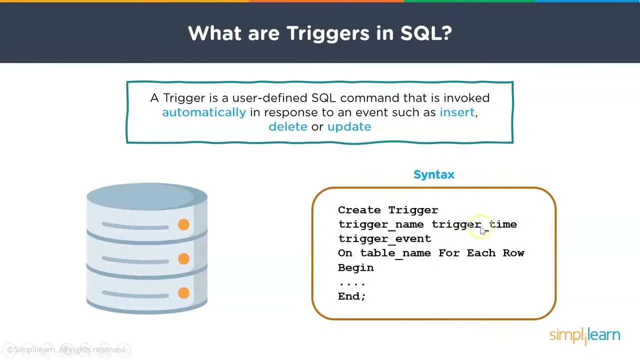 valid sql name. then we have the trigger time, the trigger event and then on the name of the table. then we write for each row: begin, followed by the list of sql statements and finally we write end. now in the syntax the trigger time represents either before or after an event and a trigger. 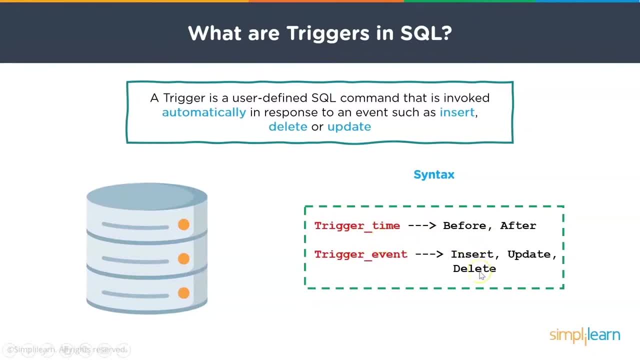 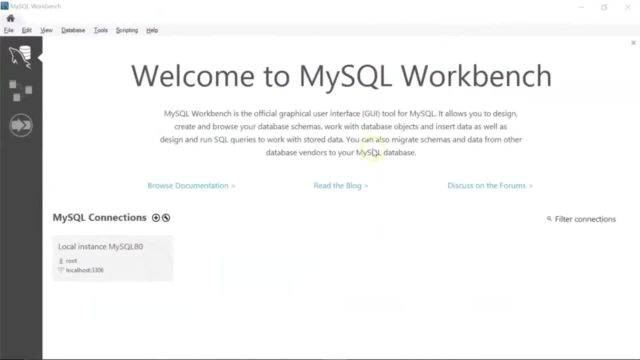 event can be an insert, update or delete operation. now let me take you to mysql workbench, where we will learn how to create triggers and explore more on how it works. so i am on mysql workbench, so first let me go ahead and create my connection. i'll give my password. 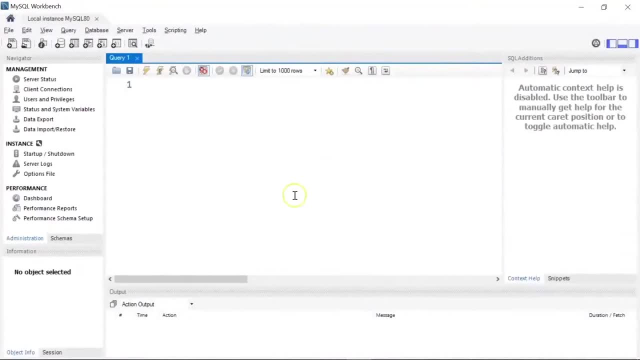 all, right now. this will take you to my sql editor. okay, so first and foremost, let me create a new database called triggers. so i'll write my sql command as: create database triggers. let me run this, okay, so you can see here one row affected. i have created my database, that is triggers. next, 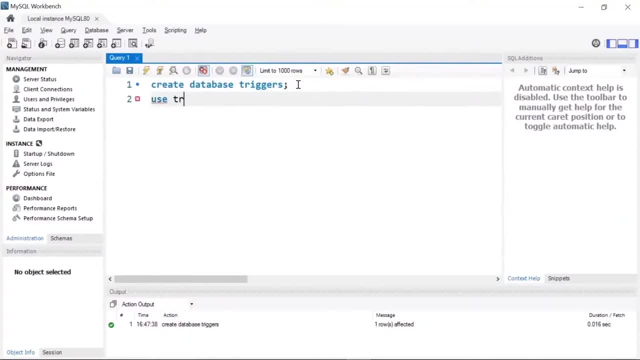 i'm going to move inside this database, so i'll write the command use triggers. let's run this. okay, now, inside this triggers database, we'll be creating our different tables. so let's check if we have any tables, i'll use the command show tables. now you see there are no tables in this database. all right, first let's see how, before insert. 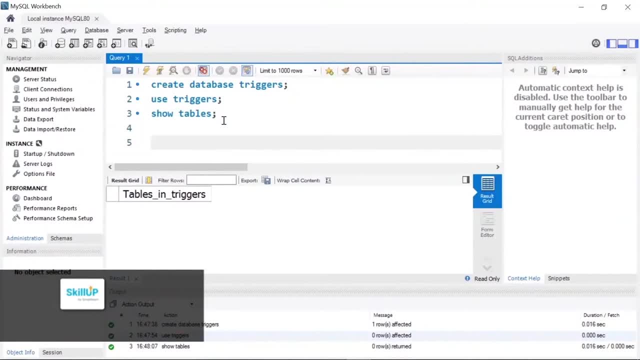 trigger works. so for before insert trigger, we'll create a table called customers and verify the age of each customer. so i'll give a comment before insert trigger. so let me go ahead and create my customers table. i'll write create table- customers and i'll give my 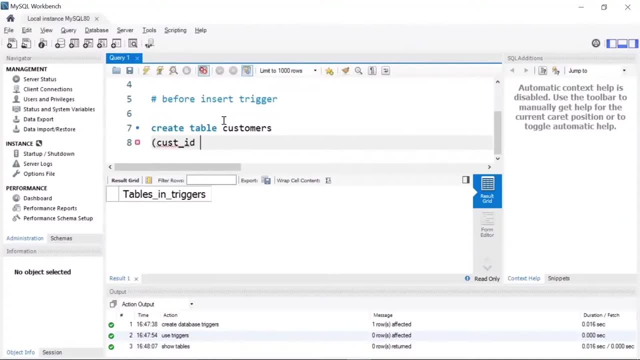 column names as cust underscore id, which is customer id. this is going to be an integer. then we have the age of the customer. this is again an integer, and we'll have the name of the customer. the name of the customer will be a varkar type. i'll give the size as 30, all right. 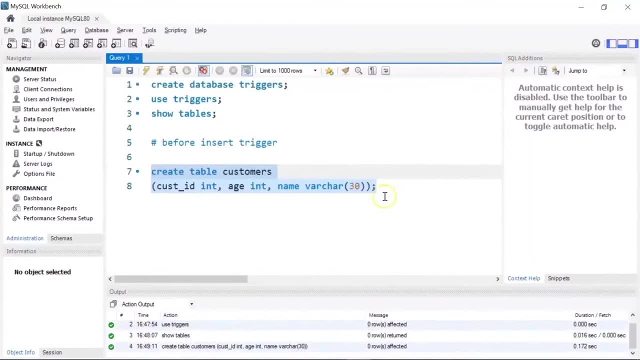 let's create this table. okay, so we have successfully created our customers table. now, moving ahead, i'm going to write my before insert trigger command. so we'll start with a delimiter. so a delimiter is a marker for the end of each command. next i'll write my create trigger. 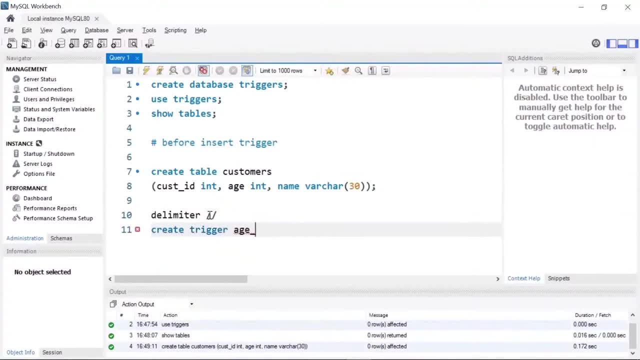 followed by the trigger name. i'll give a valid trigger name, such as each underscore: verify. i'll write before trigger. it should be before insert on my table name. would be customers. then i'll write for each row. if new dot age is less than zero, then set new dot age equal to zero, which means while inserting your values to the age column. 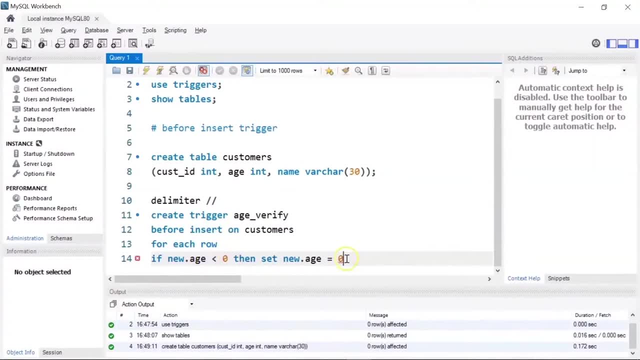 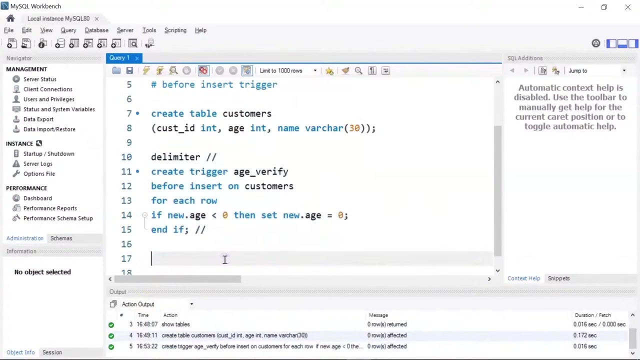 in case the age value is negative, will convert the age to zero. i'll give a semicolon and then i'll write end if i'll give another semicolon and i'll close the delimiter. now let me run this. okay, so we have created our trigger. now let's insert a few values onto customers. 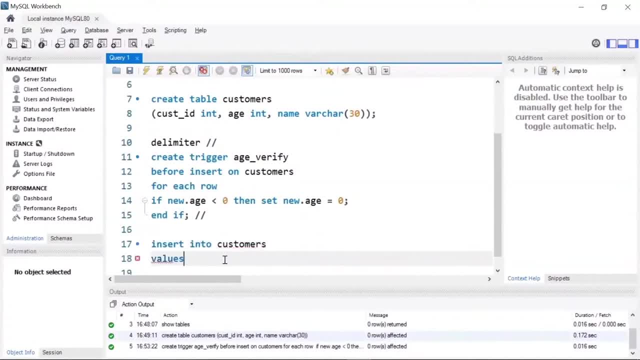 so i'll write: insert into customers values 101, which is the customer id. i'll give the age as 27 and let's say the name of the customer is james, and let's insert another record, give the value as 102, and this time i'm purposely giving the age as. 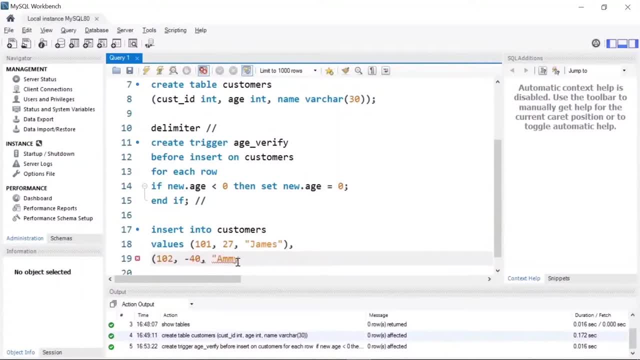 minus 40, which is less than 0, so that you can see the output clearly. i have given the customer name as amy. let's insert two more records. the customer id with 103 has an ease of 32 and let's say the name is ben. 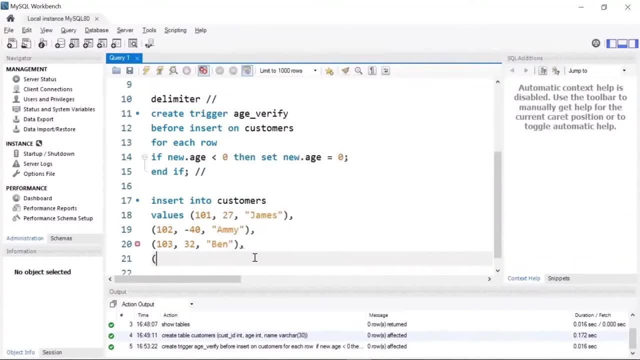 so we have given the customer name as ben, i'll give another comma and finally we'll insert our fourth customer record. the customer id is 104, the age i'm giving as minus 39, which is less than 0 again, and let's say the customer name is angela. 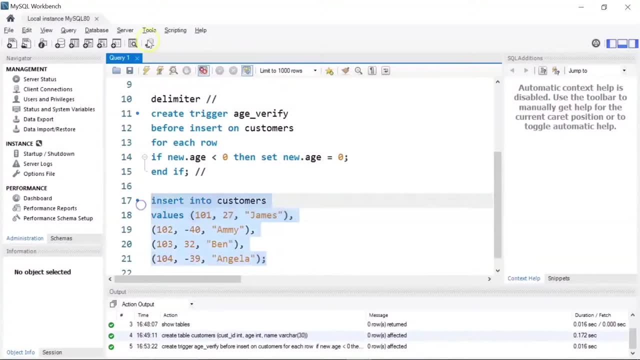 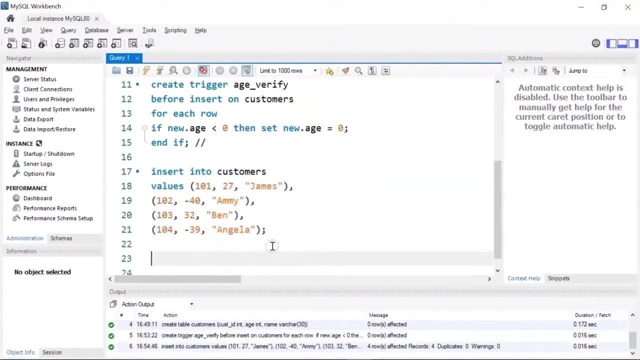 all, right now let me run this. okay, so we have successfully inserted four rows of information to our customers table. now let's see the difference, since we had created a age verify trigger which would change the values of the age column in case the age value is less than zero. so now that we have 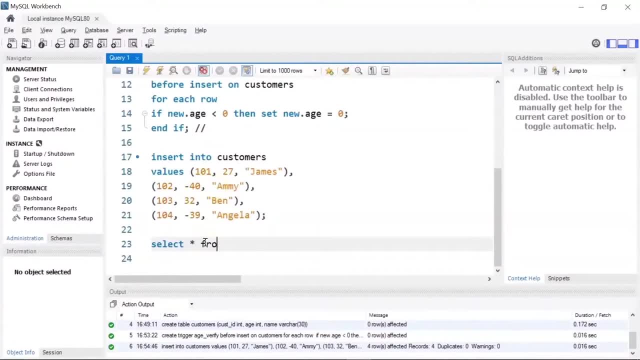 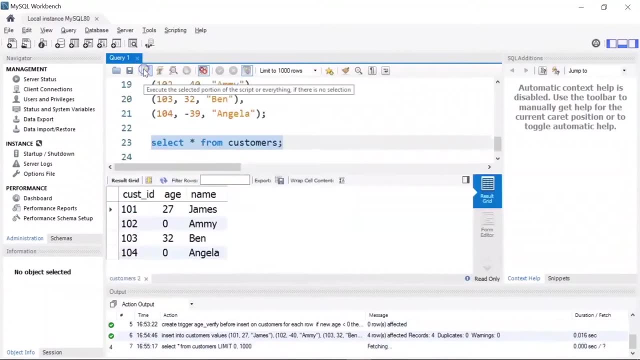 inserted four records to a customer. so let's see what we have in the customers table. now let me run it there you go. so if you see this for those customers where the age was less than zero, such as 102 and 103, you can see here our trigger has automatically converted those. 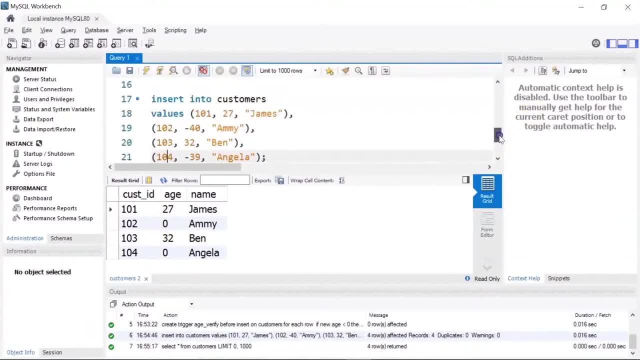 values to zero. if you can see the trigger we had created, we had set our new age to zero if the age was less than zero, and is the output we get. so here we looked at how a before insert trigger works. all right, now, moving ahead, let's understand how an after insert trigger works. so i'll give a comment here. 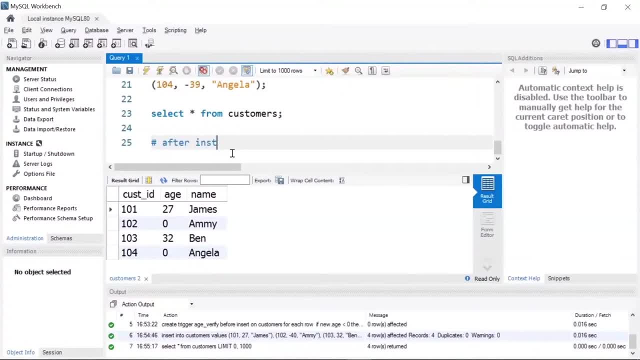 as after: insert trigger. now in this example we'll create two tables: customers and message. now the trigger will be fired. if the birthday column has a null value in the customers table, you will get a message to update your date of birth. okay, so first let me create my customers table. 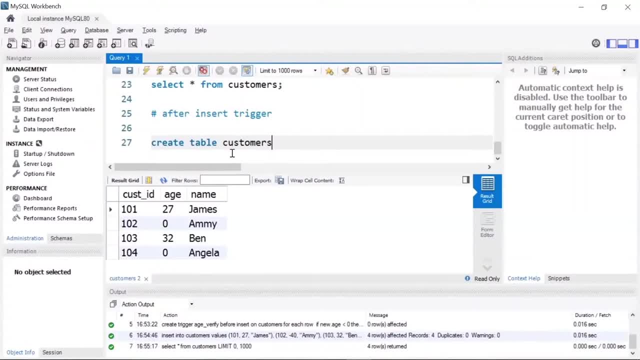 now, since we already have one customers table, i'll name it as customers one and let me give the column names. so the first column would be the id column. this is going to be an integer and i'll use the auto increment parameter and this will be my primary key as well. 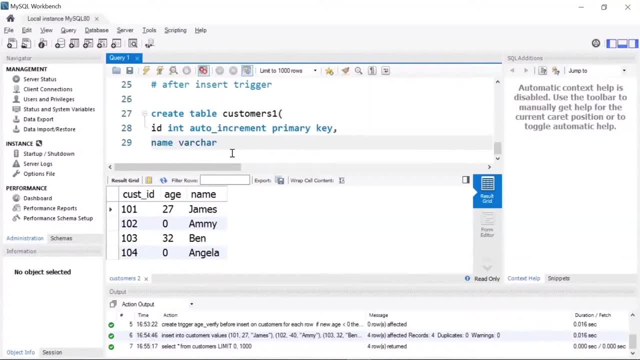 next we'll have the name of the customer. this is going to be of type worker and i'll use not null constraint. next we'll have the email id of the customer. this is again going to be of barcar type and the column we are interested in is the birthday column, so i'll write birth date. this is going to 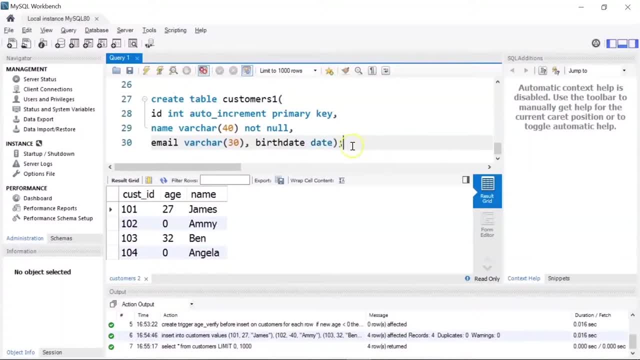 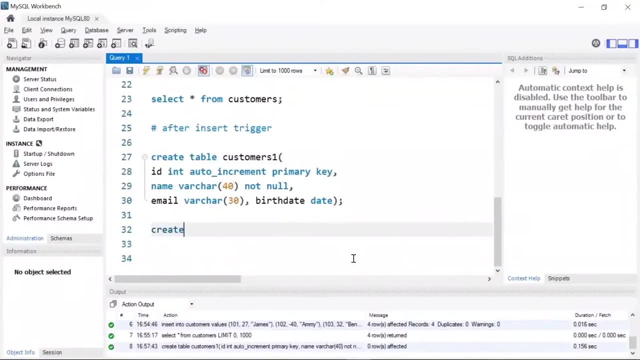 be of type date. okay, so let's create our table. all, right, now we'll create our second table, which is going to be message. let's create the columns. this will have id int and i'll use the auto increment operator. next we'll have the message id. this is going to be of integer type. we'll have a column called message. 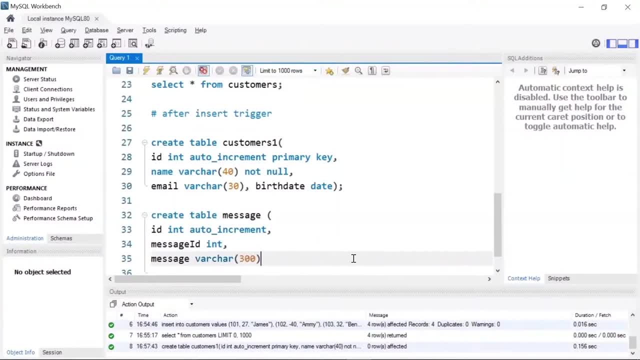 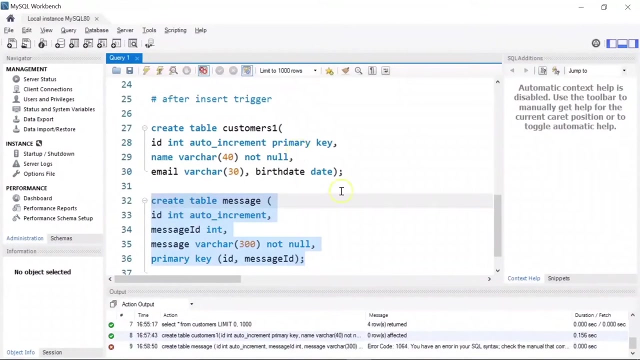 this will be a worker type, let's say 300 characters and not null, and i'm going to set my primary keys as id and message id. let's create our second table then. so we have some error here. let's debug the error. okay, so i forgot to close the bracket here. all right, now let me run this table. all right, so we. 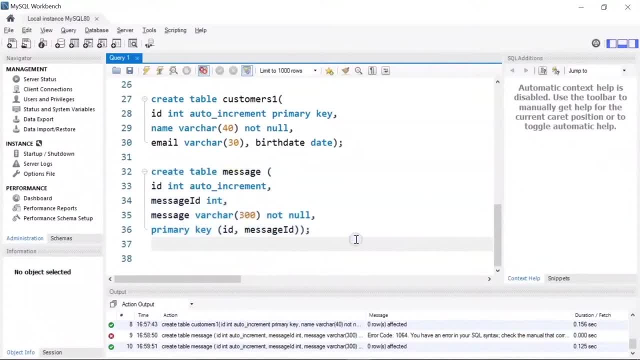 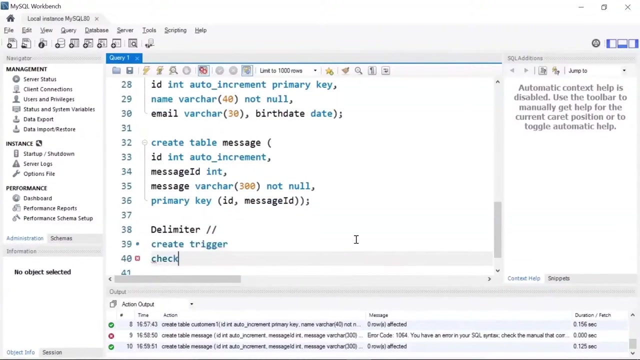 have created our message table as well. next i'll write my after insert trigger command, so i'll write delimiter. next i'll use create trigger command, so i'll write create trigger. my trigger name would be: check underscore: null underscore date of birth. after insert on customers one: 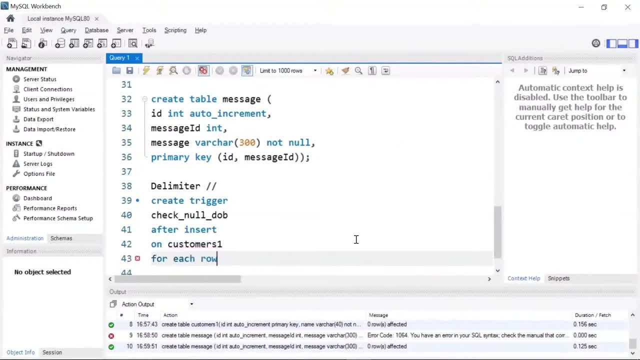 after insert on customers: one after insert on customers, one for each row: begin. if new dot birth date is null, then we are going to insert into our message table. we'll give the columns as message id and message values new dot id comma. i'm going to use the 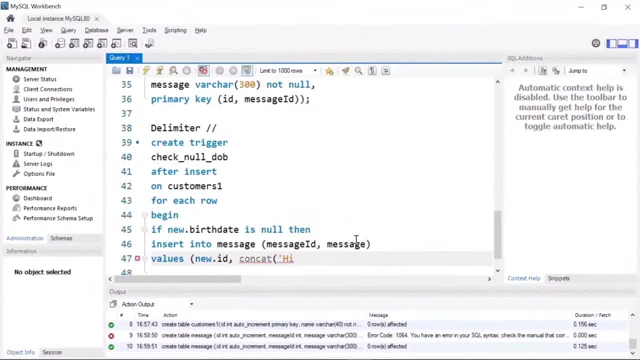 concat function where i'll give my message. let's say hi, followed by the name, followed by, let's say please, please, update your date of date of birth. okay, now i'll write ndf. okay, now i'll write ndf. okay, now i will. okay, now i will. 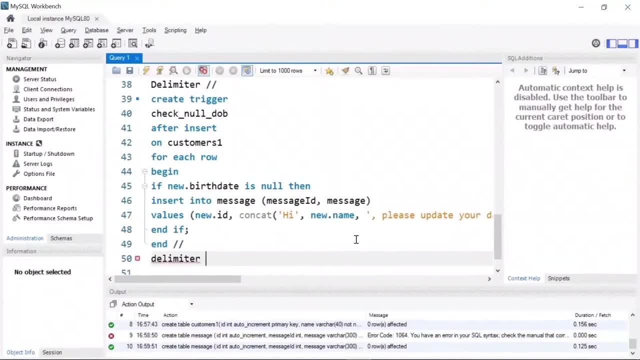 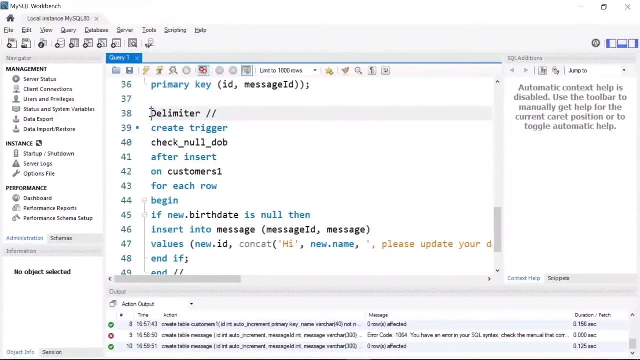 close the delimiter. close the delimiter. okay, i'll close the delimiter. okay, okay, okay, okay. so let me go to the top and recheck if you have created our trigger correctly. so i have my trigger name after insert on customers, one for each row. begin if our new birthday has a null. 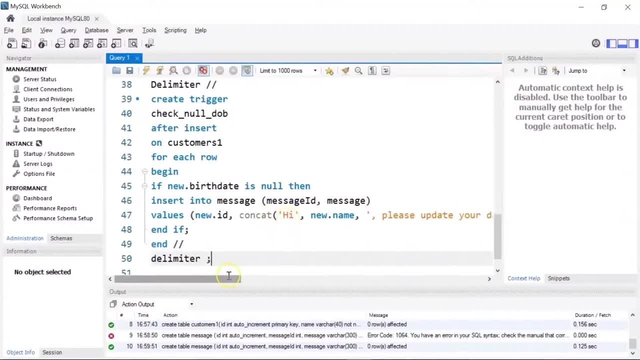 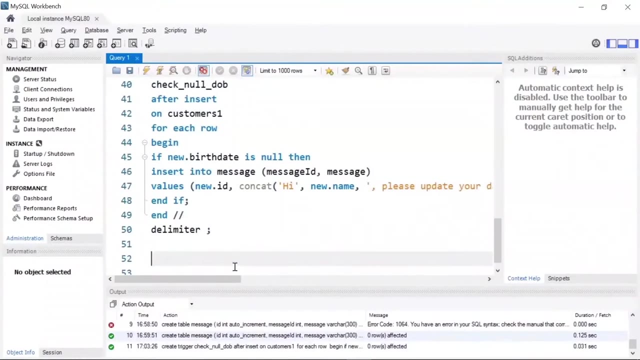 value. then we'll pass in a message saying hi, the name of the customer. then the message would be: please update your date of birth. all right, so let's run that trigger, okay, now the next step is to insert a few records to customer table. so my name of the table is customers one. 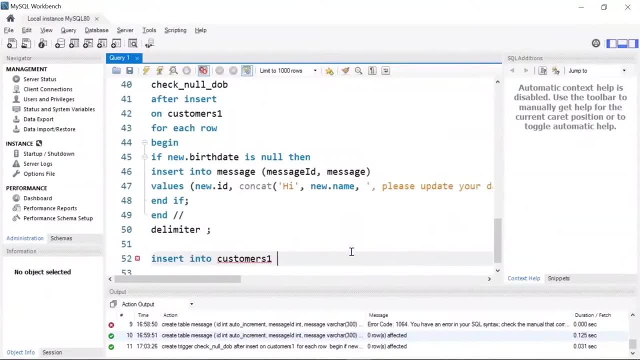 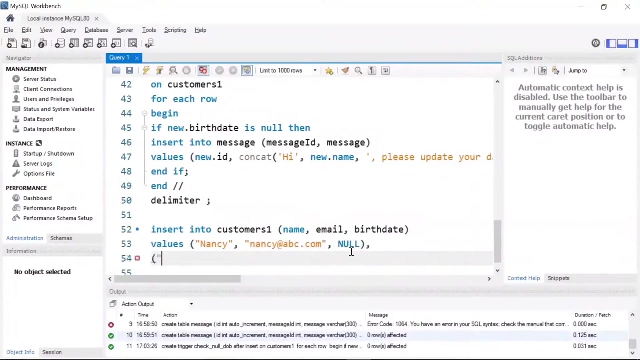 okay, i'll give the column names as name, email and birth. okay, we'll pass in a few values. so our first customer's name, let's say, is nancy, comma. i'll give my email id, let's say nancy, at the rate abccom. now, let's say i'm purposely passing the date of birth as null. i'll give a comma my next customer. 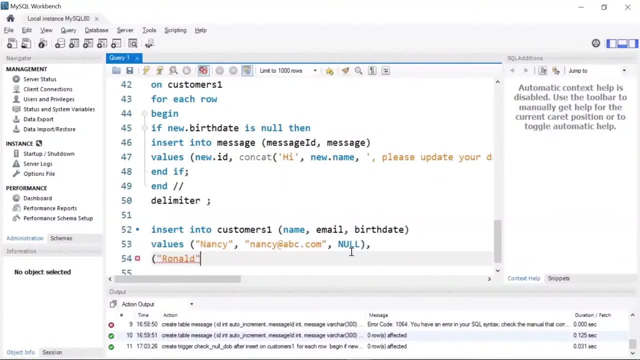 let's say the name of the customer is ronald, and then i'll give the email id, such as ronald, at the rate xyzcom, and this time i'm going to pass in the date of birth as null. and then i'll give the e-mail id nothing in control, and this time i'm going to pass in the date of birth, let's say 1998. 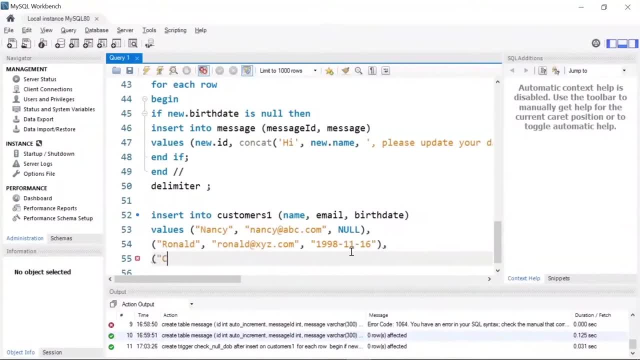 november and let's say 16th. okay, now we'll add another customer, let's say krish picture. we'll give the email id of krish, so krish at the rate xyzcom. so now i'm going to add more customers. call them the email id of chris at the rate xyzcom. 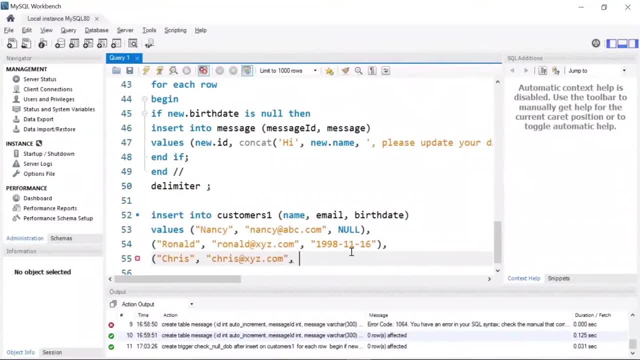 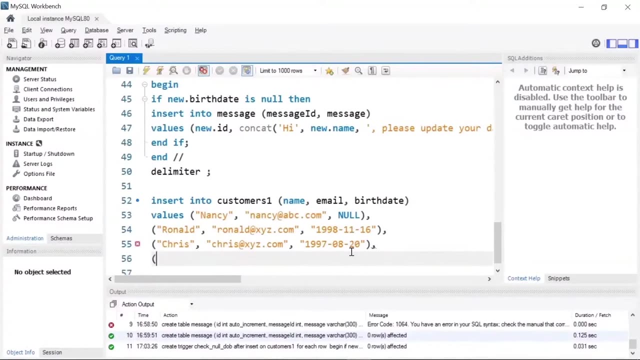 and let's say, we'll give the date of birth as 1997 08 20. and finally, we'll add one more record for another customer, let's say Alice. I'll give the email ID as Alice, at the rate ABC comm, and this time I'll purposely pass the date of. 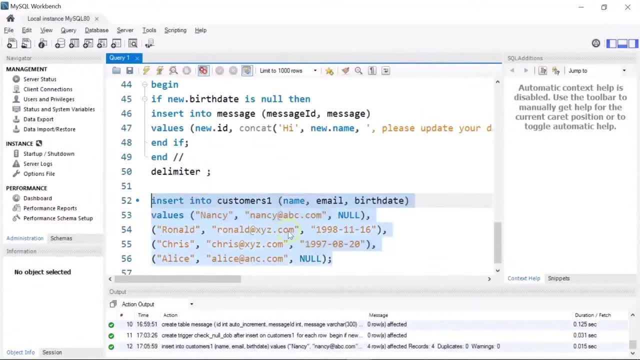 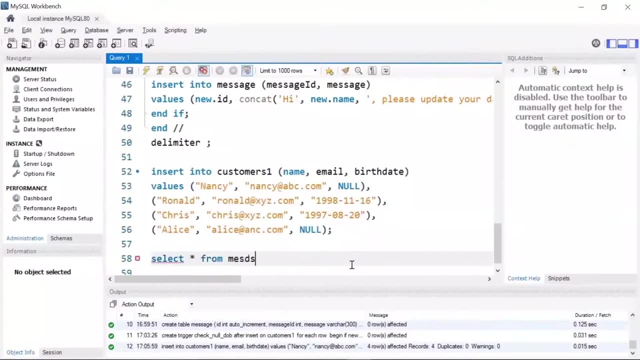 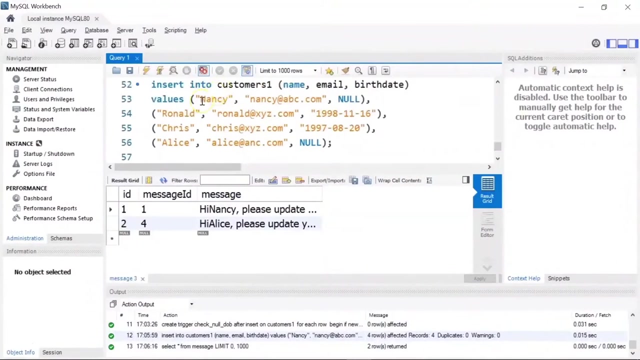 birth as null. all right, so let's run the insert query. okay, now let me display the message table for you so that you can see the output and how our after insert trigger works. there you go. so, if you see this, we had inserted four rows of information, out of which the first customer ID and the 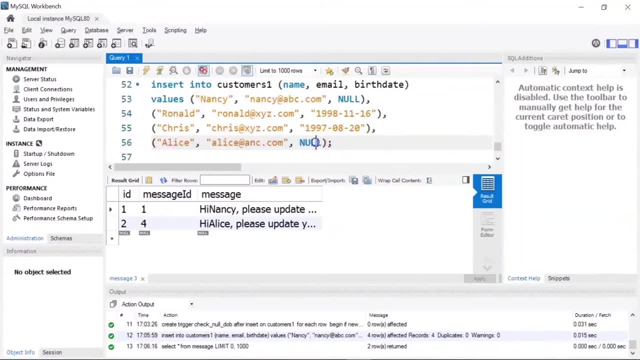 fourth ID had null date of birth. so for those two values you have the messages hi, Nancy, please update your date of birth. and then you have hi- Alice, please update your date of birth. now you can give a space between hi and the name of the customer. all right, now, moving ahead, let's understand how. 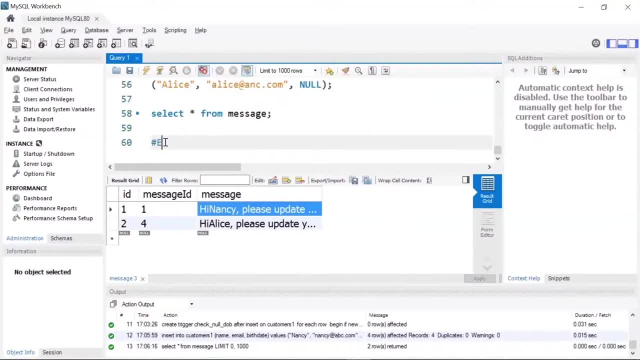 before update trigger works, so I'll give a comment here as before update. okay, now to show you how, before update works. first, we'll create a table called employees. all right, so let me create my table. that is, create table called employees. right, so let me create my table. that is, create table employees. I'll give my 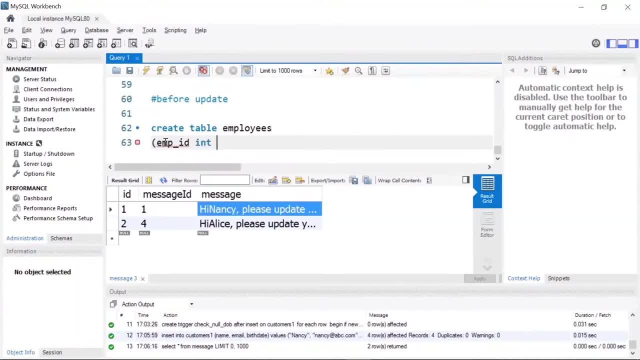 column as employee ID. this is going to be an integer type and it will be my primary key. next we'll have the employee name. this will be of varchar type and you add the number of regulations, insert приход's names into it and the name of the employee and you code number. 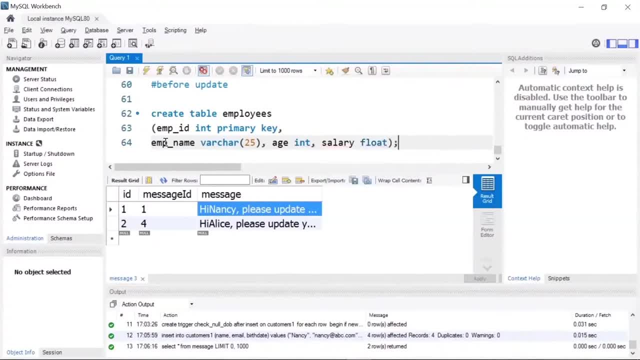 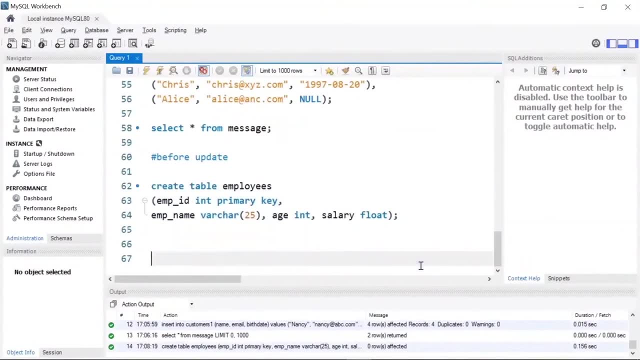 наж, sustainable actions, dan- and let's say the size would be 25 comma. then we'll have the age of the employee. age will be of integer type and finally we'll have the salary of the employee employees table. okay, so here on the notepad, I have already written my insert. 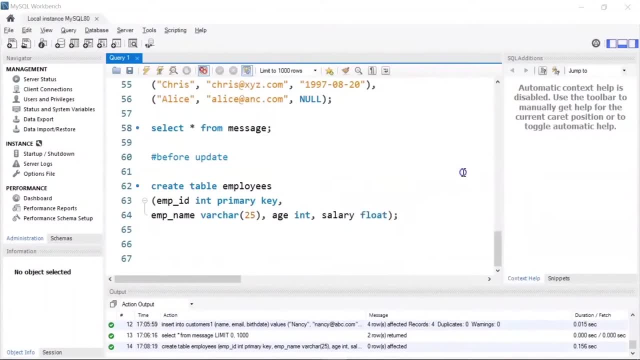 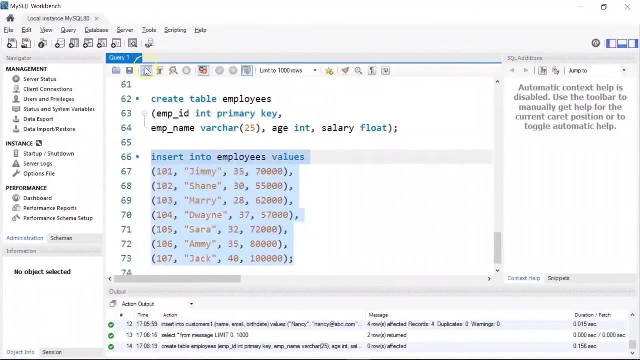 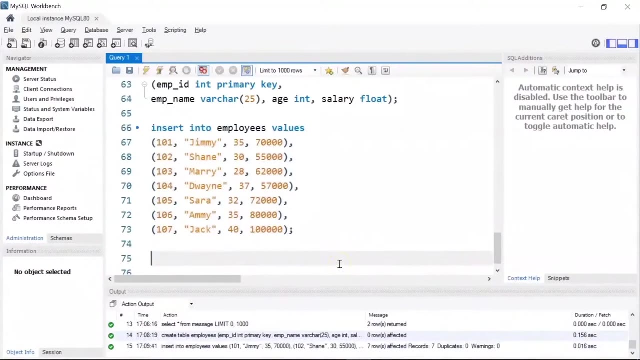 query. so I have inserted nearly seven records, so let me paste it here. all right, I'll just go ahead and run this insert query, so that will insert seven employees to our table. okay, next we'll write our before update trigger command. so first and foremost I'll write my delimiter, followed by the create trigger. 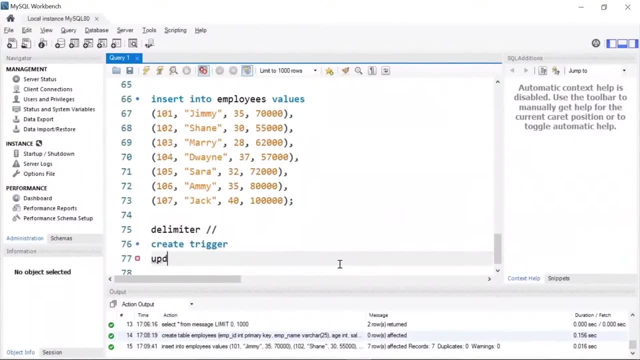 command. I'll give my trigger name as update underscore trigger. let's bring this to the top. okay, I'll use before update on my table, that is employees. for each row, I'll write begin. my condition would be: if new dot salary is equal to, let's say, $10,000, I'll write then set new dot. 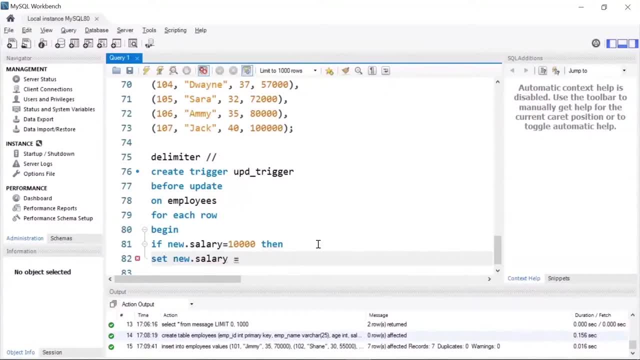 salary equal to $85,000. I'll give a semicolon. then I'll use. else, if new dot salary is less than $10,000, then I'll set new dot salary to less than $10,000, let's say $72,000. I'll give a semicolon. I'll end the if statement. I'll close the. 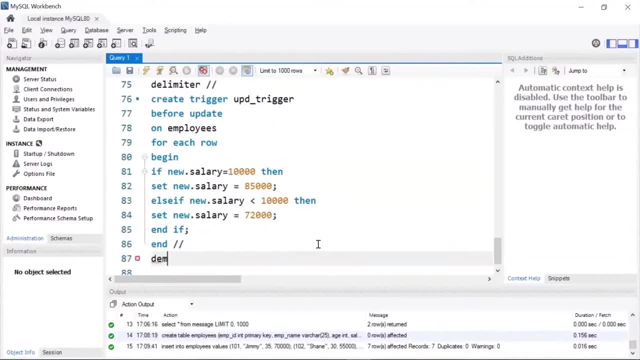 delimiter by giving a semicolon. okay, so if you see the employees table, we have the salary values here. now, in case, while updating the table, if the salary is equal to $10,000, we'll set the new salary to $85,000. else, if the salary is less than $10,000, we'll set the salary. 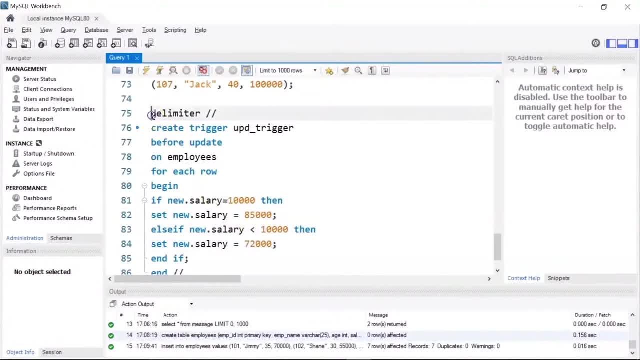 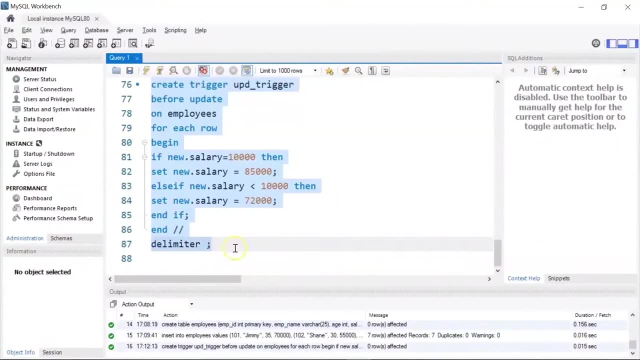 column values to $72,000. so let's go ahead and run this trigger query. all right, now let me use my update command so I'll write update employees. I'll write: set salary is equal to, let's say, $8,000. now, if you see, 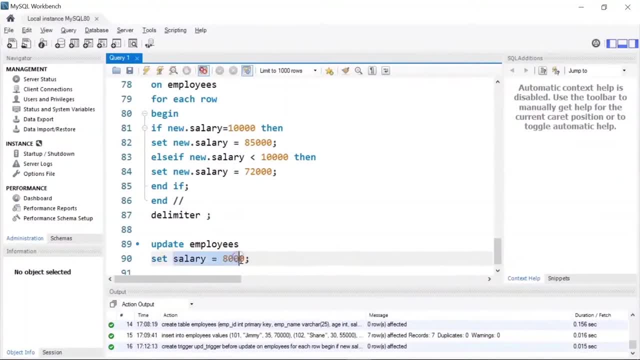 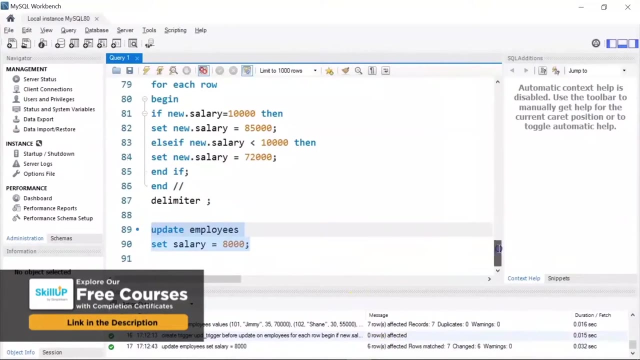 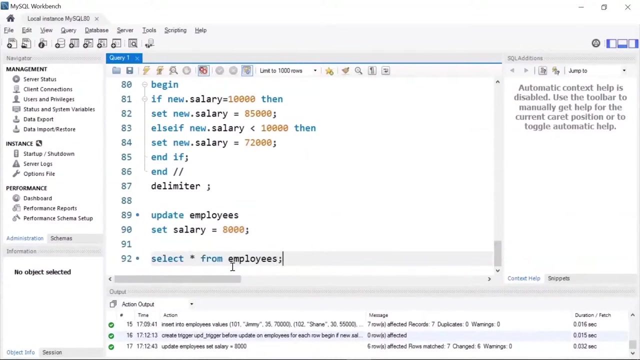 our trigger query we are setting the salary to $8,000, which is clearly less than $10,000. so our new salary would be $72,000. so let me run this, okay, so you can see here six rows affected. so I'll write now: select star from employees. let's run this okay, if you see. 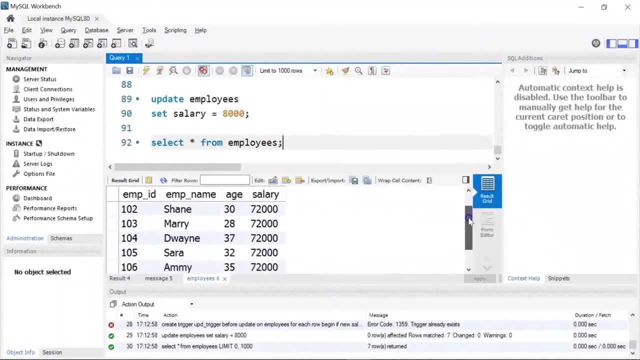 this. we have converted our salary column to $72,000, since we updated the salary to $8,000 and, according to our trigger query, if it's less than $10,000, the salary should be $72,000, which you can see here all right now. 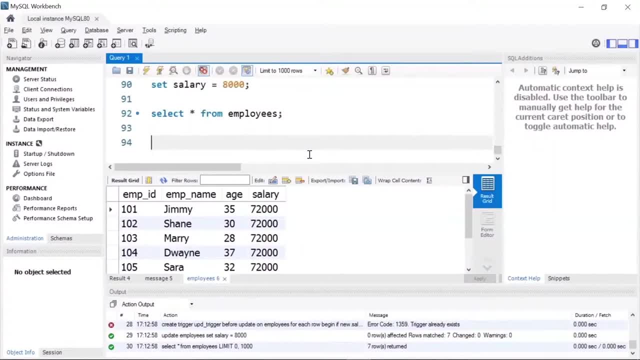 moving to our final demo. this time we are going to explore how before delete trigger command works. so in this example we'll create a table called salary. we'll store the deleted record in a new table using the before delete trigger. so first I'll give my comment as before trigger. 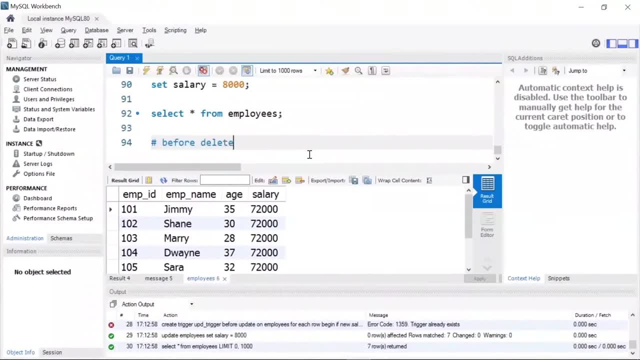 comments are always useful, since they make your query more readable. so let me now create my salary table. so I'll write create table salary. I will create my salary and set the table pedestrian on the right. make it a property. click on set table pedestrian and then select create table pedestrian and then. 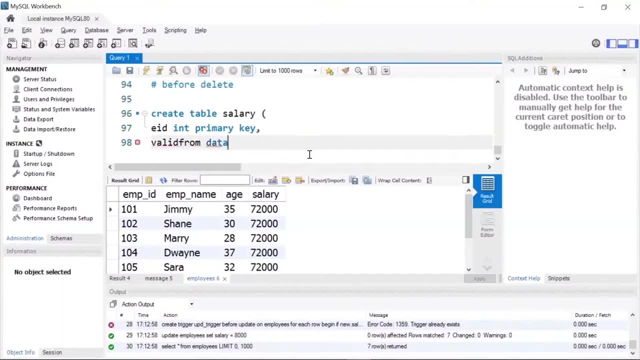 select that tree творy table pedestrian. so let me now create my salary table. so I means the date from which this salary was effective is going to be of type date and not null, and then I'll have the amount. amount will be of type float and again not null constraint. 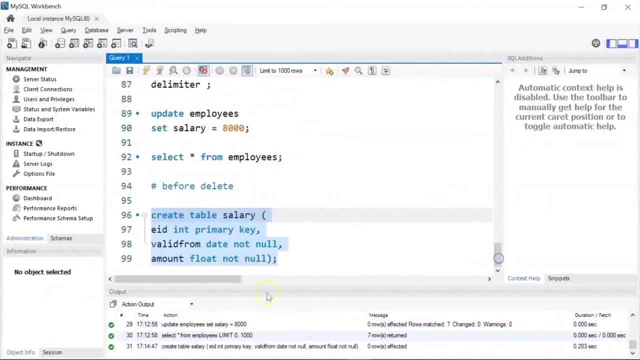 let me run the create table command. okay, so we have created our salary table. now the next thing is to insert a few values. so I'll write insert into salary. I'll give my column names as eid comma valid from comma amount. I'll write values. my first employee id would be 101, followed by a. 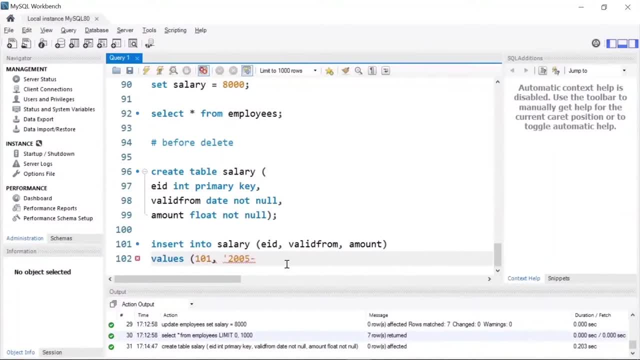 date, let's say 2005. let's say the amount is fifty five thousand dollars. I'll give another row of information. this time the employee id is 102 and I'll give a valid from date. let's say: I'll give another employee id, let's say 103, 2006. 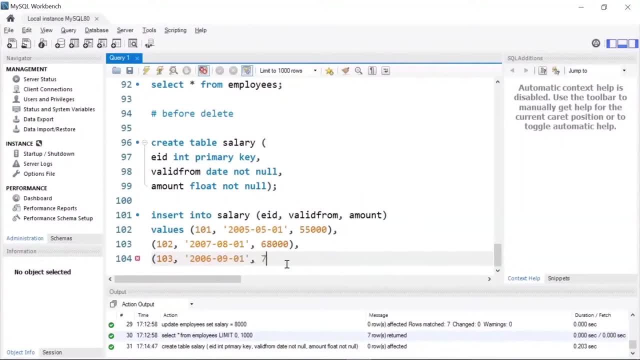 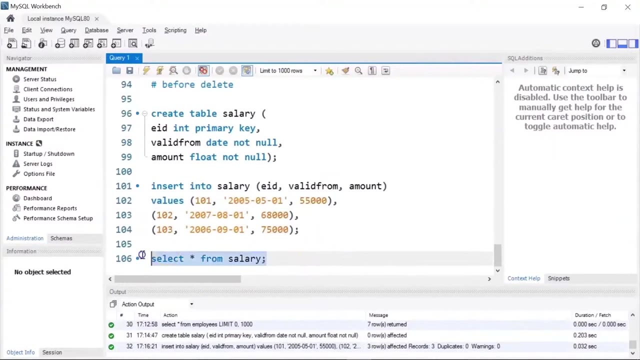 zero nine zero one, and let's say the amount is seventy five thousand dollars. okay, let's run this. all right, you can verify also, so I'll write: select star from salary. say what the minimum of salary you want to give is all right. say what the minimum of salary has been. 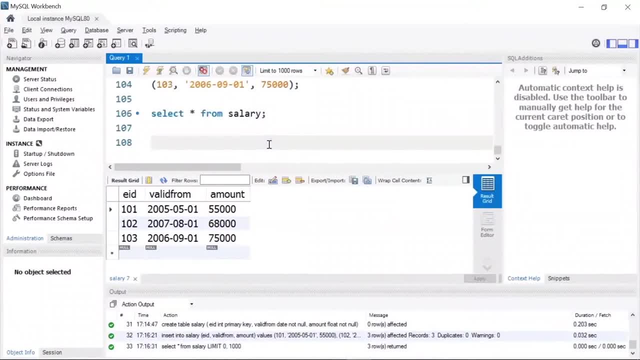 you can see, here we have displayed the results of information. the next step is to create another table. that will. so let's write create table. let's say the name of the table is create, or let's say salary delete. I'll write salaryel Now. this will have the id. 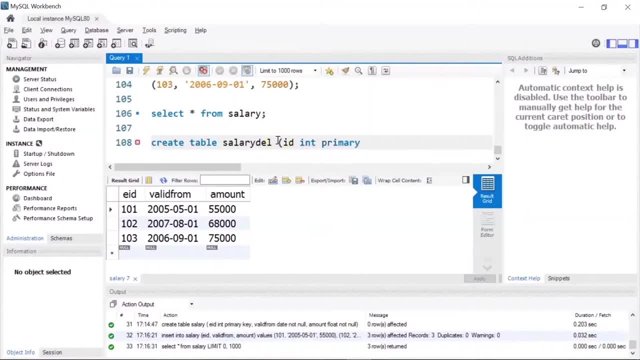 and the type of the integer and the private integer. I'll also use the auto increment operator. Next, we have the eid, which is of type integer. I'll write valid from date and not null. Then I have the amount column, which is of type float and not null. 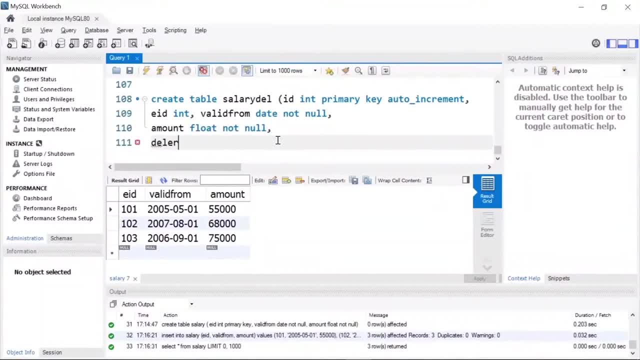 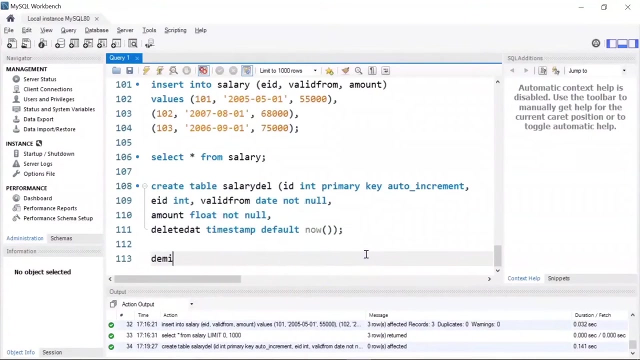 My final column would be deleted at. The data type will be timestamp. I'll use the default constraint as now, So this will return the time and the date at which the record was deleted. Alright, Let me create this table, Okay. Finally, Let me write my before delete trigger command. 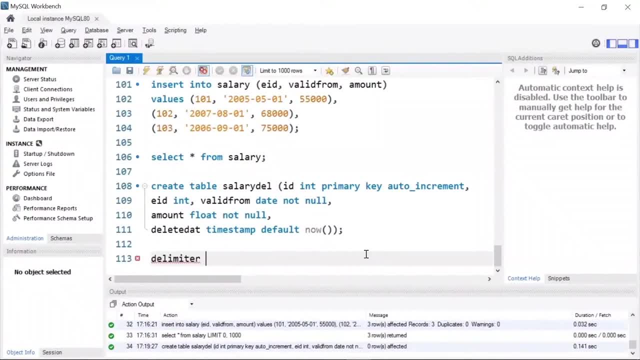 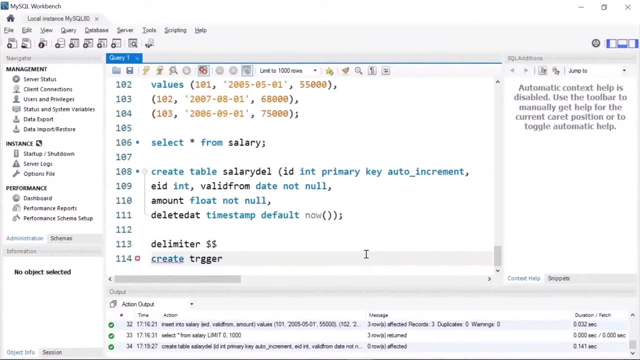 So I'll first declare my delimiter. Let's say this time I'm using the dollar symbol. I'll write create trigger. My trigger name would be salary underscore delete. before delete: on my table that is salary. for each row I'll write begin. Next, Let's insert into 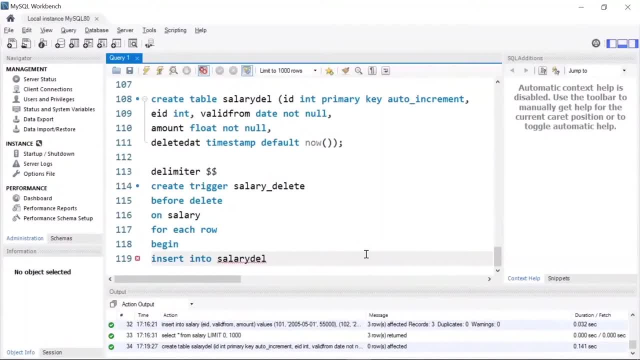 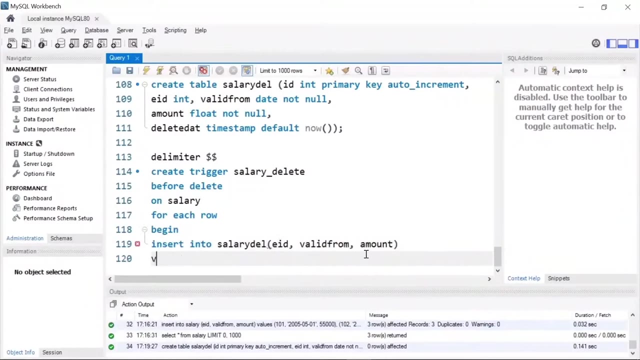 salary delete. I'll give my columns as employee id: valid from and amount. Now we'll insert a few values. I'll write values: old dot, eid comma. old dot valid from comma. old dot amount. I'm going to close with the delimiters. Now let's run our. 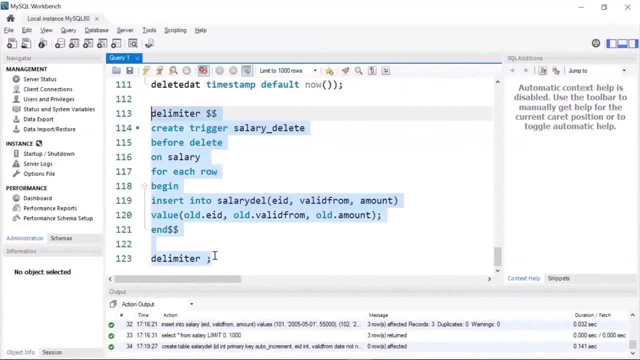 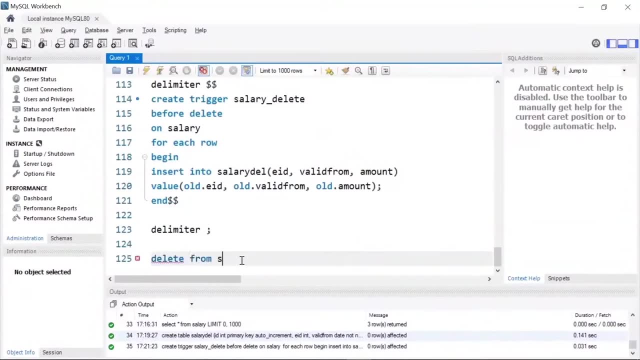 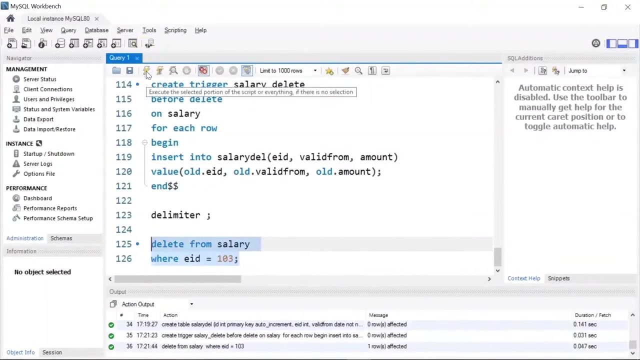 before delete trigger. Alright, Now let me go ahead and delete one of the records from the salary table. So I'll write delete from salary where employee id is, let's say, 103. Let me run this query. Okay, so you have successfully deleted one of the records from the salary table. 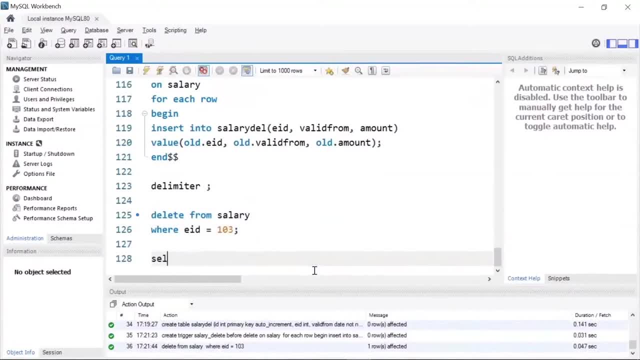 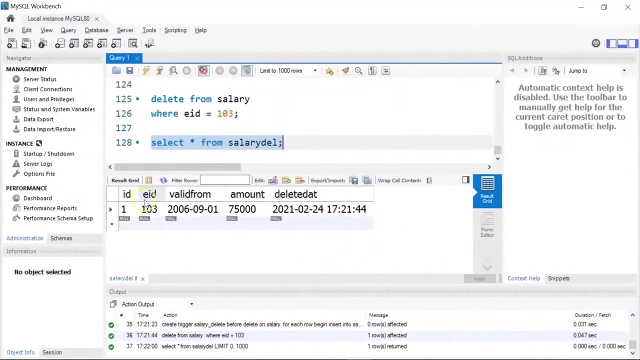 One of the records in the table. Now, if you see our other table, that is, salary delete, You will find this information present in the salary delete column. so we had deleted one row of information, that is for employee id 103, which you can find it here. Now the final. 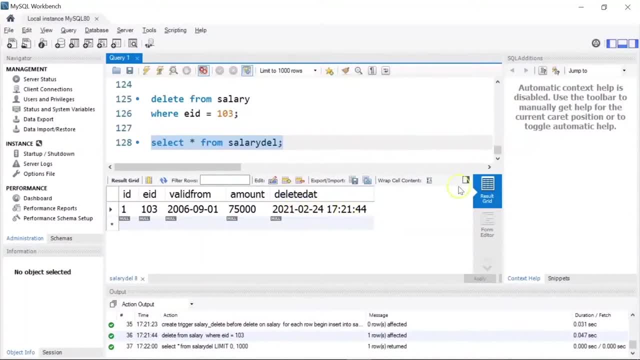 column that is delete at shows the time at which the information was deleted or the row was deleted Alright, So let me go to the top and just give you a recap of what we did in this demo. So first we created our database called triggers. then we started with 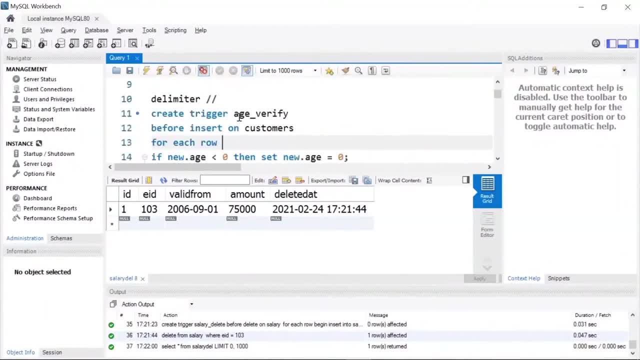 before insert trigger where we inserted customer table and then we verified the age of the customers So we saw if the age was less than 0, then we set the age to 0. We inserted a few records to the customer table and purposely we inserted some negative age records. 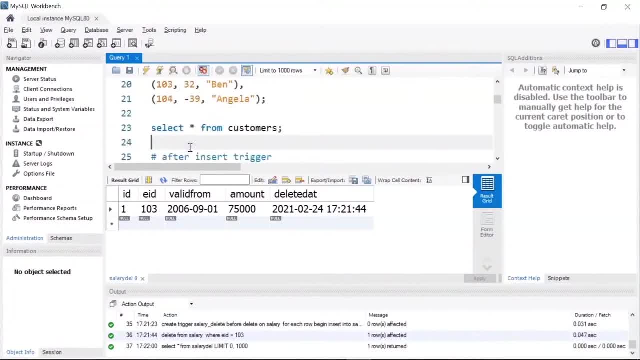 and then we converted this age records to 0. Then we learnt how an after insert trigger works. so we created two tables, customers 1 and message. so wherever the customers date of birth was missing, we passed in a message saying: hi, the name of the customer, please update your date of birth. 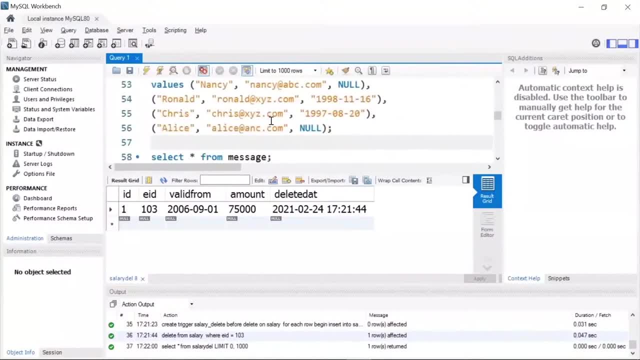 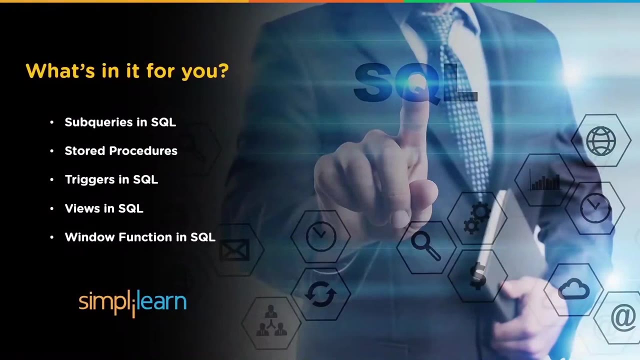 Alright, Now moving ahead, we saw how before update trigger works and finally we learnt about before delete trigger. So in this video we will learn sub queries in SQL. We will also have a look at stored procedures and learn about triggers in SQL. We will cover views in SQL. 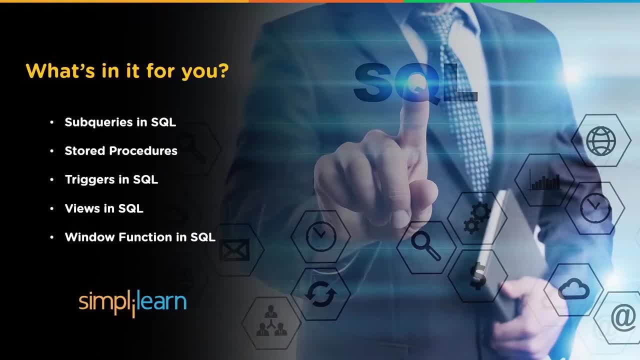 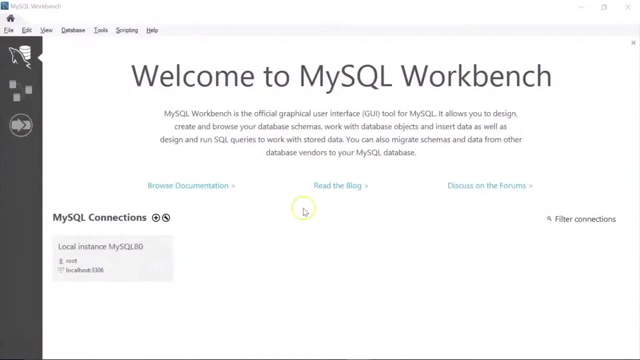 and look at some of the important windows functions in SQL. Now, to learn all of these, we will be using the MySQL workbench on windows. So let's get started with sub queries in SQL. So let me head over to my MySQL workbench. So currently I am on my MySQL. 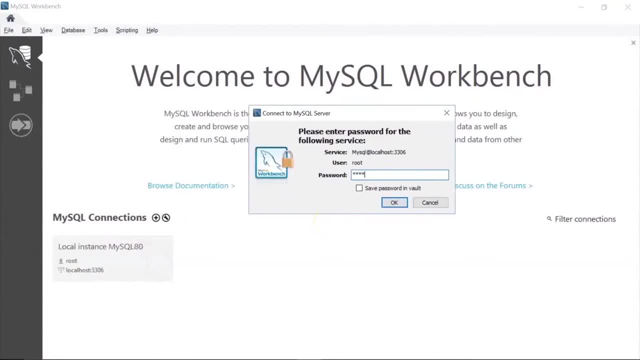 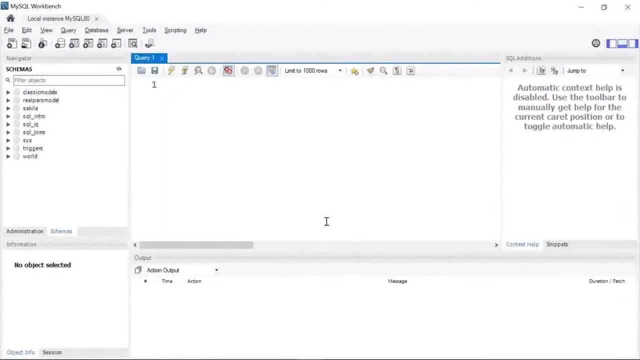 workbench. let me connect to the local instance. so I will give my password. I will click on ok, Alright. So this is my MySQL workbench query editor. so first we are going to learn sub queries. Let me give a comment and write sub queries, Alright. So first of all let's understand. 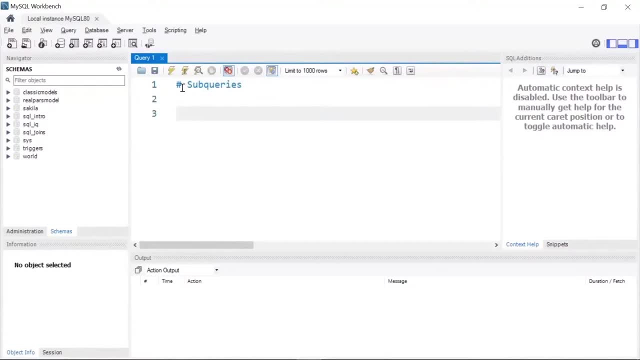 what a sub query is. So a sub query is a query within another SQL query that is embedded within the where clause from clause or having clause. So we will explore a few scenarios where we can use sub queries. So for that I will be using my database, that is, sql underscore intro. 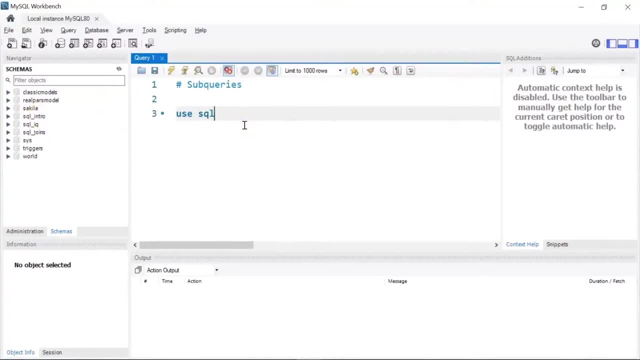 So I will write my command: use sql underscore intro. Now this database has a lot of tables. I will be using the employees table that is present inside sql underscore intro. Let me just expand this and you can see here we have an employees table, So let me first show you. 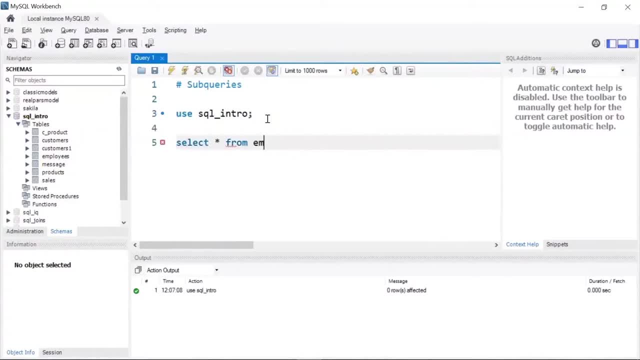 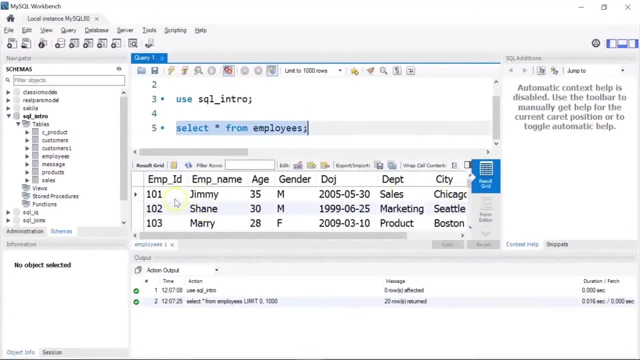 the contents within this table I will write select star from employees. Let me execute it. Ok, you can see here. we have the employee id, employee name, age, gender, there is date of join, department, city and salary, and we have information for 20 employees if I scroll down. 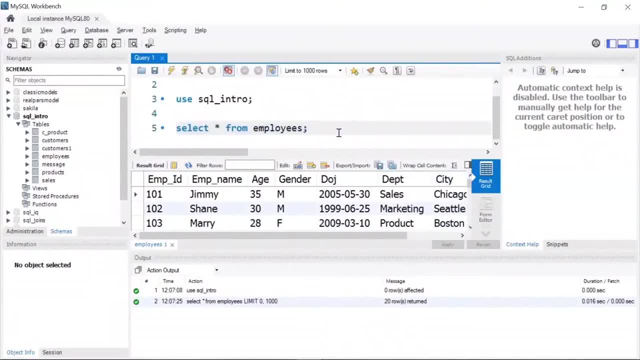 you can see there are 20 employees present in our table. So let's say you want to find the employees whose salary is greater than the average salary. In such a scenario, you can use a sub query. So let me show you how to write a sub query. 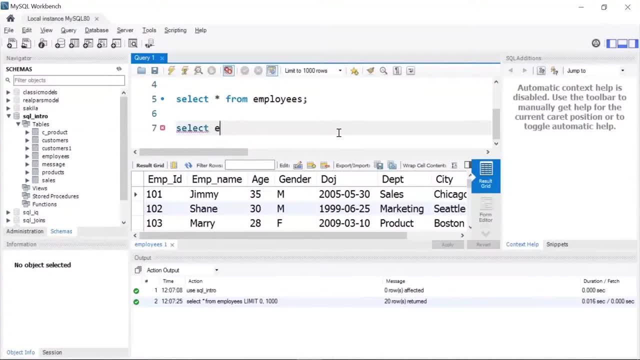 I will write the select statement. In the select statement I will pass my column names that I want to display. So the column names I want are the employee name, then I want the department of the employee and the salary of the employee from my table name, that is employees. 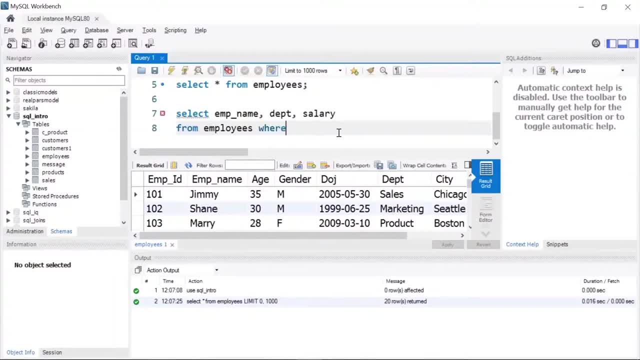 next I will use a where condition where my salary should be greater than the average salary of all the employees. So I will write salary greater than. after this, I am going to write my sub query, So I will give select average of salary from my table name, that is. 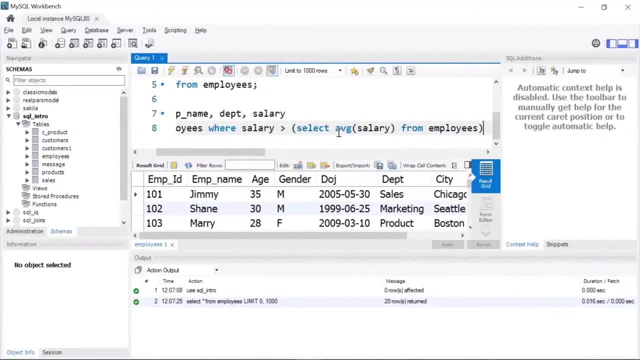 employees and I will close the bracket and give a semicolon. So what it does is: first it is going to find the average salary of all the employees that are present in our table. Once we get the average salary number, we will use this where condition where salary is greater than. 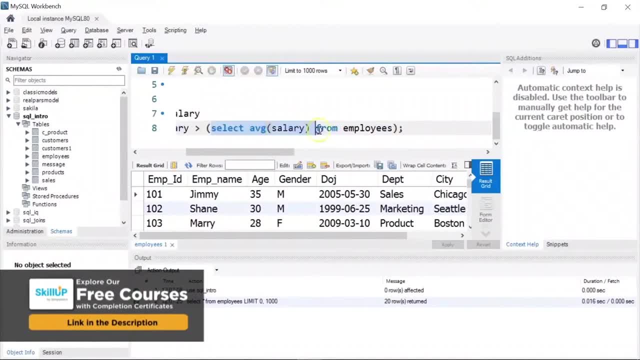 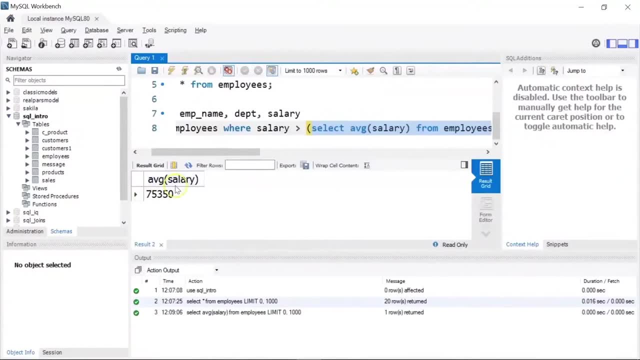 the average salary number. So the inside sub query. let me run it first. If I run this, this gives you the average salary of all the employees, which is $75,350. Now I want to display all the employees who have salary greater than $75,350. 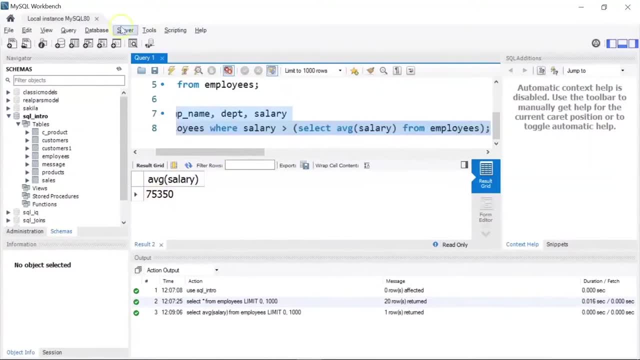 So let's run our sub query. There you go. So there are 8 employees in our table who have a salary greater than the average salary of all the employees. Alright, Next, Let's see another example. Suppose this time you want to find the employees whose salary is greater than. 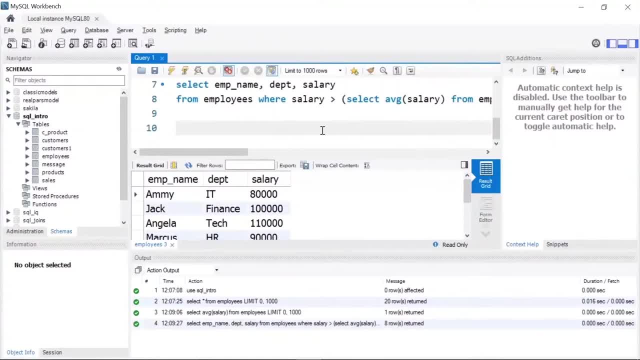 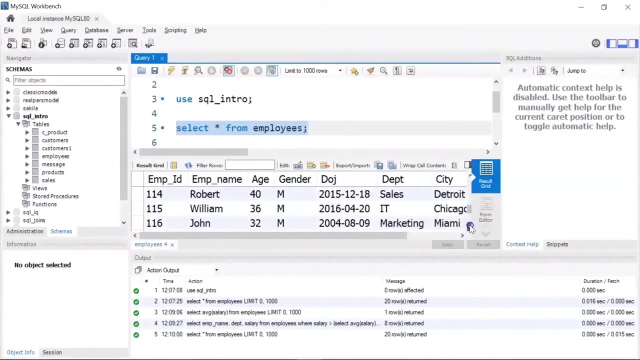 John's salary. So we have one employee whose name is John. Let me run the table once again. Okay, if I scroll down, you see we have an employee as John. You see this. Our employee ID 116 is John and his salary is $67,000. I want to display all the employees. 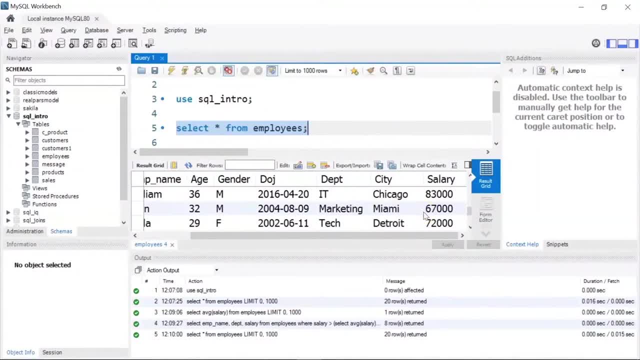 whose salary is greater than John's salary, So basically all the employees who are earning more than $65,000. I want to print them, So let's see how to do it. I will write: select- I want the employee name, comma, the gender of the employee. I also 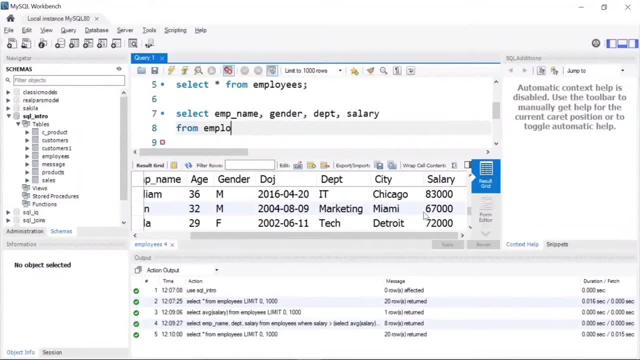 want the department and salary from my table name, that is, employees. I will write where salary is greater than I will start my opening bracket. inside the bracket I am going to give my inner query, that is, select salary from employees where the employee name is John. So within single quotations. 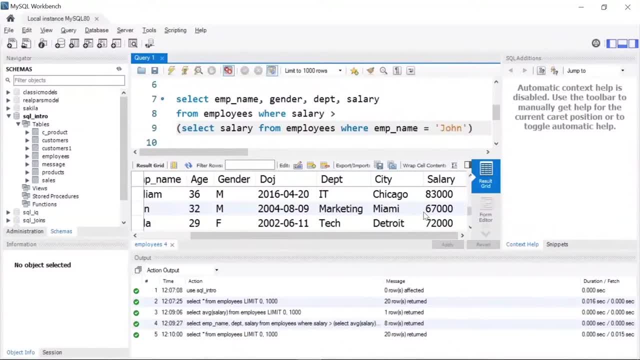 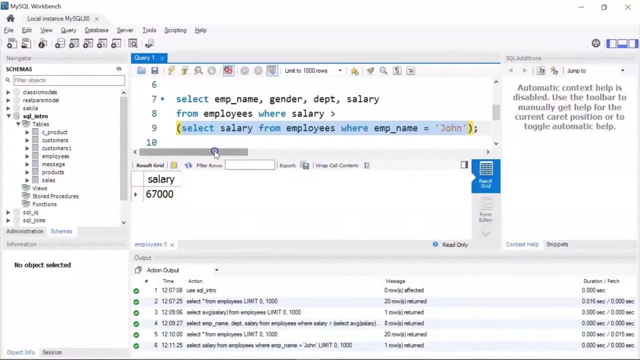 I will give John as my employee. I will end with a semicolon, So let me first run my inner query. So this will give us the salary that John has, which is $67,000. Now I want the employees who are earning more than $67,000. 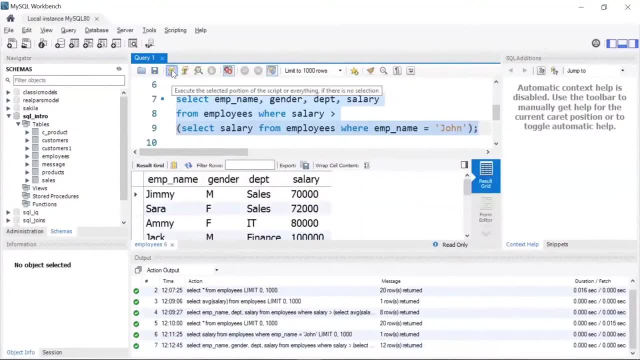 So let's run our sub query. Ok, so you can see 12 rows returned, which means there are 12 employees in our table who are earning more than $67,000. You see here, all these employees have a salary greater than $67,000. Ok. 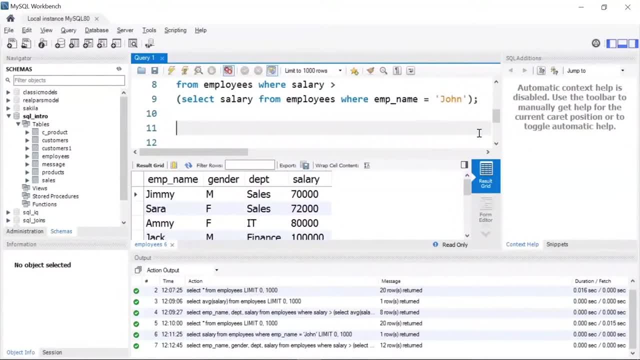 Now you can also use sub queries with two different tables. so suppose you want to display some information that are present in two different tables. you can use sub queries to do that. So for this example, we will use a database that is called classic models. you can see the first database. 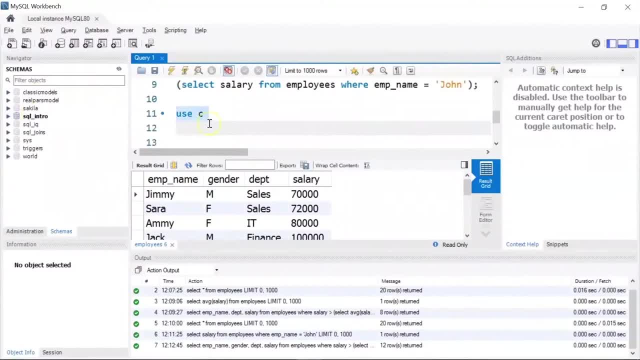 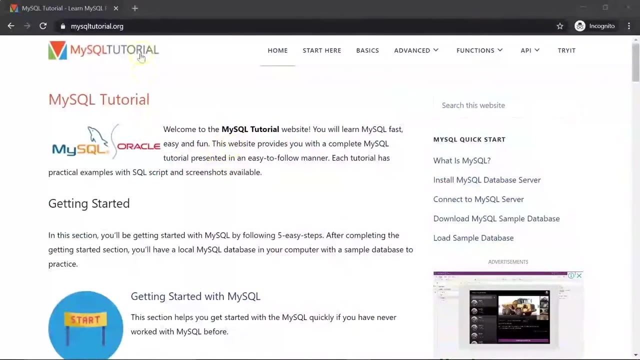 So let me use this database called classic models. I will write: use classic models. Now, this database was actually downloaded from the internet. there is a very nice website. I will just show you the website name. So this is the website, that is mysql-tutorialcom org. you can see. 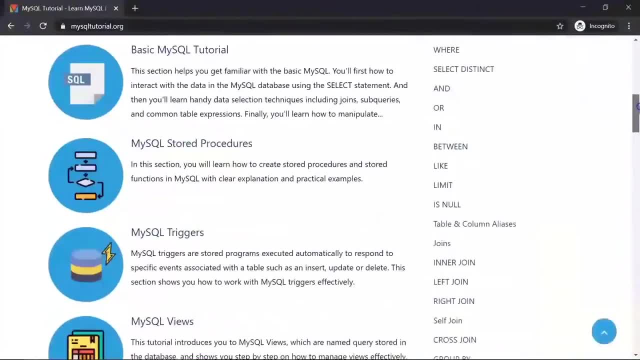 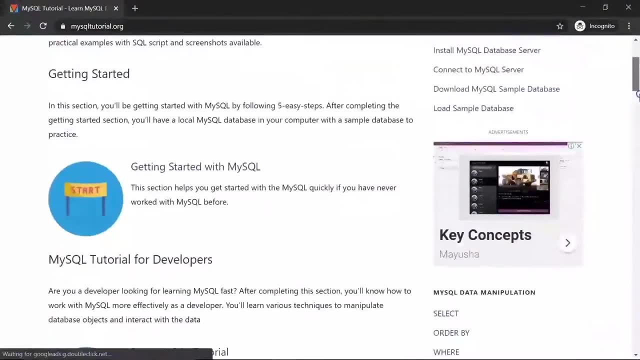 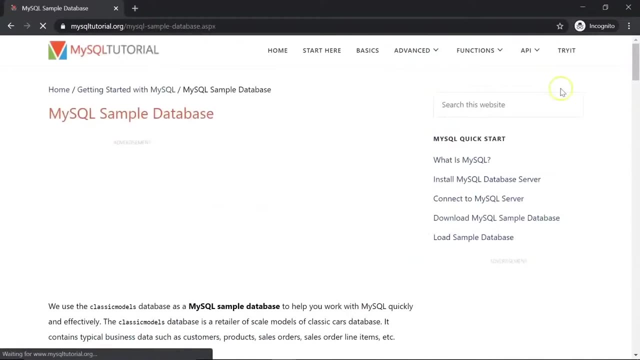 here. they have very nice articles, blogs from where you can learn mysql in detail. So we have downloaded. they have a mysql sample database. if you click on this it will take you to the link where you can download the database. so they have this download link which says: 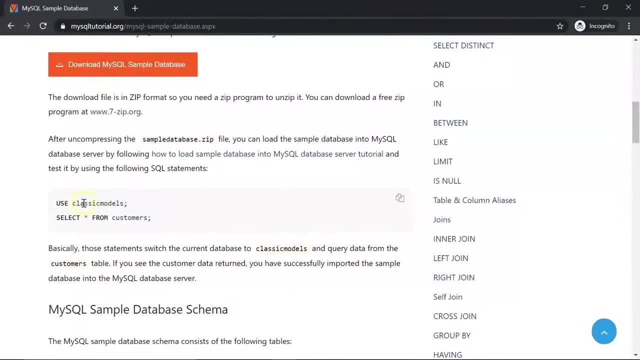 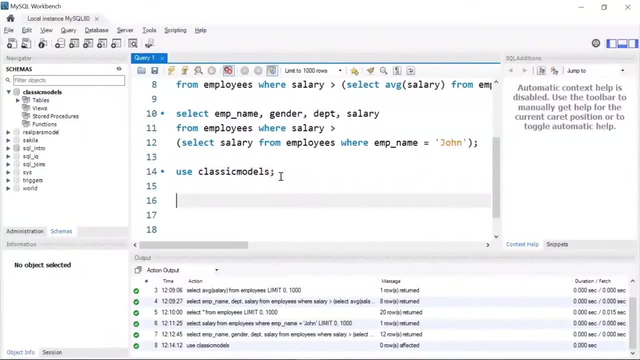 download mysql sample database and the name of the database is classic models. alright, so we are going to use this classic models database throughout our demo session. if I expand the tables section, you can see there are a lot of tables that are present inside this classic models database we have. 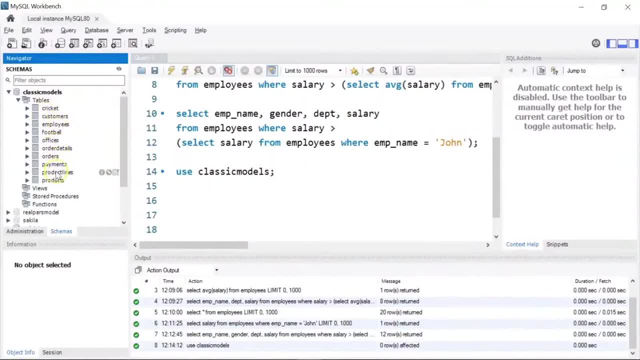 cricket customers. there is employees office, there is orders, order lines and many more. so for our sub query we will be using two tables, that is, order details and products table first. let me show you the content that is present inside the products table first. if I run this, 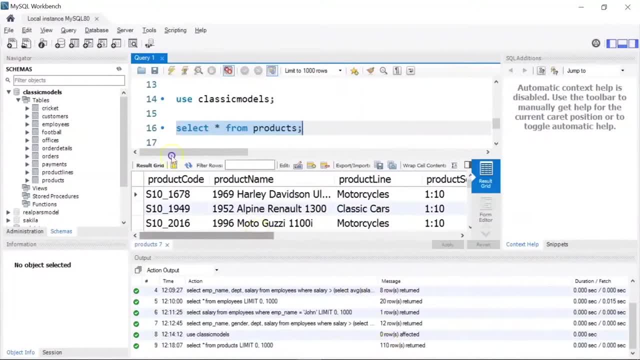 you see, here it says 110 rows return, which means there are 110 different products that are present in our table, which has the product code, the product name, product line. we have the product vendor description, quantity in stock, buy price, MSRP, the other table we are going to use. 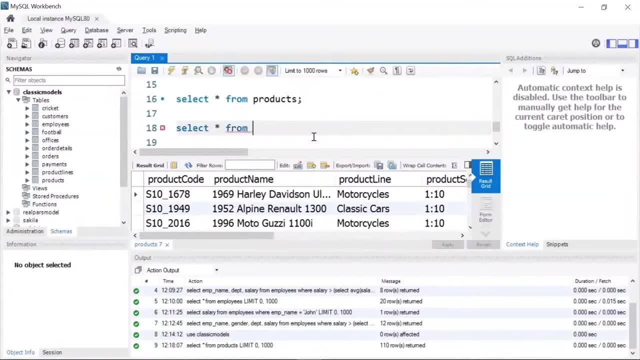 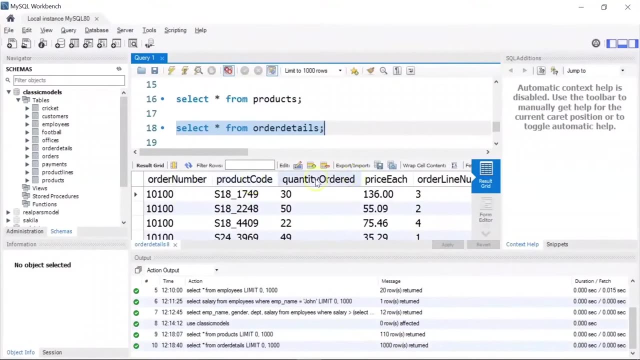 is order details, which has the details of all the orders. let me show you the records. order details tables has. okay, so there are thousand records present in this table. you have the order number, the product code, quantity, ordered price of each item. you have the order line number as well. 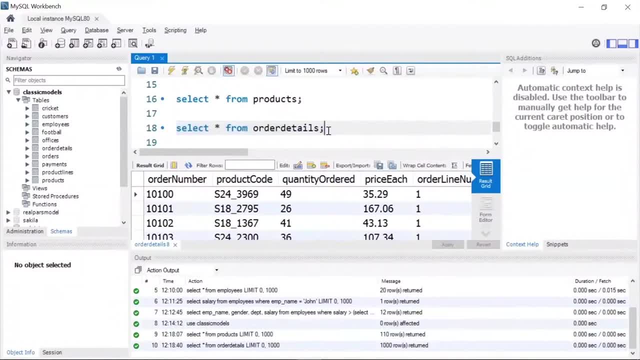 okay, now we want to know the product code, the product name and the MSRP of the products whose price of each product is less than hundred dollars. for this scenario, we are going to use two different tables and we are going to write a sub query. okay, so if you see here, 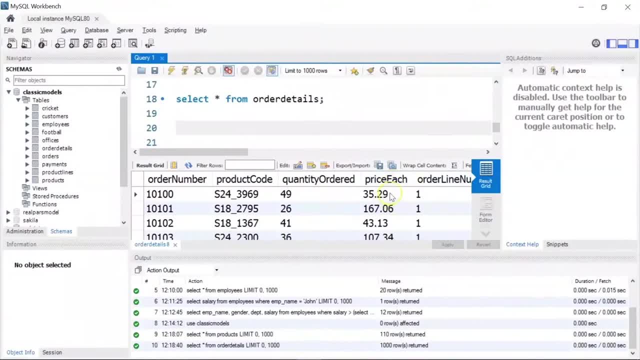 in the order details table we have a column called price each. I want to display the product code, the product name and the MSRP of the products which have a price of each product less than hundred dollars. so the way I am going to do is I will write select. 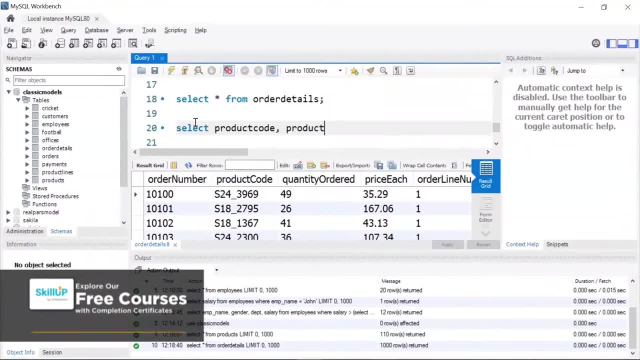 product code, comma, product name. now one thing to remember: this product name is actually present inside our products table and product code is present in both the tables, that is, products and order details. here you can see this is the product code, column comma MSRP, which is present inside the products table. 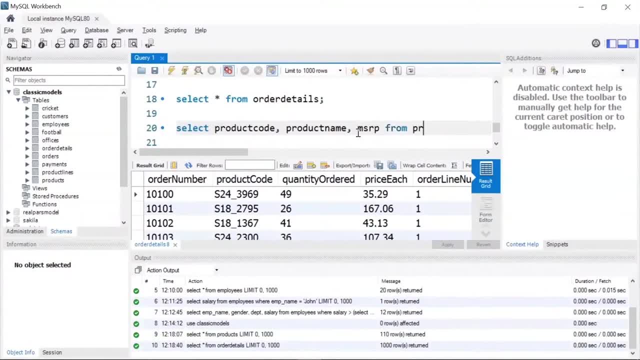 again from my table, that is, products, where I will write product code. I am going to use the in operator. next I will write my inner query, that is, select product code from my table order details where my price of each product is less than hundred dollars. let me 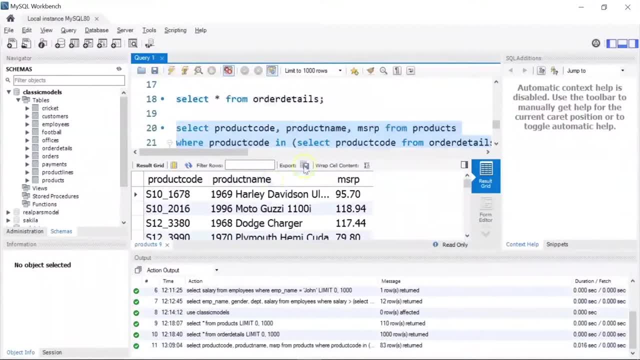 run this. ok, you can see. there are total 83 products in our table which have a price less than hundred dollars. you can see the price here. ok, now we learn another advanced concept in SQL, which is known as stored procedures. I will just give a comment saying: 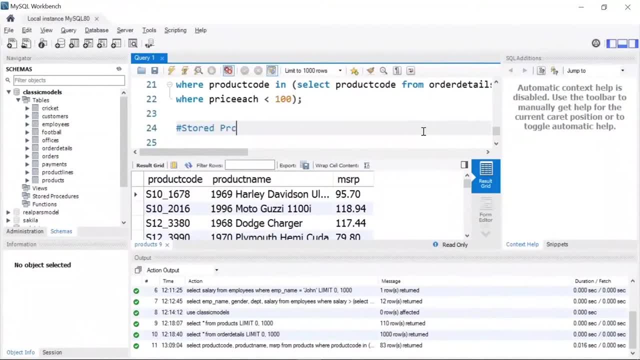 stored procedure. ok, so first let's understand what is a stored procedure. a stored procedure is an SQL code that you can save so that the code can be reused over and over again. so if you want to write a query over and over again, save it as a stored procedure. 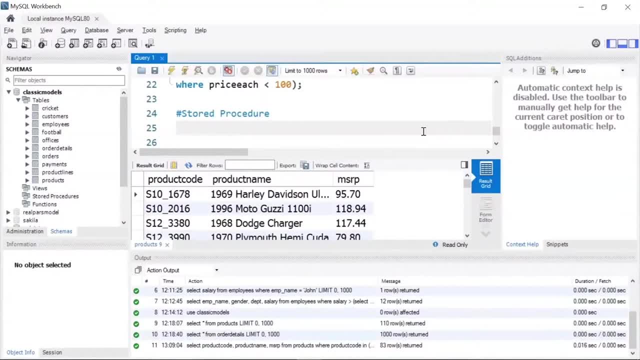 and then call it to execute it. so in this example, I want to create a stored procedure that will return the list of players who have scored more than six goals in a tournament. so I have a database called SQL underscore IQ. these are a few databases that I have already created. 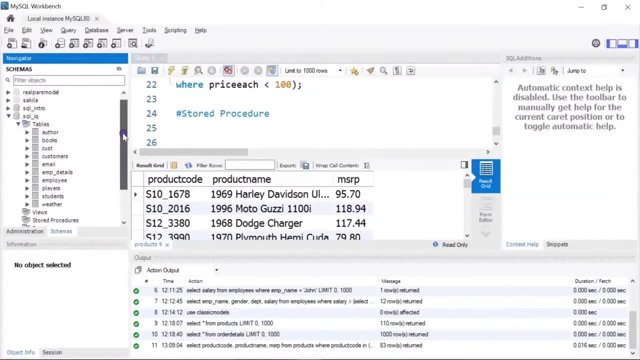 this database has a table called players. if I expand the tables option, you see we have a table called players and you can see the columns: player id, the name of the player, the country to which the player belongs to and the number of goals each player has scored in a particular 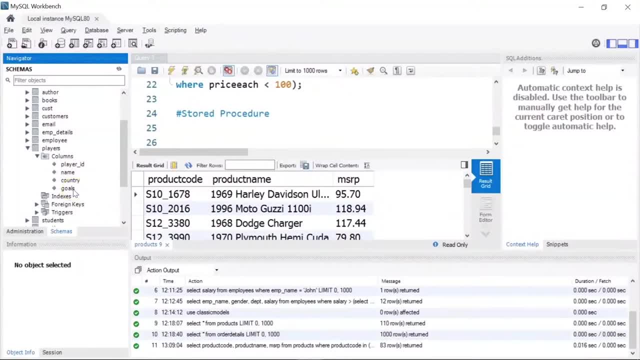 tournament. so I will write a stored procedure that will return the list of top players who have scored more than six goals in a tournament. so first of all, let me begin by using my SQL underscore IQ database. we will run it. so now we are inside the SQL underscore IQ. 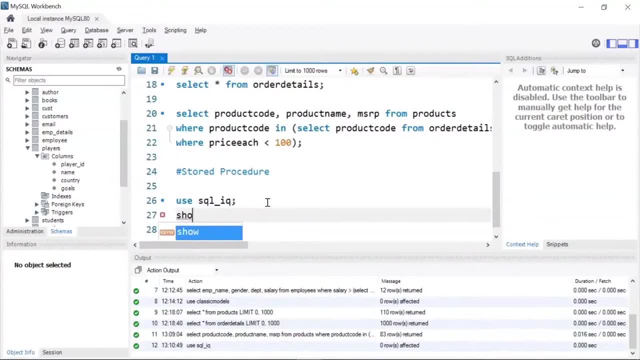 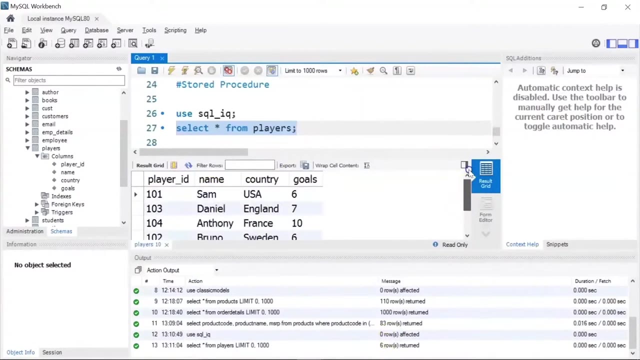 database. let me select star from players to show the values that we have in the players table. you can see there are six players in our table. we have the player id, the names of the players, country to which these players belong to and the goals they have scored. 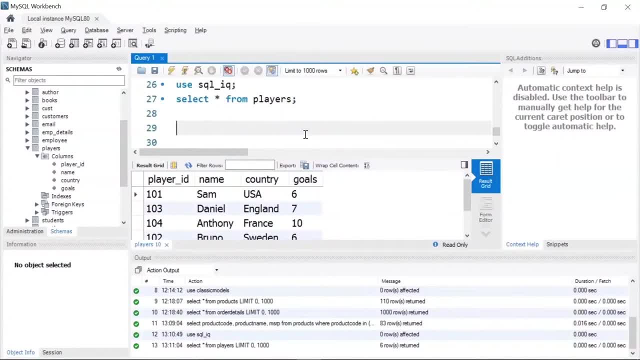 so I will write a stored procedure. so the stored procedure syntax is something like this. it should start with a delimiter. ok, in the delimiter I will write &&. next I will write create procedure, followed by the procedure name. let's say, I want to name my procedure as: 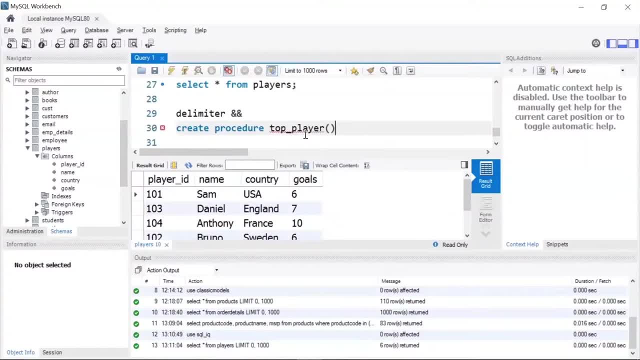 top underscore players and next statement is begin. after begin, I will write my select statement. I want to select the name of the player, the country and the goals each player has scored. from my table, that is players. where I will write goals is greater than 6, I will give a semicolon. 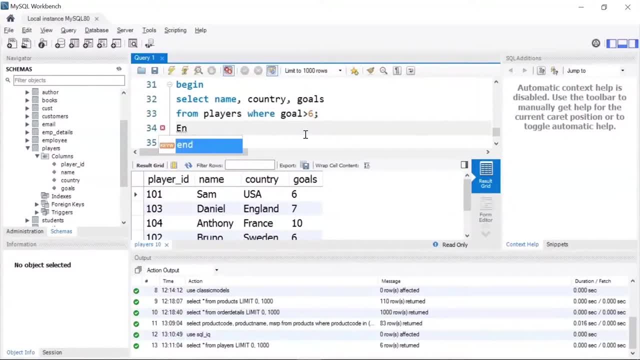 then I will end my procedure with a delimiter that was double ampersand. next I will write delimiter and give a semicolon. now the semicolon suggests this is a default delimiter. then there should be a space. ok, now let's run our stored procedure. there you go. so you have successfully. 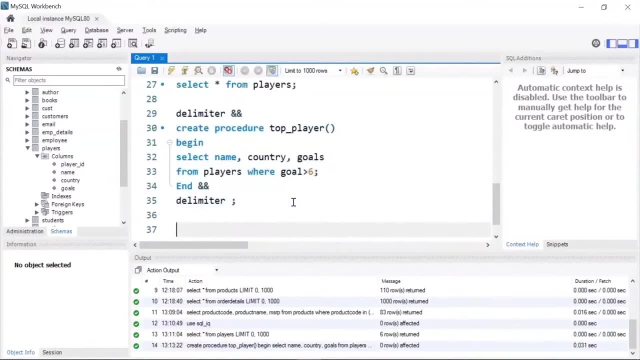 created our stored procedure. now the way to run a stored procedure is you need to use the call method and give the procedure name, that is, top underscore players, in our case, with brackets and a semicolon. let's execute it. ok, there is some problem here, so we made a. 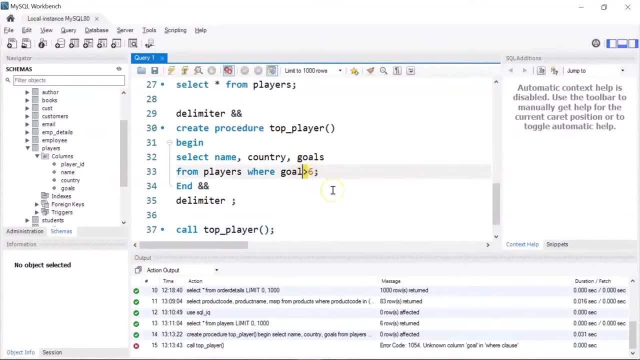 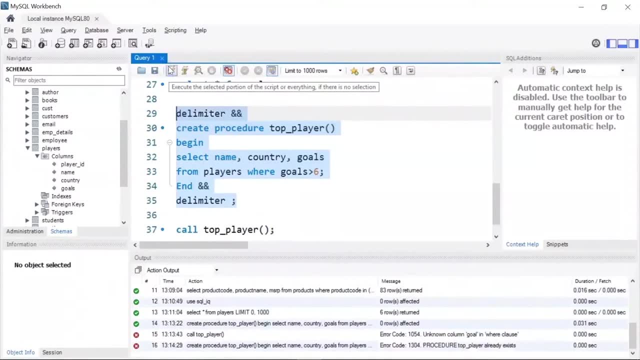 mistake while creating a procedure. the name of the column is goals and not goal. let me create that procedure again. ok, it says the procedure top underscore player already exists. let's just edit the procedure name instead of top player. we will write it as top players and similarly we will edit here. 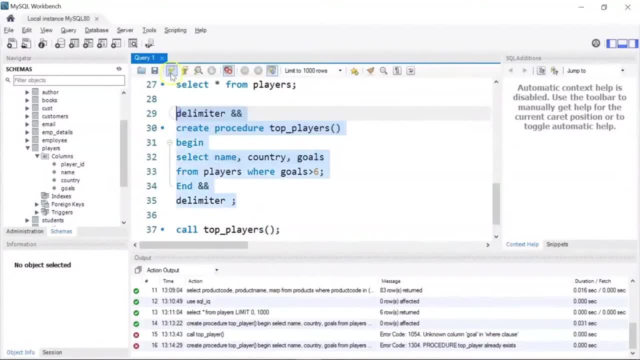 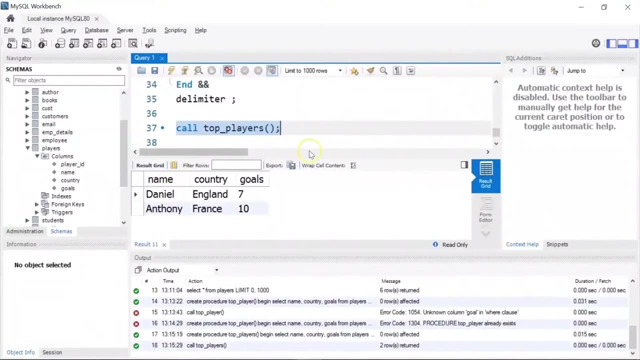 as well. now let's create it again. ok, now to call my procedure. I will write call space followed by the procedure name, which is top underscore players. if I run this, you can see we have two players in our table who have scored more than six goals, so we consider: 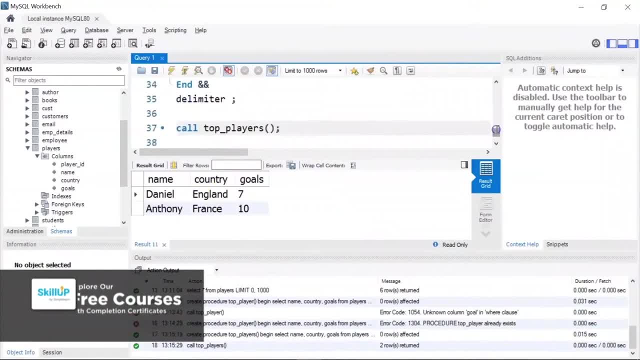 them as the top players in a particular tournament. alright, now there are other methods that you can use while creating a stored procedure. one of the methods is by using an in parameter. so when you define an in parameter inside a stored procedure, the calling program has to pass an argument to the stored procedure. 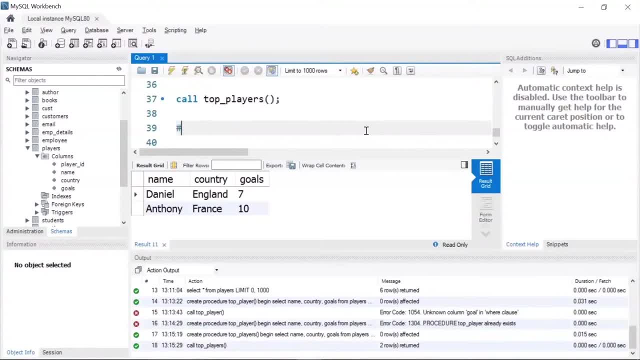 so I will give a comment. stored procedure using in parameter: alright, so for this example, I will create a procedure that will fetch or display the top records of employees based on their salaries. so we have a table in our sql underscore iq database which is called employee details. 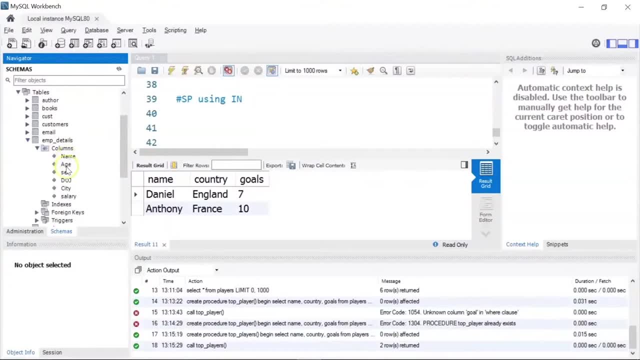 I am going to use this table. you can see we have the name of the employee, the age, sex, then we have the date of join city and salary. using this table, I will create a procedure that will fetch or display the top records of employees based on their salaries. 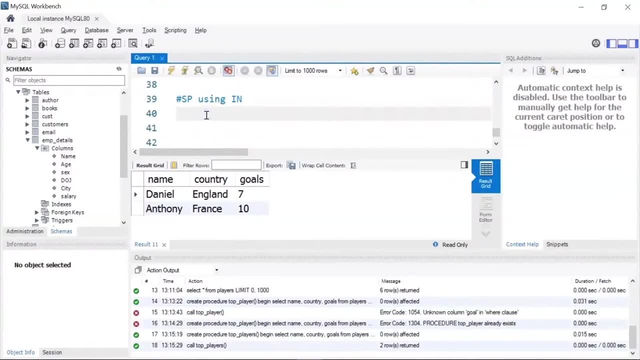 and we will use the in parameter. so let me show you how to do it. I will write in parameter. this time I am going to use forward slash. I will write create procedure followed by the procedure name, let's say SP for stored procedure. sort by salary is the name of my. 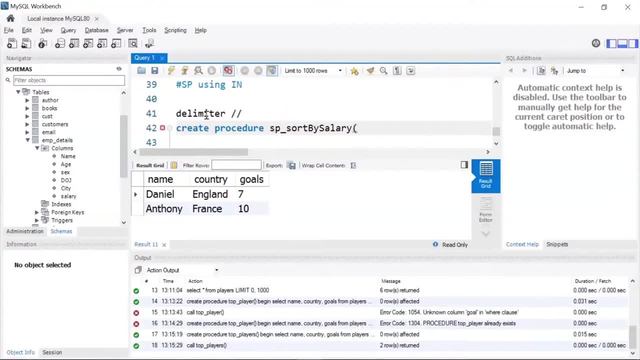 procedure and inside this procedure I will give my parameter in. I will create a variable var and assign a data type for my teacher. then I will write beginning, followed by my select statement, where I will select the name, age, salary from my table name, that is, emp details or employee details. 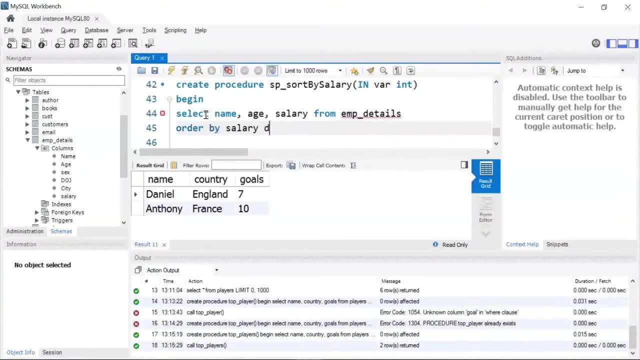 I am going to order this by salary descending and I want to display limited number of records, so I am using this limit keyword and my variable var, which I created here. I will end my select statement, I will end my stored procedure with forward slash and I will go back. 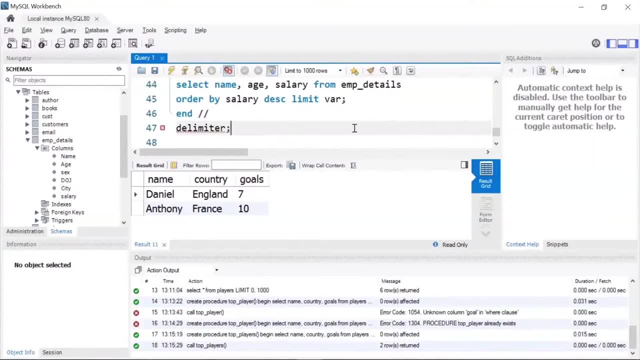 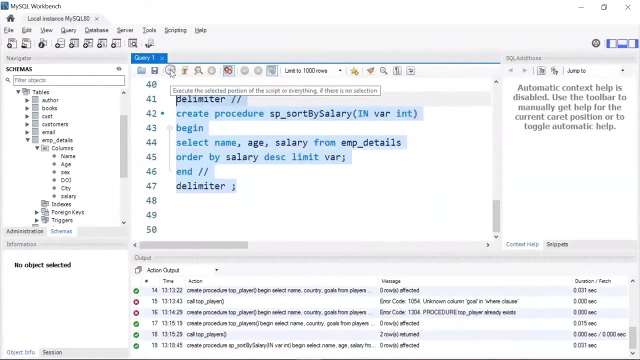 to my default delimiter, that is, semicolon. alright, so let me run this. there should be a space here, alright, so let's run this. ok, you can see we have successfully created our second stored procedure, which is SP sort by salary. now you can also check whether the 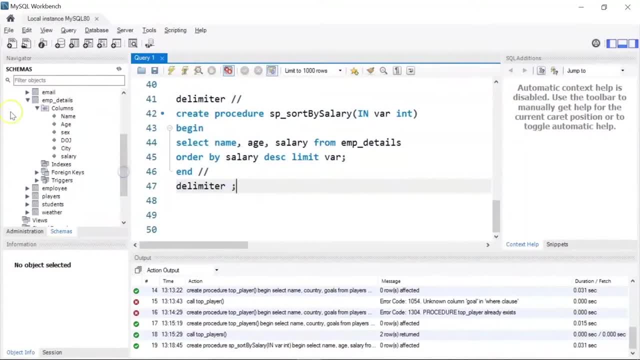 stored procedure was created or not. here you have an option to see the stored procedures. let me just refresh this and you can see we have three stored procedures that we have created so far. one is SP underscore, sort by salary. the other two were top underscore player and top underscore players. 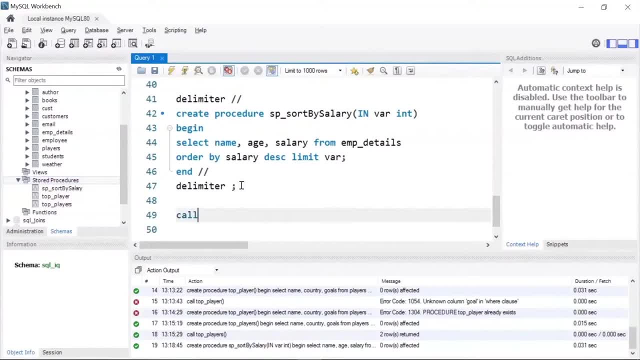 ok, now let's call our stored procedure. I will write call space followed by the stored procedure name, which is SP, underscore, sort by salary, and inside this I will give my parameter, which was actually VAR, and this VAR we have used in limit. let's say I want. 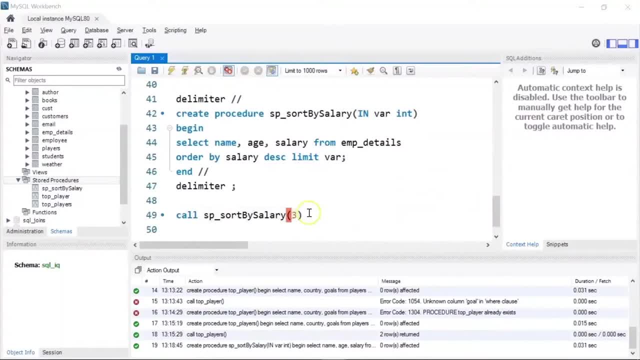 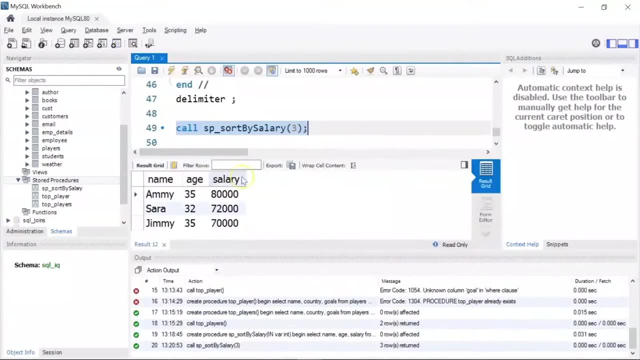 to display only the top three records of the employees who have the top three highest salaries. ok, so let me run it. there you go. so Ami, Sara and Jimmy were the top three employees who have the highest salary. so you saw how you could use the in. 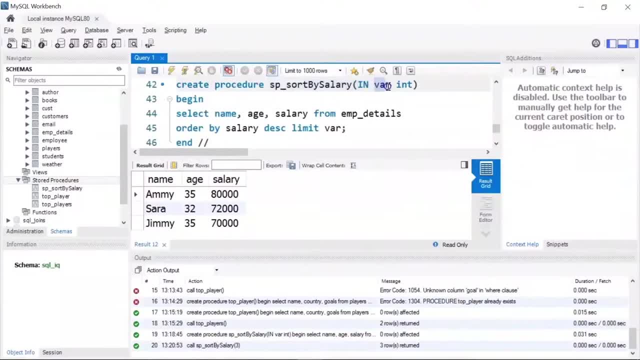 parameter in a stored procedure. we created a variable and that variable we used in our select statement and we called our stored procedure and passed in that variable. ok, now instead of a select statement inside a stored procedure, you can also use other statements. let's say update. so I will create a stored procedure to update. 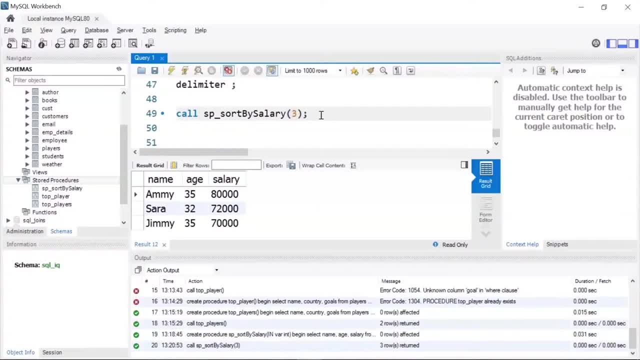 the salary of a particular employee. so in this procedure, instead of select statement we will use the update command. in this example, we will use the in operator twice. so let me show you how to do it. I will write my delimiter first, which is going to be forward slash. 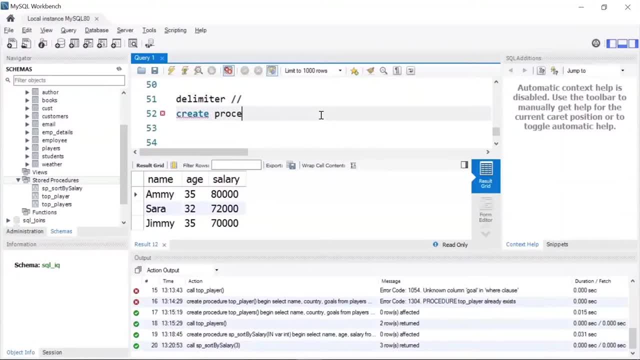 then I will write create procedure. my name of the procedure is going to be update salary and inside the update, my salary name. I will write in and then temp underscore name, which will be a temporary name variable, and the type I will assign is varchar20. I will again use my 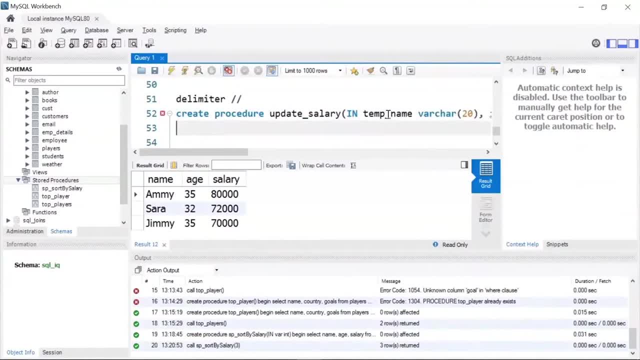 in parameter. I will write in next. my other variable would be new underscore salary and the data type would be float. I will write begin and write my update command or update statement. I will write update table name, that is, employee details. set salary equal to new underscore salary. 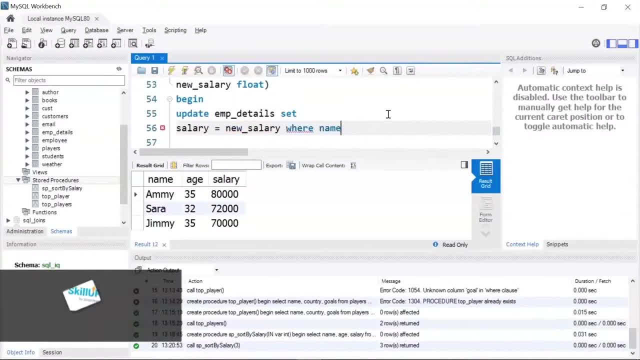 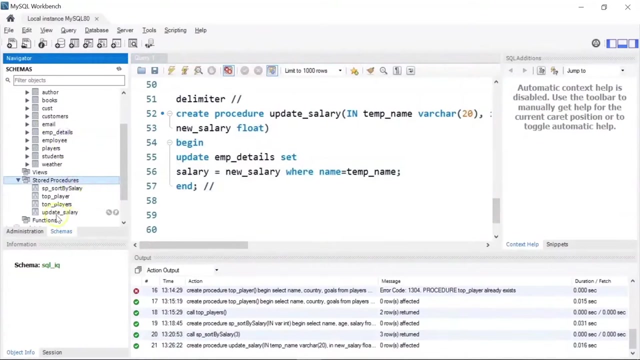 where name is equal to my temporary variable, that is, temp underscore name. so this is my update command and I will end the delimiter. alright, so let's run this. ok, we have successfully created our stored procedure. if I refresh this, you can see I have my stored procedure: update underscore. 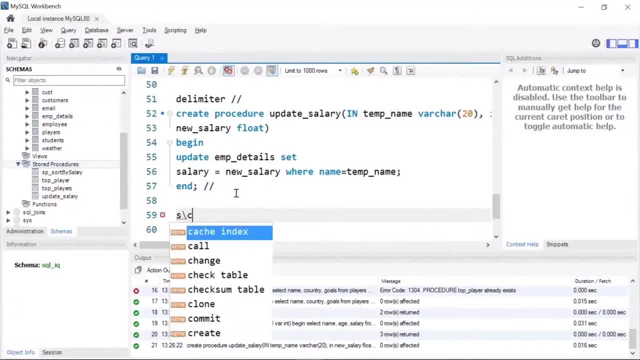 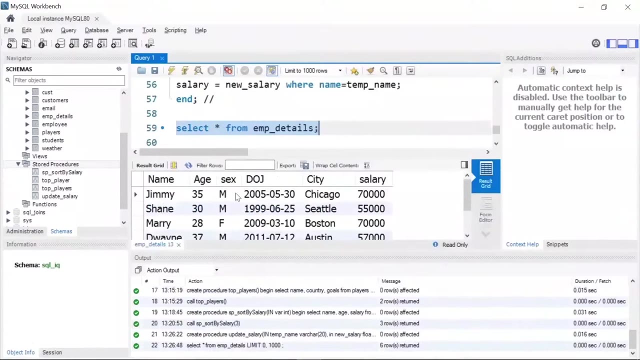 salary. ok, now let's say, first of all I will display my records that are present inside employee underscore details table. ok, so we have 6 rows of information. let's say you want to update the salary of employee Jimmy, or let's say Mary, from 70000 to. 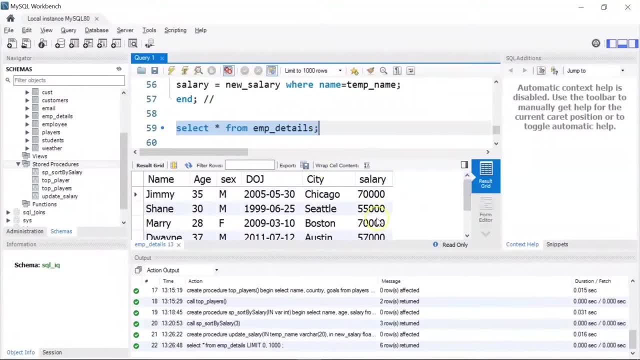 let's say 72000 or let's say 80000. so I will call my stored procedure, that is, update underscore salary, and this time I am going to pass in two parameters. the first parameter will be the employee name and next, with a comma, I will give my 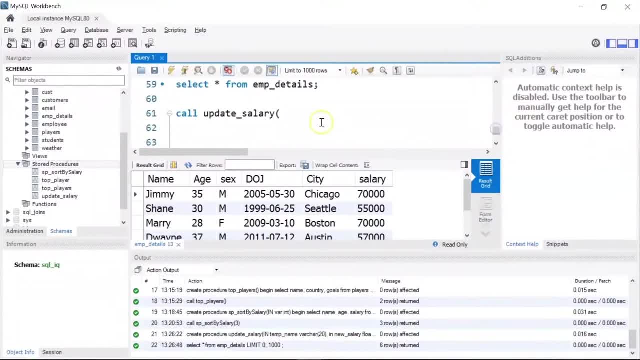 new salary that I want to. so my employee name, let's say, is Mary, and the salary I want to be updated is, let's say, 80000. I will give a semicolon and I will run it. you can see. it says one row affected. now, let's: 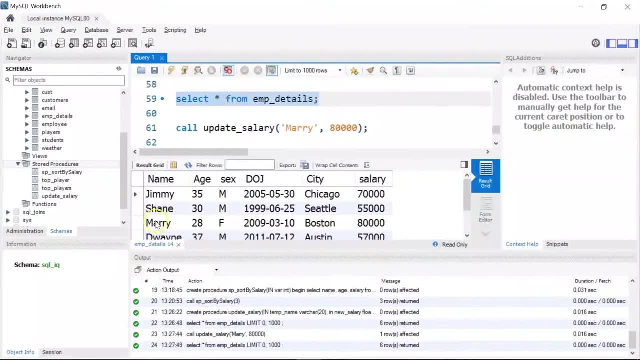 check our table once again. there you go. if you see this record for Mary, we have successfully updated the salary to 80000. now, moving ahead, we learn to create a stored procedure using the out parameter. so I will give a comment. stored procedure using out parameter. okay, 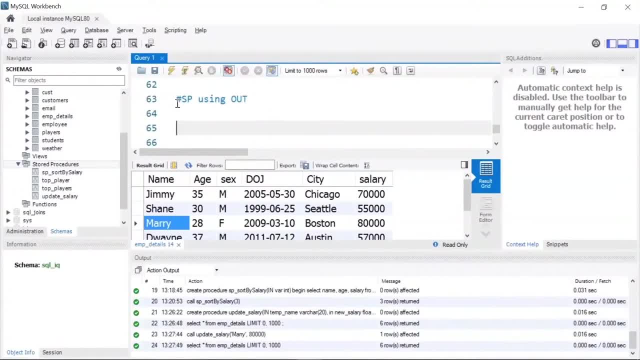 so suppose we want to get the count of total female employees. we will create total employees as an output parameter and the data type would be an integer. the count of the female employees is assigned to the output variable, which is total. underscore empace using the into keyword. let me show. 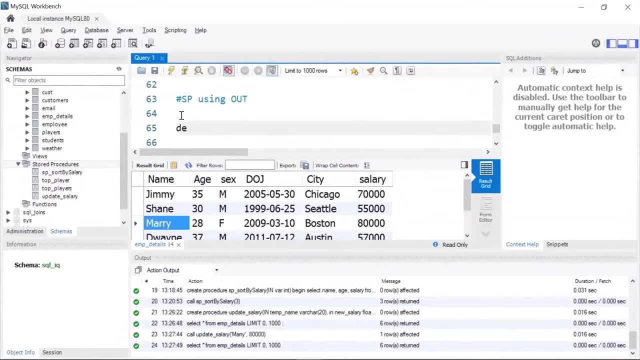 you how to write a stored procedure using the out parameter. so first I will declare my delimiter to forward slash. I will write create procedure followed by the procedure name. it is going to be sp, underscore, count, employees and inside this I am going to give my out parameter. 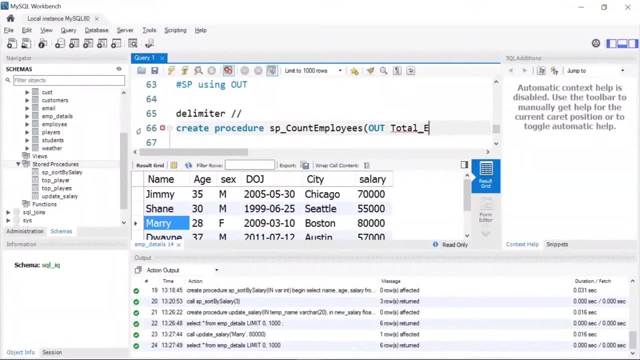 and the variable name, that is, total, underscore empace, which is total employees, and the data type will be integer. next I am going to write begin, followed by my select statement, that is select. I want the count of total employees and the output I am going to put into. 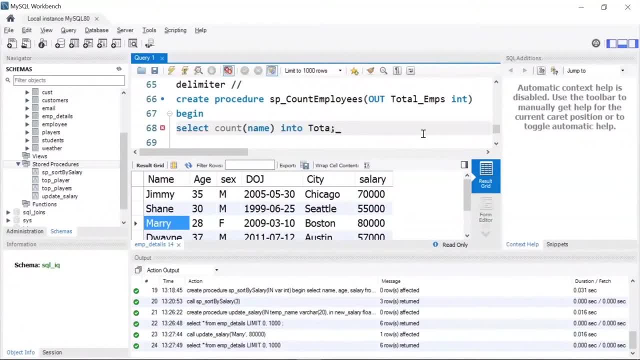 my new variable, that is total underscore, empace from my table, that is emp underscore details where sex is equal to f, which means female. I will give a semicolon. next, I will end it with the delimiter and I am going to change the delimiter to a default delimiter. 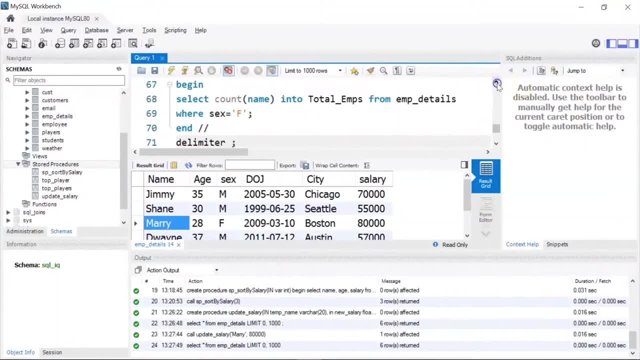 that is colon. so let me tell you what I am doing here. I am creating a new stored procedure that is sp underscore count employees. using this stored procedure, I am going to count the total number of female employees that are present in our table, emp underscore details. so I have used 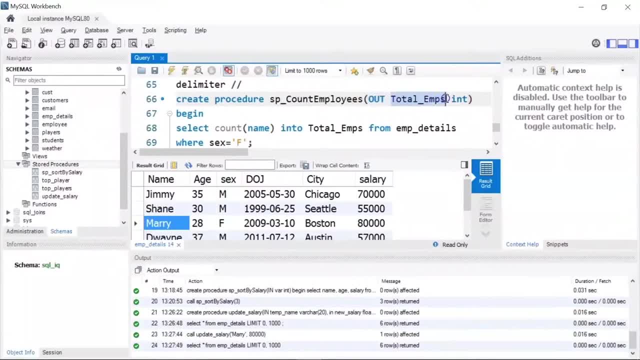 my out parameter and I am creating a new variable called total underscore emp. the data type is integer. here in the select statement, I am counting the names of the employees and the result. I am storing it in total underscore emps. I have used my where condition where. 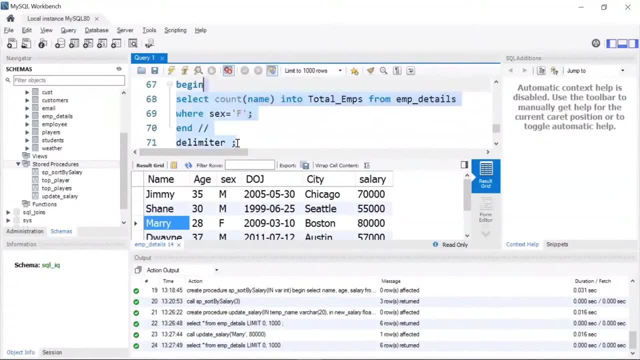 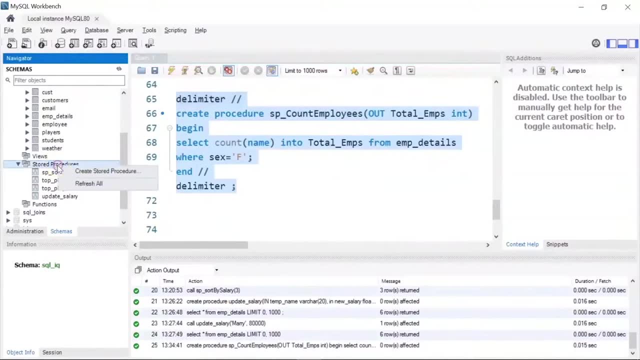 the gender or the sex is female, so let's run this. okay, so we have created our stored procedure. let's refresh this. okay, you can see we have our new stored procedure, sp underscore count employees. now to call it. I will write: call the name of the procedure that is count. 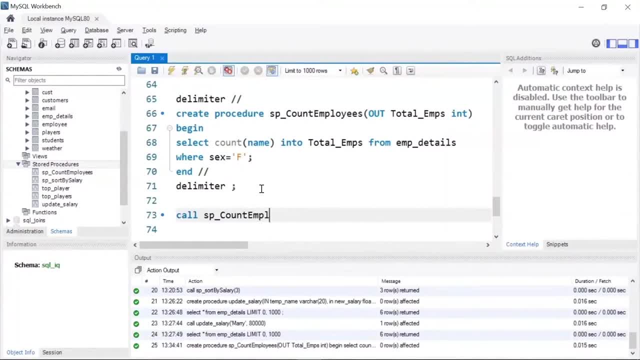 underscore sp underscore count employees within brackets. I will pass in the parameter as at the rate f underscore emp. I will give a semi colon, then I will write: select at the rate f underscore emp as female employees. okay, so as is an alias name. let's run this one by one. first I will 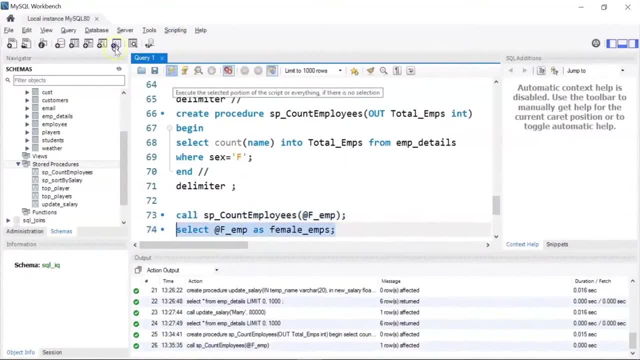 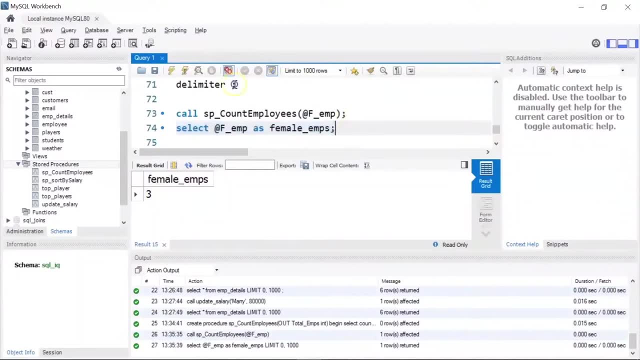 call my procedure and then we will display the total number of female employees. you can see in our table we have three female employees. alright, now, with this understanding, let's move on to our next topic in this tutorial on advanced SQL. now we are going to learn about triggers. 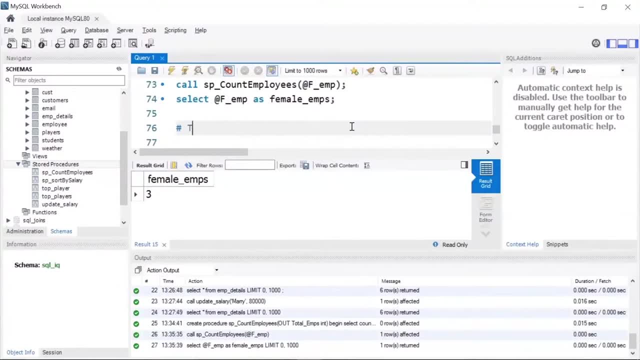 in SQL. so I will give a comment here. triggers in SQL. so first let's understand what is a trigger. so a trigger is a special type of stored procedure that runs automatically when an event occurs in the database server. there are mainly three types of triggers in SQL. we have: 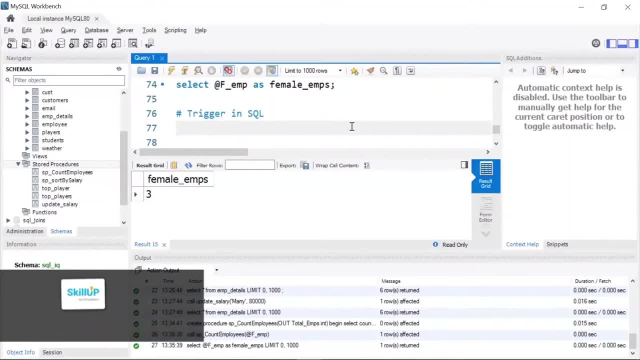 the data manipulation trigger. we have the data definition trigger and logon triggers. in this example, we will learn how to use a before insert trigger. so we will create a simple students table that will have the students role number, the age, the name and the students marks. so before inserting the 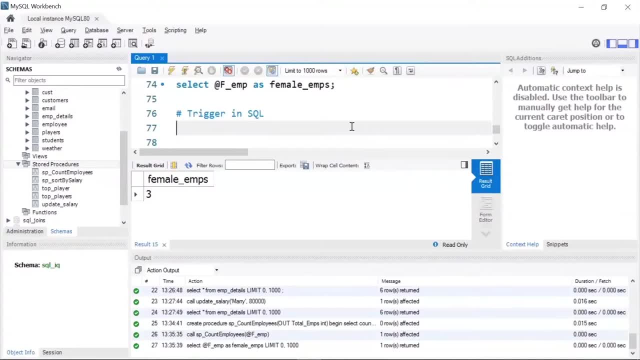 records to our table. we will check if the marks are less than zero. so, in case the marks are less than zero, our trigger will automatically set the marks to a random value, let's say 50. so let's go ahead and create our table. that is students. 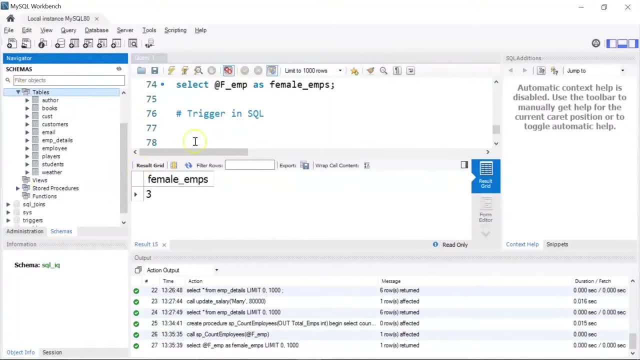 alright, so I will write: create table table- student. now this table will have the student role number. the data type is integer. it will have the age of the students. again, the data type is integer. we have the names of the students, so the third column would be name. 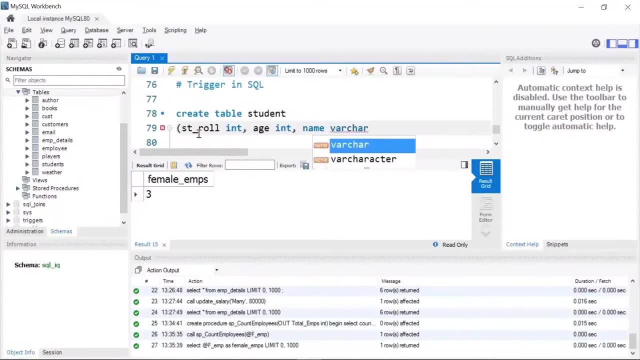 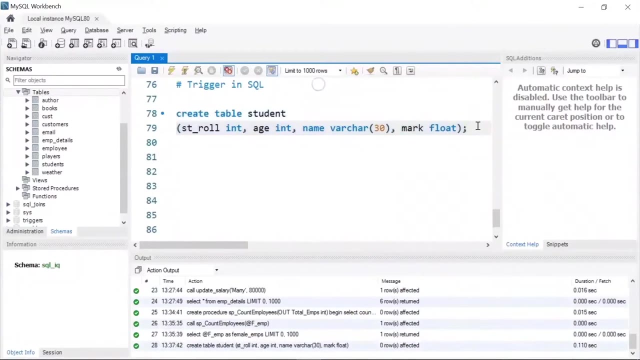 the data type would be variable or varying character size. I am giving it as 30. finally, we have the marks as floating type. so let's create this table, which is student. so we have created our table. now I will write my trigger command. so trigger command will start with delimiter, like 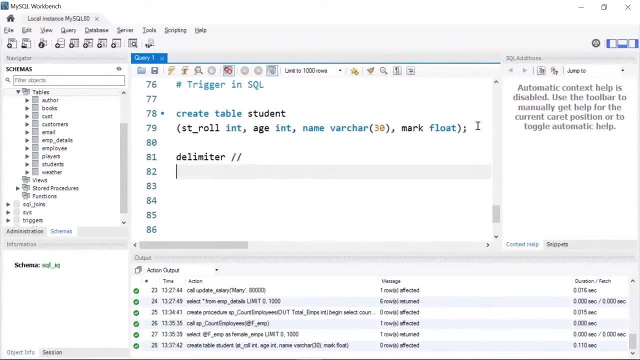 how our usual stored procedures have. next, this time I will write create trigger. then you need to give the name of the trigger. that is mark underscore. let's say verify. I am going to use a before insert trigger, so I will write before insert on my table name. that is student. 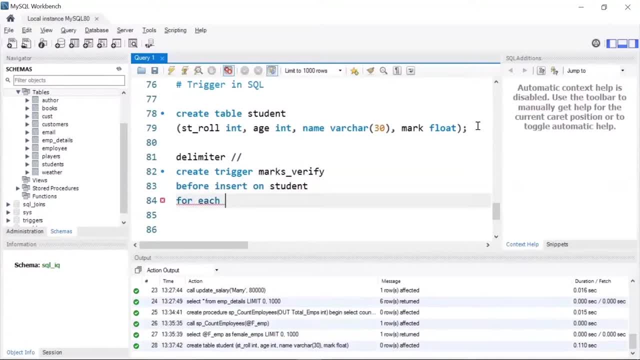 next I will write for each row. if new dot marks is less than 0, then we will set new dot marks equal to 50. so this is my condition. first we will check before inserting. if any student has marks less than 0, we will assign a value 50 to that. 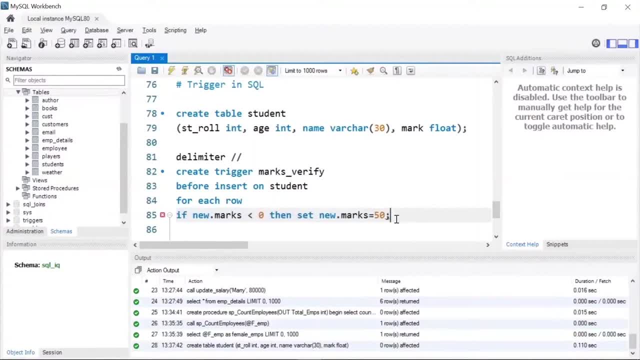 student, because usually the marks are not less than 0 in any exam. I will write end if semicolon and I will close the delimiter. so this is my trigger command. I will run it. it says trigger already exists. in this case we need to update the trigger name. let's say: 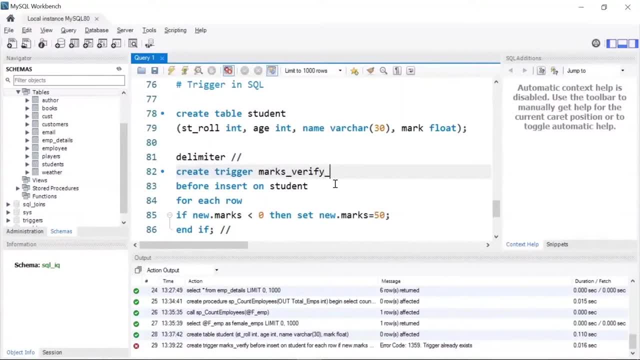 I will write marks underscore. verify underscore. student for st. let's run it again. ok, there is an error here because in our table the column name is mark and not marks, so here we need to change it as mark instead of marks. alright, let's run it. ok, so we have. 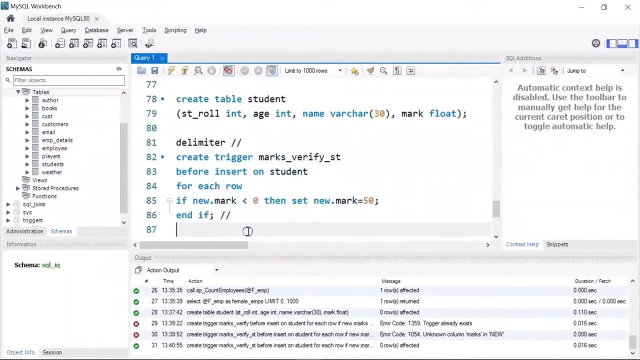 created our trigger. now let me insert a few records to the student table. so I will write: insert into student. I will write values. I will give the values as 501, which is the student role number. the age is, let's say, 10. the name is- it's a Ruth. 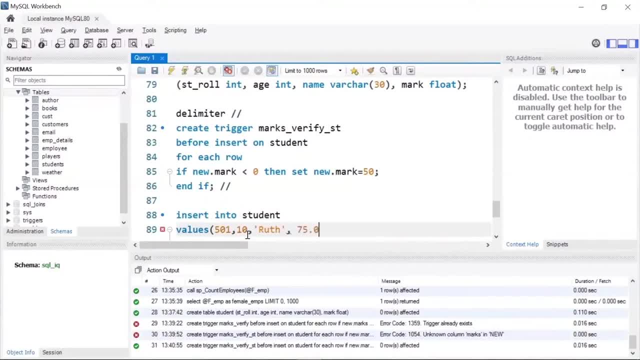 and the marks is, let's say, 75.0. give a comma. we will insert our second student record. student role number is 502, age is 12, the name is, let's say, Mike, and this time I am purposely giving a value of minus 20.5. 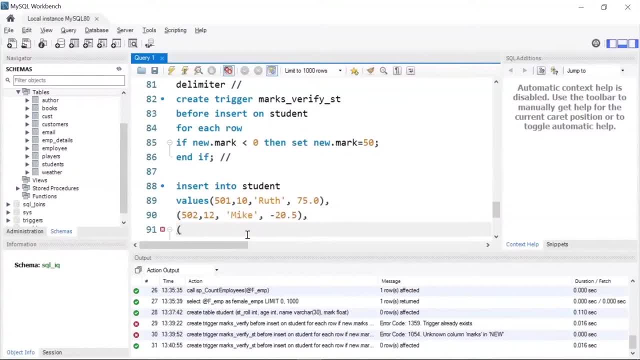 give another comma. we will insert the third record for student role number 503. age is 13, the name is Dave and let's say the marks obtained by Dave is 90. now we will insert our final record for student number 504. the age is 10. 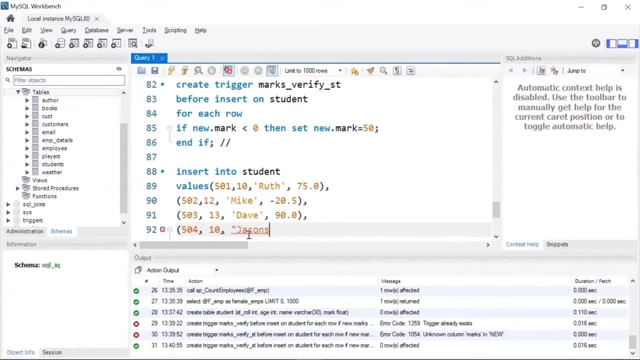 name, I will enter as Jacobs, and this time again I am purposely giving the marks in negative. 12 point, let's say 5. close the bracket, give a semicolon and I will run my insert statement. okay, so we have inserted four rows of information to our student table. 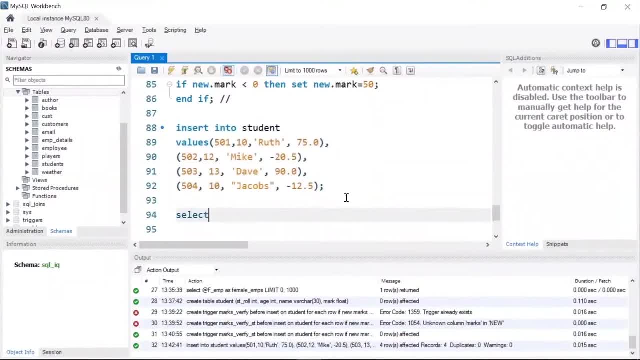 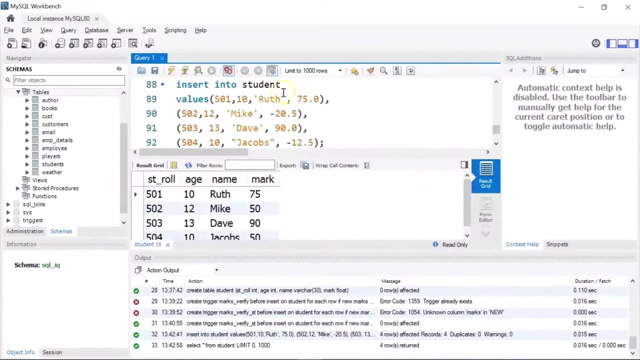 now let me run the select query. I will write select star from student. if I run this, you see the difference. there you go. so originally we had inserted: for 502, the marks was minus 20.5 and for 504, for Jacobs, the marks was minus 12.5. 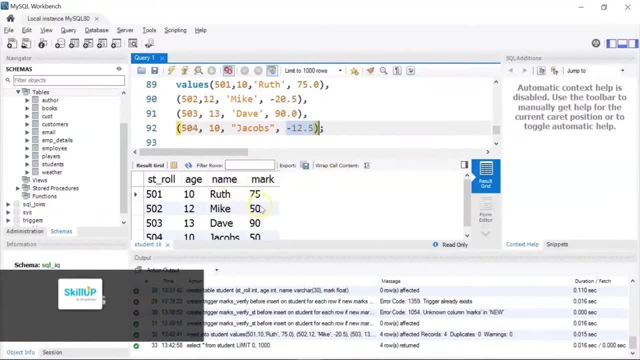 our trigger automatically converted the negative marks to 50 because when we created our trigger, we had set our marks to 50 in case the marks were less than 0. so this is how a trigger works. now you can also drop a trigger or delete a trigger. you can just write drop. 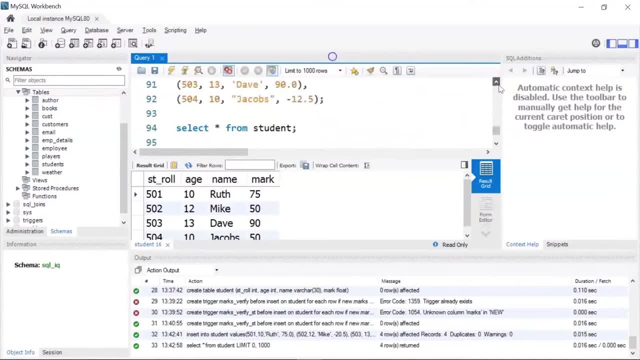 trigger followed by the trigger name. in this case, our trigger name is marks- underscore virik phi. underscore st. I will just paste this here and if you run this, it will automatically delete your trigger. I will give this as a comment. okay, now moving on. now we are going to learn. 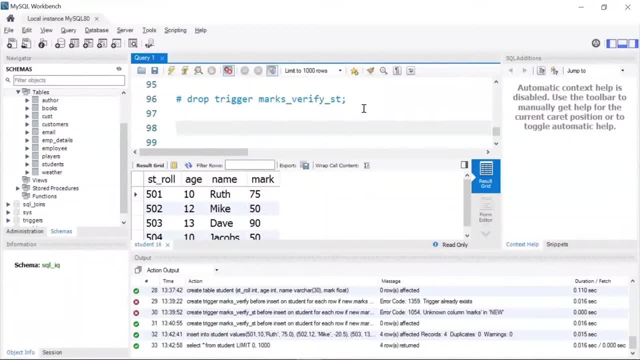 about another crucial concept in SQL, which is very widely used. this is known as views. so views are actually virtual tables that do not store any data of their own, but display data stored in other tables. views are created by joining one or more tables. I will get a comment as views. 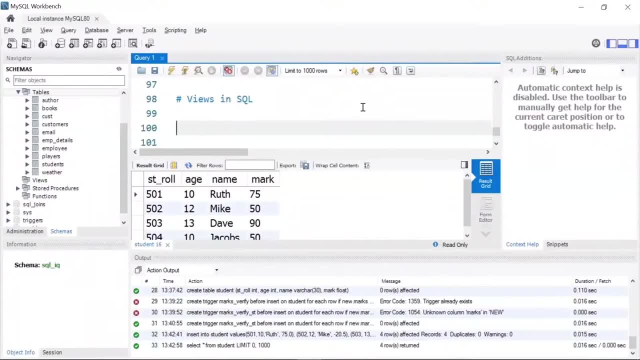 in SQL. okay, now to learn views, I am going to use my table, which is present inside classic models database. now, this database, as I mentioned, we had downloaded it from the internet. so first of all let me write: use classic models. so I will switch my database first. 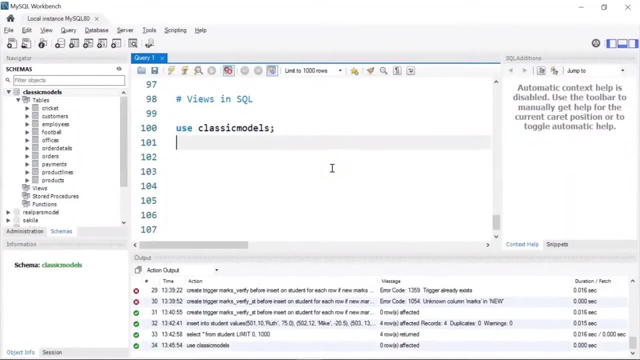 alright, now we are inside classic models, so here let me show you one of the tables which is called customers. so I will write select star from customers. okay, I missed s here, let's run it again. so this is my customer table, which is present inside classic models database. 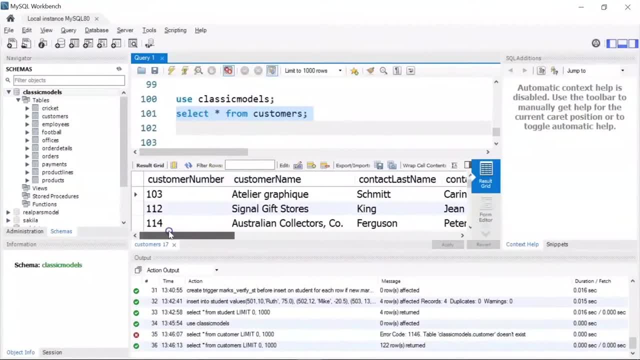 it has the contact last name, the contact first name, the customer name, customer number. we have the address, date, country and other information. now I will write a basic view command using this customer table. the way to write is: I will write create view, followed by the view name. 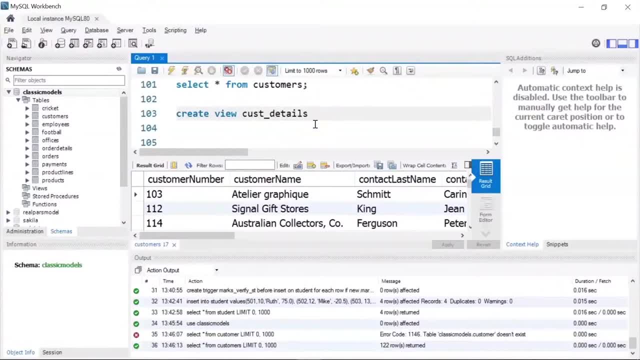 which is cust details. then you write as select. I am going to select a few column names from my original customer table, which is this one. so I need the customer name. let's say I need the phone number and the city. so you have this information here. you have the phone number. 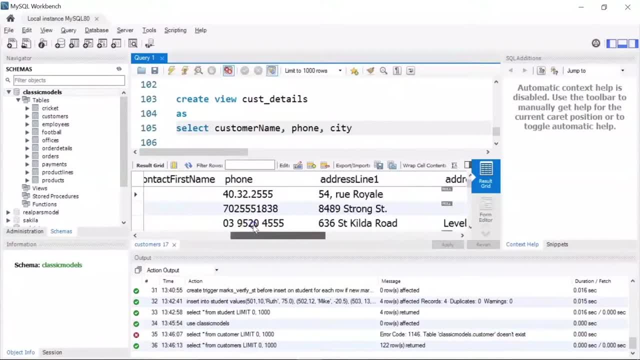 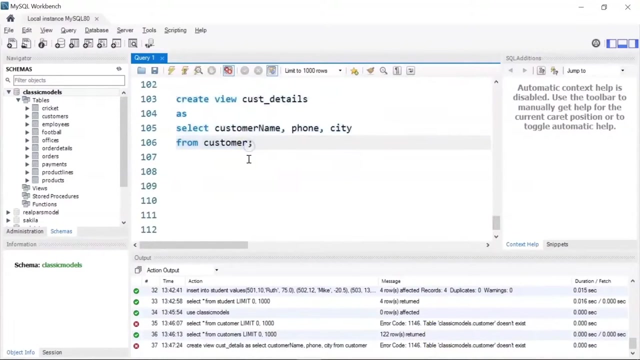 and the city. alright, I will write from my table that is customers. if I run this, my view, that is, cust details will be created. let's run it. there is some error here because the name of the table is customers and not customer. I will give an s. 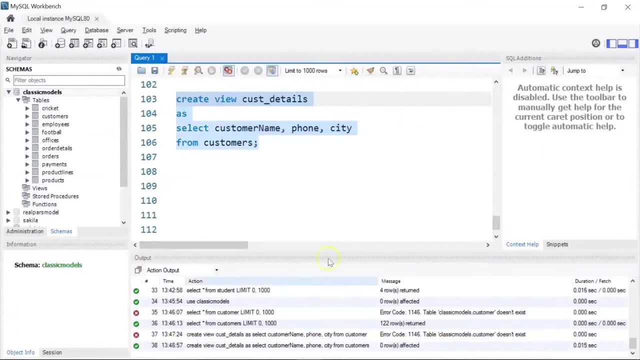 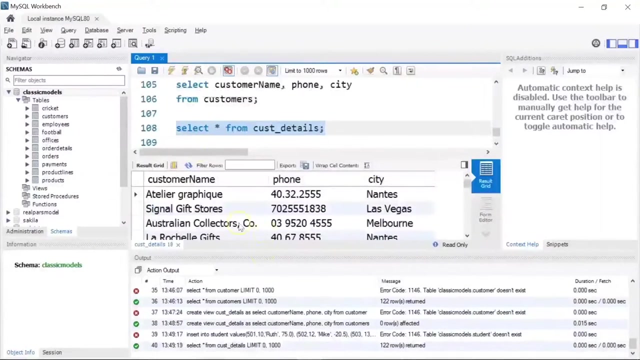 and I will run it again. alright, so you can see, we have created our view and to display the contents that are present inside our view, I can write select star form followed by the view name, that is, cust details. let's run it. there you go. so we have. 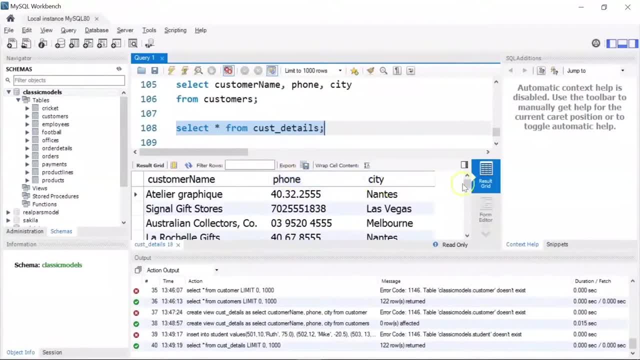 the customer name, the phone number and the city of the different customers that we have in our table. alright, now let's learn how you can create views using joins. so we will join two different tables and create a view. so for that I am going to use my products. 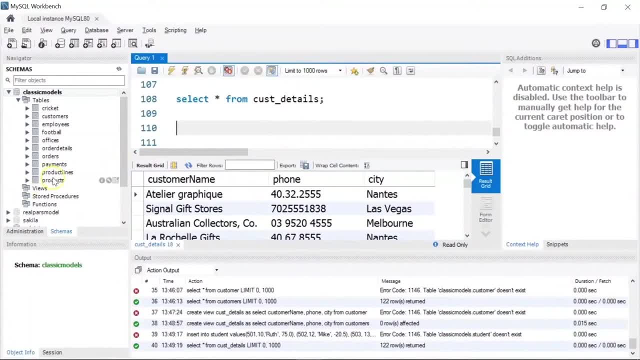 table and the products lines table. I am talking about the products table and the product lines table present inside classic models database. so before I start, let me display play the records that are present inside the products table. let's run it. so these are the different products you can see here. 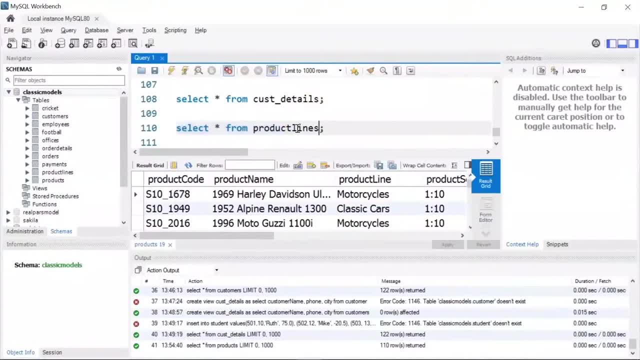 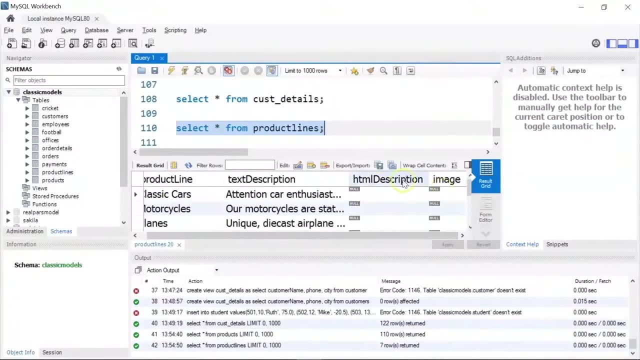 now let's see what we have in product lines table. so we have the product line, the text description and there is some html description and image. so I will create a view by joining these two tables and will fetch specific records that are present in both the tables. 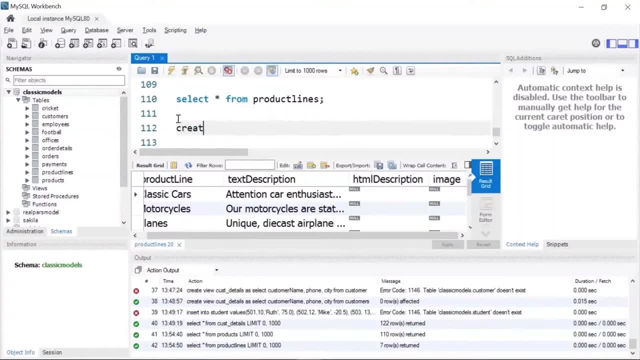 so let me first start by writing create view followed by the view name, that is, product underscore description. as I will write select product name comma, then I will write quantity and in stock. I also want the msrp. now these three columns are present inside the products table. 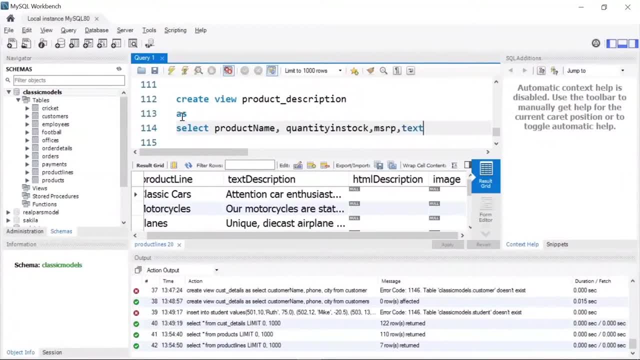 and next from the product lines table. I want the text description of the products, so I will write: from products table. I will give an alias as p, followed by my other table, that is product lines, as let's say pl on the common column. that is product line. 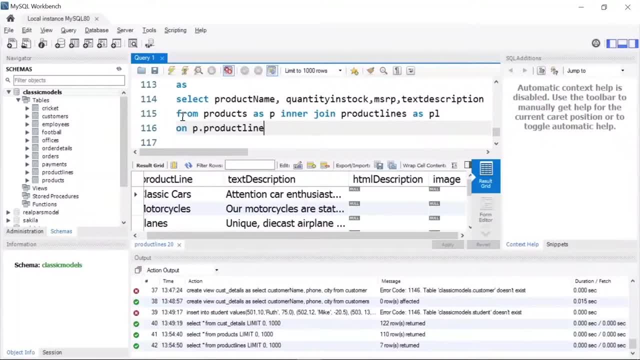 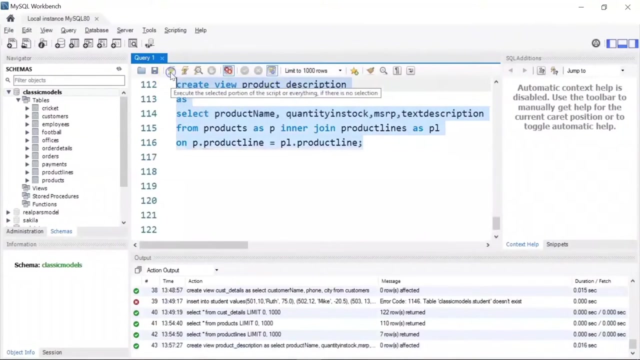 so p dot product line is equal to- I will give a space- pl dot product line. ok, so here we have used specific columns from both the tables and our view name is product underscore description. let us run it alright. so we have our view ready. now let me. 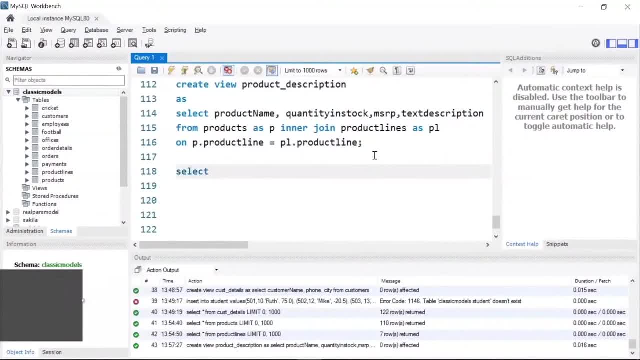 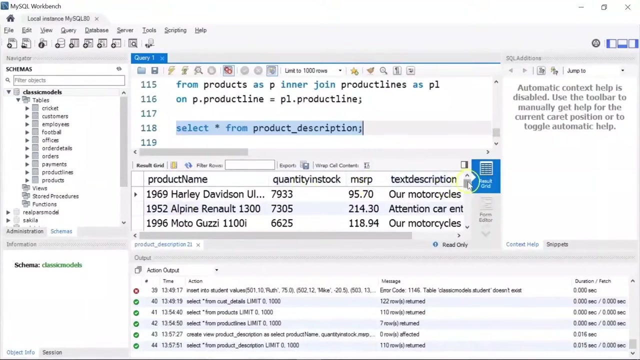 view or display what is present inside our product underscore description view. I will select star from product underscore description. let's run it. there you go. so we have the product name, the quantity in stock, msrp and textual descriptions of the different products in the table. ok, now there are a few other. 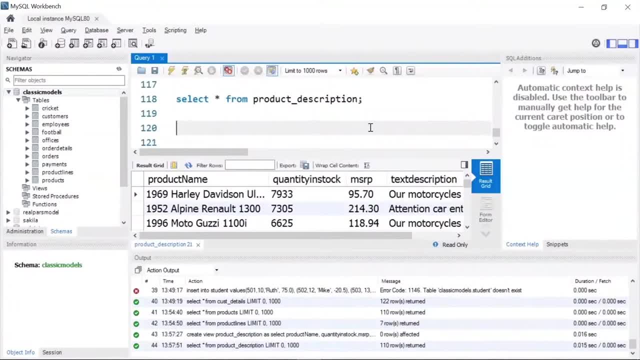 operations that you can perform. let's say, you want to rename a view instead of product underscore description. you want to give some other name, so I will just give a comment: rename description. so to rename a description, you can use the rename statement. I will write rename. 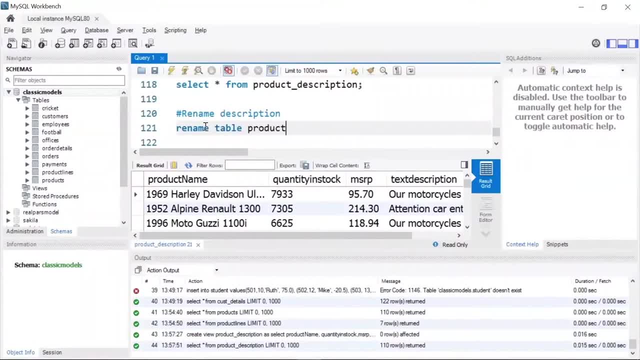 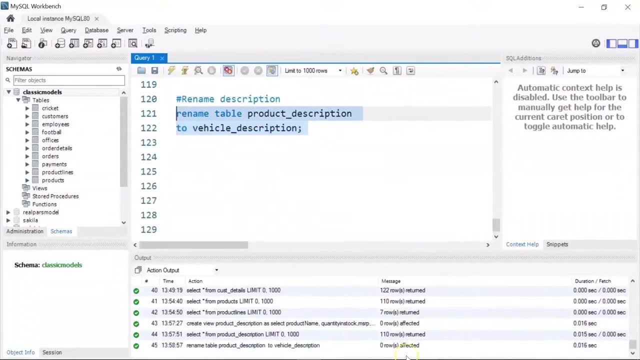 table: product underscore: description, which is my old name. I want to change this name to, let's say, I will give vehicle description, since all our products are related to some of the other vehicle, so I will write vehicle description. ok, let us run it alright. so here you can. 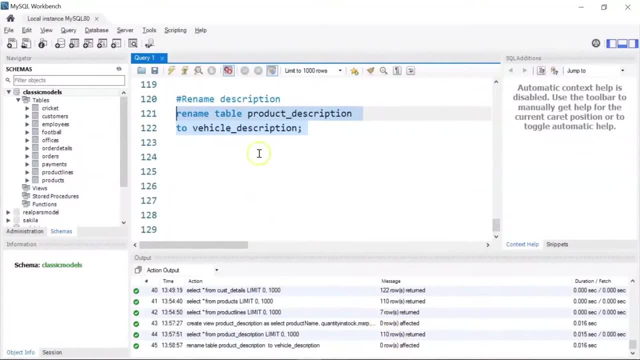 see, I have renamed my view, so here, if I just refresh it- and I will expand this- you can see we have the cars details view and we have the vehicle underscore description view. ok, now either you can view all the views from this panel or you can use a command. let's say: 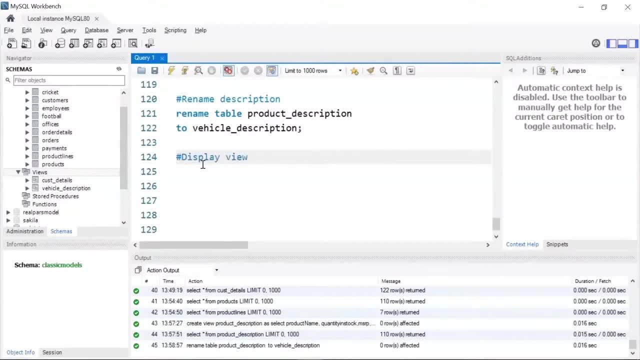 I will write display views is the comment now to show all the views you can use. show full tables. where table underscore type is equal to within single quote, I will write view. so this is the command that will display all the views that are present inside a database. 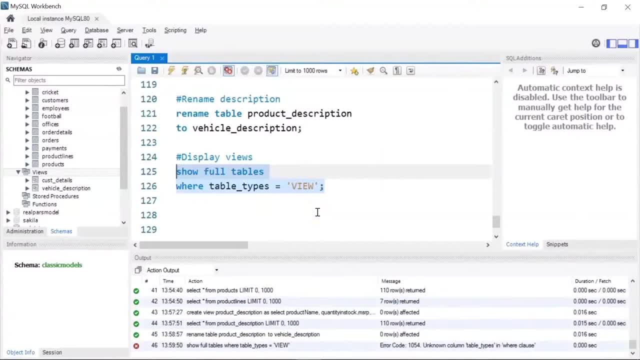 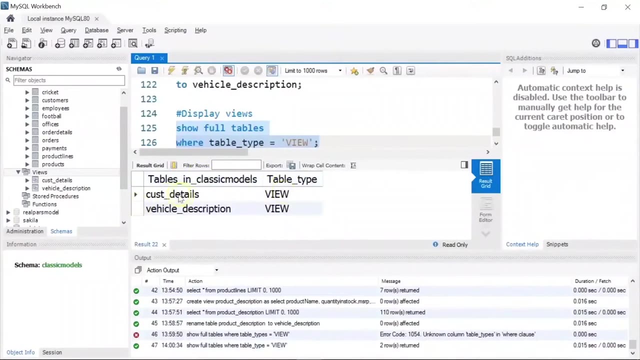 there is some error here. let's debug the error. this should be ok. so instead of table types, it should be table type equal to view. let's run it. you can see the two different views that we have. one is customer details, another is vehicle underscore description. ok, now you can also. 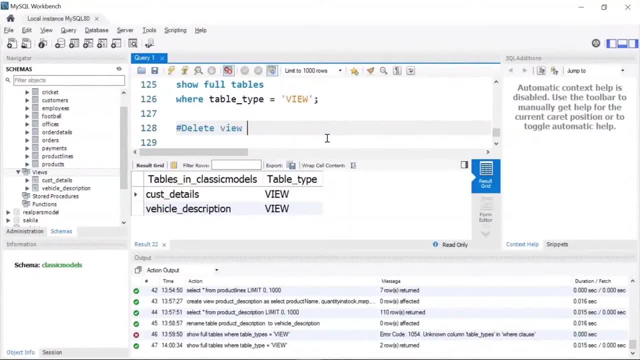 go ahead and delete a view. for that you can use the drop command. so I will write drop view followed by the view name. let's say I want to delete customer underscore details or cust underscore details view. I will write drop view- cust underscore details. let's run it. 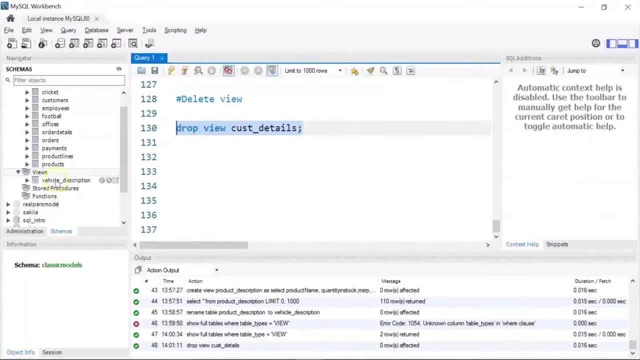 you can see here we don't have the cust underscore details view anymore. alright, now moving to our final section in this demo. here we will learn about windows functions. now windows functions were incorporated in mysql in the 8.0 version, so windows function in mysql are useful applications in solving. 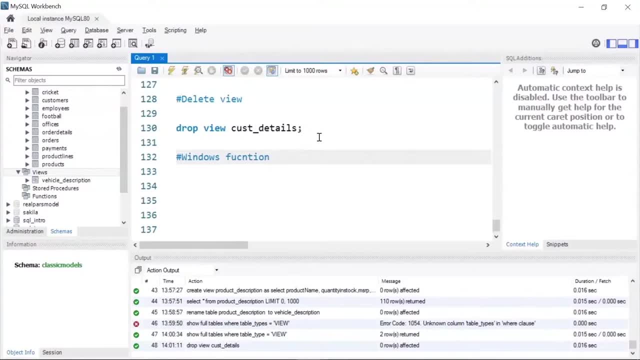 analytical problems using the employees table present inside my sql underscore intro database. so we will find the total combined salary of the employees for each department. so first let me switch my database to sql underscore intro database. I will run it. ok, I will display my table. that is employee. 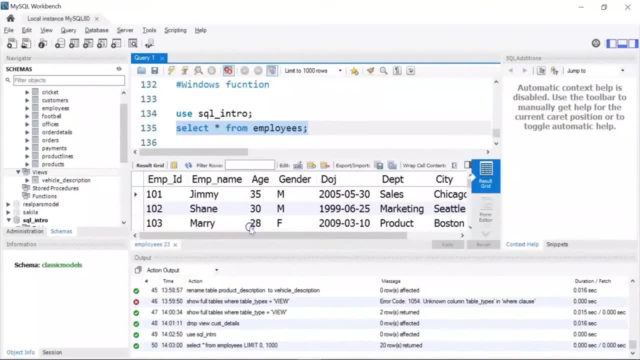 so here we have 20 employees in our table. using this table, we are going to find the combined salary of the employees for each department. so we will partition our table by department and print the total salary. and this we are going to do using some windows functions in mysql. 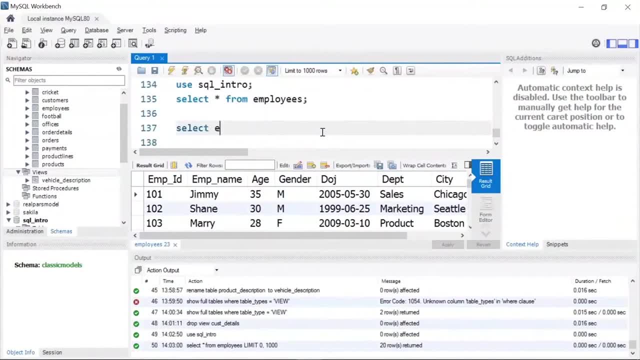 so I will write select. I want the employee name, the age of the employee and the department of the employee. comma. next I will write the sum of salary over. I want to partition it by department. so I will write partition by department which is dept and I will give an alias. 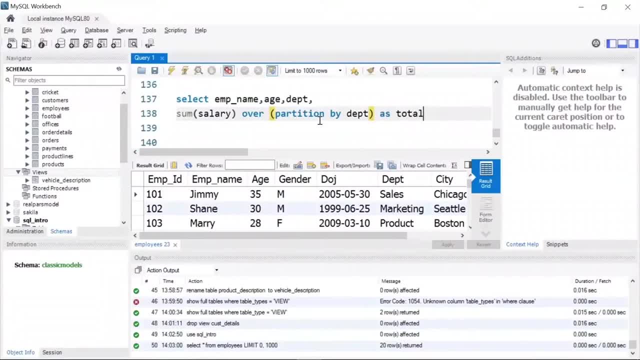 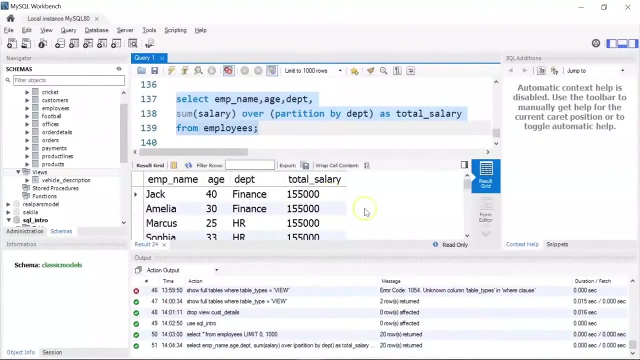 as total salary, so that it will create a new column with the name total salary from my table, that is, employees. the output will be a little different this time. let's execute it and see the result. there you go. so here we have created another column in our result that is total salary. 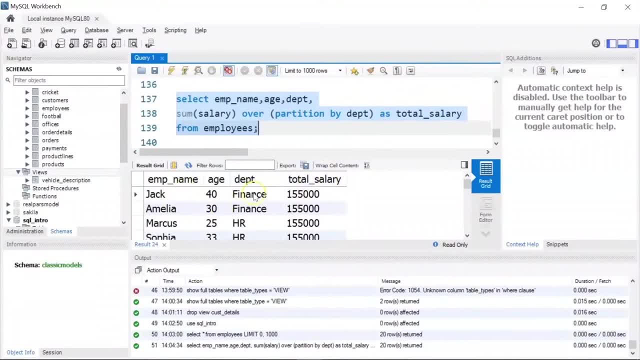 and for each of the employees and the respective departments, we have the highest salary. so in finance, the highest salary of one of the employees was $155,000. similarly, if I come down, we have the highest salary from HR. if I scroll further, we have the highest salary from IT. 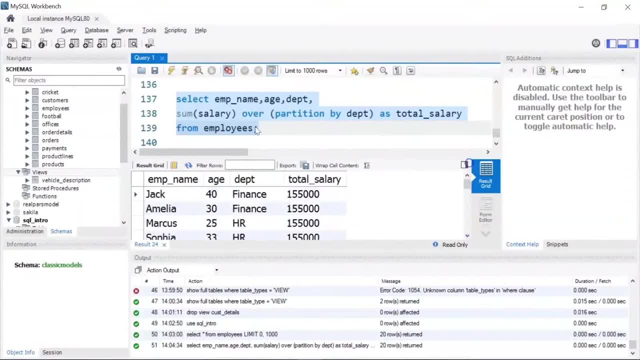 marketing, product sales and the tech team. alright, now we will explore a function which is called row number. now the row number function gives a sequential integer to every row within its partition. so let me show you how to use the row number function. I will write: select row. 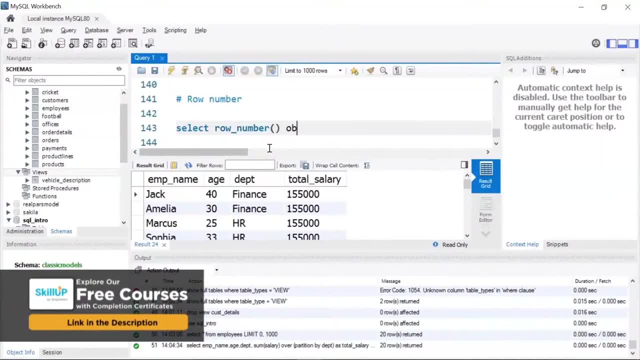 underscore number function over my column would be salary, so I will write order by salary. I will give the aliases row number, give a comma, and I want to display the employee name and the salary of the employee from my table, that is employees, and I will order by. 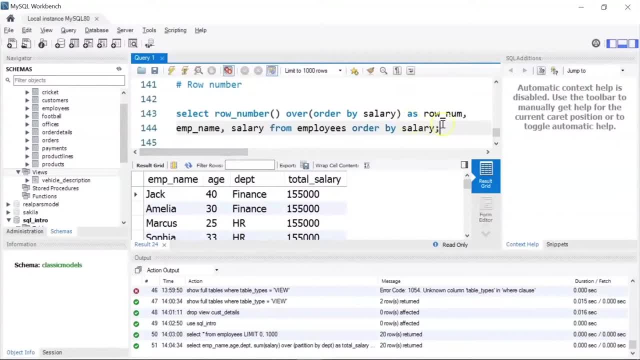 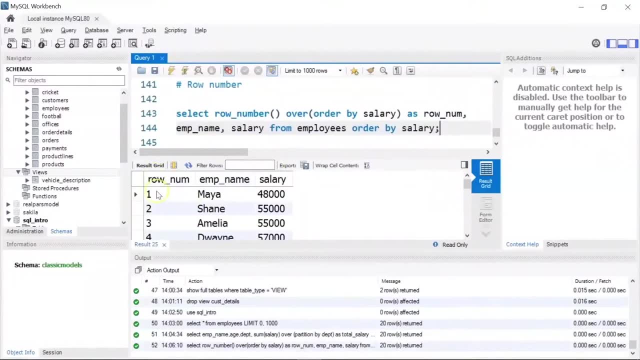 salary. so let's see how our row number function will create sequential integers. okay, you can see, here we have a row number column and we have successfully given row numbers to each of the records. you can see it starts from 1 and goes up till 20. 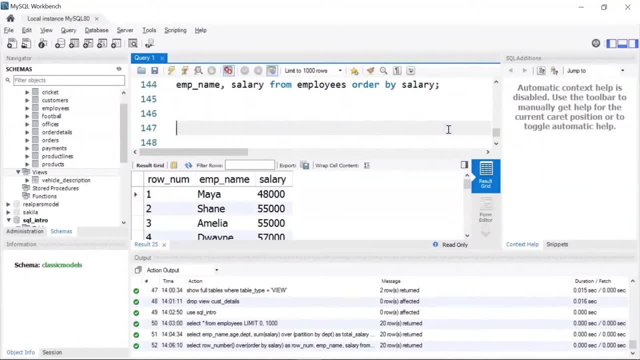 okay, now this row number function can be used to find duplicate values in a table. to show that first I will create a table, I will write create table. let's say I will give a random name, that is demo. and let's say we have in this table the. 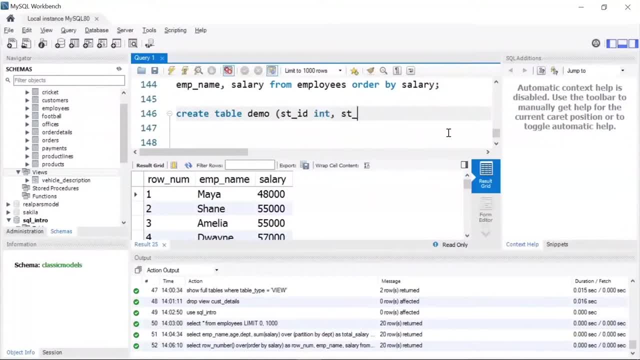 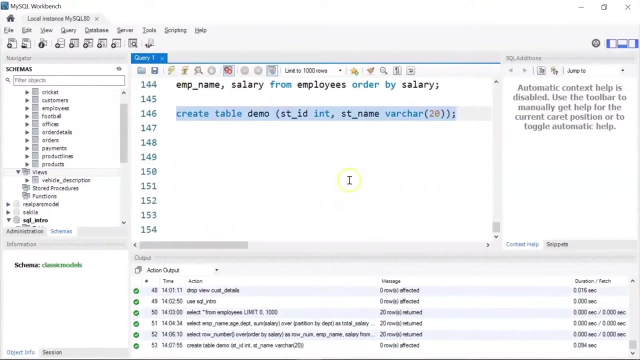 student id, which is of type integer, and we have the student name, which is of type varchar. the size is 20. I will create the small table with a few records. let's create this table first. now we are going to insert a few records to our demo table, so I will 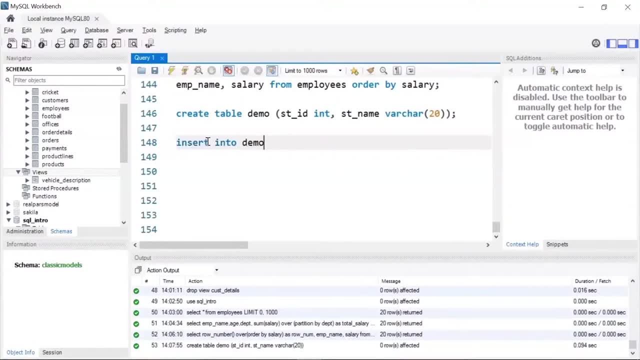 write: insert into demo values. I will give 101. the name is Shane. give a comma. I will insert the second student name, 102, the name is Bradley. give a comma this time for 103. we have two records. let's say the name of the student is Herath. 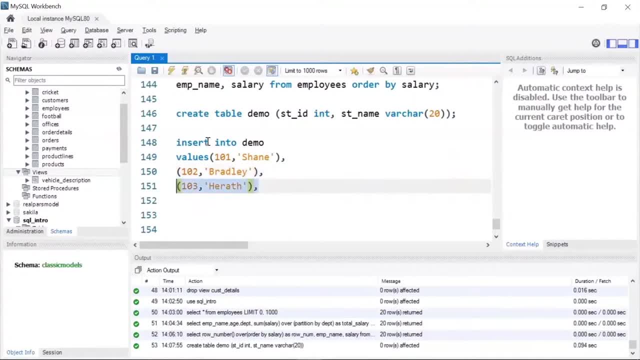 give a comma. I will copy this and will paste it again. so we have duplicated 103. next we have 104. the name of the student, let's say, is Nathan. then again, let's say, for the fifth student, which is Kevin. we have two records. I will copy this. 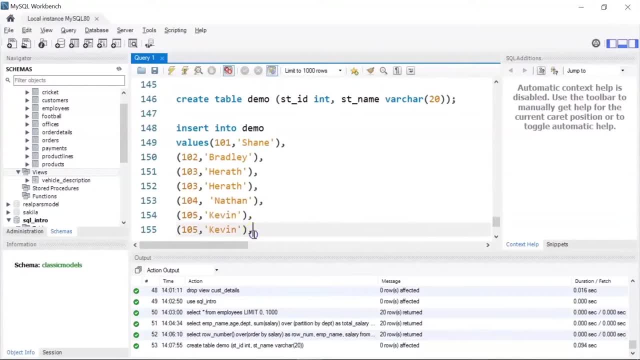 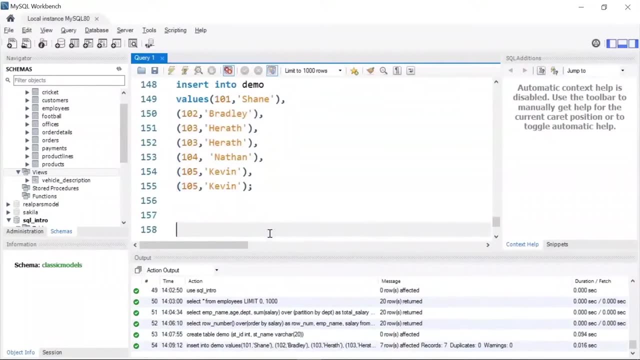 and I will paste it here. let me give a semicolon and we will insert these records to our table demo. alright, now let me just run this table for you. I will write select star from demo. if you see this, we have a few information that are duplicated in our table. 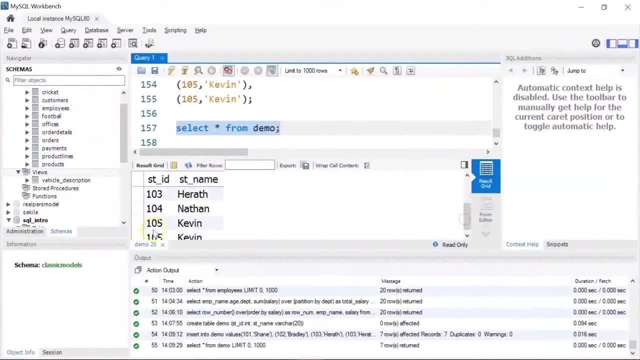 that is for student id 103 and student id 105. now I am going to use my row number function to find the duplicate records present in my table. I will write select student underscore id comma. student underscore name. I will give another comma and write row underscore number. 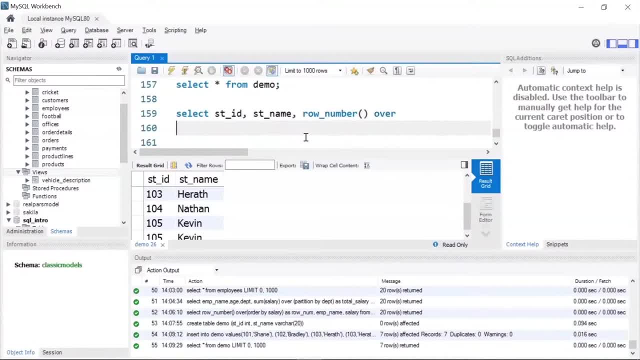 over within brackets. I will write partition by st underscore id, comma, st underscore name. ok, then I will write order by st underscore id. close the bracket. I will give an alias as ronum from my table. that is demo. let's just run it. you can see here, ok. 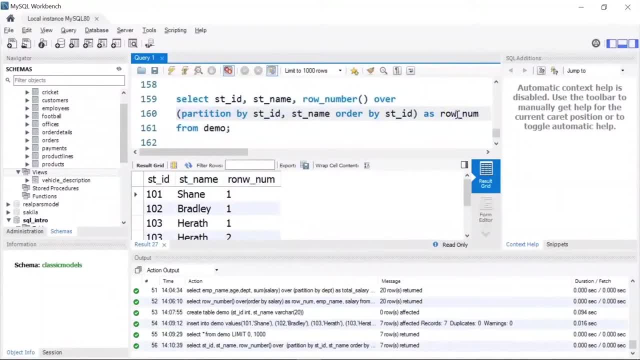 let me just delete n from here and do it again. alright, if you see, here there is just one student in the name shane. we have one student in the name bradley, but here, if you see, for herath, the second record, it says two, which means 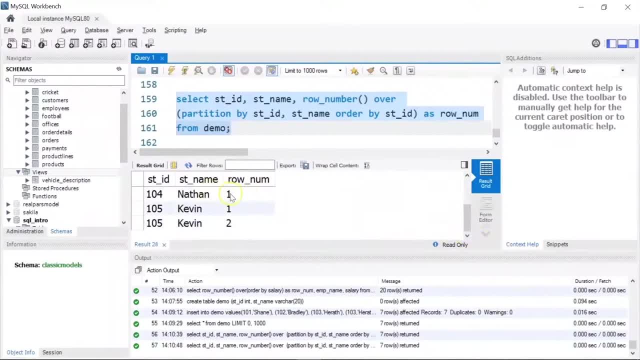 there are two records for herath and if I scroll down, there is one record for nathan and there are two records for kevin, which means kevin is also repeated. ok, now we are going to see another windows function that is called rank function in mysql. so the rank. 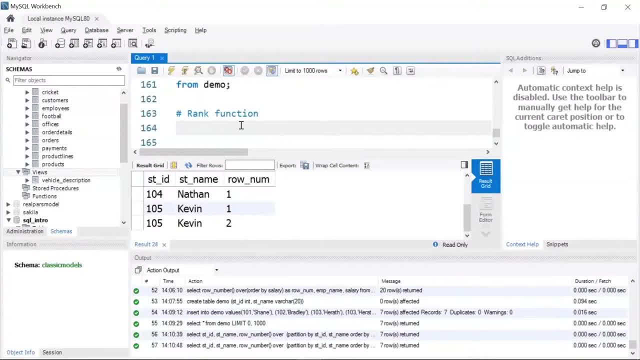 function assigns a rank to a particular column. now there are gaps in the sequence of rank values when two or more rows have the same rank. so first of all, let me create a table, and the name of the table would be a random name. we will give it as let's say: 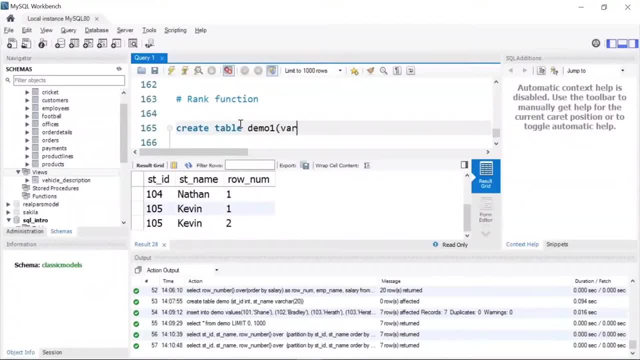 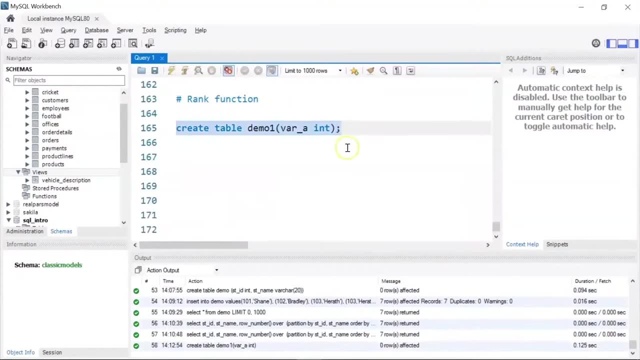 demo1 and it will have only one column, let's say variable a, of type integer. we will create this table first. ok, now let's go ahead and insert a few records to our table, which is demo1. so I will write value 101, 101, 102. 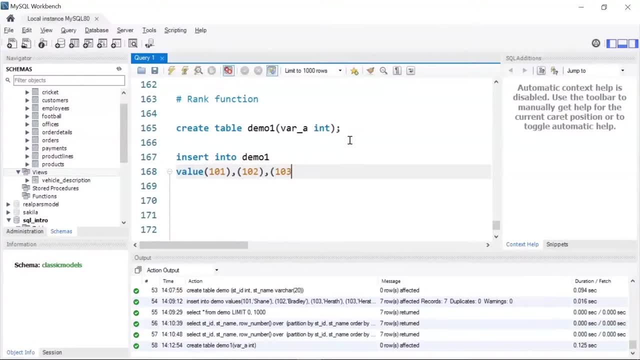 let's say 103 is repeated. I am doing this purposely so that in the output you can clearly distinguish what the rank function does. next we have 104, 105, we have 106 and let's say 106 is also repeated. finally, we have 107. 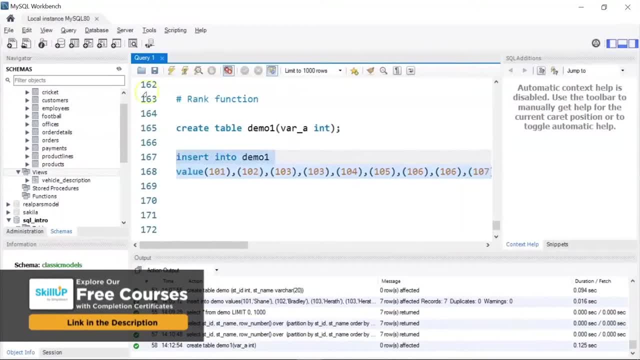 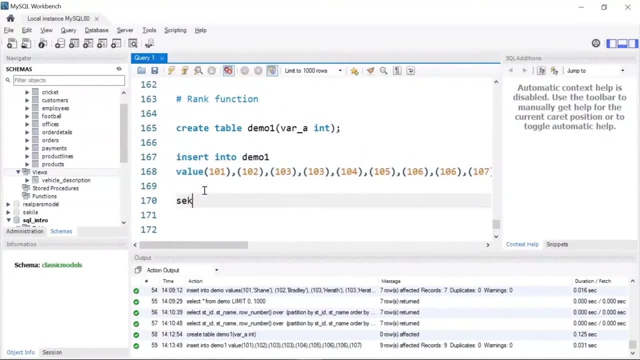 ok, let me insert these values to my table. that is demo1. ok, this is done. now if I write select var underscore a and use my rank function, I will write rank over. then I will order by my variable, that is var underscore a, as an alias name, let's say test rank. 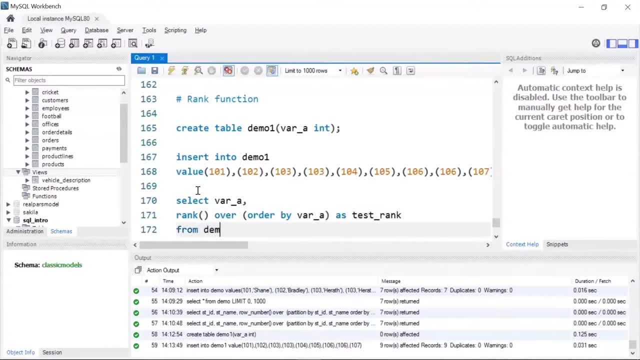 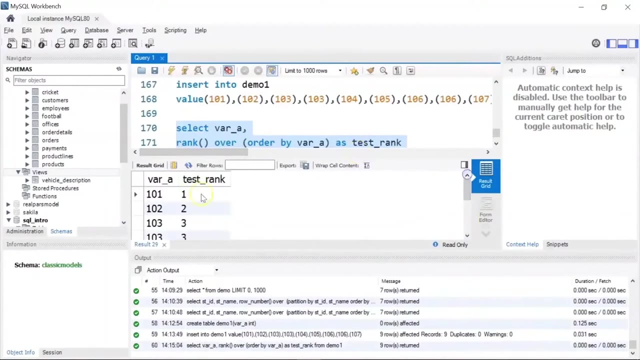 from my table, that is demo1. let me execute this and show you how the rank function works. now, if I run this there you go, so here. if you mark so for variable a101, the test rank is 1. for 102 the test rank is 2, but 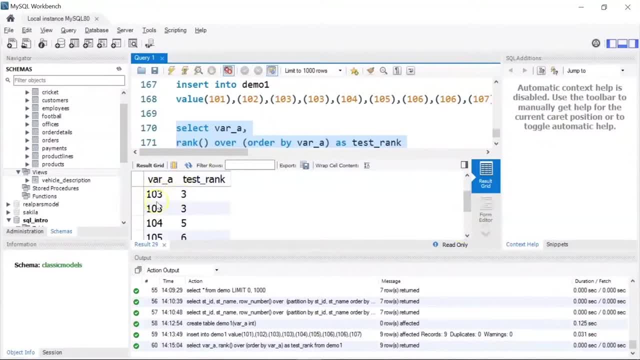 for this value, which is 103. the test rank is repeated because there was a repetition for 103, so we have skipped the rank 4 here for 104. the rank is 5, now for 105. the rank is 6, now for 106, again since 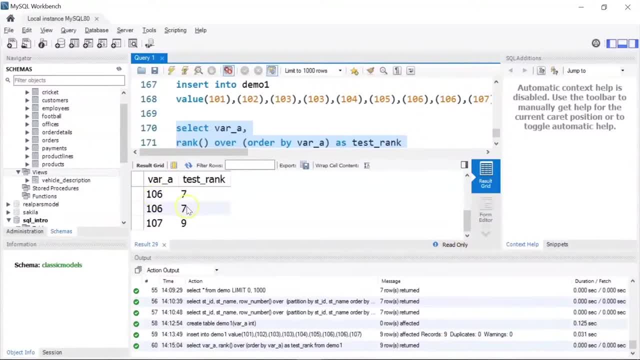 the record was repeated twice. we have skipped the 8th rank and our rank function assigned the same value, which is 7, for 106 and for the last value, 107, the rank is 9. alright, now moving ahead, we will see our final windows function, which is called: 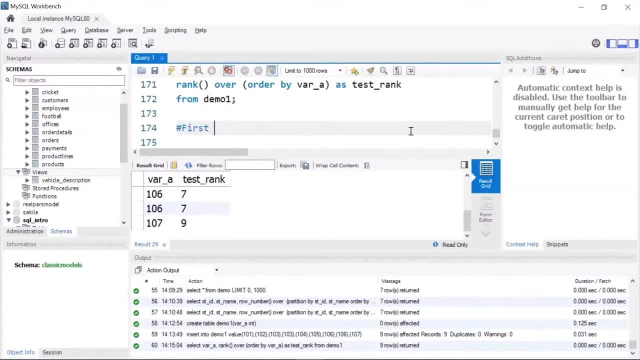 first value. so first value is another important function in mysql. so this function returns the value of the specified expression with respect to the first row in the window frame. alright, so what i am going to do is i am going to select the employee name, the age and salary. 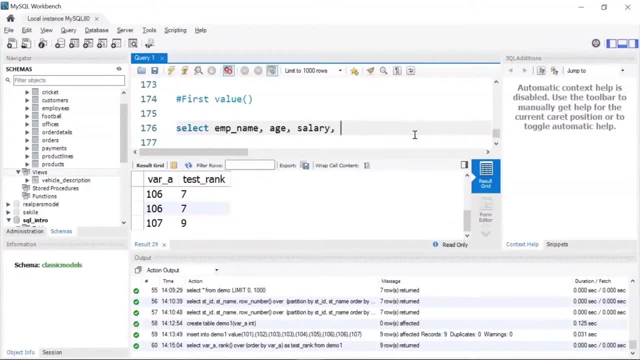 and i will write first underscore value, which is my function, and pass in my employee name and then i will write over order by order. by my column that is salary descending, i will give an alias as highest underscore salary from my table, that is employees. so let me run this and see how. 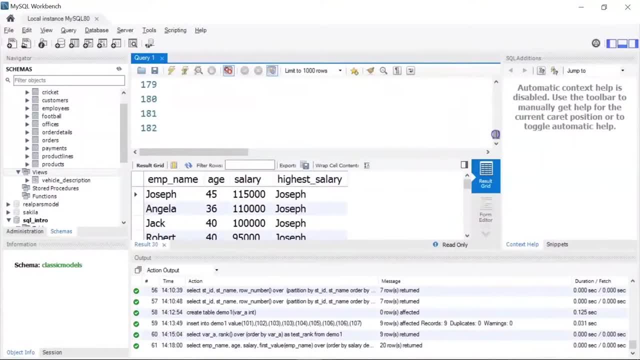 the first underscore value function works alright. so in our table joseph was the employee who had the highest salary, which was hundred and fifteen thousand dollars. so the first value function populated the same employee name throughout the table. you can see it here. now you can also use the first. 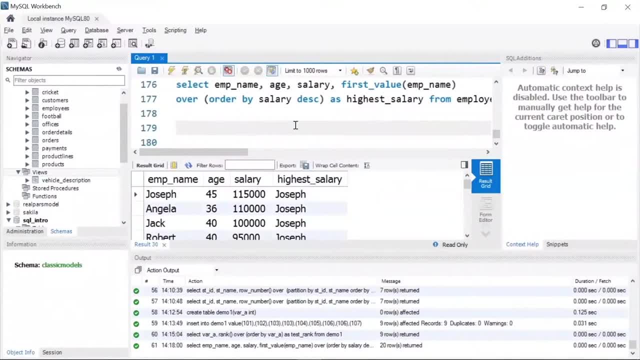 underscore value function over the partition. so let's say you want to display the employee name who has the highest salary in each department. so for that you can use the partition. i will write select emp underscore name comma. i want the department and the salary comma. i will use my function. that is first. 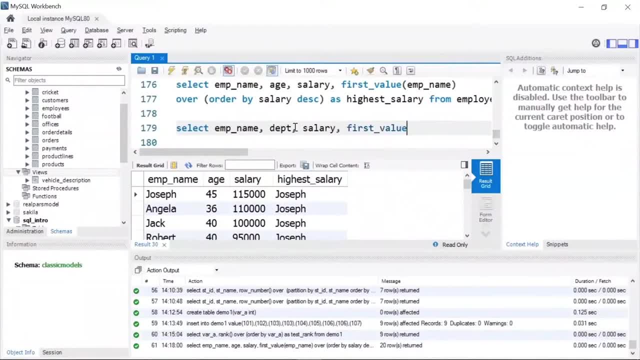 underscore value followed by the name of the employee inside my first value parameter. i will write over here. i am going to use partition. i am going to partition it by department, since i want to know the employee name who has the highest salary in each department, and i am going to 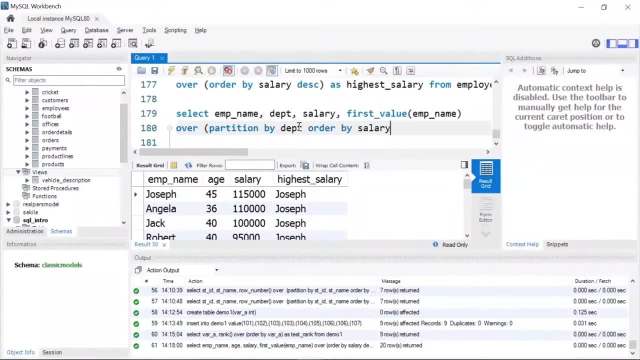 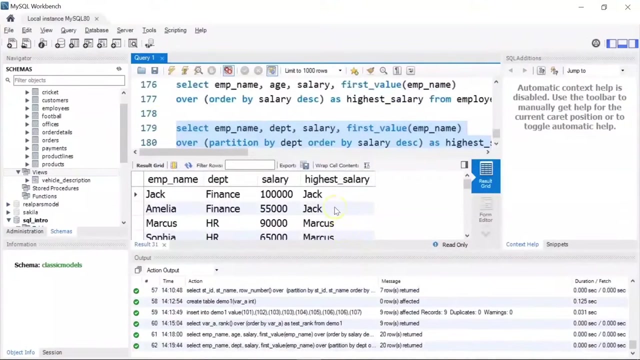 order by salary descending, and i will give my alias again as highest salary from my table, that is, employees. so let's run this and see the difference in the output. okay, so, as you can see, here we have the employee who had the highest salary from each department. 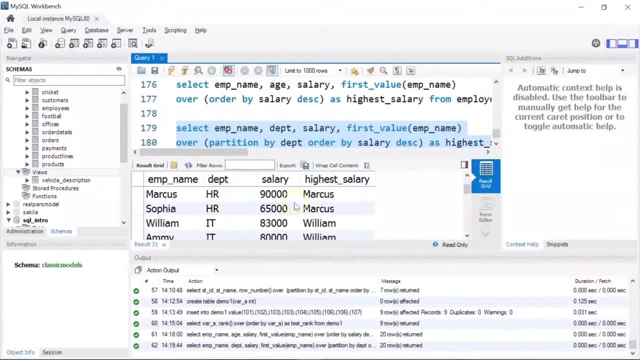 so for finance, jack had the highest salary. from hr it was marcus. similarly in it it was william. if i scroll down, for marketing, it was john. for product, it was alice who had the highest salary. similarly, in sales we had joseph, and in tech we had angela. 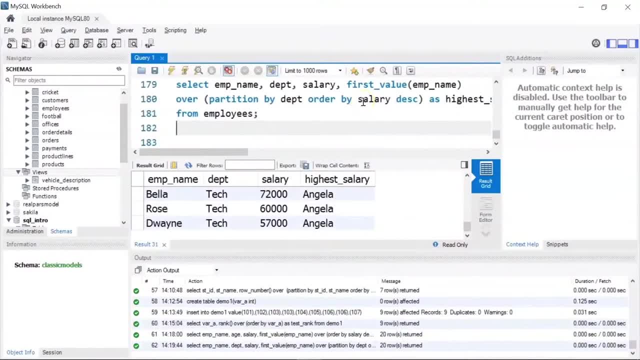 so this is how you can use the first underscore value function using partition. alright, so that brings us to the end of this demo session on our tutorial. so let me just scroll through and show you what we did from the beginning. first, we learnt about sub queries in sql. 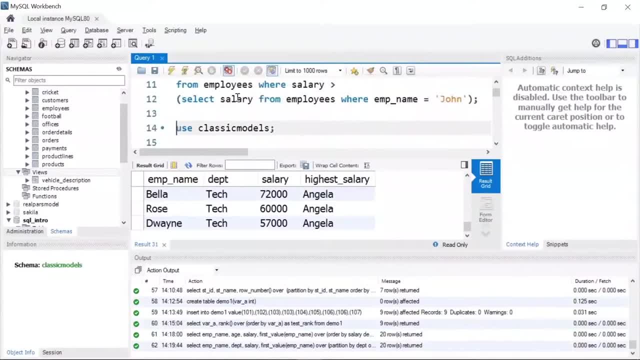 so we initially wrote a simple sub query and then we used our classic models database, which was downloaded from the internet. i had also shown you the link from where you can download this database here. we used two different tables and we performed a sub query operation. we learnt how to create. 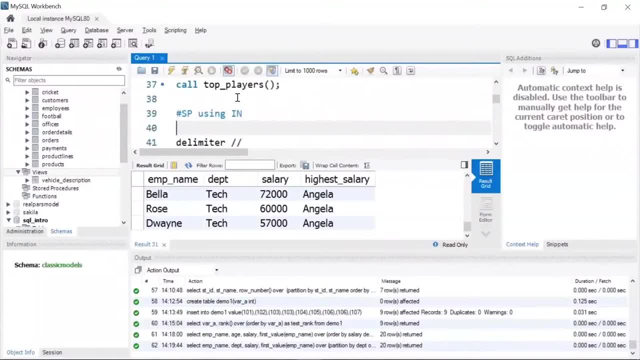 stored procedures. so we learnt how you can use the in operator or the in parameter as well as the out parameter in stored procedure. after stored procedure we learnt another crucial concept in sql, which is called triggers. now triggers are also special kind of stored procedures, so we saw how to. 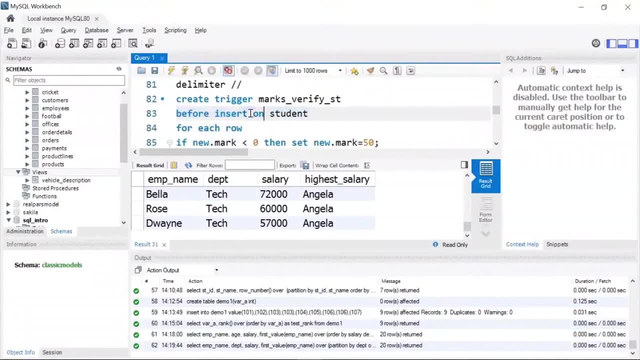 write a before insert trigger. you can see it here. next, we learnt how to delete a trigger. we also saw how to work with views in sql. so views are basically virtual tables that you can create from existing tables. we also saw how you can use views using two different tables and an. 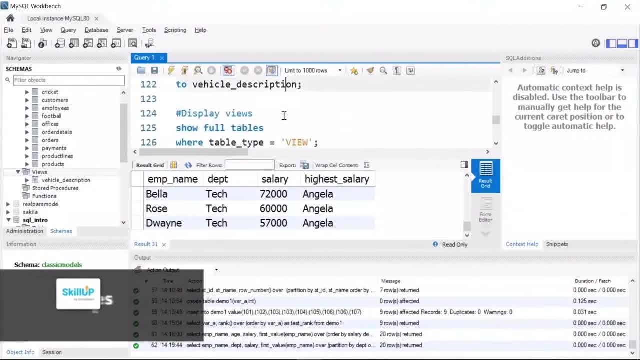 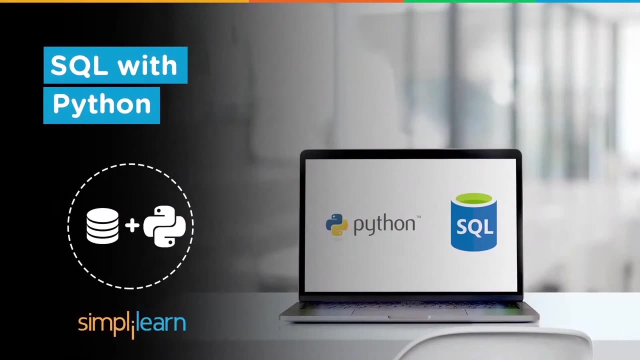 inner join and we learnt how to display views, how to rename view names, how to delete a view and, finally, we explored a few windows function. in this tutorial we will learn how to work with databases and tables using sql, with python. to do this demo, we will be using our jupyter notebook. 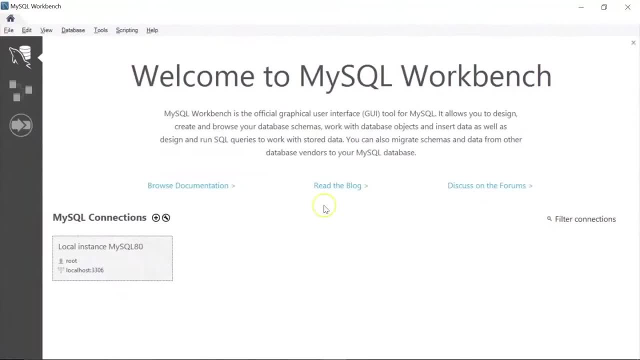 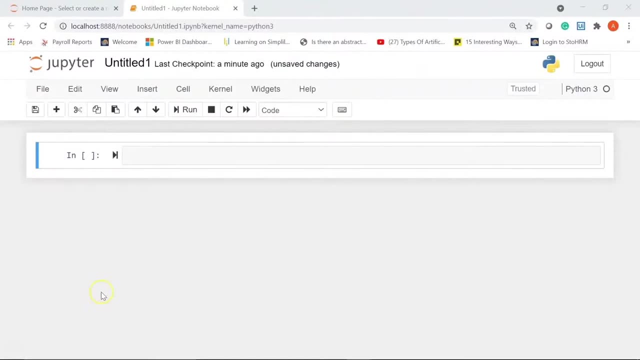 and the mysql workbench. you can see it here. so we will write our sql queries in the jupyter notebook with python like syntax. if you don't have mysql or jupyter notebook installed, please go ahead and install them first. while installing the mysql workbench, you will be asked to give the 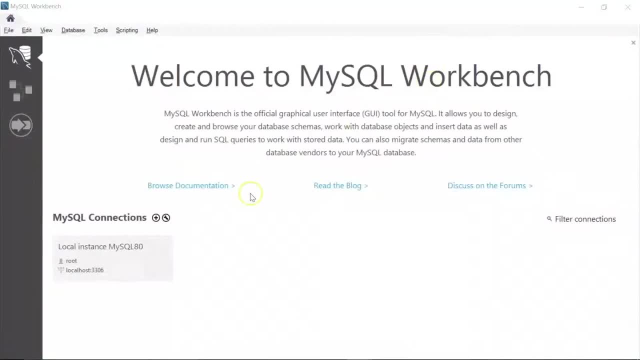 username and password. let me show you so. i am on my mysql workbench. so once you connect it will ask for the username and the password. so i have given my username as root and password you can give while installing it. we will be using the same user id. 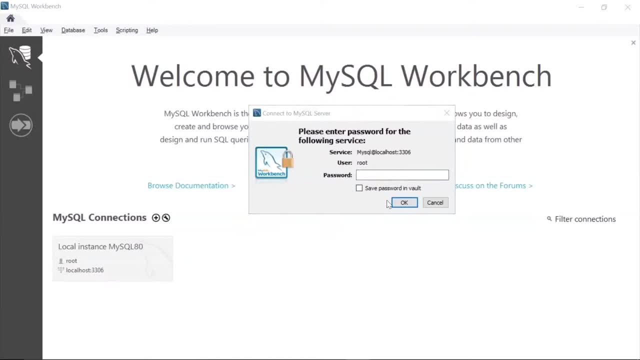 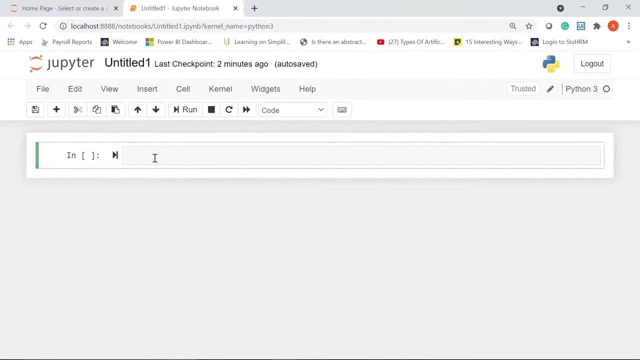 or the username and the password to make our connection. so let's get started with our hands on demonstration part. first and foremost, let me go ahead and import the necessary libraries. i will give a comment as libraries, alright. so first i will import mysql dot connector, next from: 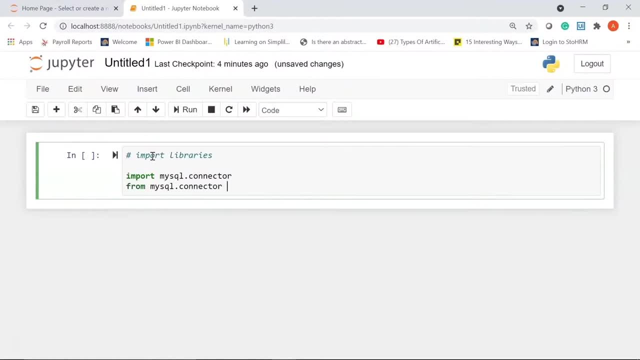 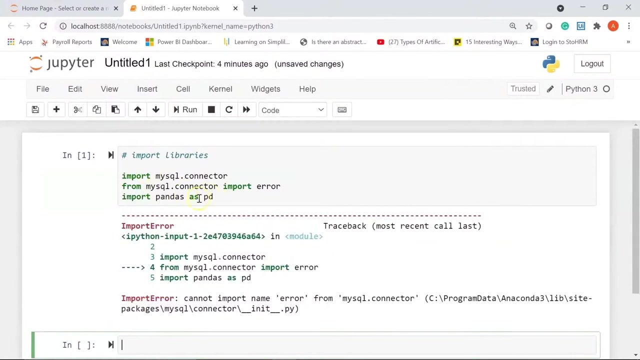 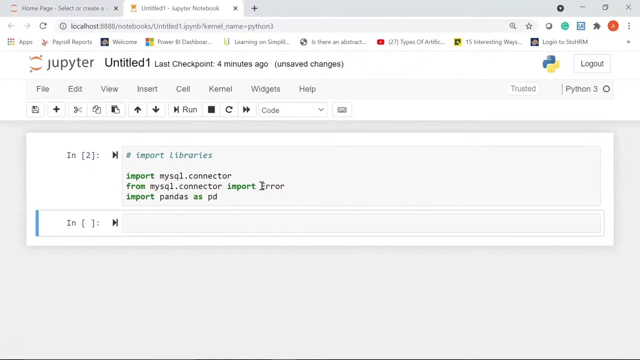 mysql dot connector. i am going to import my error method or the error module. next i want to import pandas as pd, so let's run this. ok, there is some error here. this should be capital e and not small e. alright, you can see, i have imported my important. 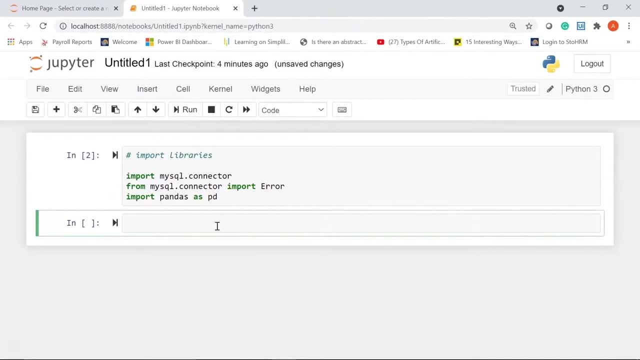 libraries. now i am going to create a function that will help us create a server connection. so i will write my user defined function by using the def keyword. i will write: create underscore server server underscore connection. this is going to be my function name and it will take in. 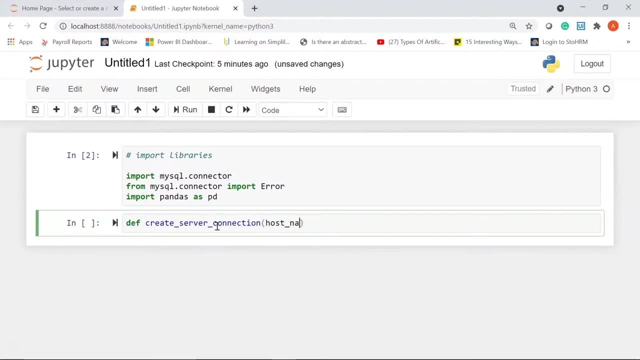 three parameters: first is the host name, next is the username and then we have the user password. alright, i will give a colon and then, in the next line, i am going to define a variable which is going to be connection, and i will assign it to a value called none. 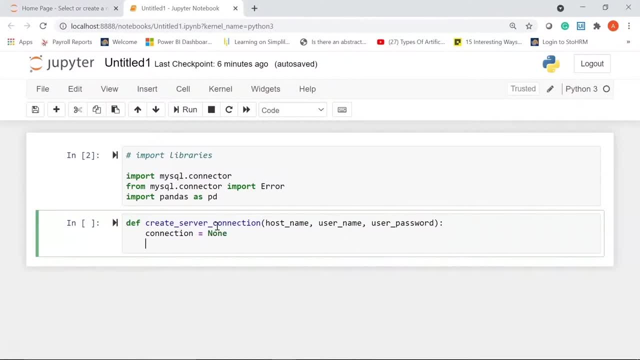 now we will be using exception handling techniques to connect to our mysql server. the try block lets you test a block of code for errors and the accept block will handle the errors. so i will write try and give a colon, and then i am going to reassign. 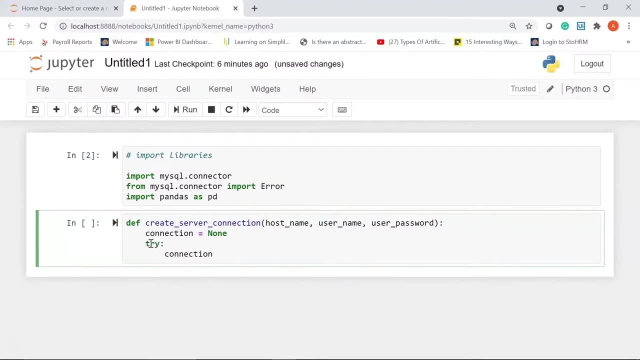 the connection variable to a method which is mysql dot connector dot connect. now this mysql connector dot connect method sets up a connection, so it establishes a session with mysql server. if no arguments are passed, it uses the already configured or default values. so here we are going to pass. 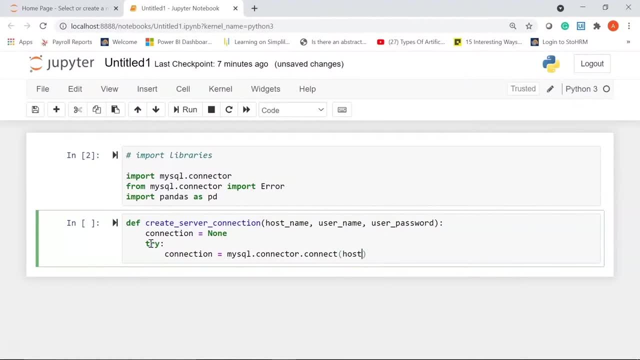 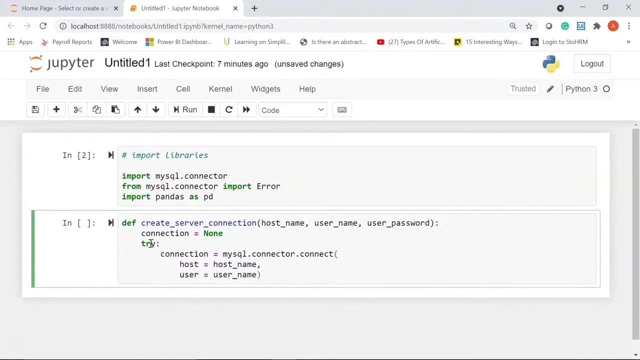 in three parameters. the first is the host name. i will write host equal to host name, which is host underscore name. i will give a comma. then i will write user, equal to user underscore name. next will be my password and i will assign the value: user underscore password. 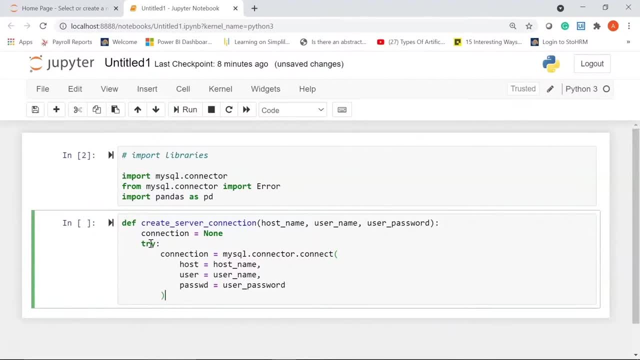 alright, now i am going to use a print statement and write mysql database connection successful. after this, i will give my accept block, so i will use the keyword accept here. i will write error as err, give a colon and then i am going to use the print statement. 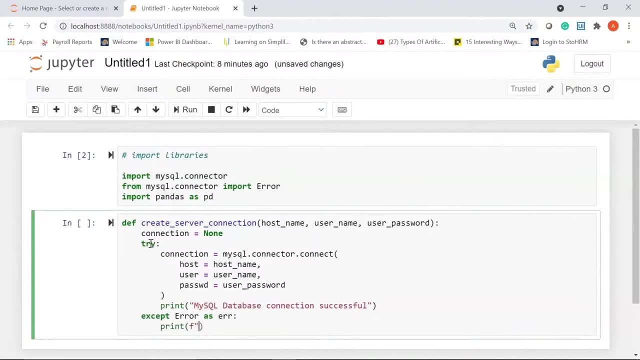 here i am going to use some print formatting techniques. using the f letter, i will write error colon and i will use curly braces, give err and then i will close the double quotes. after this i am going to return my connection. alright, let me give a comment here. 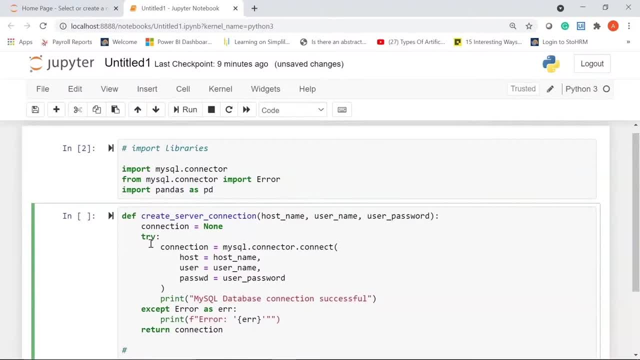 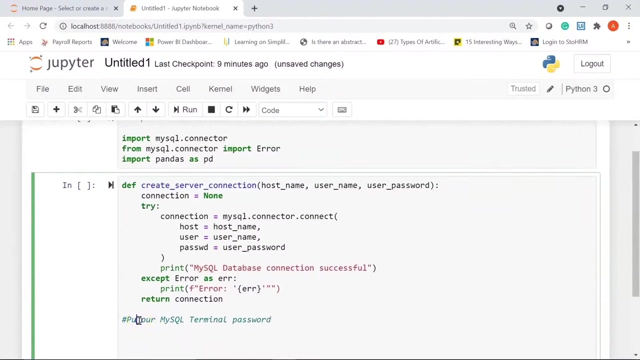 we are going to assign our password, so we need to put our mysql terminal password. so this password you assign it while installing mysql workbench. i will write mysql terminal password, pw, and i will give my password, which is simply at the rate 12345, and then 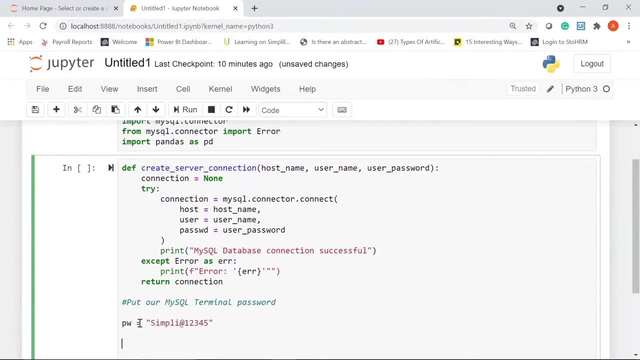 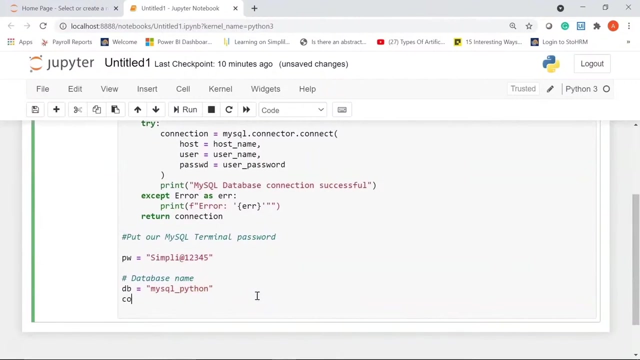 i am going to give my database name, so i will give database name. here i am going to write db e equal to this is the database i want to create, which is going to be mysql underscore, python. let me just scroll this down. okay, now i will say connection. 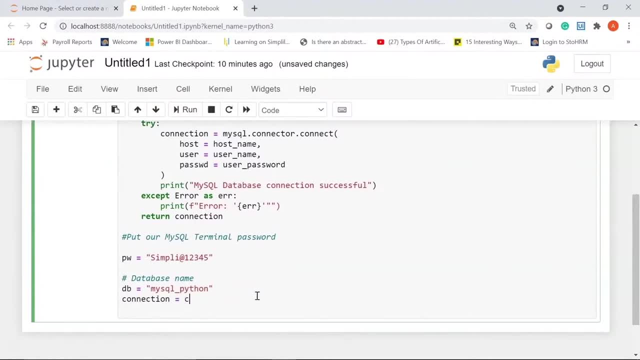 equal to: i will pass in my user defined function name, which is create server connection, and the parameters which are going to be localhost. that is my host name, my username, which is root, and then i will give pw, which is my password. that is exactly, simply, at the rate 12345. 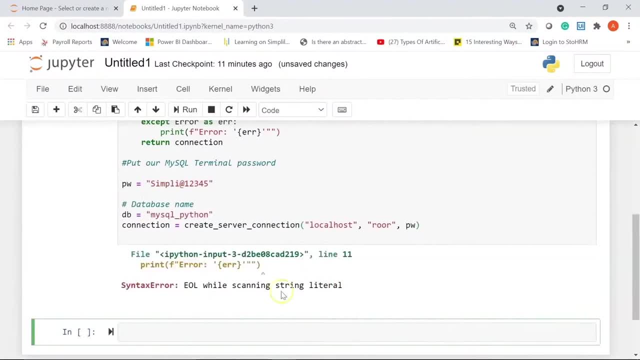 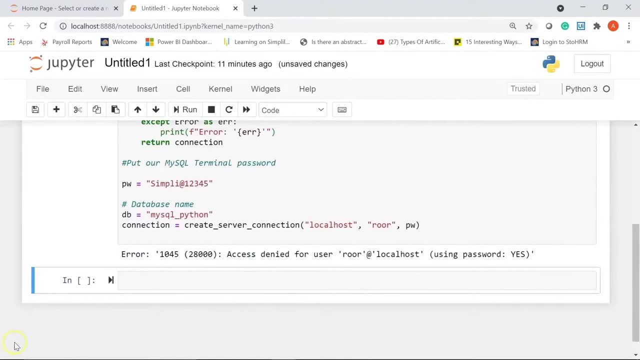 let's just run it now. okay, there is an error here. we need to remove this double quotation. all right, made another mistake here. this should be root. okay, you can see here mysql database connection successful, all right. next we are now going to create a database that is mysql underscore. 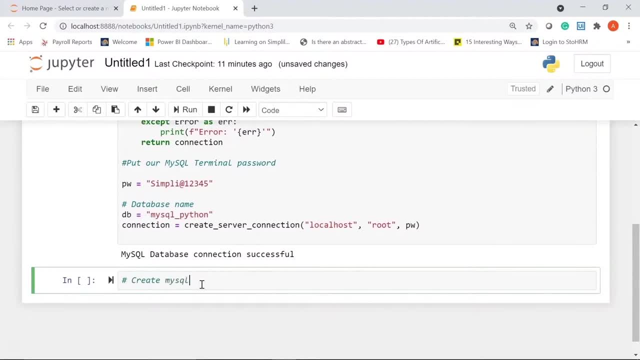 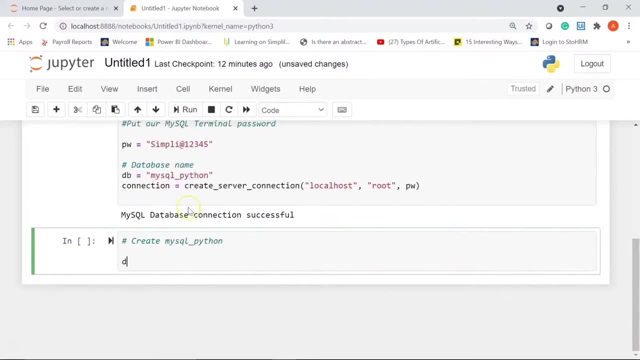 python. so i will give a comment: create mysql underscore python database. again, to create this database, i am going to create another user defined function using the def keyword. i will write the function name as create database. pass in the parameters as: connection comma query. give a semicolon. 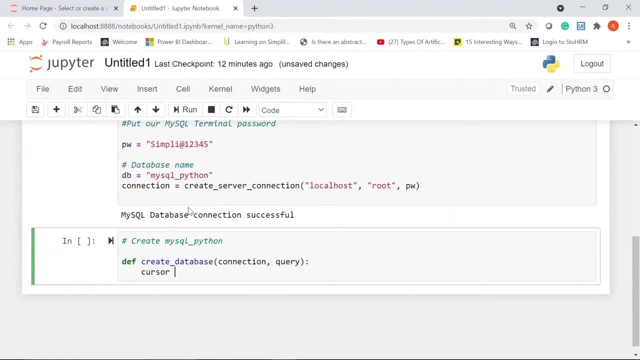 and in the next line i will write cursor equal to going to make the connection. so i will write connection dot cursor and i will give the parenthesis. so this mysql's cursor of mysql connector python is used to execute statements to communicate with the mysql database. the mysql cursor. 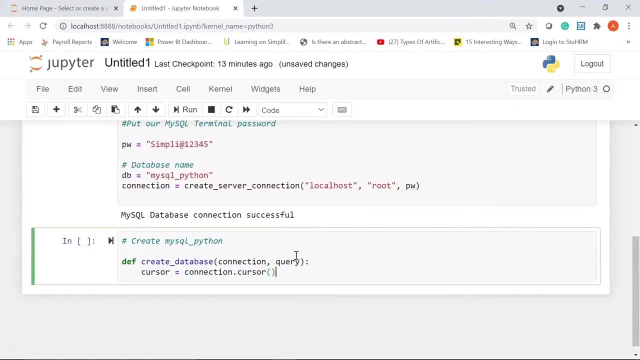 class initiates objects that can execute operations such as the mysql statements. okay, next i am going to again use my try and accept block, so i will write try, give a colon, and here i am going to use cursor dot execute. within that, i am going to pass in my query. 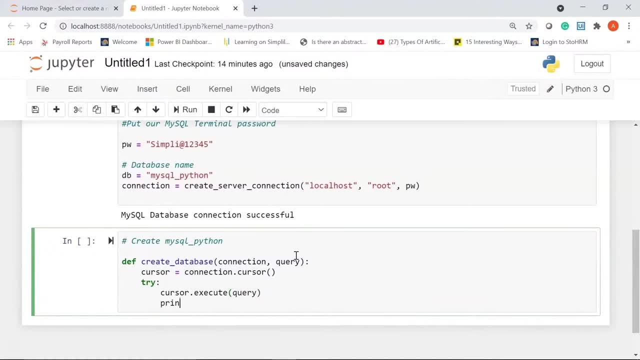 next i will use a print statement and the message i am going to display is: database created successfully. after this, i am going to write my accept block. i will write accept error as err. give a colon and then i will use a print statement. i will write print. 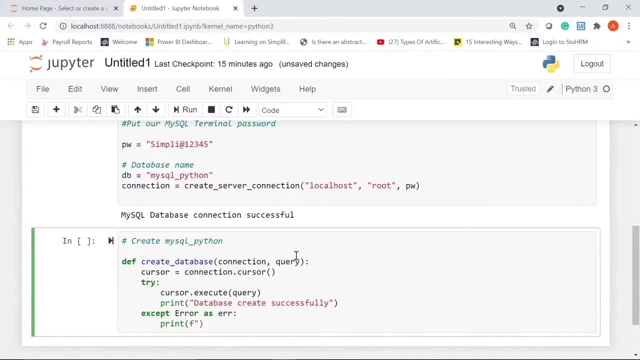 i will use the formatting again, error, colon, and i will write within single quotes: i will give curly braces, err, and then i will close the double quotes. next, let's use the variable create underscore database, underscore query, and here i am going to write my sql query to create the database. 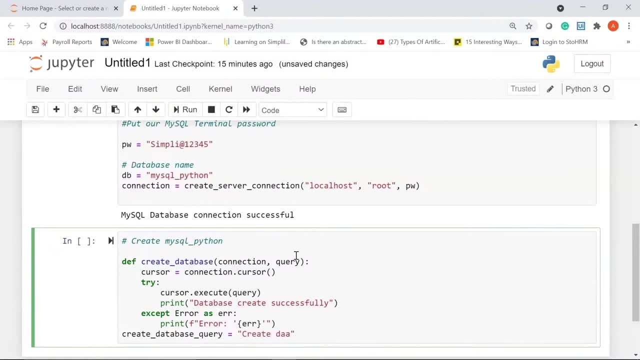 so i will write create database and followed by that i will give my database name, which is going to be mysql, underscore, python. ok, after this i will call my function, which is create database, and i will pass in the parameters. the first one is connection and next the query is: 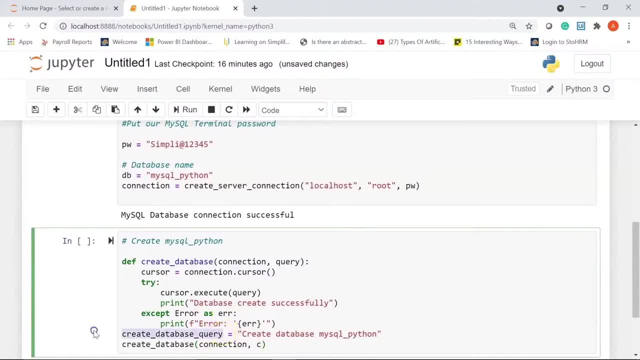 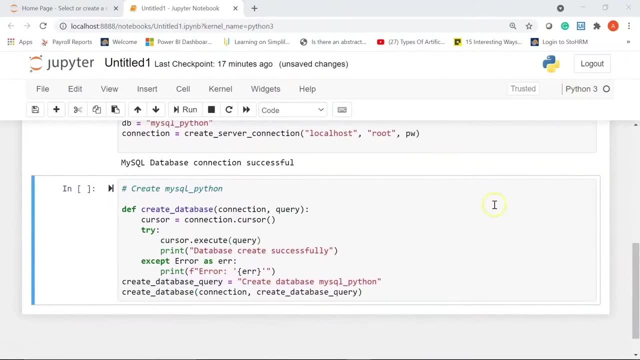 create underscore database- underscore query. let me just copy it and i am going to paste it here. alright, so what i am doing here is i am creating a new function, that is, to create a new database with the name mysql underscore python, which you can see it here. now, this function: 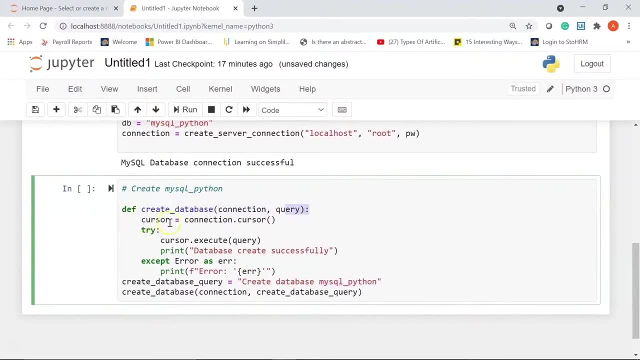 takes in two parameters: connection and query. i am using the connection dot cursor function, which is often used to execute sql statements using python language, and then i have created my try and exit blocks. so this try block statements will try to create my new database, which is mysql. 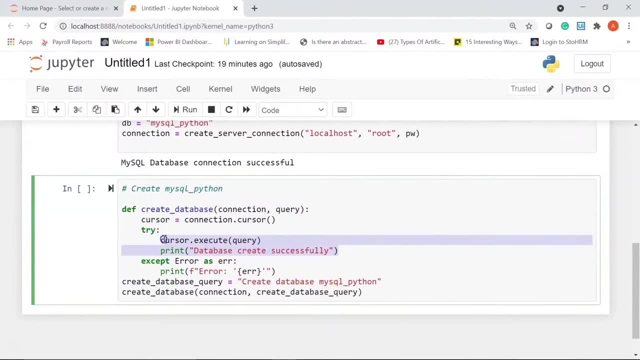 underscore python. in case it fails to create the new database, the exit block will work. so here i am writing my sql query to create a new database, which is create database, followed by the database name, and i am assigning it to a variable which is create database query, and then i am calling my function. 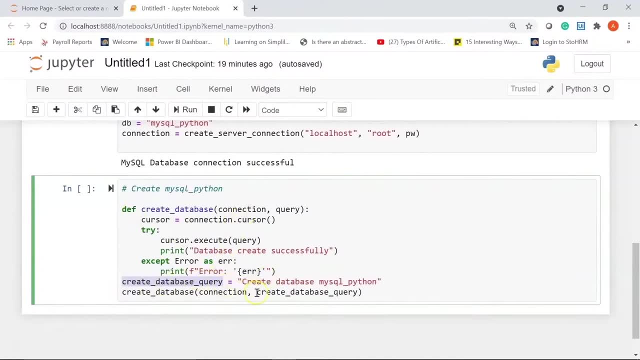 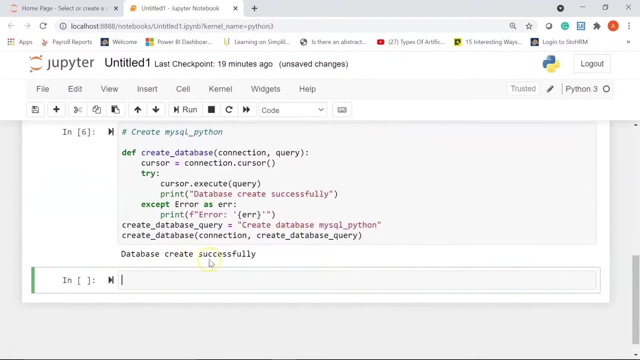 create database and passing in the two parameters, connection and the query. alright, so let's just run it. alright, you can see here it has created my database successfully. now you can verify this by checking the mysql workbench or the mysql shell. you can see on the mysql workbench: 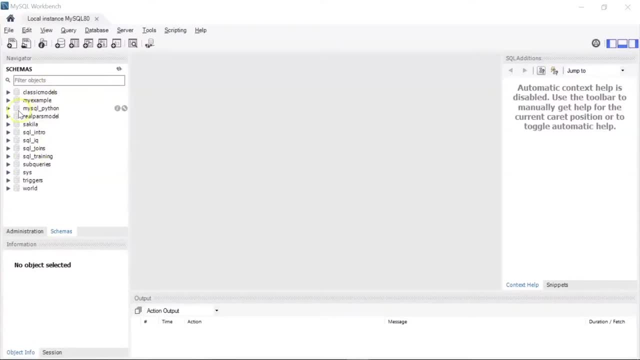 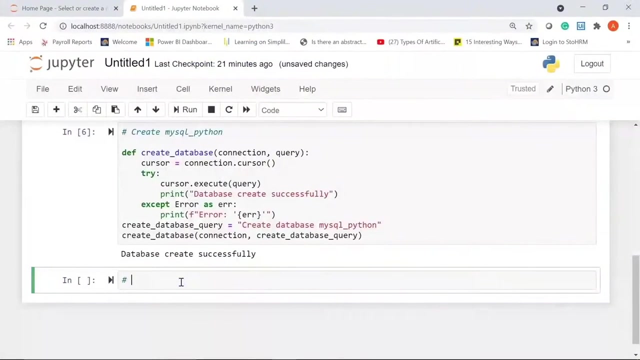 here on the left panel, under schemas, there is a database called mysql underscore python. let me just expand it now. we haven't created any table, so it's not showing it. now the next step: we are going to connect to this database, so let's go ahead and connect to our database. 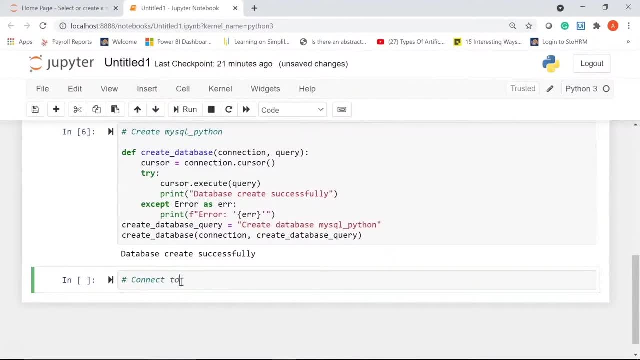 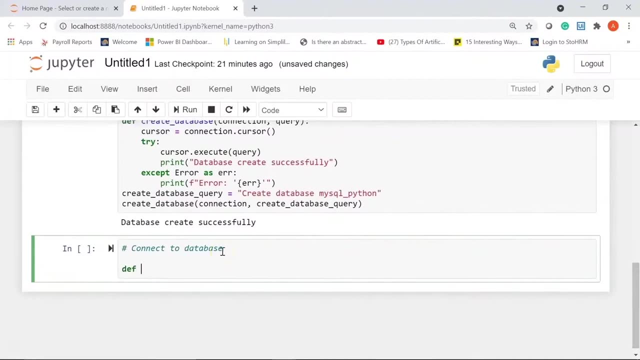 that we have just created. i will write the comment as connect to database. now, to connect to our database, i am again going to create a user defined function using the def keyword. i will write create underscore db, which is for database underscore connection, and the parameters it will take is the host name. 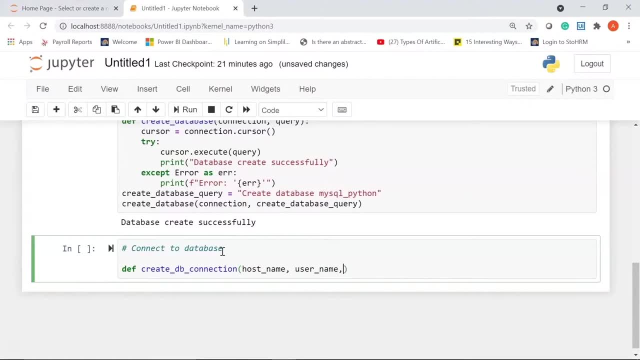 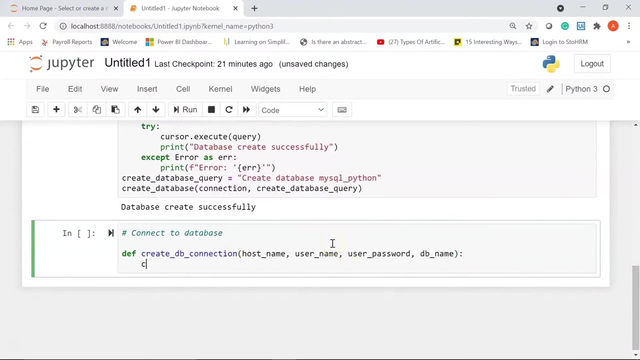 followed by the user name. then we have the user password now and finally, we have the database name. i will give a colon in the next line. i am going to create my variable, which is connection, and then i will assign it to a value. none after this, i am going to use my exception. 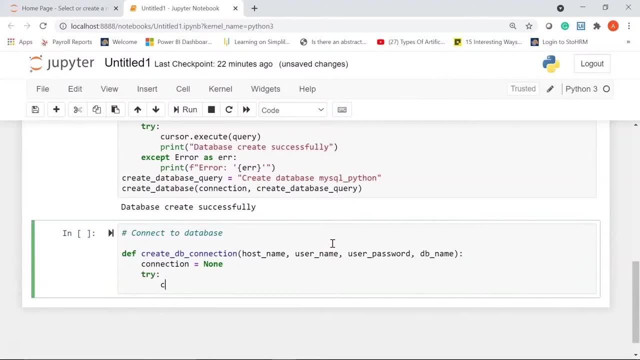 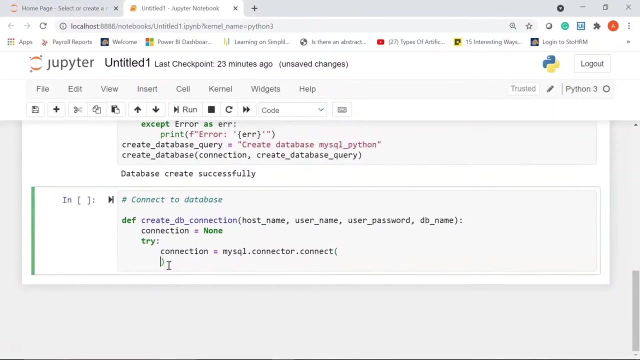 handling techniques. so i will write my try block first. i am going to reassign my connection variable using the mysql connector method. so i will write mysql dot connector, dot connect. so this method will take in the parameters. so first it will take the host name. i will write: 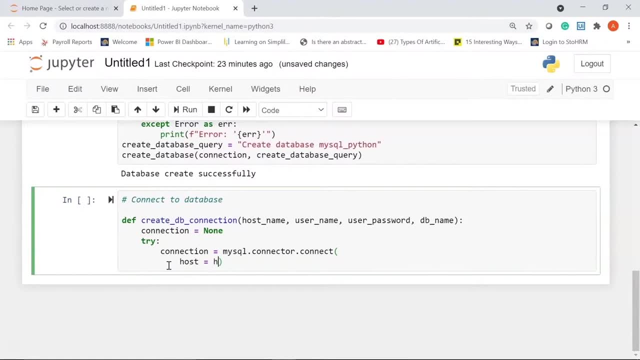 host, equal to host underscore name. i will give a comma. next it will take the user name. so user equal to user underscore name. give another comma. next it will take the user password. i will use passwd, equal to user underscore password. i will give another comma, and this time: 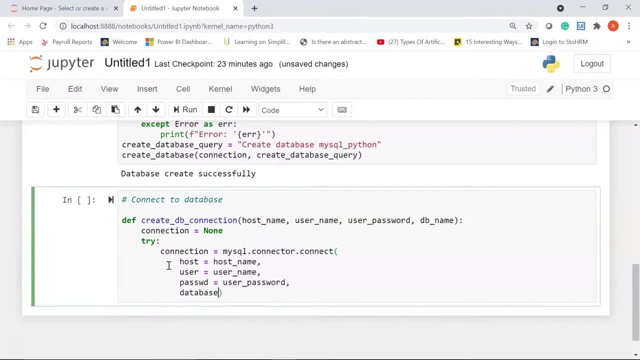 it is going to be the database name, so i will write database equal to db underscore name. now let's use the print statement and the message we are going to print is mysql database connection successful. alright, finally, we will write my accept block. i will write accept error. 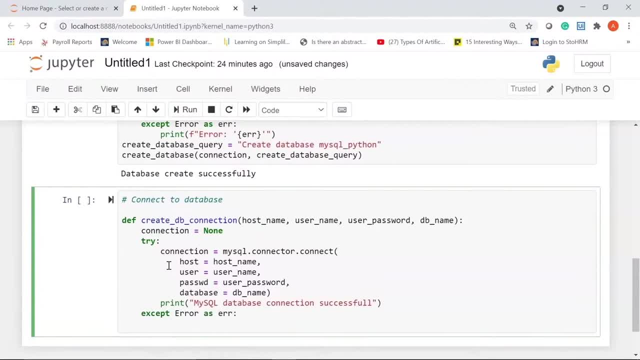 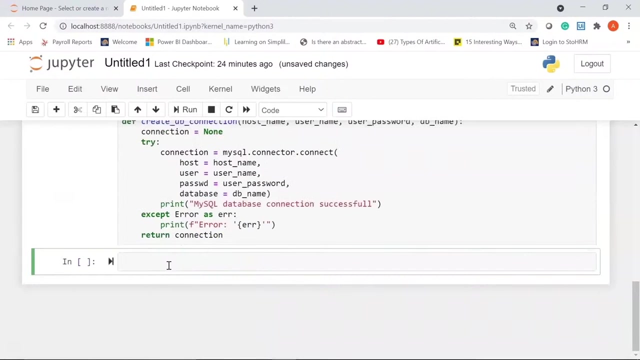 as err. give a colon, and then i will use the print statement f. within double quotes, i will write error: colon. within single quotes: curly braces. i will write err and will close the double quotes. finally, this function will return the connection value. alright, let's run it, and there you go. 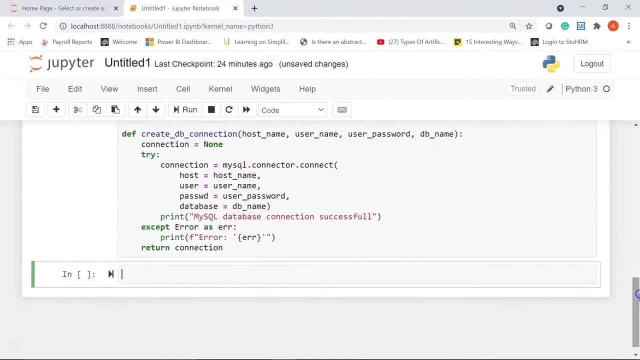 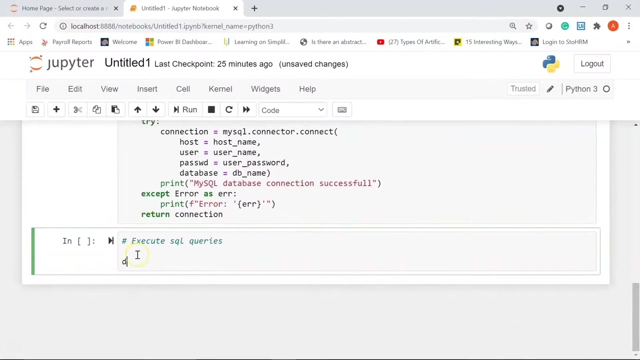 it has run successfully. so we have connected to our database. now it's time for us to execute sql queries. i will give another comment saying execute sql queries. alright, now to execute our sql queries, i will use another user defined function, which is execute underscore query, and i will pass. 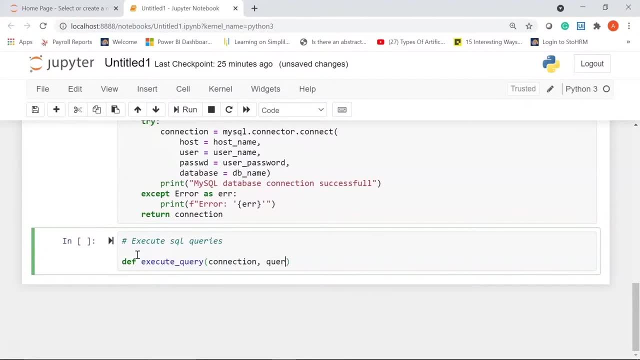 in the parameters as connection and query give a colon, i am going to write cursor equal to connection dot cursor. now this is used to establish a connection and run sql statements. next we will use the try and accept block, so i will write try cursor dot execute this. 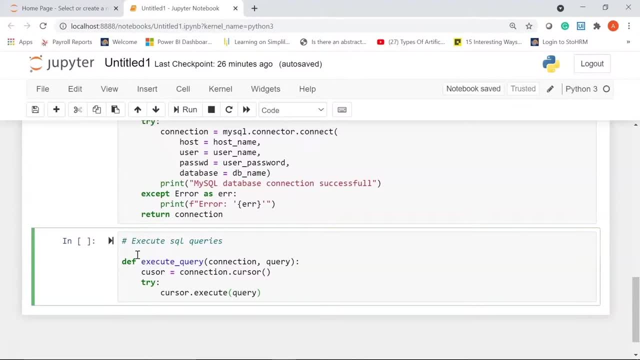 will take in one parameter, which is going to be my query, and then i will write connection dot commit, which is another method. now let's use the print statement, so i will write print. let's say the message would be: query was successful sql and then we will write our accept block. 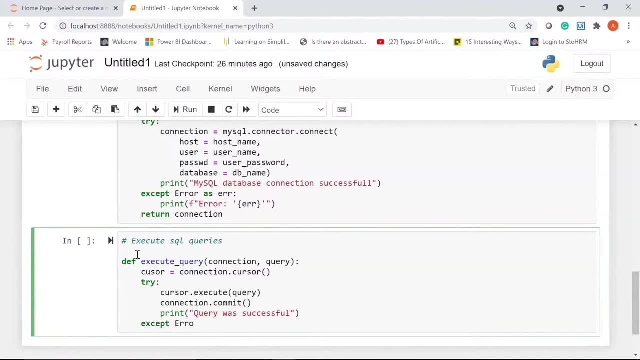 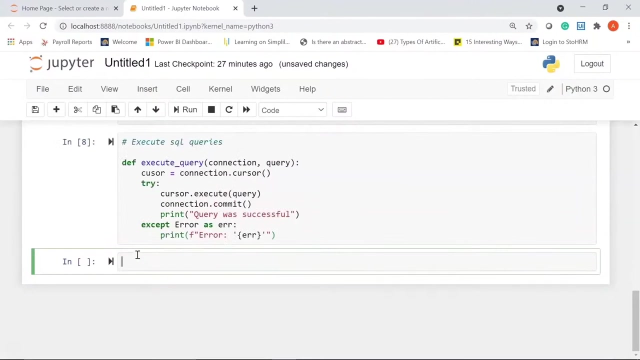 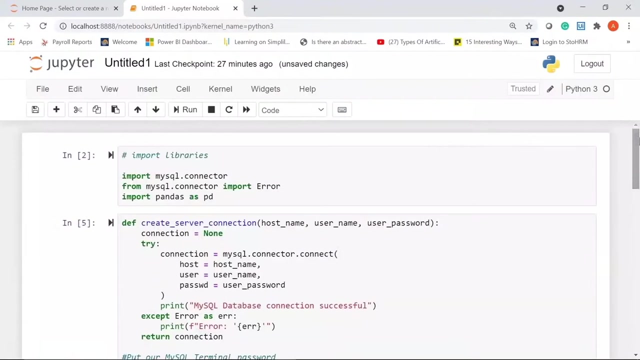 which is accept. if the try block doesn't work, throw an error using the print statement within double quotes, inside the curly braces, i will write err and close the double quotes. alright, so let's run it ok. so we have successfully created our various functions that we needed to. 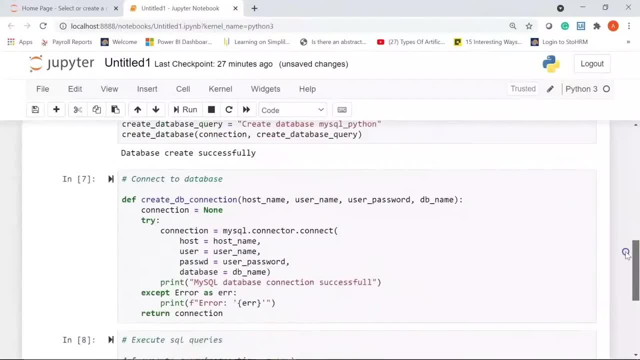 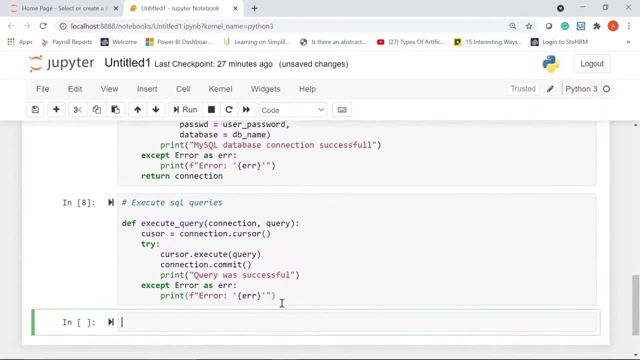 create a database, establish a connection and to execute our queries. alright, now it's time for us to create our first table inside the mysql underscore python database. so to do that, i am going to write my create command in sql. so first we are going to assign our sql command. 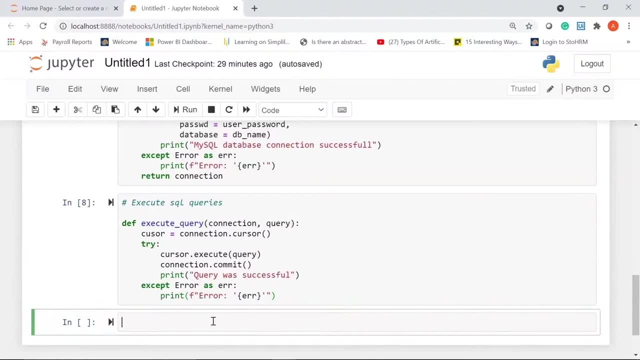 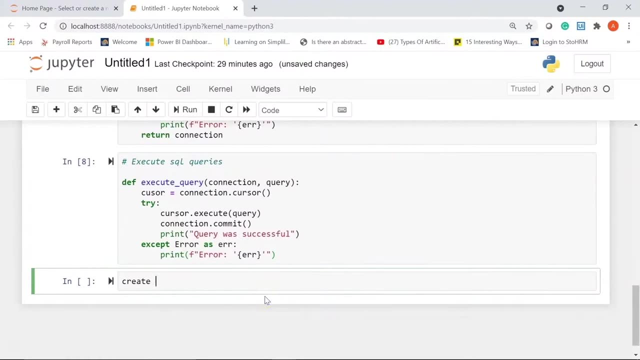 to a python variable using triple quotes to create a multiline string. so let me show you how to do that. i will write my variable name, which is going to be create orders table. it is always recommended to use relevant variable names to make it more readable, and now i am going to use 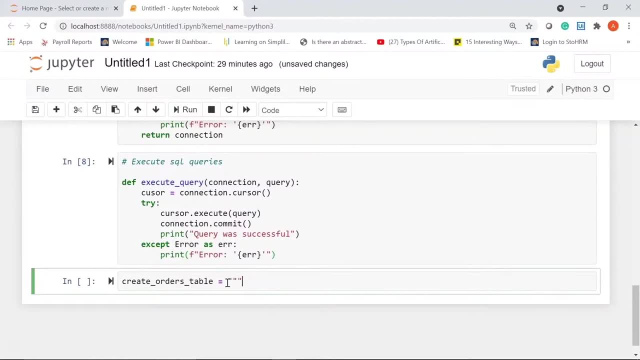 triple quotes. so the triple quote will ensure i can create my multiline string. inside the triple quote i am going to write my create command, which is create table. here i am going to create an orders table first and inside the orders table i am going to create my 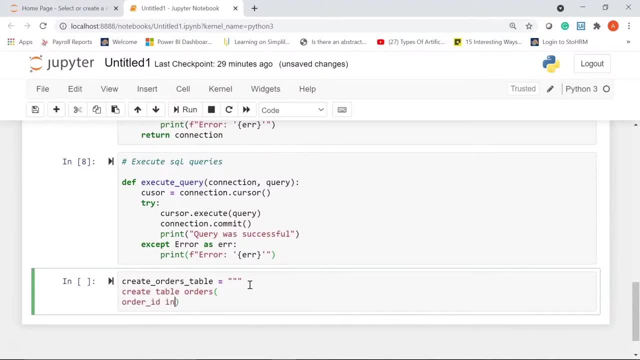 column names. the first column would be the order id. it is going to be of type integer and i will assign this order id as my primary key column. i will give a comma next. the second column would be customer underscore name. the customer name column would be of type. 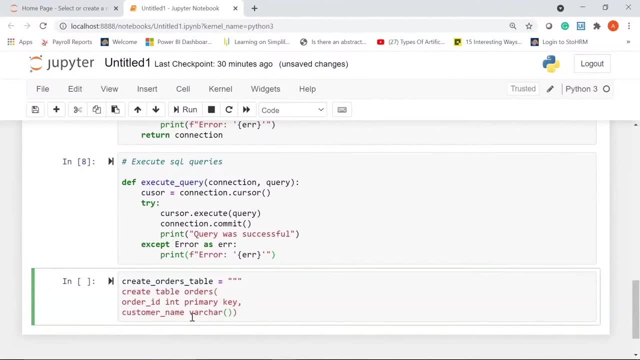 varying character. so i will write varkar and i will give a size of 30, and this is also going to be not null. moving ahead, my fourth column would be the product name column. so i will write product underscore name. product name will be of type varying character. the size is: 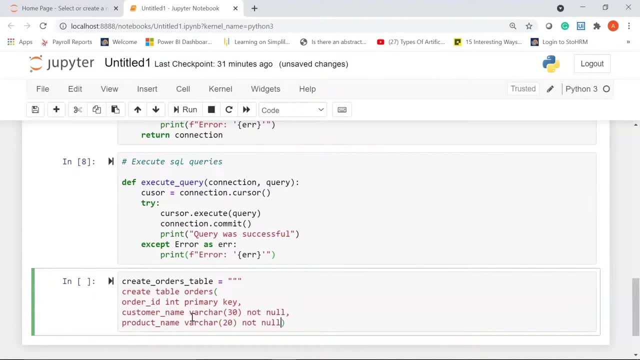 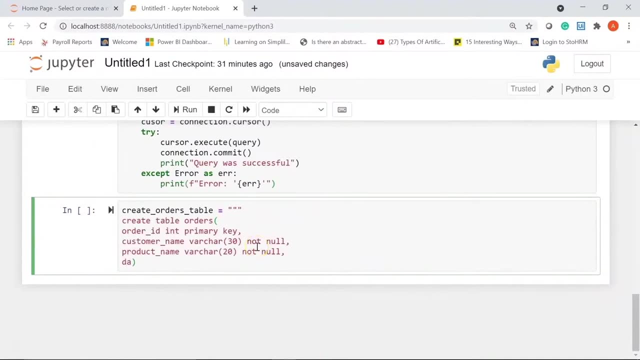 let's say 20, and it is also not null. next, i am going to create my fourth column, which is the date on which the item was ordered or the product was ordered. so i will write date ordered. the data type will be date. next i will create: 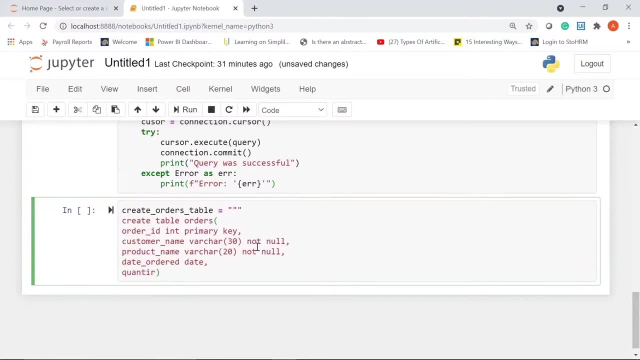 a quantity column to keep track of the number of quantities that were ordered. this is of type integer. my next column would be unit price, which will basically have information about the price of each unit of product. unit price can be of type float. and finally, i will have the 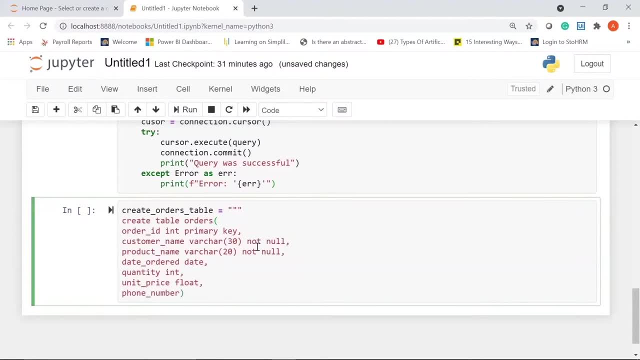 phone number of the customer. i will write phone number. phone number can be kept as of type varying character. i have assigned a size of 20. now let's give a semicolon and will close the triple quotes. alright, so this is how the syntax would look like. 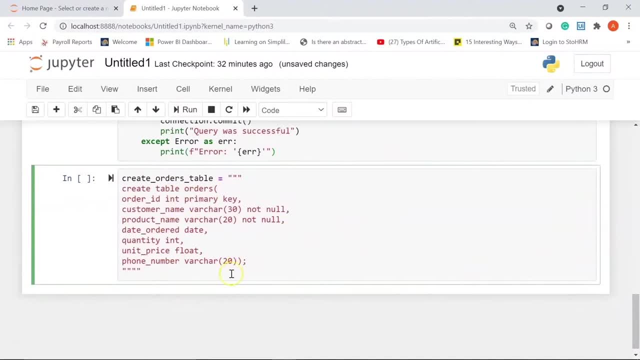 next to run this, we are first going to call our create db function. so let me give a comment. as connect to the database, i will write connection equal to create underscore db, underscore connection. my parameters would be my host name, which is localhost, my username, which is root. 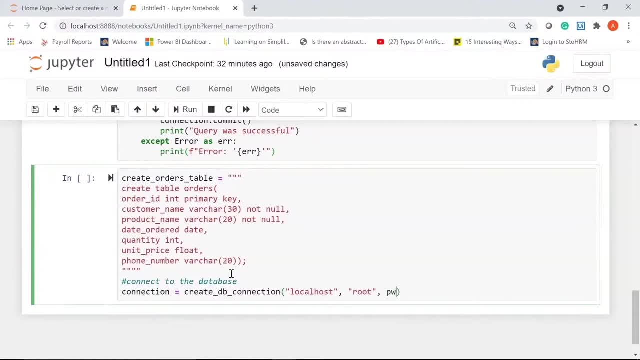 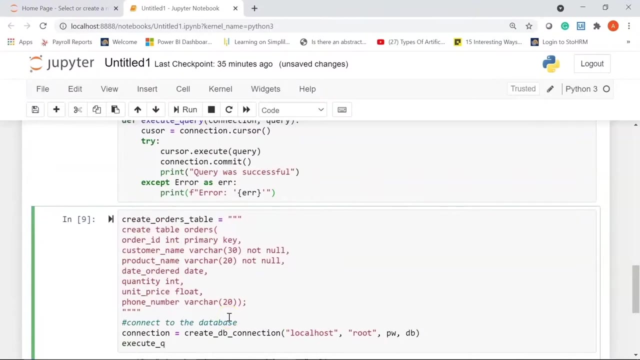 comma, my password and then my database name, which is mysql underscore python. so i will write just db, alright. finally, let's execute this query using the execute underscore query function that we had created earlier. this takes in two parameter. the first one is connection, followed by the variable. 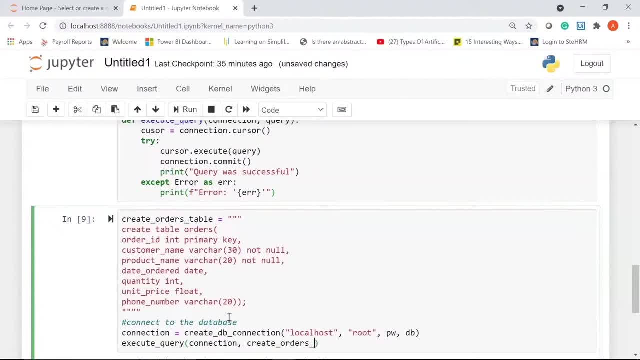 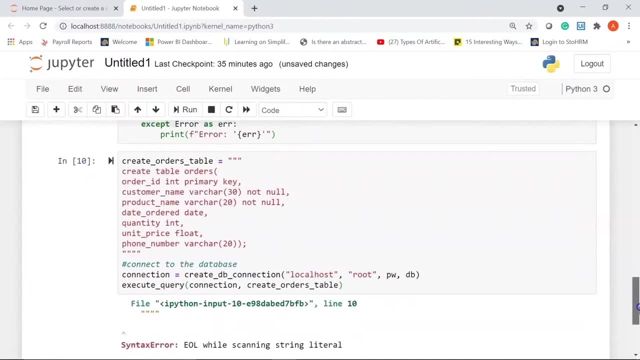 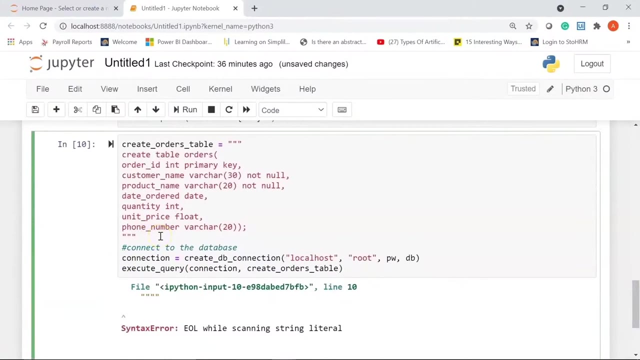 name, which is create orders underscore table. let us run it. ok, there is some error here. let's see what's the error. ok, so here we have put four double quotes. this should be triple quotes. now let's run it. ok, there is another here. let's debug it. 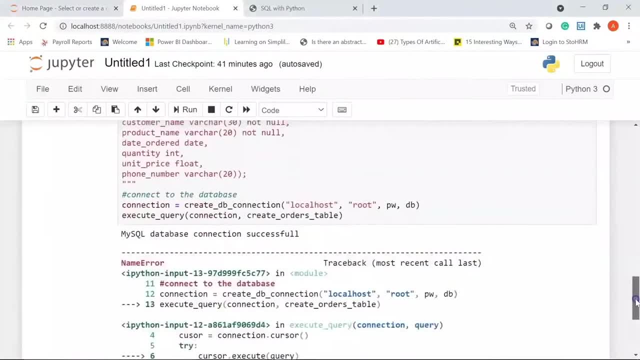 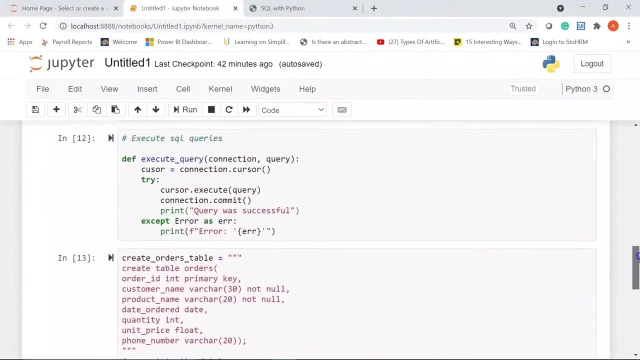 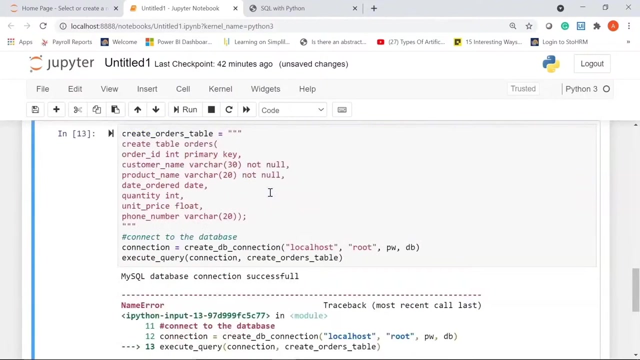 it says name cursor not defined. let me just roll it to the above cell. if you see here in our execute underscore query function, instead of cursor i have written cursor, so r is missing. let's redone this. and now let's run this again. there you go. you can see here: 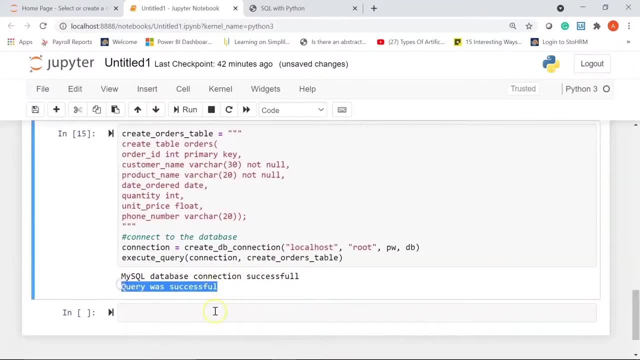 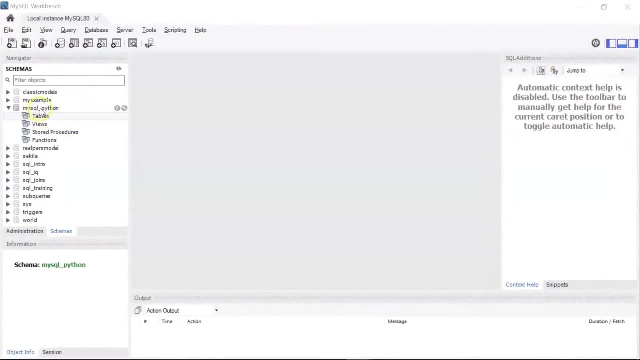 mysql database connection successful. even our query was also successful. now, if you want to recheck if the table, that is, orders, was created or not, you can check it on the mysql workbench. so let me show you how to do it. so i am on my mysql workbench and under 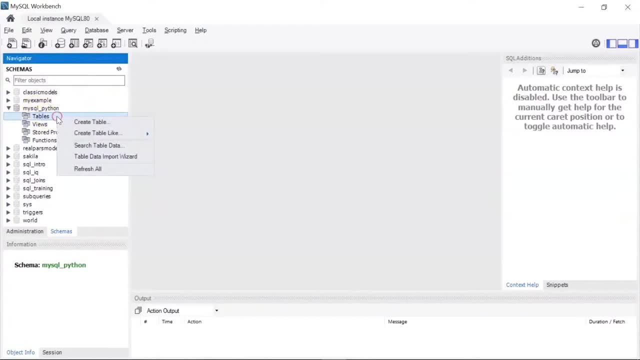 mysql underscore python database. you have something called as tables. let me just right click and i'll select refresh all. there you go. you can see this arrow. just click on this arrow and here you can see we have a table called orders. so we have created a table called orders. 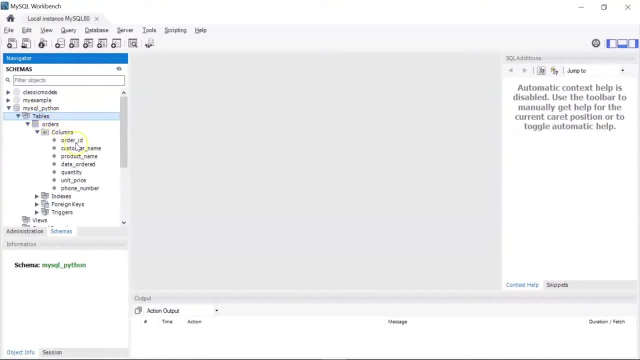 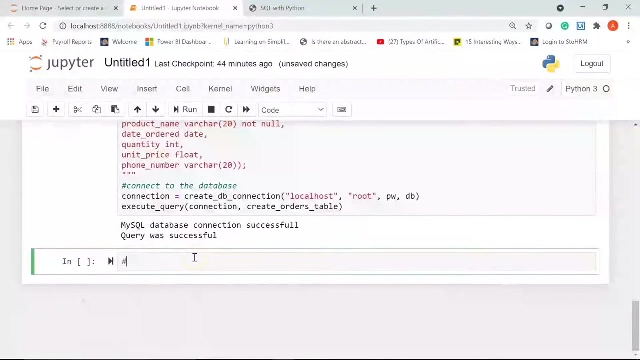 now you can check the columns as well. you have the order id. you have the order id, the customer name, product name, ordered date, quantity, unit price and phone number. now it's time for us to insert a few records to this table, which is orders. now to insert records, i'll 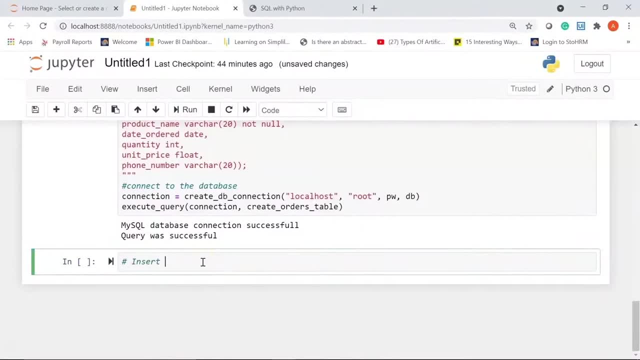 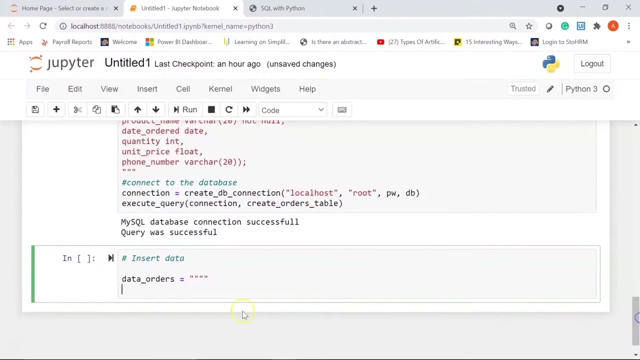 give a comment as insert data. i'll start with the variable name. let's say the variable name is data, underscore orders. i'll give triple quotes. next i'll write my insert into command. so i'll write insert into my table name, that is, orders, followed by values. and now 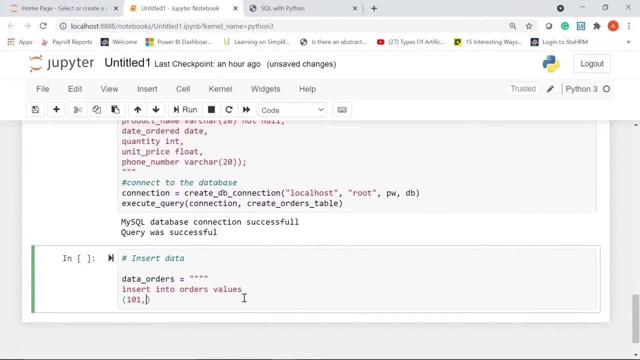 i'll start entering my records for each of the rows. so first i'll give 101, which is the order id, then i'll give the customer's name, let's say steve, and the product he had ordered is, let's say, laptop. then i'll give my date in which the item 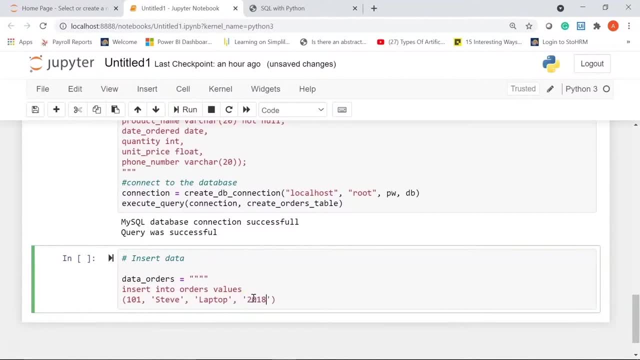 was ordered. let's say it is 2018. i'll choose 06 as the month and the date is, let's say, 12. we'll give another comma. this time we'll pass in the quantity, which is 2. let's say the price of each laptop was $800. 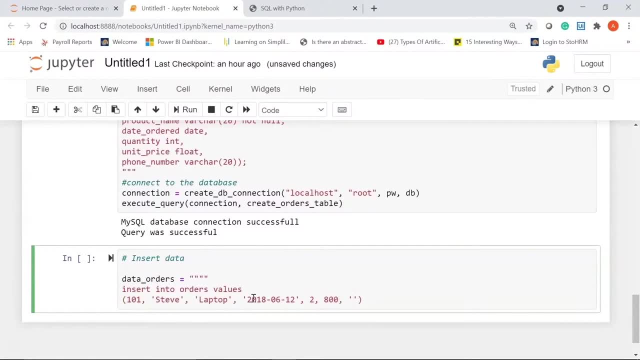 and we'll give a phone number. this is random, let's say 6293, 730, let's say 802. alright, similarly, i'm going to insert 5 more records of different customers and their items that they have purchased to this table orders. so here on my notepad i have 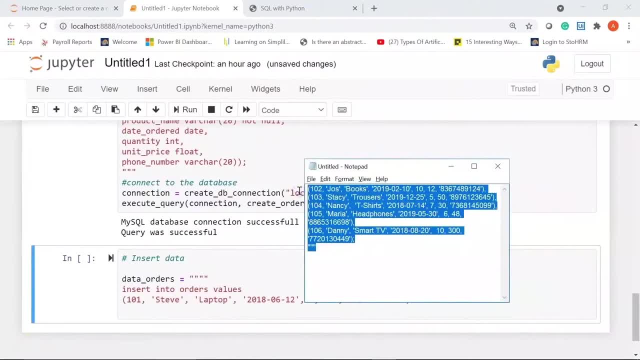 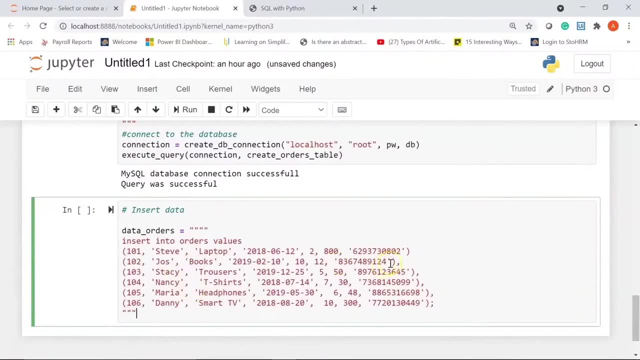 my rest of the 5 records. let me just copy it and we'll paste it in the cell here. this will save us some time. ok, let me recheck. if everything is fine, i'll give a comma here. alright, so we have 6 customers in our table which have their. 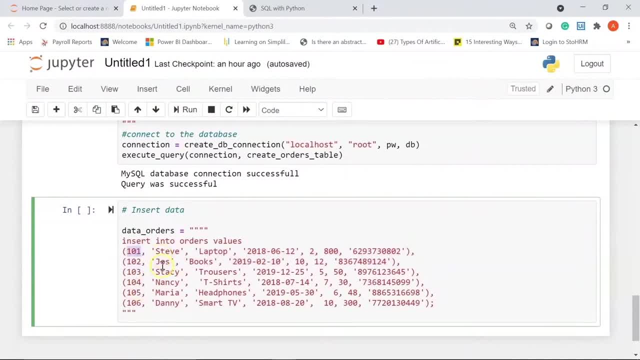 customer ids from 101 to 106. you have steve, joss, stacy, nancy, maria and danny. you have the different items they have purchased: laptop, books, trousers, t-shirts, headphones and smart tv. this is the date on which they had ordered this item. the number of 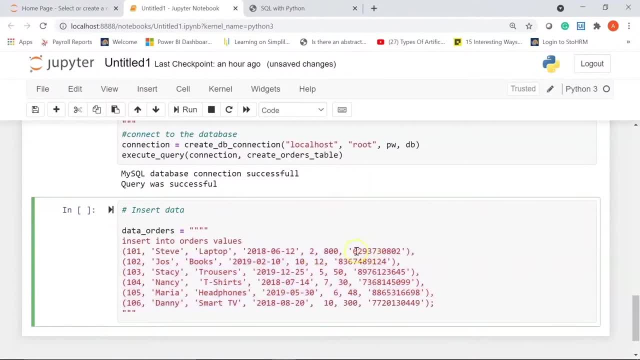 quantities they had ordered, and then we have the unit price and some random phone numbers. so let's create the connection. now. i'll write connection equal to. i'll write create underscore db underscore connection. then i'll going to give my same parameters. let me just copy it from the top, which is local. 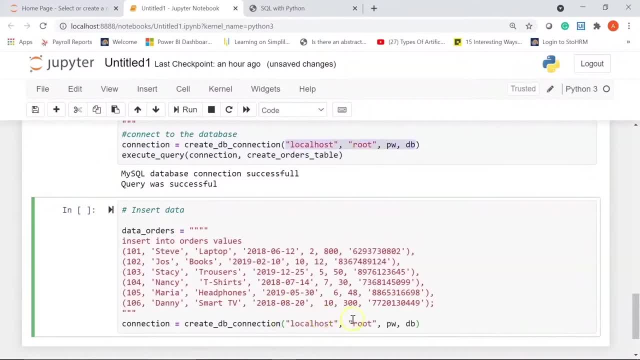 host. the host name root is my username, then we have password and the database name and then i'll use the same query as above, which is execute query. i'll copy this, paste it here and instead of create orders table variable, i'll put as data underscore orders. 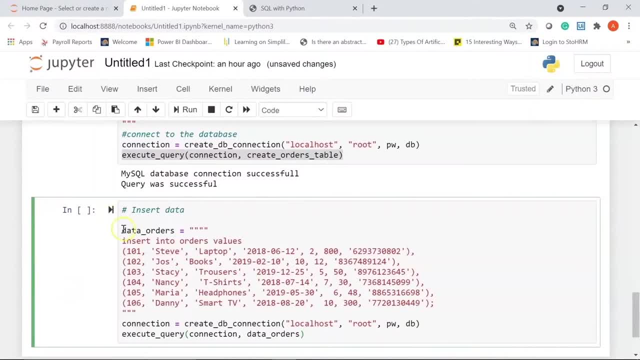 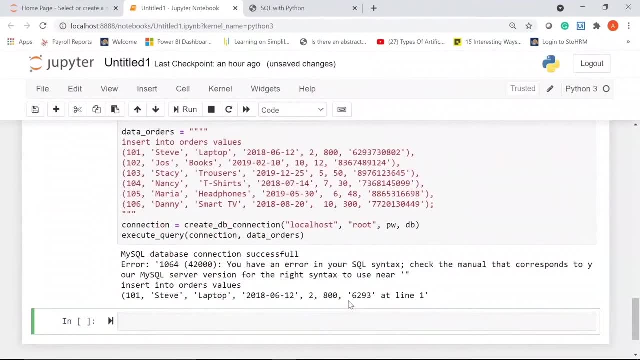 so this will store my insert into command. you can see. the variable i've used here is data underscore orders. now it's time, let's just run it. alright, there was some mistake here. let's debug it again. this should be triple quotes and not four. now let me rerun it again. 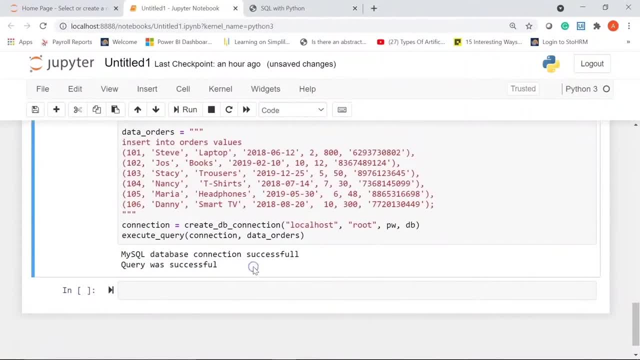 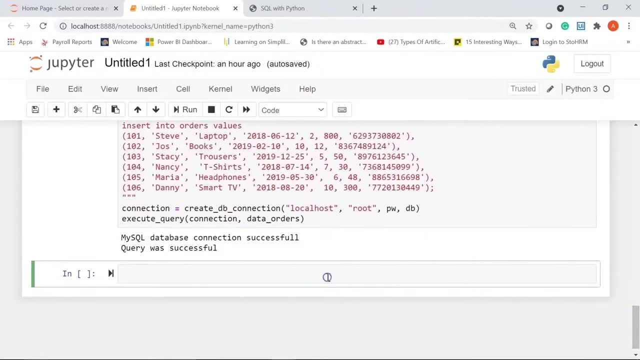 there you go. you can see here my sql database connection successful and my query was also successful. now we'll create another user defined function which will help us read query and display the results. so i'll write my function name as df: read underscore query. this will take in two parameters: connection and 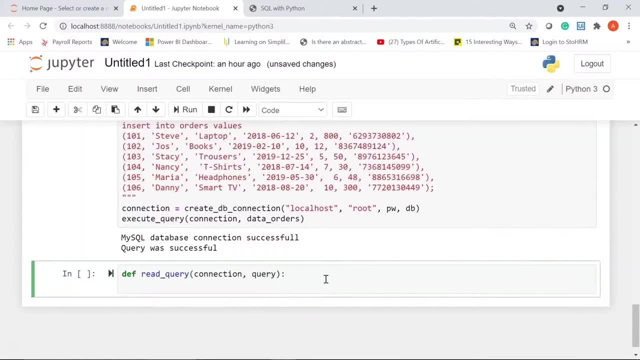 query, then i'll write cursor equal to connection dot cursor. i'll put my result as none and then i'll use my try and accept log. i'll write try cursor, dot execute. this will take in one parameter, which is query, and then i'll give another variable. 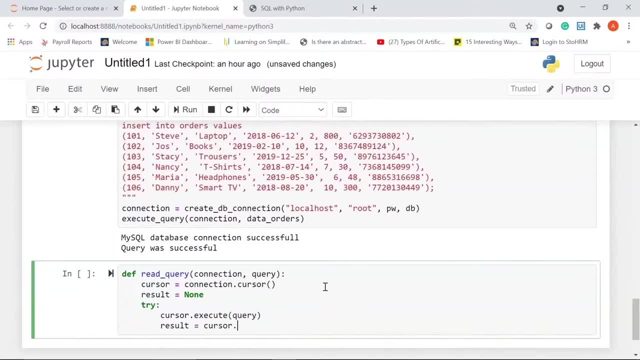 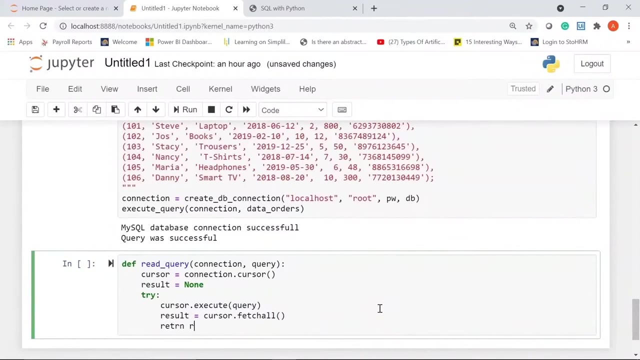 which is result equal to cursor dot. fetch all. now this fetch all method will return all the results in the table. i'll write return result. next, we'll use the accept block. so i'll write accept error as err. give a colon and i'll use my print statement. 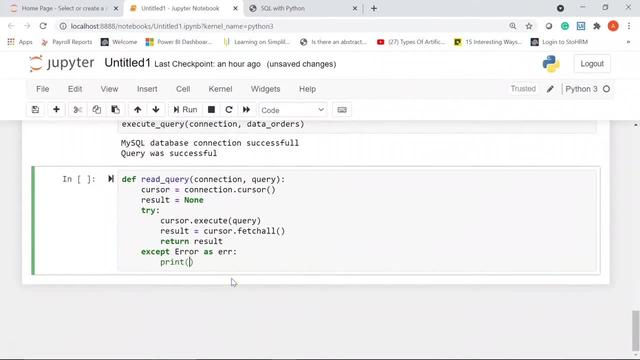 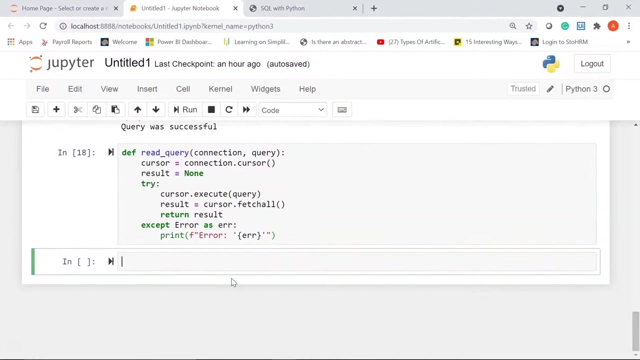 scroll this down. i'll use my formatting f: error: give a colon followed by a space within single quotes, inside curly braces. i'll give err and close my double quotes. let's run it alright. so now we are all set. now we are going to use our select. 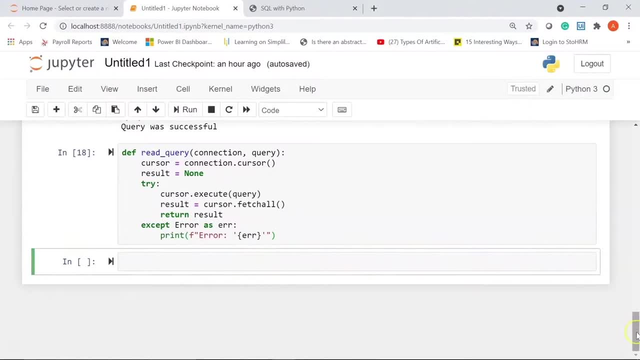 clause having, whereby then we'll see how to use, order by clause, some inbuilt functions, we'll update some records, delete some records and do a lot of other stuff. so let's start with the first query. so our first query is going to be using the select statement. 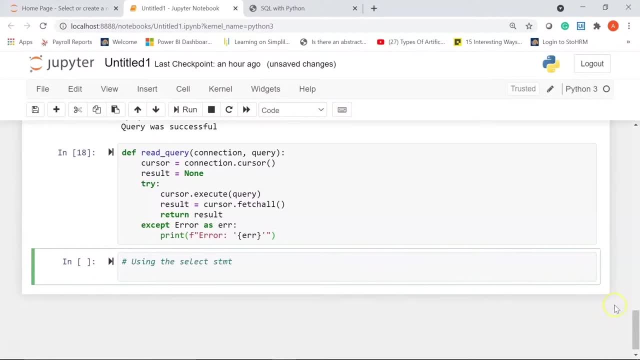 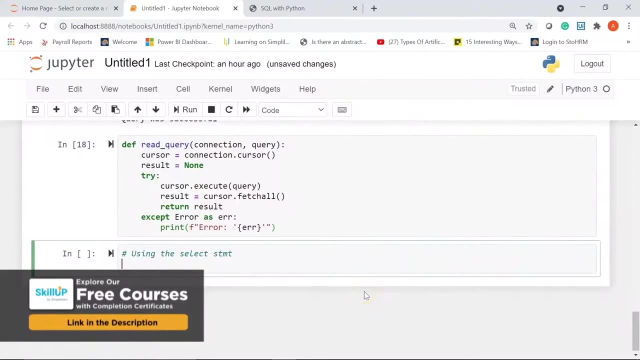 alright, so suppose i want to display all the records that we have inserted into our orders table. so the way to do is i'll assign my query to a variable, let's say q1. i'll give triple quotes. within triple quotes i'll write: select star from. 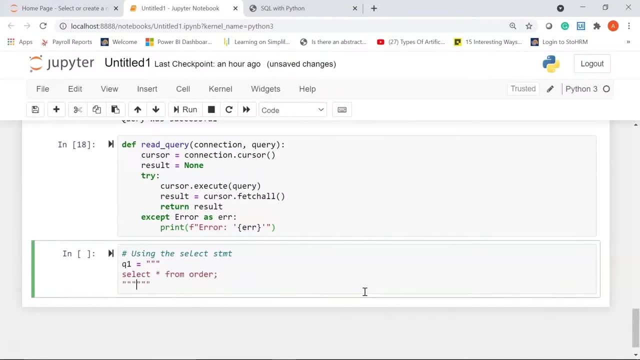 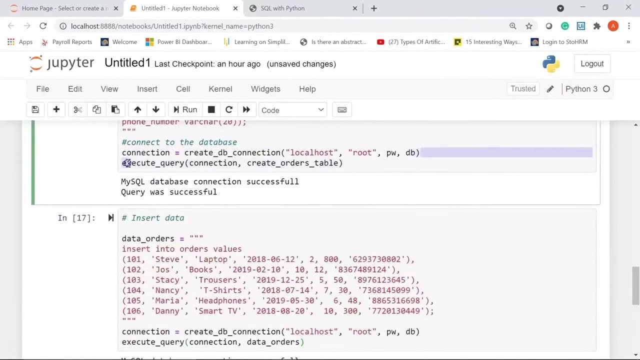 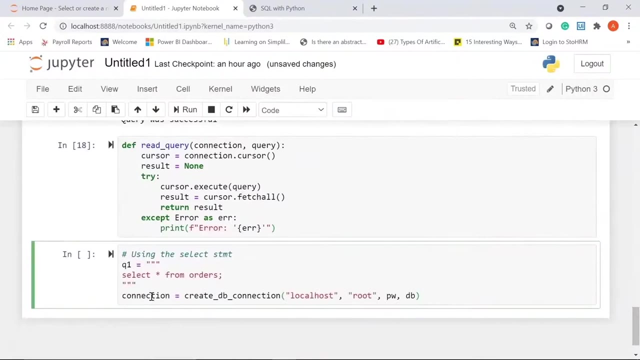 orders. i'll give a semicolon followed by the triple quotes. now we'll establish the connection. so let me just go to the top and i'll copy this line, which is to connect to our database. i'll paste it here. now we'll create a variable called results. that will store. 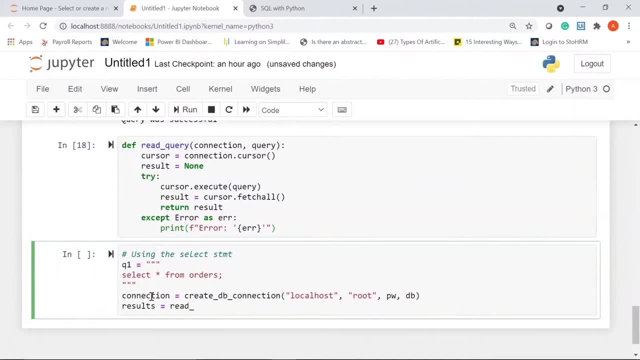 the result of this query and we are going to assign this variable to our function, that is, read query, and this read query will have two parameters: the connection and the variable name, which is q1 for the query next to display. i'm going to use a for loop. i'll write. 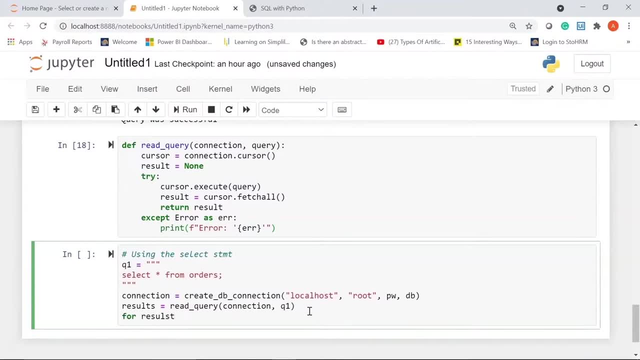 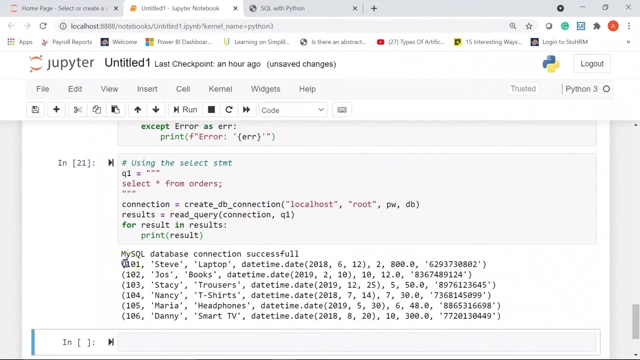 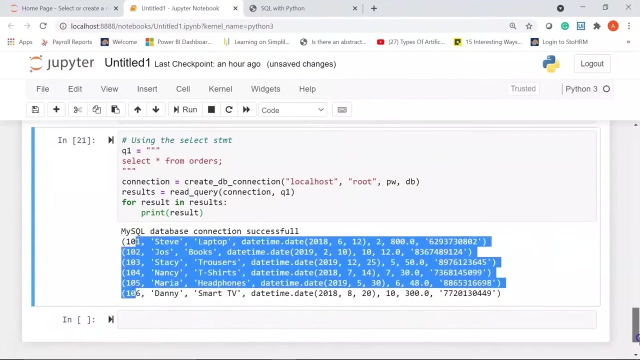 for results. for result in results print. i'll say result. now we are done, let's just run this query. there you go. you can see here we have successfully printed all the rows in our table, which is orders. you can see we have six records in total. now we are going to explore. 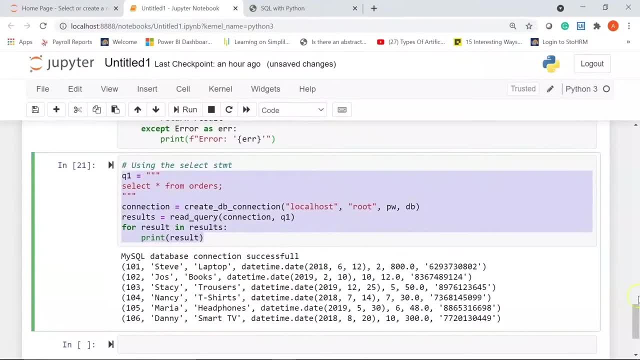 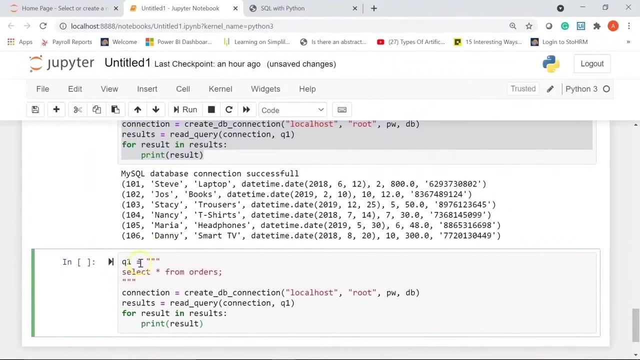 a few more queries, so let me just copy this and we are going to edit in the same query. i'll paste it here. next, let's say you want to display individual columns from the table and not all the columns, so let me. let me create the variable q2. 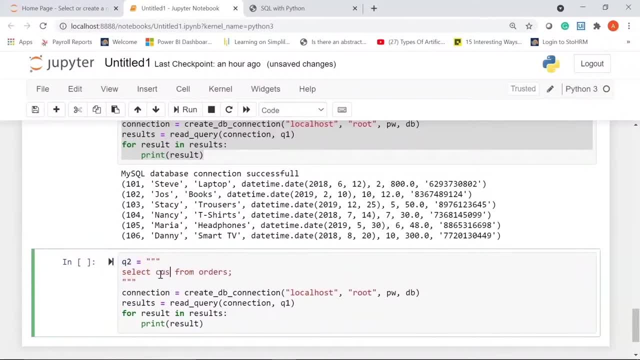 now, instead of star, i'm going to display only the customer name and let's say the phone numbers of the customer. so i'll write phone underscore number. alright, the rest all remains the same. let me just recheck it and here, instead of q1, we'll put 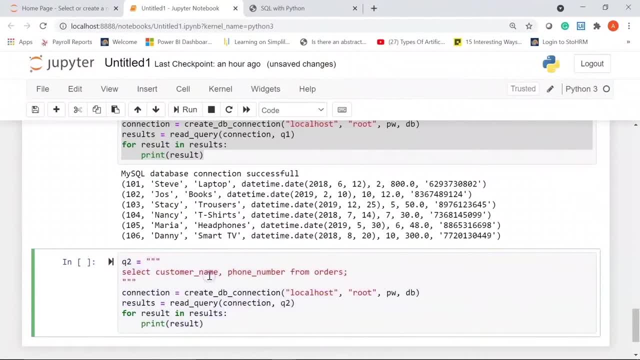 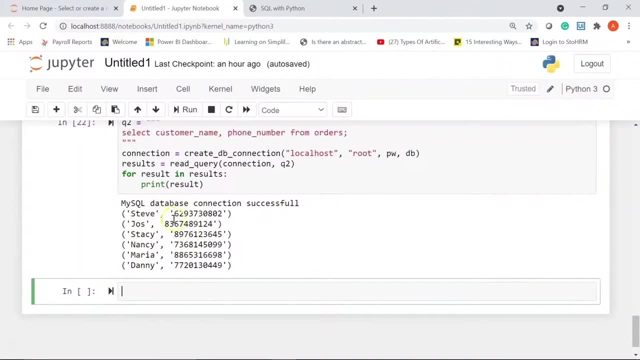 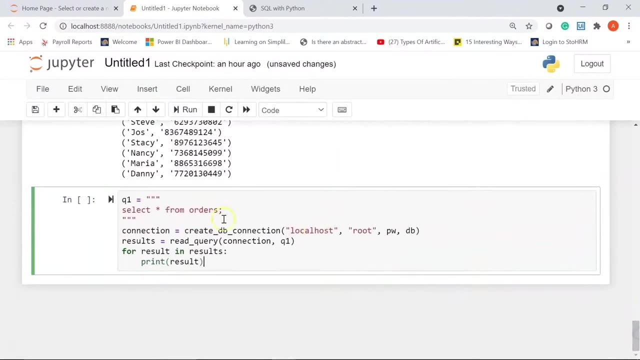 q2 and let's run this cell. alright, you can see here now we have displayed only two columns. the first column is the customer name and then we have the respective phone numbers. ok, now let me just paste that query again. now we are going to see how you can use. 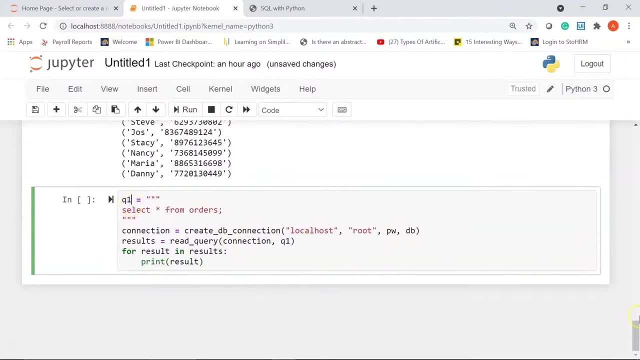 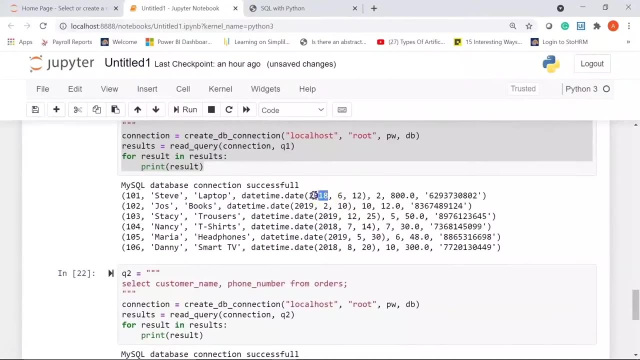 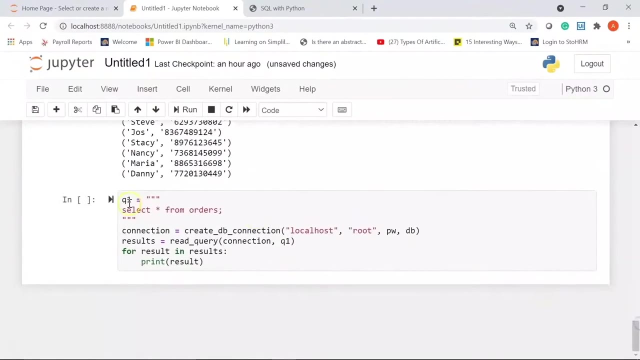 an illbuilt function that is in our table. we have the order date and from the order date we are only going to display the different years that are present in the order date. so to do that, i'm going to use the year function. i'll add this query: 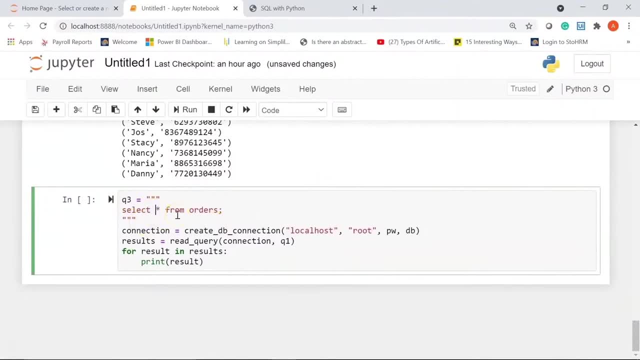 instead of q1 i'll make it q3, and here i'm going to write select year, which is my function name, from my column, which is date ordered from orders, and here i'll change this to q3. q1, q2, q3 are basically query 1, query 2 and query 3. 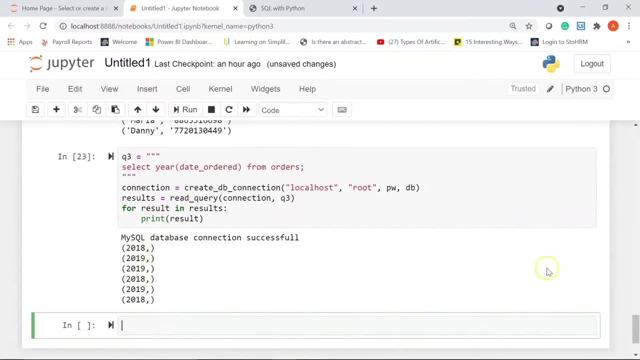 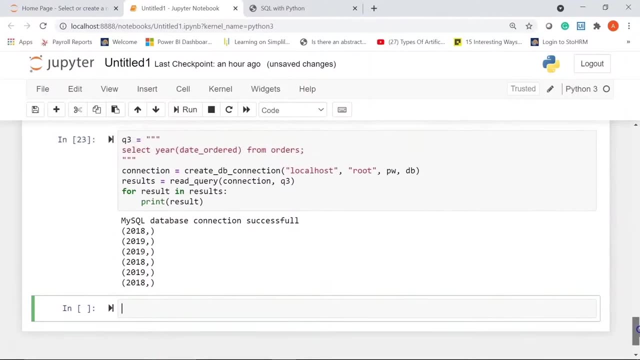 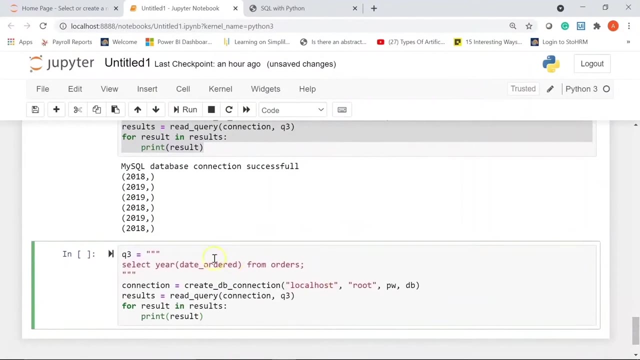 let's run it. there you go. so we have successfully extracted the different years present in the order date column. now, if you want to display the distinct or the unique dates present in the column, you can use the distinct keyword in the select statement. so the way to do. 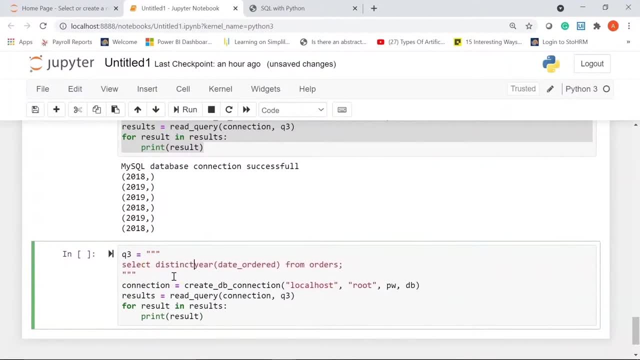 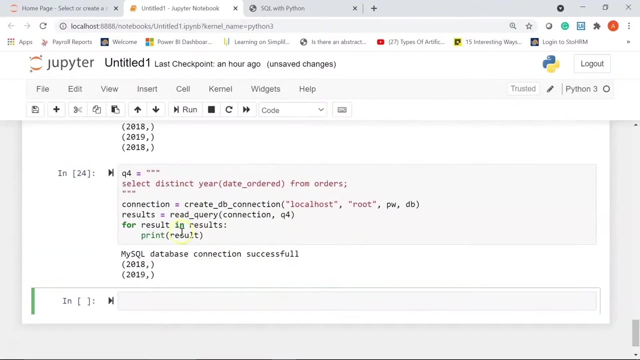 it is. i'll write select distinct. give a space. the rest of the query remains the same and here, instead of q3, i'll write q4. i'll make this as q4. let's run it. you can see. 2018 and 2019 are the unique year values. 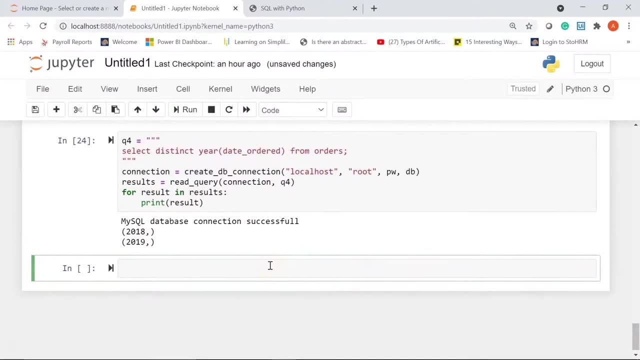 that are present in the order date column. okay, now moving ahead, let's write our fifth query, and this time we are going to explore how you can use the where clause, so i'll change this to q5 before i write my query. so let's say you want to display all the 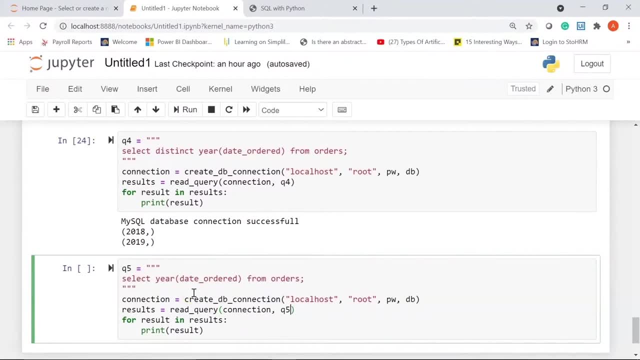 orders that were ordered before 31st of december 2018. so to filter this, we are going to use the where clause, so i'll write select star from orders. next, i'll write: where my date underscore ordered is less than within quotes, i'll give my date value. 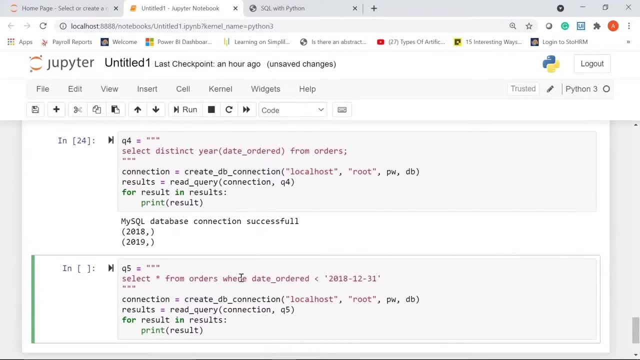 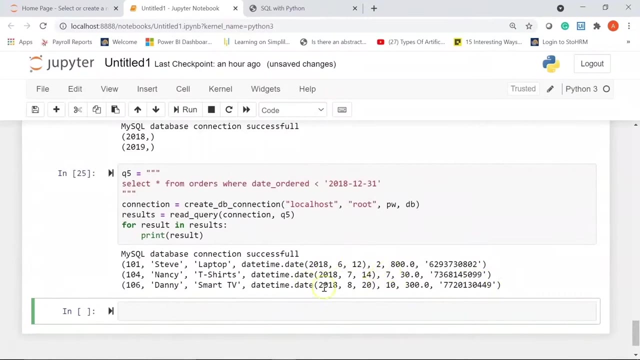 which is 2018 december 31st. so all the items or the products that were ordered before 31st of december 2018 will be displayed. so let's run it alright. you can see here there are three orders in our table which have been ordered before. 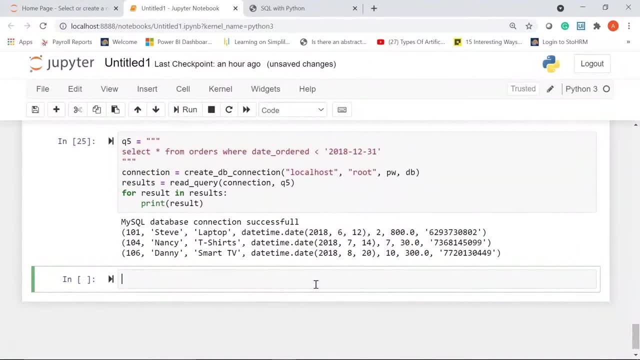 31st of december. now, moving ahead, we want to display all the orders that were made after 31st of december. so here what you can do is i'll just copy the above query again. i'll copy this line. so, instead of less than 31st of december. 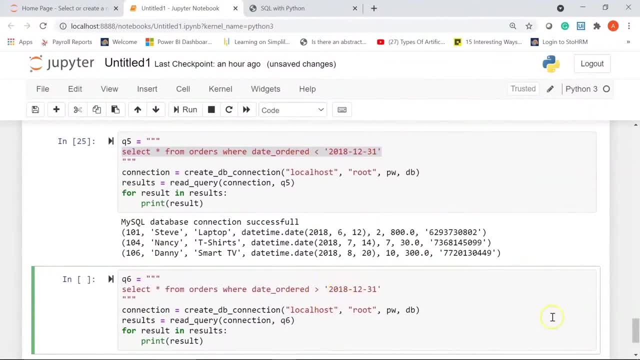 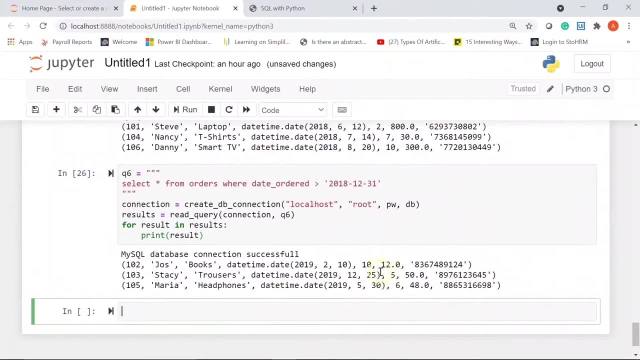 2018. i'll make it as greater than so. every order that was placed after 31st of december will be displayed, if you run it. so you can see here there are three orders in our table which were ordered after 31st of december 2018. 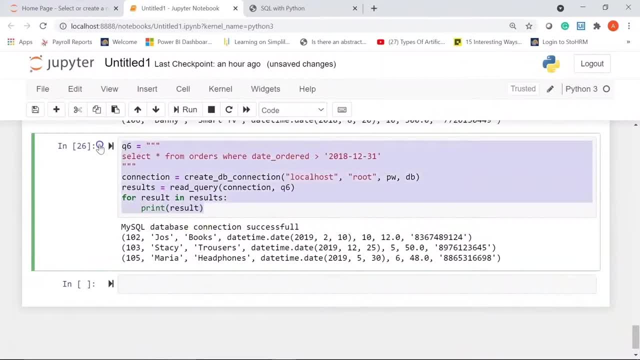 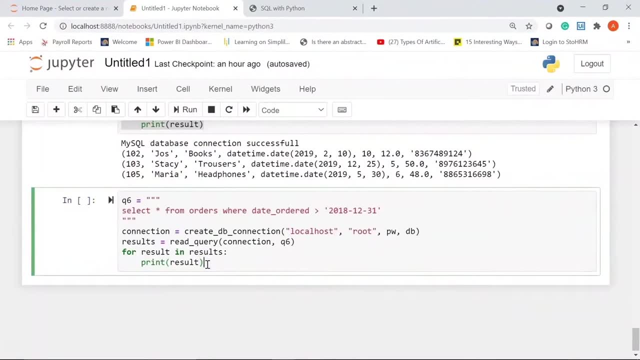 now moving ahead. let's write our seventh query. now let's see how the order by clause works in sql, so you can filter your results based on a particular column or sort it based on a particular column. so this is going to be my query 7. i'll write it from scratch again. 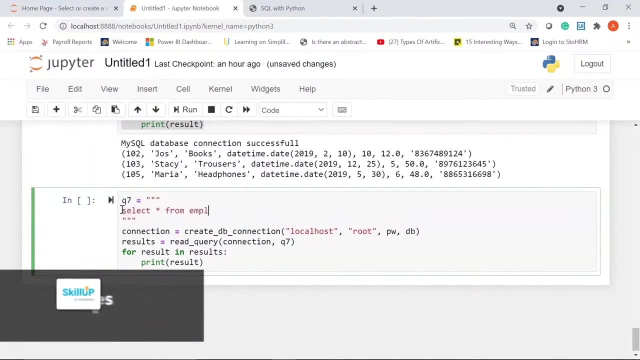 let's say you want to display all the columns from the table, so i'll write select star from orders. then i'm going to use order by unit price. i'll give a semicolon. let's run this query and see the output. if you see the result here. 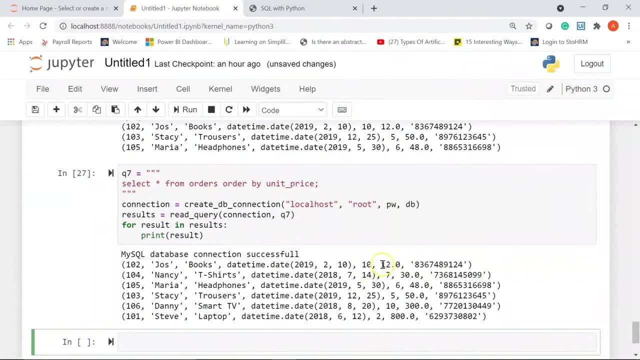 and you mark the unit price column. the result has been ordered in ascending order of unit price. you see, here it starts with the lowest price and then goes on with the highest price towards the end. now, if you want to order it in descending order, you can use the keyword desc. 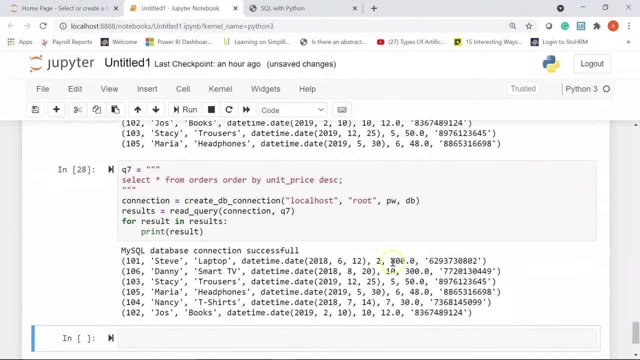 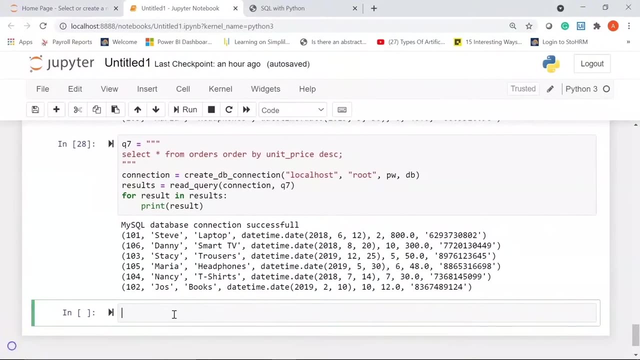 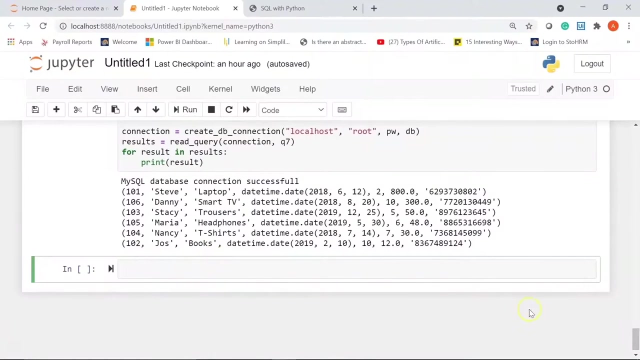 so this will ensure your top or the most expensive products appear at the top and the least expensive products appear at the bottom. alright, next now let's see how you can create a data frame from the given table. so, as you know, using jupiter notebook and pandas, you can. 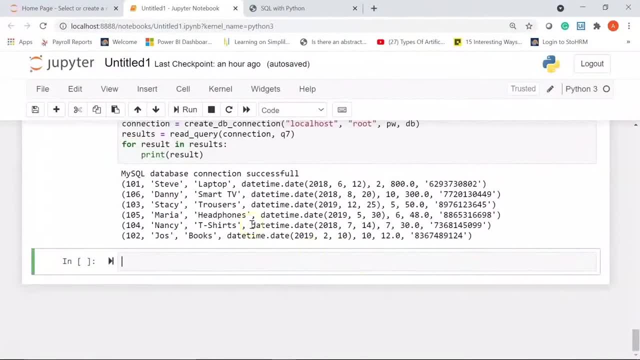 create data frames and work on it very easily. so with this table also, we can create our own data frame. so for that, let me create an empty list. first i'll write from db equal to. i'll assign this as an empty list. so we are going to return a. 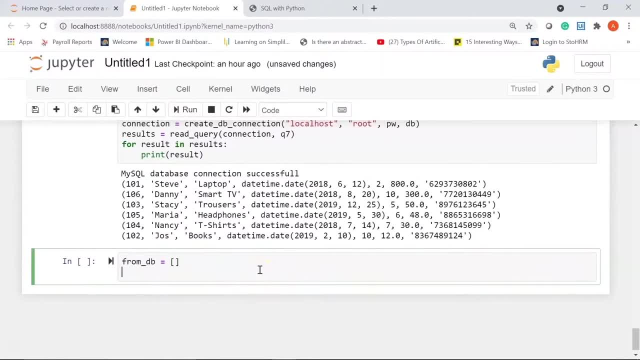 list of lists and then create a pandas data frame. next i'll write my for loop. i'll write for result in results. i'll assign result to list of results. so i'm converting the result into a list and then i'm going to append it to the 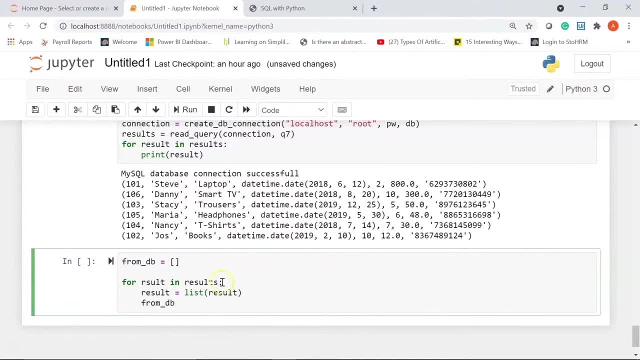 empty variable or the empty list which is from underscore db dot append. i'll append the result to my empty list. next we need to pass in the columns. now that will be part of our data frame, so i'll write columns equal to this column. i'll pass it. 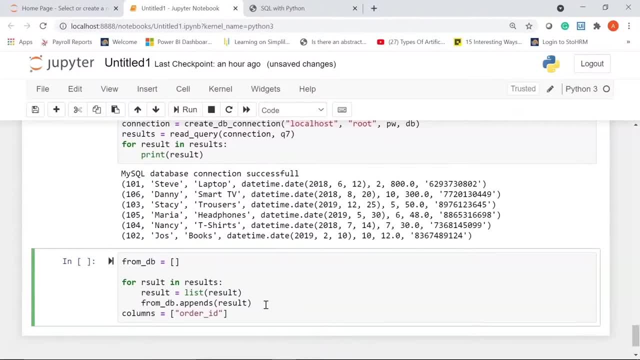 within a list. so i'll give my first column as order id, then we have the customer name. next i have my product name, then i have the date on which it was ordered. give a comma, then we'll have the quantity column. let me write it in the next line. 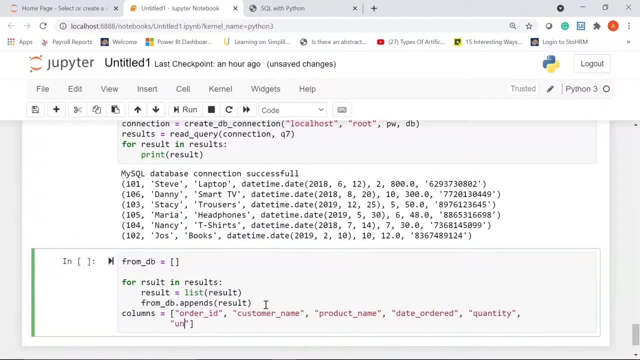 next we have the unit price column and finally we have the phone number column. so i'll write within double quotes phone number and this. we are going to assign it to a data frame. so i'll be using pd dot data frame, which is my function, to convert a list into a 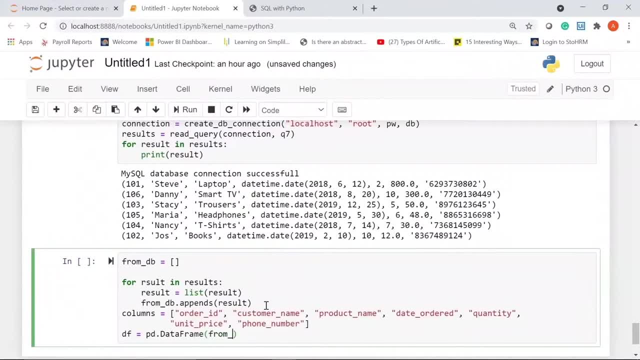 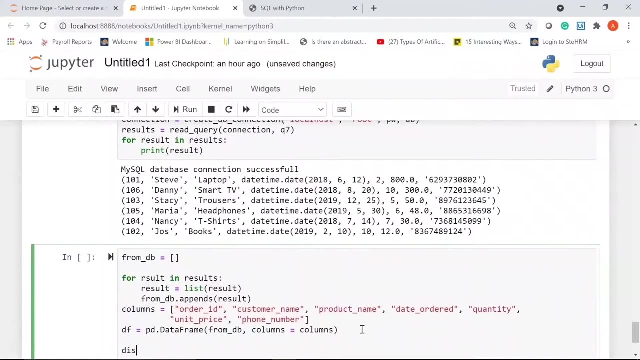 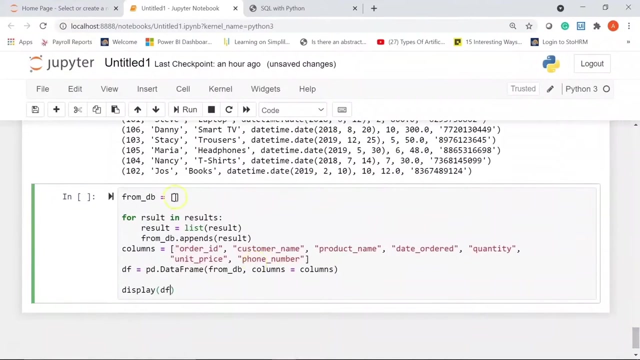 data frame. my variable i'm going to pass is from underscore db and i'll write: my next argument is columns, equal to my variable name, that is columns. finally, let's display the data frame, which is df. alright, so here i'm creating a empty list first and then 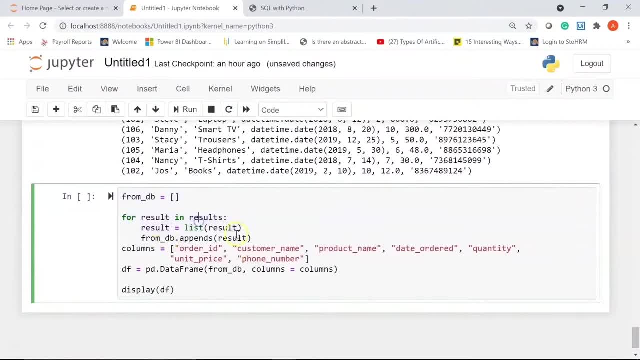 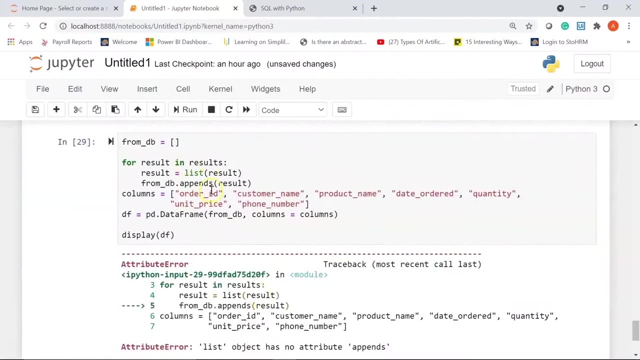 i'm creating a for loop and i'm appending the results to my empty list. here you can see i have created my column list and using pd dot data frame, i'm converting the list into a data frame for run. this. this is append and not appends. 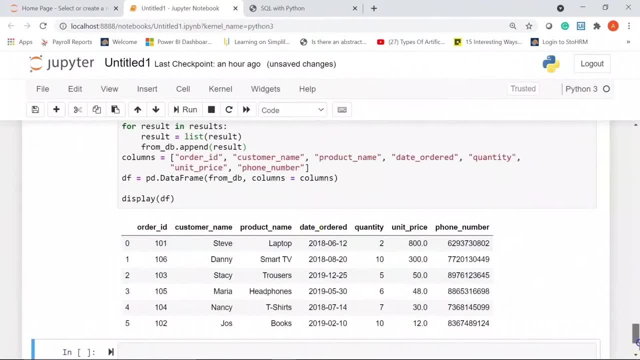 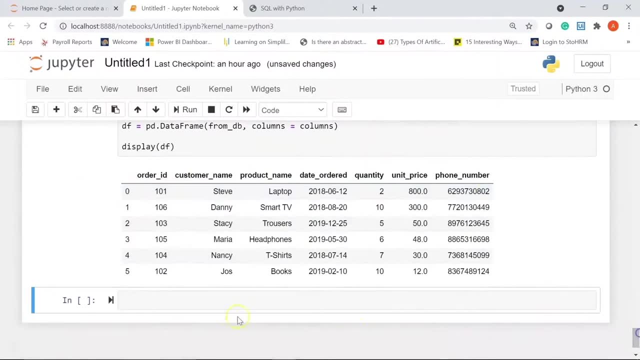 alright, you can see we have our data frame ready. this is the index column. it starts from 0 onwards and then we have the different columns. ok, now let's see how to use the update command button fingerprint. do i have to take them all out, or suppose? 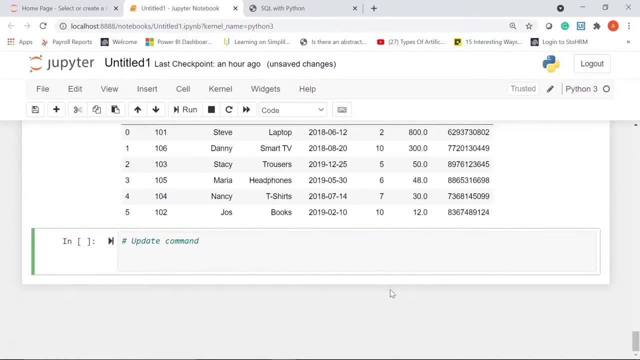 you want to change the unit price of one of the orders, you can use the update command. so the way to do it, i'll first create my variable, let's say update, and i'll give three quotes or triple quotes. then i'll use my update command, which is: 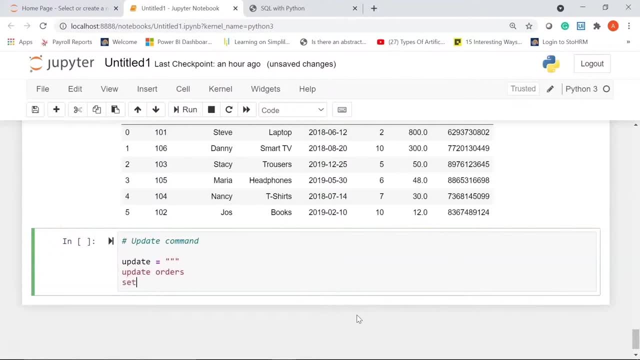 update, followed by the table name, that is, orders. next i'll write set, let's say, unit underscore price. if you see this. let's say i want to set the unit price of trousers from 50 dollars to, let's say, 45 dollars. i want to update this particular record. 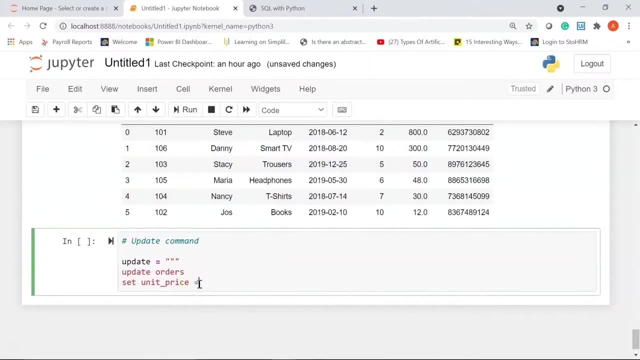 so i'm going to write: set unit price column equal to 45 dollars where the order id equal to 103. so this query will update the third row in our table, which is order id 103, so it will update from 50 dollars to 45 dollars. 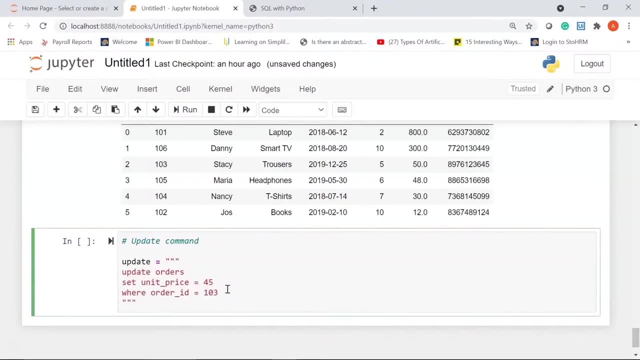 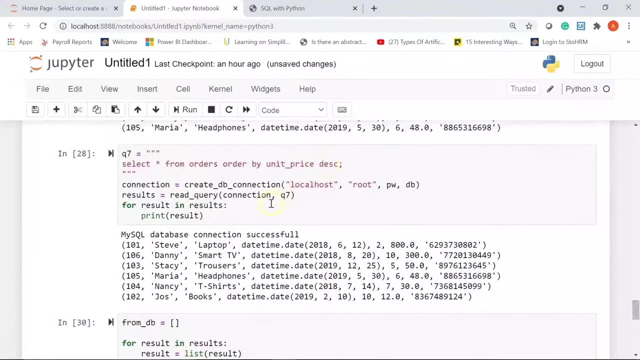 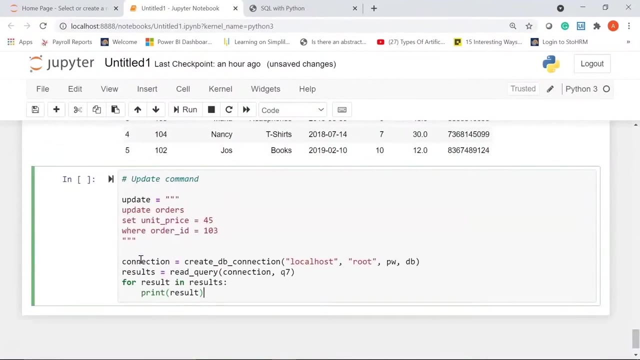 i'll close the triple quotes and now i'll use the connection queries again. let me just paste it here. all right, i'll delete these three lines of code and instead of that i'll put execute underscore query and this will take into parameters, as always, which is going to be connection followed. 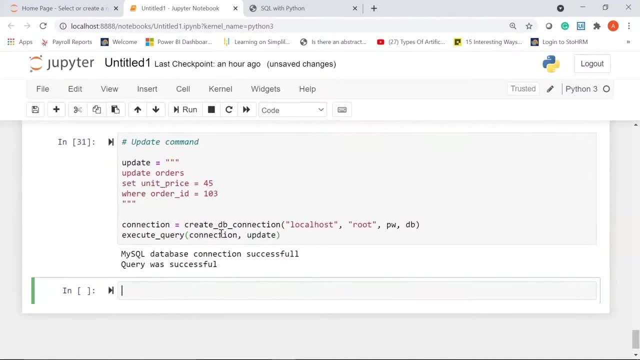 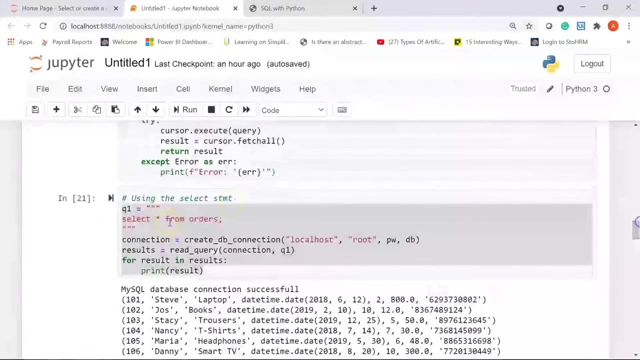 by the variable name. that is update. let's run it. you see, here it says my sql database connection successful query was successful. now you can check that. to do it, let me just go to the top and we'll just copy our first query, which is q1. i'll 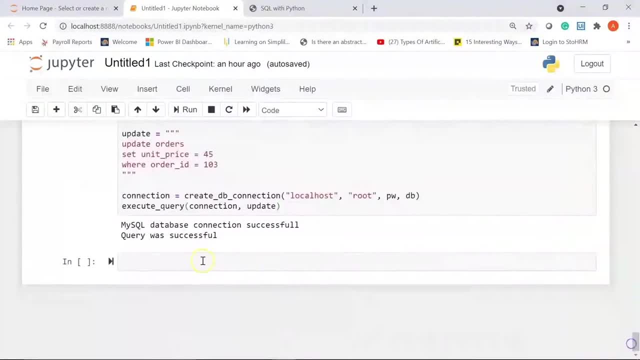 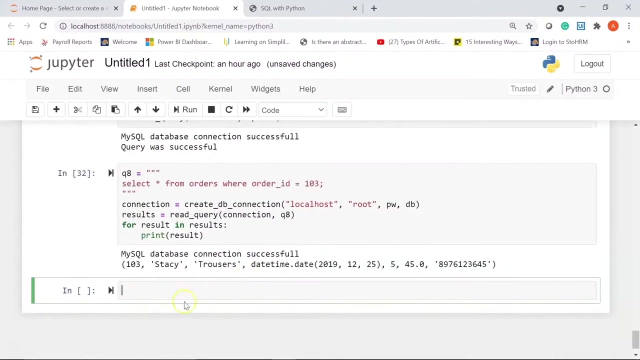 copy this and i'll paste it here. let me just rename this now. this will be q8 and i'll change this as well. i'll write select star from orders where my order id equal to 103. let's see the unit price of 103. now you can see here. 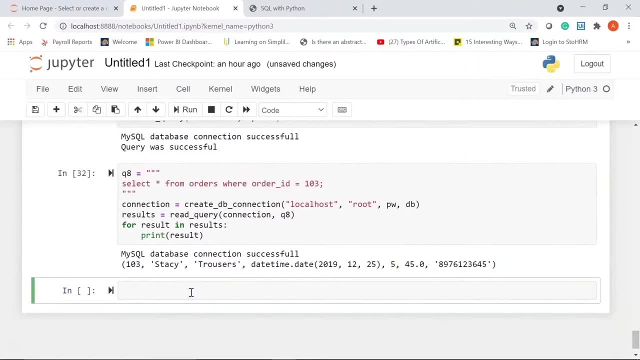 instead of 50. now we have updated it to 45 dollars. all right, now the last command we are going to say is how you can delete a record from the table. i'll write delete command as my comment. now to delete a query, i'll first give my variable. 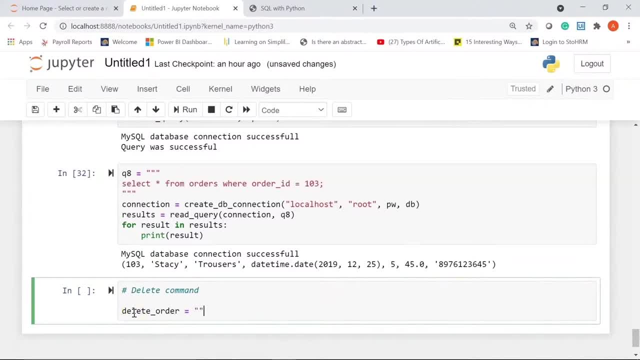 name, which is delete, underscore order, and i'll pass in within triple quotes. next i'll write my delete query, which is delete from my table name, that is orders. then i'll give my where clause where let's say, i want to delete my order id 105. 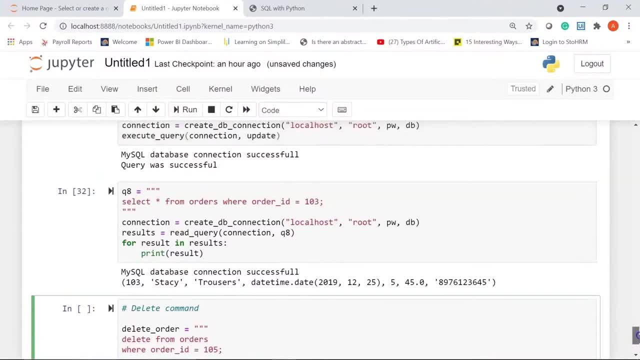 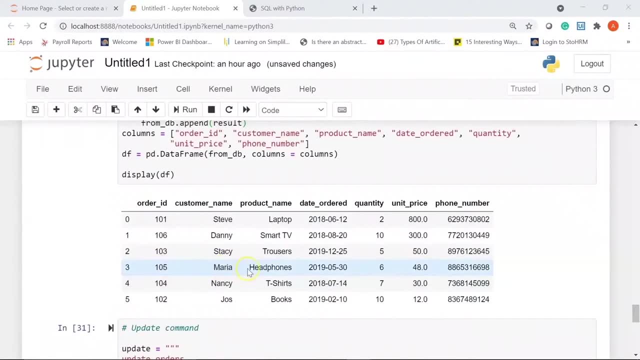 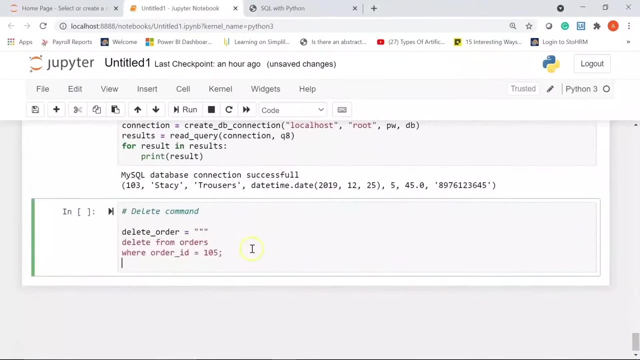 let me just go to the top and explain you again. so if you see this, we want to delete the order id 105 which was for customer name maria and she had ordered headphones. we want to completely remove this particular record. so i have my delete query ready. 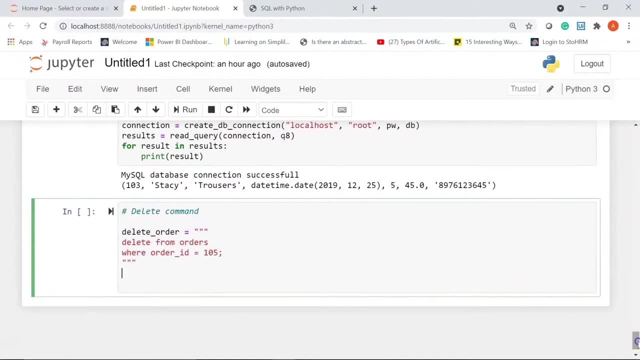 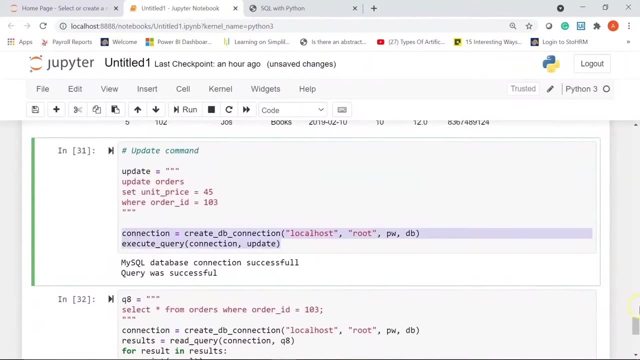 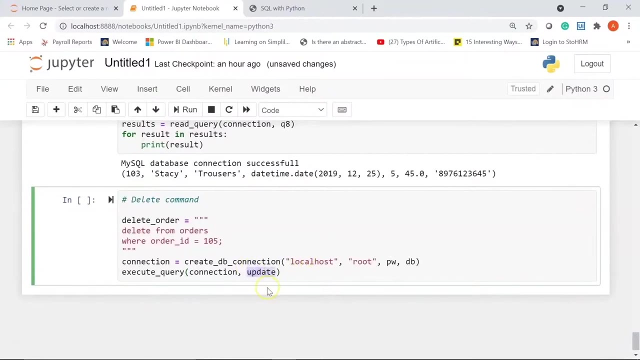 now let me just create my connection and display the results. so i'll go to the top and i'll copy this connection command, which also has the execute query command, and i'll paste it here and i'm going to make a change here. instead of update, we'll write: delete underscore. 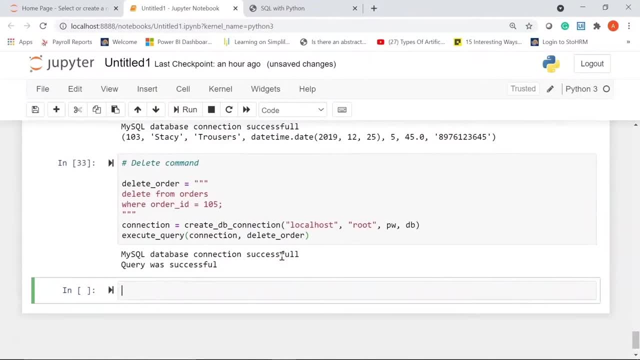 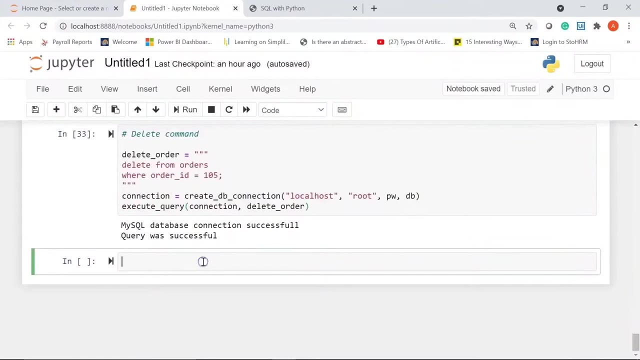 order. everything looks good. let's just run it. you can see our query was successful and now, if you want to print it, let me just show you. i'll just copy this. we'll paste it here. i'll make this as q9. i want to verify if my order id 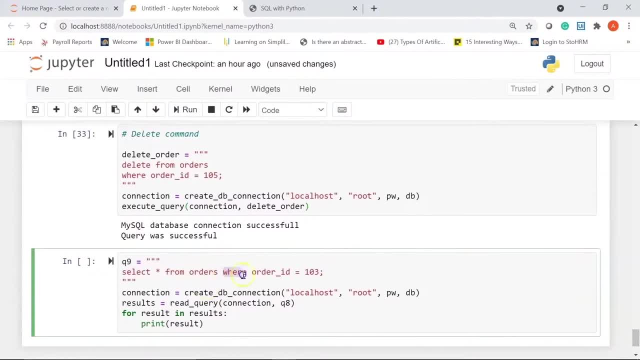 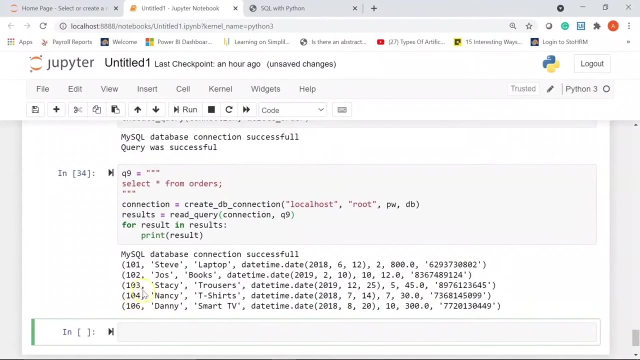 105 was deleted or not. instead of this statement, i'll write select star from orders and here i'll change this to q9. if i run this, you can see it. here you can mark order id 105 was deleted and it no more appears in this. 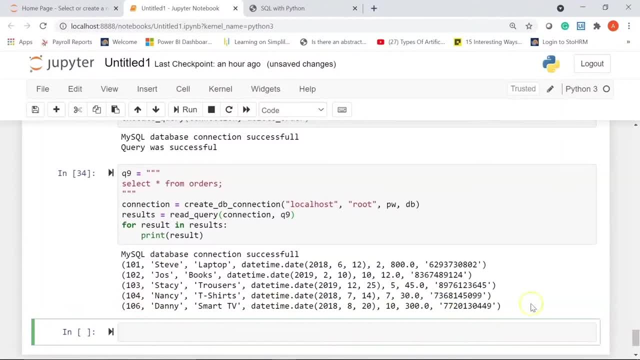 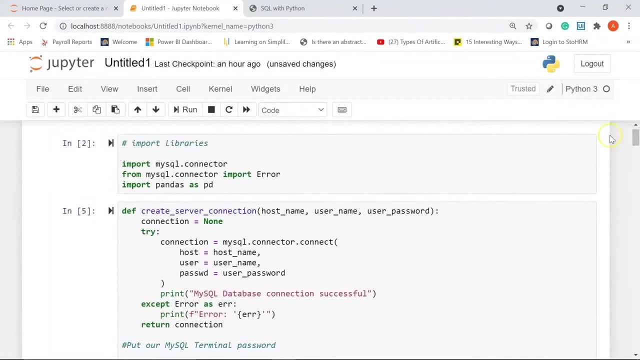 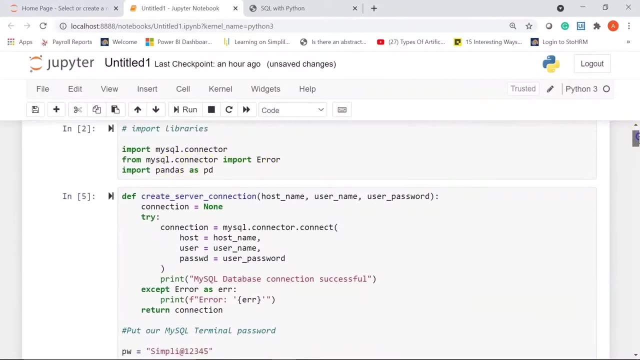 table. alright, so this brings us to the end of the demo session on sql with python. let me just scroll you through what we did. so first we imported the important libraries, mysql connector, then we imported the error function. then we imported pandas. using pd, we learnt how to create a. 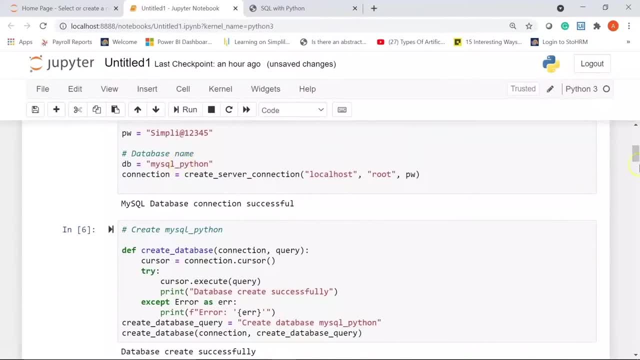 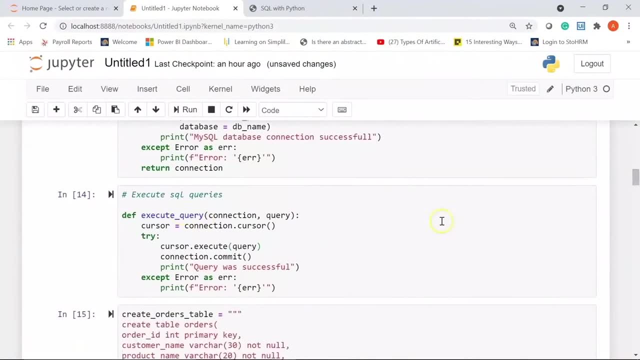 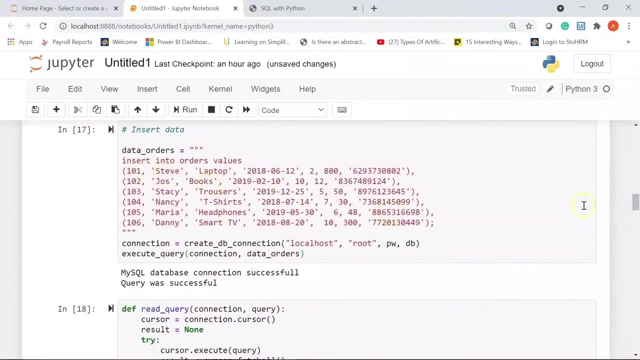 server connection to mysql database. we created a new database that is mysql, underscore, python, and now we connected to that database. we created a function to execute our queries. we saw how you can write create table command. then we inserted a few records to our orders table. we created. 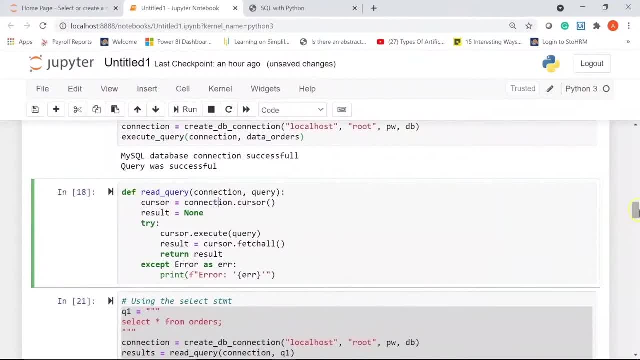 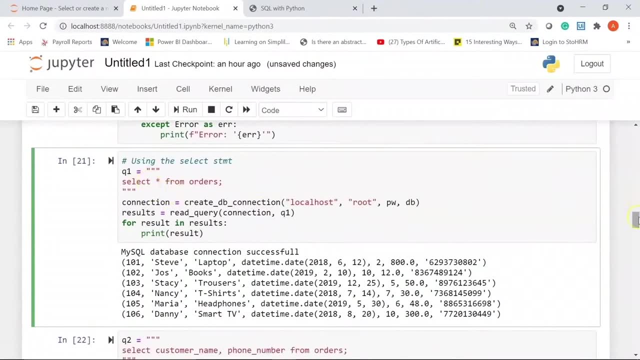 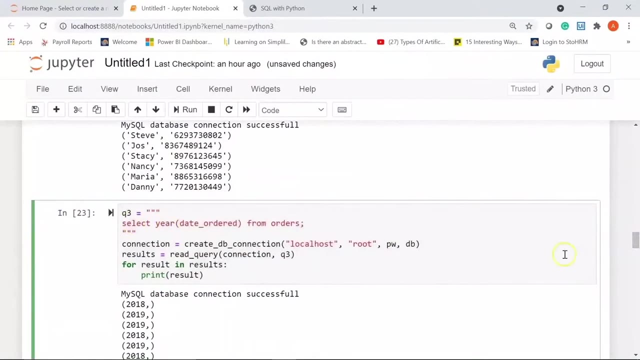 a read underscore query command to read the queries and display the results. then we started exploring our different sql commands, one by one. we saw how to use select query. then we selected a few individual columns from our table, followed by using a inbuilt function, which was year. then we saw how to use 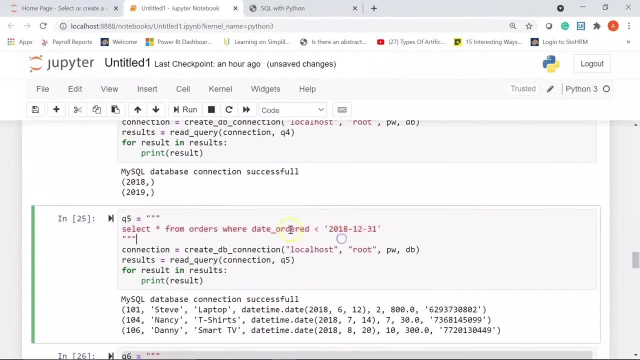 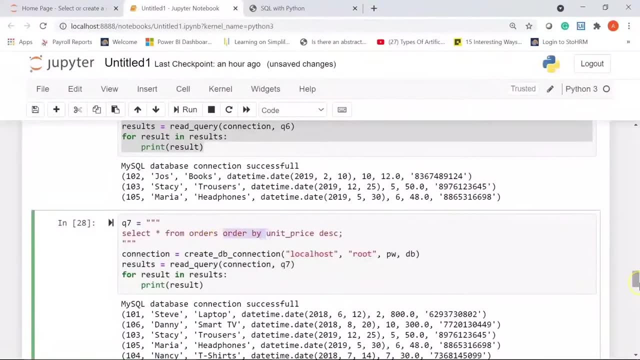 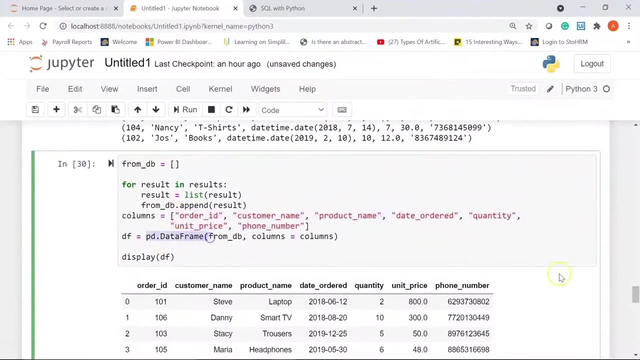 the distinct keyword. after that, we used our where clause to filter our table based on specific conditions. we saw how to order your results based on a particular column. then we saw how you could convert the table into a data frame using pd dot data frame function. finally, we learned 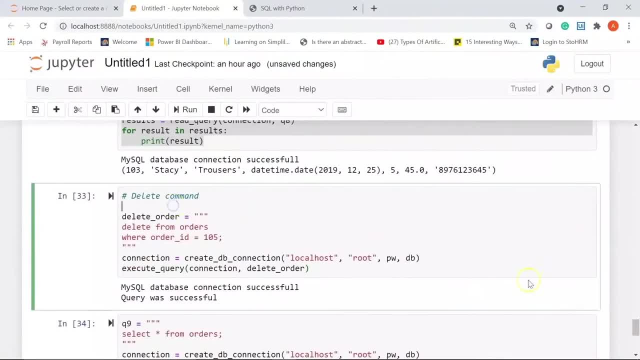 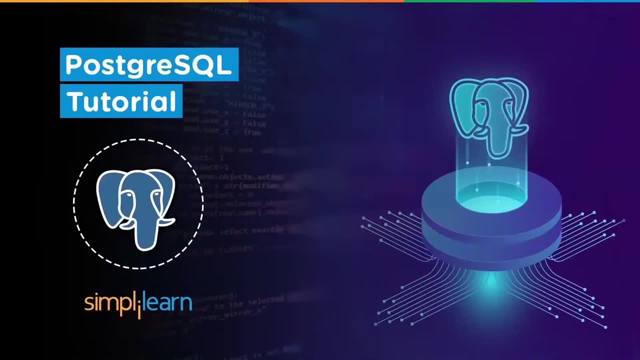 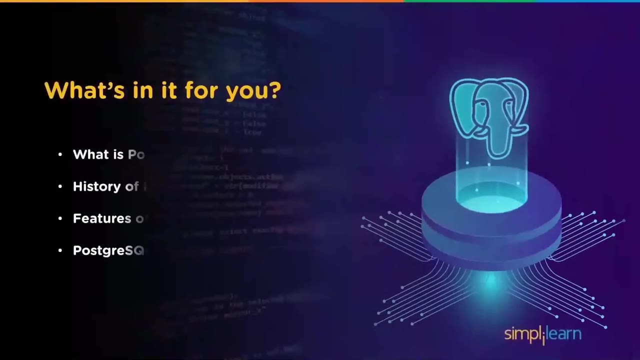 how to use the update command and the delete command. postgres sql is a very popular and widely used database in the industries. in this tutorial we will learn postgres sql, or postgres sql, in detail with an extensive demo session. so in today's video we will learn what postgres sql is. 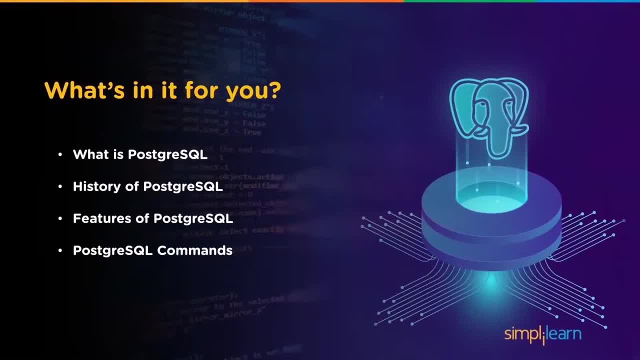 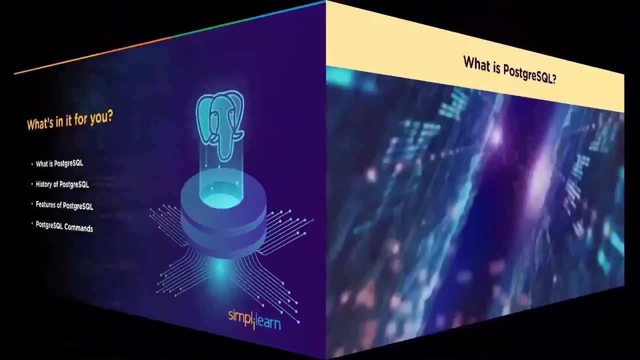 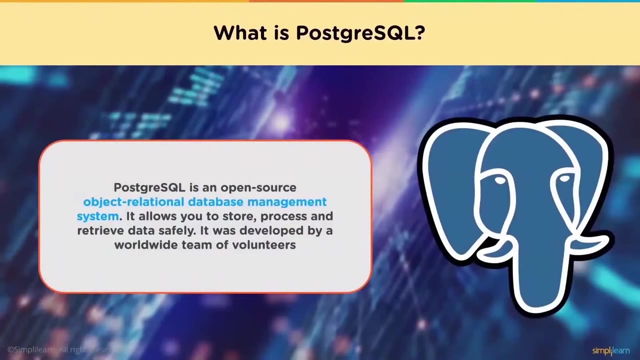 and look at the history of postgres sql. we will learn the features of postgres sql and jump into performing postgres sql commands on the sql cell and pgadmin. so let's begin by understanding what is postgres sql. postgres sql is an open source object: relational database management system. it stores data in. 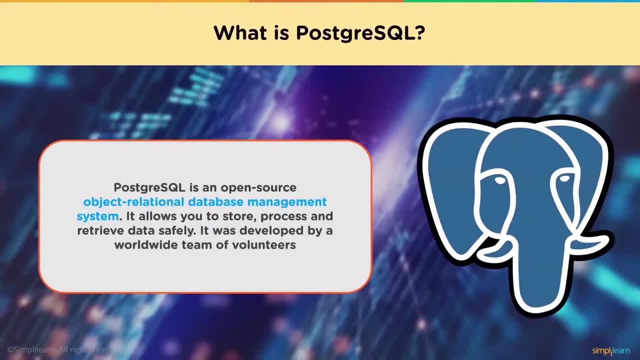 rows with columns as different data attributes. according to the db engines ranking, postgres sql is currently ranked 4th in popularity amongst hundreds of databases worldwide. it allows you to store, process and retrieve data safely. it was developed by a worldwide team of volunteers. now let's look at the history of postgres sql. 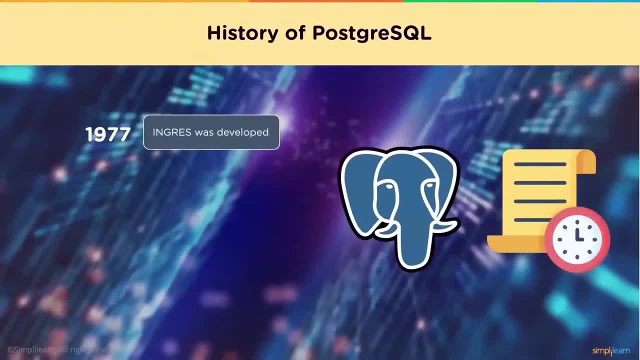 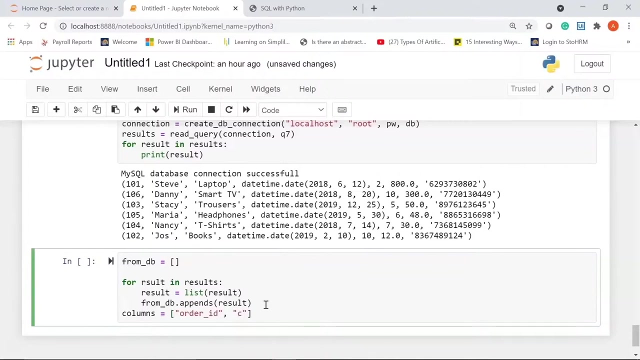 so in 1977 onwards, the ingress project was developed at the university of california, berkeley. in 1986 the postgres project was led by professor michael stonebreaker. in 1987 the first demo version was released and in 1994 a sql interpreter was introduced to postgres. 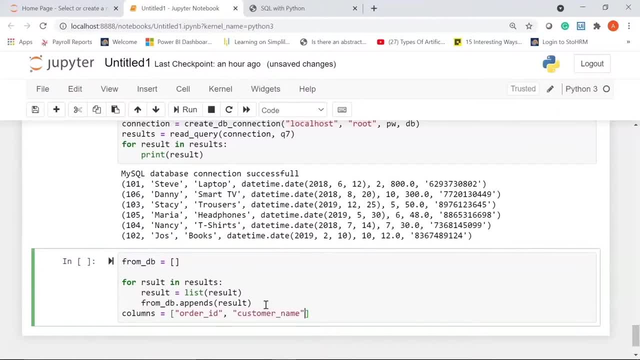 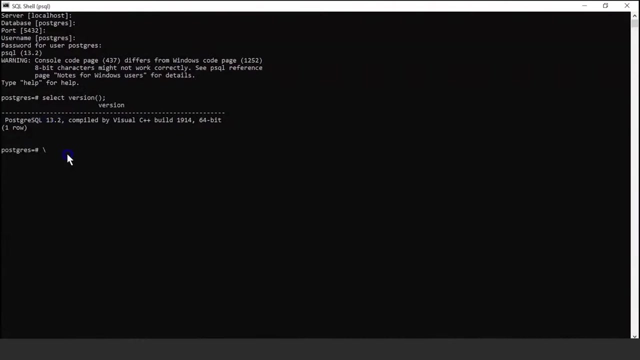 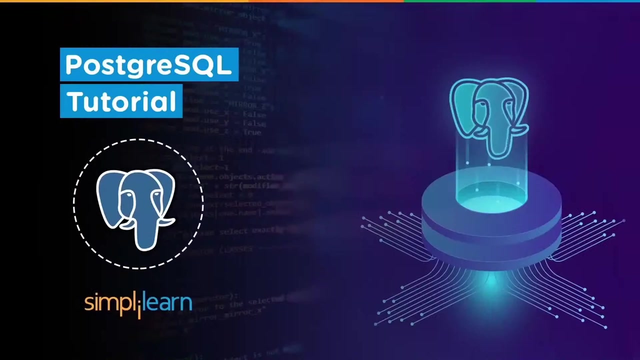 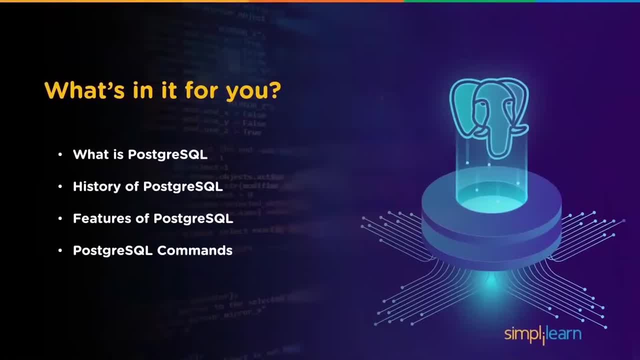 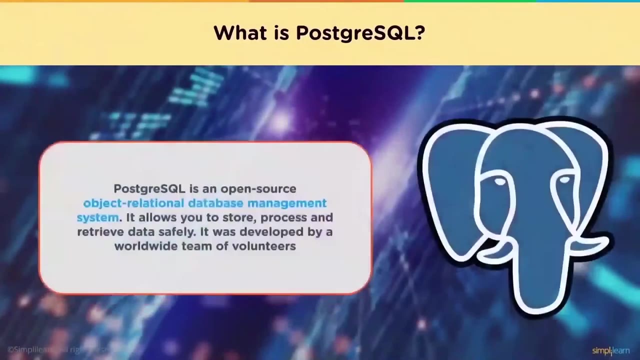 So in today's video we will learn what Postgres SQL is and look at the history of Postgres SQL. We will learn the features of Postgres SQL and jump into performing Postgres SQL commands on the SQL cell and PG admin. So let's begin by understanding what is Postgres SQL. 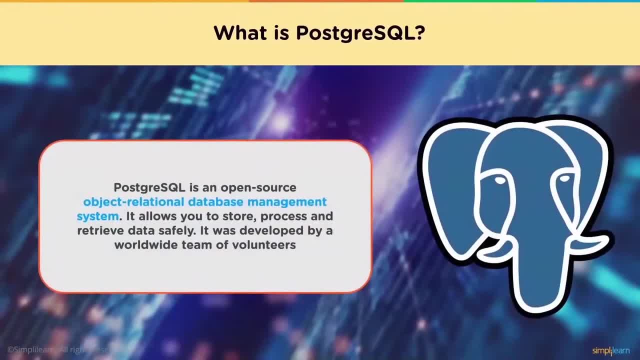 Postgres SQL is an open source object relational database management system. It stores data in rows with columns as different data attributes. According to the DB engines ranking, Postgres SQL is currently ranked fourth in popularity amongst hundreds of databases worldwide. It allows you to store, process and retrieve data safely. 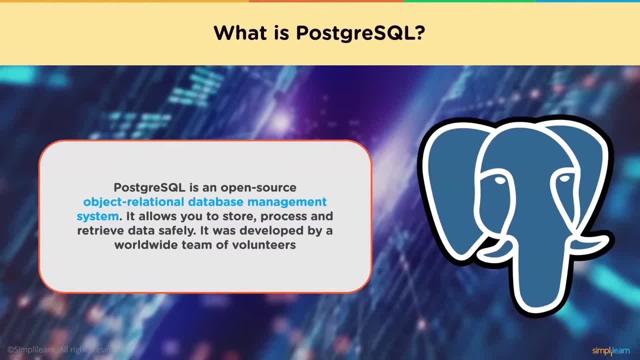 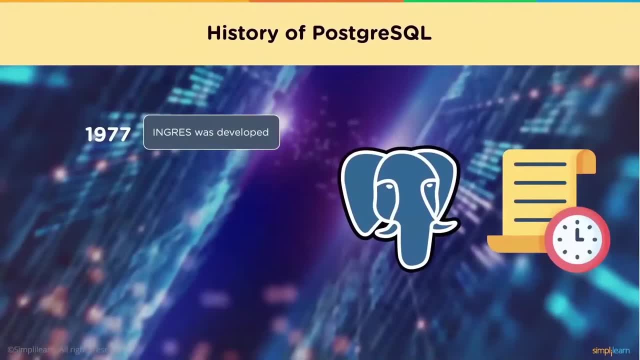 It was developed by a worldwide team of volunteers. Now let's look at the history of Postgres SQL. So in 1977 onwards, the Ingress project was developed at the University of California, Berkeley. In 1986,, the Postgres project was led by Professor Michael Stonebreaker. 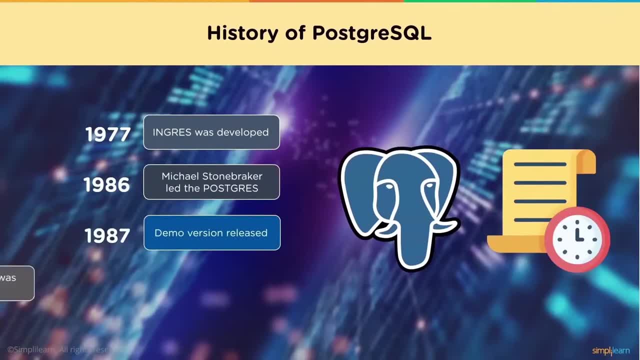 In 1987, the first demo version was released And in 1994, a SQL interpreter was added. Postgres SQL was developed by a team of volunteers. Postgres SQL was developed by a team of volunteers. The first Postgres SQL release was known as version 6.0 or 6.0, on January 29, 1997.. 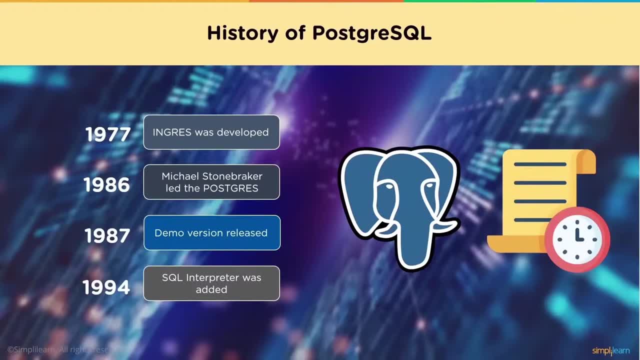 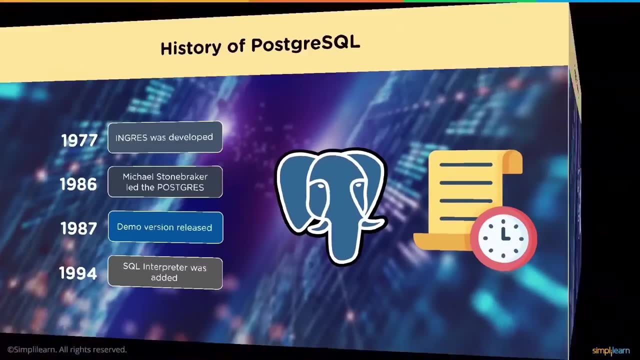 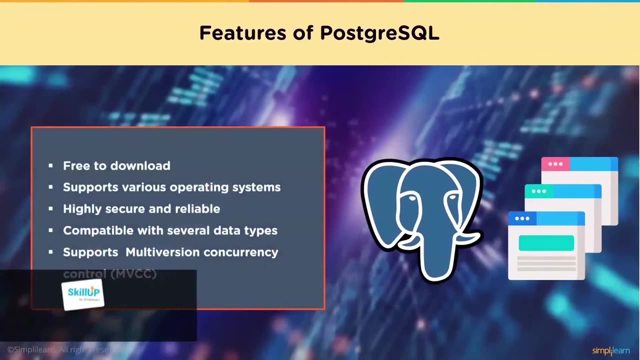 And since then, Postgres SQL has continued to be developed by the Postgres SQL Global Development Group, a diverse group of companies and many thousands of individual contributors. Now let's look at some of the important features of Postgres SQL. So Postgres SQL is the world's most advanced open source database and is free to download. 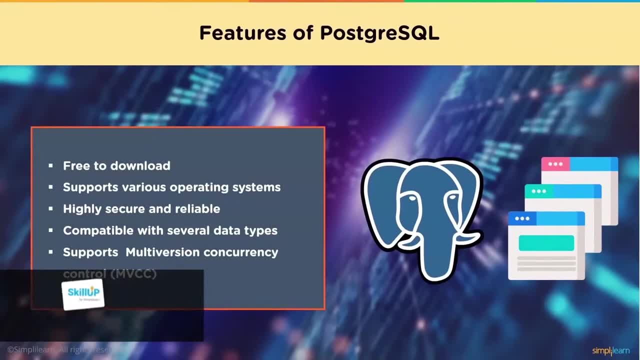 It is compatible, as it supports multiple operating systems such as Windows, Linux and Mac OS. It is highly secure, robust and reliable. Postgres SQL supports multiple programming interfaces, such as C, C++, Java and Python. Postgres SQL is compatible with various data types. 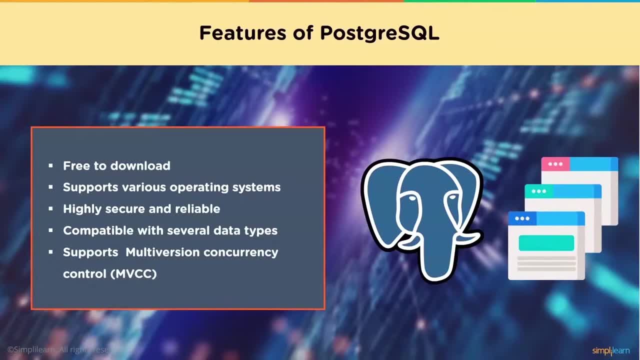 It can work with primitives like integers, numeric string and Boolean. It supports structured data types such as datetime, array and range. It can also work with documents such as JSON and XML. It is compatible with multiple operating systems such as Windows, Linux and Mac OS. 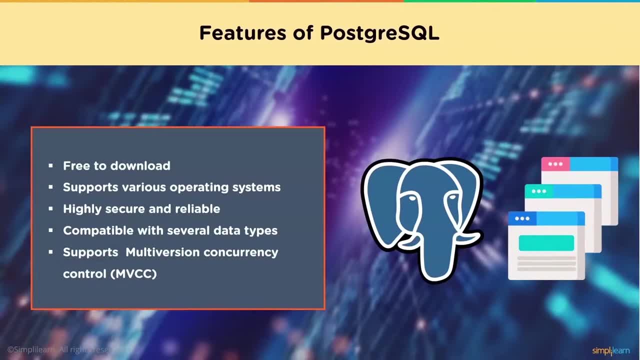 It can also work with multiple operating systems such as C, C++, Java and Mac OS. It can also work with multiple operating systems such as JSON and XML. And, finally, Postgres SQL supports multi-version concurrency control, or MVCC. Now, with this theory knowledge, let's look at the Postgres SQL commands that we will. 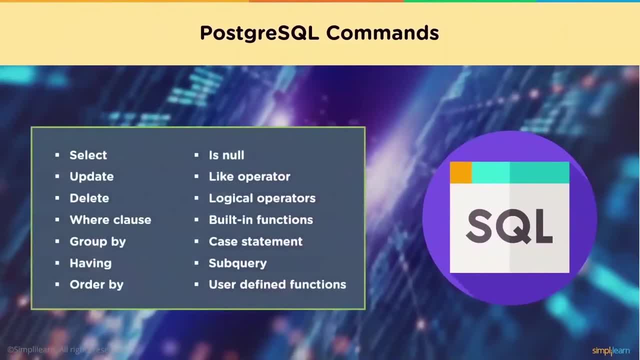 be covering in the demo, So we will start with the basic commands, such as SELECT, UPDATE and DELETE. We will learn how to filter data using WHERE clause and having clause in SQL. We will also look at how to group data using the GROUP BY clause and order the result using 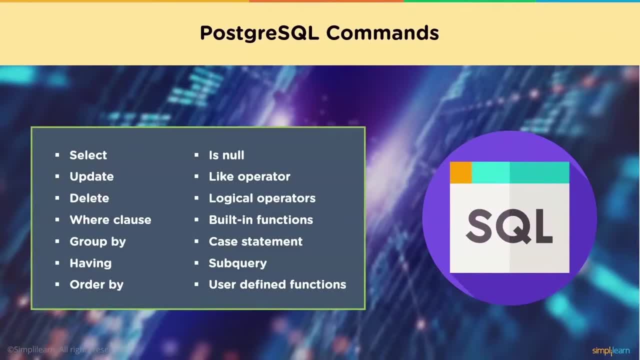 the ORDER BY clause, You will learn how to deal with NULL values. You will learn how to filter data using NULL values. You will learn how to filter data using NULL values. You will learn how to filter data using NULL values. get an idea about that LIKE operator and logical operator such as AND OR. 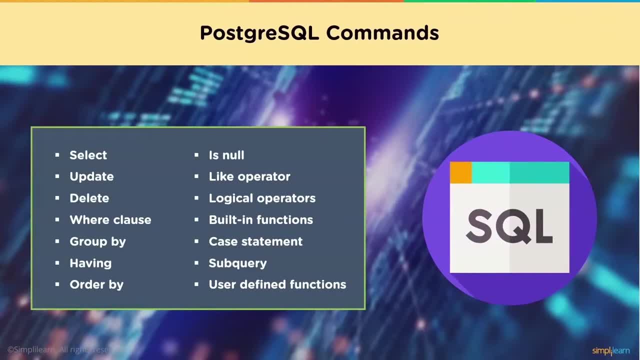 We will also explore some of the popular inbuilt mathematical and string functions. Finally, we will see some of the advanced concepts in Postgres SQL, that is, to write case statements, subquery and user defined function. So let's head to the demo. 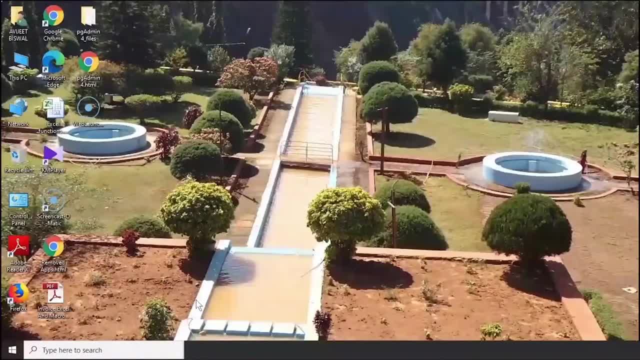 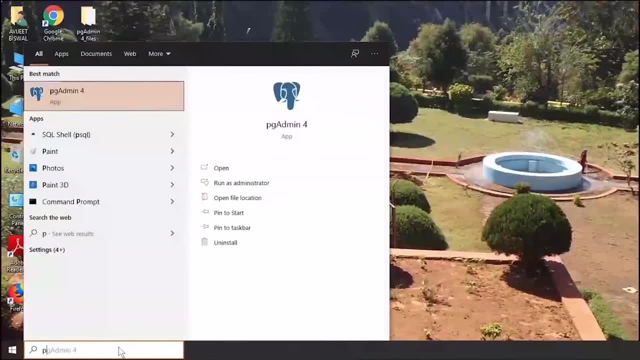 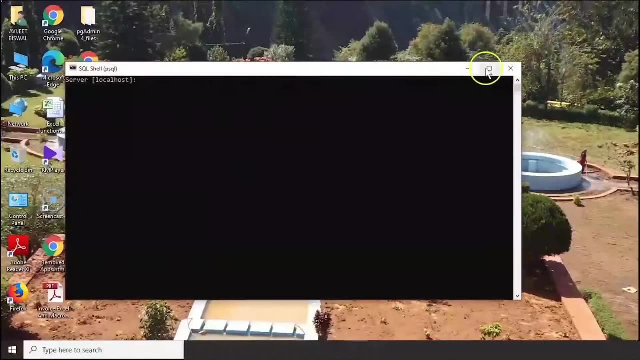 OK, so let's now start with our demo. First We will connect to Postgres SQL using psqlcell. So here Under here to search, i'll search for psql. you can see this is the sql cell. i'll click on open. let me maximize this. okay, so for server, i'll just click enter database. i'll click enter. 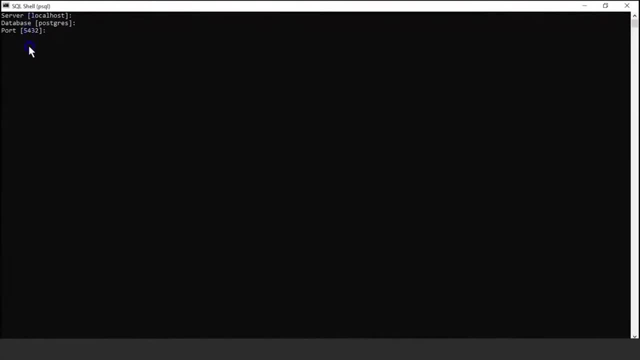 port number is already taken, which is 5432. i'll hit enter. username is already given and now it is going to ask for password. so here i'll give my password so that i can connect to my post chris sql database. so it has given us a warning, but we have successfully connected to post chris. 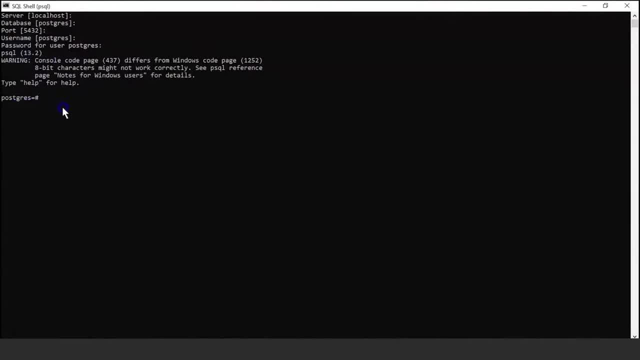 sql. all right, so now to check if everything is fine, you can just run a simple command to check the version of post chris sql that we have loaded. so the command is select version with two brackets and a semicolon. i'll hit enter. okay, you can see the version post chris sql 13.2. okay, 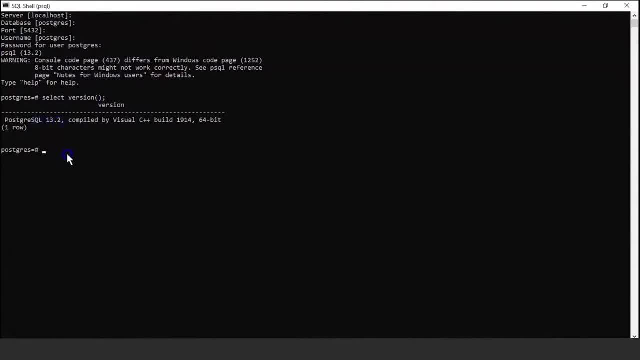 so now let me show you the command that will help you display all the databases that are already there. so if i hit slash l and hit enter, it will give me the list of databases that are already there. so we have post chris sql, there's something called template 0, template 1 and we have a 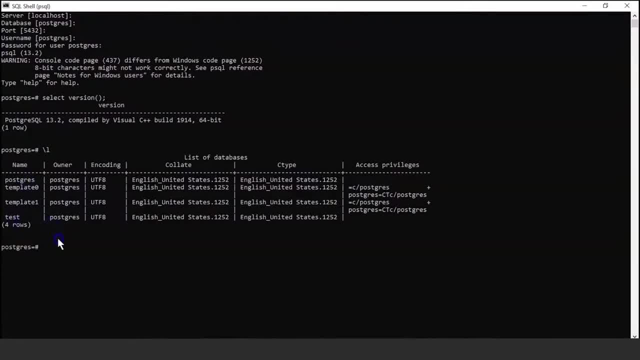 test database as well. okay, now for our demo. i'll create a new database. so first i'll write create space database and i'll give my database name as sql underscore demo. i'll give a semicolon and hit enter. you see we have a message here that says create database. so we successfully created our sql demo. 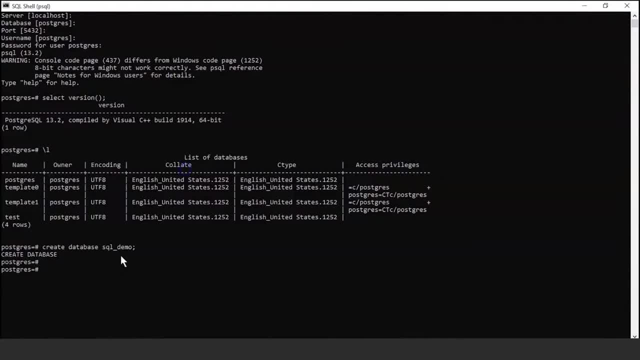 database. now if you want to connect to that database you can use backslash c space sql underscore demo- sql demo database. there you go. it says you are now connected to database sql underscore demo. so here we can now create tables. we can perform insert operation, select operation, update, delete, alter and much. 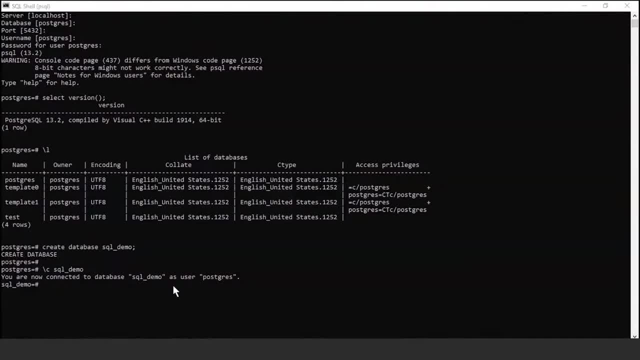 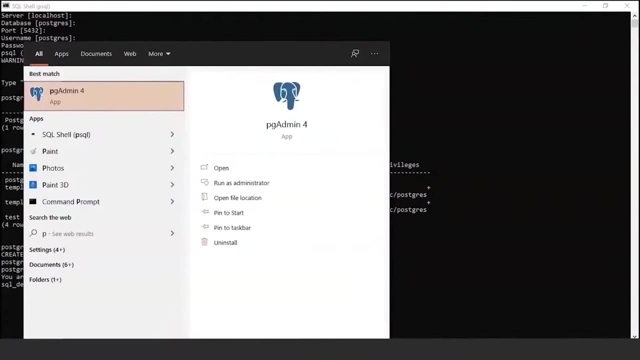 more. now i'll show you how to connect to postgres sql using pg admin. so when you install the postgres sql database you will get the sql cell and along with that you also have the pg admin. so i'll just search for pg. you can see here it has prompted pg admin. i'll click on open. 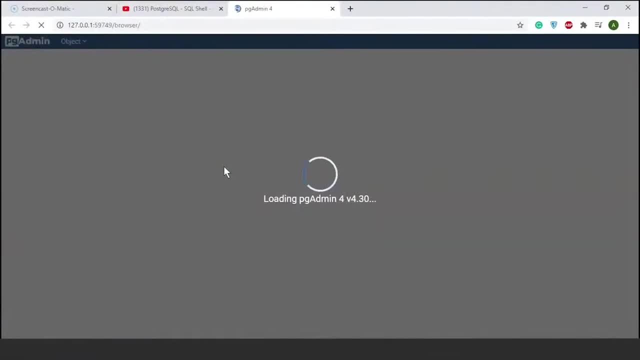 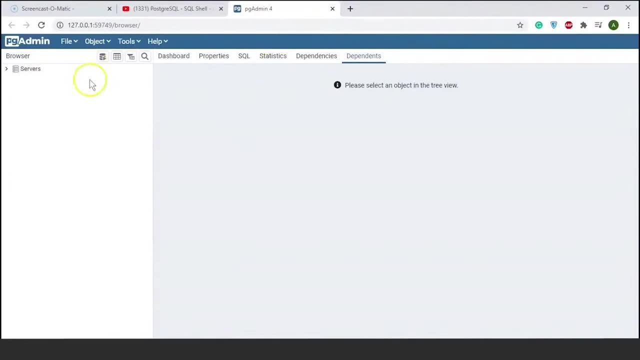 this will open on a web browser. you can see it has opened on chrome and this is how the interface of pg admin looks like. it is a very basic interface. so on the top you can see the files. we have object, there's tools and we have the help section as well, and here you have dashboard properties, sql statistics. 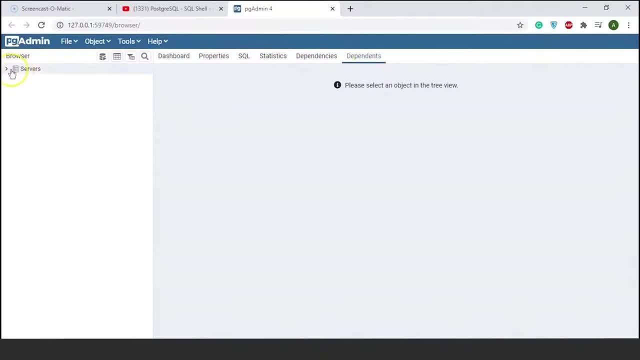 and you can see the file is in the same place. and here you have the dashboard properties. and here you have the dashboard properties, sql statistics. and here you have the script afections, dependencies, dependence. and here on the left panel you have servers. let me just expand this, so it 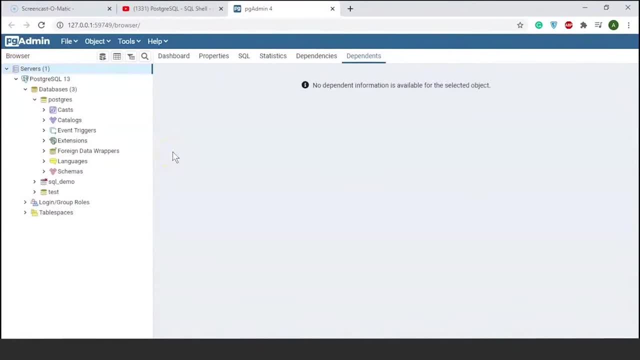 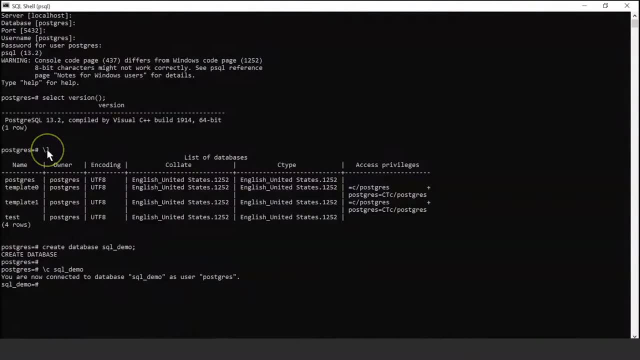 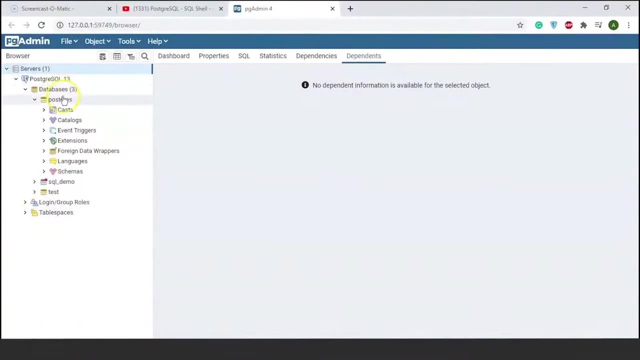 will connect to one of the databases. all right. so if i go back, you see, when i had run backslash l to display the databases, it had shown me postgres sql and test. now you can see, here we have the postgres sql database and the test database. all right, now we also created one. 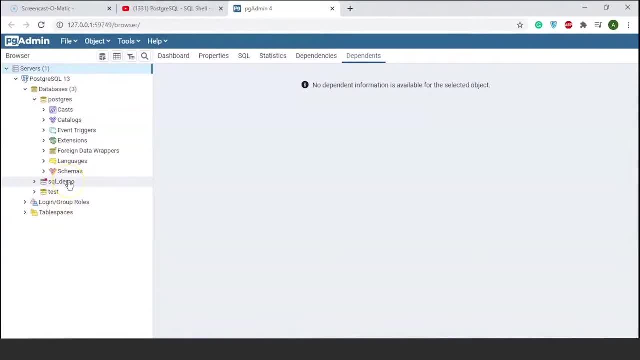 more database, which was sql demo. so let me show you how to work on this pg admin and the query tool. all right, so i'll right click on sql demo and i'll select query tool. i'll just show you how to run a few commands on the query tool. 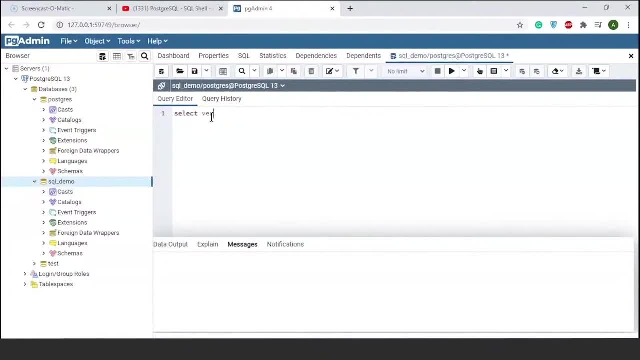 so let's say you want to see the version of postgres sql that you are using, so you can use the same command that we did on psql cell, which is select version, closed with brackets and a semicolon. i'll select this and here you can see we have the execute button. so if i hit execute or 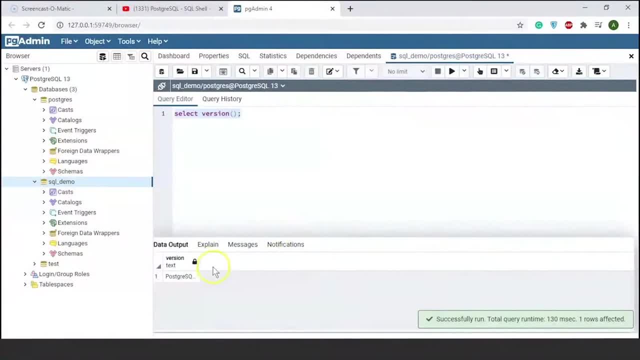 press f5, it will run that query. you can see we have the output at the bottom and it's says postgres sql 13.2, compiled by visual c++. it has a 64-bit system. okay, now let me tell you how to perform a few basic operations using postgres sql commands. so here let's say i'll. 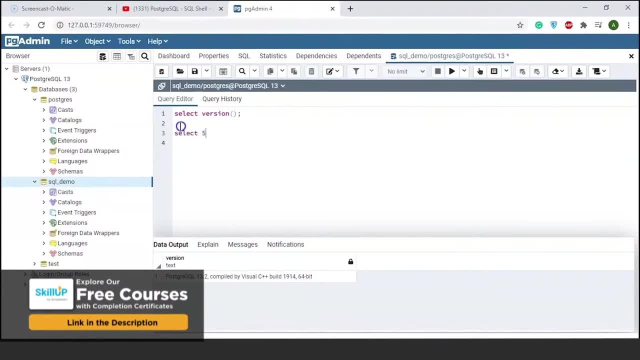 write: select 5 into 3. i'll give a semicolon, select this and hit f5. so this will run the query and it returns me the result that is, the product of 5 and 3, which is 15. similarly, let's edit this. let's say i'll write 5 plus 3 plus, let's say, 6. i'll select this and hit. 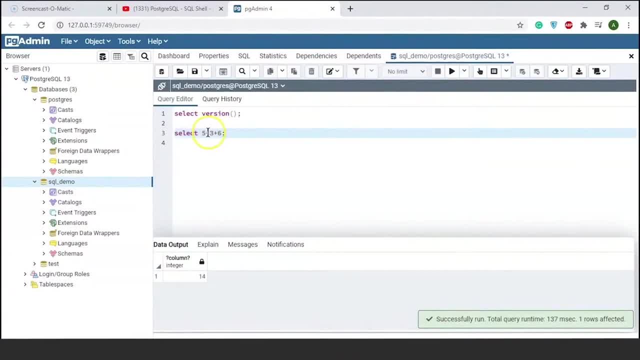 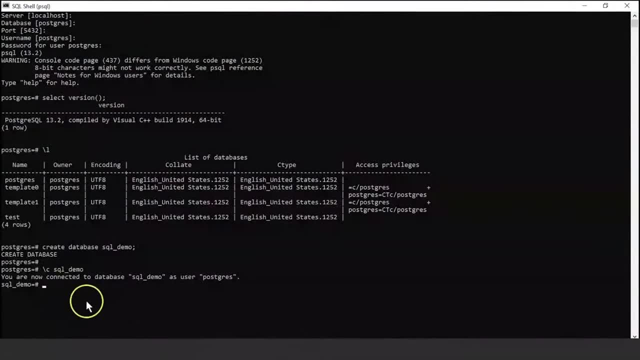 f5 to run it. it gives me the sum of 5 plus 3 plus 6, which is 14. now the same task. you can do it on this cell as well. let me show you how to do it here. so let's say i'll write select. let's say i want to multiply 7 into, let's say, 10. you know the result. 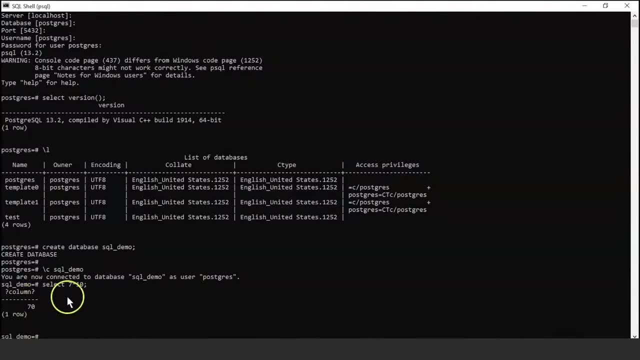 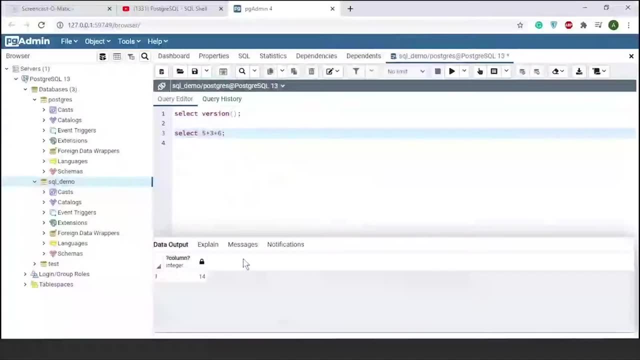 it should be 70. if i hit enter, it gives me 70. now this question mark column question word will deal with this later. all right, let me go back to my pg admin again. let me do one more operation. let's say, this time i'll write select 5. 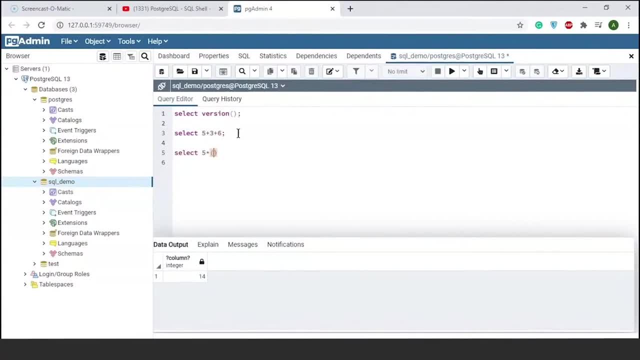 multiplied by, and within brackets i'll write 3 plus 4. i'll give a semicolon. so what sql will do is first it will evaluate the expression that is there inside the bracket, that is, 3 plus 4, which is 7, and then it will multiply 7 with 5. now let me select this and i'll hit execute. 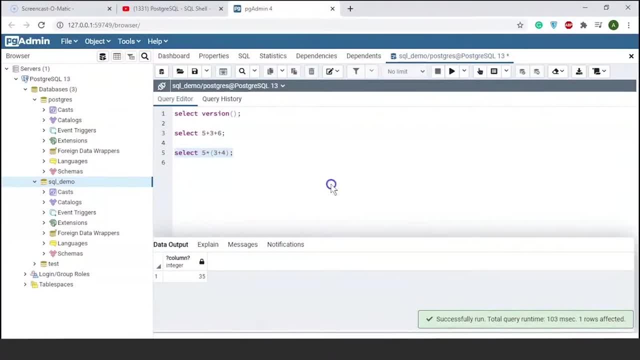 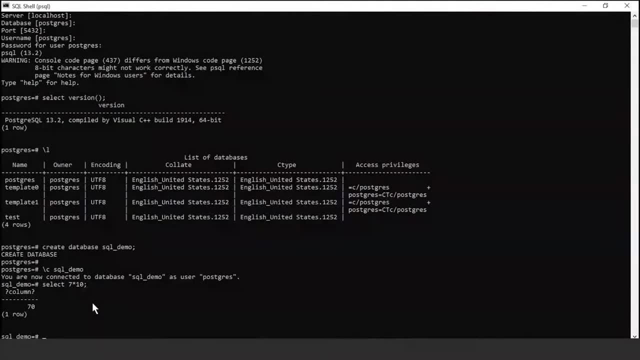 so you can see: 7 multiplied by 5 is 35. all right, now we will go back to our cell and here i'll show you how to create a table. so we are going to create a table called movies on the cell that is psql cell. so here we will learn how you can create a table. 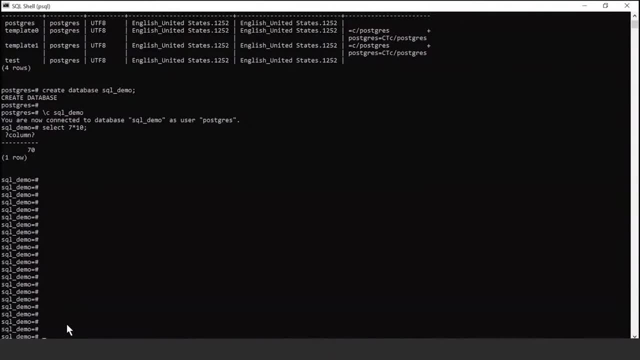 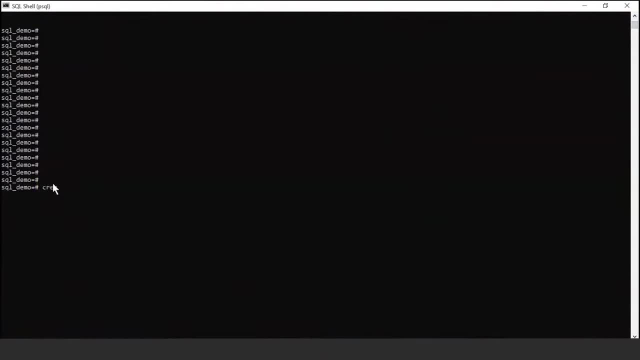 and then you can enter a few data into that table. all right, let me just scroll down a bit, okay, so my create command goes something like this, so i'll write create table by the table name, that is, movies. next my movies table will have a few columns. 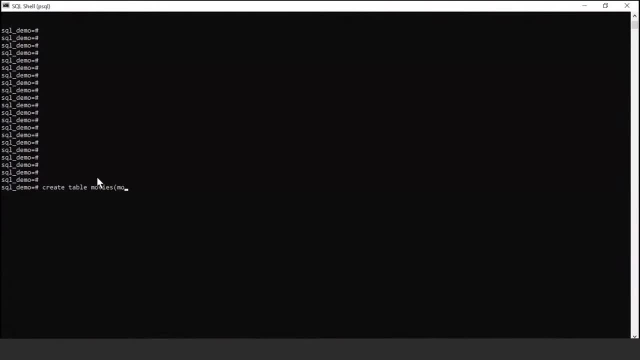 let's say I want the movie ID. after the column name we need to give the data type, so movie ID. I'll keep it as integer. so integer is one of the data types that is provided by Postgres SQL. next my second column. the table would be the name of the movie. so I'll write movie. 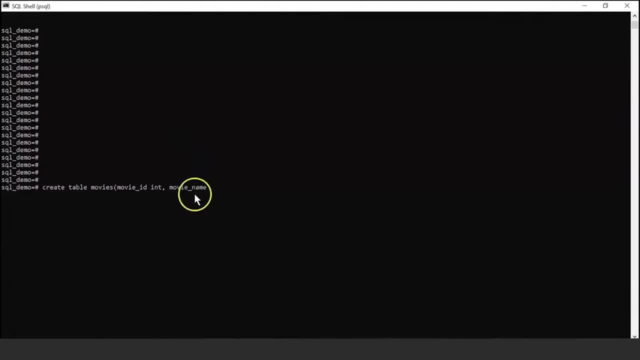 underscore name. so all the variables of the column name should be as per SQL standards. so there shouldn't be any space between the column names. so I have used underscore to make it more readable. so my movie name will be of type: var, char or variable character, varying character, and I'll give this size as 40 so that it can hold 40. 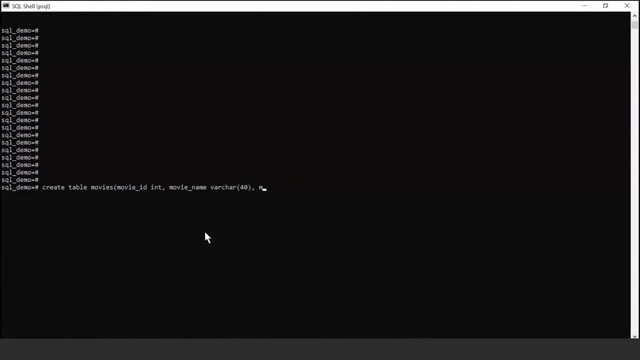 characters maximum. next, my third column will have the genre of the movie, so I'll write movie underscore, genre, again, genre is of type var, char. I'll give the size as, let's say, 30. and my final and the last column will have the IMDB rating, so I'll 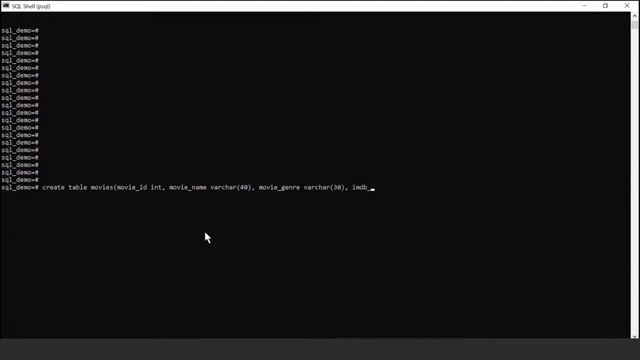 write IMDB underscore ratings. now the ratings will be of type real, since it can have floating or decimal point values. if I close, the bracket will give a semicolon and I'll hit enter. there you go. so we have successfully created a table called movies. now let me go back to my PG admin. alright, so here I have my database that. 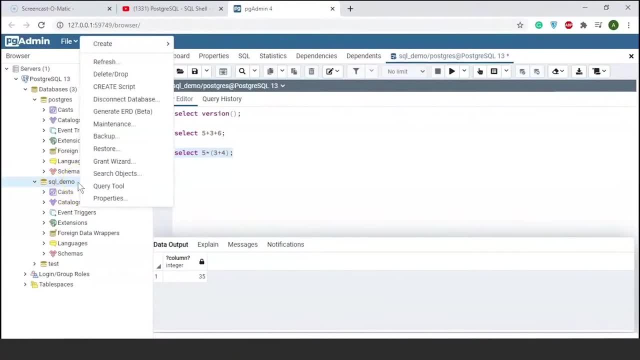 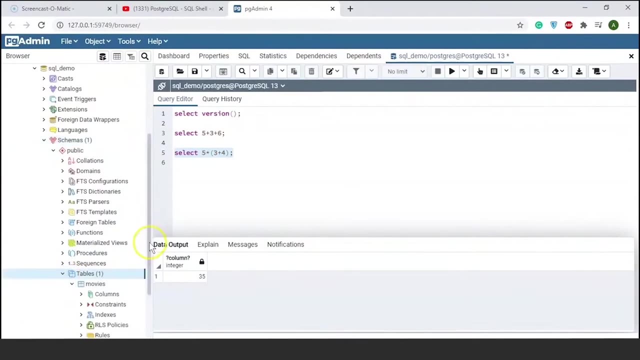 is SQL demo. I'll just right-click on this and click on refresh. now let me go to schemas. I'll just scroll down a bit here. under schemas we have something called as tables. let me expand this, okay, so you can see we have a table called movies in the SQL demo. 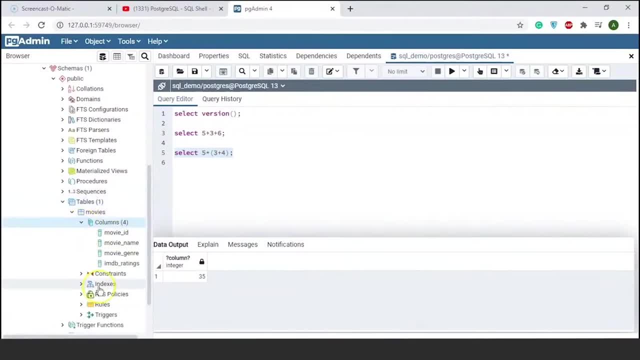 database now and here you can check the columns that we have just added so you can see the table is filled in. alright, so I'll click available. now it sayscommerce table and our table is filled in already, so it's entered somewhere. finally, the table is answered. I'll click ankle, select 등. the method is alright. we. 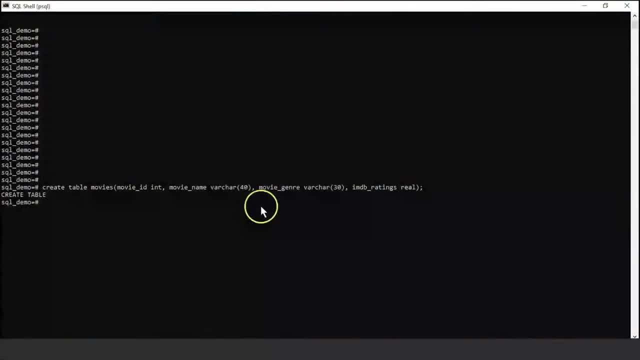 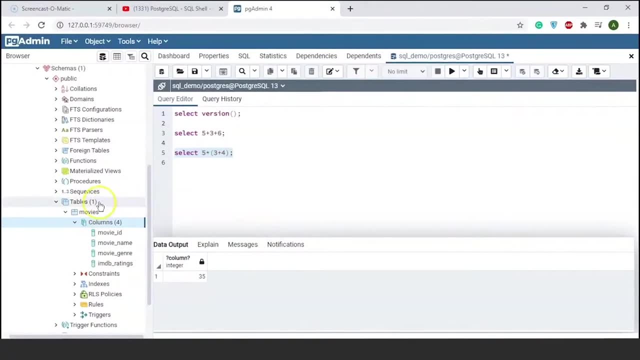 should not want an keywords search option here. let's create a table for role performances. so our movies table has movie ID, movie name, genre and ratings. all right, now there is another way to create a table. the previous time we created using the SQL cell. now I'll tell you how to create a table using the. 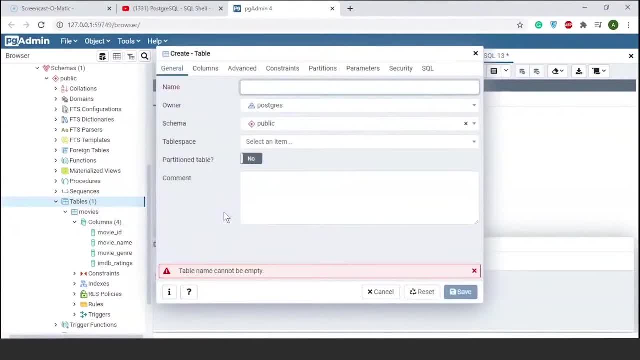 PG admin. so here under tables, I'll right-click and I have the option to create, so it's asking me to give the name of the table. so this time we are going to create a table called students, so I will write my table name as students. alright, these will. 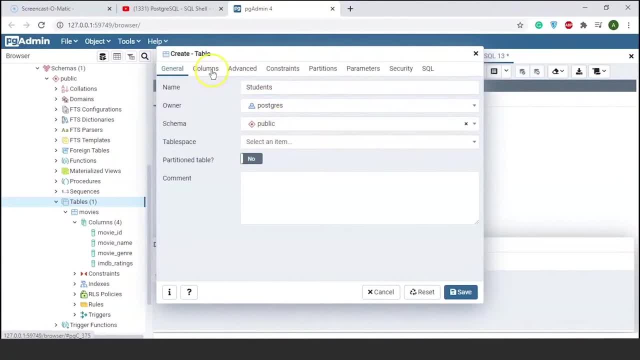 be default as it is. now I will go to the columns tab, so here you can create the number of columns that you want. so you can see, on the right I have a plus sign. I will just select this so that I can add a new row. so my first column would be, let's say, the student roll number. 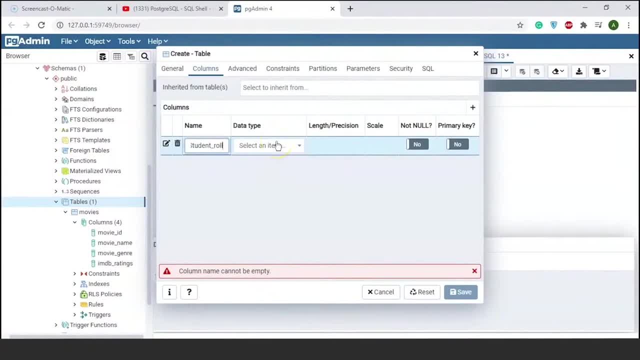 I will write student underscore roll number again. the column name should be as per SQL standards. the data type I am going to select is integer. alright, now, if you want, you can give these constraints such as not null, so that student roll number column will not have any null values. and I'll also check primary key, which means all the 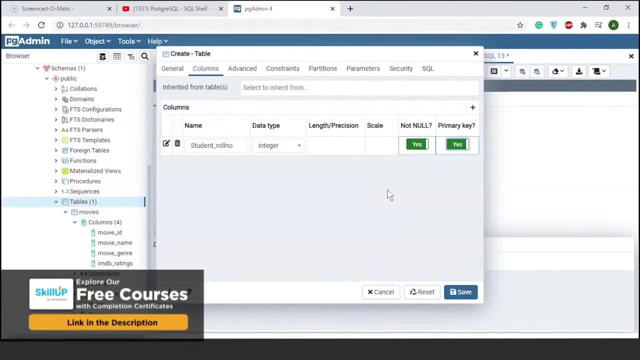 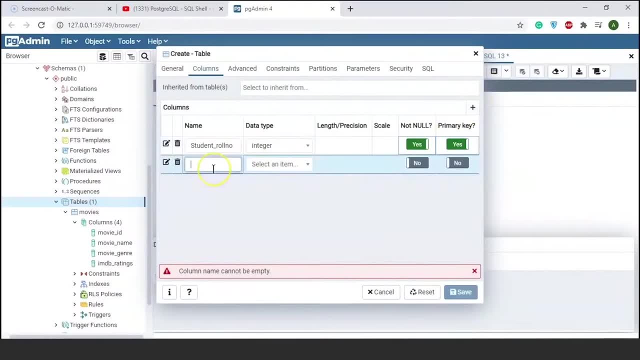 values will be unique for roll numbers. alright, if you want to add another column, you can just click on that plus sign. and let's say, this time I want to give the student name as my second column, so I'll write student underscore name. student name will be of type. 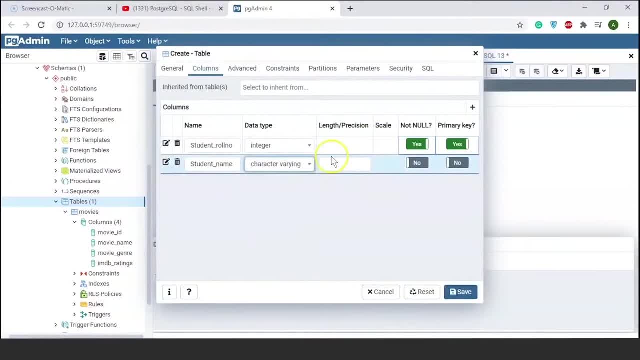 character varying. if you want to give the length, you can specify the length as well, let's say 40. I'll click on the plus sign again to add my final column. the final column would be gender. so gender I'll keep this time as type character. okay, now you can click on save. 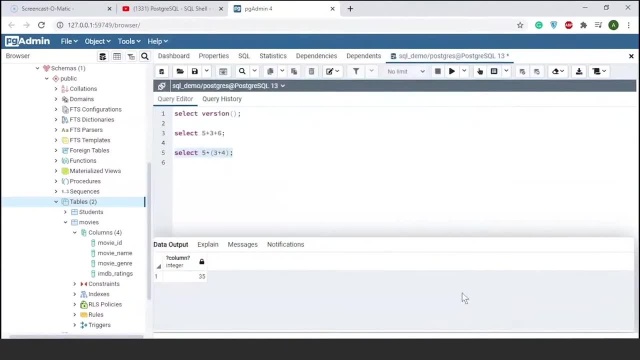 so that will successfully create your students column table. there you go. so here on the left panel you can see earlier we had only one table, that was movies, and now we have two tables, so one would be added, that was students. if I expand this under columns, you can see we have the three columns here: student roll number. 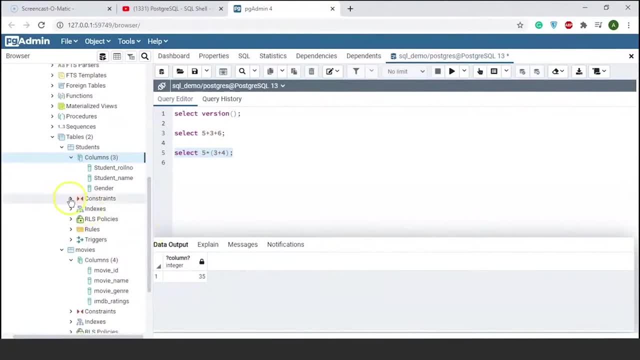 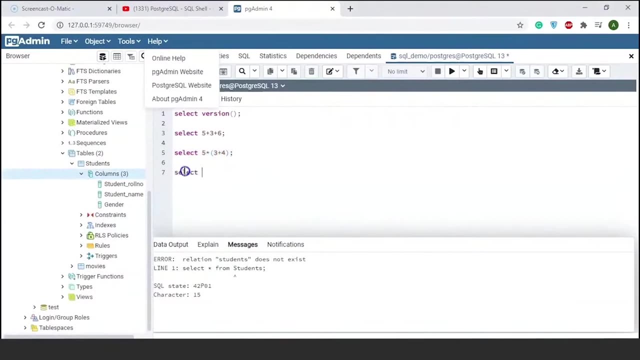 student name and gender. you can also check the constraints. it will tell you if you have any constraints so you can see. it says students roll number. there's one primary key. alright, now let me run a select statement to show the columns that we have in the movies table. 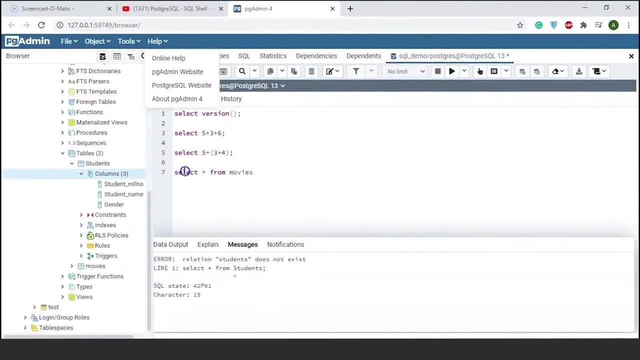 so I'll write: select star from movies. give a semicolon and let me execute this. okay, so here on the at the bottom, you can see we have the movie ID, the movie name, movie genre and IMDB ratings. now the next command we are going to learn is how to delete a table. so there's. 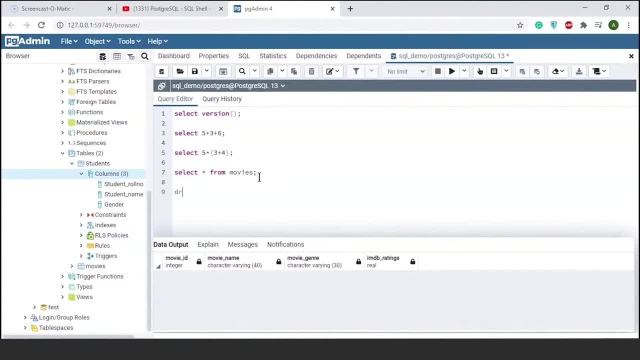 one way by using the SQL command. that is drop table followed by the table name. let's say you want to delete students, you can write drop table students and that will delete the table from the database. this is one of the methods, so you just select and run it. now the 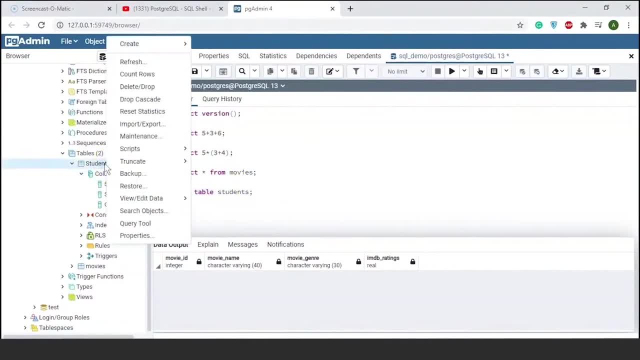 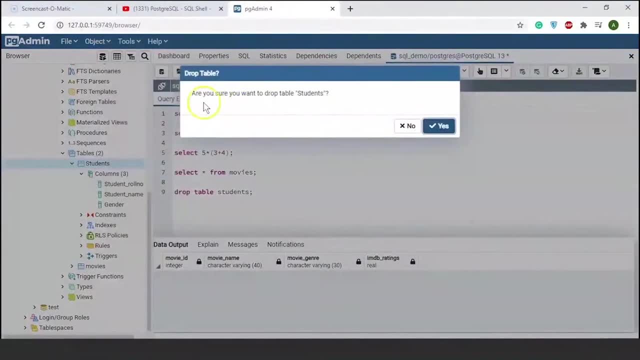 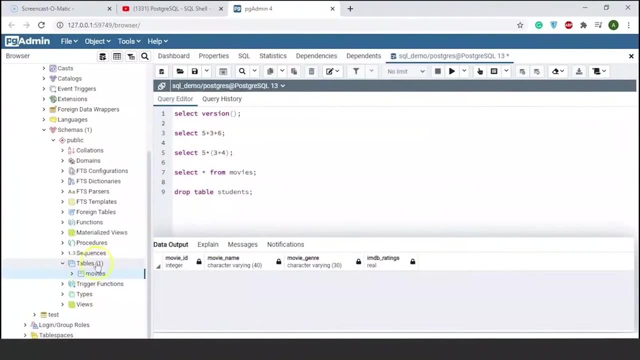 other way is to you just right click on the table name and here you have delete slash drop. If you select this, you get a prompt. are you sure you want to drop table students? I'll select yes, so you can see we have successfully deleted our students table. alright, now let's. 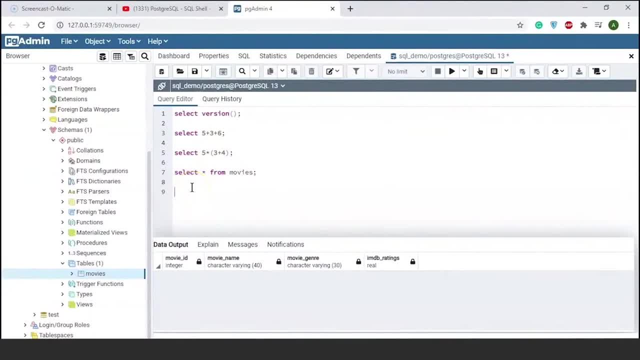 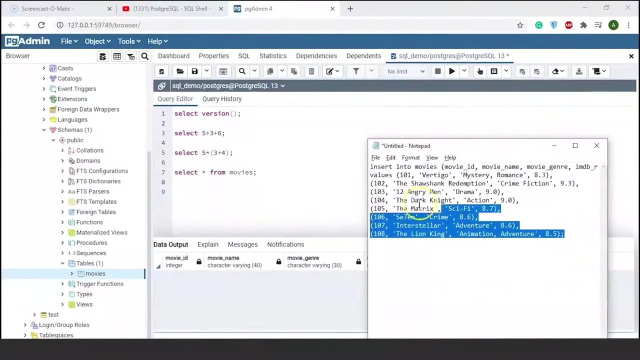 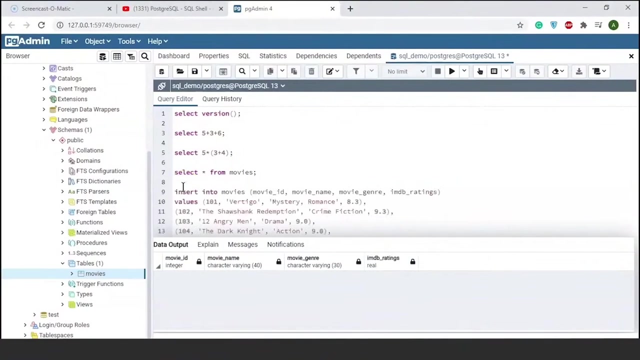 perform a few operations and learn a few more commands in PostgreSQL. so to do that I'm going to insert a few records to my movies table. so for that I'll use my insert command. so I have my insert. So here you can see. I have used my insert command, so I have written insert into the. 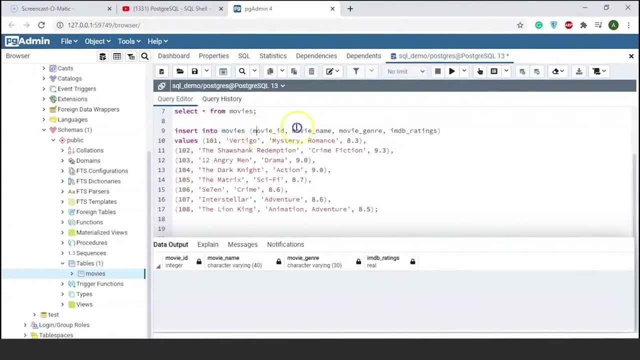 name of the table, that is movies, and we have the movie ID, the movie name, movie genre and IMDB ratings. And These are The records, gods or the rose. so we have the first record as movie id, 101. the name of the movie is a very 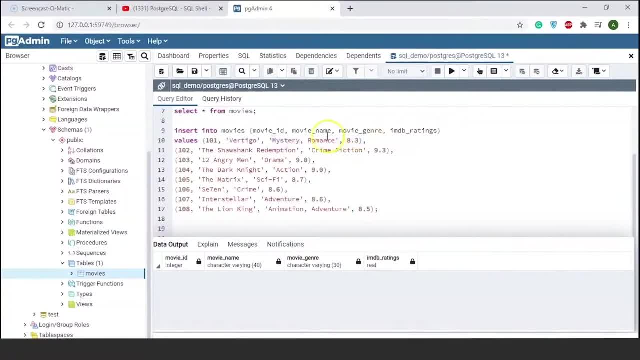 popular movie, which is vertigo. then we have the movie genre, that is mystery. it is also a romance movie. and then we have the imdb ratings. the current imdb rating that is 8.3. similarly we have saw shank redemption. we have 12 angry men. there is the matrix 7 interstellar. 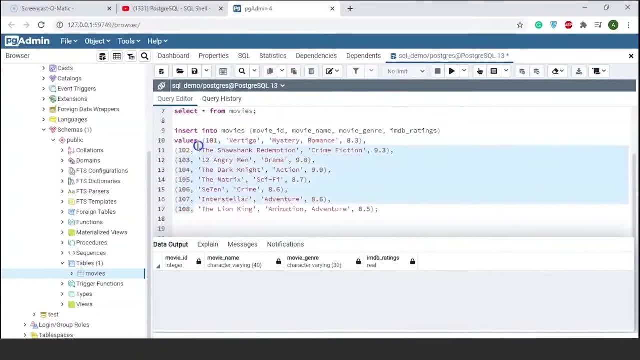 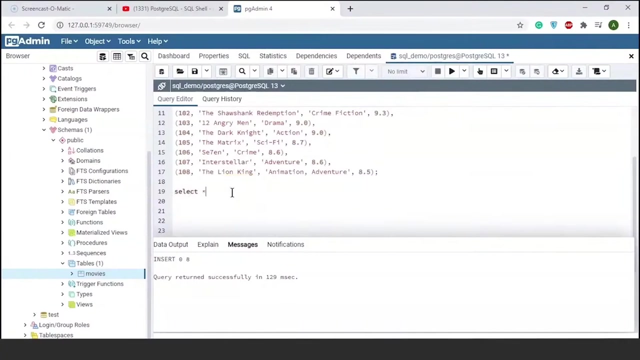 and the lion king. so there are total eight records that we are going to insert into our movies table, so let me just select this and hit execute. okay, you can see it has returned successfully eight records. now if i run select star from movies, you can see the records that are present in the table. so i'll write: select star from movies. 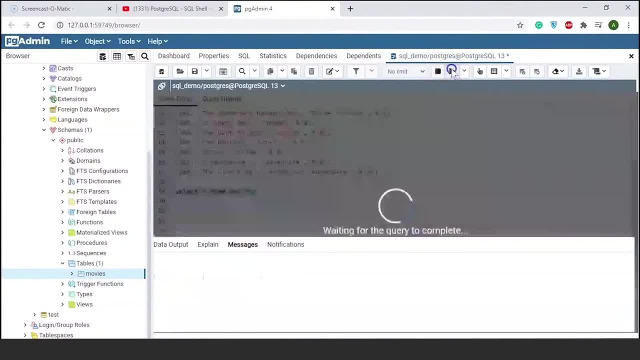 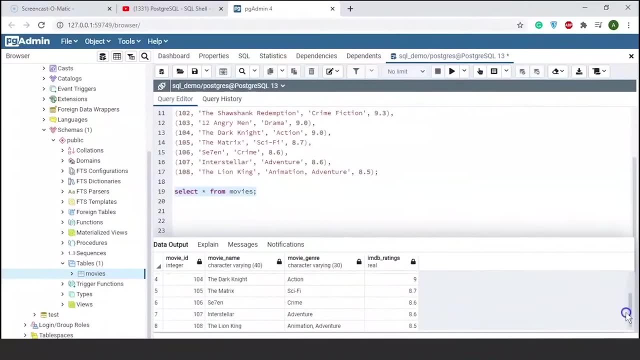 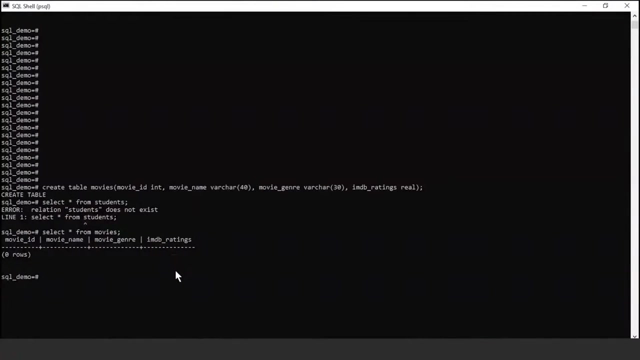 i'll select this and i'll execute it. there you go. at the bottom you can see eight rows affected. if i scroll this down, you have the eight records of information in the movies table. all right now. if you want to describe the table, you can go to the sql cell and here, if you write backslash, d and 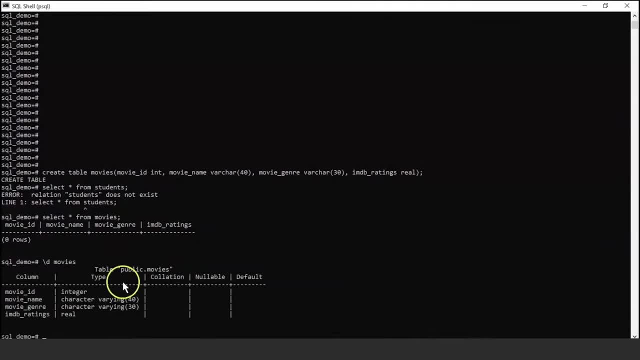 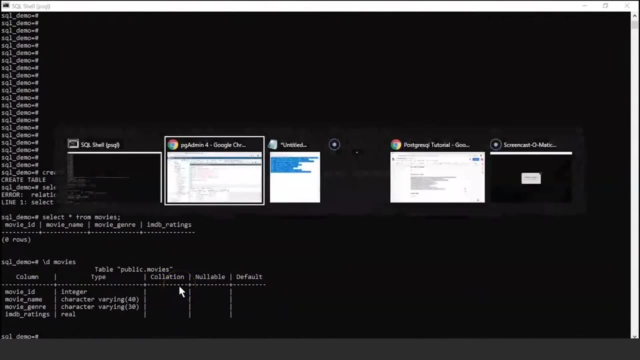 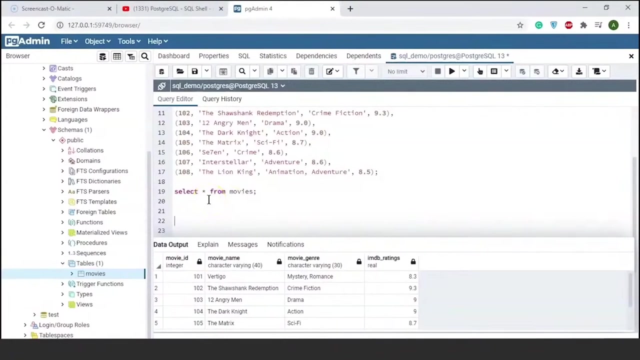 the name of the table, that is movies. this will describe the table. so here you have the column names. this has the data type and here you can specify if there are any null values or any constraints, like default constraint or primary key or foreign key and others. let me go back to my pg admin. okay, now, first and foremost, let me tell you how to update records. 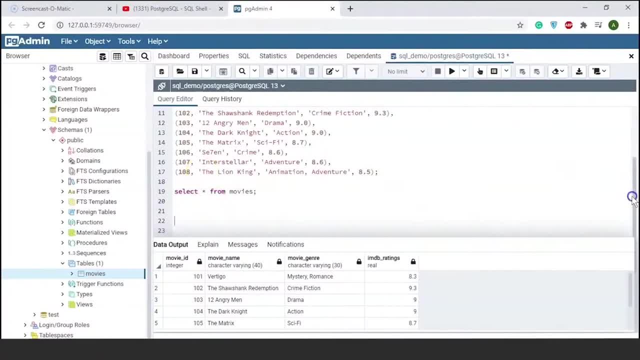 in a table. so suppose you have an existing table and by mistake you have entered some wrong values, want to update those records later? you can use the update query for that. so I am going to update my movies table and I'll set the genre of movie: ID 103, which. 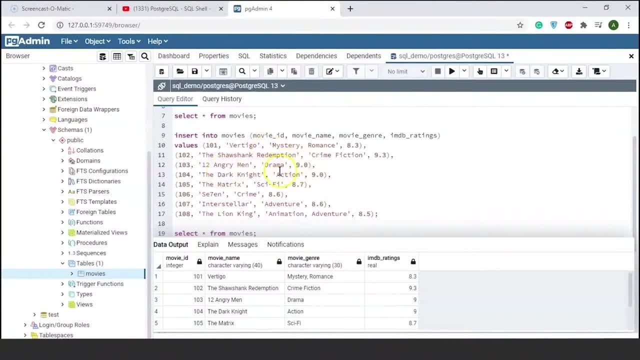 is 12 angry men, from drama to drama and crime. so in our current table we only have genre as drama for 12 angry men. I am going to update this column, which is the movie genre to drama and crime. okay, so let me show you how to do it. 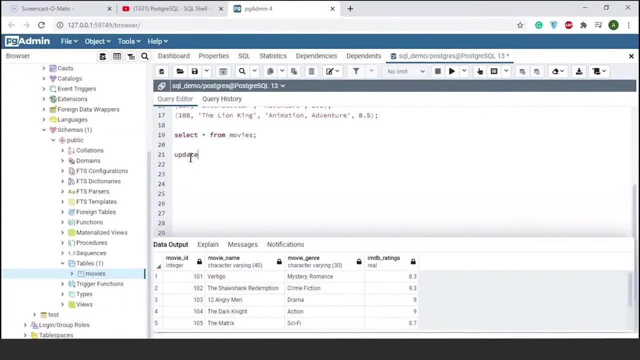 I'll write update, followed by the name of the table, that is movies. go to the next line. I'll write set, then I'll give the column name, which is movie underscore genre equal to. I'm going to set it as drama, comma crime. earlier it was only drama and I'll give my condition using 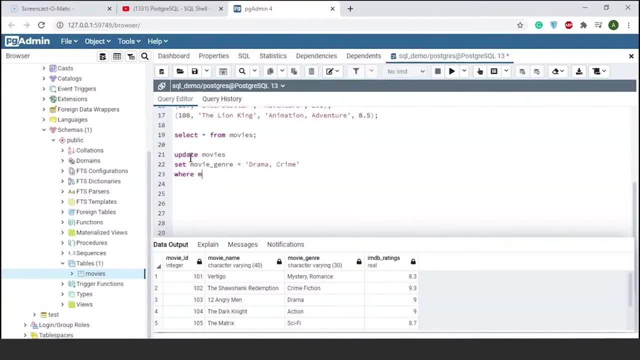 the where clause. we'll learn where clause in a bit, so I'll write where movie underscore ID is equal to 103. so here our movie ID is the unique identifier. so it will first look for movie ID 103. it will locate that movie and will change the genre to drama and crime. so now you can see the difference. 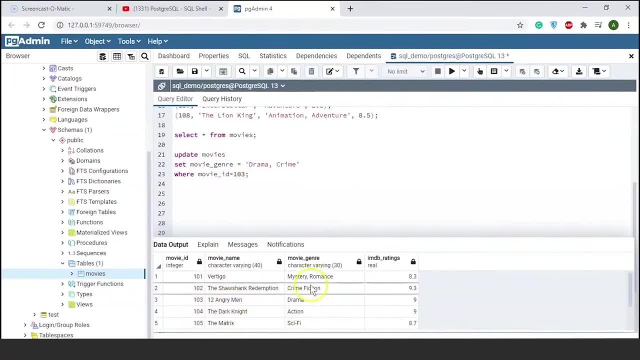 earlier we had 12 angry men as drama, as the movie genre. now if I run this update statement, okay, you can see we have successfully updated one record. now let me run the select statement again. okay, so here you can see if I scroll down, there you go. so movie ID 103. movie name: 12 angry men: we have successfully. 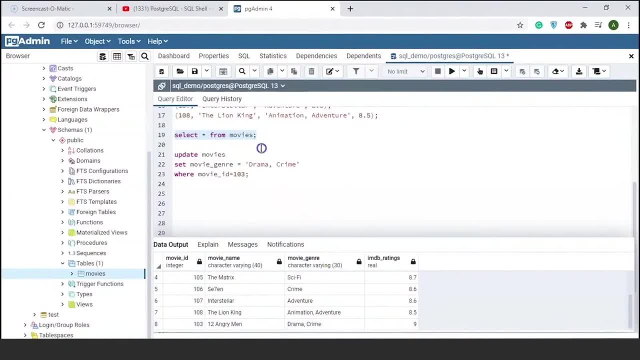 updated the genre as drama comma crime. okay, now let me tell you how you can delete records from a table. so for that you can use the delete command, so you'll write delete from the table name. that is movies where let's say I want to delete the movie ID 108, which is the Lion King. so I'll write where, movie underscore: I'm. 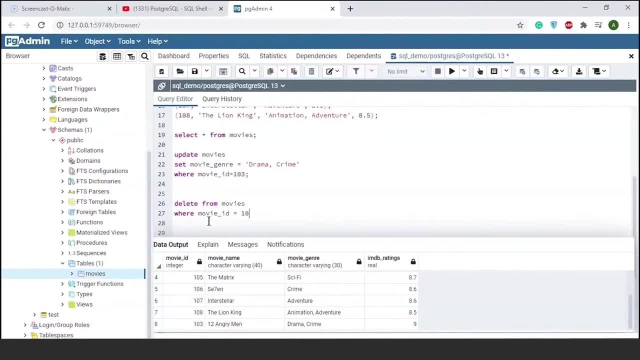 ID is equal to 108. this is one of the ways to delete this particular movie. or you can give, let's say, where movie name is equal to the Lion King. let me select this and I'll hit execute now if I run my select query again. you see this time. 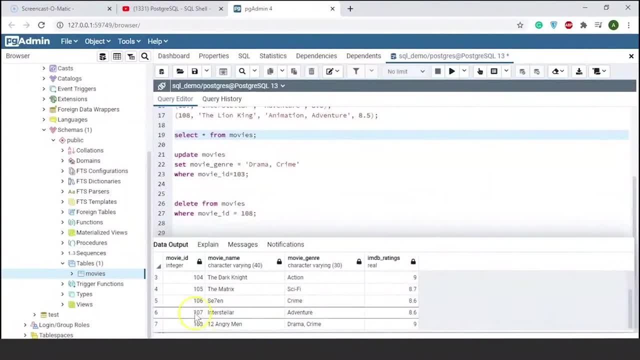 it has returned seven rows and you cannot find movie with movie id 108. that was the lion king, so we have deleted it all right. next we are going to learn about where clause in postgresql. so to learn where clause, i'll be using the same movie table again. 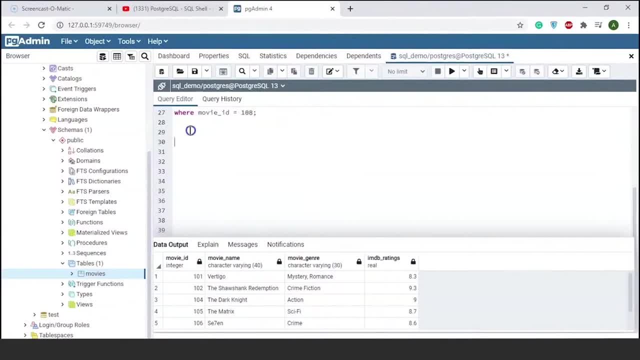 let's say we want to filter only those records for which the imdb ratings of the movies is greater than 8.7. so this is my updated table. now i want to display only those records or those movies whose imdb ratings is greater than 8.7. so we'll display 12 angry men, which is 9. then we are going to 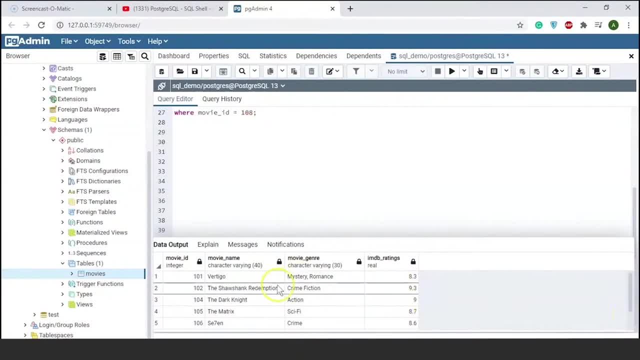 display the dark knight, which is again 9, and we are also going to display the shawshank redemption, which has 9.3. the rest of the movies have an imdb rating less than 8.7, so we are not going to display those. all right, so let me show you how to write a where clause. 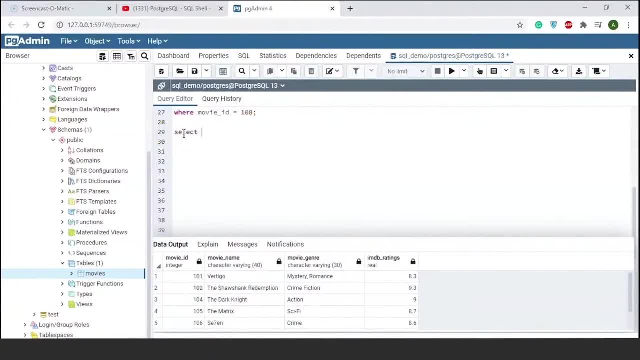 so i'll write select star from movies where i'll give my column name, that is imdb. underscore ratings is greater than. i'll use the greater than symbol. then i'll pass my value. that is 8.7. i'll give a semicolon and let's run it. i'll hit f5. there you go. so we have returned the shawshank redemption. 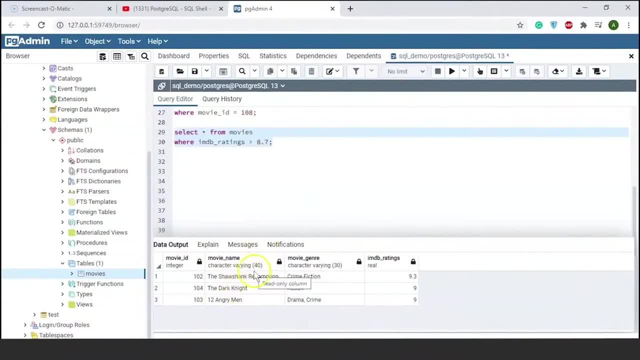 dark knight and 12 angry men, because only these movies had imdb ratings greater than 8.7. okay, now let's say you want to return only those movies which have imdb ratings between 8.5 and 9.. so for that i am going to use another operator called between, along with the where clause. so let 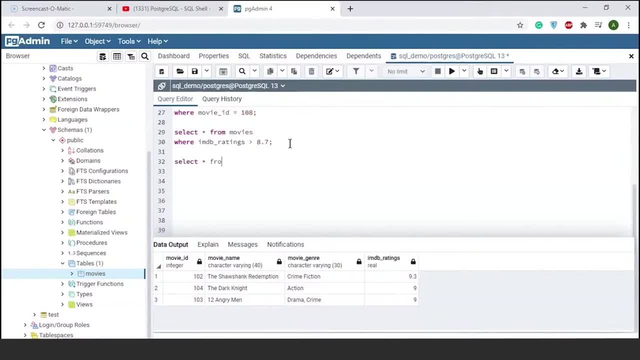 me show you how to use between. with where clause, i'll write select star. from movies where my imdb underscore ratings is between, i'll write 8.5, i'll give an and operator and 9.0. so all the movies that are between 8.5 and 9.0 ratings will be displayed. so let's select this and i'll run it. there you go. 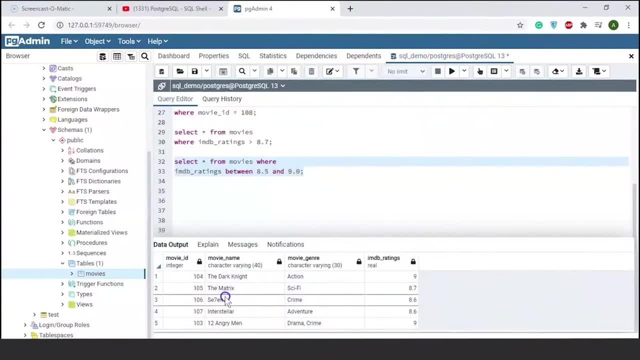 so we have returned the dark knight, the matrix, the seven interstellar and we have the twelve angry men. so a few of the records that we missed out, where i think vertigo, which has 8.3, and there is one more all right now. moving ahead, let's say you want to display the reverse spec. subluet que. 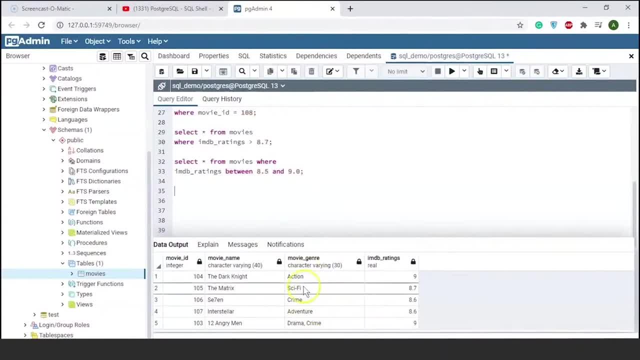 movies whose movie genre is action. you can see in a table. we have a few movies whose genre is action movie, so you can do that as well. i'll write select star from movies where the movie genre i'm writing this time in one line. you can break it into two lines as well. i'll write movie. 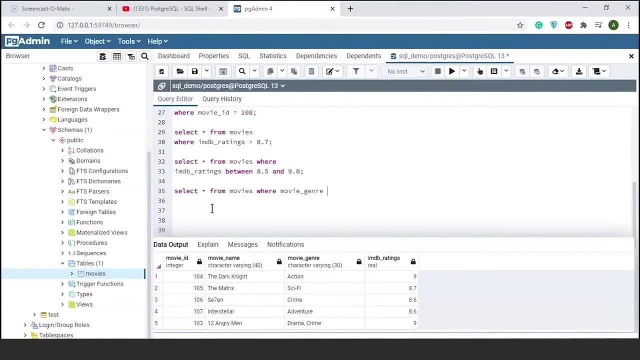 underscore genre, which is my column name equal to, i'll give, within single quotes, action. now, why single quote? because action is a string, hence we need to put it in single quotes. if i run this, there you go. so we had one movie in our table whose movie genre was action, that is the dark knight. okay, 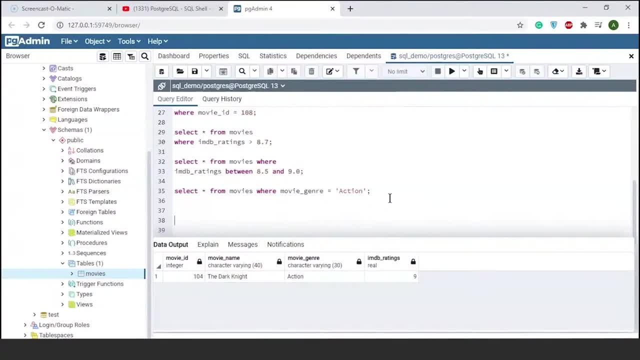 now you can also select particular columns from the table by specifying the column names. now, here, in all the examples that we saw just now, we are using star. now star represents. it will select all the columns in the table. if you want to select specific columns in the table, you can use the. 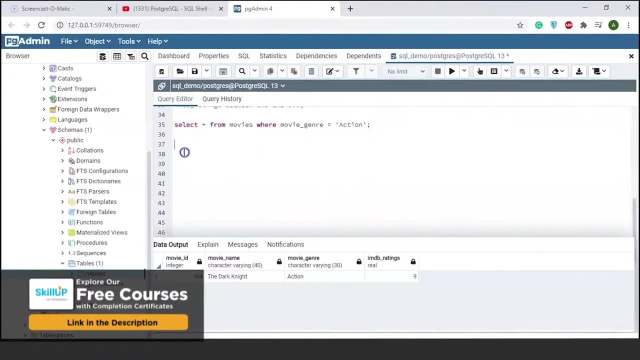 column names so you can specify the column names in the select statement. let me show you. let's say you want to display the movie name and the movie genre from the table so you can write select movie underscore- name comma. i'll give the next column as movie underscore. 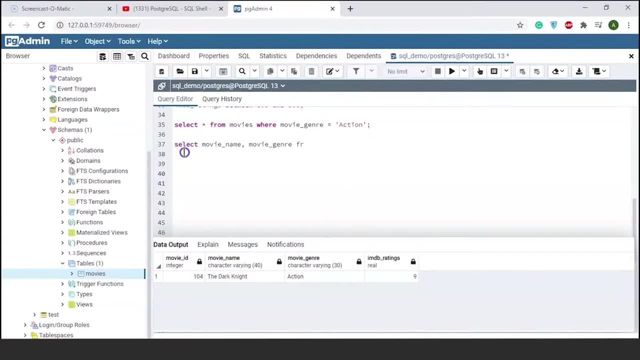 genre from my table name, that is, movies where, let's say, the imdb underscore ratings is less than 9.0. so this time in our result it will only show two columns, that is, movie name and movie genre. let me run it. there you go. so these are the movie names and the movie genres you can. 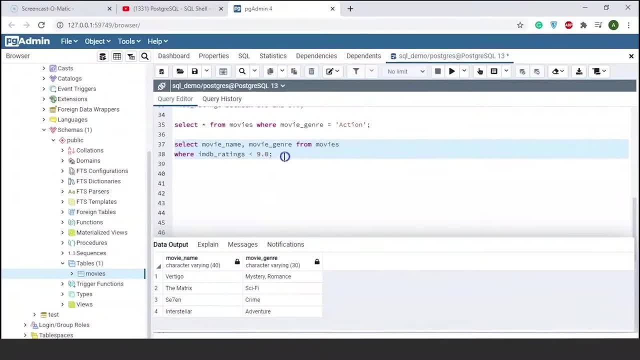 see that have an imdb ratings less than 9.0. all right, like how you saw, the between operator, there is one more operator that you can use, with the where clause. that is movie name and movie genre, the in operator. so the in operator works like a or clause or an or operator. so let's say: 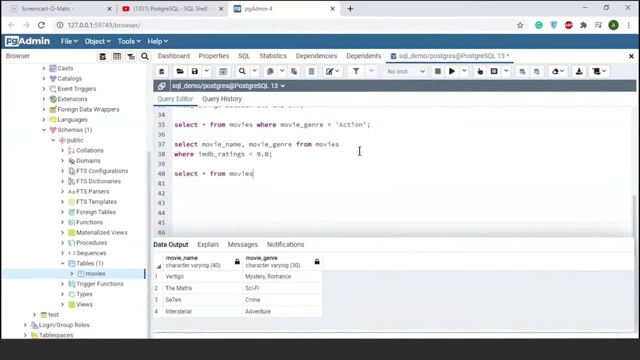 i want to select all the columns from my movies table where the imdb ratings is in 8.7 or 9.0. if i run this, it will display only those records whose imdb ratings is 8.7 or 9.0. all right, so up to now. 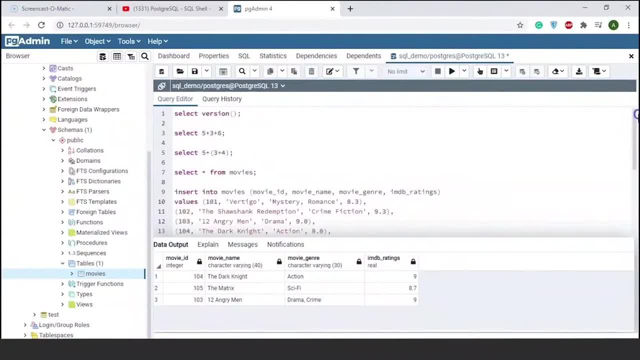 we have looked at how you can work on basic operations in sql, like your mathematical operations. you saw how a select statement works. we created a few tables, then we inserted a few records to our tables. we saw how you can delete a table from your table and then we created a few. 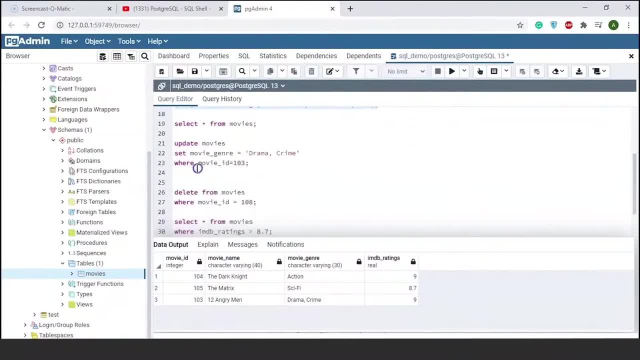 records to our tables. we saw how you can delete a table from your database and we have performed a few operations like update, delete, and we saw how a where clause works. now it's time to load a employee csv file or a csv data set to postgres sql. so i'll tell you how you can do that. but 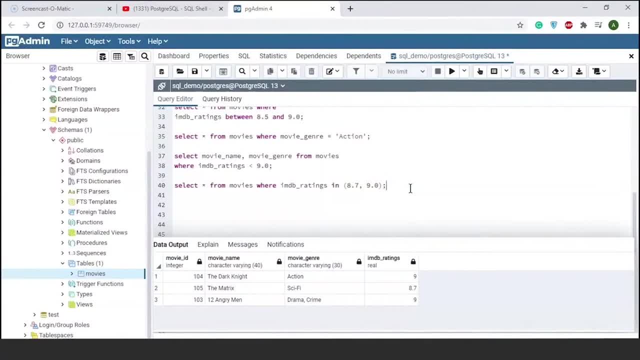 first of all, before loading or inserting the records, we need to create an employee table. so let me first go ahead and create a new table called employees in our sql underscore demo database. so i'll write: create table. my name of the table would be employees. next i'm going to give my 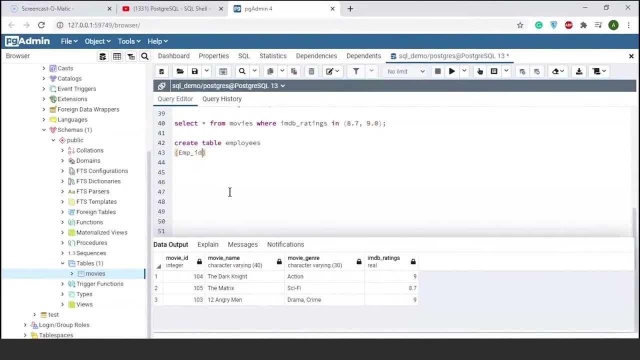 column names. so my first column would be employee id. so the employee id will be of type integer. it is not going to contain any null values. so i'll write not null and i'll give my constraint as primary key. so the employee id, as you know, is unique for all the employees in a. 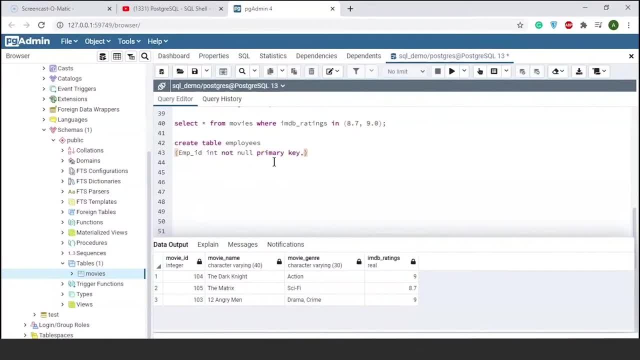 company. so once i write primary key, it will ensure that there are no repetition in the employee ids. okay, next i'll have my employee name. so my employee name is going to be of type worker and i'll give my size as 40. okay. next we'll have the email address of the employee. again, email address would be of type. 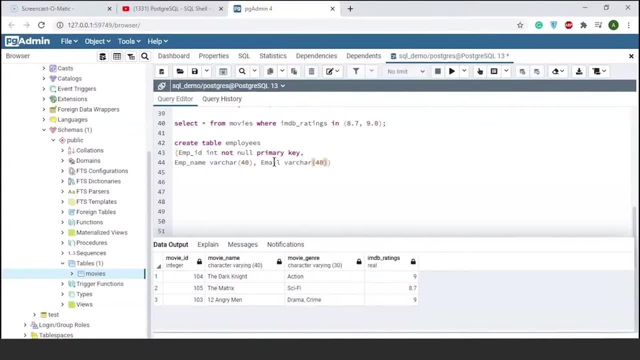 worker and the size is 40. again, i'll give another comma. this time we'll have the gender of the employee. gender is again worker, of size, let's say 10. okay, now let's include a few more columns. we'll have the department column, so i'll write department. 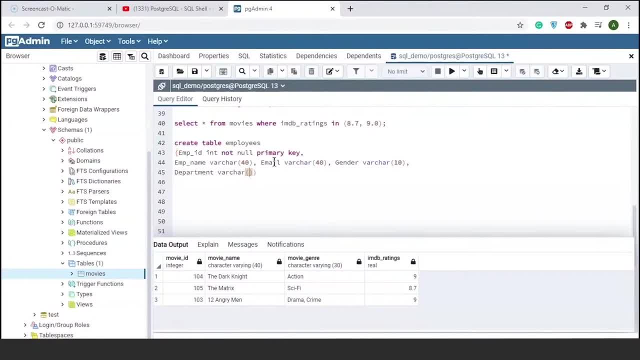 worker. let's say the size is 40. then let's say we'll have another column that is called address. so the address column will have the country names of the employees. address is also worker. and finally we have the salary of the employee, salary i'm going to keep it. 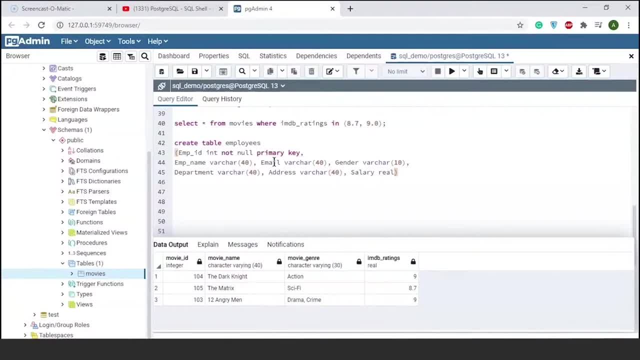 as type real. and finally, we have the salary of the employee salary. i'm going to keep it as type real, so real will ensure it will have decimal or floating point values. okay, so now let me select this, create table statement and execute it. all right, so we have. 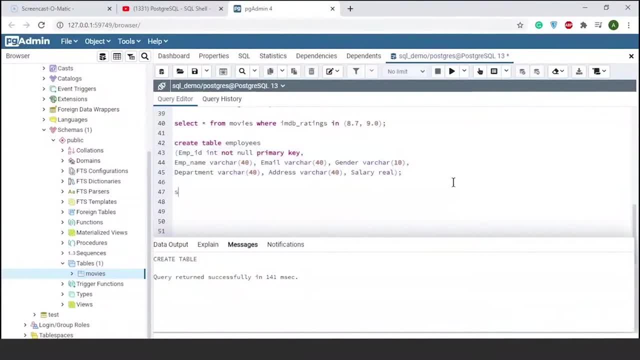 successfully created our table. if you want, you can check by using select star from employees. let me select this and i'll hit execute. all right, you can see. we have our employee id as primary key. there's employee name, email, gender, this department address and salary, but we don't have any records for each of these. 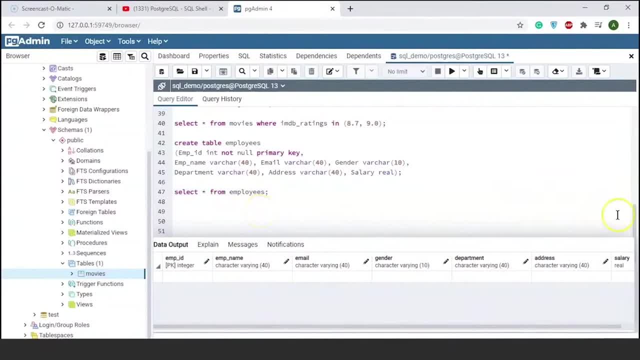 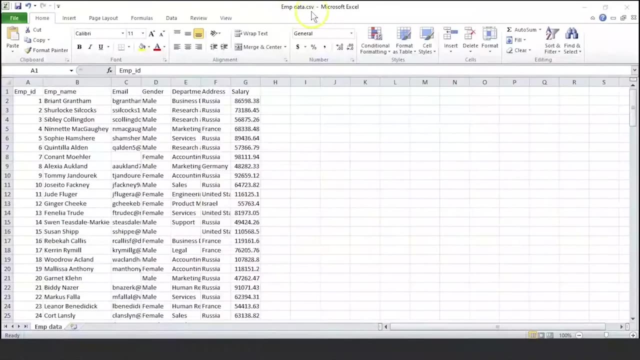 columns. now it's time for us to insert a few records to our employees table. now, to do that, i am going to use a csv file, so let me show you how the csv file looks like. okay, so now i am on my microsoft excel sheet and on the top you can see this is my employee datacsv. 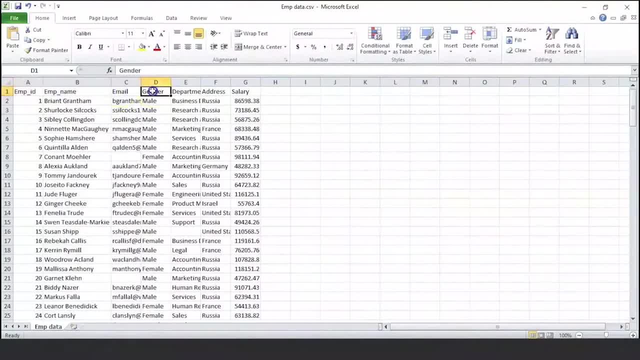 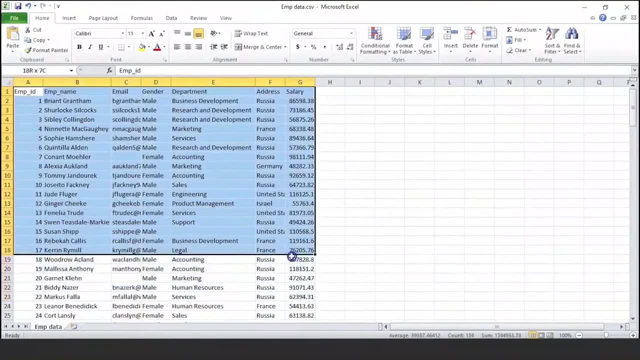 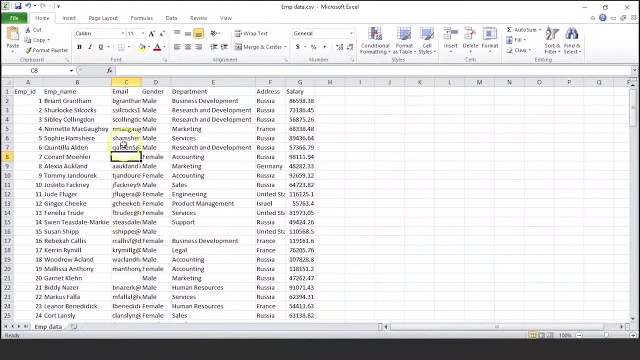 file. here we have the employee id, the employee name, email gender, this department address and salary. now this data was generated using a simulator so this is not validated and you can see it has a few missing values. so under email column you have a few employees who don't have an 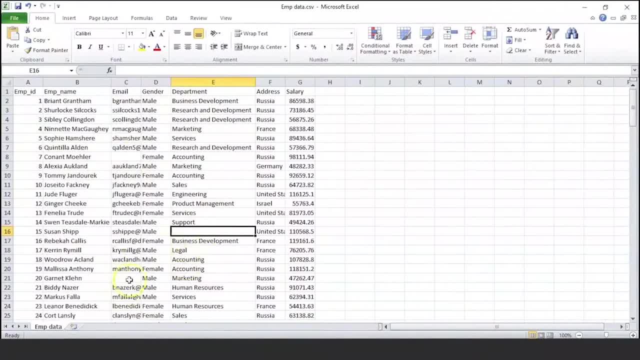 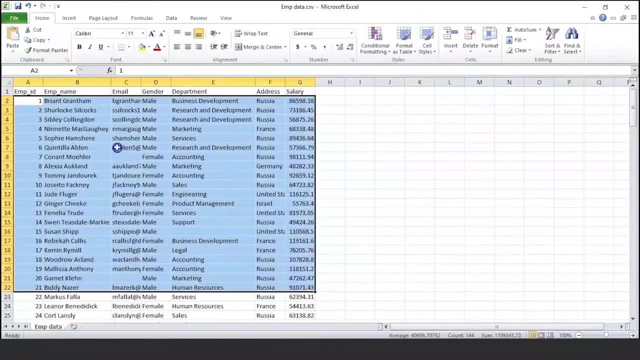 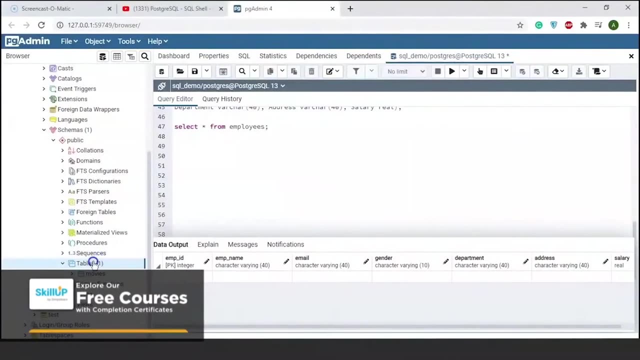 email id. then you can see under department. also, there are some missing values here as well. all right, so we'll be importing this table or the data for this table. so we'll be importing this table or the records present in this csv file onto postgresql. all right, so here in the left panel. 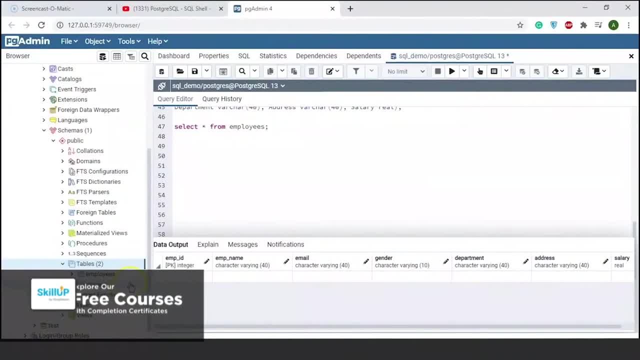 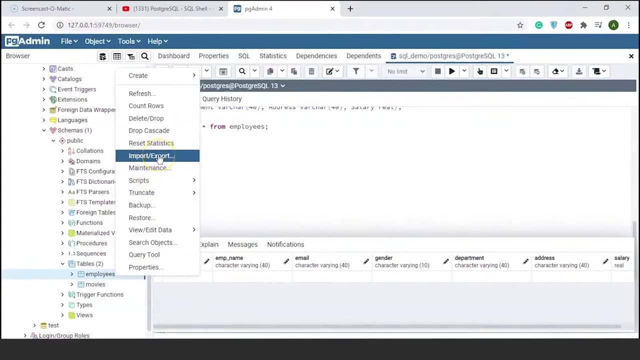 under tables. let me right click and first refresh this. there you go. so initially we had only movies table, and now we also have the employees table. now what we need to do is i'll right click again and here you see, we have the option to import or export. let me click on this and 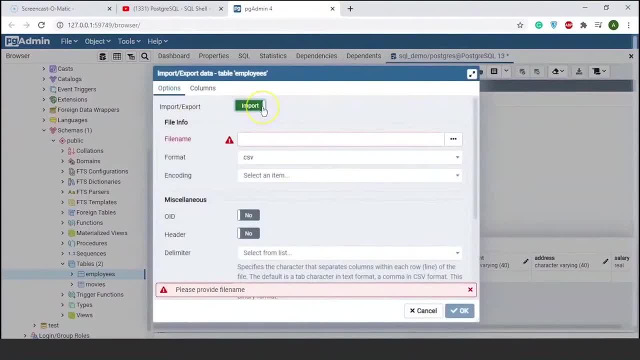 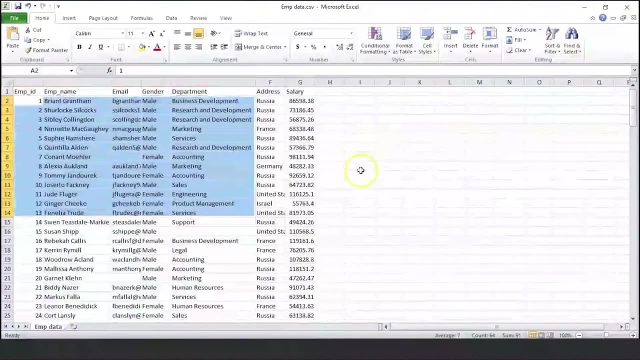 i don't want to export, i need to import, so i'll switch on import. all right, now it is asking me to give the file location, so let me show you how to get the file location. so this is my file location actually. so my excel file, which was this, is present in my e drive under the data analytics. 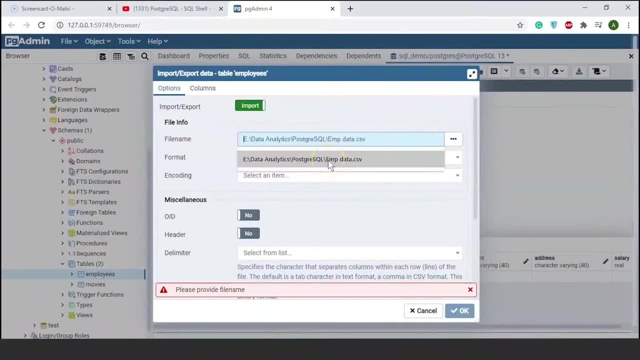 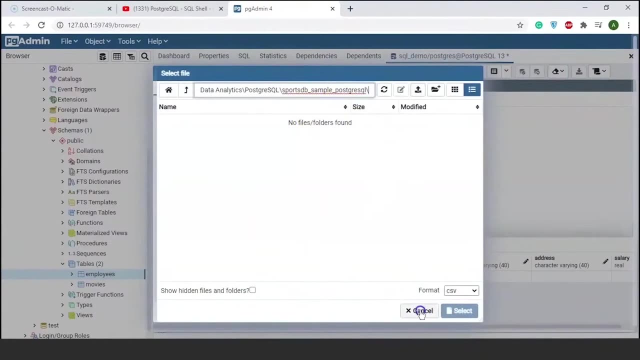 folder i have another folder called postgresql, and within the postgresql folder i have my csv file together. so, as you see, both my file configuration is unique. that's why in here you candefine one fullfile, otros 32, advertisement, cert, anges, etc. else, but this time it's going to be three. 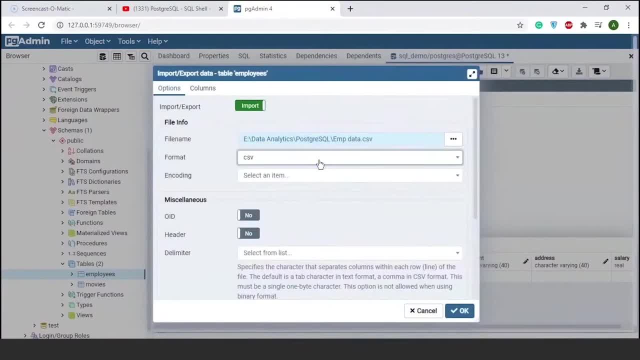 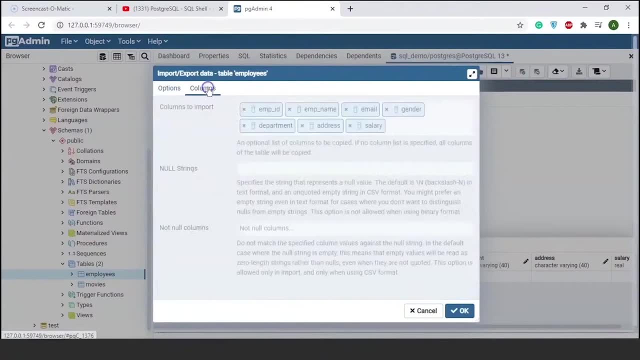 different files for. so i am going to control the format. i am going to use in this case csv and not other files. but let's change the format. so i am taking the lambda googles from here to that one of the here: my psv file. all right, so in here we have one file which is the department. 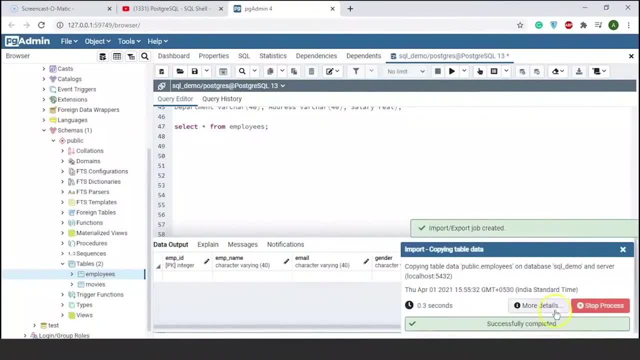 file and there is another file. i am going to change this to the file if i want to control the records. see, i have a message here which says import, underscore export. all right, so here you can see: successfully completed. we can verify this by using select star from employees. again, if i run, 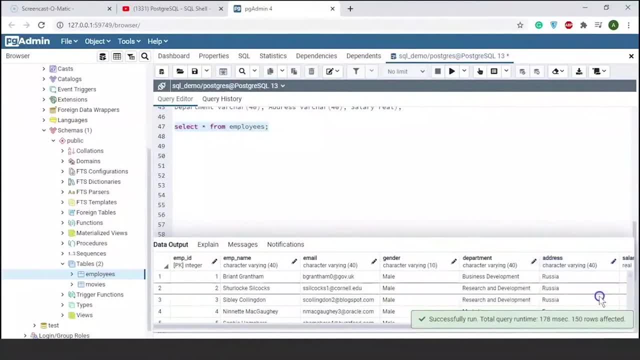 this. all right, let me close this. there you go. it says 150 rows affected, which means we have inserted 150 rows of information to our employees table. you can see we have the employee id. these are all unique. we have the employee name, the email, we have the address and the salary. let me scroll down. 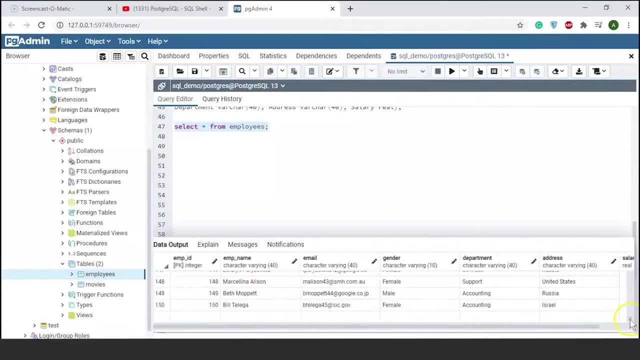 so that, okay, you can see we have 150 rows of information. that means we have 150 employees in our table. okay, now we are going to use this employees table and explore some advanced sql commands. now there is an operator called distinct. so say, if i write select address from employees, this is going to give me 150. 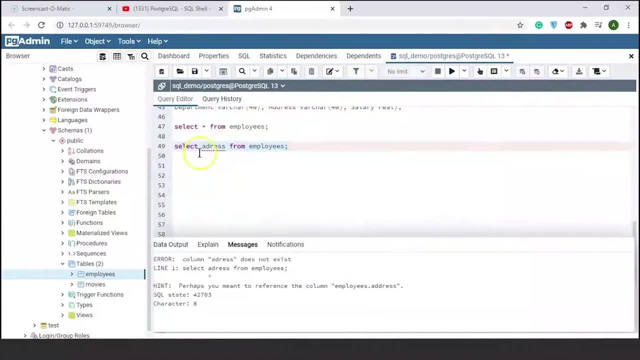 address of all the employees. there's some problem here. i did a spelling mistake. there should be another d. if i run this again, alquery will return 150 rows. you can see we have the different country names under address. that is russia, we have france, there's united states, we have germany, okay, and i think we have israel as well. 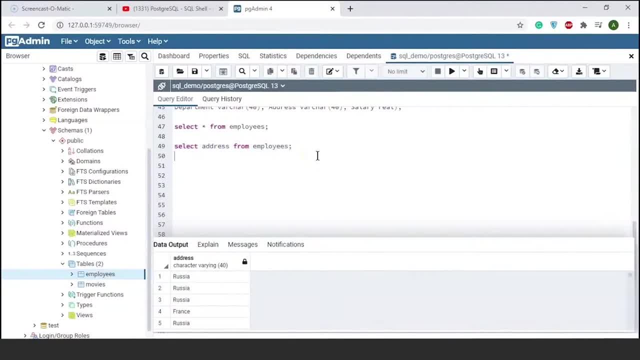 yeah, now suppose you want to display only the unique address or the country names, you can use the distinct keyword before the column name. so if i write select distinct address from employee, it will only display the unique country names present in the address column. if i run this, 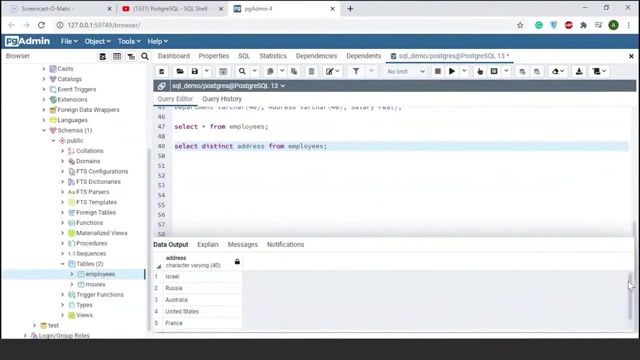 we have six rows of information, so we have israel, russia, australia, united states, france and germany all right. now, as i said, there are a few null values which don't have any information, so you can use the is null operator in sql to display all the null values that are there. suppose i want to. 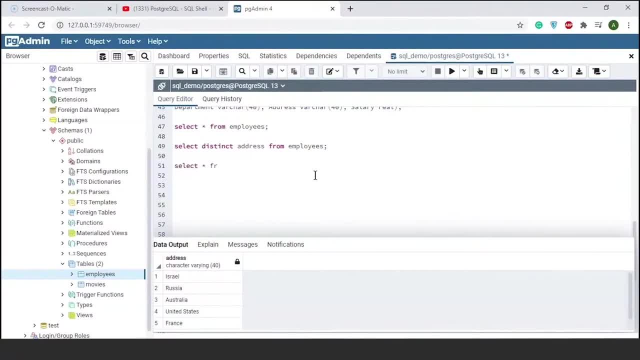 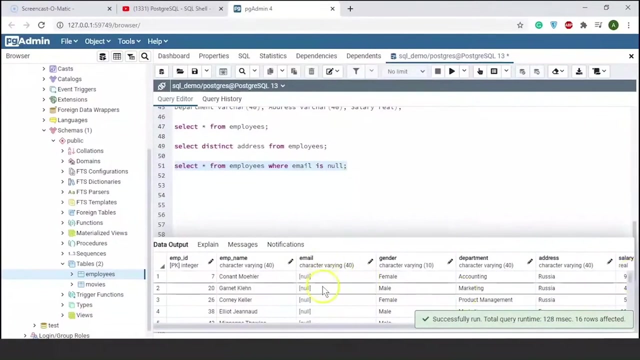 display all the employee names where the email id has a null value. so i like select star from employees where email is null. so this is another way to use your where clause. if i select and run this, there you go. so you see here for all these employee names. 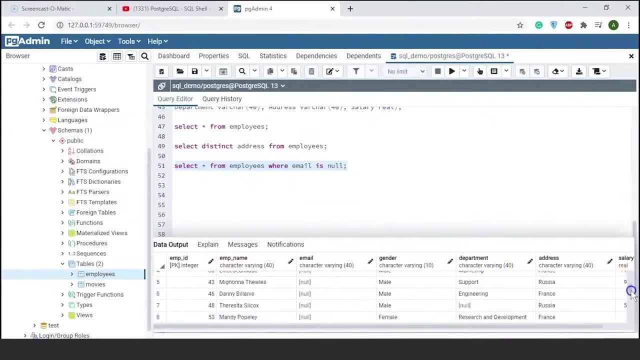 there was no email id present in the table, so it has returned us 16 rows of information. so around 10 of them do not have an email id and if you see, a few of them do not have an email id and also they don't have a department. so if you want to know for those employees which do not have a department, you 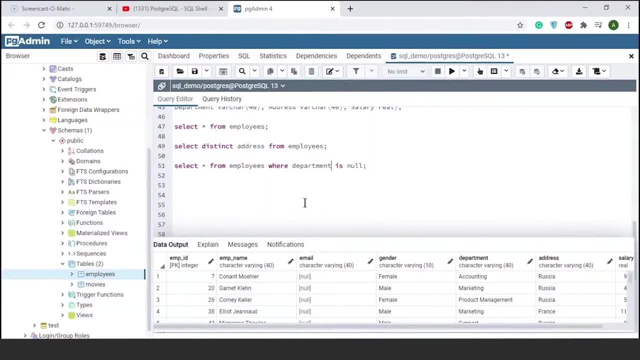 can just replace where department is null instead of where email is null. now, if i select this, okay, it has returned us nine rows of information, which means around five percent of employees do not have a department. moving ahead now let me show you how the order by clause works in sql. now the order by is used to. 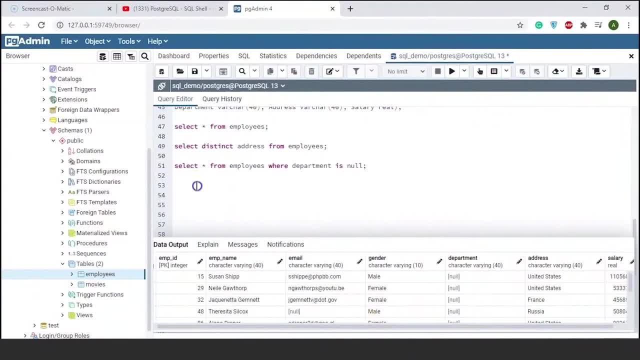 order your result in a particular format, let's say in ascending or descending order. so the way to use is: let's say i want to select all the employees from my table, so i'll write select star from employees order by order by s. I want to order the employees based on their salary, so i'll write order by salary. let me 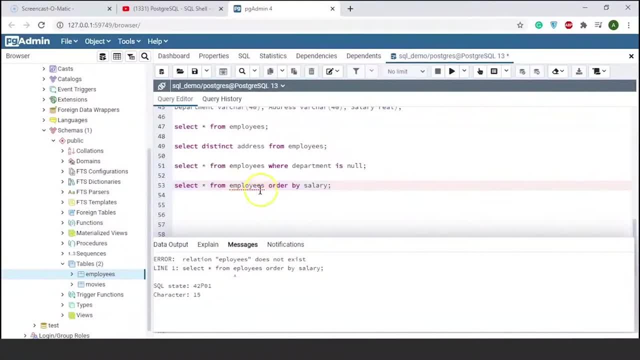 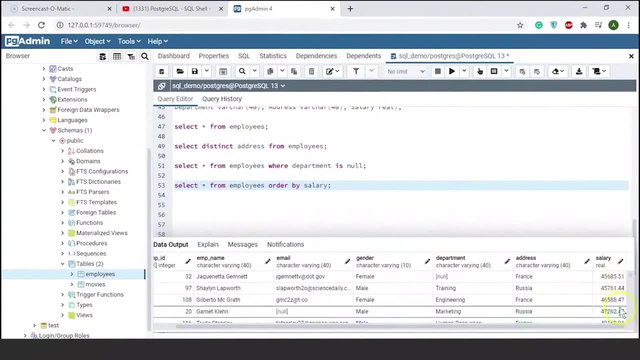 select and run it. okay, there is some problem. i made a spelling mistake. this should be employees. let me run it again. okay now, if you mark the output ordered in ascending order, so all the employees which have salary greater than $45,000 appear at the top and the employees with the highest salaries appear at the bottom. so this has 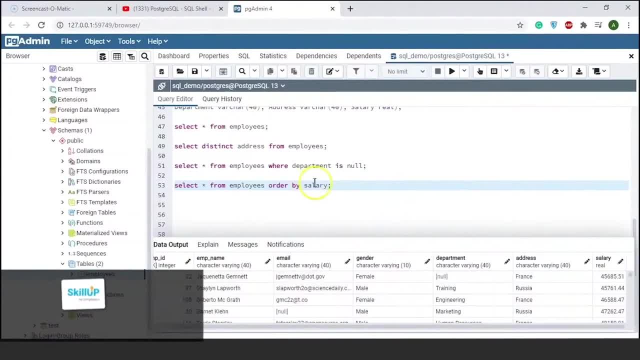 been ordered in ascending order, which means your SQL or Postgres SQL orders it in ascending order by default. now let's say you want to display the salaries in descending order, so that all the top ranking employees in terms of salary appear at the top. so you can use. 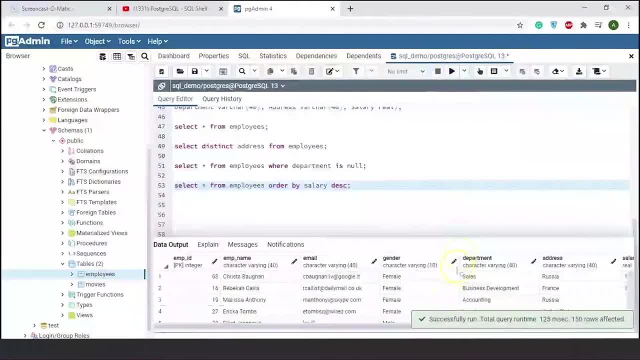 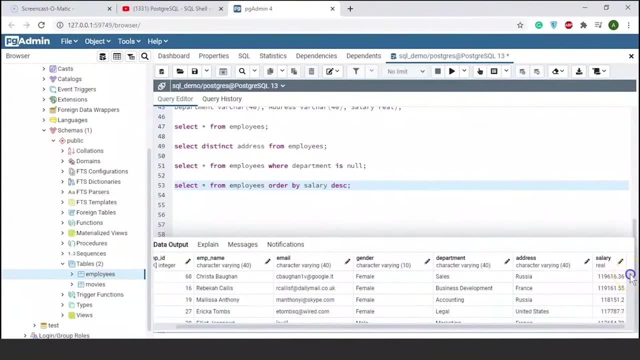 the DESC keyword, which means descending. if I run this, you can see the difference now. so all the employees with the highest salary appear at the top, while those with the lowest salaries appear at the bottom. so this is how you can use an order by clause. okay, so now I want to make a change in my existing table, so here: 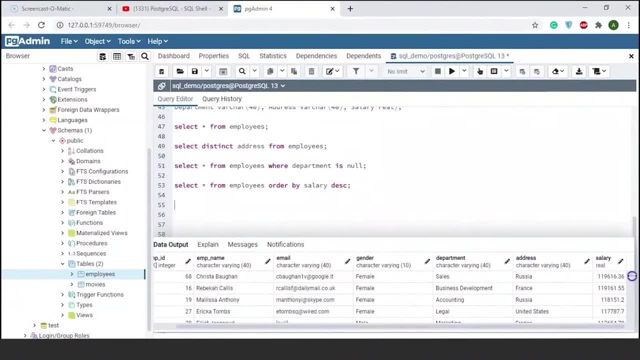 if you see, under the address column we only have the country names. so it would be better if we change the name of the address column to country. so I want to rename a column. you can do this using the alter command in Postgres SQL. so let me show you how to rename this. 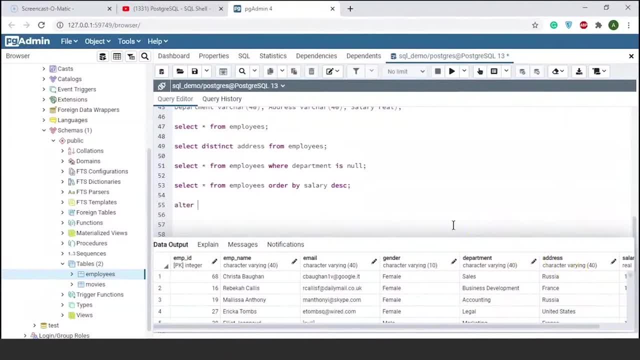 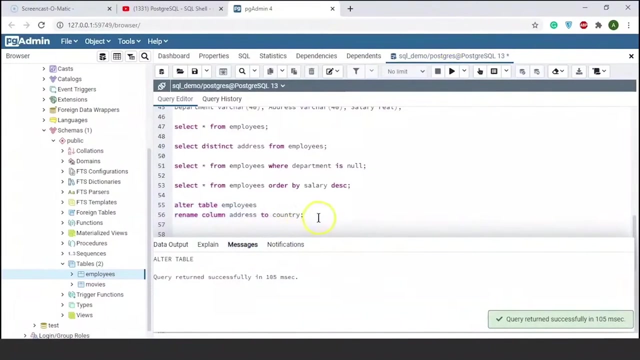 column that is address. so I'll write alter table followed by the table name, which is employees. then I'm going to use a rename column address. I'll write to: I want to change it to country. if I give a semicolon and hit execute, it will change my column name to country. 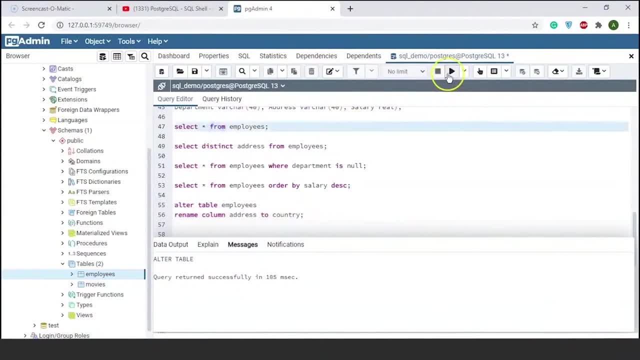 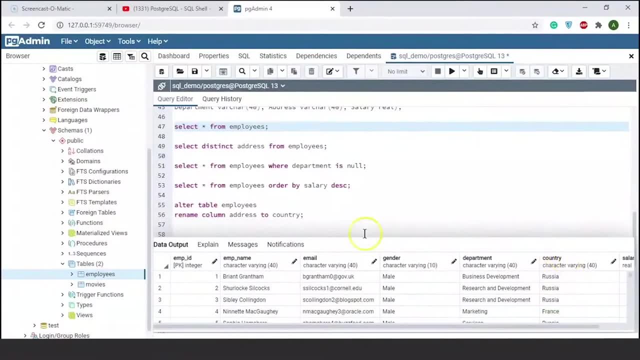 okay, now you can verify this if I run the select statement again. there you go. earlier it was address column, and now we have successfully changed it to country column. okay, let me come down now. it's time for us to explore a few more commands. so this time I am going to tell you how an and and an or operator works. 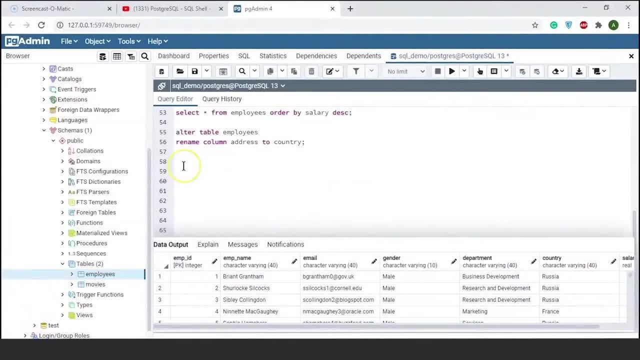 in SQL so you can use the and and or operator along with the where clause. so let's say I want to select the employees who are from France and their salary is less than $80,000. so let me show you how to do it. I'll write select star from. 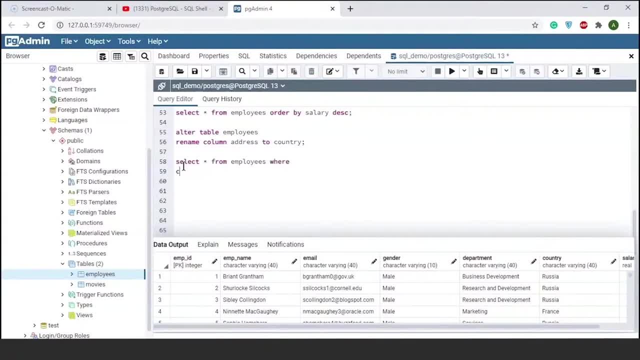 employees, where I'm going to give two conditions, so I'll use the and clause or the and operator. here I'll write where country is equal to France, now mark. here I'm not using address, because we just updated our table and changed the column name from address to country, so I'll write country. 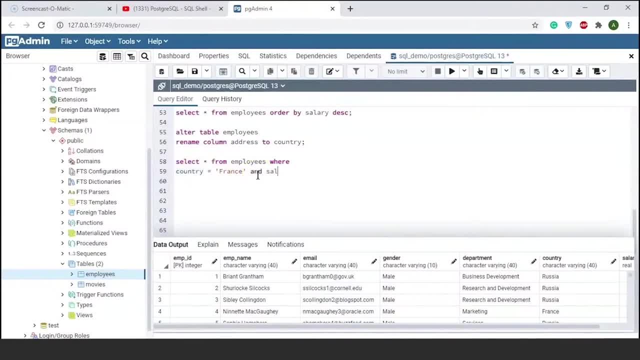 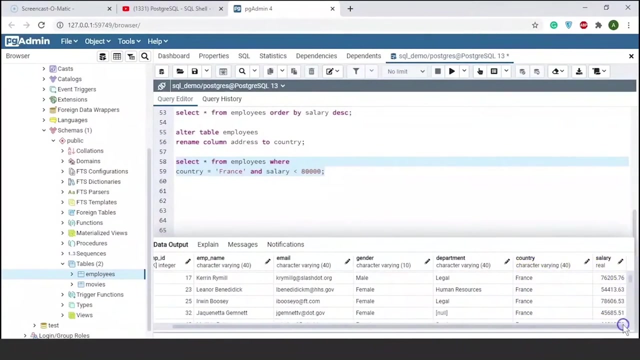 equal to France, and my next condition would be: my salary needs to be less than $80,000. I'll give a semicolon. let me run this and all right. so it has returned 19 rows of information. you can see all my country names of France and the salary is less than $80,000. so this is how you can use. 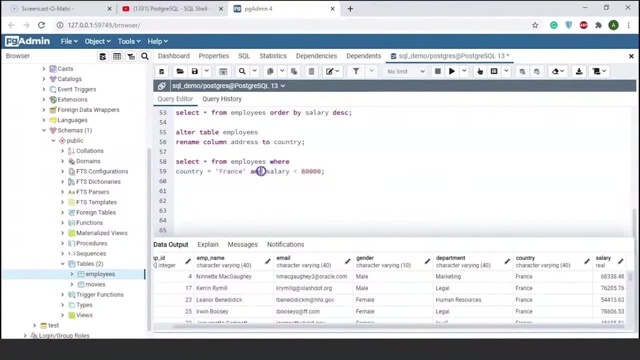 or give multiple conditions in a where clause using the and operator. now let's say you want to use the or operator and let's say you want to know the employees who are from country Germany or the department should be sales. so I'll write select star from employees. 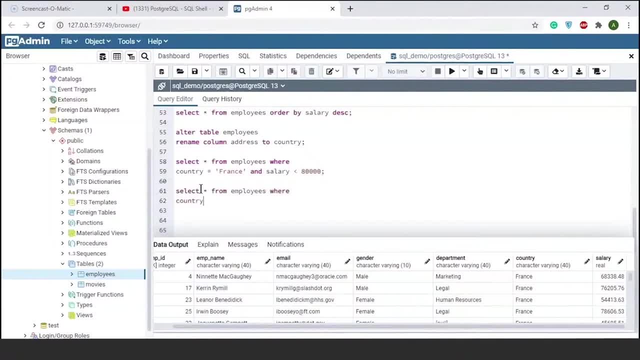 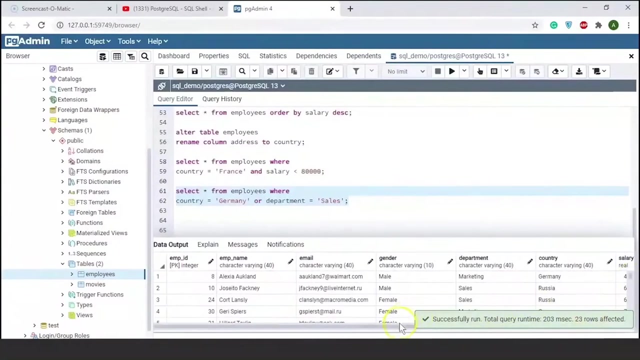 where country is equal to Germany and instead of- and I'm going to use or their department, should be sales. okay, now let's see the output. I'll hit f5 this time to run it all, right? so we have 23 rows of information. now let me scroll to the right. you can see either 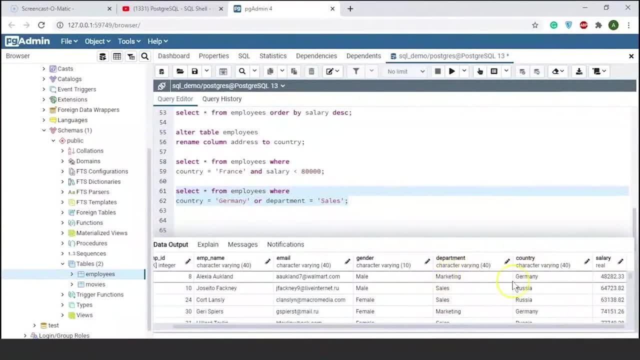 the country is Germany or the department is sales. you see one of them in the table. so here, for the first record, the country was Germany. the second record: the department was sales. again, sales again. for the fourth record, the country was sales is germany. so this is how the or condition works. so if one of the conditions are true, it will. 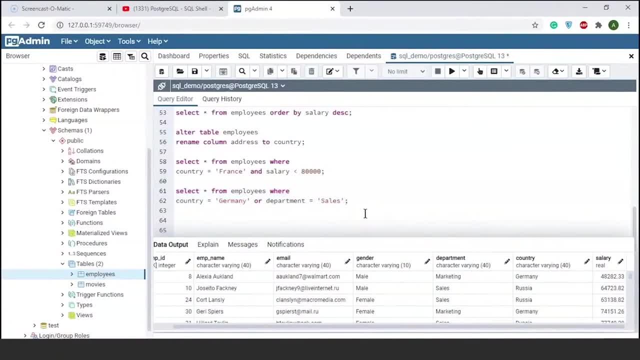 return the result. it need not be that both the conditions should satisfy. now in postgresql there is another feature that is called limit. so postgresql limit is an optional clause on the select statement. now this is used as a constraint which will restrict the number of rows written by. 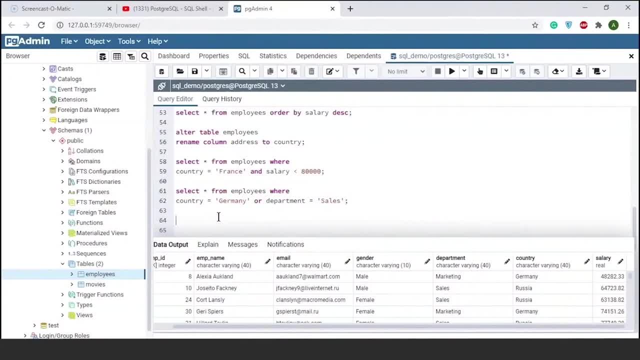 the query. suppose you want to display the top five rows in a table. you can use the limit operator. suppose you want to skip the first five rows of information and then you want to display the next five. you can do that using limit and offset. so let's explore how limit and offset works. 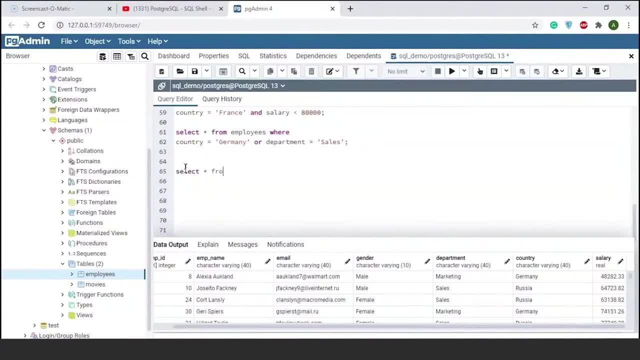 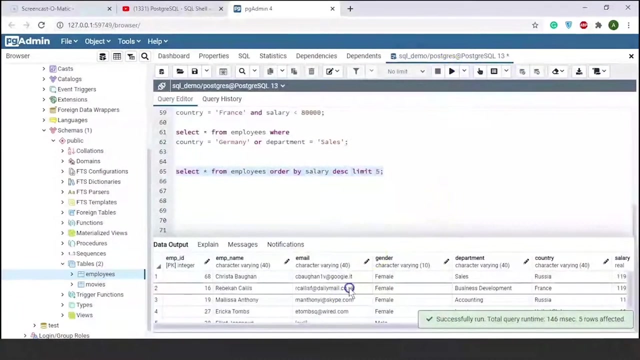 i'll write select star from employees. let's say: i'll use my order by clause. i'll write order by salary. let's say in descending, and limit it to five. this is going to display the top five employees which have the highest salary. if i run this, there you go. you see it has given us five rows of information and these are the. 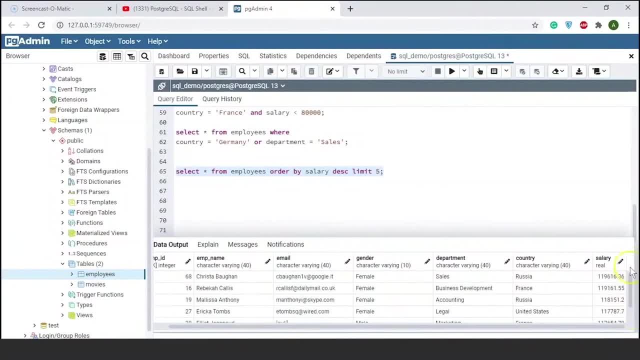 top five employees that have the highest salary. okay, so this is one method of, or one way of using the limit clause. now, in case you want to skip a number of rows before returning the result, you can use offset clause placed before the limit clause. so i'll write: select star from employees, let's say order by: 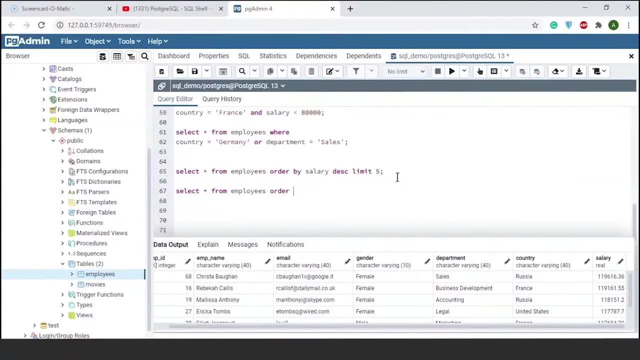 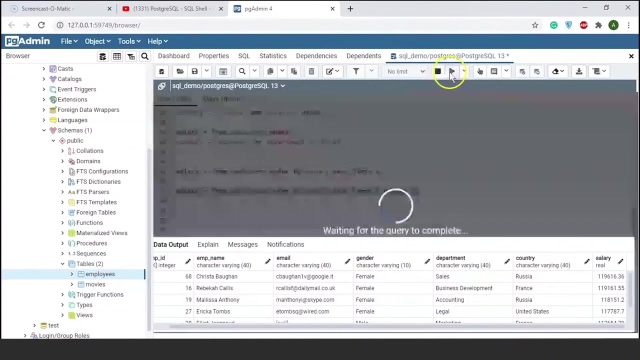 salary descending. this time i'm going to use limit 5 and offset 3.. so what this query will do is it will skip the first three rows and then it will print the next five rows. if i run this, there you go. so this is how the result looks like. 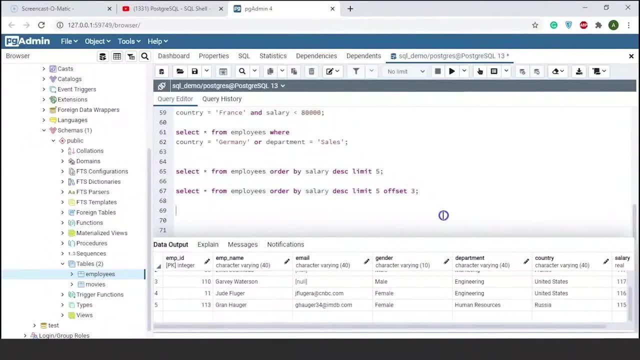 okay, now there is another clause, which is called fetch. let me show you how that works. i'll copy my previous sql query. i'll paste it here and here, after descending, i'm going to write fetch first, three row only. so my fetch is going to give me the first three rows from the top. 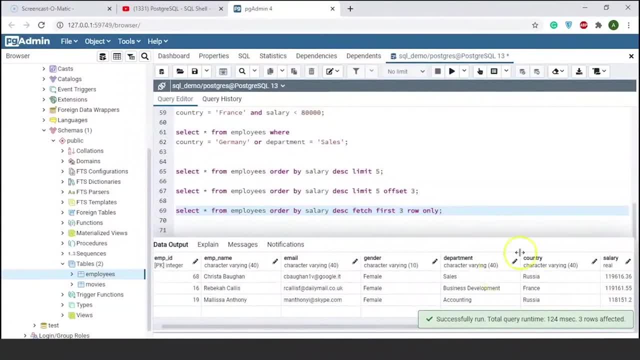 there you go. it has given us the first three rows and you can see the top three employees that have the highest salary, since we ordered it in descending order of salary. all right, you can also use the offset along with the fetch clause. i'll copy this again and let me paste it. 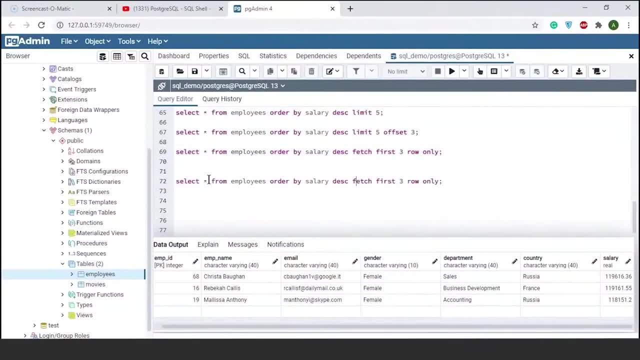 here you can also use the offset along with the fetch clause. i'll copy this again and let me paste it here now, after descending. i am going to write offset, let's say three rows, and fetch first five rows only. so what this sql query is going to do is it will skip the first. 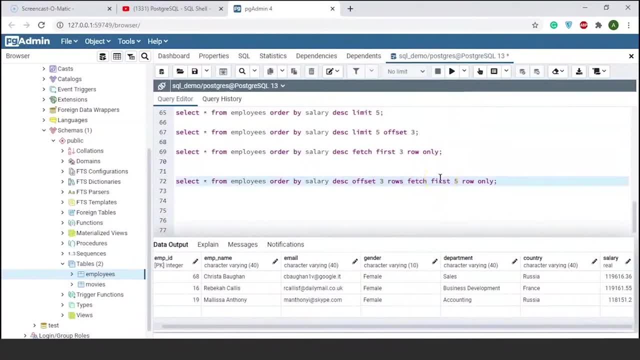 three rows of information and then it is going to display the next five rows. it is going to work exactly the same as we saw for this query. let me run it. there you go. so these are the first five rows of information, after excluding the top three rows. all right, we have another operator that is called as like in postgresql, so like is used to. 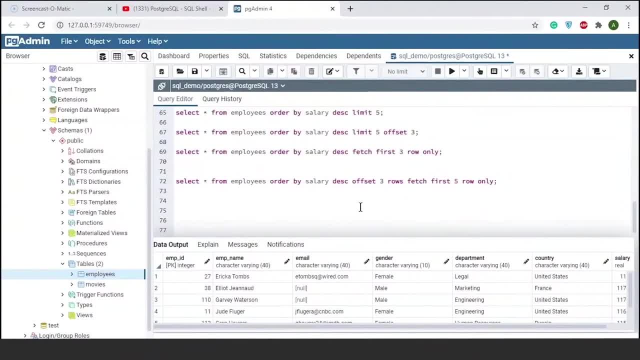 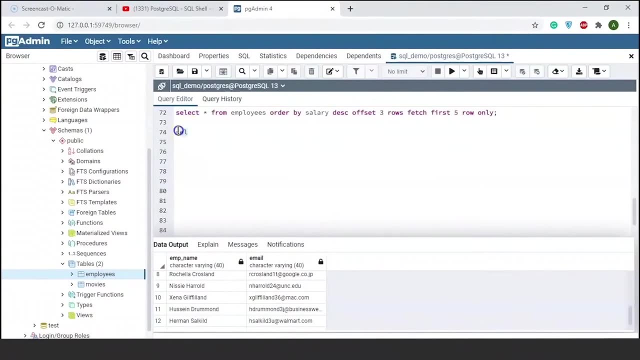 do pattern matching. so suppose you have a table that has the employee names. you forgot the full name of an employee, but you remember the few initials so you can use the like operator to get an idea as to which employee name it is. now let's explore some examples to learn how. 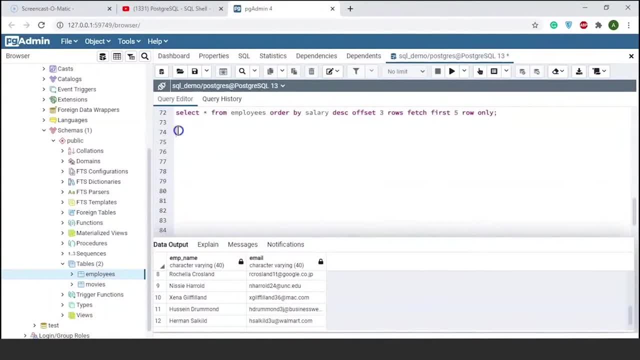 the like operator works in postgresql, so suppose you want to know the employees whose name starts with a, so for that you can use the like operator. let me show you how to do it. so i want to display the employee name and let's say i want to know their email ids from the table name that is. 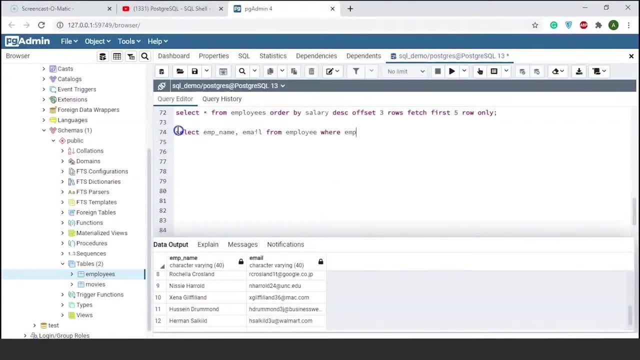 trade employee where disease would be there. since i want to know the employees whose name starts with a, so i'll write employ name like now. to use the pattern is within single quotes. i'll write a and then followed by percentage. now this means the employee name should have an a in. 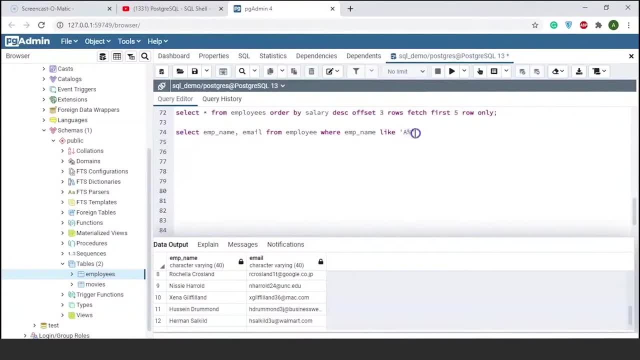 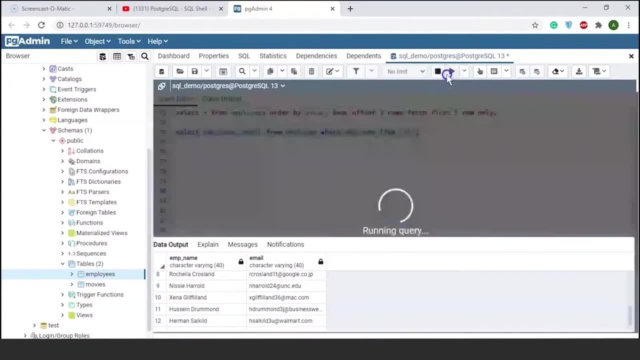 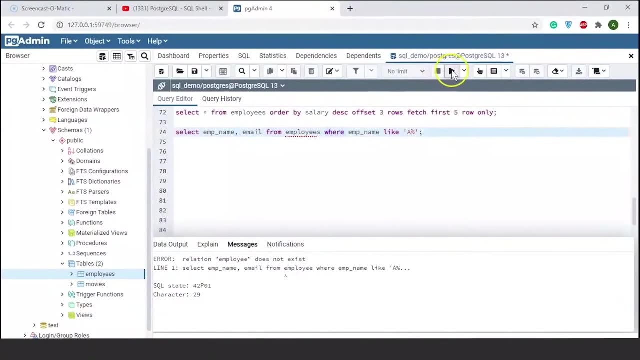 the beginning and percentage suggests it can have any other letter following a, but in the beginning or the starting should be a. if i run this, so there is an error here. the name of the table is employees and not employee. let's run this again. there you go, you can see there are 16. 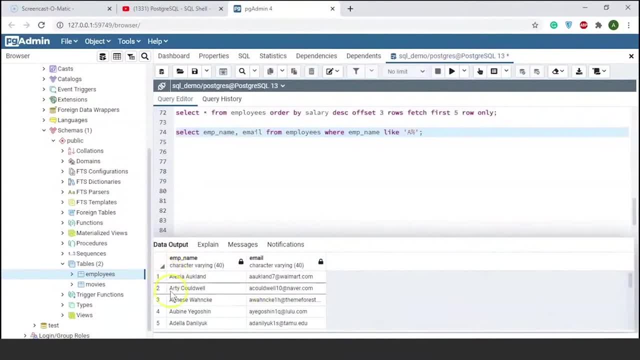 employees in our table whose name starts with a. you can see this column employee name. all of them have a letter a in the beginning. okay, now let me just copy this command or the query. i'll paste it here. let's say this time: you want to know the employees whose name starts with s. 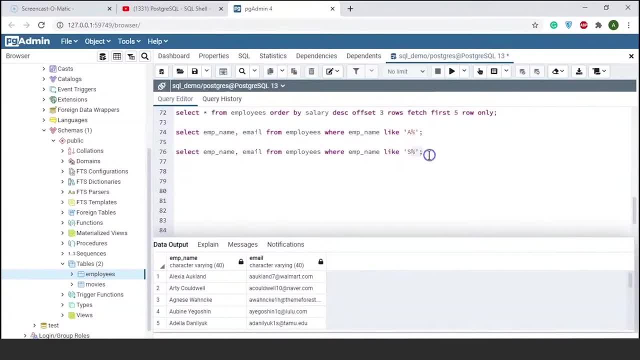 so instead of a, i'll write s. so this means the starting letter should be s and followed by it can have any other letter. if i run this, so there are 10 employees in the table whose name starts with s. okay, let's copy the query again, and this time i want to know the employees whose name ends. 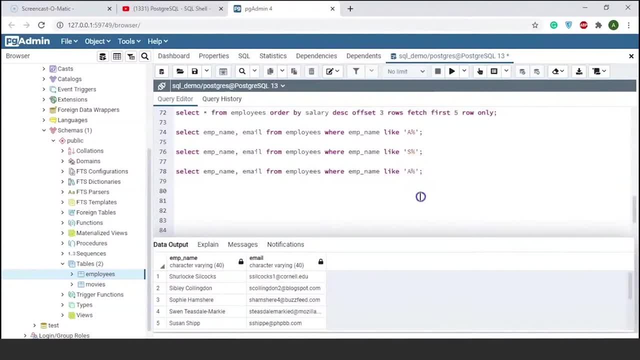 with d. now the way to do it is, instead of a percentage, i'll write this time percentage d, which means at the beginning it can have any letter, but the last letter in the string or in the name should be ending with d. now let me copy and run this. so there are 13 employees in the table whose name ends with: 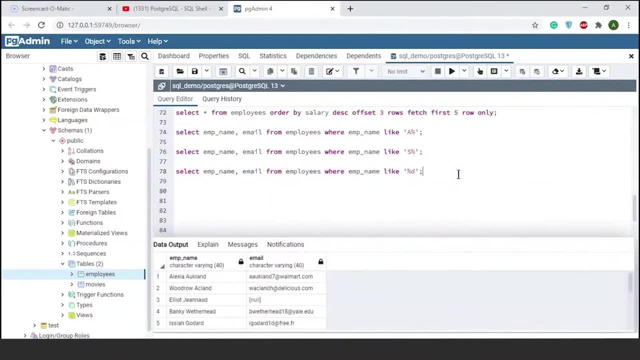 a, d. you can see it here. all right now. let's say, you want to find the employees whose name contains ish or have ish in their names, so the way to do is something like this. so i'll copy this now here: instead of a percentage, i'll replace this with percentage. 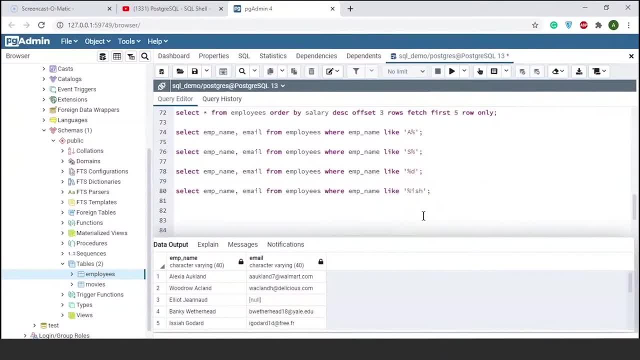 ish percentage. now, this means that in the beginning it can have any letter and towards the end also it can have any letter, but this ish should appear within the name. let me run and show it to you, okay, so there is one employee whose name contains ish. 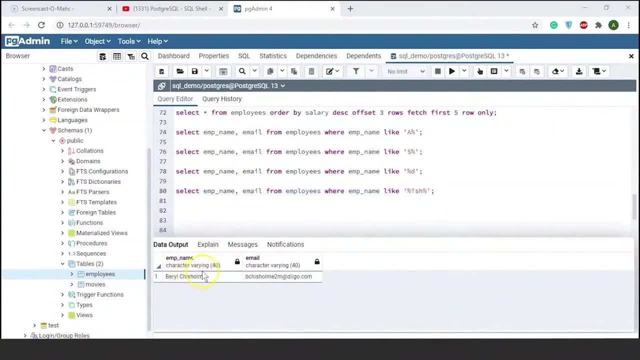 you can see here, there is an ish in the last name of the employee. all right now. suppose you want to find the employee name which has u as the second letter. it can have any letter in the beginning, but the second letter of the employee name should have u. now the way to do is i'll copy this and: 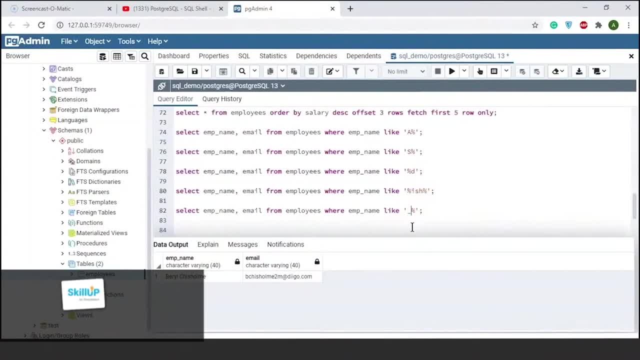 instead of a percent, i'll write underscore u, followed by percent. now, this underscore, you can think of a blank that can take any one letter, so the beginning can start with a, b, c, d or any of the 26 alphabets we have. then then it should contain u as the second letter, followed by any other. 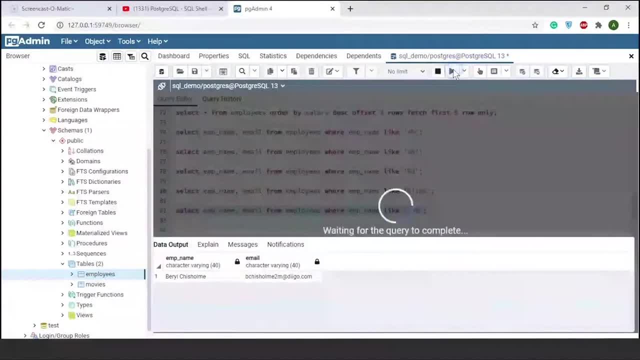 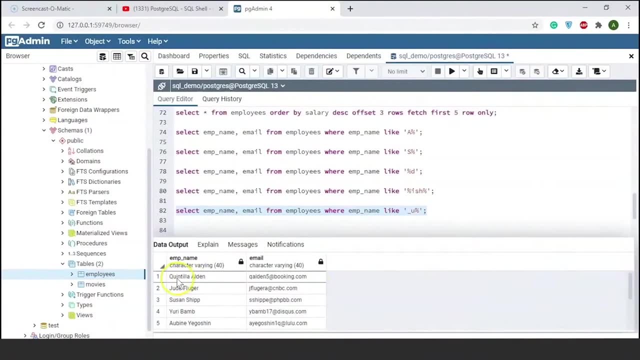 letter or letters. let me run this okay. so there are 10 employees in the table whose name has a u as the second letter. you can see these, okay. now, moving ahead, let me show you how you can use basic sql functions or inbuilt functions. so we'll explore a few mathematical functions now. 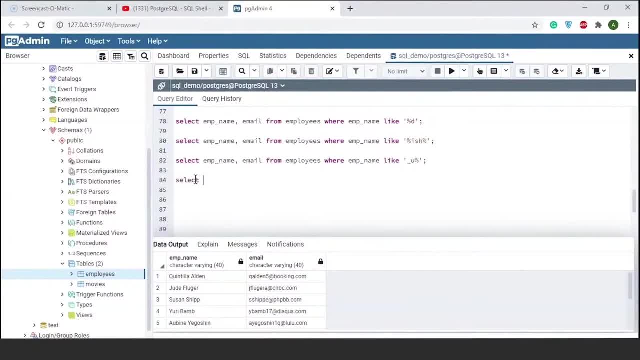 so let's say you want to find the total sum of salary for all the employees. so for that you can use the sum function that is available in sql. so i'll write sum and inside the sum function i'll give my column name, that is salary, from my table name, that is employees. let's see the result. this will return one unique value. 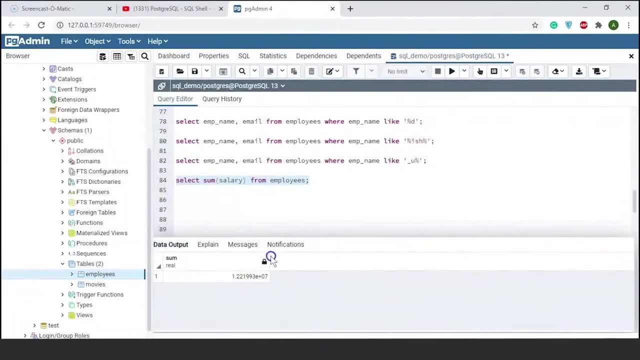 there you go. now. this is the total salary. since the value is very large, it has given in terms of e. now one thing to note here is if you see the output, the column says sum real. so this output column is not really readable. so sql has a method which can fix this. that is called an alias. so since we are doing an operation, 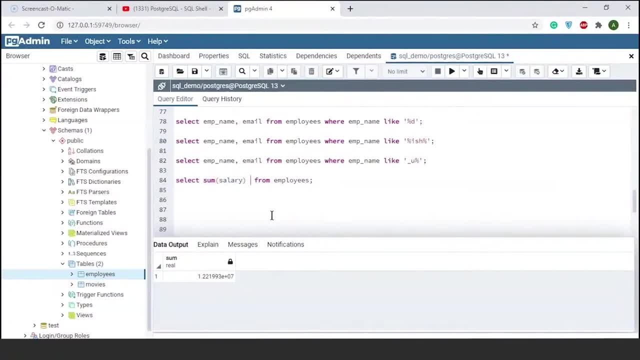 of summing the salary column. we can give an alias to this operation by using the as keyword. so if i write sum of salary as, let's say, total salary, then this becomes my output column. you can see the difference if i run this. okay, you can see. now in the output we have the total salary. now this is much more readable than 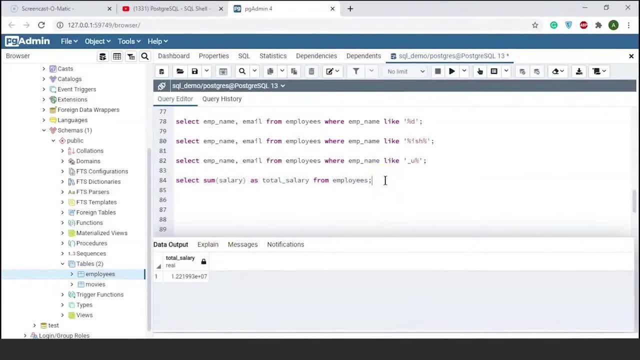 the previous one. so this is a feature in excel where you can use or give alias names to your columns or your results. now, similarly, let's say you want to find the average of salary for all the employees. now sql has a function called avg which calculates the mean or the 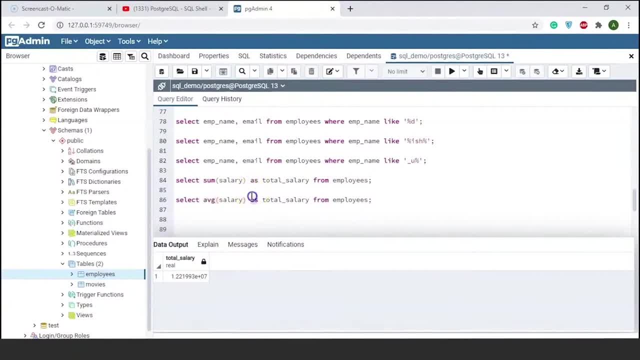 average salary. if i write avg and i can edit my alias name as well, let's say i'll write mean salary. let's run it. you can see the average salary for all the employees: it's around 81 000. okay, now there are two more important functions that sql provides us, which is max and minimum. 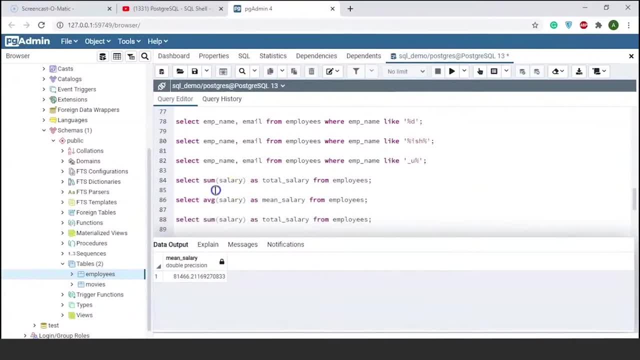 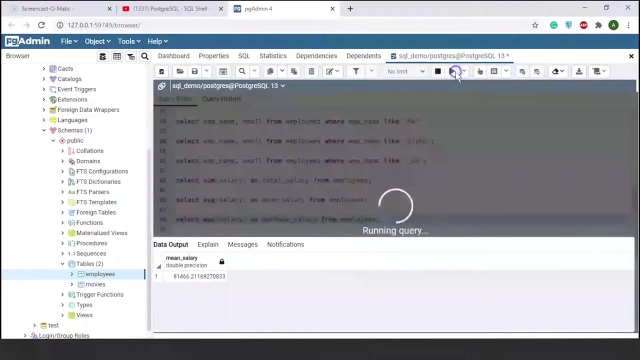 so if i write select maximum or max, which is the function name of salary, as, let's say, instead of total i'll write maximum. so this will return me the maximum salary of the employee. let's run it and see what is the maximum salary that is present in the salary column. all right? 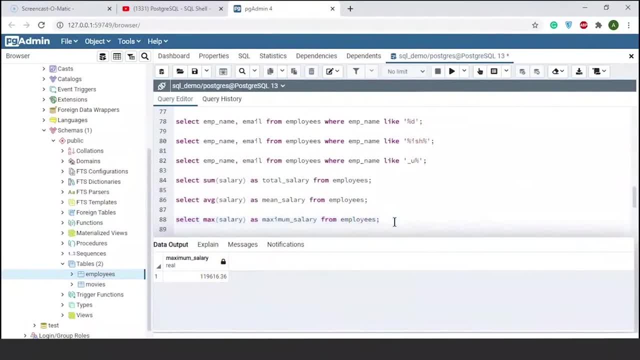 so we have one like nineteen thousand six hundred and sixteen dollars as highest salary of one of the employees. similarly, you can use the min function as well. i'll just write minimum and this will return me the minimum salary of one of the employees in the table. i'll replace the alias name as minimum. 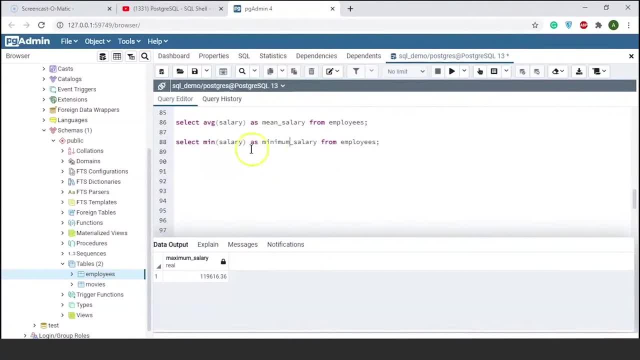 okay, now run it. this will give me the minimum salary that is present in our table. so it is forty five thousand six hundred and eighty five dollars. okay, now, let's say you want to find the minimum salary of one of the employees. you can find the count of department in the employees table. you can use the count function. 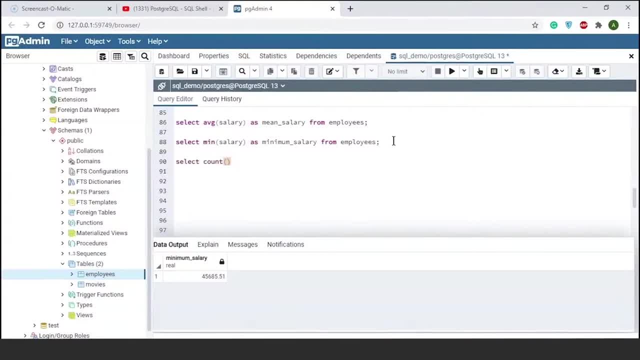 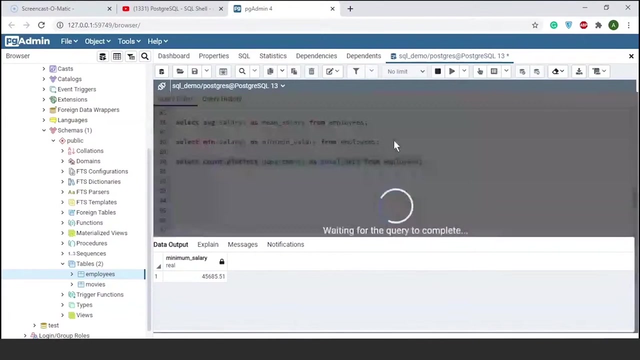 so if i write select count, let's say i want to know the distinct department name so i can write inside the count function distinct department as total departments. okay, okay, okay, okay from employees, let's run this. this will return me the total number of departments that are there. 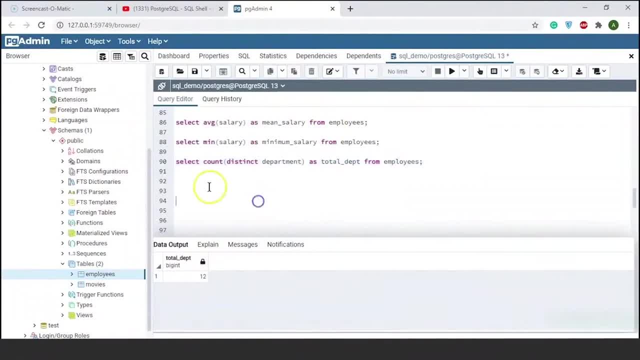 so it gives me there are twelve departments. okay, now let me show you one more thing here. if i write select department from employees, let's run this okay. so it has returned me hundred and fifty rows of information, but what i'm going to do is i'll place my 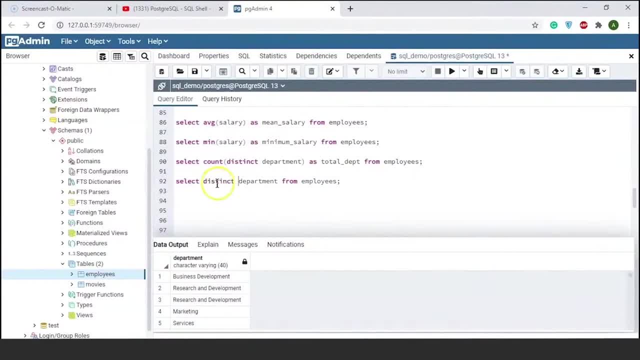 distinct keyword here, just before the column name, so that i can verify how many departments are there in total. there you go. so there are thirteen departments and one of them is null. so, moving ahead, we'll replace this null with a department name by updating our table. okay, so now let's update our department column. 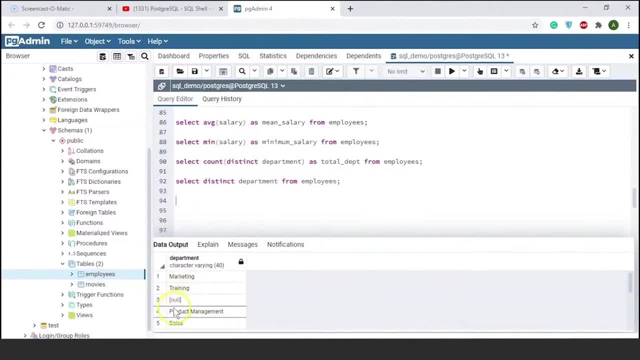 so what we are going to do is, wherever the department has a null value, we are going to assign a new department called analytics. so earlier we have also learned how to use the update command, so i'm going to show it again. so we'll write update, followed by the table name. 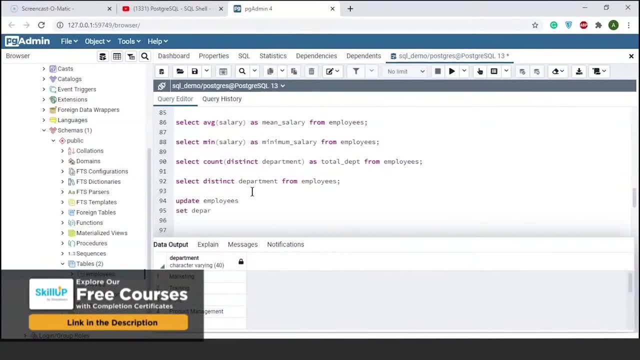 that is, employees. i'm going to set my column that is department equal to, within single quotes. my name of the department would be analytics. where department is, i'll say null. so wherever the department is, i'll say null. so wherever the department is, i'll say null. so wherever the 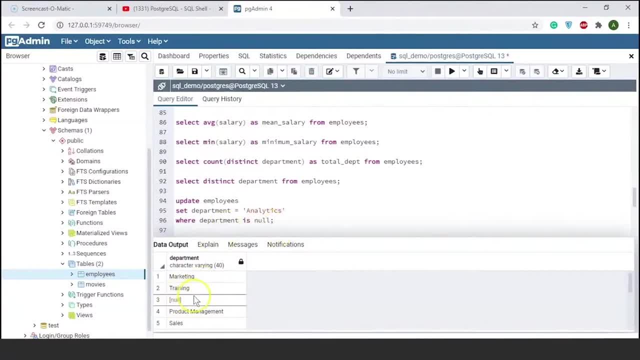 department has a null value will replace those information with department. that is analytics. let's run this. you can see query returned successfully. now let's say, i'll run this command again and this time you can see the difference. there you go. so we have 13 rows of 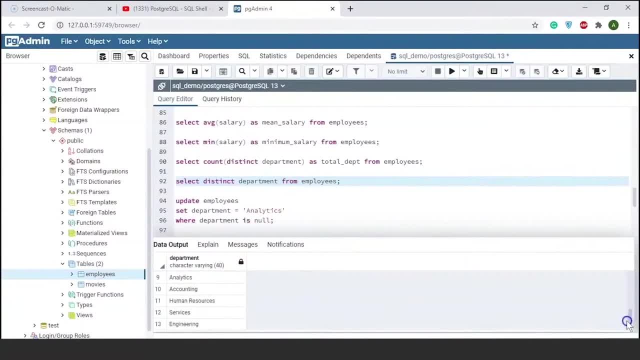 information and there is no null department. now we have added a new department, that is analytics. okay, now we are going to explore two more crucial commands or clauses in sql. that is group by and having. so let's learn how group by clause works in postgresql. so the group by statement groups. 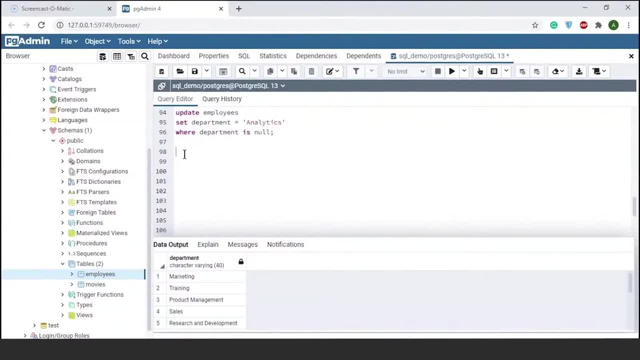 rows that have the same values into summary rows. for example, you can find the average salary of employees in each country or city or department. so the group by clause is used in collaboration with the select statement to arrange identical data into groups. so suppose you want to find. 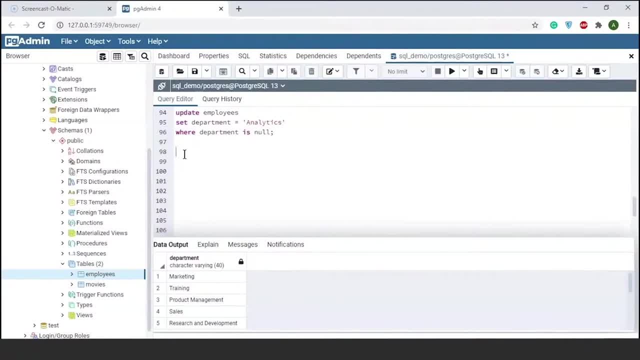 the average salary of the employees based on countries. you can use the group by clause, so let me show you how to do it. i'll write select. i want the countries and the average salary for each country, so i'll use the average function, that is, e, v, g, and inside the function i will place a group or a. 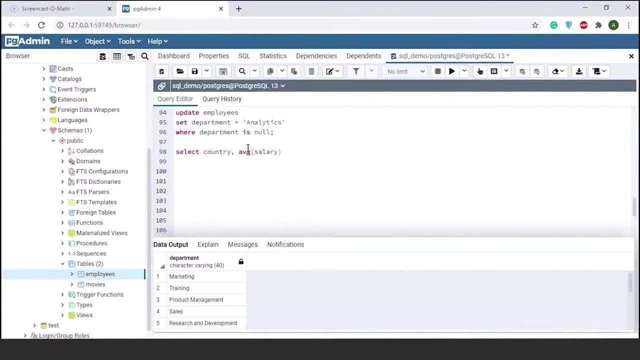 function. I'll pass my column, that is salary. I'll give an alias name as, let's say, average underscore salary from my table name. that is employees. next, I am going to use my group by clause, so I'll write group by, since I want to find the 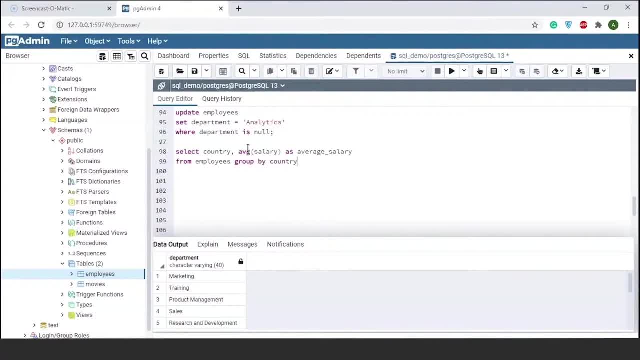 average salary for each country. so I'll write group by country name. let's give a semicolon and let me run it. I'll use f5. there you go. so here on the left you can see the country names. we have Israel, Russia, Australia, United States, France. 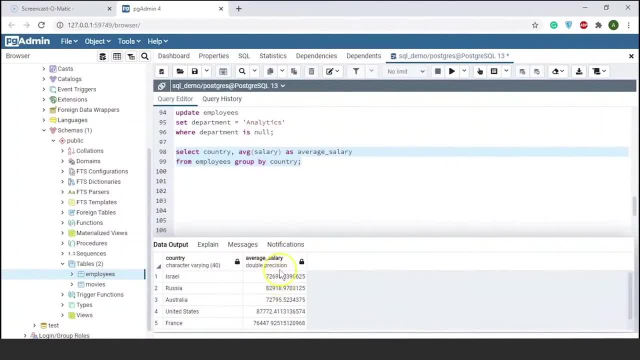 and Germany, and on the right, the second column, you can see the average salary for each of these countries. now you can also order the result in whichever way you want. suppose you want to arrange the results based on the average salary, so you can use the order by clause. 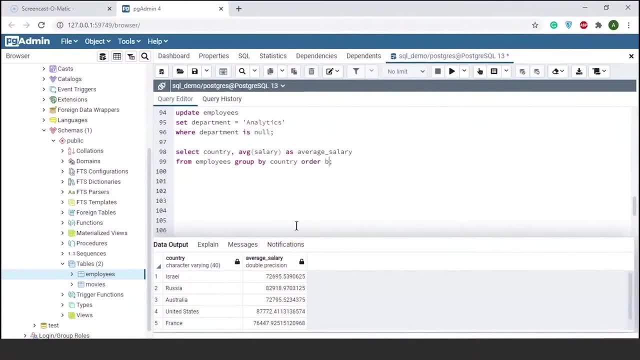 after the group by clause, so I'll write order by here. you can use the alias name. that is average salary. this is actually average underscore salary, and let's say I want to arrange it in descending order, so I'll write DESC. now let's run this. you can mark the difference in the average salary column. there you go. 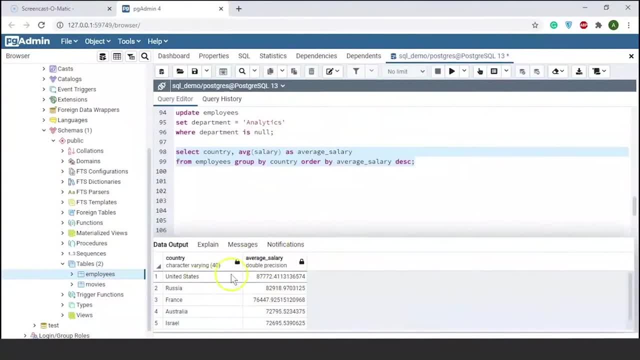 so, as per our result, in United States the average salary is the highest, and, if I scroll down, the average salary is the lowest in Germany. now let's see one more example, using group by suppose, this time you want to find the maximum salary of male and female employees. you can do that too, so let me show you how to do it. 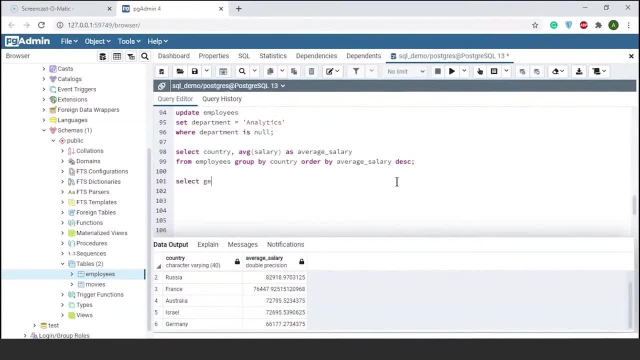 so I'll write select. this time we want to find the maximum salary based on gender, so I'll select my gender column comma and this time I'll use my max function. since I want to find the maximum salary for male and female employees, I'll give an alias name as maximum underscore salary from my table, that is employees. 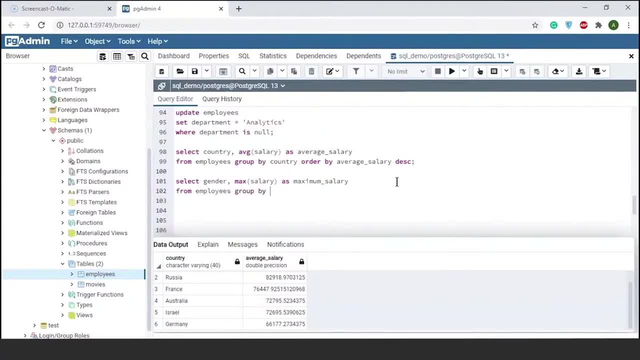 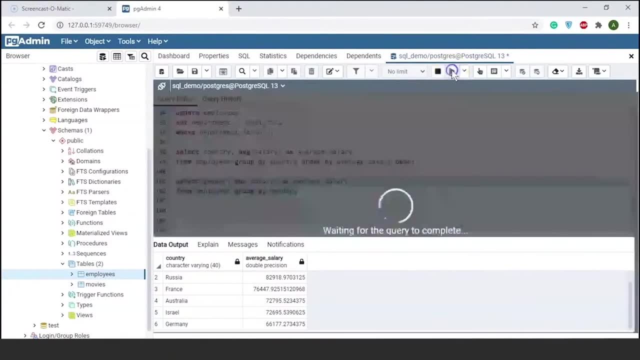 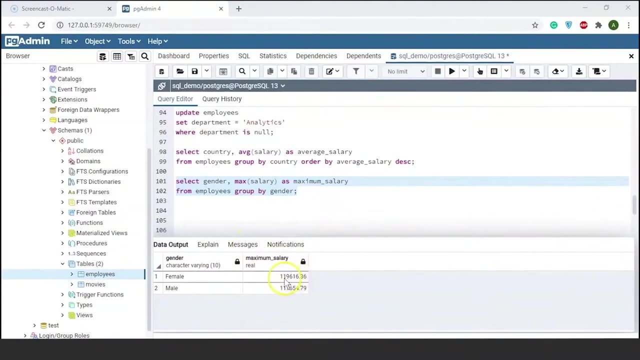 grouped by. I'll write gender, okay, so let's run this. there you go, you can see. so one of the female employees had a higher salary of $1,19,616, while of that of a male was $1,17,654. alright, now suppose you want to find the count of employees based on each country. 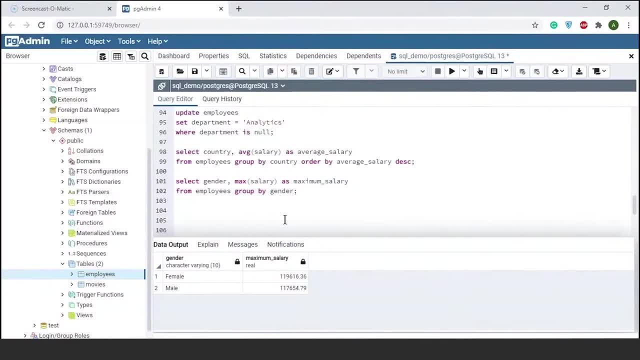 you can use the count function along with the group by clause. so I will write the select statement, select- since I want to count the employees based on each country. so I will first select my country column and then I am going to use the count function. I will write count- emp. underscore id. 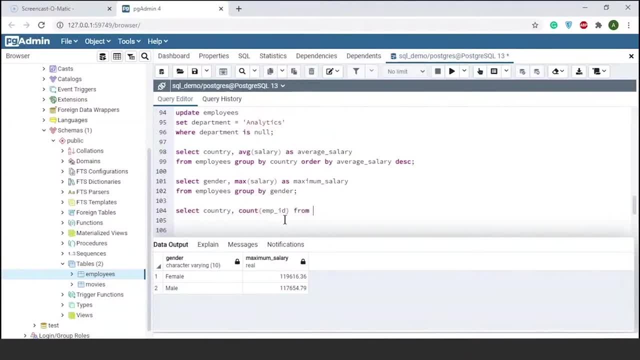 from my table name, that is, employees. I am going to group it by country, so this query will give me the total number of employees from each country. you can see here: Israel, there are 4 employees. in Australia, there are 4 employees. in Russia, we have 80 employees. 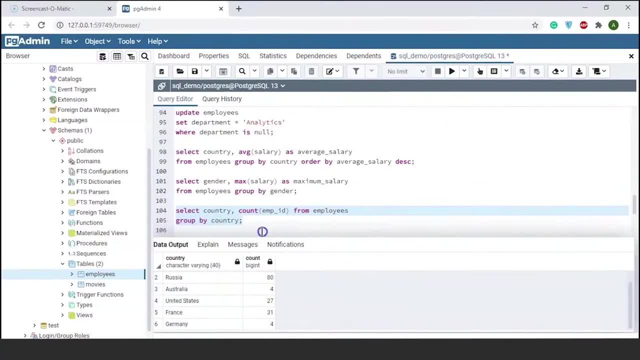 in France, there were 31 in United States, we have 27, so on and so forth. let me scroll down. ok, now it's time to explore one more clause, a very important clause that is used in Postgres SQL, that is having. so the having clause works like the where clause. 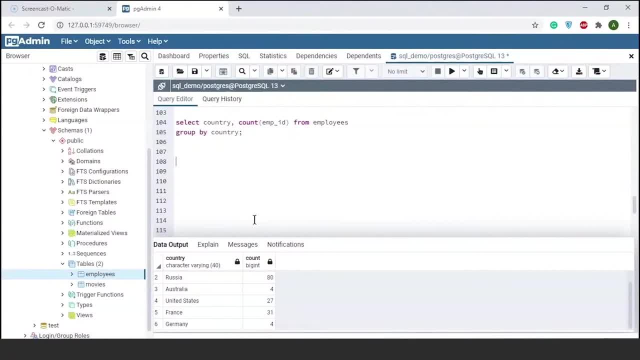 the difference is that the having clause works like the where clause. where clause cannot be used with aggregate functions, the having clause is used with the group by clause to return those rows that meet a condition. so suppose you want to find the countries in which the average salary is greater than $80,000. 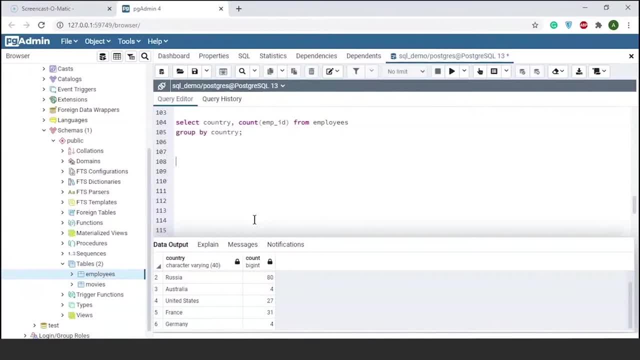 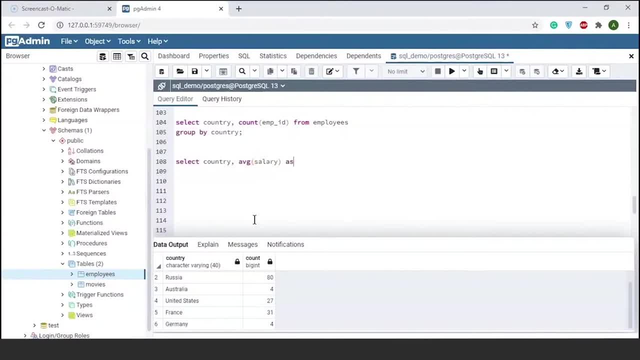 so I will write avg of select country. so I will write avg of select country. I can give an alias name as average salary from employees. now I am going to group it by each country, so group by country column, since I want to find the countries in which the average salary is greater than 80,000. 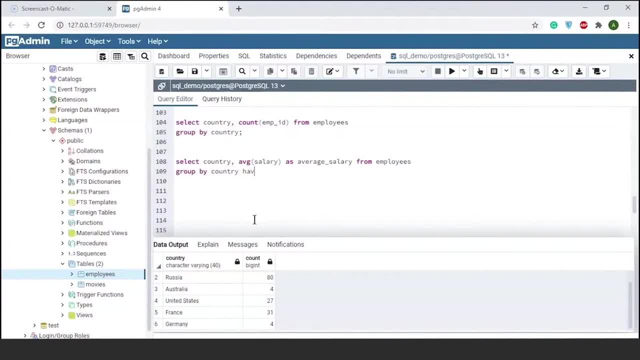 so I will use having clause. after the group by clause, I'll write: having average of salary is greater than 80,000. now, this condition cannot be specified in the where clause, so we need a having clause. you cannot use aggregate functions along with where clause. let me 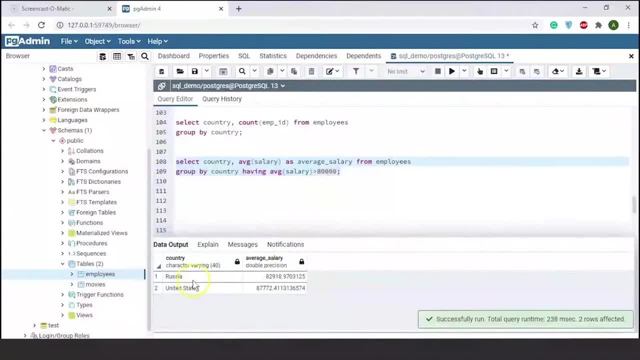 just run it now. there you go. so we have Russia and United States, where the average salary is greater than $80,000. all right, now let's say you want to find the count of employees in each country where there are less than 30 employees. so for this I am going to use the count function first. 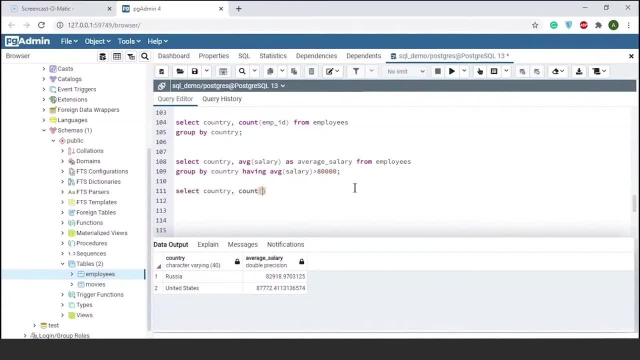 let me select the country column. then I'm going to use the count function and in the count function I am going to pass my employee ID so that we can count the number of employees from my table, that is employees. now, if you want, you can use an alias name for. 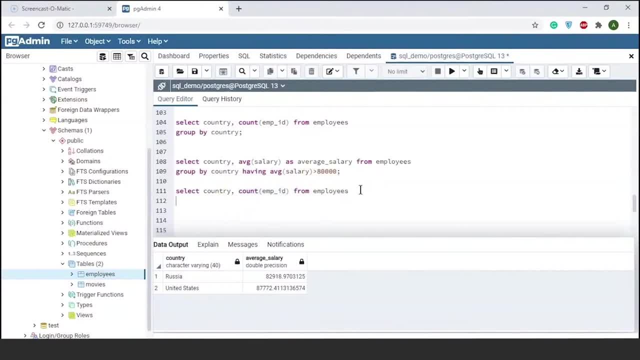 this as well, but I am just keeping it for the time being. I'll write group by country. next I'll write having count of employee ID less than 30. so this is the number of employees. so this will return me the countries in which there are less. 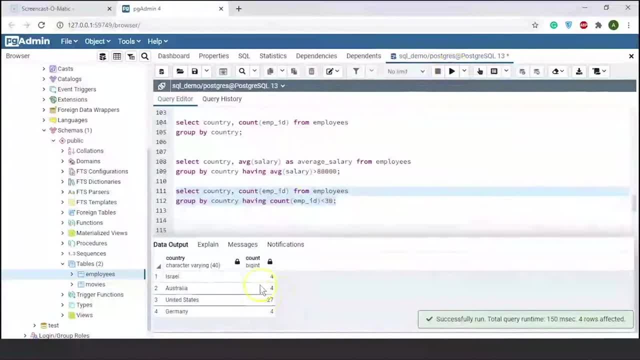 than 30 employees. let's run it. you can see here: Israel, Australia, United States and Germany are the countries in which there are less than 30 employees. okay, now, if you want, you can use the order by clause as well, so suppose I will write here: order by count of employee ID. 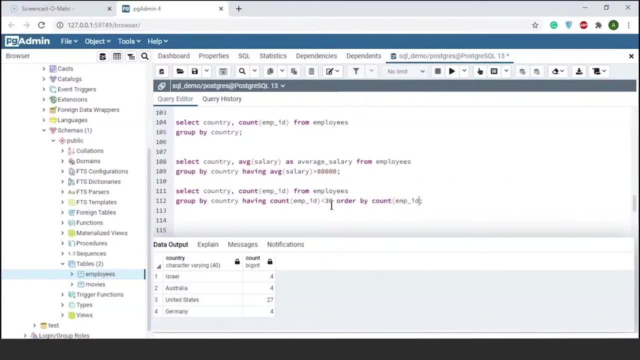 you suspension. so in the query column after that you can mark this land chart as label for employees and then in an actualгов, let's say, ID count: soрей mc kor завис submitted ox. what does this do? so what does this do? wonder, i have get people has, so I can. 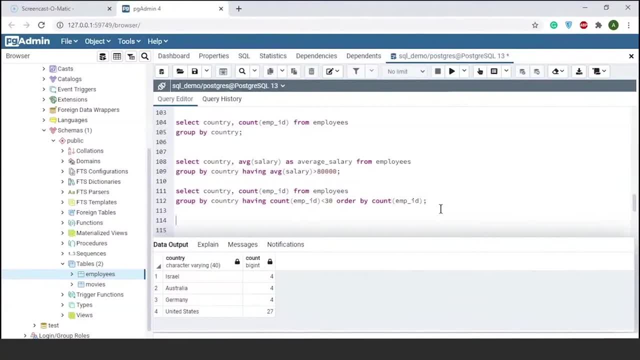 see there are no new people, correct? see, I got few people. has indicated field somebody, Everything the rest of them in case it's something you can do if you want to filter the dollars a little bit. So what this will do is it'll arrange my result in ascending experiences. 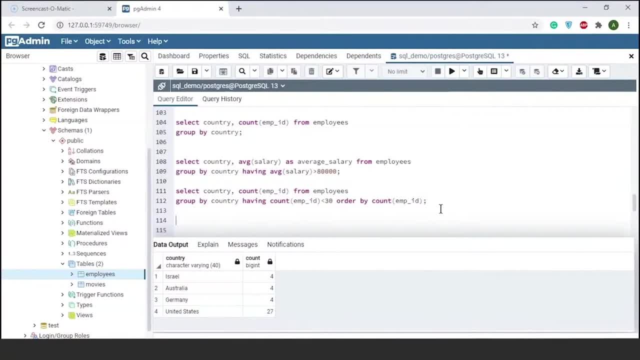 Now in PostgreSQL, the case expression is same as if-else statement in any other programming language. It allows you to add if-else logic to the query to form a powerful query. Now let me just scroll down and I'll show you how to use a case statement. 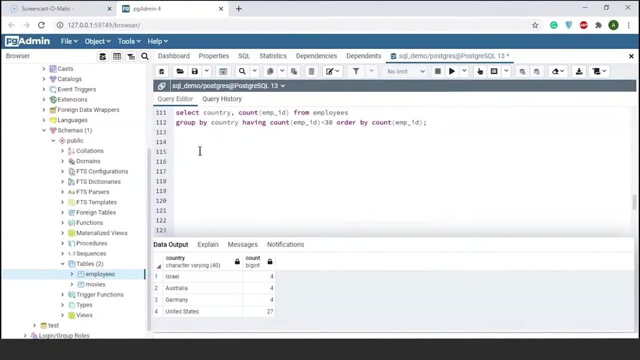 This is very similar to your if-else statement that you use on Excel, in C++, in Python or any other programming language. So what I'm going to do is I'm going to write a SQL query that will create a new column. 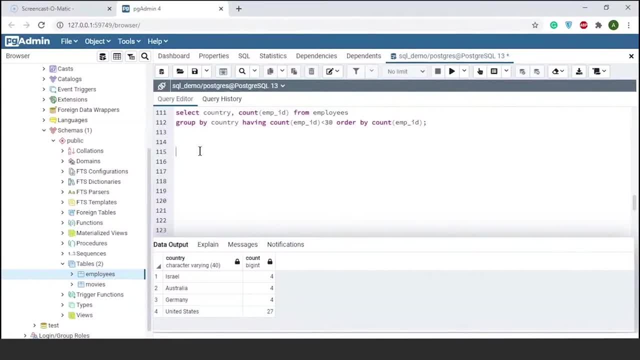 And the name of the column would be, let's say, salary range. So I'm going to divide my salary- Suppose if the salary is greater than $45,000 and if it's less than $55,000, in the new column that is, salary range, we are going to assign a value: low salary. 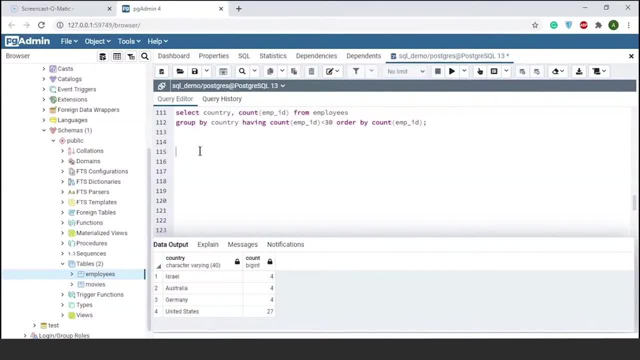 Now, if the salary is greater than $55,000 and if it is less than $80,000, we are going to assign a value, that is, medium salary. If the salary is greater than $80,000, we'll assign a value: high salary. 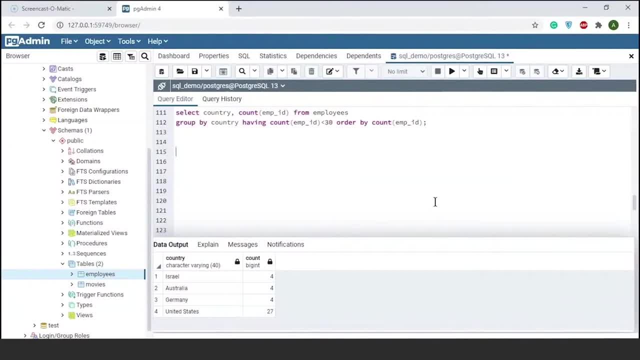 So all this we are going to do using our case expression in PostgreSQL. So I'll start with my SELECT statement, But before that, let me show you how to write a comment in PostgreSQL. So you can write a comment by giving a double dash. 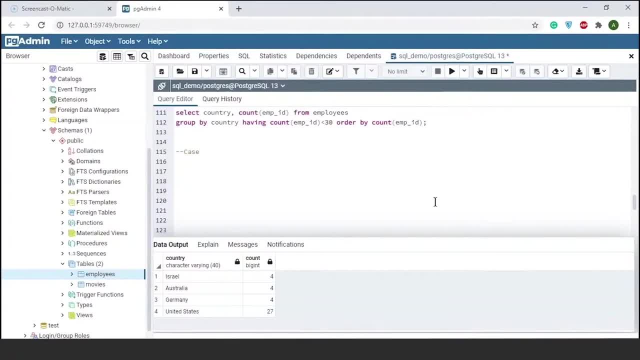 Comments are very helpful because they make your codes or the scripts readable. I'll write case expression In PostgreSQL. Similarly, if you want, you can go to the top and let's say: here you can write with double dash having clause. 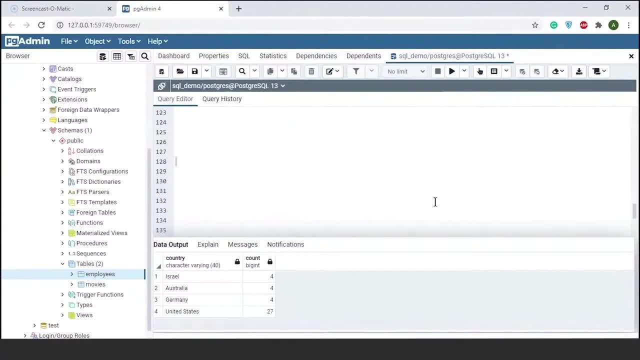 Okay, let's come down. So I'll write my SELECT statement. as SELECT I want the department, The country and the salary column. I'll give a comma and I'll start with my case statement. I'll write case when my salary is greater than $45,000 and my salary is less than $55,000. 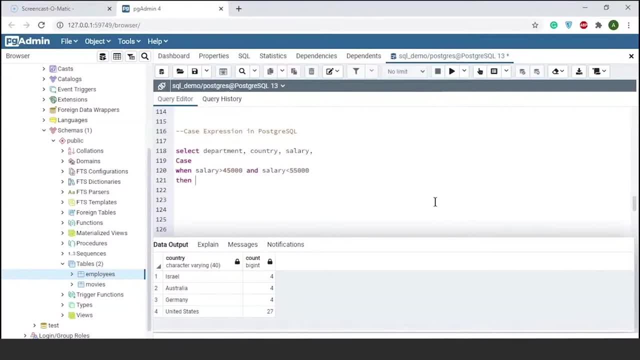 Then the result would be: within single quotes, I'll write low salary, So this is exactly like an if-else condition. Next, I'll write another case when salary is greater than $55,000.. And salary is less than $55,000. 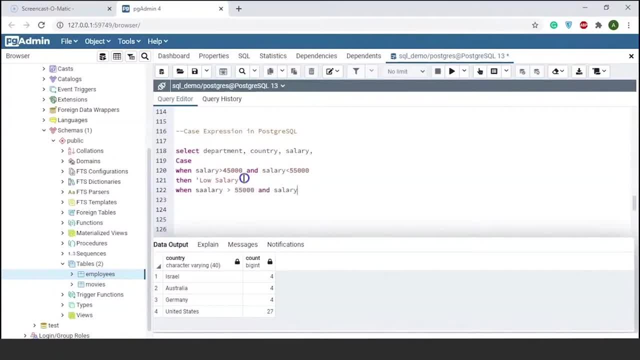 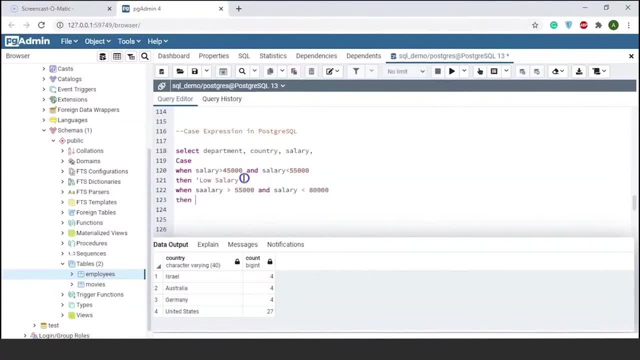 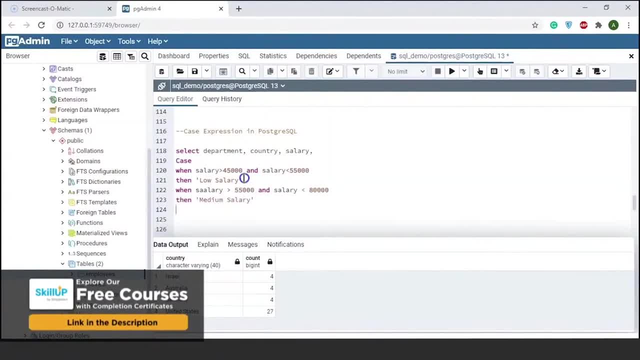 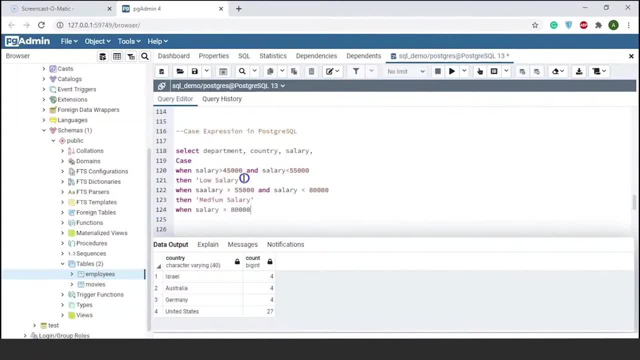 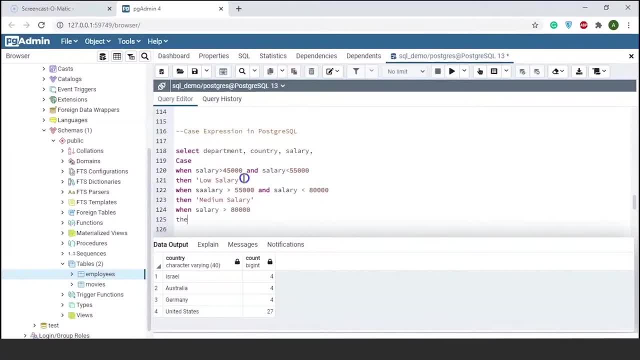 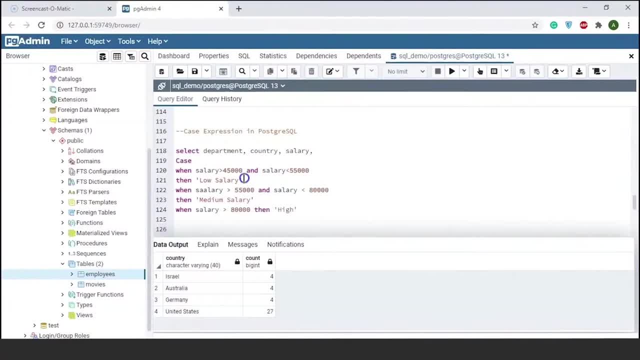 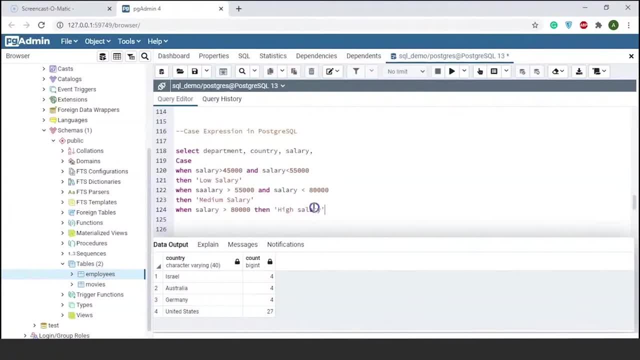 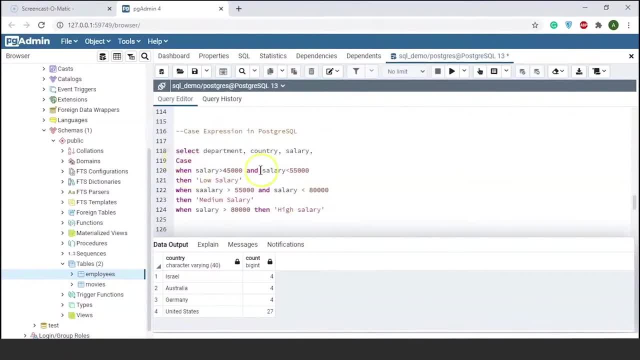 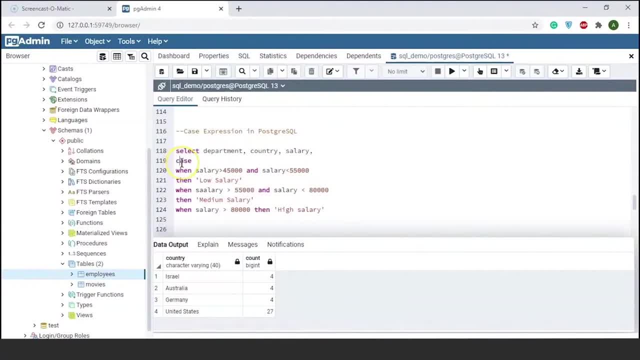 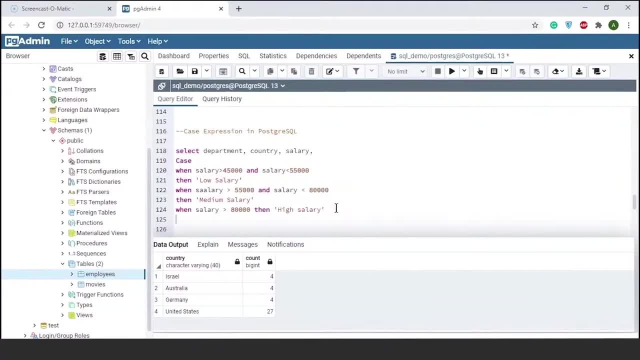 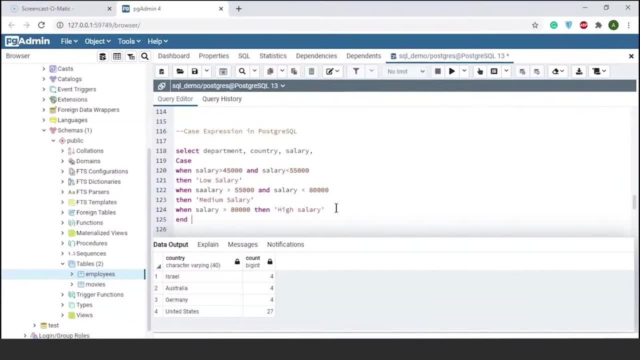 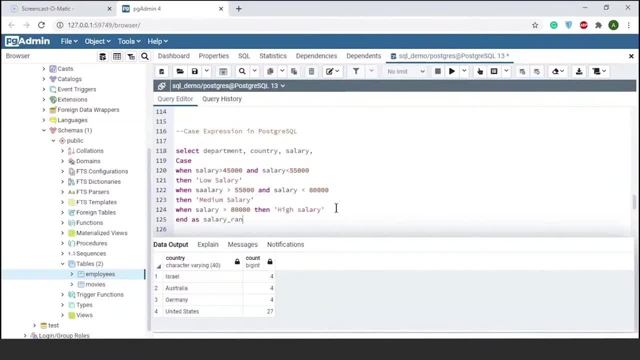 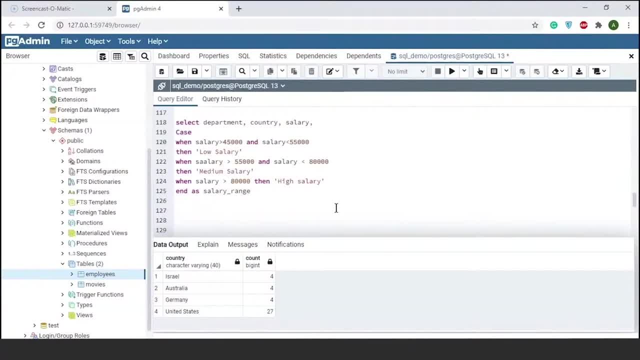 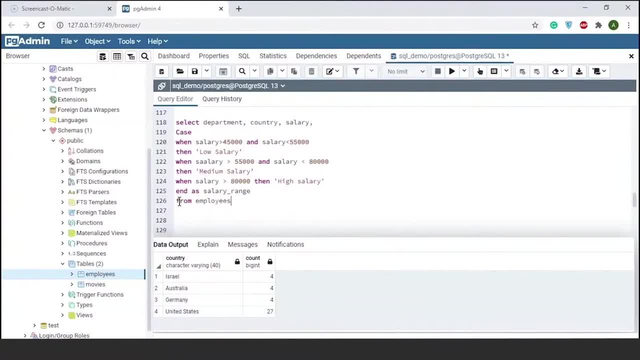 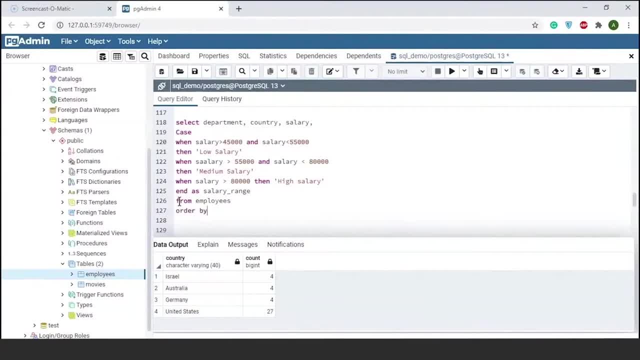 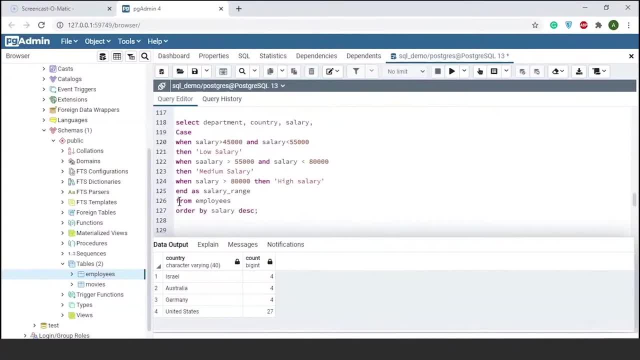 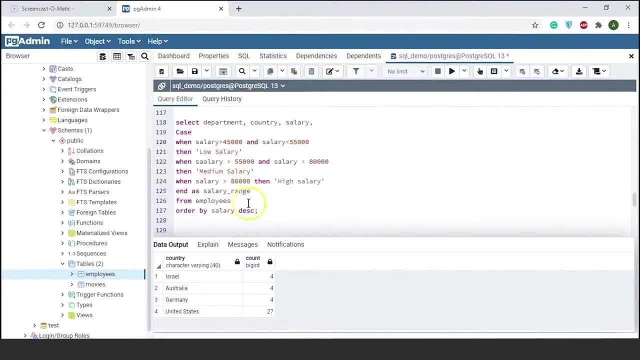 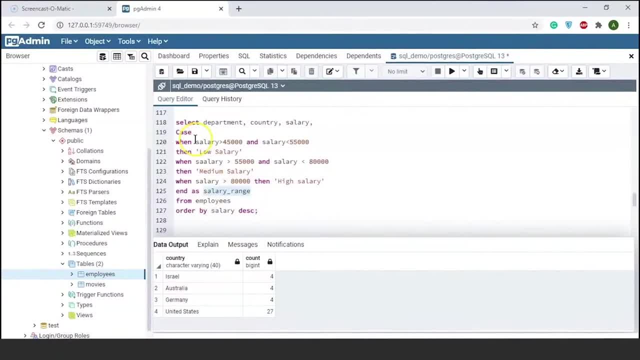 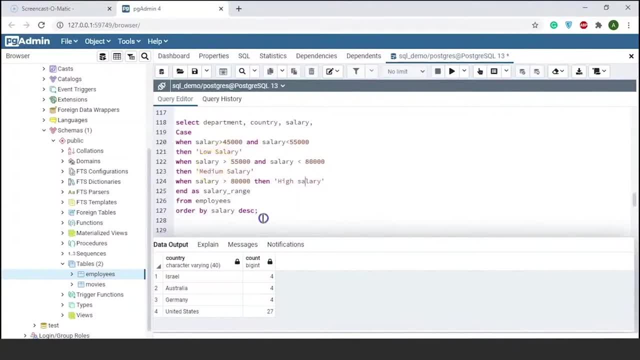 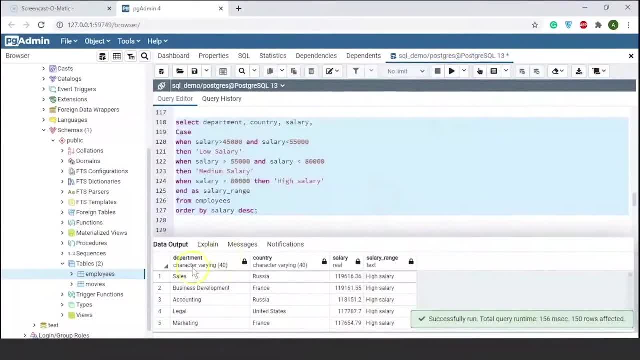 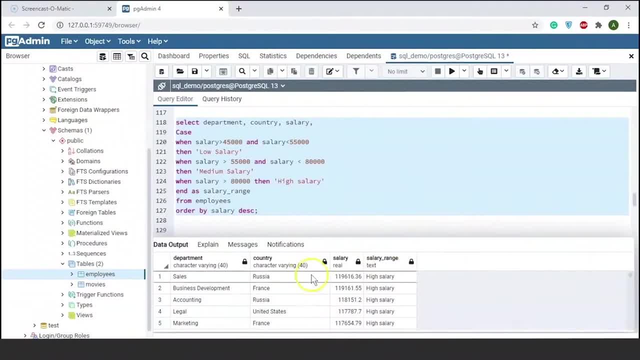 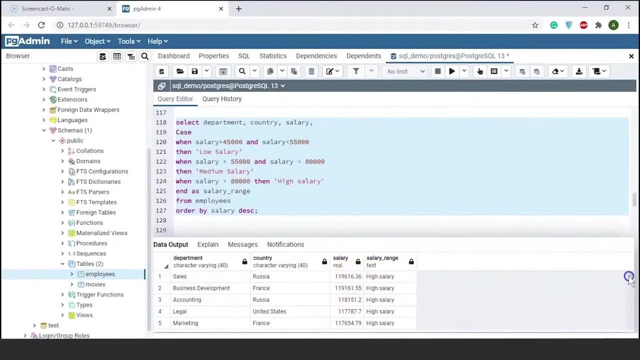 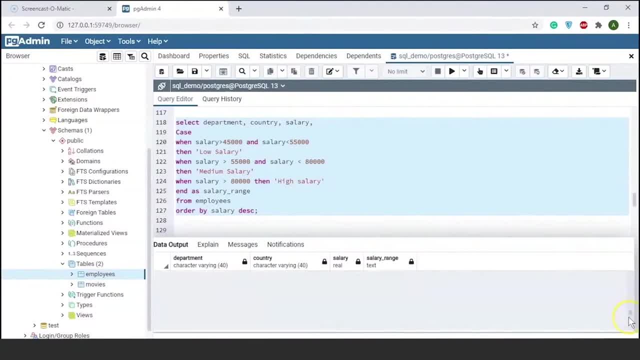 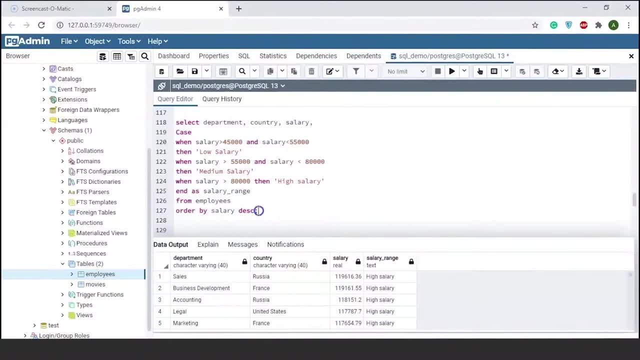 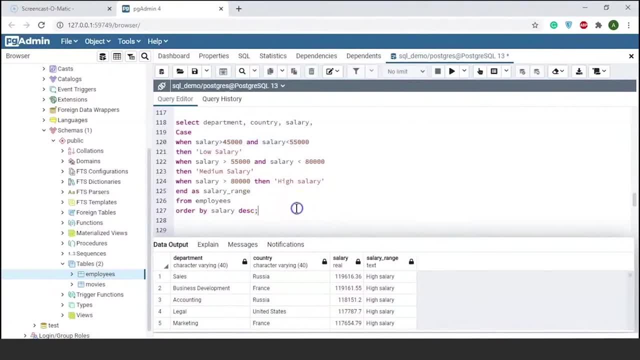 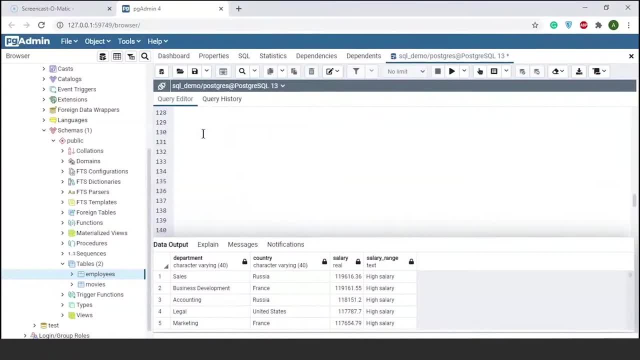 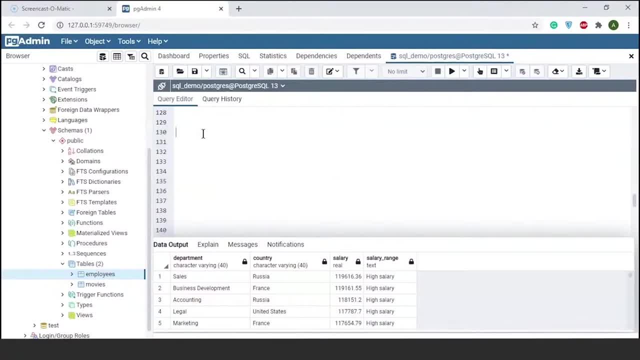 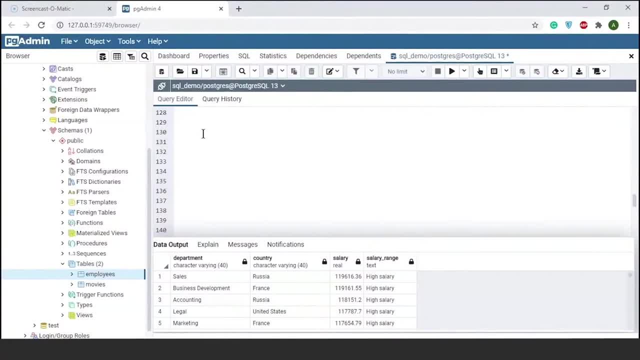 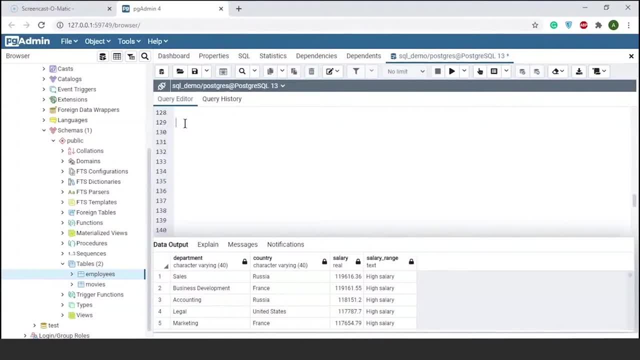 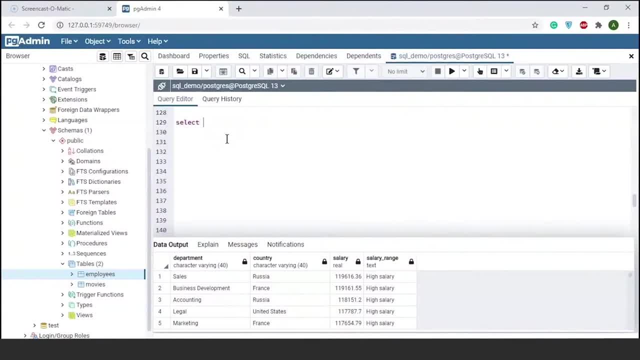 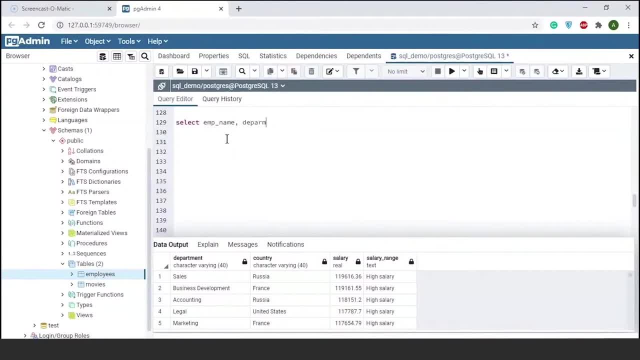 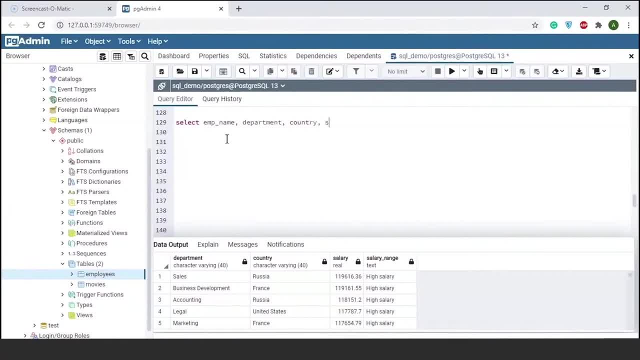 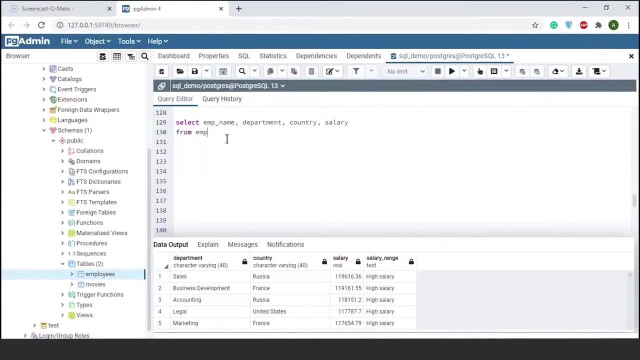 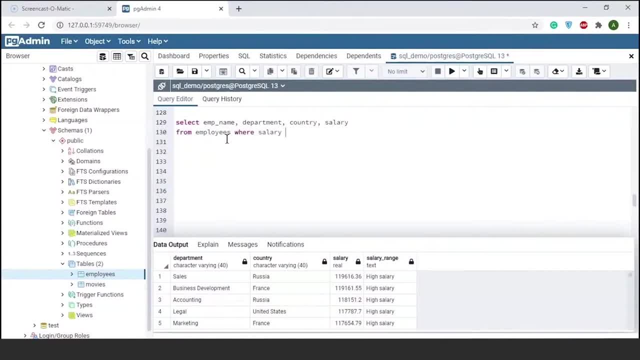 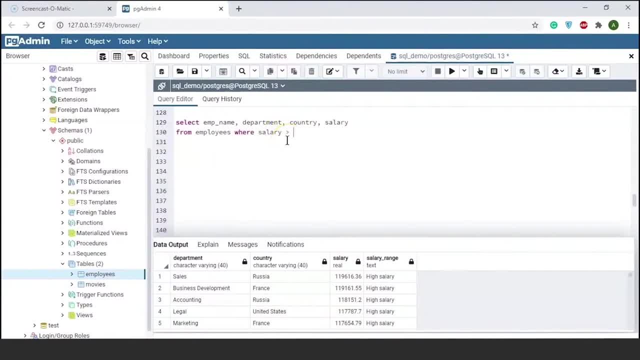 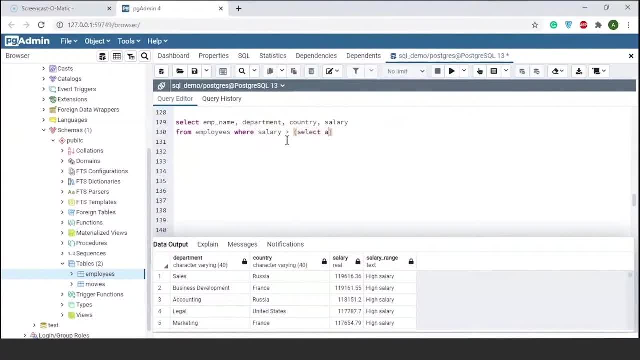 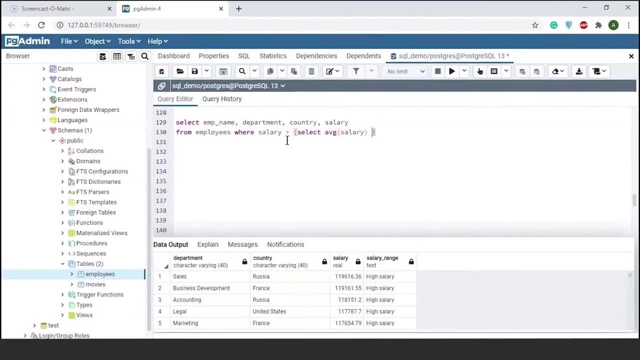 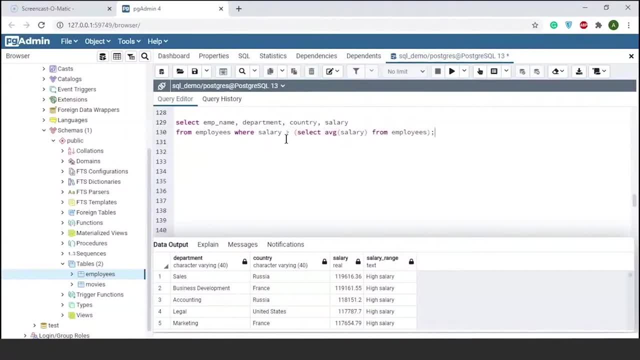 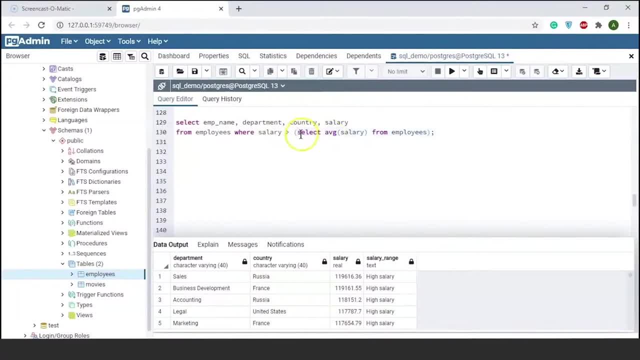 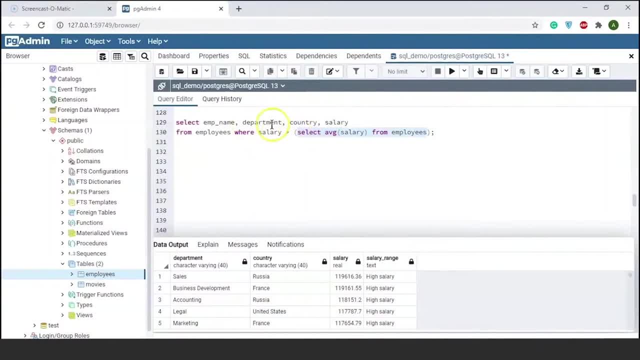 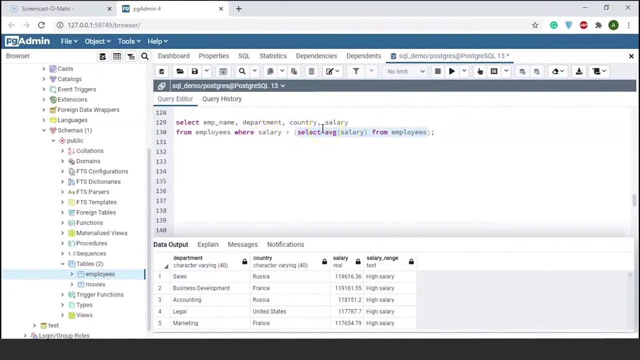 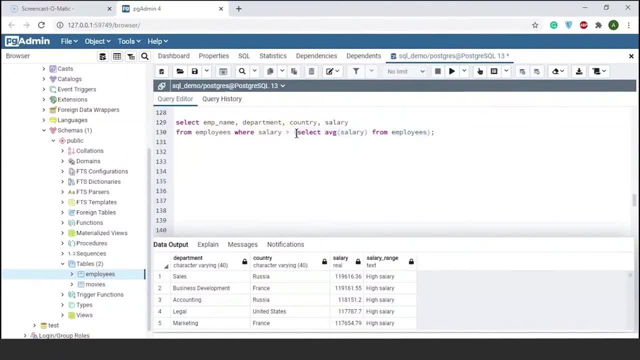 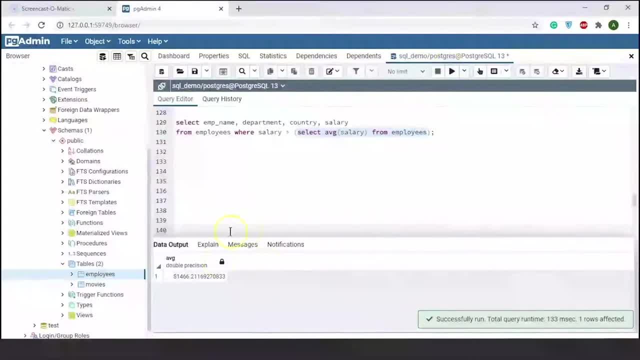 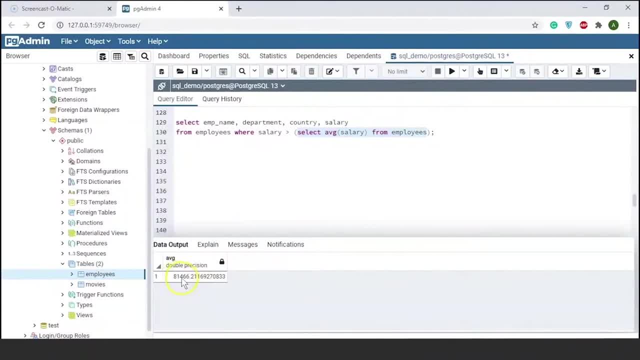 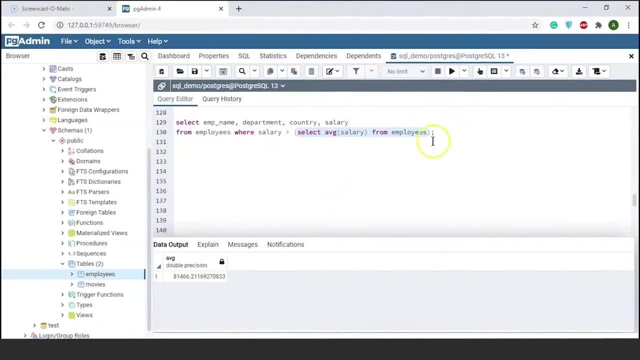 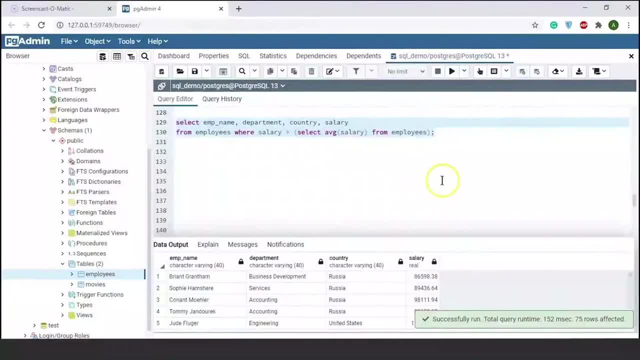 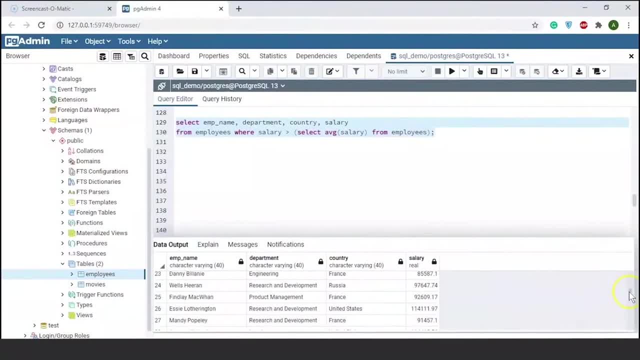 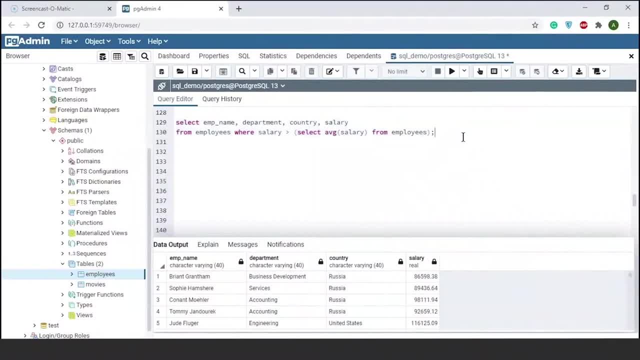 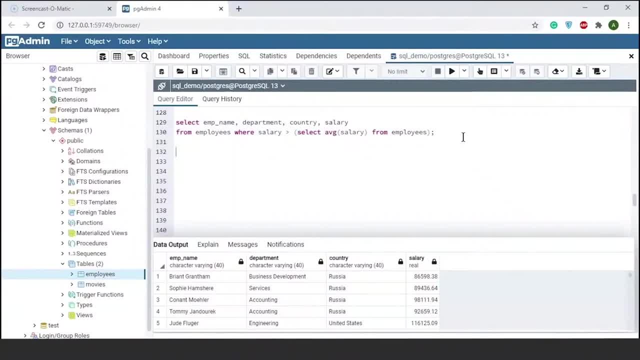 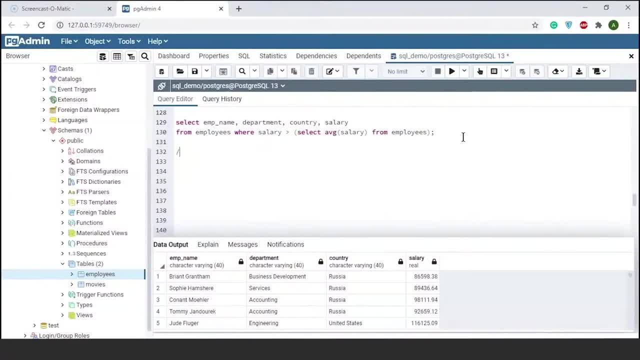 instead of a double dash you can use the forward slash, an asterisk, and inside the asterisk you can write, let's say, SQL functions and you need to close this. so I'll give another asterisk and a forward slash. this is also a comment in PostgreSQL. 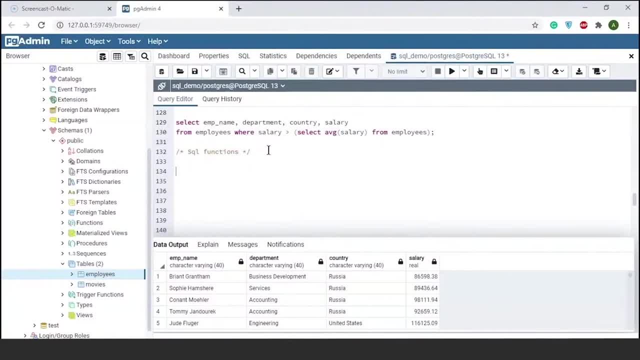 all right. so first of all we'll explore a few math functions. so there is a function called aps which is used to find the absolute of value. so if I write select abs of, let's say, my sub-constants, I'm always speak with the ball. 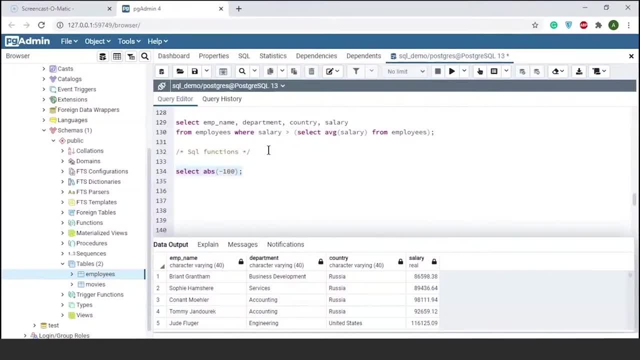 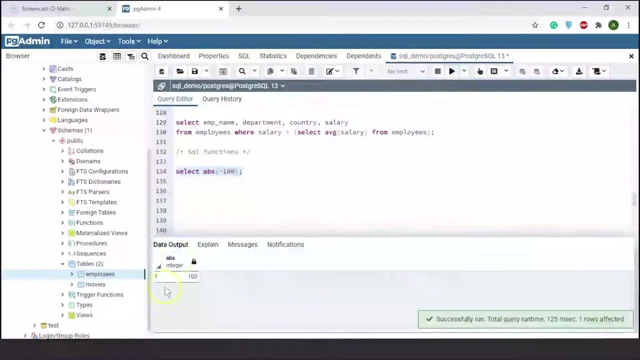 it is going to return me positive 100 or just 100. because, as you know, it is going to return me positive 100 or just 100. because, as you know, the absolute of any value now will remove the negative sign involved in the thoughts. there you go. original input was minus 100. the absolute of minus. 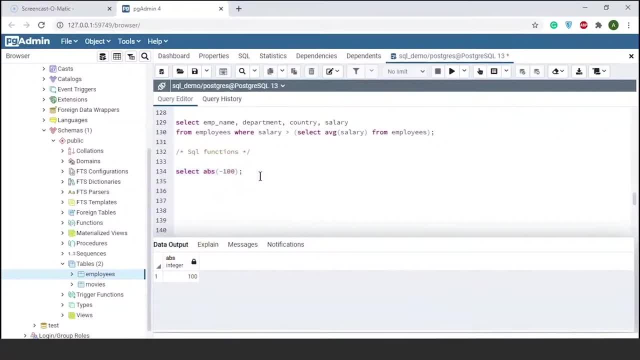 hundred is plus. I don't thinking about that, but my subconscious. let's see they thinking. another reason: that is called the greatest function in postgreSQL will return the greatest number in a range of numbers. so suppose I write select greatest important thing. I knew it and inside the greatest function and it's a. 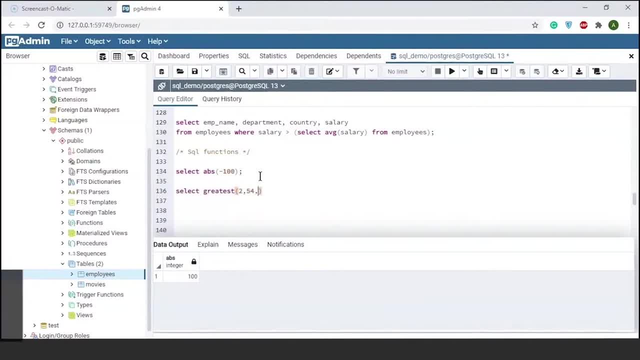 I'll pass in a few numbers. let's say two. we have everything. we're just randomly passing a few numbers. I have millions and billions food, but the most important thing, it's the family. keep your family healthy. good, and let's say your family, because this is the most important. you will see that of course you have. 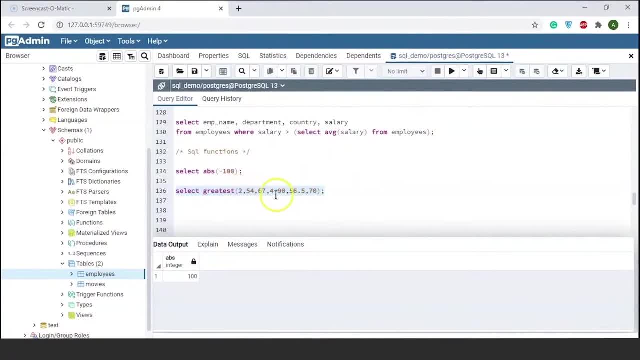 greatest function live on the greatest life integer value or greatest number, that is, in this case, 90 was the largest number or the greatest number, so we got the result as 90 again. you can use an alias for each of these statements. I'm always say it was like greatest. we also have function called least, because when I left my 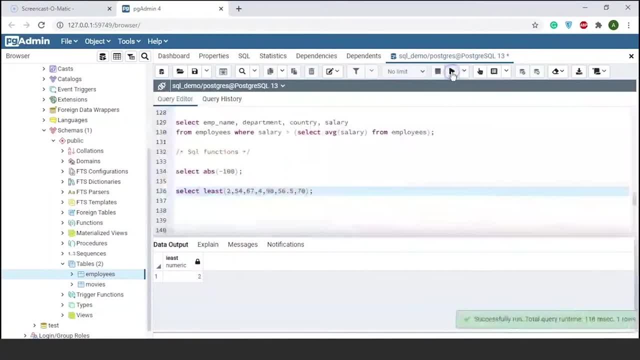 family with 11 years old to live in a different world. this is Lisbon, so the result is 2, because we used the least number that is present different part of the world in this selection. I was cried almost every day to miss my family, but I'm not going to bardzo. 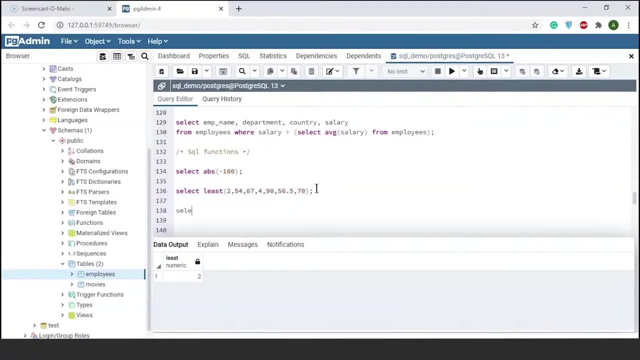 regret return the semicolon division probably the more right. more sins moments are in my life that I livester who sticks to parenthesis. so let's say, without速ie files you cannot slightly nothing, so I did it, as you can see, will sacrifice foot, my family too, and I think it was so. is that, as did, a good option? 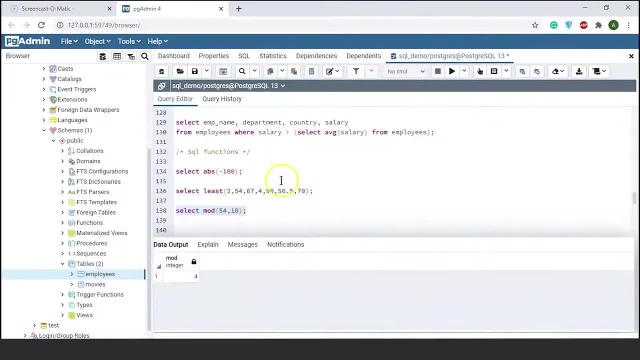 it has written the remainder 54 divided by 10. that is for all right. scroll down. now let's see how to use the power function, so i'll write select power. hi there. if you like this video, subscribe to the simply learn youtube channel and click here to. 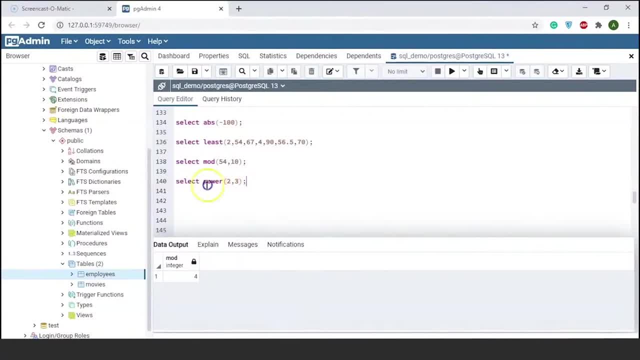 watch similar videos, which is turned up and get certified. click here. let me just run this. there you go. so the result is 8. you can also check, let's say, power of 5 comma 3. it should be 125, all right. next you can use the sqrt function that is available in postgresql to 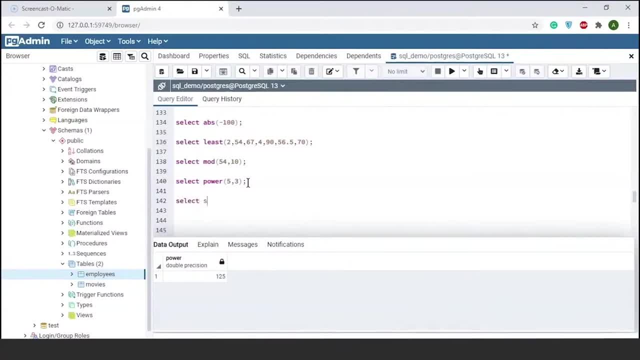 find the square root of a number. i'll write sqrt and let's say i want to find the square root of 100. you can guess the result. output should be 10. if i run this, you can see the output here: 10. let's say i want to find the. 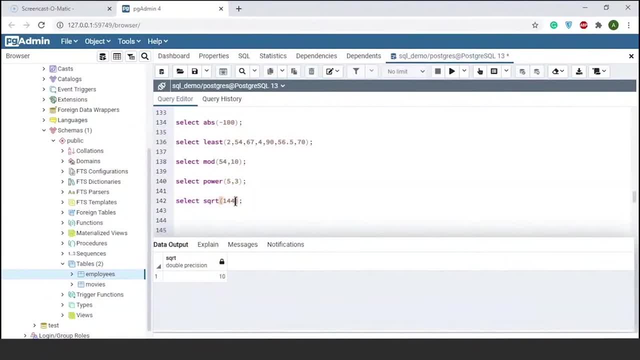 square root of, let's say, 144. you can again guess the result. it should be 12. let's verify it. okay, there is some error. let me verify it again. there you go, it is 12.. now there are a few trigonometric functions as well. you can use the. 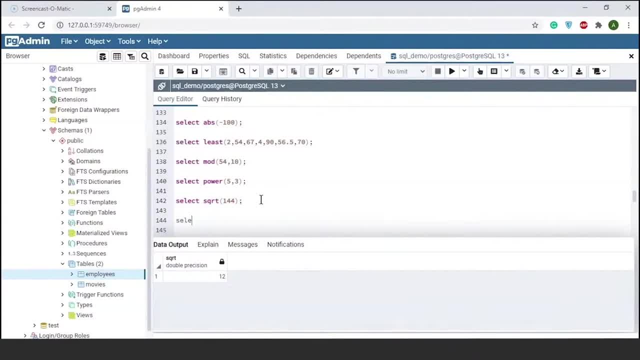 sqrt function and the power function to find the solution. so let's see. let's see if we take the sine function, the cos function and the tan function. let's say i want to know the sine of zero. if you have studied high school mathematics you would know the sine of 0 is 0. you can see the result: it is 0. let's say you want to know sine 90. 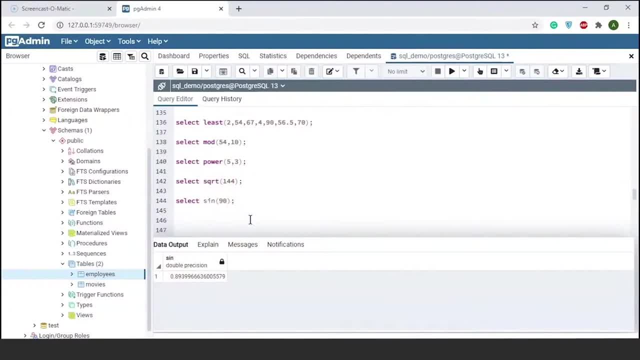 if i run it, you can see the output here: 0.89. all right, you can use. so let me show you what the ceiling and floor function does. i'll write ceiling, let's say i'll pass my floating value as 6.45 and let me run it. you can see the ceiling function returns. 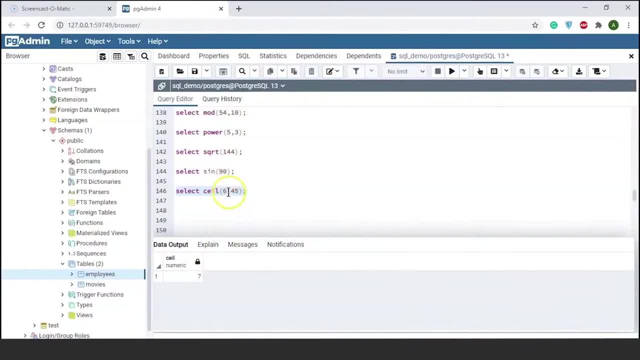 the next highest integer, that is 7 in this case, since the next highest integer after 6.45 is 7. let's see what the floor function does and let me run it. as you can see, the floor function returns the next lowest integer, that is, 6 in this case, or the nearest lowest integer to any provided. 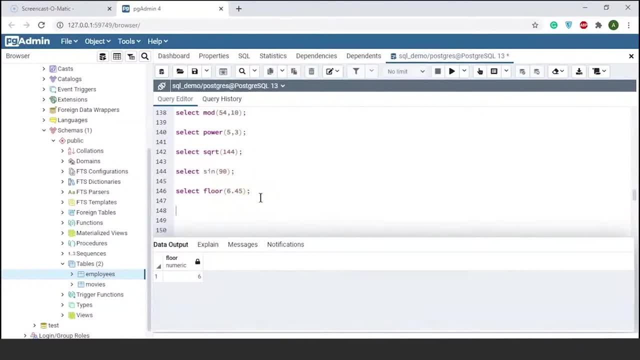 decimal value. okay, now that we saw how to use mathematical functions, there are a few string functions available in postgresql, so let's explore them as well. i'll write string functions. okay, scroll down. cool. there's a function called character length that gives you the length of a text string. suppose i write select, give the function as character length. 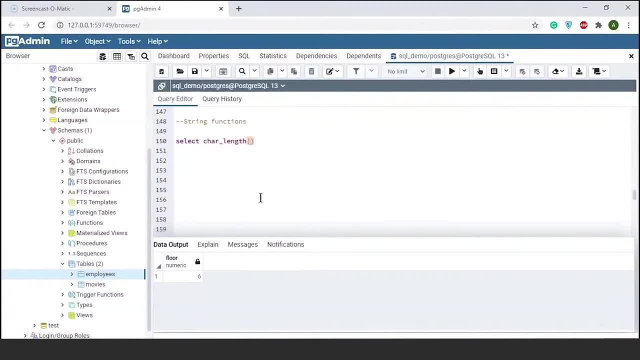 and inside this function, i am going to pass in a text. let's say, india is a democracy. this is my text. let me run this. okay, you can see the result here, which is 20, since there are 20 characters in my string that i have provided. all right, now there's another function called concat. 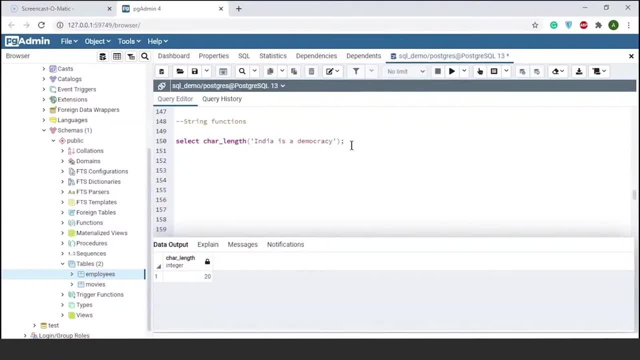 in postgresql. so concat is basically used to merge or combine multiple strings. so i'll write select concat within multiple strings. so i'll write select concat within multiple strings. so i'll write select brackets. I'll give the text string. now let's say I want to combine postgres. 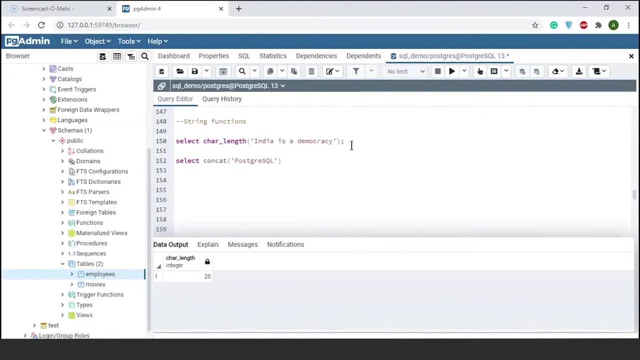 sequel, I'll give a space comma. I want to merge postgres. sequel is. I'll give another comma and write my final word. that is interesting. now, what we have done is, inside the concat function, we have passed in separate strings and now, using the concat function, we want to merge the three strings. 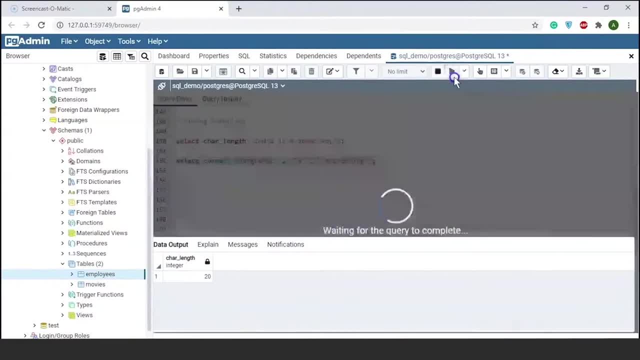 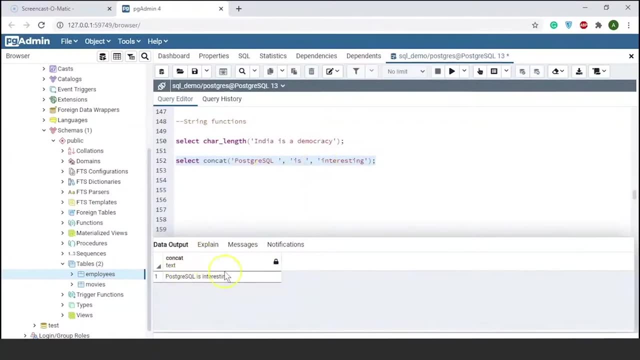 let's see what the result is. I'll run it all right, let me just expand this. you can see here we have concatenated the three string successfully, so So the output is: postgresql is interesting. Okay. Now there are functions like left, right and mid in postgresql. 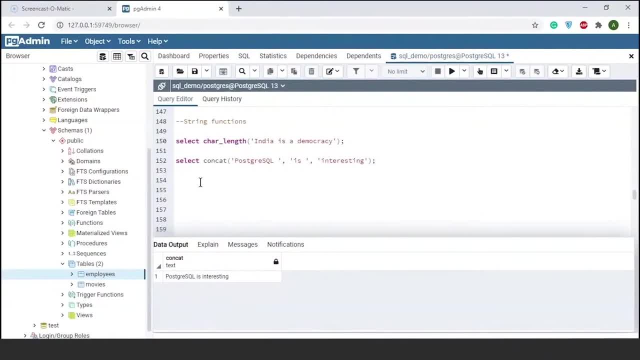 So what the left function does is it will extract the number of characters that you specify from the left of a string. Let's say I'll write select left and I'll pass in my text string: as India is a democracy, I'll copy this and I'll paste it here. 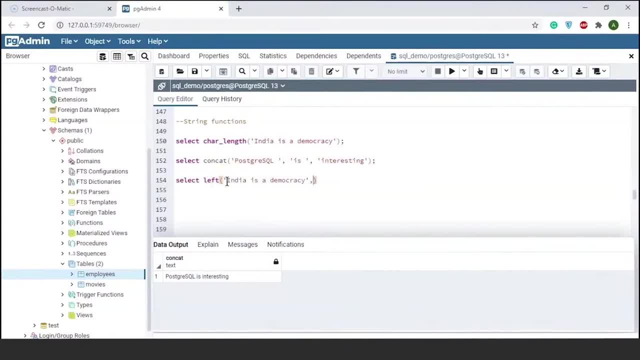 Let's say I want to extract the first five characters from my string, So I'll give five. So what it will do is it will count five characters from left, So one, two, three, four and five. If I run this, it should ideally print India for me. 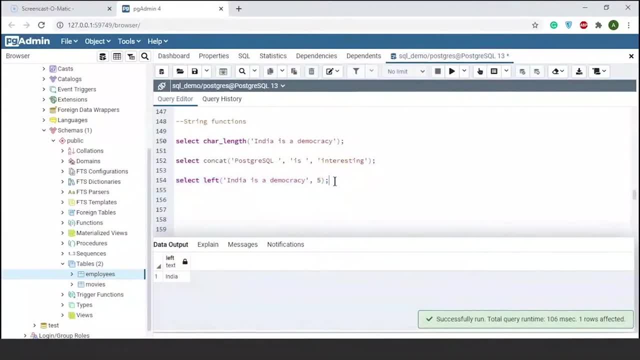 There you go. It has printed India for us All right. Similarly, you can. You can use the right function to extract a few characters from the right of a string. Let's say you want to extract. Let's say I'll give 12 characters from right. 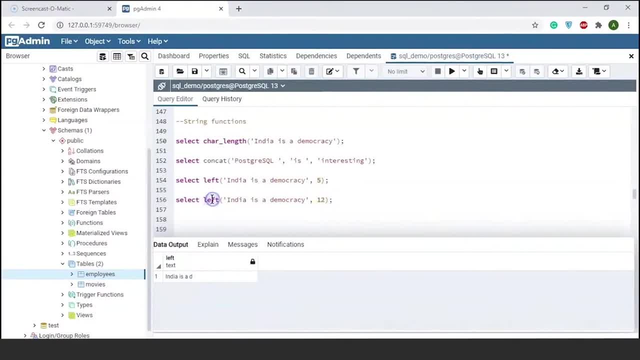 So from here onwards it will count 12 characters. I'll change left to right. now Let me select this and run it So you can see here. this is the output from the right. It has counted 12 characters and returned a democracy. 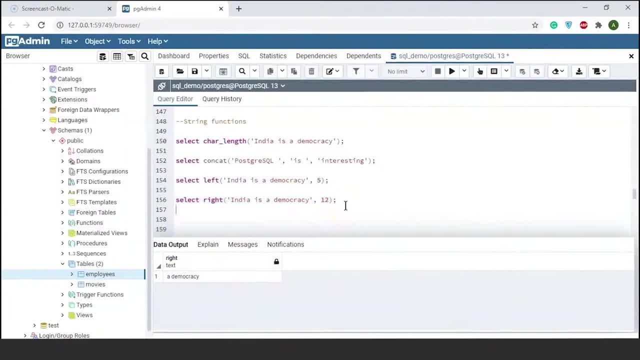 Okay, Now there is A function called repeat, So the repeat function is going to repeat a particular string, The number of times you specify. Let's see. I want to select And use my repeat function And inside the repeat function I'm going to pass in, let's say, India. 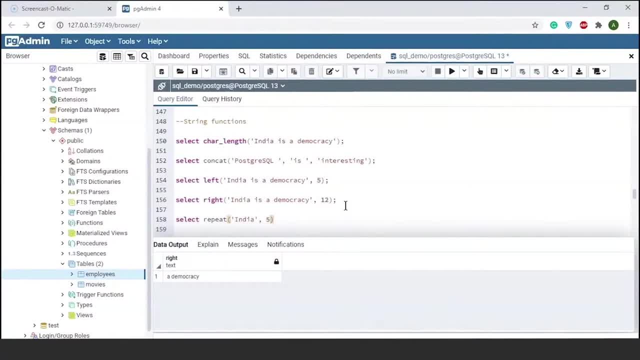 And I want India to be displayed five times. I'll give a semicolon and run it in the output You can see India has been printed five times. Okay, Let's scroll down. There is another function, a string function in PostgreSQL called as reverse. 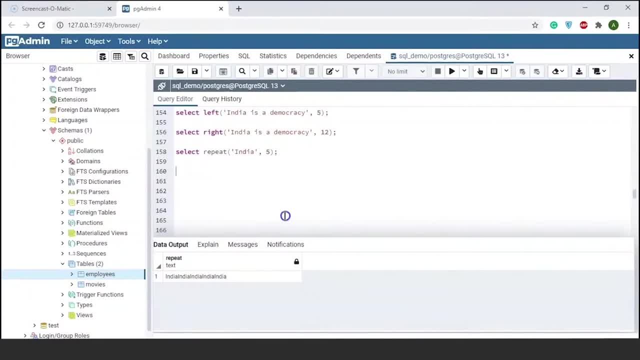 So what reverse function is going to do is it is going to print any string passed as an input in reverse order. So if I write select And inside the reverse function I'll pass in my string that is, India is a democracy, I'm going to use the same string and copy this and I'll paste it here. close the course and the brackets. 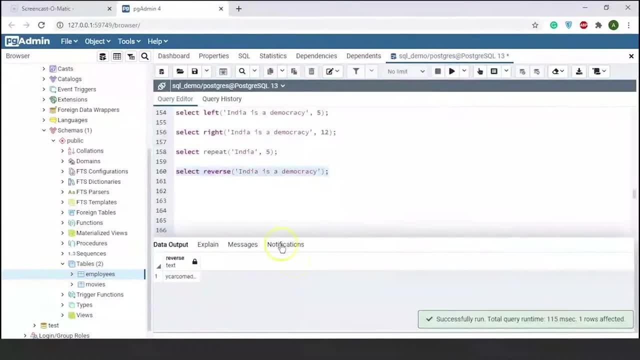 Let's print this. You can see it here: India is a democracy has been printed in reverse order. There you go, All right Now. this time we explored a few inbuilt functions that are already present in PostgreSQL. Now PostgreSQL also has the feature where you can write your own user defined functions. 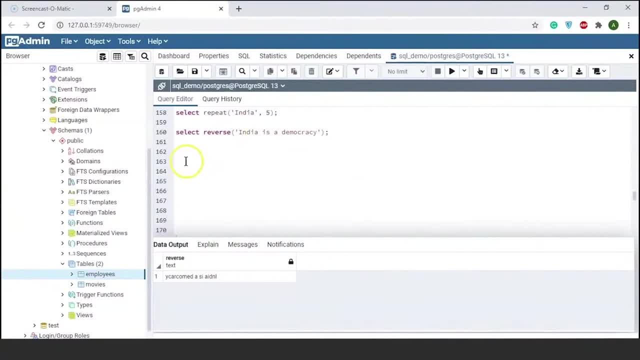 So now we will learn how to write a function of our own in PostgreSQL. So let's create a function to count the total number of email IDs that are present in our employees table. So for this we'll write a function. We'll write a function, a user defined function. 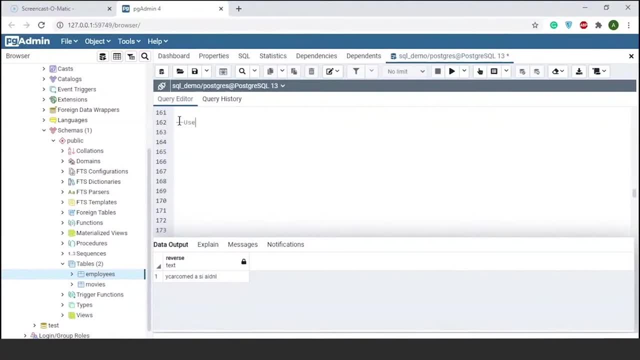 So let me give my comment as user defined function. Okay, So let me start by first writing create. So this is the syntax to write a function in PostgreSQL. So I'll write create or replace function. then I'll give my function name as count emails and, as you know, functions have 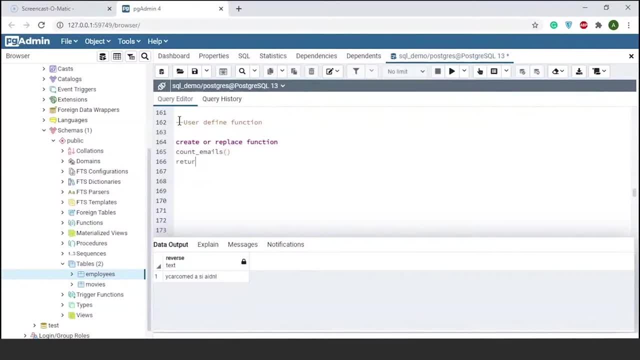 brackets. then I'll write returns, the return type as integer, then an alias with dollar symbol. I'll write total emails, since I'm going to display the total number of email IDs that are present in my table. I'll close the dollar symbol. then I'm going to declare a variable. the variable name is going to: 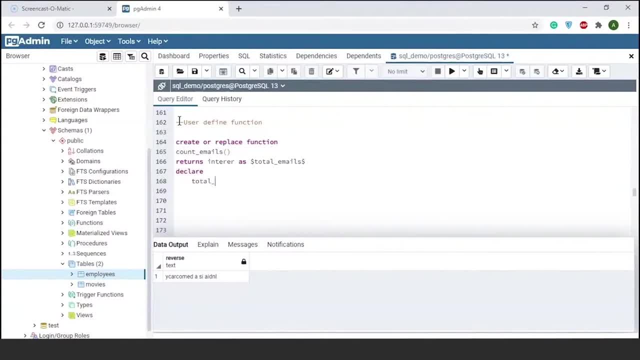 be total underscore emails. this is of type A, integer. I'll write begin and inside begin I'll write my select statement. so I'll write select. I want to count the email IDs that are present, so I'll pass my column name- that is email- into total emails. 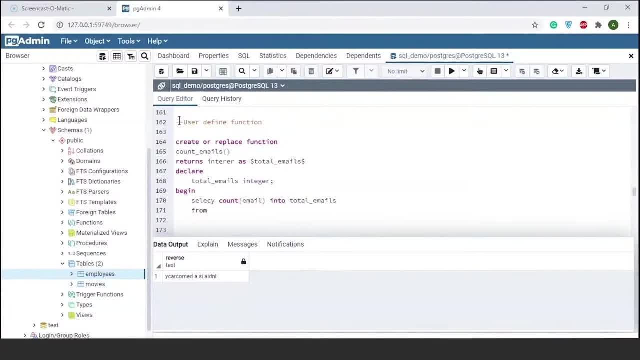 from my table name, that is, employees, I'll give a semicolon and then we'll write return totally: meals. as you know, user-defined functions often return a value, so hence we have mentioned the return statement as well, and now I am going to end my function. then you can now give a sort as aitt, an actor, as a. real name name set it as an author name. that isfrom we give the fifth condition here and now. I have three forms. I will put a result of the form auto with어설� Katie equals and being a, and alot and also a. I will go with a set of points. we have two. 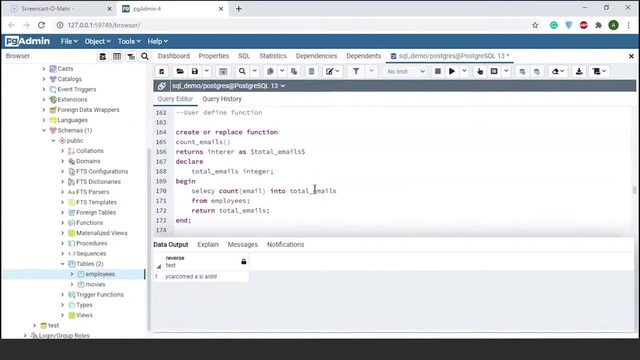 specific functions. I'll give a semicolon and then a and a heir, that y. that makes a debit from the. the next syntax would be: let me just scroll down, okay, so here I'll give my dollar symbol again, followed by total underscore emails. next I'll write my 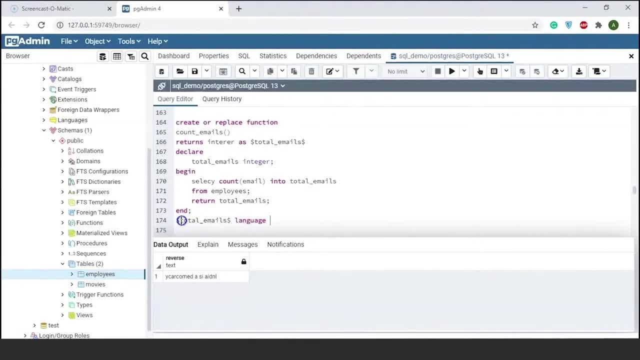 language as postgresql, so the way to mention is pl, p, g, sql. let's give a semicolon and end it. so this is my user defined function that I have written. so I created a function with the function name count underscore emails, and this would return integer as an alias, which is total underscore emails. we declared 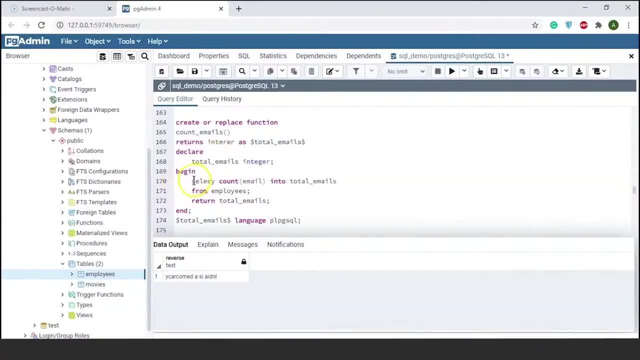 that variable as an integer and this would return integer as an alias, which is total underscore emails. we declared that variable as an integer. then we started with a begin statement that has my select statement, where I am selecting the count of email IDs that are present in the employees. 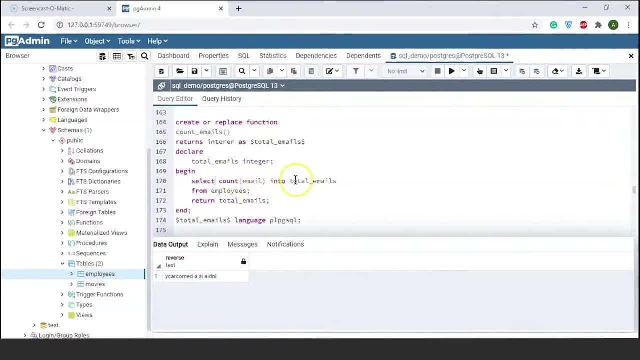 table and I am putting the value into total underscore email. so I have used the into keyword and this returns the result as total underscore emails and I've ended. let's run this. okay, there is some problem. there is an typo, so this should be fine. so let's run this. okay, there is some problem. there is an typo, so this should. 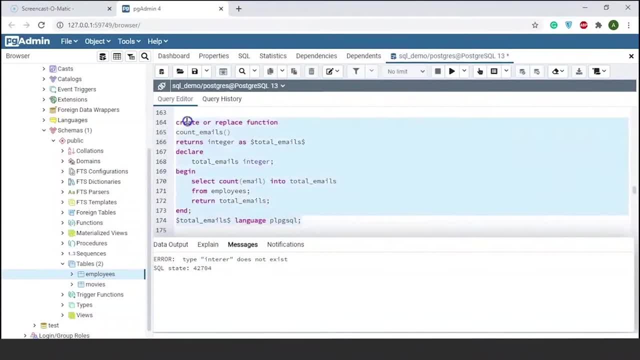 be integer. okay, let me run it once again. there you go. so you've successfully created a user defined function. now the final step is to call that function. now, to call this function, I am going to use my select statement and the function name, that is, count, underscore emails. I'll give a semicolon. let's execute this. 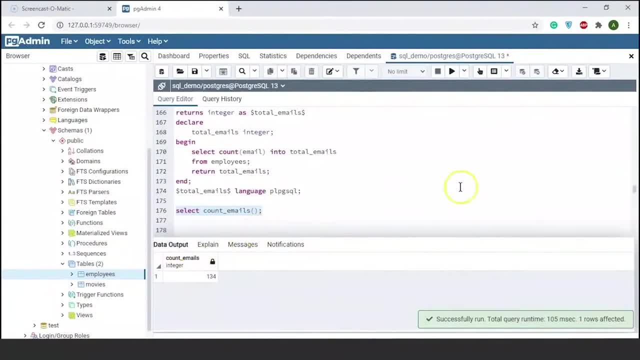 there you go. so here you can see, there are hundred and thirty-four email IDs present in our employees table. now, one thing to mark is there are total hundred and fifty employees in the table, but out of them, hundred and thirty-four employees have email IDs. the rest of them don't have, so they would ideally have null values. 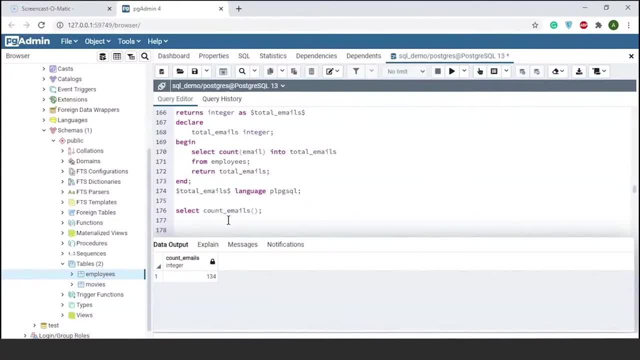 alright. so that brings us to the end of this demo session on Postgres SQL tutorial. let me go to the top. we have explored a lot, so we started with checking the version of Postgres SQL. then we saw how to perform basic mathematical operation, that is, to add subtract multiply. then we saw how to 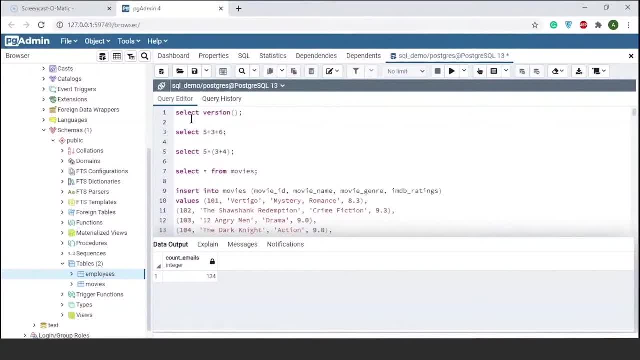 create a table that was movies. we inserted a few records to our movies table. then we used our select clause. we updated a few values, then we deleted one row of information. then we learnt how to use the where clause. we learnt how to use the between operator. we also learnt how to use the. 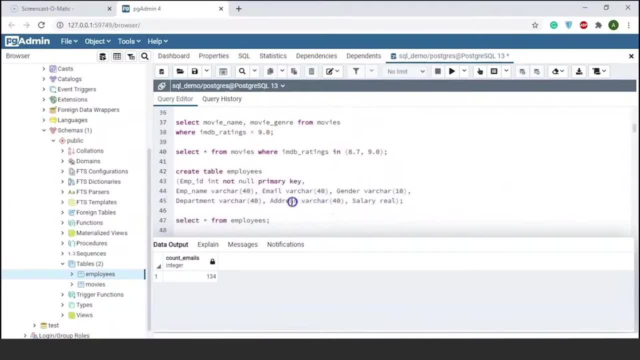 in operator. let me scroll down. we created a table called employees and then we learnt how the distinct keyword works. we also learnt how to use is null. with where clause. we learnt about the order by clause. we saw how to alter or rename a column. then we explored a few more examples on where clause. we learnt. 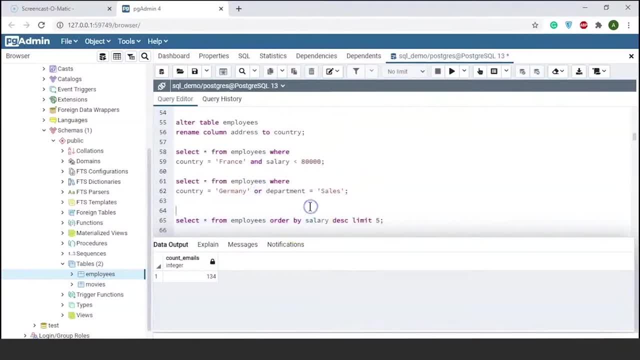 about and and or operator. then we learnt how to use limit and offset as well as the fetch operator or the fetch keyword in PostgreSQL. moving further, we learnt about the like operator in SQL, which was used to perform pattern recognition or pattern matching. you can say: here we saw how to use basic inbuilt PostgreSQL functions like some average. 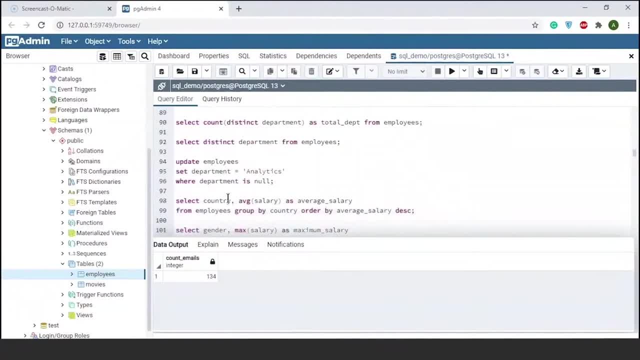 minimum count, maximum. next, we saw how to update a value in a column using PostgreSQL update command. we learnt how to use group by then we learnt how to use having clause. then we learnt how to use case expressions in PostgreSQL. so we saw how case expression is similar to our, if else in. 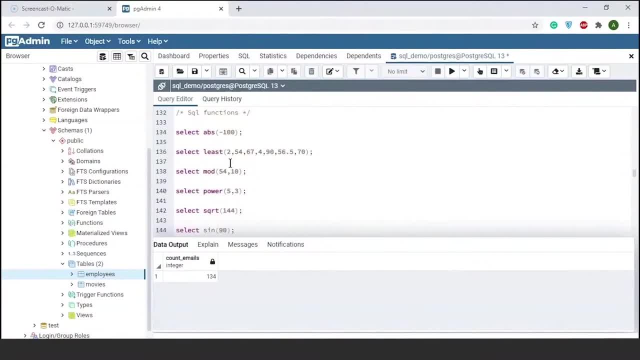 any other programming language. we explored a few mathematical and string functions and finally, we wrote our own user-defined function. so that brings us to the end of this tutorial on PostgreSQL. now, if you want to get this SQL file that we have used in the demo, you can give your email IDs in the 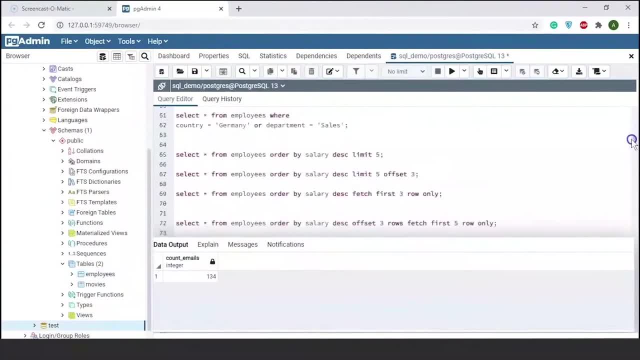 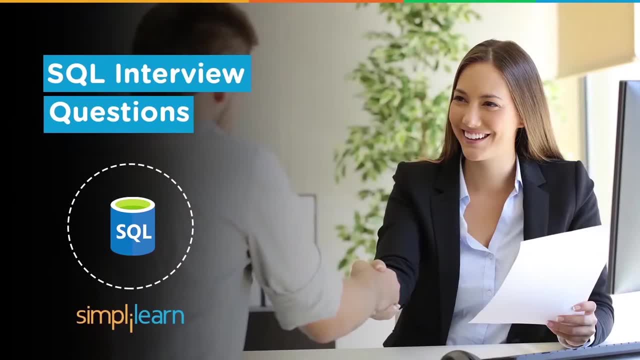 comment section, and our team will share this SQL file with you in the next video. SQL is a very important technology that is used in the IT industry. professionals working as application developers, web developers, data analysts, data scientists, software testers and cyber security experts need to know SQL. in this video, we will cover 30 important SQL. 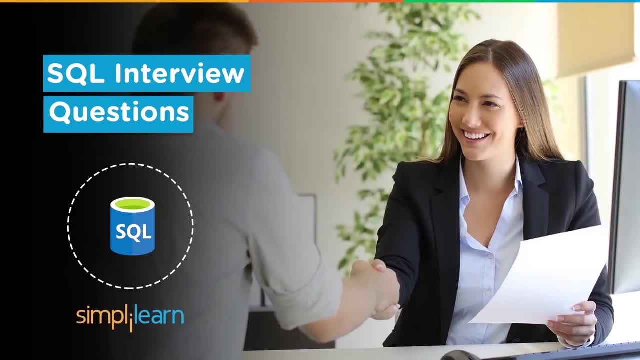 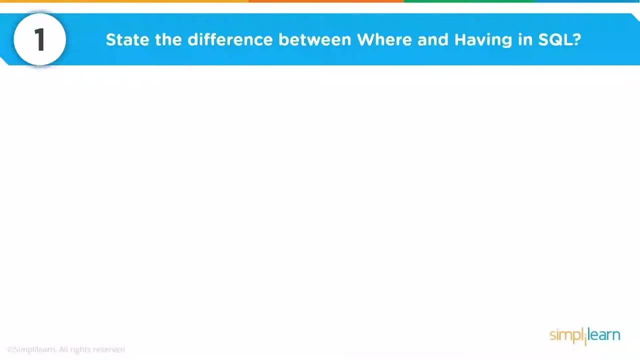 questions that are most frequently asked in the interviews. now, these questions consist of a set of theoretical and practical questions, so we will use different commands, functions, joins and other functionalities in Excel to solve the problems. so let's get started with the first question. so the first question is to state the difference. 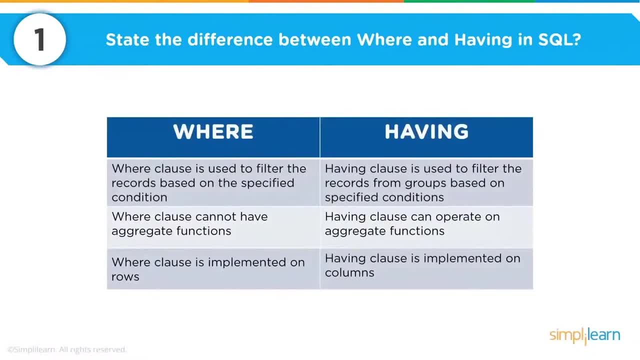 between where and having clause in SQL. now, where and having are very widely used in SQL to solve specific problems. now let's look at the difference one by one. so where clause is used to filter, the records from the table based on the specified condition can be used without the group by clause. on the other hand, having clause is used to filter. 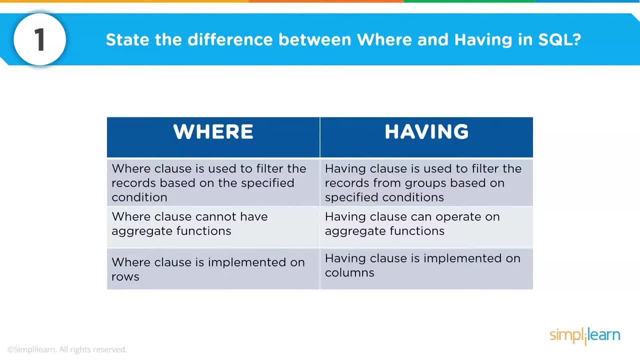 the records from groups based on specified conditions. now where clauses cannot have aggregate functions. so you cannot use sum, count, average, min and maximum functions in the where clause, while in the having clause you can operate on aggregate functions and those aggregate functions are used to filter values from a group. now where clause is implemented on rows. 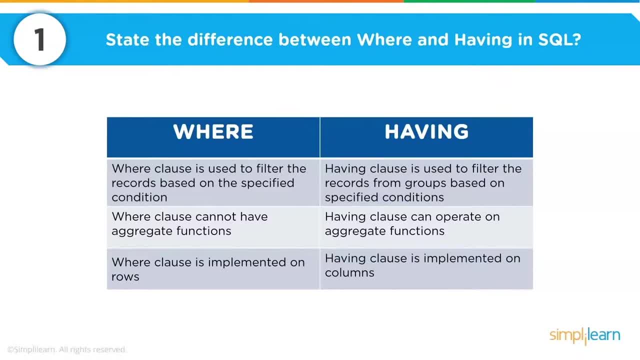 or at row level. so for each row of data, you have the where condition applied now. having clauses are implemented on columns, so for each column of data, you have the having condition applied now. another important difference between where and having is that the where clause is executed before the execution of the group by clause and after the execution of the from. 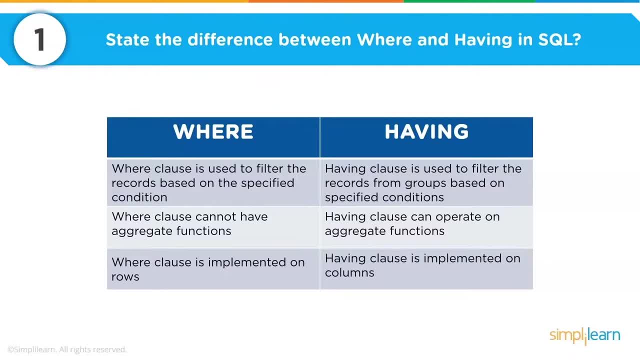 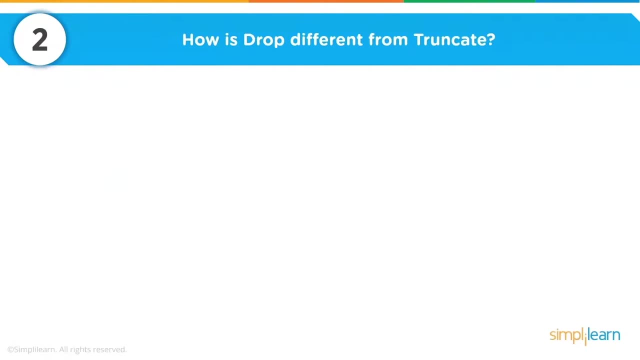 clause. on the other hand, the having clause is executed after groups are created. now let's move on to our next question. now we will learn more about where and having and understand the usage better when we tackle practical problems in this video. now moving to our next question, which is: how is drop different from truncate? so drop and truncate are two different. 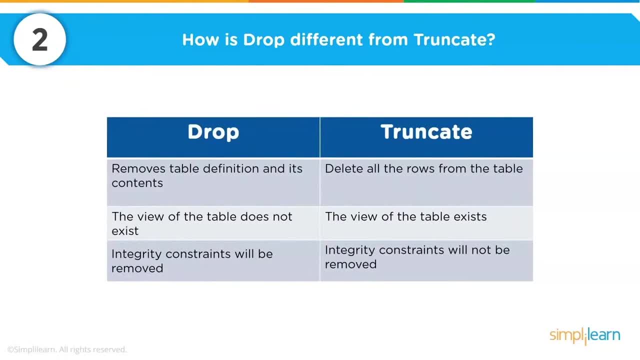 commands. so drop command is used to drop the whole table, removing the table definition and its contents, while truncate deletes all the rows from the table. now we can drop the whole table structure in one go, so the view of the table does not exist. by using the truncate command, the existence of all. 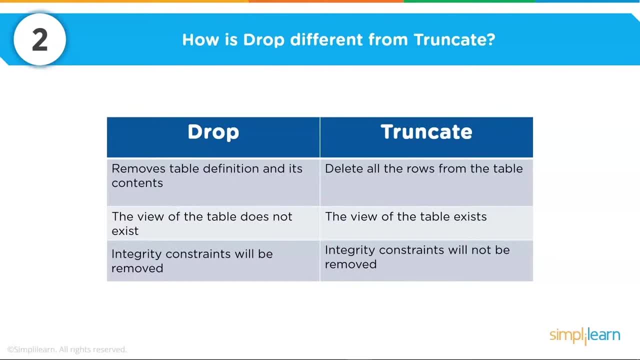 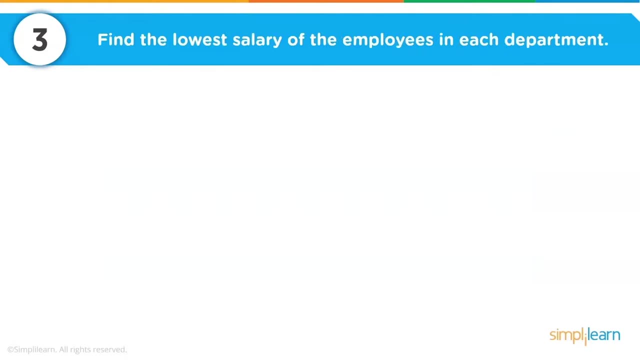 the rows in the table is lost, but the view in the table exists. now integrity constraints will be removed in drop command, while the integrity constraints will not be removed when you use the truncate command. now moving to our third question. now, this is a practical question, so we will be using a table which is present in my mysql database. so the table name is called: 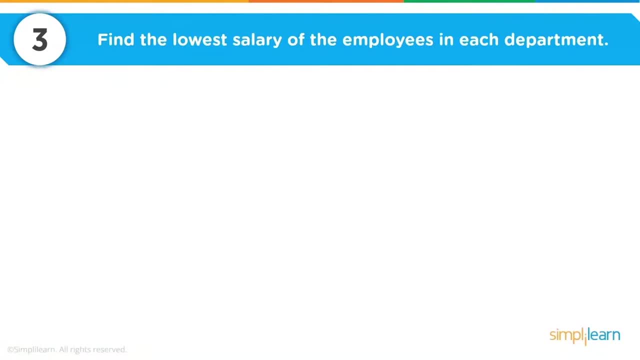 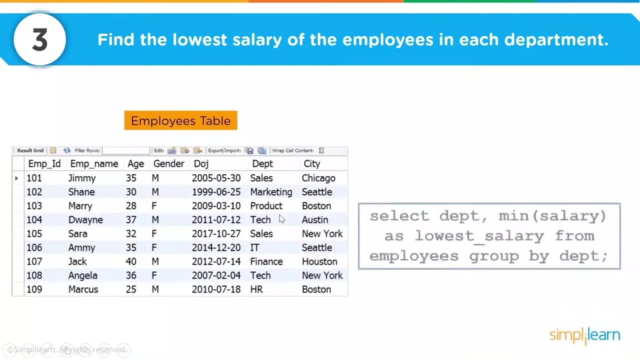 employees and i want to find the lowest salary of the employees in each department. you can see here: this is how my employees table looks and the output query would be something like this: so here, since i want to find the lowest salary of the employees, so i am using a min. 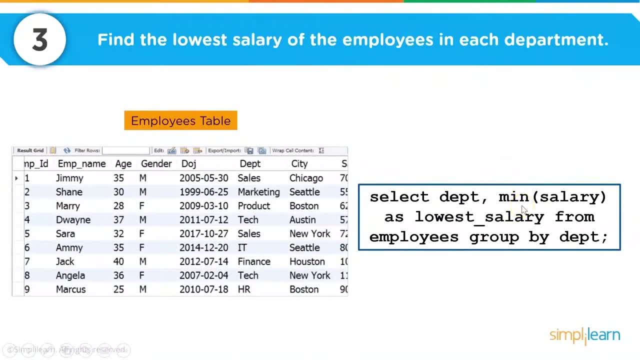 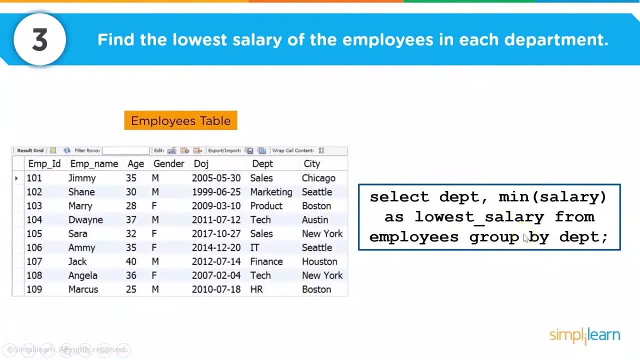 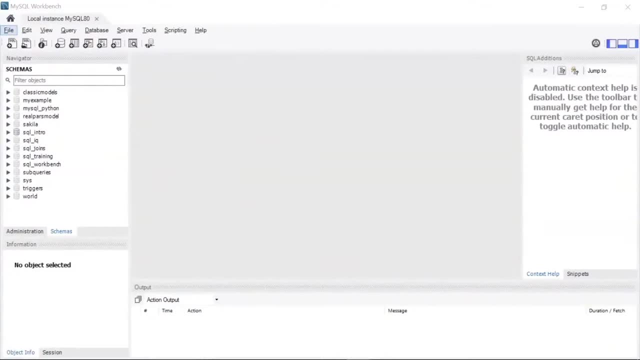 function to find the lowest salary in the table, and then i am grouping all the employees and the results by department. so let's do this on mysql workbench. okay, so here i am on my mysql workbench. first let me go ahead and create a new sql script. so i'll click on this and that will create a new script. okay, so here. 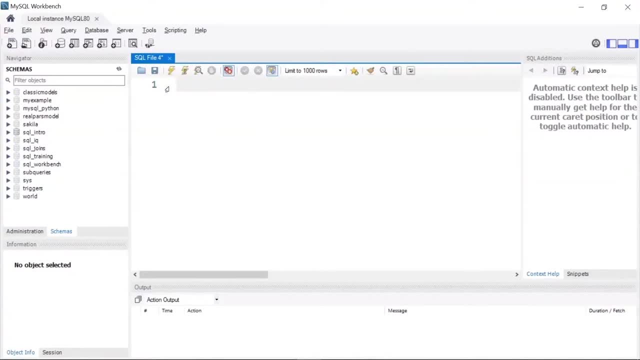 we'll write our commands, all right. so our question was to find the lowest salary for each department. okay, so i have given my comment to make my commands and whatever i am doing more readable. so first, before i proceed, i need to select my database. so i am going to use my sql underscore intro database. so i'll write: use sql underscore intro. 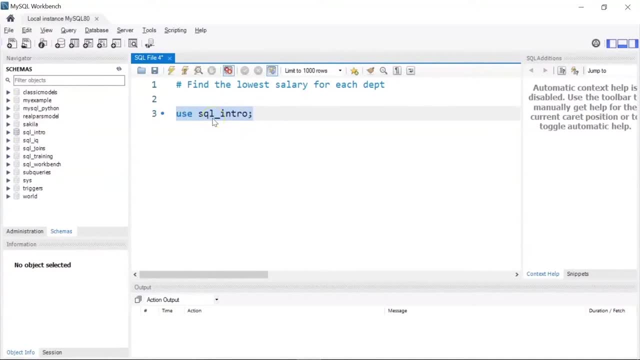 now. this database has a lot of tables that we'll be using in this interview questions video. i'll run it. okay, we are in our sql intro database now. there is a table called employees. let me show you the table first. if i write select star from employees, 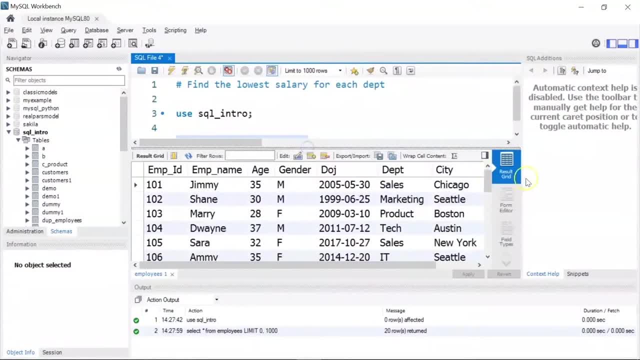 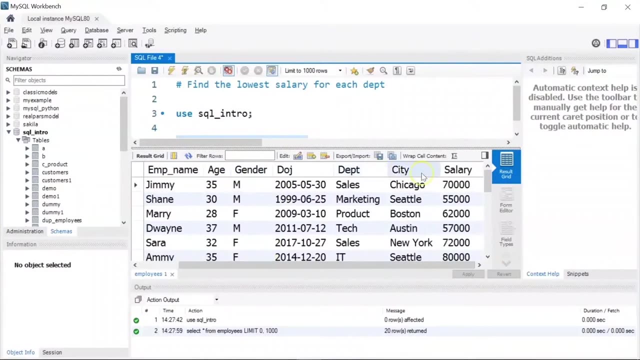 okay, so here you can see. this is the table i am talking about now. these are the rows that are present in the table. we have 20 rows and here you can see the different columns. we have the employee id, employee name, age, gender. we have the department, city and salary. now this: 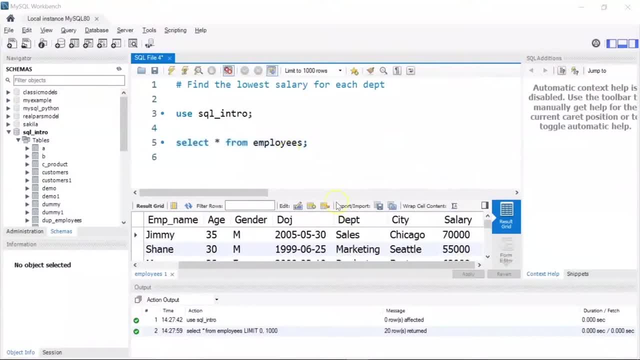 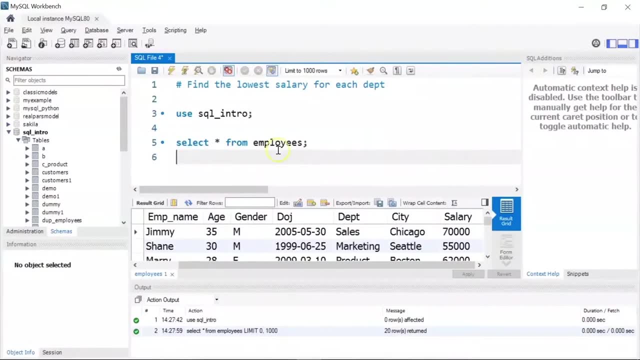 is the same table that we have also used in our other videos that are already live on youtube. okay, so let's solve our question: to find the lowest salary for each department. now. for that i'll write select. i'll select my department column, which is dpt. 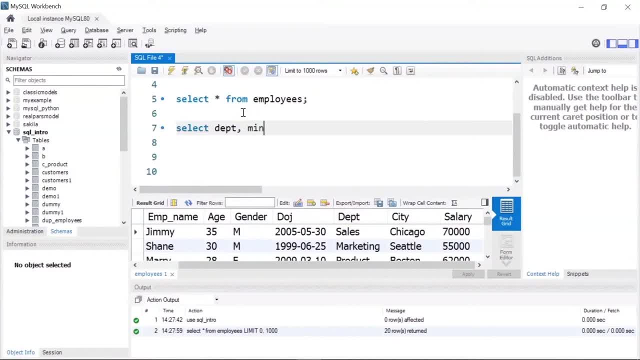 comma and then to calculate the lowest salary or to find the lowest salary, i am going to use the min function so that will return the minimum salary present in the salary column. so i'll write min salary as i'm giving an alias name as, let's say, lowest underscore salary. 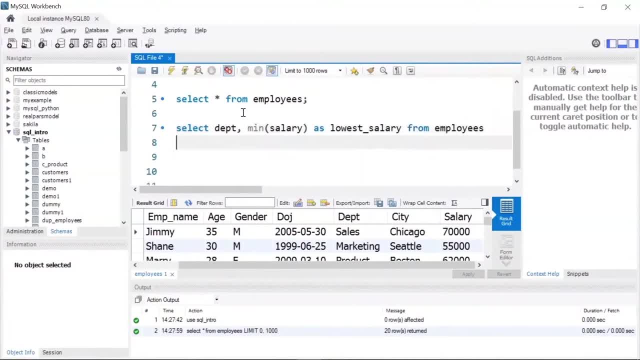 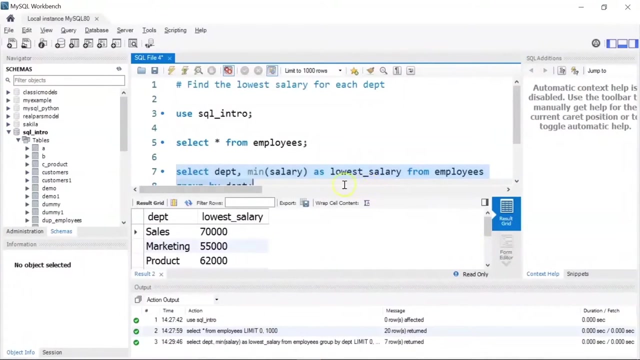 from my table name, that is, employees. then I'll write group by department. now I'm grouping it by department because we want to find the lowest salary of the employees in each department. now let's run and see the result. there you go. I'll just move it to the top so that you can. 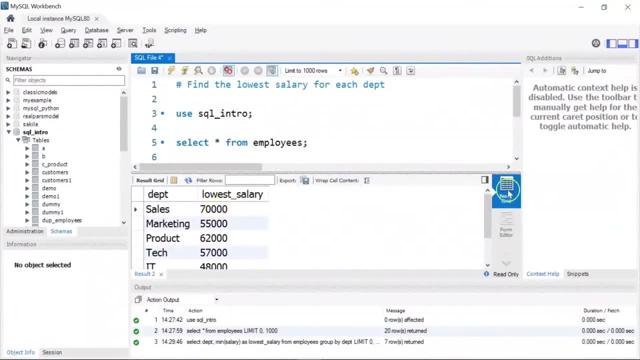 see the results clearly. okay, so here we have total seven departments. you can see at the bottom. and in these seven departments you can see in sales, 70,000- let's say dollars- was the lowest salary. in marketing. we had 55,000 dollars as the lowest salary. similarly, if I scroll down, we have 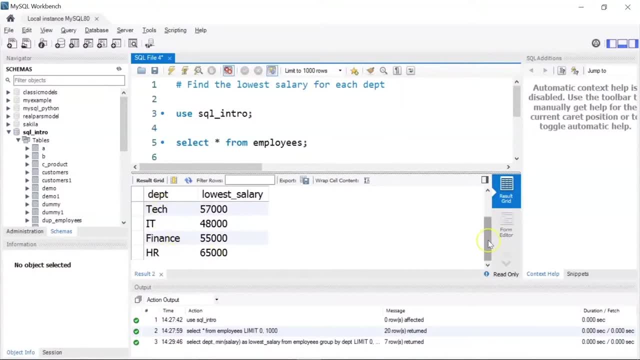 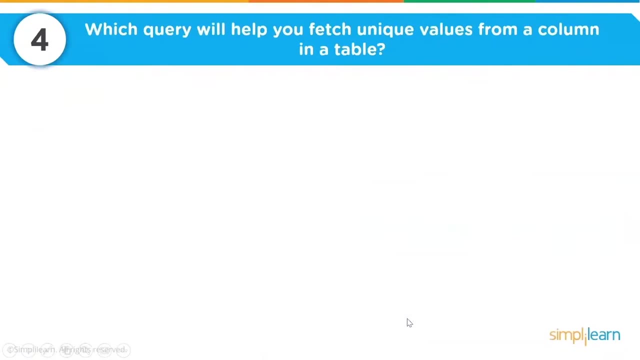 other departments like tech, IT, finance and HR. so these are the lowest salary in each department. all right now moving to our next question. so our fourth question is: which query will help you fetch unique values from a column in a table? so this is a multiple choice question, which is another type of question that is often asked in the SQL interviews. now we have 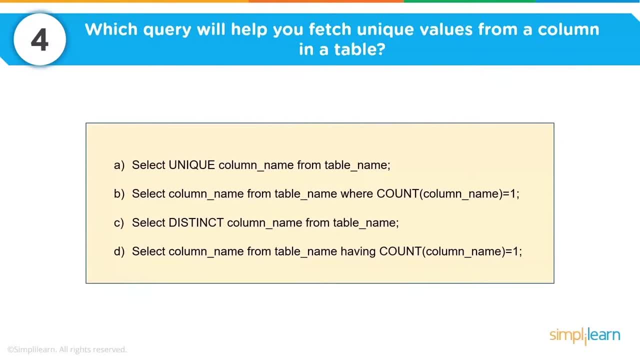 multiple queries here and you need to choose the right query. that will solve our problem. so, since I want to get the unique values from a column in a table, so the right option would be to use the distinct keyword in the query. so if I write select distinct, followed by the column name, let's 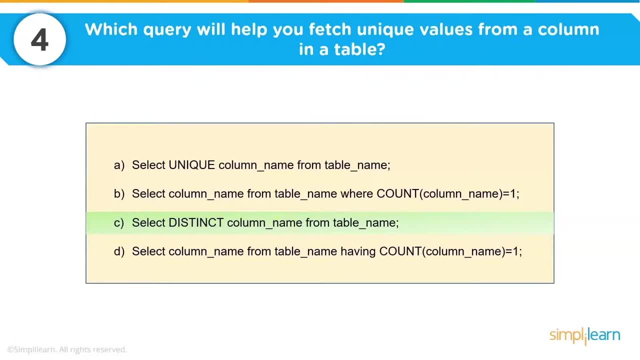 say, you want to find the distinct cities or the distinct departments in the employees table. so the query would be: select distinct City or, let's, a department from the table named, that is, employees. hence this is the label, that's also called logo, called a division, and at the global level you can. 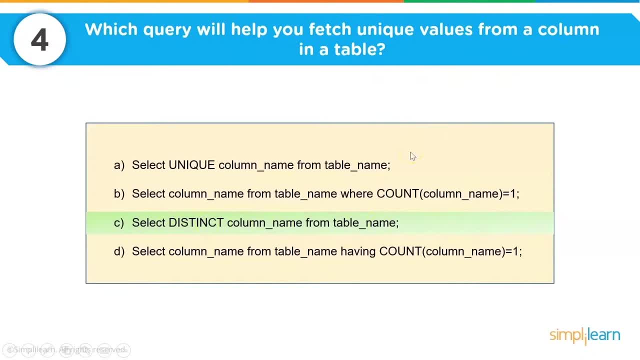 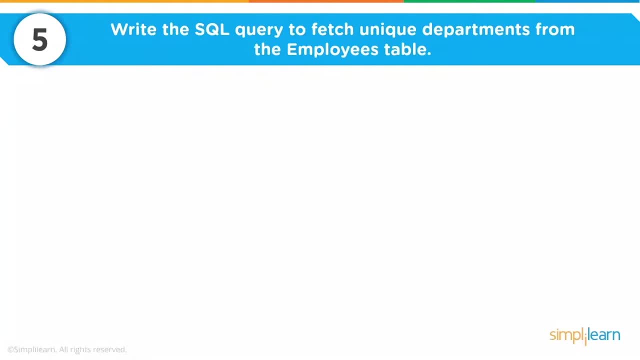 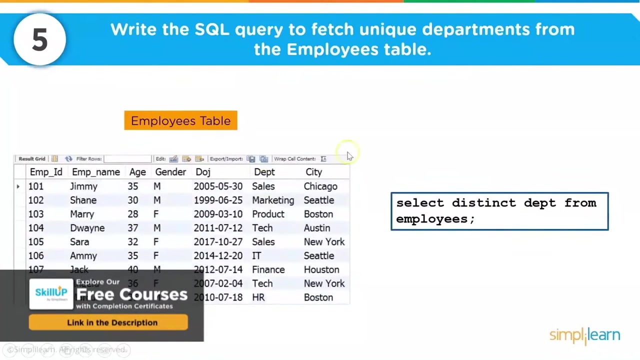 write option if you want to find any unique values from a column. now moving to the fifth question. now, the fifth question says it is actually a similar question. here we want to write the sql query to fetch unique departments from the employees table. so, as we saw, this is our employees table and if you want to find the unique departments from, 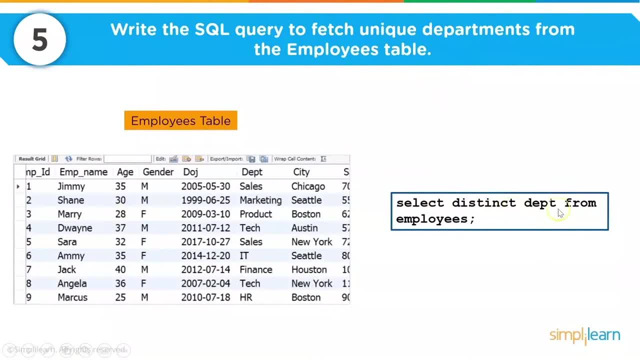 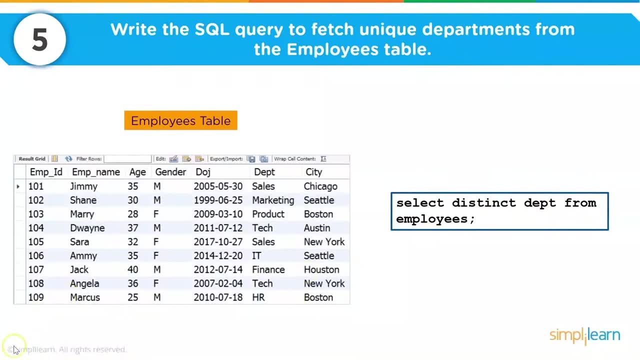 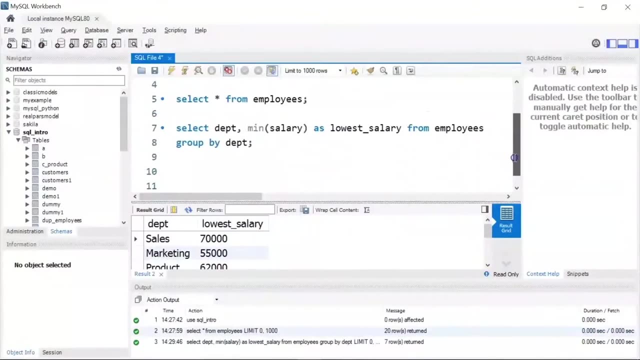 the employees table you can just write select distinct, then followed by the column name, which is departments here. so, dept from employees. let's do this on our mysql workbench, okay, so let me just scroll down and i'll give a comment here. that is, we want to find the unique departments. 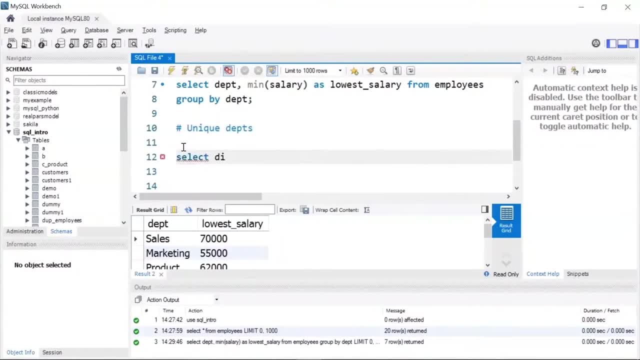 so the query would be select. then i'll use the distinct keyword. if i hit tab, it will auto complete. then i have my column, that is department from my table name, that is employees. if i run this, the query will give us the unique departments that are present in the table. so here: 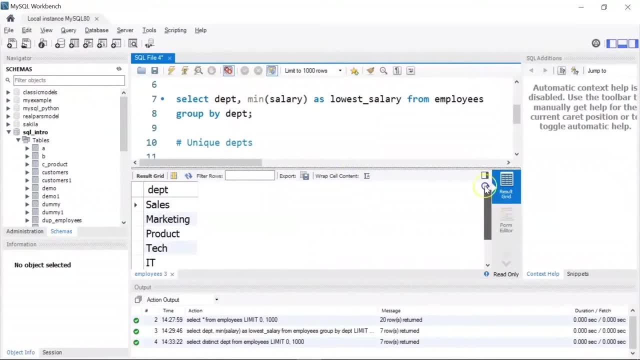 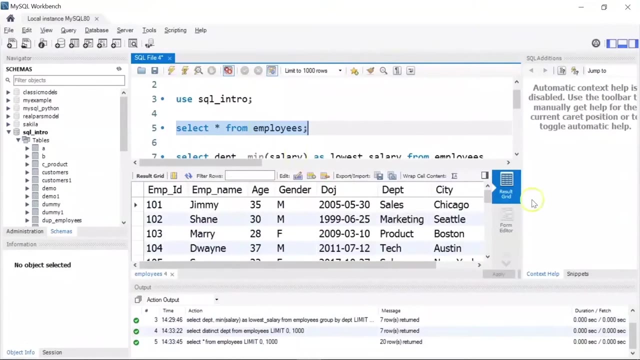 we have total seven unique departments in the table. you can see here we have sales, marketing, product tech, it, finance and hr. but if you see our original table, which is the employees table, so there are total 20 records and if you see the department column there are 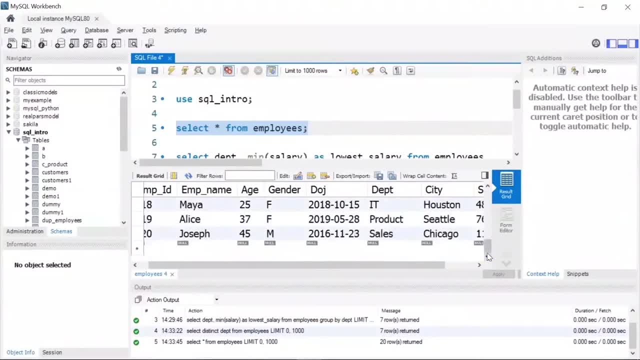 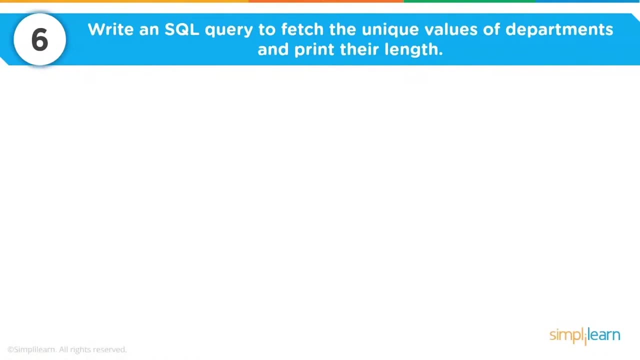 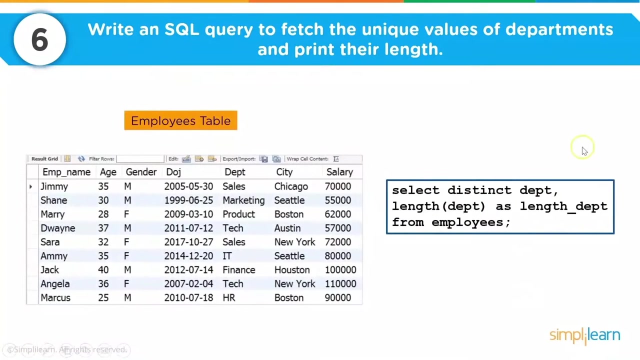 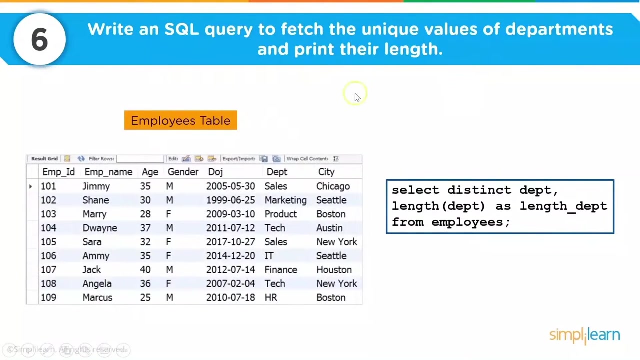 multiple departments to which each of these employees belong to. okay, now moving ahead. so the sixth question is to write an sql query to fetch the unique values of departments and print their length. now this question consists of two paths. first we need to fetch the unique values of departments that we saw in our fifth question, and then we want to print the length of each of. 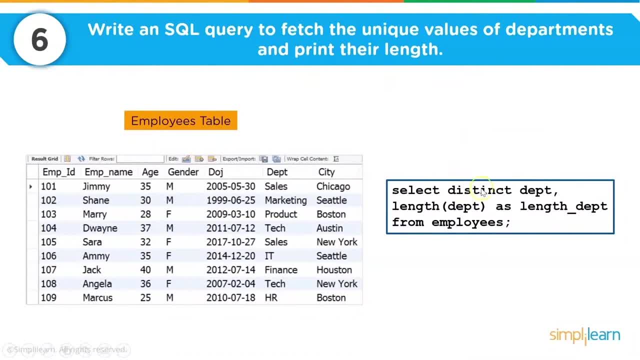 the departments. so for that i am using the distinct keyword to find the unique departments and then i'm using the inbuilt keyword that came in the departments aaa- is that correct length function that is present in MySQL to find the length of the department. and then I am using an alias that is length underscore: department from employees. so 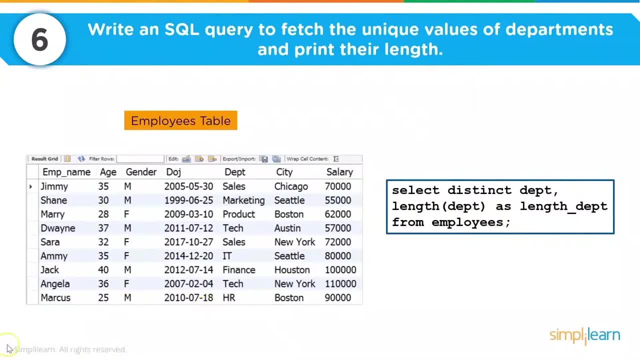 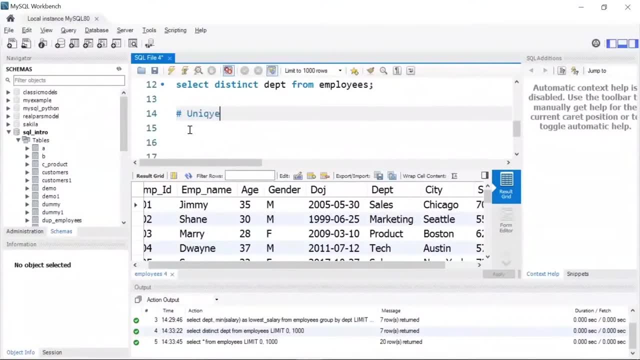 let's say this on our workbench: okay, so let me give a comment. I'll say unique departments and length. okay, so the query would be: I'll write select distinct department and then let me just scroll down. you give a comma and use my inbuilt length function. see, I'm hitting tab to autocomplete and inside the length. 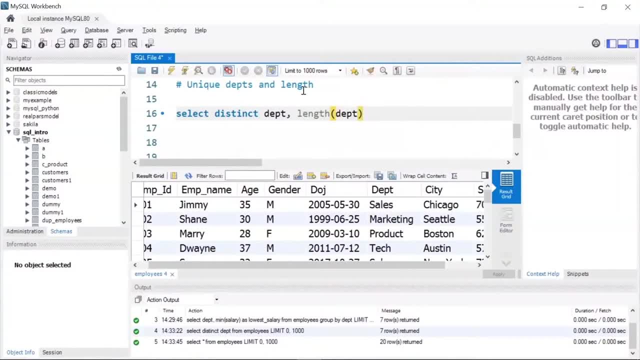 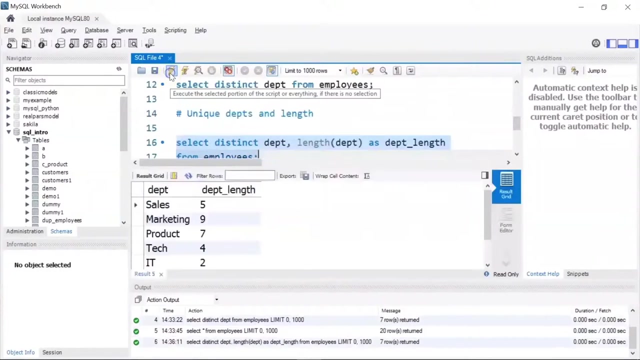 function, I will give my column name, that is, department. I'll give an alias as department underscore length from my table, that is employees. this is pretty simple. so first I am finding the unique departments and then, using the length function, I am finding the length of each department. let's run and see. okay, you can see the result here. so sales, the. 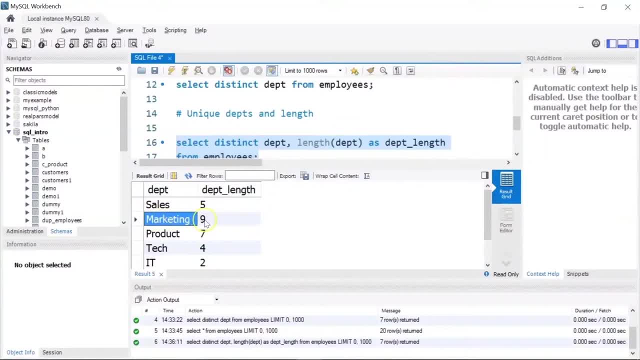 length is 5. marketing: the length of each department is 5 and the length of each department is 9. so basically you are counting the number of characters that are present in each of the departments. so in sales there are total 5 characters. in marketing, there are total 9. 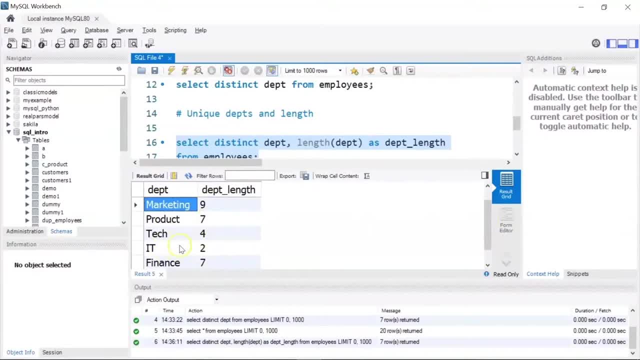 characters in product. there are total 7 characters. in IT. we have just two letters, I and T, so hence the length is 2. similarly, finances 7 and HR is 2, because we have just two letters, H and R. okay, so this is another variation of using distinct along with. 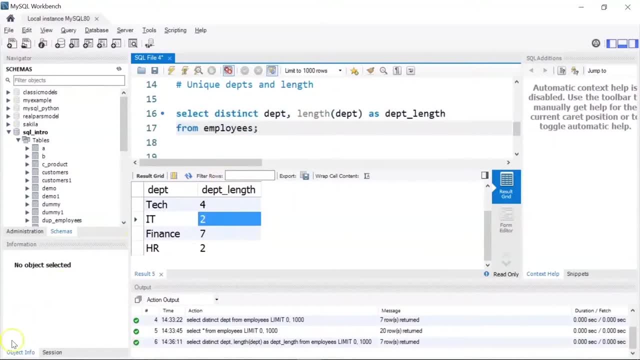 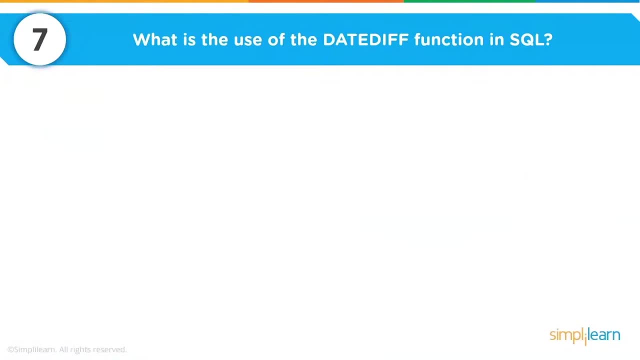 inbuilt function. all right. now, moving to the seventh question. the question is: what is the use of date diff function in SQL? now, date diff returns the number of days between two date, or date, time or timestamp values. so date diff is another crucial inbuilt function that is present in MySQL. so here is how you can use the 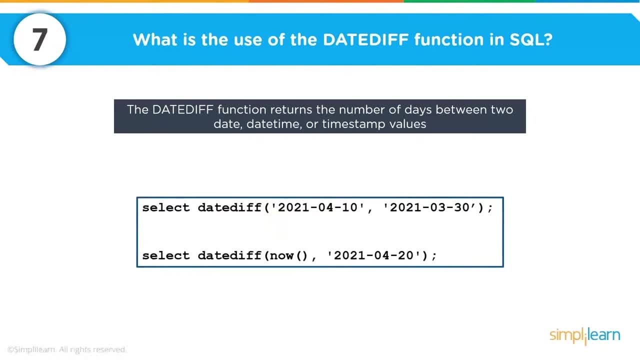 date diff function, so it will return the number of days between two dates, or date time or timestamp values. so here I have two date values, that is 10th of April 2021 and I have 30th of March 2021, so this query will give us the total number. 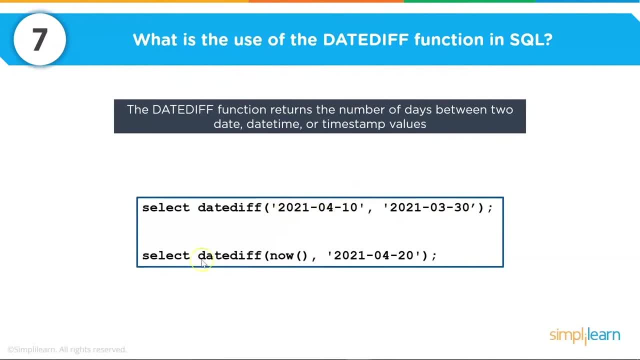 of days that lie between these two dates and similarly, here is another example of using the date diff function. so I want to calculate the total number of days that are present between today's date- so I am using the now function- and between 20th of April 2021. so let's do this demo on the workbench. 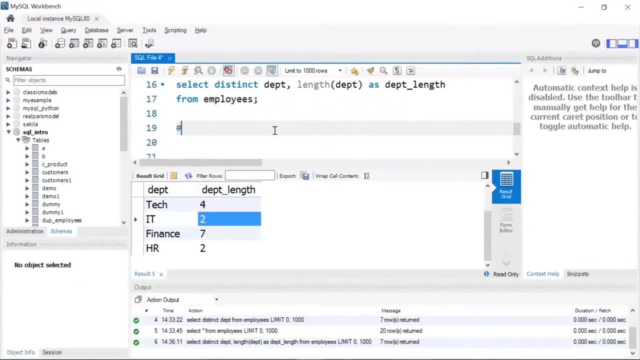 all right. first I'll give a comment saying date diff function. okay, now the way to use is: I'll write select and then you can see here: once I type date, MySQL, workbench is automatically suggesting some of the inbuilt functions. I'm going to use date diff. 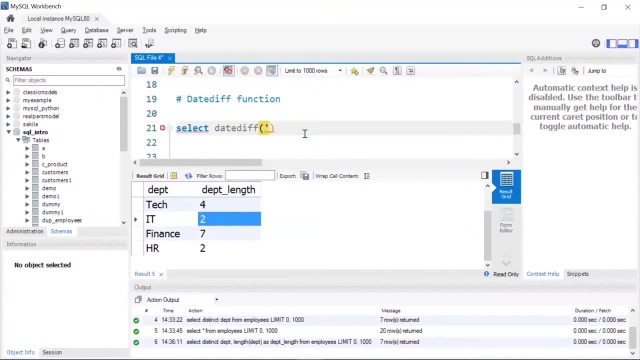 and within date diff, I'm going to pass in two values. so I'm passing in two date values. let's say 2021 April, so I'll write 04 and let's say 10th of April. I'll give another comma and I'll pass in my second date. 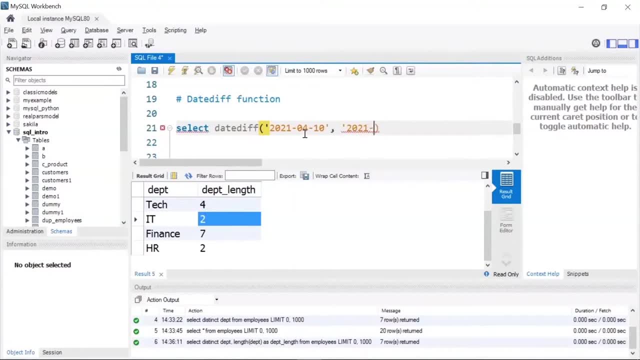 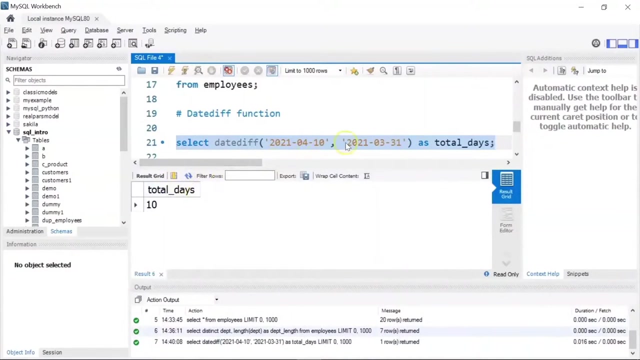 value, that is going to be 30th of March 2021. all right now. another thing to note here is: the date value should be present inside quotations. if you want, you can give an alias as well. I'll write as total days. let's run it. there you go. it has given us the output as 10, so there are total 10. 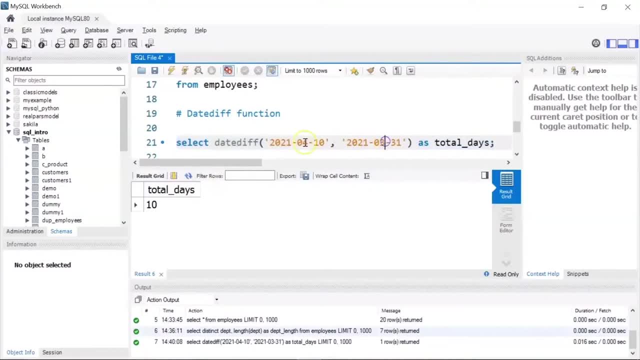 days between 31st of March to 10th of April. now let's see another example. I'll write select date diff and we'll pass in my now function. so the now function returns the date diff function returns the current date, that is, today's date, and I'll give another date value, let's say 2021. 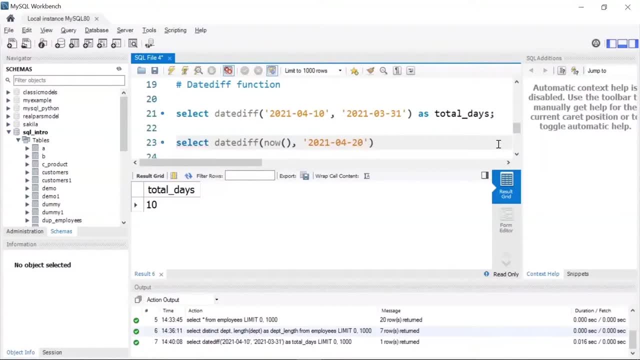 April 20th. now we'll see the results. if you want, you can give an alias name so that the output is more readable. here I'll run it okay. so between today's date and my previous date- that's the date diff function- that was 20th of April, the total: 49 days. so today's date is actually 8th of June. so between 20th of 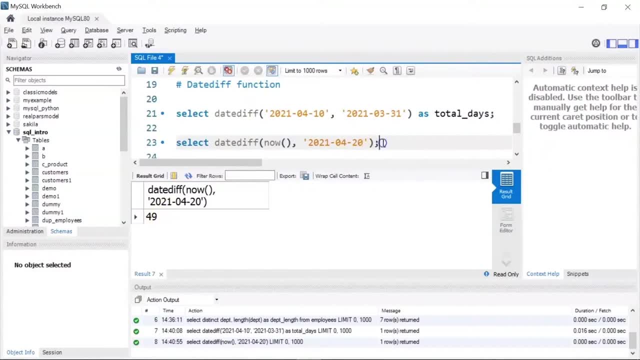 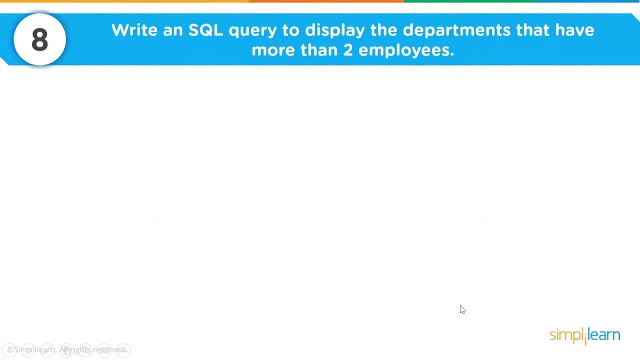 April and 8th of June. there are total 49 days. alright, I'm moving ahead. now in the eighth question, we want to write an SQL query to display到 thesequeryy the departments that have more than 30 dates to date. that is what the total is for a day and, depending on objectively, I will write. 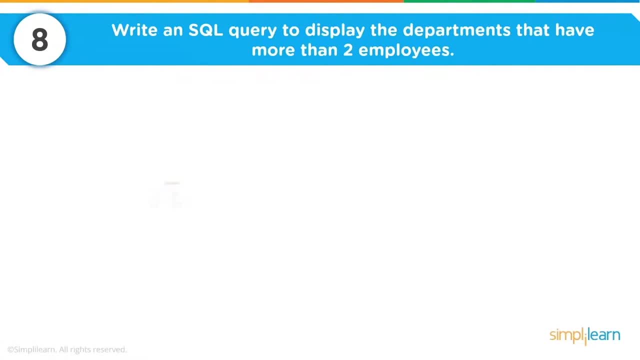 I will say what are the actual dates. so I'll write anul onideed here and if I do that, ♥ ppymo Jeff lines. now I scroll down. I will say Deswegen auf ach er. in a simple field, this more than two employees. so this is our employees table that we have been using. 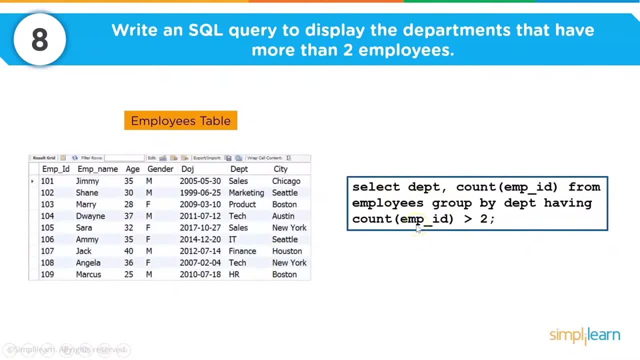 and here is how the command looks like. so here we are using both group by and having. now i am grouping by department because i want to display the departments that have more than two employees. now for the second filter, i am using the count function of the employee ids and checking. 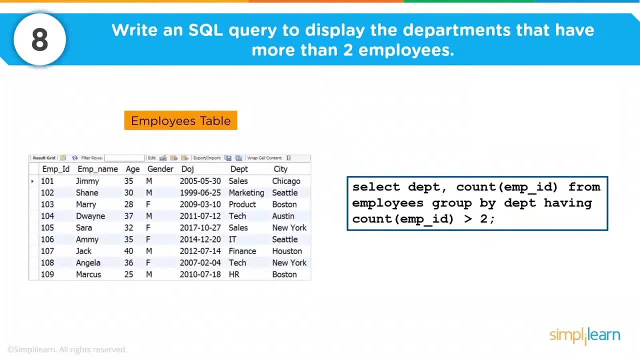 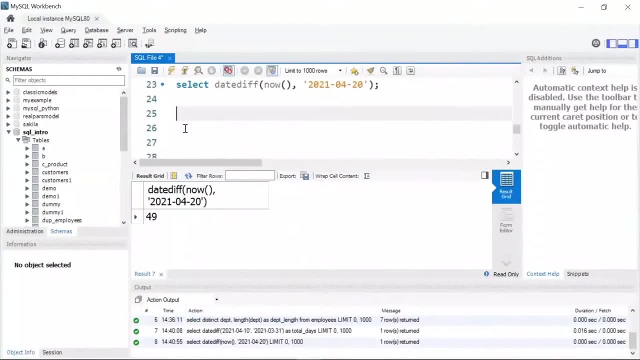 if the employees in each department are more than two or not. let's do this. let me move down a bit and i'll give a comment. departments with more than two employees. okay, now let's write our query. so i want to select the department and then i am using the count function to count the employee ids in each department or the employees. 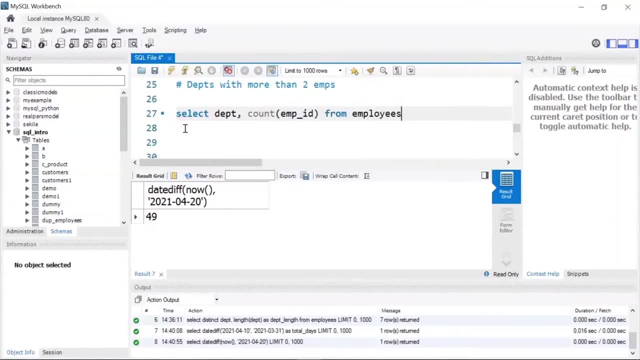 present in each department from my table, that is, employees. i'm going to group by department and then i'll use having my count of employee id. this should be greater than two, so our query will return only those departments which have more than two employees. let's run and see. there you go. 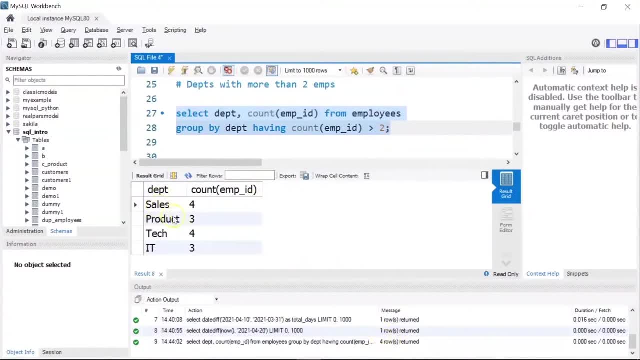 so we have total four departments, that is, sales, product, tech and it, where we have more than two employees. you can see here: sales has four employees, product has three, tech has four and it has three. the rest of the departments, like finance, hr and others, have less than two employees. 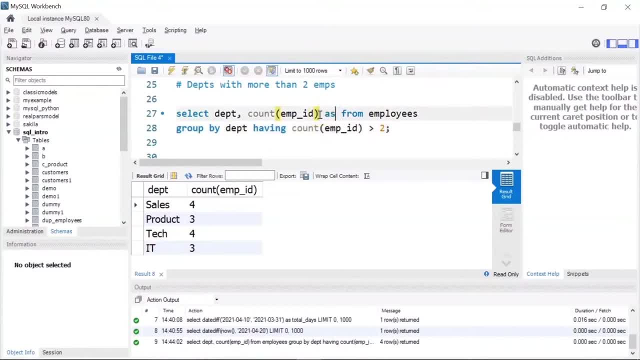 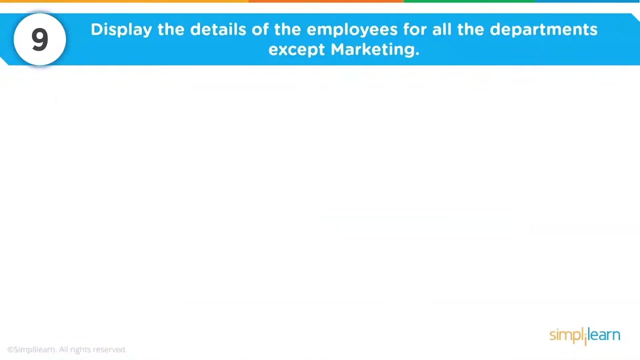 now, if you want, you can give an alias as well, let's say as total employees. okay, let me run it again, and here you can see i have the column name as total employees. okay, so moving ahead. the ninth question: we want to display the details of the employees for all the 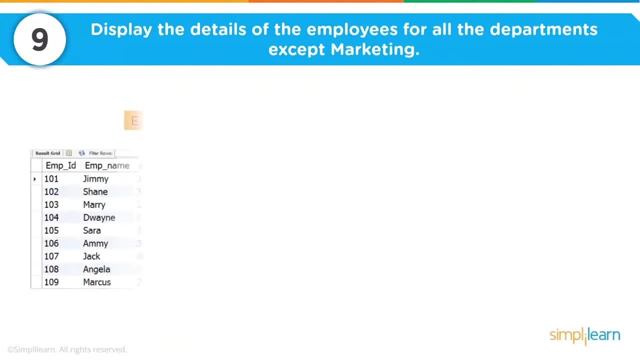 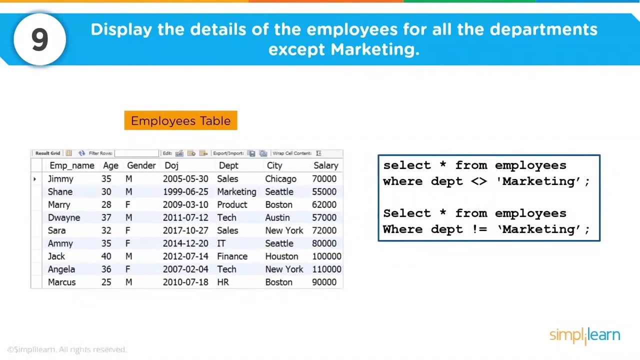 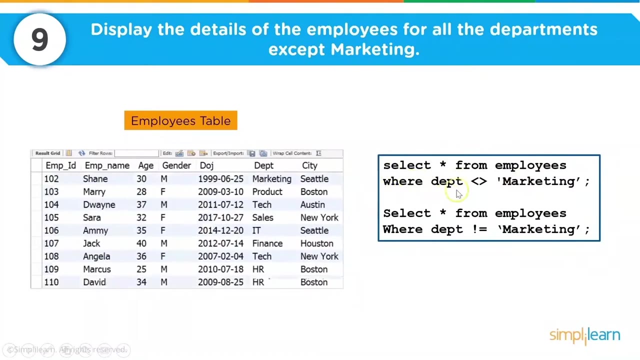 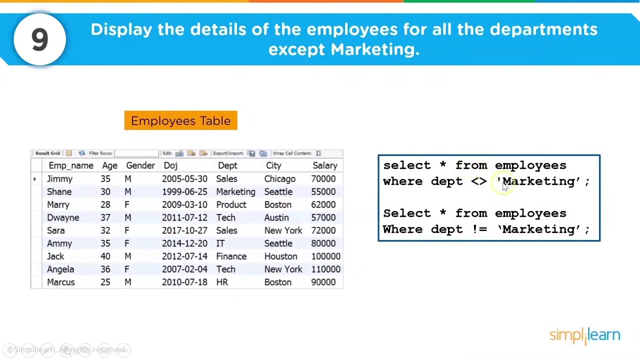 departments in each department except marketing. now here i have my employees table. now, if i were to display all the details of the employees apart from marketing department, i can give a condition like where department not equal to marketing. so this is the way how you write: not equal to. so you use the less than. 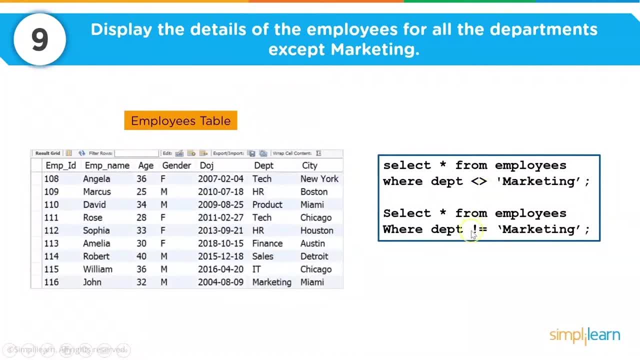 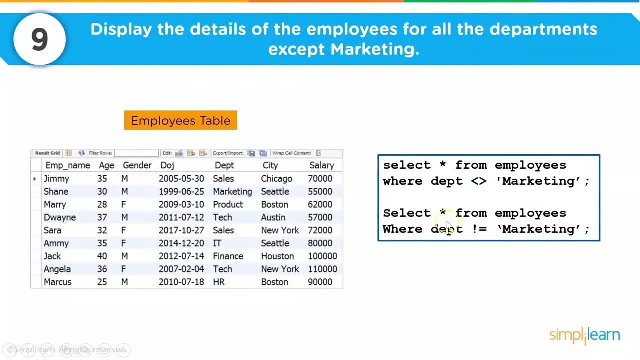 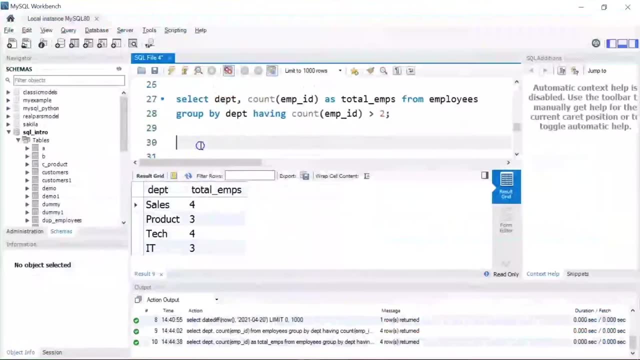 and greater than symbol. another way to do is use the exclamation mark and give equal to, so this means select all the employees where department is not equal to marketing. now, let's do this. i'll move down a bit and we'll give a comment as details of employees apart from marketing. 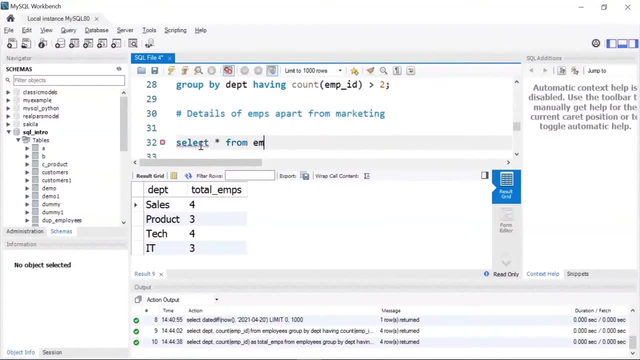 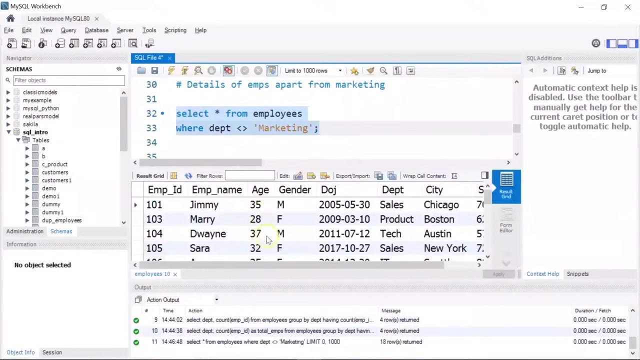 so the query would be: select star from employees using star, because i want to display all the details, that means i want to display all the columns. then i'm going to use my where condition, where department not equal to marketing, i'll put marketing under quotes. let's run it and see the results. there you go, so we have total. 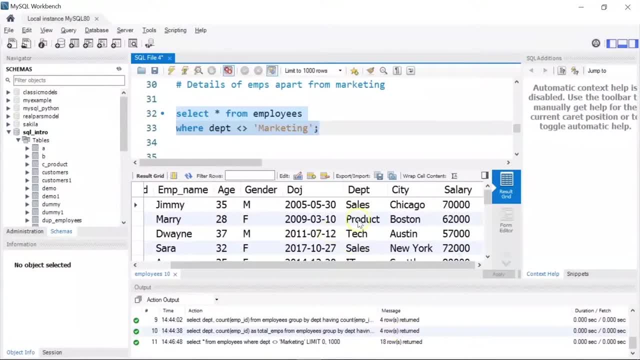 18 rows of information and if you see the department column, we have all the departments apart from marketing. now, if you remember, our employees table had total 20 rows of information, out of which two are missing, which means there were two employees who were from marketing department and those departments were not displaying. now, another way to do is: 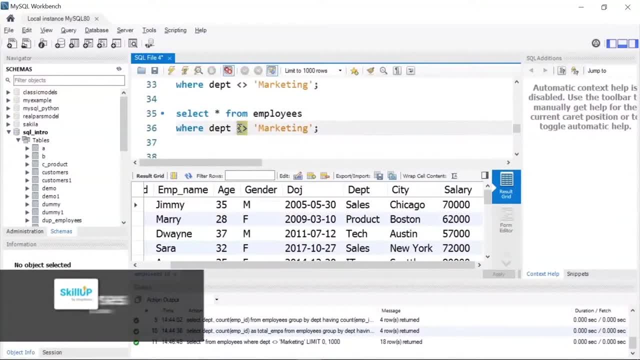 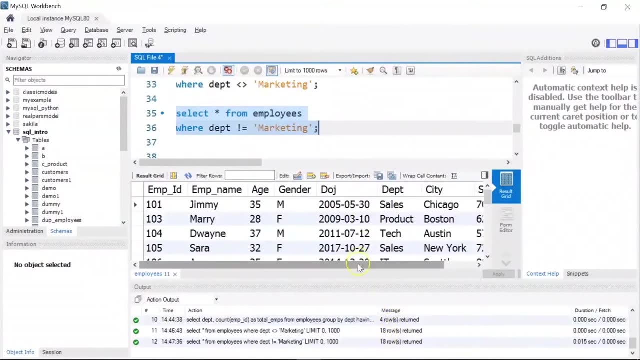 to use exclamation mark and equal to so this also means select all the employees where department is not equal to marketing. let's run this. you see here it gives us the same result and has written us 18 rows of information, leaving apart the employees from the marketing department. all right, 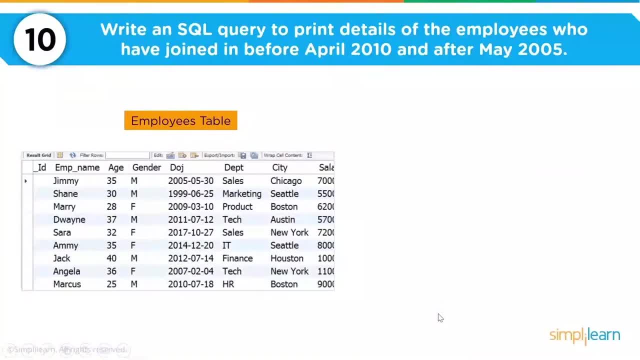 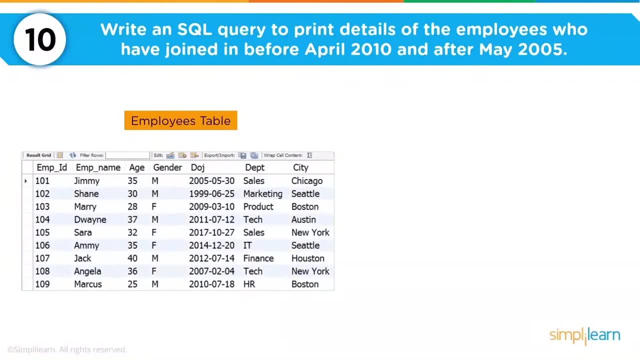 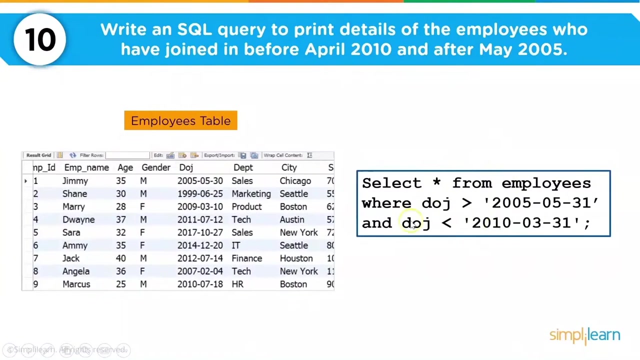 moving ahead. so our 10th question is to write an sql query to print the details of the employees who have joined before april 2010 and after may 2005. so here is my employees table and this is my sql query. so here we are, using just a where condition to filter our results and 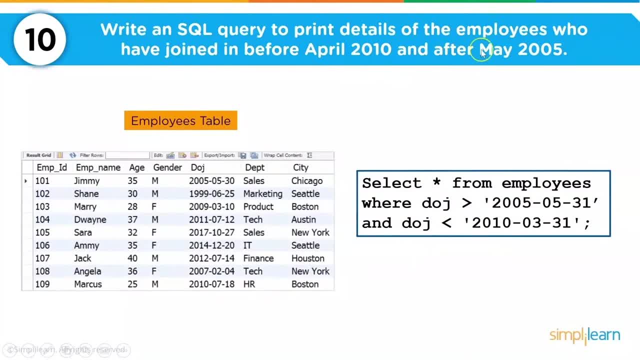 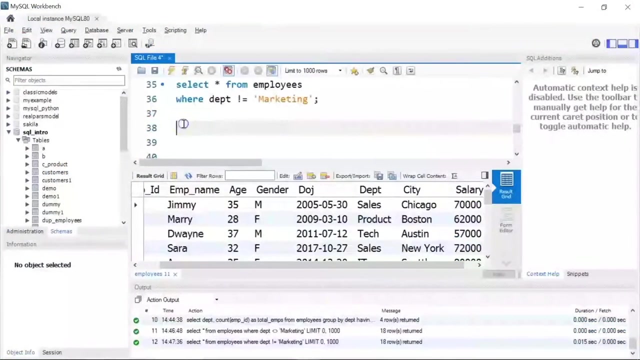 my condition is the employee should have joined after may 2005. so i have written after 31st of may 2005 and before april 2010, which is before 31st of march 2010. let's do this. i'll give a comment here. 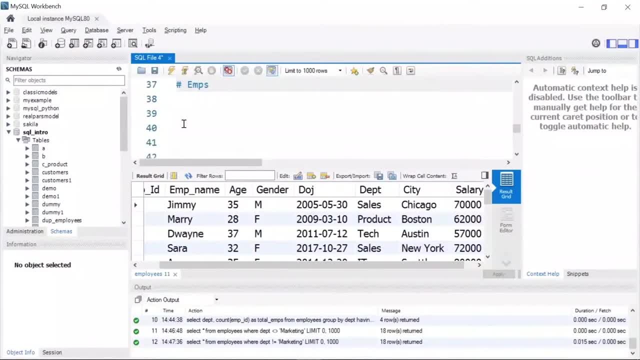 we'll write employees joined before april 2010 and after may 2005. now let's write our sql query. so i'll write select star from employees where my date of join. if you see, here i have a column called date of join which has the details about: 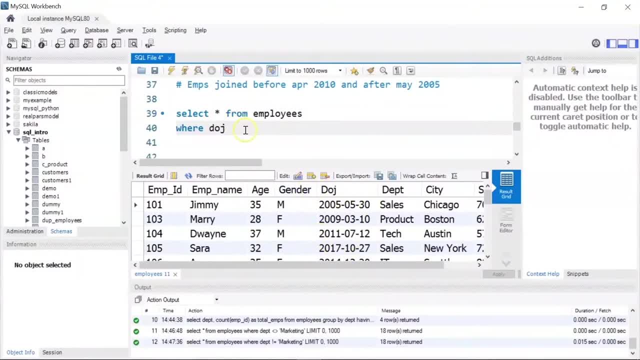 the day on which the employee had joined the company. so i'm going to write where date of join is greater than 31st of may 2005, so i'll write 2005. this is one of the formats to use date values. so this is the year value, this is the month value and this is the day value. and 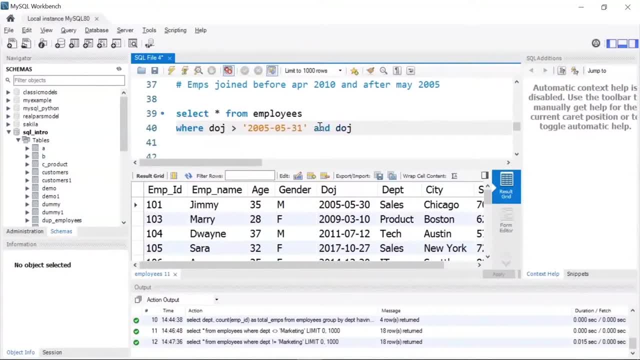 my date of join should be less than 31st of march 2010, so i'll write 2010, march 31st. i hope you were able to understand this. date of join greater than 31st of may 2005 means after may 2005 and date of join less than 31st of march 2010: this means employees joined before. 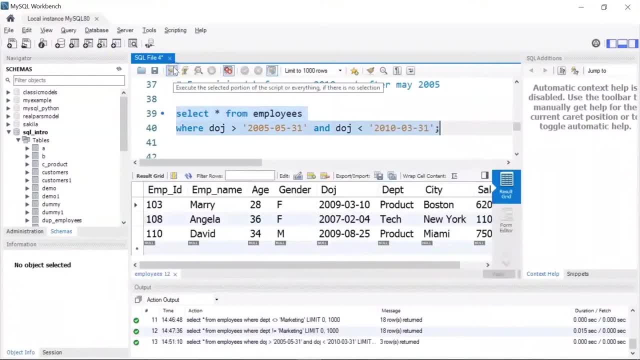 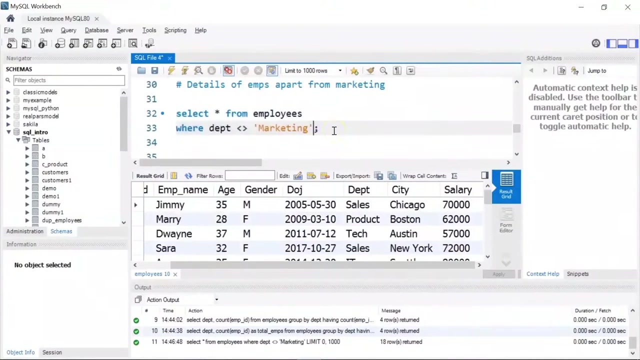 2010, april. let's run it okay. so we have total three employees in our table. you can see the date of join and all of them have joined after me, 2005, and before April 2010. department column: we have all the departments apart from marketing. now, if you remember, our employees table had: 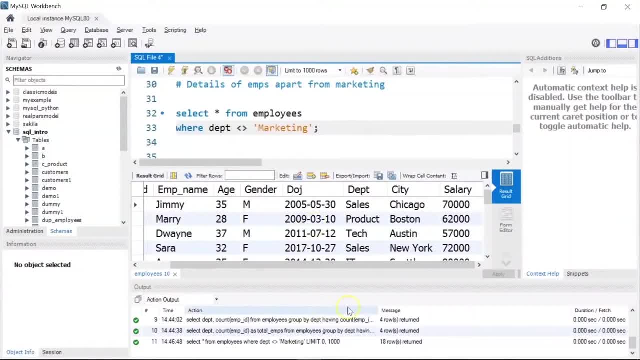 total 20 rows of information, out of which two are missing, which means there were two employees who were from marketing department and those departments we are not displaying now. another way to do is to use exclamation mark and equal to so. this also means select all the employees where. 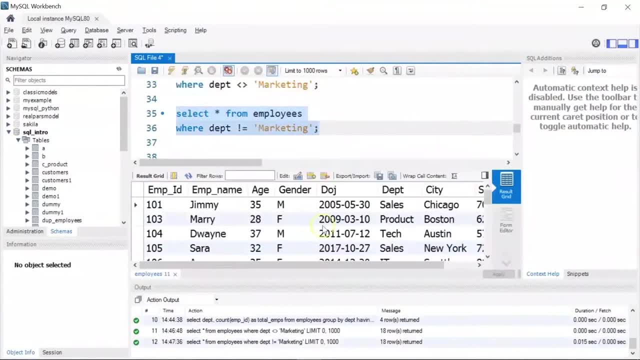 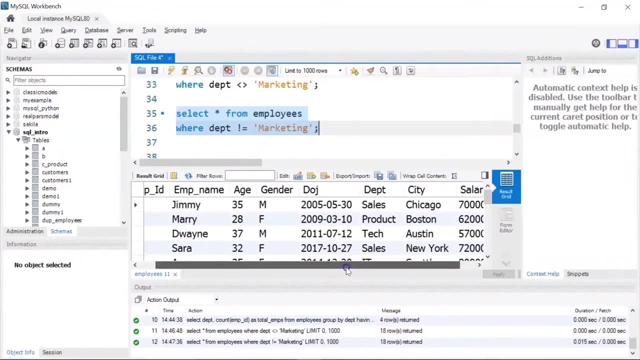 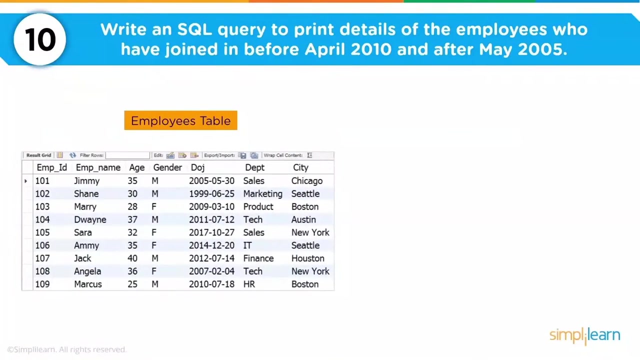 department is not equal to marketing. let's run this. you see here, it gives us the same result and has returned us 18 rows of information. let's run it again, leaving apart the employees from the marketing department. all right, now moving ahead. so i tenth question is to write an SQL query to print the details of 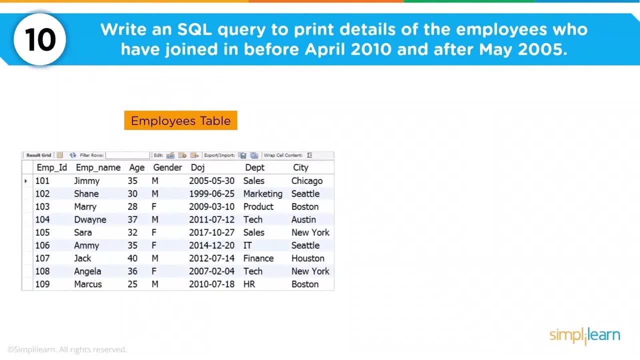 the employees who have joined before April 2010 and after May 2005. so here is my employees table and this is my SQL query. so here we are using just a where condition to filter our results, and my condition is the employee should have joined after May 2005. so I have written after 31st of May 2005. 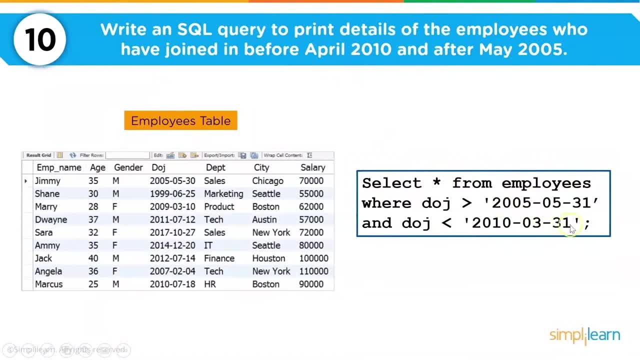 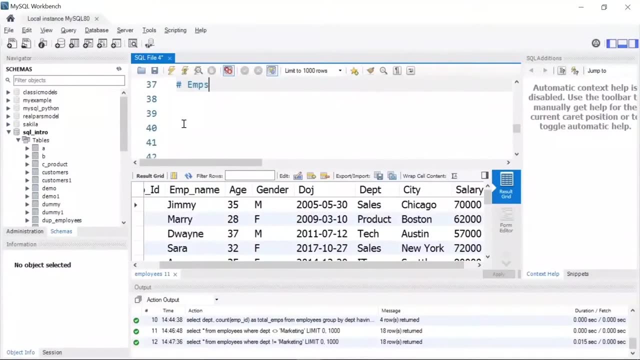 and before April 2010, which is before 31st of March 2010. let's do this. I'll give a comment here. we'll write employees joined before April 2010 and after May 2005. now let's write our SQL query. so I'll write select star from employees where 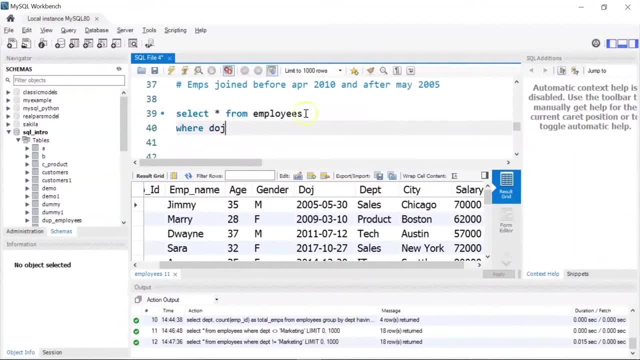 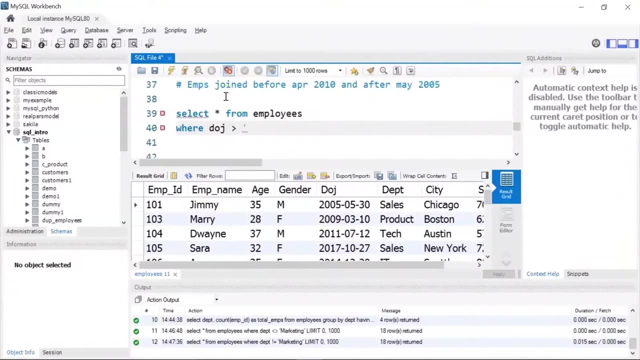 my date of join. if you see, here I have a column called date of join, which has the details about the day on which the employee had joined the company. so I'm going to write where date of join is greater than 31st of May 2005, so I'll write 2005. this is one of the formats to use date values, so this is the. 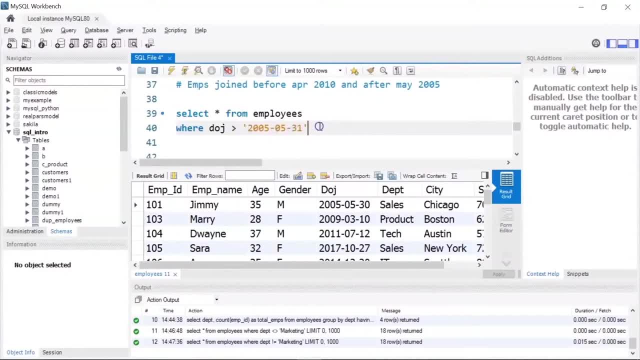 year value, this is the month value and this is the day value. and my date of join is greater than 31st of May 2005, so I'll write 2005. this is one of the formats to use date values. so this is the date of join should be less than 31st of March 2010, so I'll write 2010, March 31st. I hope you. 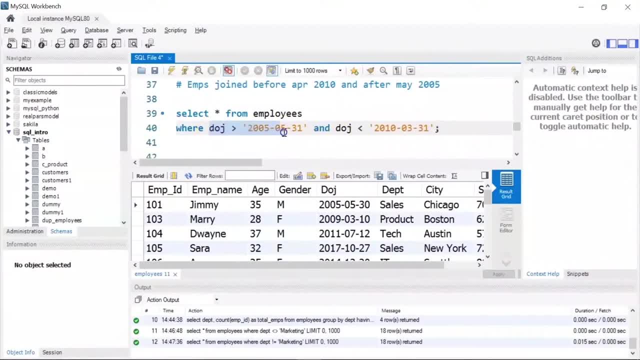 were able to understand this. date of join greater than 31st of May 2005 means after May 2005 and date of join less than 31st of March 2010. this means employees joined before 2010- April. let's run it okay. so we have total three employees in our table. you can see the date of join and all of 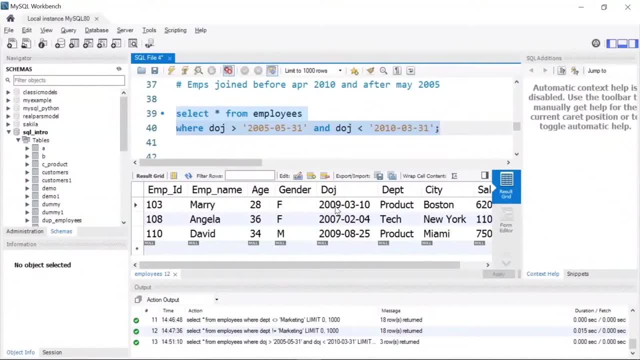 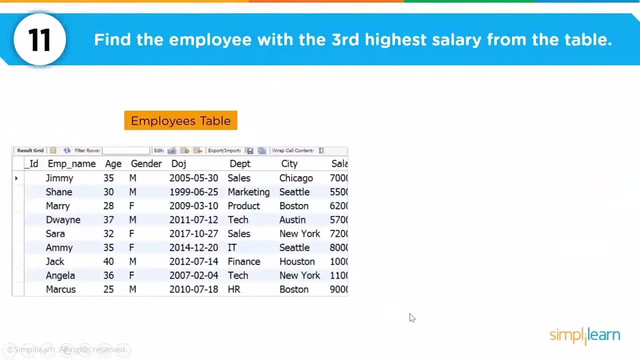 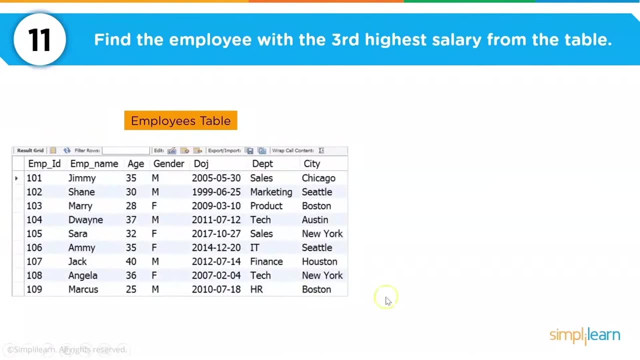 them have joined after may 2005 and before april 2010. okay, now moving ahead to the 11th question. so here we want to find the employee with the third highest salary from the table. so i have my employee staple here and my command would look something like this: so here we are going to. 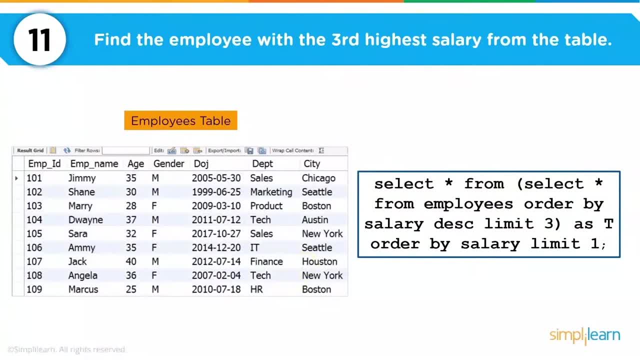 explore how to write sub queries in sql. so i'm using a sub query here where i'm trying to find the employees who have the top three salaries, or the top three employees who have the highest salaries, and from that i'm going to filter out my third highest salary employee. so let's do it on. 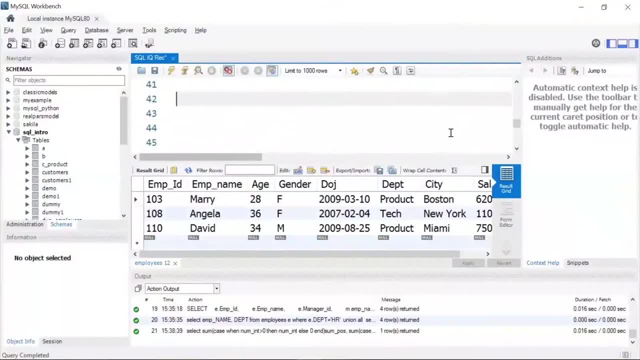 our workbench. okay, so i'll come down and let me give a comment as third highest salary. okay, so let me first write down my sql query and then i'll explain. so i'll write select star from. after that i'll start a bracket and write my inner query so i'll write select star from. 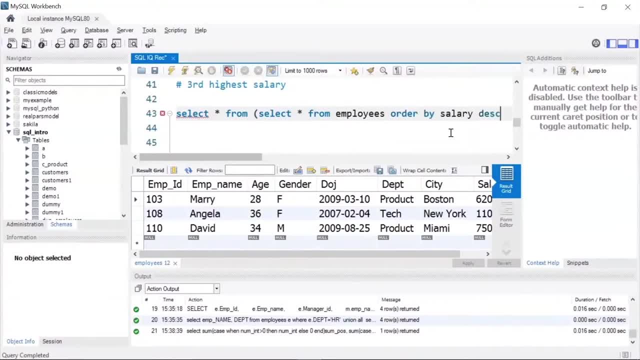 order by salary descending. then i'll use my limit keyword and i'll write limit three, as i'll give an alias name, let's say t, and then i'm again going to use my order by salary, limit one. okay, now let me explain you the flow. so first let me run the inner query. i'll select my inner query. 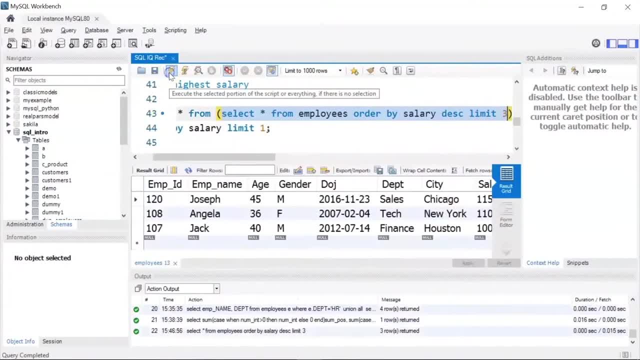 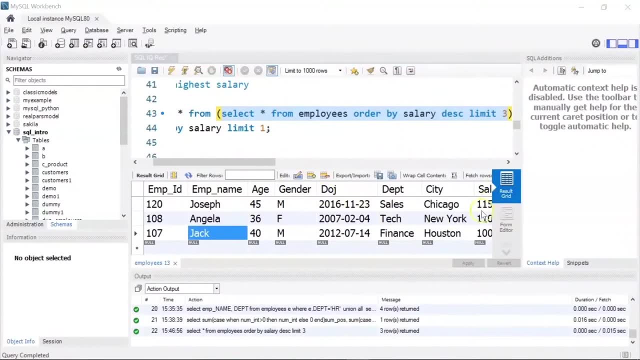 and i'll run it. so the inner query returns my top three employees who have the highest salary, and this is ordered in descending order. since i used salary descending, now let me just use this. okay, now you can see it clearly. so these are my top three employees who have the highest. 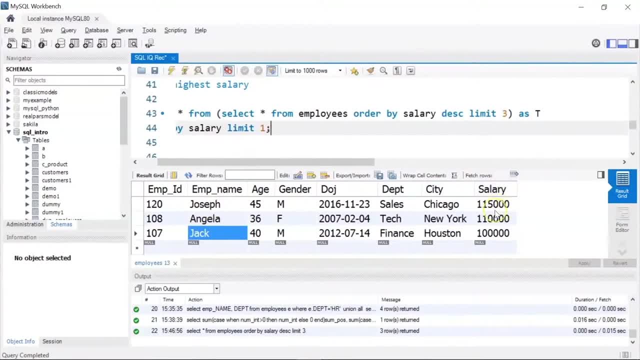 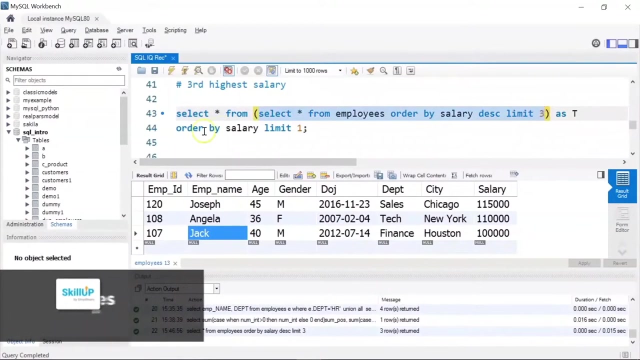 so Joseph has the maximum salary, followed by Angela, and then we have Jack. now from this I want to return only the record for Jack, because Jack is the employee who earns the third highest salary. so for that I am going to use the result returned by my sub query or the inner query, and on top of this I am 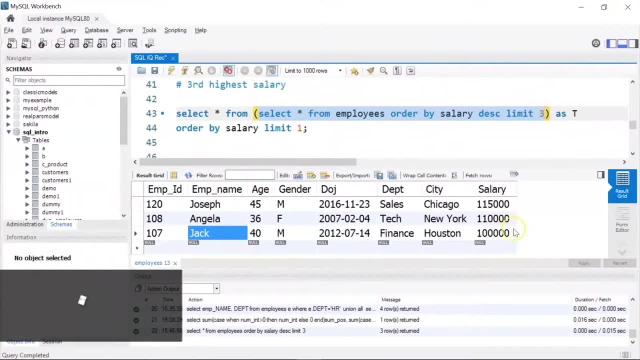 going to order the salary and say limit equal to 1. so I am again ordering this salary in ascending order. so what will happen? Jack will appear at the top, Angela will be at the second place and Joseph will come to the third place and from there I am using limit 1 so that I can only get the record for Jack now if 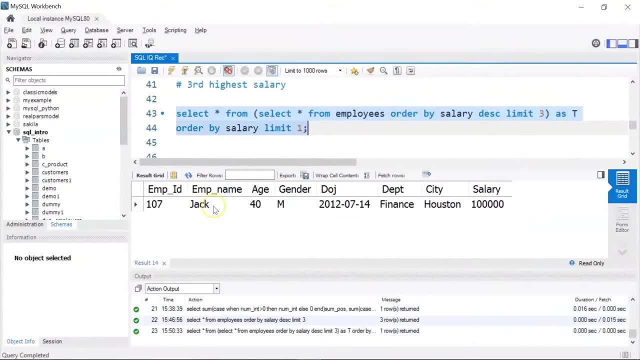 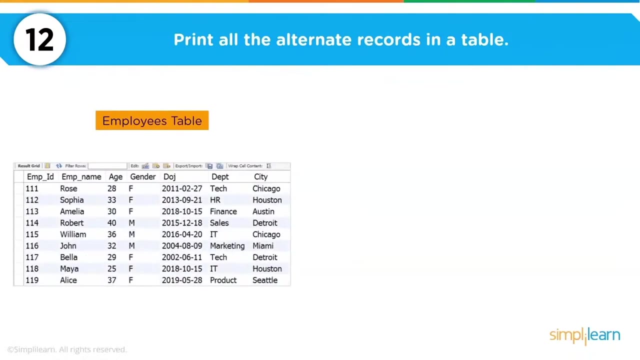 I run the entire query. you see the result. I have my employee name as Jack, who owns the third highest salary. okay, now, moving ahead to the 12th question. the question is to print all the alternate records in a table. so here is my employees table and from this 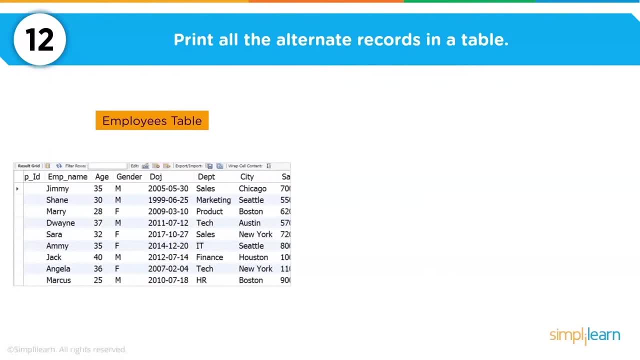 table. I am going to print all the alternate records. for example, I am going to print my employee ID 101, then I am going to skip 102 and print 103, followed by 105, 107, 109, so all the employee IDs that have an odd value. 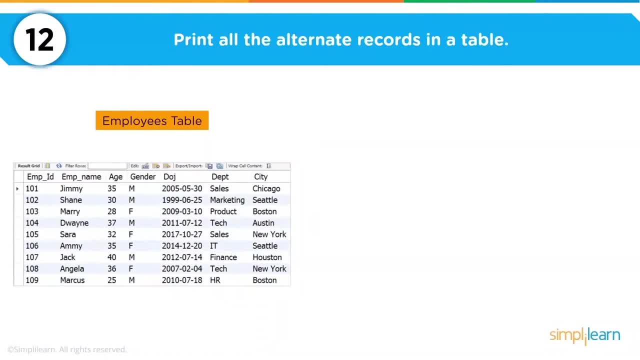 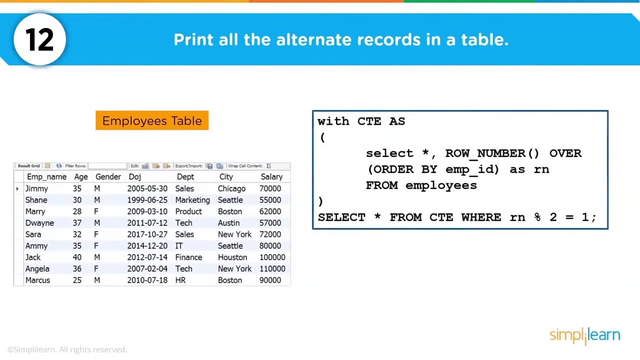 and you can look at this example in another way of displaying the employees which have an employee ID of even numbers, so 102, 104, 106 and so on. now the way to do is either you can use a simple select clause and say employee ID percentage or modulus to equal to 0, which means I want to filter only those. 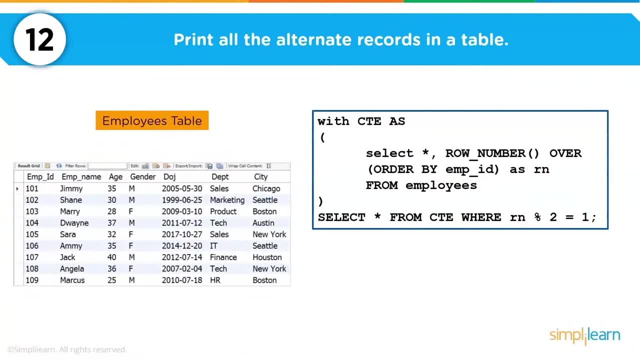 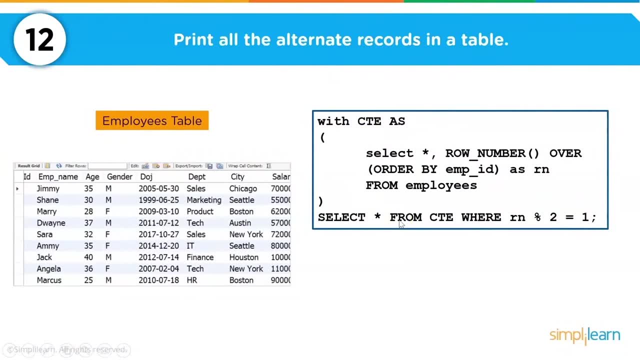 employees which have an Olympic plus equal to 0. broad future, only those employees which have an even employeeверse value. this means I want to filter only those employees which have an bruise, no even employee ID. else what you can do is you can use a CTE, as you can see here. so CTE. 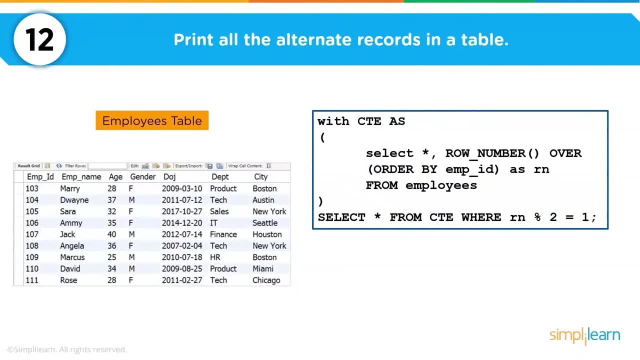 or the common table expression, is a temporary named result set that you can reference within a select insert, update or delete statement. now it is used to simplify complex joints and sub queries and to provide a means to query hierarchical data. now let's write this query on our workbench and see how it. 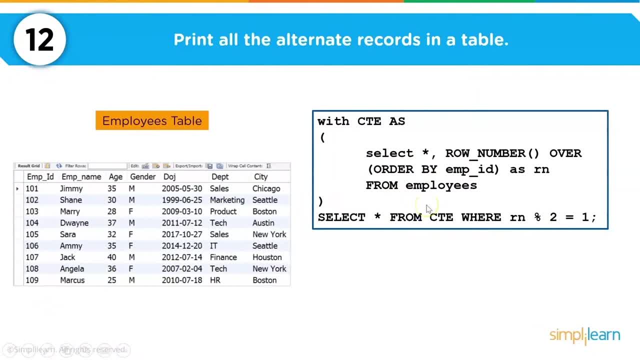 works. before that, let me explain you. I am using a few new functions, such as row number. this will create a row number for each of the rows or the records present in my table, and then, from this city, I am going to use my filter clause or the. 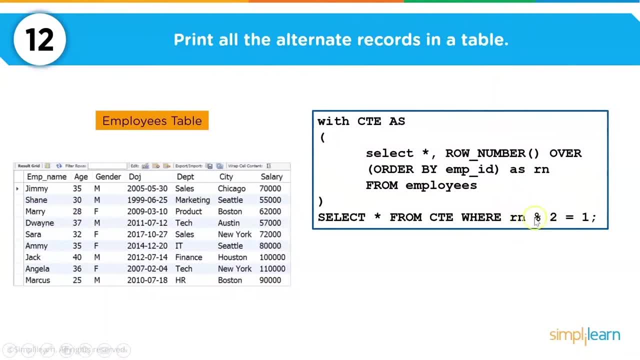 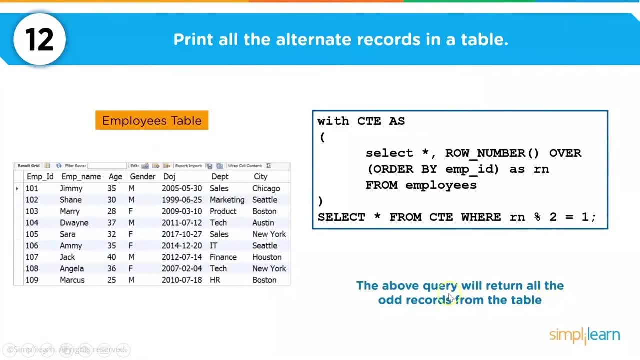 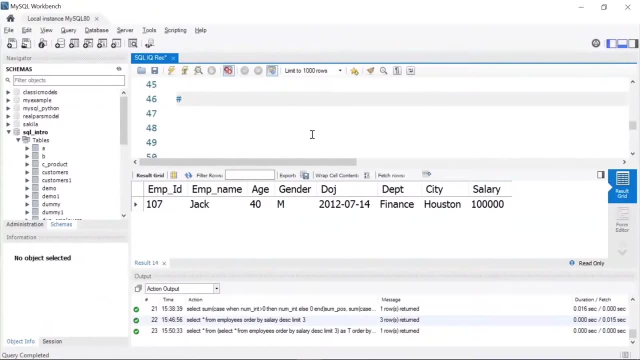 where clause: where RN, which is row number, percentage 2 equal to equal to 1. so this will return only the odd records from the table. let's see how to do it okay, so I'll give a comment. print alternate records. okay, now I will start with my simple query, which is: select star from employees. 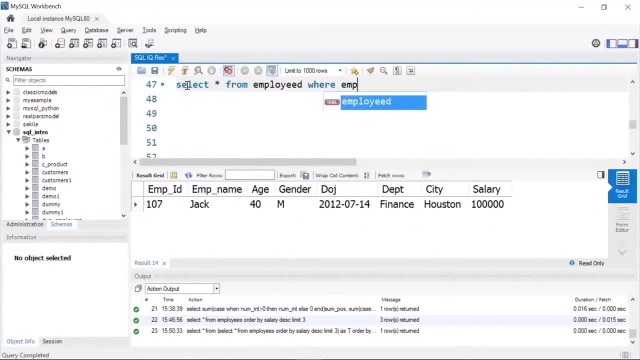 where, let's say, I want to find only the even employee IDs or the employees who have an even employee id, so i can use employee id percentage 2 equal to 0, so it has to be a perfect division and the result should be 0. only then i can get only the. 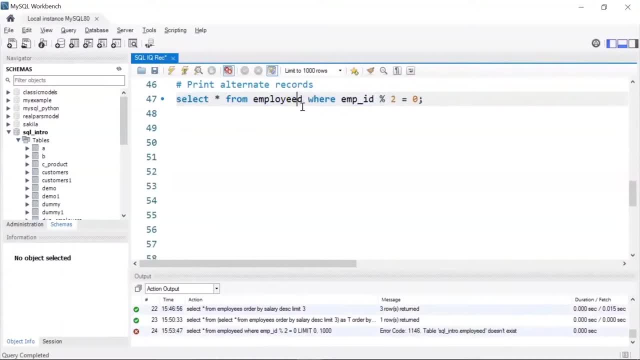 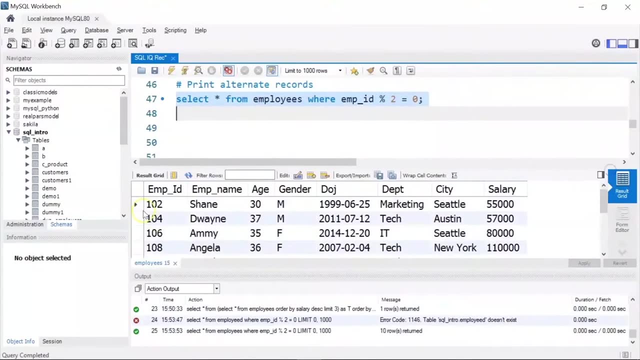 even employees if i run this. okay, there was an error here, it should be employees. i'll run it again. you can see here i have printed the alternate records in a table, so we have skipped 101, because it is not divisible by 2. i've started with 102, followed by 104, 106, 108 and then finally. 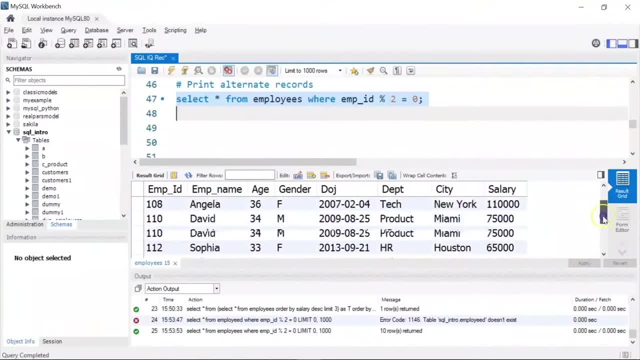 we have 120 or 120.. now, if you want to print only the odd records in the table, you can use employee id. percentage 2 equal to 1. so you can see here i have 101, 103, 105, 107, up to 119. 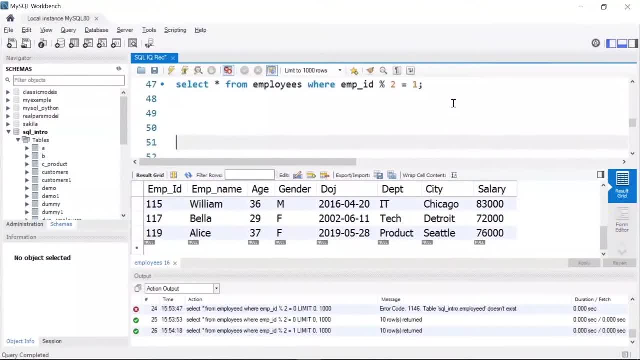 now, the best way to do this is to use a common table expression of cte. so i'll start with my command, that is, with cte. as i'll start with my bracket, i'll write select star comma. then i'm going to use my row number function, so i'll write row number. 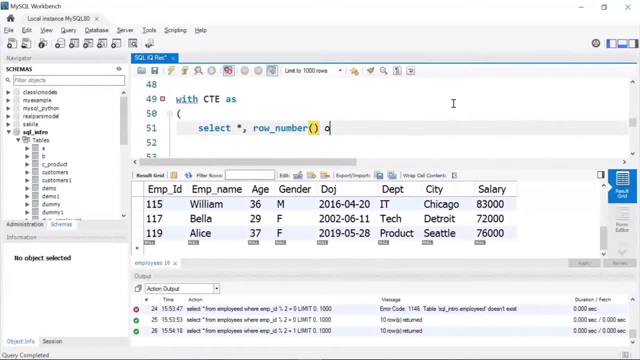 then i'll write over. then i'll use order by employee id. so this row number for each of the rows is going to be created over my employee id column and that is sorted in ascending order. i'll give an alias as rn, which stands for row number from my table, that is, employees. 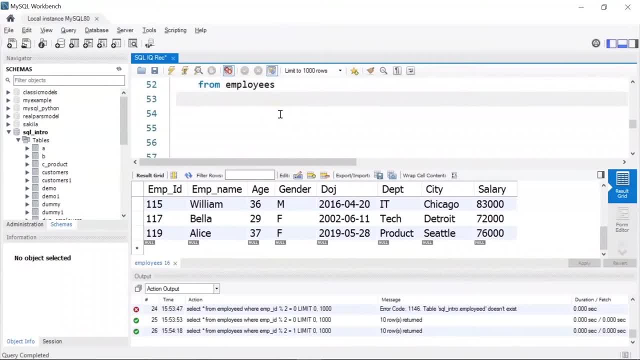 i'll scroll down and then i'm going to close my bracket. i'll write select- let me remove the space here. okay, i'll add select star from cte, where my row number percentage 2 equal to 1.. now let's see this from the top. so i have my common table expression where i am: 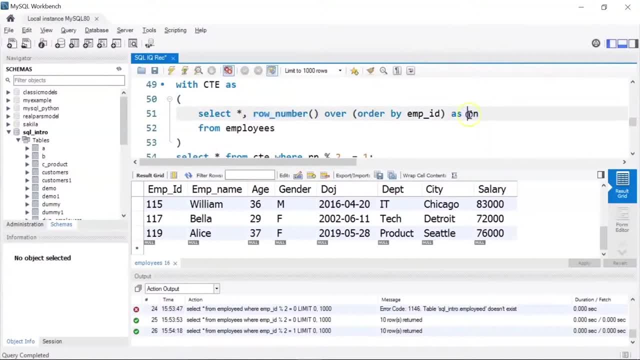 going to create a row number column named as rn, and this row number column is based on my employee id column, which is sorted in ascending order, and from that i am going to filter only those row number values that are not divisible by 2, or i am going to print: 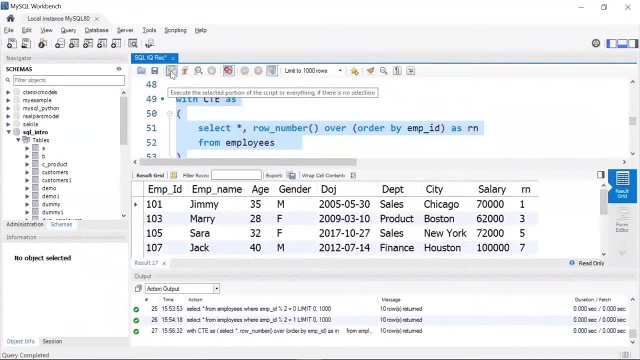 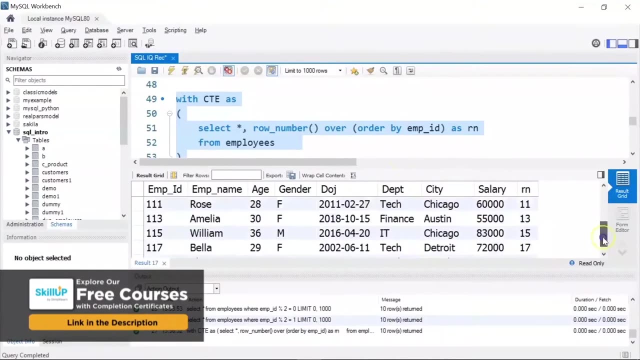 only the odd records from the table. so let's run it and see the results. there you go. so here, if you mark, i have my row number column created and i am filtering only the odd records in the table. so it starts with 1, 3, 5, 7 and goes up to 19,. and similarly, here you can see the employee id's, the. 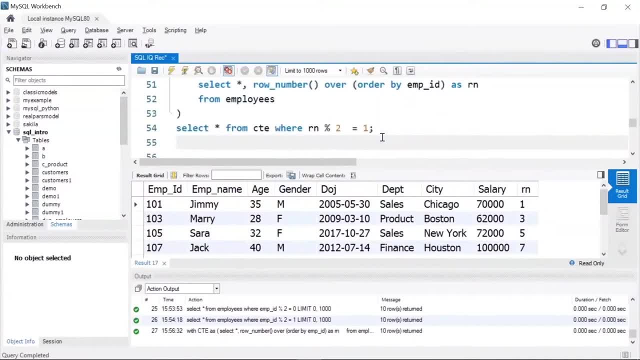 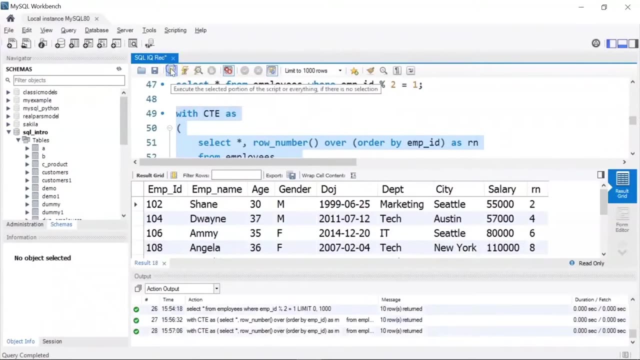 name, the age, gender and other information. now, if you were to print the even records in the table- alternate even records- you can use rn percentage, 2 equal to 0. let's see the difference. i'll run this. there you go. so i have my even row number, starting from 2, which goes up to: 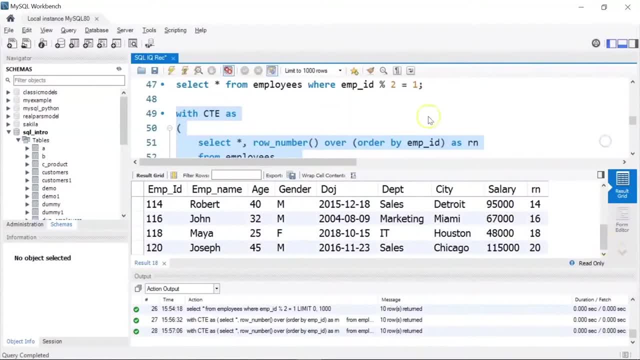 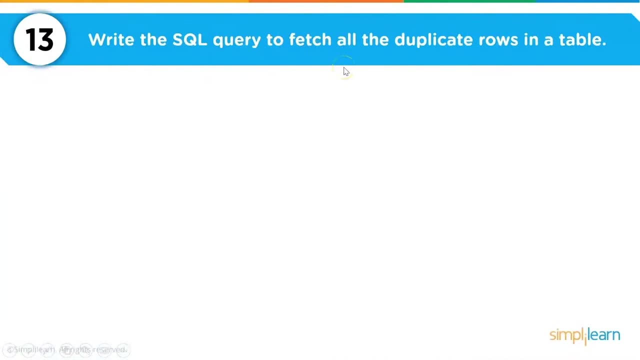 20. okay, so this is how you can print alternate records in a table. now moving to the next question. now, in the 13th question, we want to write an sql query to fetch all the duplicate rows in a table. now, this is another crucial interview question that 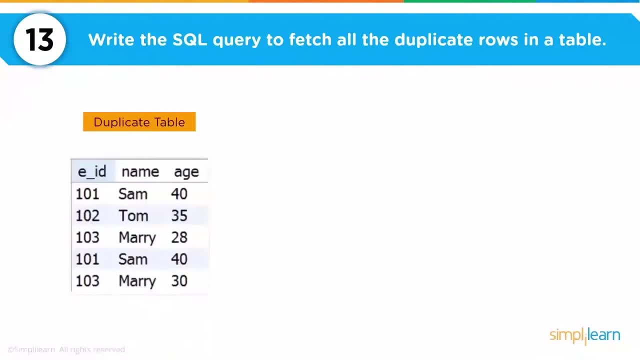 is often asked in most of the interviews. now i have a table which is named as duplicate table and here you can see i have some employee id, name and age and a few records are duplicated. for example, 101, 101, 101, sam 40. the first record is duplicated and you can see here it has the same. 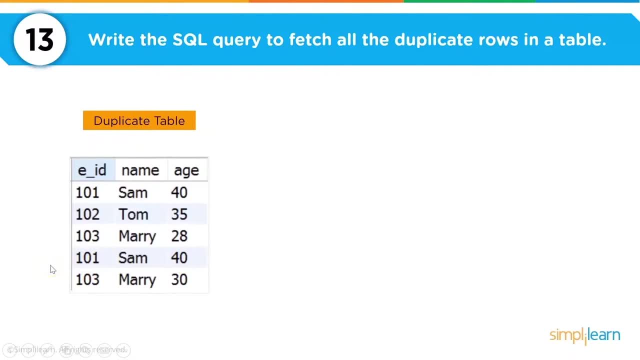 values. now, if you mark 103, mary and 28 is not duplicated, because here the age is different, so this is a different person than compared to the third name that you have. so this is how you can find the duplicate rows in a table. so i'm going to. 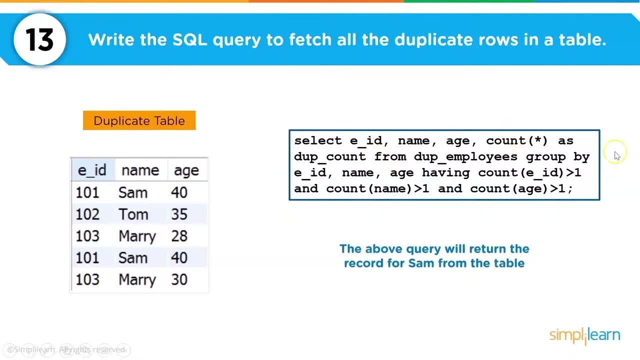 select my employee id name and age and then count all the employee ids- the names and age- and compare them with whether they are greater than 1 or not. so if they are greater than 1, then i'll say that particular record is duplicated or is present more than one time in the table. let's do this. 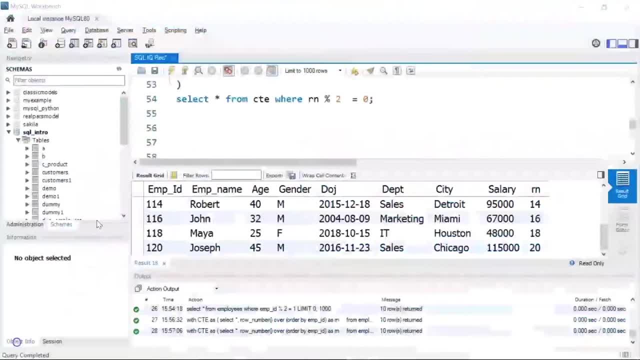 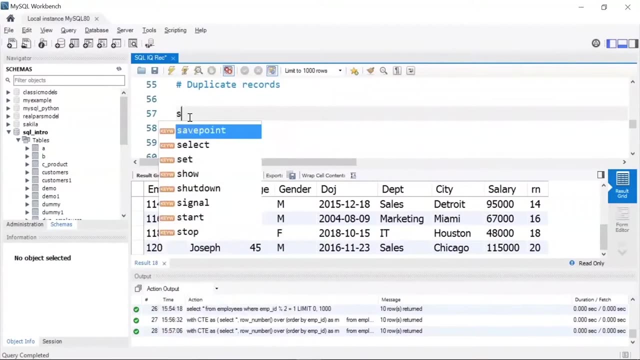 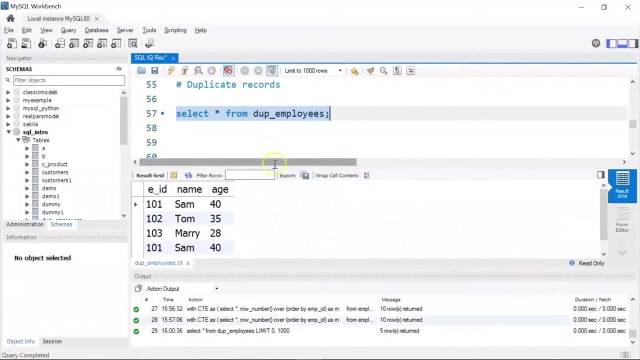 implementation on our workbench. okay, so i'll come down and let me give my comment as duplicate records. okay, so let me first show you the records that are present in my table. so i'll write select star from dup, underscore employees. so i'll run it. okay, you can see, here i have my table that we saw in the slides. 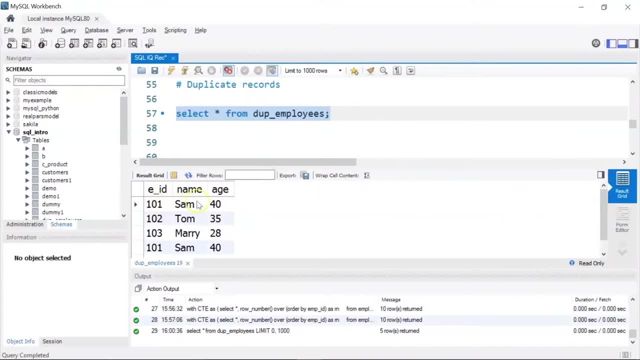 so employee id 101 with name sam and age 40 is duplicated. so we want to find this duplicate record. the way to do is i'll write select e underscore id which is employee id comma, name comma, age comma. i'm going to write e underscore id. 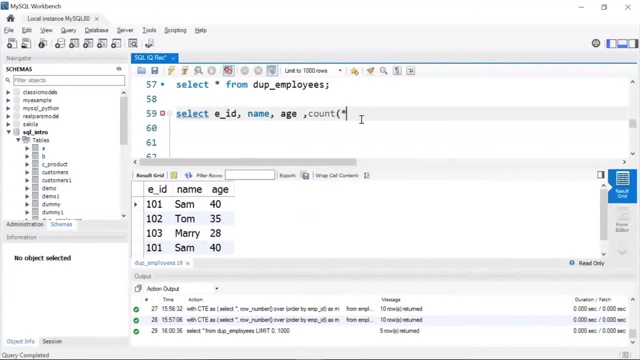 to count all of them, so i'll write count star as duplicate count. this is my alias name from my table that is dup underscore employees. i'll say group by employee id, name and age, and then i'm going to use my having clause saying having count of employee id is greater than 1 and 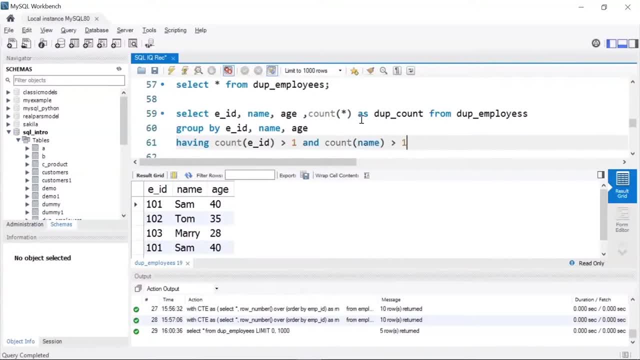 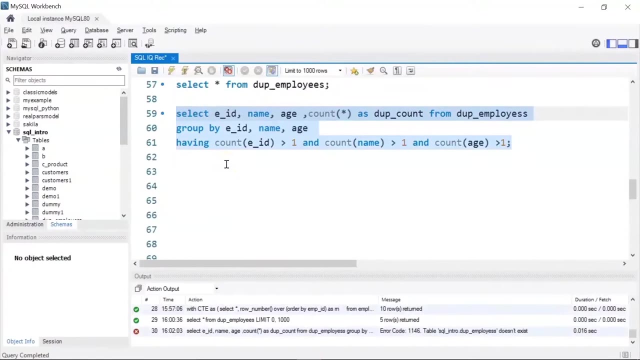 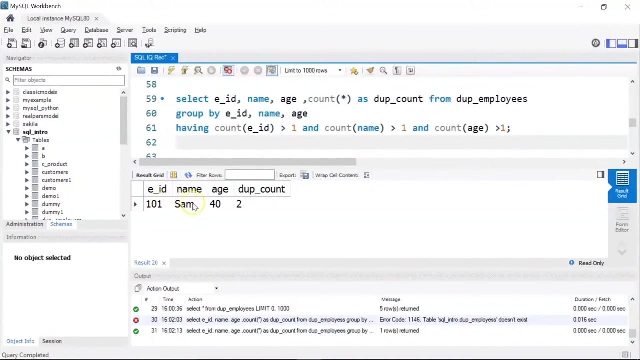 count of name should also be greater than 1 and my count of each should also be greater than 1. let's run it and see the results. okay, there is some error here. the name of the table should be employees. okay, let's run again. we have our correct result. that is employee id 101 with name sam and age 40 is duplicated. 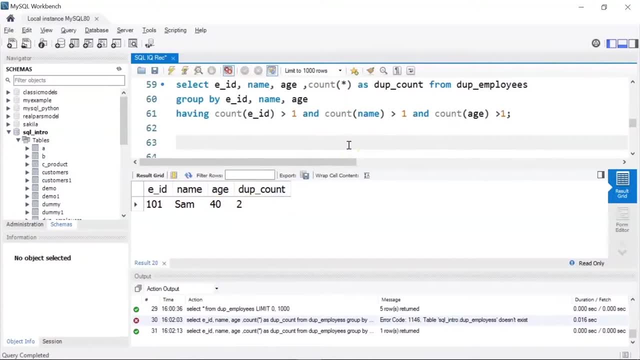 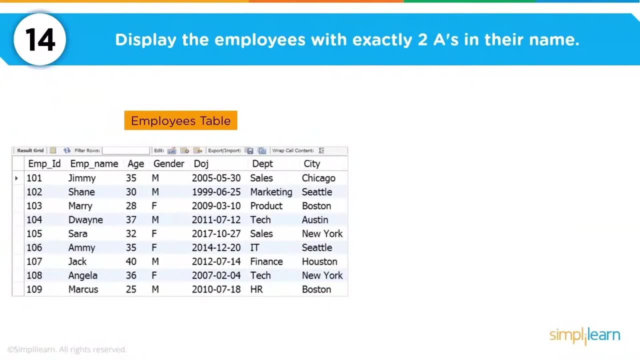 so the value is 2. great, now moving ahead. now the 14th question is a bit tricky, wherein we want to display the employees with exactly two a's in their name. so you see, here i have my employee names and there are certain employees who have just two a's in their names. so i want to find 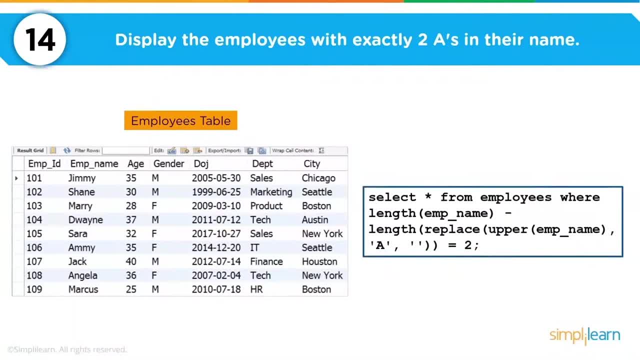 those employees. only now the way to do is- it is a bit tricky to understand. i am going to break it down and make you understand. on my mysql workbench, so here you can just have a glance- i write select star from employees, where i am finding the length of my employee name, and then 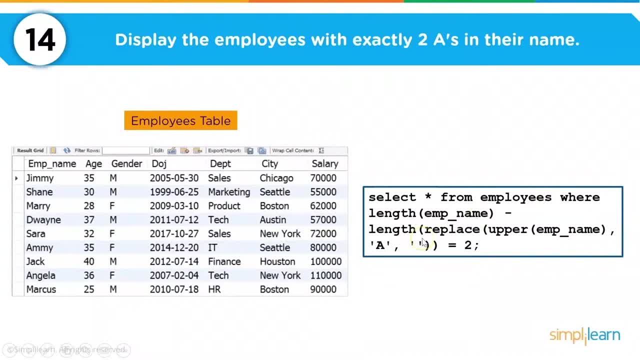 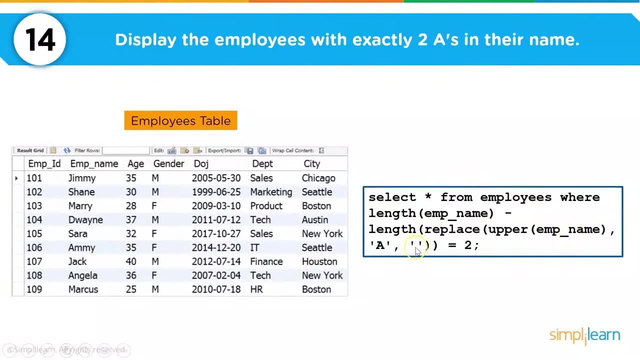 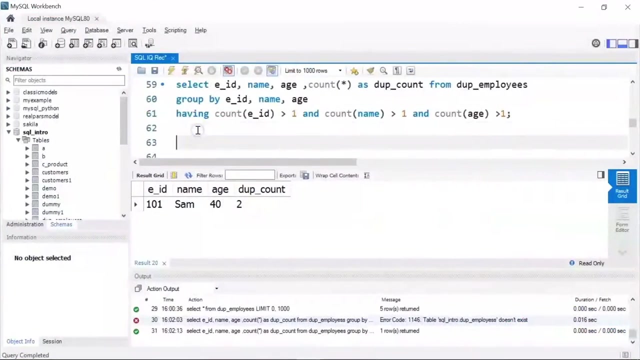 subtracting my length, wherein i have replaced my employee name that has a with a blank, and if this subtraction is equal to 2, then that particular employee has two a's in their names. so let me show this first. let me first give my comment as employees with two e's- okay. 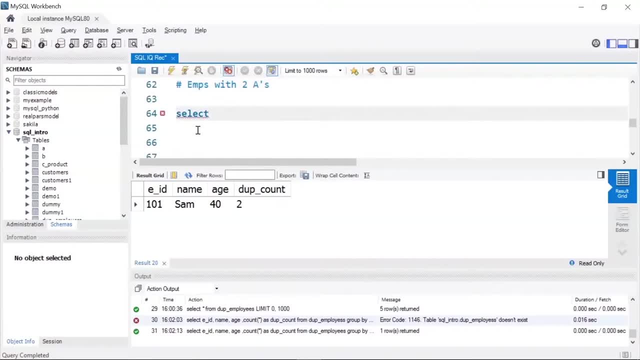 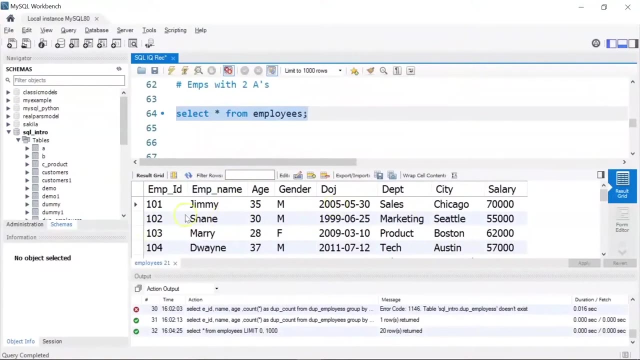 so first i'm going to write a select statement, okay, before that i'll show you the records present in my table. okay, if you see here shane is one of the employees that has just 1a in its name, then we have mary 1a. dwayne has 1a, but if you see 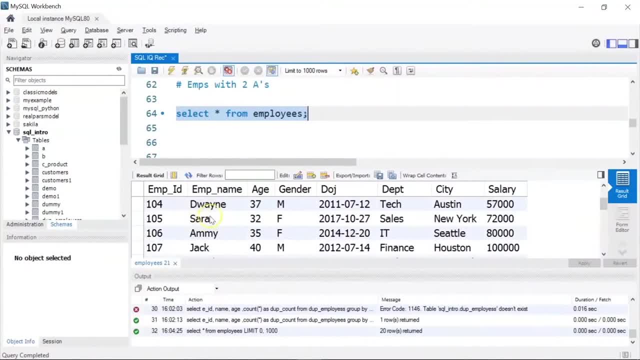 sara. sarah has 2 a in the name, so we want to extract sarah. then jack has 1a again. if you see angela, angela has 2a. it doesn't matter if it is uppercase a or lowercase a, we just need to find her name. i am going to write a little b in the name, start and single a there. 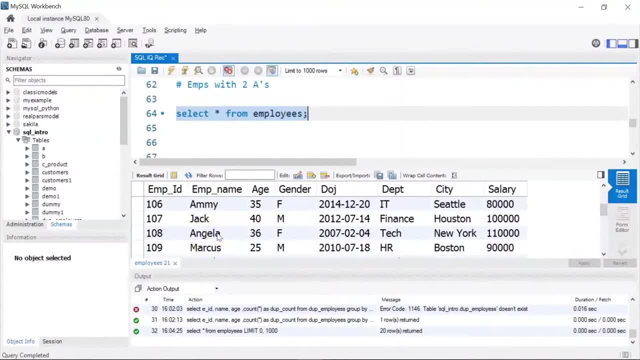 just need to find if the employees have two a's in their name and similarly, if i scroll down, let me check if we have any other employee with two a's in their name. marcus has one, david has one, sophia has one. we also have amelia that has two a's in its name or in her name, and we also have 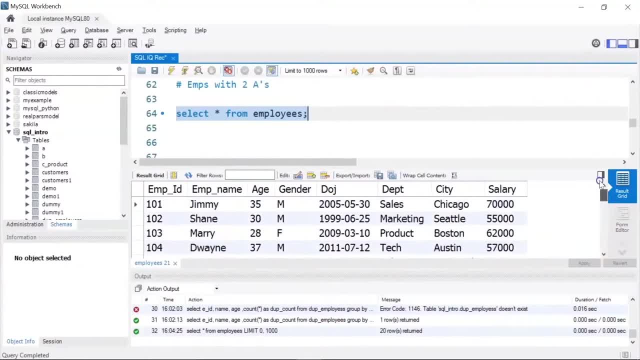 maya. okay, now let me go ahead and write a sql query and then i'll explain you what i'm trying to do. i'll write select- i'm using the length function and in the length function i'm going to replace. then i'll use another function called upper, on top of employee name. 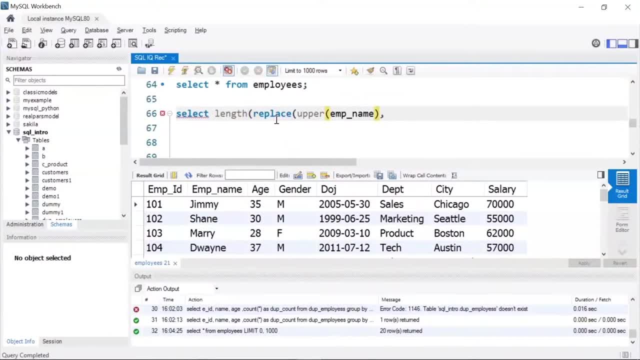 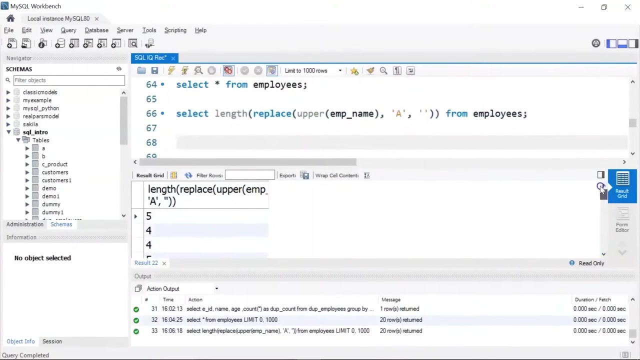 i'll write a and then replace it with a blank. so i'm using quotations to represent blank from employees. okay, let's run this and see the results. you see here it has given us the length of the employee string after replacing all the a's with a blank. so here i'm essentially converting my employee. 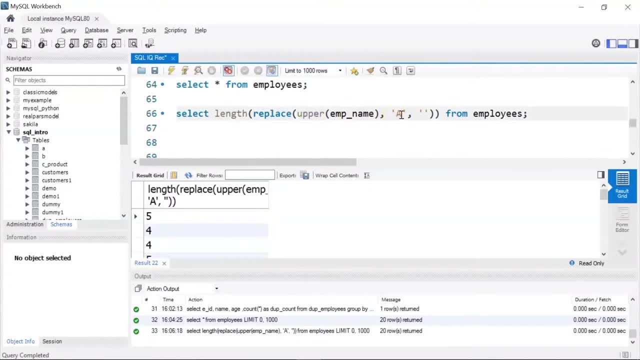 names to uppercase and i'm changing. wherever there is an a, i'm replacing that a with a blank and then i'm finding the length. so this trick i'm going to use in my final query. so i'll write select star from employees, where what i'm going to do is i'll bring this to the next line. i'll write length of. 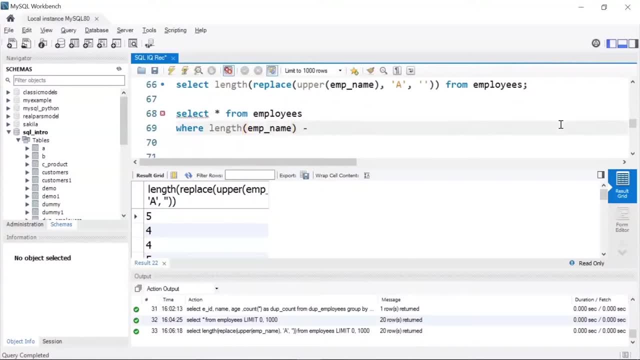 employee name minus, then i'm going to use my above condition. i'll copy this, i'll paste it here, and this value should be two. so what i'm doing is i am first finding out the length of my employee name. from that i'm subtracting the length after replacing the a's present in the employee name. 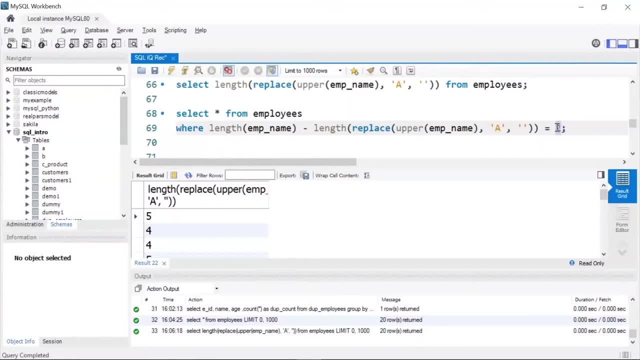 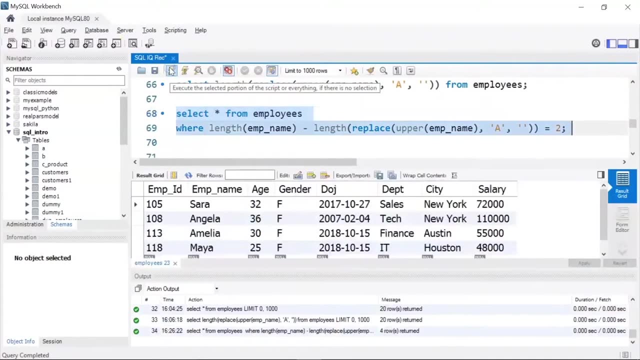 with a blank, and this value should be equal to two, the reason being we are only trying to find the employees who have two a's in their name. let's run and see the results. okay, if you see, here we have sarah, angela, emilia and maia, who have 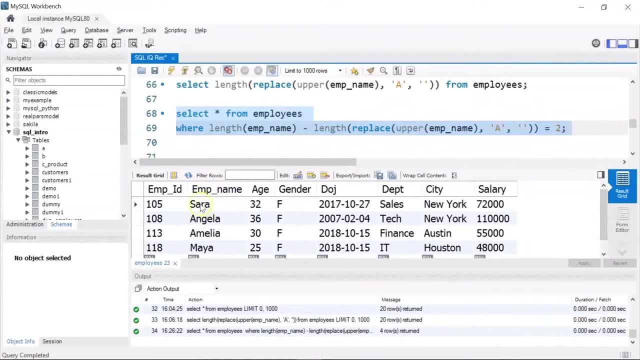 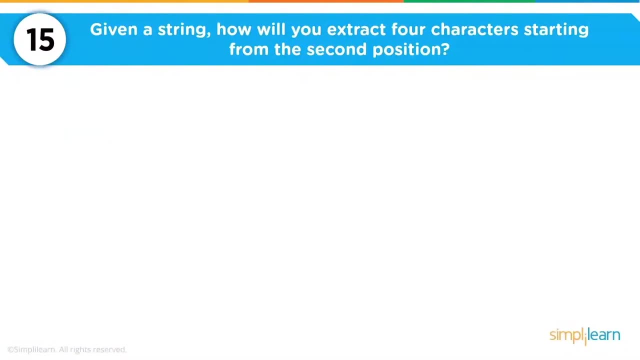 two a's in their name. so we have sarah that has two, a angel has two, a emilia has two ways and then maya also has two a. okay, now moving ahead. now the 15th question is given a string. how will you extract four characters starting from the? 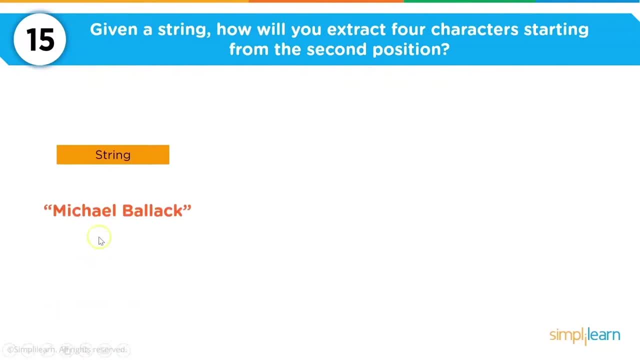 second position. so i have my string here which says michael balak of. michael balak, you must be aware, is a popular footballer, he is from germany and also was the captain of germany. so from the string michael balak, i am going to extract four characters, starting from the second position. 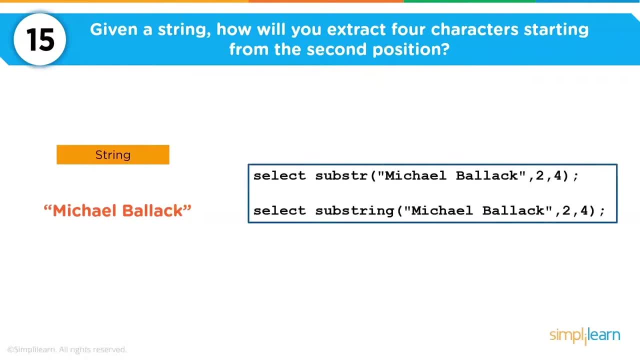 you can use two inbuilt mysql functions to do this. the first is called substr, wherein we pass in the string, then we give the position from where we want to extract the characters. so here i am going to extract from the second position. so hence two, and then the number. 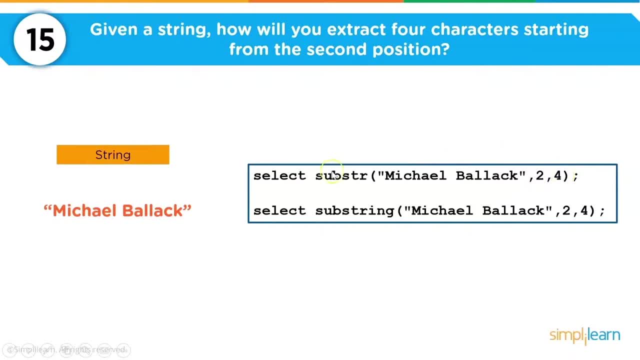 of characters that you want to extract, which is four. the other way is to use the substring function, which is again similar to the substr function. in the substring function also, i am first passing in my input string and then giving my starting position, which is two, and then i want to 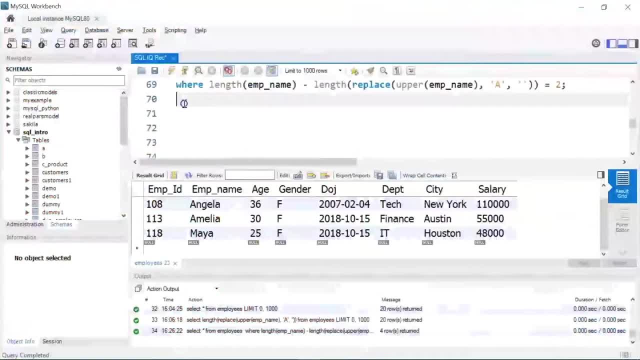 extract four characters from it. let's do it. i'll give a comment: extract strings. so here i'm going to write select. first i'm going to use substr, which is my inbuilt function. i'm going to pass in my input string which says michael balak. 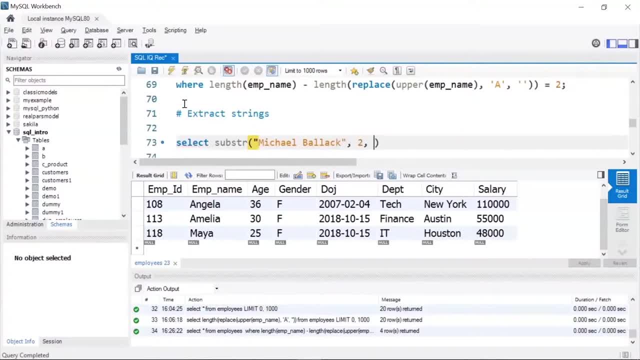 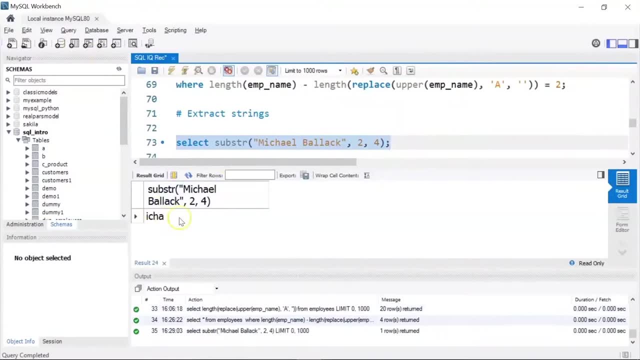 and then i'll give my starting position, which is two, and then the number of characters, that is four. let's run it and see the results. you can see here it has given us icha. so if you see, m is at the first position. from the second position onwards, i needed: 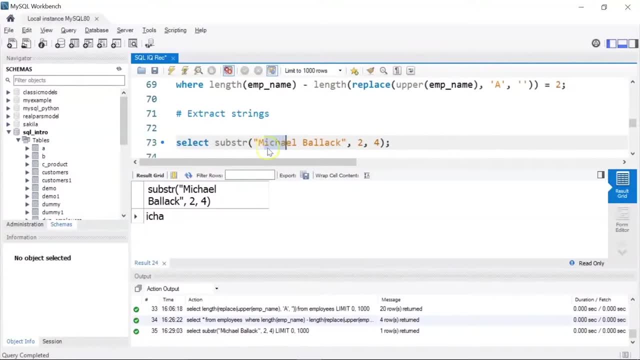 four characters, so m, c, h and e. these are the four characters starting from the second position. similarly, let me just copy this, and instead of substr i'm going to use the substr function. i'll write just ing. that becomes substring. let's select and run it and this: 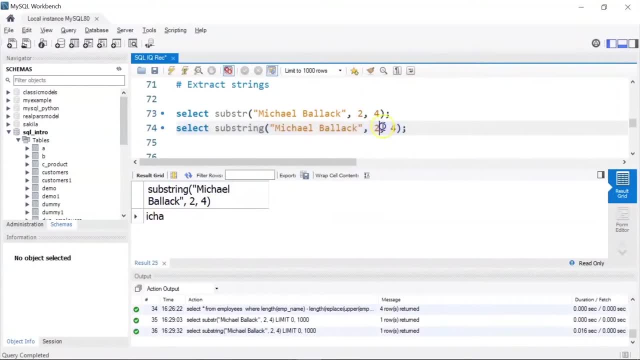 also returns the same result. suppose you wanted to extract from the fourth position. you wanted to extract, let's say, three characters. let's see the results. it gives us: h, a and e. if you see here, m is the first position, i is at the second position, c is at the third position. 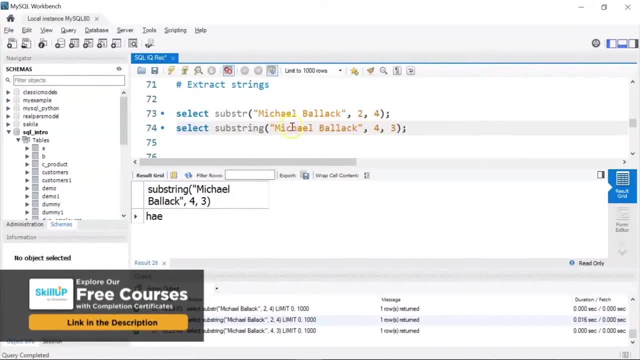 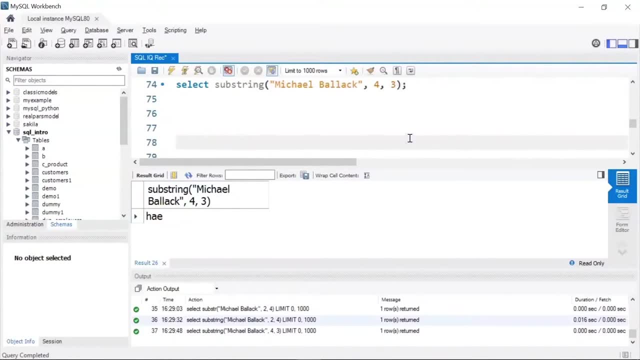 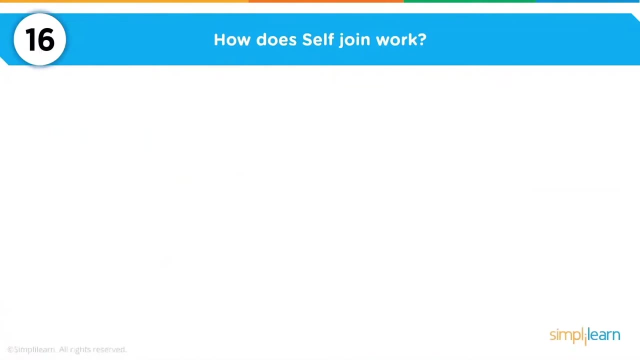 h starts from the fourth position, so h, a and e are the next three characters starting from the fourth position. so hence, this is the result. all right now, moving ahead now. my sixteenth question is on how does self join work? so self joined joins a table to itself, so the table must. 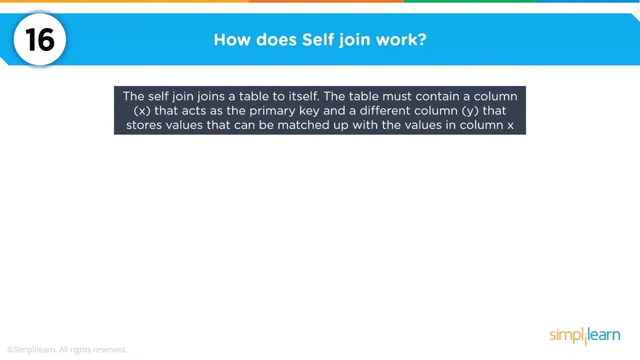 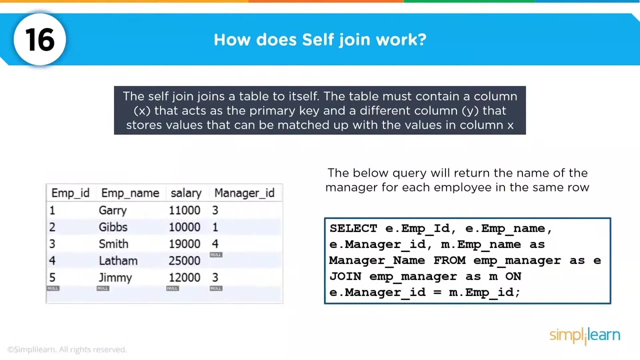 contain a column x that acts as the primary key and a different column- let's see y- that acts out to that stores values that can be matched up with the values in column x. now, this might not be really easy to understand. you'll get to know once we do this demo. so i have a table. 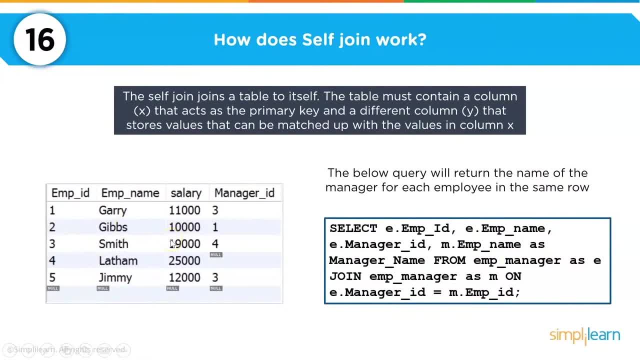 which is called employee manager. so this is my table. now let me tell you how to interpret this table. we have five different employees, starting from employee id 1 to employee id 5. gary, gibbs, smith, latham and jimmy are the different employees we have. 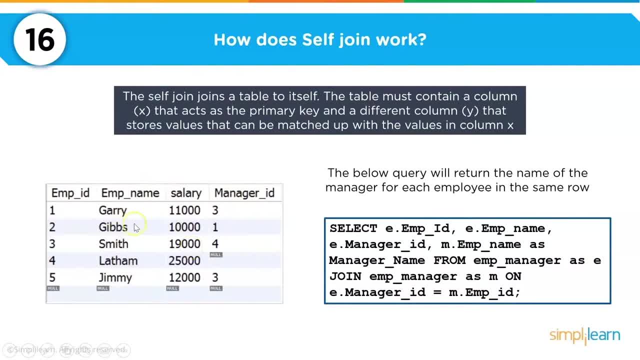 you have their salaries and now you have the employees reporting to which manager. now, if you see here, gary's manager id is three. so if you see a table at three, we have smith. so gary is reporting to three, or in other words, smith has a employee. 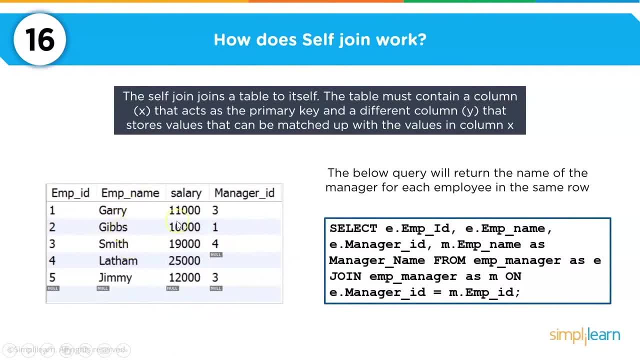 under him, who is gary. similarly, gibbs is reporting to manager id 1 or employee id 1, which is gary. so gibbs manager is gary. similarly, if you see for smith, smith is reporting to the person with manager id 4 or employee id 4. 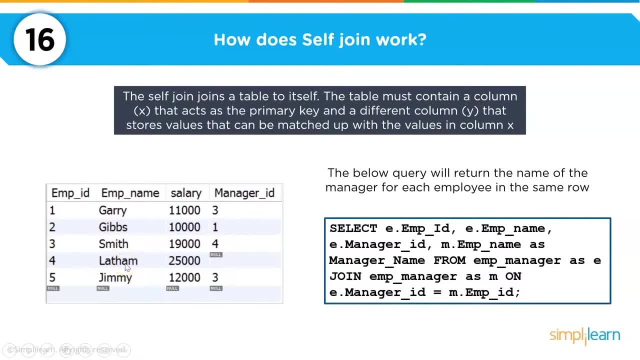 we have latham, so latham has one employee under him who is smith. now latham, in our table, has no managers. then we have jimmy, who is reporting to the employee id 4, who is gary, the employee id 3, who is smith. okay, now i want to use this table. 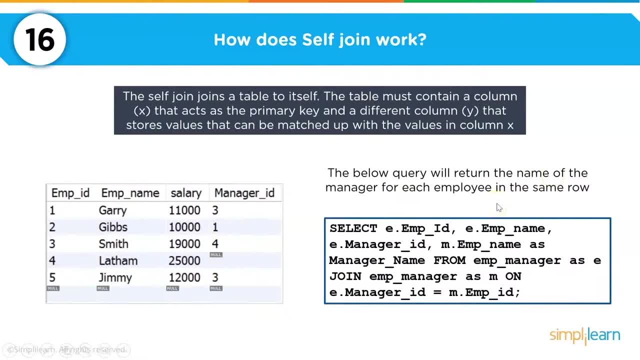 and return the name of the manager for each employee. to do that i am going to use my self join. so here i am using a self join to join both the tables here. both the tables mean i am using the same table twice. so i have written select e dot employee. 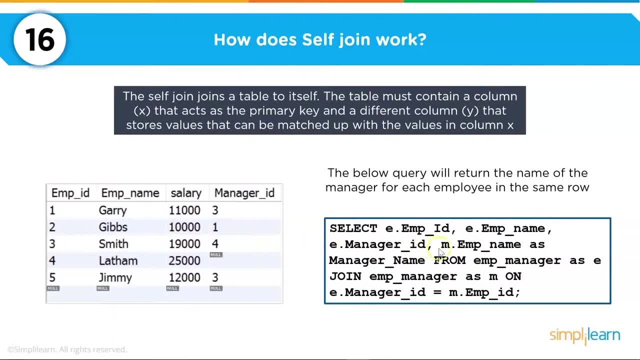 id. e dot employee name, then we have e dot manager id. then i am using another alias for managers, so m dot employee name as manager underscore name from employee underscore manager as e. this join means self join. employee underscore manager as m on e dot manager id equal to e dot employee id. 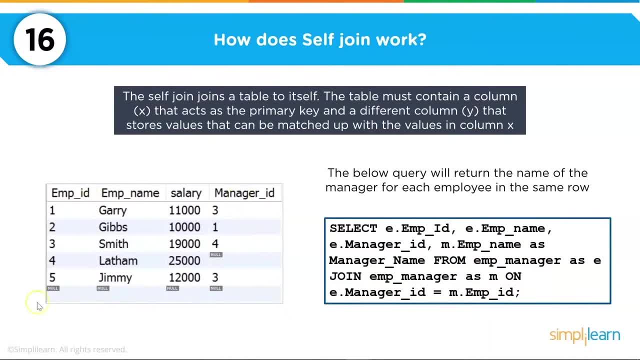 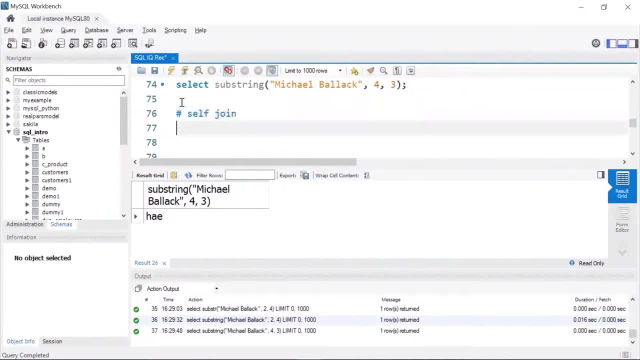 so this is my common column, that is, employee id and manager id. let's do it all right. i'll give a comment here saying self join and i'll start with my self join. i'll write select. let me first display my table. i'll write select star from and my 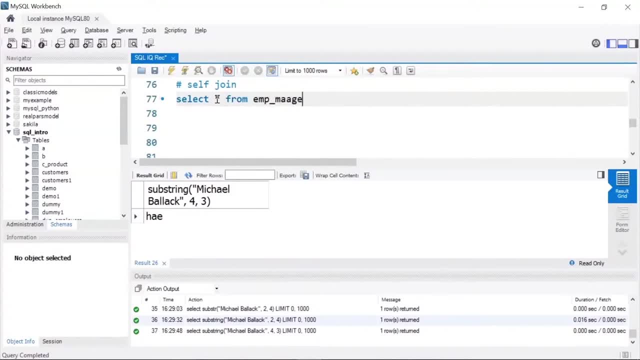 table name is emp underscore manager. i'll run it. you can see the table here. this is the same table that we saw here in the slides. now i'll write my joint query. i'll write select e dot. employee id: comma e dot. employee name: comma e dot. 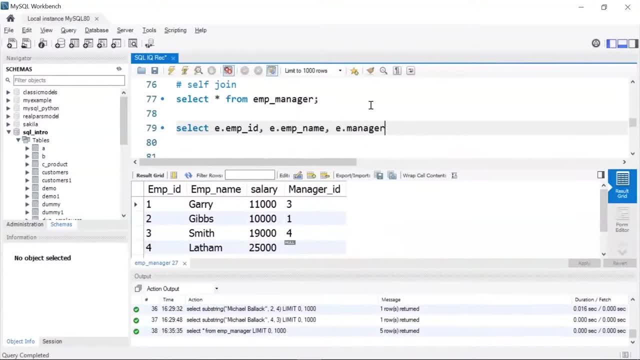 manager id comma. then i'm using another alias as m for finding the manager name. so m dot employee name as manager name. there shouldn't be any space in the alias name. then i'll write from emp underscore manager as e in 201.emp tamblao. 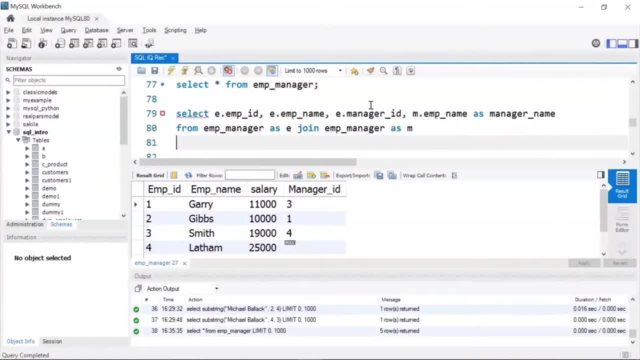 emp. underscore manager as m on ep. underscore manager as e. from emp. underscore manager as e join email p. underscore manager as m on e dot 원래 FOR EMP LAO. EMP Darren Dan, hear my comment from me. c? omf? u manager. underscore id equal to m? dot emp. underscore id. 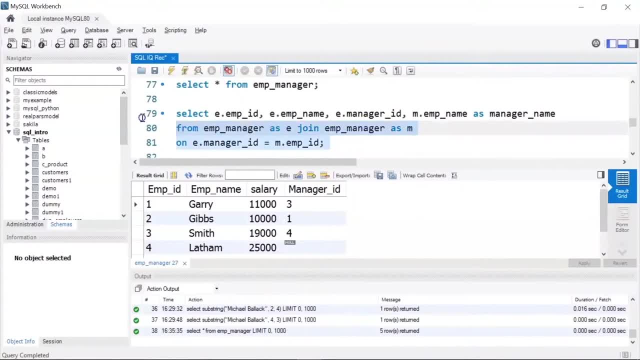 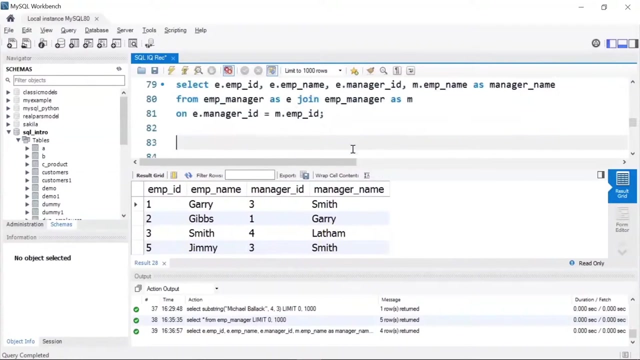 let me run this and we'll see the results. there you go. so gary reports to the manager, id 3. so from the table, 3 is for smith. so gary's manager is smith, gibb's manager is gary, smith's manager is lethem and jimmy's manager is smith. okay, so this is how you can use self-join. 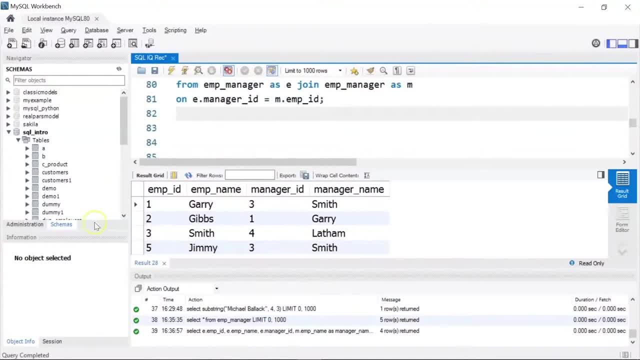 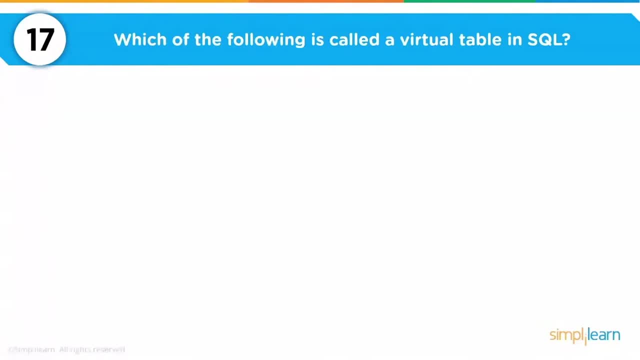 now moving ahead with our next question. so the 17th question is on which of the following is called a virtual table in sql. so again we have a multiple choice question. so the answer is view. you can see here. so view is a virtual table that has rows. 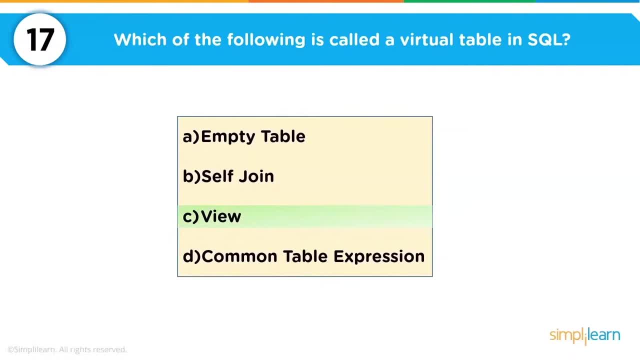 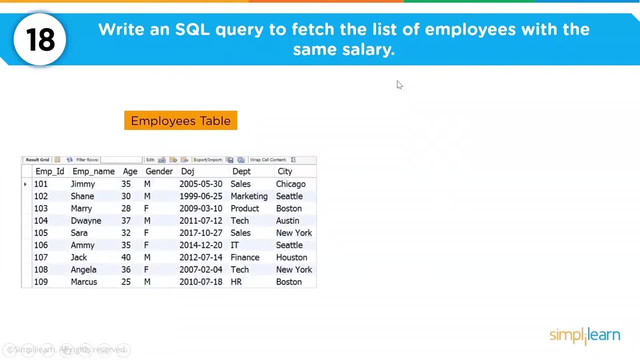 and columns as they are in a real table in the database. now we can create a view by selecting fields from one or more tables present in the database. next, moving to the 18th question. so here we want to write an sql query to fetch the list of employees with the same salary. 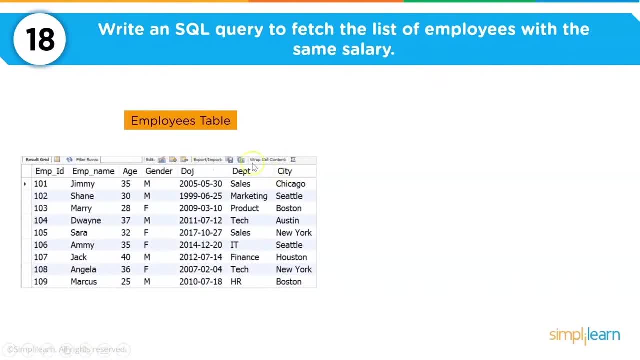 again, i am going to use a self-join here wherein i'll join the same employees table and this is how my query would look like. so i am selecting distinct employee id, so eemployee id, eemployee name, esalary from employees. then i'm joining employees as e on employees e1, where esalary equal to e1.salary, because 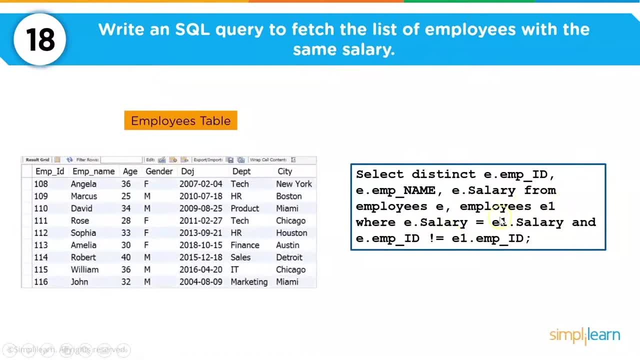 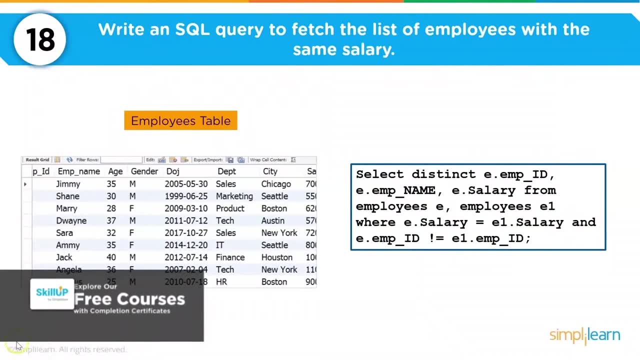 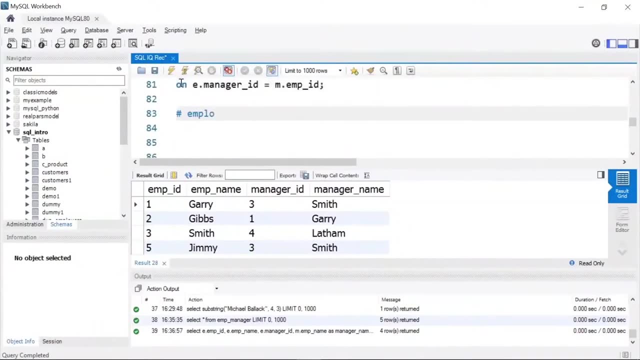 i want to fetch the list of employees with the same salary and i'm ensuring that the employee ids from both the tables are different. let's do it. i'll give a comment here and write: if i have 4 different employees at work- employees with same salary, and i'll start with my query, i'll write select distinct eemployee id. i'll write e downstairs letter. 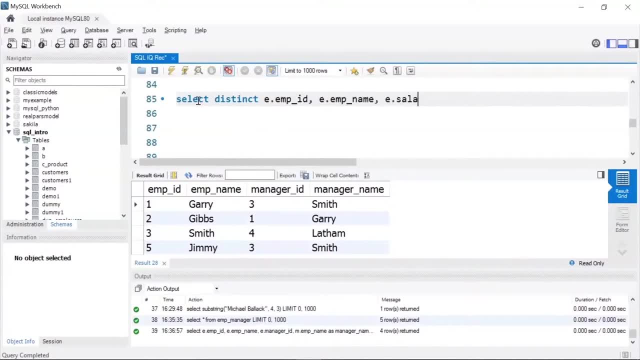 auto login: e. entrepreneur: employee name comma: e dot salary from employees as e, then employees as e1, where e dot salary equal to e1 dot salary and e dot employee ID is not equal to e1 dot employee ID. I'll give a semicolon and let's print the results. you see, here we have Amelia, Bella, Shane and Sarah, who 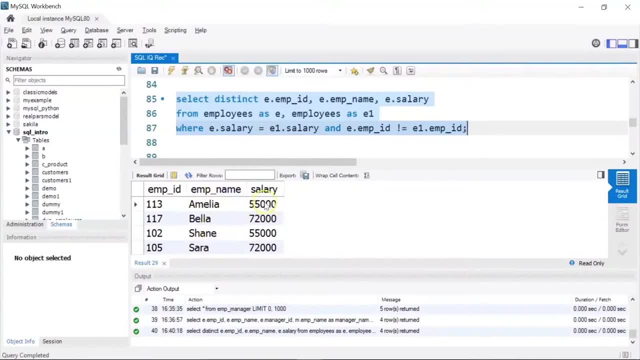 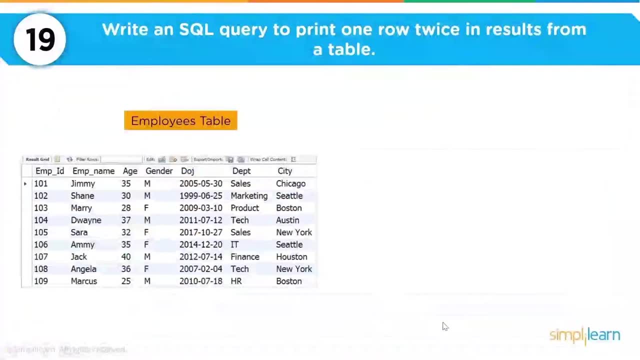 have the same salary. so Amelia and Shane have the same salary of $55,000, Bella and Sarah have the same salary of $72,000. okay, now moving to the 19th question. so the question is to write an SQL query to print one row twice in results from a table. so I have a table here called employees. 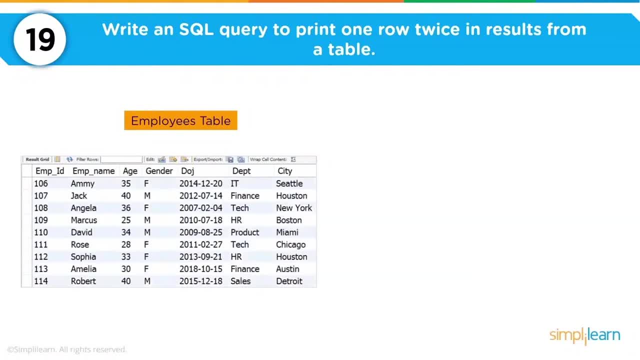 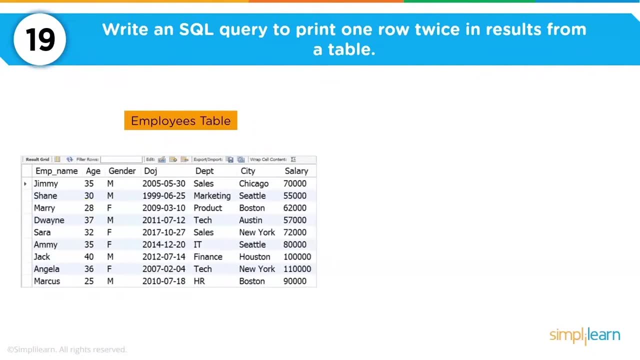 and I want to print one row twice in the results. so to solve such kind of problems you have to print one row twice in the results. so to solve such kind of problems you have to use the union all operator in SQL. so union all combines the result sets of two or more select. 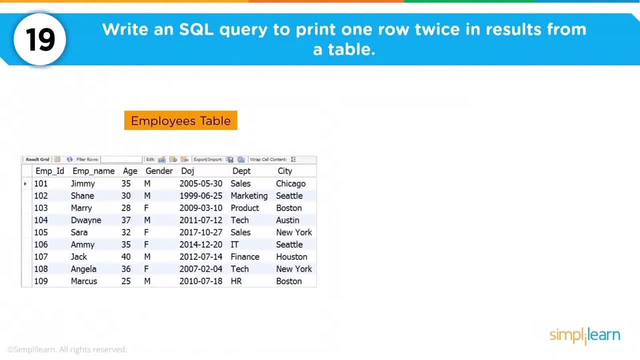 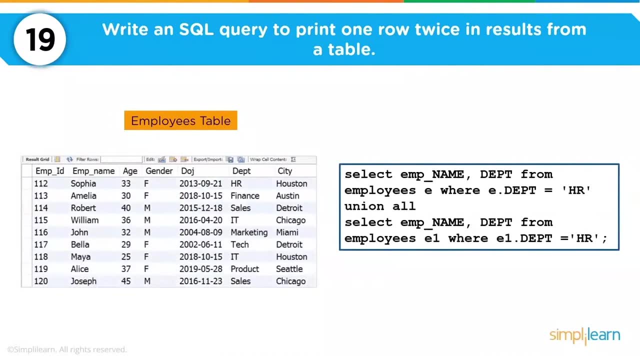 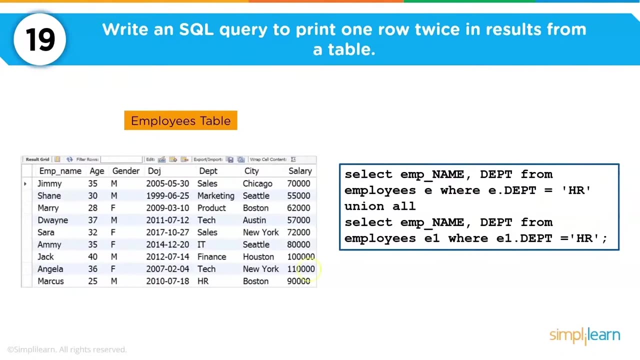 statements. it does not remove duplicate rows between the various select statements. all the rows are returned. so let's say I want to print the employee name and department for those employees who are from the HR department now. to do this we can use the union all operator. you can see it here. so I'm selecting my employee name, the department, from my table. employees as E. 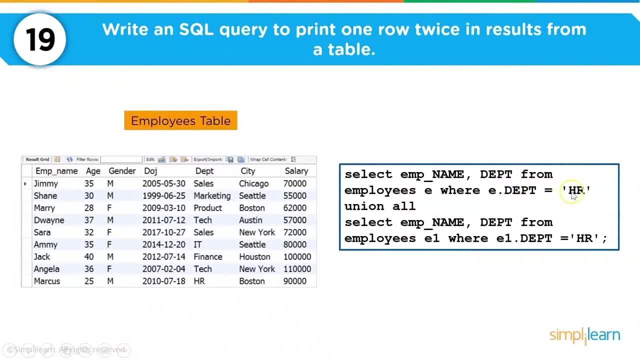 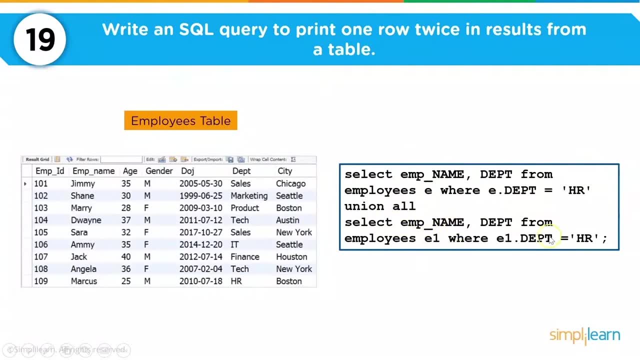 then I'm giving my where clause where E dot department equal to HR, and then I'm using the union all operator. then I'm again selecting my employee name department from employees with another alias as E1, where E1 dot department equal to HR. so let's do this. 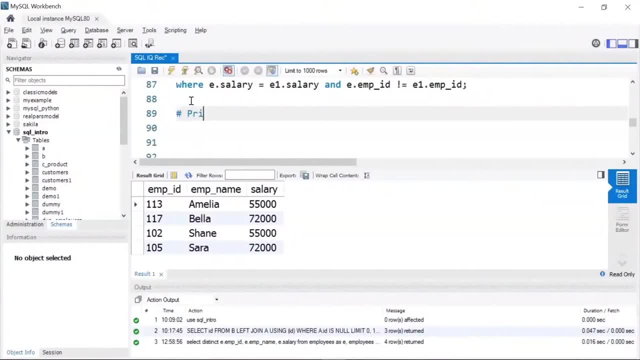 okay, comment as print row twice. okay, now I will start with my query. I'll write: select my employee name comma the department from my table that is employees as e. then I'll use where e dot department equal to HR. then I am going to use the union all operator, so the union all will combine the result. 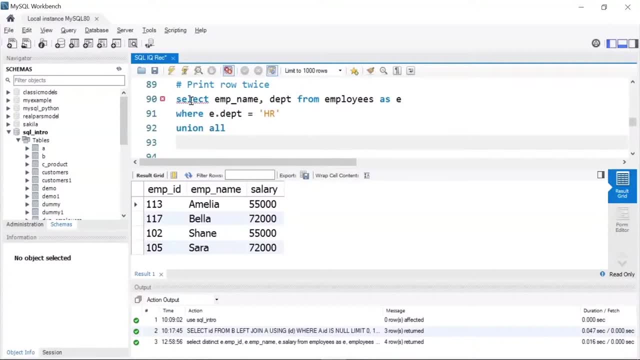 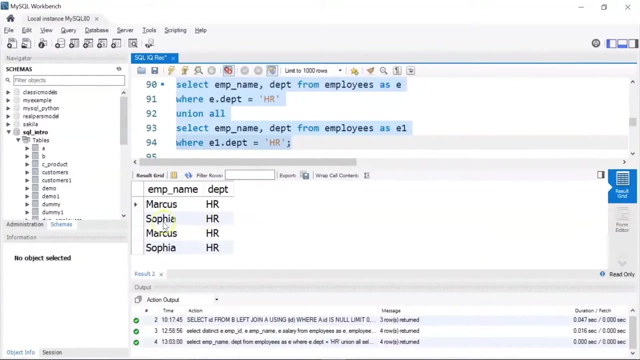 set of two or more select statements. then I am going to write select EMP underscore name comma: my department from employees as e1, where even dot department equal to HR. I will give a semicolon now. let's run it. there you go. you can see here Marcus and Sofia are from the HR department. 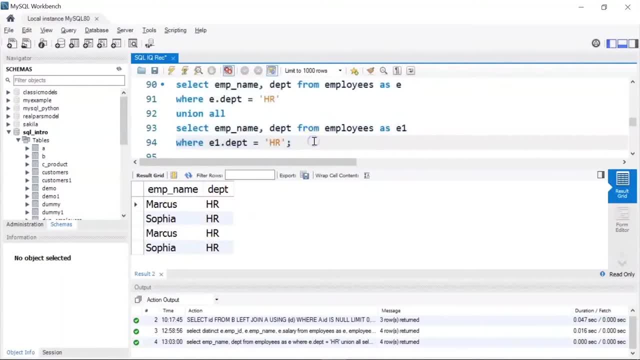 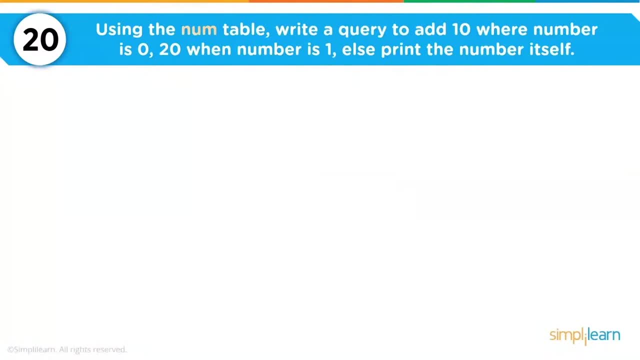 I will give a semicolon now. let's run it. there you go. you can see here Marcus and Sophia are from the HR department and we have printed them twice in our results. coming to the next question, the question is, using the num table, write a query to add 10 where number is 0, 20 when number is 1. 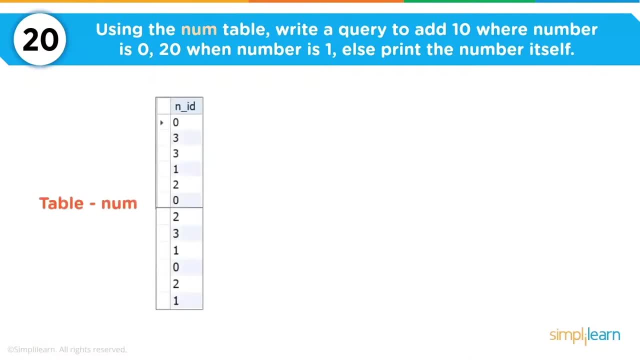 else print the number itself. so you can see, here i have my table called num and it has just one column which is num id or number id. we have some numbers here, and from these numbers i want to add 10 if the number is 0, 20 if the number is 1, else i would print the number itself. so 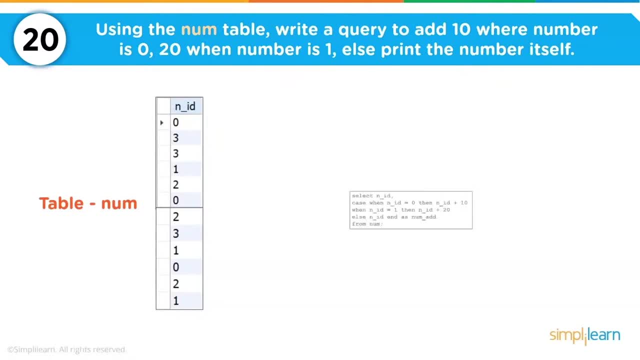 to answer this question. we'll use the case statement in sql. so the case statement is sql's way of handling. if, then logic the case statement is followed by at least one pair of when and then statements. so here you can see. i have my case statement. i'm writing when case my column name n, underscore id equal to 0, then add plus 10. 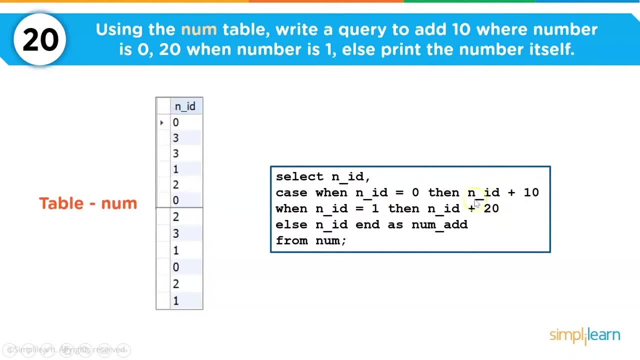 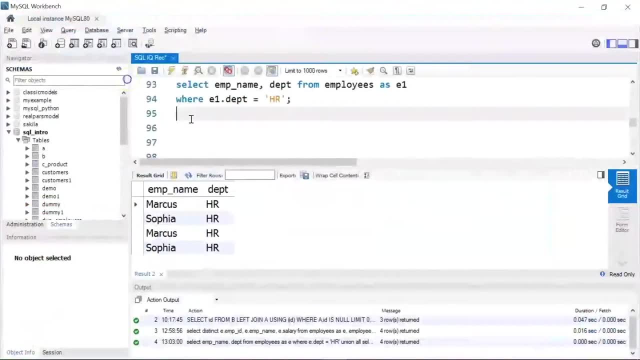 if it is 1, then add plus 20, else we'll just return the number id. now let's do this. okay, i'll give a comment saying using case statements. okay, first of all, let me display the values present in my num table. you can see here this: 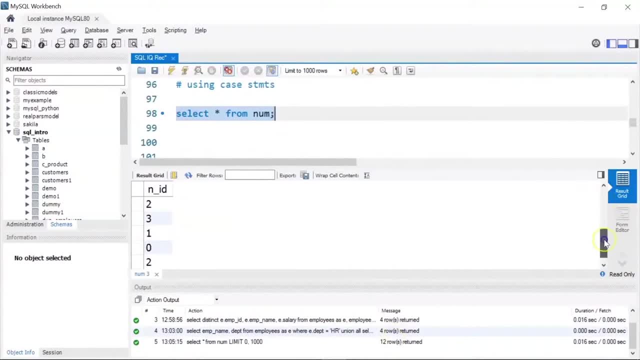 is my table, and there are total 12 rows of numbers. now let's start with our query. i'll write select n underscore id comma. then i'm going to write n underscore id comma. then i'm going to write n underscore id comma. i'm going to write my case statement, so i'll use the keyword as case when n underscore. 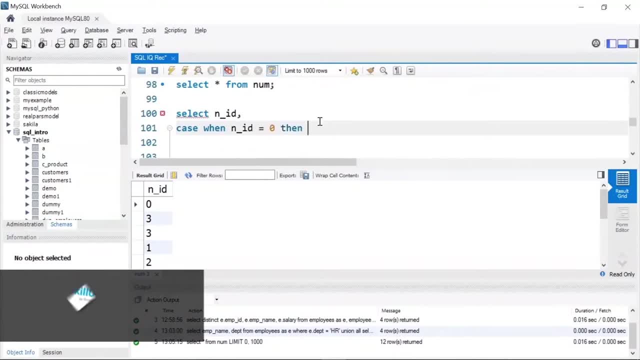 id equal to 0, i'll use then n underscore id plus 10. i'll write: when n underscore id equal to 1, then n underscore id plus 20, else I'll just print an ID. now I'll end my key statement. I'll write: end as an. 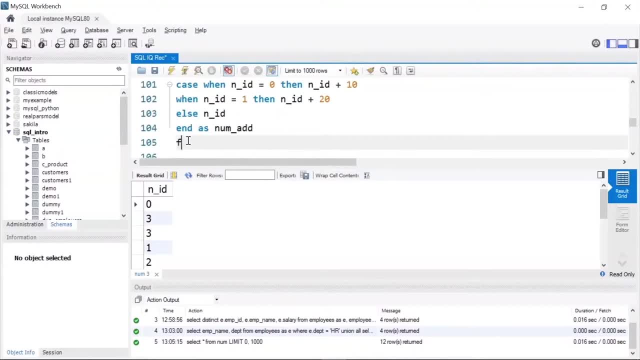 alias name, let's say num. underscore: add from my table that is num. let's run and see the results. okay, you can see here. my first number was zero. so since it was zero, we have added num ID or N ID plus 10, so the result is 10. now, wherever the 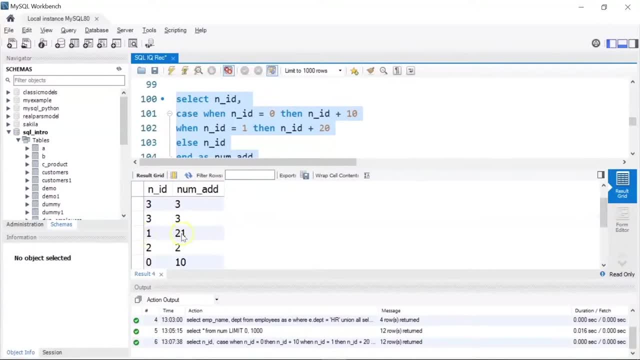 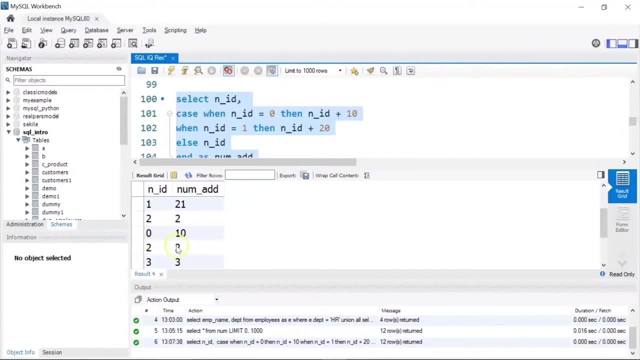 similarly, here the value was 0, so we have added 10, the output is 10, and you see here again, here we had another one, so we added 1 to 20, so the result becomes 21, and for the rest of the numbers, for example 3, we had 2 the values. 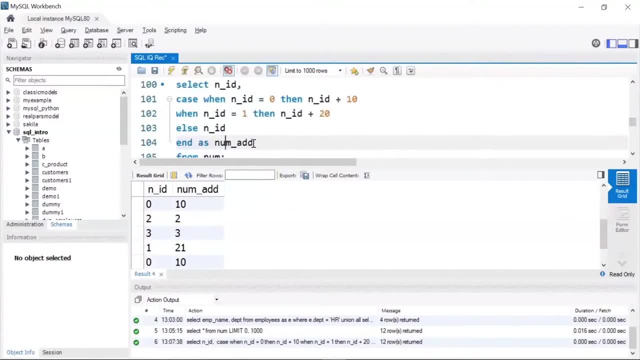 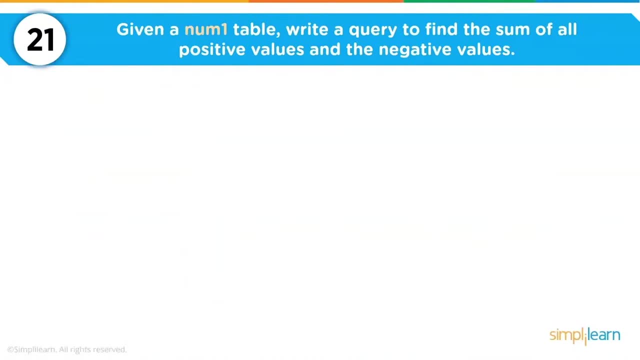 are the same. okay, now moving ahead. so we have a table called number 1 and using this table, we want to write a query to find the sum of all positive values and the negative values. so let's see the table first. so this is my table, which is num 1. you can see, here we have a 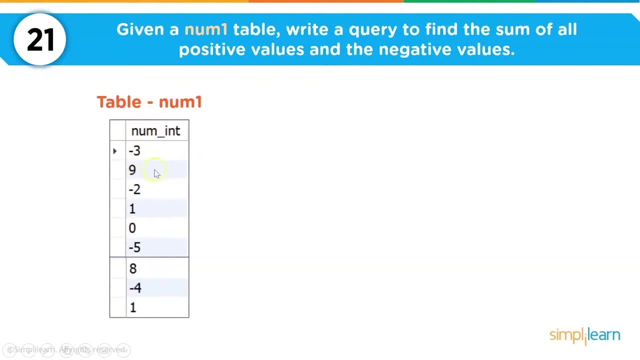 list of integers and there are positive as well as negative integers. so for positive values as well as negative values, then we need to write a query which is a and the negative values. we want to find the sum separately. so again, for this we are using the case statement. you can see, here I have used two case statements. I'm 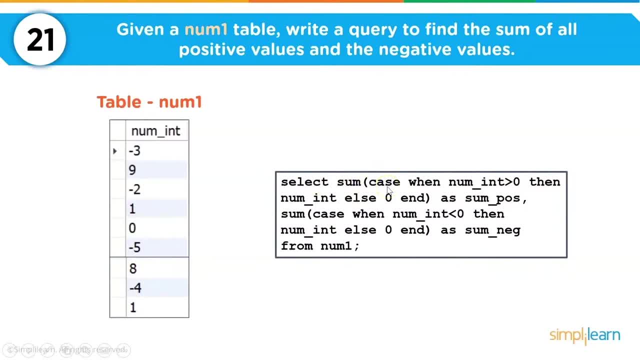 writing. select and then I'm using the case to find if the number is greater than zero, which means it's a positive number. so I'm finding out the sum and then I'm checking case when the integer is less than zero, so it's a negative number, and I'm finding the sum for the negative numbers as well. let's do this. 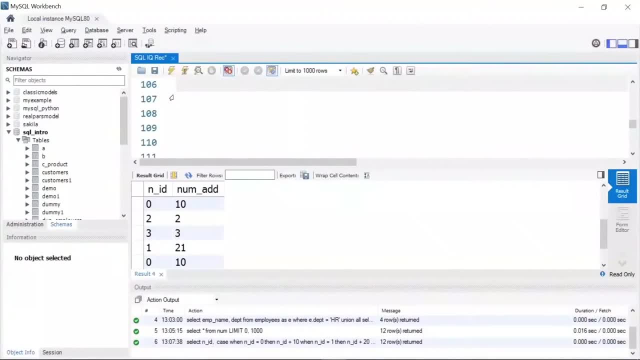 okay, so I'll give my comment as: add positive and negative numbers. okay, so let's start with our select query. I'll write select, I'll use the sum function and inside the sum function, I'll use my case statement. so I'll write case when num underscore integer. okay, before that. 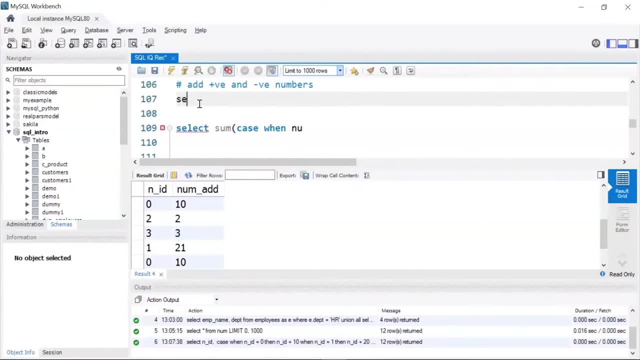 let me just print the values present in my table. so I'll write select star from my table name. that is num1. okay, so you can see here these are the values or the list of integers that we have. there are some positive as well as negative numbers. okay, let's continue with our query. so here I'm going to write case. 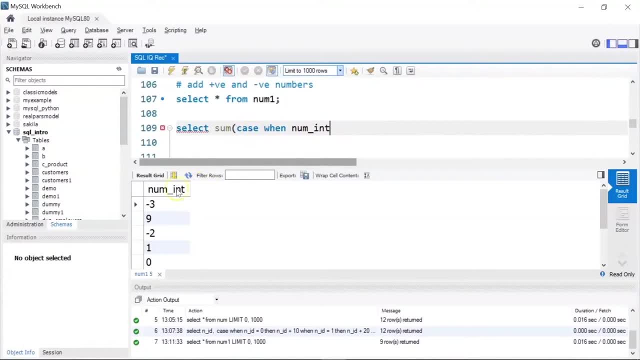 when num underscore integer or int, which is my column name. if it is greater than zero, then I'll return num underscore int, else I'll see 0 and end my case statement. I'll give an alias as sum of, let's say, plus zeros, and now I have three letters, so I choose 3 and all my numbers do not look anyOOLE and let's move on here. I need two somewhere. really I need to use the truly number, which means it's Pun and info here. so we need to use the C present and I need to get 2 numbers and let's try mentioning all. okay, so let's cut. this is a participle. 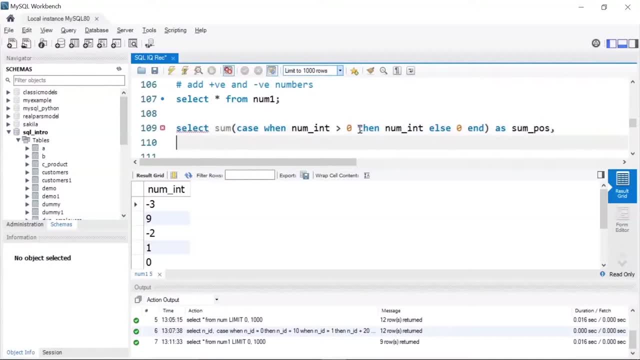 positive numbers, I'll give a comma, then I'll use another sum function and inside the sum function we'll use the case statement to find the sum of negative numbers or integers. so I'll write num underscore int. if it is less than zero, then num underscore int, else zero and I'll end. 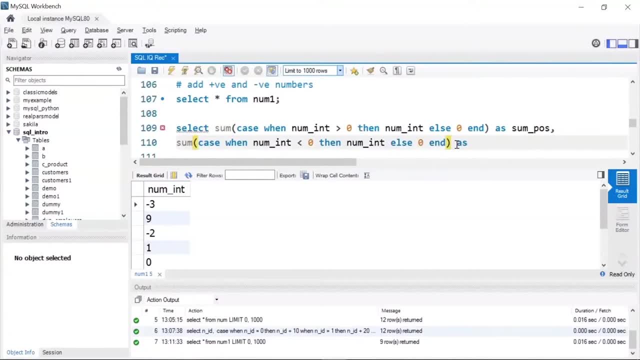 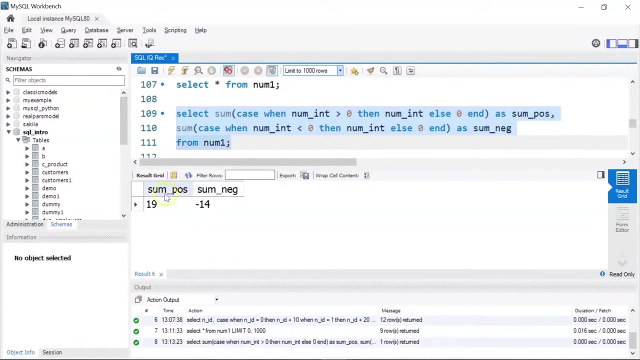 here, okay, and I'll give another alias name, as, let's say, sum, underscore neg, which stands for negative, pos is for positive integers, and then I'll write from my table: that is num1. let's run it okay. there you go, we have our results. so we have two columns: sum of positive. 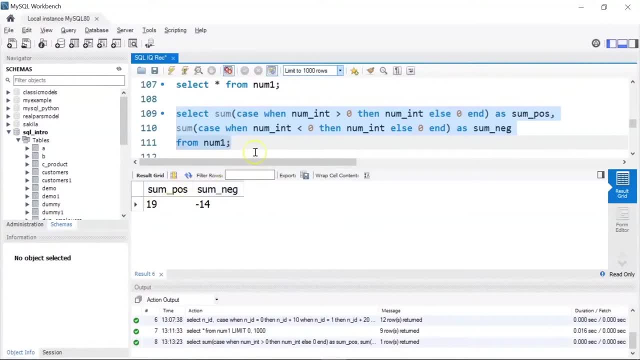 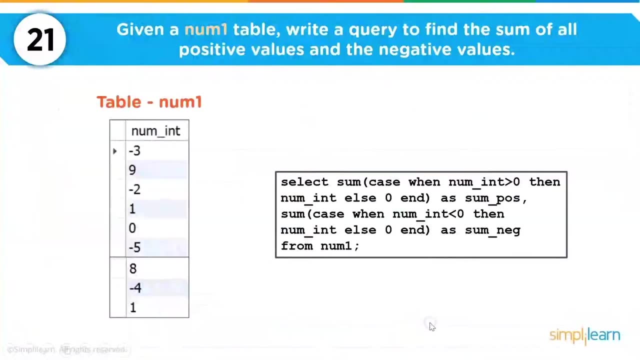 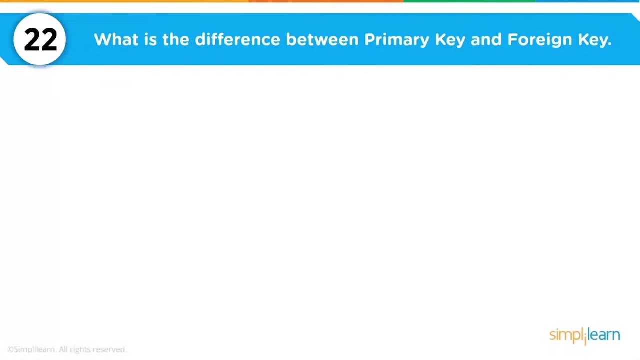 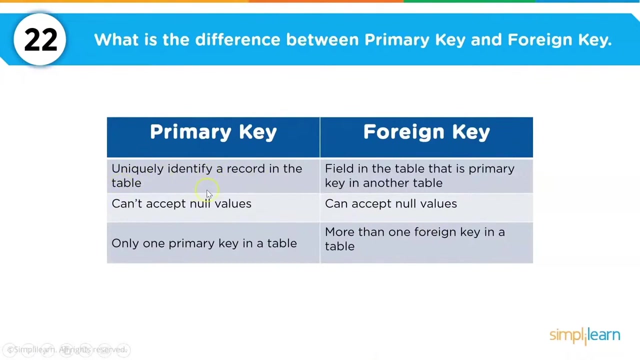 integers and sum of negative integers. you can see the results: 19 and minus 14 respectively. okay, now moving ahead. now, in question number 22, we want to list a difference between primary key and foreign key. so, as you can see here, primary key is something that can uniquely identify a record in a table. so if you consider a school database, a primary 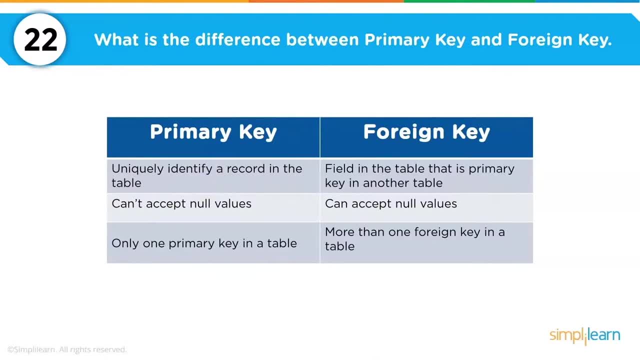 key would ideally be the rule number or the registration number of the school student, because that is unique to all the students in a school. now, foreign key is the field in the table that is primary key to another table. so suppose you have another table called courses, to which the students have enrolled to now. 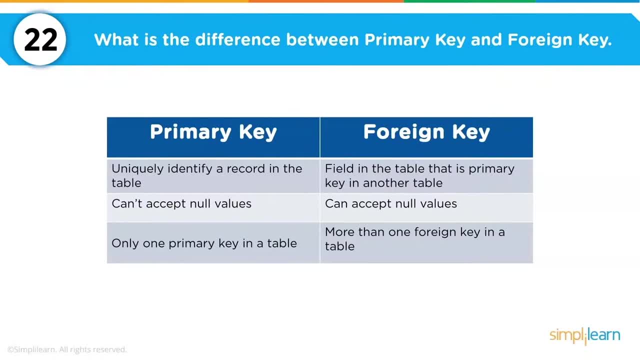 if you have a roll number or a registration number column in the course table, that becomes the foreign key. now the other difference is: primary key don't accept or cannot accept null values, while foreign key can accept null values. you can have only one primary key in a table, but you can have more than. 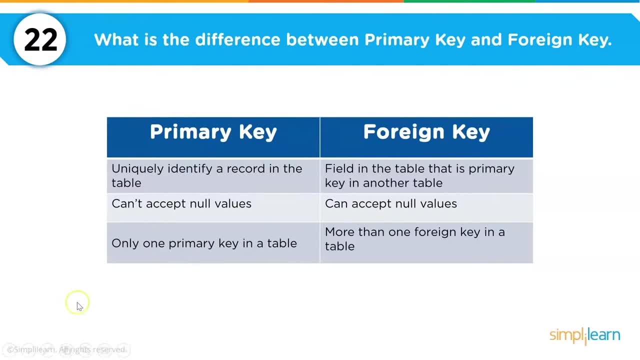 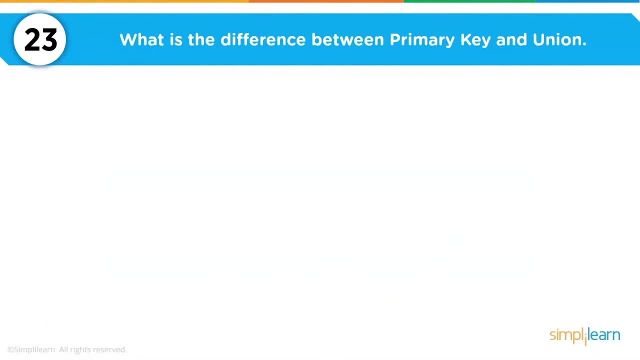 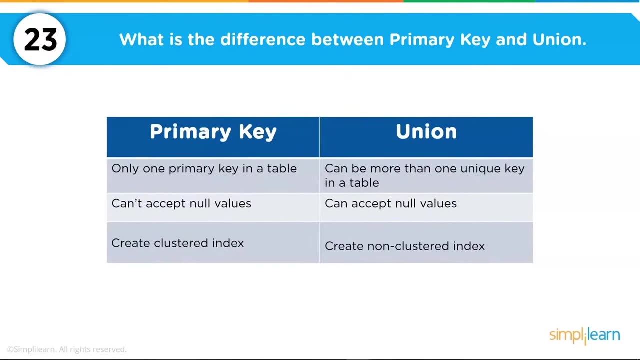 one foreign key in a table. now, coming to the 23rd question: what is the difference between primary key and foreign key and union? so you can have only one primary key in a table, as we discussed in the previous question, but you can have more than one unique key in a table a. 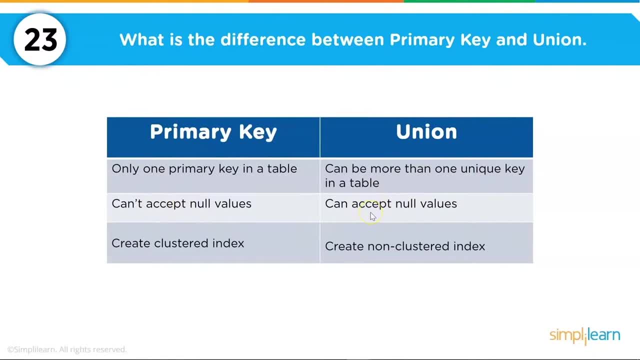 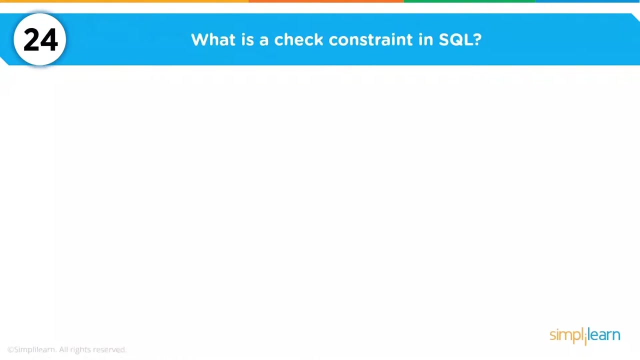 primary key column cannot have null values, but union can accept null values. now, if you assign a column as a primary key, you create a clustered index, and similarly, if you assign a column with union, you create non clustered index. ok, now coming to the 24th question: what is a check constant in SQL? so check. 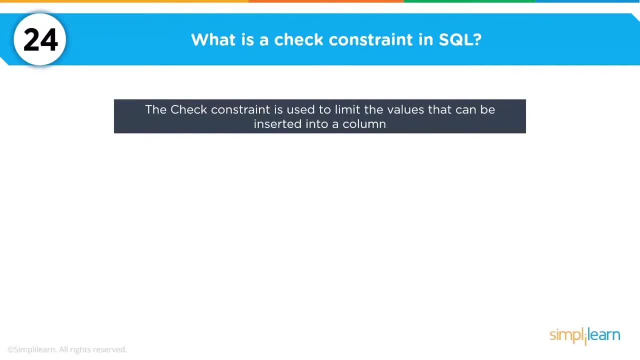 constraints are used while creating tables. check constraint helps to limit or restrict the values that can be inserted into a column. for example, we have a table here, let's say dummy one, and you want to ensure that every time you insert the age of people, of persons, and the table want to. 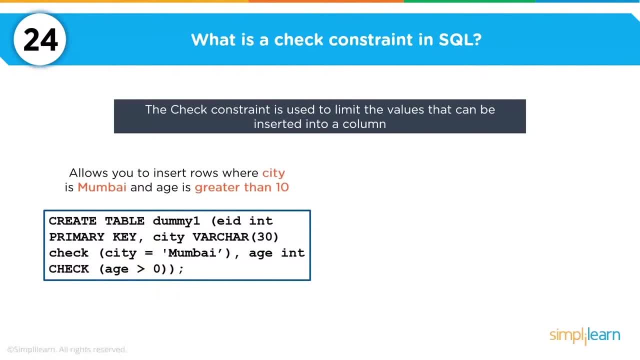 make sure that each should be always greater than zero. reason being: a person cannot have, or an animal cannot have, or a tree can have a negative wage. similarly, you can set a constant for the salary column in a table to ensure that it is always greater than 0, because you cannot earn a negative salary or it. 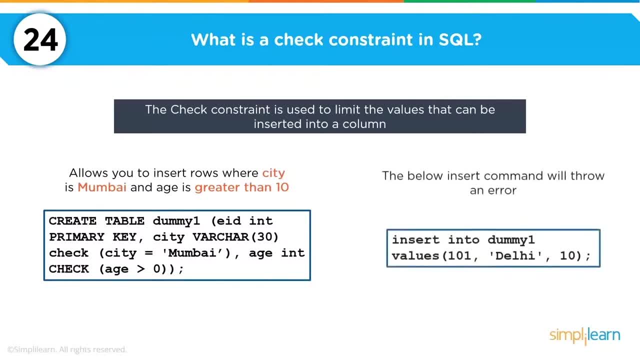 cannot be less than 0. now we are going to follow the this table over here and mark theBER and 84, 13 plus estado behavior, and then click the purchase button. foriß twitter: 20, number 12. we are going to take the purchase and opportunity item. 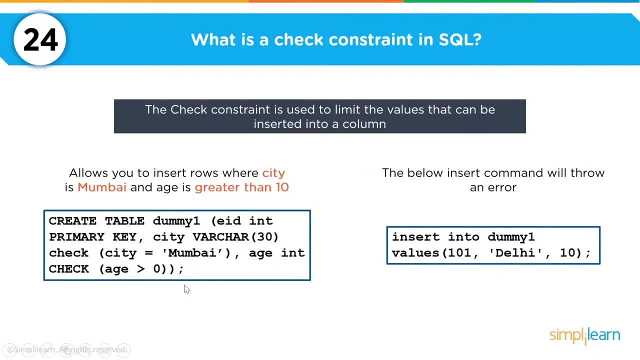 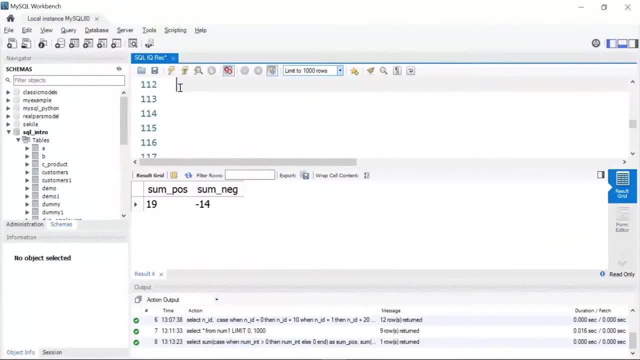 create a dummy table on my mysql workbench and see how check constraints can be applied. okay, so let's give our comment as check constraints. all right, so I'm going to create a table called dummy, let's say underscore SQL. now this table will have a few columns. first we have, let's say, a ID which stands for: 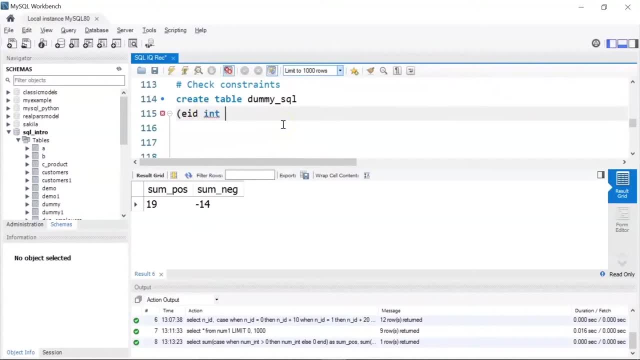 employee ID. the data type is integer and I'm going to assign employee ID as my primary key, so I'll write primary key here. okay, I'll give a comma. next we'll have a city column. city column is of type var, char or varying character. I'll give the size as 30 and 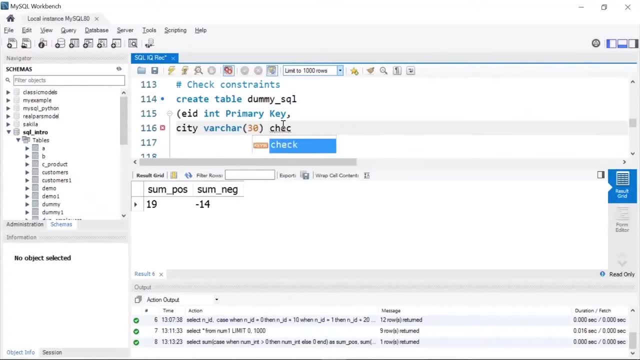 here I am going to apply my check constraint to this city column. I'm going to check the city should t only values as Mumbai, let's say. I'll have my final column, that is age. age is of type integer. and here I am going to check my age should always be greater. 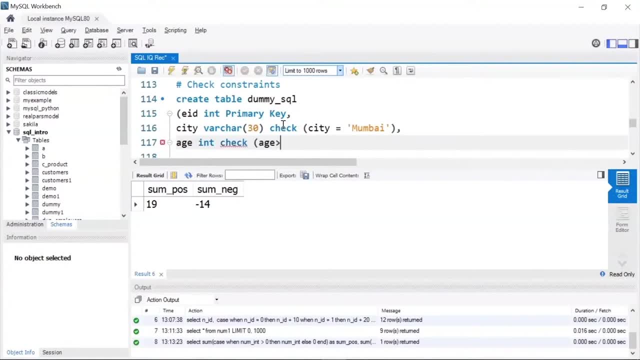 than 0, so I'll write check: age: greater than 0. okay, so our dummy SQL table has one primary key constraint and we have applied two check constraints on city and each column. let's run this. okay, so we have created our table successfully. you can see it here. now let's insert a few records and we can see the difference. 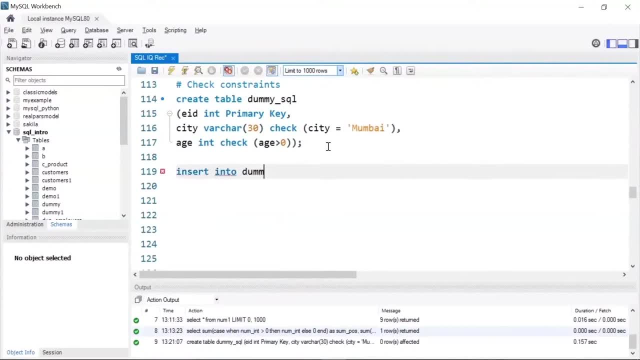 I'll write insert into dummy underscore SQL, I'll write values and then I'm going to. I will have my employee ID as 101, I am giving my city as Mumbai, which is what we want, and let's say, I will give my age as 10. now, this should perfectly work because my city is Mumbai. 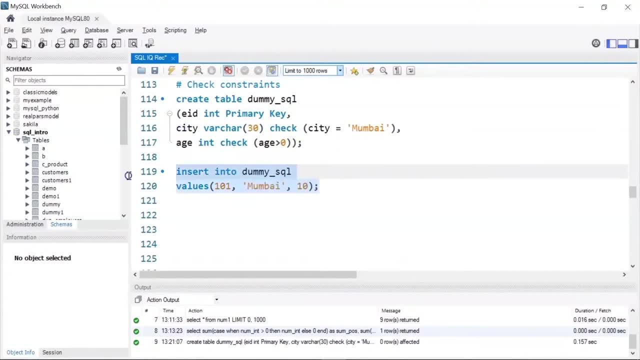 and my age is greater than 0, so I should be able to insert this record successfully. you can see here. I have inserted this record to the table. I'll write select star from dummy SQL so that you can check. let's run it. oh, there is some mistake. I should write from: okay, let's run it. you can see. 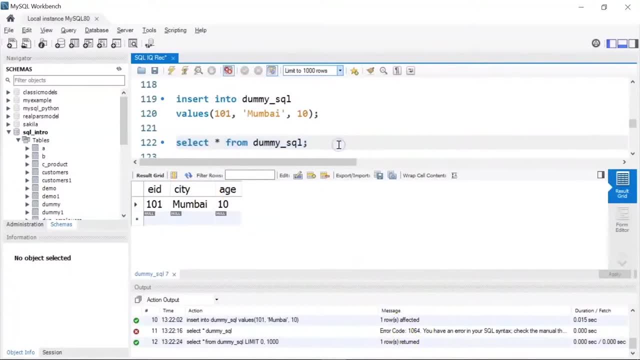 it here. we have one record, or one row, returned. now let's see, we'll insert another record, and this time I am going to give my employee ID as 102, because it has to be unique, and this time, instead of Mumbai, I am going to give my city, as, let's say, Delhi. so I am NOT following my check constant. 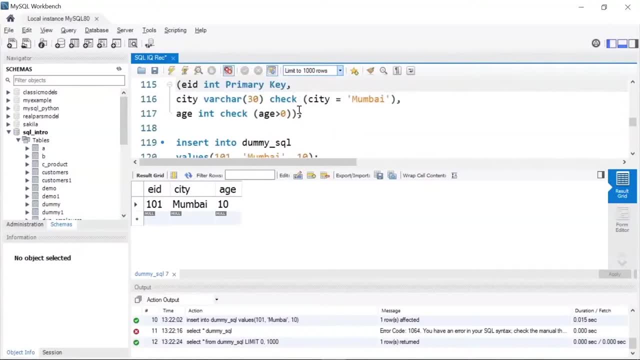 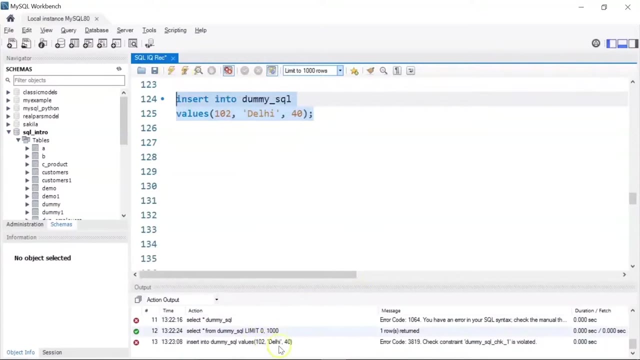 where I am supposed to give only Mumbai, I am but giving Delhi. here to see the difference: if I run this, let's say we'll have ages 40 which is greater than 0. let's run it. you see, here we get an error saying check constraint dummy underscore SQL underscore check is violated. similarly. 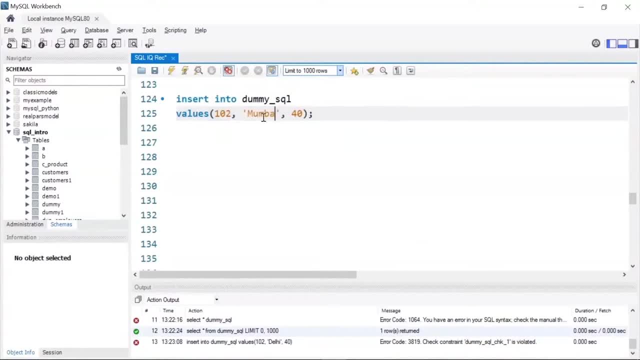 let's say I change this to Mumbai again, and instead of 40, let's say I'll give us minus 30, so your each can never be in negative numbers. if I run this, I get the same error. my check constraint has been violated because each should be greater. 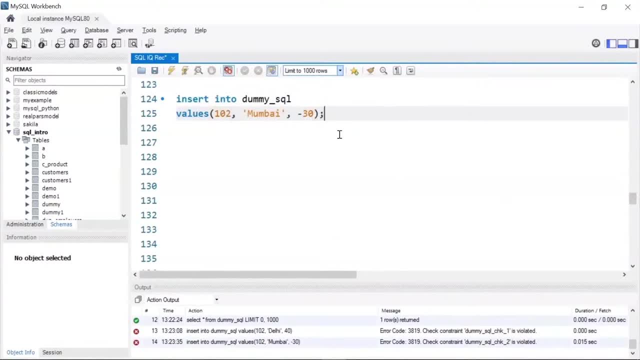 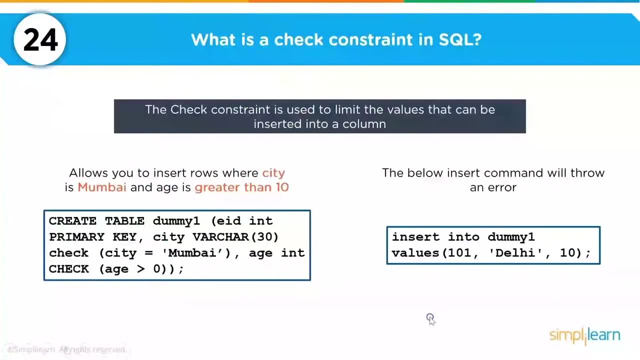 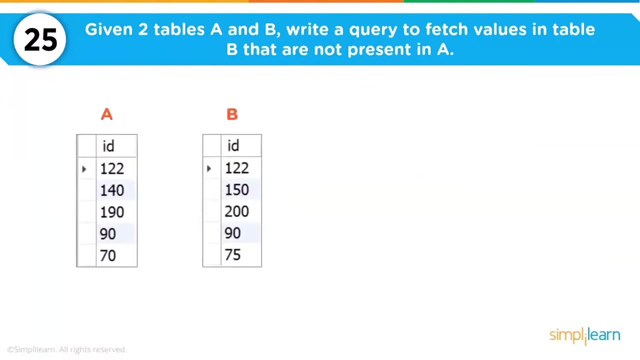 than 0. okay, so this is how you can use check constraints in SQL. now coming to the 25th question. so, given two tables, A and B, you want to write a query to fetch values in table B that are not present in table A. now, to answer this question, you can use the left join. so 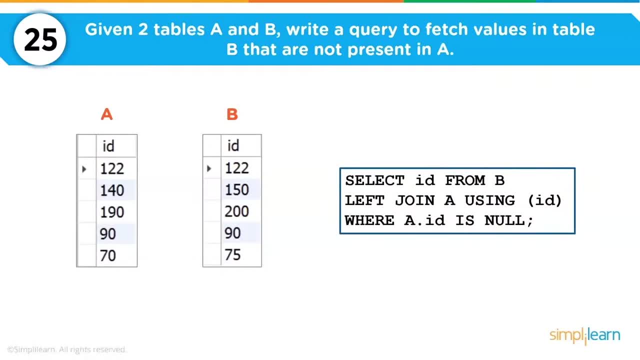 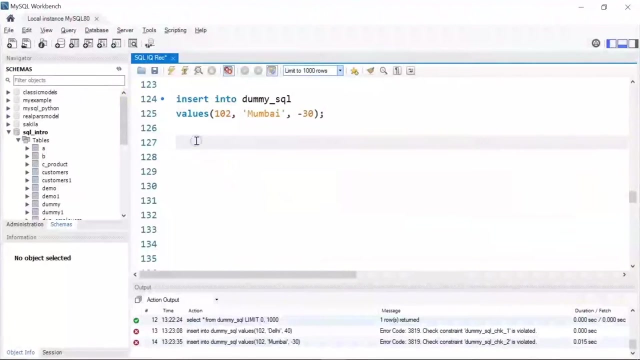 what left join does is it returns all the rows from the left table and only matching rows from the right table, and I have used my condition as 80, and a dot ID which is in the right table should be null. let's write this query on the workbench. okay, so I'll give my comment using left join. first of all, let 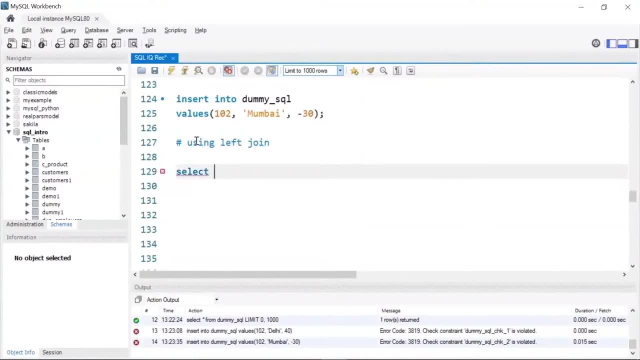 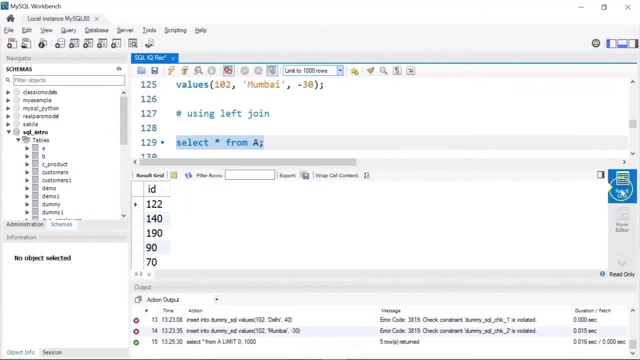 me display my tables. I'll write select star from a, where on this I have the ID's. there are total five IDs in table a. similarly, I'll copy this and we'll see the values that are present in table B. so again, I have five values. there are a. 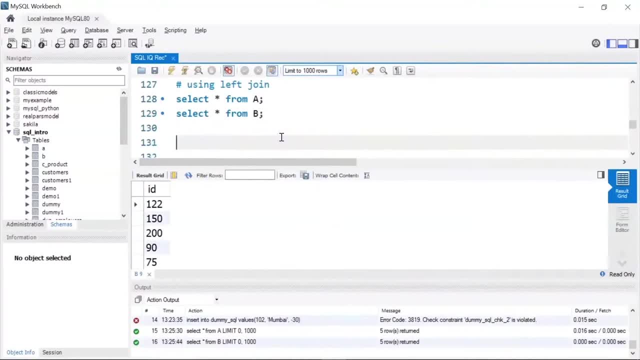 few non matching values as well. so I want to return those non matching values that are not present in table a. so for that I'll write select ID from table B and I'll use left join a using my ID column. this is another way to give the 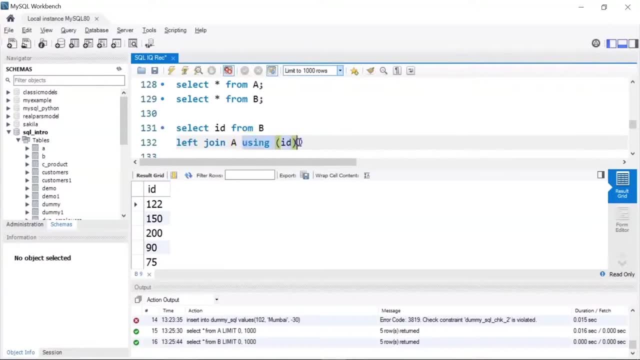 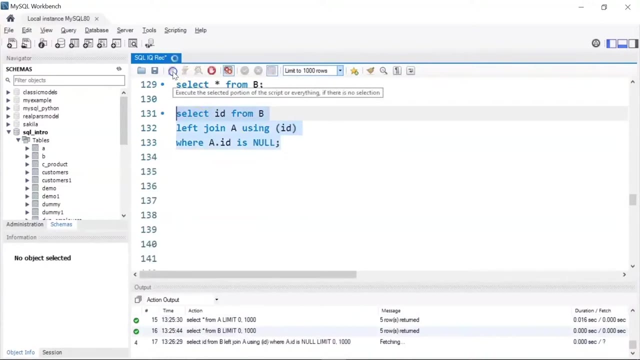 condition, or you can use the on operator, then I'll give where a dot ID is null. let's run and see the results. there you go, so 150,, then this is the result. so 15,, then 15,, then 15. so again I'll write this: 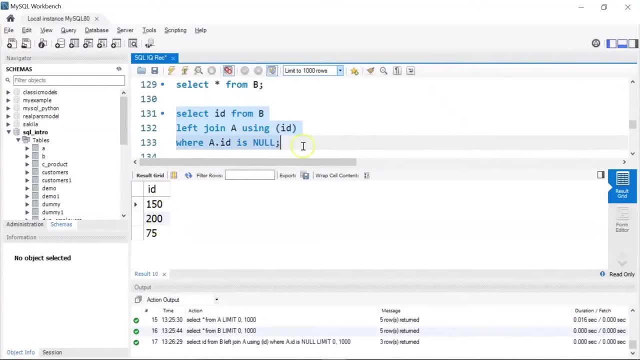 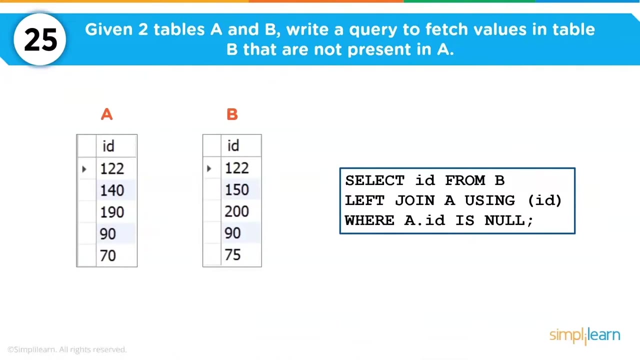 50 275 are not present in table a but are present in table b. okay, now moving ahead. so now we'll look at the last set of five questions. so these questions are based on the popular north wind sample database provided by microsoft. there are several tables in this. 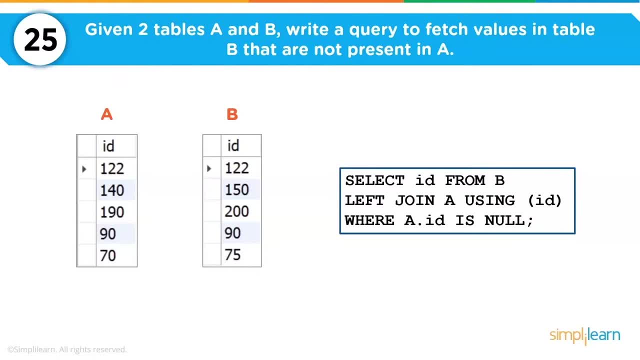 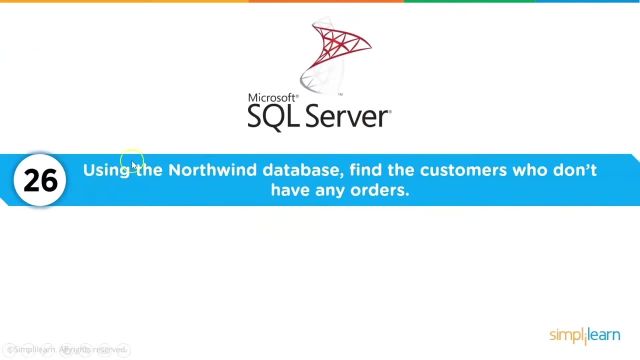 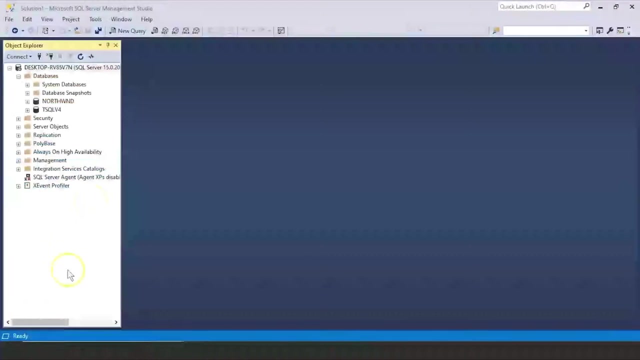 database. so we have an order table, customers, employee products, region table and others. we'll use our microsoft sql server to solve the five questions. so my next question, which is based on microsoft sql server, the question is: using the northwind database, find the customers who don't have any orders. okay, so i am on my microsoft sql server. 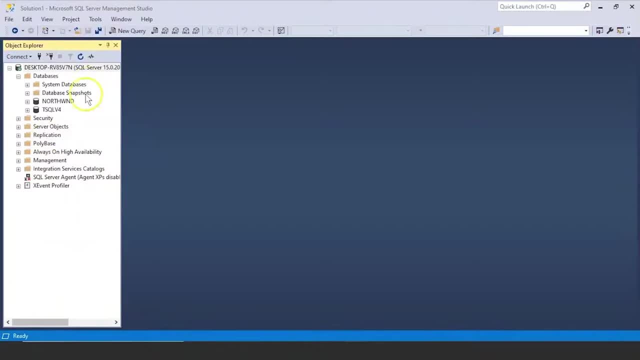 management studio. so this is how the interface works, looks like, and here you can see i have a list of databases. now to solve the last five questions, i am going to use the northwind database. if i expand this, i'll click on the plus sign. you can. 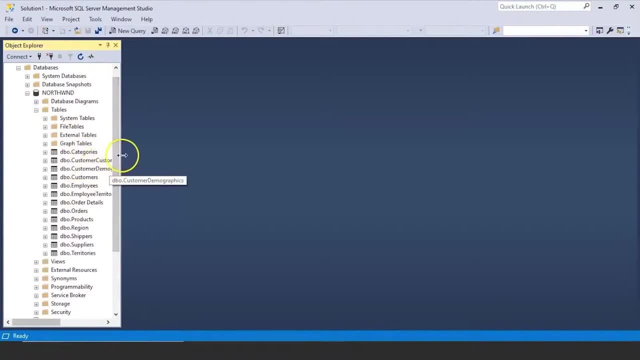 see, there are a lot of tables that are already present in the database. you can see, here we have customers, employees, employee territories, order details, orders, products, region, shippers, suppliers, territories and more. okay, so, aproximadamente now, let me just collapse this. all right, so to write my queries, i'm going to 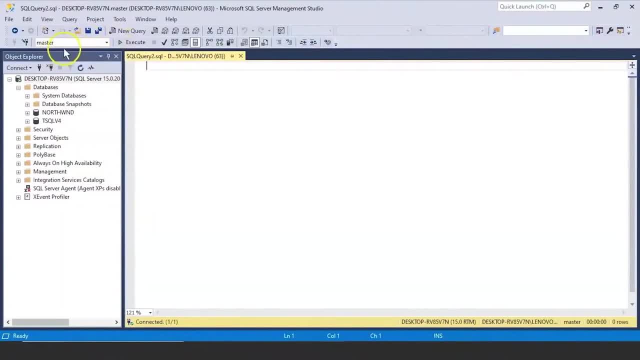 create a new query file. and here you see, i am currently on my master database. i'm going to change this to northwind database so that we can utilize all the tables that are present. so my 26th question was to find the customers who don't have any orders. 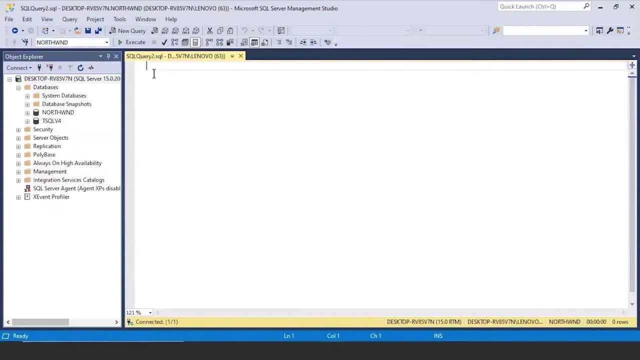 that I'm going to use two tables- customers and orders. so let me first give a comment saying customers with no orders. and now let's go ahead and display the columns that we have and see the records present in the tables: customers and orders. so first time, checking all the columns and the rows. 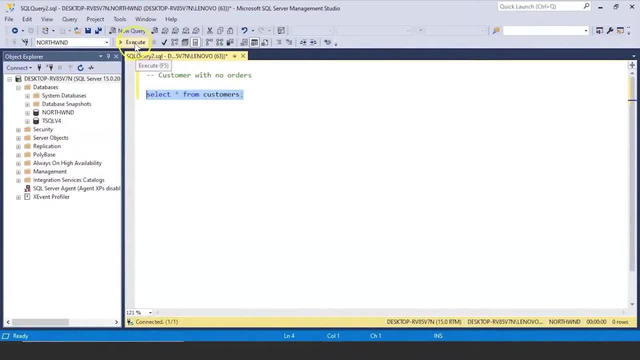 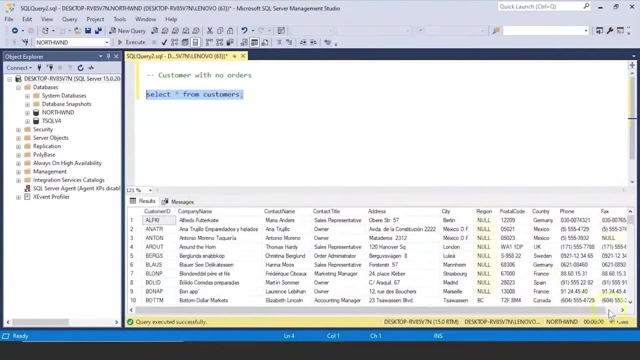 present in the customers table. I'll execute using this button or you can hit f5 as well. okay, you can see here there are total 91 customers. these are all unique customers. you have total 91 unique customer IDs. you see here the company name of the customer. you have the contact name, the contact. 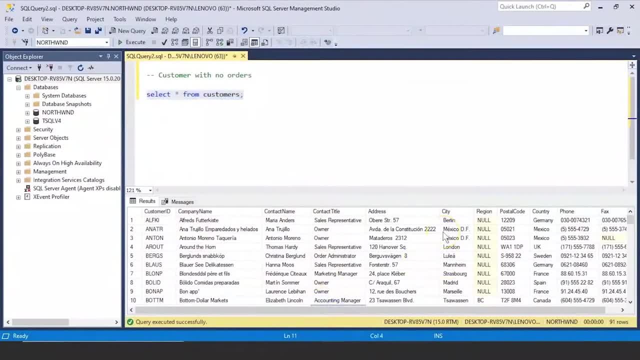 title, address, city to which the customers belong to, then the region, postal code, country, phone, fax number. okay, now let me just copy this query, and now we'll check for the orders table. I'll write select star from orders and let's execute it or run it. okay, so there are total eight hundred and 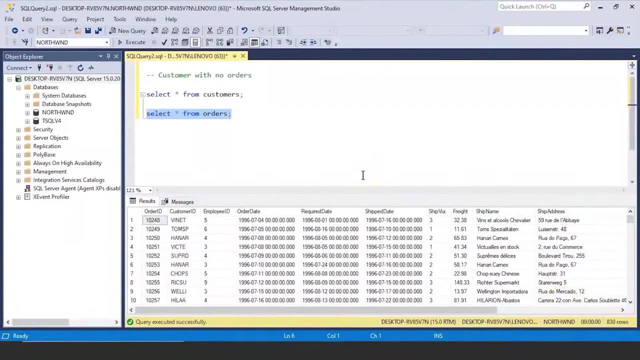 three hundred customers and we have total one hundred and three hundred customers and we have total one hundred and three hundred customers and we have 30 rows of information. so there were total 830 orders or order IDs. you have the customer ID now. this customer ID is actually the foreign key for the orders. 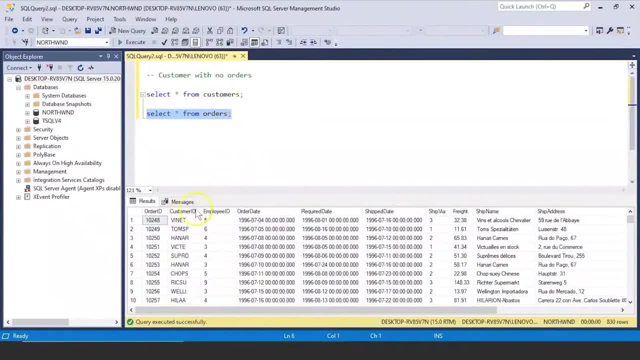 table, but for the customers table, customer ID is the primary key and in the orders table, order ID is the primary key. you also have the employee ID. again, this employee ID is the foreign key for this orders table. you have the order date and we have the required date. ship date, ship via which means by which medium the 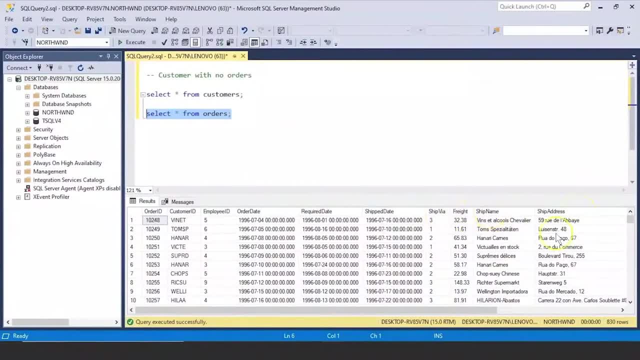 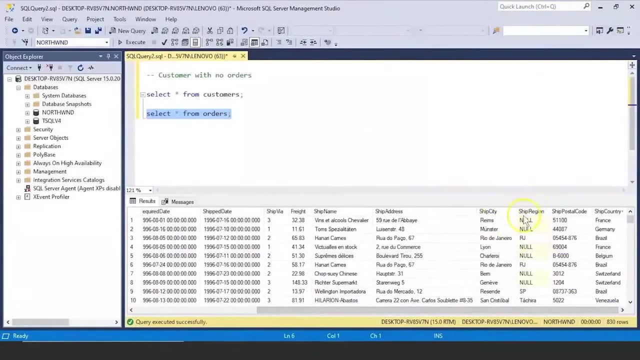 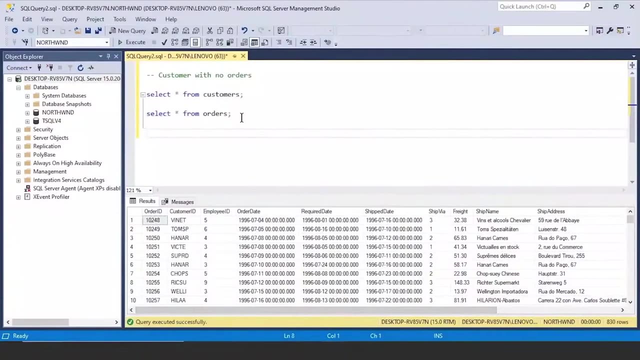 order was shipped. we have the freight charges, ship name and ship address as well. then you have the city from which the item was shipped, the region, postal code and the country. okay, now let me use the distinct keyword. I'll write, select and find out if it is bitrnt or if it is bitrn't. okay, so it's a very valid NRID. 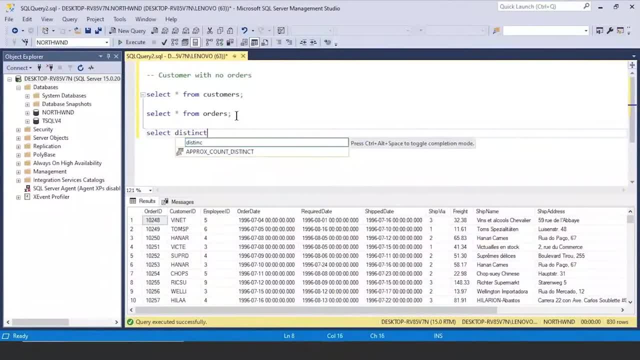 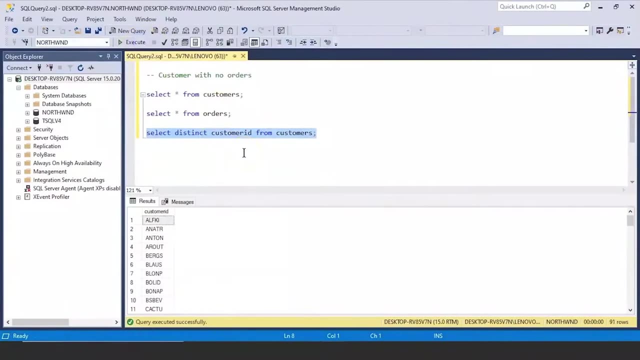 okay, so it's a very valid NRID. I want to find the distinct customer IDs from my customers table. let's run and see how many unique customer IDs we have. so there are total 91 customer IDs or customers. now let's check for the orders table. let's run it and see the 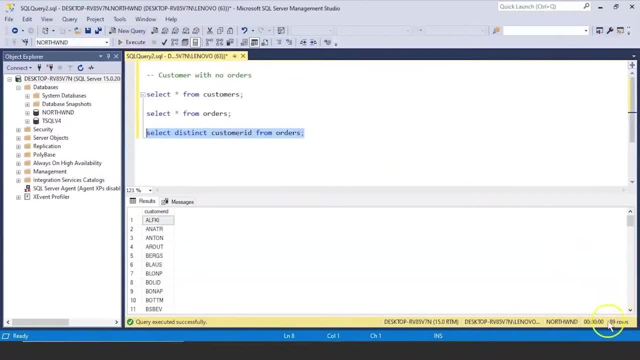 difference. now, if you see here, there are total 89 customer IDs in the orders table, which means there are two customers missing from the orders table and that implies those two customers don't have any orders. so to get the result, I will use two different queries to derive at the same output. so I'm 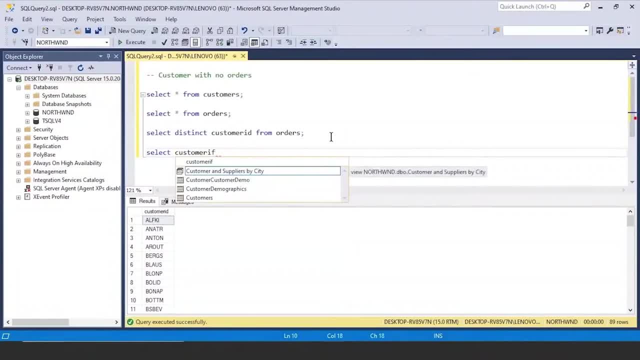 going to select my customer ID from my table. that is customers. I am going to use where my customer ID and then I am going to use the NOT in operator. I'm going to use a sub query: select customer ID, enter and select there I am going to. 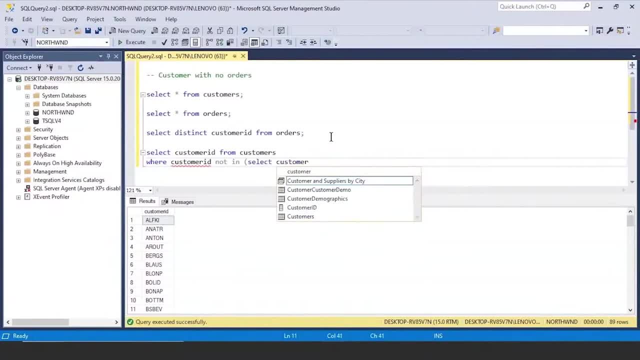 drive to the provider the order in which I did so, notice there has be no service ID from my orders table, close the bracket and I will give a semicolon. now what this query essentially does is, it is first going to find all the customer IDs that are present. 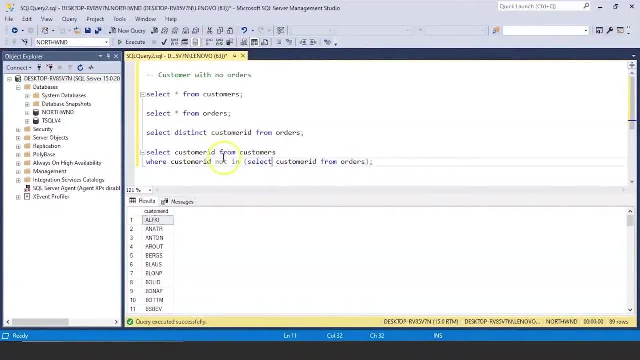 in my orders table and in the outer query. we are only going to return the customer that are present in both the tables and we are going to exclude those customers which are not present in the orders table. so let's run and see the results. we should get two customer. 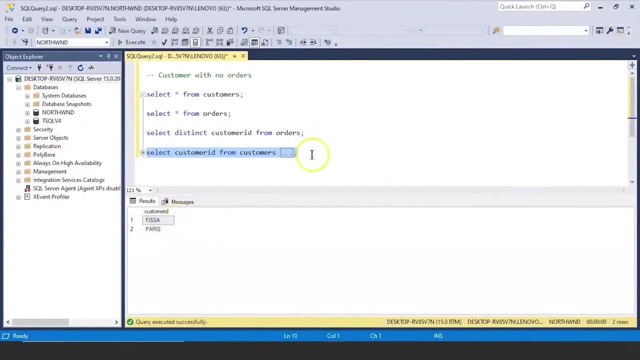 IDs. there you go. so these are the two customer IDs which are present in the customers table and are not present in the orders table, meaning that they don't have any orders in their name. now there is another way to do it. that is to use the not exist operator wherein you 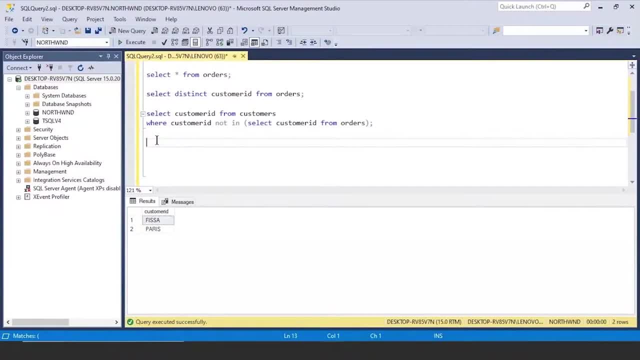 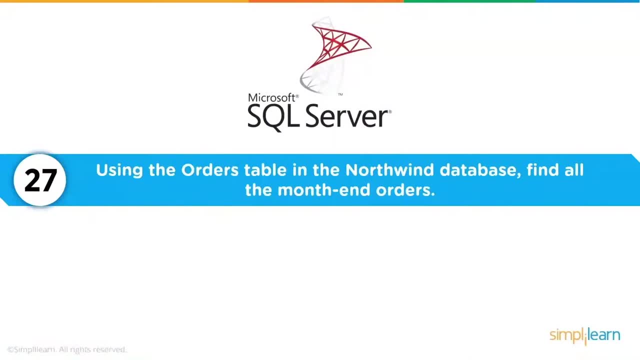 can write another sub query to get the same result. we will leave that to you. you can try this out using the not exist operator as well. coming to the 27th question, using the orders table in the northwind database we want to find all the month end orders, so such problems. 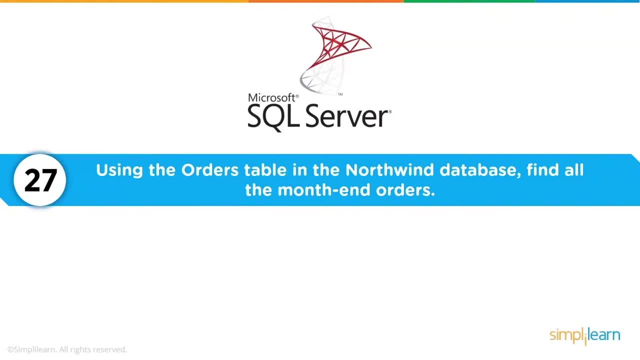 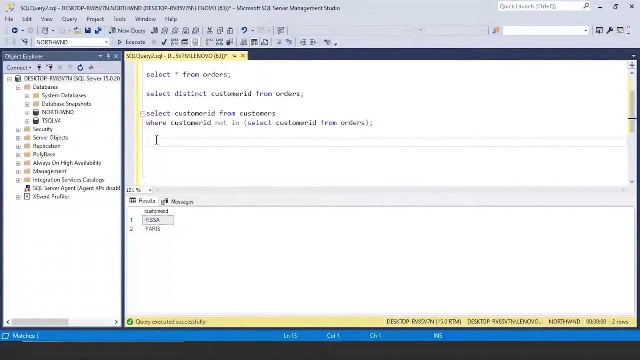 you will face while dealing with sales data, so very often sales executives would try hard to meet their month end targets. we want to display all the orders made on the last day of the month, so let's solve this question on our Microsoft SQL server. okay, so let me first give my comment for the 27th. 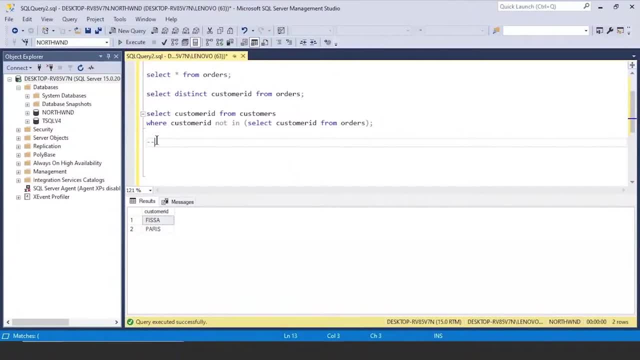 question. so the question is to find all the month end order. so I'll just write month end orders and the time is okay now to get the month end orders. we are going to use a built-in EO month function which stands for end of month. so let's start with the query. I'll write select. we are going. 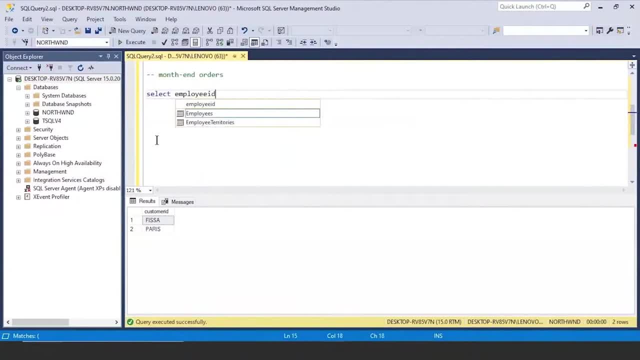 to select the employee ID comma. I also want the order ID and we want the order date from my table, that is orders. i'll then give my where clause, i'll write where my order date equal to and i'll use my inbuilt function. that is end of month. i have hit tab to autocomplete. 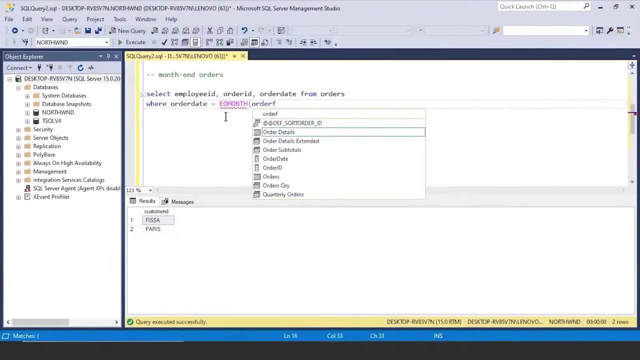 and inside this function i'll pass in my order date column. then i'm going to use the order by clause. i'm going to order it by employee id and the order id. i'll just move down and hit tab. okay, let's, let's run the query. there you go. we have got 26 rows of information. you see, on the 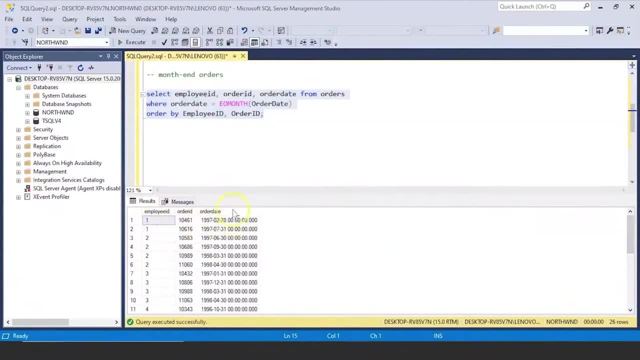 left side of the table we have got 26 rows of information. you see, on the left side of the table- left side- we have the employee ids, the order ids and then we have the order date column. now, if you mark the values present in the order date column, these are all the end of month date values. you. 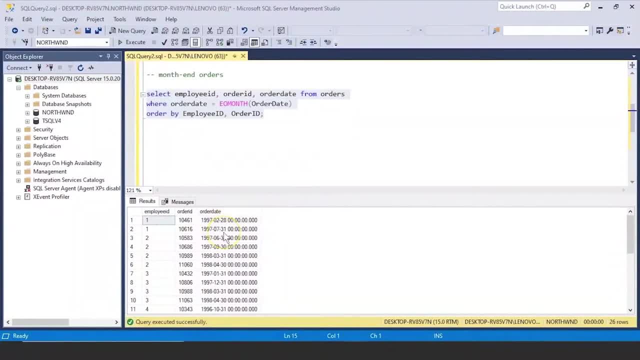 see, this is 28th of feb, then we have 31st of july, we have 30th of june, so on and so forth. so these are the list of all the orders that were placed. on the left side we have the employee ids, the order ids and then we have the order date column. 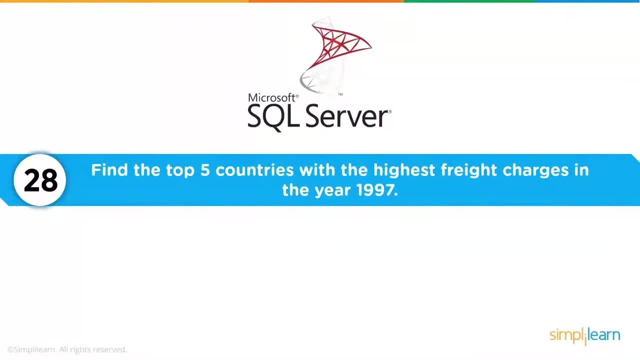 the last year of the month. coming to the 28th question, we want to find the top five countries with the highest freight charges in the year 1997. so freight charge is the amount paid to a carrier company for the transportation of goods from origin to another location. 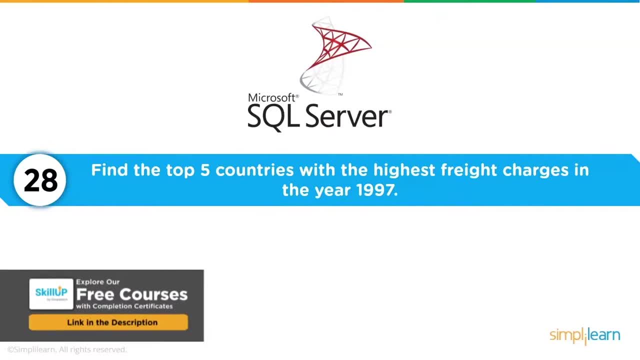 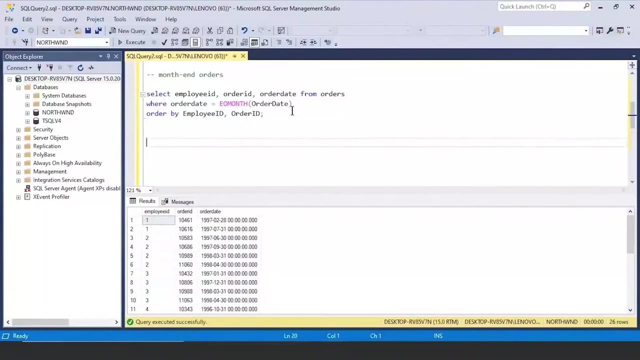 the freight charge is calculated based on the mode of transportation and the distance between the pickup place or the pickup location and the destination. so let's try this out on the continent. now. i was at the service station of microsoft server management studio. okay, so let me go ahead and give my comment. so, since we want to find the top five countries, 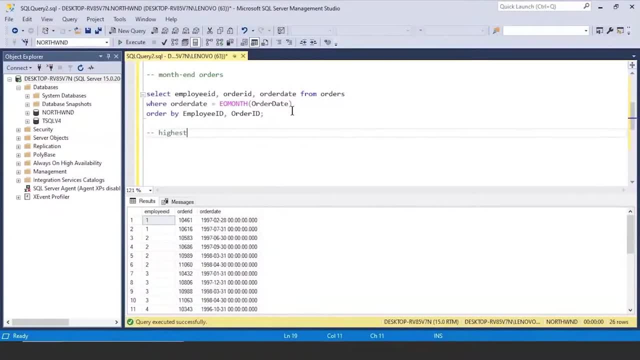 with the highest freight charges. i'll just give my comment as highest freight charges. Okay, Now to solve this question, I'll just change this to ght. Okay, We are going to use our orders table. So the way to do is I'll write select. I'm going to use the top five, So top is another keyword or an operator. 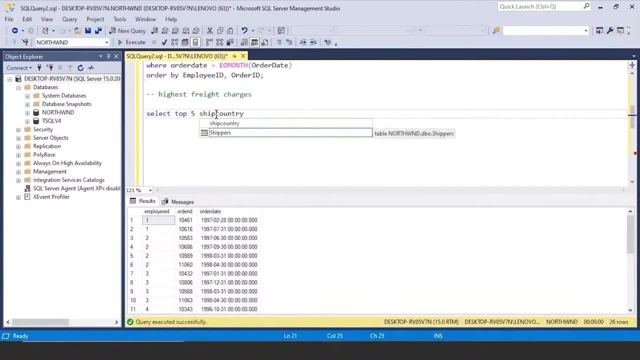 So I'm going to find out the ship country and then I'll calculate the average freight prices. So I'm going to use the average inbuilt function on top of my column, that is freight. I'll give an alias as, let's say, average freight. 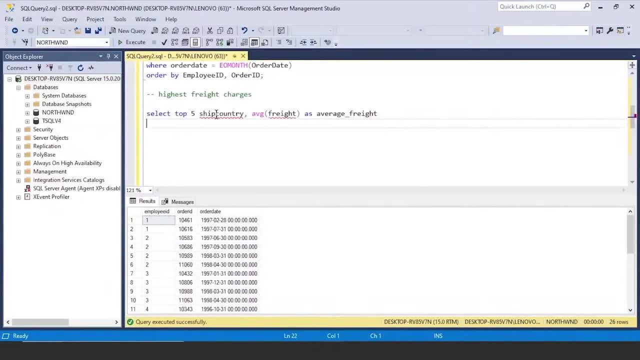 There should be no Space. I'll give a underscore. I'll write from my table that is orders. I'll use my where clause, where, and then I'm going to find the year from my order date column, and this year should be 1997.. 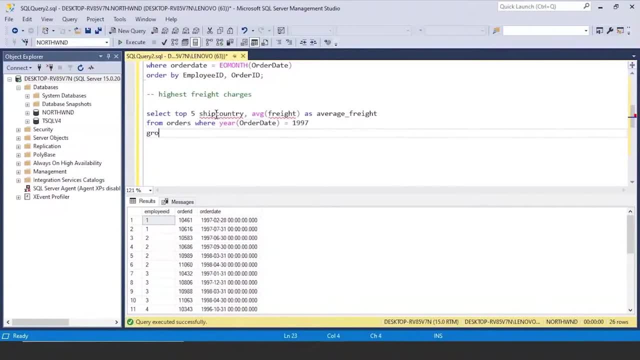 I'm going to group it by my ship country And I'll use order by my alias name. that was average freight and in descending order I'm going to sort it. Let's see the top five shipping countries who have the highest freight charges. 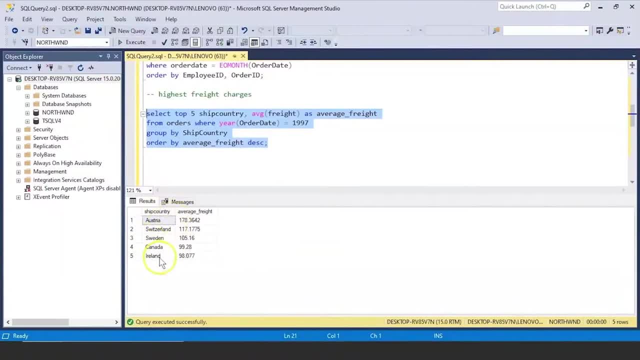 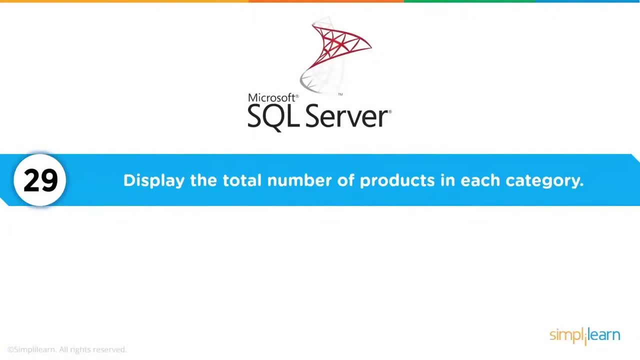 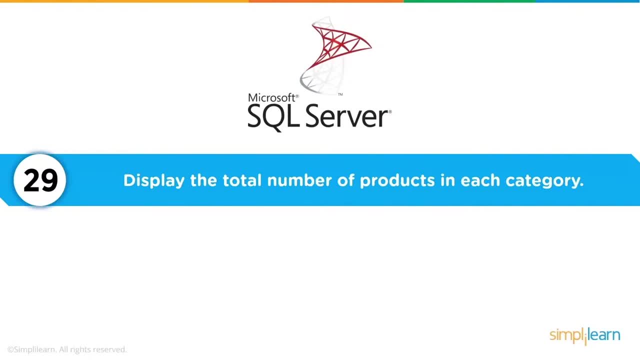 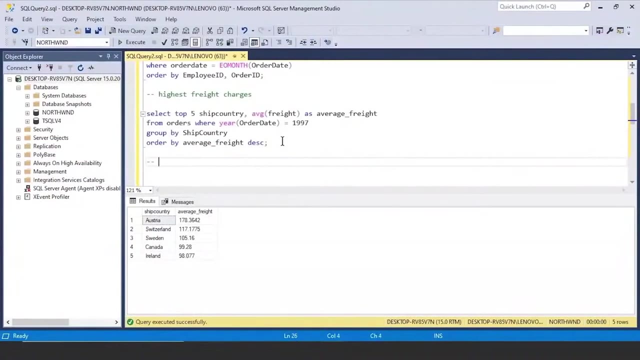 So we have two different tables, products and categories. So both these tables we are going to use to find a solution to this problem, that is, to display the total number of products in each category. So first let me give my comment. to display the total number of products in each category. 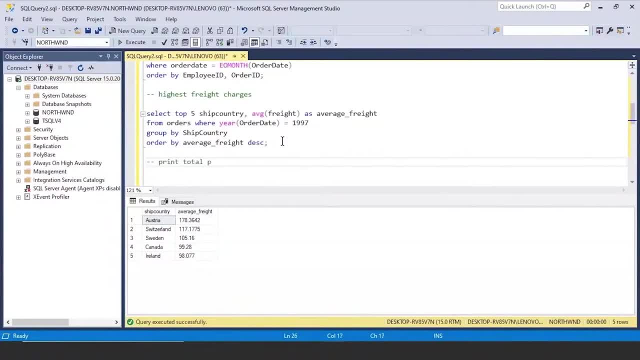 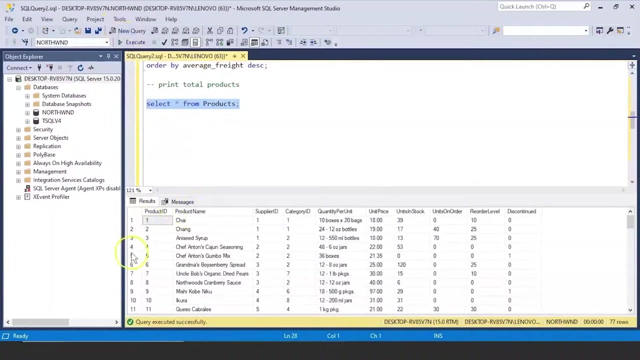 I'll just write: print: total products. okay, so to solve this problem, we are going to use our two tables, so let me first display the rows and columns from both the tables. the first table is products. okay, it is products. let's run this and see the columns that we have in this table. okay, so you have the product id. 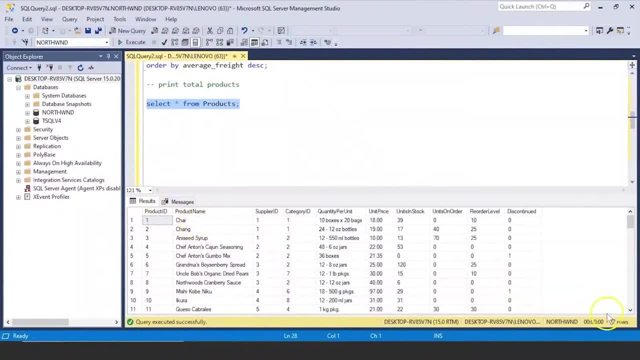 which is the primary key. you have the product name, so there are total 77 different products. okay, and then you have the supplier id. you have the category id, so these two columns are the foreign key columns. you have the quantity per unit unit price units in stock, units in order. 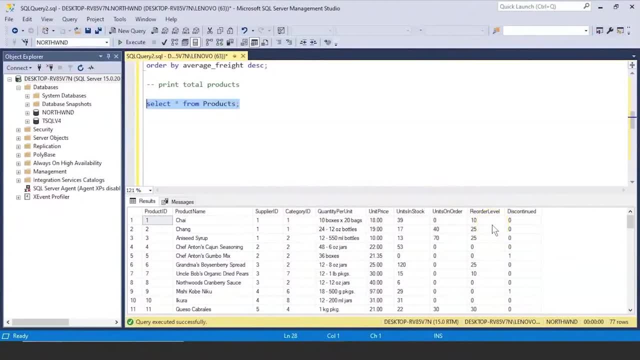 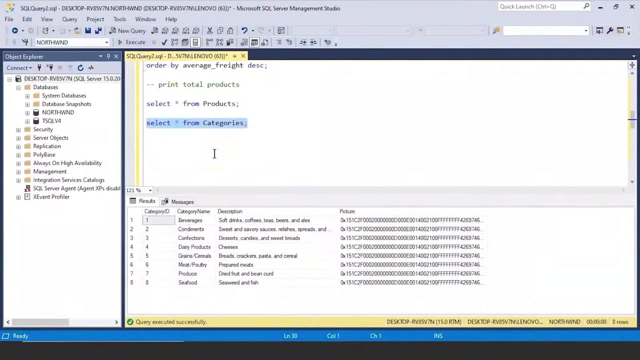 and if you want to reorder some product to fill in the stocks, so you have information for that as well, and if the product has been discontinued or not. i'll copy this and let's see what rows and columns we have in my categories table. okay, let me execute this. okay, so we have total eight categories of products. 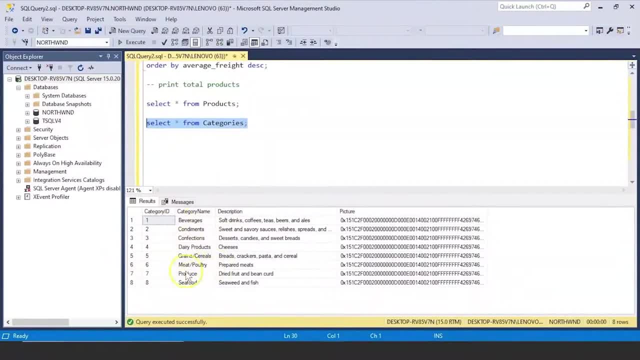 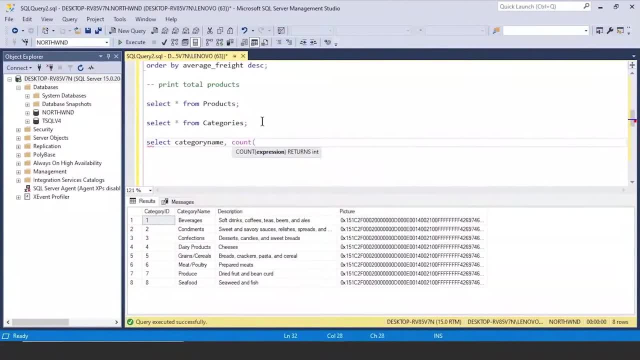 name, comma count star. i'll give this an alias name as total products given. underscore and write products from my first table, that is, products given, alias as p. i'm going to use an inner join with my categories table and i'll give my alias as c on my common key column, that is p dot. 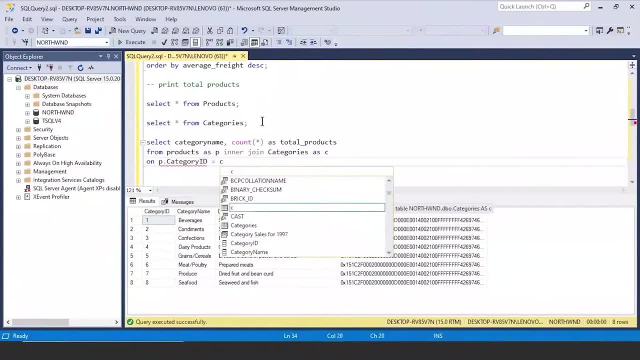 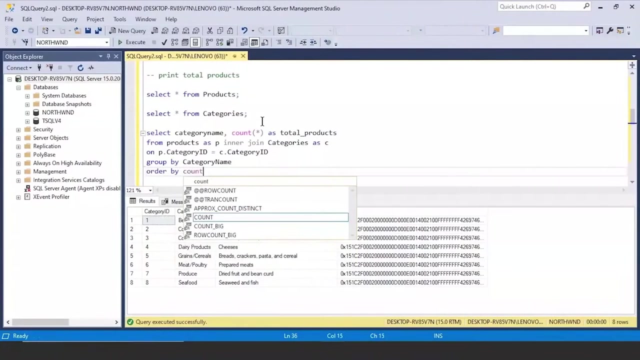 category id is equal to c dot category id, then i'm going to group my results based on the category names. so i'll write category name and we'll use the order by clause. i'll write order by count star as descending. so let's see the total number of products that we have in each category. 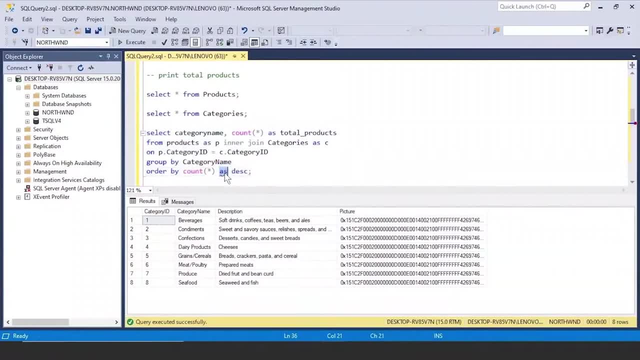 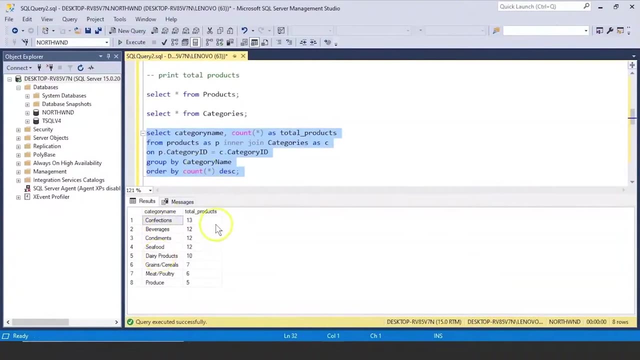 so this shouldn't be as descending, should be just count star descending. okay, i'll select and run it. there you go. so here, on the left hand side you have the different category names and on the right you have the total number of products that belong to each of the categories. all right? 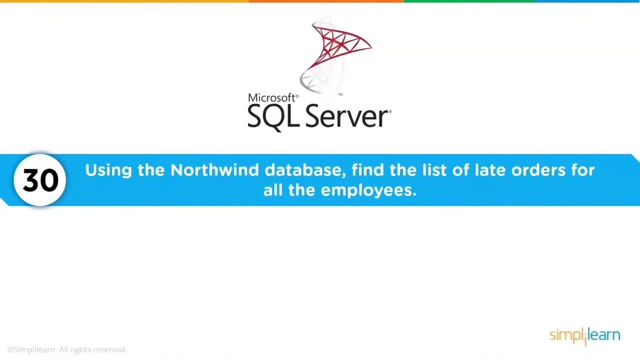 now moving on to the final question. so the last question is to use the northwind database and using this database, we want to find the list of late orders for all the employees. so this is a real world problem that often occurs, so the shipment of your orders might get delayed due to logistic issues. 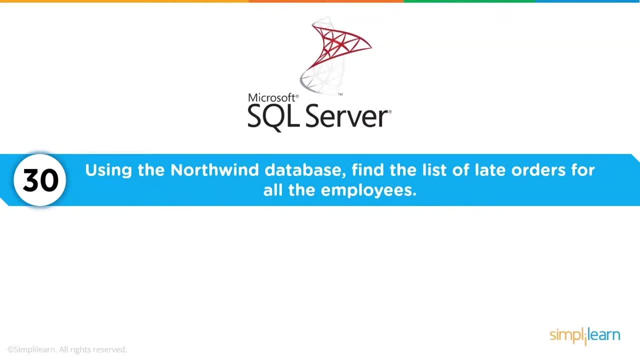 or if the products are not available on time. there can be various other reasons as well. so here we want to find those orders for the employees where the required date is less than the shipment date. we are going to use two different tables, that is, orders and employees. 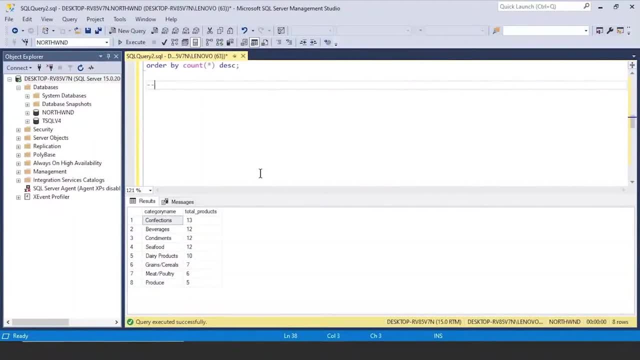 okay, now let me give my comment for the final query that we are going to write in this interview questions tutorial. so, using the orders table, i want to find the list of orders for all the employees, so i'll just give list of late orders, not just orders for employees. i write emps which 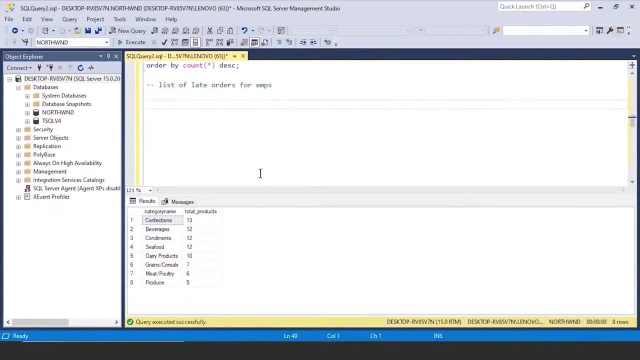 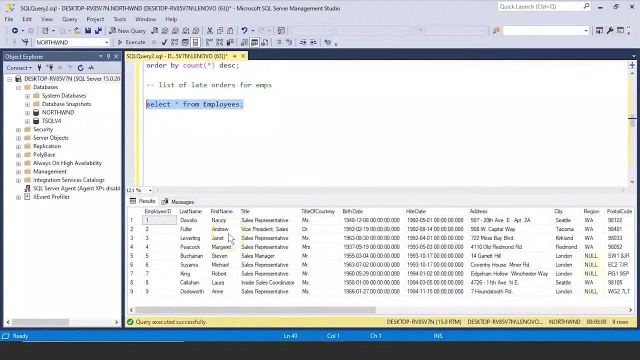 stands for employees. so here i'm going to use two tables: orders and employees. orders table. we have already seen. let's see the rows and columns that are present in the employees table. i'll write select star from employees and let me run it. okay, so there are total nine employees we have, so we have the employee id. this is the primary. 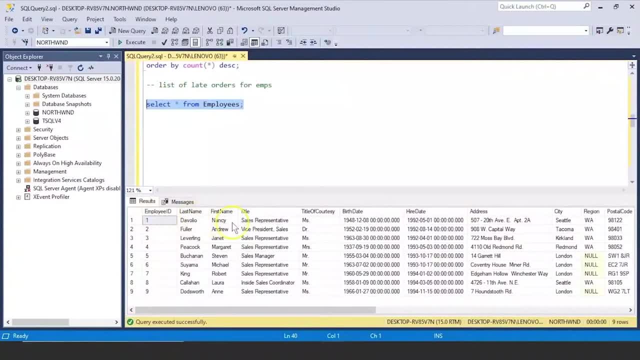 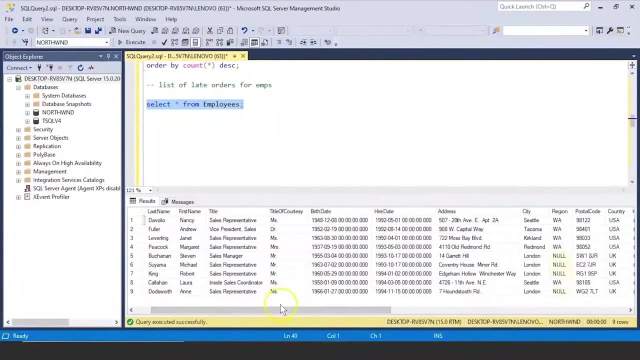 key column which goes from one to nine. we have the last name of the employee, the first name of the employee, we have the title, then we have the title of courtesy, whether doctor, mr, mrs. we have the birthday of the employee, the higher date or the date of joint. 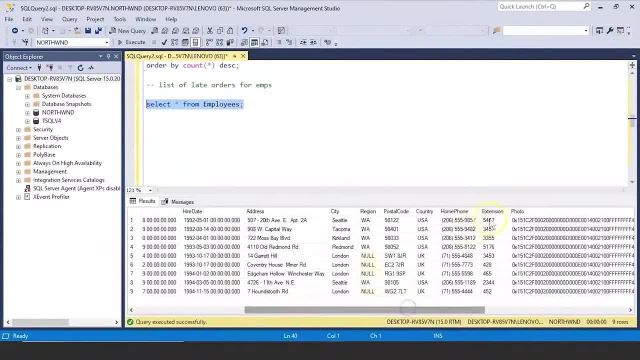 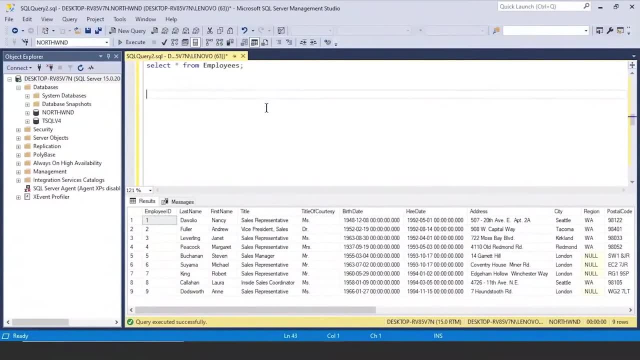 you have the address, city, region, postal code and other information, all right. so let's see how you can join the orders table and the employees table to get the list of late orders. and we must remember that late orders are those where the required date is less than equal to the shipped date. so i'll start with select e dot. 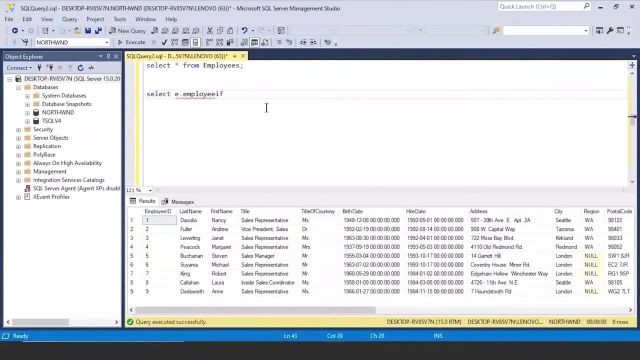 i'll write emps- employee id comma. i want the first name comma. i'm going to count star as late. orders from my table: orders as o. then i'll use my inner join. i'll write employees as e. it doesn't matter actually if you use small e or capital e. 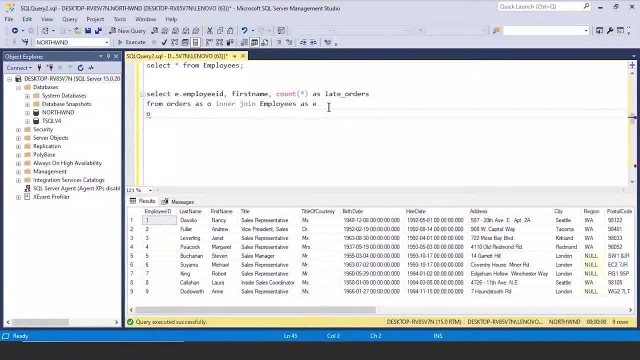 then i'm going to use my on condition on e dot, on e dot employee id equal to o dot employee id. so this is my common key column that is present in both the tables. then i'll use my where clause where i'm suppose you should be careful and you should give the right clause. so my required date: 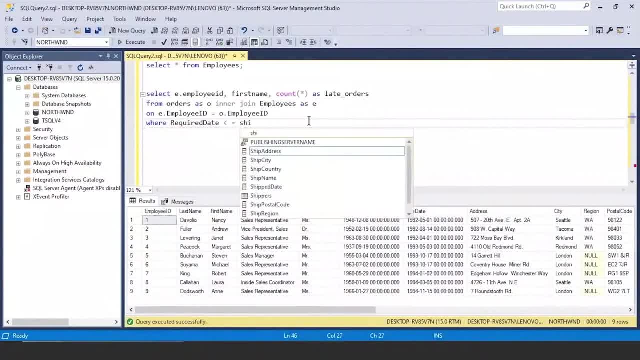 should be less than or equal to my shift date. so this is my condition and then i am going to group by e dot employee id comma, e dot first name, and then i'll use my auto by clause order by my alias name. that was the date of this order by clause. 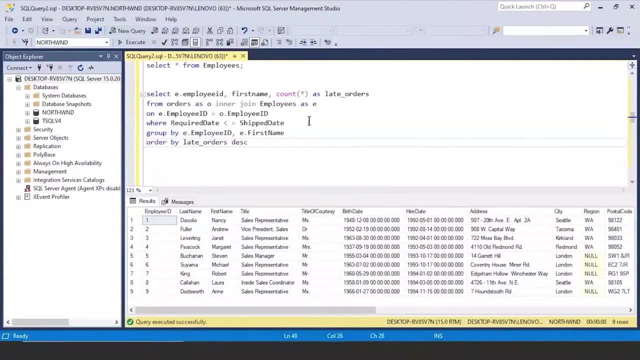 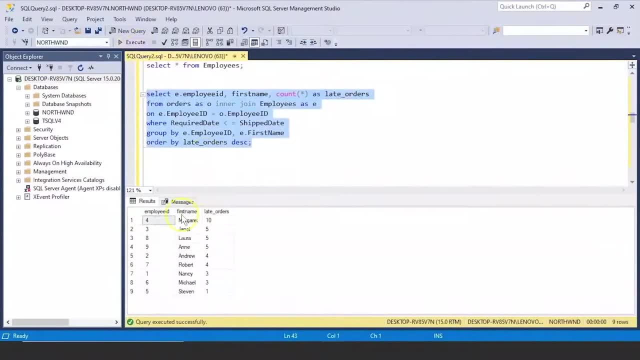 name. that was late orders and i'll arrange it in descending order. so let's run this and see our result. okay, so you have the employee ids on the left, then you have the first name of the employee ids and then you have the late orders for each of these employees. so if you see here, employee id 4. 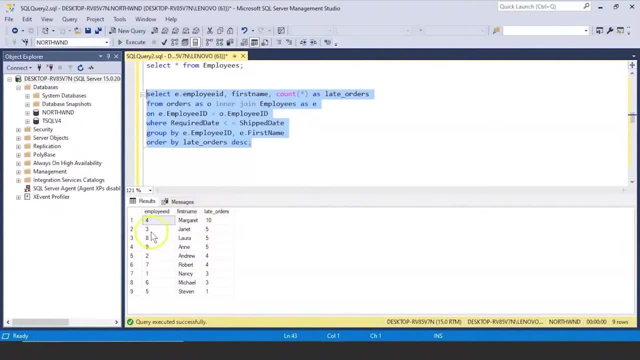 has the highest number of late orders, followed by employee id 3 and 8, as well as 9, who have five late orders. then we have the employee id 2, which has four late orders. even employee id 7 has four late orders. employee id 5, that is, steven, has only one late orders. 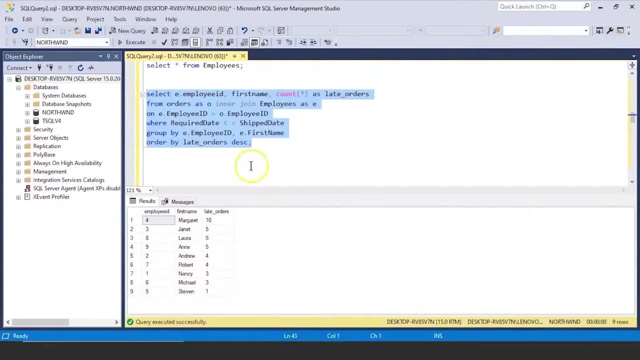 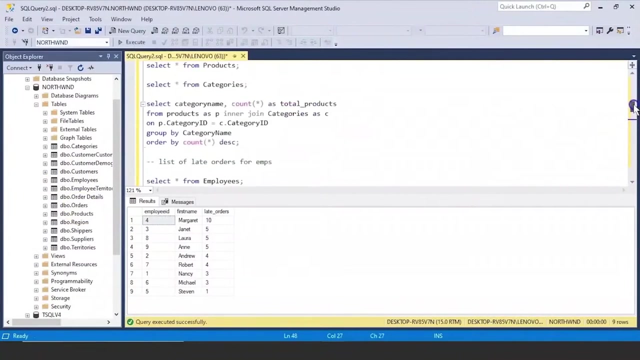 so we are done with our demo section and we have covered all our 30 questions, out of which 25 questions were based and used on mysql server. and to address the last five questions, we used our northwind database. you had a lot of tables- you can see it here- and using those tables we solved some interesting questions. 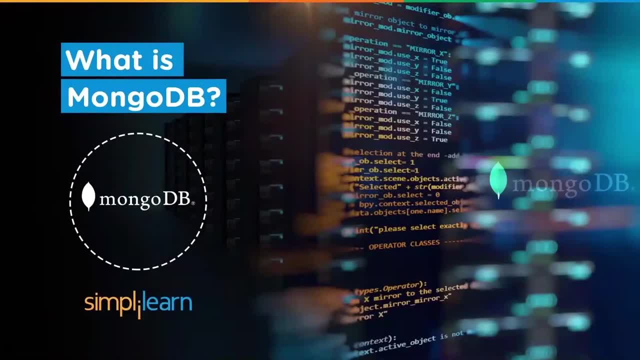 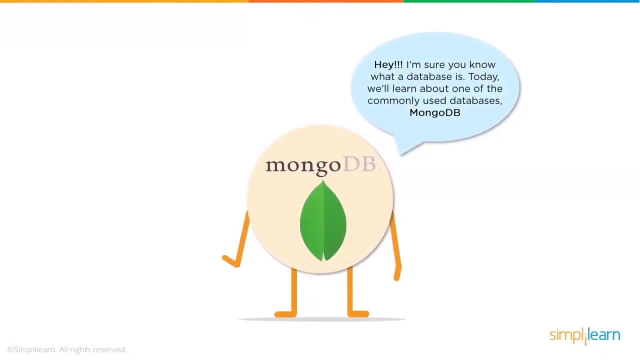 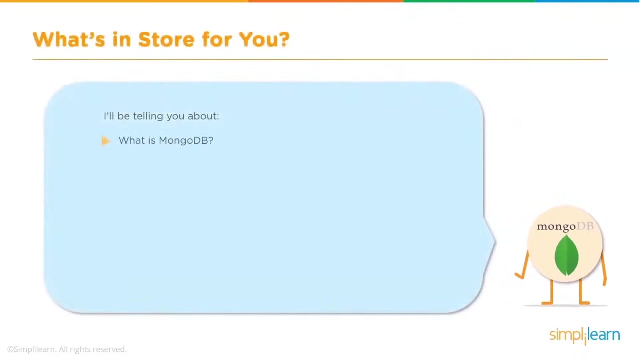 in this video we'll understand what exactly mongodb is and what are its key features. now i'm sure you must have heard about databases, but mongodb is a popularly used- not only sql- database. now, without further delay, let's begin and understand what exactly mongodb is. so here's what's in store for you. first we'll understand what mongodb is, then we'll understand. 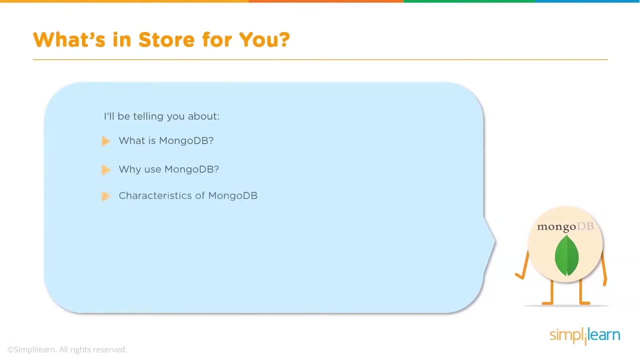 why exactly mongodb is used. then we'll understand the characteristics of mongodb. after that we'll understand the working of mongodb and how it functions. we'll also look at some of the commonly used applications of mongodb and finally we'll look at the top companies that readily deploy mongodb. so what exactly is mongodb? it is a document oriented no. 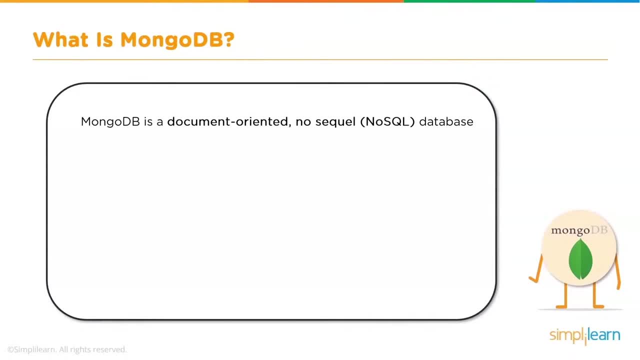 NoSQL Database. It was initially released in August 27, 2009.. MongoDB replaces the concept of rows of conventional relational data models with something called documents. It offers developers the flexibility to work with evolving data models, Since it's document-based, MongoDB allows embedded documents arrays and represents 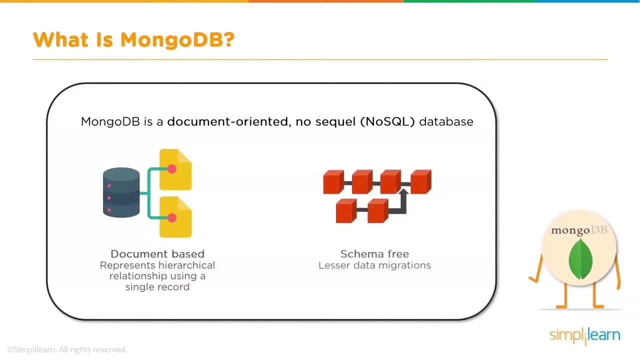 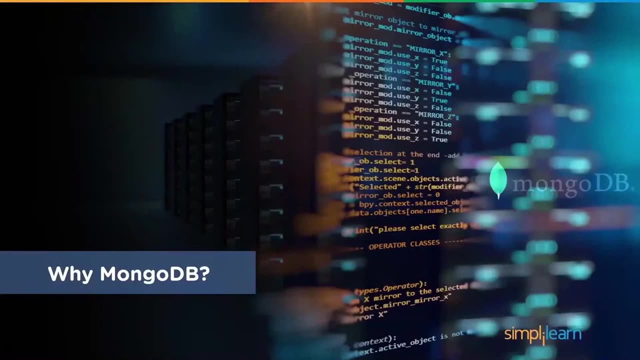 complex hierarchical relationships using a single record. It is also schema-free, which means that the keys defined in the document are not fixed. As a result, massive data migrations can be ruled out. But you must be wondering: when there's something like SQL, why is NoSQL or MongoDB used? 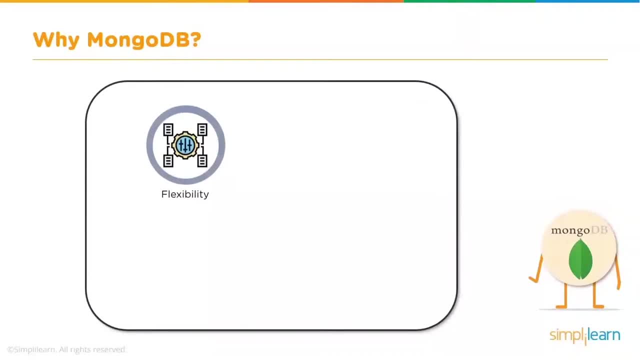 There are a few reasons why MongoDB is widely used. First up is flexibility. MongoDB's notion of documents that can contain sub-documents nested in code, Complex hierarchies, is really expressive and flexible, Flexible query model. A user can selectively index some part of a document or a query based. 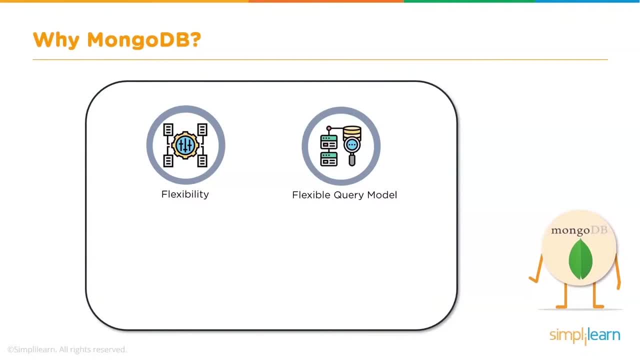 on attribute values, regular expressions or ranges. Next up is native aggregation. Native aggregation allows its users to extract and transform data from MongoDB and either load them in a new format or export it from MongoDB to other data sources. It makes it extremely compatible. 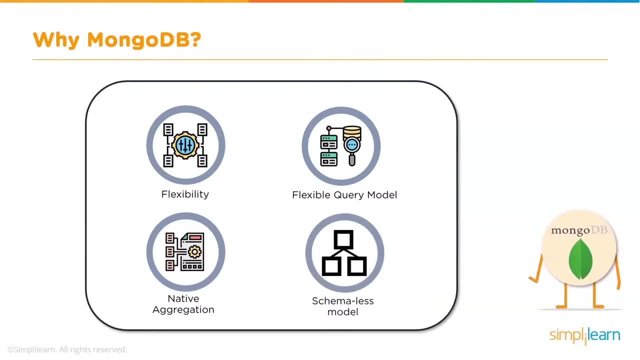 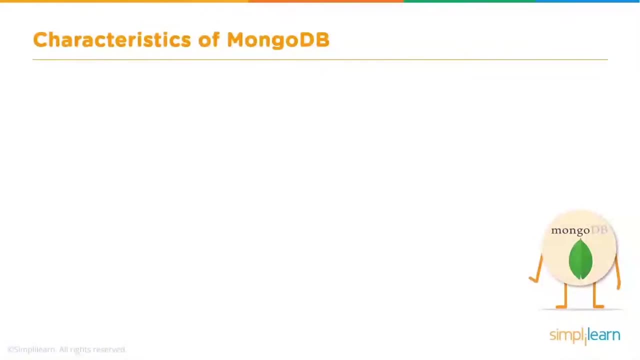 Lastly, as mentioned earlier, the schema-free model. Now applications get the power and responsibility to interpret different properties in different ways. Now that you know what MongoDB is and why exactly it's used, let's have a look at the characteristics of MongoDB. 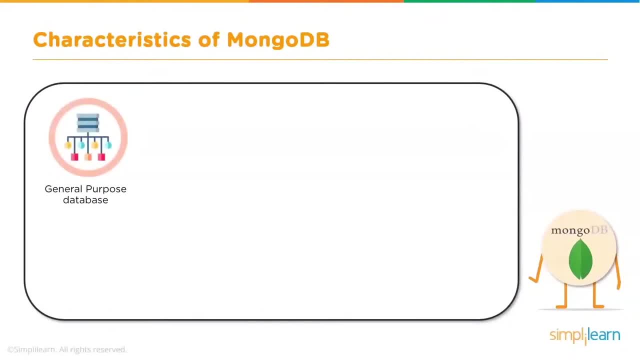 Firstly, it's a general-purpose database. Now MongoDB can serve heterogeneous loads and multiple purposes within an application. Again, it has a flexible schema design. Document-oriented approaches with non-defined attributes that can be modified on the fly is a key contrast between MongoDB and any other relational database. 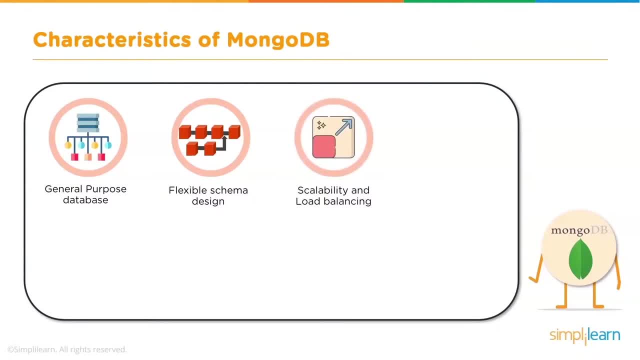 Next up is scalability and load balancing. It's built to scale both vertically but, most importantly, horizontally. Using sharding, an architect can share load between different instances and achieve both read and write scalability. When it comes to load balancing, this happens automatically. 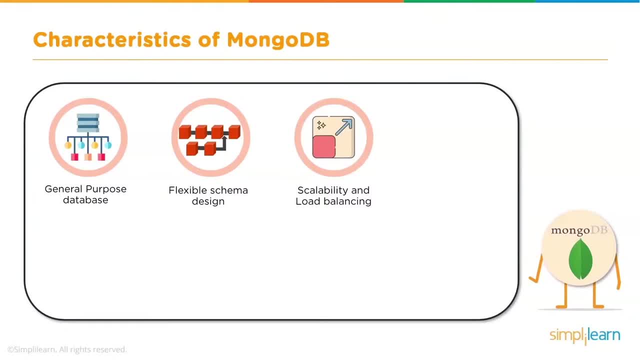 The load balancing is done automatically and transparently to the user by the shard balancer. Again we have the aggregation framework. MongoDB offers an extract, transform and load framework that eliminates the need for complex data pipelines. Native replication Data will get replicated across a replica set without complicated setup. 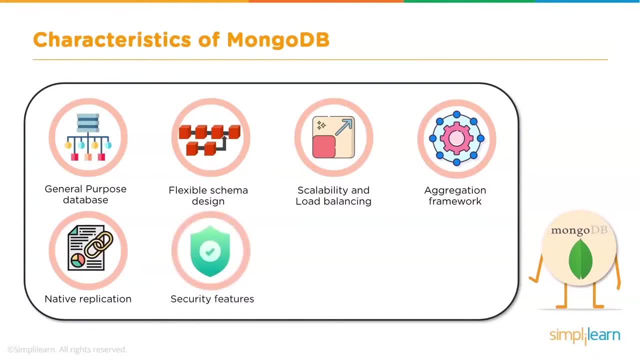 Security features, both authentication and authorization, are taken into account in MongoDB. Next up is JSON. now, JSON is widely used across the web for front-end and API communication and, as such, it's easier when the database is also compatible with the same protocol. 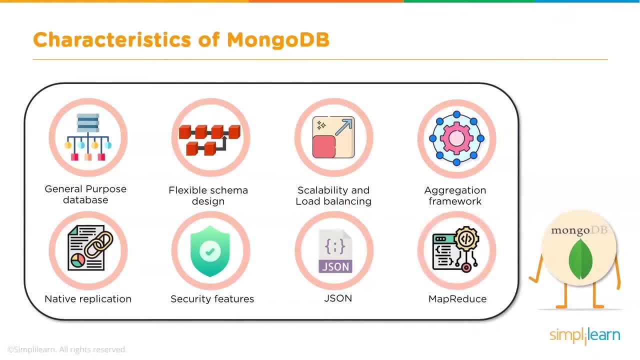 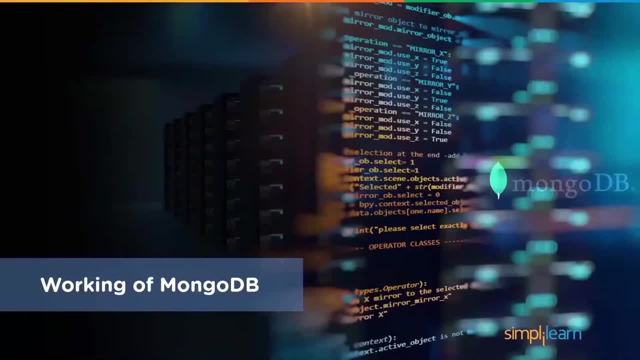 Lastly, we have MapReduce. now again. MapReduce is an excellent tool to build data pipelines, and MongoDB uses MapReduce readily. Now let's quickly have a look at the working of MongoDB. Data is stored in documents with the help of key-value pairs. 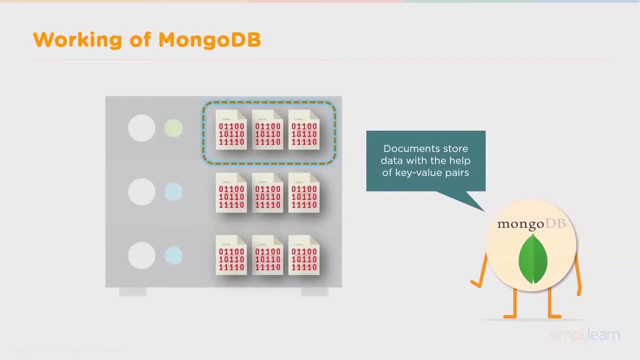 Now the data is stored in the BSON format. At the backend. MongoDB converts JSON data into a binary format known as BSON. MongoDB also makes provision for nested data. Now all of these documents are stored in a collection. These collections hold multiple documents and, since MongoDB is schema, less the documents. 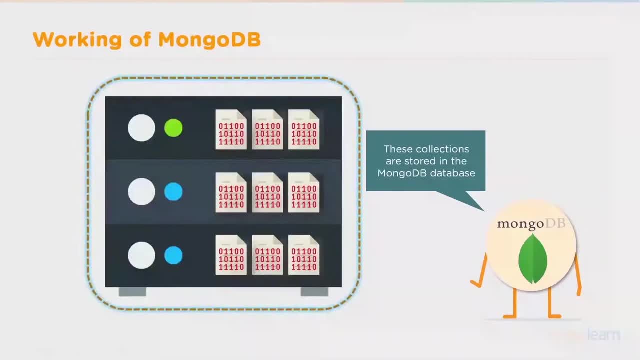 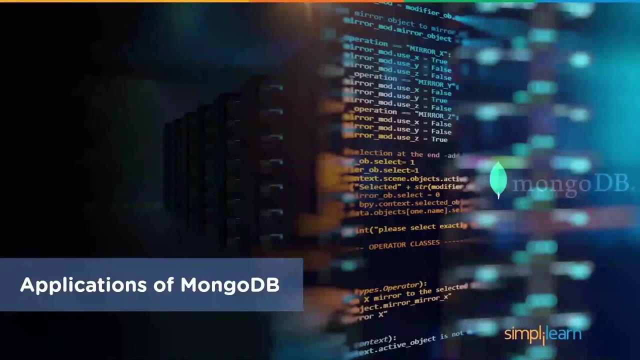 in one collection need not be similar. Now again, these collections are stored in a collection, stored in the entire MongoDB database. As mentioned earlier, MongoDB makes provision for nested data. This makes fetching of data extremely efficient when compared to other databases. Now you must be wondering where exactly MongoDB can be applied or used, So let me help you. 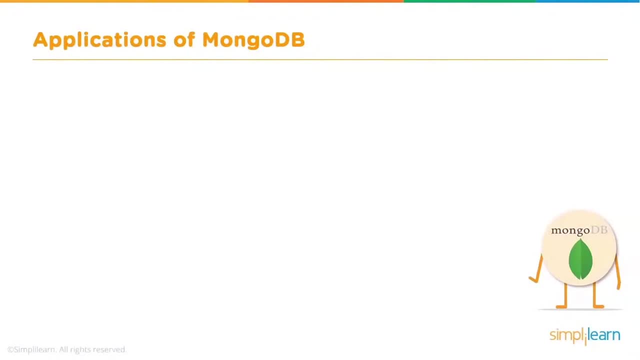 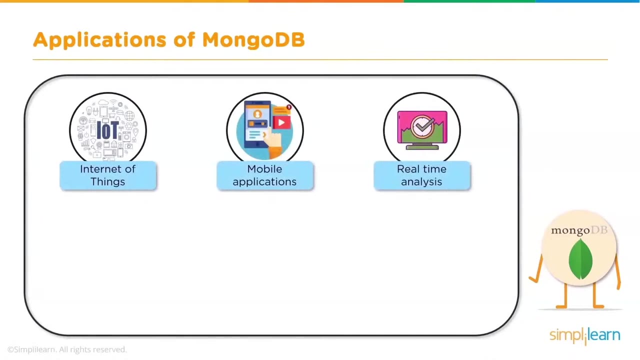 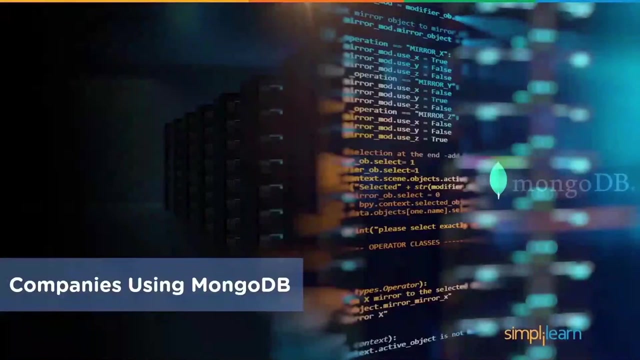 with that, Several areas of technologies use MongoDB as their DBMS currently. Some of them are Internet of Things, mobile applications, real-time analysis, personalization, catalog management and content management. Now, all said and done, let's look at some of the companies that 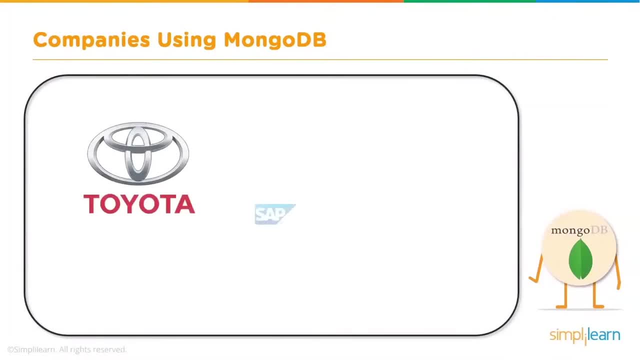 use MongoDB currently. Companies like Toyota, SAP, AstraZeneca, Adobe, Verizon, Cisco, Barclays and Google, among others, readily deploy MongoDB as their database management system. In this video, I'm going to show you how MongoDB can be used as a database management system. 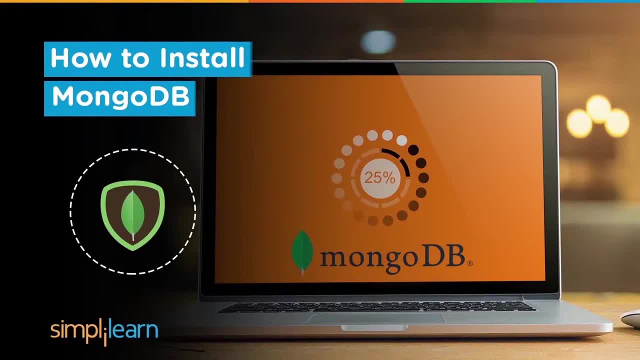 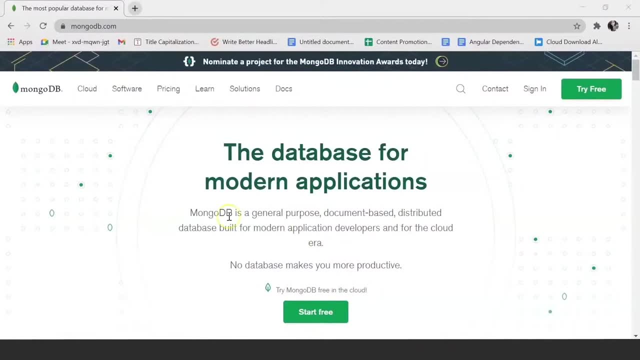 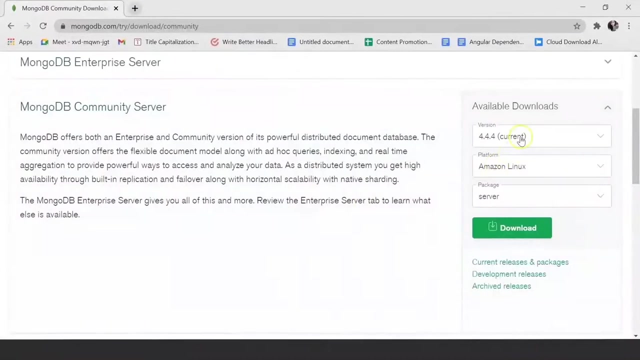 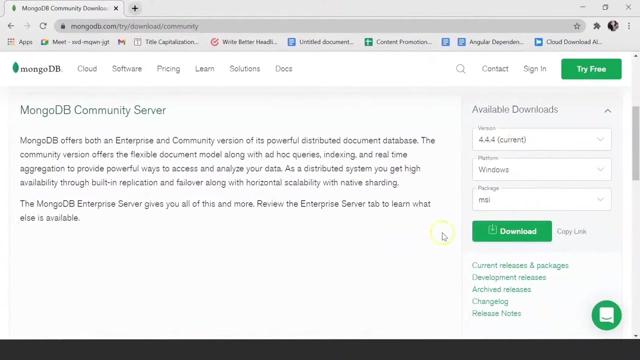 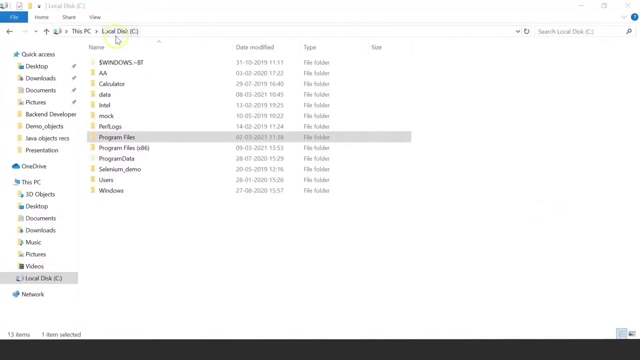 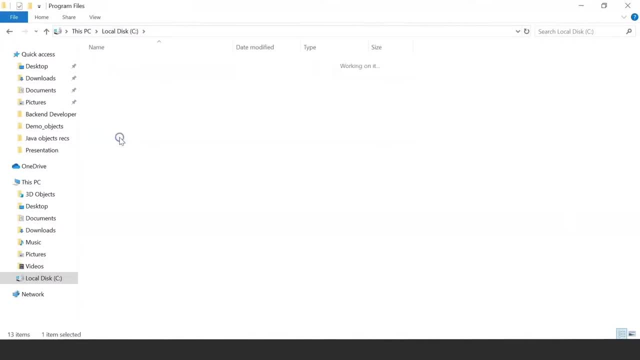 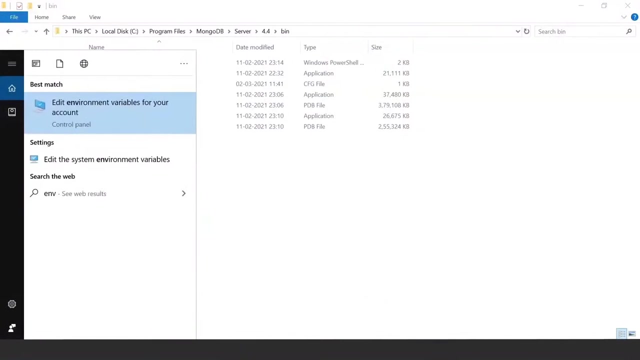 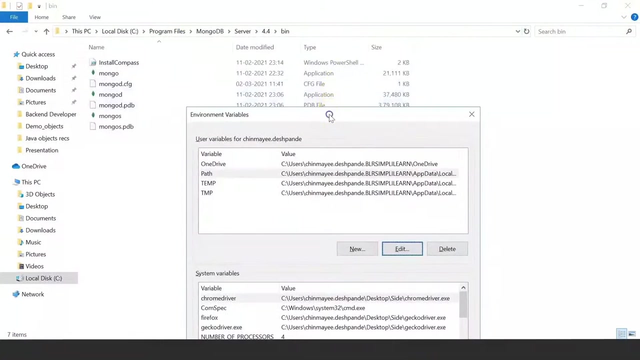 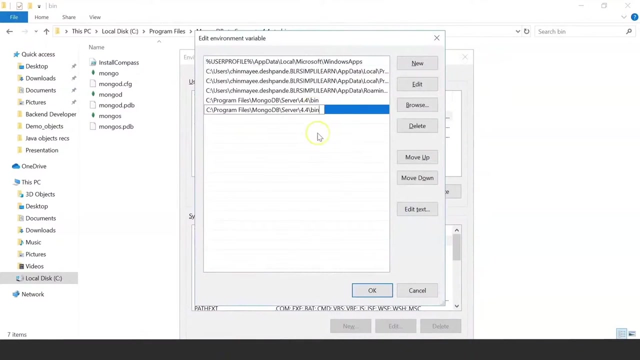 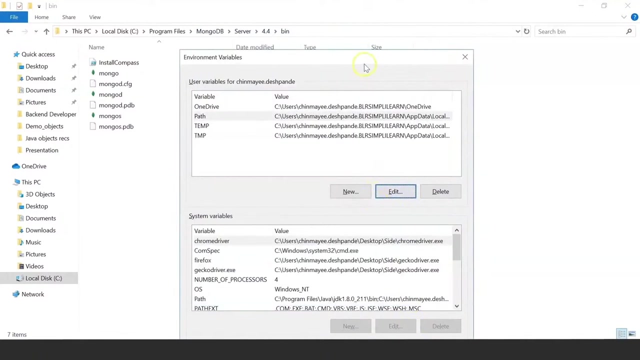 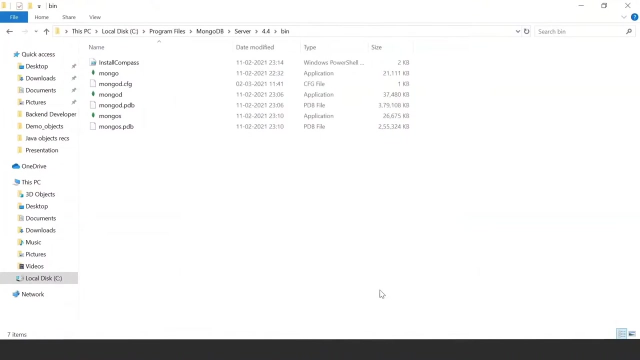 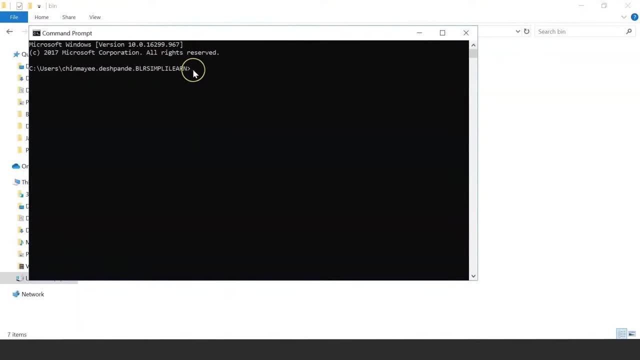 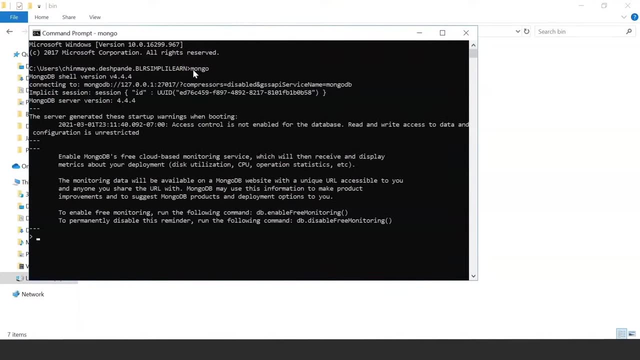 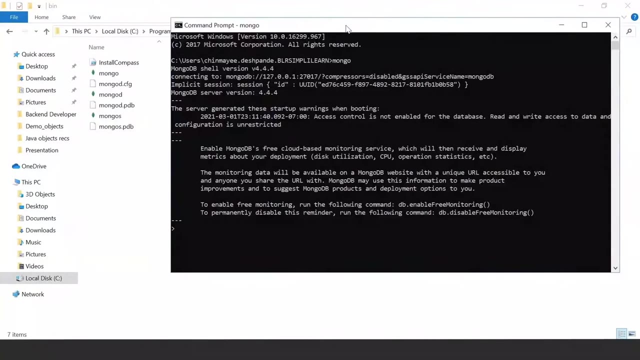 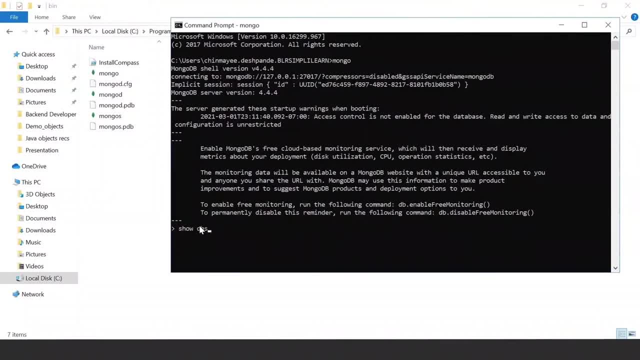 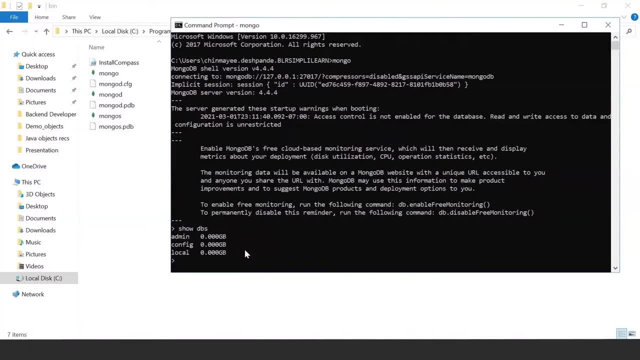 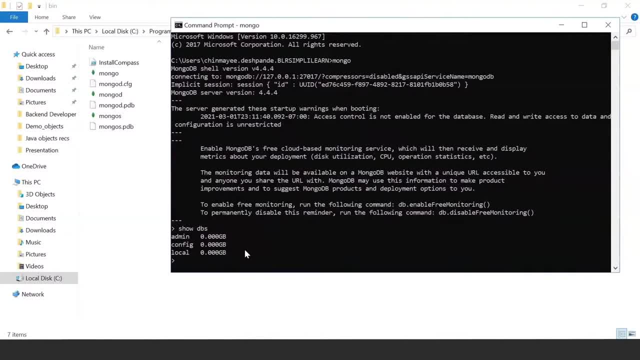 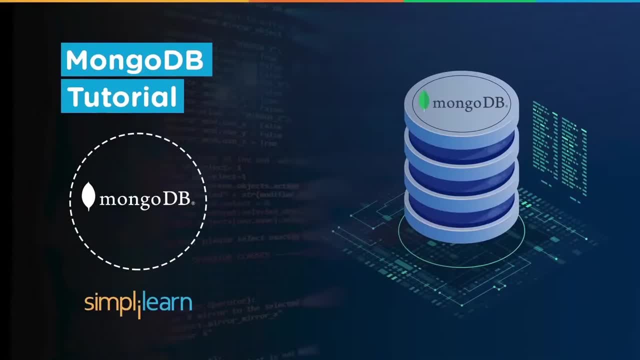 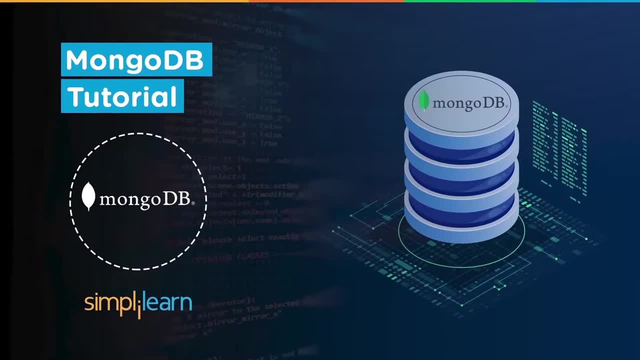 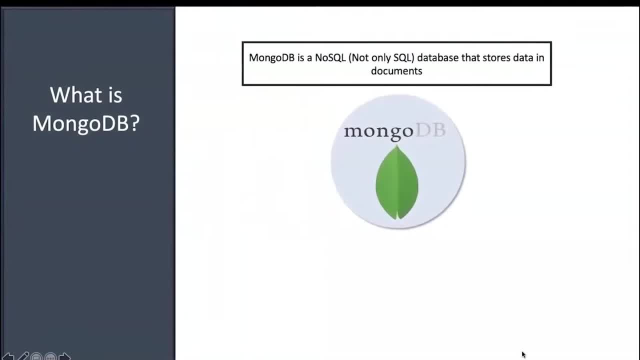 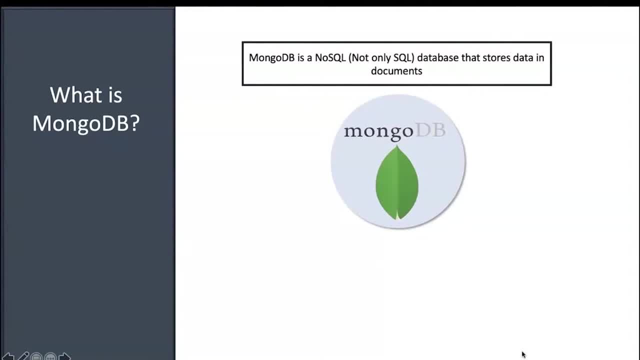 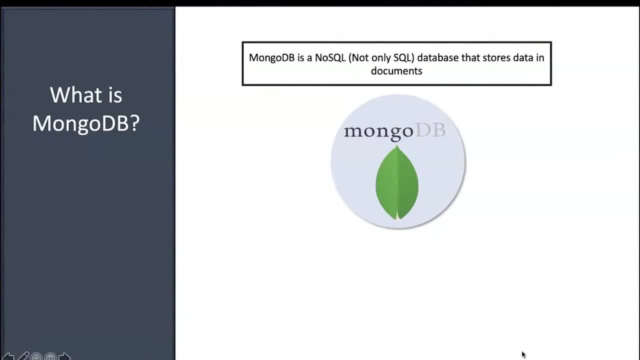 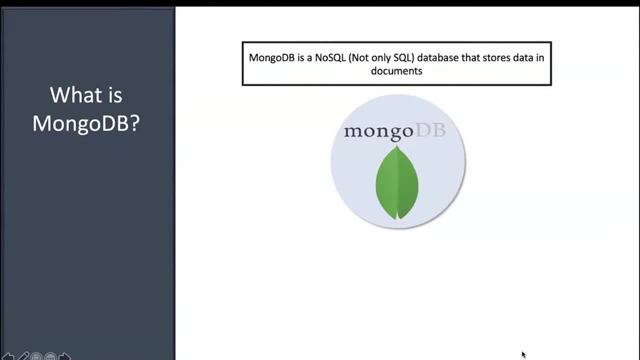 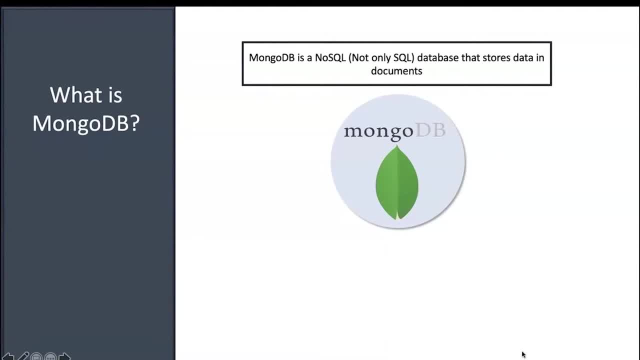 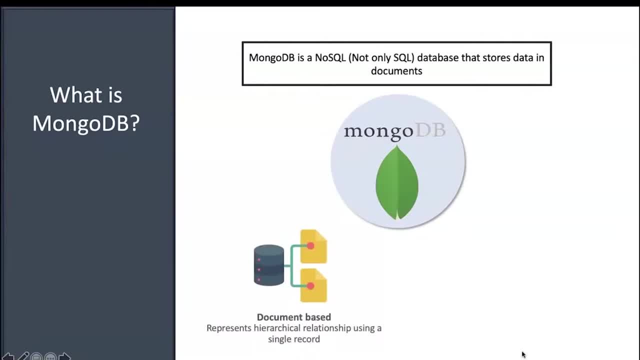 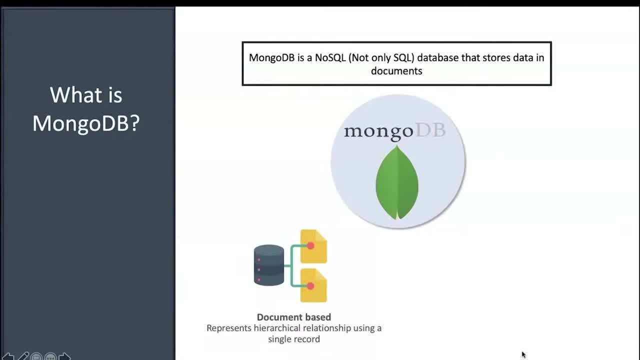 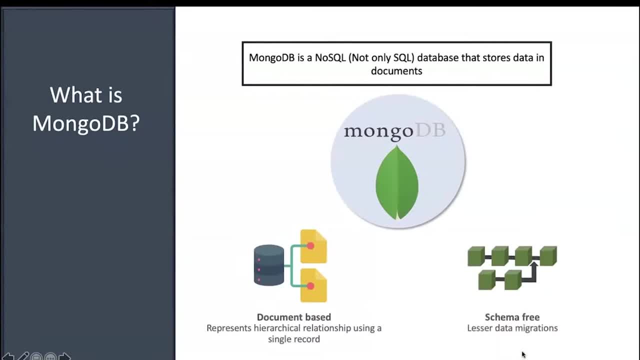 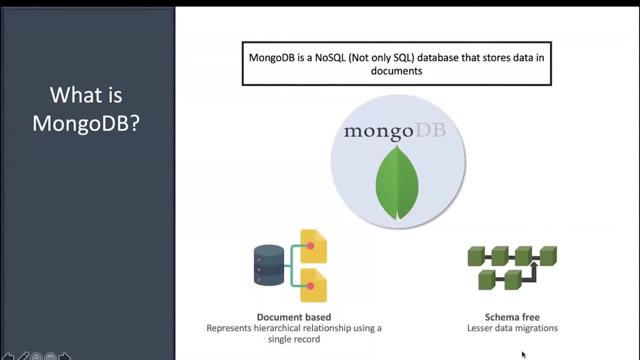 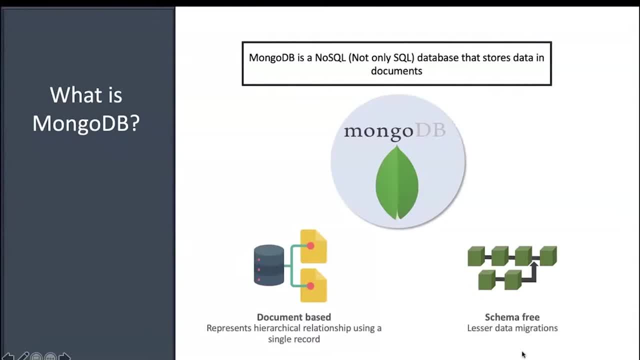 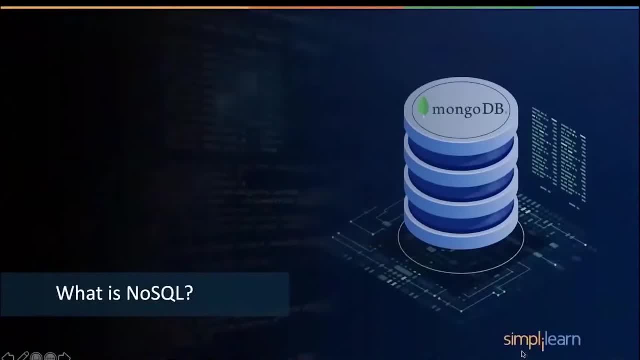 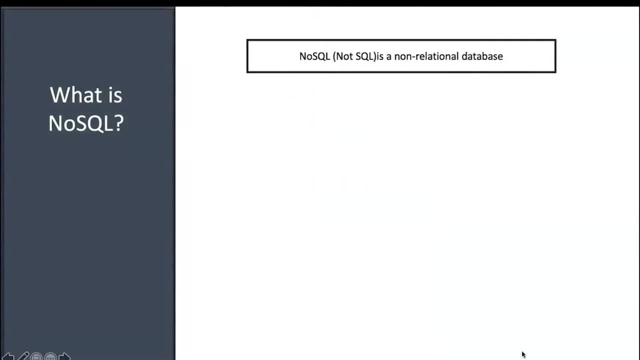 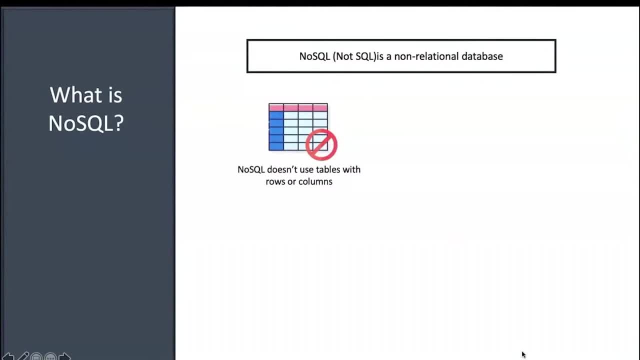 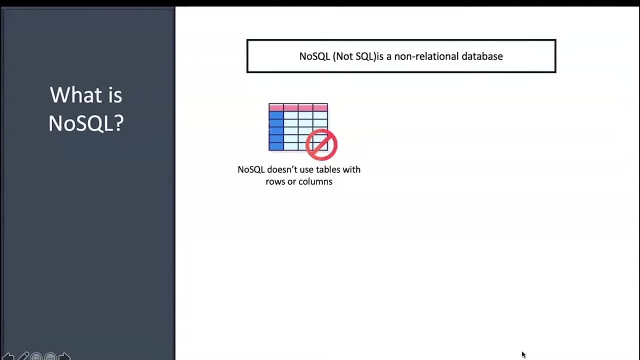 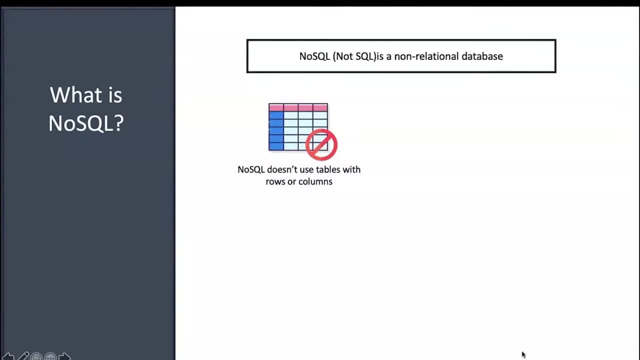 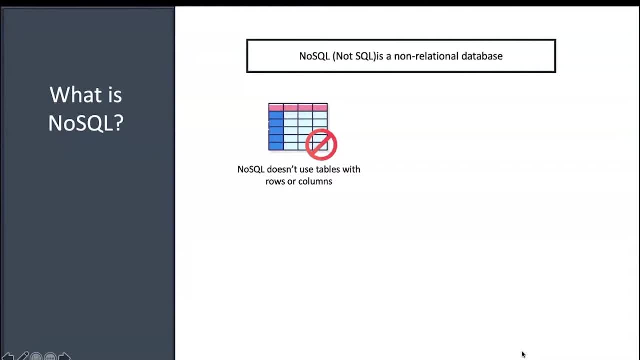 In this video I'm going to show you how MongoDB can be used as a database management system, complete table structure. like they talk about columns, they talk about rows and are all about so here in nosql it stores the relationship data in the documents, so the different type of 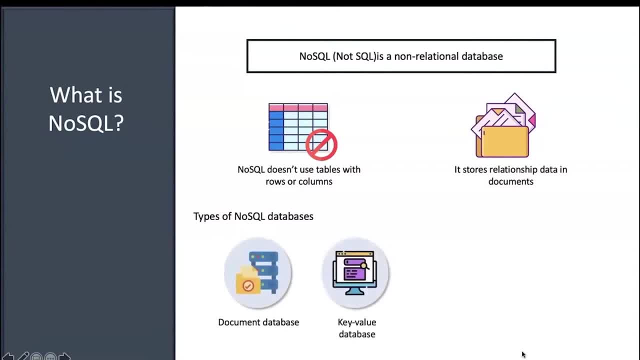 nosql databases are available, like you talk about, called document based. you talk about key value base. you talk about white column based and graph based. different options are available for the nosql, but the one which we are using it mongodb. it is a purely document based database. now, 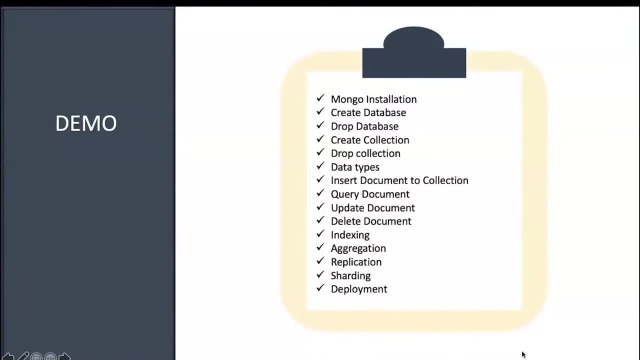 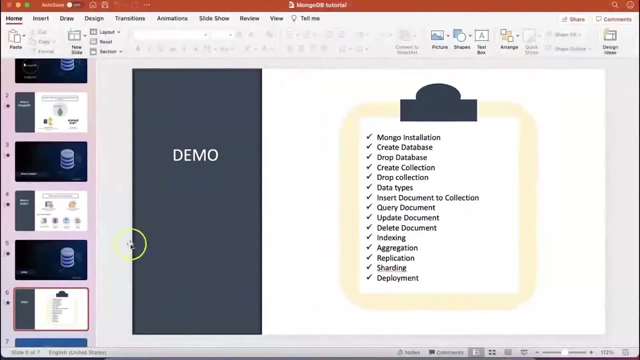 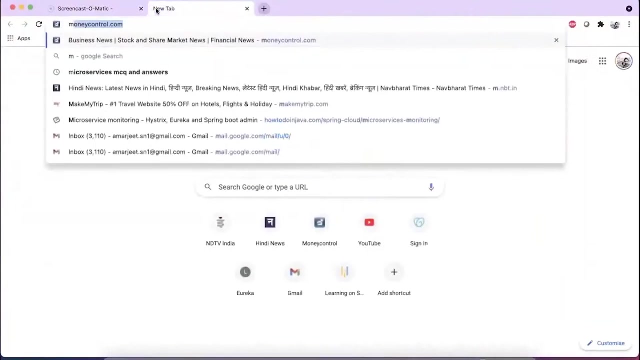 here we would like to go ahead with some demonstrations, like talking about, like, how mongodb installation works and the other aspects. okay, everyone. so now we're going to start working on the first option, called mongodb installation. okay, see, mongodb installation is very simple. if you open a website and go for this website name called mongodb download. 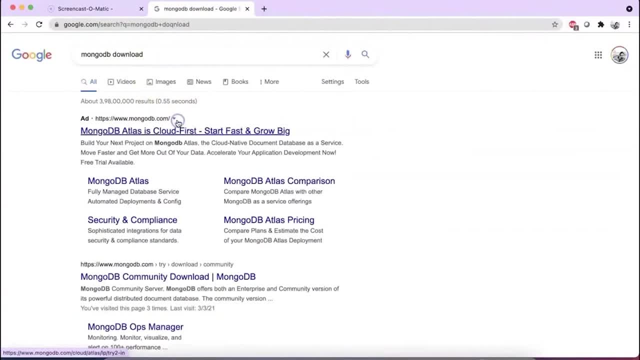 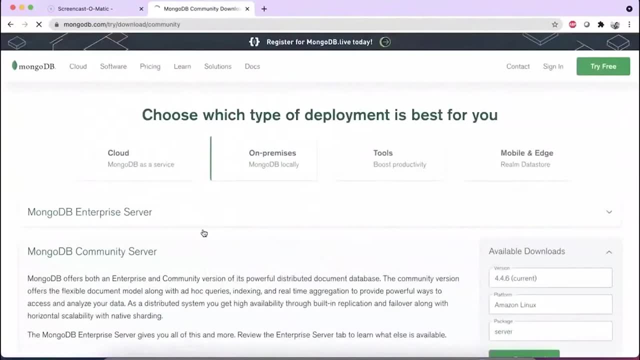 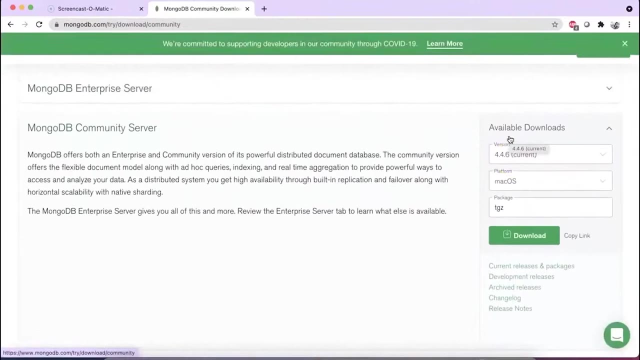 if you talk about mongodb download, you're going to see the official website called mongodb community download is available when you click here so you can see. it is taking the current version to 4.4.6 mac os. it by default detected my platform. however, you can select, depends on which platform you have. 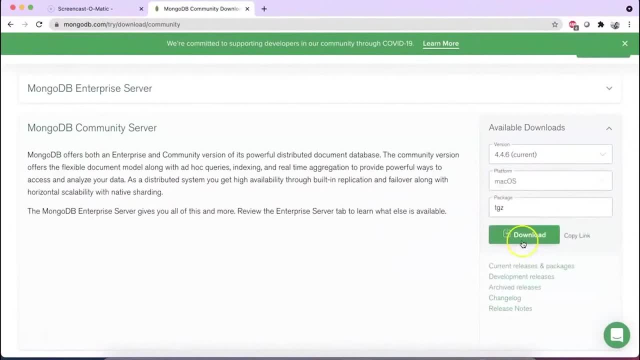 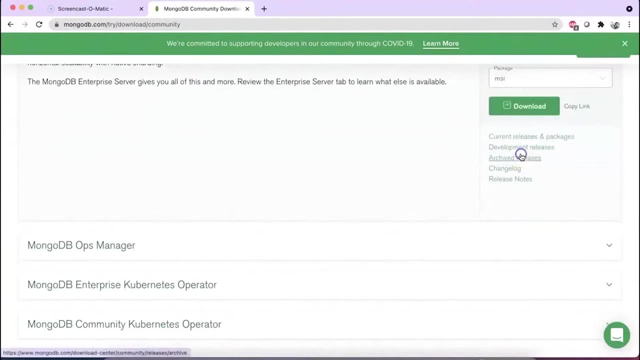 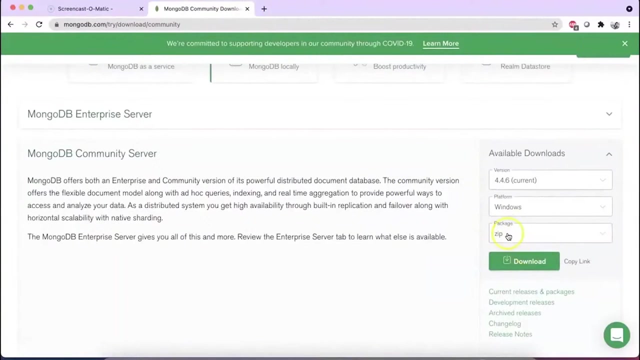 it and after that you will be clicking on this download. okay, now you can see that, the mongodb, so it will get ready. for if you're from windows, i would say, in this windows you can select appropriate option. like two options are available. you can talk about msi or talk about zip. my recommendation is you can stick to the. 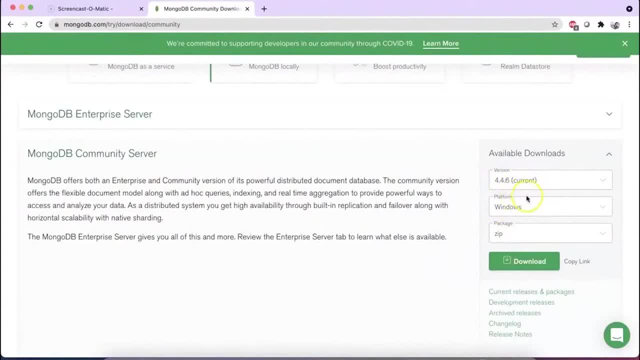 zip power portion because it won't start any mongodb services behind the scene. that is really helpful because you really do not want the mongodb to be there running an unnecessary even if it is not required. my situation is to stick to the zip file. so here, once the mongodb is there, so you will be seeing there are two files available inside the mongodb. 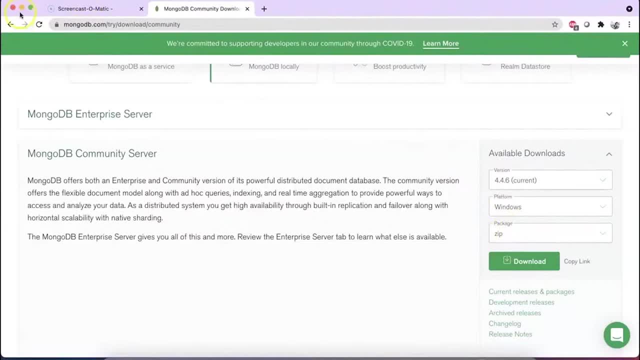 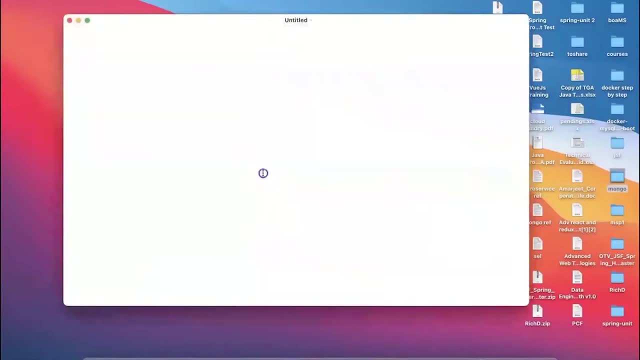 folder inside the bin. so once you download the zip you will find two different type of files are available. let me mention those. so inside the bin folder you will see two files. one is called mongodb- okay, the other file which is available, called mongo. mongodb is to basically start the mongodb. 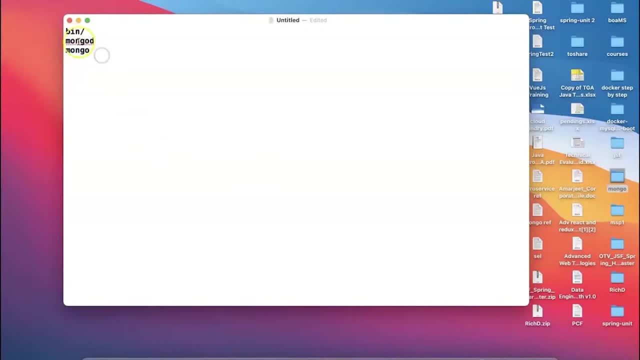 server and the mongodb. mongo is actually the client which will connect with the mongodb clear. so if you are in windows environment, so once you are inside this bin folder of your zip file, you will get the mongodb. so you have to double click on this. it will start a new command prompt. 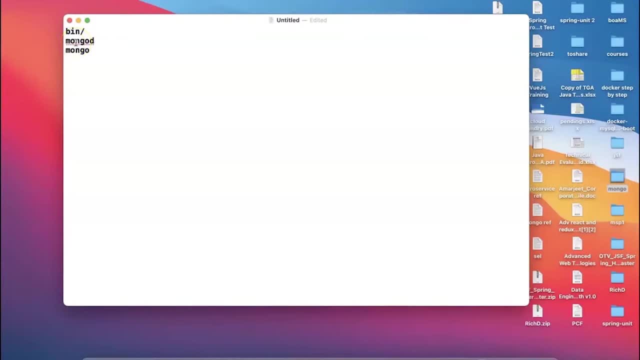 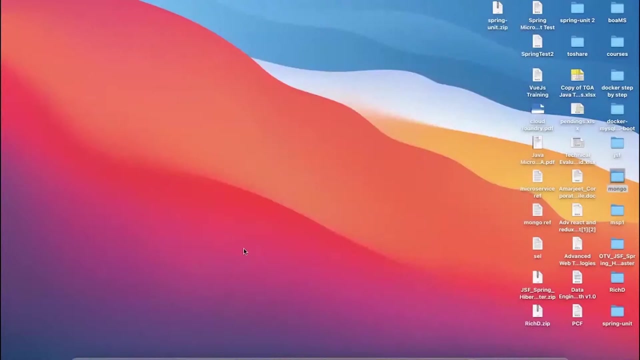 so you do not need to do anything further. just minimize this command prompt and go inside the bin folder again and click on the another binary file called mongo. so it will get start as a client. okay, since i am using the macbook here, the concept is little different about how mongodb can be used, okay. 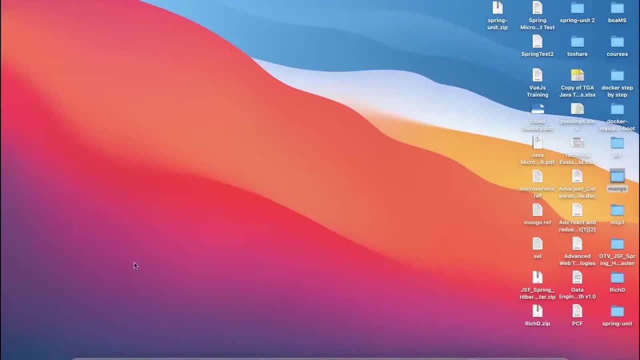 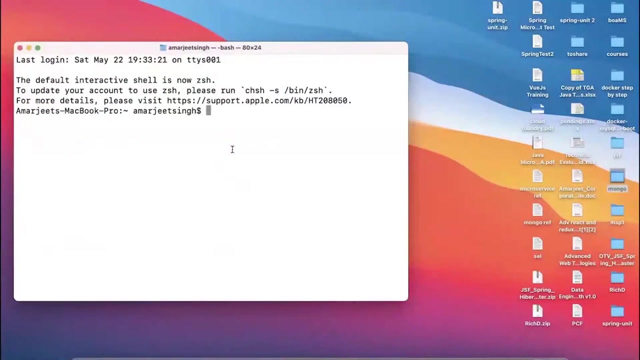 so this is just a basic way of how the mongo is being used into your code. okay, everyone. so now let me show you how to start the mongodb, mongodb, mongodb is a very special way to start with. so here i'll start with my terminal, and here i would like to paste one very simple command to start my. 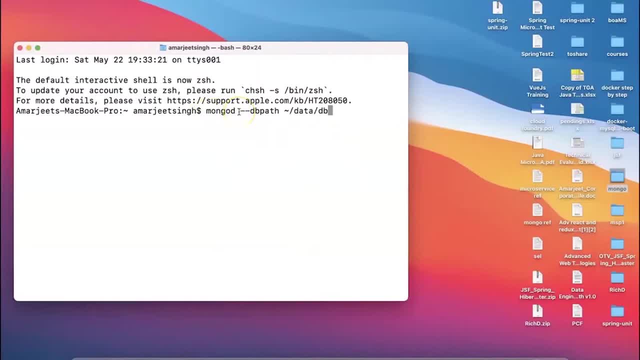 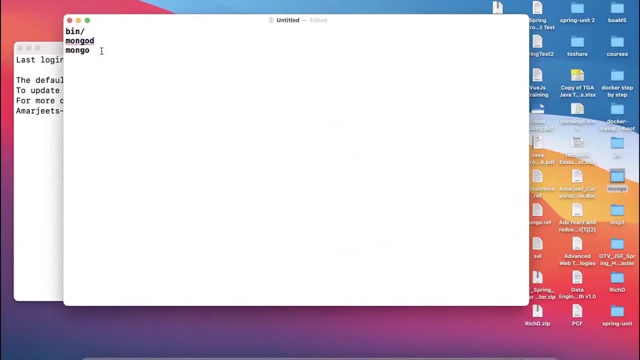 mongodb database that is called mongod and after that you have to say hyphen, hyphen, db path. it is a place where your database will be starting. and one more important thing i forgot to mention: like modi would not start automatically inside your windows machine unless inside your c drive you have to create a new folder name called data. 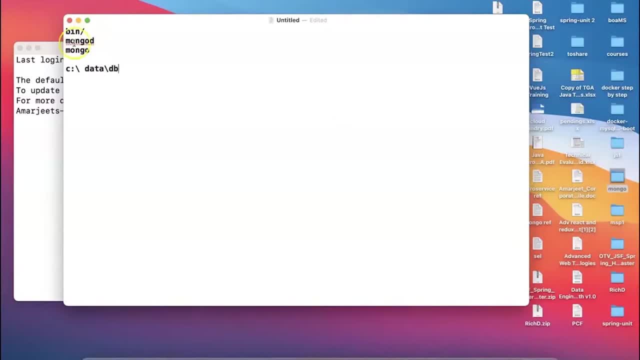 and under this you have to create a new folder name called db, because automatically when the modi starts it looks inside the c drive data, inside the db folder. there your all records will get stored. so do not forget whenever you're trying to use the mongodi. so you must make have. 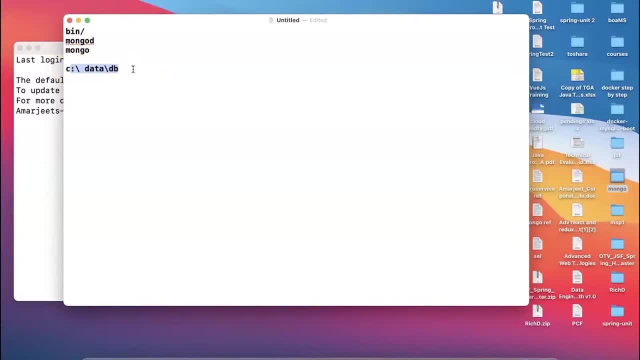 you must have this particular folder structure in place of the mongodb, mongodb, mongodb folder in place in your local machine, otherwise this is not gonna start. every time you start your mongodi without this location, it automatically terminates. so to avoid those, make sure that you have this data db folder ready with you. however, you can also change the location of this particular 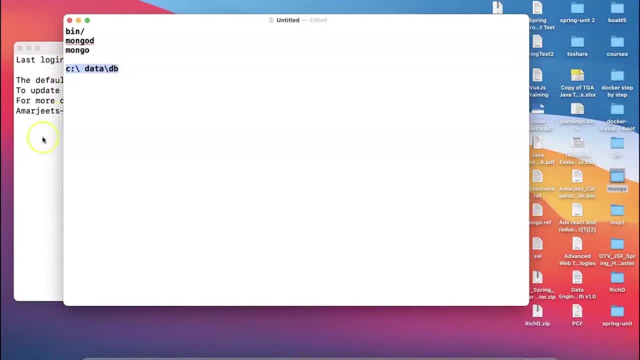 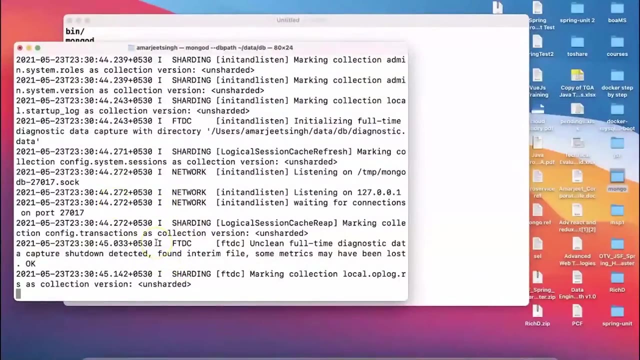 folder structure for which we will discuss it a little later on, but as of now we can see. i'm giving my location. that is called hyphen. hyphen db, path slash data db. i hit enter. you can see. now my mongodb is starting now and since it's stuck, so i have to start the new. 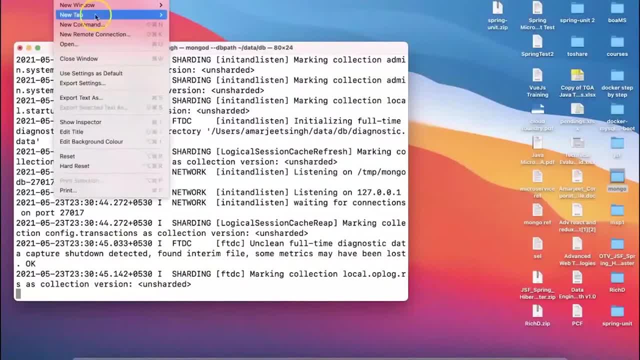 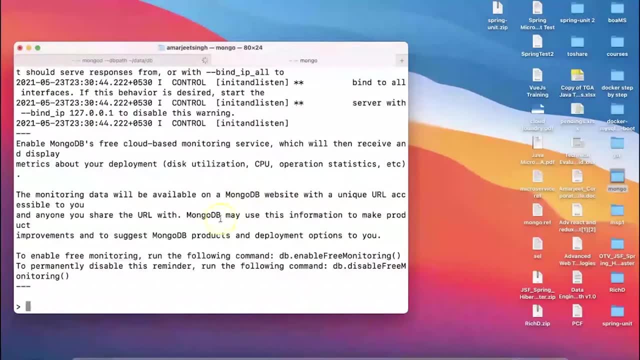 terminal now. so here i open the another tab and type mongo and the modi. type mongo. now you can see it is now connected with my mongodb and now it is ready. that's the first thing you need to remember. okay, now to check which other databases are available to you, so you can just type: show dbs. 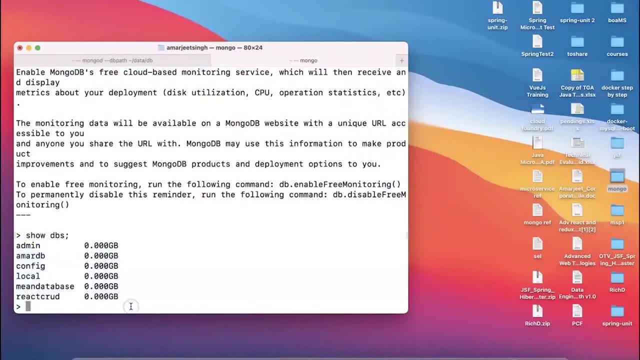 so it will show you the number of databases which are already there inside your existing, newly installed mongodb. but you can go back and create new database too. here you can see some databases are already present. however, you go back and create the new databases into your system and to create 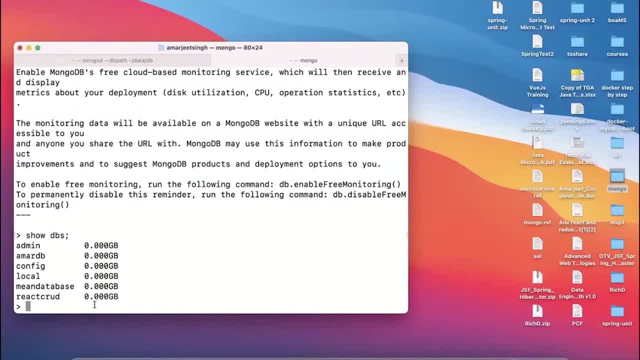 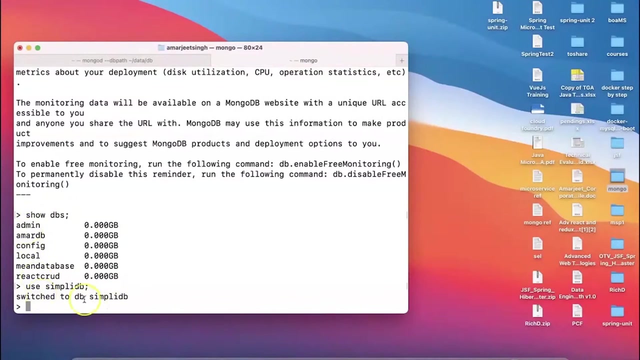 this database. we have a very simple option available here, name call use simply db. if i say use simply db, it automatically creates this database and take you inside. let's see now you can see. you say use simply db, it automatically creates- though it is not there, but automatically takes you in while creating those. okay, so that means you are. 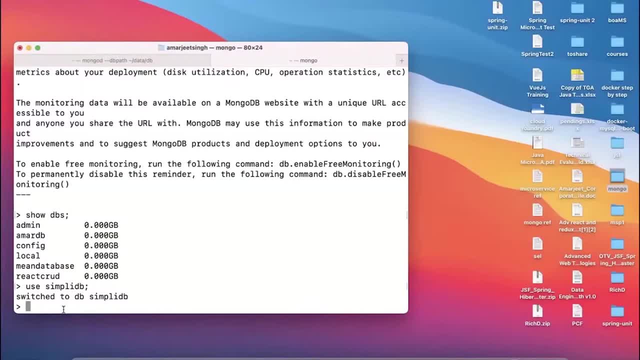 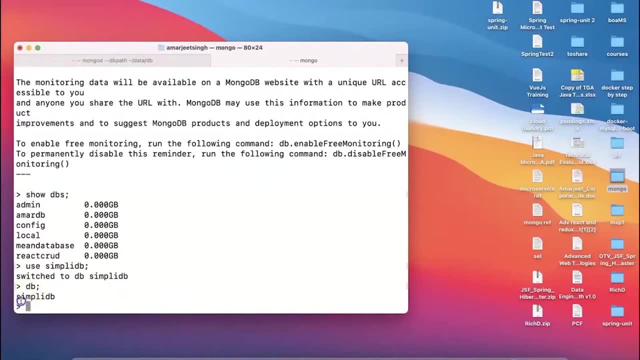 in current database name called simply db. so if you are not sure which database you are in, so you can just type dbs or db and it will show you that your current database is simply db. that's it. so your database is set and we are all good to go ahead with our next level development. hello everybody. 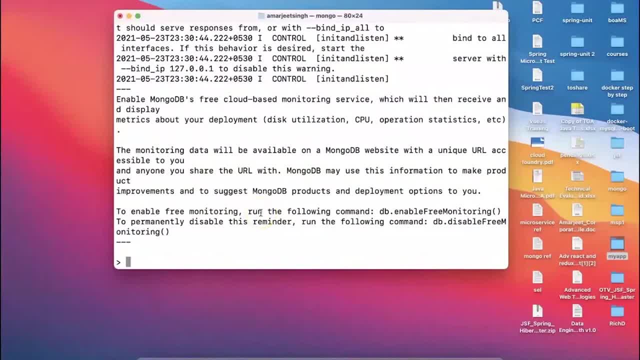 and welcome back. in the previous videos you have seen like how to create a database and how to identify whether my database is there or not. so, if you remember, previously we have created our database using use keyword. so if i just see my databases, which we have created is last. 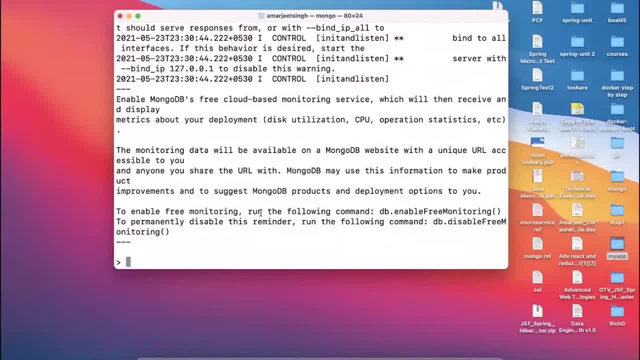 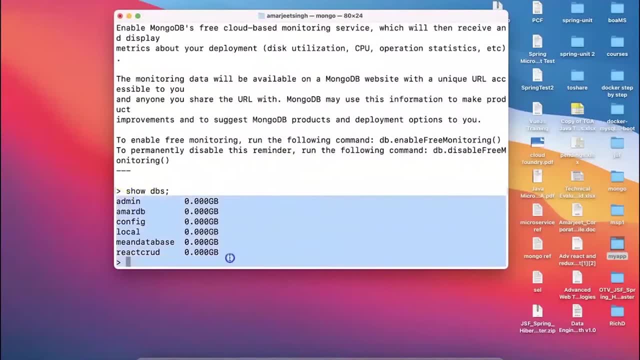 time. so how we can check this out, we can say: show space dbs- okay, so you can see we have a got database list, but we do not have any database which we have created last time, so we cannot create the db in here. something is missing. we could be creating database according to this list. 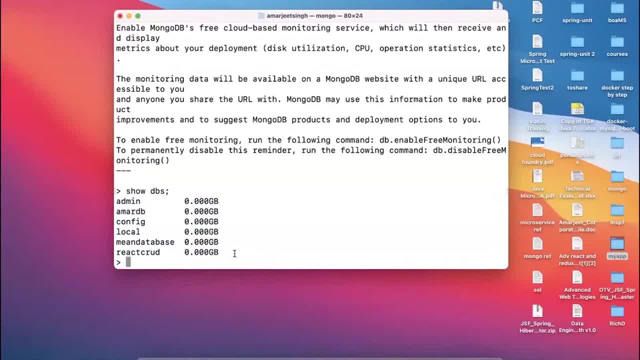 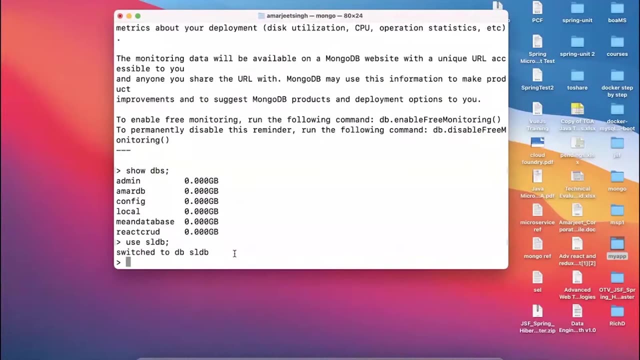 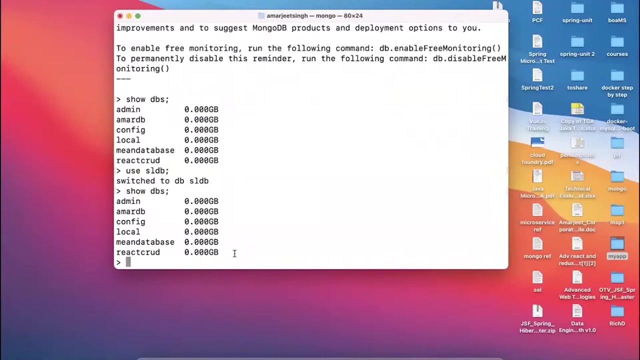 time is registered here. That's quite surprising, because when we have created our database it should be listed here, but it is not. Let's do one more time. I am saying use SLDB and I am saying switch to SLDB Now when I say once again, show DBS. so I still don't see. 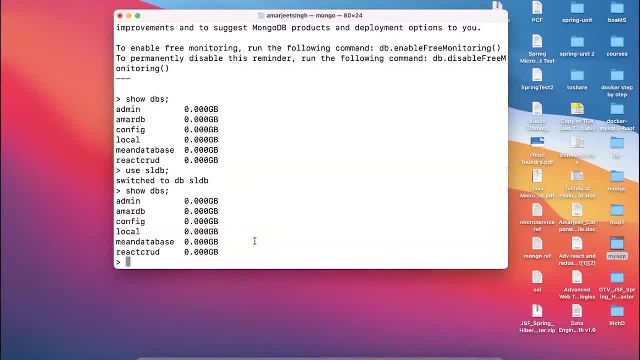 my database is listed here. There is a reason. The reason is, according to the MongoDB rule, unless we have minimum one record or collection stored inside my MongoDB, it really can't show in the list. Now I want to tell you about a few important things Now here, when we talk. 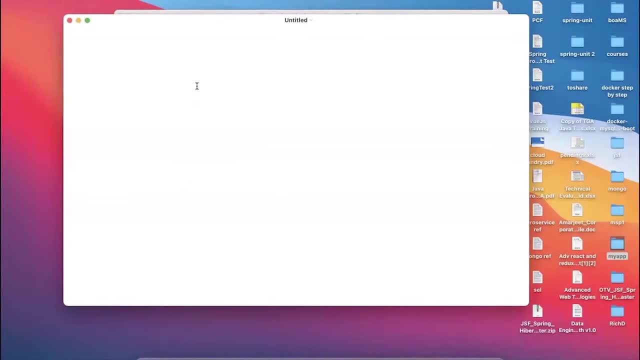 about called MongoDB. in this MongoDB, compared to the relational database, here the table, which is actually in RDBMS- it is called. here it is called collection. Okay, DB is still called DB here. Okay, That means the database will be still called database, but row what. you use this word in a traditional 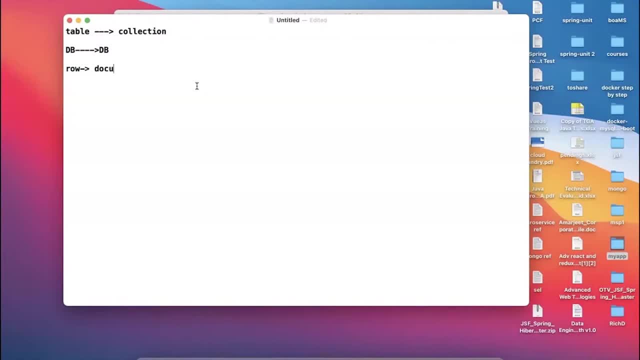 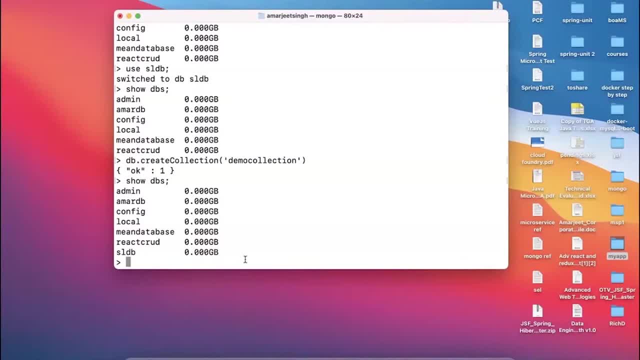 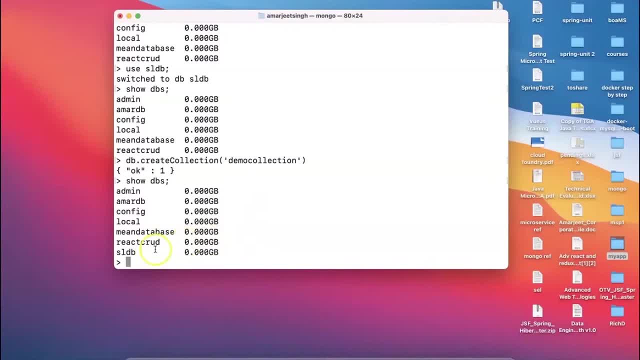 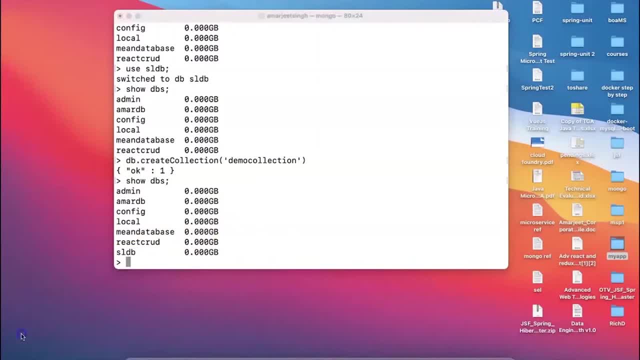 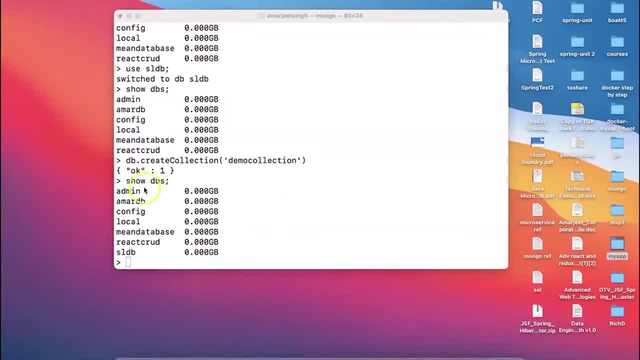 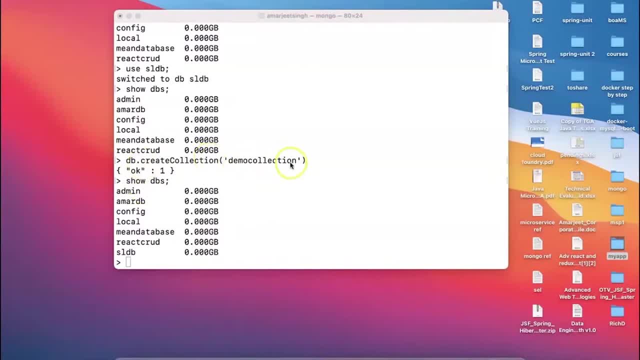 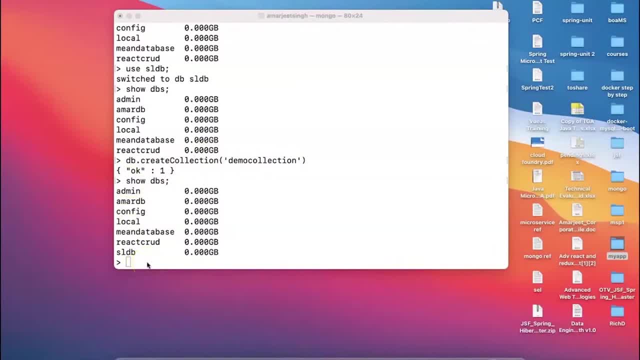 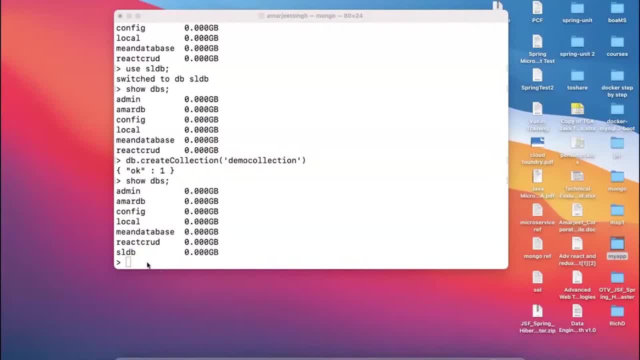 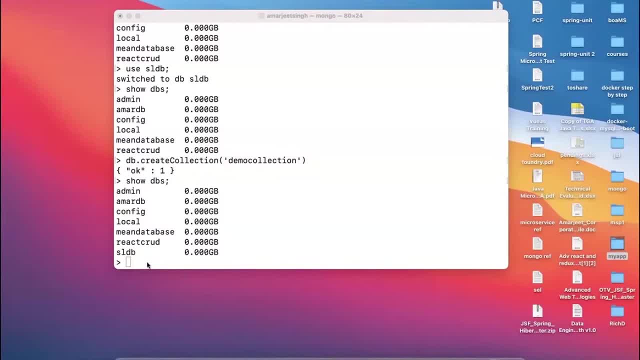 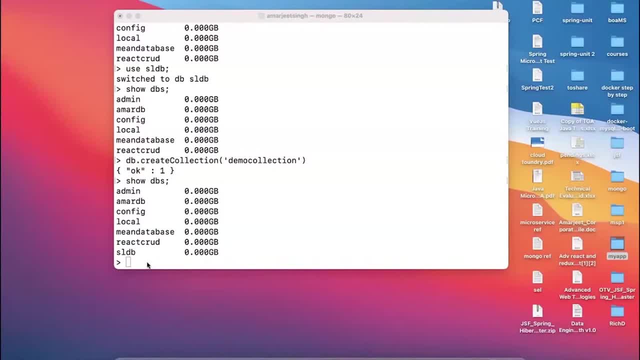 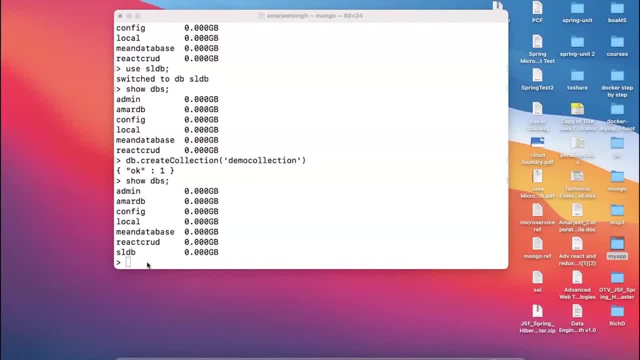 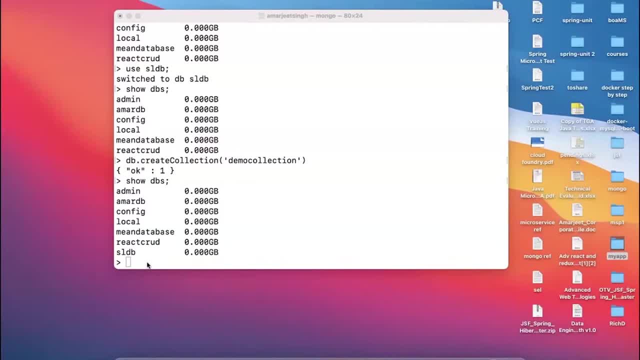 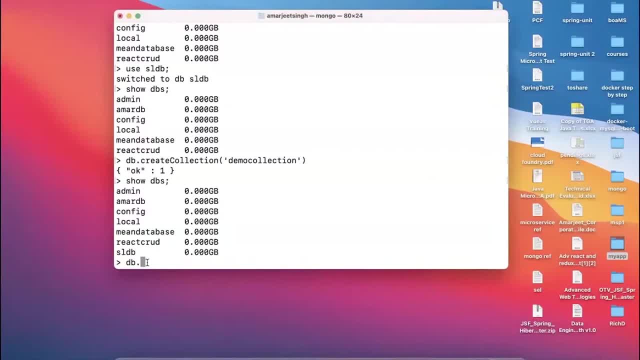 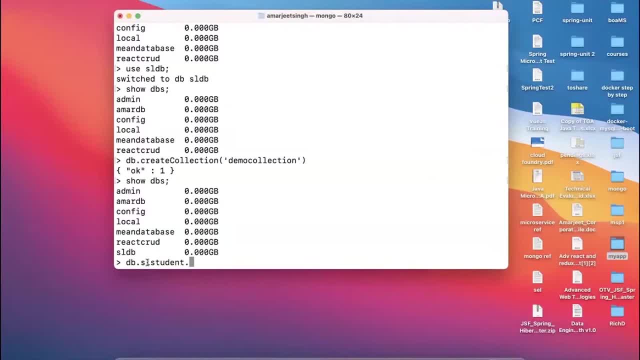 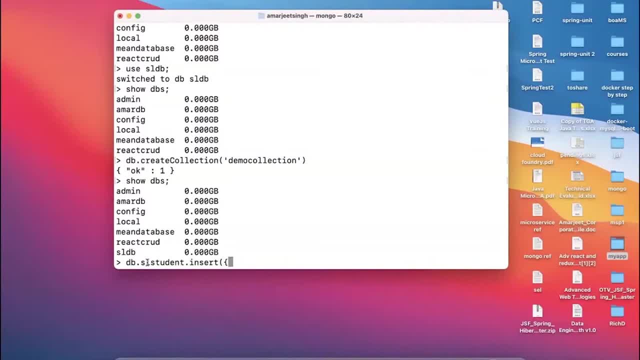 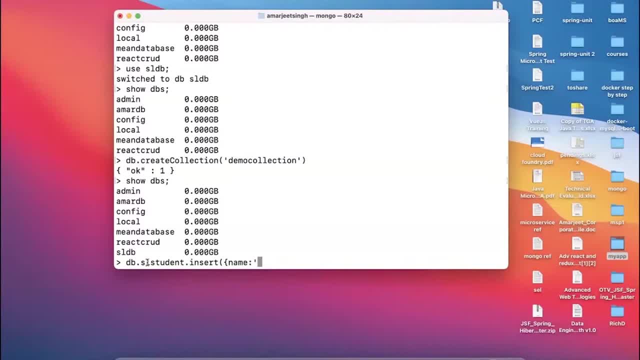 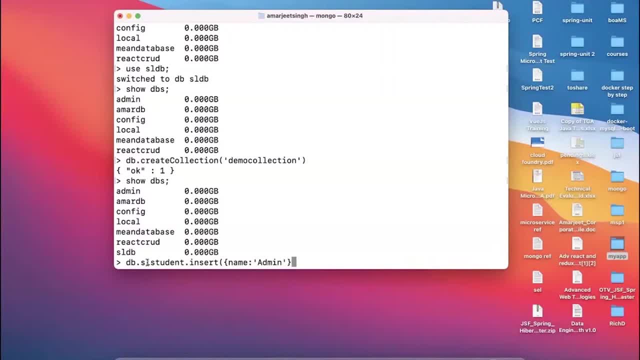 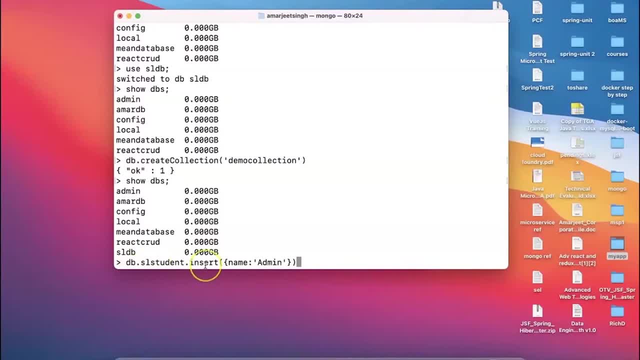 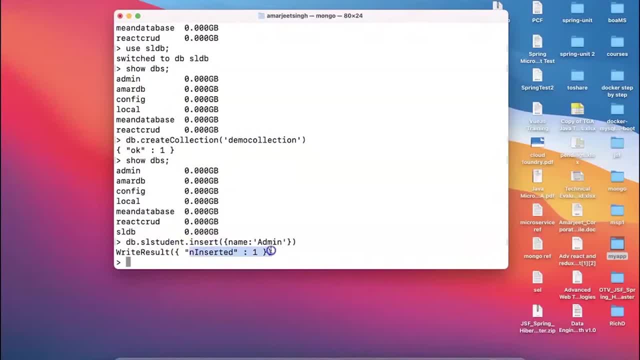 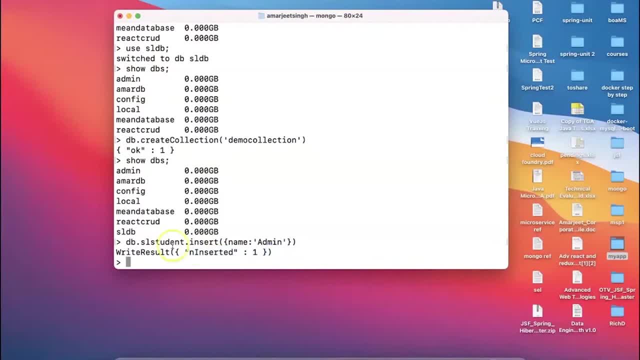 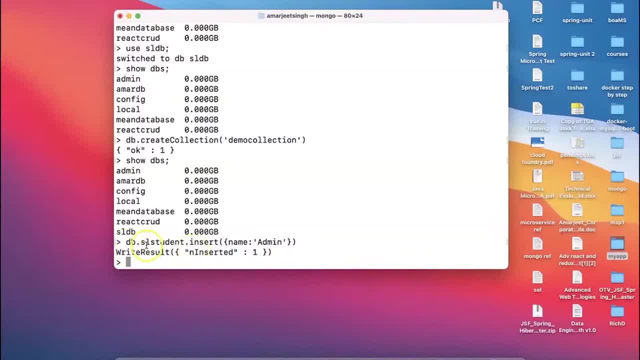 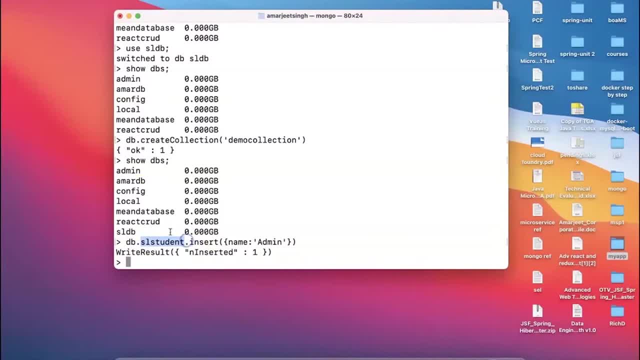 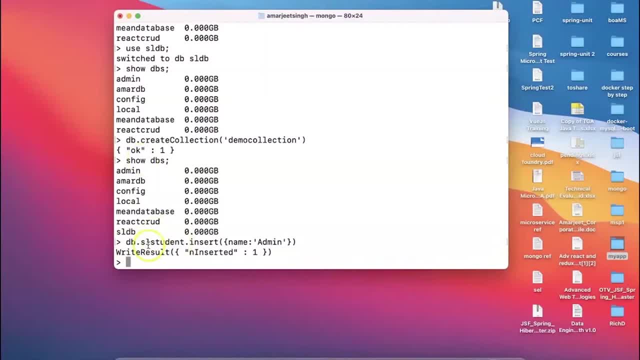 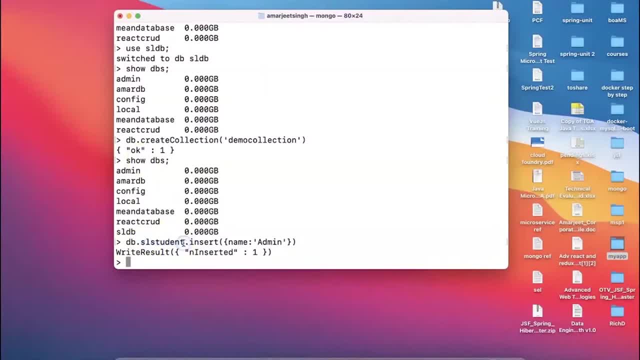 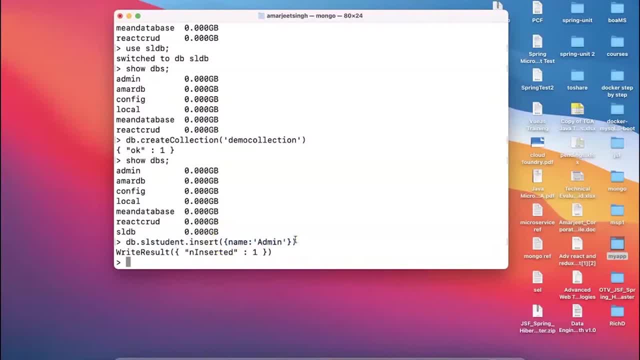 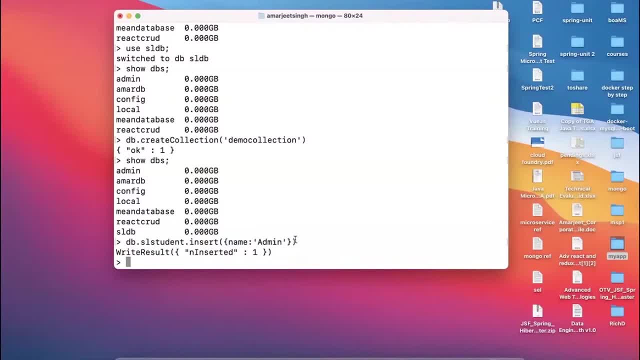 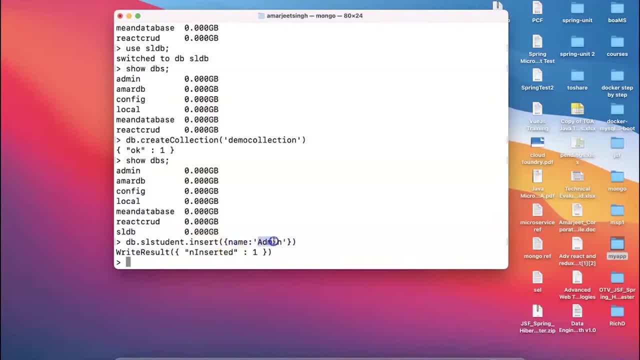 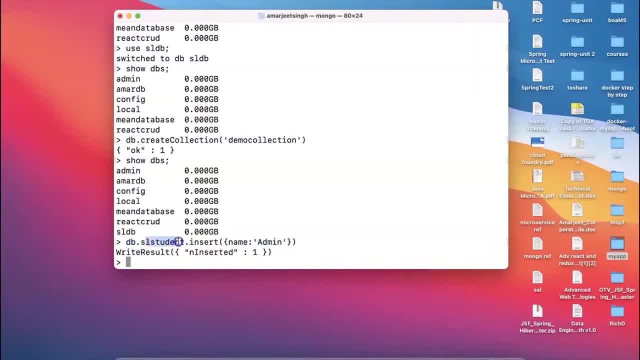 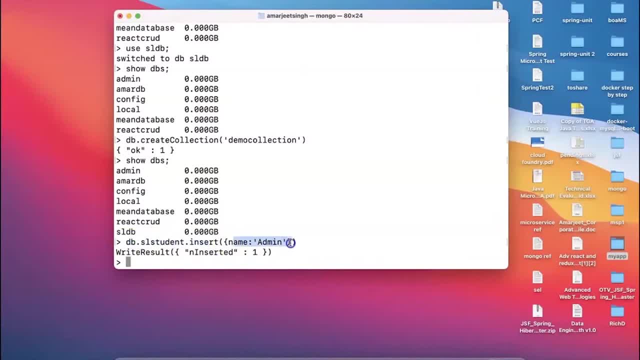 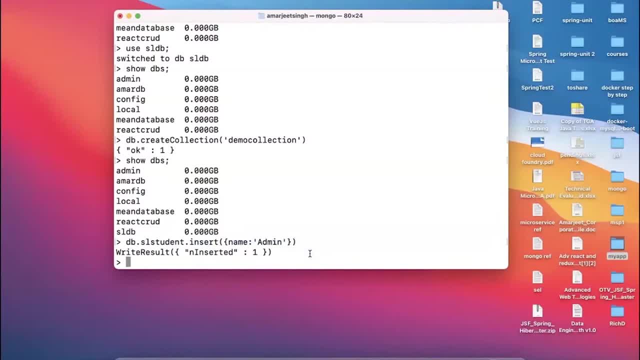 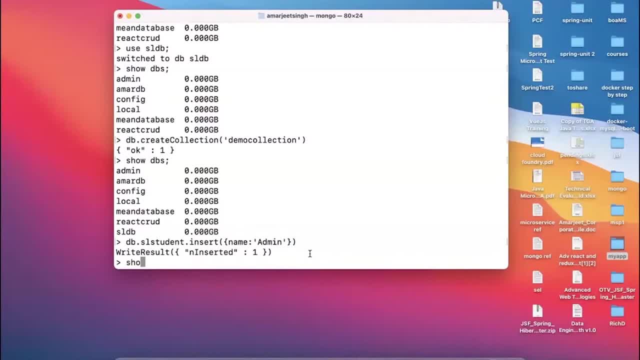 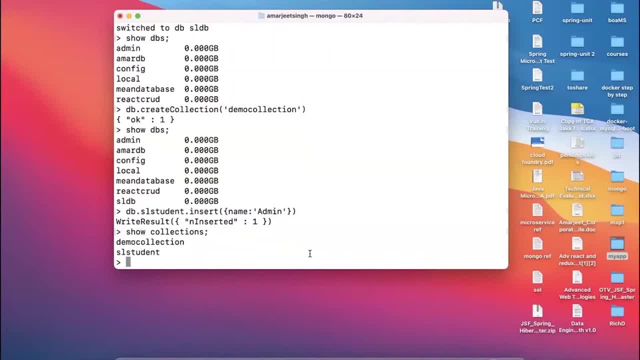 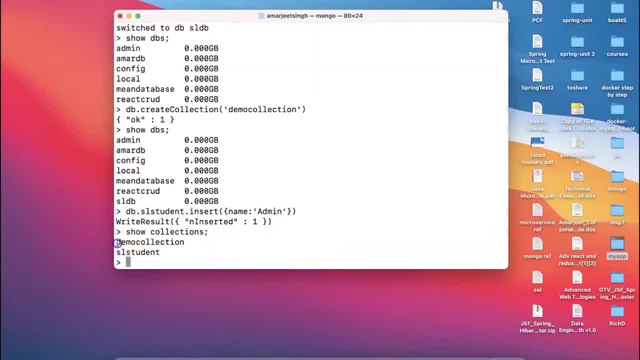 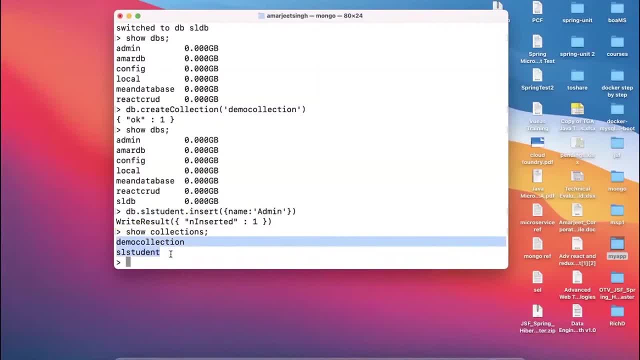 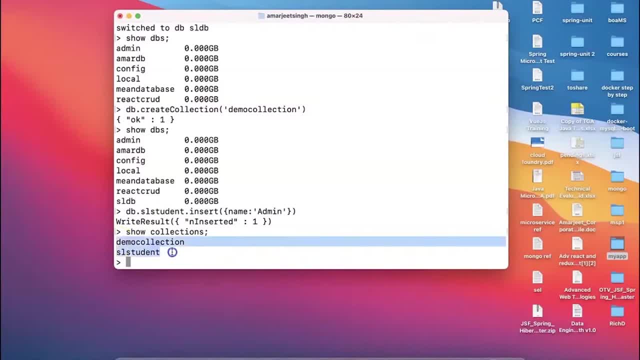 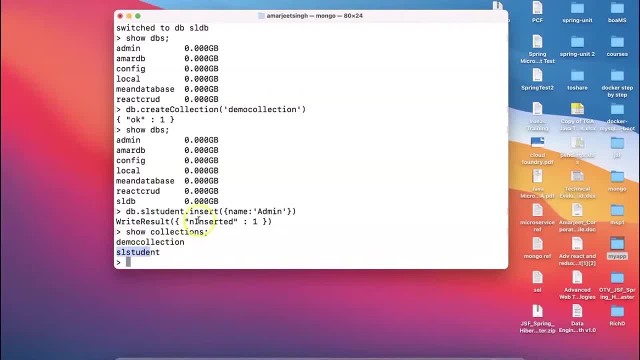 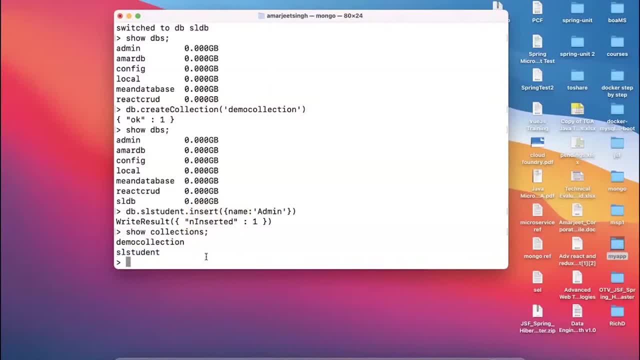 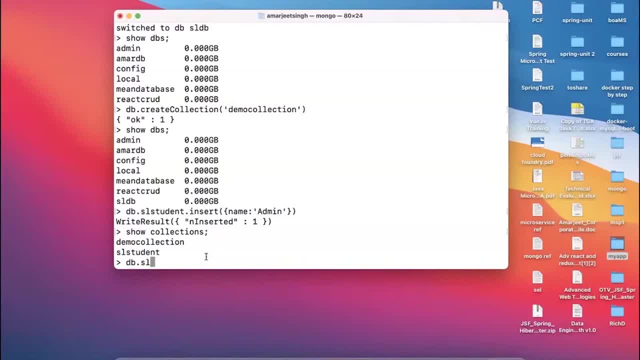 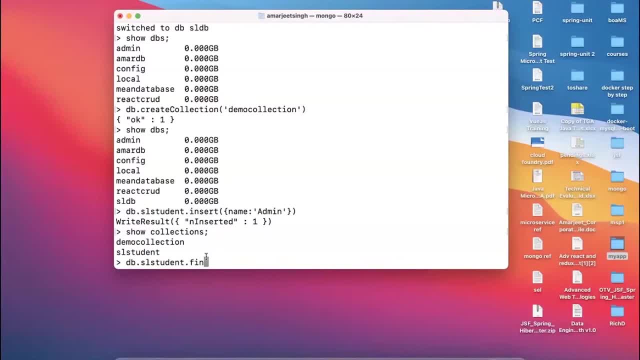 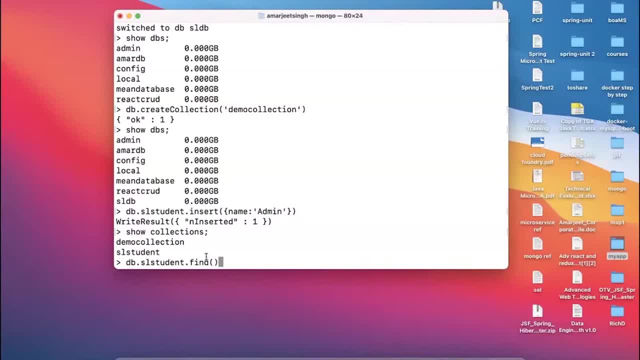 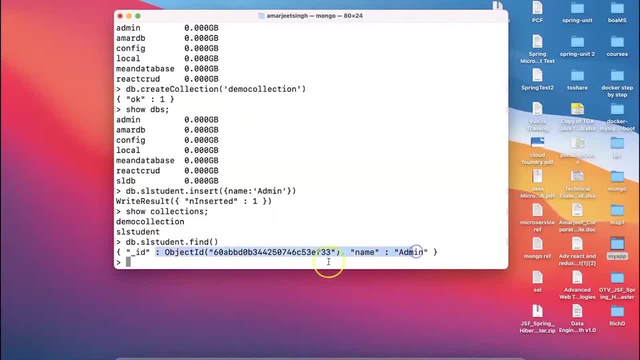 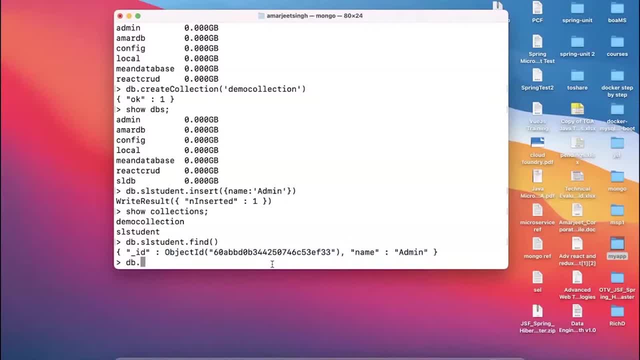 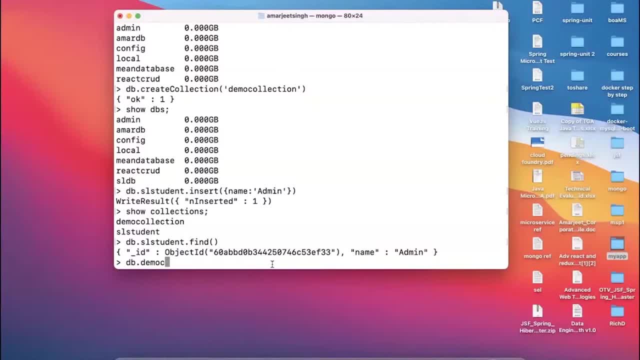 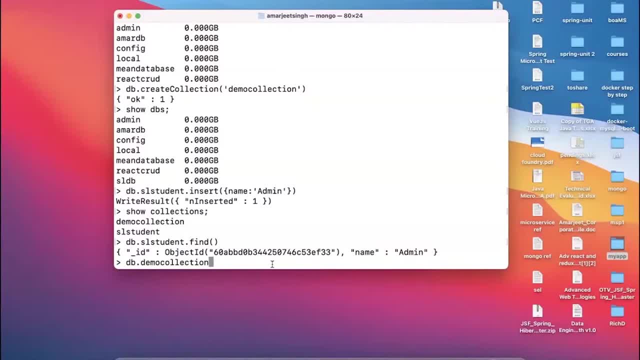 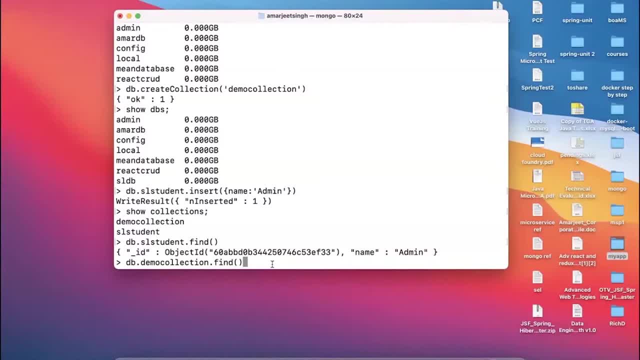 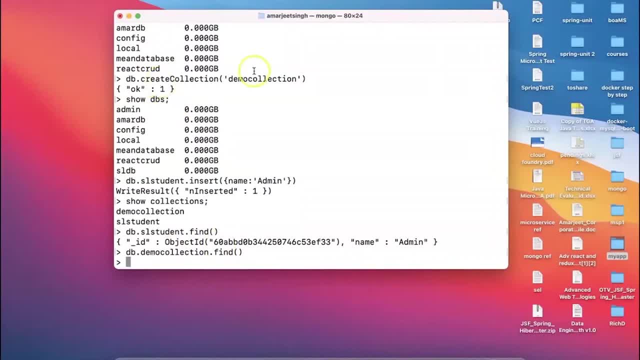 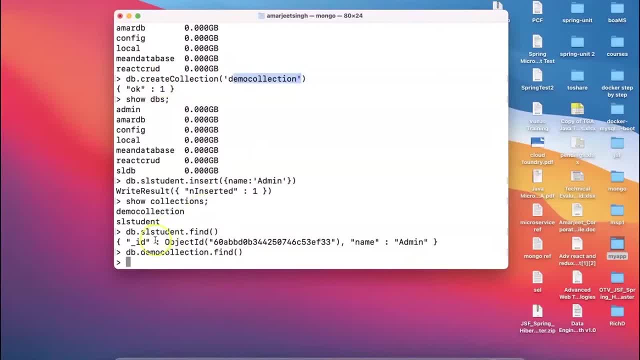 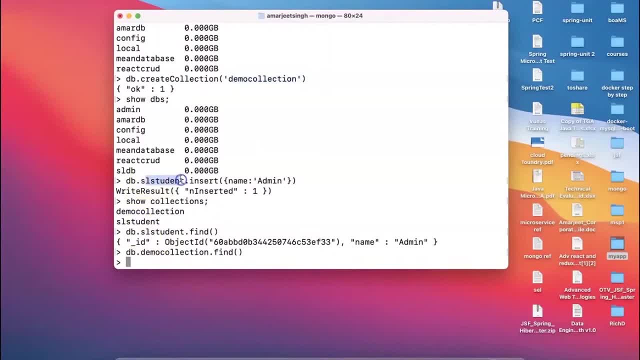 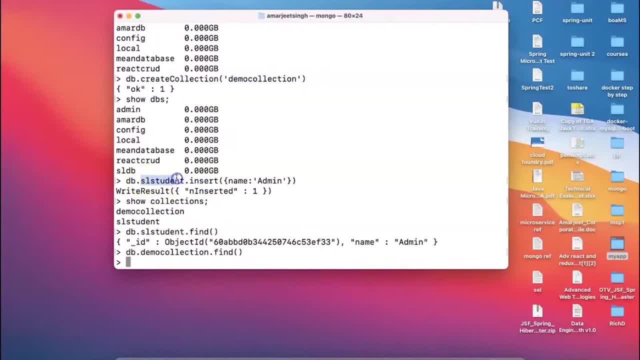 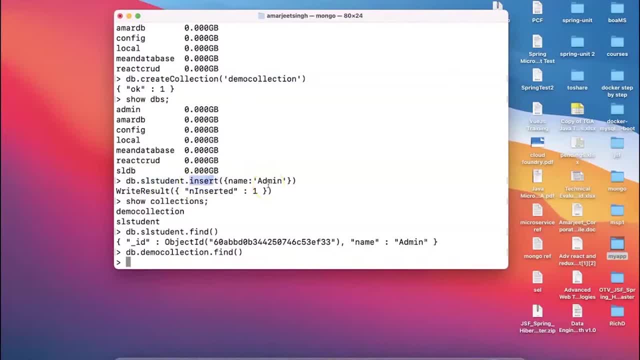 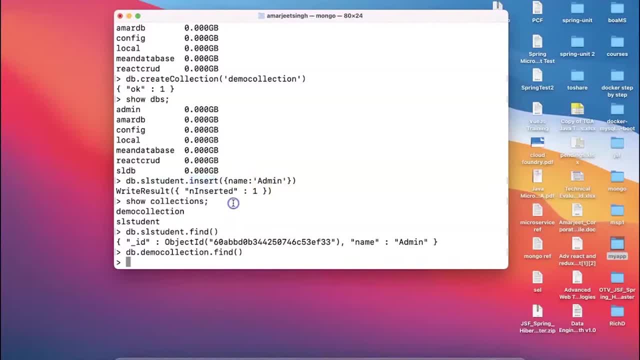 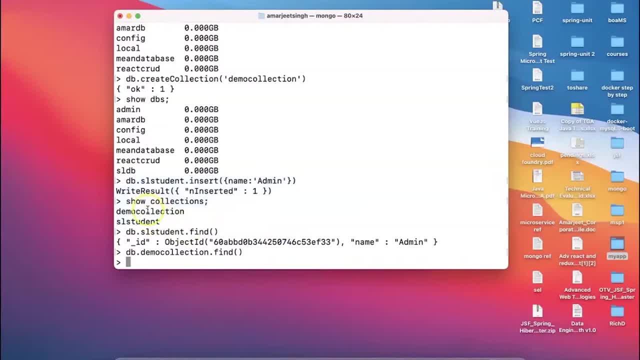 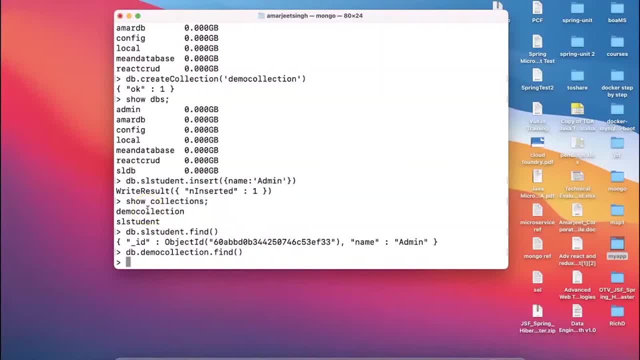 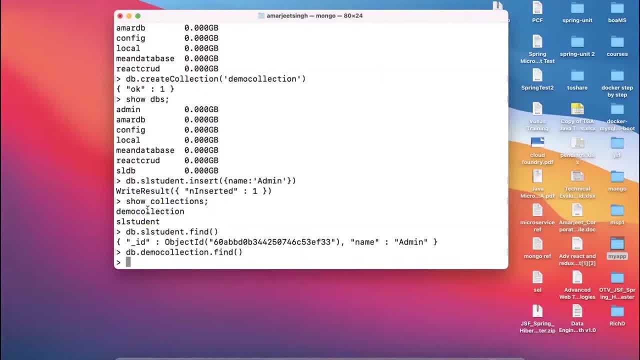 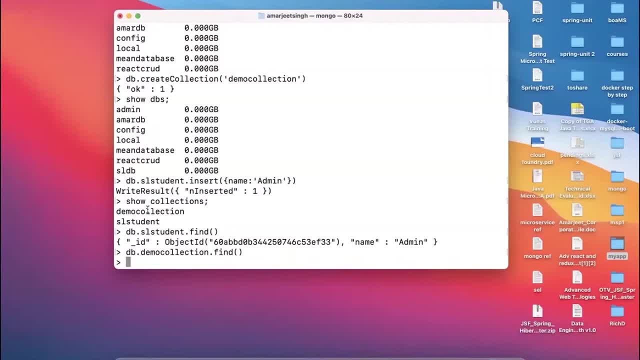 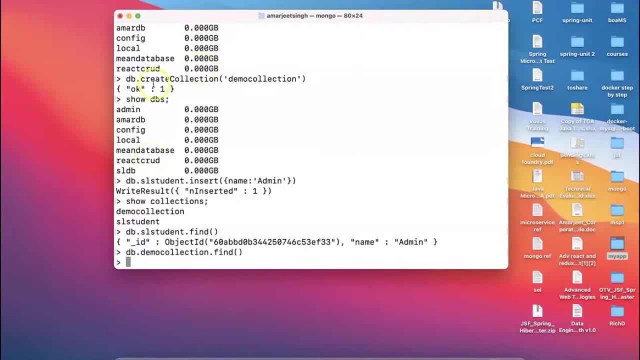 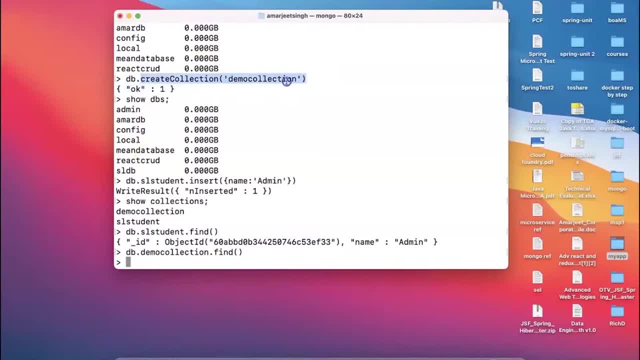 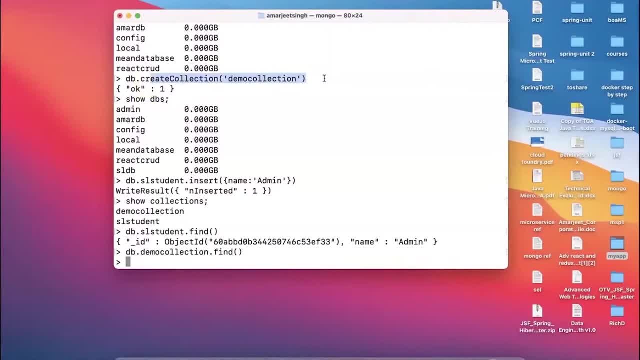 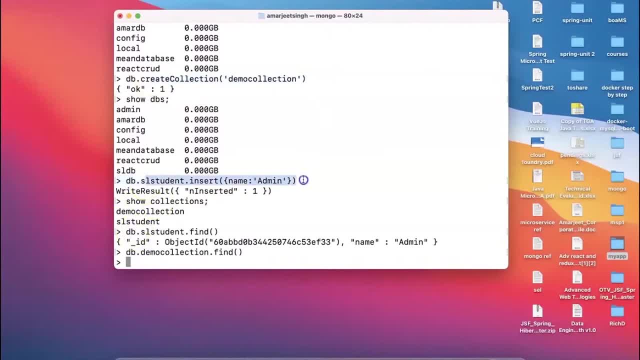 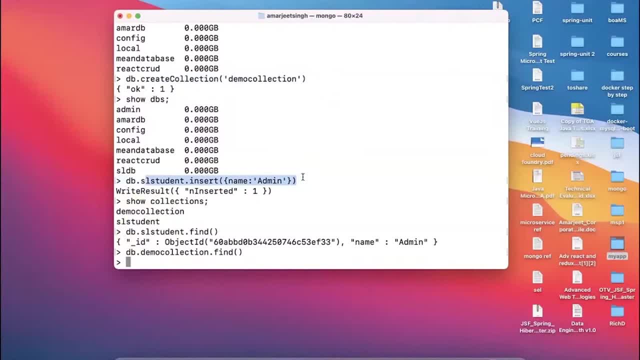 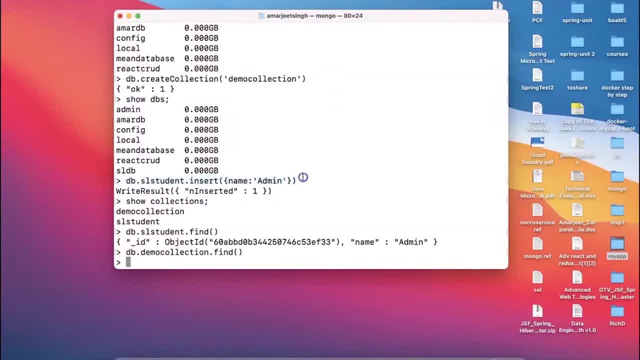 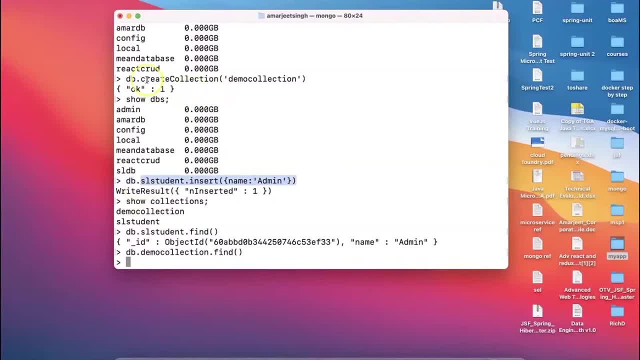 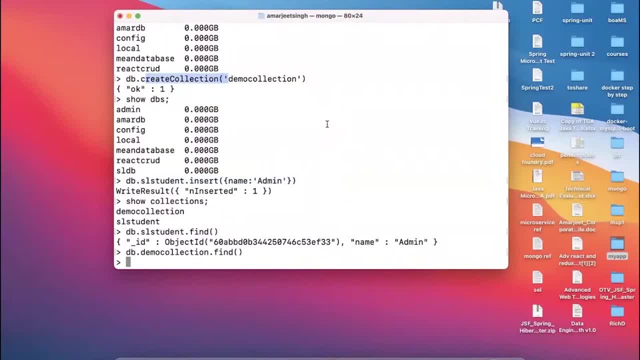 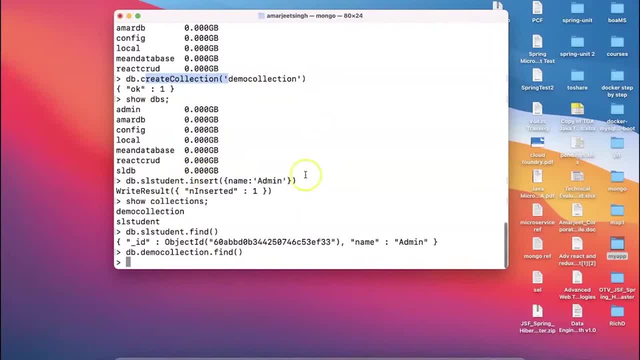 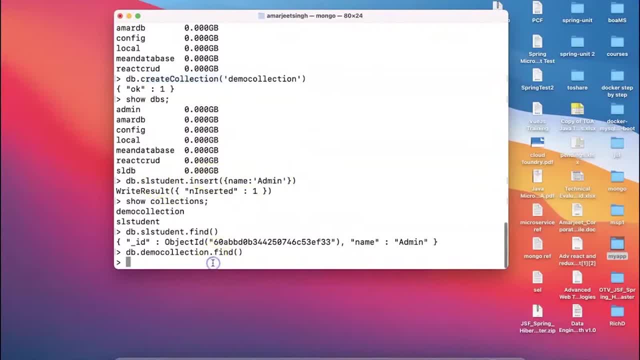 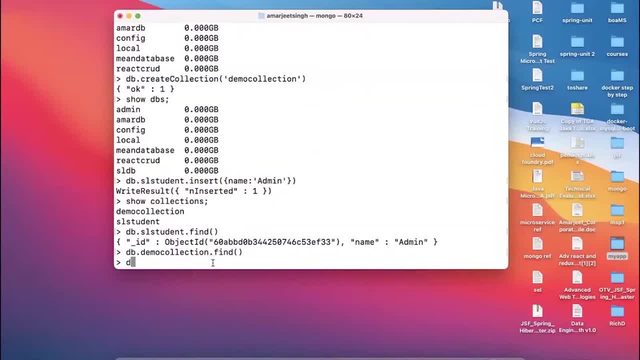 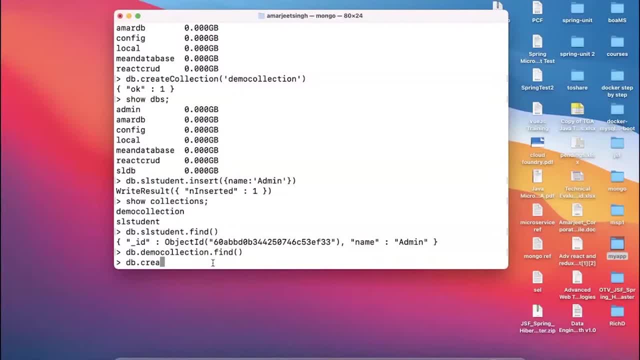 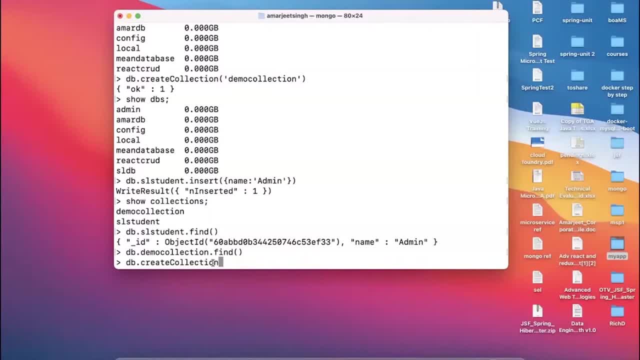 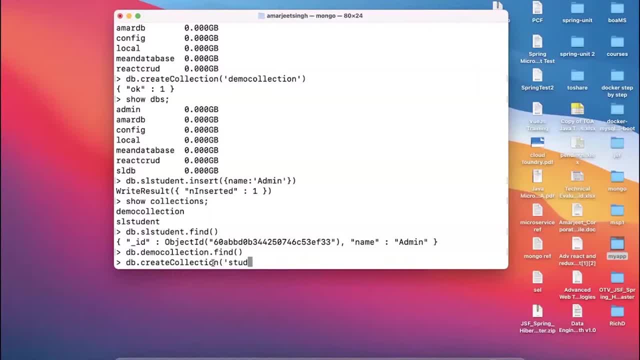 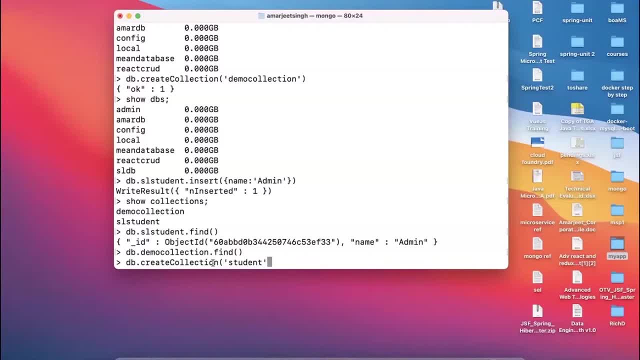 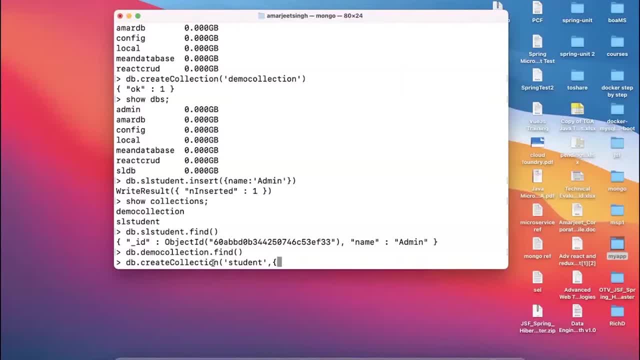 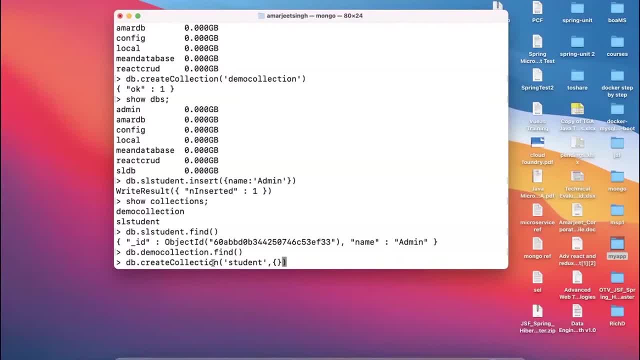 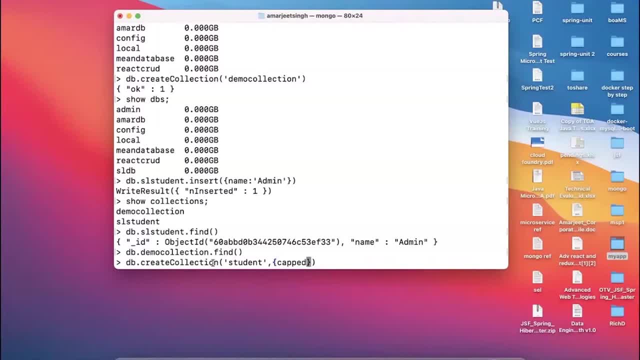 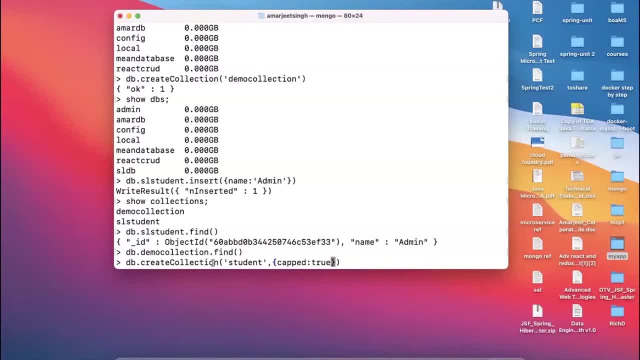 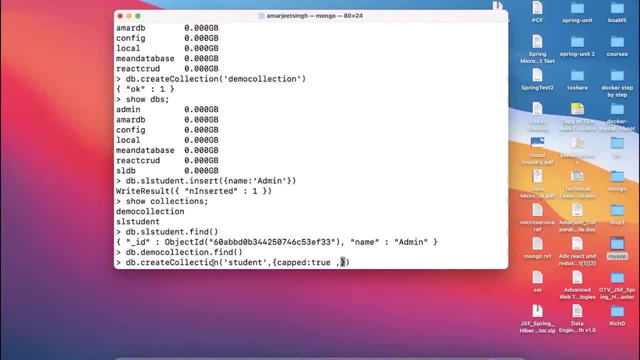 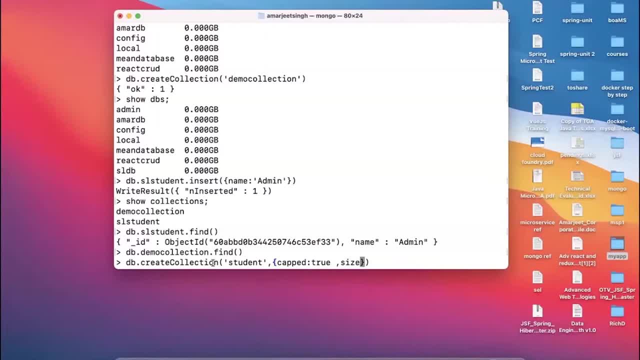 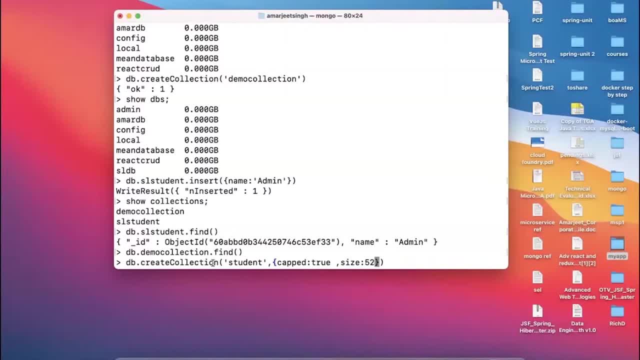 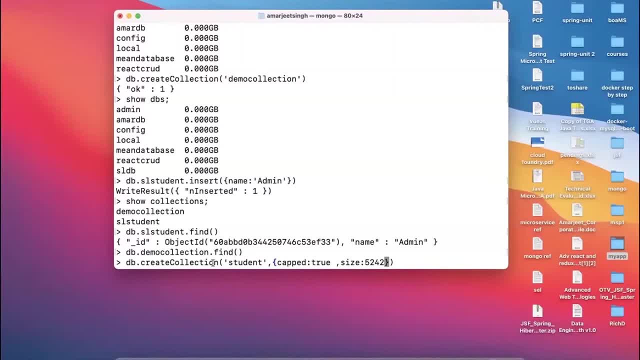 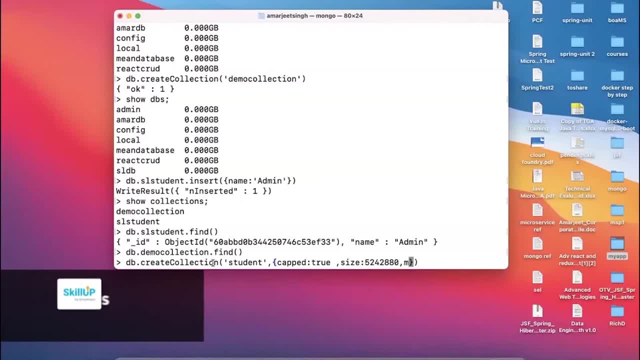 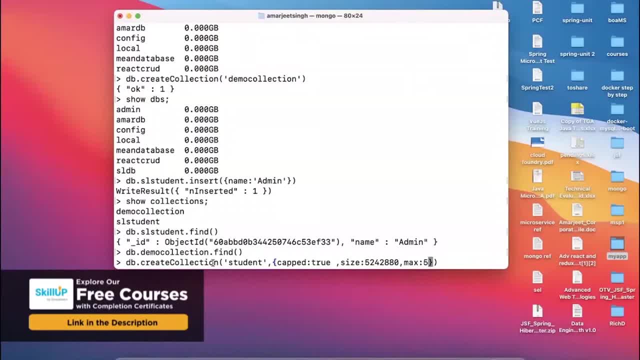 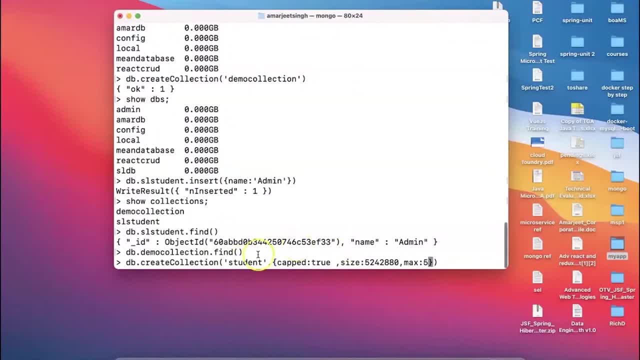 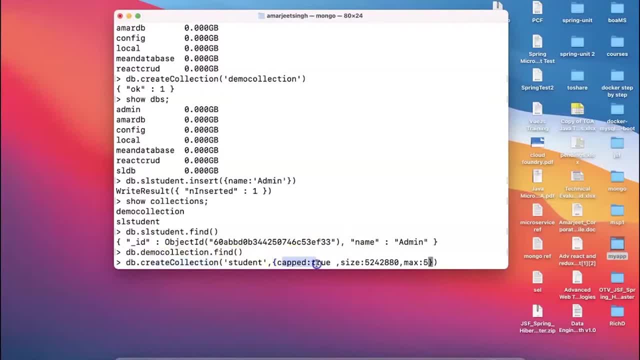 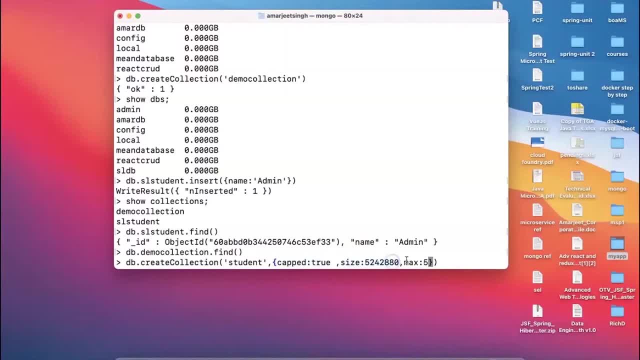 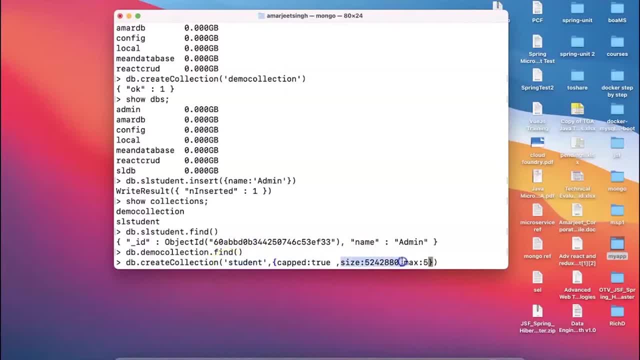 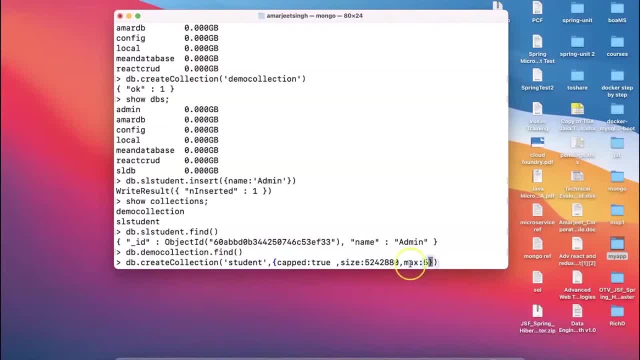 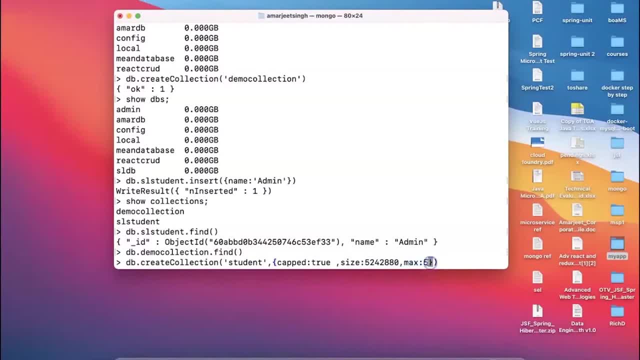 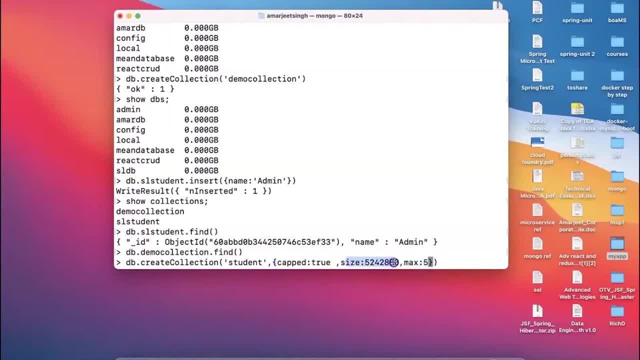 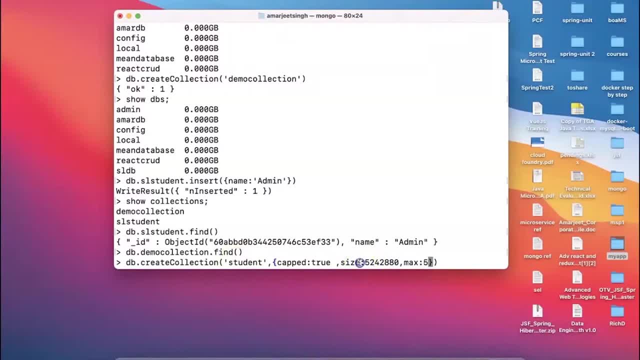 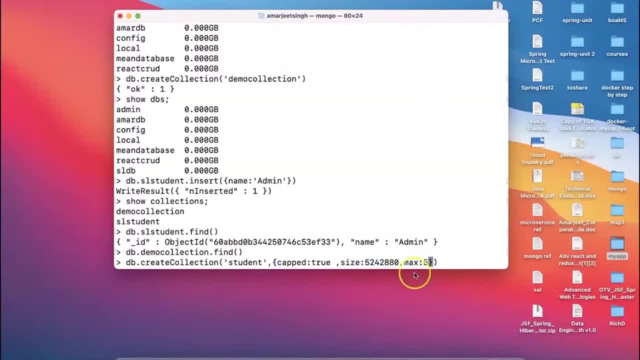 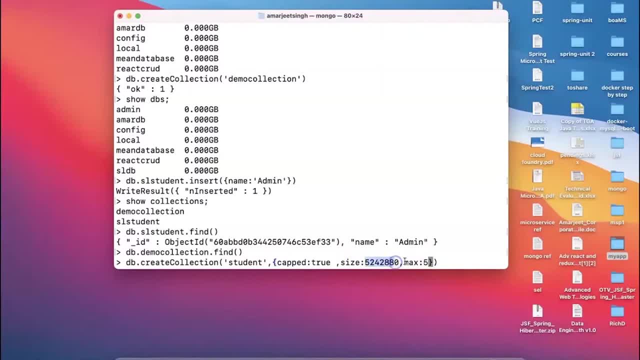 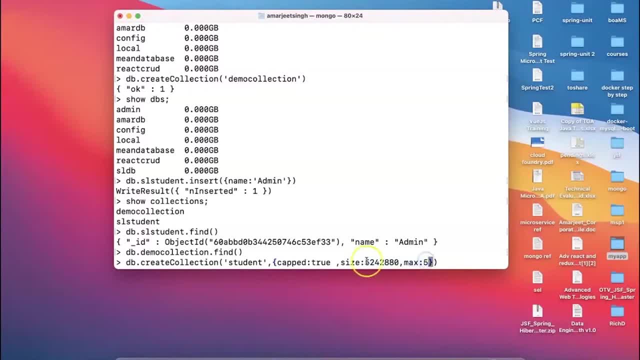 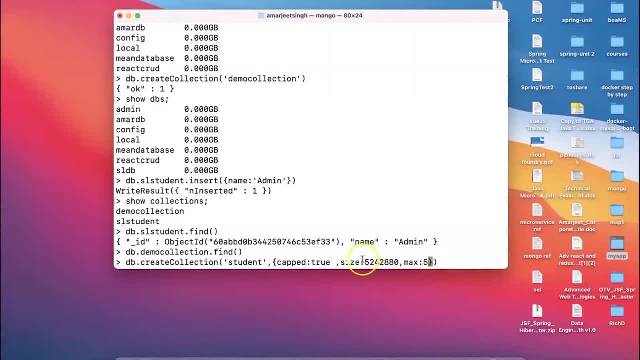 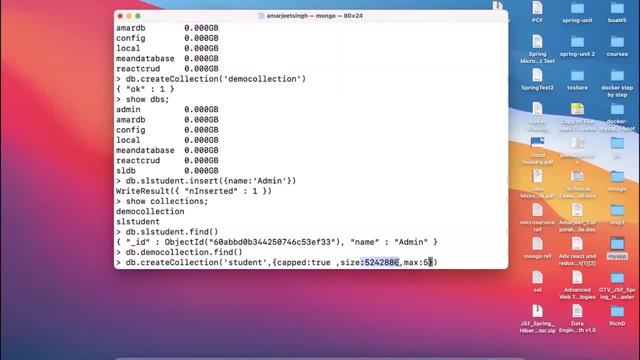 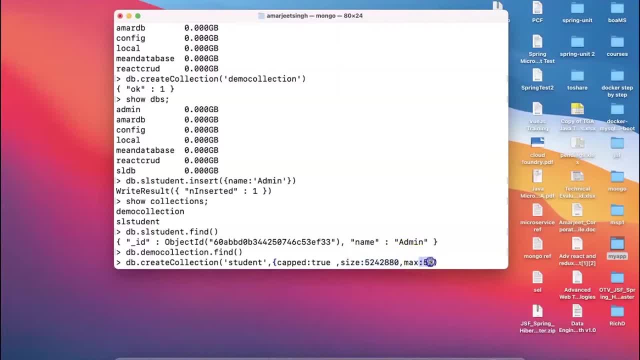 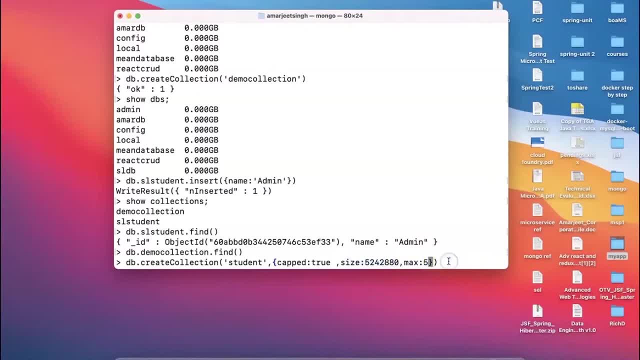 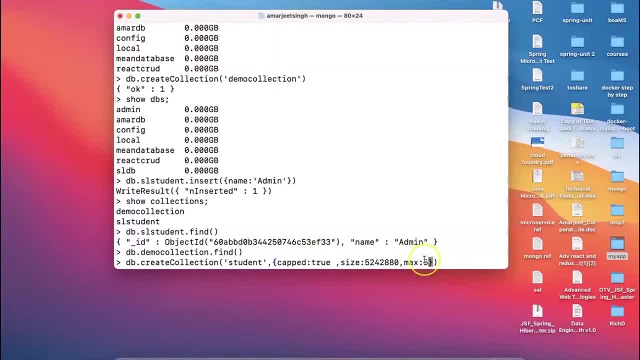 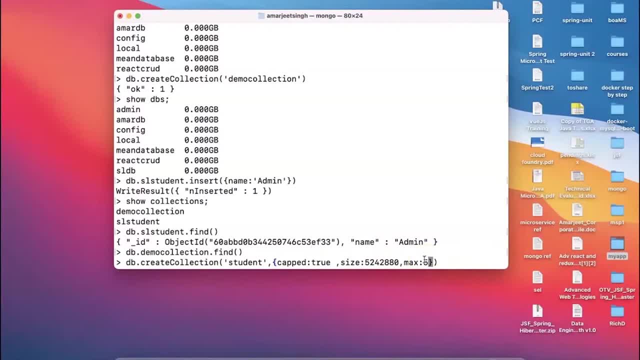 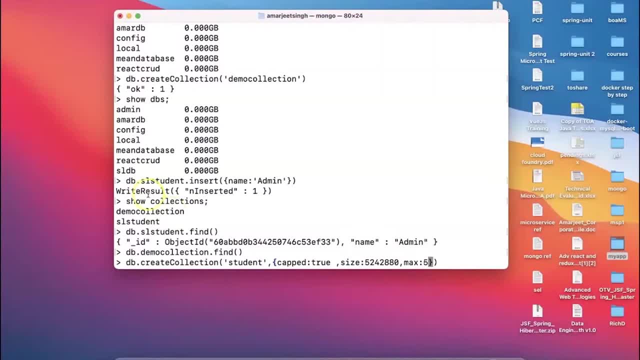 trying to say dbcreateCollection. This option is not possible when you're trying to use this. So that's the benefit of having this dbcreateCollection, and this is what we always recommend. Well, now we would like to talk about our next feature here inside the same. 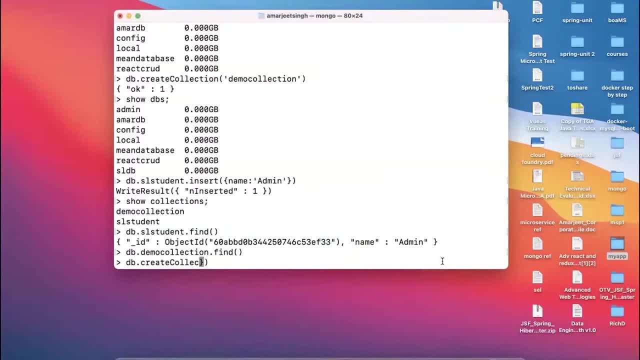 MongoDB. So we now know how to create a collection, how to create a database and how to switch from one database to another database. Now we will tell you, like, how to insert a document. So far, we have already seen how to insert a document inside the MongoDB. Now we would. 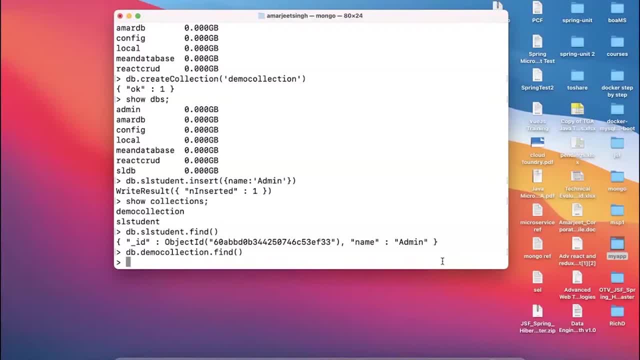 like to also show you how we can insert the documents using multiple techniques. So remember one thing: MongoDB comes with two different types of documents. One is called relational document and second is called embedded document. Mostly, while working with MongoDB, we always recommend you to use embedded documents, because that 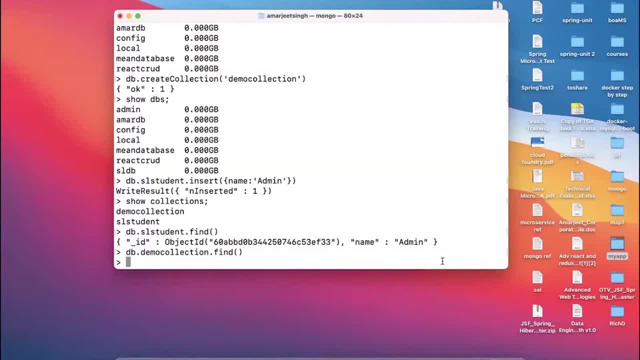 helps you to scale up your application without any hurdle. Okay, the embedded documents means what that means? the, I would say, the parent record as well as the child records, both stores in the same location. Fine, So how exactly that is? let's take a look about this example. 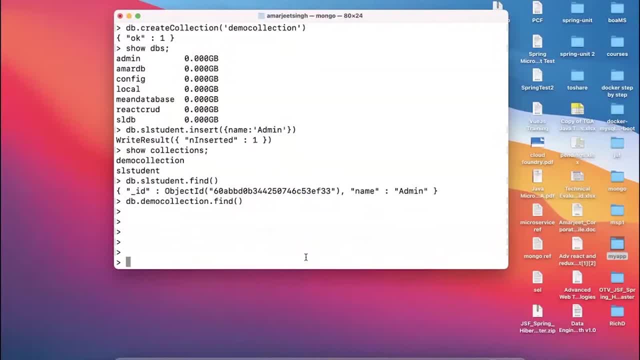 Here we would like to insert some records by saying dbstudent. I do not have a student collection, but I'm just telling you dbstudentinsert. Here we would like to add some records. I'm trying to say the registration number. registration number, I'm just saying one, two, three, four. five, six, seven, eight, nine, 10,, 11,, 12,, 13,, 14,, 15,, 16,, 17,, 18,, 19,, 20,, 21,, 22,, 23,, 24,, 25,. 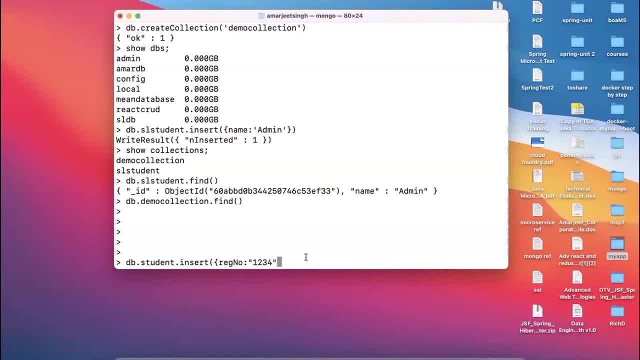 26,, 27,, 28,, 29,, 30. You can give anything. Now, the next one we will talk about called name. This name, we can say student one, followed by the next one. I'm talking about which courses? 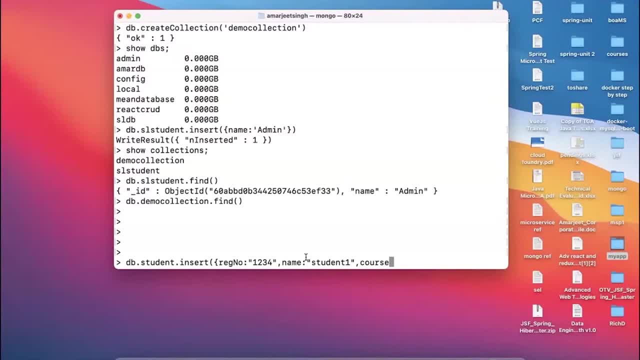 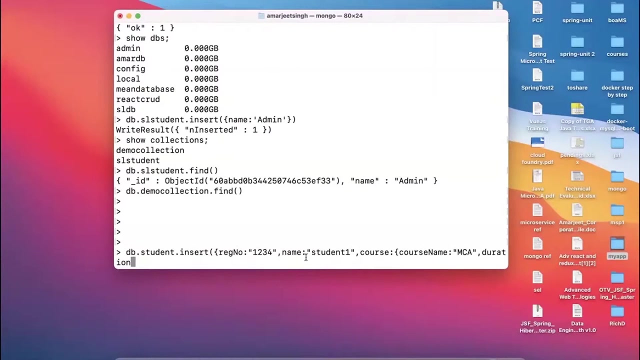 student has registered. So we can say course. Inside this course, we would like to say the course name. Let's say course name, Okay, name. we are giving the course name called MCA- okay, followed by another property called duration- okay, I'm giving this. duration is called three years, like. 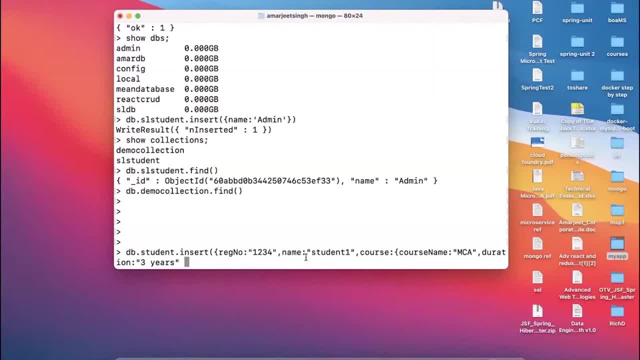 that after that, this curly braces is closing. that means, see, the idea is like you see, the course is an embedded document because from course, you have a few more properties, like, in course, name and duration. I'm closing this and starting the another property and that is called address. okay, sorry, let me. 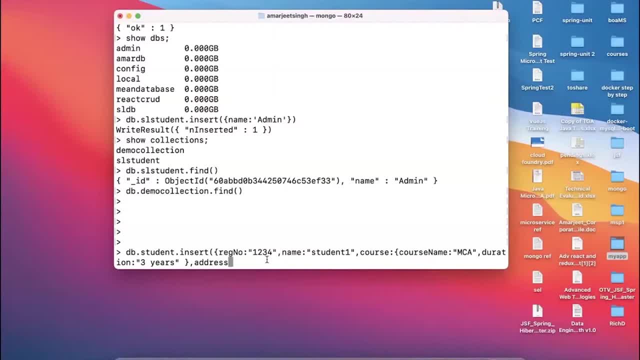 remove from here and from actress and address. we can say one more curly braces and insert this. I just we can say city and address, we can say city and inside this address we can say city and inside this address we can say city. I am giving the name called what bangalore, the another one we are using that is called 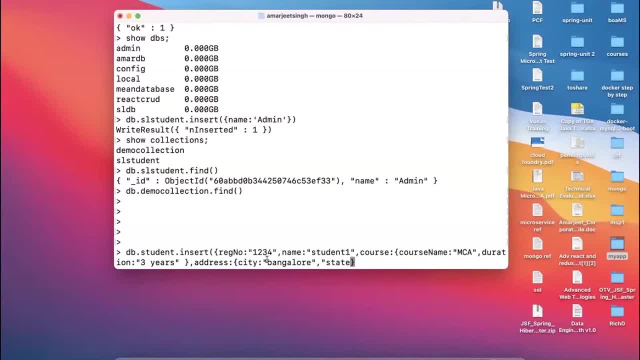 state. let me remove this state, colon ka. ok, and the third property we are using that is known as called country. here you are saying: ie, that is called india, so it is closing here. ok, and it is closing here. so the inner document and outer document, both are closed. hit enter. 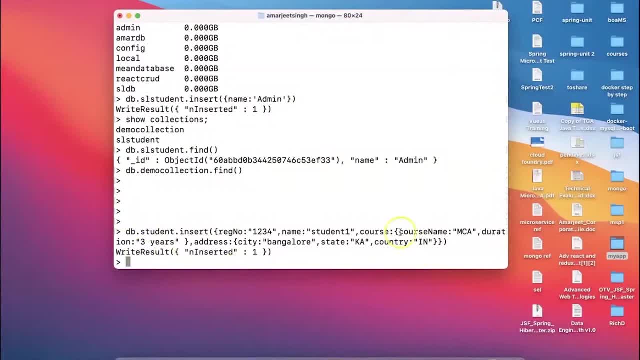 and now you can see the records are inserted. one thing you might notice: the course and the address. these two are embedded documents and they do not have any primary key that is the primary key of its own. instead, the course and address: both are directly dependent on the student object or the student database. so i will say: student, have the registration. 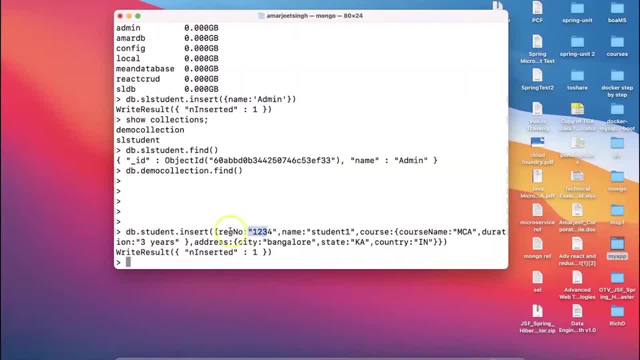 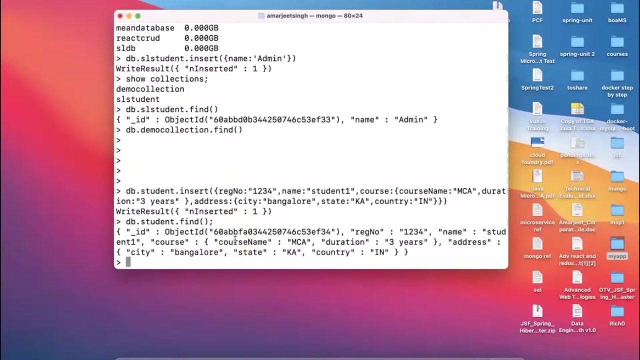 number, fine- and the primary key. so the primary key will be associated with the most outer document and the inner documents are directly associated, associated with them. and now when i try to say db, db, dot, student dot, find you can see now the records are fetched. i can understand many of you are. 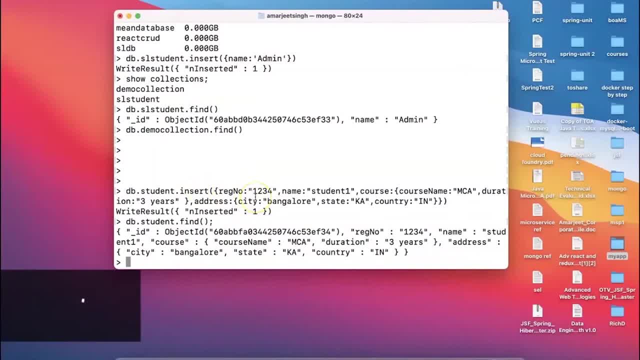 thinking every time, while adding the record, we do not add any object id. and here you might have observed- and there also you have observed, then, what exactly that id is. now let me brief you. this id is nothing but a unique primary key your mongodb has offered you. that means: 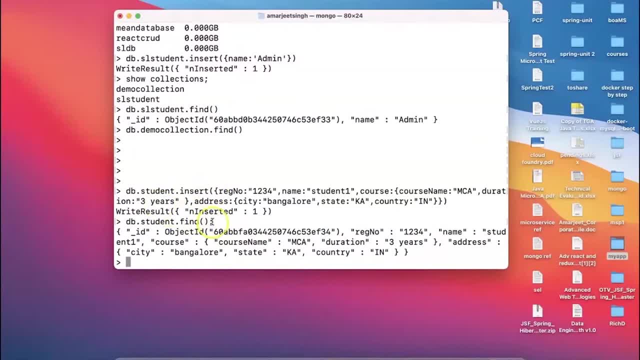 mongodb says: whichever data you're inserting it. so by default, with every single document, mongodb will associate this by default property called underscore id, which you can't even ignore. however, you can override. i haven't provided any underscore id as a property because this is a predefined property. 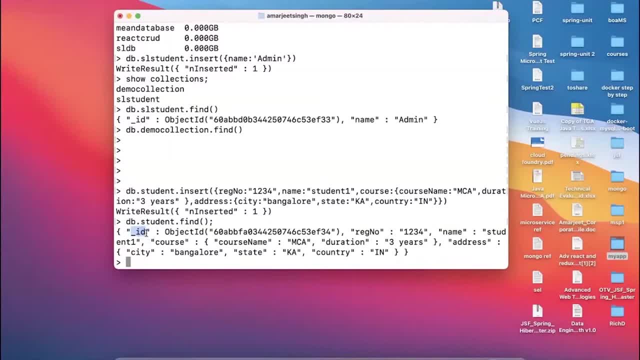 associated with every single mongodb document. if you want to override it, you can override from this value to any value, because if you do not pass any value, this value will be automatically provided. that is a typical hexadecimal value. however, if you want to override it, you can override the value of underscore id, but you can't change the key name. let's try with some. 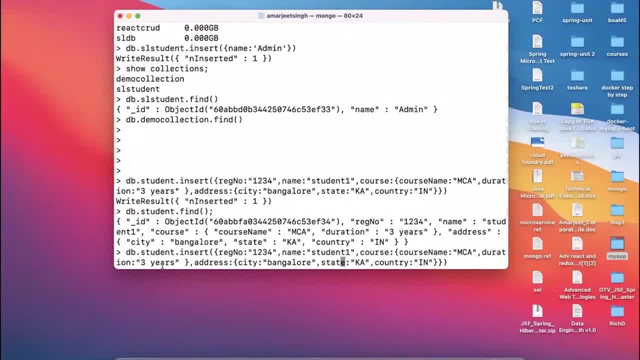 another record, so same record. if i try to add, let's go, i'm using call student2 and here i'm saying one, two, three, four, five. here if i want to override it i can just say underscore id colon. now i can give the value called what. 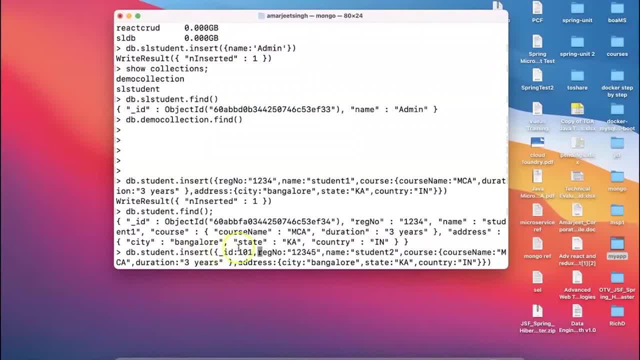 one zero one. this you need to remember. so i'm overriding this value with one zero one now, adding it now. records are added now. let me call find now. you see, i'm overriding this value with one zero one now, adding it now. records are added now. let me call find now, you see. 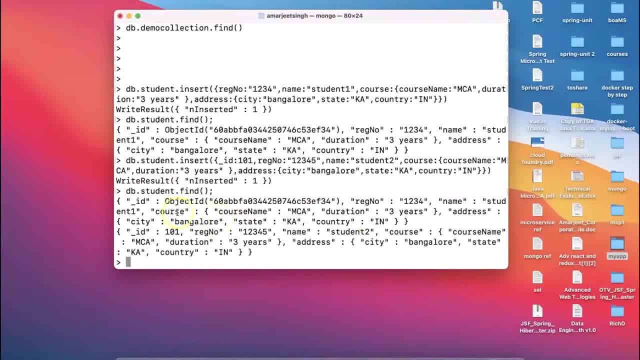 this time the records when i fetched. so in this record, the first record contains a default underscore id. in a second record it is the one which i have provided. and remember one thing: in mongodb you really can't offer any property other than underscore id as a primary key. 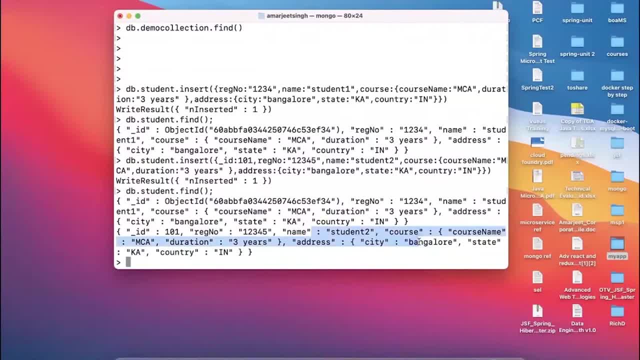 here there is no concept of having the cons like in composite key, which you used to do in traditional idb miss. here you have only underscore id and this is the only property which you can override. it else, by default, the new value will be given to you. so this is the first. 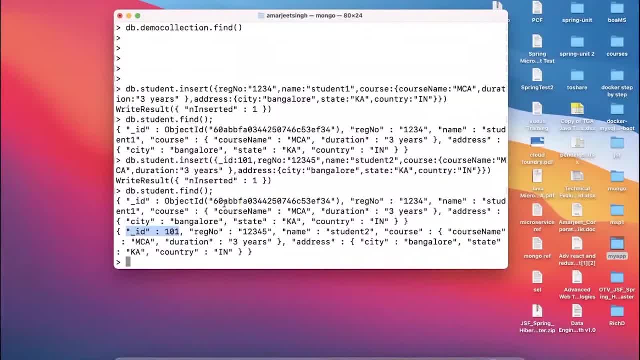 way of how the insert document has been done. we'll be telling you the other ways where the other documents are also added. okay, so in the previous examples you have seen like how we can add the records, but i also tell you there is another. alternative options are available if you want to. 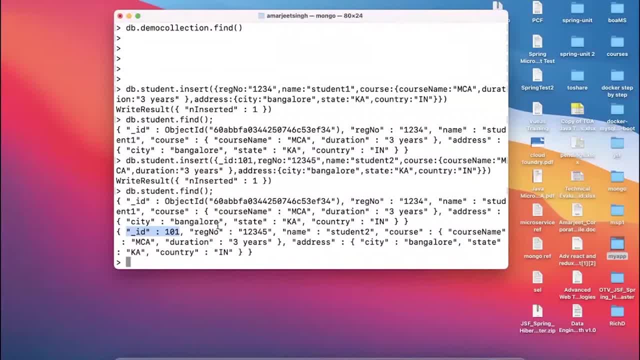 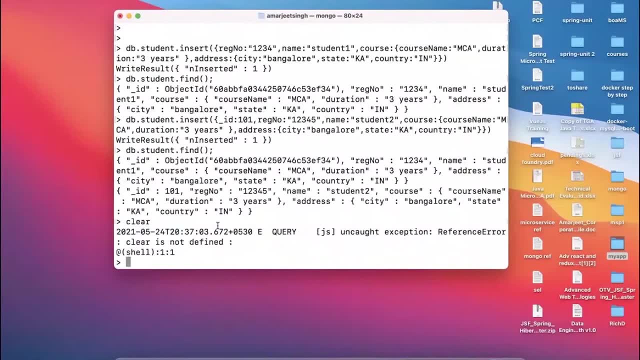 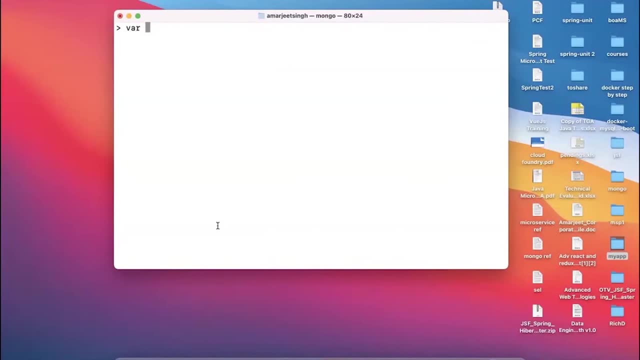 insert the records in a bulk. that option is also possible in mongodb. how we can do, let's try to understand here. here we would like to use one very simple concept called var, my emp, equal to now, starting with a typical object like this, and after that i'm adding this, and within this i'm adding the first property. 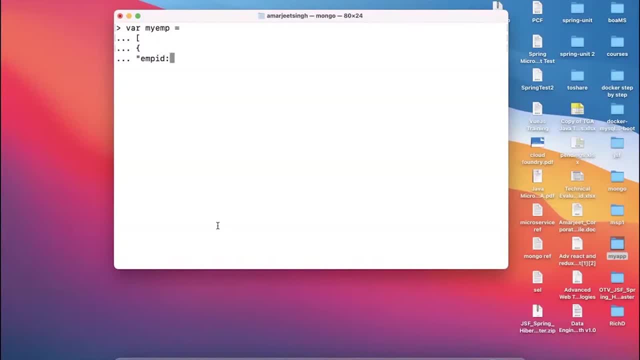 emp id, colon 1 after this: okay, now you can see. it is not understanding because there is a challenge when we talk about call uh, you know the logical part. because you go with multiple lines, it is not supporting. however, you have to follow the same lines. now. emp id 1 and we just give the second. 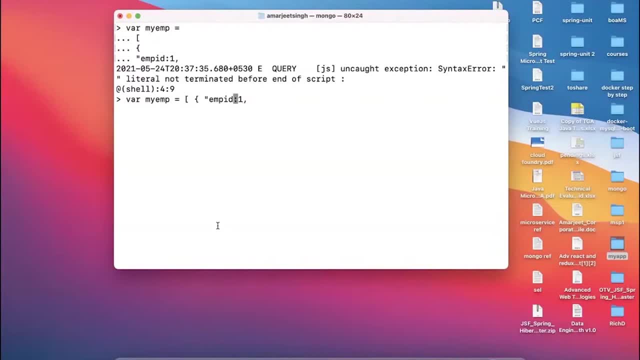 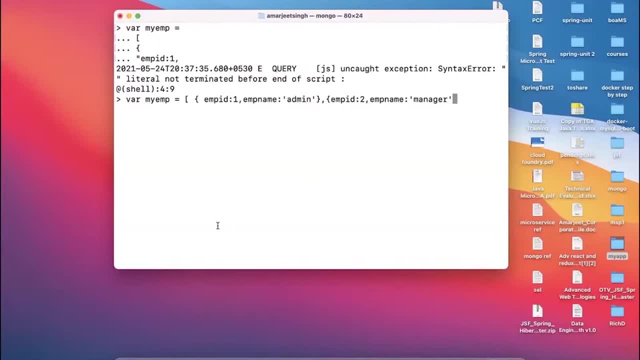 first record: here again i'm adding another one that is called emp id, colon 2. first record: here again i'm adding another one that is called emp id, colon 2. okay, and this curly braces is closing. after this your square bracket is also closing, and once it is done, come down and say DB, dot, new, AMP dot, insert. okay. 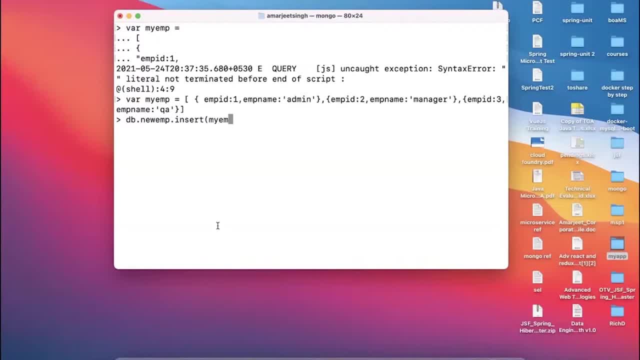 and here you pass the name of the object called my AMP and you can see. now it is telling you an inserted tree that is known called bulk insert. we are inserting multiple records in a single shot. see how easy it is for you. ok, now you simply use DB dot. the collection name is what your new emp dot find, and 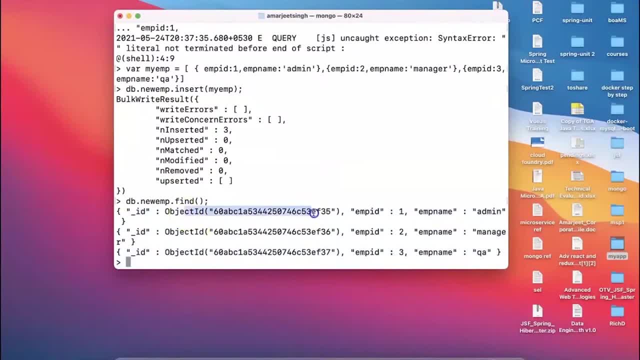 you can see now all three records are inserted with its default object definition id. okay, so that's is a really nice idea to have the id to be provided. okay, remember this statement. so you understood finally how we can add the records in a book. going forward, we will also. 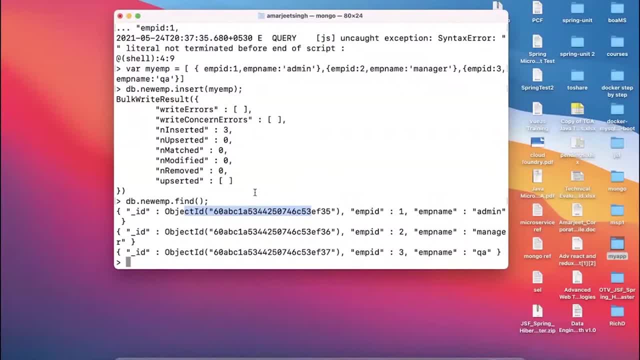 talk about, which is related to your update, as well as delete in your upcoming demos. okay, but here, that is the first thing which you realize it how we can perform those kind of operations in very, very simple and straightforward manner. okay, everyone. so now we have got three records with us and, in case, if i'm planning to perform update on any of my records, 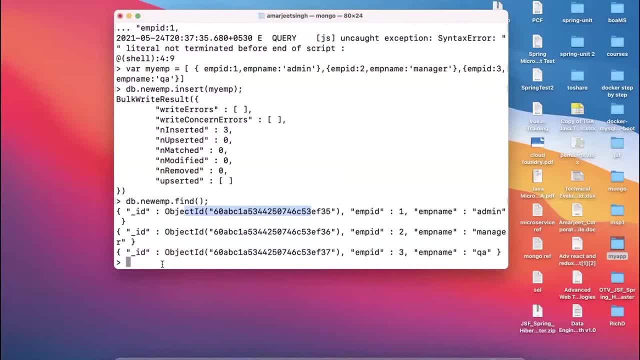 how will i do this now? so we have a predefined functions available name called update function. let's see how this update function can really work. so we use this statement name called db dot. what is my collection name, which is known as call a new emp- new emp. 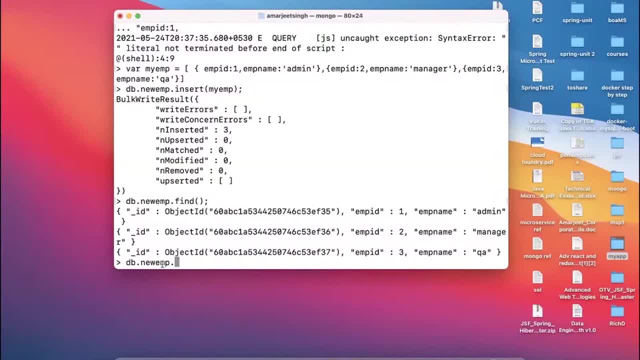 okay, dot update. okay. so what i will do? i will say db dot new, emp dot update here. okay. now, when we talk about call update, we have a statement available. okay, what is that? that is called emp id. we will call emp name. so we say wherever the emp id is. 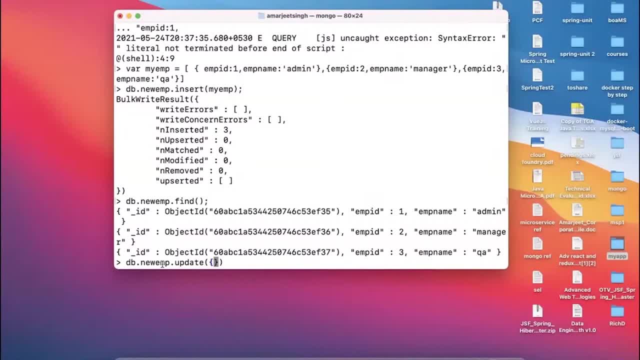 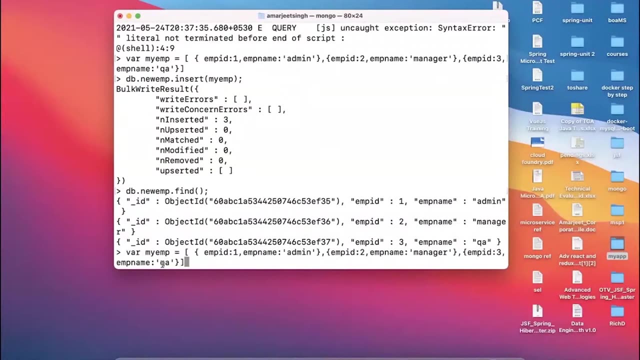 this. i want to change what the name. how can i do this? now? very simple, uh, to perform this. what i would like to do now, i want to basically add few more records to give you some more better idea. you can see now, here we have a call admin. 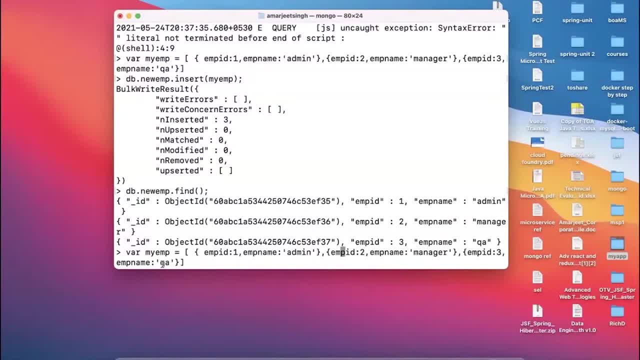 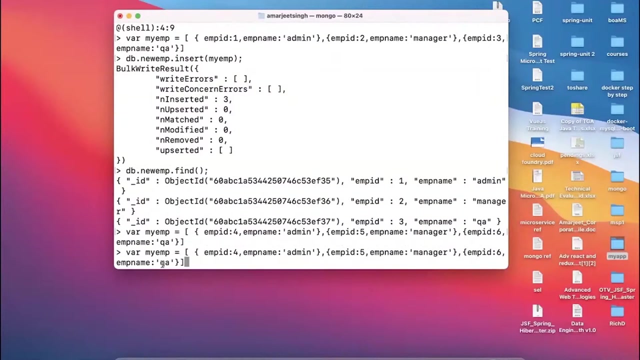 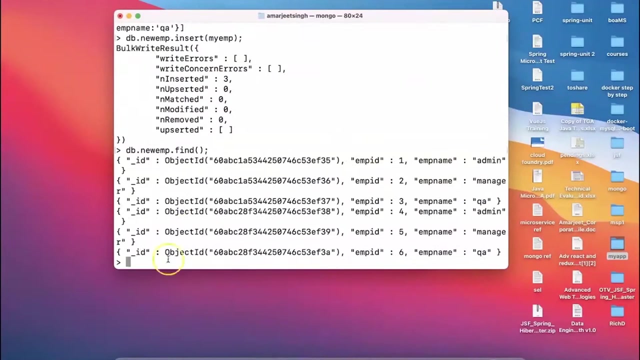 id name. so i just do one thing, i just change the ids. uh, one, two, three, i just say four, i say five, i say six. okay, and i call this again. the three records are inserted. now let me try to call: find now we have total number of six records are available where 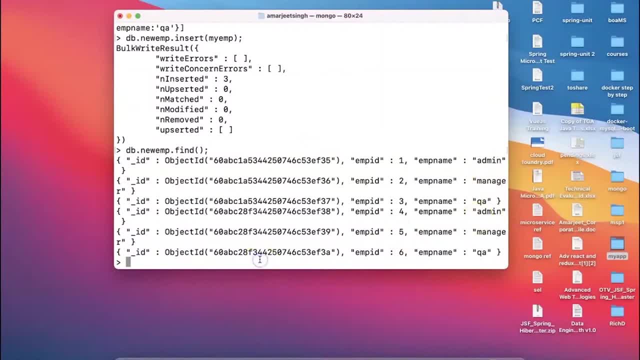 admin is repeated, manager is repeated, qa is repeated. now let me try to update the record. okay, now i want to say db dot new, emp dot. update. here i would like to perform the property like in what uh name? i say emp name, amp name colon. i say admin. 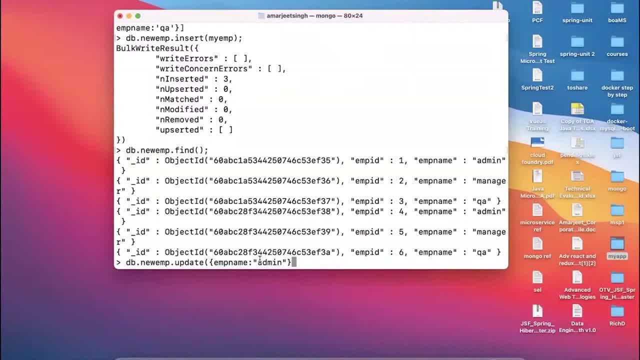 okay, so i just close that and i use another curly name, another curly braces with dollar set. set means you want to set the new value here we are giving EMP name. okay, what I want to do. I say, wherever the name is admin, change to what admin new that name. I want to change it closes. closes- run now. 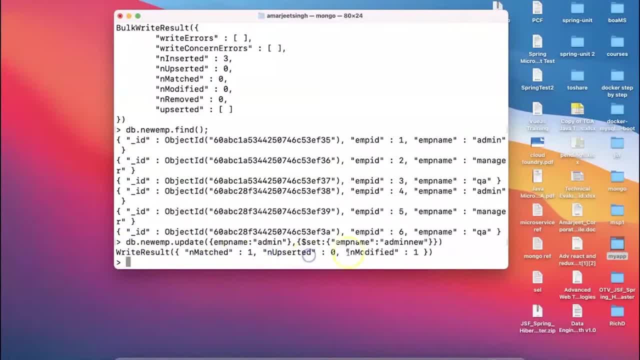 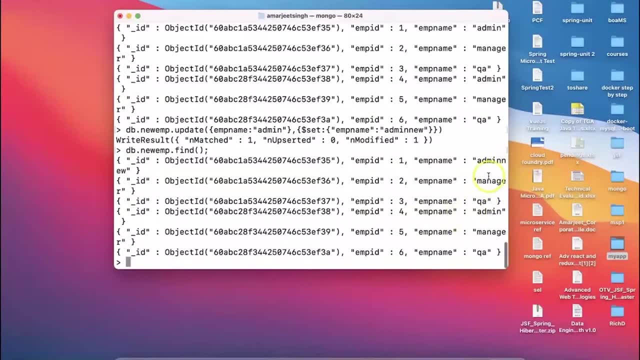 I can see it is saying n match to 1 and the record fields are updated like this. let me check well here. I will see the value called admin- new- is updated, but I have one more admin called admin. it is not changed. and there is something which you need to notice. what you need to notice is 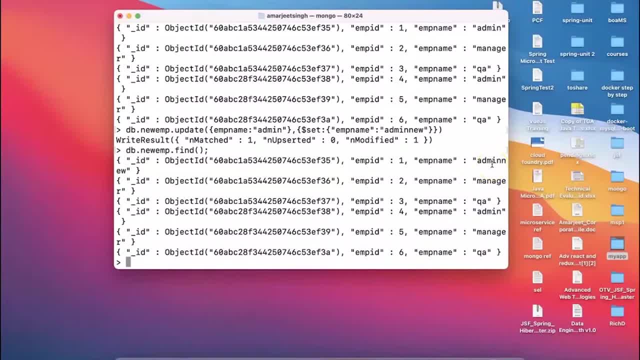 notice is like when you try to perform update. so what MongoDB does? it starts from the top, find the first record, change the value or modify the value and come up from the loop. it doesn't carry forward its search process for the next level of results. and there is something which is I really want to do that. so in 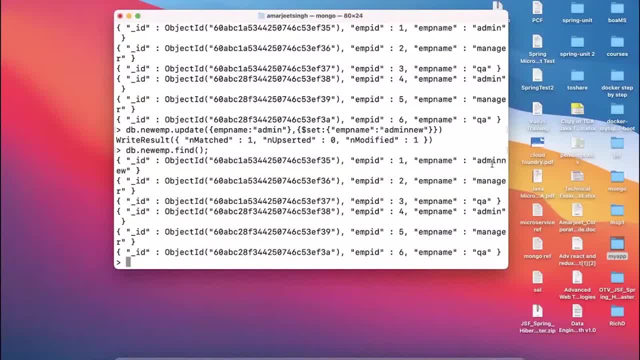 case if you are planning to change those values multiple times. so what you need to do. let's take a look here in the similar example. here we have a call name admin. second property, we have a call manager. let's try to say managers are repeated twice. we just want to change to new. 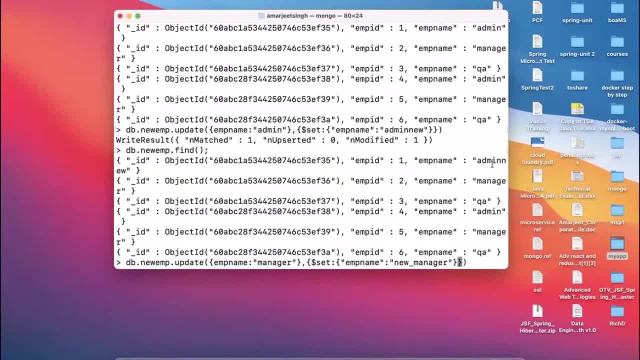 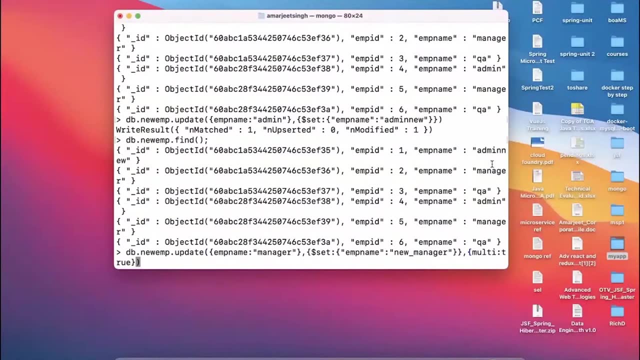 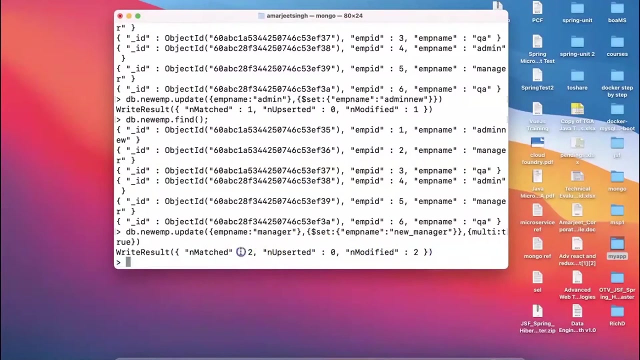 underscore manager and I want to update multiple values. what I will do here? I will put comma and say multi colon. shoot, okay, saying multi colon, true that you want to say: hey, I want to update multiple search or multiple repetitions? hit enter. this time you can say it is saying: and match to and modify to. that means two records found and two. 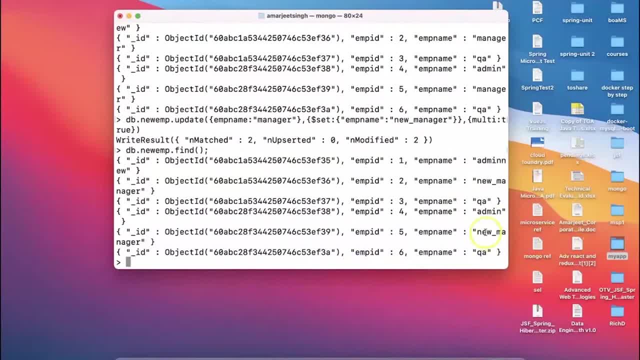 records are modified. let's check there we go. we have got new manager is updated in both the location. that's something which is really awesome, because this is how you try to perform the multiple changes. well, in our previous examples you see, like how we can perform the update part, but we have a one more beautiful feature available. 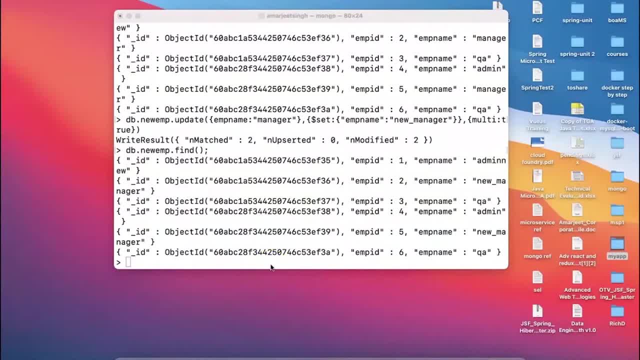 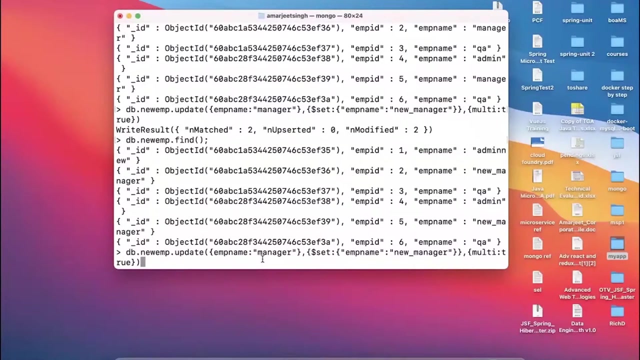 inside the MongoDB and that is called how exactly we can perform absurd, clear. let's talk about absurd. absurd is a combinations of update and insert. let me try to show you one magic here. when we talk about an update part, you see now here we are trying to say this. 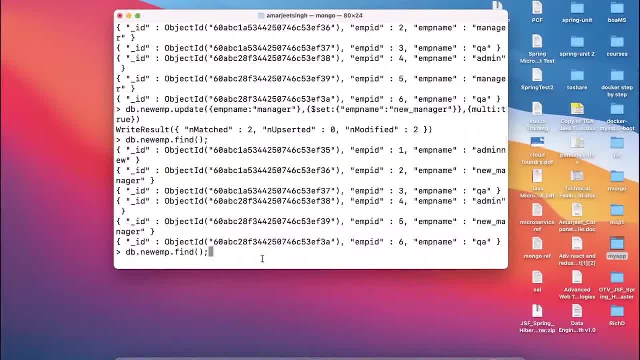 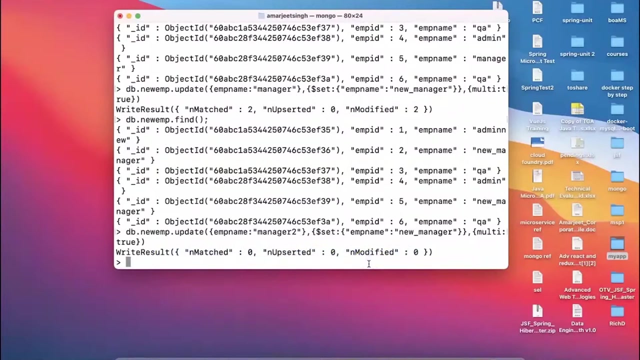 point. yeah, you see what multi true we have used. now here this multi true is: we're trying to update, but let's talk about something called manager to and enter. now you can see it is saying no records found. clear, no records found. but there's one concept available in called absurd. absurd means. if I try to perform. 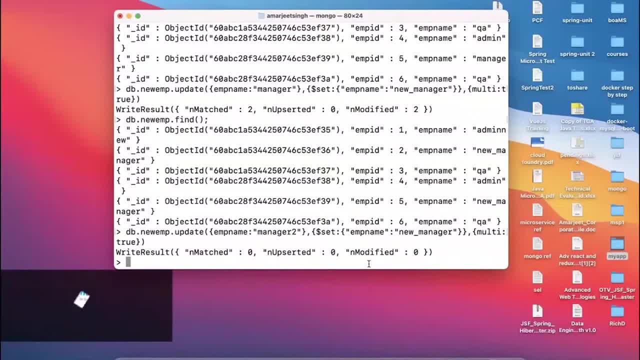 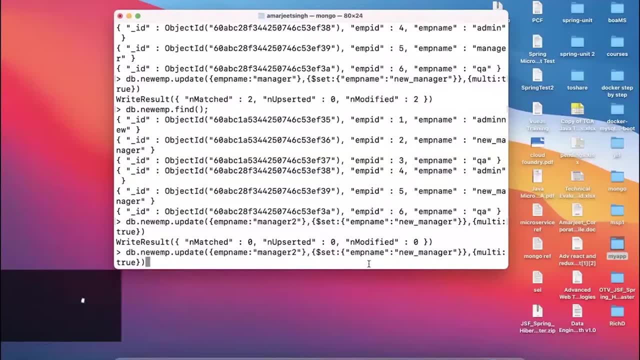 absurd. it means if the records are not available, it'll insert the record. I want to show you one simple example now. here we are using multi, true, okay. so, as I can see, we're using something called name and we're performing this update part. so in this update part we are using this dollar set, new manager. so here, rather, 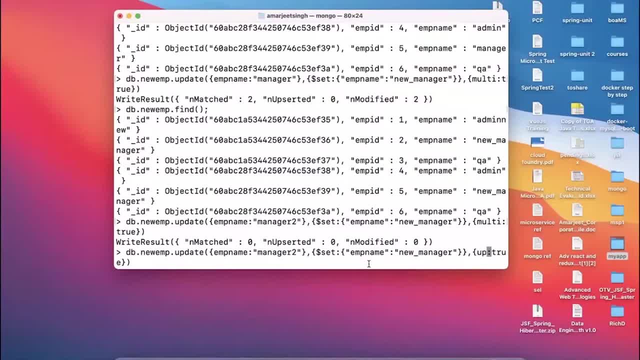 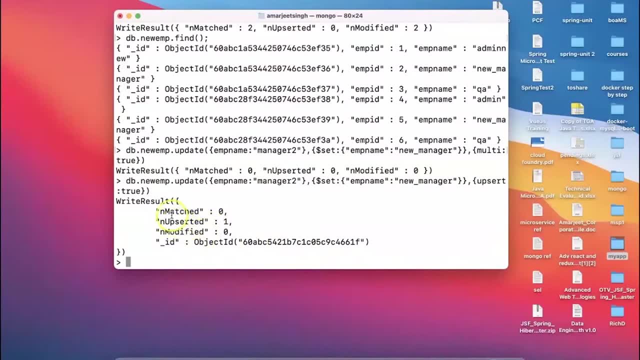 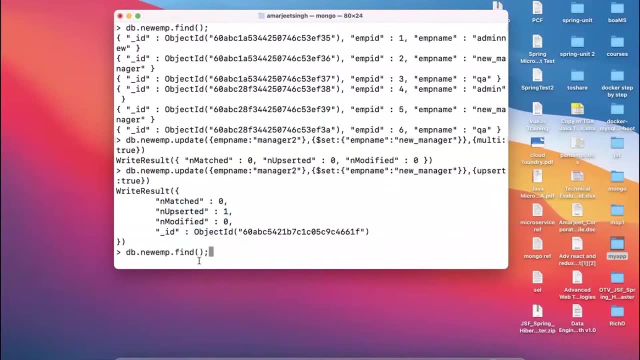 than using multi true, we are saying upset true when I say upset true. so what happened? now they say: and matched 0 and up inserted 2 and modified with ID. this that means when I try to call this find function, you'll be seeing. now we have a. 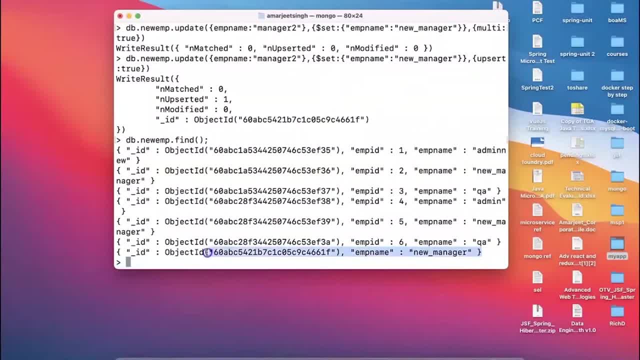 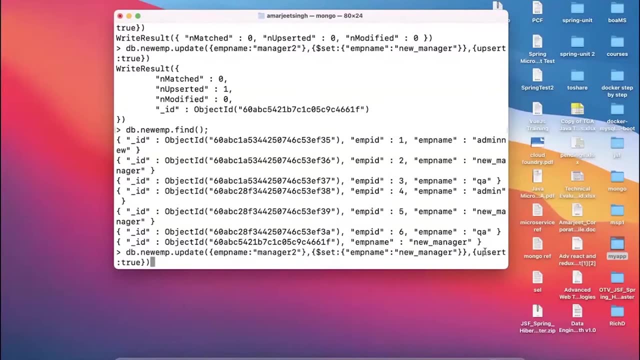 got. the another record has been added. are we clear now as a new record? so absurd does what absurd says like: if the records are found, I will update it, if it is not, I will insert it. that means, if I try to call the same thing, manager 2. 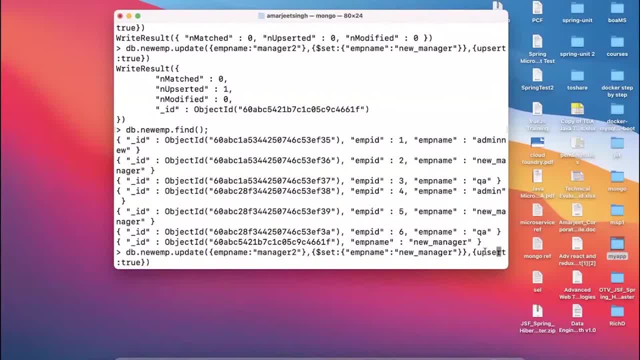 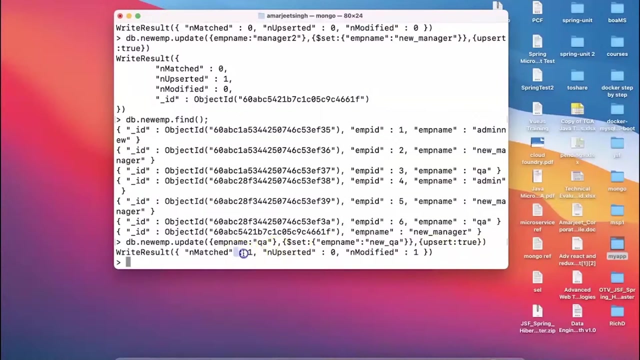 fine, it is added as a new manager- now if I just try to say not manager, to our call QA, QA, and here we sing EMP, could new underscore QA? and now you can see it is saying n matched 1, n upset at 0 and modified 1. so it is. 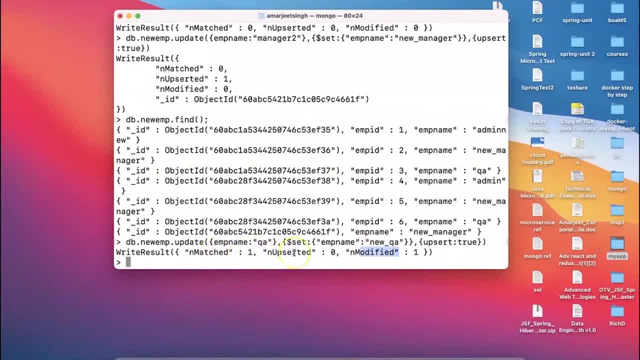 clearly telling you like, hey, I did not find any inserted part, but yes, I matched one record. I found one record and the one record is updated. now that is very, very beneficial feature when you really want to perform absurd. so that is a advantage of absurd at school: update plus insert very important. 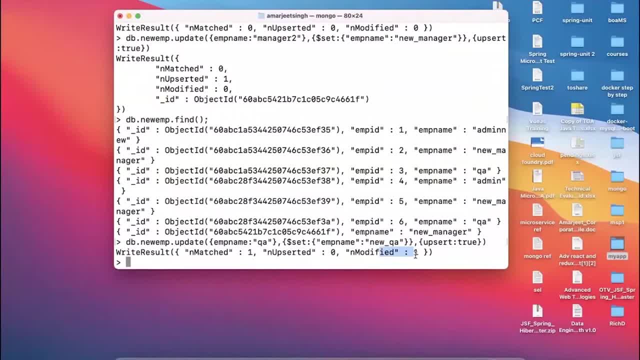 feature then depends on the requirement. if you want to add, you can certainly add this. so the way we have tried to add this absurd part, we can also try to perform the delete part also. okay, so MongoDB also helps you to perform the delete part and how you will be trying to add it. now let's try to understand here in my code: if 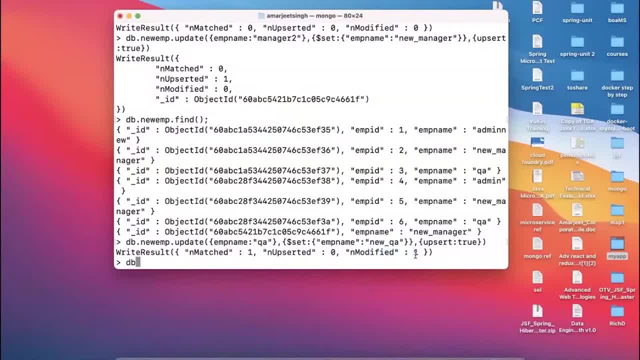 I want to perform any delete part. I have this statement name called DB dot. the option we are using it. that is known as collection name: EMP- new, EMP, sorry, dot. we have option name for remove in this remove we would like to offer the property. okay, and what we're talking about now here, let's try to add. 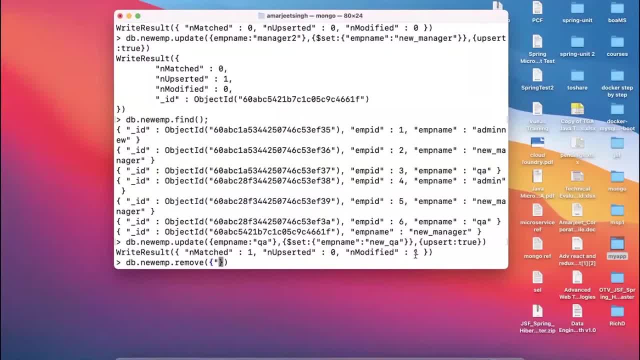 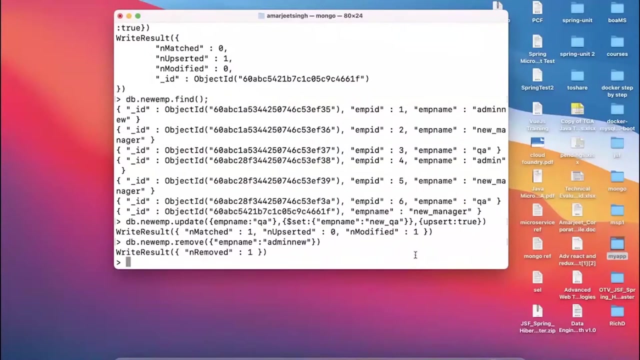 the ID here or the name which you would like to import. so I want to say, like: EMP name, admin new. so we just say we name okay and then you name is called. what admin new? okay, emp name, admin new. when i say remove, you can see it. 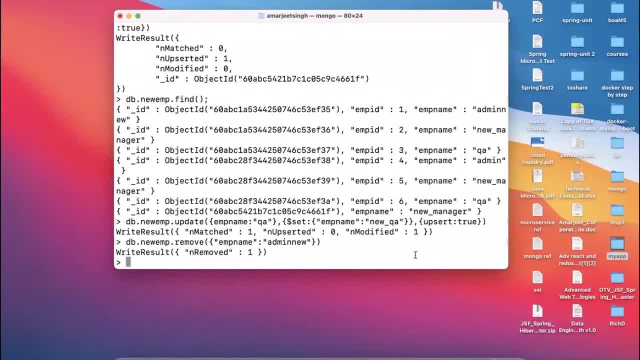 is record, removing the first record. so you can see: now the records are removed. fine, because there is only one admin. new is available. okay now. in a similar way, if i try to remove the property, call a new underscore manager. new underscore manager. hit enter. now you can see. 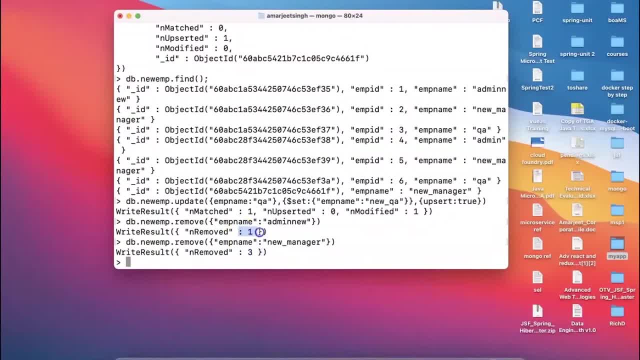 the three records are removed. so it's not like update which removes the only one. sorry, update only one record. it can also eliminate more than one records at the same time. that's the benefit of remove. so now you can see we have already implemented some records, as i seen earlier. 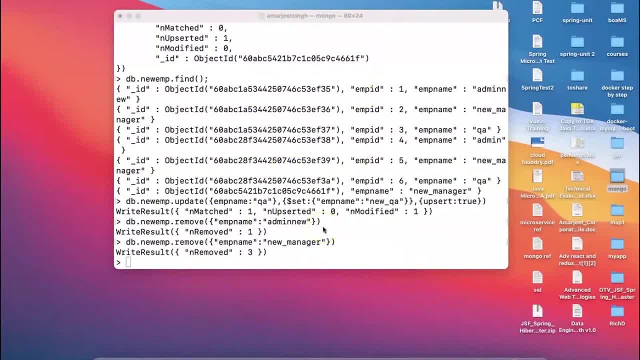 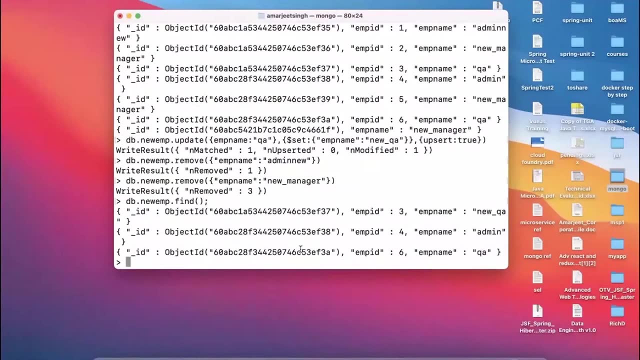 like we have performed the delete part now. now when i try to say dbnewempfind, three records are available with me: three, four and six. now when it comes to see insert part, we have seen update part, we have seen delete part, we have seen. now it's time to basically fetch the records, so find function. 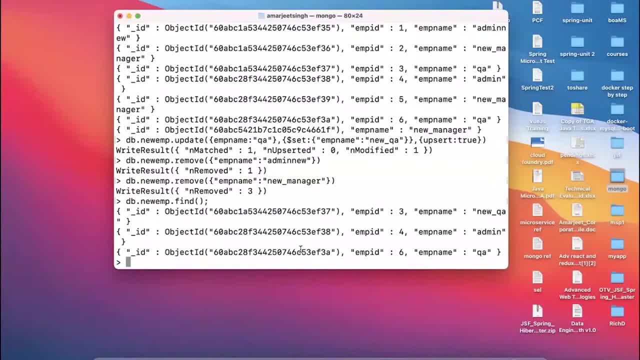 we've already seen. but in find function we also have some conditions, so called queries. so in case if you want to limit the number of records into your application, you can also do that. let's see dbnewempfind clear now. so in find you can also pick up the specific records too, like when i'm saying dot find and here: 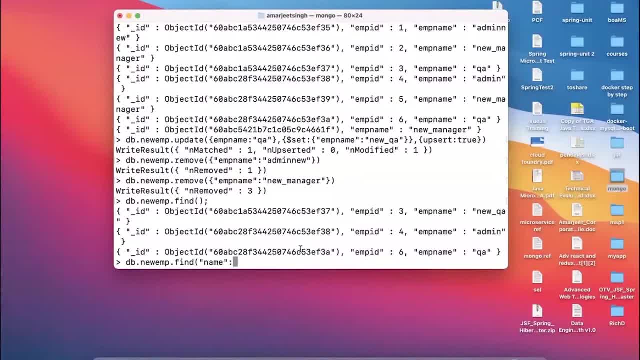 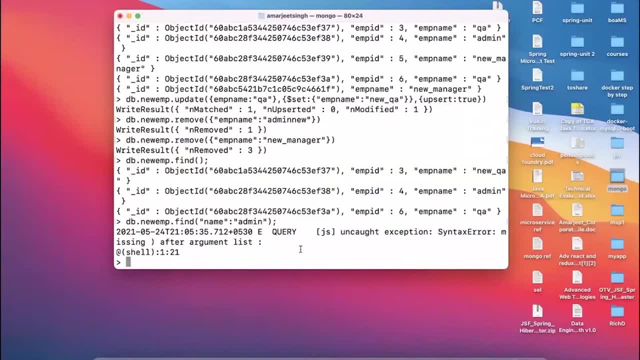 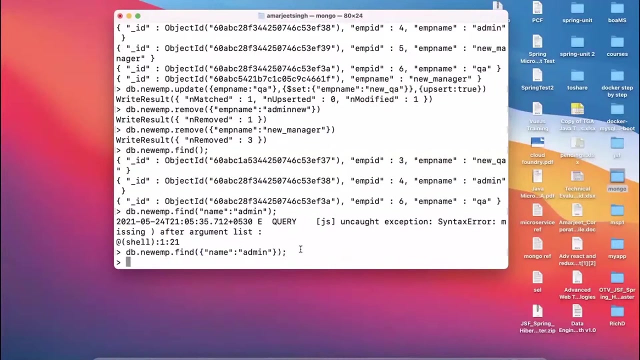 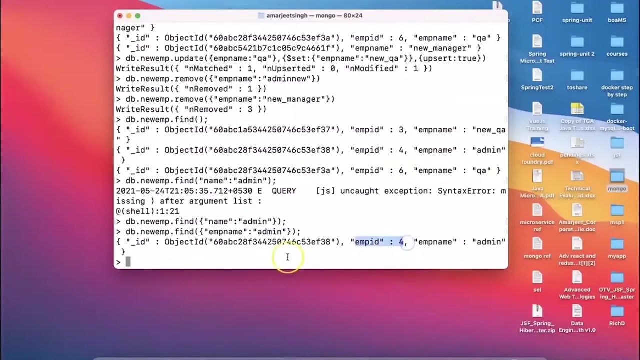 we can just say name colon admin. sorry here to put curly braces. it says there is no record with the name called admin. because it says there is no record with the name called admin, it is a emp name, not a name. so let me change back to now i can see it finds one record. 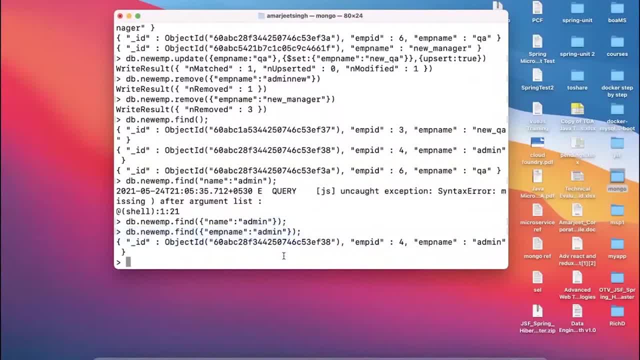 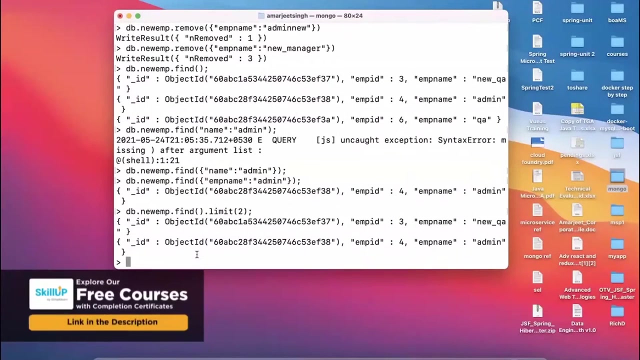 so, like that you can also apply a condition. okay, enter your code now in a similar line. if you really don't want to offer any condition, okay, but you want to limit the number of records to be shown, so you have this function available. name, call, limit two: two means only two records. now you can see, though, i have three records, but 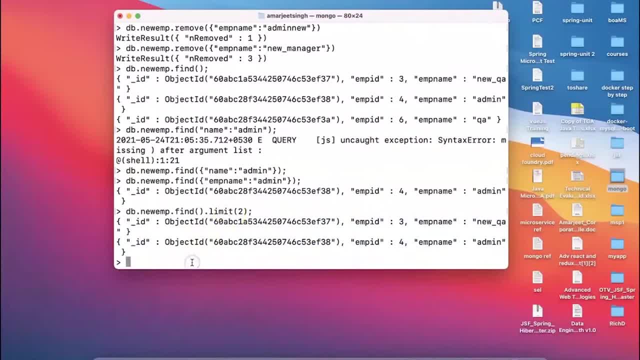 it is only showing me two records because i have limit those number of records into my code. also we can perform sorting, in case if you want to perform the sorting in ascending and descending order, that also you can also do so here, rather than saying limit with this. 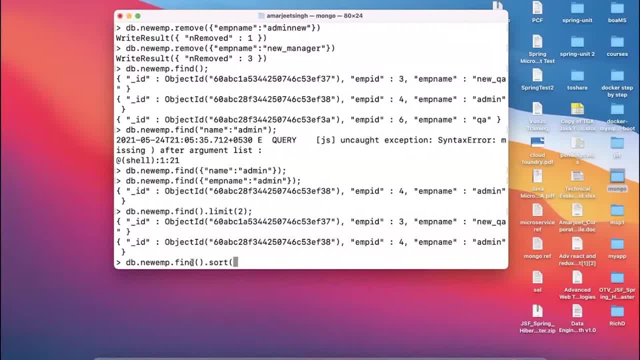 put this option name called sort and in this sort on which property you want to sort it. that are, so you can mention. so we can just say the mp name. okay, and using ascending order or descending order. so you can just say minus one. that is called descending order. hit now you can see it is showing in a descending order. now, if 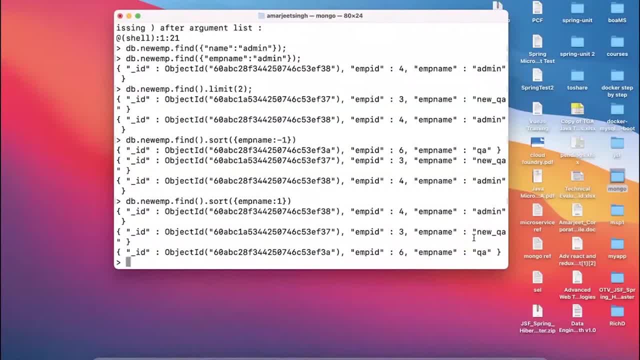 i just say minus one. if i just say one, what is showing you is that it is showing you a in an ascending order, so you can pick up the specific property we have on which you can tell it should be either on descending order or ascending order, so that option really works. 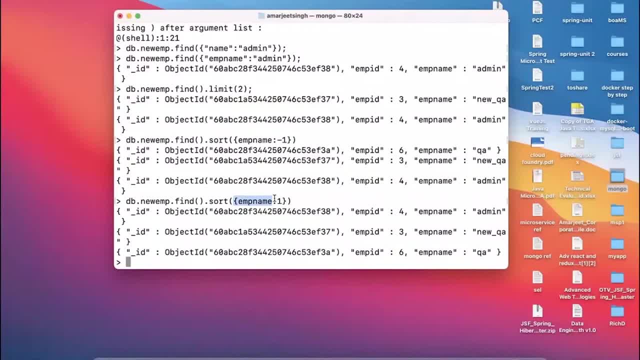 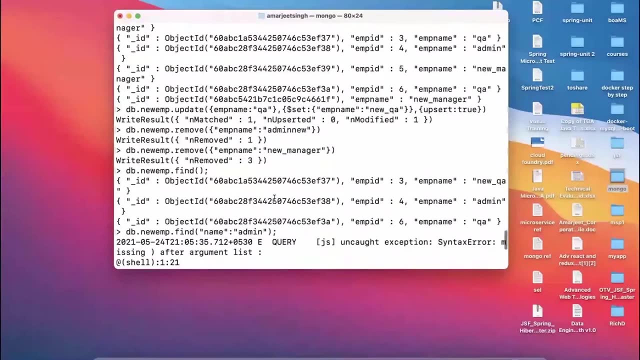 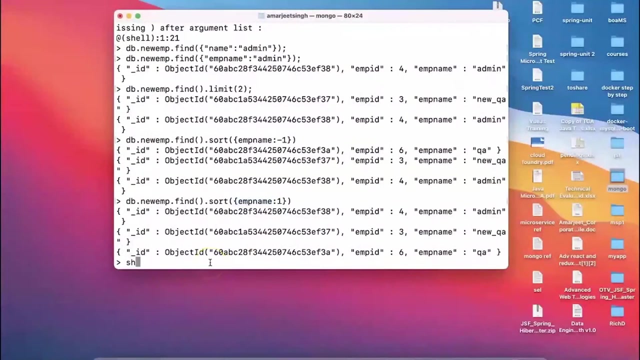 very fine, okay, so that's like how you can perform the queries. but remember one thing: you can also search the records based on the embedded columns too, because if you see in a previous records, we have some records added. okay, that is, let me try to say show. 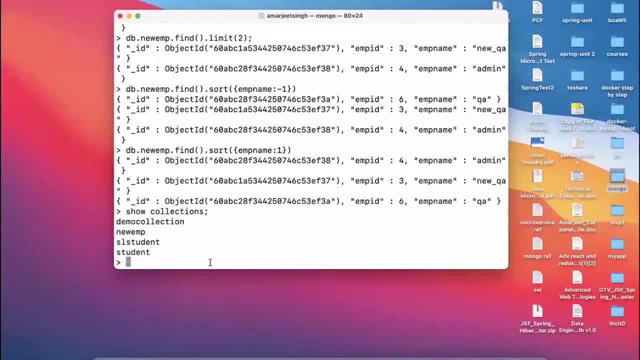 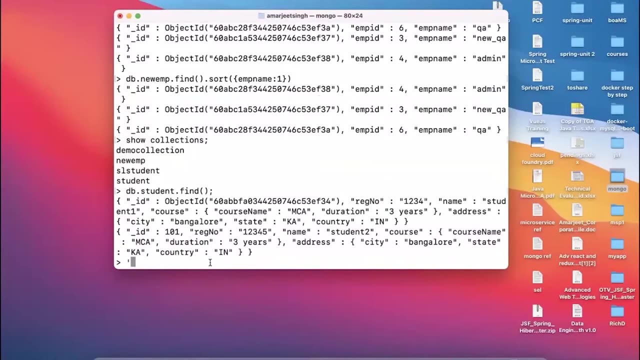 collections. i will call sl, student and student. okay, db dot, dot. find. okay, you can see we have records which are embedded records. now, if you want to search the records based on their embedded properties- like- and i'm talking about address, this is one property named city- fine, so if you would like to pick, 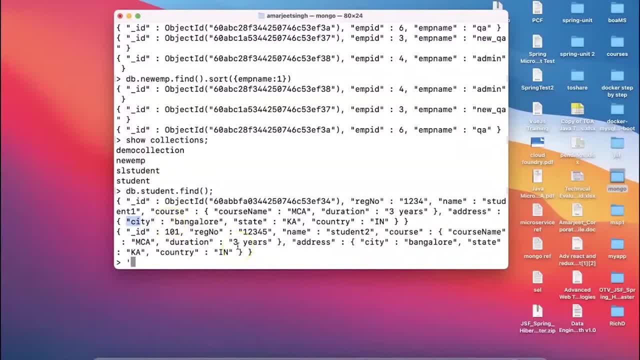 up those records. these are also possible. so how you can do this? very simple. so you say db dot, student dot, find, okay, so inside this, fine, you can provide the specific properties. like my outermost property name is called what address, so we are using this option called address. 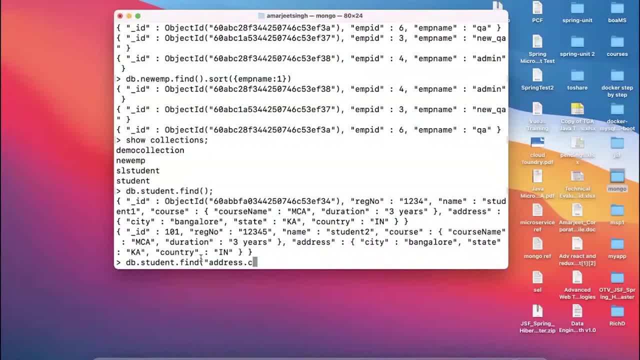 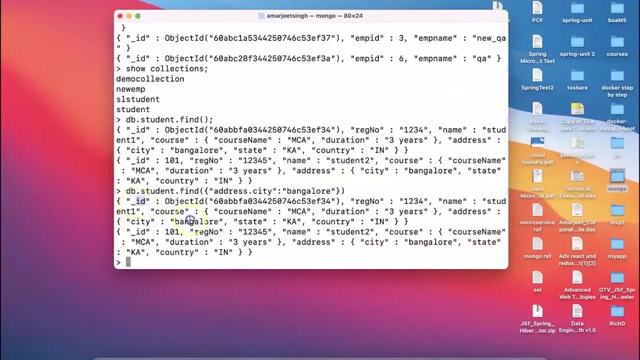 dot city, so we say city. are we clear colon? I'm giving the city name called what, Bangalore. let me close this and that's it okay. so we have to start passing another curly braces here. hit, enter and you can see. now I find two records, because both the records belong to what. 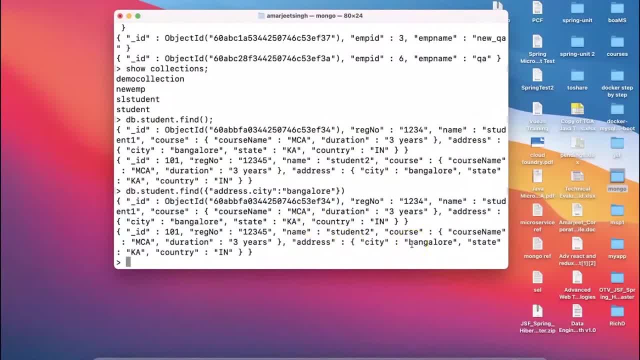 Bangalore, so I'm getting this city Bangalore with me. that's really awesome. like you can also pass the city accordingly. a part of that. we also have the other details, also okay, in which you can have the conditions based on less than, greater than or whatever values you would like to make. it is 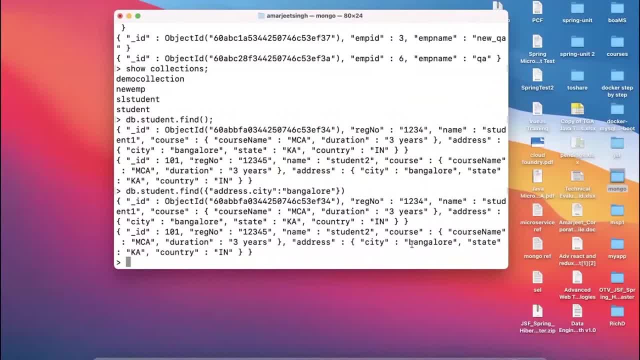 available and possible. okay, so that's how the conditions are satisfied. so suppose, if you would like to pick the users' I'll be clear where the range which you would like to consider. so those are also possible. like you can see, we have this property name called what? EMP ID 3. 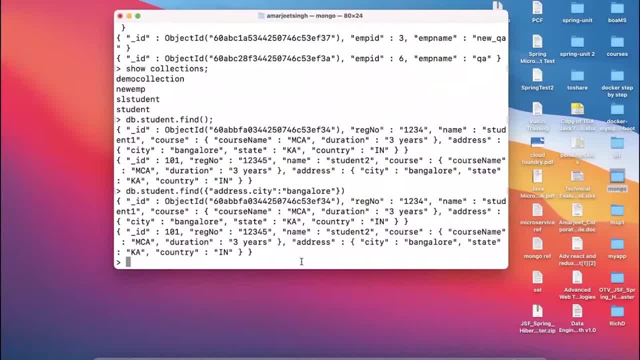 and 6. I just want to pick up only those records whose ID is greater than what. 2, what I can say? DB, dot, new, EMP, okay, dot find. and inside this find we can say the property, okay, so what's property? we're using EMP ID, we're saying EMP ID here. 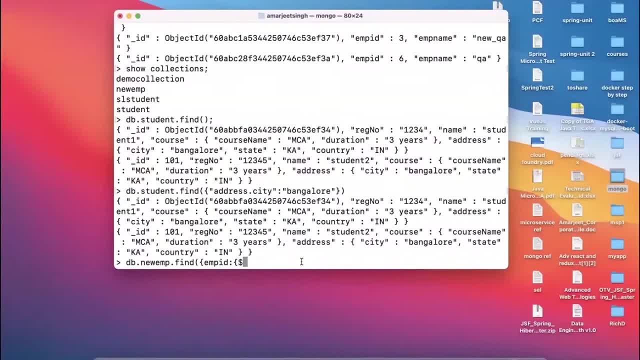 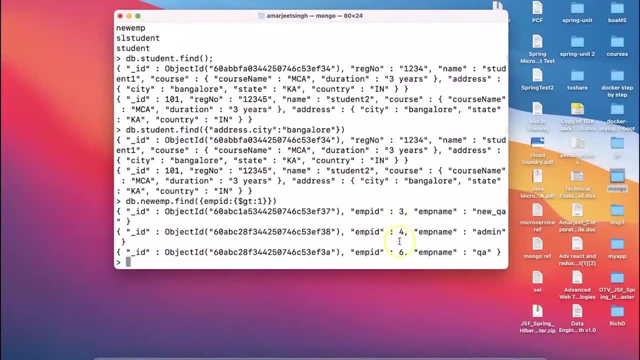 colon. here we'll be using dollar. GT. GC stands for what greater than colon. we're giving the value called what 1- 5. close this run. you can see you've received three records: 3, 4 and 6. in case, if I just look forward for higher than 5, you. 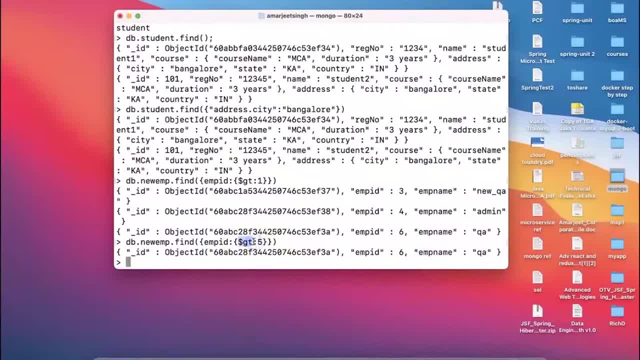 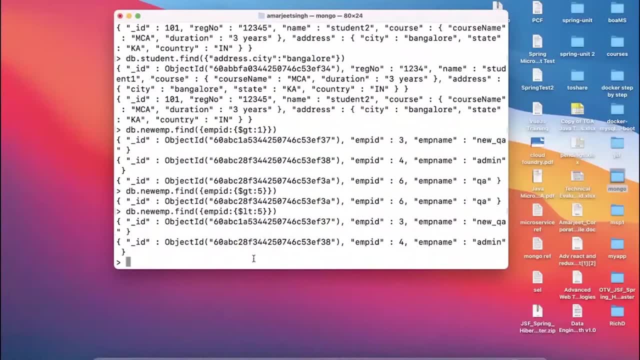 will see only one record so greater than that's called GT. okay, same option. if I just say LT, you can see we have found two records so less than greater than okay. so that's how exactly you offer it. okay. and also you can provide the condition, so-called limit, as I can say. 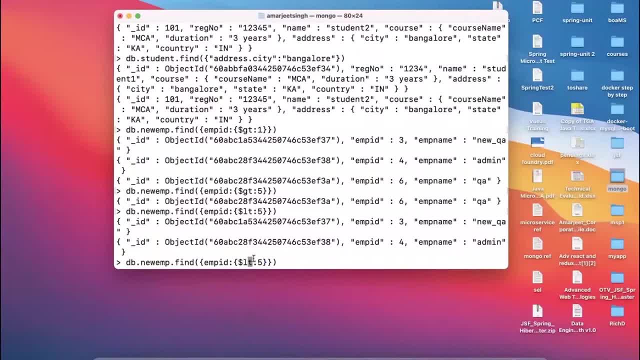 let me provide it. so here I will not use less than okay. instead I'll be providing another property. let me show you what. so here in EMP ID, whatever we've taken. so let me try to take the property, call find, and here we providing EMP ID. and then I'm going to use another curly braces. we're using the dollar in. 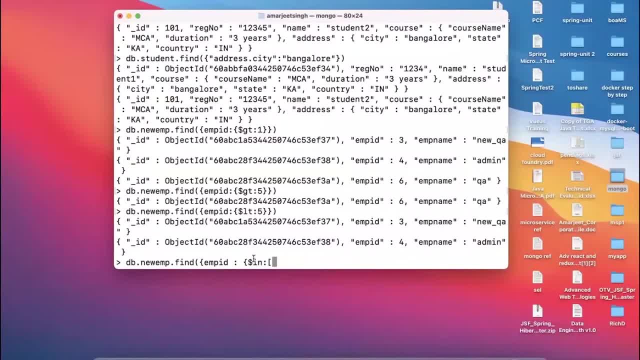 is that in part? oh, I can see this is $5.5. now we're going to use $5.5, that's all property dollar in colon. here you provide the details I'm saying inside. so the property is three, four, six. we are saying three comma six, close this and. 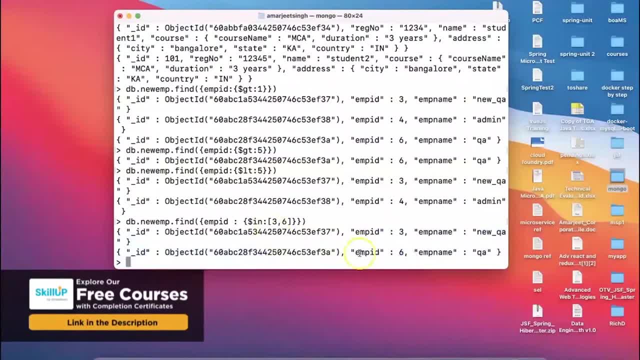 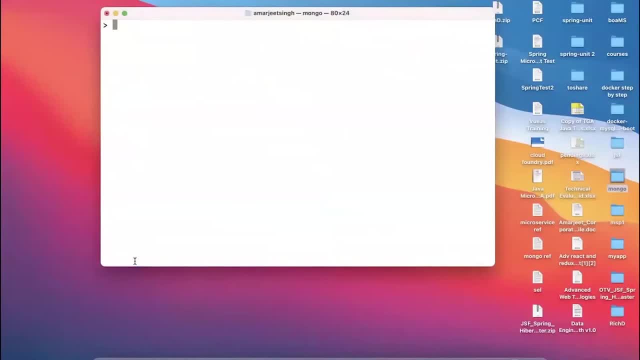 you can see, we got two records which matched with three and six. that's the benefit of having this, okay, everyone. so in a previous example we have already seen a lot many activities. this time we are trying to offer you something very interesting feature and that is known as called working with indexing, see Mongo. 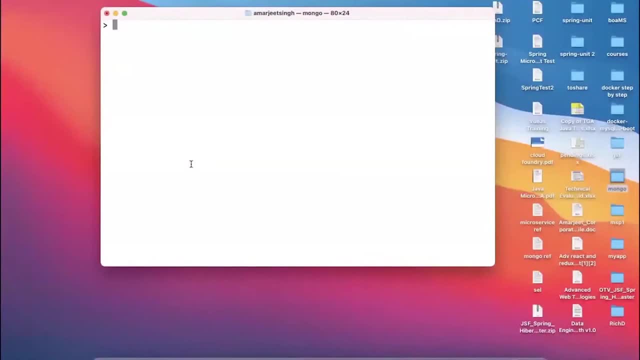 DB is one of the most popular tool and one of the reason why it is very popular because it is having the facility of having indexing. now, what exactly the index does? so, friends, main job of having this index is to basically give you the concept of indexing and what exactly the index does. so, friends, main job of having this index is to basically give you the concept. 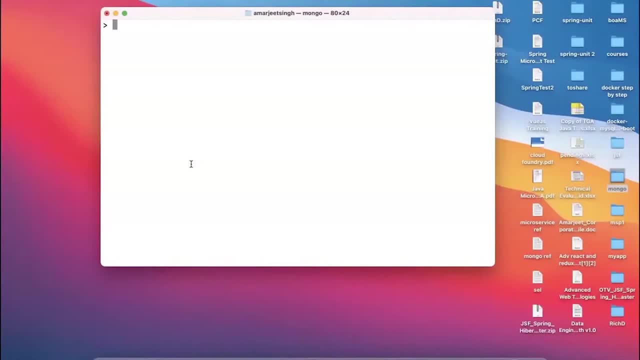 of like how one particular document, which is huge document, in case, if you would like to perform any sort of indexing inside this, how you will be applying this. so to apply indexing into my code. let's try to understand why index is really required without indexing and with indexing, how you'll be. 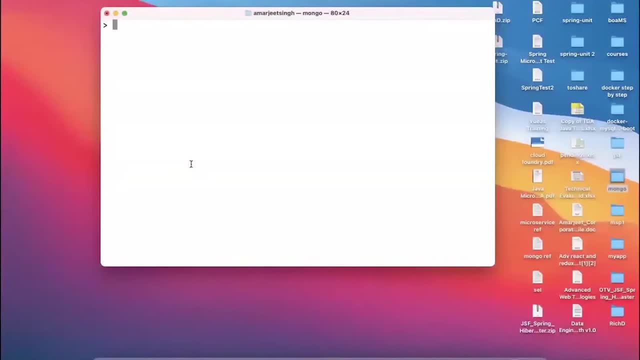 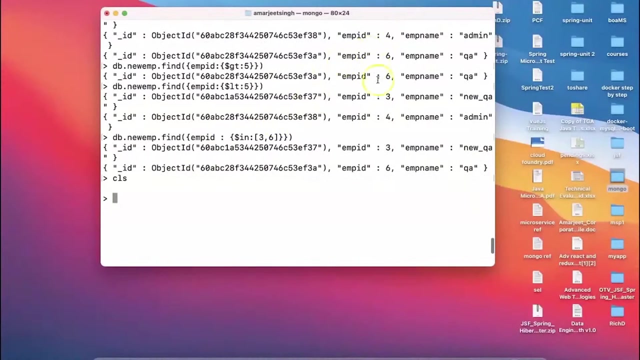 making a difference into the code. so to make it happen, we would like to insert some records to confirm. okay, so what I will do is, in step number one, previous records. if I see I have got four, six, three, four one. depends on what earlier records we had it. 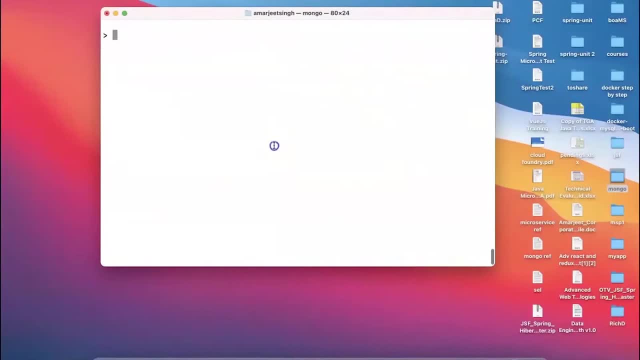 so we had a call new EMP. so DB dot. new EMP dot find. so we have total number of three records are available, so it's all one-time. okay, we can have this three records with me. now let me try to apply indexing without indexing if I want to find the result, what outcome I'm gonna receive. so to know about how much time it gonna be taking if, if I have a got large number of records with me, I'll be using this statement. name called DB. The name is called new EMPExplained. 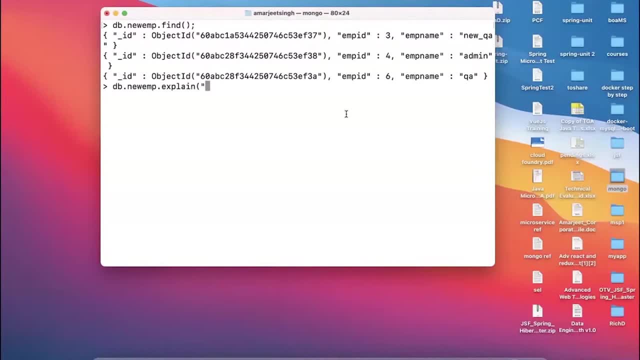 and here I will be using one predefined functionality called execution stats. execution starts. okay. now here, after the execution starts, will be using dot. fine, will be using the first property here. okay, and what user would like to find it that you need to basically offer it? so we are giving the name called EMP name. 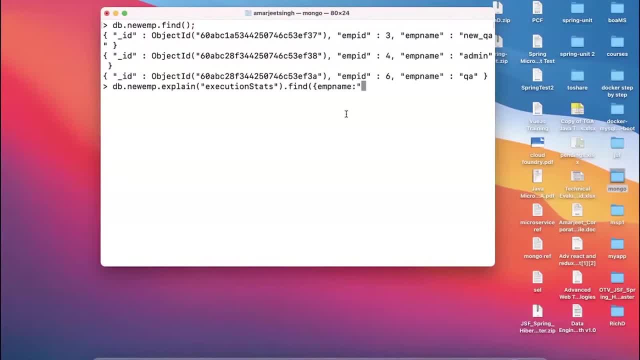 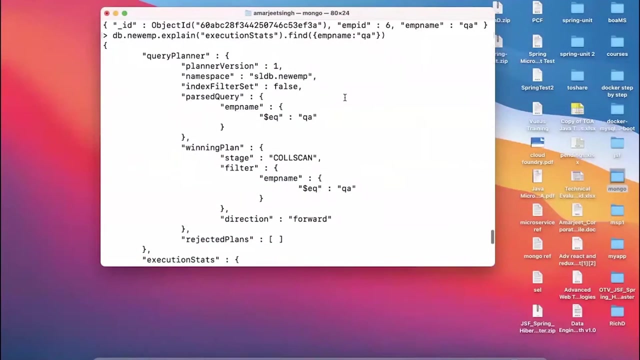 colon. give the name call QA. okay, let's close. okay now. when I pressed hit enter, execution stats is a predefined functionalities which will tell me when the query was executed, what exactly the query plan was. hit enter and now you can see. a lot of details are available with me, like you. 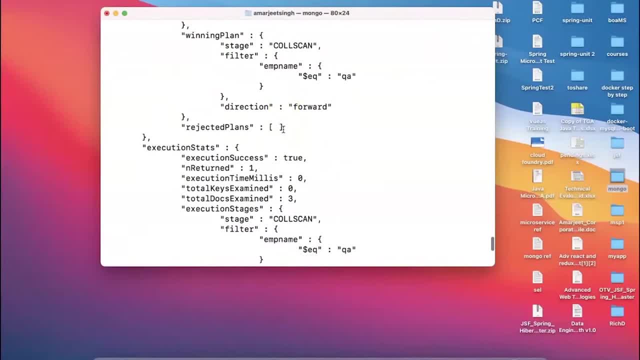 can see pass query winning plan and everything. one thing you need to remember: by default here when I try to run, it says: and return one advanced one need time. total everything it is showing me. but one important thing which you will see here is total number of documents is scanned, so it is telling me total. 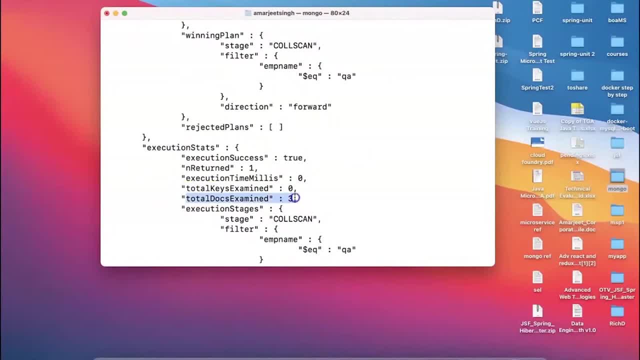 number of document examined is three. clear now and return one. that means one result is returned and the total number of documents examines three in order to find this record. just imagine a use case here where I say total number of documents examined: three in case, if I have got millions of records with me, that means to search the record, it will examine all the millions. 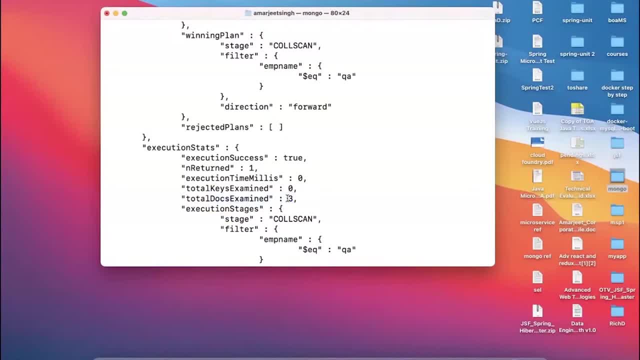 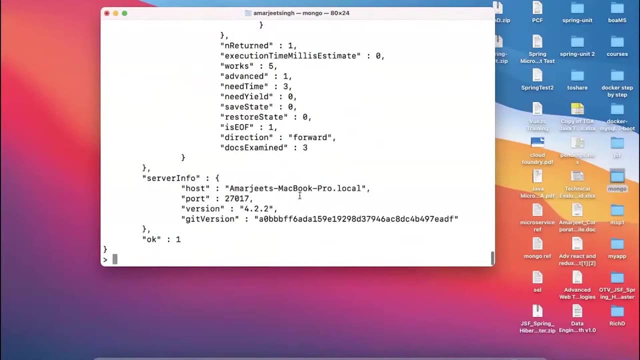 number of records to search the result, which certainly gonna be taking huge amount of time. and that's where, exactly, when you try to search the record, fine, when you have no indexing is available, okay. so you need to understand. one important thing is: by default, index is applied on your. 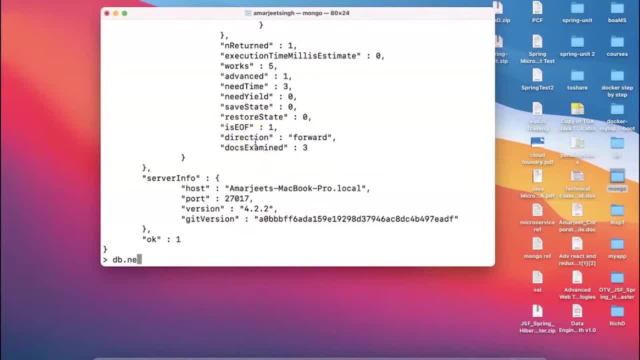 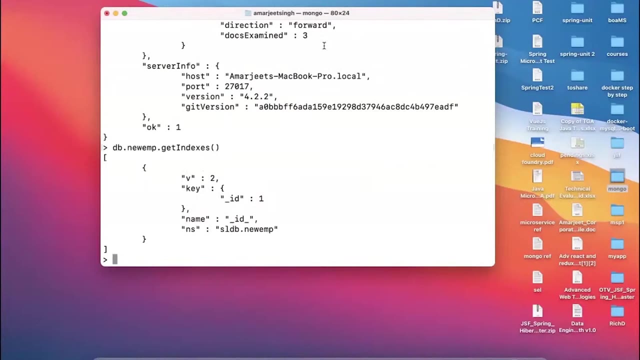 underscore id dbnuemp. when I say dbnuempgetindex is a predefined function, it tells me like hey, by default, index is applied your underscore id. that's a Fact, because by default, index is applied on underscore ID, not on the other properties. 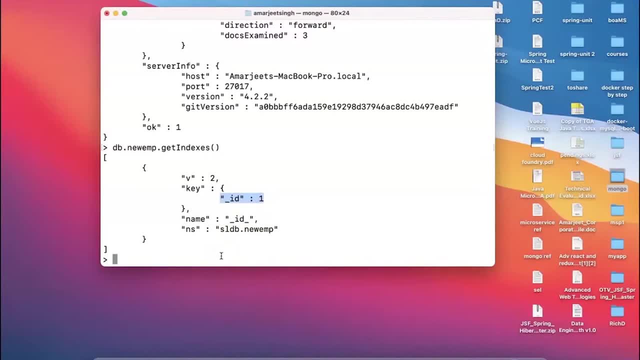 So I need to identify which of the properties are required to be get indexes. MongoDB advantages: it is supporting multi column indexes and that's what exactly we would like to see. Let's see in our next demo. Now we will try to apply index in on our own property. 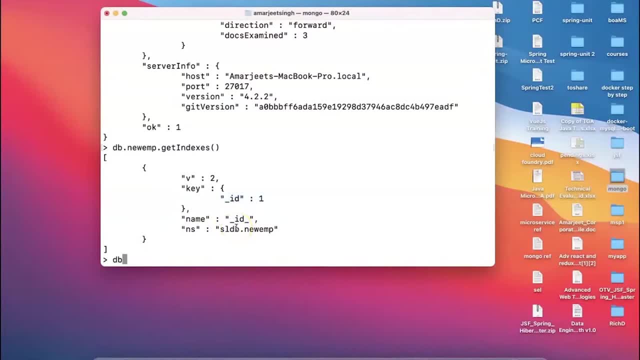 Okay. so to apply the index, what we need to do? we have to say DB, dot. certainly we will be talking about collection name. call new EMP dot, create index. Here you have to pass two things: number one, on which property you would like to apply, okay, and it has to be ascending or descending. 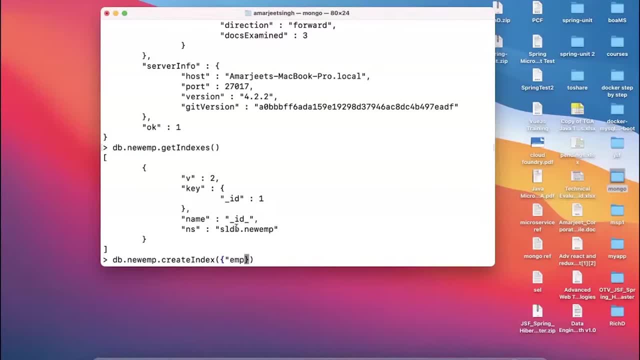 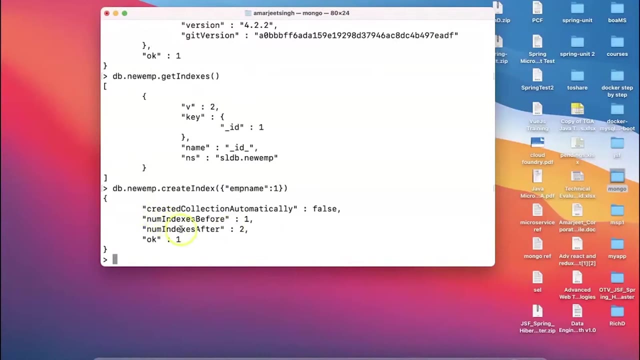 So I'm trying to apply on EMP name and I want the index to be applied on ascending order. Okay, so here, colon one, hit enter. you can see. now it is telling me like number of indexes before one and number of indexes after two. that means earlier index was available only. 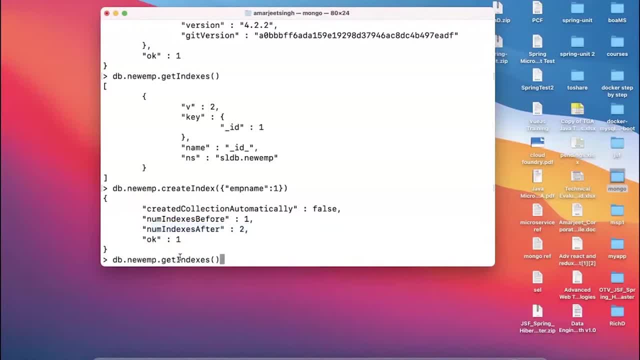 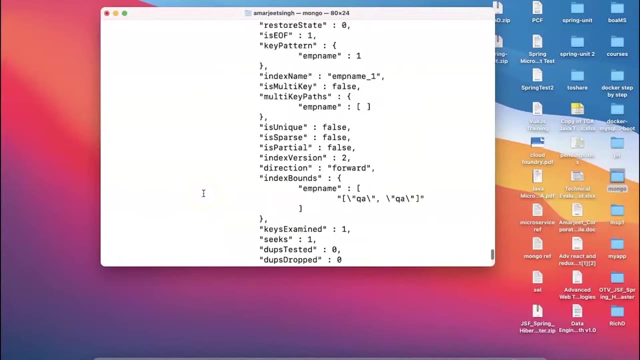 on one particular property. now it is applied on two properties. If you want, you can check. Now you can see there's another property is added called EMP, underscore one. Now if I try to execute a similar query which I executed earlier, QA. now you'll be seeing. 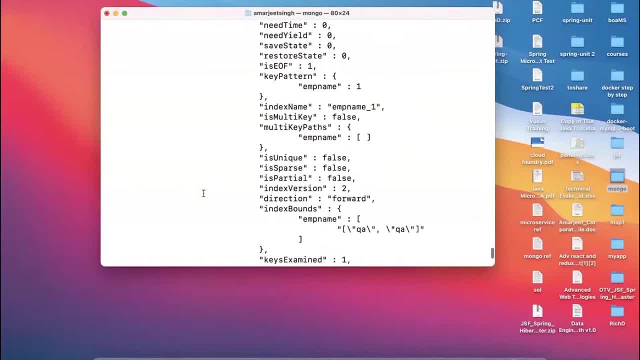 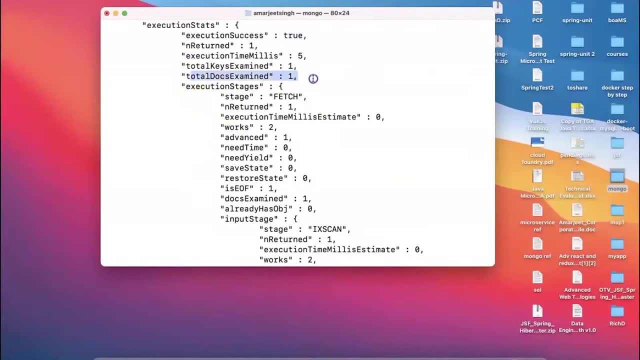 there's a different statistics altogether Here. if I see in my code, see, it will tell you total document examined: one. See now. earlier the number of document examined were three, But since this index is applied, Okay, Now it is telling me the total number of document examined is one. 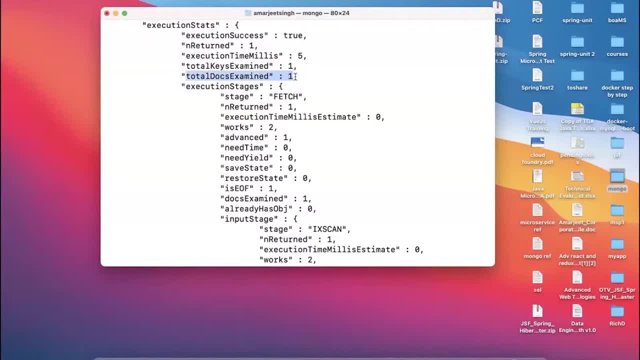 So performance is certainly improved. So to search your document, it won't be searching the complete collections, Okay. rather it will search what? only that particular column in which it is actually applied for. So that's the benefit, In fact, I would say, when you will be using these kind of indexes into your code. 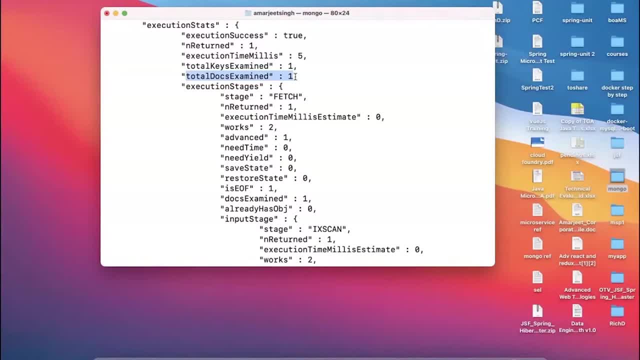 Okay, So hope we all are clear and understood about this concept. So let's go ahead and get this implemented into our system. Well, this is the first way of how the index can be applied, So you can also apply index on multiple properties. 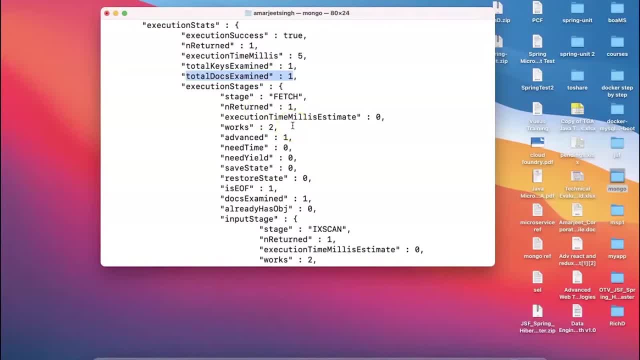 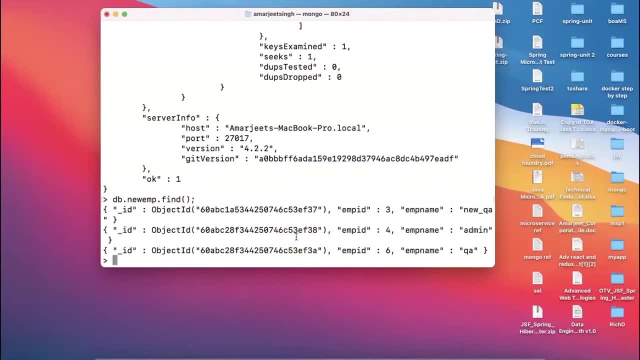 Clear So that we will show you one by one how it is Okay everybody. so we have already seen in our previous example how we have applied indexes In our existing MongoDB application. So it is also a possibilities where we want to also apply the index on other number of. 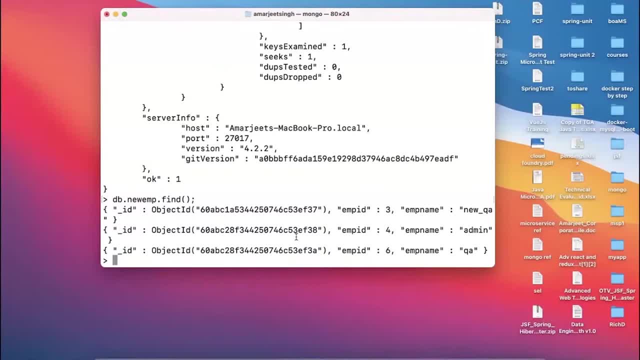 properties too, As you can see in our existing database- Okay, an existing collection. My collection name is new EMP, which contains two different properties. One is called EMP ID and second called EMP name. Just now, we have applied index on our EMP name. 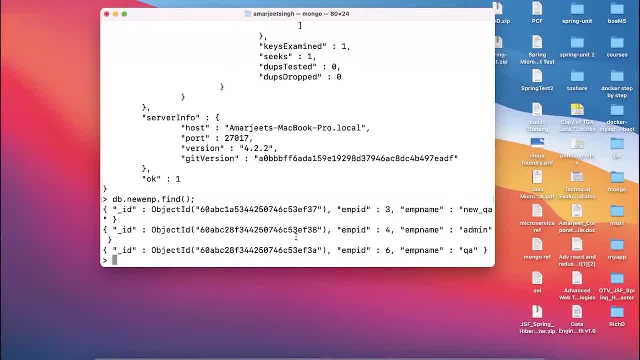 Okay, So in case, if I want to apply index on EMP ID, I'll be using the same technique. Okay, Let's try to apply index on the same. So first of all get indexes. I'm having this index applied on two different property. 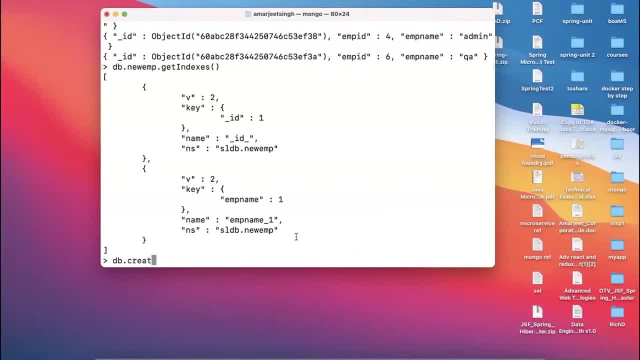 Now we would like to say DB dot create index. And here in this DB dot create index, we can just I will say DB dot collection name. So we have a collection name is called new EMP, New EMP. new EMP. dot create index. First parameter is certainly the name of which property we are applying. 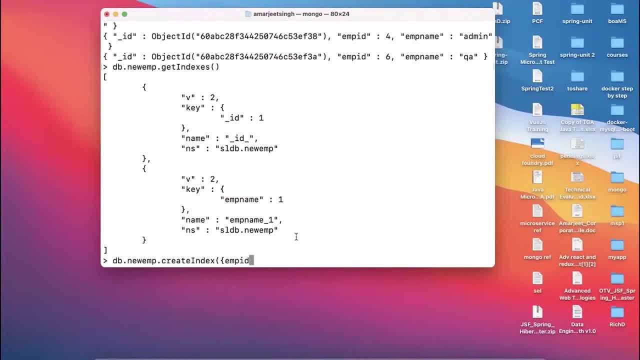 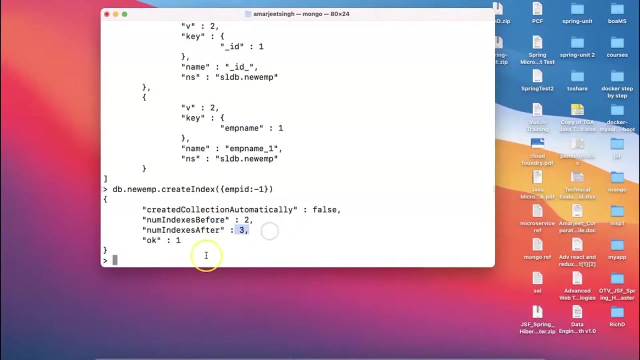 So here we are saying EMP ID and in this EMP ID we will just offer it has to be ascending or descending. Let me decide descending order. So we are saying minus one. Okay, Now let's press enter and check. Okay, Now you can see earlier indexes which we have created. that was two, and now it turns to three. 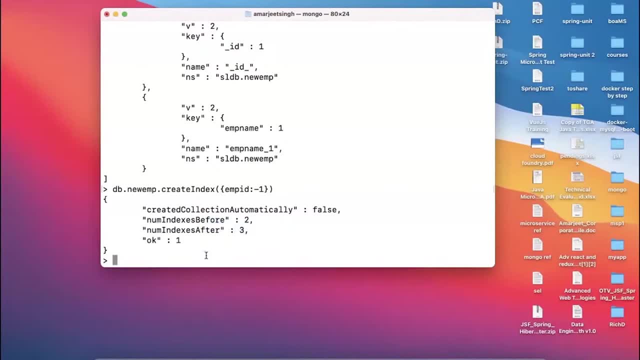 So it is very clear that index is improving. Now let's check this out: DB dot, new EMP dot. get indexes. Now we have a total number of three indexes are available, So you can apply index or n number of columns if you want. 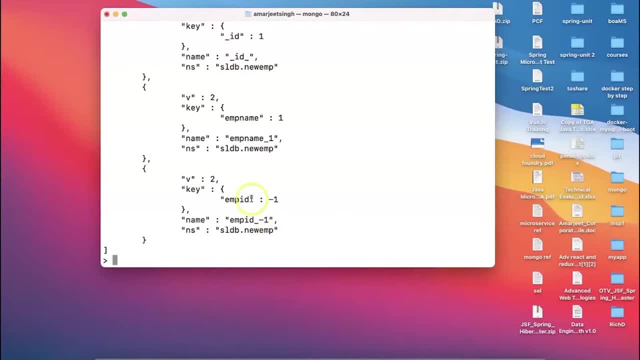 Okay, At the same time, the way we have created the index, in case if I want to drop an index, So we can also drop. So what we can do: DB dot new EMP dot. drop index, drop index. and in this drop index we have to provide which particular index we would like to drop. 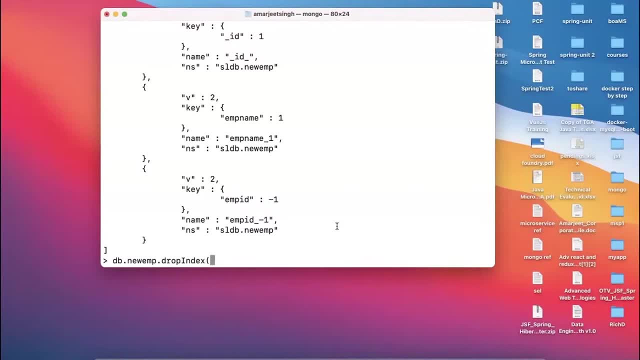 Remember this point. Okay, We are not trying to drop any sort of index, So you need to provide which index, So you should have that particular index name. Okay, So here we are providing my index name, So it should not be- I would say, the traditional name- called EMP ID. 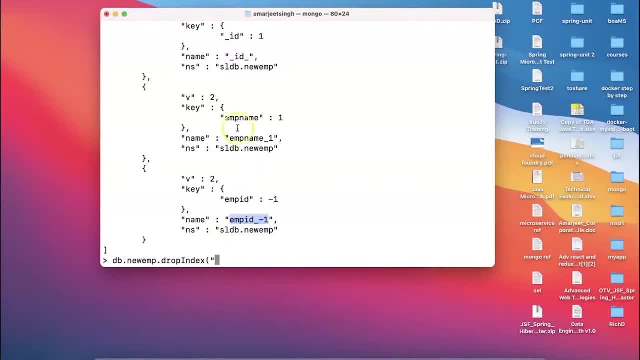 No, it has to be EMP ID underscore minus one or EMP name underscore one. So this should be the name. I'm saying EMP name, In case, if you try this You see It is saying index not found with the EMP name because internally it maintains with 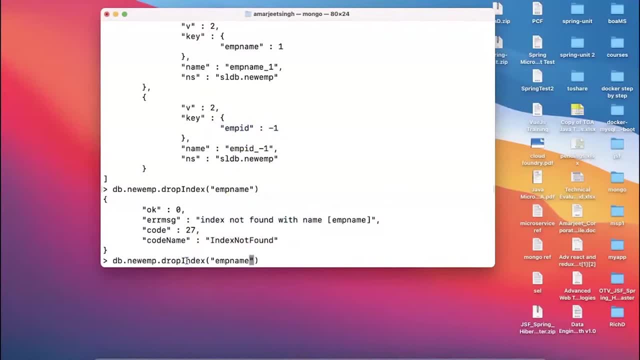 this name. Let's try this out. We say EMP name, underscore one, Let's try. And now you can see new index was three Okay, one Okay. Now you can see we have a call, EMP ID and underscore ID. So 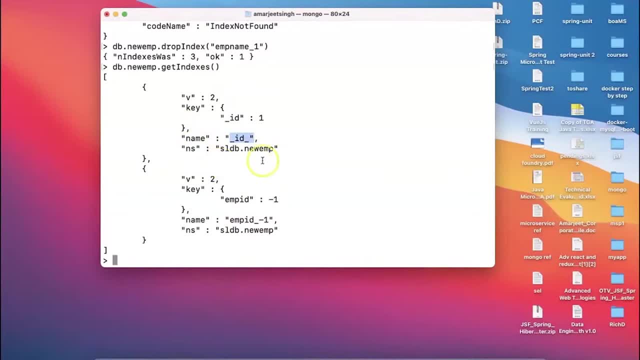 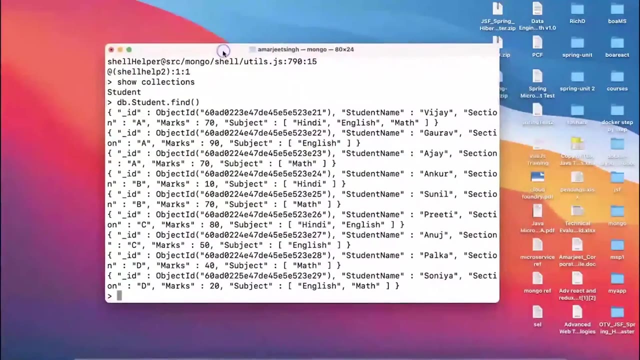 Now we have only two indexes left. There's no EMP name anymore. This is how exactly you can drop the indexes. So it is very simple and straightforward way of how, in MongoDB, you can perform your activities. Hello everybody and welcome back. In a previous examples of MongoDB you might have considered. 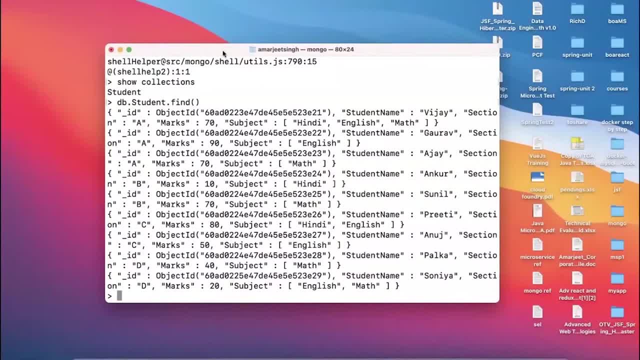 We have used lot many operations. in our last video we have seen how to utilize indexing into our code. Now, in our next journey of our MongoDB, we will see how aggregation works. See, in MongoDB, aggregation plays a vital role and aggregation comes with so many handy functions. 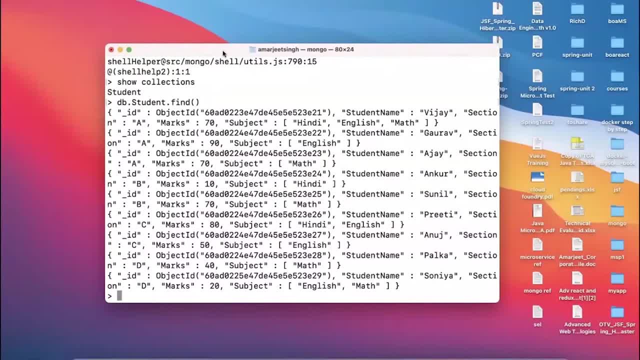 with MongoDB, which will help you to perform and to apply some very simple code snippets into your ongoing, I would say the requirement which can make your query so much seamless. Now we will see. Now we will see how this aggregation really works, and to work on an aggregation we have 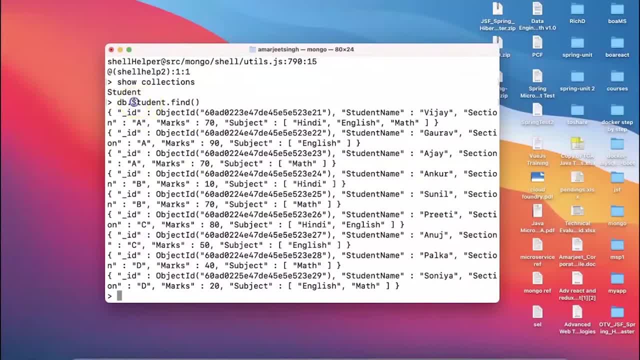 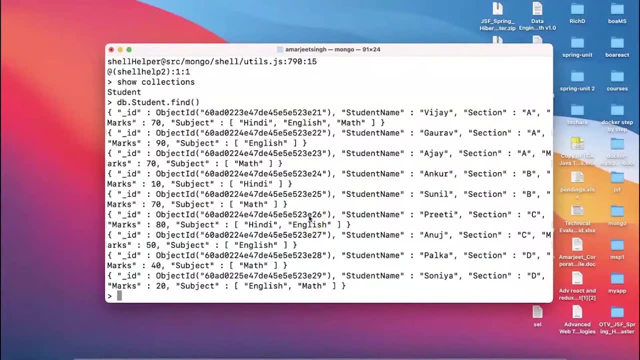 taken some default database name called aggregate DB and here we have a call student as a by default collection in which we have some set of records are already added. Now, if I just want to apply aggregation now, I would like to tell you about what exactly the aggregation is. 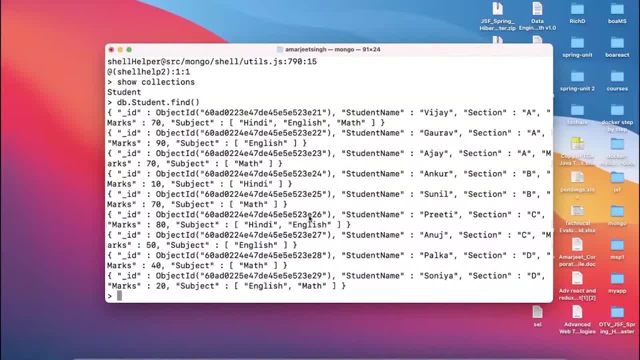 See ideally when you talk about call aggregation. Okay, So Aggregation is nothing but a call aggregate, like already we miss if you see biblical aggregation there. So the Unix command, like you talk about shell pipeline, means the possibility to execute an operation on some input and use that output as an input for the next command. 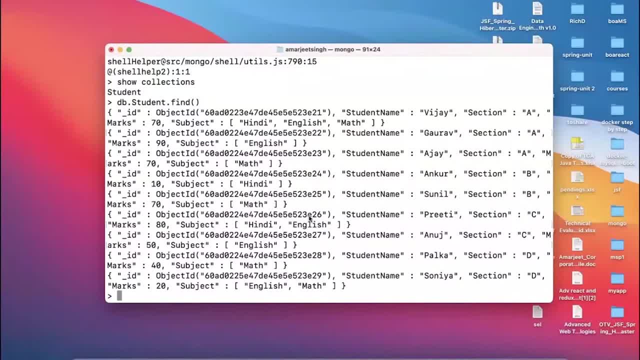 That means the output of one particular execution becomes an input for others. So MongoDB also supports same kind of concept. in aggregation framework there's so many type of Functionalities are available, which we will see one by one into our next code. Okay, Now here we want to confirm about a few important things. 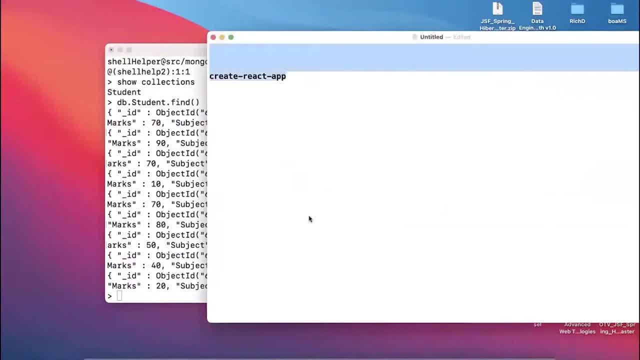 Now here let me try to bring some of the important, well known, I would say, the functionalities of our aggregation framework. First, we use a term name called dollar project. The project is basically designed for select Specific Feeds. Dollar project is designed to select what is specific fields from a collection we used. 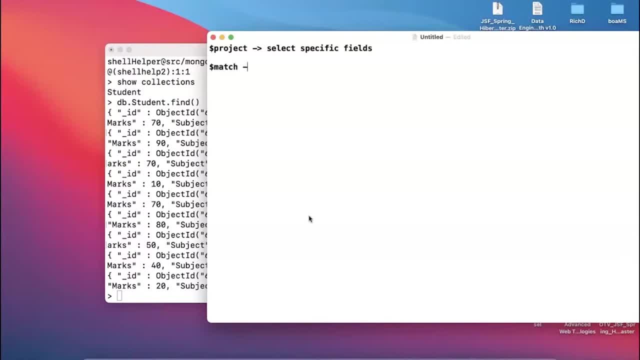 to talk about called what Dollar match. The match is responsible to filter out the operations. Are we clear now? It is designed to filtering out the operations. You talk about dollar group. Talk about column group. You talk about column group. You talk about column group. 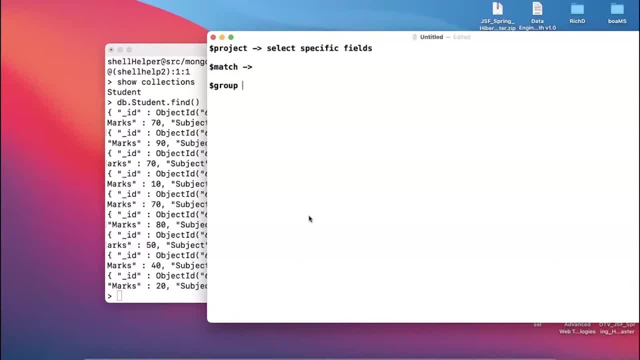 You talk about column group, So it does the actual aggregation. Fine, We talk about call Dollar sort, Okay, It basically sort the document. Okay, Like that. there is so many operations are available that you will see one by one in our aggregation behavior. 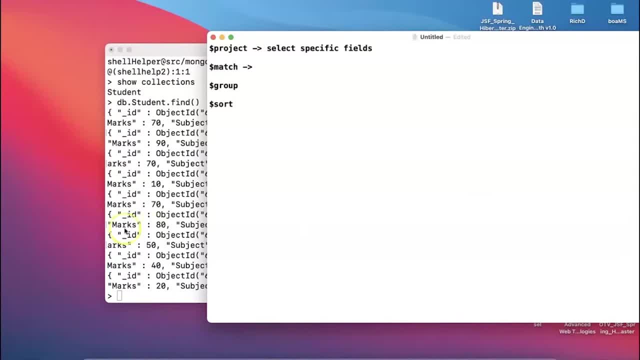 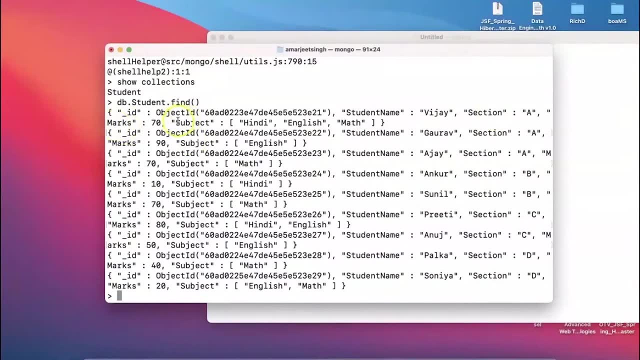 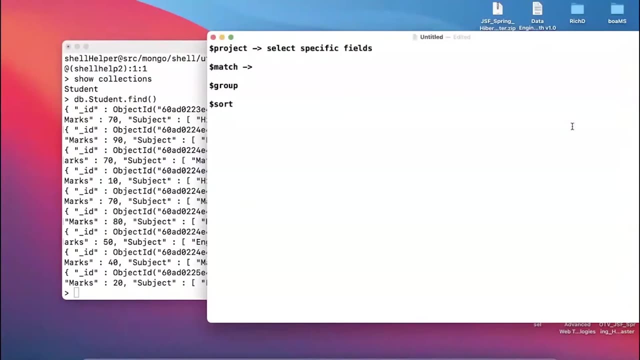 Now my first example, the one which I want to execute. I have a called student record with me which contains the student name- Okay, the section And the marks And the subject, which subject the person or the student is appeared now here. my first requirement is: we want to filter data based on a section a, because students 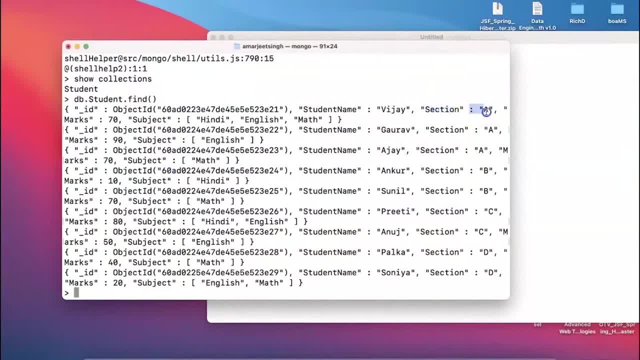 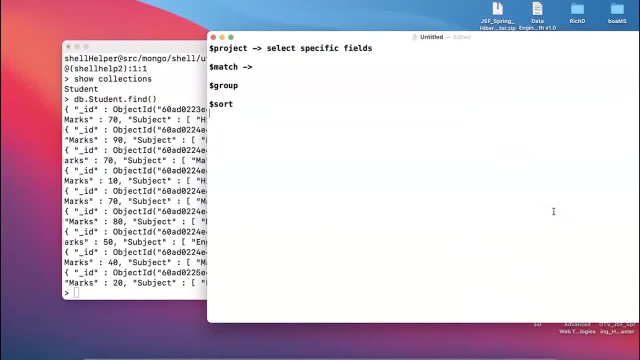 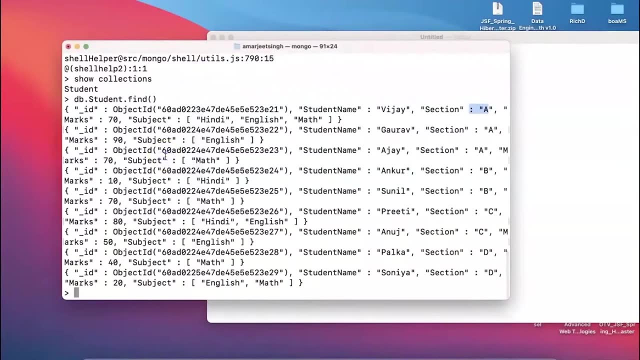 belong to different sections. as you can see, now it is a, they belong to this different section, section ABCD. so I just want to filter the data based on a section a. okay, so for filter out I would like to use dollar match. let's see how it works. so I just would like to filter out only those students who belong to. 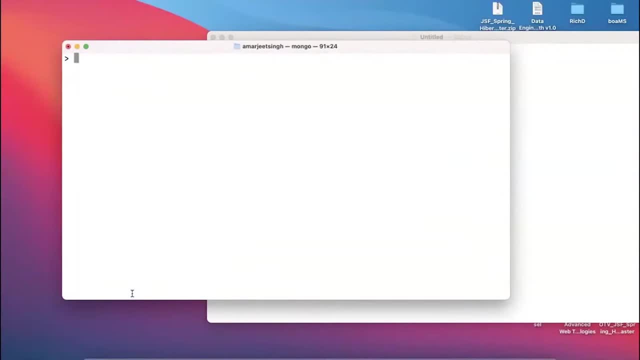 the section a. so how you would like to use it now, I will say DB, dot, student, dot, aggregate, and inside this we would like to use this square brackets and then curly braces and then use dollar match match with this. I would like to use another curly braces and I say section a: okay, 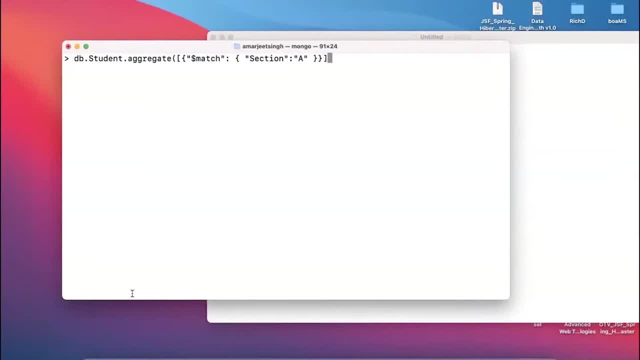 and I close this, close this, close the square bracket, close this. okay, so DB dot, student dot. aggregate aggregate should be always associated. match is not the aggregate functionality section a. hit enter and it will take care of your Hit enter and you can see now it lists down all those students who belong to the section a. 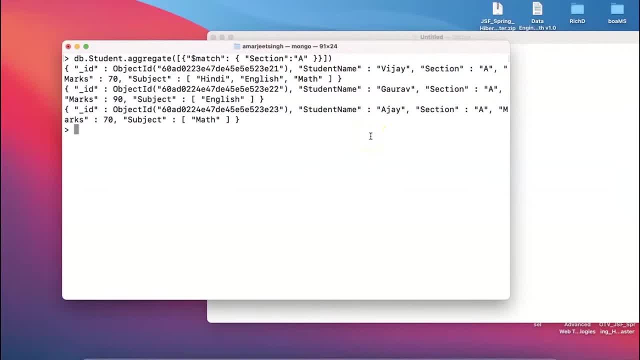 Okay, very simple and straightforward example. Now we would like to use the second example. so we want to find out all the records where this section is a and we are using and operator marks is Greater than 80. There are so many students over different marks, like 17, 19 and whatever. 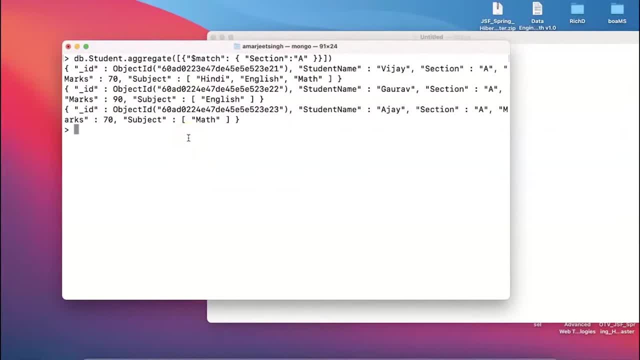 So we want to use both the conditions together. So how are you going to be using this now? Remember not only the section a, but also marks over greater than 80. So similar thing: we have a call match. Okay, after this match, we are starting this curly braces. 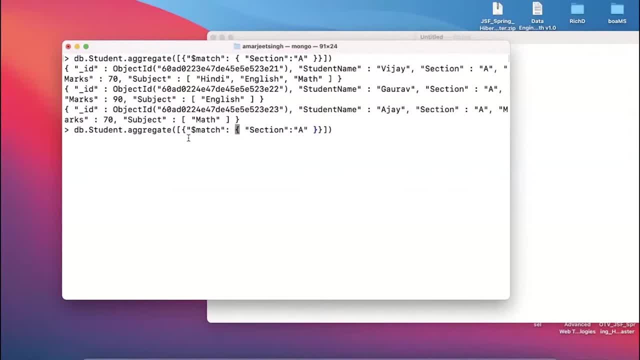 Okay, so after this match, we would like to bring and We say dollar, And and again colon. again We are starting. This is quite like it now. Okay, we talk about what section? a number one, and after this, the first Curly braces. we would like to use marks. we say: 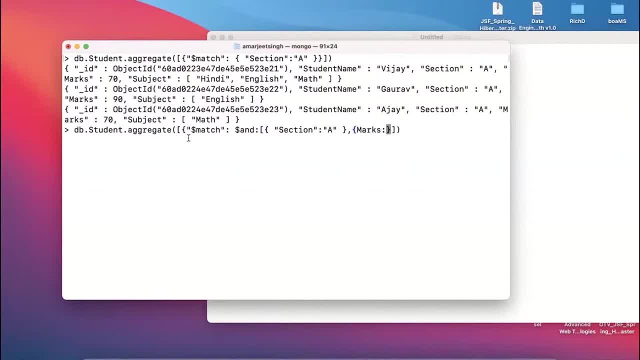 marks colon and I once again. They would like to start curly braces, and here we use Dollar and JT. that is called what a greater than colon 80. Okay, all are closed. so you see, like here we have got this square bracket and noun brackets. so What else is left? 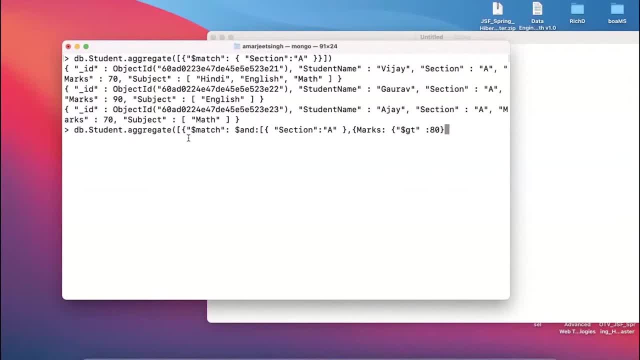 So we have a call 80. we are using another. curly braces needs to be closed here and then square bracket, okay, and followed by again curly braces, again, curly braces, again. square back it again around packets- Okay, Let's see where it is going on. So we are using this. DB dot, student dot, aggregate- We are use this. 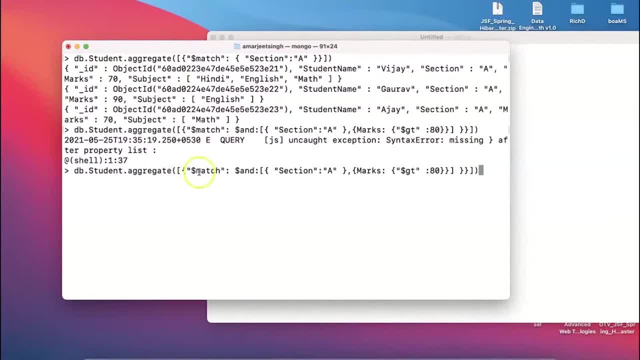 Yeah, square bracket, then curly braces and we use dollar match. okay, after the dollar match We are using another curly braces and you call and operated after this and we have a call: Let's go around: square bracket, then curly braces, section a Out. this section is getting closed. We are using another curly braces, marks colon, dollar GT. 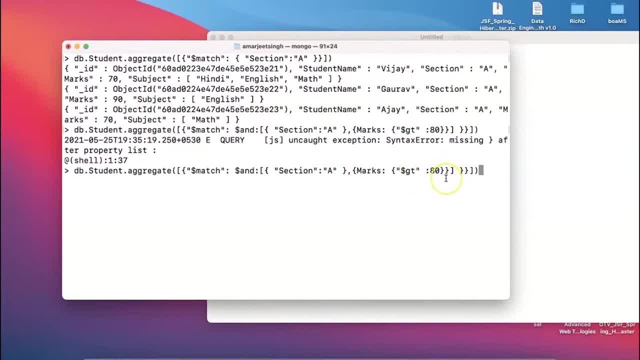 Okay, and we are using what? colon 80, after that we have closed this and using two more curly braces, square bracket in this. okay, so this where exactly you can utilize that. so DB dot, student dot, aggregate, and like this it will be able to get it now. okay, so in a previous example that was the only. 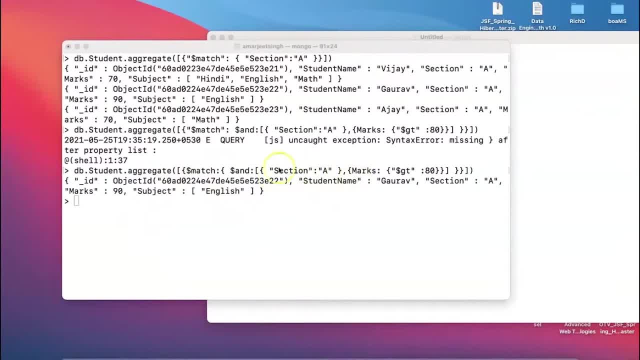 missing point was after this, this dollar match. we didn't apply this curly braces, that was only missing point which was there, and now we have applied. another code is giving me this outcome and I have only one user who's scoring greater than 80. well, that was the first thing which we have it now along with this. I. 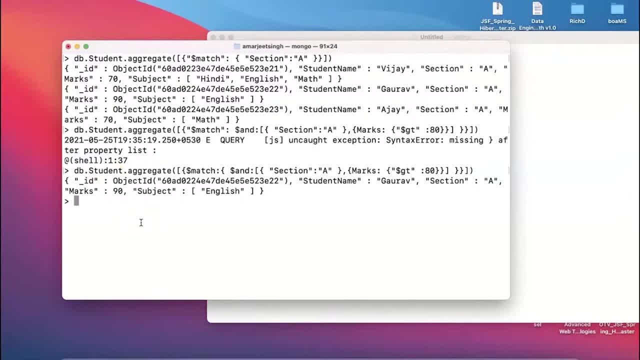 would like to go ahead and talk about few more things now. I just would like to bring selective fields, not all the fields, like. as you can see, we have a call student name section marks everything I'm getting it, so I really don't want to bring all the properties from this document. I would like to 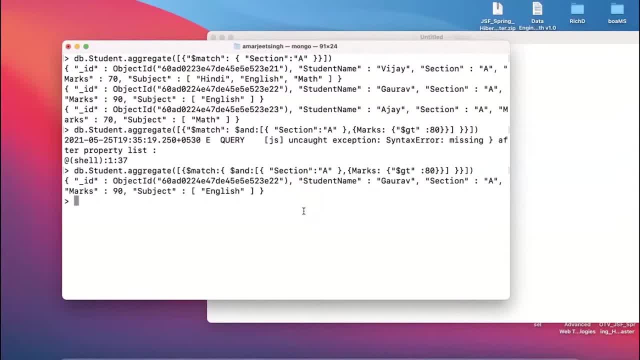 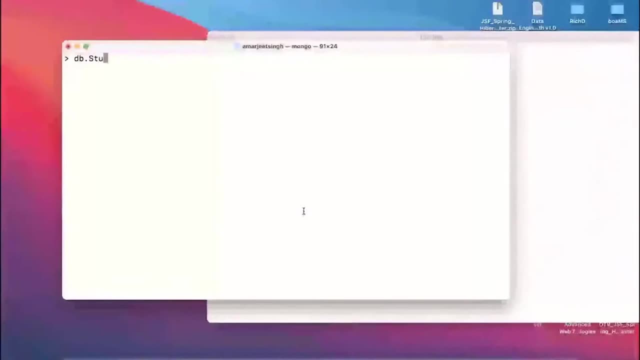 selectively takes specific property. so let's talk about how we can use this. so we'll be using project- you remember about project is responsible to select the specific record. so I just use the statement name called DB, dot, student. okay, dot aggregate. we are using it now. after that: now square bracket and curly braces. 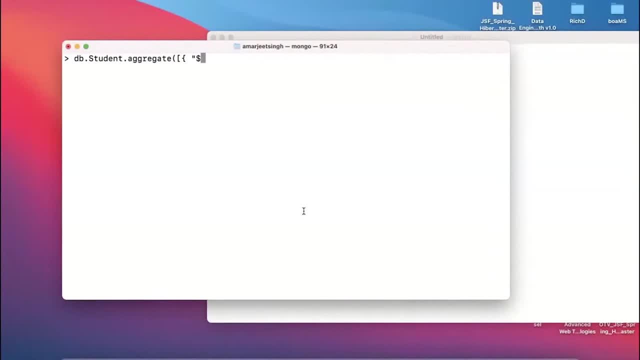 now we are trying to say dollar project, what you would like to use, dollar project. and colon. we are trying to use student name. okay, colon, okay, remember one thing: one means I want to, zero means I don't want, so whichever property will be enabling it by giving the one as a digit, that means it is. 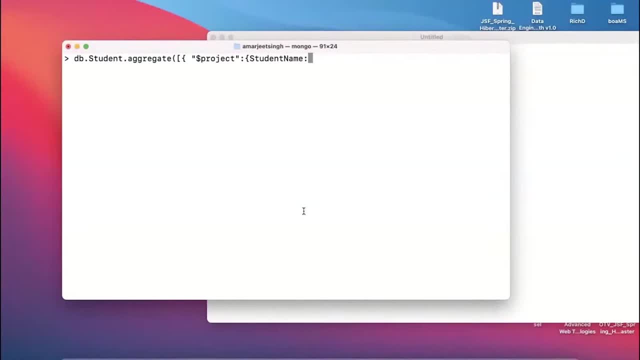 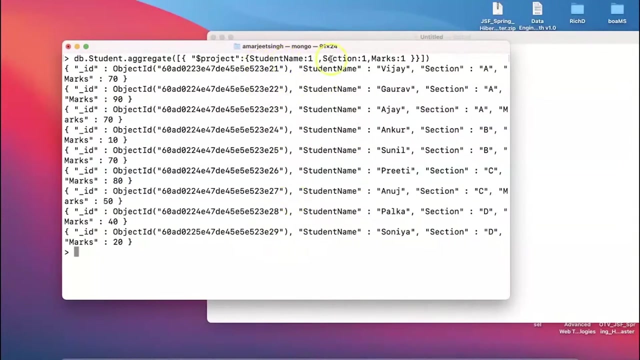 it is expected to be displayed. so I'm saying one comma, I'm saying section, colon one. okay, and I'm also looking forward for marks, colon one. that's it. so now you can see, now I am once again picking up only those like student section and marks. now if I go back and remove some properties like 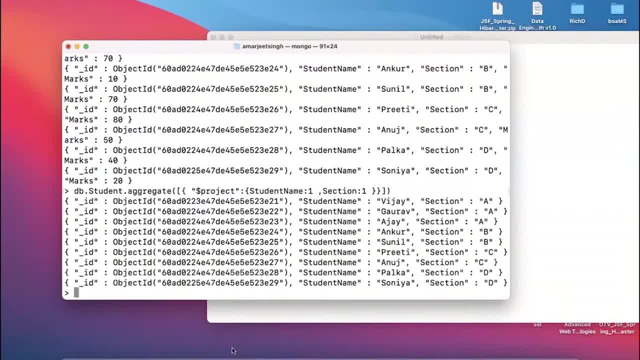 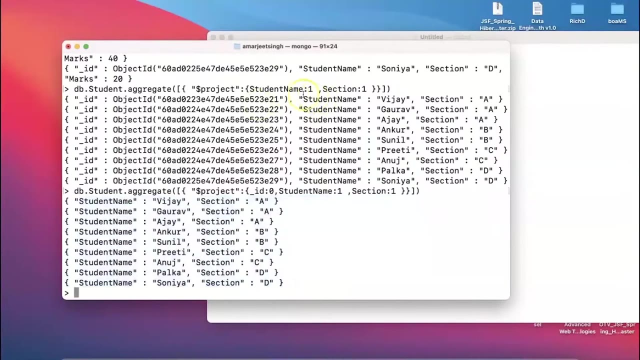 I only want a student and section, you can see I have only student and sections are used here. if I just use this a statement: name for underscore: ID colon zero, now you can see only the names and sections are visible. ID is not because I really don't want ID. by default ID is shown. but if I say: 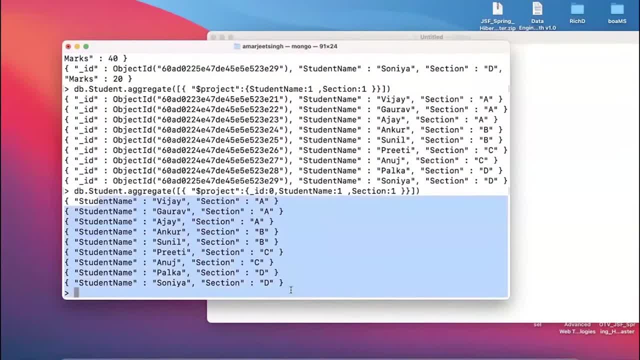 zero, that means the ID will not be visible here, so like that, you can select the columns or the properties accordingly. that was a one-way. now one other thing I would like to use: what if you want to find out the student name section and marks from student? once again, we want to find out the student. 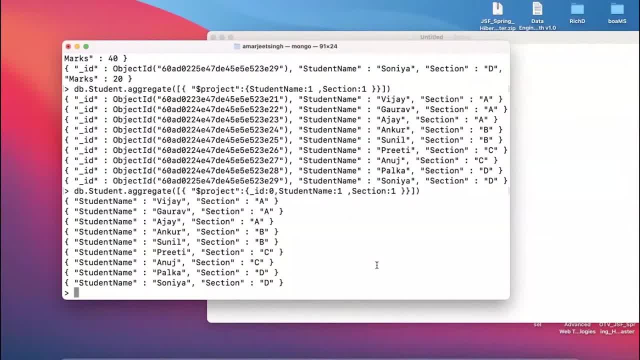 name section and marks from the student collection, where the section and marks are not visible. so I'm going to use the student name section and marks from the student collection. okay, so here it will be the combinations of match as well as the project, how we can use this. let's take a look towards my implementation. if you see the previous, 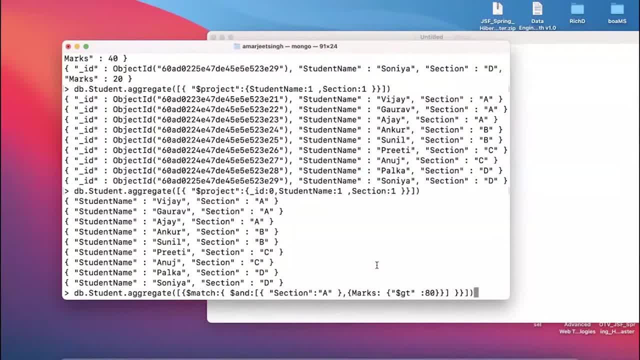 one. what we have used here, you remember about, we have used this statement called aggregate match. okay, so now we would like to go back and utilize, after this, dollar match. this is a curly braces. I'm giving section colon a, okay, section colon a, and after this I'll close this. okay, and close this again. again. I'm opening it up by using: 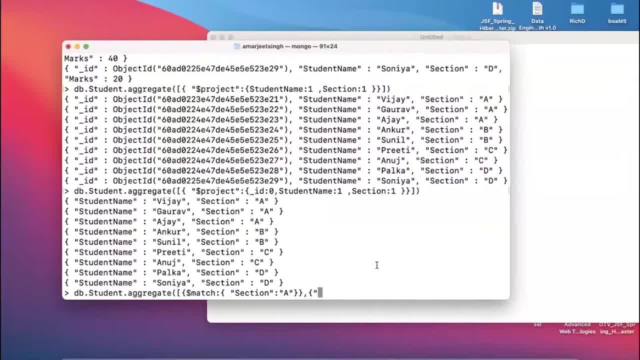 this option called process. okay, so I'm going to go back and use this option called process project, dollar project. we're picking up the project right now and here with this colon symbol we can use again and say student name, student name, colon. we're using one comma section, colon one and 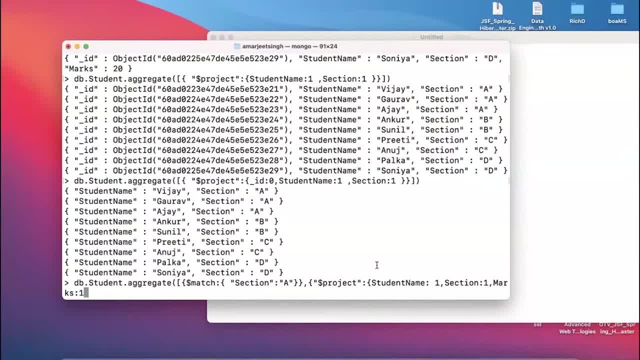 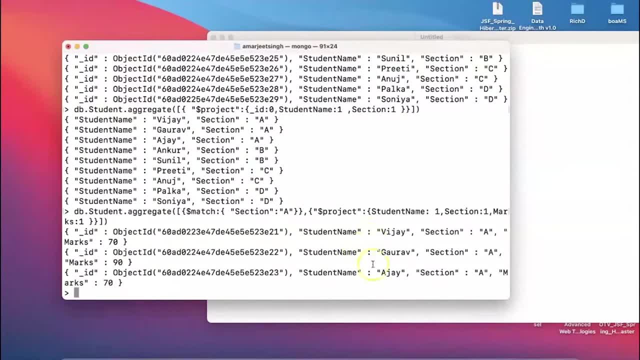 now closing this. now you can see I got those. so the requirement was: we want to find out the student name section and marks from student collection, with the section is a. so you are not only using the match okay, but also using what the selective. that is like this: you can. 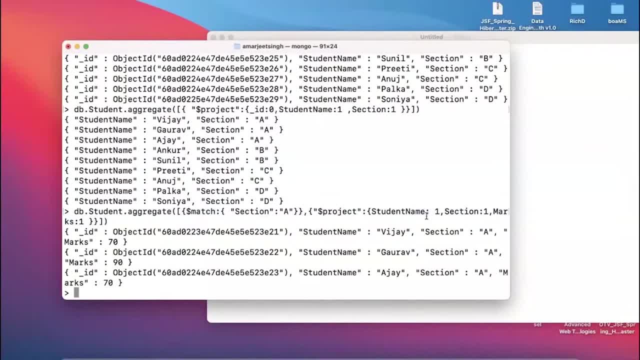 implement it okay. that's where exactly the projection really works. so projection gives you lot many opportunities which you can utilize it for your own, and also it comes with lot many predefined functions, like in some avg and on, so let's talk about those functionalities too. so this is the first thing. 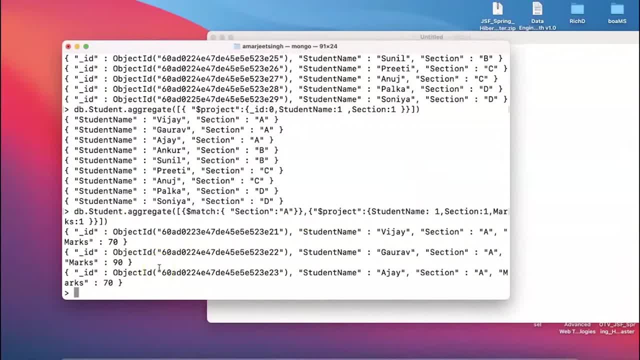 which we have seen aggregations are taking place. now in case, if you would like to perform the group, like if I want to find out a total marks group group by okay section, like each and every section, I would like to confirm the total marks in every section. then how do I basically do that? so let's try to get. 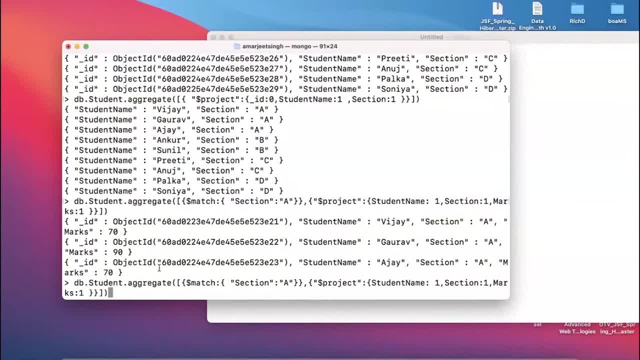 this example also. so here let me try to go back, and we will not be using match here because I would like to use the group part. so after this curly braces, we want to use dollar group. okay, let's go group by an ID. we miss how you use it. here we use this curly. 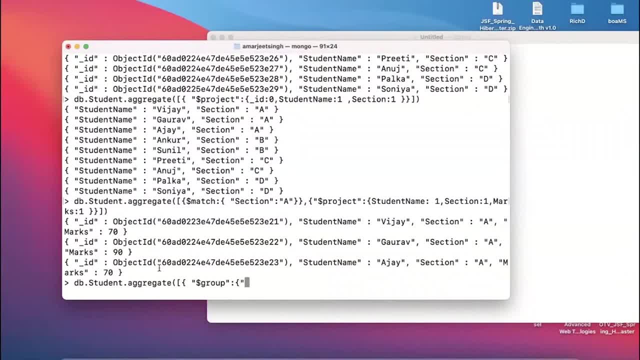 braces. again, here we are passing this underscore ID. okay, you have to provide underscore ID in a group because you cannot skip it. that part you need to be always remember. you really can't skip dollar ID whenever you're trying to talk about code group. this is a compulsory field. you need to have it. 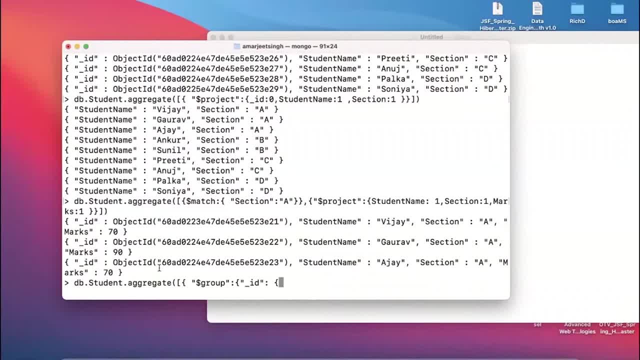 after that, now using this section, in this section we are saying dollar section, as we would like to make an initialization of the chose it on a section basis. after this closing, and here we are using what total marks seekers is similar to the fancy store. I don't need to ж pasado. 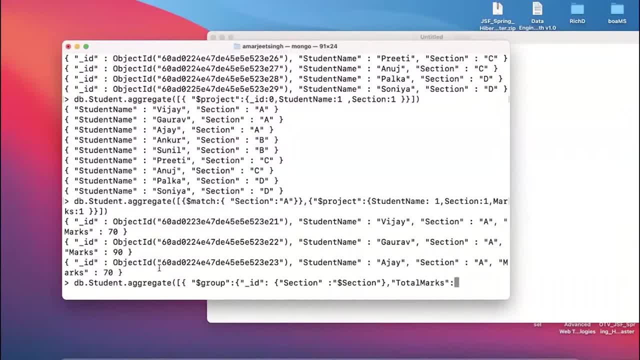 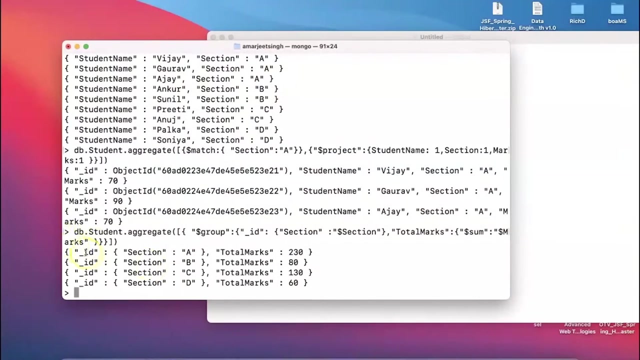 map colon here curly braces again dollar some okay, colon on which behalf I want to use in mark so I can say dollar marks. naming convention is very important because it is a JavaScript, so it is a case sensitive. okay then, and you can see now section wide, I'm able to get all the marks. isn't, is an. 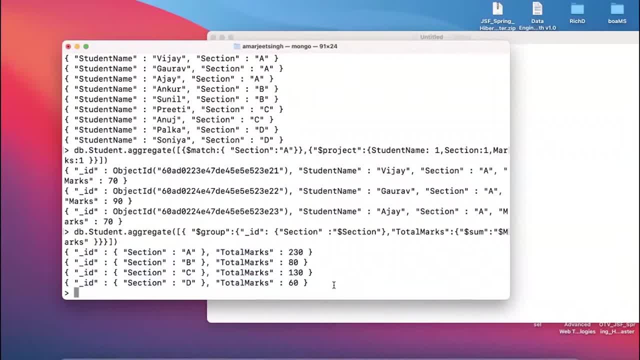 amazing. that's where exactly the aggregations are playing very important role while retrieving such kind of records. so hope you're clear about how we utilize this together. so in a previous example we got it like how you're basically taking this marks in my application. fine, so we are clear about. 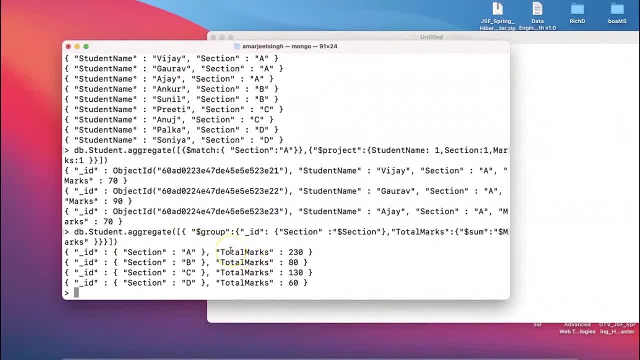 how we are picking that up. but what in case if I would like to take marks for the specific section? so it is also possible. so we'll be using the same group, but only thing is what will be bringing the match between, because here we are trying to get the all the section. 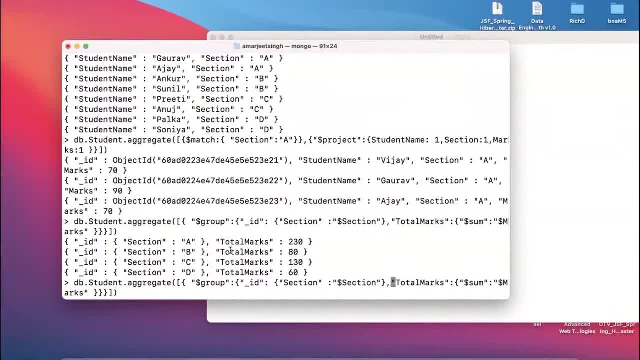 marks. but if you would like to bring it only for the specific section, we know it very well what we need to do. so here, before I talk about called dollar group, we can use one more curly braces here. okay, so we can use this option called dollar match. okay, and here we are using this option called section a. so here, 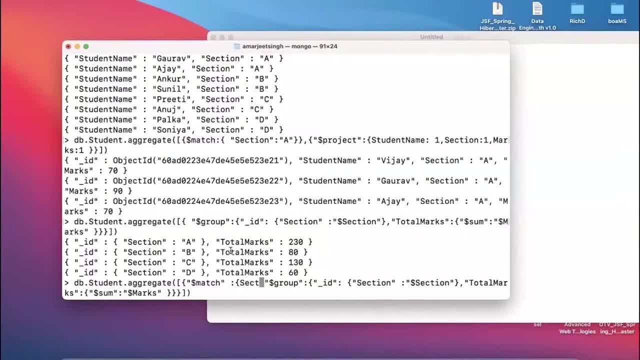 in dollar match. we are giving this call section colon here. we're giving this for closing this. closing this followed by the other areas, like a group which you want to start now so you can start with this curly basis. hit enter and you can see now only the specific section here. you want to receive the. 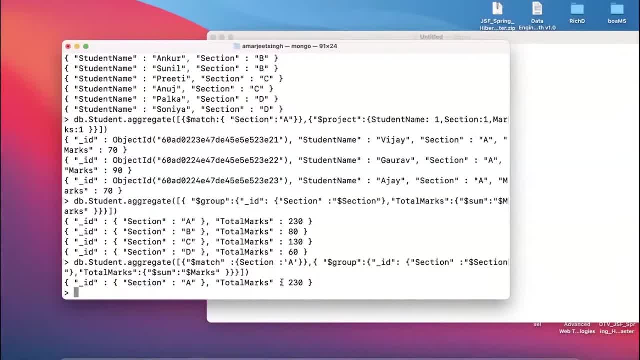 records and that's very simple now. okay, so that's where exactly you would like to perform and there's another option, like it's in case, if you would like to perform at an average, suppose, if you want to fetch the count of students in each section and total. 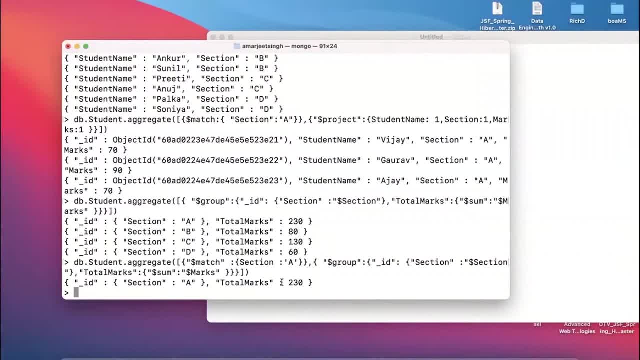 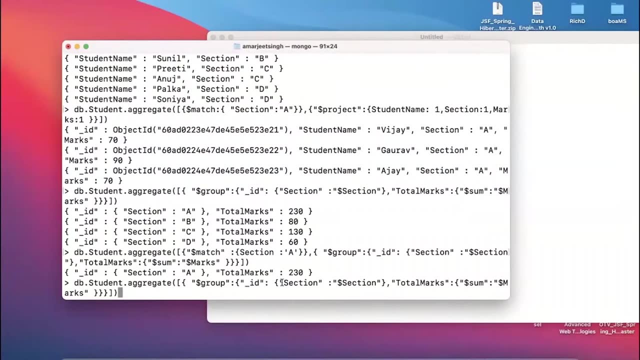 marks and average marks as well as so total marks as well as the average marks. we want to get it so, however, able to take it now. so it is very simple, as you have seen earlier, also into a code, how you're taking called group underscore ID section. talking about section total marks, with the sum we are also using. 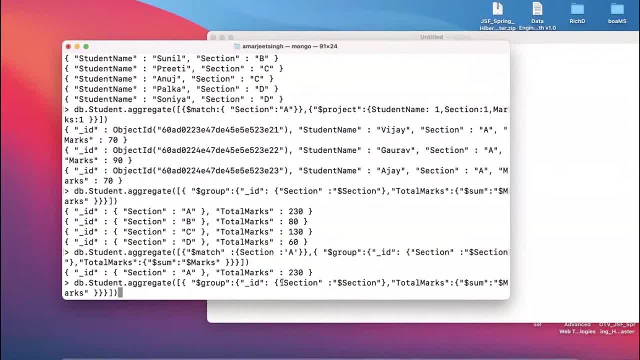 this. after that we can also use the average. okay. so this is we have taken called group underscore ID sum. so here onwards we will start so when we say some marks, after that we can just put curly braces and we can just use count. okay, and after this we'll be using this colon curly braces and use dollar. so okay. 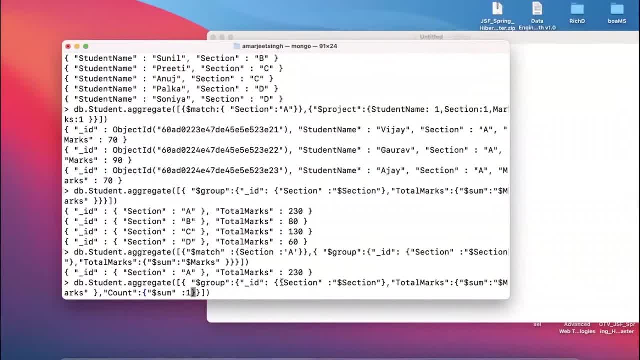 colon 1: okay, and after that I'll put comma here and we use average, and inside this average I will use in curly braces we can say dollar, a BG. okay, colon of what? dollar marks, very simple. so curly braces is closed. okay, so total how many? three, three, three, three. 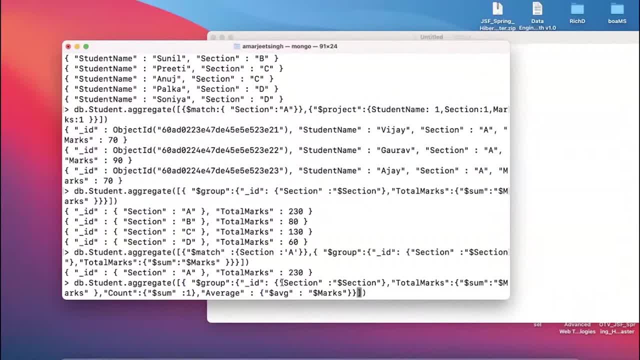 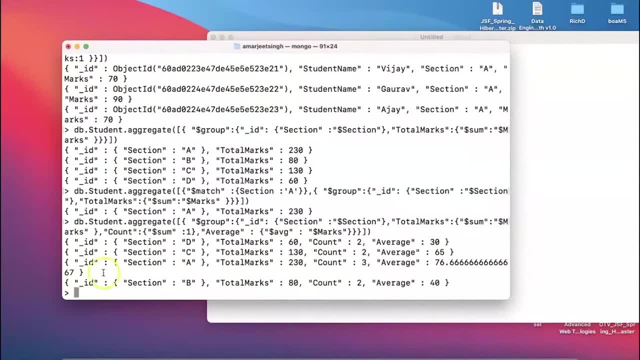 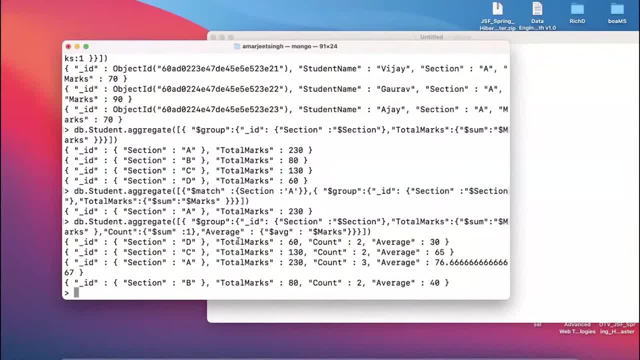 aggregation seems to be very, very simple approach, provided by mobo TV, that really create a difference of how the aggregation changes the way how you react, okay, everybody. so, after going through the idea of like how we can utilize the concept of our aggregation, it's time to talk about like how, when it works with. 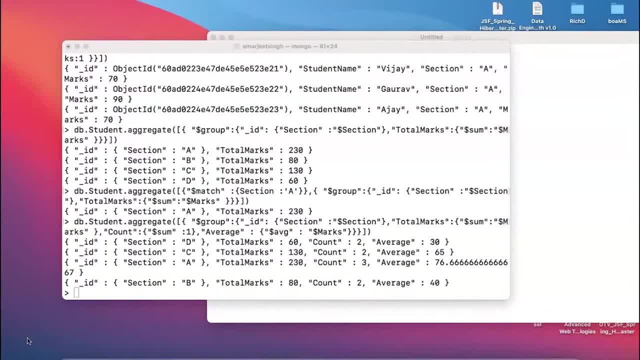 mobo DB. mobo DB is properly known for, I will say for replication. that is called high availability and that feature comes by default with MongoDB. you really don't need to install any software for this, because it is a built-in feature for the MongoDB. so when you download that, it comes along with this, so no additional. 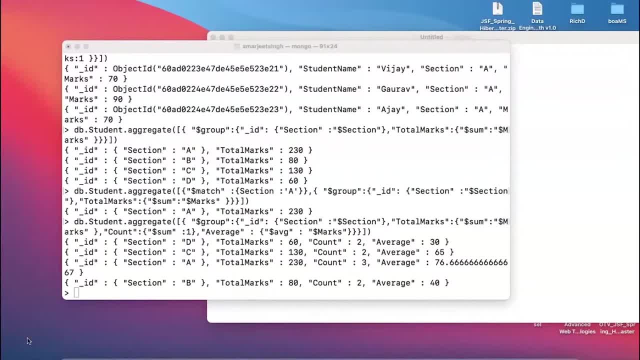 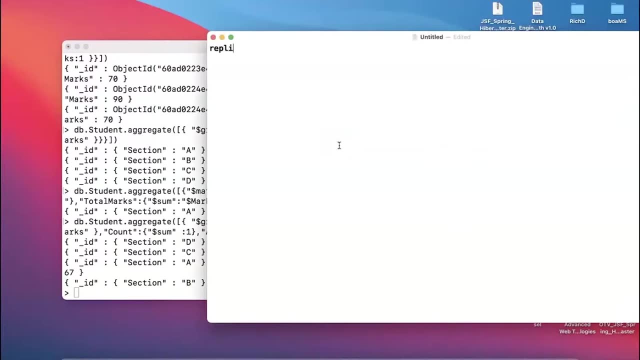 configuration setup is really required. when it comes to the MongoDB part, okay, so let's get started and talk about how MongoDB can offer the replication. see, the idea behind the replication is what the idea behind a replication is like. you are replicating it. okay, so we'll talk about cause application you are. 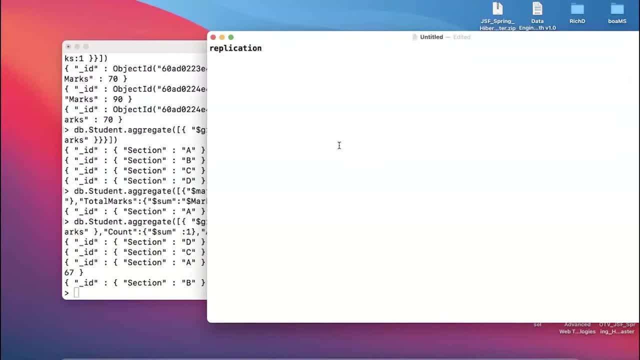 replicating your data to it, to multiple child. so here, MongoDB, we have one concept available, okay, that is known as called master. okay, and slaves: okay, master is one and there will be multiple slaves. okay, so these slaves where your records are actually stored, and this is a master which will 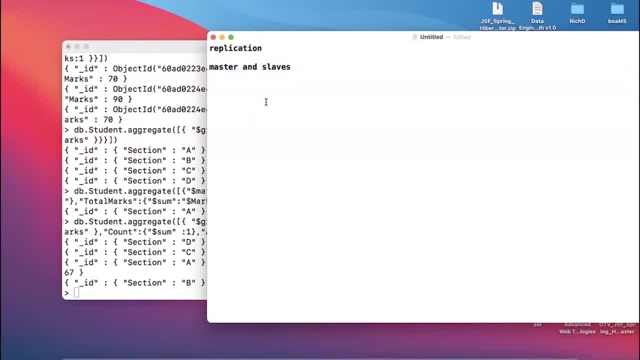 be responsible to replicate the data to all its child's when the request comes. due to that, in case, if one particular node fails, so automatically, the data will be taken from the other nodes. that's the beauty of having this master and node slave process. so to make this possible, we have a very simple option. 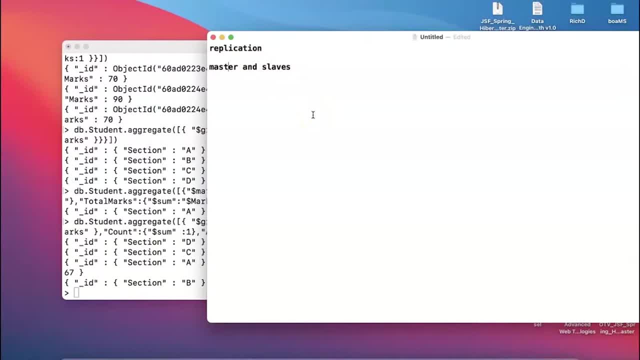 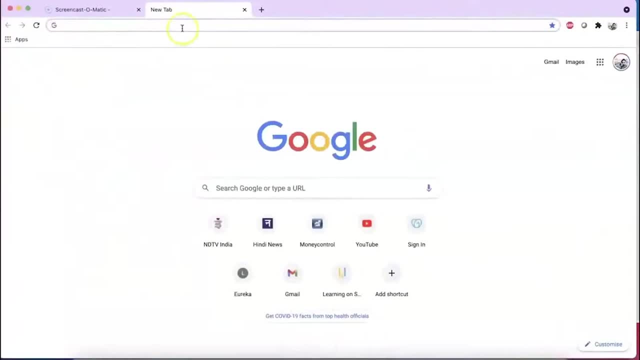 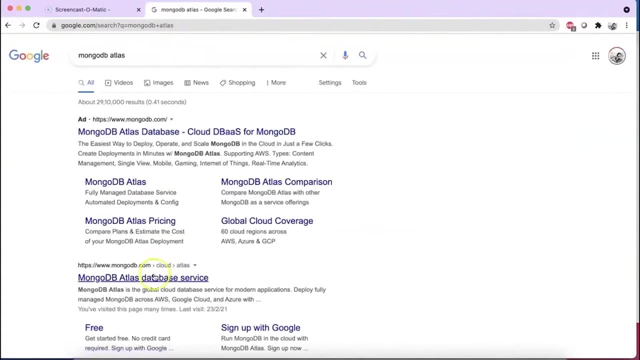 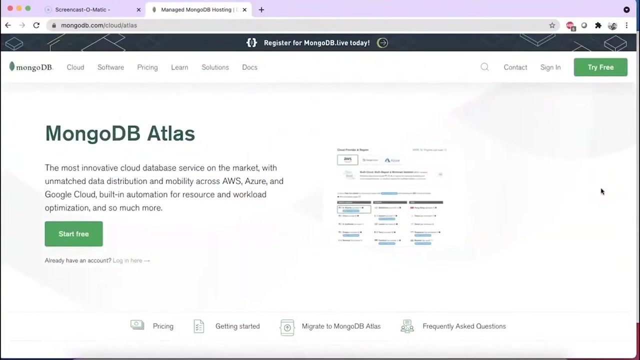 available in MongoDB. we have a one concept like called MongoDB Atlas, so there we can go and get our cluster ready. so here we start with the concept name called MongoDB Atlas. let's search for MongoDB Atlas and here I see MongoDB Atlas database as a service. see, this is a free tool. it's a cloud environment where you really don't. 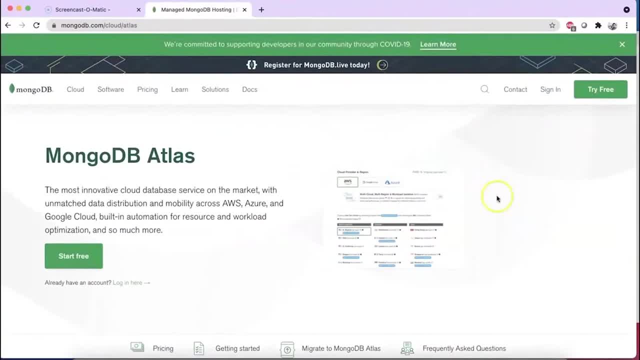 need to install MongoDB in your local machine. it is a cloud-based MongoDB support which is free to use, with a limited amount of space. but yes, for the testing purpose that is the best suitable. so I can start with the start free, or else I can say the login here. 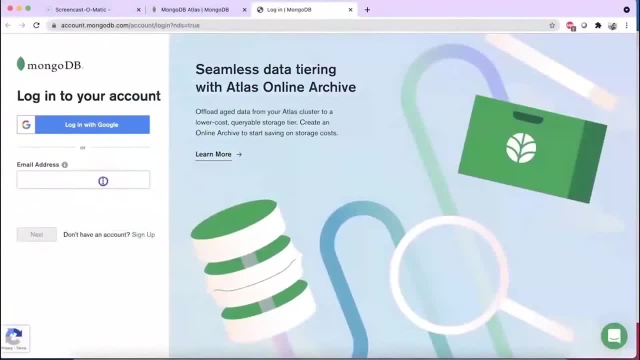 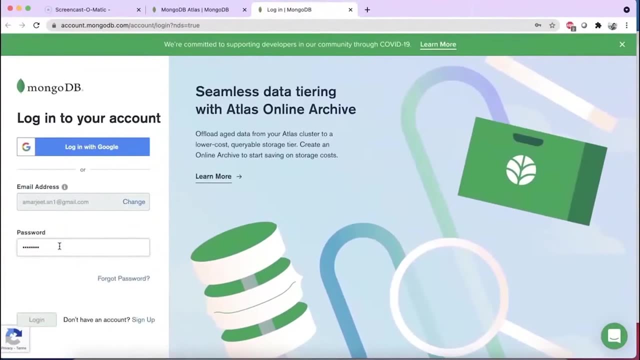 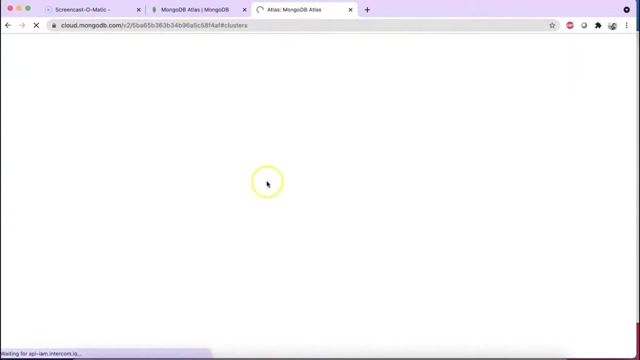 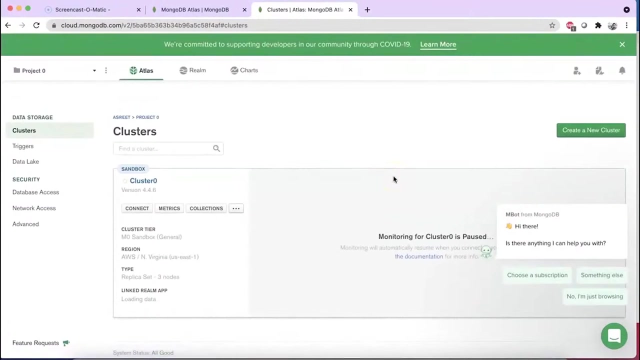 okay, from there onwards, I can go ahead. now it is getting ready. now this is a place from where you can start working on your cluster. see, as I've told you like, initially, when you will be working on this MongoDB, it will ask you to create a cluster initially. okay, since I already have a cluster with me, okay, so? 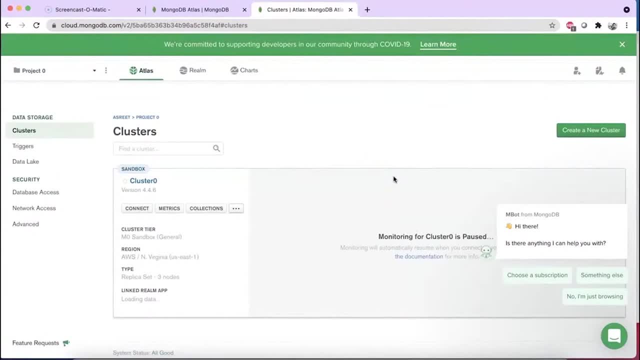 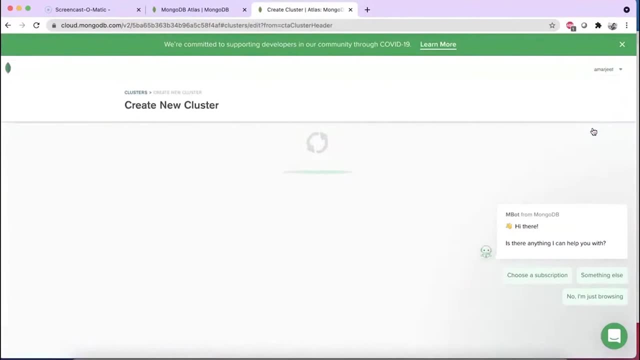 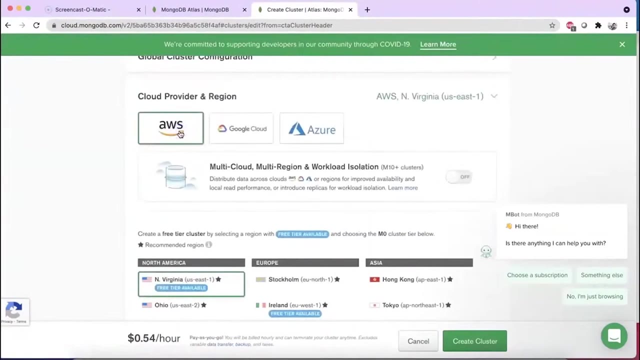 I really don't need to create it and as a free tier, it will not allow me to have more than one cluster set up ready. so if I say create a new cluster, okay, and I say by default AWS okay, and I've been closed on this notification, AWS is a. 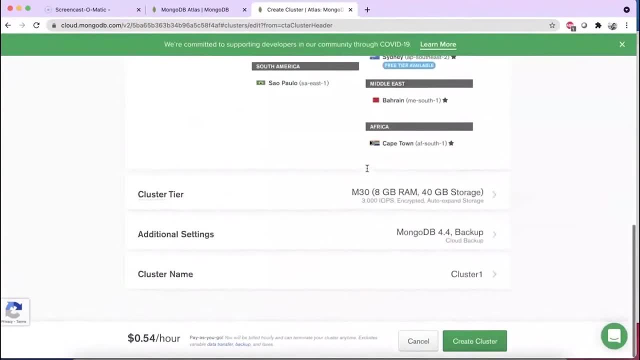 very easy way to create a cluster and AWS can select any of the cloud provider and a GB RAM cloud backup cluster name. you can see now it is taking me point five, four per hour. reason being: because I already have a cluster with me. hence, more than one cluster is not allowed in a free tier cluster, so I have to cancel. 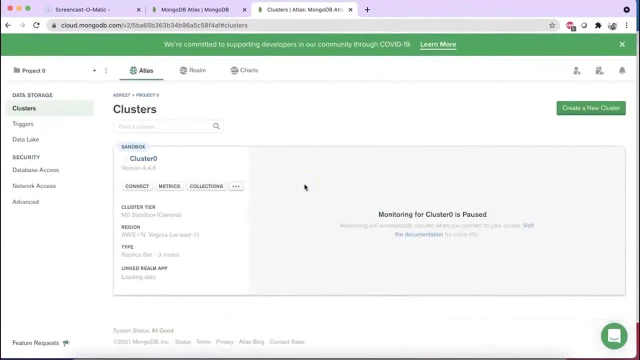 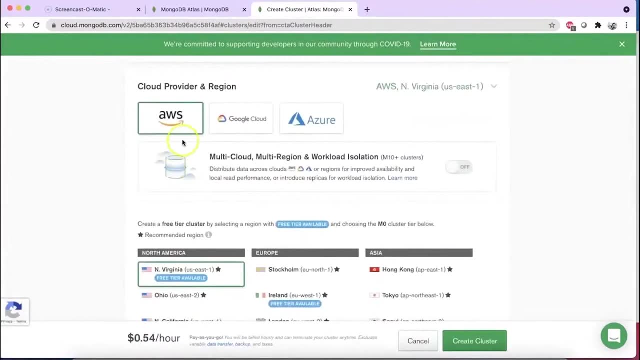 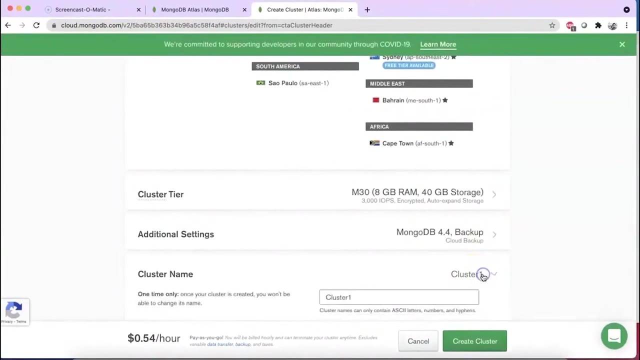 this, but you can go and create a cluster the way it was offered there. so if you want to create, you can just go ahead and del nothing. just select by default. aws, select your location. okay, give the name of the cluster. you want to give anything, you can give it here, otherwise let it be the by default name. 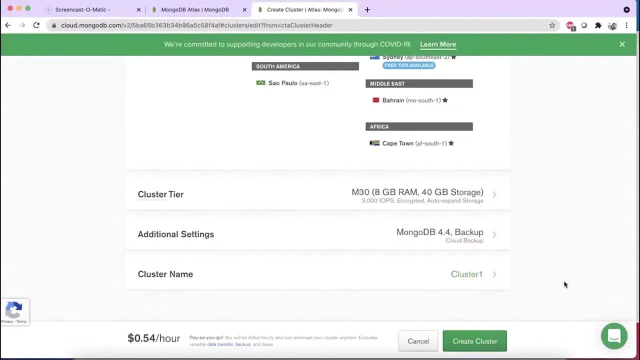 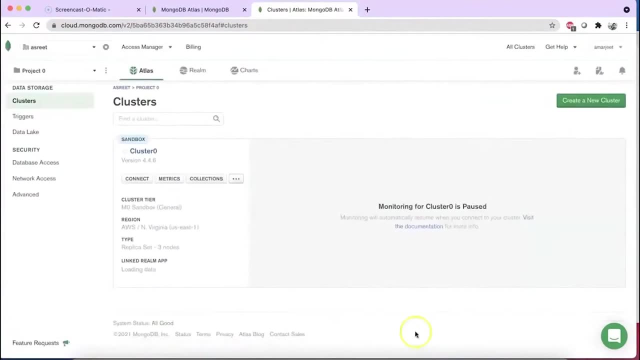 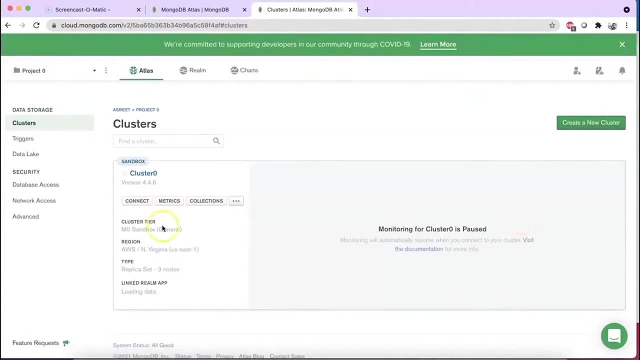 cluster. when they create cluster it will take a while- minimum two to three minutes depends on the availability. it creates a cluster for you and your cluster. once it is ready, it looks like that. okay, so here in this application you have to go back and understand what is there in. 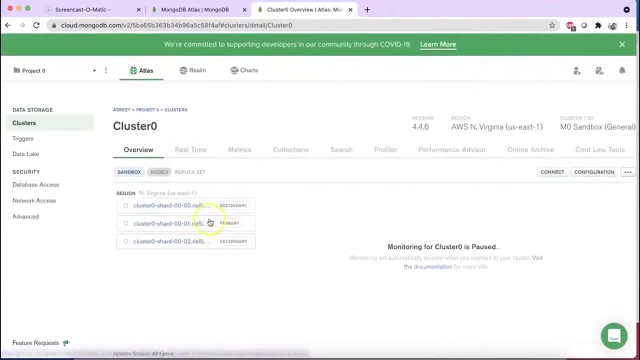 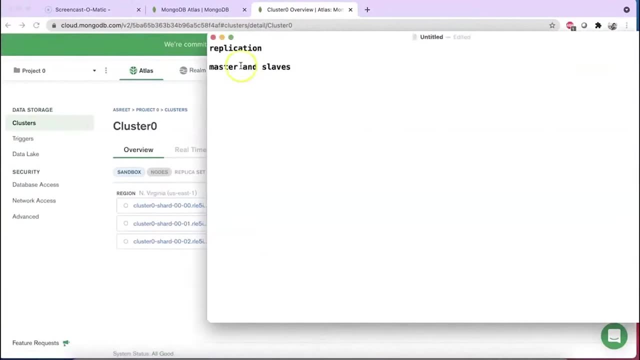 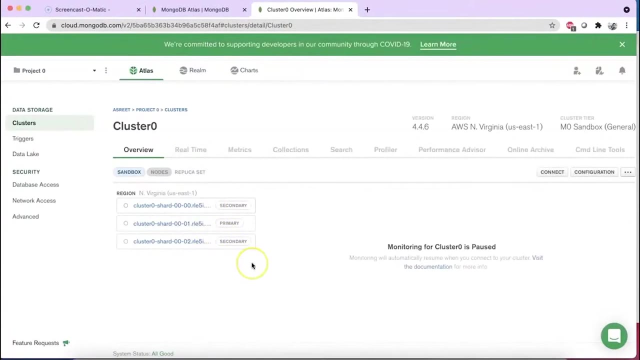 a cluster. so when i click on cluster 0 you can see: now here we have got three nodes available. one is called primary node, which is called master, as i suggested earlier, and now we have called slaves. automatically when the clusters are created inside this mogul db, by default it will be three. 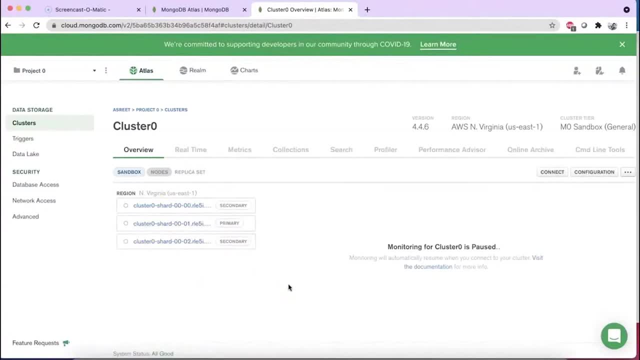 node cluster where the one will be the primary node and the other will be the primary node, two will be secondary. based on your package, whichever you have taken it, you can increase the number of nodes later on. but as a free i'm gonna get, or i will be receiving, total number. 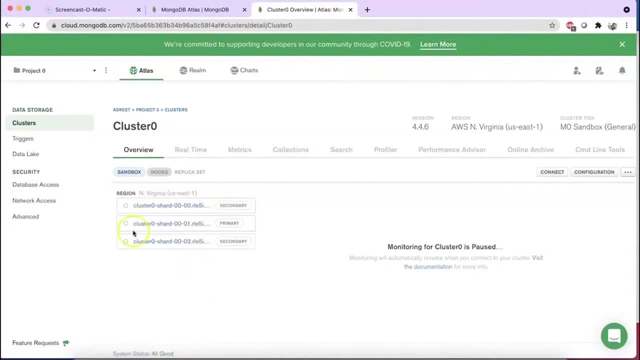 of three nodes available here. so records, whichever will be stored, it will get stored automatically in both the nodes- secondary nodes- and from the primary i can insert the record and secondaries i can read the records. remember you can't insert the records into the secondary. you can only insert a record only in your primary record. secondaries are not allowed. 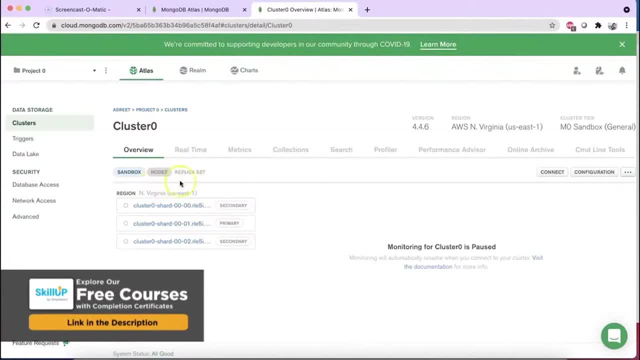 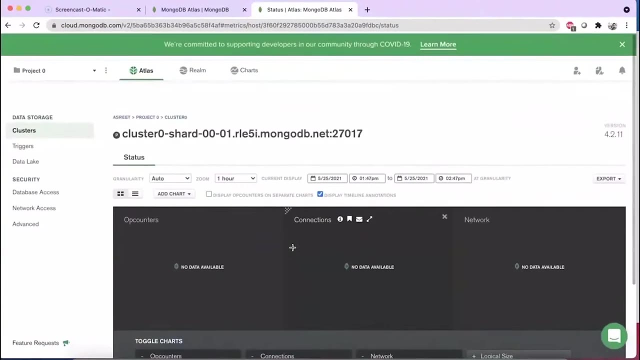 to insert. so this is your replica set. okay, these are the nodes which are available to you. so when you click on this primary here, you will see it is telling you: no, no, no data available, no data available. nothing is there, because i haven't stored any records as such. so i just go back to my 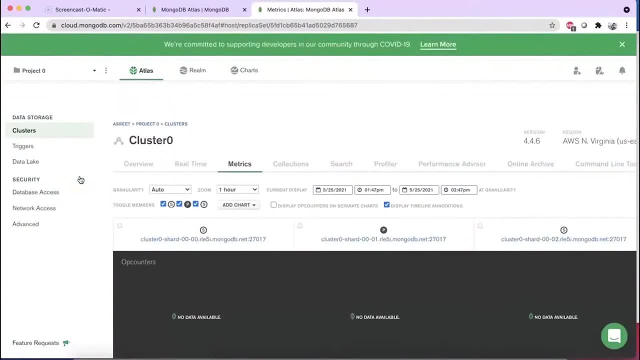 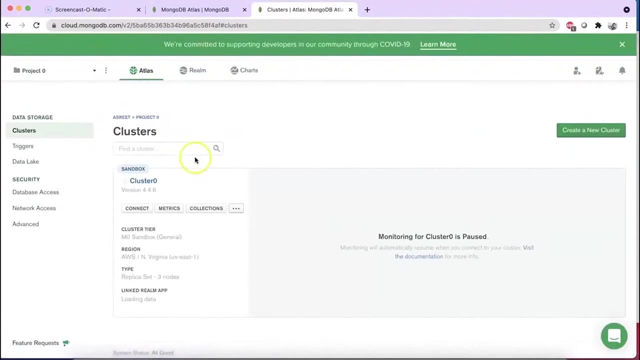 cluster. so initially i would like to go back and create few things now. okay, i would like to go back and set up few initial things at a time of creating the cluster, because when a cluster is created- clear now, so in that point of time no setting is configured. you have to do few settings. 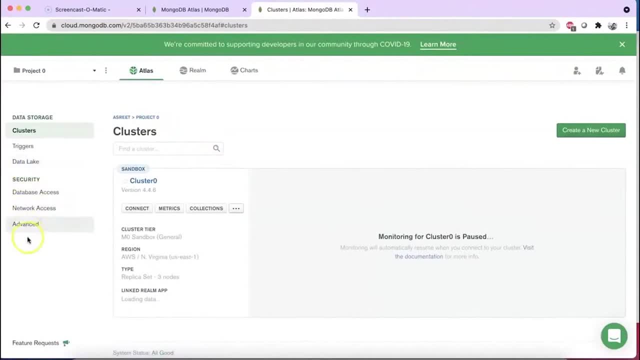 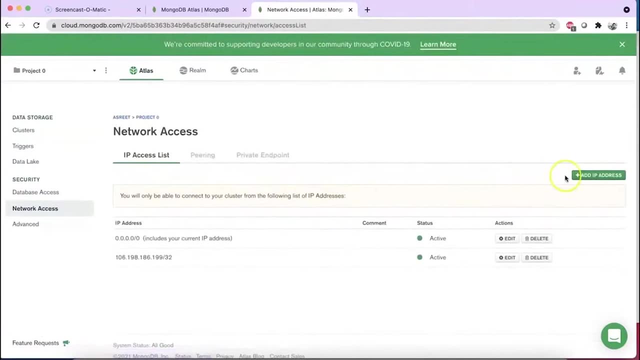 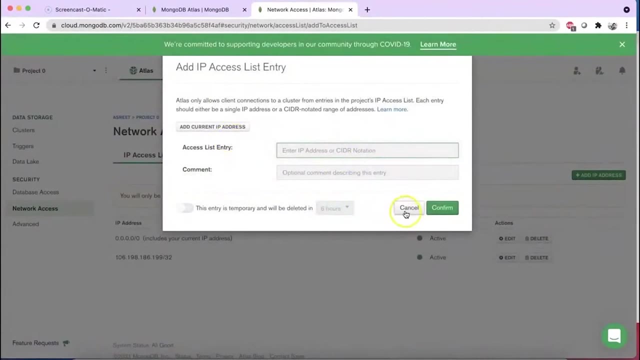 now first setting is- you have to put it and remember the steps. first step will be your network access. so in network access you have to go and you have to say add ip address and in this add ip address you have to select this option, from which location you would like to accept. only those ip addresses will be whitelisted. 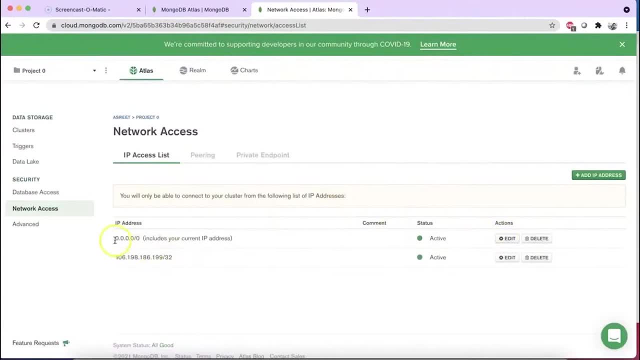 otherwise, what you can do you can see here in my options. i have given 0.0.0. that means all ip addresses are acceptable. so all ip addresses are used, okay. so this: you have to enable it, otherwise you won't be able to get network access from any third-party locations. next you have to talk about 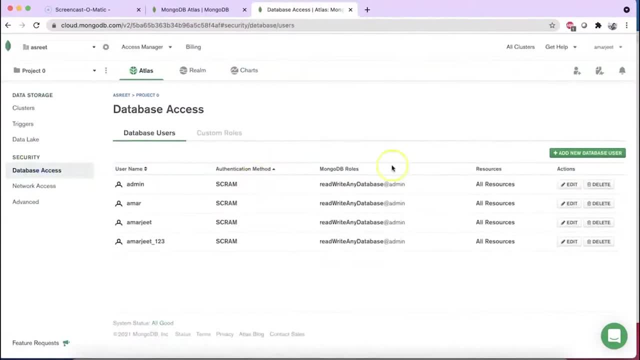 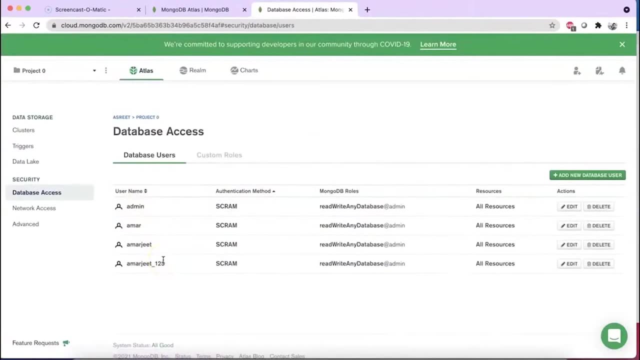 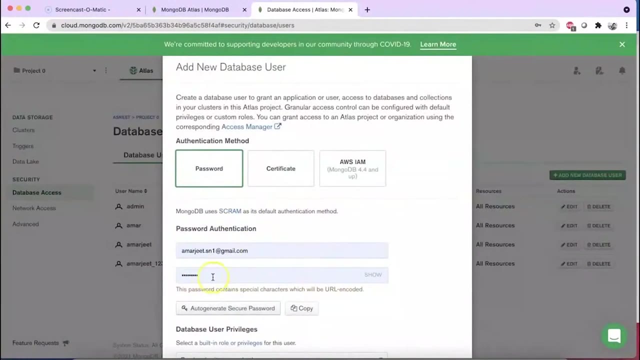 call database access, which is required for you to create a new user there. already some new users are created, but it is recommended that you to go and create a new users here. okay, so you can go back and add a new user. so by default it is username and password is given. so you can go back and create a new user. 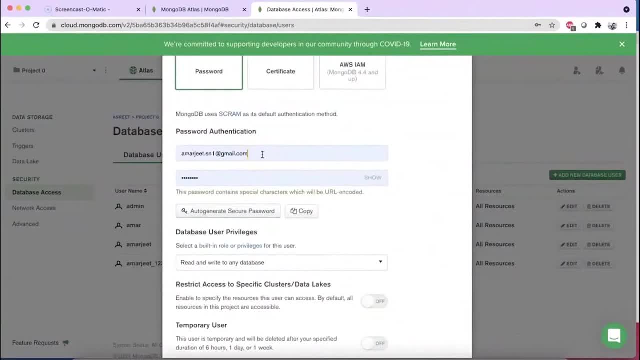 when I say add user, you can give the username as well as the password as per your own convenience. so new user I'm going to create it at is known as called SL okay user and here we giving call admin 1, 2, 3. so SL user- admin 1, 2, 3. 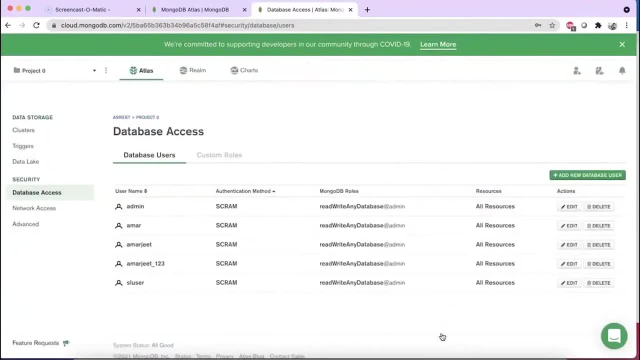 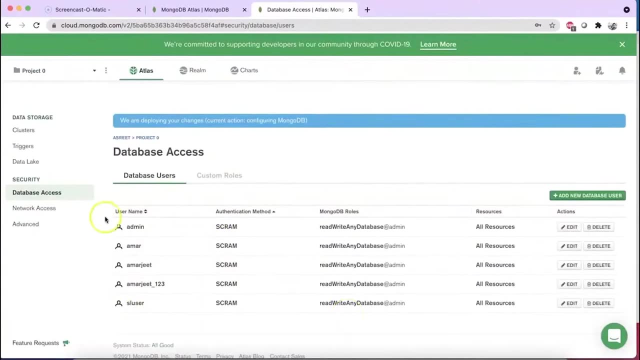 remember this will be the username and password. I'm saying add user. new user is automatically added: SL user: admin: 1, 2, 3. so once you have provided this network access database access, next you have to create a new data. so what you need to do and you go back to your statement. okay, network access database. 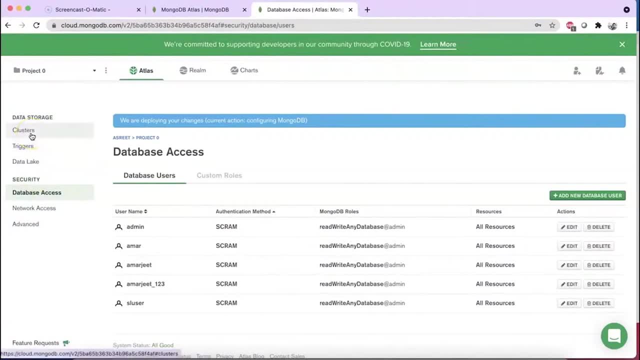 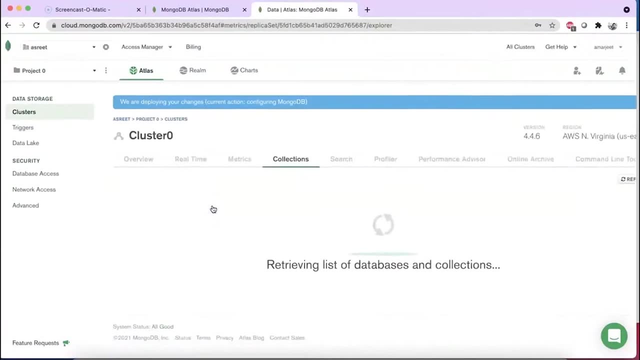 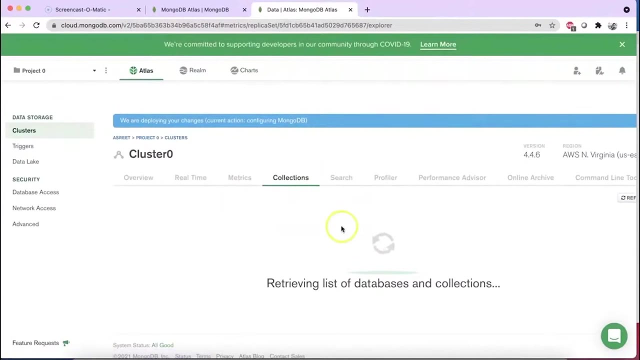 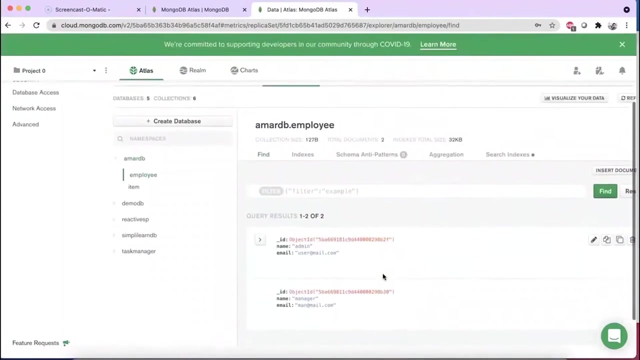 access. it will ask you like you want to create a new database. so I just go back to my project. zero will be on an option you call collections. you have to go back and create a new here. now it is retrieving the list of databases. now you can see there are already some collections. 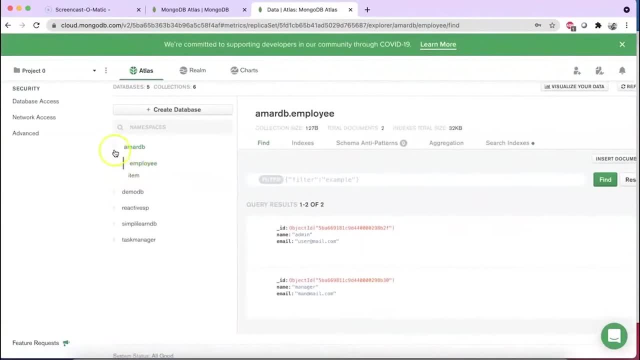 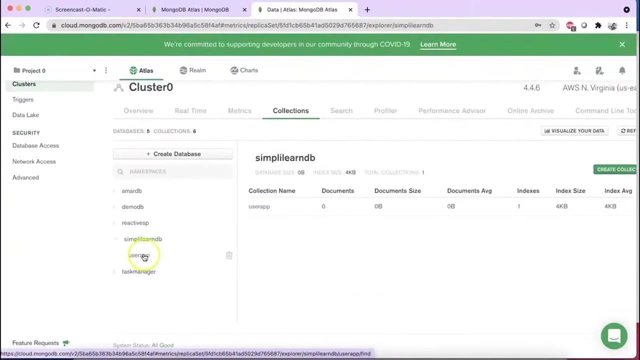 are there. amma db is one of the database which is there. demo db is there. not many databases are there so you can go back and create some new database and connect through. so if i just create database, i already have a simple db with me. user app is already even collections i've created. 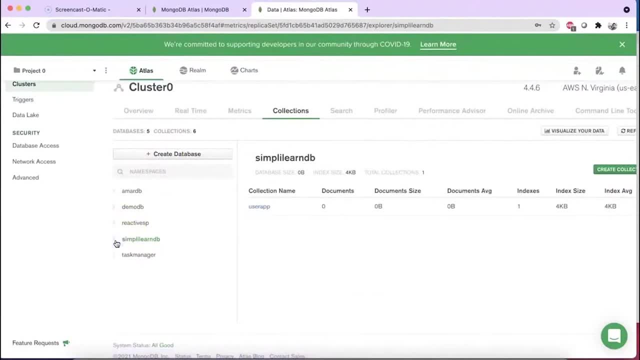 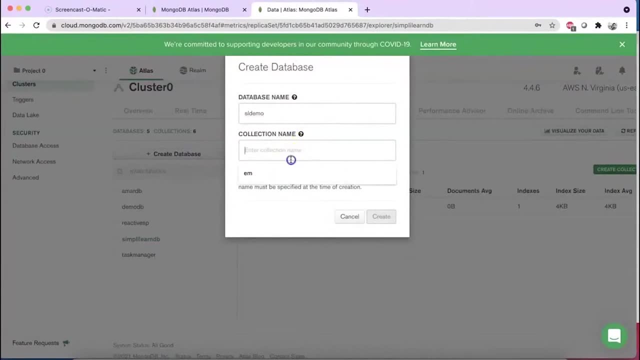 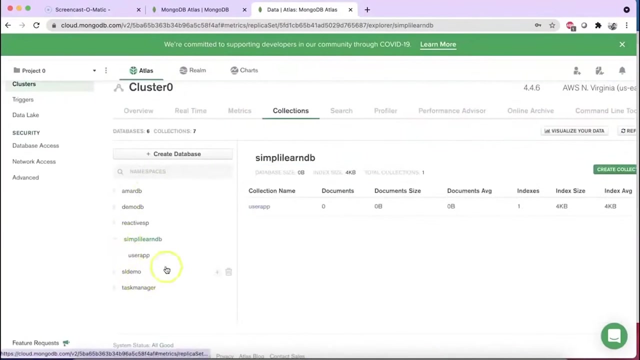 so creating a database in collection is very easy. if i give you the quick demo, i say create database. give the collection name: call sl demo, okay. and give the username: call uh amp sl demo employee. i say create now you can see sl demo create. it is there with me so there is no record right now and 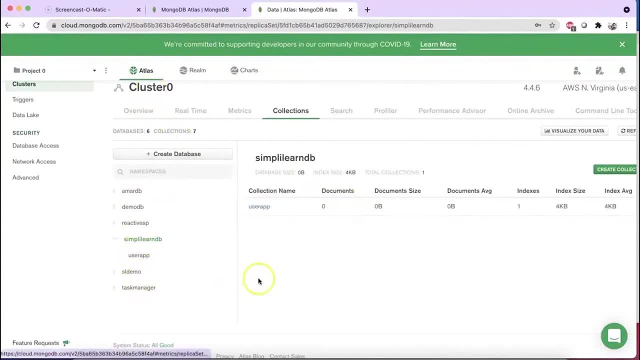 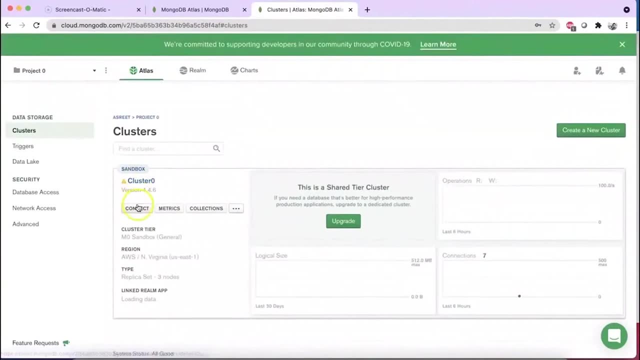 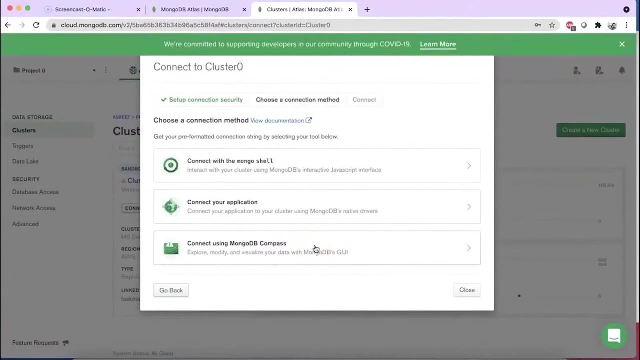 once it is there ready. so remember sl demo and employee. i'll go back to my uh code again, project zero, and from here i can say connect. because i want to connect it, so to connect it from, because your mongo db is already there, so you want to connect it through, so to connect. 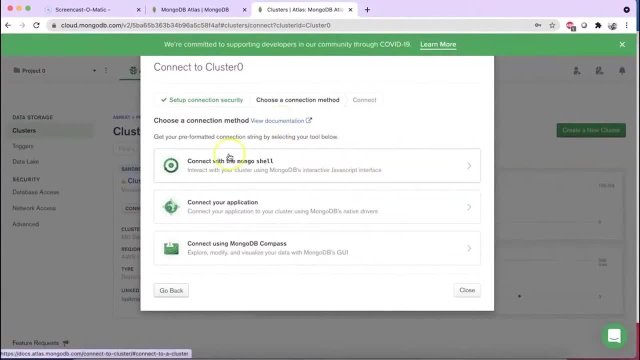 it through. we have very simple option available. you can just click on this connect option. multiple options are there. through mongo share, connect your third-party application of the mongo db compass. so, since i already have a mongo shell with me, so mac os, i have this mac os. 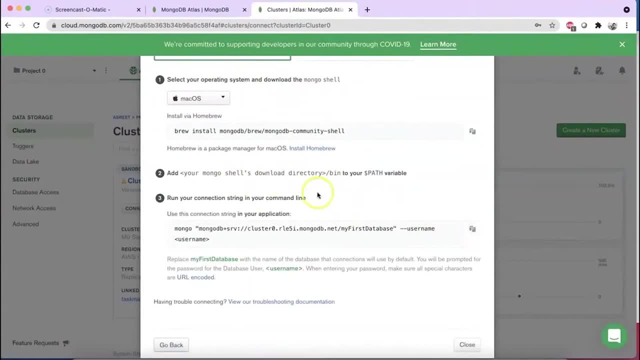 with me so you can just use this line. okay, so if you have a window, you can select your window. since i have this mac os, i'm selecting this line, but i need to replace with this: you can see this username. okay, and you have to give the username here. i'll, i'll select this. i'll open my terminal. 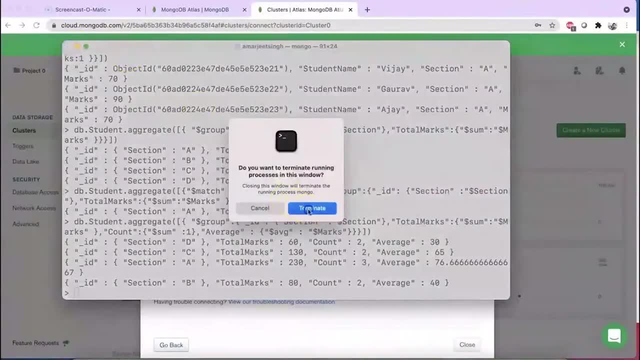 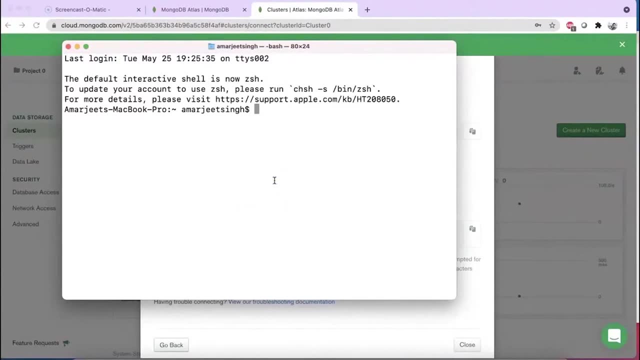 okay, and this is. i'm just closing this and opening up another terminal here, since i want to connect to the mongo shell now. so what i need to do here in this, i'll just paste that, the command which i have it now. username is you remember? i told you? 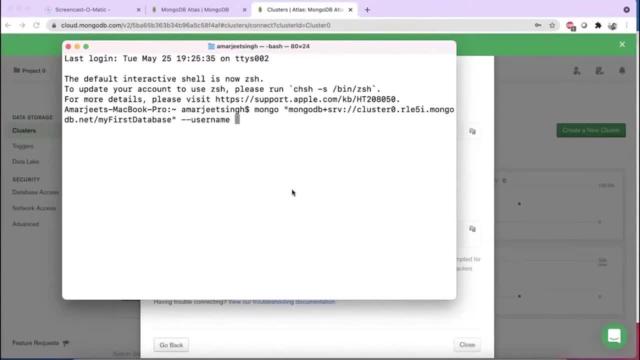 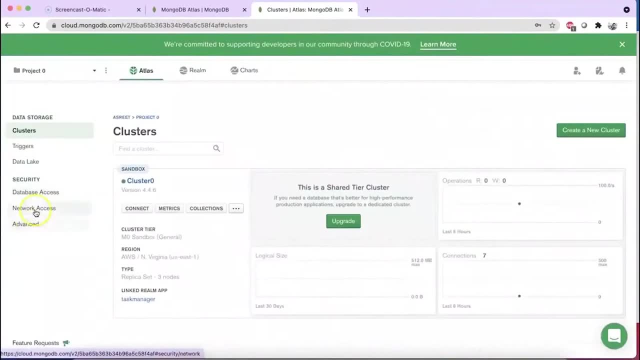 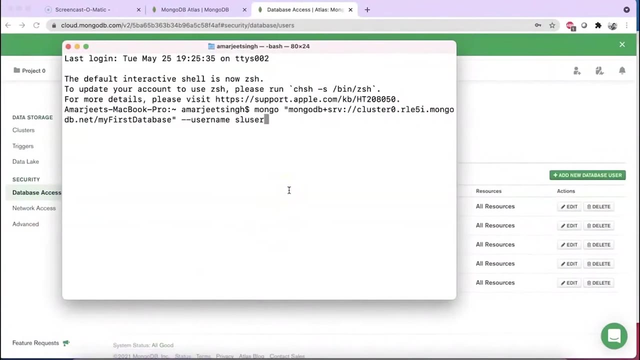 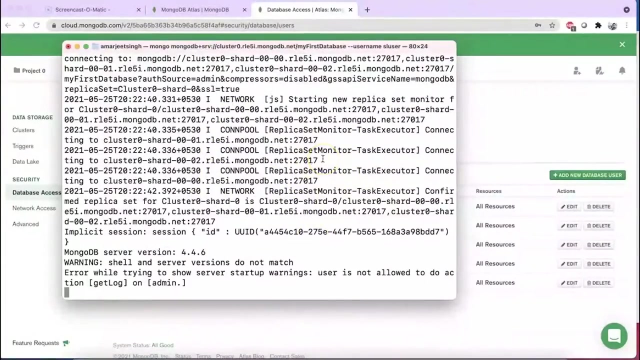 i will call some users which you have already created. let's check here: sl user. i say sl user, i hit enter. it'll ask me the password. so i'll give the password: admin. and now you can see it is connecting with me to this particular see. now see it is connecting me to this. a particular replica set you can see in a logs it. 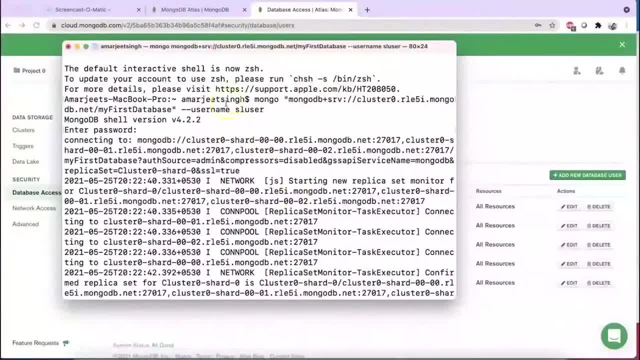 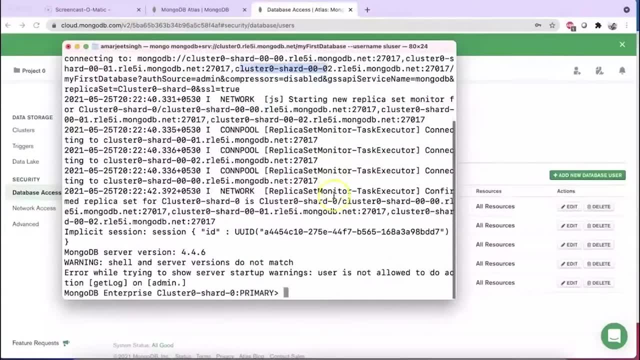 is telling you very clearly, okay, saying that it is a username 4.2 and you can see it is connecting with your shard cluster, the cluster which is created, and this is where exactly i have it with me. so i'm connecting with this environment. so primary is there. if i just want to go back and say 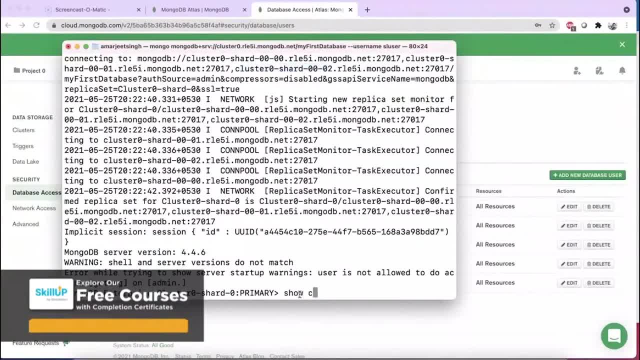 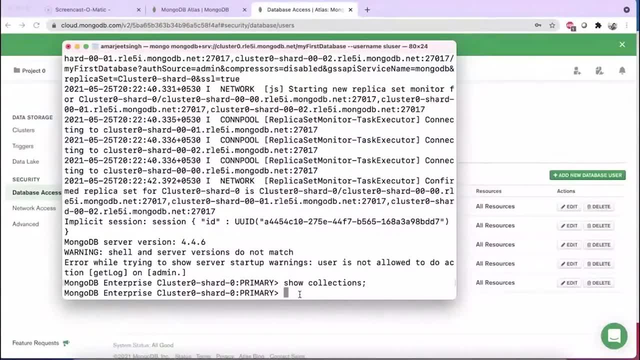 i'm going to go back and say show, show collections. so i can go back and create a new collection here. okay, so it's up to you. now, by default collection which is their employee. so i can say db, dot, employee, dot, insert, and now there we can just add: 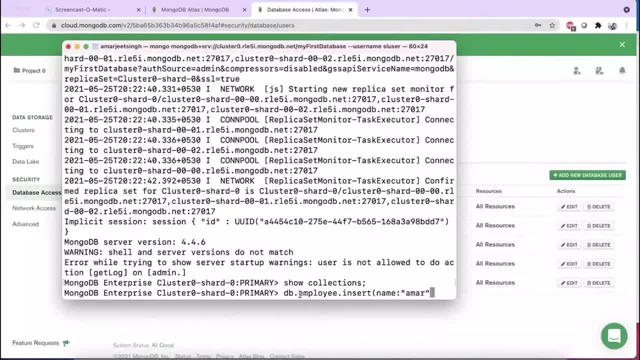 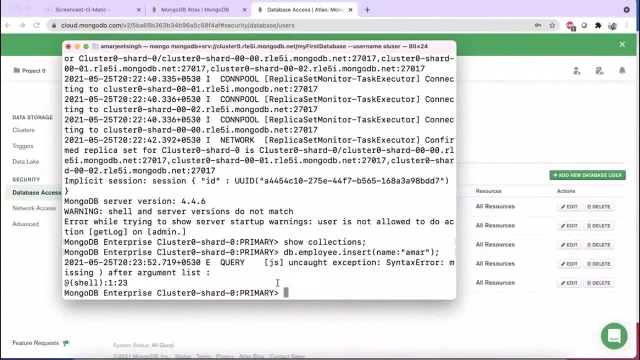 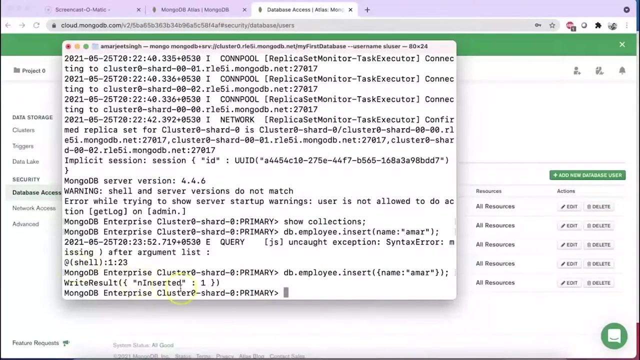 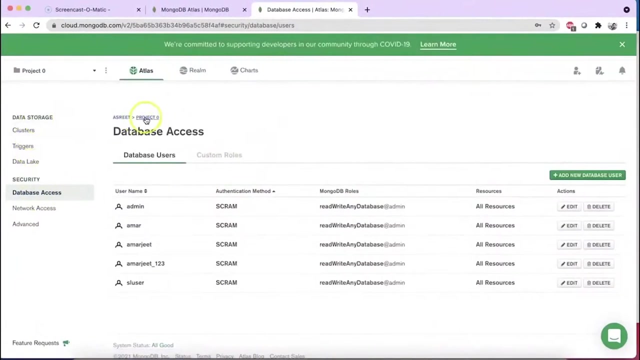 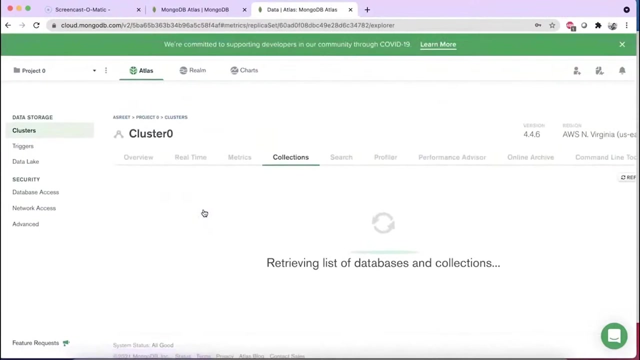 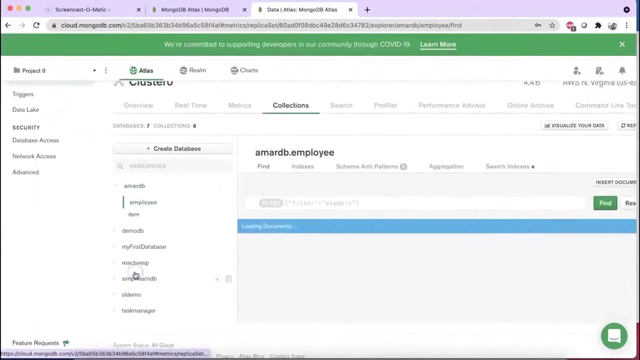 the name. okay, coffee. now you can see some exception is raised. so you understand. now you can see the records are added into my primary cluster. so if i just go back and go back to my project zero, where we have got collections, here, you will be getting the sl demo employee. 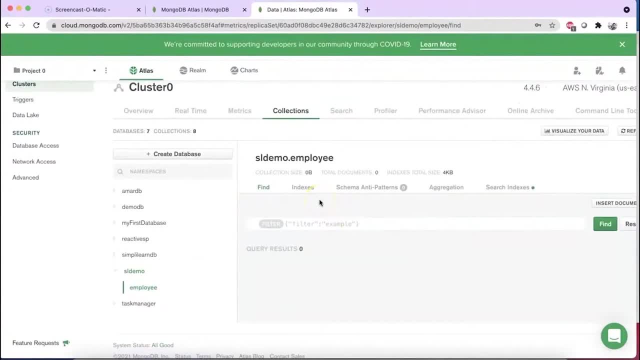 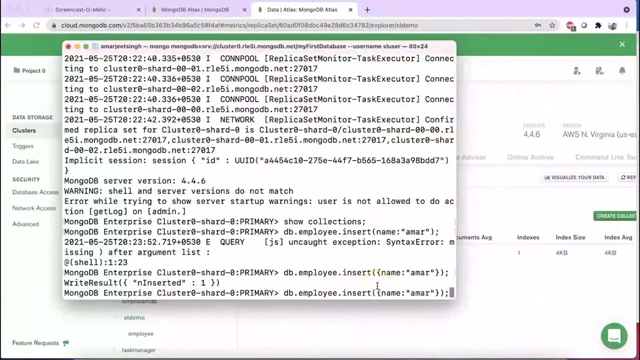 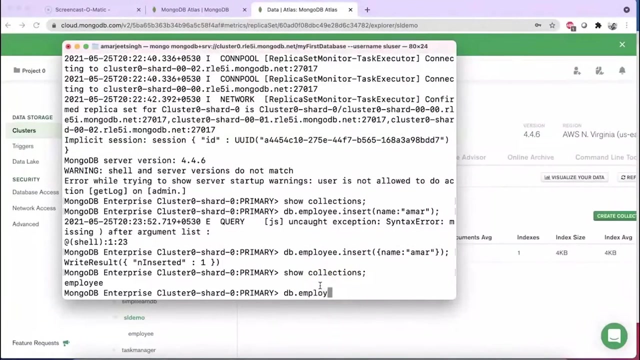 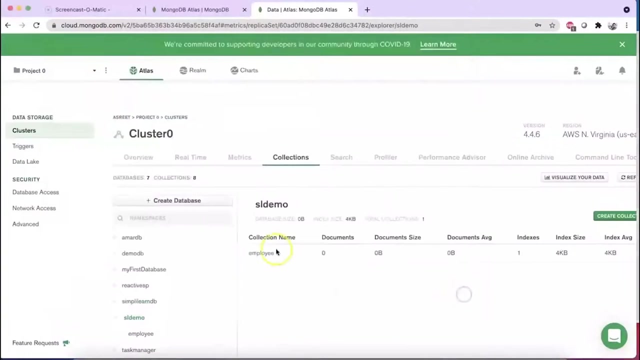 loading the dois document, loading the documents. so it takes time to get this, but this is where exactly your see, the records will be stored. ok, so that's where exactly it works. fine for all of you. so we have this record, okay. so when i say and i say dbemployeefind, so i can see we have got new collection name call. 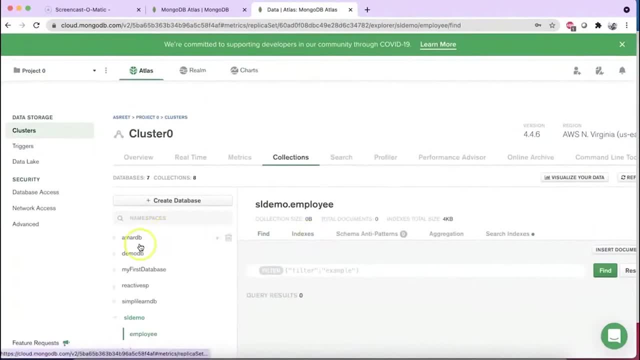 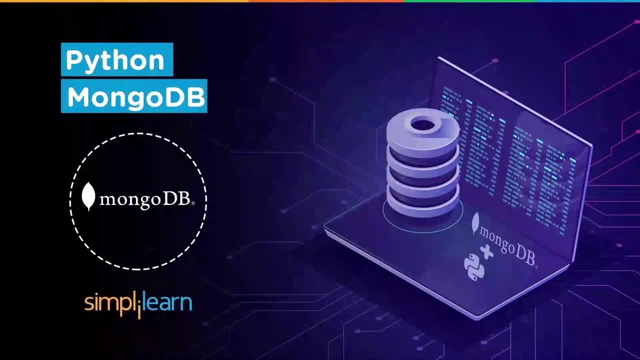 this is added right now. okay, so like this, you have got the first connection established and the records have been inserted. in this particular tutorial, we will help you to connect your mongodb with the front end that is called python, as we know it very well about the popularity of python. 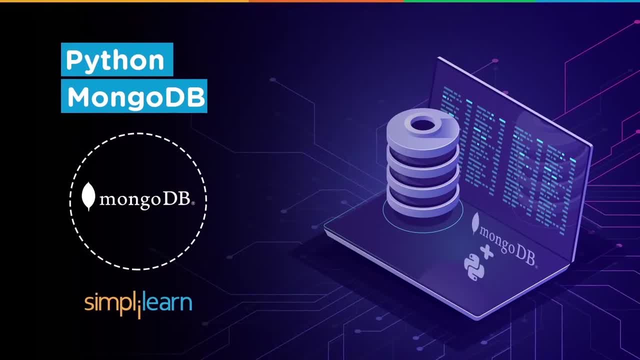 in last recent years. it is growing like anything. so we thought, why not to offer you this connectivity where you can have the mongodb not in a local environment but in a cloud environment? so here we will tell you how to create the mongodb complete environment of cluster in your cloud. 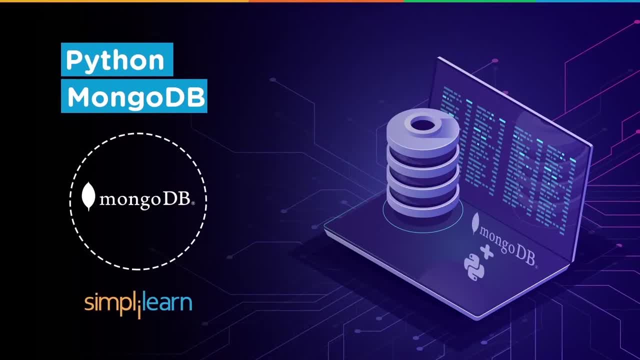 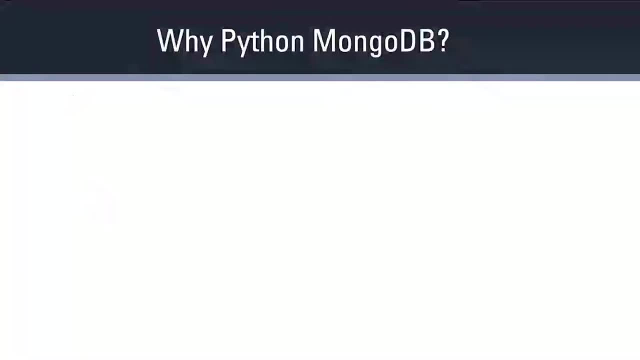 and we can have this connectivity with our python, which is running local to my system. so i show you what few important things one by one. so why python? mongodb? we understand. mongodb is one of the most important database, which is so called document based database, available in market and it is fantastic, phenomenal. 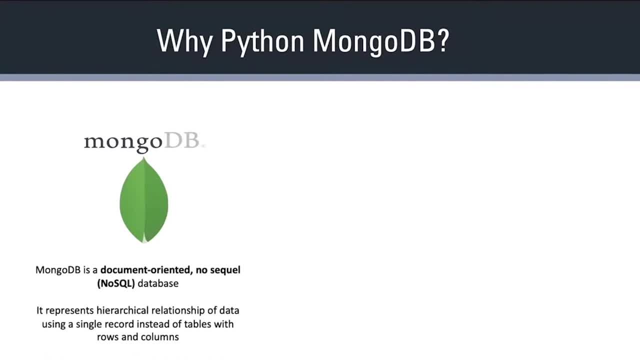 in terms of speed and the reliability. it is purely called no sql database okay and helps you to go schemaless. now, python is one of the most commonly user friendly programming language for creating a complete web-based framework, so it offers you huge amount of libraries with flexibility of connecting. 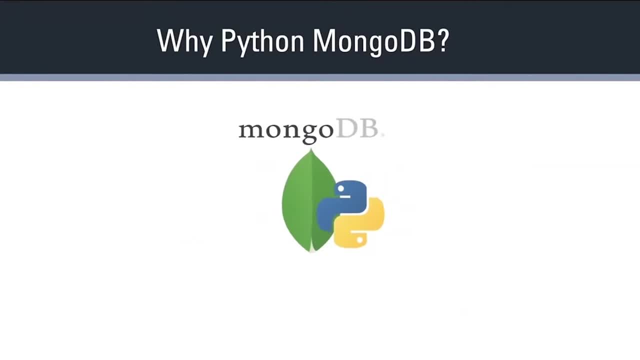 wide variety of applications. so we would like to give you the idea of like how python and mongodb works together. okay, so you can use both the products together to develop different varieties of applications which can suits to different type of ideas. now here we have one of the very very 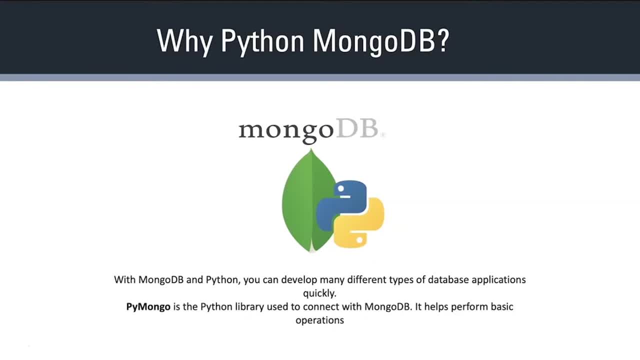 popular tool available name called pi mongo. so pi mongo is actually the python library, which is a kind of a driver through which you will be able to connect with your mongodb and perform basic operations, whichever you expect. okay, so let's go ahead and start working on those demos, okay, 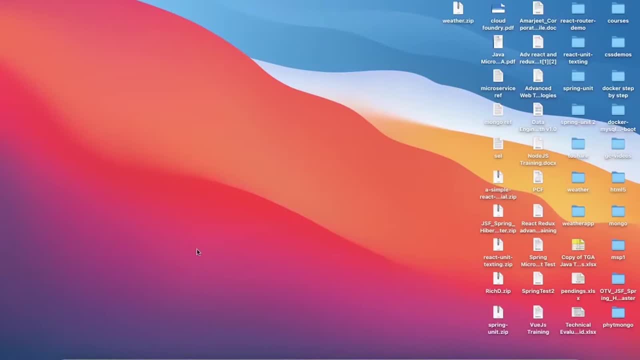 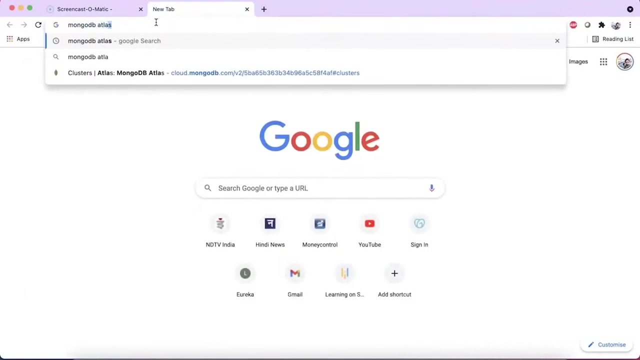 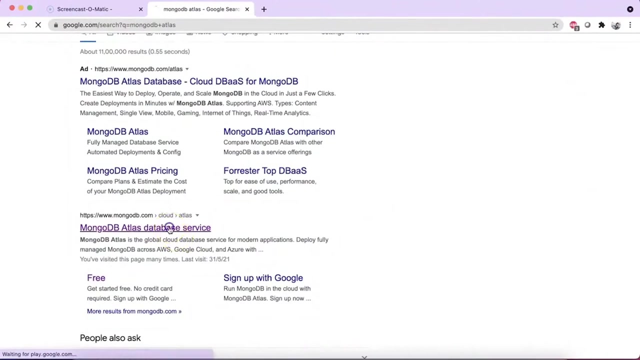 so we will start with creating a mongodb environment with cluster in one of the very, very popular tool that is known as called mongodb atlas. so we'll be opening our website and go here and talk about called mongodb atlas. i search for mongodb atlas. that is basically the mongodb. they are called database as a service. i'll be selecting the first. 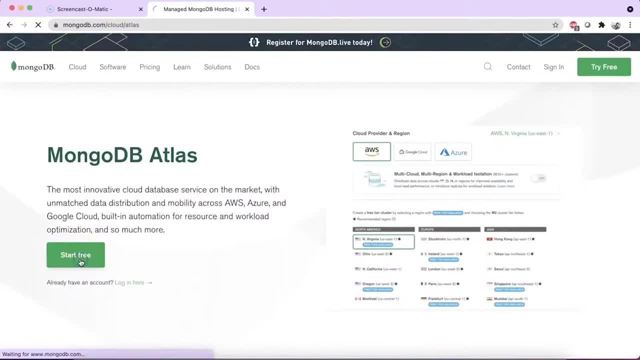 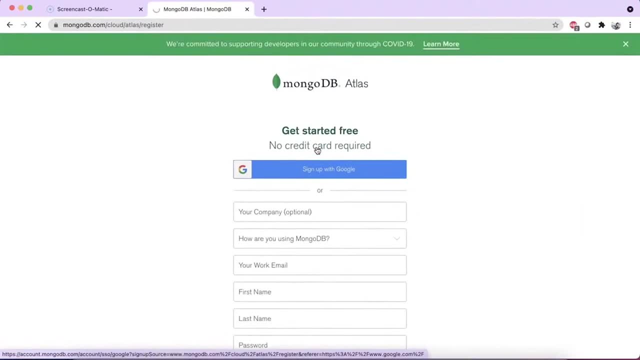 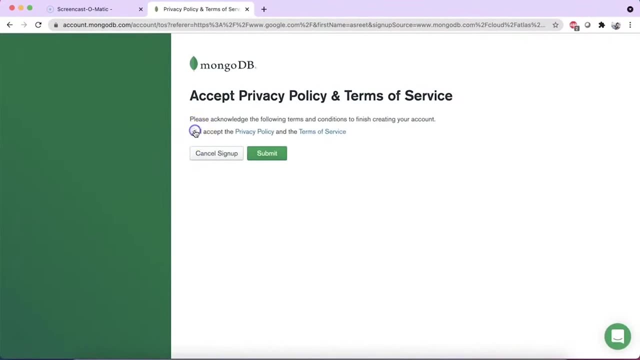 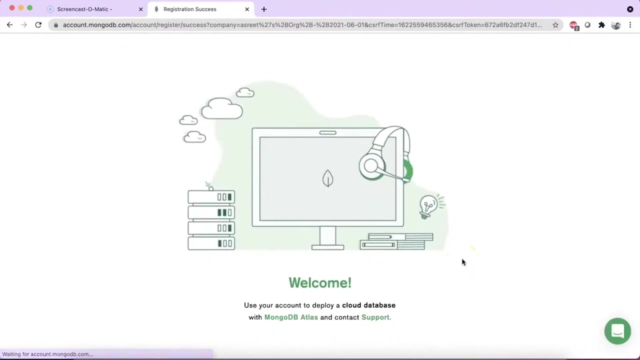 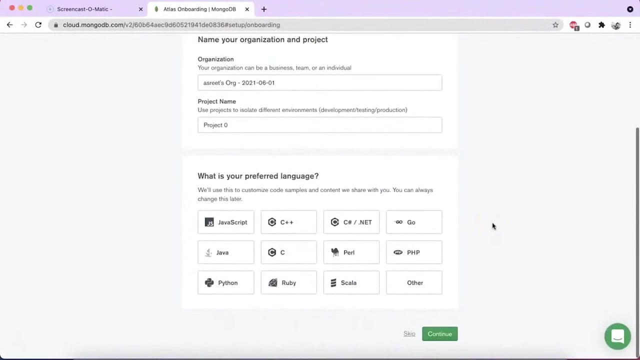 option and go to the start free, because it's going to offer you by default some 500 mb of free space. i say sign up with google, i'm going ahead and selecting this, okay. i say accept and say submit. okay, it's starting up. now it'll ask you about a few things. i would rather say to select, skip and continue. 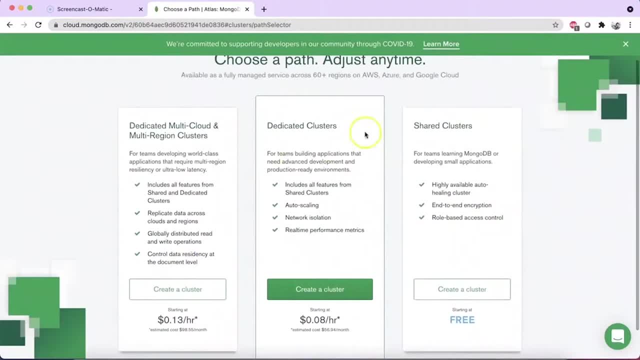 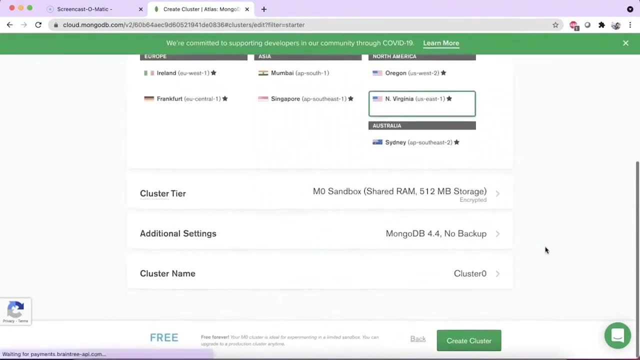 well, it'll ask you about which environment you would like to take. so i like to take this shared cluster. i say: create cluster now here. it will take a while to get yourself ready, for we can see it is offering the sandbox of having 500 mb of free space. 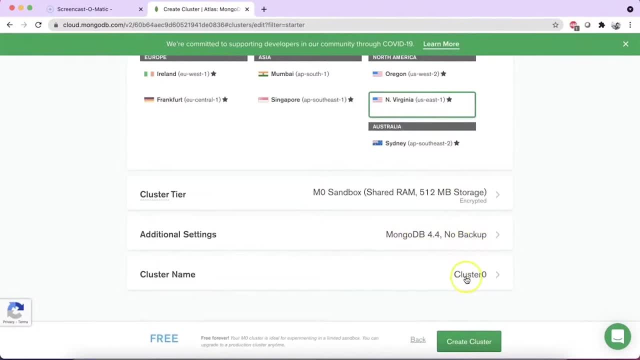 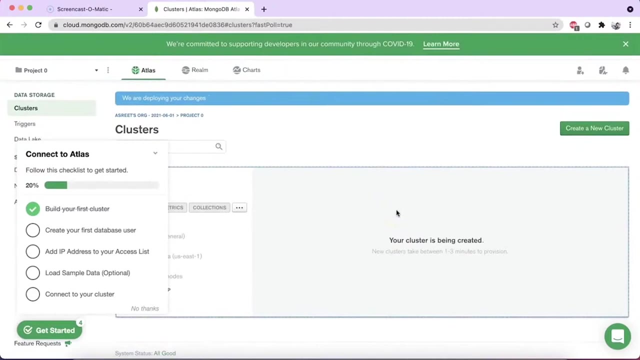 and this mongodb, no backup. that is a by default cluster name. you can give the name of the cluster if you want, but let it be by default cluster zero. i'm saying create cluster so my cluster is being ready, so it will take a while to get your cluster set up. so just wait till the time your cluster is. 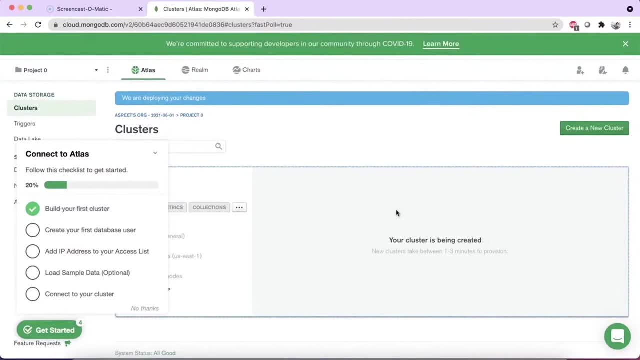 getting ready. so i tell you about this cluster is going to give you by default two child and one parent, so called one master and two child nodes where your cluster will get ready. so you really don't need to set up any kind of cluster in your local environment, and that is the best. 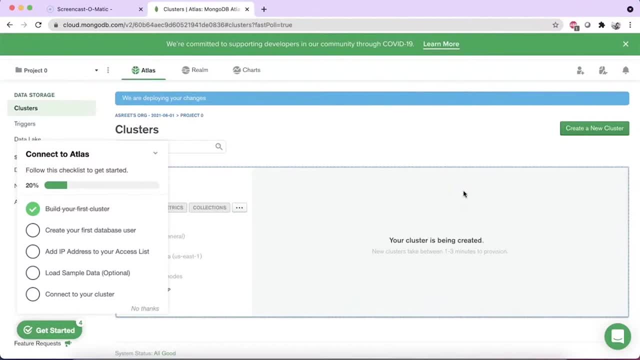 most of your development where your time reduced. there will be no software requirement because sometimes version to version changes and you can get all the benefits of clusters. so we're just waiting till the time the cluster is getting ready. so once the cluster is ready, you will be. 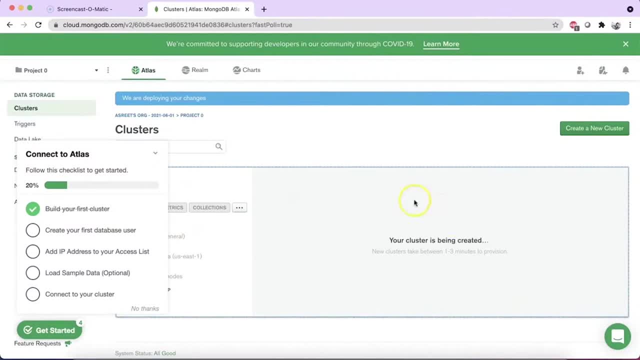 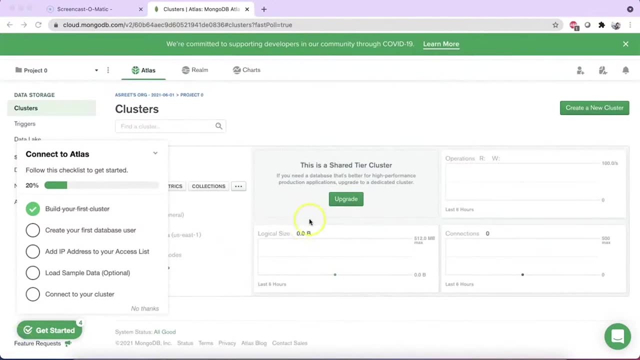 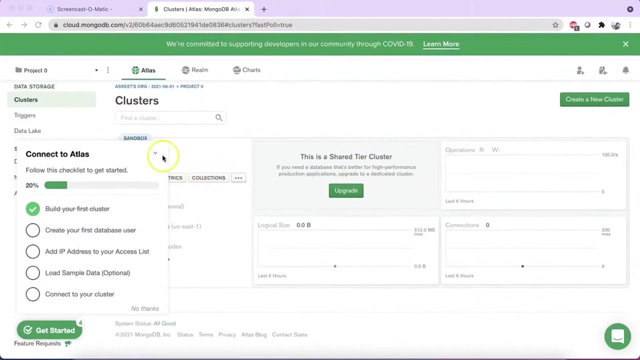 seeing some options where will help you to create the clusters in your upcoming demos. so, friends, your cluster is now ready. you can see now, in this cluster you have got this environment. so in this environment you will see there are some options. they have given you one by: 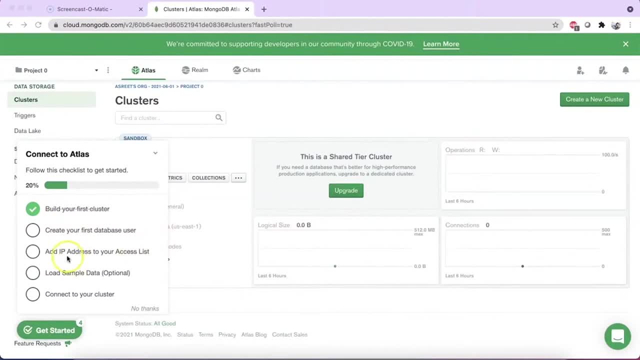 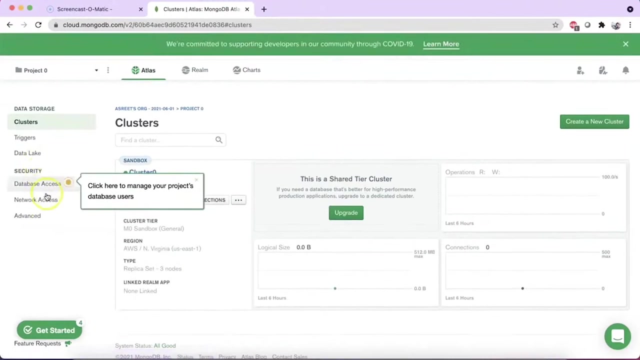 one. build up your cluster, create a first database user, add an ip address, multiple options, they're telling you now, so how to set up. so the first build of the cluster, which we have anyways done next, is called create your first database user. so select this so it will highlight this area. now you can say, like database access, and i'm going to create a. 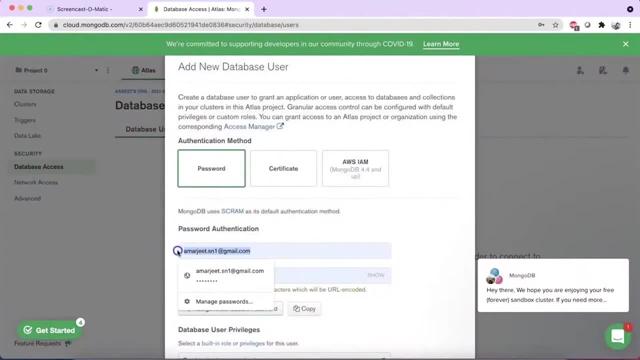 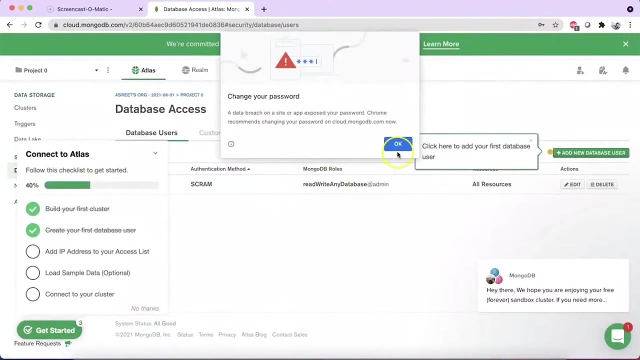 first, new database user and new database user giving the user name for admin. let's keep very simple: username and password: admin 123. so admin, admin 123, yeah, same, and say add user. now you can see the user is created. now let's go back to the next option. 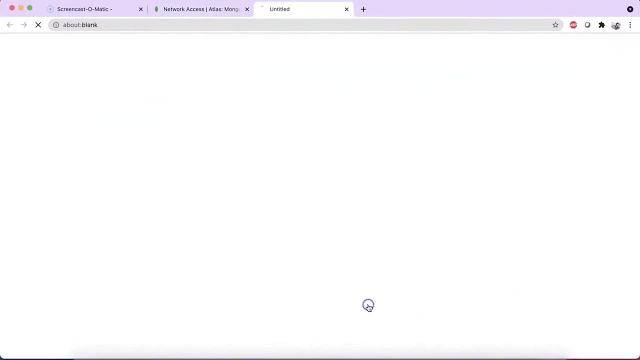 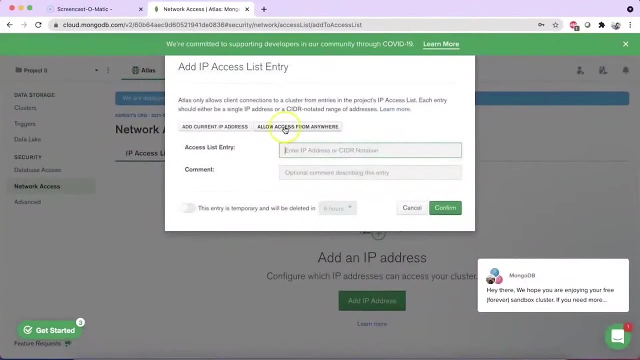 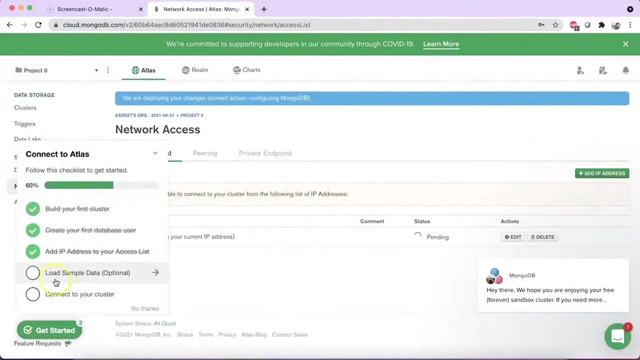 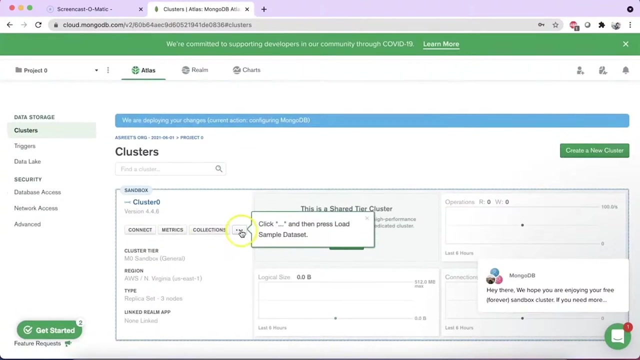 it's telling me the network access. now go here and say sorry. now say add ip address and i'll say allow access from anywhere so that i can take it from anywhere. i say confirm. now it is telling me about the progress. i select this and tell me about which type of collections you want. okay, so i select this. 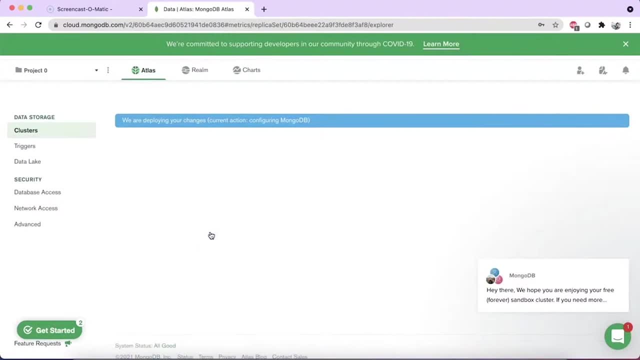 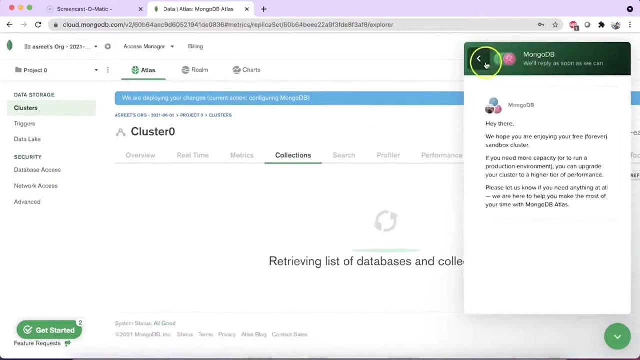 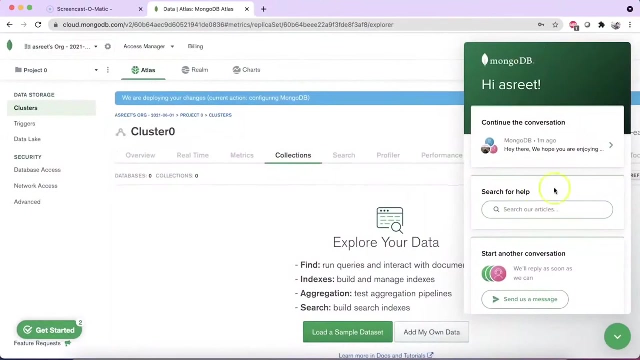 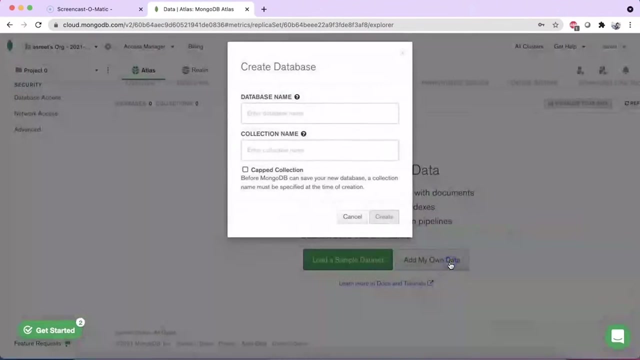 and inside this i'll be selecting this called collections. okay, and it's getting ready, so it is giving me some options. well, two options that will give you load sample data set: add my own data. i'll say: add my own data. give the database name: sl demo. give the collection name: emp. 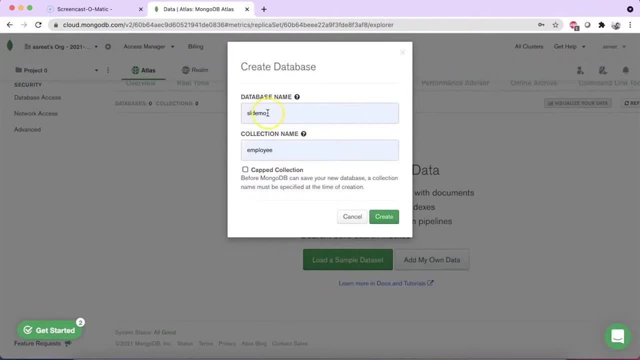 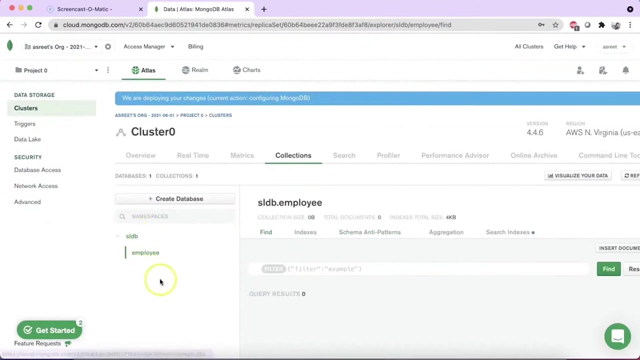 or employee. remember database name: sl, demo or i can better give the name code sldb, sldb. and employee. i say create. that is getting ready. okay, so my database and table is ready. that's it. so i think we are all set with this environment, okay. well, once it is ready, your collection is also ready. i'll go back and click on my 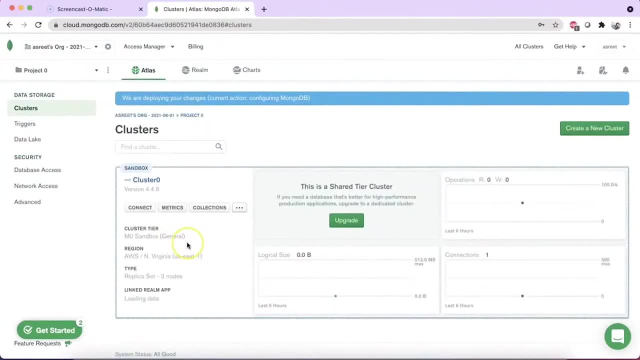 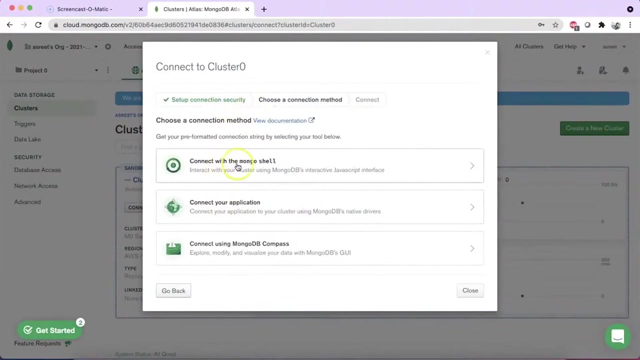 project zero and here yeah. so once it is there, then i'll be clicking on this option called connect. now it will give me the multiple options how to connect. so it will say: correct for the mongo shell. or it will say: connect with your application. connect using mongo compass. 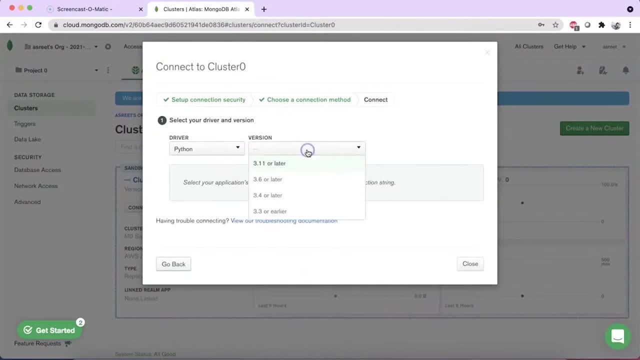 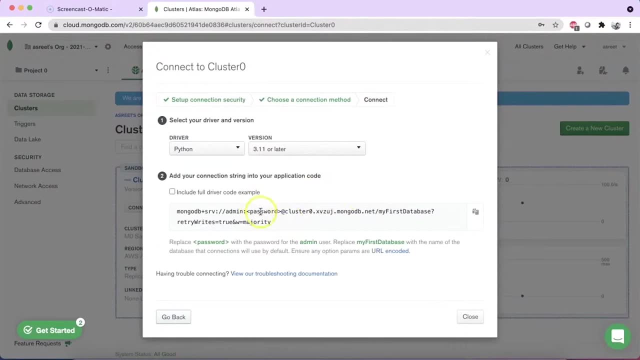 i'll select the python version 3.11 or later, so certainly i'll be using those version only. okay, and in this i'm having this, so i'll be using this to connect with my backend. so that's how exactly you have the setup of mongo db cluster 3-1. so we are all ready now with our 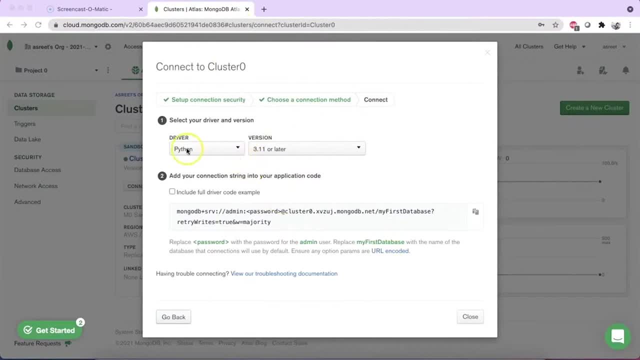 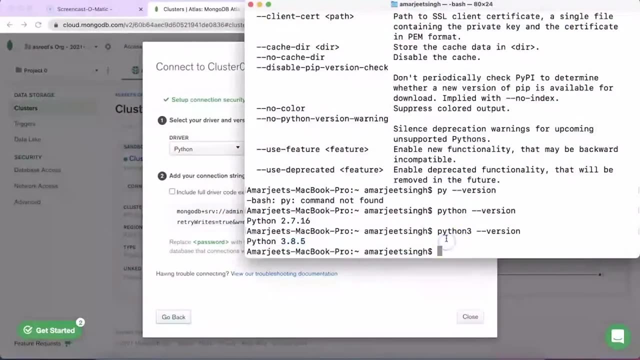 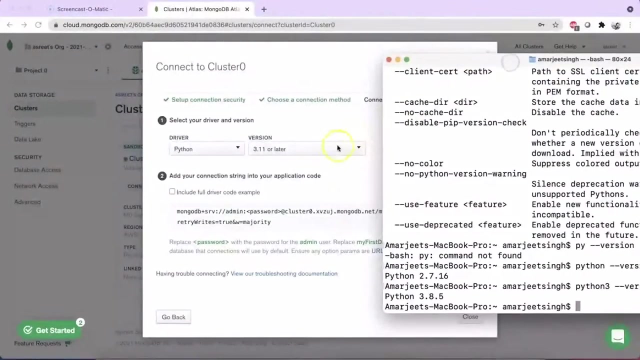 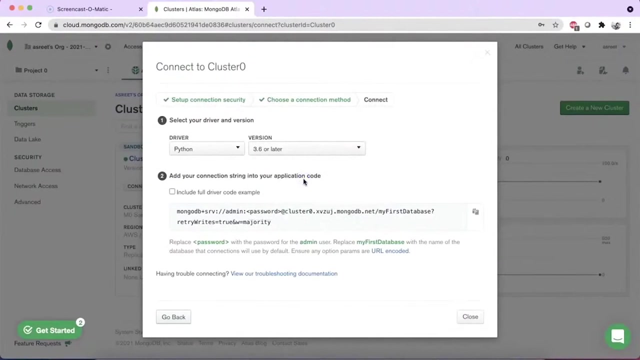 setup cluster. cluster we have already created earlier. you remember about we have taken python 3.11 or later. so here, if i just go back and check, i have a god 3.8.5 which is python 3 version which is available. so you can select based on whichever we have it. let's say 3.11 or later, we can say 3.6. 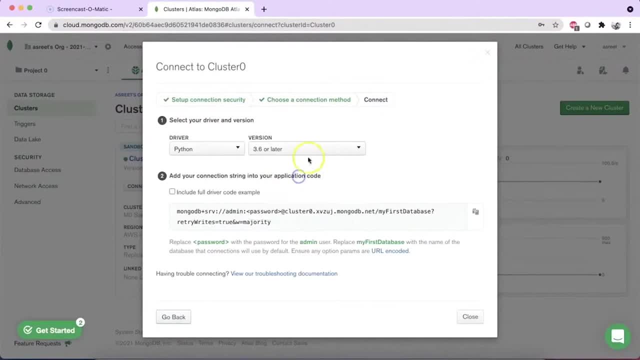 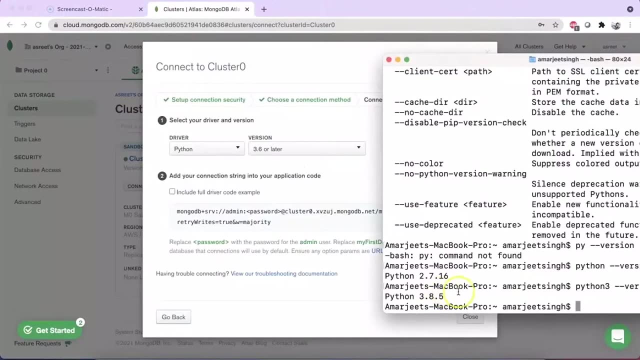 or later, so there'll be no much difference. if i just see, even if i just talk about 3.4, there's some change, but here's 3.6 or later, it is same. so i have a 3.8.5, okay. so. 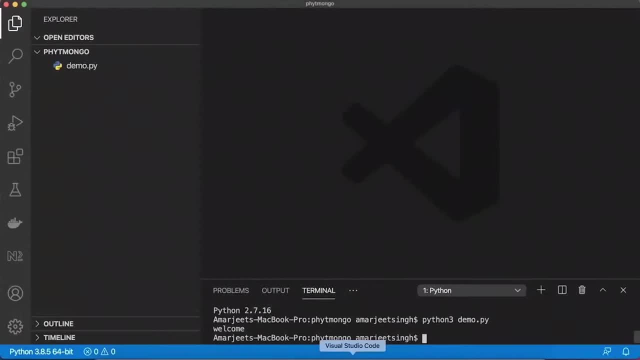 i can use the same option. so here in my vs coordinator i am using for my development. so here's a simple demopy. i have used welcome to check if it is working fine. so yes, it is working fine. i'll start working with my first program with mongodb. so i just go back and say demo. 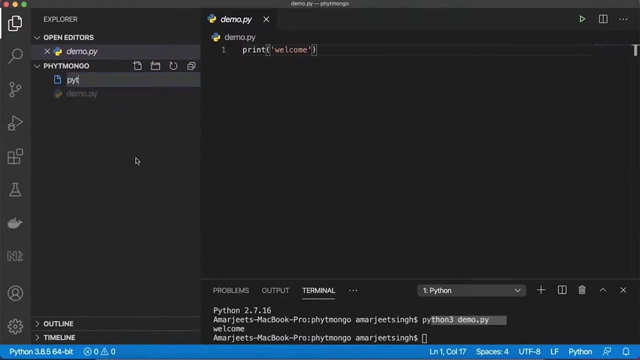 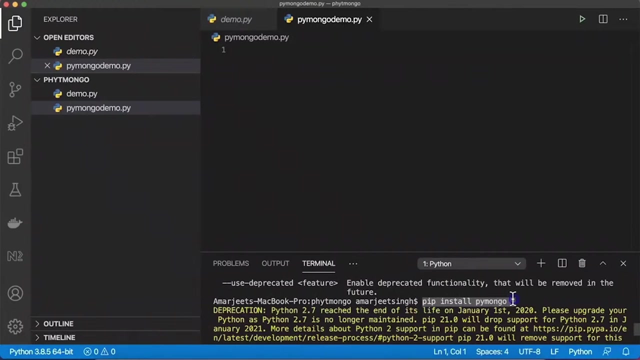 py, or i can say py, demo, dot, py. okay, and here, if i want to go back and start working on the development, remember one thing: we need first dependency called pi, mongodb, and we download that dependency in your system. it becomes the mongodb type by version and that's all furthernity. actually, this is the device we are needing. done that'sRY. 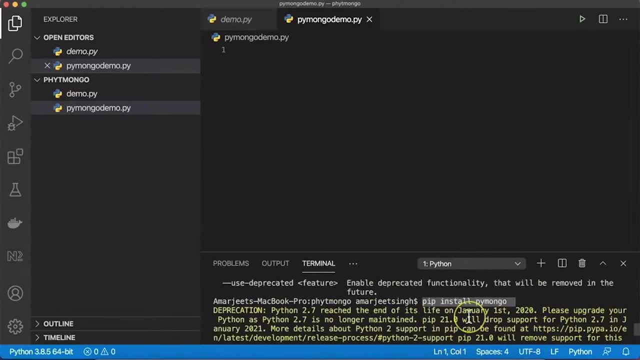 ng. okey, so let's decide how this works with our system. so let's go back to our lyon rom system. okay, so we have. this is statement name called why p ip install by mango, and for this we have already installed this dependency here sometime back. this is how you need to install. okay, so we have this: a statement named wipei. installed file. then is the first dependency which you need to download. you know, to learntop monk, that is the first dependency which you need to download. okay, so that's what we have taken this installed by mobilize. that's the first dependency which you need to download in order to work with this. 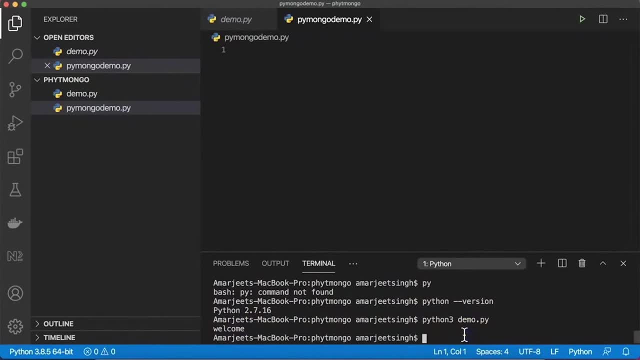 is installed by mongo. so if you just see, you can go back and start developing this statement. okay. so let's go back and start working on this step number one. you need to always say import. number one: the one dependency which you've installed is called by mongo, so as you can just say p y m? o and. 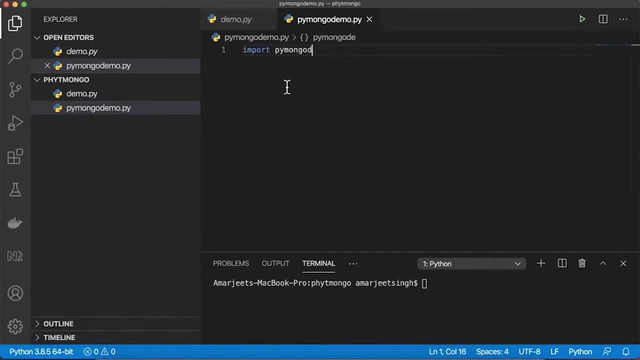 geo. that is the dependency we have recently imported from okay. let me go back and search from next point. so import by mongo from here, we are saying by mongo, okay, by mongo, and we're also saying import mongo client. that's the first thing you need to remember. 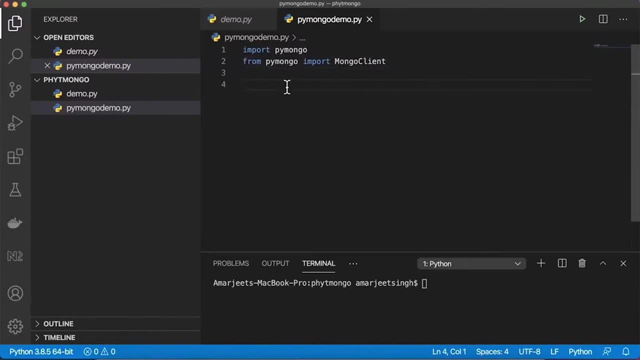 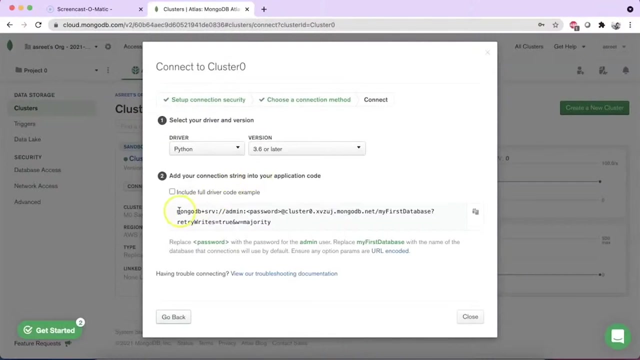 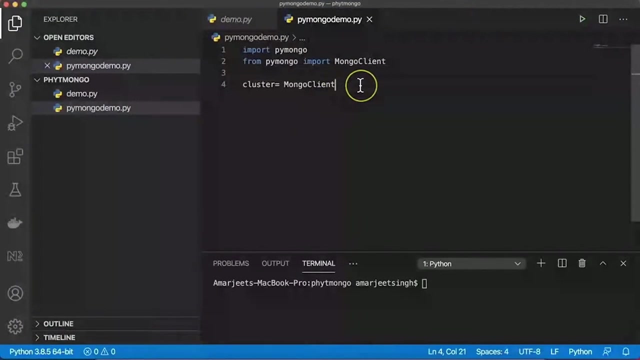 okay, after that we would like to go back and use the cluster. so we say cluster equal to mongo client, and here i'll be parsing the complete values, the one which we have taken. so this complete line, i just take it, go back and here i'm pasting it now. here i have to basically replace this password with admin123. 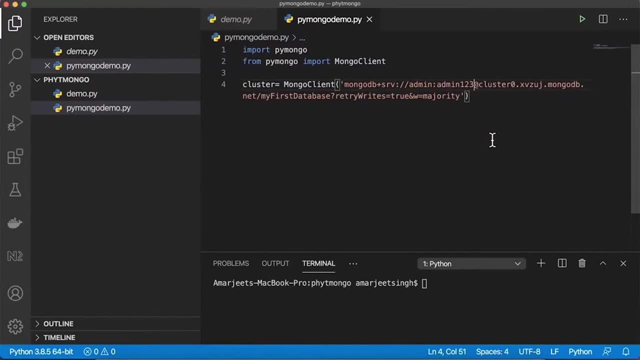 okay, and we are all set. okay, now, once it is ready, we can go ahead and define db equal to. and we are all set, okay, now, once it is ready, we can go ahead and define db equal to cluster and provide which database you're talking about. okay, so you remember about? we had a database which was available to us that is known as called. 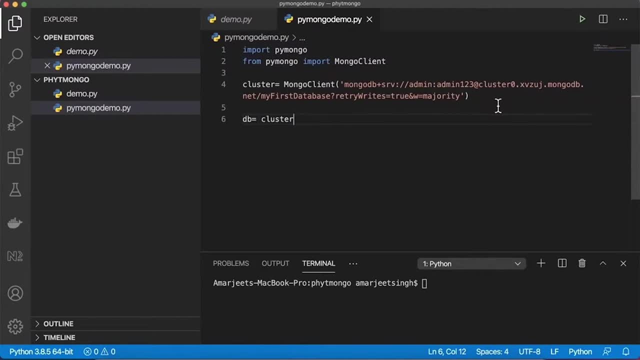 sldb, so i can just use the same sldb there and accordingly i can use which collection i'm connecting it to. so accordingly, i can go back and insert a record. okay, everybody, so i can see i have got this uh collection i'm connecting it to, so accordingly, i can go back and insert a record. okay, everybody, so i can see i have got this uh. 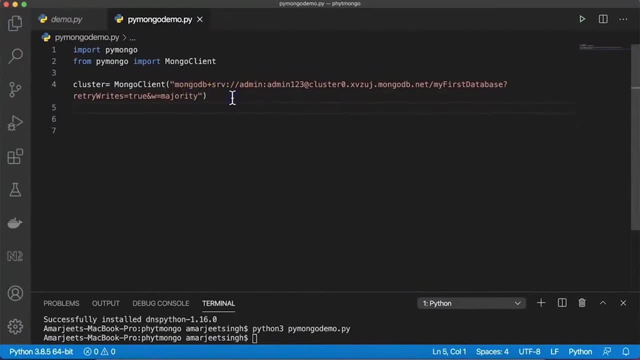 file with me going forward, i have to tell. so this is what exactly the connection url you've received. now, if you define which database you're working on, let me say dp equal to cluster and we have to provide in double quotes the database name called sldp, if you remember the user. 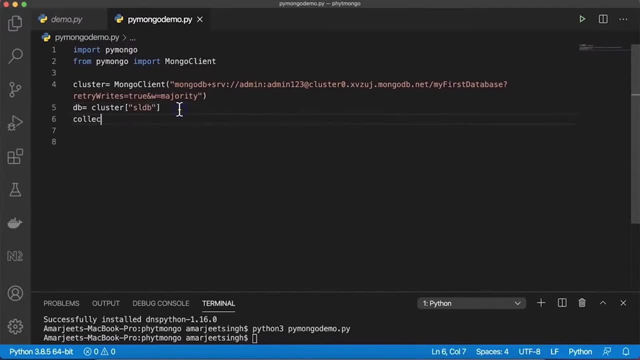 after that we have to mention which collection it was. so collection equal to db and here we just give the name call employee. that was our collection name. so once it is ready, then i have to basically perform some insert operation. so i just say post: okay, it's just a name equal to. 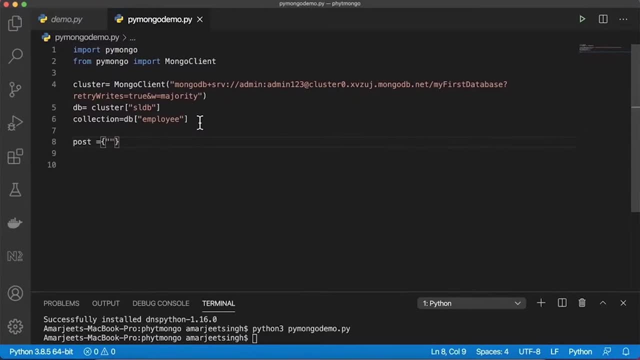 and here we just provide the properties, like i would say name. so you know, it is a json based database, so i can just use the name, i say amr, and once again i can just say email and say i'm at the emailcom, that's it. so this is just the data which i have. now i want to insert. 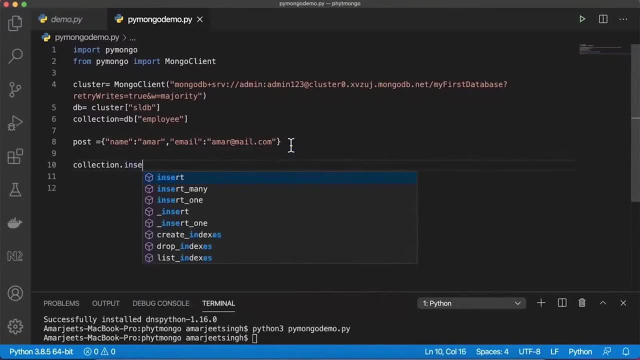 so i can certainly say collection dot, because i want to insert only one record. you can see i have one functions coming up: collectionsinsert one and pass post as a parameter. now we are all done. let's try to run this. so i'll be running this with python 3: py momodemopy hit enter. 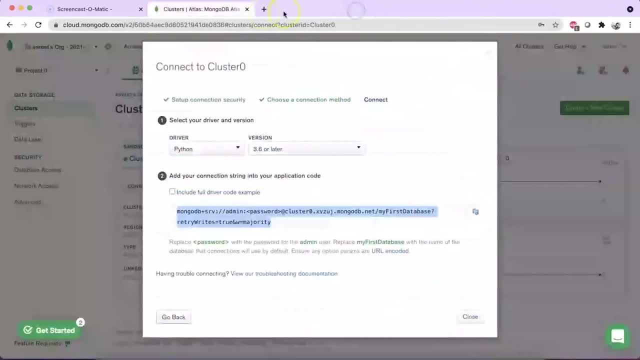 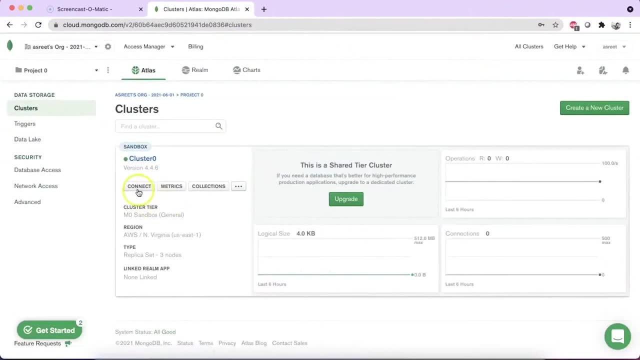 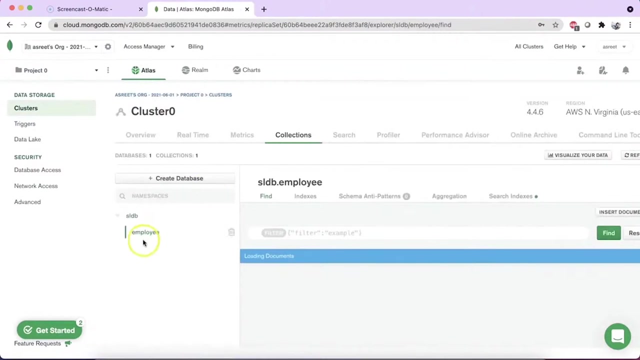 now it's done, let's confirm here into my code. i will just go back and check here inside my applications. i can just go back to my collections and in employ. yeah, there we go. we have got some records coming up here. okay, so these records are nothing but the one which we have recently inserted in our application. 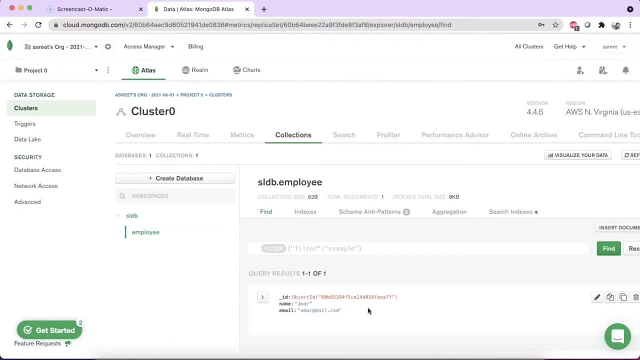 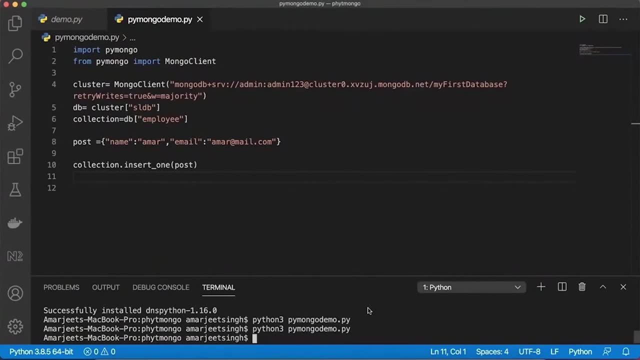 okay, so fantastic. so first example is working perfectly fine. how we can have the records coming from the python. let's just go back and check for some records, okay, so now let's go back and check, insert it there like that I can have as my number of records, I can add it. so how? 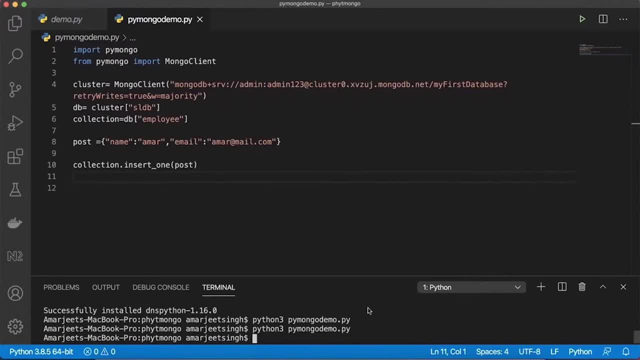 we can basically add. if I want to add more than one records, let's see this now here in encase: if I want to add more than one records, so I can just use called post one, I copy this url and paste it below and I say post to. I say: 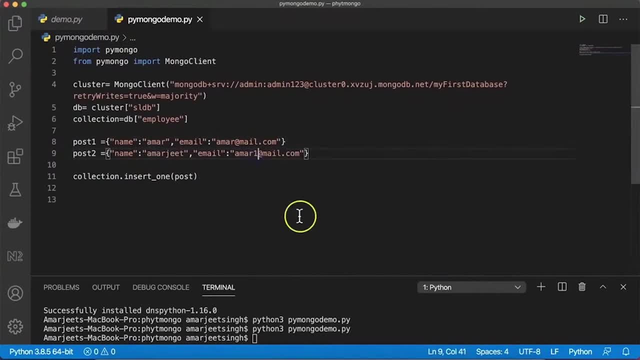 Amar G, email amar12 at the rate mailcom. and rather than saying insert one, I can use insert many, and inside this I'll be using this square brackets and pass post post one, comma post two. that's it okay. so let's change the little name, because it's already there. let's insert: 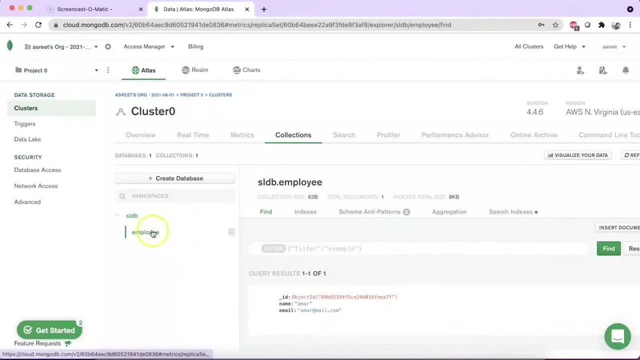 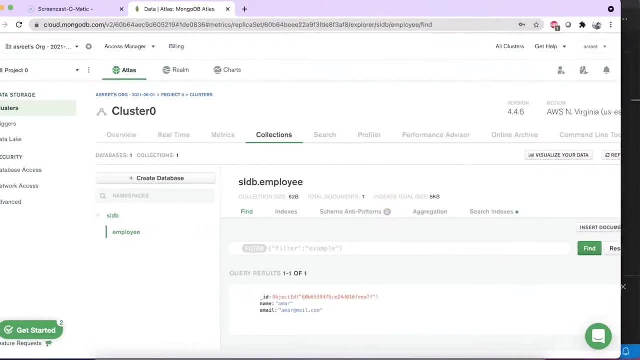 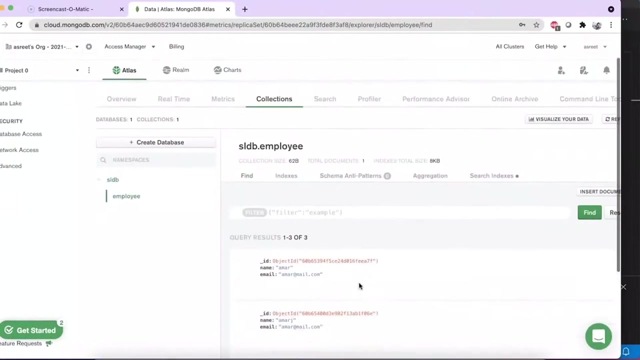 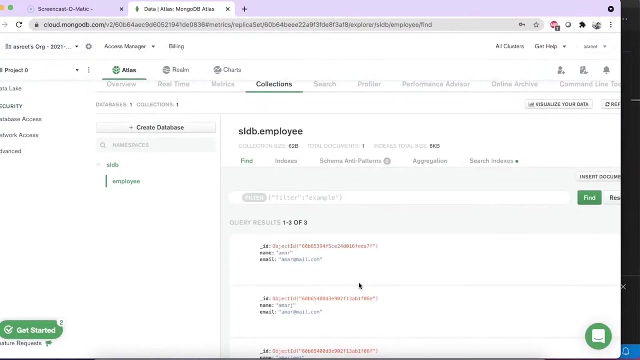 yeah, the cards are inserted. let me verify once again by refreshing it. but now we have a total number of three records are available. yeah, there we go. so the cards are added. perfect. so like this you can have as my number of records. you can basically add it in a similar one, the way we have basically used this. I. 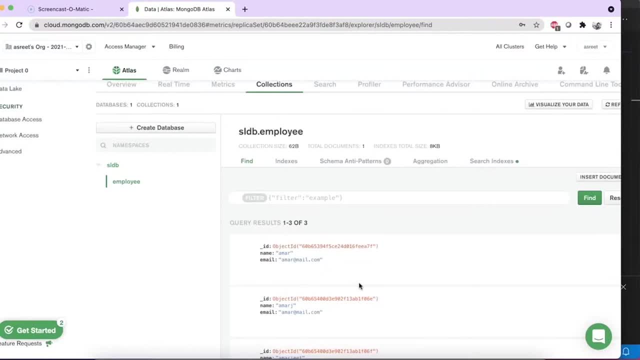 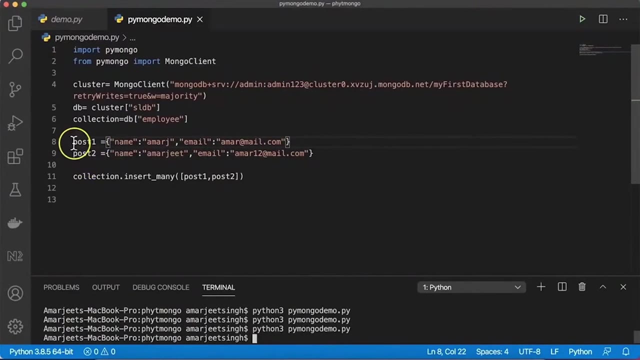 can also perform the search bar too, okay. so in case, if you want to perform the search part, we have a very simple statement available with us. what I'll go here, the way we have added this, so in this I'll just these records which are added inside my application. I would not execute this. 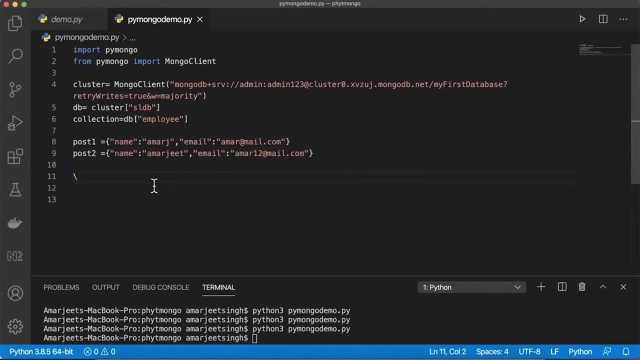 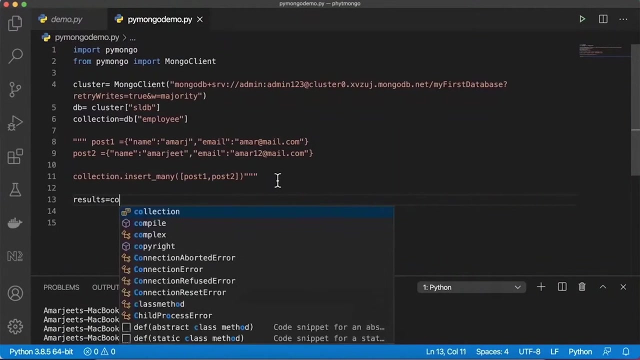 rather, I would like to go back and say you: no, we are basically comm printing them and in fact I would like to use this also. okay, I'll go here and find results. results equal to same collection dot find. if i want to find a name, we can just use: 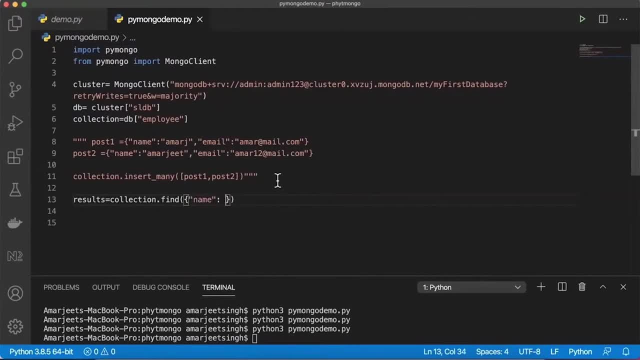 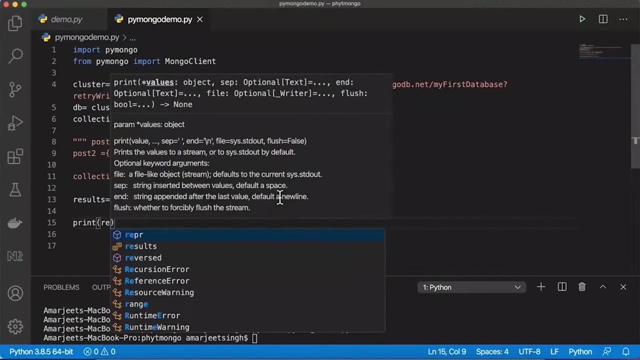 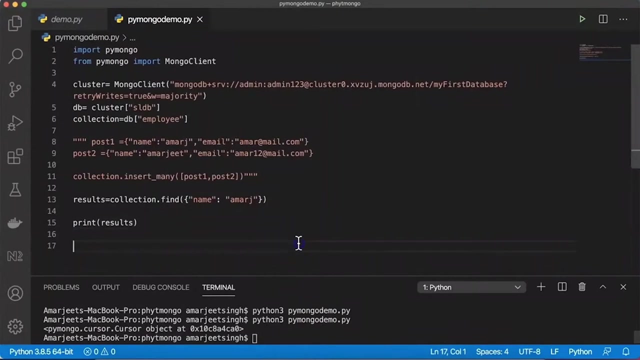 curly braces: name, colon number. okay, so let me say print and path results. okay, let's run this. okay, so it will print what the results for me. okay, so it is just printing what the cursor object for me, saying: hey, this is what the record is available to me. we can also change in case if we do not. 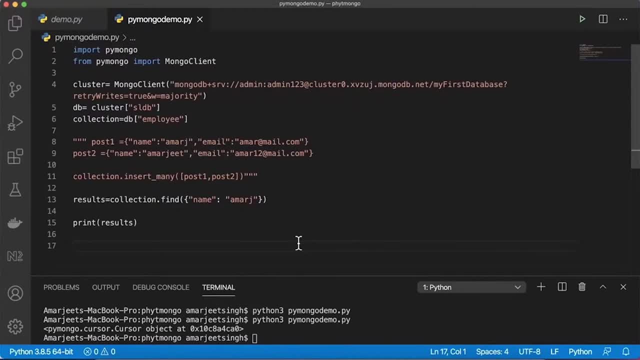 think the correct result is coming up. we can also go back and we can use some alternative option that is called for okay. so what we can do, let's take a look here. we can use for with this, for i can say result okay in results and print this result. that could be one option through which you can get. 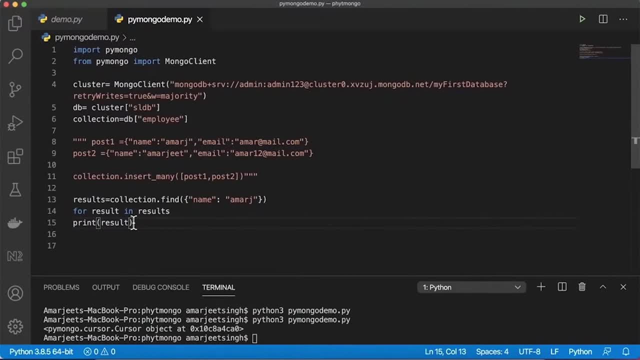 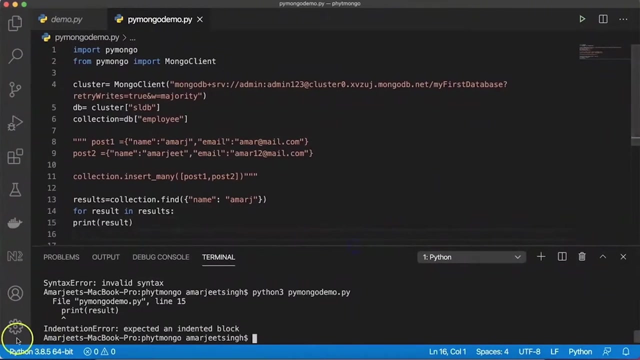 the details with you. okay, so what you can do, you can run this code again. i forgot to put this semicolon here, or we need to check. well, that was my requirement was, so i'm having this. let's try to run this. well, i got my result and this is what the detail which i have available to me. so, very simple, how. 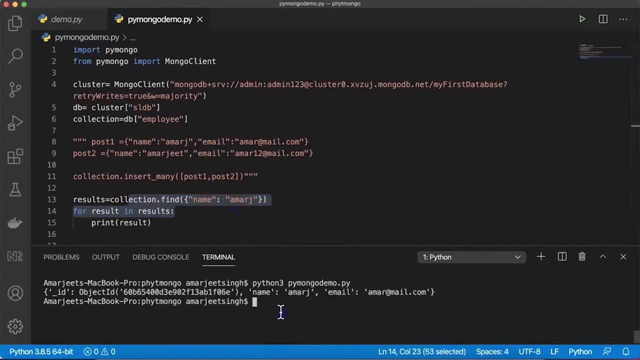 you can basically find a record and how you can basically retrieve the records at the same time, if you want to have the specific field rather than all the fields, so here in my code, in this result, okay, you can just put the square bracket and tell which field you really want it. now suppose if you 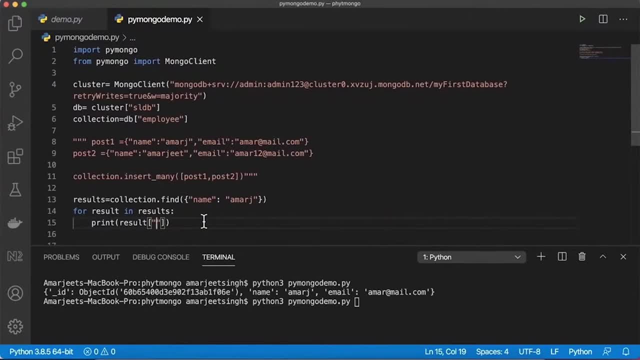 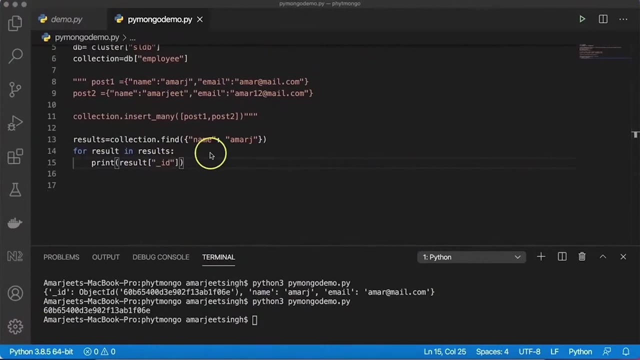 just want id, or else if you want name, you can basically pick that up, okay. so if i just want that id, like only id is printed, that's it, okay, everyone. so you have seen, like in my previous code, how we were basically trying to fetch all the records we were using this fine. now in a similar line, you: 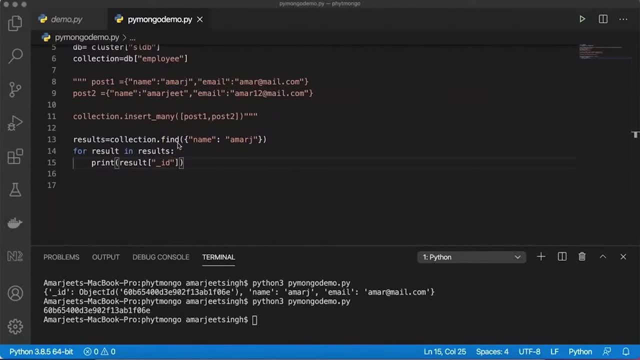 can also have the option available in the library as well. so what i want to do is: let's go back to the because even we used to talk about called fine. it gets me a lot many records, fine, and because of that we were using this loop. but in case, if you want, 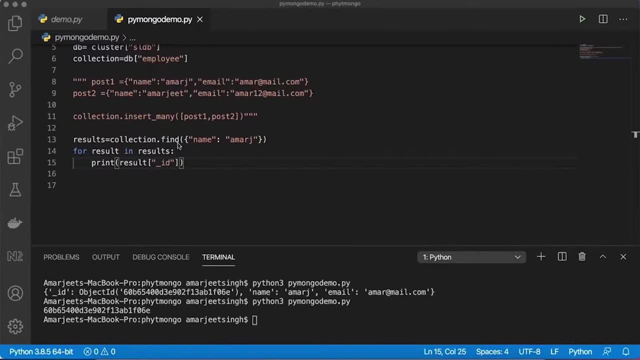 to fetch the individual records. I'll be clear. so in such cases you really do not want to use fine, you can just use find one. so what you can do is, rather than using find, I can also use one more option, called fine one and for which I 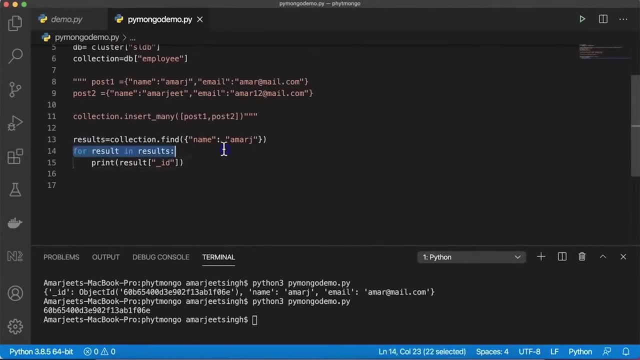 can come back. just remove this all. yeah. so here, in this case, rather than using this fine, I can use fine underscore. you can see this option called fine one. here we talk about which are the properties you want to skip and which are the properties you want, so I can just use this option called underscore. 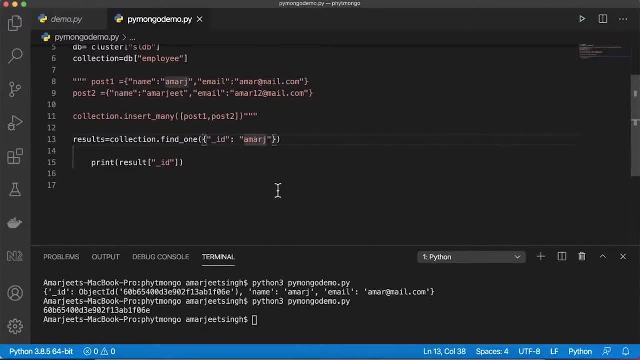 I do. okay, colon zero. okay, I just remove this and it's already zero and here just print what results. that's it, let's run so that will try to fetch some of the records for you, because if you do not have that ID which you over it in, it will certainly not found. that depends on what you would like to. 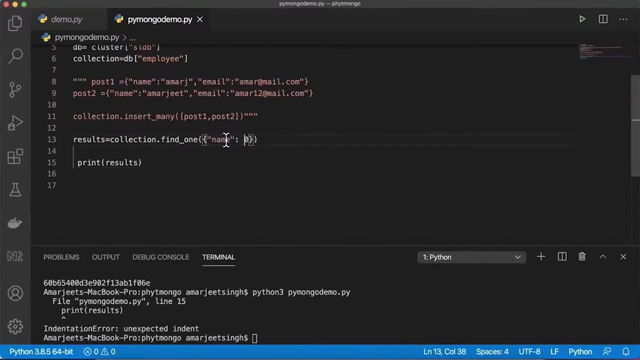 take. so if I just say, is having some issues, but no problem, but you know it very well how it basically takes. now, in a similar line, we would like to also perform one more activity to talk about delete. so for which what I will do is this: I just want to uncomment. 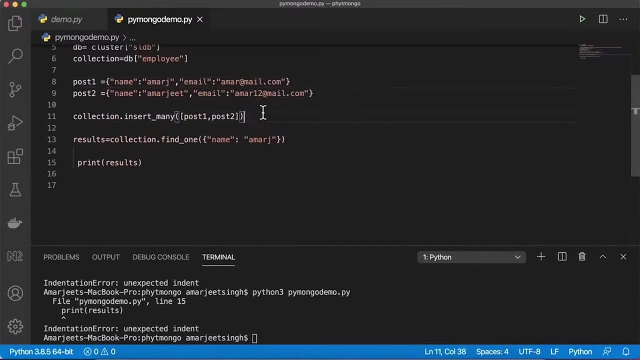 it okay, and I would like to insert some records here. so here I want to add the ID by my own with name. so we already have this name email. I have it. I would like to use underscore ID. okay, so we have this property. underscore ID go to. 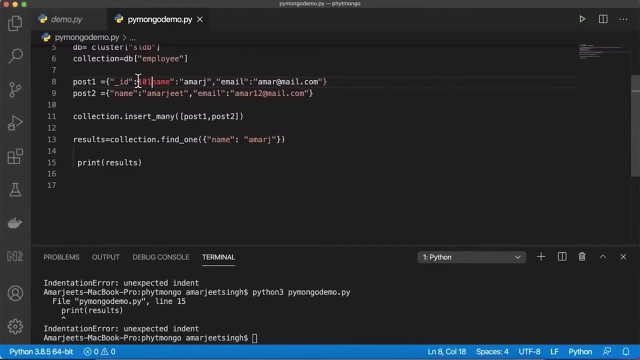 in 101, okay, comma, like this, copy the same, using it here, and this time I'm using 102 name and everything, it will be taken. let me say user one here. we try to say user two. okay, so collections dot many. result five one. I'm just deleting it all and let's try to execute it first. 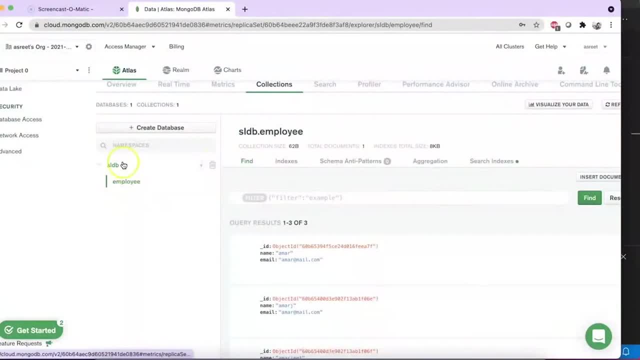 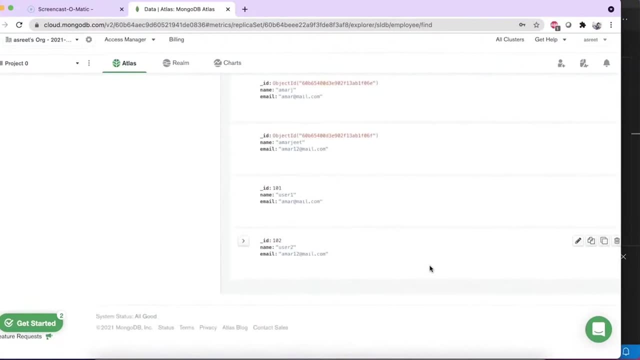 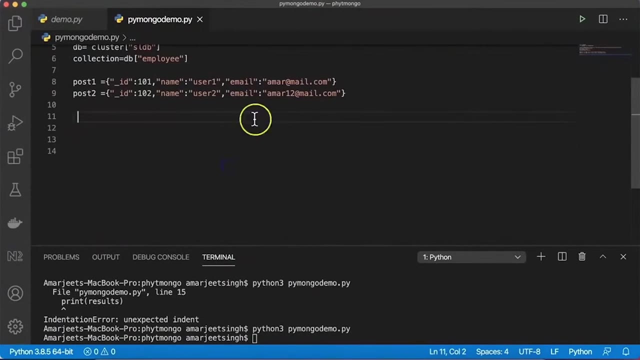 okay, so it's executed. going back: okay, so I have some records with ID 101 and 102. now here I just delete this and perform some actions here. here we say: results equal to collection, dot- delete. see the options are available. delete one and delete many. it totally depends on. 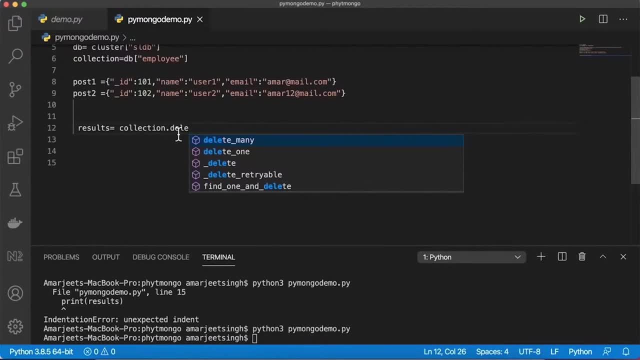 what you really want, okay, so if I just talk about call delete one, it will be only deleting one. they call delete many means where are the matching records that are available? you delete it? fine, so I'm just using this option called delete many, okay, wherever the property names are match. 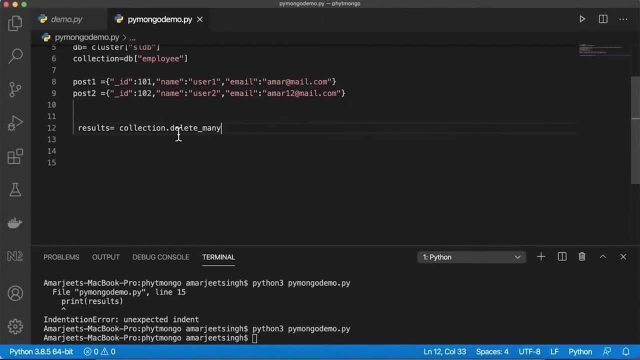 cause quite possible. names sometimes match or whatever it is. just did delete many, so the option is up to you now. for you want, so the selected name, you have to offer it, whether you want to match it with the name, or whether you want to match it with the email or whatever. it is so that 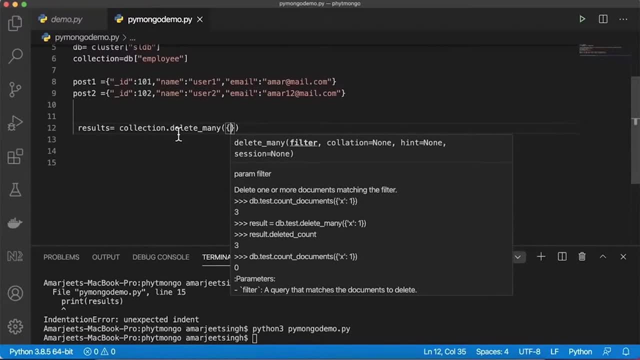 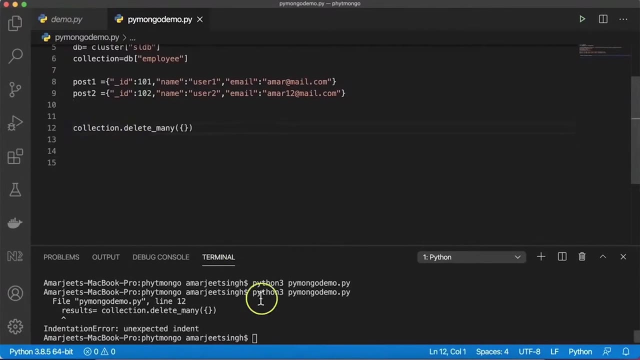 will be offering it, but there's also an option available where you would like to delete everything. are we clear? so if you're planning to delete it everything, what you can do, you can just leave it as a blank and try to run this. so: collection dot, delete, underscore many. 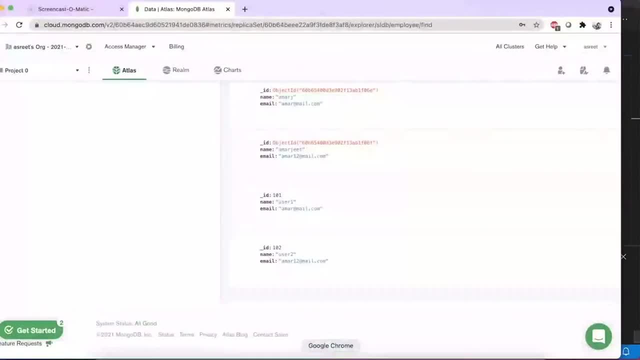 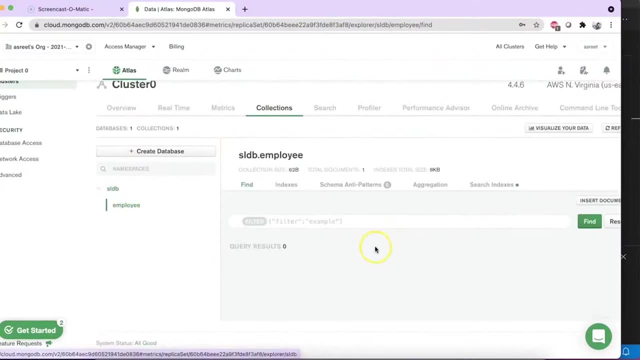 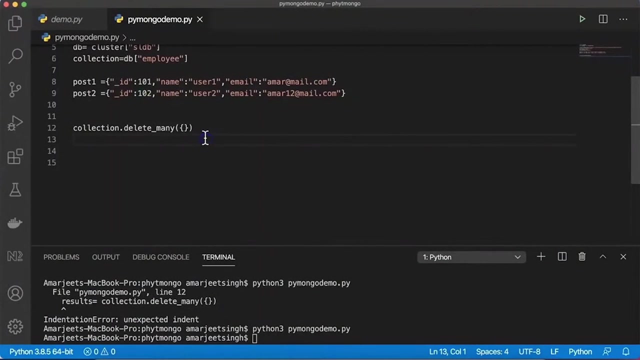 let's check: great, all records are deleted. so, as I told you earlier also, so delete many means what. it will delete all the records, whichever are present in your code. now clear in a similar one. if I want to perform insert- so you remember about- we have an option called what. 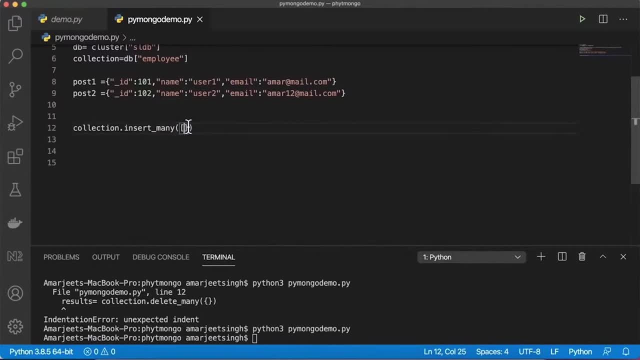 insert many, and here we would like to pass post one, post two. let's execute, so it'll add the records inside this, okay, and next time what I want to perform after adding this record, I would like to perform the update part. okay, so what I really wanted, my update. let's take a look. update means certain properties. I'm looking. 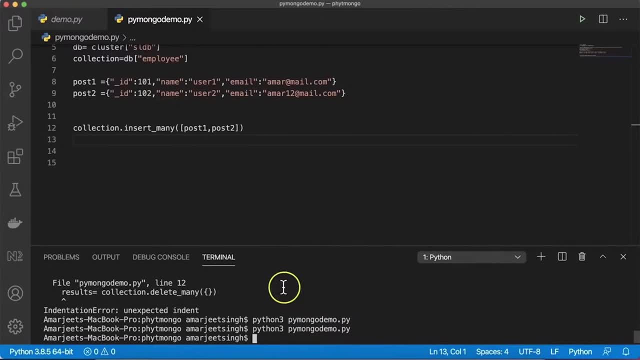 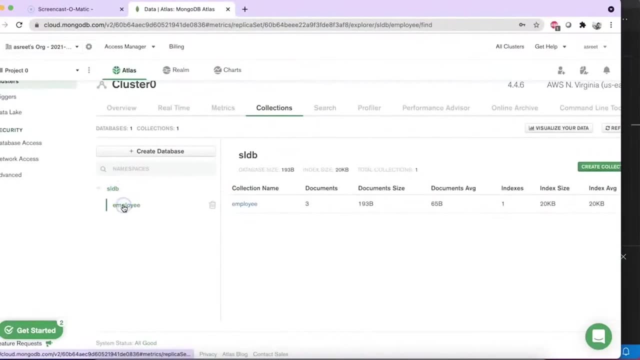 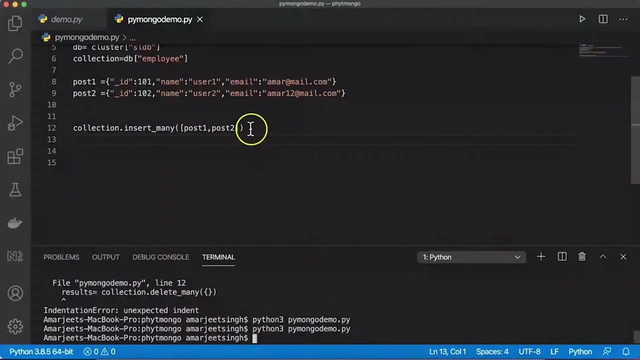 forward to we get updated. okay, so in case, if I want to check whether record has to be updated, I would first go and check whether the record does exist or not. yeah, we have two names, user one and user two. let's go back and update path here. 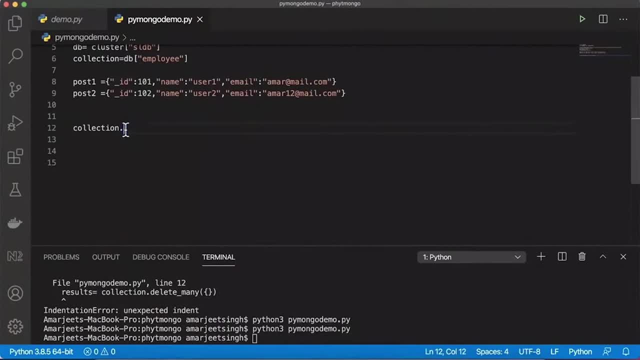 I just say collections, okay, dot, update one update. you can see update one here. very simple functionality here you will go and tell which id you would like to perform an update by saying underscore id colon, which id you want to consider. i'm saying 101, okay, and what else? so i just use another curly braces and i say sorry, dollar set. 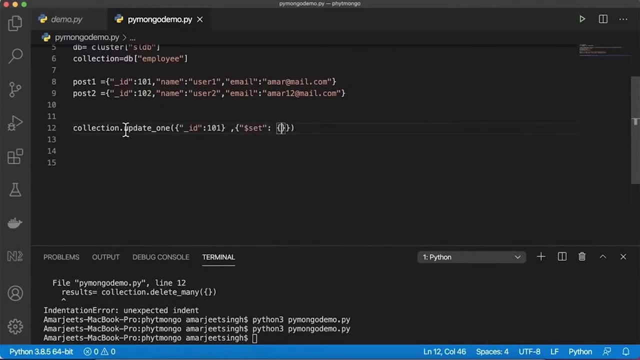 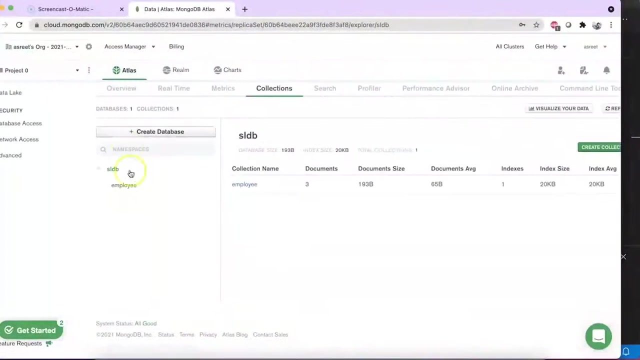 and after this i use this colon: use the curly braces name. okay, and use what name you want to use it. so suppose there is a user one, i'm saying user one, two, three. okay, let's see it is loading and you can see the record. user one to three is updated. 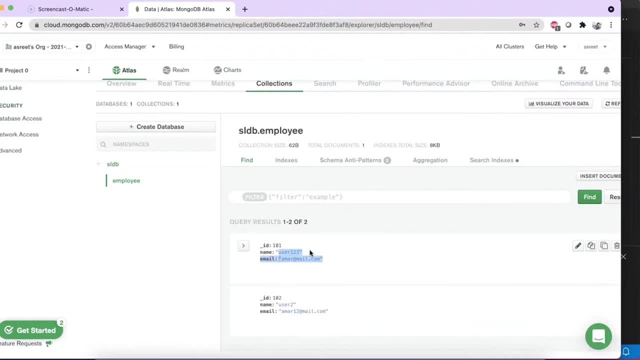 perfect. so your code is absolutely working fine. so you talk about either insert, you talk about what update, you talk about anything, it works. so insert, update one, delete one, insert one, as the name suggests, they'd be taking care about inserting, updating and deleting one-one records. 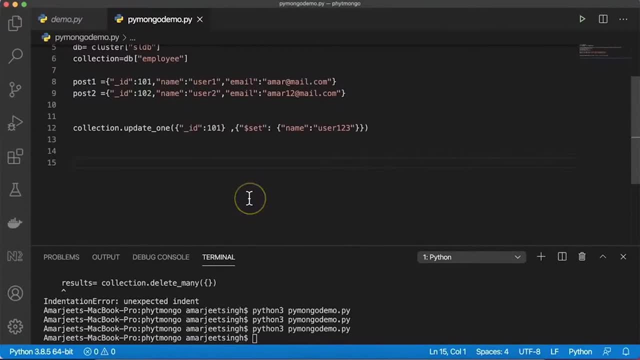 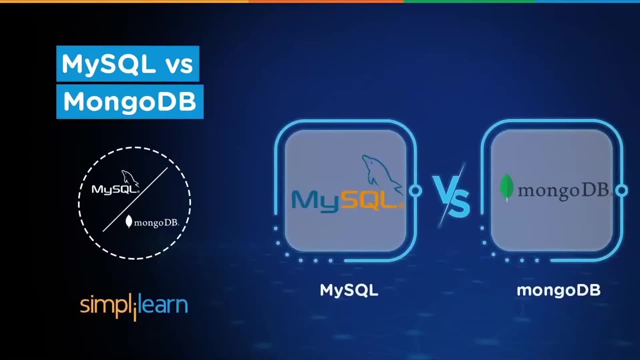 But the moment you use many, they'll be performing multiple records. So this is a very simple way, like how the Python will connect with your MongoDB. In this video, we're going to learn about the differences between MySQL and MongoDB. Now I'm sure you must have heard about these database management systems, but do you exactly? 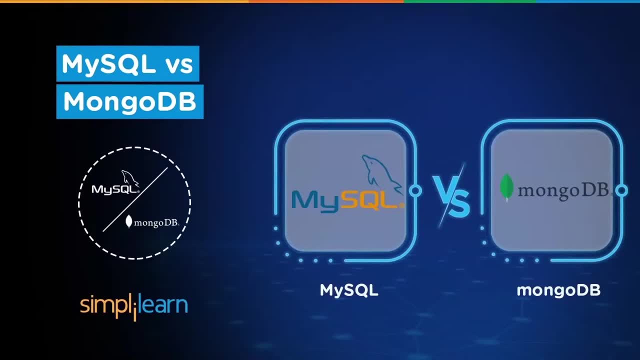 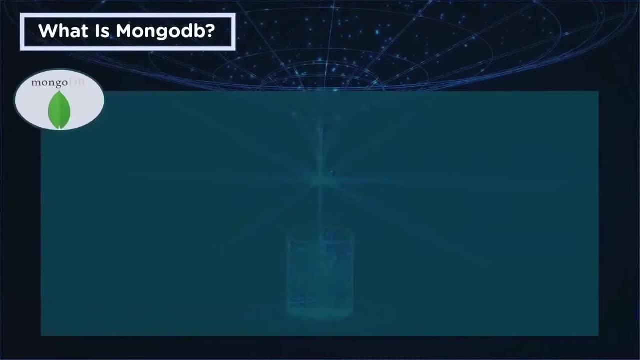 know what set them apart. Don't worry, I'll help you in this video. First, let's look at what exactly is MongoDB. Now, as you all know, MongoDB is an open source, document-oriented NoSQL database. It is document-based, which means that the data stored is represented in a hierarchical 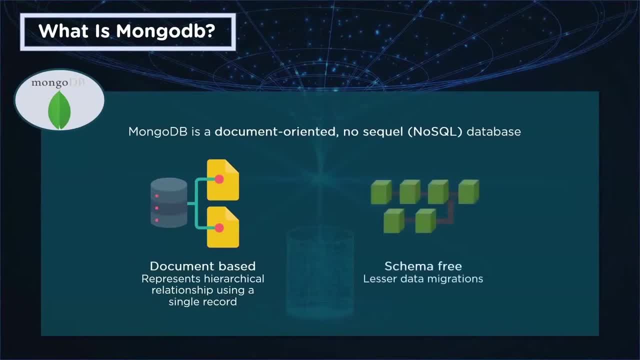 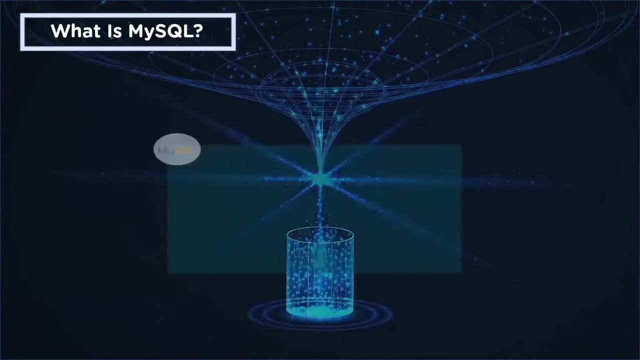 relationship using a single record, And also MongoDB is schema-free, which means there's no set schema to define how the data is being stored in the database. This causes lesser data migrations. But what exactly is MySQL then? Now, MySQL is an open source relational database management system. 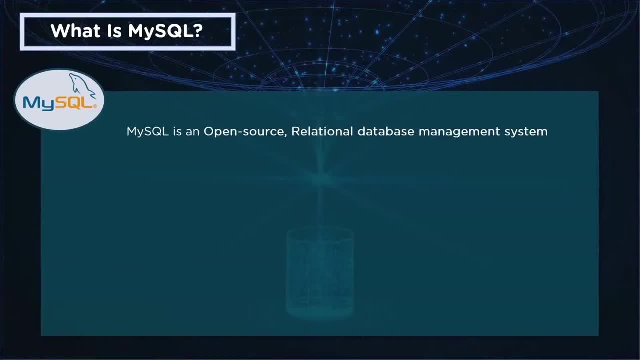 Unlike MongoDB, which is document-oriented, MySQL is a relational database system. Now, this uses something called as a structured query language, and this is used to access data which is stored in the form of rows and columns. Now, as mentioned earlier, data here is stored in the form of tables with rows and columns and each data field. 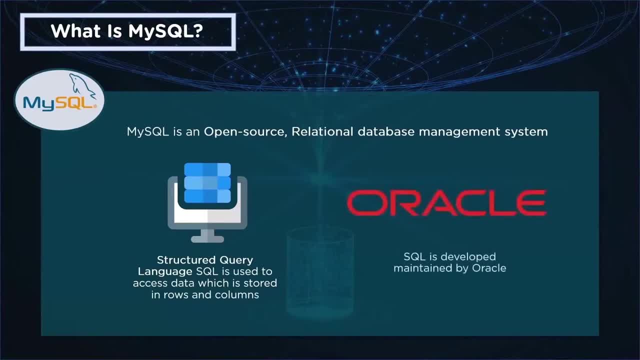 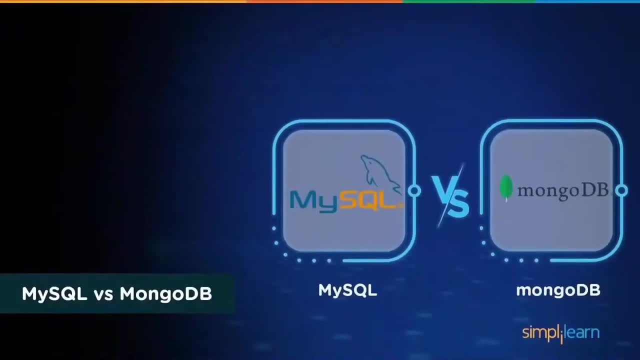 comes with an index representing the data in the table, And SQL is developed and maintained by Oracle. So then, what exactly sets them apart? So in the coming section, we'll look at some of the differences between MySQL and MongoDB, depending on certain features. 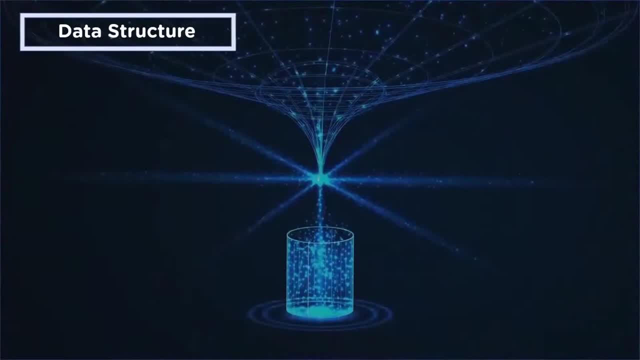 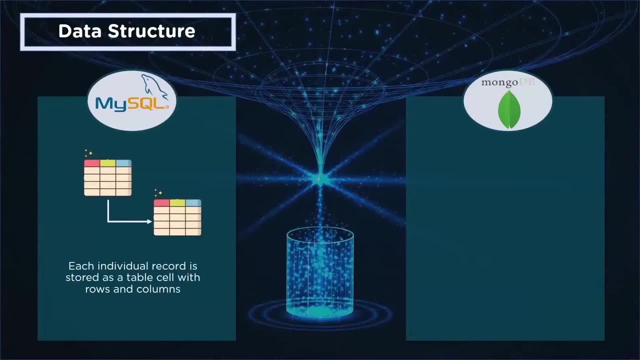 First up is the data structure. Now, MySQL requires you to define your tables and columns before you can store anything, And every row in a table must have the same columns. In MongoDB, you just drop the data in these documents. Also, the data in the MongoDB database is stored in a binary format called as BSON. 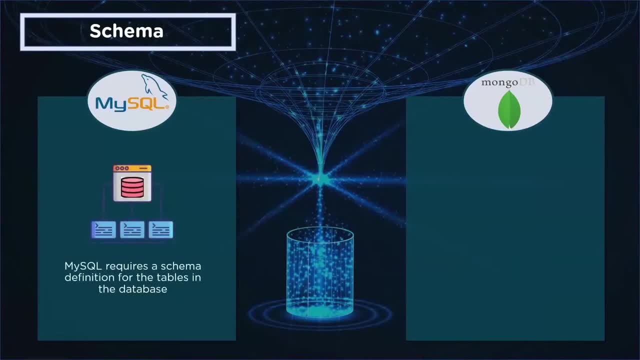 Next up, we have schema. Now, as discussed earlier, MySQL requires a set schema to define the tables in the database. Now the database administrator is called a schema. Now the database administrator is called a schema. The MicroStat-Histor is requested to define a schema which defines how the different tables 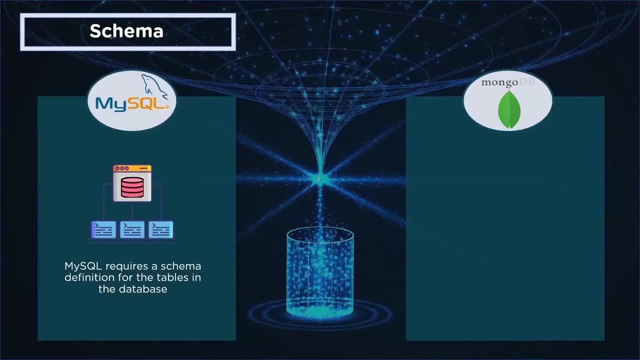 are being stored in the database Now. this schema is crucial in case of MySQL. On the other hand, MongoDB doesn't require a prior definition of a schema. Next up is languages. MySQL uses the Structured Query Language to perform actions on the database. 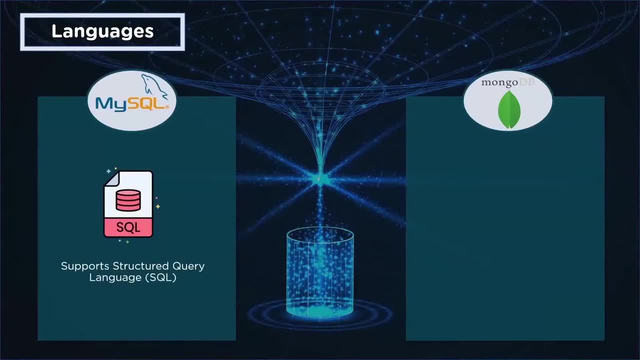 It is used to retrieve data, add data, update, create a new data set, etc. respond to my queries problem. it supports the JSON query language to work with data. Next up is foreign keys. Now MySQL supports the usage of foreign keys. If you don't know what? 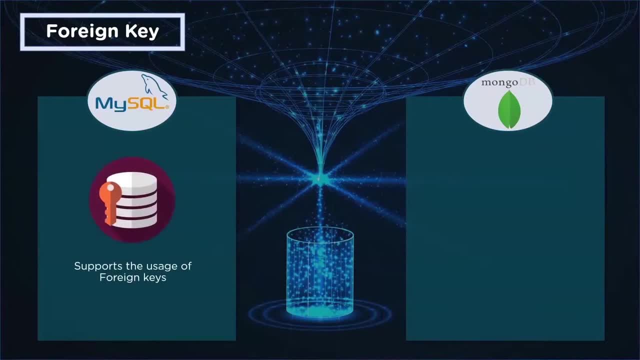 exactly a foreign key is, then SQL uses foreign keys to link one table to another. Now, these foreign keys make data retrieval easy, especially when there are multiple tables interlinked with one another. In case of MongoDB, there's no support for foreign keys. Next up is replication. Now MySQL supports the 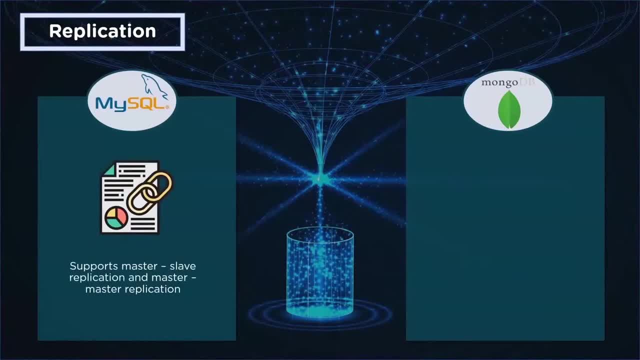 master-slave and the master-master replication. In this setup, dataset from one master database server can be copied to other servers. In case of MongoDB, it uses something called a sharding. Now, sharding allows partitioning of data across multiple servers using a shard key. Don't worry if you're not able to. 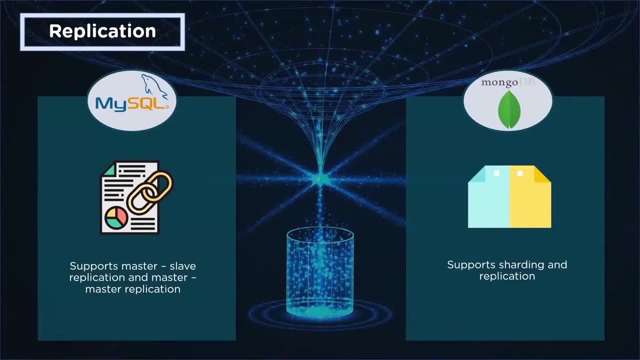 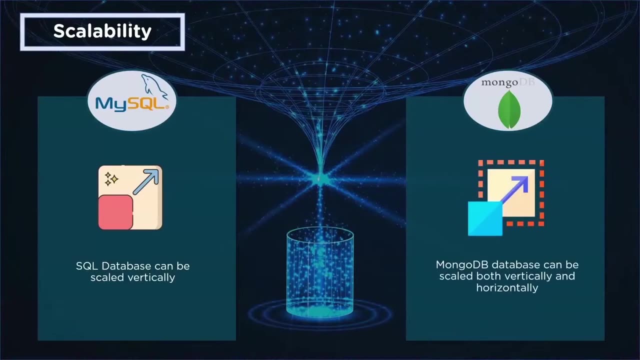 understand these concepts well. in the coming videos, we'll explain these concepts in detail. Next up is scalability. Now SQL MySQL database can be scaled vertically, while MongoDB can be scaled both vertically and horizontally. Now, horizontal scaling means scaling by adding more machines to your pool of resources, while 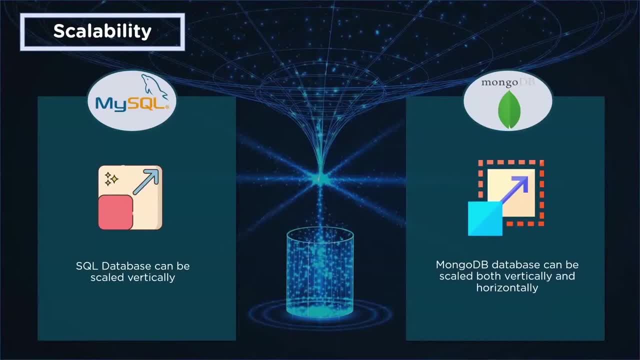 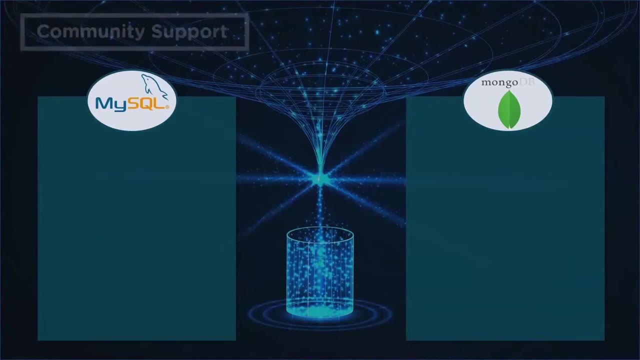 vertical scaling refers to scaling by adding more power, like, for example, CPU or RAM. Moving ahead, let's look at performance Now. MySQL is optimized for high-performance joins across multiple tables, while MongoDB is optimized for write performance. Talking about community support, some of the popular GitHub repositories on MySQL currently. 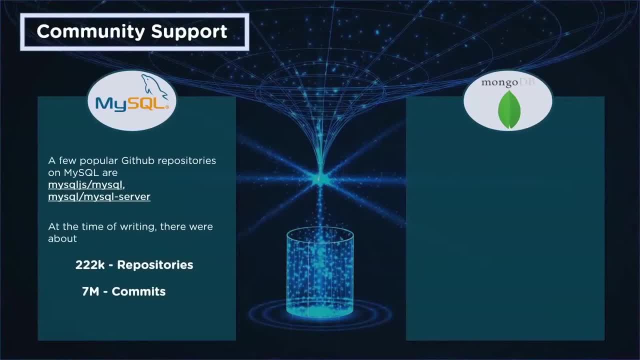 are mysqljs- slash mysql, and then there's mysql server and at the time of writing, there were about 222,000 repositories on GitHub with 7 million commits for MySQL. In case of MongoDB, few popular GitHub repositories are mongodb slash mongo and doctrine slash. 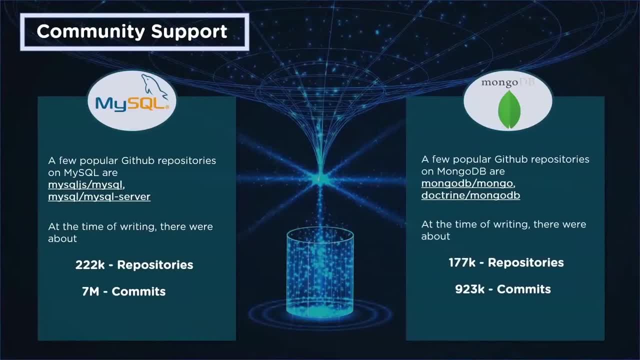 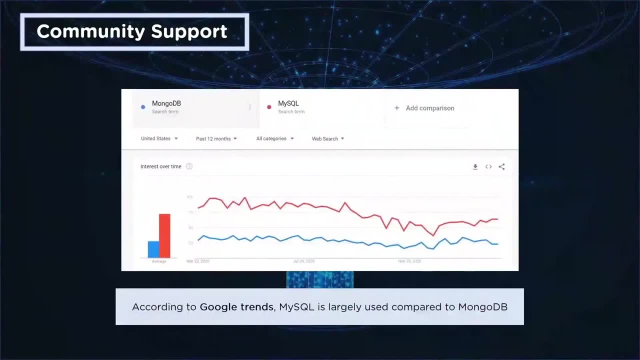 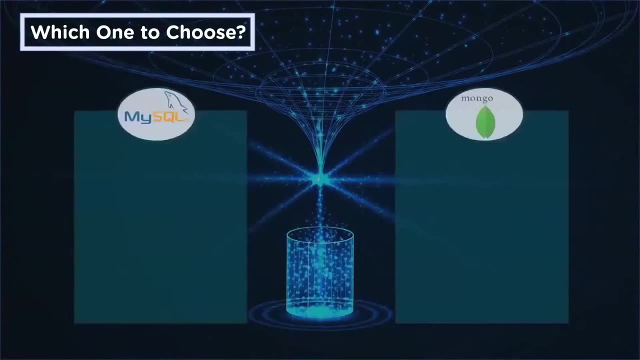 mongodb And at the time of writing, there were about 177,000 repositories with about 923,000 commits. According to Google Trends, MySQL is largely used compared to MongoDB. So now the question arises: which one should you choose? Well, if your application requires multi-row transactions, like, for example, an accounting, 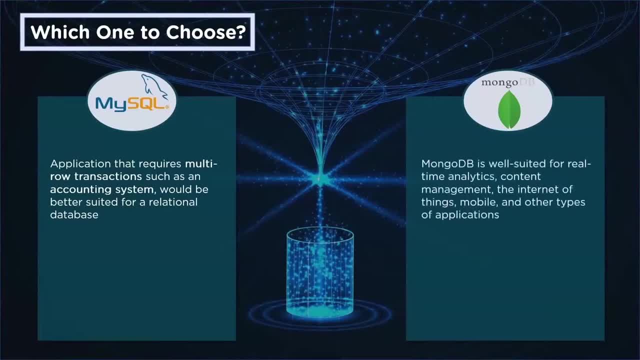 system, then a relational database would be more ideal. But if you're using MongoDB, then it is more suitable for MongoDB. And if you're using MongoDB, then it is more suitable for MongoDB. But if you're using MongoDB, then it is more suitable for MongoDB. 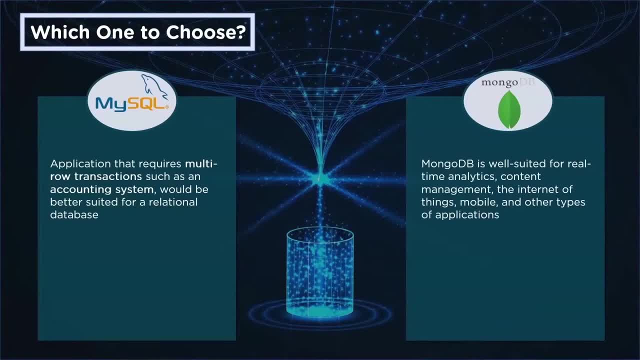 And if you're using MongoDB, then it is more suitable for MongoDB. And if you're using MongoDB, then it is more suitable for MongoDB, But if you're using MongoDB, then it is more suitable for MongoDB. So it is more suitable for real-time analytics, content management, Internet of Things, mobile. 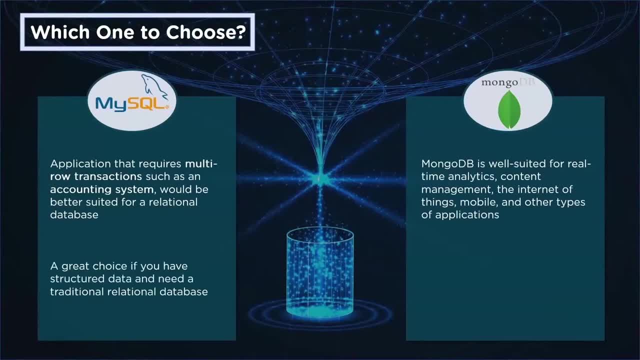 applications and so on. Also, MySQL is a great choice if you have structured data and need a traditional relational database. In case of MongoDB, it is an ideal choice if you have an unstructured set of data, So you could pick your choice. 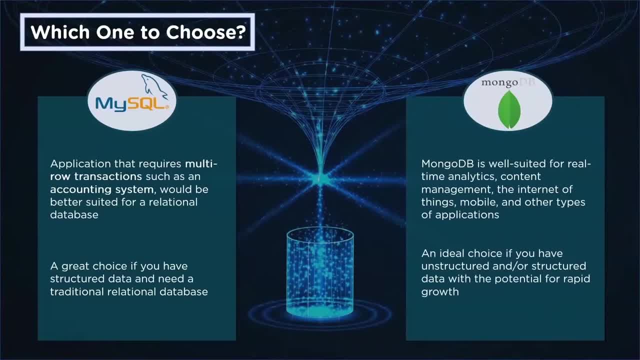 And if you are partial towards one DBMS, let us know in the comment section below as to why you like that particular DBMS, And so with that we come to the end of this session. Thank you so much for watching. This was a great session. 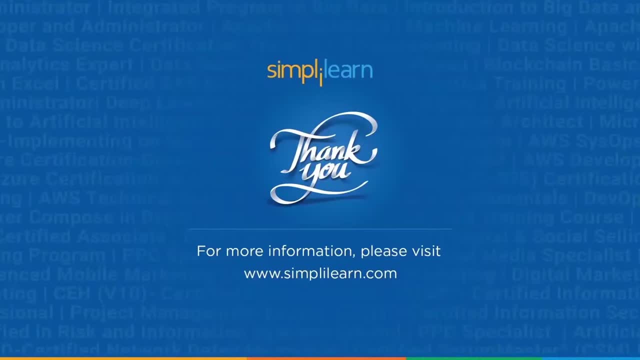 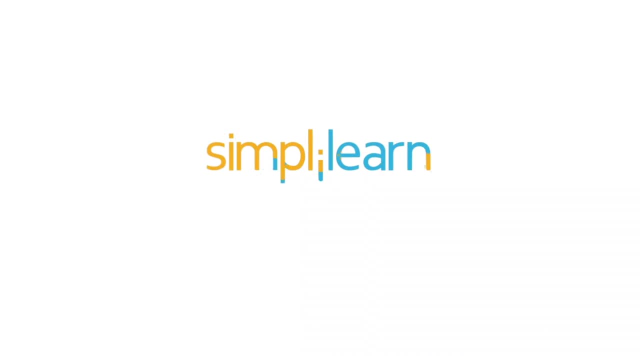 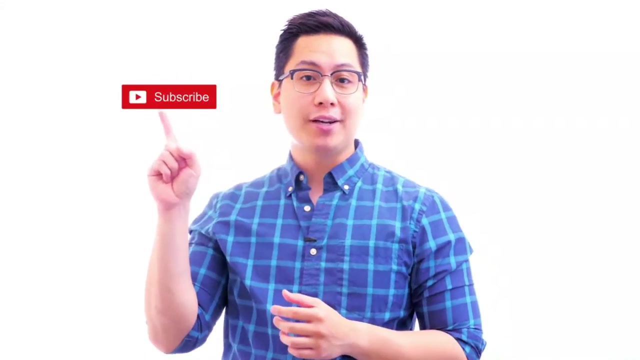 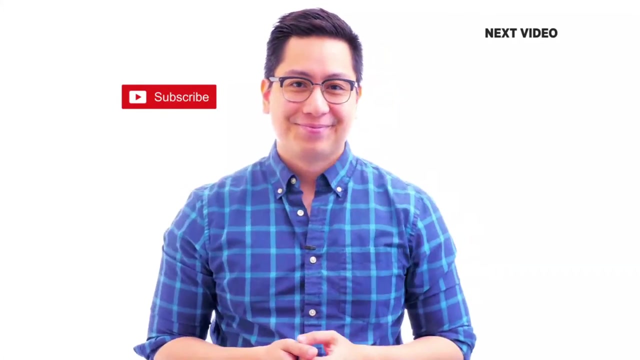 full course. we hope you enjoyed watching it. if you have any queries, let us know in the comment section below. thanks again, stay safe and keep learning hi there. if you like this video, subscribe to the simply learn youtube channel and click here to watch similar videos. to nerd up and get certified: click here. you.